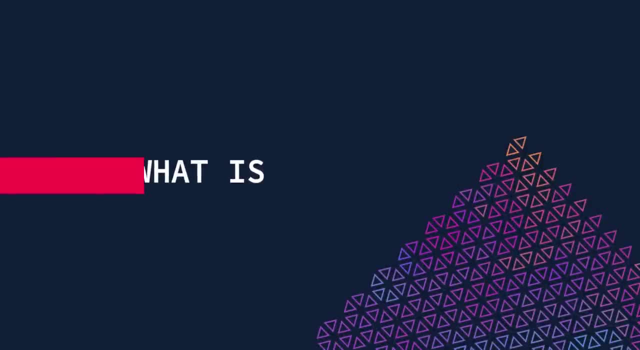 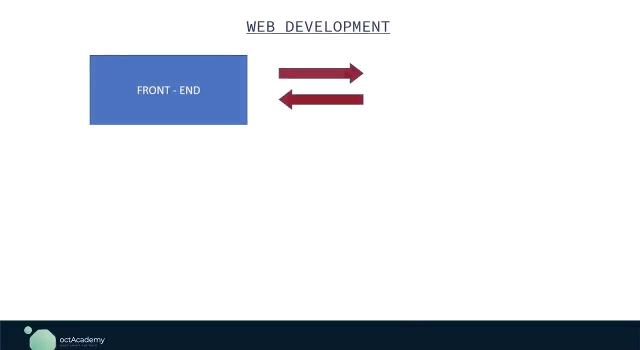 In web application development we have to look at two sides: Front end and the back end side. The front end side will load on the client side inside the web browser And the back end side loads inside the web server. The end user will only see the front end, not the. 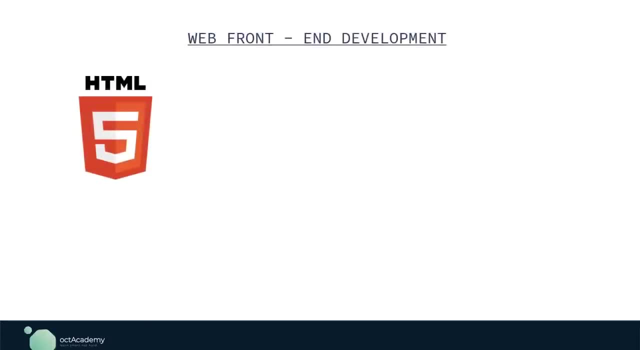 back end To design front end. we use- you guys already know- HTML, CSS and JavaScript. We use HTML to build the structure of the web page. We use CSS to make the website looks better by adding colors, fonts, etc. With the usage of JavaScript, we can make the website more logical, Which means we can make. 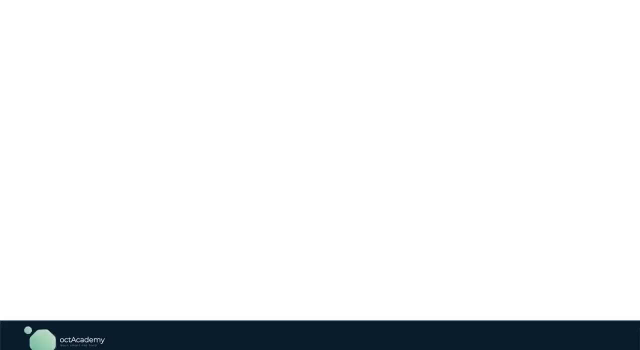 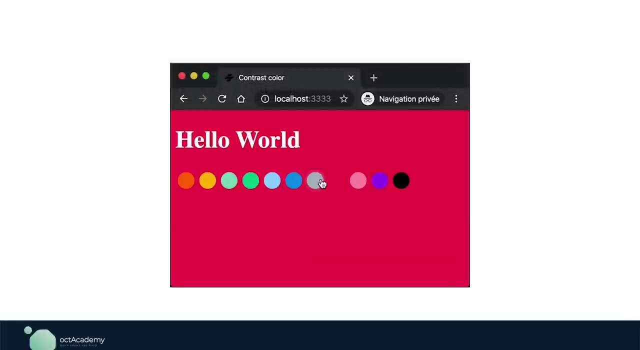 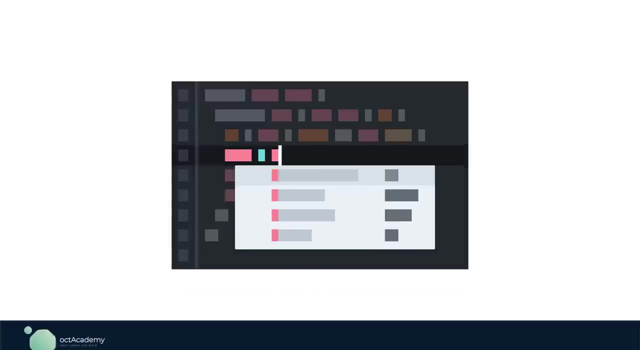 the website dynamic. We can say something if someone clicks this button, Show an alert or change this color to something else. Likewise, we can manipulate the DOM using the JavaScript. Doing this, manipulating the DOM using the only JavaScript- It is very hard and also. 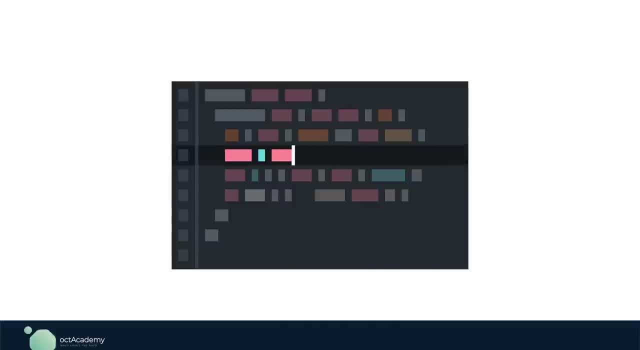 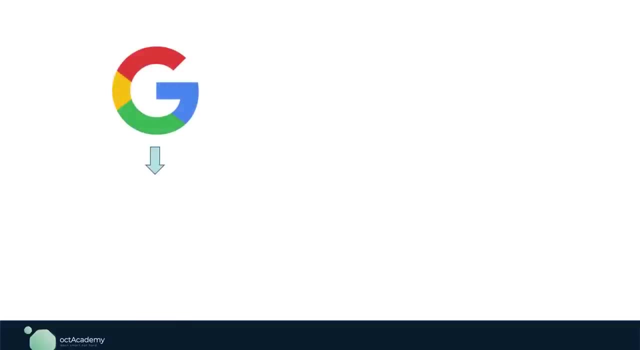 it consumes lots of time. As a solution for this, big companies like Google, Facebook are introduced some JavaScript frameworks. Google introduced the Angular and Facebook introduced the React. So what is Angular? Angular is a front end framework built using the JavaScript by Google. 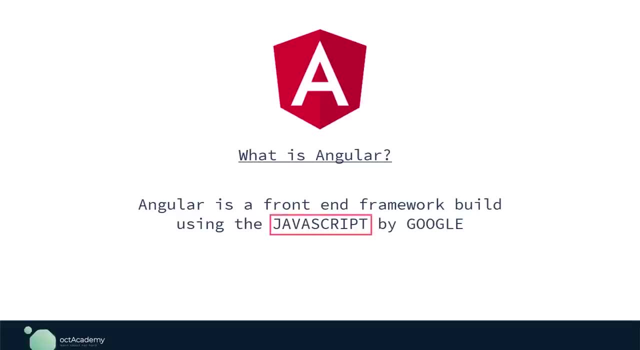 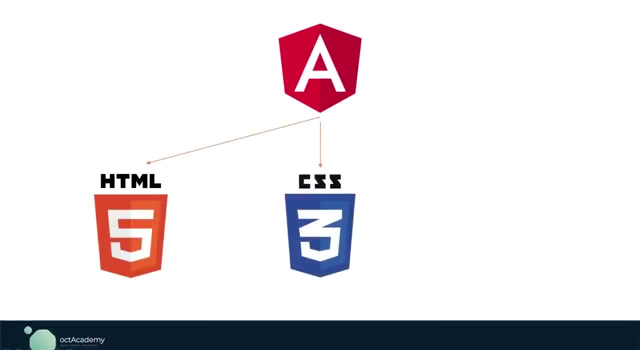 So this is not something new. This is built with JavaScript, So keep this in your mind. In Angular application, still, we gonna be using the HTML, CSS and JavaScript, But with the Angular framework we can build our web application fast and robust with pre build JavaScript. 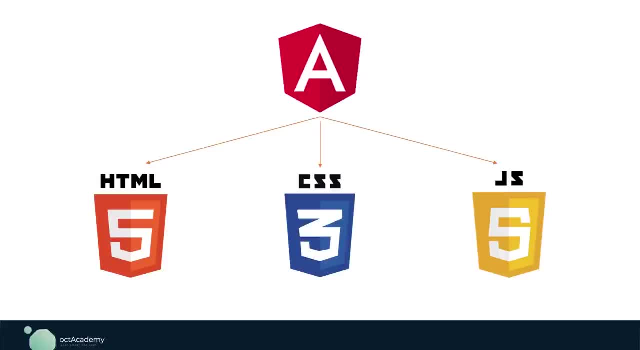 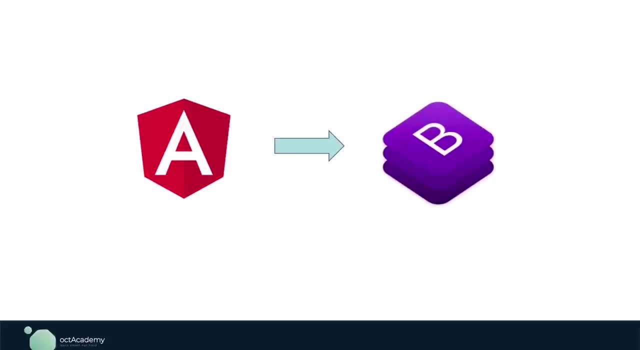 methods, So we don't need to write everything from scratch. Like the Bootstrap CSS Framework, we learned about Bootstrap in the previous section. So, if you can remember, in Bootstrap we have some pre styled CSS frameworks, Which are just a few. We will see them more in the 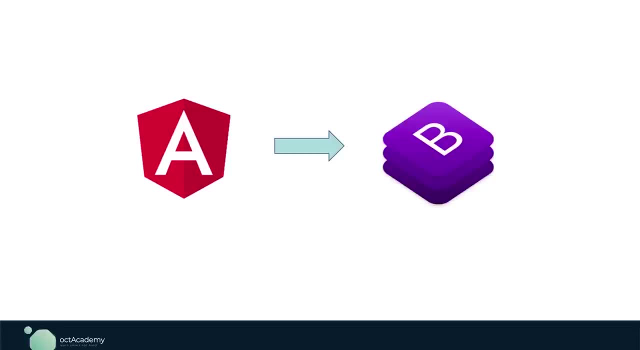 future. So if you are interested in coming to the chat, we can post a lot more content, CSS classes- So by importing them to our website, we can design our web application fast. We don't need to write styles from scratch, right. 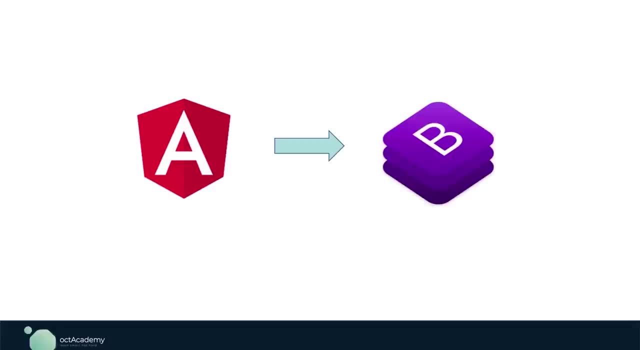 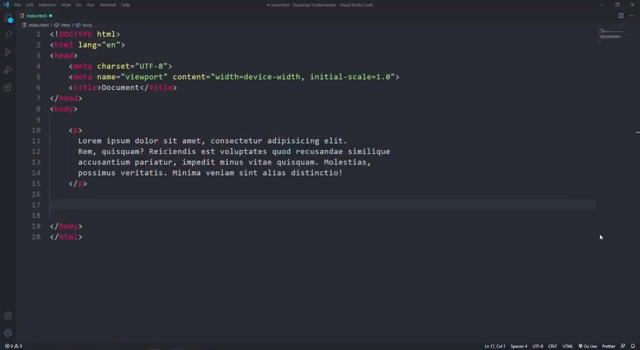 So once again, Angular, also something like Bootstrap CSS framework. In Angular also, we have some pre-built methods and techniques. By using them, we can build our web application fast and more robust. So let me show you a quick example. I think I have a paragraph. 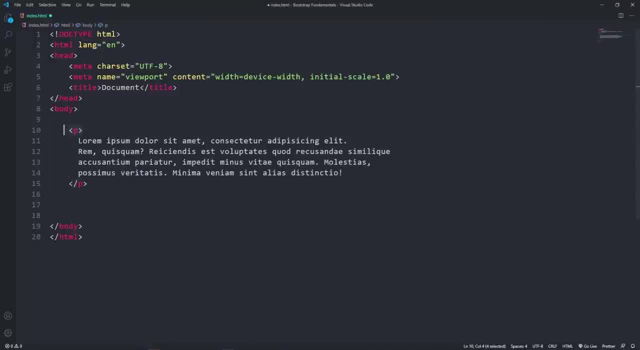 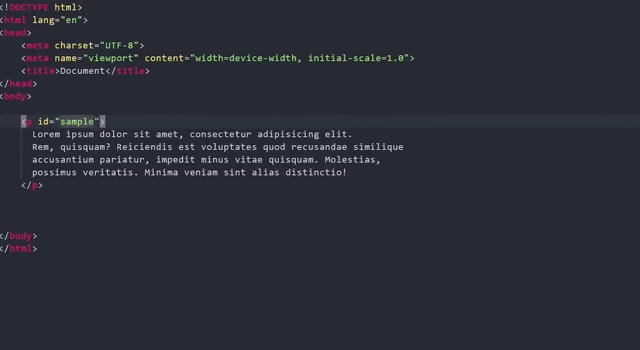 tag in my website. So I want to add a CSS class to this paragraph tag using the JavaScript. So if you are doing this using the pure JavaScript, So first I have to add an id tag to this p tag to identify this paragraph tag in JavaScript. So after that we have to capture this p. tag. So after that, we have to capture this p tag to identify this paragraph tag in JavaScript. So after that, we have to capture this p tag to identify this paragraph tag in JavaScript. So after that, we have to capture this p tag to identify this paragraph tag in JavaScript. 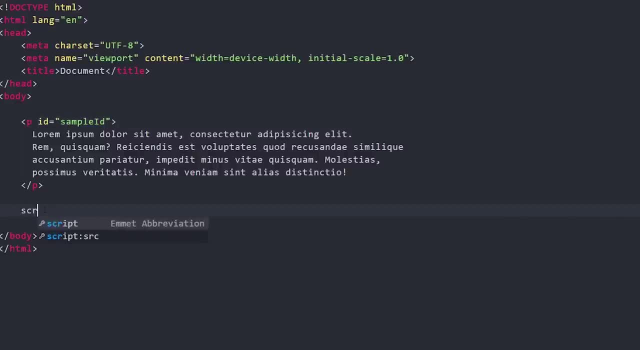 For that we have to use the documentgetElementById. So let element assign documentgetElementById and inside the brackets we have to pass this paragraph id. As you can see here, this is the id of this p tag. Alright, next we have to assign the CSS class. 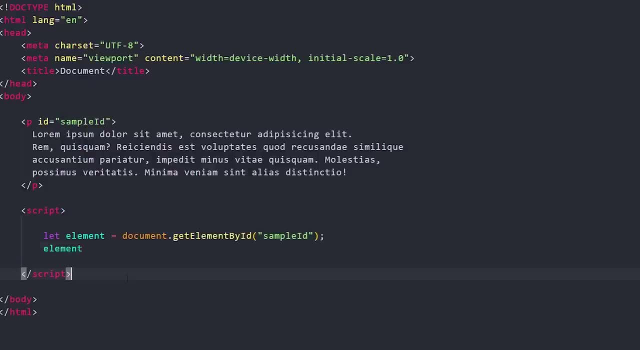 class to this paragraph tag element, which is this paragraph tag we captured earlier- dot class name. assign css class name. so i am using this example dash class. so in here we are using the css class name property, which is this example class, and assigning the css class to this p tag. so this is. 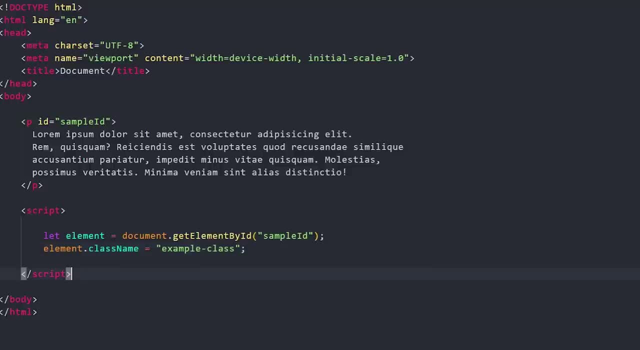 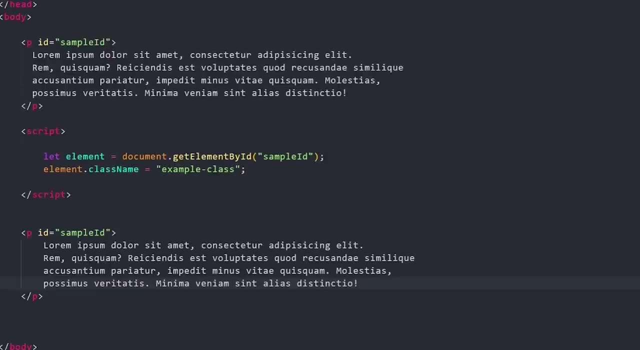 the dumb manipulation in plain old javascript. let's look at how to do this in angular. this is very easy. in angular we have class name property binding. just put this inside the p tag. this will something looks like this: and assign the css class name. so, comparing to the javascript way, this is easy and 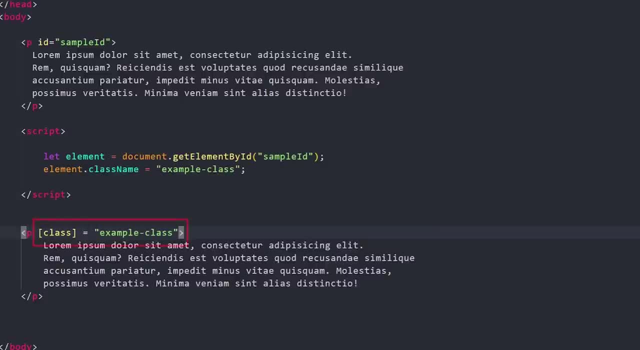 very clean, right? so this angular property binding class name is a pre-built technique in angular, but at the end of the day, this class name property will compile to this javascript, because browser doesn't know about angular thing, browser only knows javascript. with the angular framework we can do this by a single line of code rather than typing three, four of lines. so once again, angular. 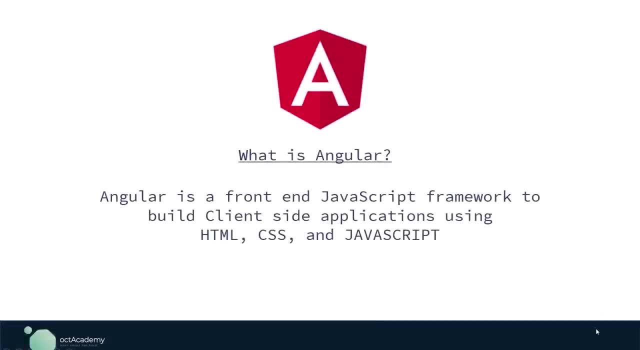 is a front-end javascript framework for building client application in html, css and javascript. hope you guys got the idea. so what is this spa? this spa stands for single page application. a single page application is an app that doesn't need to reload the page during its use and works with it. 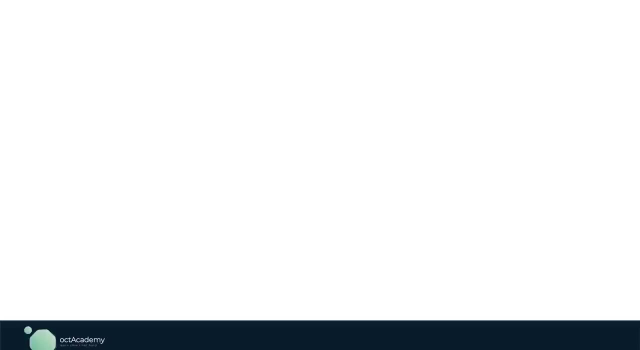 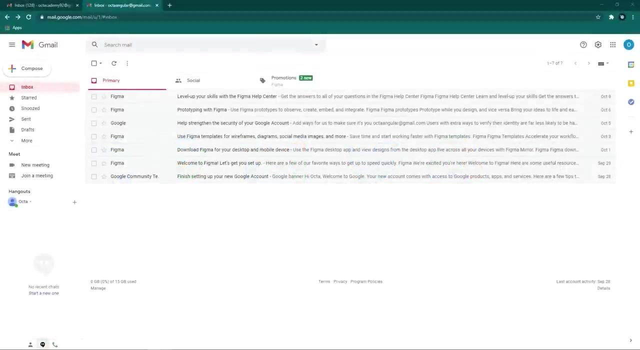 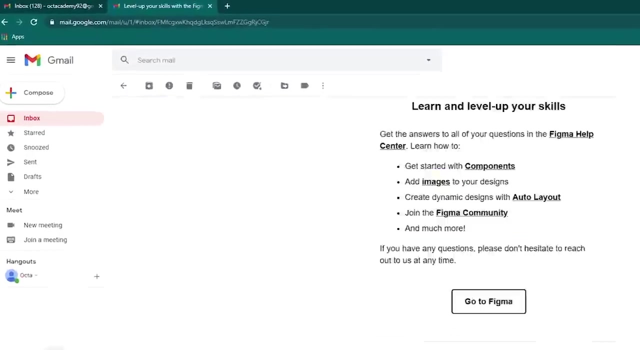 in a browser. think of the apps we use daily: facebook, google maps, gmail, twitter, google drive or even github. all these are examples of a spa. let me show you an example. go to the gmailcom. after you log into your gmail account, you can see your inbox. click one of your emails if you 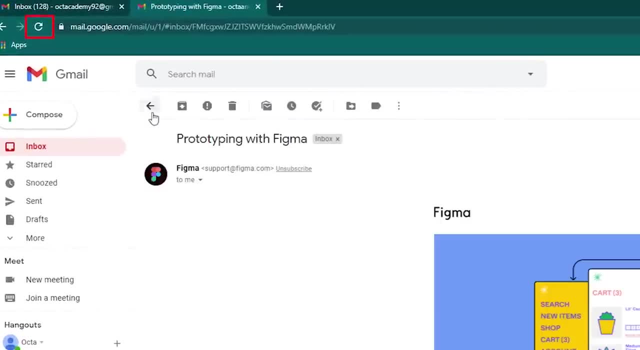 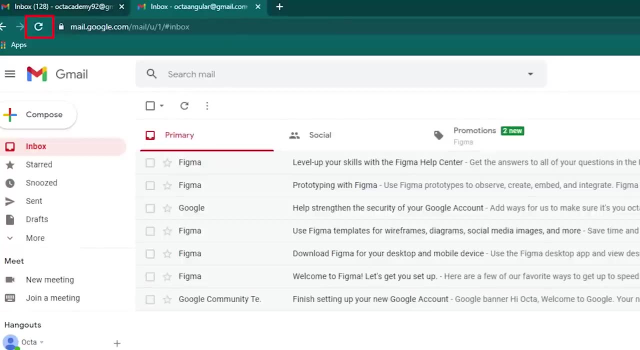 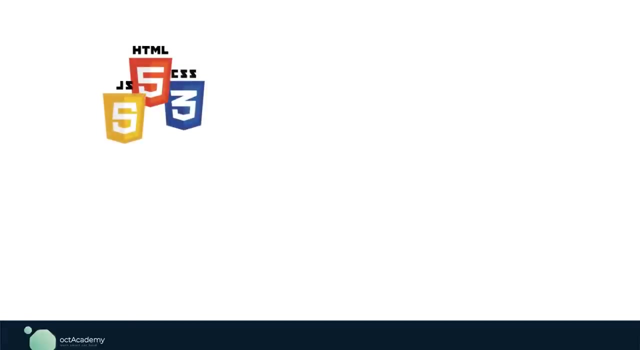 look at this carefully. you can see this will open the email without refreshing the page. so this is what single page application. so what is happening here? most resources single page application needs like html, css and scripts are loading at the launch of the app and don't need. 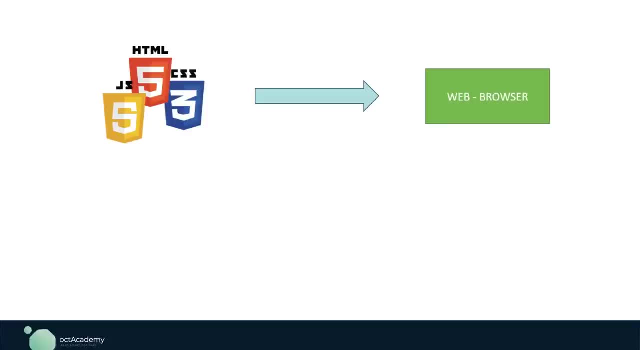 to be reloaded during the usage. the only thing that changes is the data that is transmitted to and from the server. as a result, the application is very responsive to the application and the user's queries and doesn't have to wait for client server communication all the time. 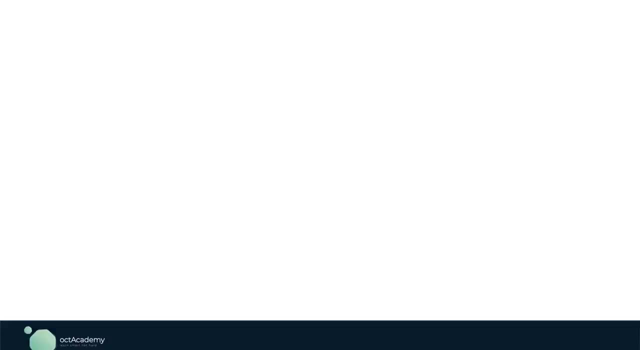 one of the best advantages of a spa is the user experience and the speed. the user enjoys a natural environment of the app without having to wait for the page reloads and other things. you remain on the same page which is powered by javascript programming language, so we can build or develop. 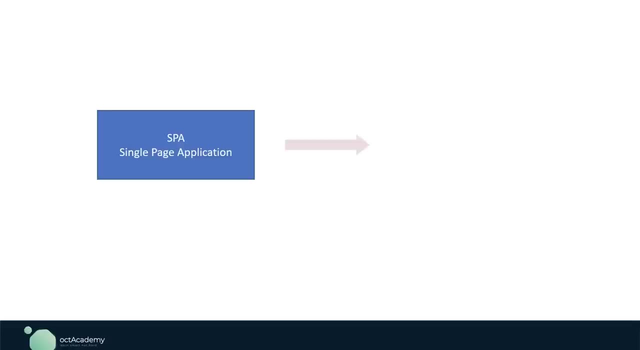 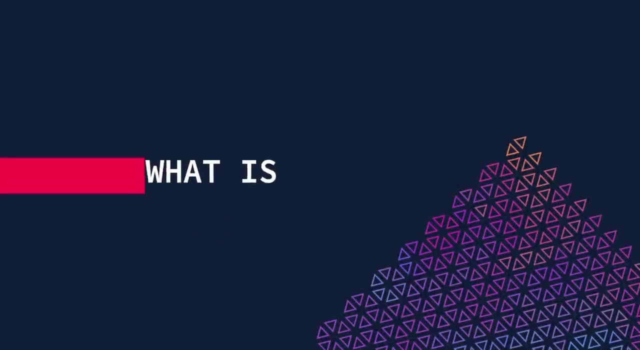 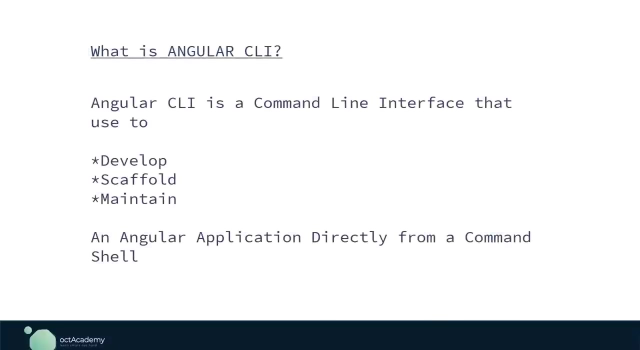 single page applications with most of modern javascript front-end frameworks, including the angular, so we can call an angular app as a single page application. the angular cli is a command line interface tool that use to initialize, develop, scaffold and maintain angular applications directly from the比如, a command shell. In other words, if you can remember, Angular is a JavaScript framework. 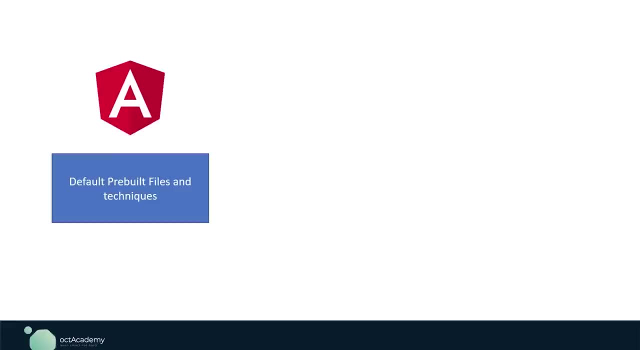 This framework has default pre-built files. In order to work with Angular, we need those files and techniques. With the help of this Angular CLI, we can create an Angular new app without any problem with a single line of command. Not only that, I told you earlier. 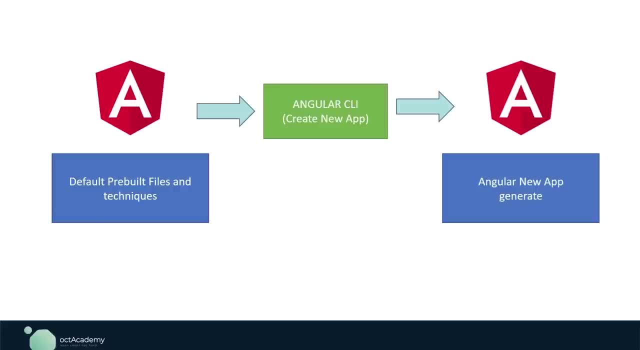 but browser also doesn't know Angular. So at the end of the day, we have to compile Angular to JavaScript Or we have to build Angular app to production So we can build the Angular app using this Angular CLI. Likewise, we can update, maintain scaffold and develop. 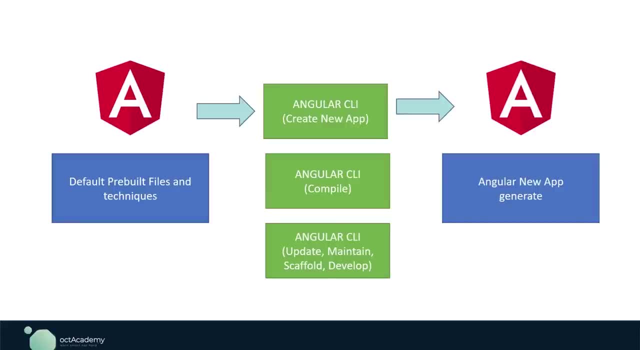 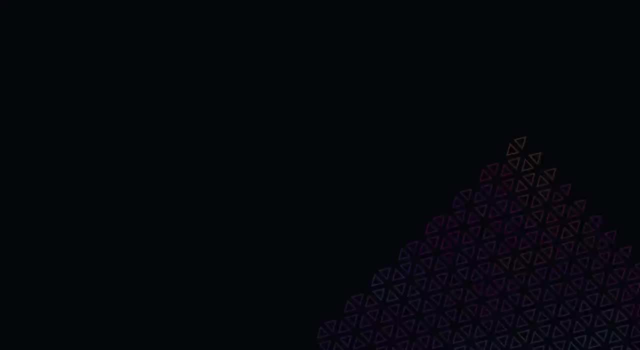 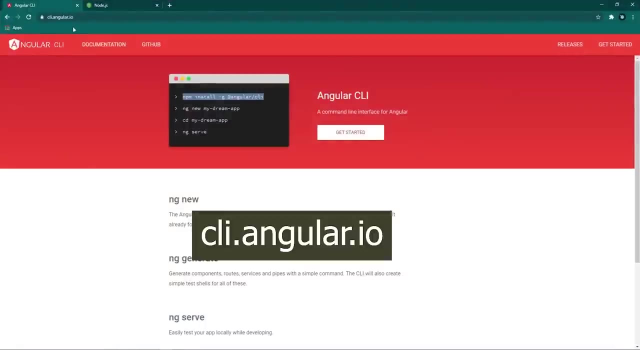 an Angular app using this Angular CLI. Hope you guys got the idea. So let's set up the Angular CLI. Go to this Angular CLI website, cliangularcom. This is the official website of Angular CLI. To use Angular CLI, first we have to install. 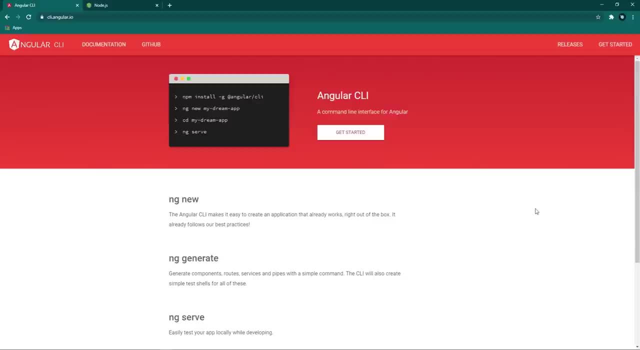 Angular CLI globally on our computer. To install Angular CLI we need Node Package Manager, Node Package Manager bundled with the nodejs. So we have set up the nodejs. We have set this in the first section of this course. So if anyone of you not installed 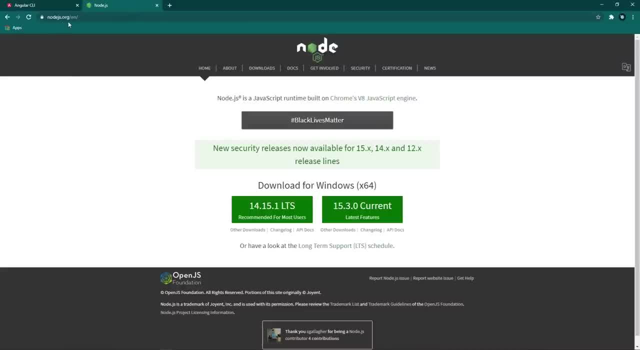 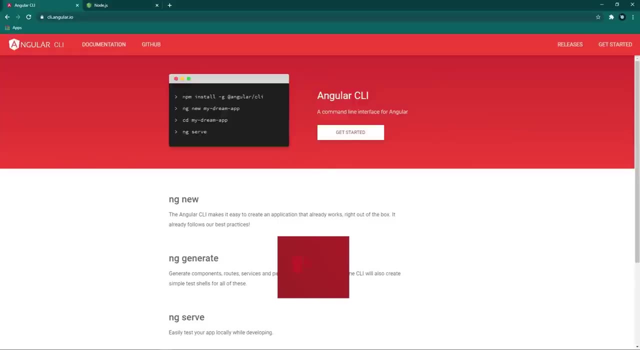 the nodejs. just go to the nodejsorg and simply download and install this recommended version. After this installed, let's install the Angular CLI. All we have to do is just run this command, Copy this command and paste it inside your command prompt or the terminal. 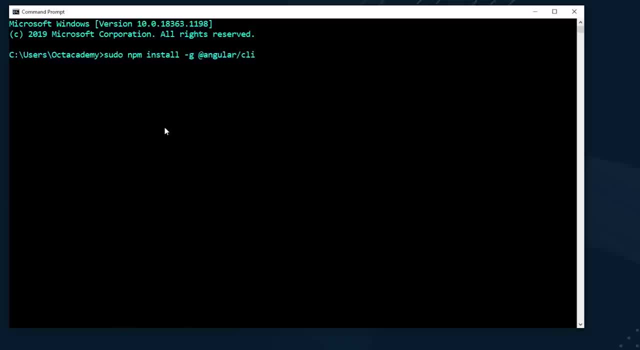 Ok, So we have installed the Angular CLI. Now we have to install the Angular CLI. So if you are on a Mac, add sudo beginning of this command, Otherwise you guys will get a permission error. PC users don't need to modify anything, Just run this command: npm. 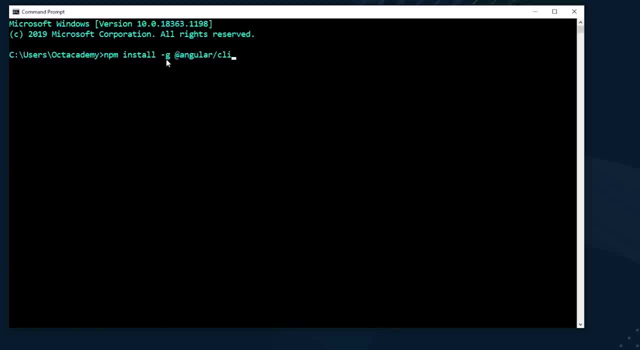 install dash g at angular slash cli. So this command will install Angular CLI on our computer globally, So we can access this Angular CLI from anywhere on our computer. This g is the command that will install Angular CLI on our computer globally, So we can access this Angular 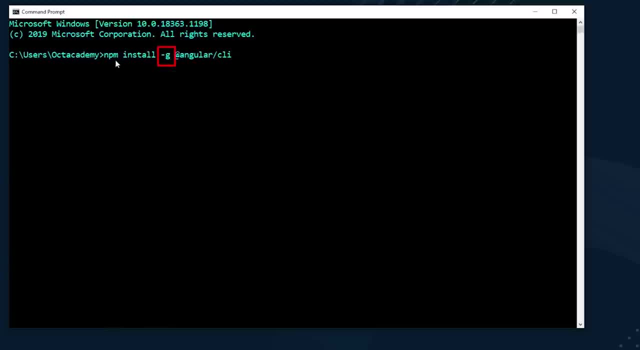 CLI from anywhere on our computer. This g is the command that will install Angular CLI on our computer. So this command will install Angular CLI on our computer. This g flag stands for global right. This npm is the node package manager and this is the angular CLI We have. 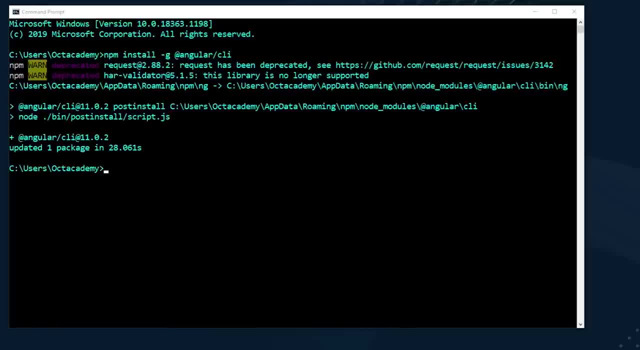 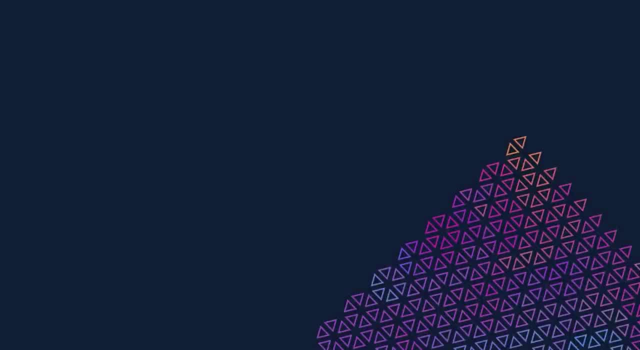 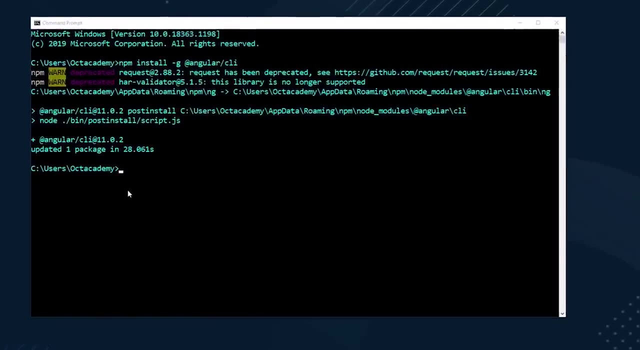 installed Angular CLI on our computer. Now we can use the Angular CLI commands. In the previous video we have successfully installed Angular CLI on our computer. Unless you wanted, Now we can generate an angular app using the angular CLI. So first create a project folder. 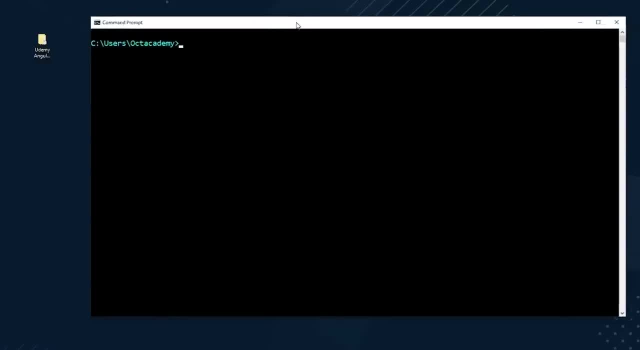 In previous, we have created a project folder inside the desktop, So I'm gonna use this same folder as my project folder for this section as well. This is optional. You guys can create this folder wherever you want. Now open the command prompt or the terminal. 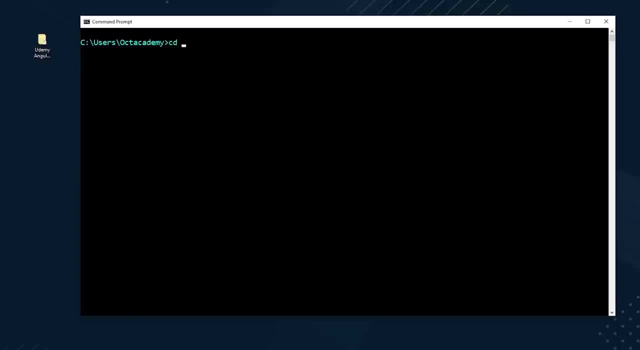 Navigate to the project folder cd desktop. hit enter again. cd udemy- angular course folder. As you can see here, this is the project folder name that I created earlier. Now what I want to do is I want to create an angular app inside this project folder. 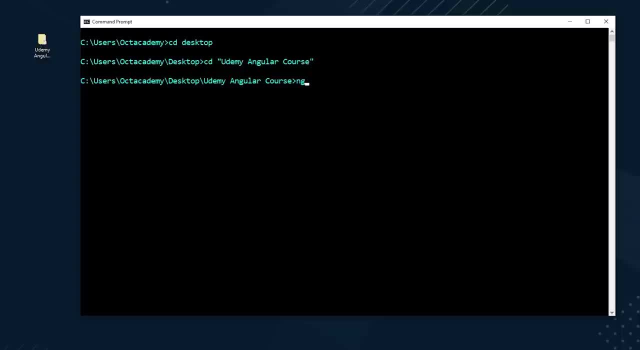 To access angular CLI, We have to use this folder. We have to use the ng command, Just n and g. Ok, If you can remember, we used the npm command to access the node package manager. Like that, we can access the angular CLI by using the ng command. 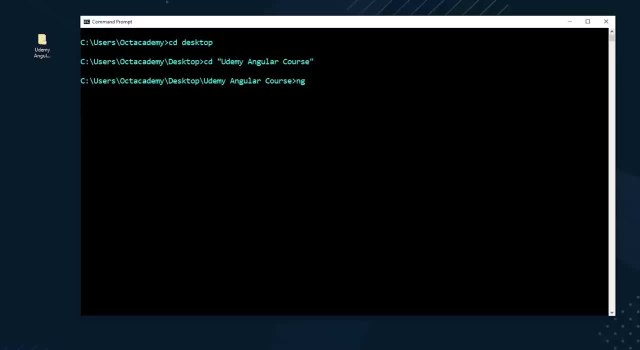 To create a new angular app, we have to use the niv command after this ng command, So ng niv. then pass the project name. I am giving the project name as ang-intro. This project name can be any name as you wish. 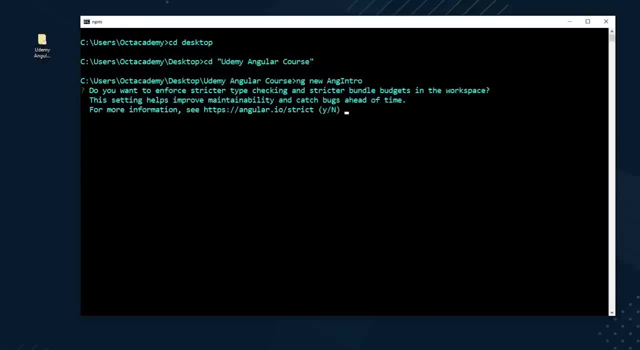 Then hit enter. At first, this will ask about the angular strict mode. For now, give this to no. In a later section we learn about this strict mode in detail, So give no to this and hit enter. After this, we get this router option. 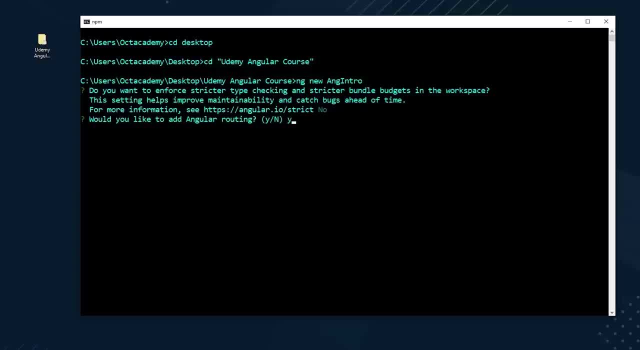 For this: give no to this and hit enter. After this, we get this router option. For this: give yes. So don't worry about this angular router thing. We will learn about this in detail in a later section. Next, this will ask about the styling method: CSS or SCSS or SAS or LESS. 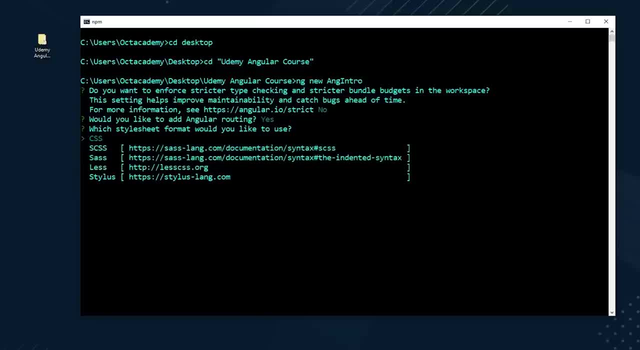 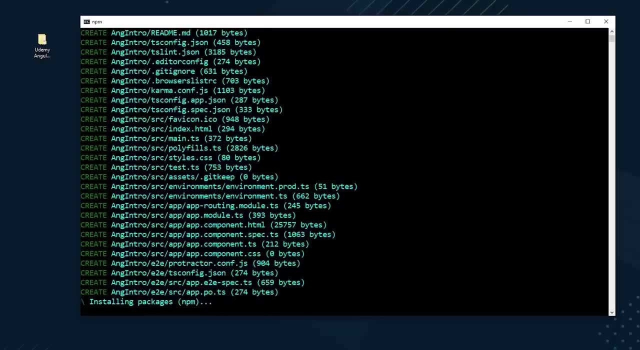 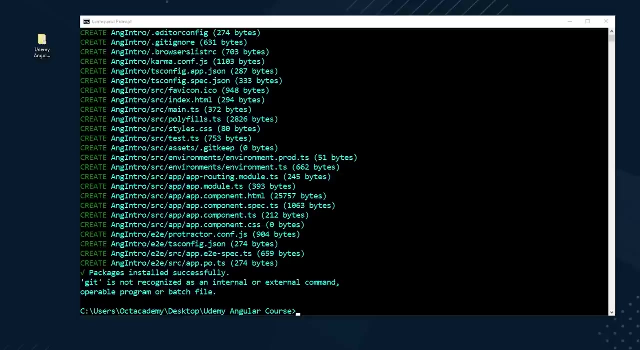 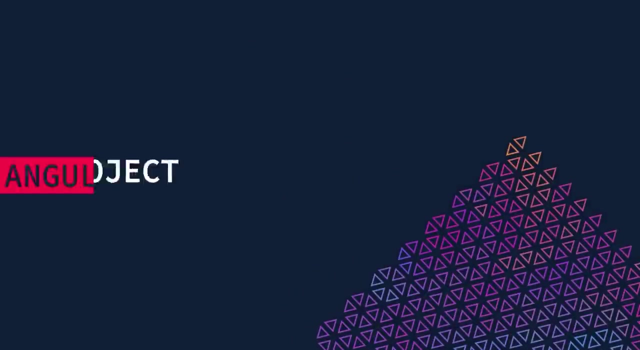 We can select our preferred method. So in this course we gonna be use only the CSS. So select the CSS. This will generate The new angular app And install all the dependencies for us. Wait until this complete. This may take several seconds to minutes, depending on your computer and the internet speed. 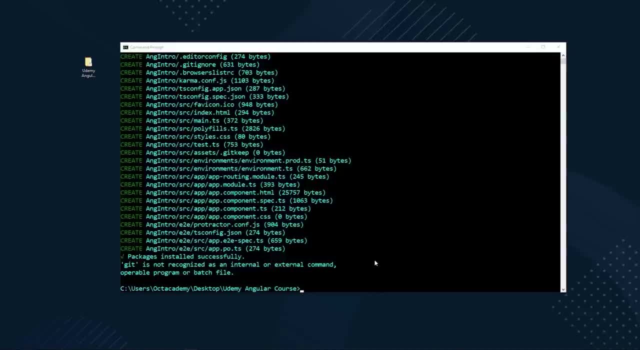 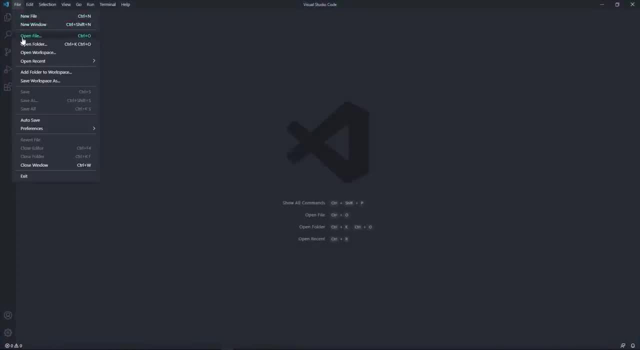 Our new angular app is ready. Now open this angular project inside the Vscode text editor. Now open this angular project inside the Vscode text editor. Now open this angular project inside the Vscode text editor. Open the Vscode. Go to the file and select open. 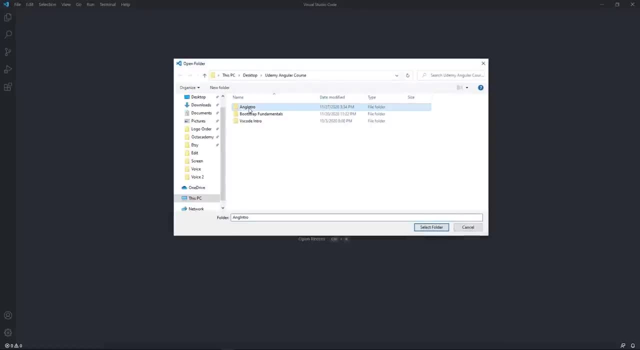 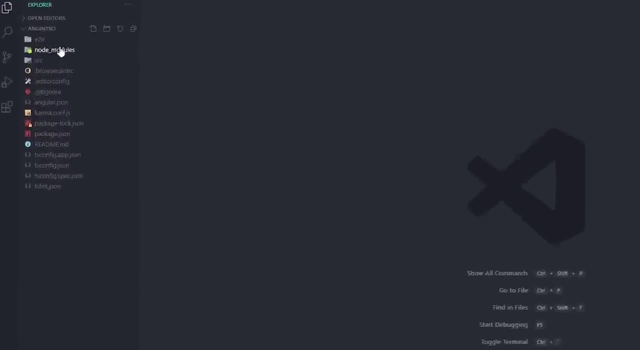 Navigate to the project folder- In my case it is inside the desktop- And select the project folder. Inside that I have this ang intro angular app. So select that folder and give open Alright In Vscode. inside the file tree we can see all these files. 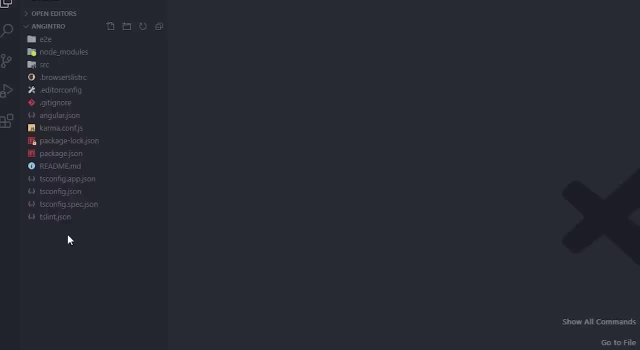 This is the default file structure of Vscode structure of an angular project. Now you guys may get scared by looking at these files. These all files are required files and default configuration files for the angular framework. So we are not going to touch any of these files or the folders. We are only dealing. 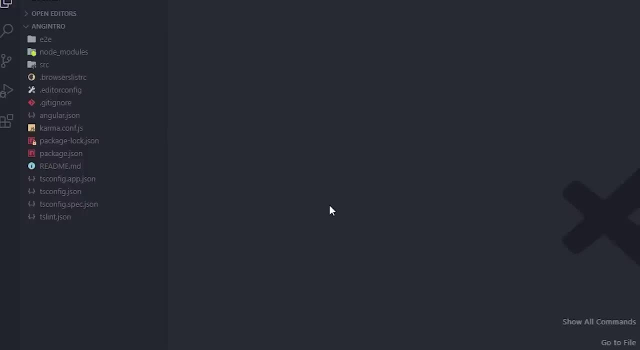 with this src folder. Ok, so don't get confused. But I will explain these all files one by one so you guys can just get to know what are these files and what these files are doing with the angular framework. So angular is using typescript, instate of javascript for. 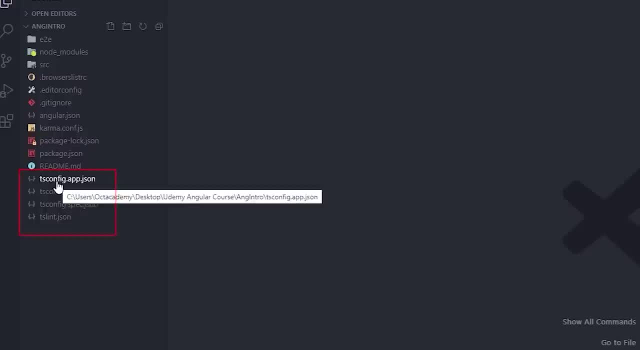 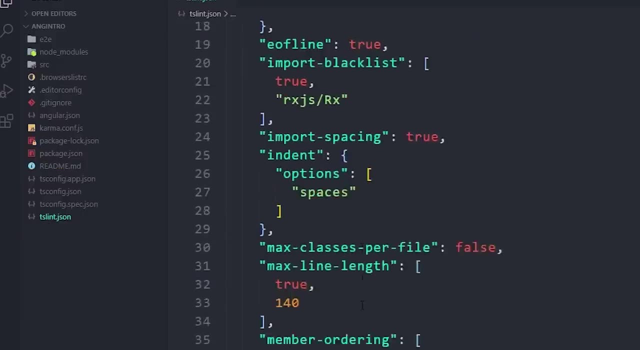 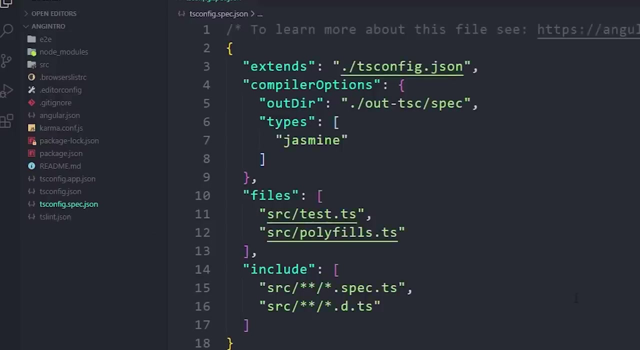 better maintainable, bug free codes. So these last 5 files are related to the typescript. So this last file, ts-lintjson file, is looking for typescript functionality errors. So next, this file, configspecjson file, is responsible for TypeScript configuration for the application test. 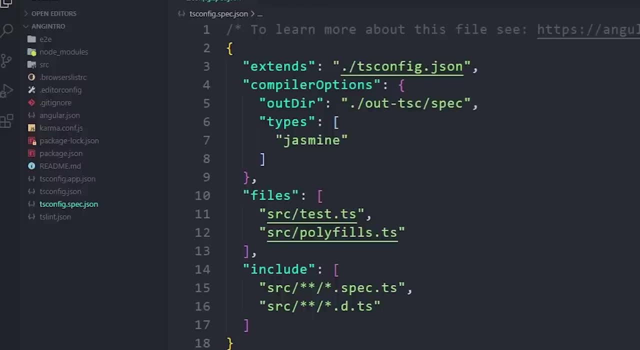 Application testing is a different topic which is not covered with this course, So just keep this in your mind. This file contains TypeScript configurations for application test. The next one is this: tsconfigappjson file. So this file includes TypeScript configuration for this Angular app as well, as this includes. 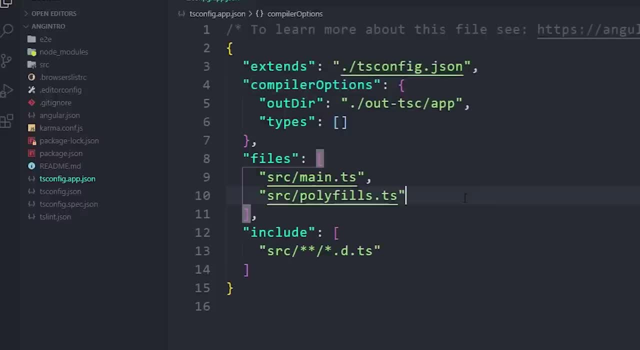 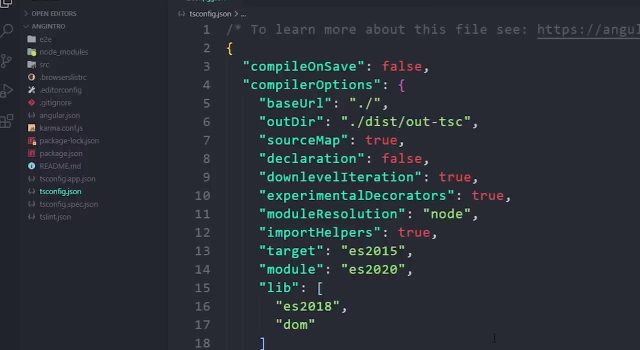 TypeScript and Angular template compiler options. Alright. next file is this tsconfigjson file. This is a solution style tsconfigjson file. This is used by editors and TypeScript language servers to improve the development experience. So this file is not doing anything with the compilers. 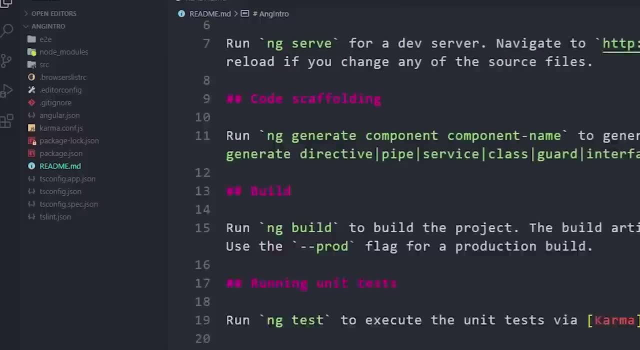 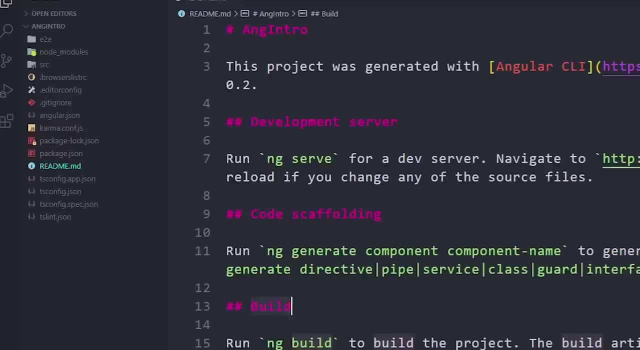 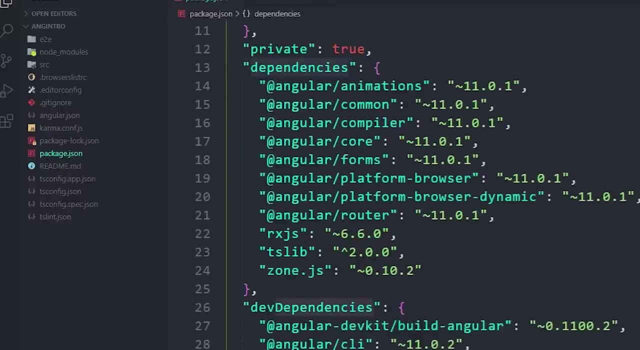 So next we have a readmemd file which includes some Angular CLI instructions: how to run development server, how to build the app, how to generate components, etc. etc. So next we have these two files. This first file, packagejson file. This file includes all the required npm package dependencies and also app details like name. 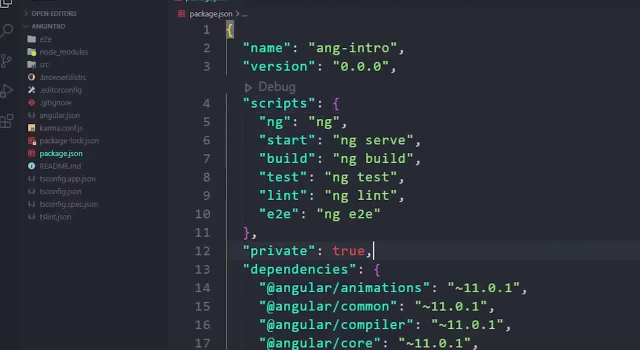 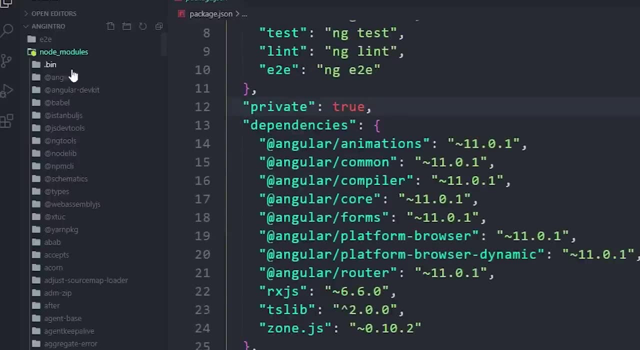 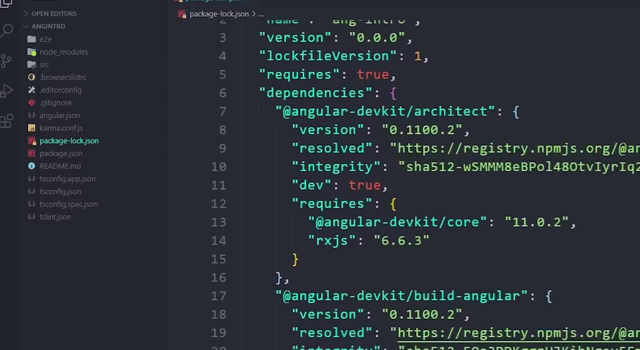 version And also the npm commands. These are all dependencies that we need in angular project. So these all dependencies installed inside this node modules folder, As you can see here, all the dependence files installed inside this folder. Next we have this file, package-logjson file, which includes version information for all. 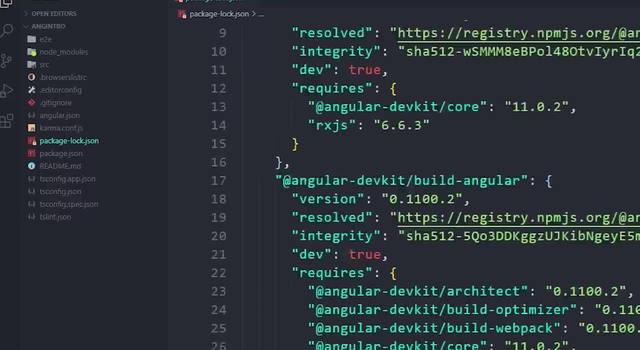 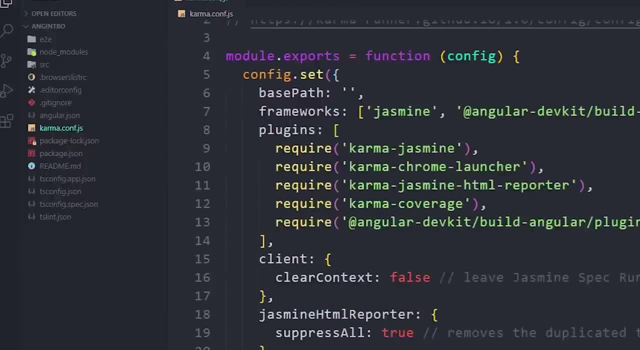 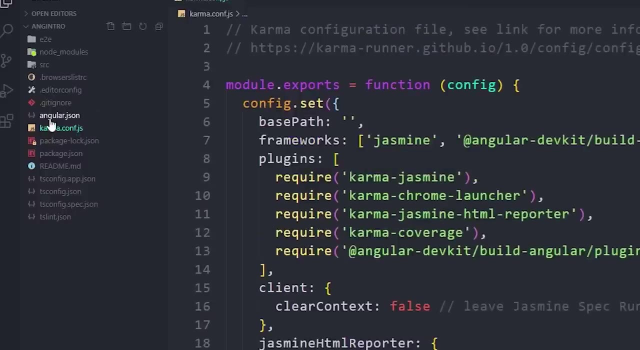 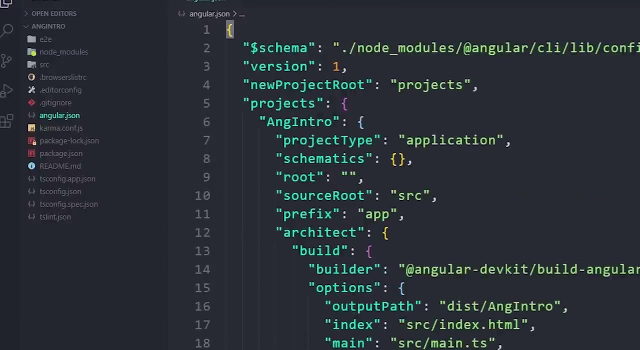 packages installed into node modules By the npm client. Alright, next we have this karmaconfjs file, which includes karma unit test config for this angular app. Next, we have this angularjson file. This is the angular CLI configuration file for this angular project. 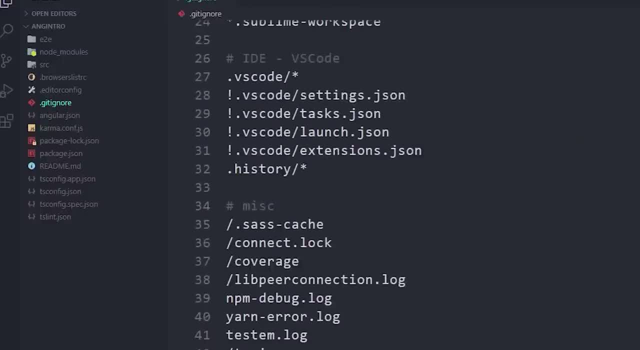 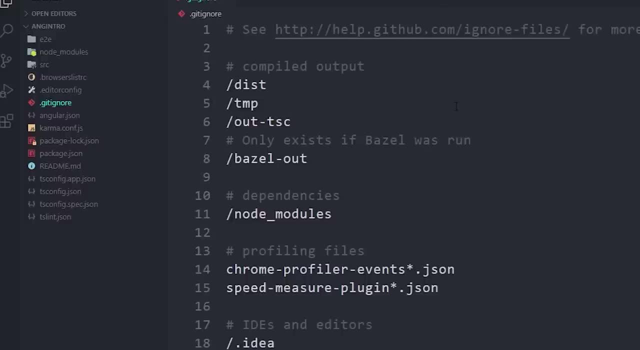 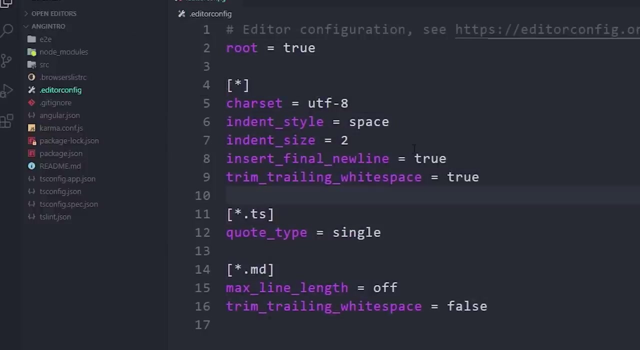 Next we have this gitignore file, Which is for specified ignored files for github rigs. So if you guys may wondering what is gitup, gitup is a version control system. So next we have this editor config file. This includes code editor configuration for this angular project. 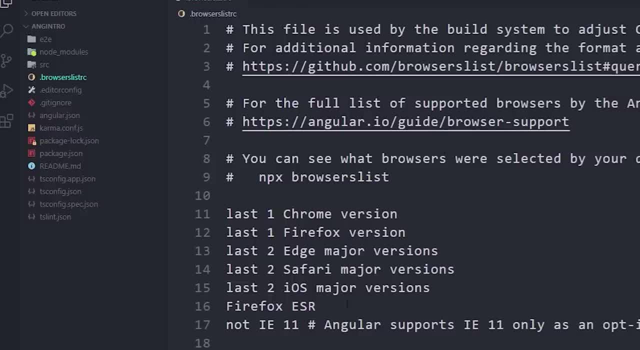 Next, we have this browser list src file, which includes different browser specific config details. Next we have these folders: This e2e folder for the end to end test files For the angular app And this node module folder, as i mentioned before, all the required files for angular. 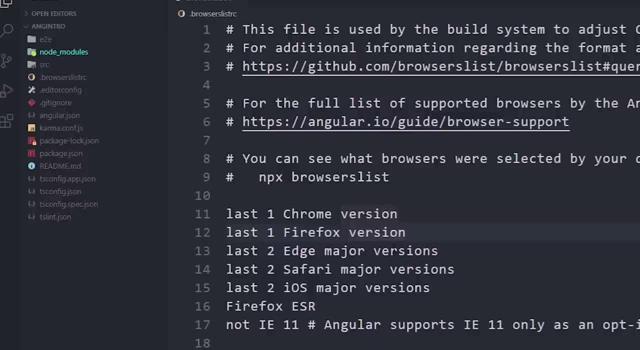 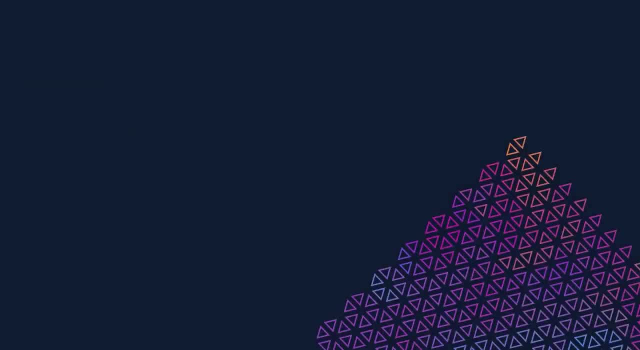 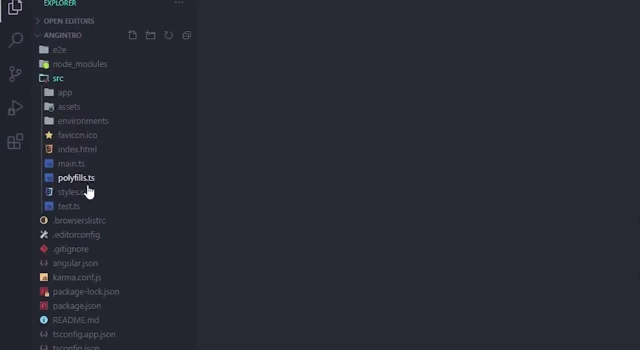 framework installed inside this node modules folder. So this is the folder we are dealing with. Inside this src folder, We can see these three folders and these files. So this is the folder we are dealing with. Inside this src folder, We can see these three folders and these files. 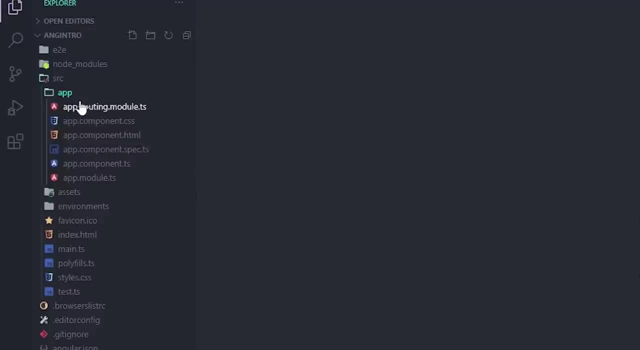 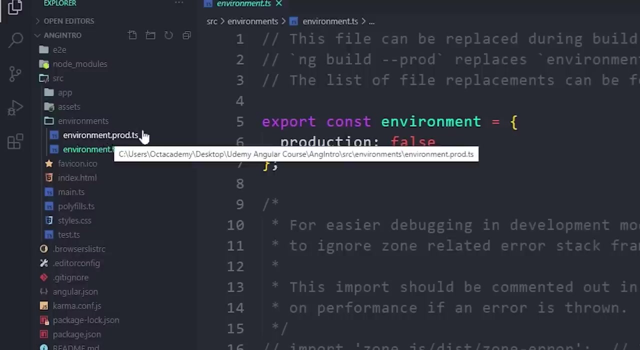 This app folder. we mostly work inside this app folder. We will generate all the files and logics inside this folder. Next, we have this assets folder where we can put our media files like images, sound files, icons, etc. etc. Inside this folder we have environment variable files, which contains all the environment variables. 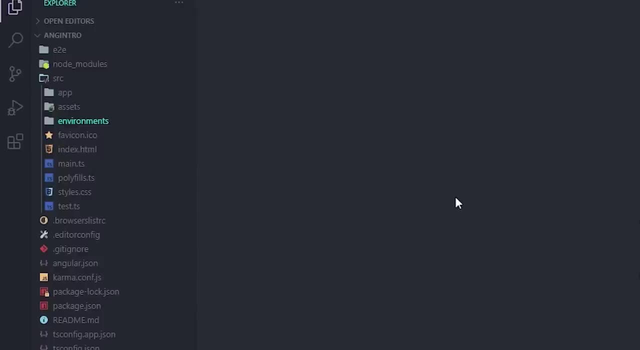 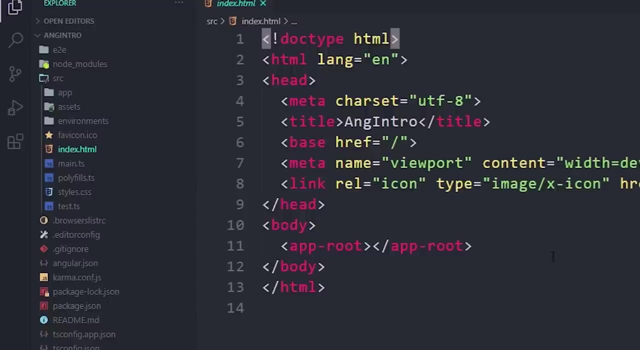 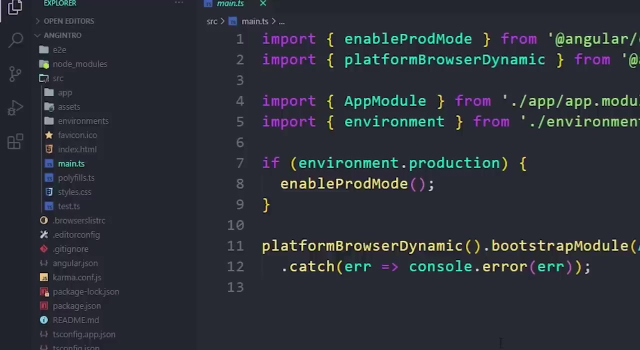 Next we have the favicon folder. This is the website icon. Next we can see the indexhtml file. This is the main index file for our angular app. Next we can see this maints file. This is the main entry point for our application. 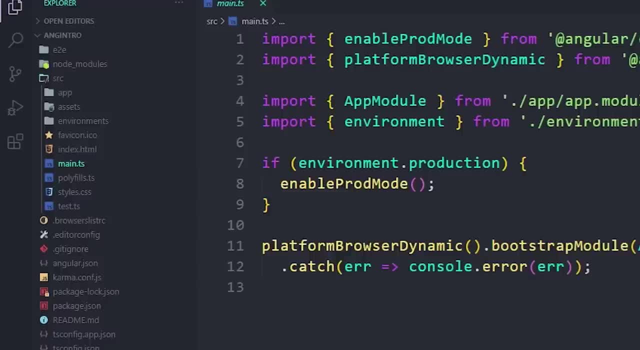 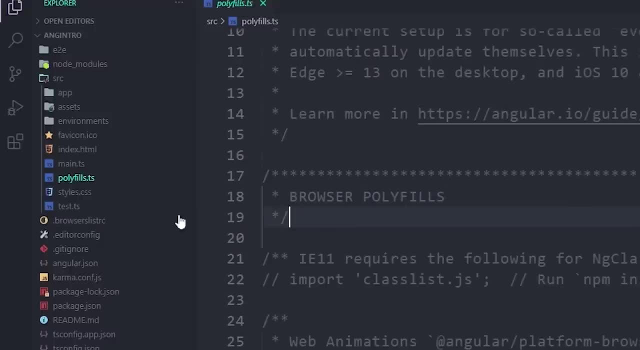 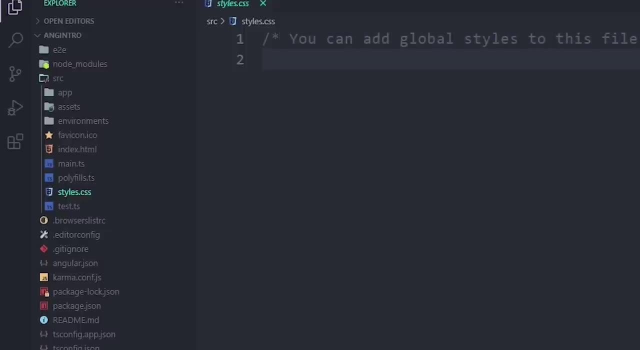 This file compiles all app modules to run in the browser. Next, this polyfillsts file provides polyfill scripts for browser support. Next, we have this stylescss file. This file is like a global main css file where we can write our css codes for the angular. 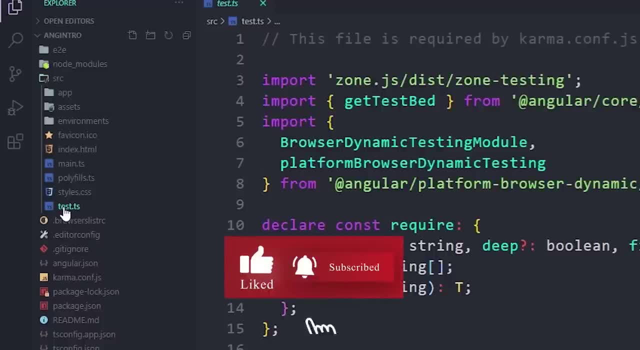 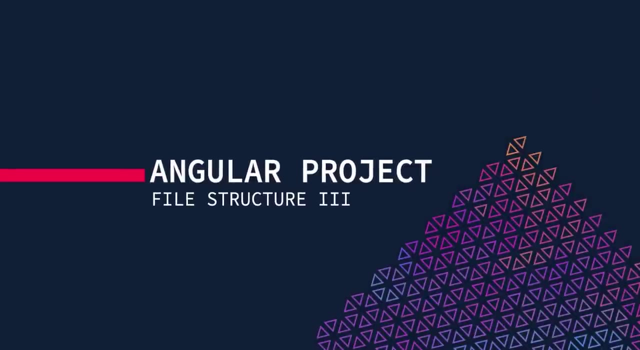 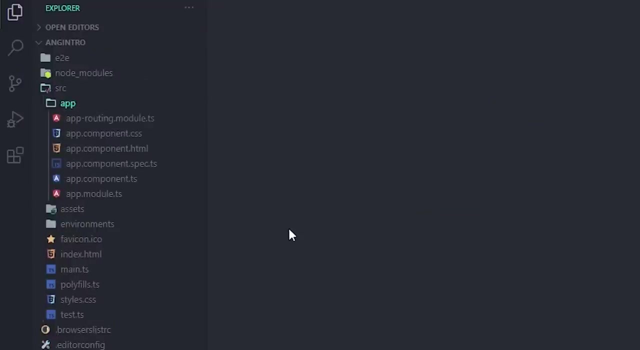 application. The last file inside the src folder is the testts file, which is the main entry point for testing angular application. Next Next, we have this app folder. If you can remember, I said earlier, this is the folder we are going to work mostly. 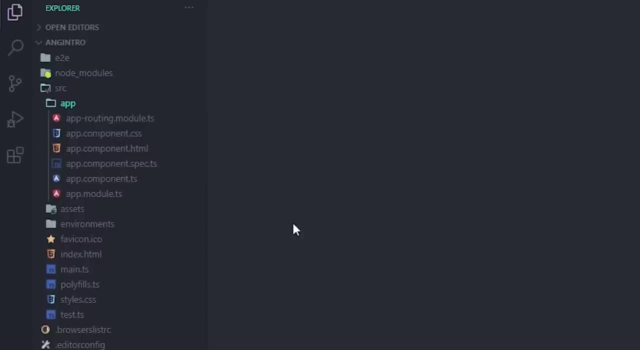 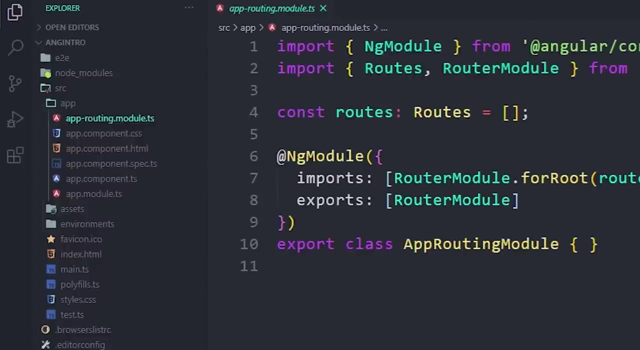 For now, I give you a rough idea about these files. In later section we will learn and work with these files in detail. Okay, This first file- app-routingmodulets file- is dealing with our app routers. If you can remember, when we creating a new angular app using the angular-cli, it was 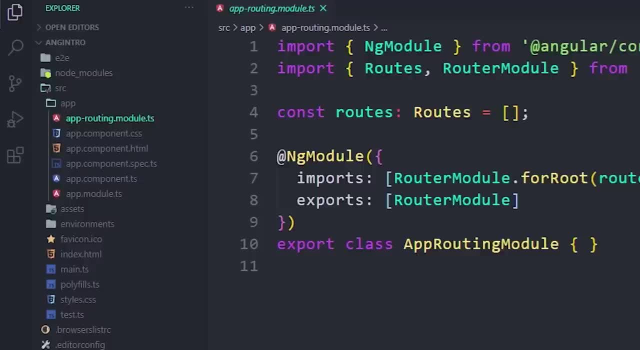 asked a question that we want to add the angular router to our angular app, So I gave yes to this. That's why we are getting this file. This is automatically generated with the angular-cli. If, in some scenario, we don't need angular routers, so that case we can give no to that. 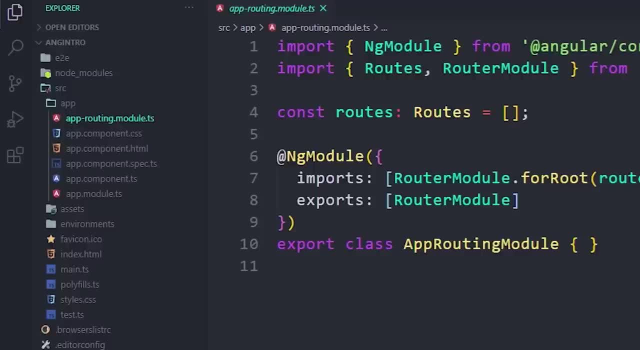 question. Then we don't get this routing file. I know some of you may think: what is this router For? now just get to know about this file. We have a separate section for this. In that section we will learn all of these in detail. 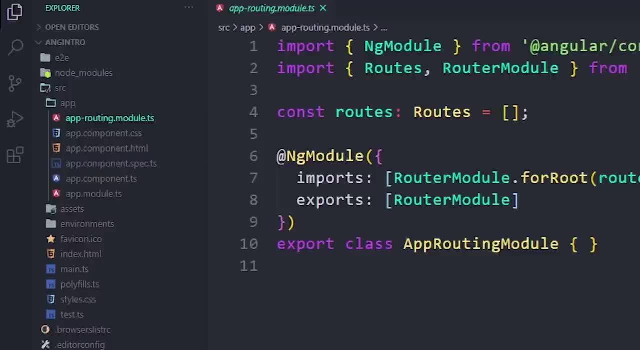 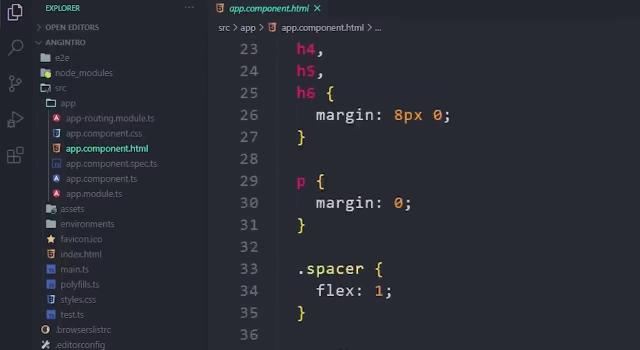 If you don't get it, leave it. Next we have this four app component files. Angular is a component based framework, So this is the main root component for our angular app. With this html file, we can markup all html codes Okay. 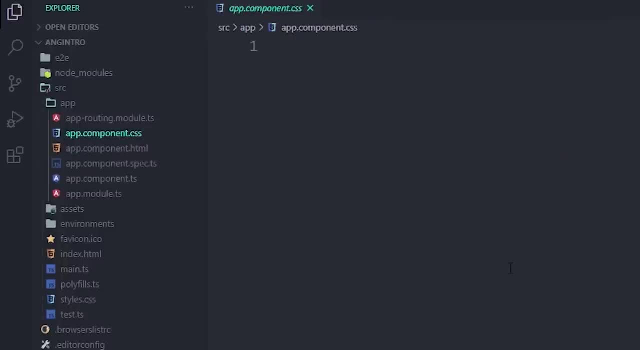 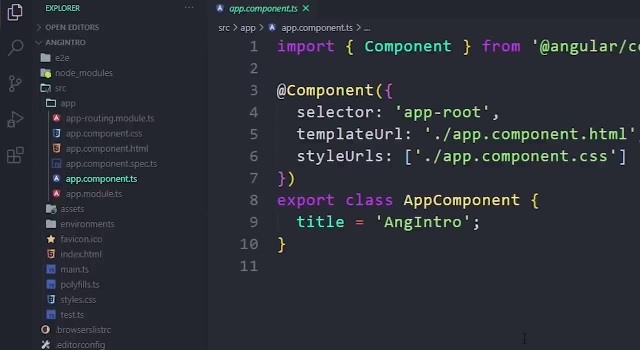 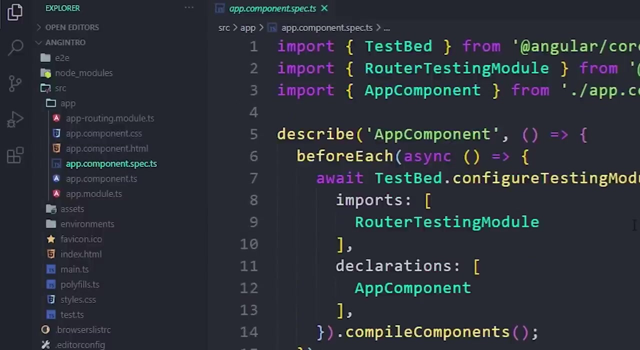 This ss file we can add the styles for this app component, So all the logics will code inside this app component ts file. And this app component spects file is for unit test file for this app component. Next we have the appmodulets file. 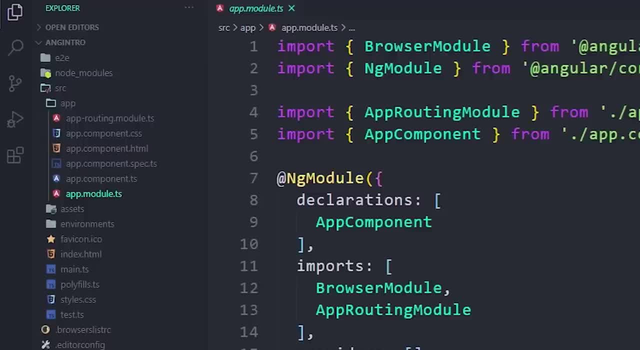 In here we define the root modules. that tells angular how to assemble the application. So inside this file we can see these imports. With these module imports we are telling to angular we are using these modules for this app. So import them and apply those modules to our app. 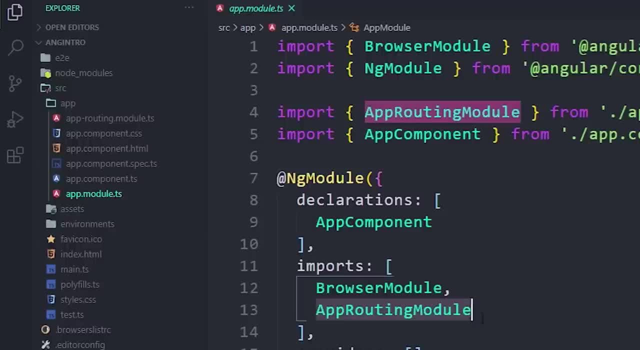 So we can see this app routing module which is for the Angular router. If we don't add this inside this app module file, angular doesn't know whether we are using the angular router or not in this app. Without this import, Angular router could not be anymore. 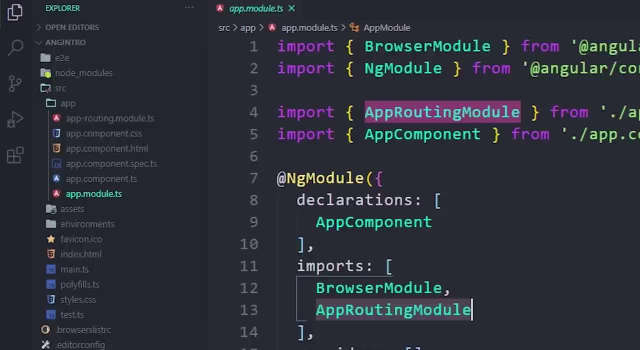 Andrew, this onsite is coming from. Next we can see this modular CI file type. an Indian informalacaknl and ic stadium democratic will not work. Likewise, here we can see this app component import. So with this angular knows, we have a component called app inside our angular app, So this file is very important. 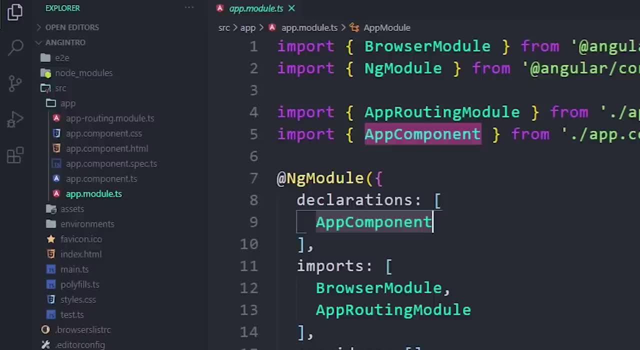 So we have to add all the modules inside this file that we are using with the, our angular app, Otherwise we will get errors. So this is it for the file structure of angular section. Some of you don't get these words: components, routers, modules. Just leave it for now By. 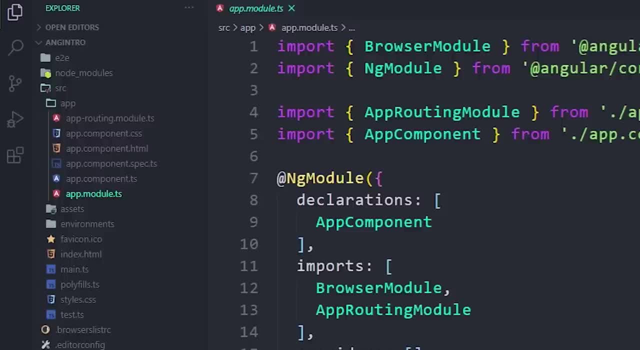 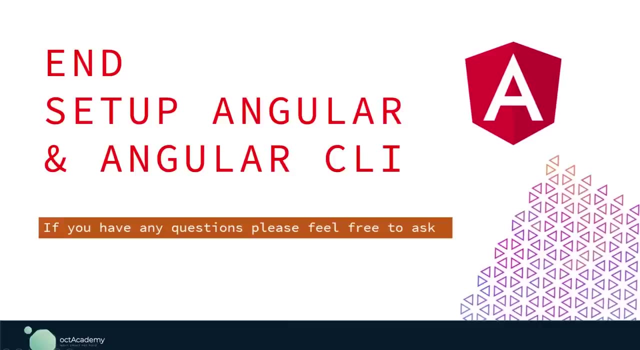 the end of this course you will get used to these words. Alright, this is it for this angular introduction. In this section we learned all about angular, Angular CLI and angular file structure. This is the start of learning angular, So you might be get lots of questions in your mind Or sometimes you may not get technical words. 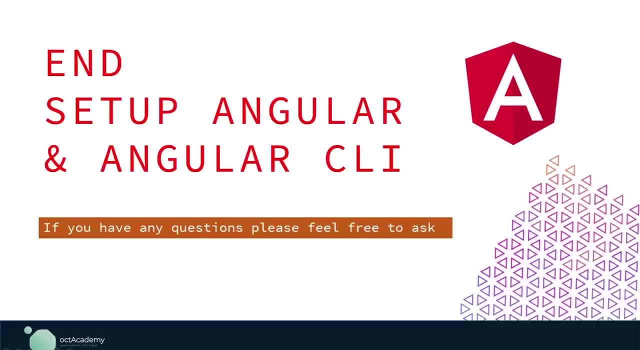 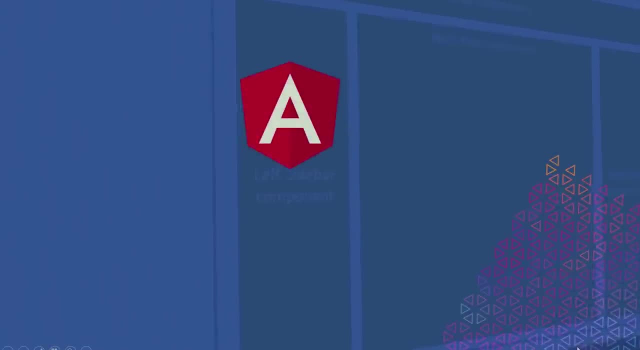 but don't worry, in later sections we will dive into the angular in detail. And one more thing: if you have any question, please feel free to ask in the Q&A area. Let's meet you in the next section. In this section we gonna get to know about angular components and its 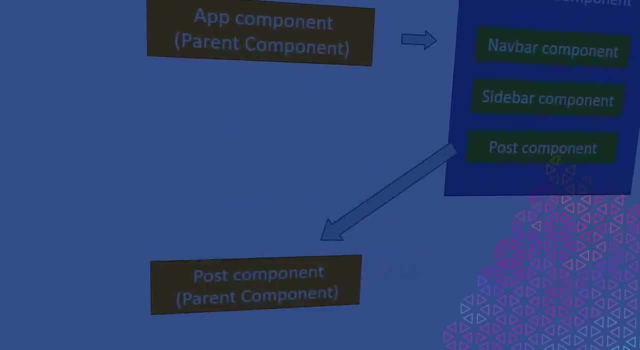 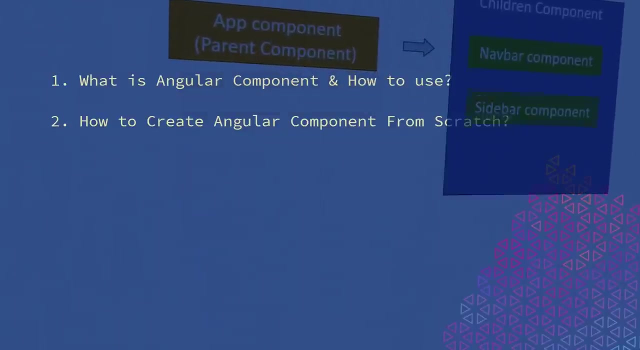 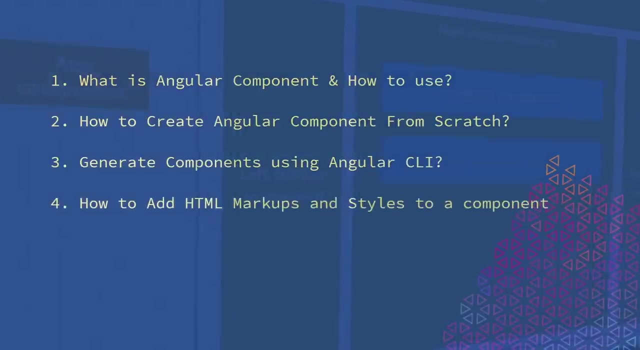 use cases. By the end of this section, you will learn what is angular component and how to use them: How to create an angular component from scratch. How to generate an angular component using the angular CLI. How to add HTML markups and styles to a component. At last, we will learn how to communicate and 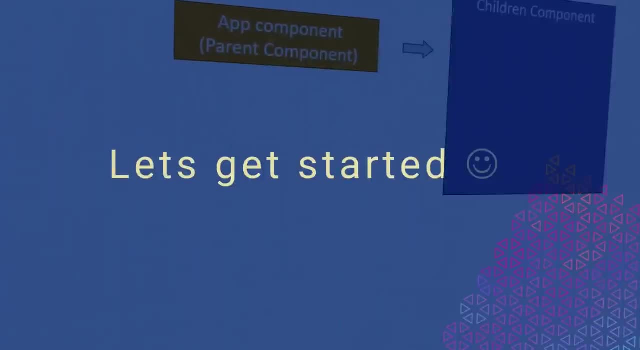 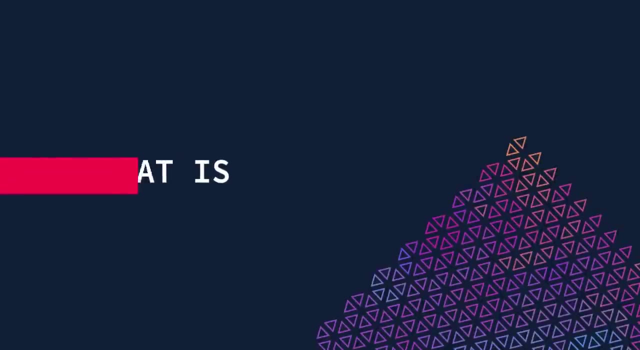 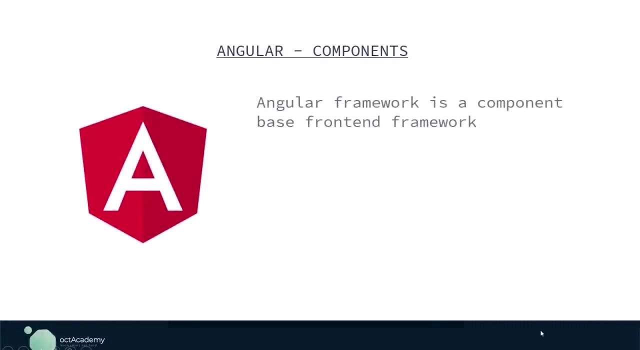 parse data between two components. So let's get started. The angular framework is a component based front end framework. The main building block of angular is angular components. Without components, we cannot build proper angular. So what is this component? The component is a combination of data: html. 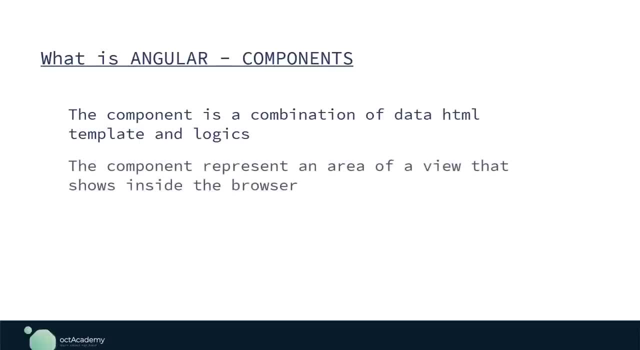 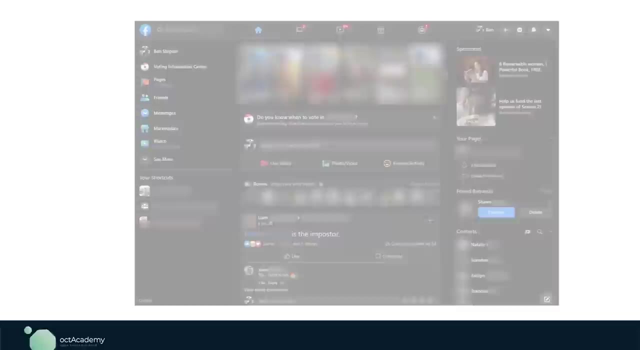 template and logics, Which represent an area of a view that shows inside the browser. So this is the view that users can see, Coz components are loads inside the browser. So let's look at a real world example. So if I take the facebook layout as an example, Facebook has this navbar right, sidebar left. 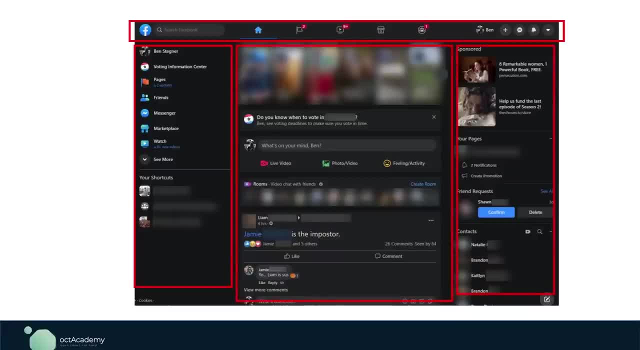 sidebar and this facebook wall which shows facebook posts In angular. we can create components for each of this layout area. We can create reusable components For this navbar. we can create the navbar component. This sidebar- left side and right side- we can create separate. 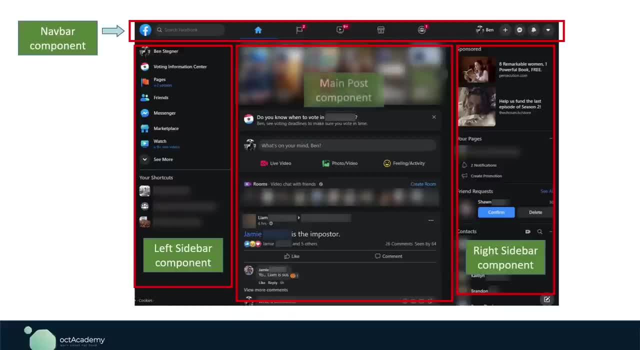 components And also for this post list we can create a main post component And also inside this main component we can create a component for a post list, So we can create this all in one page, like traditional web designs. In traditional web design we added: 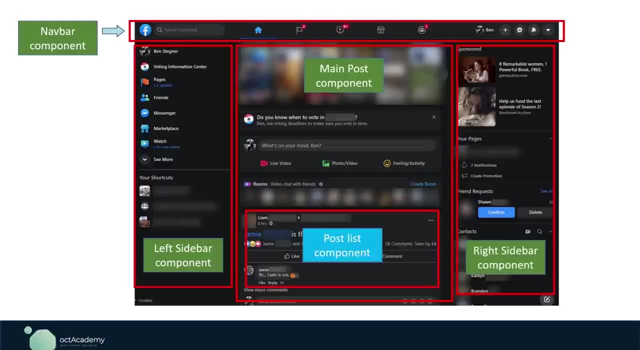 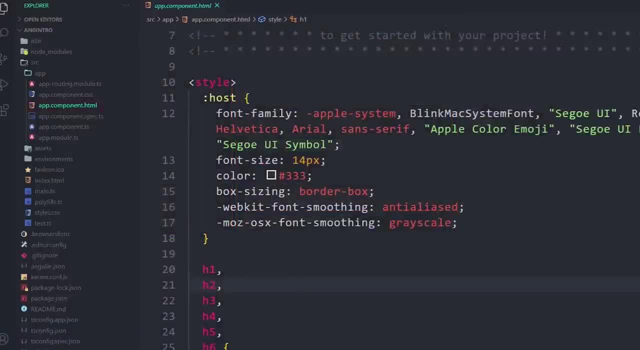 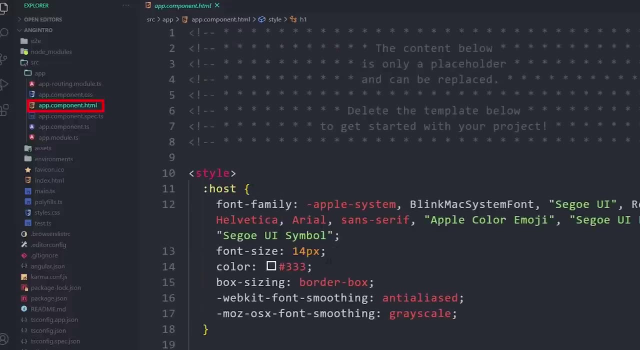 all the markups for the home page inside the indexhtml file, So like that we can add all the markups for the home page inside the appcomponenthtml file. So, if you can remember, I show this appcomponenthtml file. This is the main root file of the angular, But it's not a good practice in angular coz. 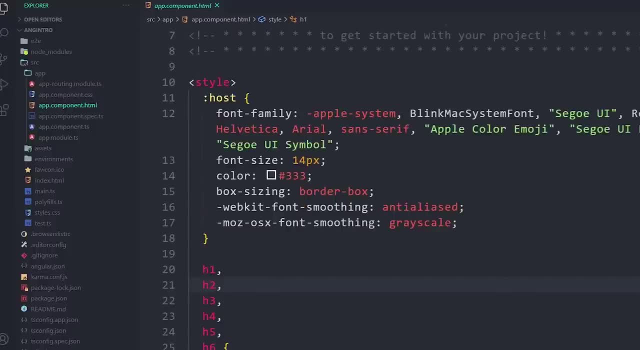 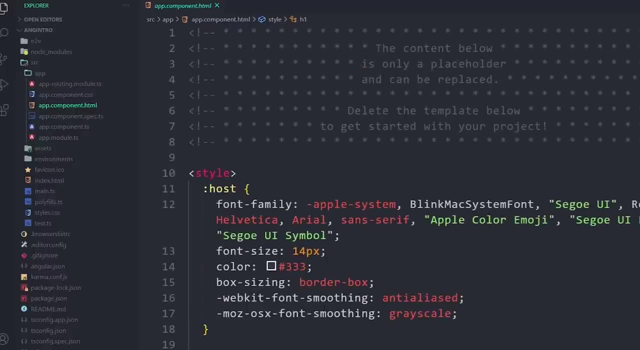 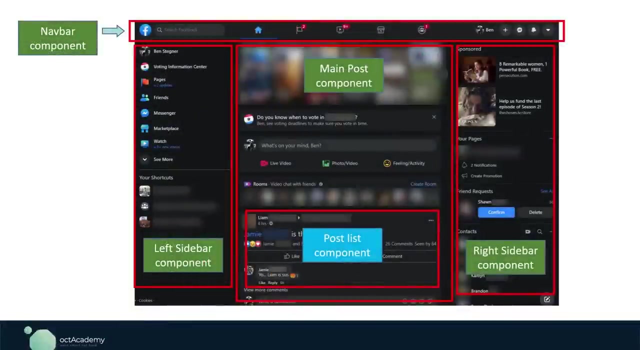 we can create separate components in angular. If we create separate components, rather putting all in one component, we can reuse those components again in our application without coding it again. This is reusable thing. For example, this navbar must be shown on all pages In this home page. 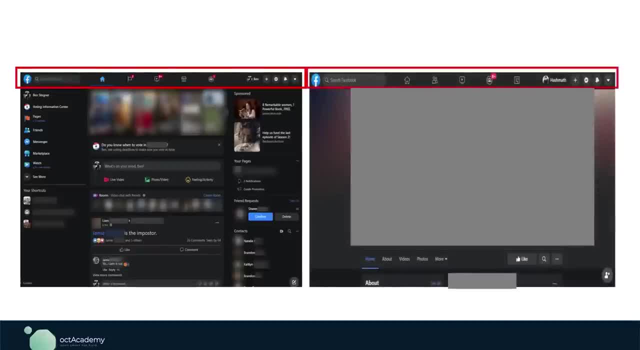 and if we navigate to someone's profile on that page also, we can see this navbar. In that case, in angular we can reuse this navbar component inside all other pages. We don't need to write the code for navbar again and again. Hope you guys got the idea. 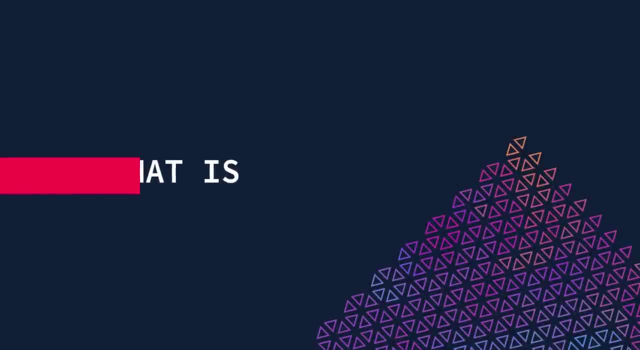 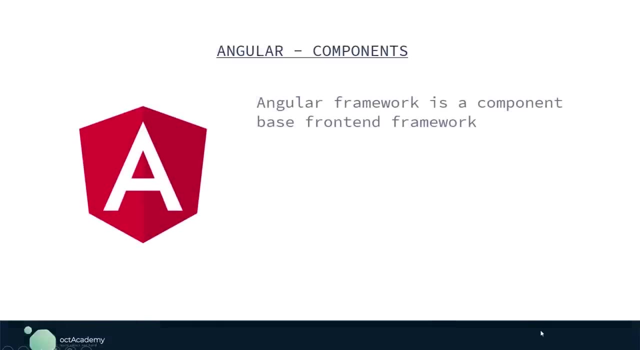 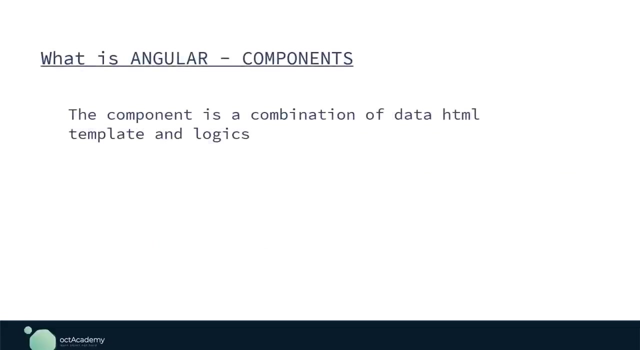 The angular Framework is a component based frontend framework, So the main building block of angular is angularcomponents电子续Choice Demo. Without components, we cannot build a proper angular App. So what is this component? The component is a combination of datahtml, templates and logics which represent an area. 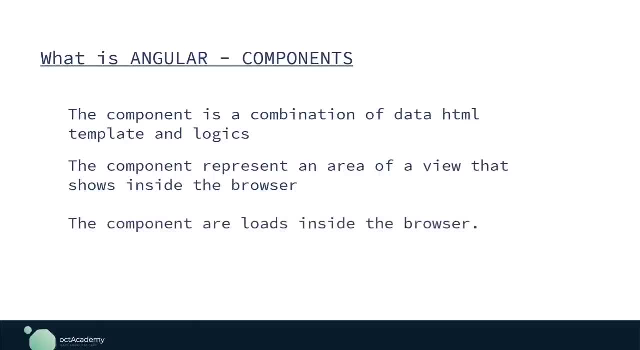 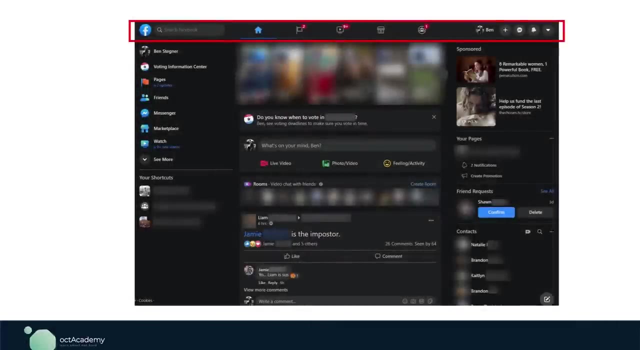 inside the browser. So this is the view that users can see, coz components are loads inside the browser. So let's look at a real world example. So, if I take the Facebook layout as an example, Facebook has this navbar, right sidebar, left sidebar and this Facebook wall. 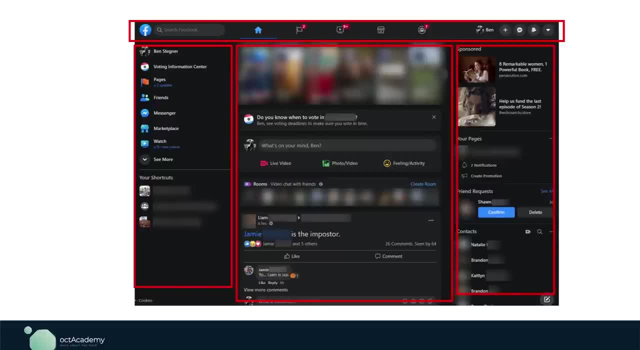 which shows Facebook posts In angular. we can create components for each of this layout area. We can create reusable components For this navbar. we can create the navbar component, this sidebar, left side and right side. we can create separate sidebar components. And also for this post list, we can create a main post component and also inside this main component. 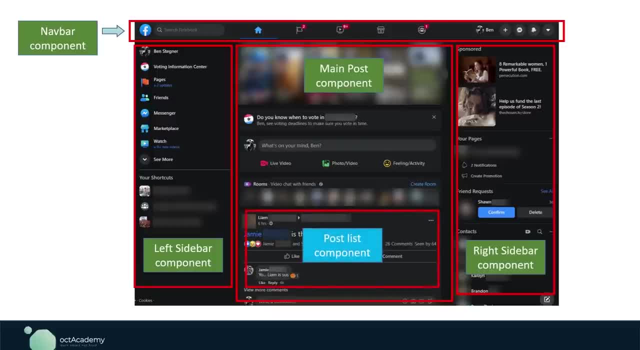 we can create a component for a post list, So we can create this all in one page, like traditionally. In traditional web design we added all the markups for the home page inside the indexhtml file. So, like that, we can add all the markups for this Facebook home page inside the appcomponenthtml. 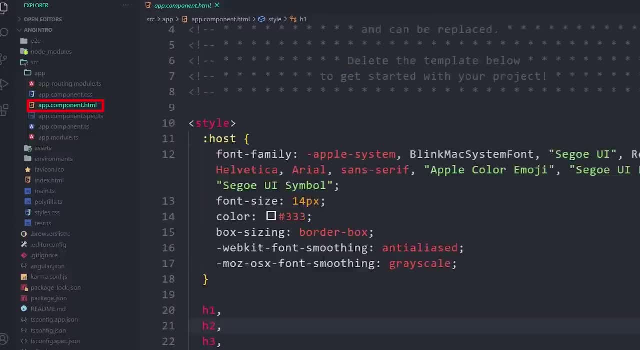 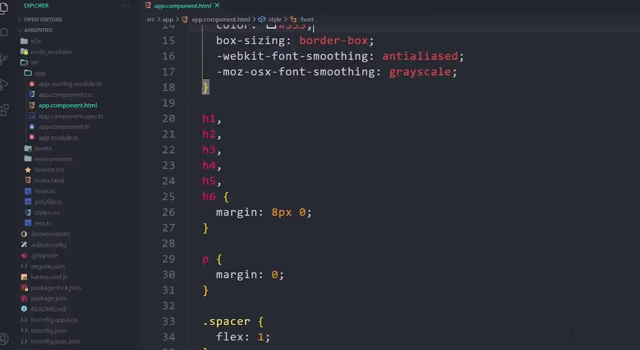 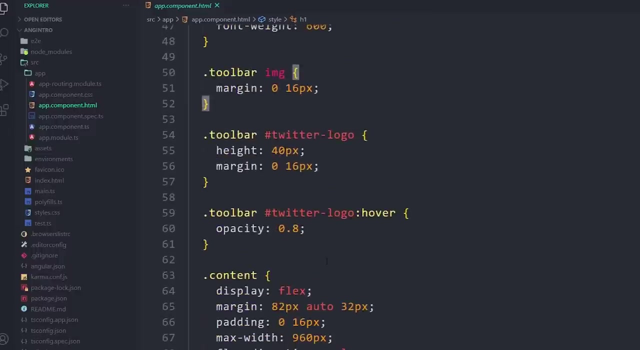 file. So, if you can remember, I show this appcomponenthtml file. this is the main root file of the angular. But it's not a good practice in angular, coz we can create separate components in angular. If we create separate components, rather putting all in one component, we can reuse those components. 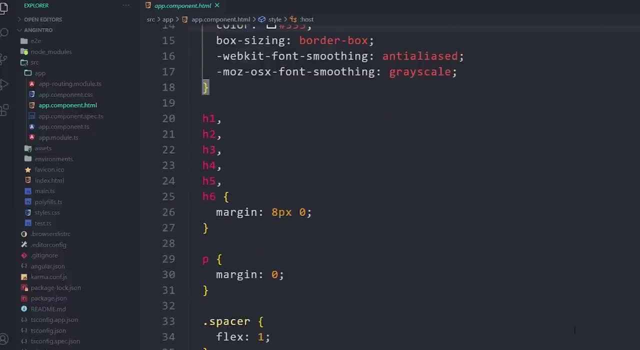 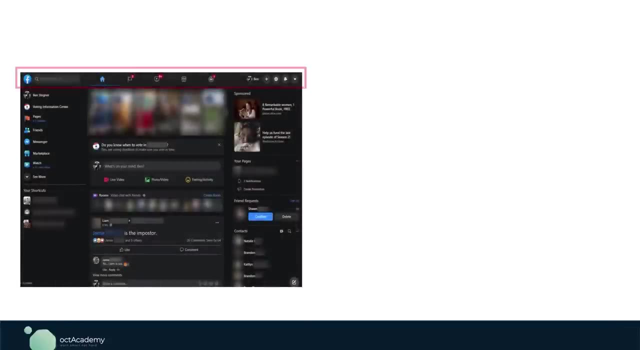 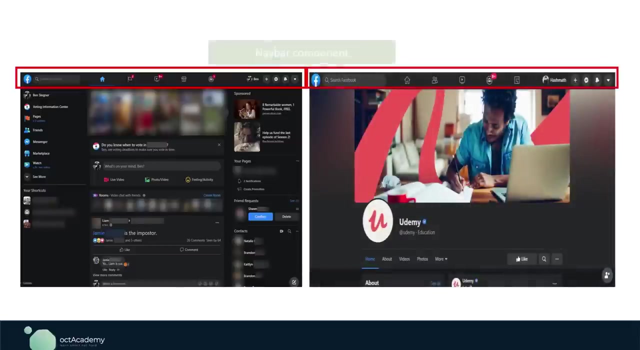 again in our application without coding it again. So what is this reusable thing? For example, this navbar must be shown on all pages In this home page, and if we navigate to someones profile on that page also, we can see this navbar In that case. 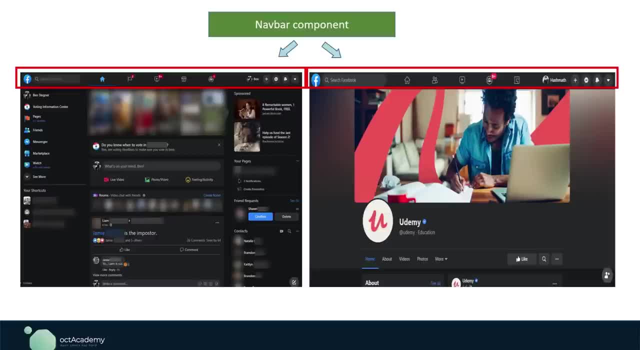 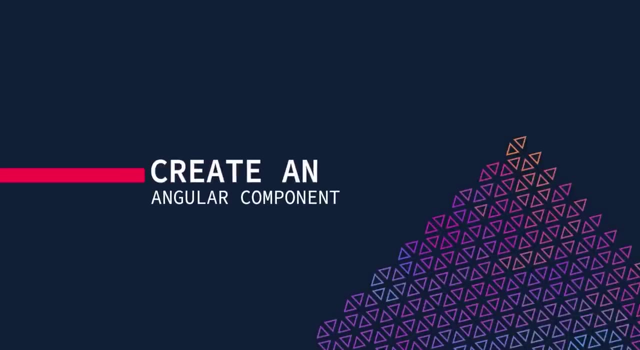 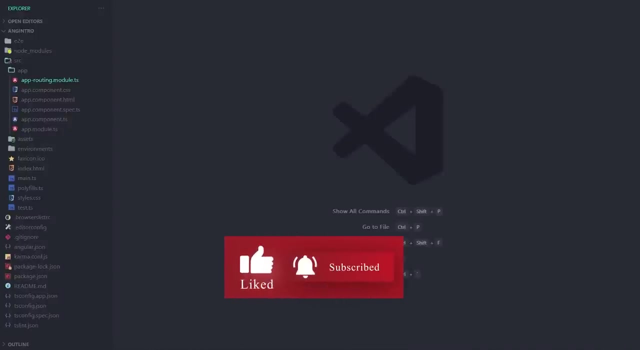 in angular. reuse this navbar component inside all other pages. We don't need to write the code for navbar again and again. Hope you guys got the idea. So now we have an idea about the angular component. Now let's see how to create an angular component. 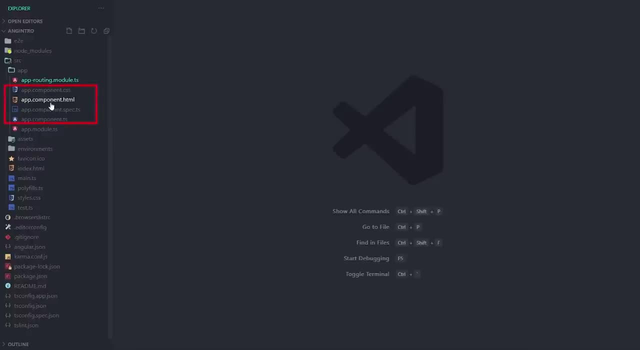 When we creating a new angular app, we got this app component, So this will be the main root component in angular. Alright, let's create this simple layout using the angular component, So we create separate components for each of this layout and we will import that component. 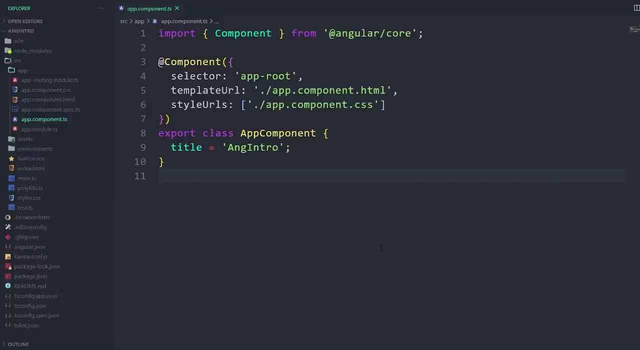 inside this root app component. So, as our example, first let's create this navbar component In angular as a good practice, we will create all the components inside this app folder. So first create a folder Inside this app folder. the folder name will be navbar, coz we are creating a navbar component. 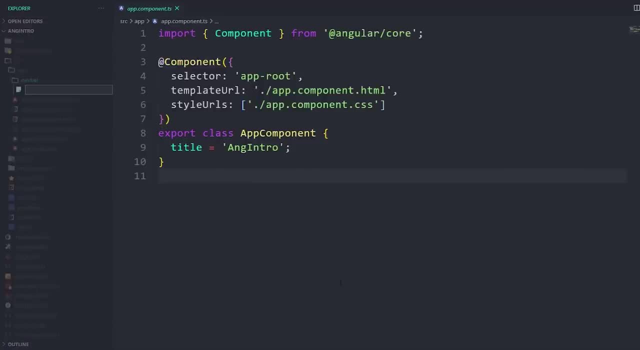 Next, create a file inside this folder. Give a name first the component name, navbarcomponent, and the file extension will be ts. If you can remember, in angular we use typescript instead of javascript. for better and bug free code experience, Angular already inbuilt the component function. 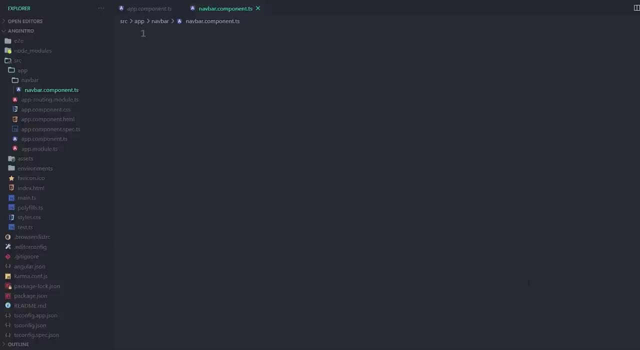 So first we have to import the component module in order to work with angular components. If you can remember, when we learn typescript we learn typescript modules. The same thing we gonna apply here. All the features of angular components are inside of another file. 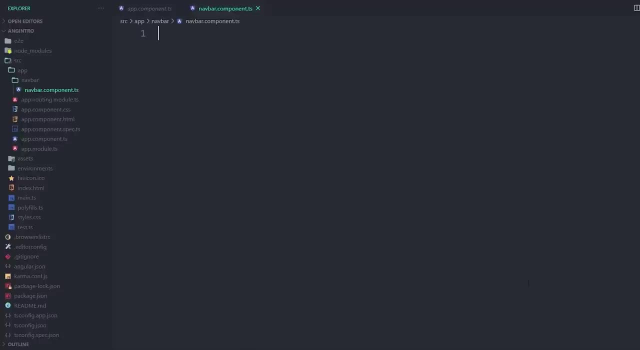 So we have to import that file to this component file. At the top of this page type import, Inside the curly brackets Modules. So module name is component. This c will be capital, Next from: So in typescript for this we have passed the path for that importing module. 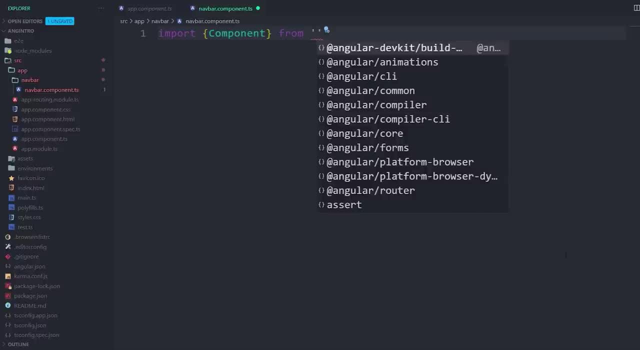 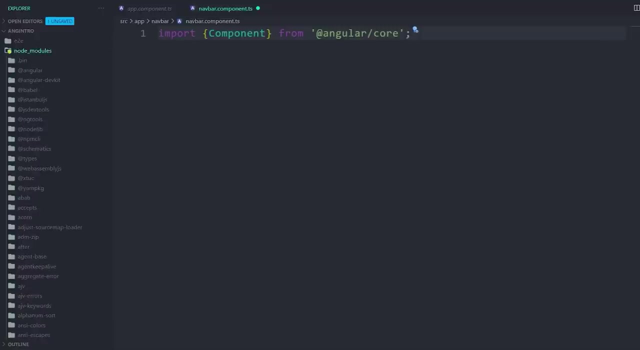 But in angular we have to import the module name Inside quotes at angular slash co. So this will be the path for this component. Actually, this is also like a path. All of the angular files are installed inside this node Modules folder. Inside this we can find this at angular folder. 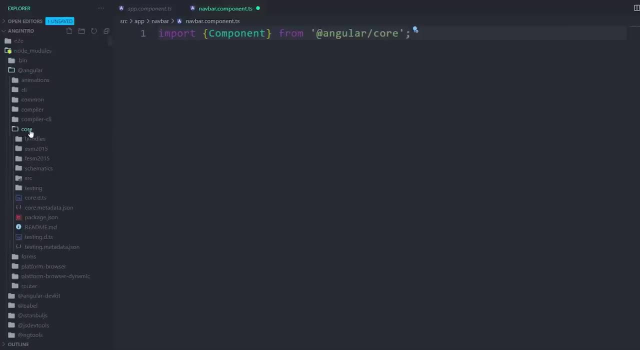 Inside this folder we can see this co folder. So this is the component modules path For this import. we are not added this node modules folder path. Cause angular already knows these files are inside the node modules folder. That's why we didn't add the node modules folder path in here. 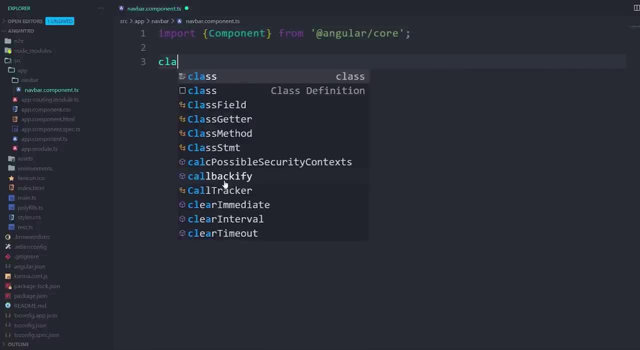 Ok, next we have to create the typescript class, First the class name navbar component. So carefully follow this. capital, simple letters: Usually we use the camel case naming convention for class names. So first letter and all the new words first letter are capital. 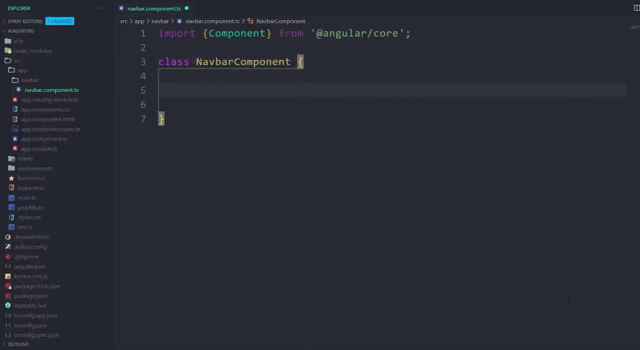 Like this: After this, add the class scope curly brackets. So still, this file is not an angular component In here. we just created this typescript class. In order to transfer this typescript class file to an angular component, We have to add the typescript decorator class called component. 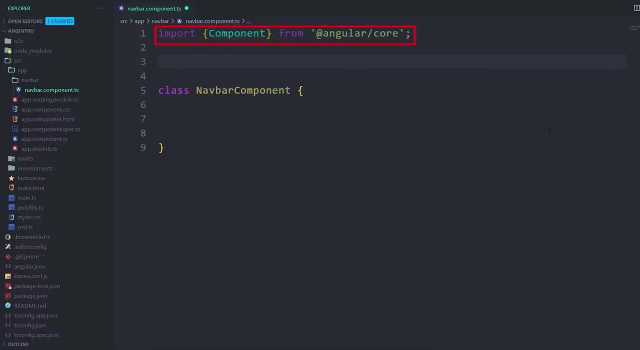 So this is the decorator we imported earlier. Now we have to use this. So in typescript we can define a decorator like this: First add sign and the decorator class name component. This also like a function. So after this parenthesis, Inside this parenthesis. 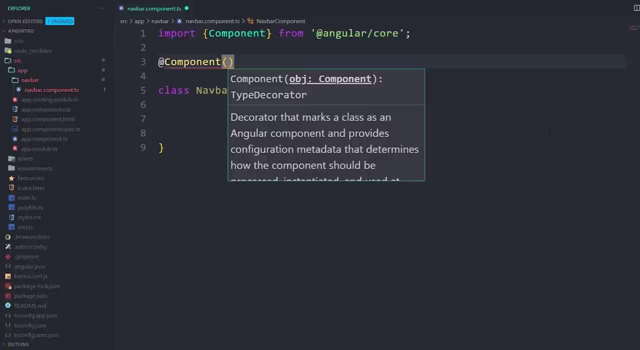 We have to pass Some values as an object. Alright, first we have to pass the selector value for this component Selector. colon and selector name will be app-navbar In angular. for this component selector we give app as the first name And then we will give the component name. 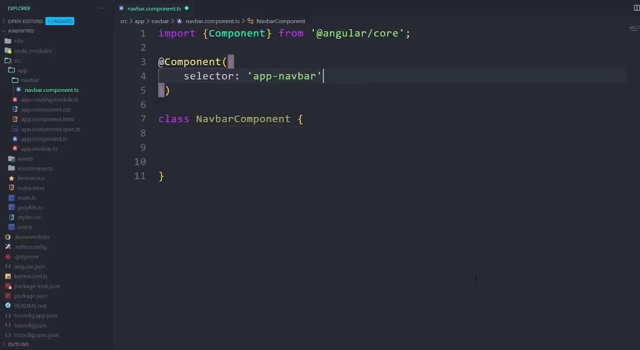 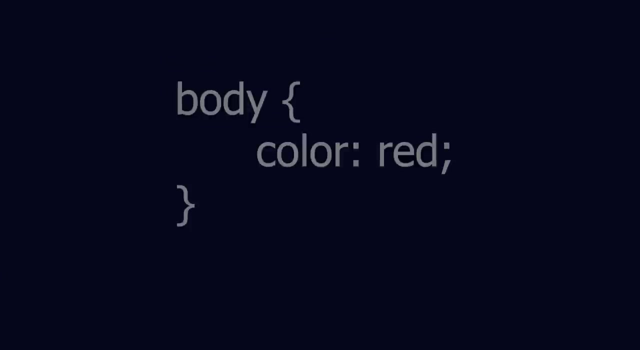 So this is just a common naming convention for an angular component. So you may wonder: what is this selector? This selector also similar to css selectors. in css We use selectors to define css For html element. we use the html tag name like this: 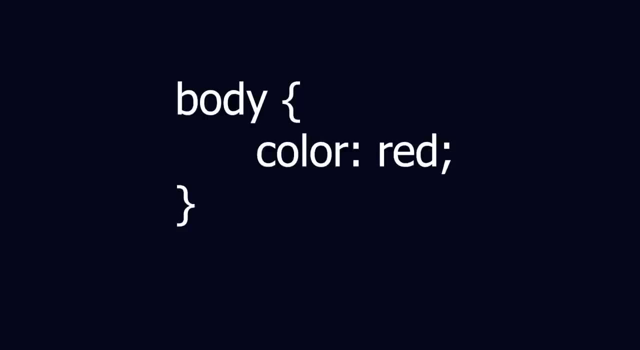 If the element is body tag, we use the body selector. If we have a css class, we use something like this and the class name. You got the idea right. This is simple css. 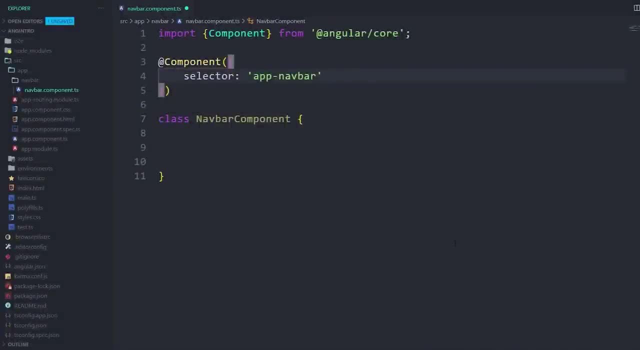 Like these css selectors In angular component also, we use selector value to identify this component. Hope you guys got the idea Alright. Next we have to pass the template parameter for this. 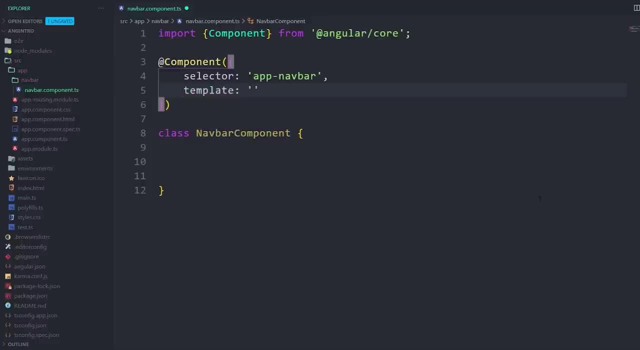 So we have to pass the html markup for this component. For example, for now, I pass an h1 tag here And between this h1 tag add this, The navbar component, and save this file. Now we have created the component with this component decorator. 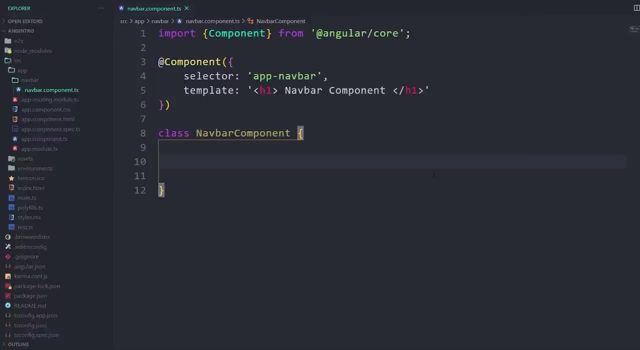 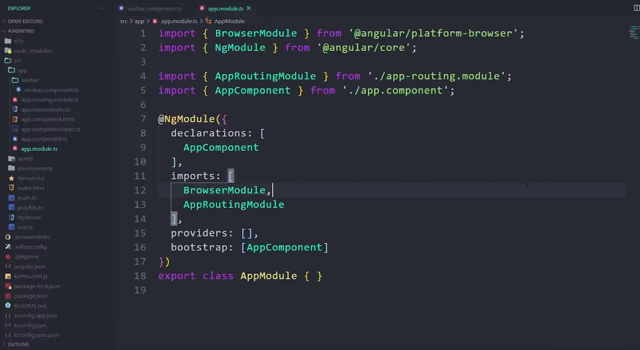 Next we have to register this component in angular modules. then only angular knows this app as a navbar component, otherwise this component will not work. So open this appmodulets file. This is the main app module file. In here we have to register our newly created navbar component. So inside this appmodulets file we can see these declaration: 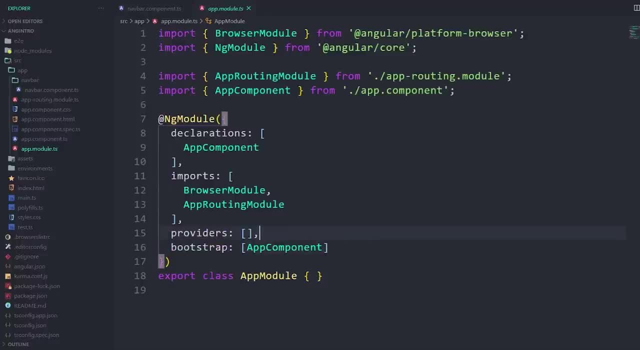 imports providers and this bootstrap inside this ngModuleDecorator. So don't worry about these all. we will learn this in later section. So in this component section we will learn about this first declaration. As you can see here, the main default app component is already registered here. 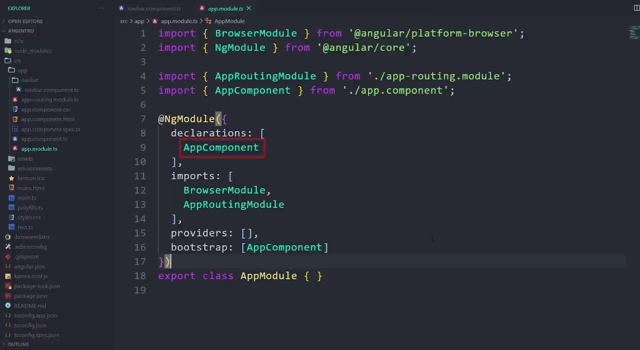 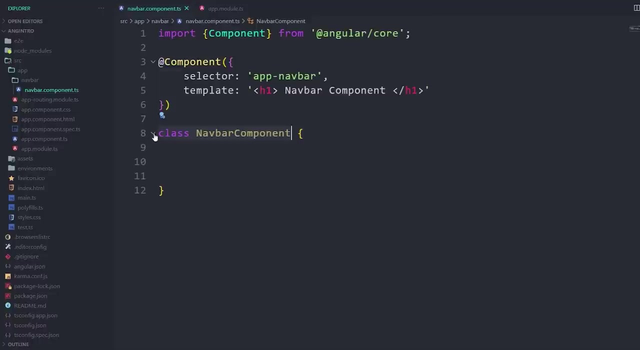 Like this: we have to register our navbar component First we have to import the navbar component to this file. So before we import the navbar component to this file, first we have to make the navbar component class export. Otherwise we cannot access this navbar component class inside. 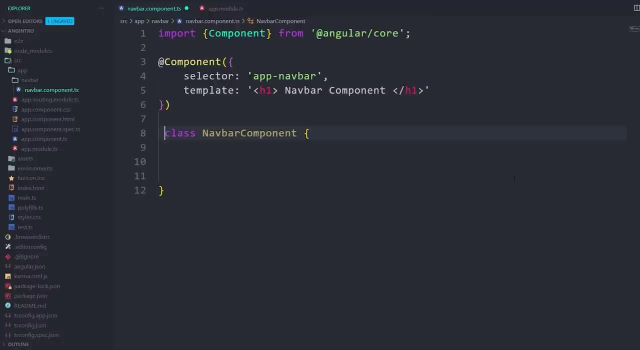 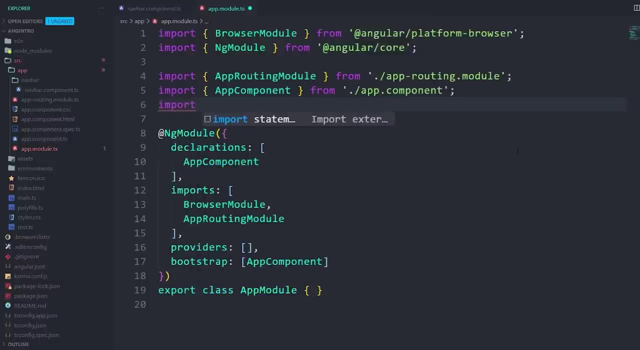 another file. So back to the navbar component file and add this export before this class keyword. So if you can remember, we learn about this in the typescript section. Next, back to the appmodulets file, Top of the page. add the import Import inside curl brackets. 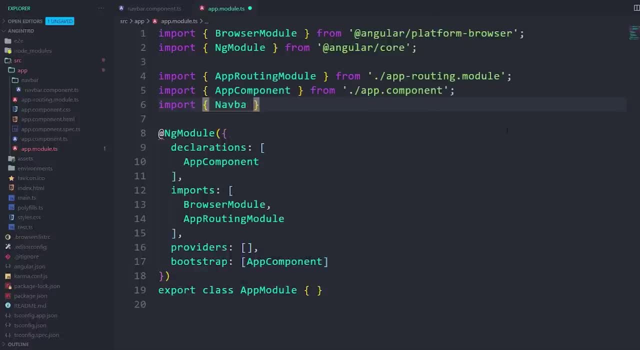 The component class name is navbar component. So once again follow the capital simple letters carefully. After this from: and the path inside quotes dot slash. This is inside the navbar folder. So navbar slash, navbar dot component. And one more thing: We don't have to pass the file extension. 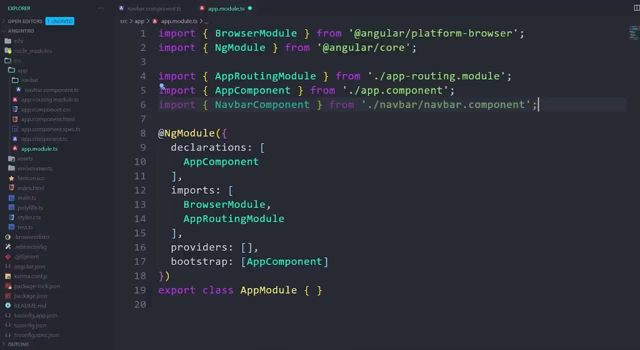 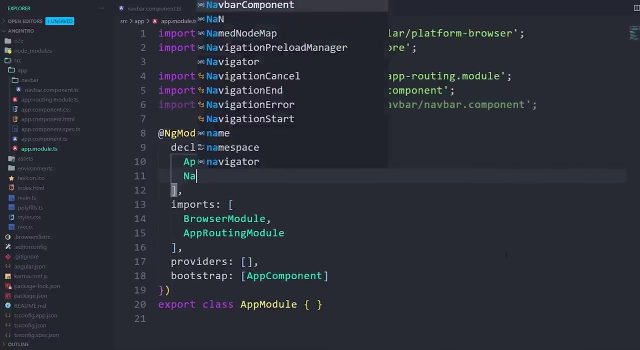 The angular compiler already knows this extension. If you put the extension here, we will get this compile error. Ok, next we have to add this imported component inside the declaration, Like this app component, After this comma, and add the navbar component. Alright, we have successfully registered the angular. 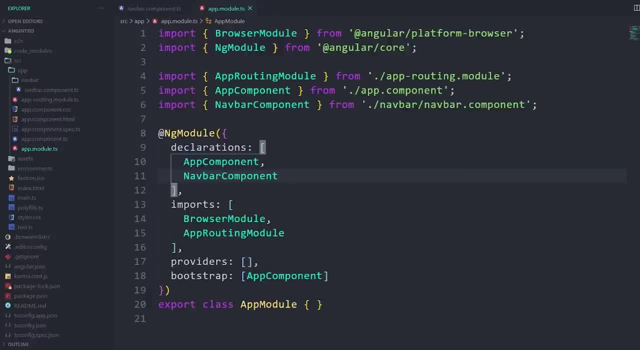 navbar component. Now we have successfully registered the angular component in navbar, So in order to see this component, first we have to run this app. so let's run this app, open the integrated terminal on VS code, go to the web and select this terminal, or we can. 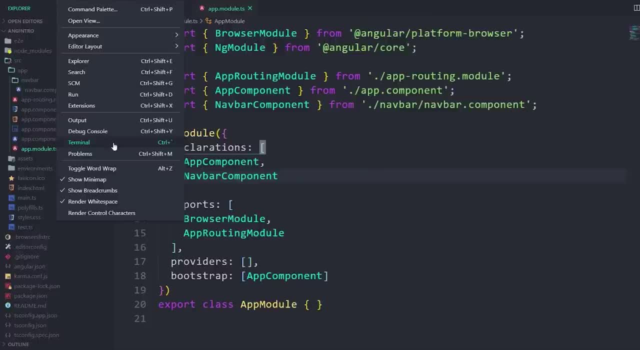 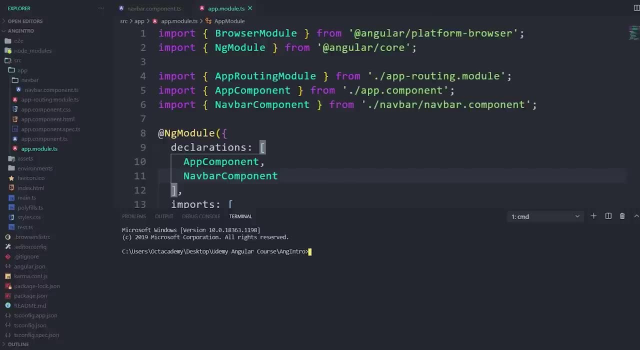 use this keyboard shortcut ctrl and the backtick key inside the terminal. run this angular CLI command to run the angular app ng serve and hit enter. so once it's completed, go to this URL on your browser. I will use Google Chrome as my default browser throughout this course. if you guys also can use the same. 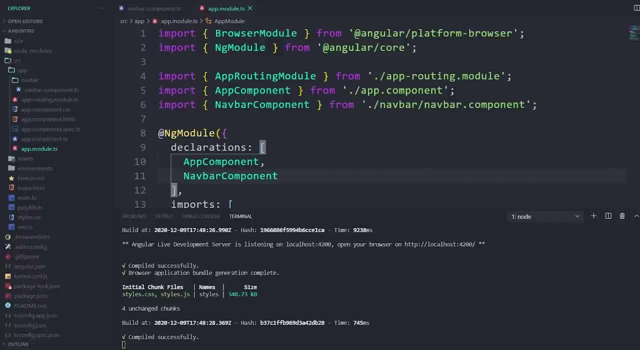 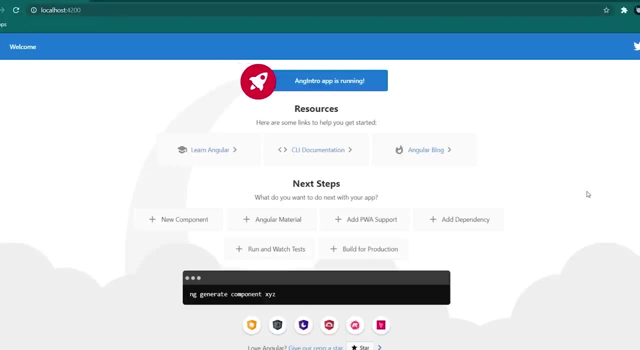 browser. this will reduce the most of the errors. so go to this URL, localhost, colon 4200, for an angular app. the default port will be 4200 in case, if your computer using in this port for any other servers, we can use this port to run the angular app, and if you want to use this port for any other servers, we can. 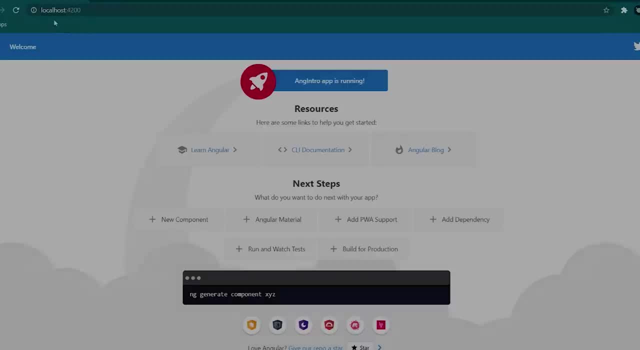 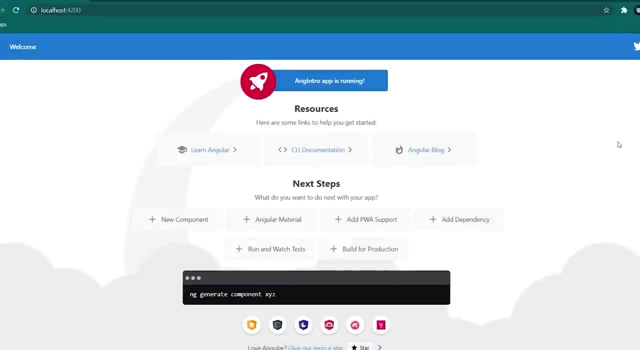 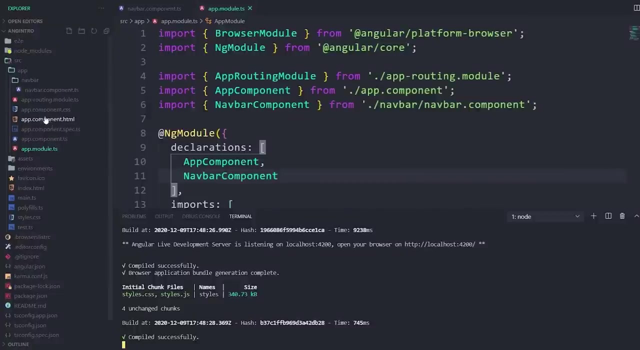 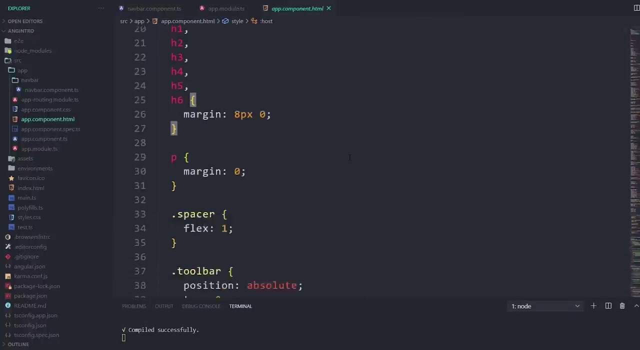 define the port when we running the ng serve. just simply put the port flag and type a different port number like this: alright, this is how the default angular app landing page looks like. all these markups are inside the app component HTML file. so I don't want this, so I will remove this. so back to the VS code and 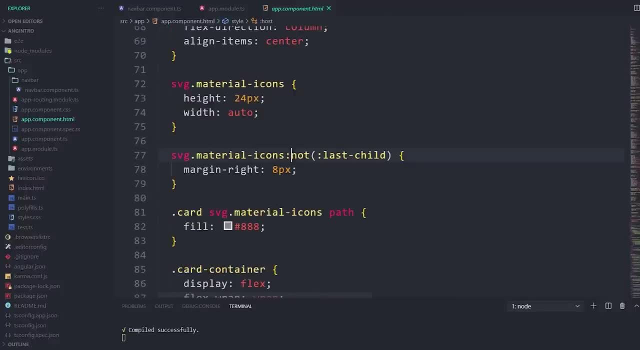 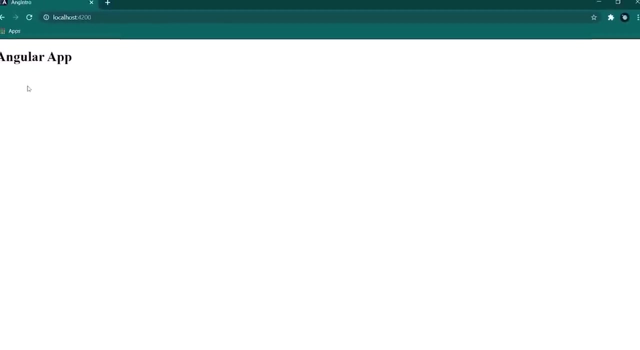 go to the app component HTML file and remove all these softwares. then go to the Menny add dying type return. LET read this after this: just put an h1 tag inside this h1 tags. add this angular app, save this file and incorporate this file. 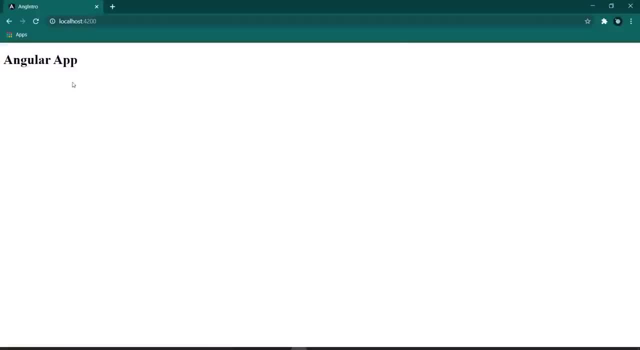 in the which case, comment tracing and return back to the browser. so now we can see this h1 tag and I add such a dot in the top values also to the thing element or the using keyboard shortcut control shift and I, so inside this we can see the h1 tag with some angular attributes. these attributes are coming. 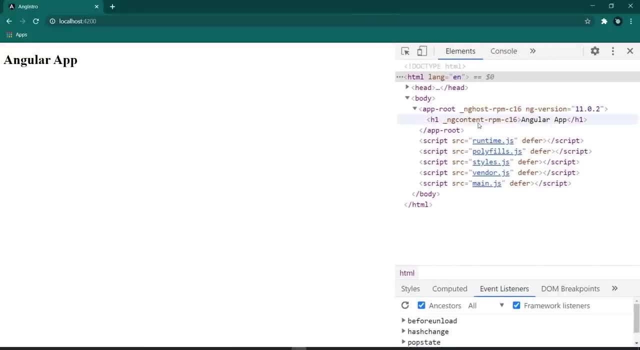 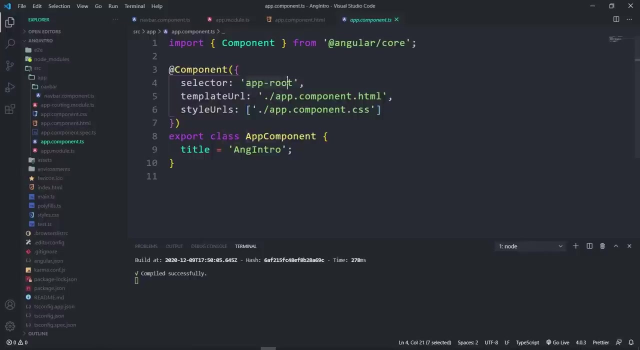 with the angular, so don't worry about that. we are not going to deal with these attributes. so what I want to show is this: app-root-tag. in HTML there is no element something like this. so what is this? if we open the app component is file inside this component decorator we can see this selector app-root. so this is: 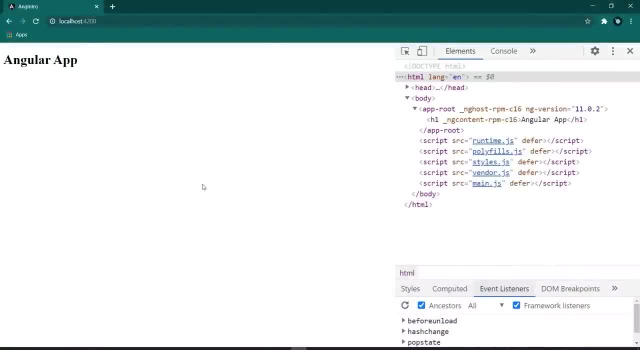 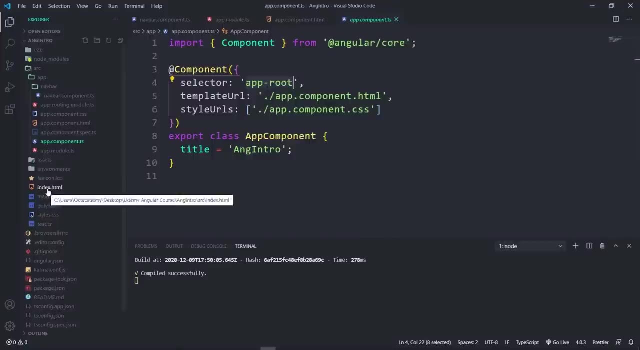 what we see here. now you may wonder how this appears inside the browser in angular component. in order to show a component inside the browser, we will use this selector as an HTML element. so open this indexhtml file. as you guys know, this is the first file load. 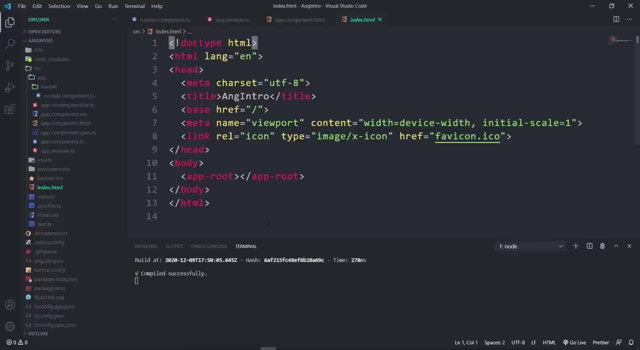 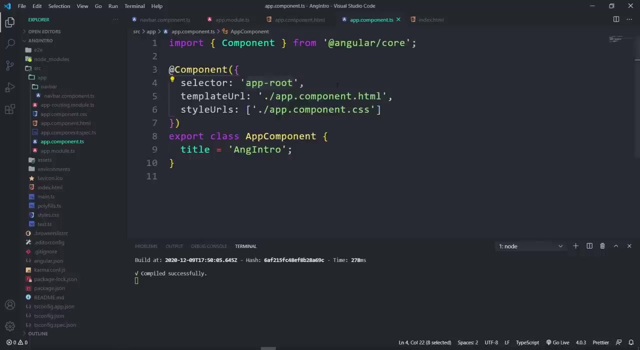 inside the browser. when we open the angular app inside the browser, inside this indexhtml file we can see this app-root-html custom tag. so this app-root-tag represents the app component. so this is how we got this app-root element inside this inspect file element. if I remove this component element from here, remove this now we. 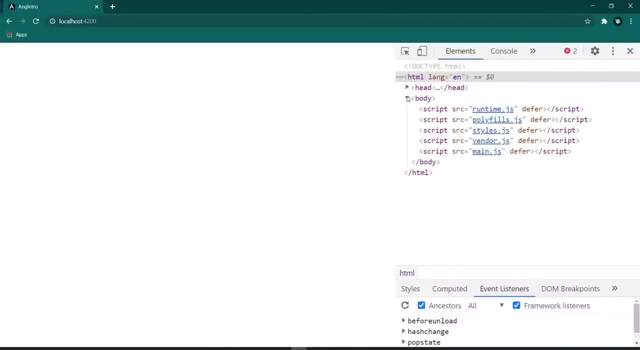 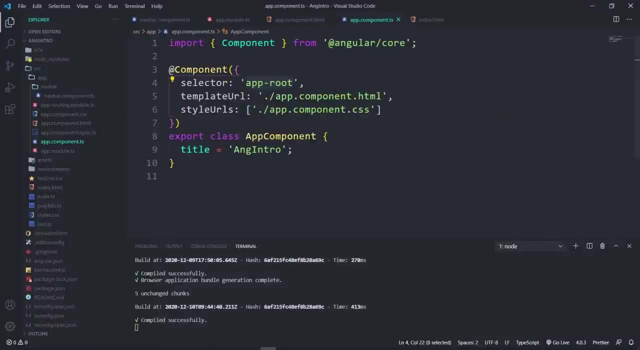 cannot see anything here, and also now we don't have the app-root tag inside this inspect element. so once again, we use this component selector as a component identifier. in order to render this component inside the browser, we use this component selector as an HTML custom tag. hope you guys got the. 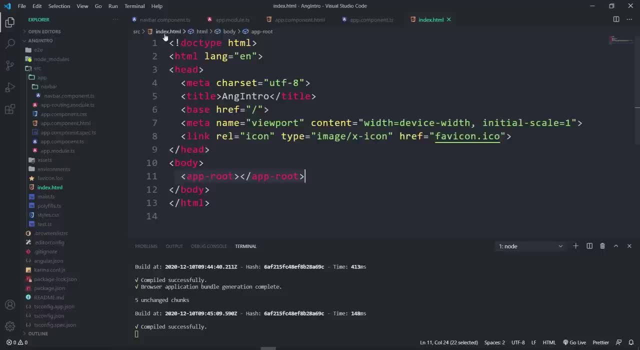 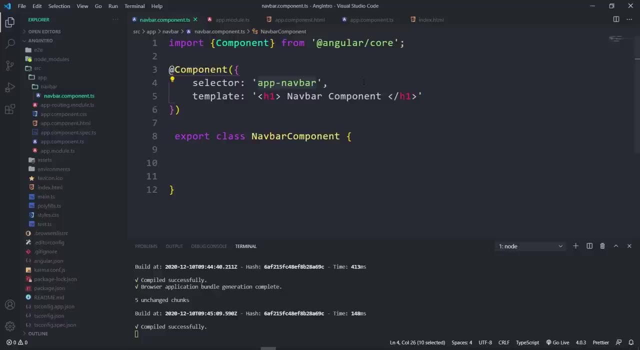 idea right. so now, like this: I want to show this navbar component inside the browser. so the navbar component selector is the app-navbar. so inside the app component HTML file, after this h1 tag, add the navbar component selector, app-navbar, and hit the enter. so you guys may wonder why do? 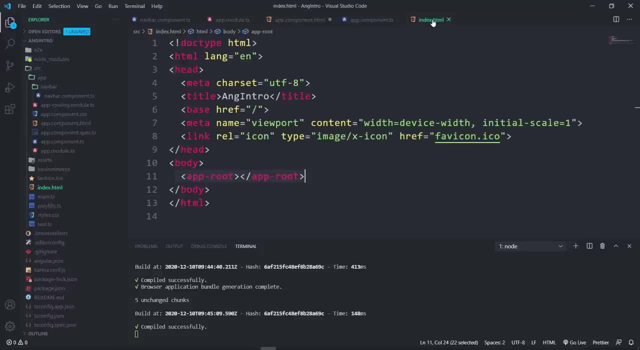 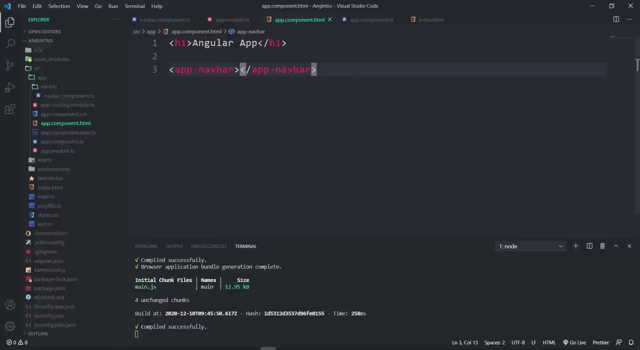 we had this navbar component inside this app-daMakeи ade component file, rather adding this straightly to this indexhtml. like this app component Coz in angular, we consider this app component as our main root component. we don't touch this indexhtml file, we only work within this app folder and we put all our components. 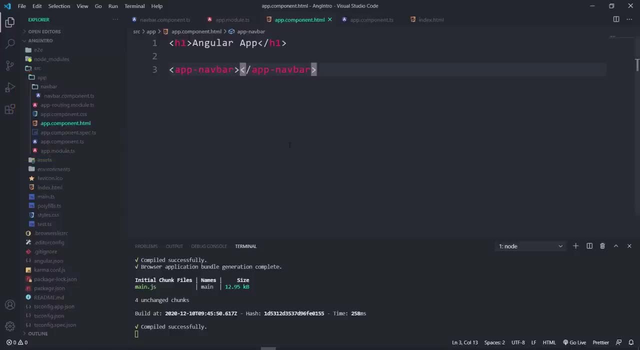 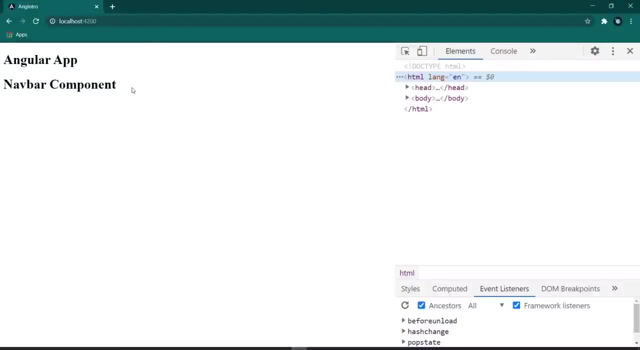 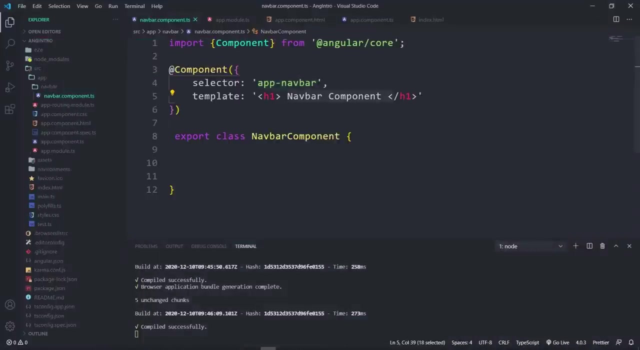 inside this app component. So this is just a standard in angular. Alright, now save this all and back to the browser. Now we can see this navbar works text, which is coming from this navbar component, And also we can see this angular app h1 tag. so this is coming from our main app component. 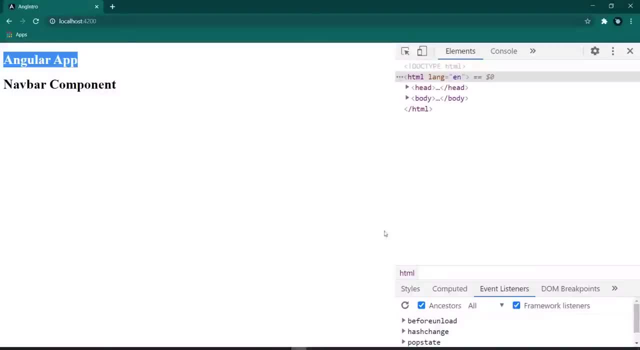 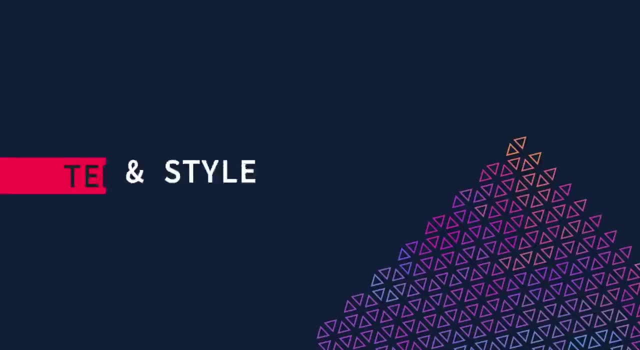 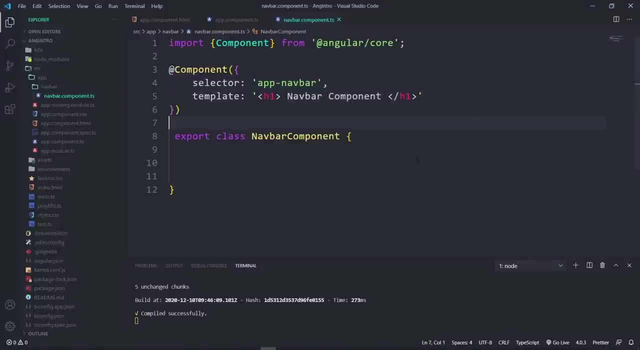 So this is how we work with components in angular. So in previous we added this selector and template property inside this component decorator. You guys now know what is happening with this selector property. If we recap this, we use this selector to identify and render this component inside the browser. 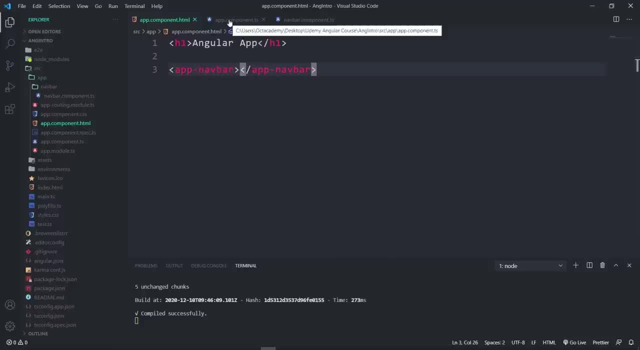 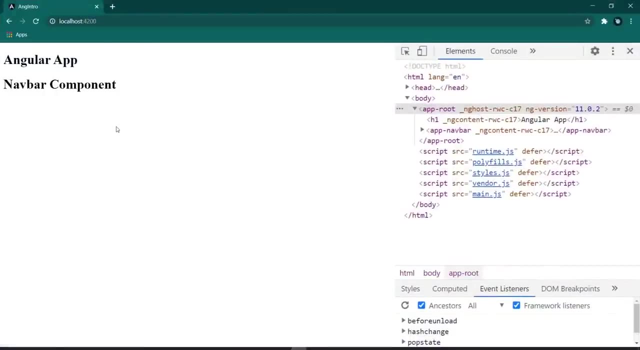 So now let's see what is the use of this template selector. You guys may already noticed this inside this browser. we got this navbar works from. where do we get this? If we look at inside the code on the inspect element, we can see this app navbar tags. 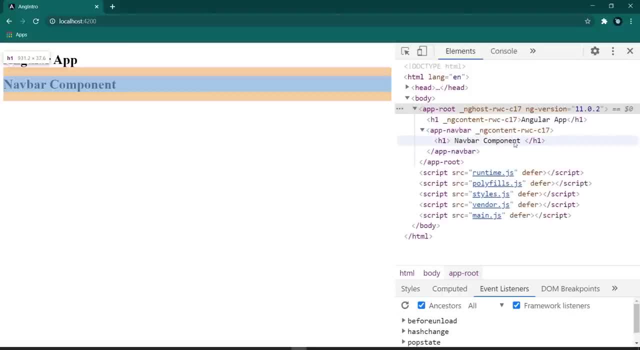 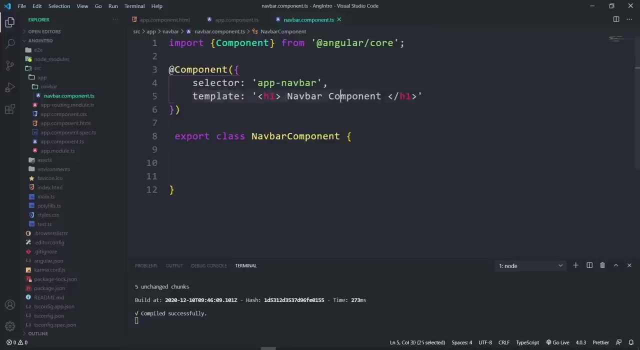 Between this app navbar tags. we have this h1 tag with this navbar works. So what is this app-navbar-tag? So this is the navbar component selector. Inside that we got this template values this h1 tag. So inside this component decorator. 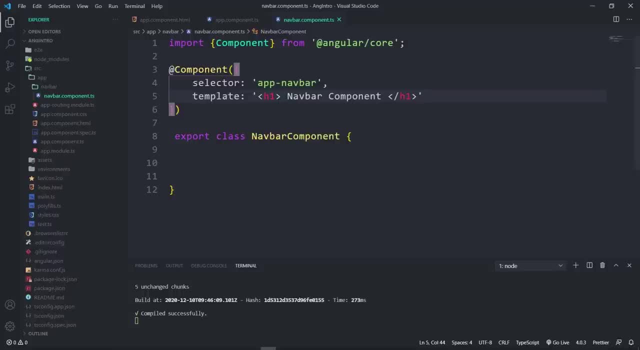 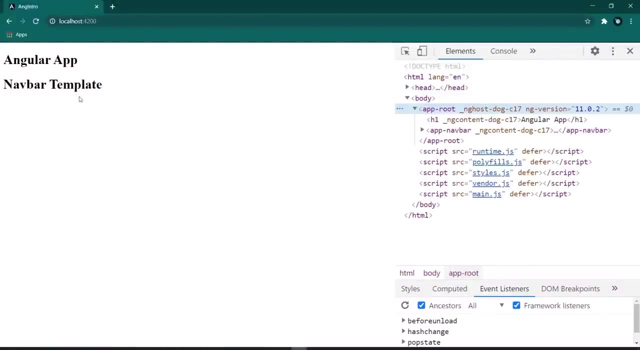 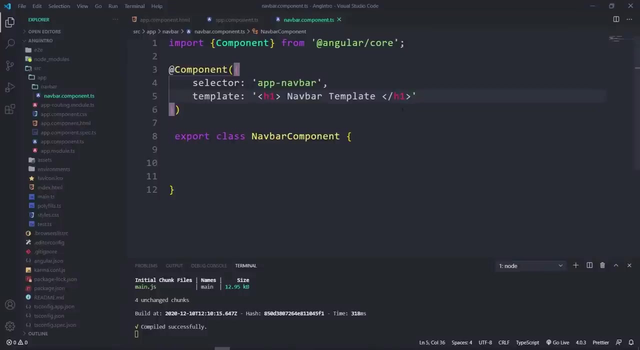 We got this template values this h1 tag. If I change this text to navbar-template, save this. look at this. this value also changed to this navbar-template, As we can see here. now we can understand. this template is loaded inside the browser. 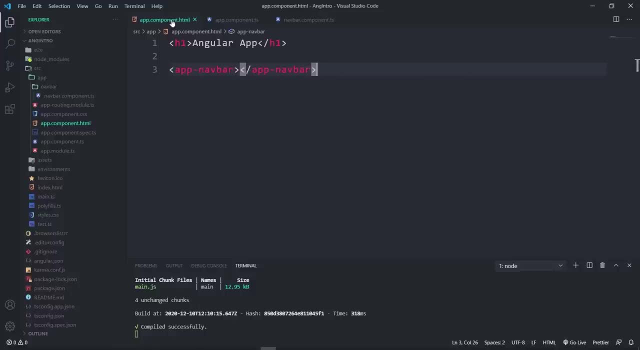 for this navbar component. So what is happening here? when we load this component inside the browser using this app selector, This will display all the content of this template value inside the browser. So we use this template property to load html tags inside the browser. 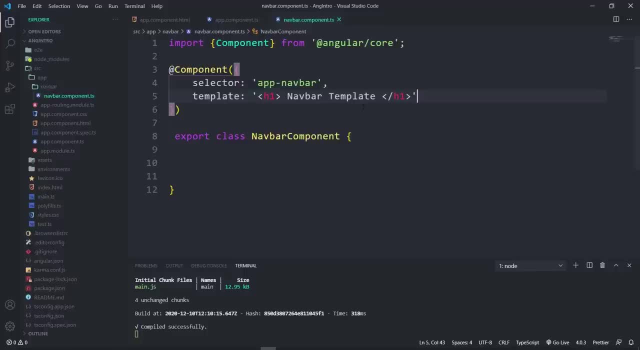 Hope you guys got the idea right. So now we know how to show this component inside the browser using this selector, And also we can show html markups for this component using this template property. Now think If we want to add the CSS structure. 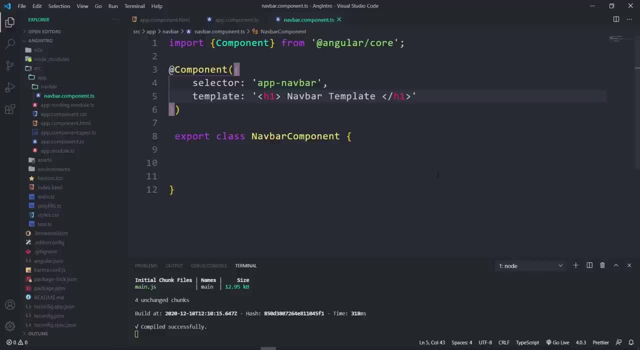 We can add the CSS structure. We can add the CSS structure. We can add the CSS style to this html element inside this component file. How do we going to do that? In order to add CSS for this template, we can use another component: decorator property. 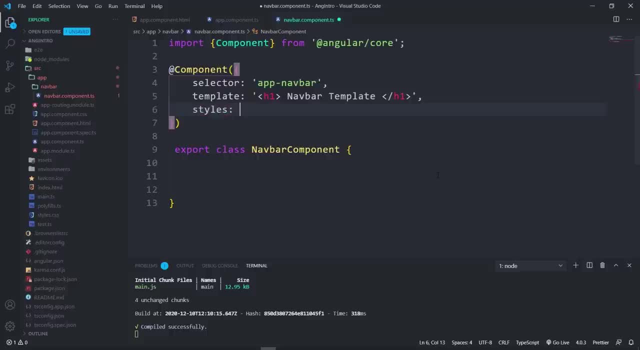 called style. Using this style decorator property, we can add CSS style to this component. Alright, lets see that in action. So lets change the color of this h1 tag. So, in our case, CSS selector is blue, CSS selector is this h1 tag. 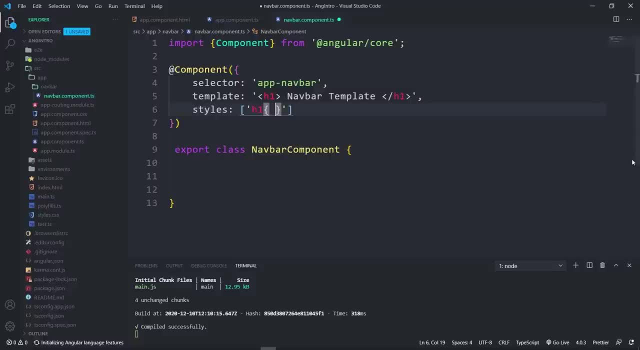 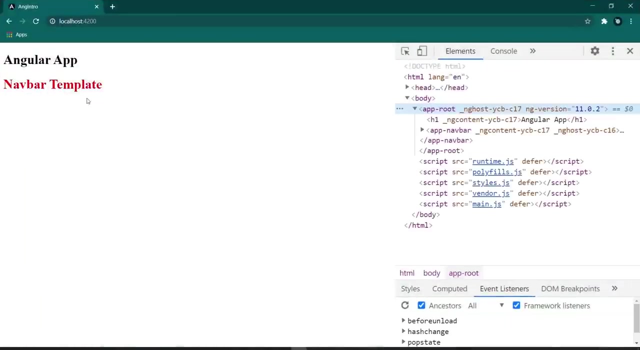 Next, the CSS scope. So inside this we are changing the color of this h1 text. So CSS property is color colon and value is something red. Alright, save this and back to the browser. Perfect, So now, as you can see here, now this h1 text is in red color. 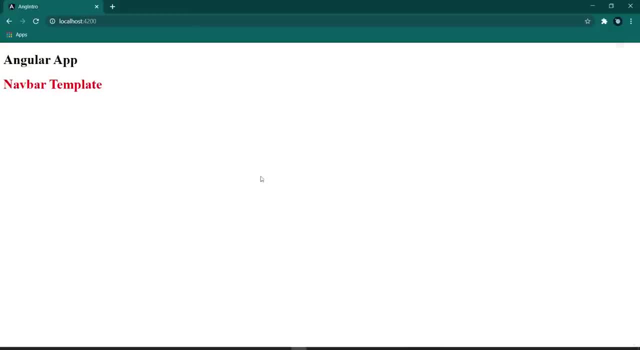 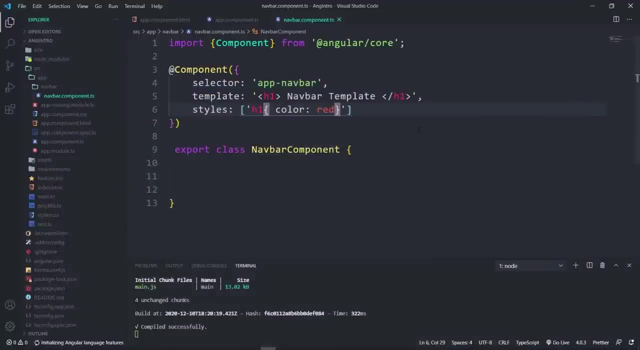 So this is how we add CSS styles to component Alright. some of you may noticed this. usually we write CSS in multiple lines, Not in one line like this right, But in this component ts file. inside these codes we cannot write multiple lines. 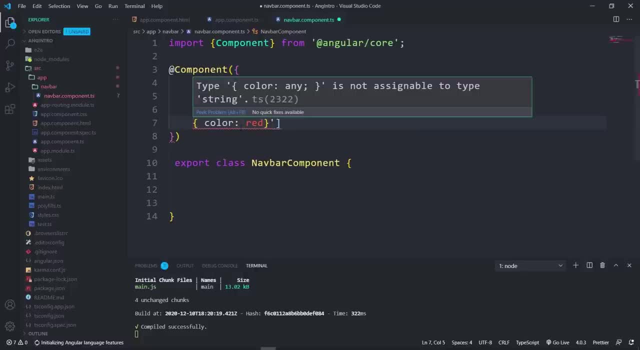 If we add line break here, we get this compile error, So we have to put everything in one line. For something simple CSS style like this, this is ok, But if any case, we want to write some multiple lines of styles for this component. 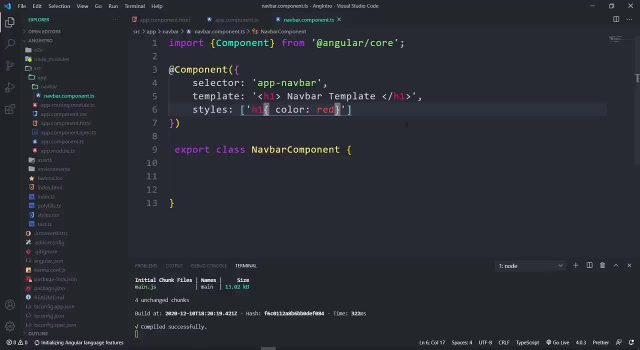 How do we going to do that? So in angular component decorator, we can do that by using the back tick symbol instead of this codes, which is located before the number 1 key in the keyboard. So lets remove this previous style and put the back ticks. 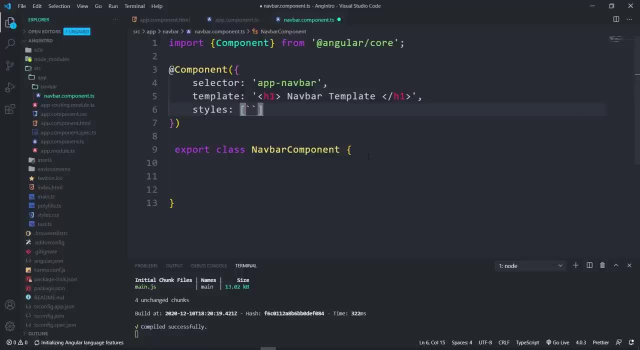 Inside these back ticks we can write multiple lines of styles. So let's write the previous style again, but this time we can write this in multiple lines. CSS selector h1. and this is a scope. Inside this scope, set the color to red. 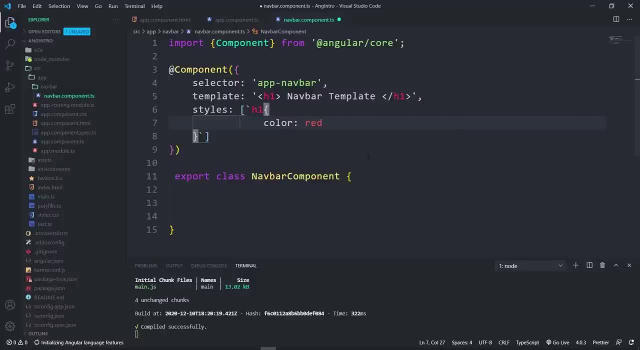 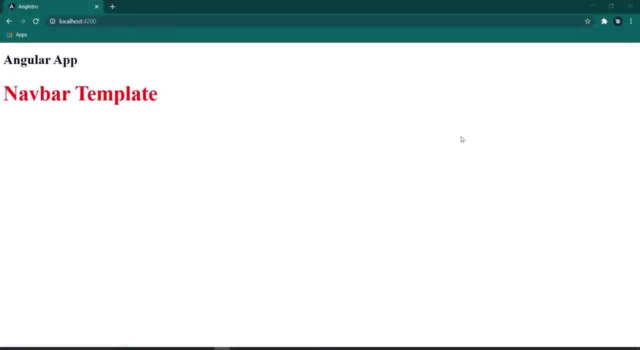 After this, let's add another style inside this. So change the font size to something big: 50 pixels Now. save this and back to the browser. Beautiful, right Now. we have successfully wrote multi lines of CSS inside our component ts file using the back tick symbol. 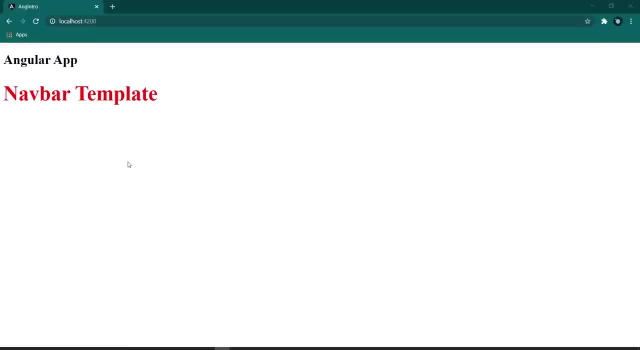 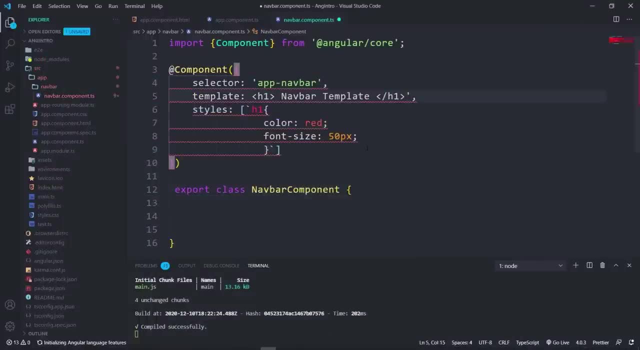 And one more thing, guys. I forget to mention that we can use this back tick method to write multiple lines of HTML markups also. So remove these codes and add back ticks for this template. After this, let's put another paragraph tag and add some dummy text. 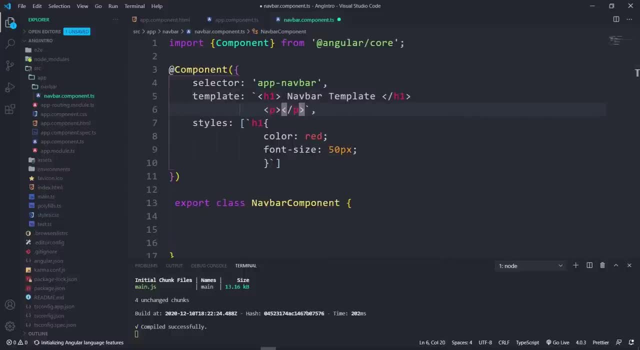 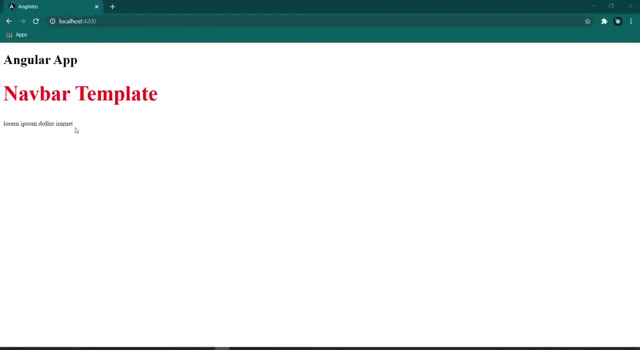 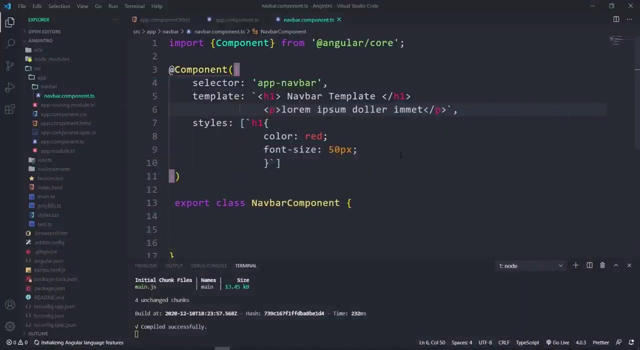 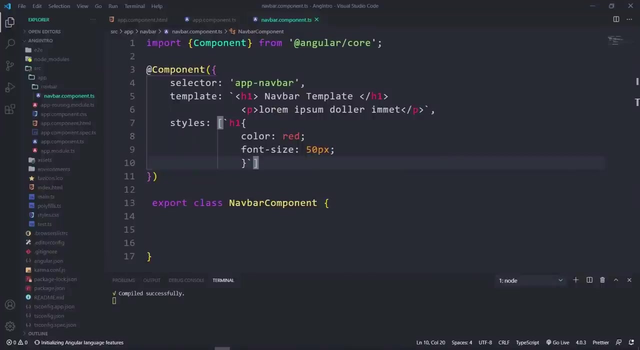 Now we have successfully wrote multi lines of CSS inside our component ts file using the back tick symbol. Save this all and back to the browser. Awesome, right Now we know how to write multiple lines of codes inside this component decorator. So in the previous section we have created this navbar component. 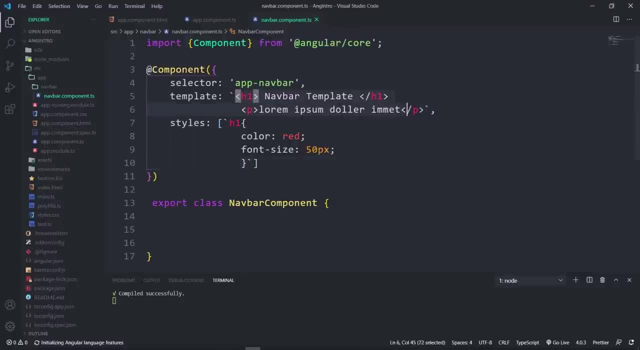 We put the HTML tag And here we have 100 lines of HTML markups and styles inside this same page, using these component decorator properties. So it's okay. But think if we have 100 lines of HTML markups and 200 lines of CSS styles putting them? 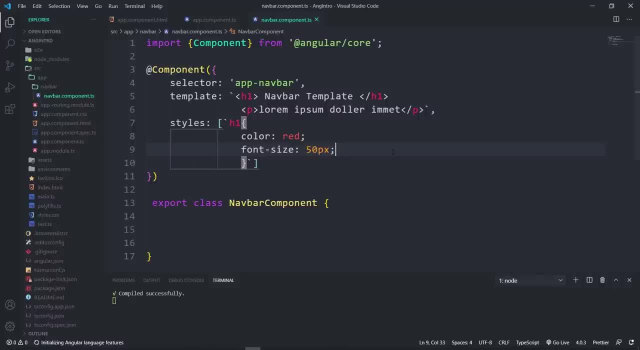 all inside this ts file. it's make our code very noisy and unreadable, So that can cause lots of problems and bugs When it's come to debugging. Oh, can't even imagine, I can't even imagine. Right. As a solution for this, we can create a separate file for the HTML markup and a separate file. 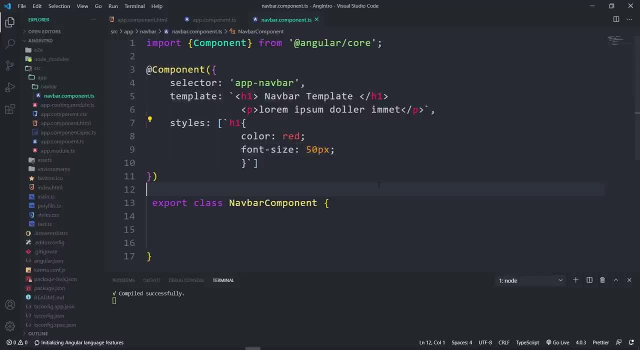 for CSS. How do we do that? First, let's create the files. The first file is for the HTML template. So we are creating these files for the same navbar component. So create this file inside the navbar component folder. So create a new file. 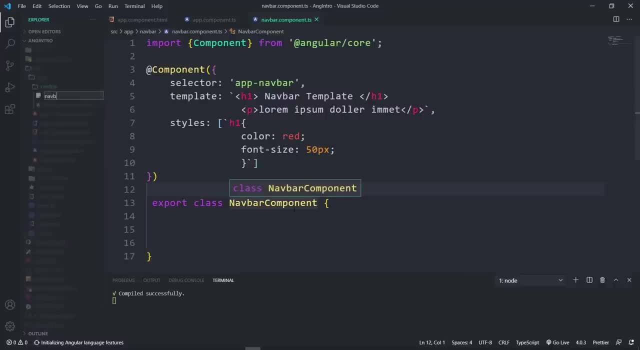 And name this navbarcomponent. This time, this is an HTML file, So the extension is HTML. All right, Next create the CSS file. The file name will be navbarcomponent And extension will be CSS. Please note this carefully. The naming convention is css. 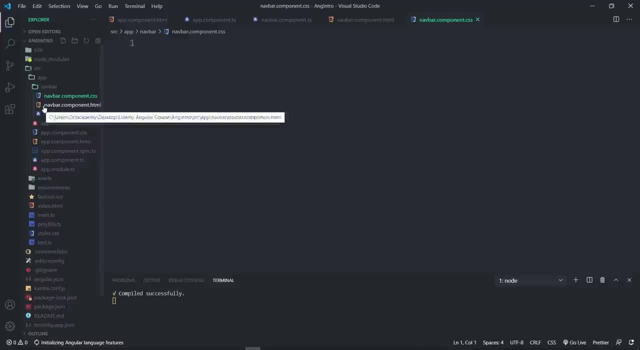 And the extension will be css. The name of the file is the same on these all three files: First, the component name, navbar, and second the component keyword and third, the file extension. So this file extension can be various depending on the file types. And one more thing. 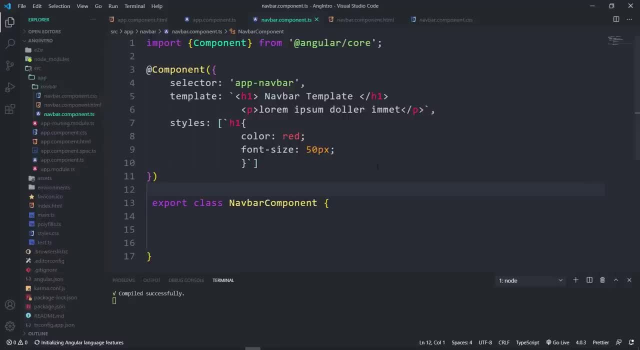 This ts file is the main file for a component, So without that file we cannot create a component in angular. So hope you guys got the idea. All right, we created the component html file and the component css file. Now we have to link these files to the navbar component. 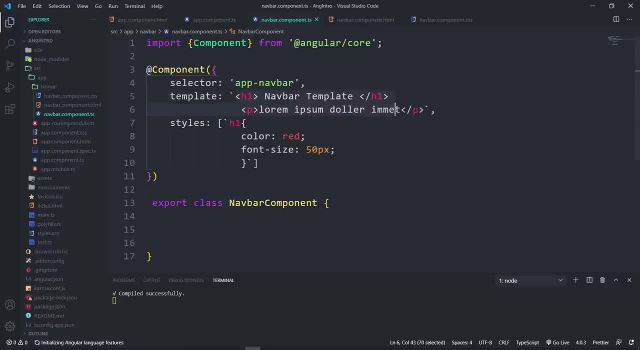 So go to the component ts file. In previous we have added these html markups inside this template. Now we have to link the external component html file instead of these inline markups. For that, first, remove these all markups. Next we have to add the html file. 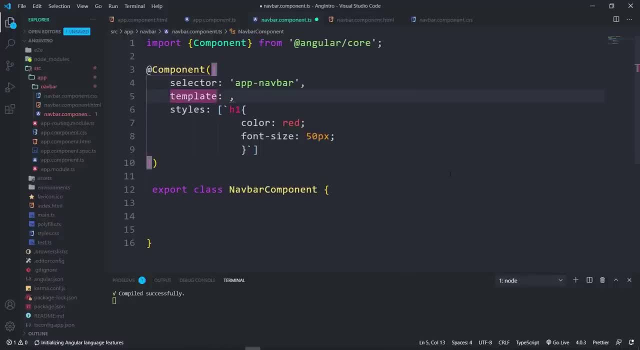 Next we have to do a small change to this template property, So change this template to template url. So this u is capital. So now, this time, this component decorator property is template url. All, right, now pass the component html files path as a path to this template url property. 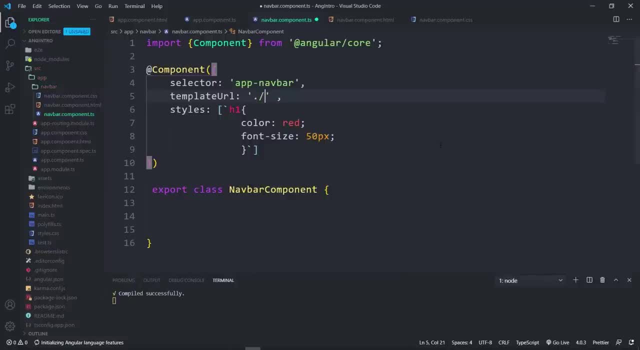 The file is inside the same folder, so dot slash, And the file name is navbarcomponenthtml. That's it, Simple, right? So likewise, now we have to link the css file. So again, remove the existing inline css and change this style property to style url. 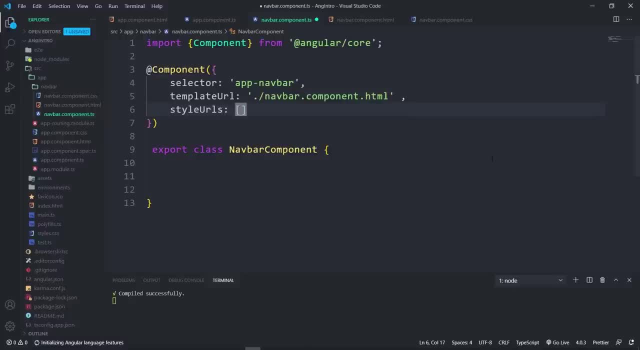 Then give the path of the component css file. Inside quotes: Dot slash- Navbarcomponentcss- Beautiful. We have successfully linked the external files for this navbar component, So save this file and go to the browser. Wait, what's going on here? 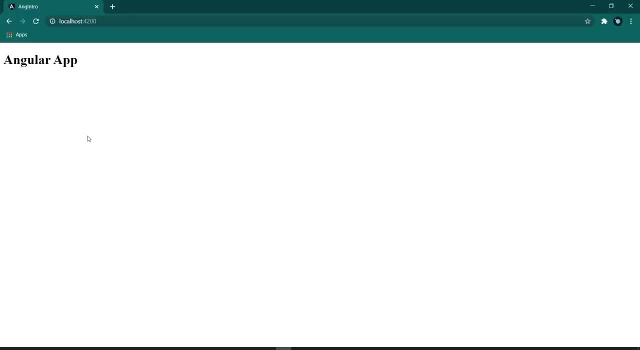 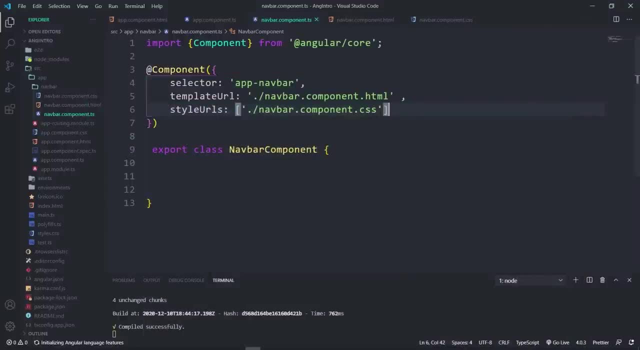 We only see this app component, But we cannot see the navbar component markups. Why is that? Cause, if you can remember, we removed all the inline markups and we linked the external html and css files. So inside the navbar component html file we don't have any markups. 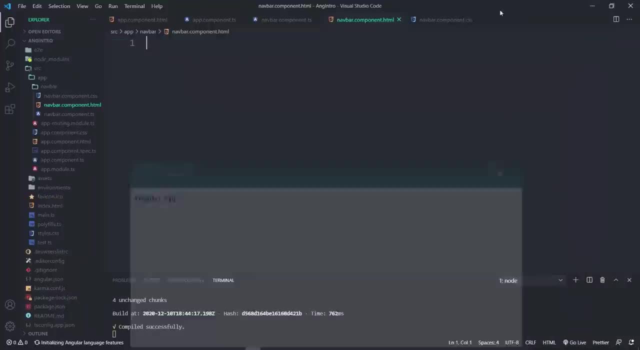 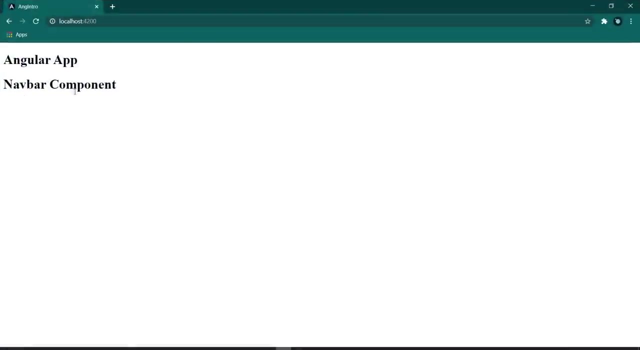 So this file is empty. That's why we are getting nothing inside the browser. So now let's add an h1 tag and put this navbar component inside this navbar component html file. After this, save this file and back to the browser. Perfect, right. 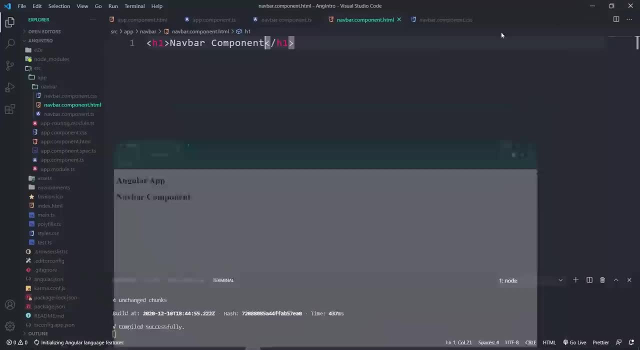 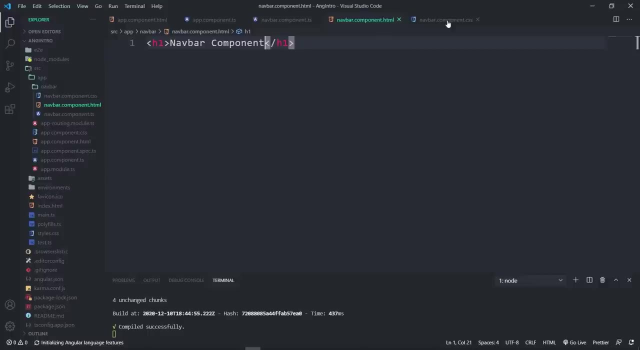 Now we got this h1 navbar component which is marked in html. Alright, let's add some style to this h1 tag. So inside this navbar component css file, write the style for this h1 tag, h1, and in this scope the color will be red. 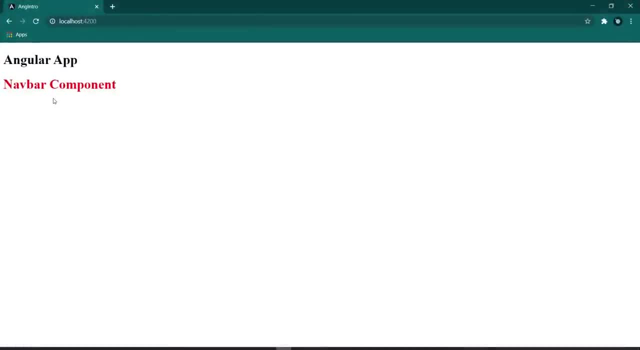 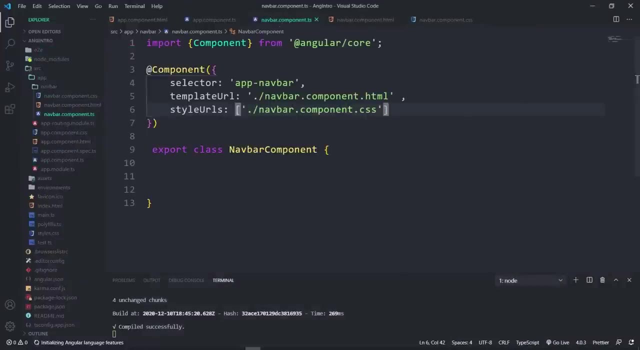 Save this and again back to the browser. As you can see here, external css style is applied to this h1 tag. That's why this h1 text turned into red. Ok, Now we have separate files for html markups and for the css. 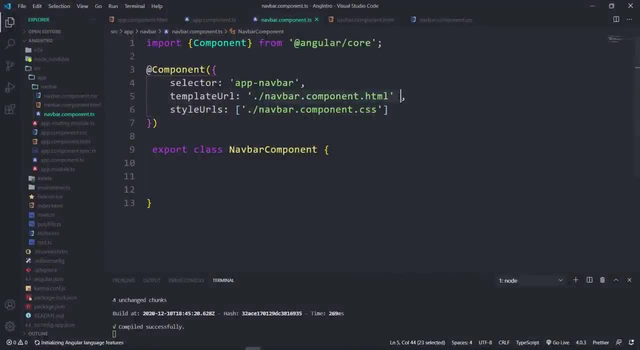 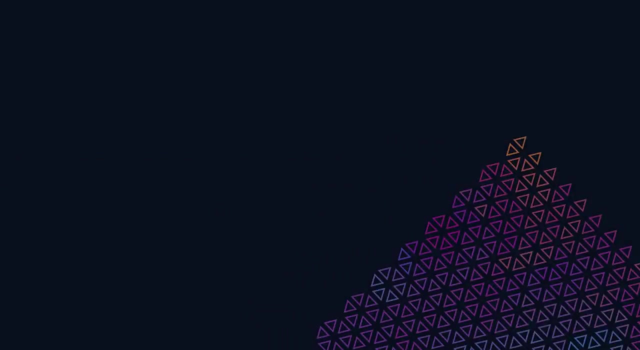 So we write all the markups inside the html file, We add all the css styles inside this css file and we add all the logics inside this tgs file. So now we can work on this navbar component more efficiently. So in the previous section we have created this navbar component from scratch. 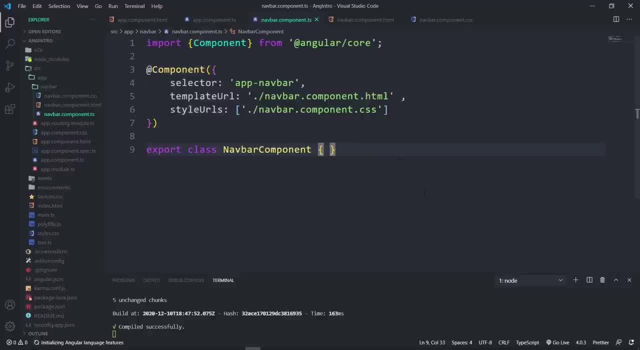 Record all of these from the beginning. Some of you may get these creating components very hard. some of you may not, But don't worry, we have an easy way for this. We can create angular components using the angular cli with a simple line of command. 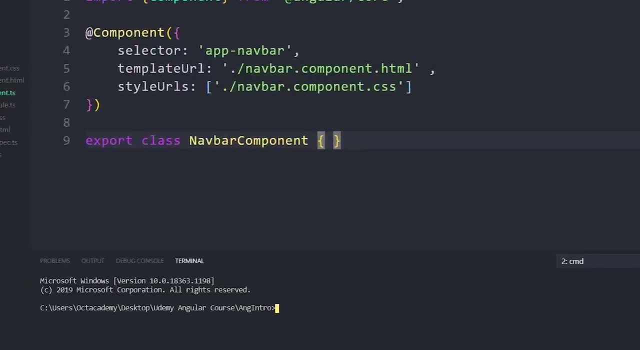 So inside the integrated terminal, just run this command. So ng. this command is coming from the angular cli. So g- this g stands for generate. Next, c- this c stands for component, because we are creating a component here And at last we have to give the component name. 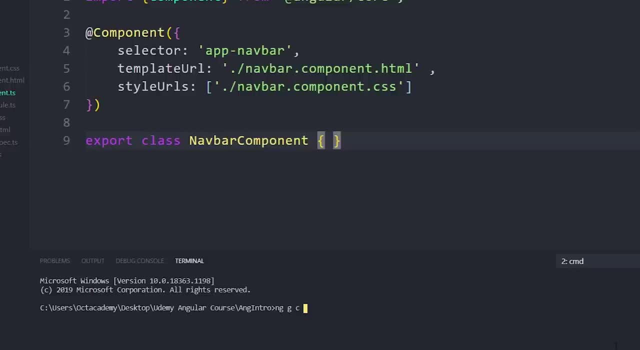 So we already created the navbar component, So now let's create this post component. So the component name will be post. That's it. To run this command, just hit the enter. Alright, post component is generated successfully. If we look at the file structure, we can find this post folder inside this app folder. 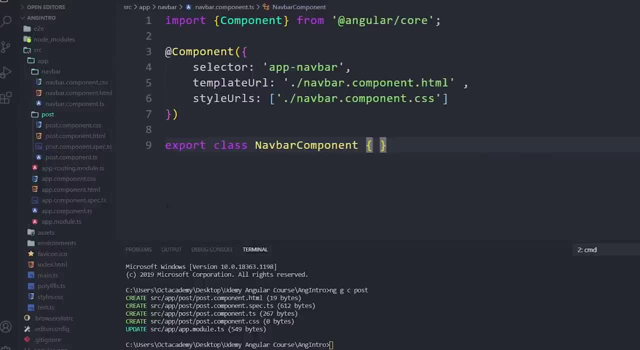 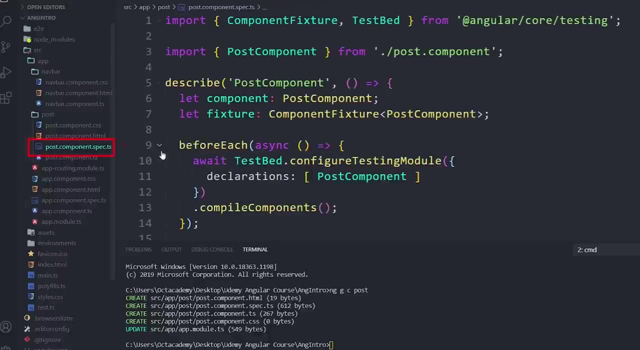 So inside this post folder we can see these files: Post component: ts file, html file and css file. So we learned about these all files And created these files in previous section. Now, if you look at this further, In addition to these files we got this another new file. 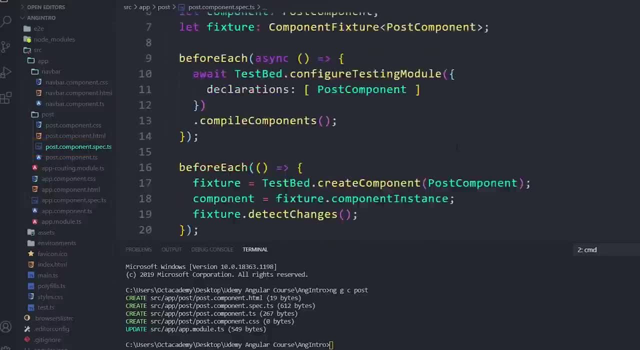 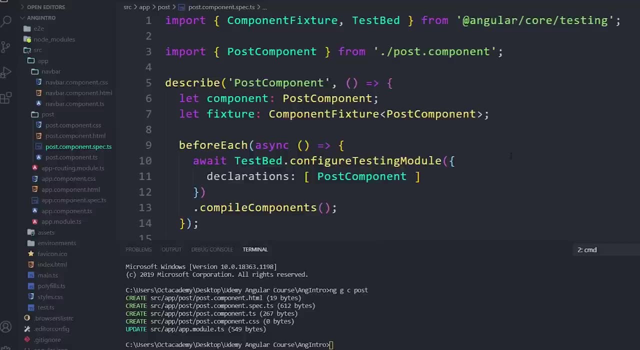 This post: componentspects file. What is this file? This file is responsible for unit testing in angular, Which is a beyond the scope of this course, So don't think too much about this file. So we are not going to deal with this file. 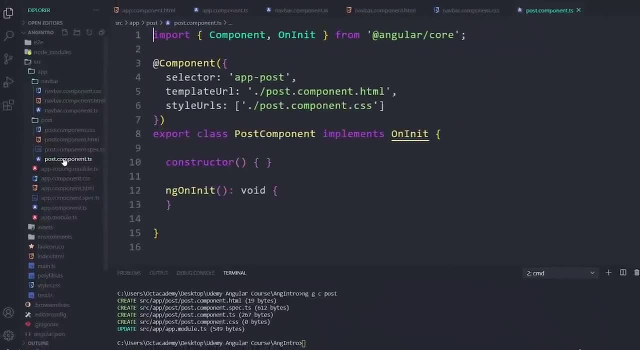 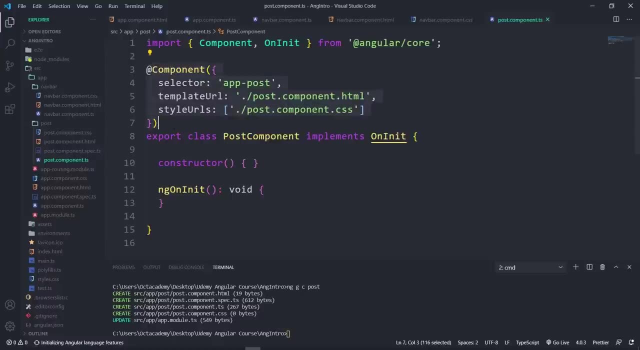 Alright, First let's look at this ts file. So inside this we can see this import component And this component decorator. So inside this component decorator We can see this property selector. Now this is app-post, So this selector will be used to identify this post component. 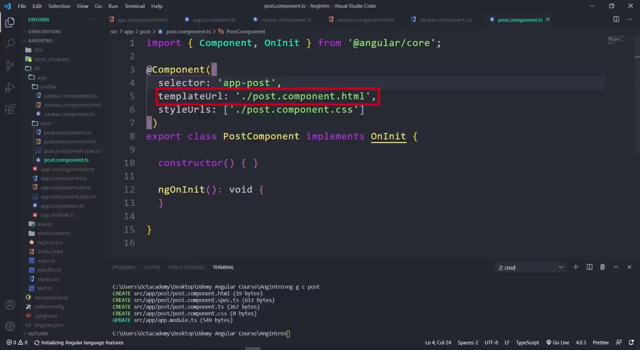 Alright. next, we can see this template url for the component html file And we can see this style url and the path for the post css file. So if you look at this carefully, we can notice some few additional things on this page. Just leave these for now. we will come to this in a moment. 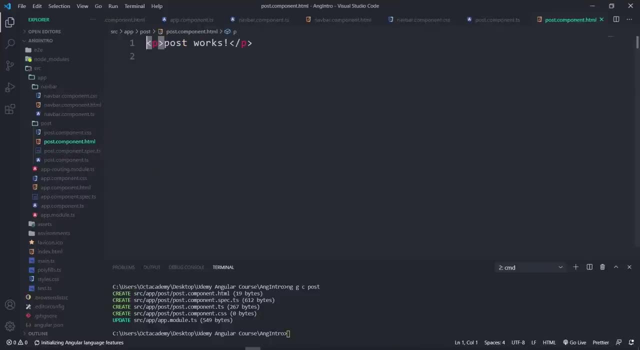 Now let's look at inside the post component html file. inside this we can find this simple default markup p tag saying that post works. So inside the css file we got nothing. it's just a simple empty css file. Now go to the appmodulests file. 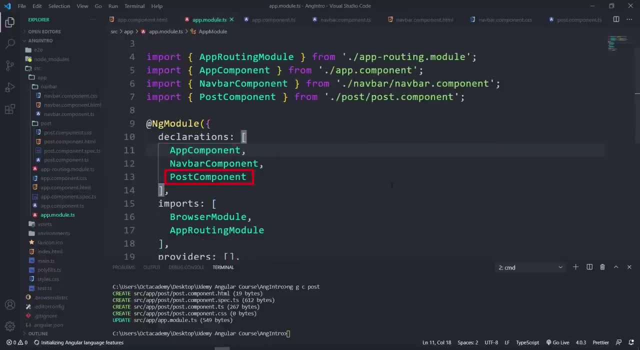 Inside this declaration we can see this post: component register. This is the beauty of angular cli. If we create an component manually, we have to do this all step, one by one, from scratch. If we missed one of these steps, our app will break, And also 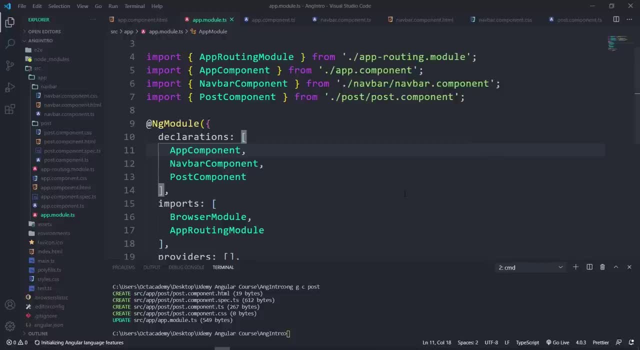 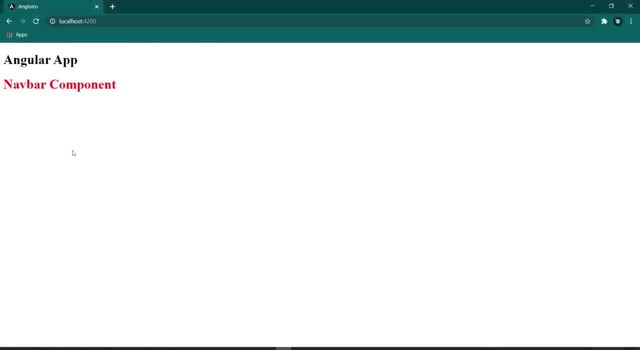 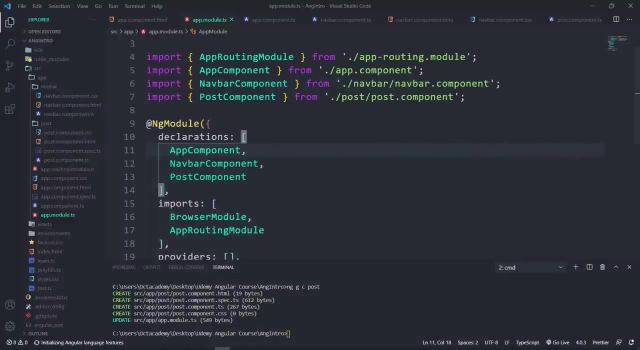 component using angular CLI. can you imagine how much of time this saving for us? Awesome, right, Alright, now go to the browser. Still, we cannot see the post component here. Why is that? Coz we just only created the component. That is not enough in order to show the component. 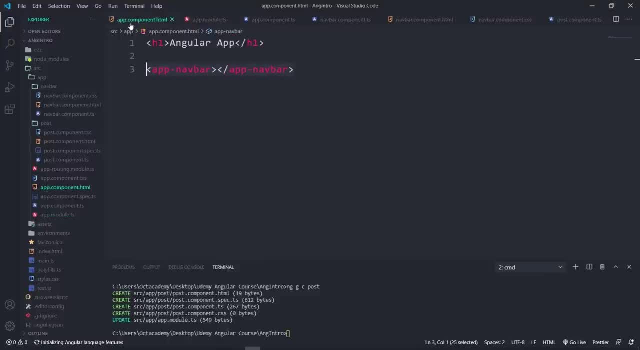 inside the browser. We have to put the component selector inside this app component. So, if you can remember, we use the app component selector as an html custom tag. Go to the app component html file So the selector is app-post, and hit enter So the vs code intellisense. 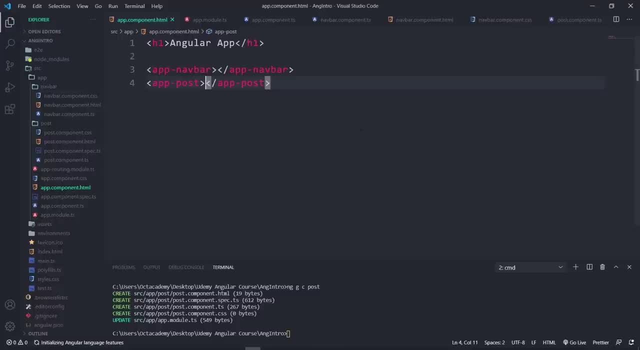 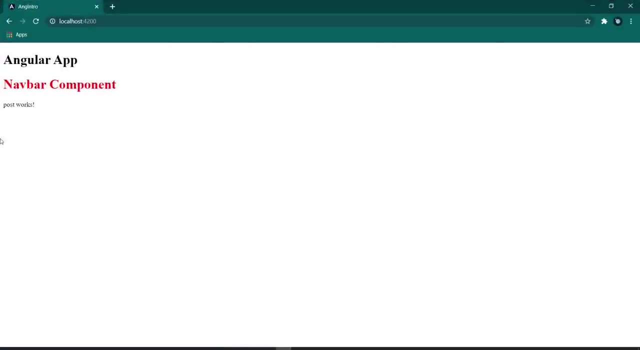 will complete this as an html custom tag. So now save this and back to the browser. Perfect, Now we can see this post works, Which means post component is now rendered inside the browser. So open this inspect element and if we look further inside the 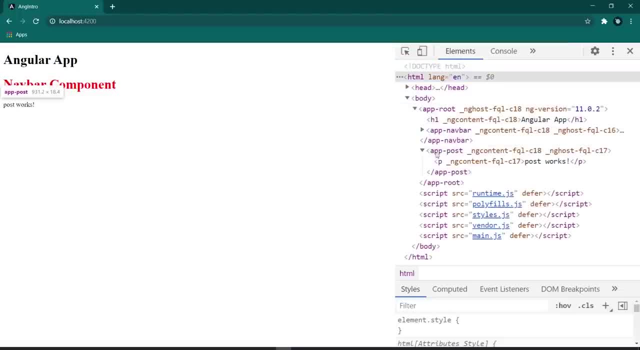 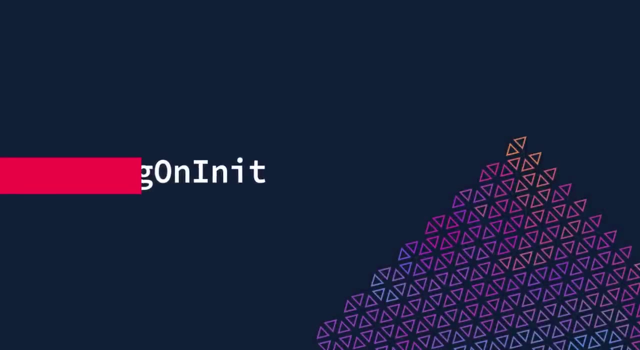 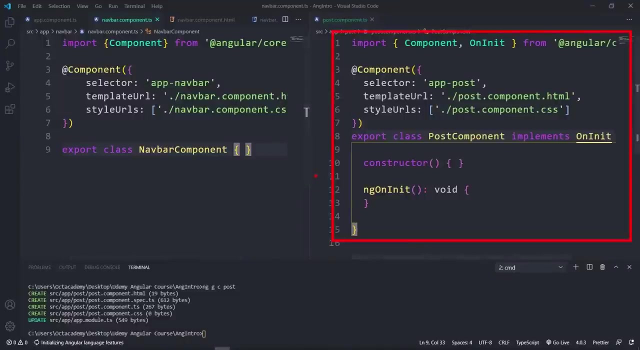 elements, we can find this app-post tag. So this is how we can generate angular components using the angular CLI. If we compare this angular CLI generated post component TS file with our navbar component TS file, which is created from scratch, We can notice a few different things. The first one is this: import In the navbar component, we only imported 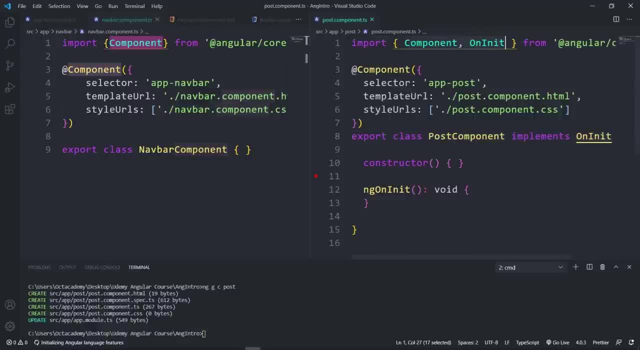 the component module. But in post component which is generated from the angular CLI, has this onInit module import. So you guys may wonder what is this and what is happening with this? So actually this is an interface and also we called this onInit interface. 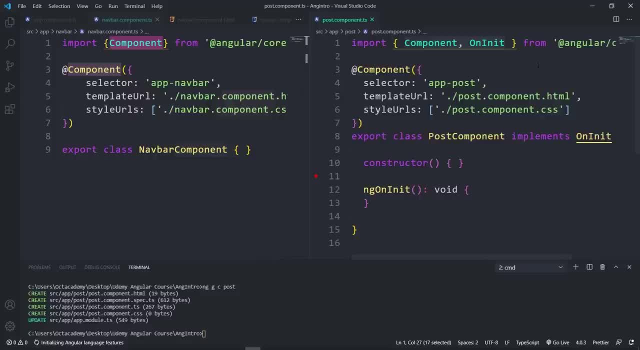 as a lifecycle hook. With this onInit interface, we got this ngOnInit method. So what is this ngOnInit? ngOnInit is a callback lifecycle method which is invoked after this particular component fully initialized inside the DOM. This is different than the constructor, If you can remember. 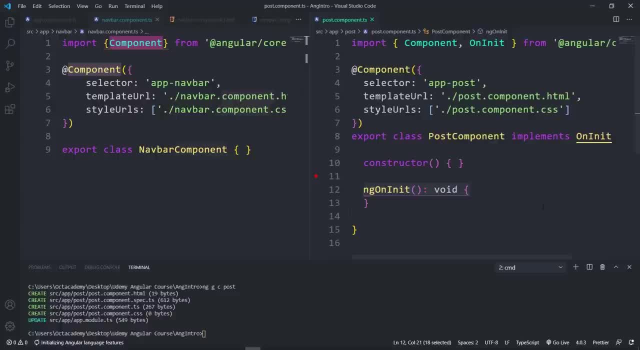 constructor will work soon after the object class created. We learned about this in the typescript fundamentals section, But this ngOnInit will execute soon after this post component fully initialized in the DOM, Or in other words fully loaded inside the browser. So this constructor and this onInit lifecycle hook are two different methods To work with. 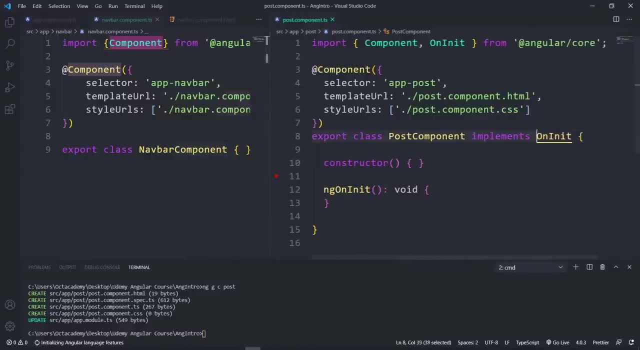 this ngOnInit. we have to implement onInit function to this class. That's what happens with this line of code. We will work on this ngOnInit method throughout this course, So don't worry if you don't get it At the end of the course, you guys will get used to it. 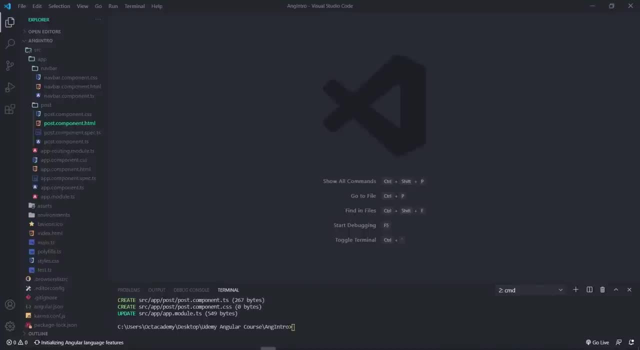 Alright. In the previous lectures we learned how to create a component in a hard way and the easiest way. The easiest way is creating a component using the Angular CLI, So we will use the Angular CLI method to generate component throughout this course. So an Angular component. 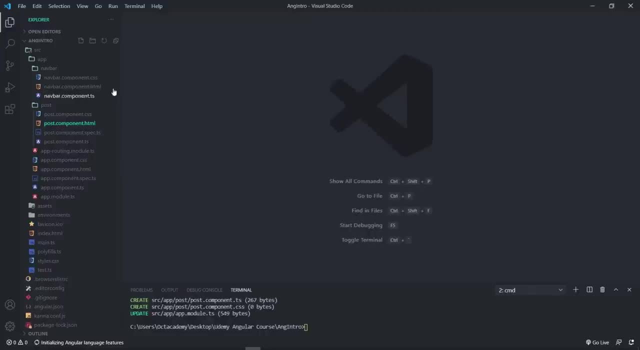 has mainly these three files: CSS file, HTML file and this typescript file. So this HTML file is the component. HTML and CSS files are carrying the HTML and CSS markup and this typescript file carries the logical part. So inside this post component we have this h1 tag. Inside this we have this static. 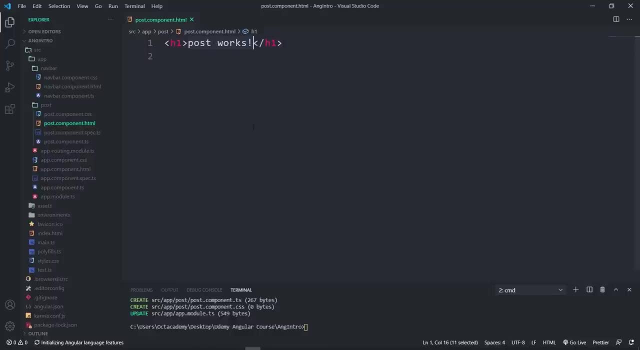 text. Let's make this static h1 tag to dynamic. As I mentioned earlier, we put all our component logics inside this typescript file, So open the post component file and create a variable Title, and the variable type is string. Let's assign list of post to this. 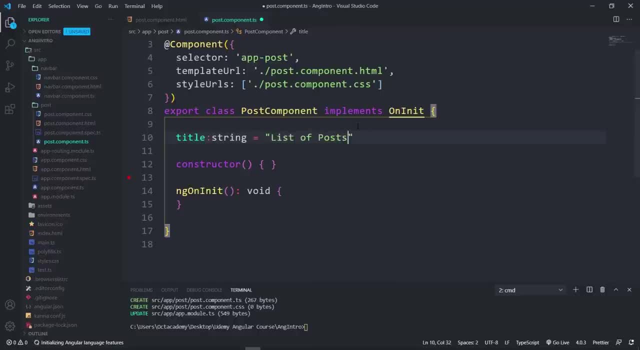 variable. Now what I want to do is I want to show this title variable inside the HTML file. We cannot directly put this typescript variable inside HTML file. For this, first we have to create a JavaScript scope inside the HTML file. So this is a simple thing, right, Usually, if you. 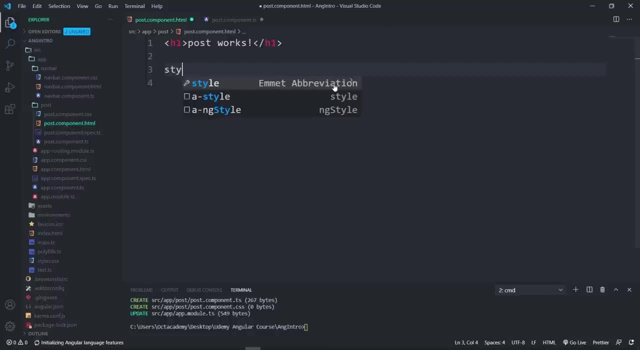 want to write a CSS code inside the HTML file. First we create the CSS scope using the style HTML tag. You guys already know that, right? So between the style tags you can write CSS, Because this is now a CSS scope, not an HTML scope. Inside this style tag we cannot write HTML. 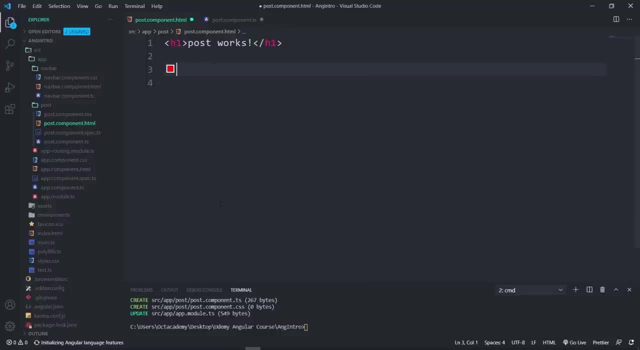 So think, if you want to write some JavaScript codes in an HTML document, We put JavaScript codes between script tags. Okay, So like this: now we are going to show this typescript variable inside the HTML. So first we have to create the typescript scope inside this HTML file. 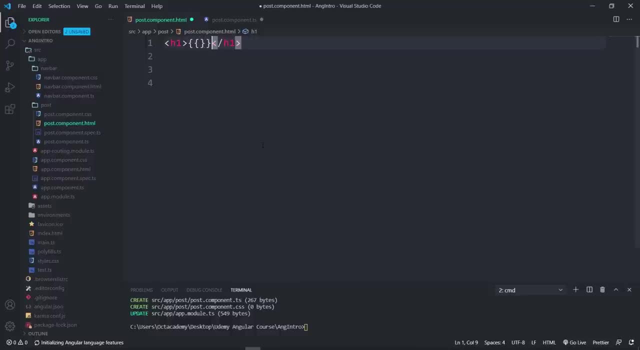 For that in angular we have a special type of syntax, which is two curly braces, So this will create a typescript scope inside this HTML file. Next, between these, pass the variable name title. Now save this and back to the browser. Beautiful right. 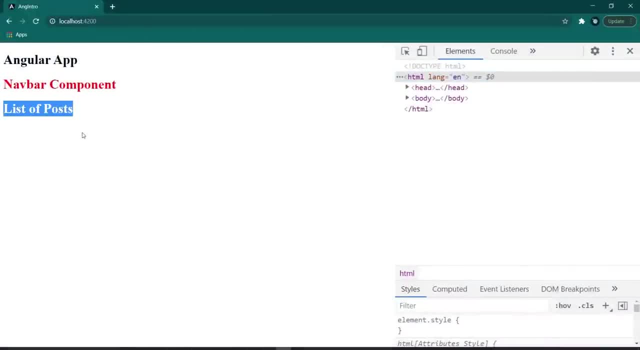 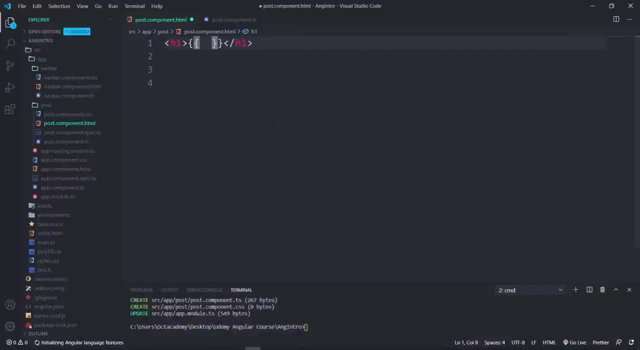 Now this title has changed to this title variable value. So this is what we call data binding in angular. So inside these curly braces we can write any valid JavaScript code. For example, let's add two numbers, Remove this variable title And let's put 100 plus 50.. 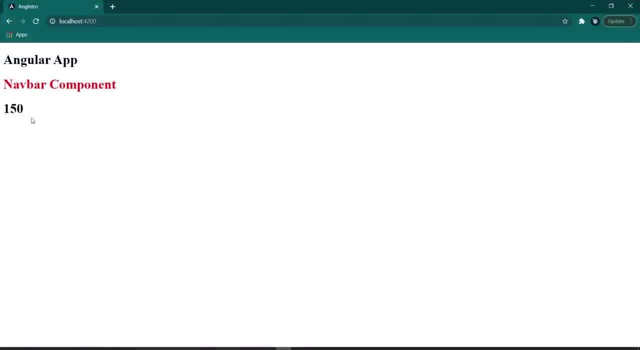 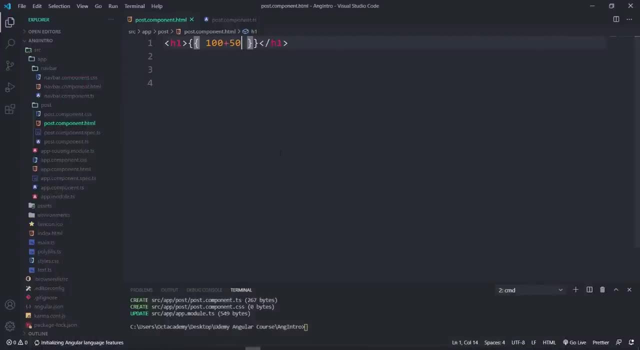 Save this and back to the browser. Awesome, right, We got the sum 150 here. And one more thing: For this process we call data binding And also we call this special type of syntax string interpolation in angular. In the previous lecture we learned how to bind data in components. We created this variable and 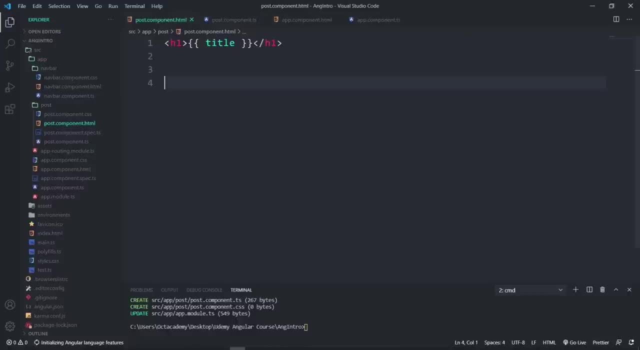 we bind that variable to the HTML file to show this inside the browser. Think, if we have to show this variable inside another component, How we gonna do that. This variable is only accessible inside this component. We cannot access this title variable from another component. 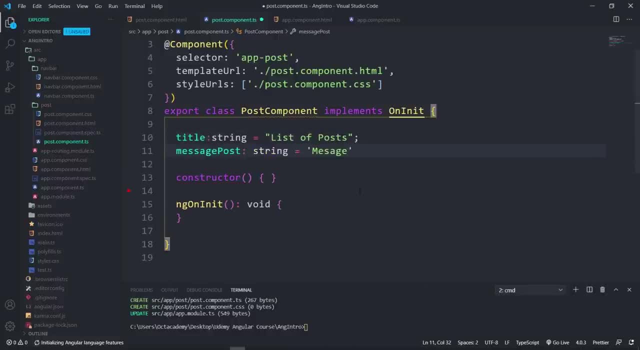 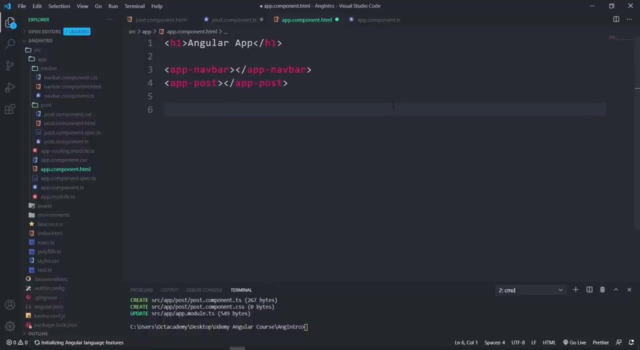 For example, let's see: we have this message- post variable- inside this post component. For some reason, I want to access this variable inside the app component, So in that case we can't show this variable inside the app component using this string interpolation Cause this variable is. 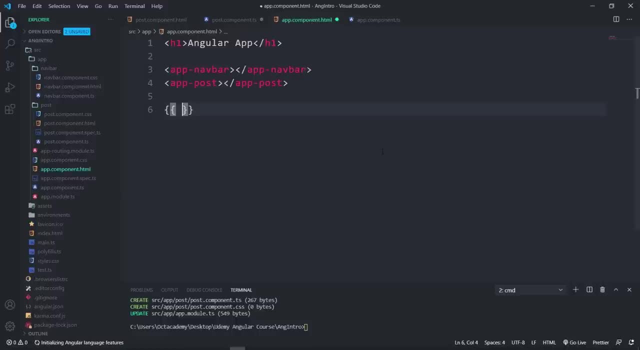 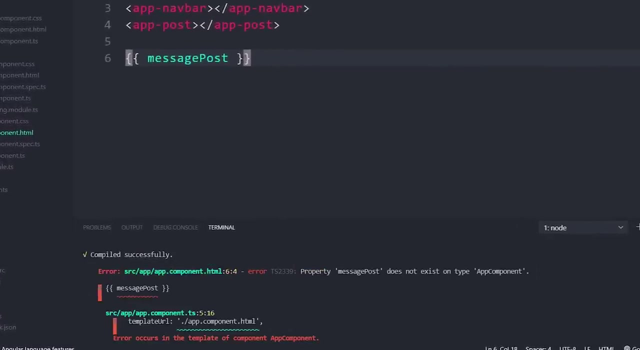 inside this post: component. Wait, I show you this in action. Inside the app component HTML file. let's bind this variable using this string: interpolation: Double curly braces between this variable name is this message post: Save this Now. look at this. We are getting a runtime error that saying property message dost s not. 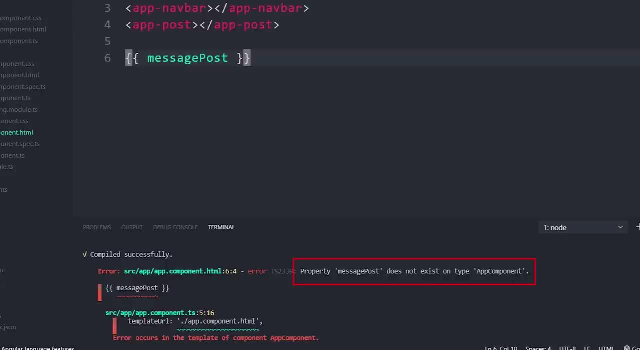 excist on Copy Life AppContent inside this terminal And also we can find this Error and line number. This is one of the of Angular. This will give the error and also this will give us the line number of that error. So this will make debugging like easier. Ok, back to the error. This error is telling: 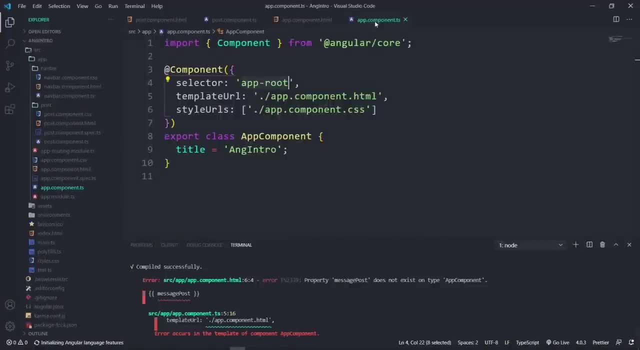 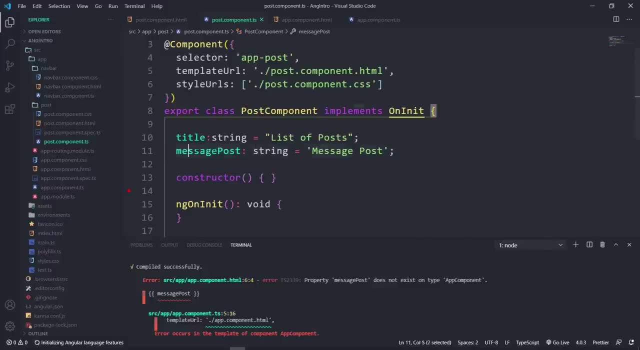 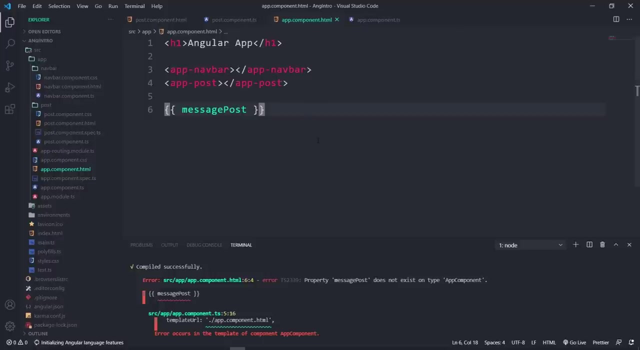 us. we cannot find this messagePost variable inside the app component. So this is what I was tried to tell you guys: We cannot access this messagePost variable from outside of this component. So for this we have a solution. Actually, not a solution, We have solutions. 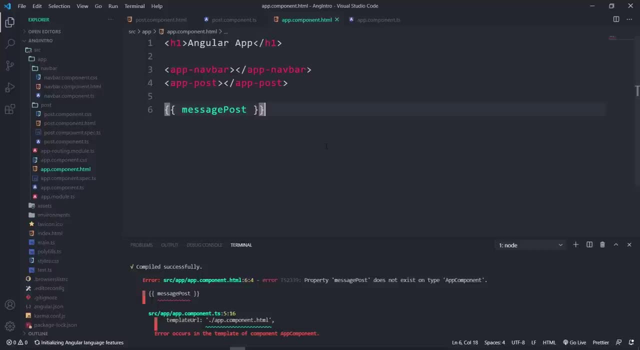 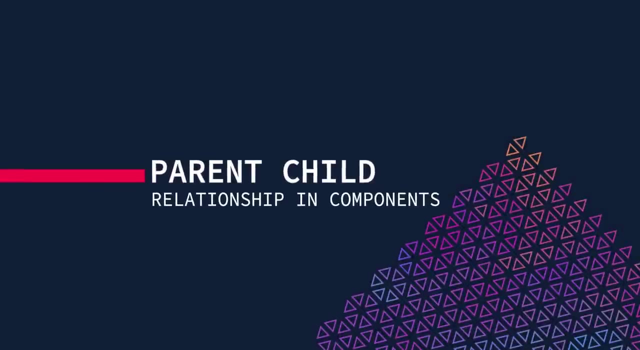 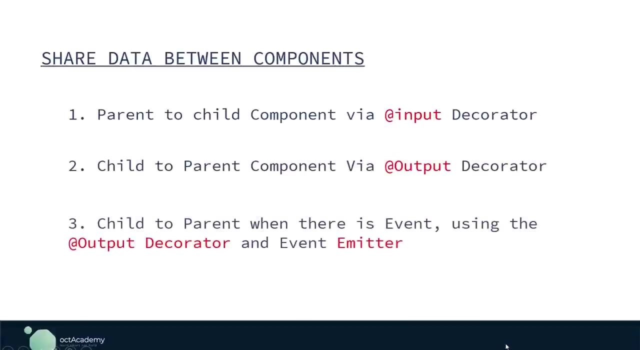 for this for different situations, Not only one. So we will continue this in the next video. So we have three methods to share data between components for three different situations. Let's look at one by one. The first method is sharing data using input decorator In angular. we have this special 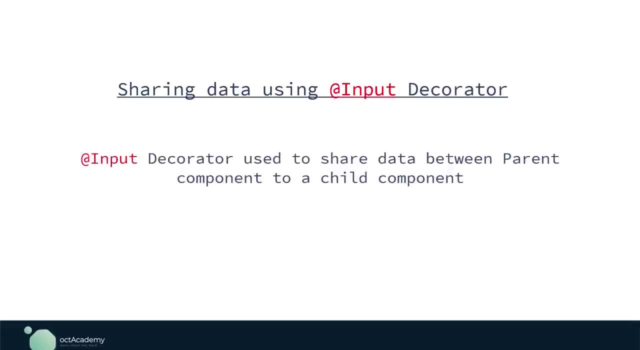 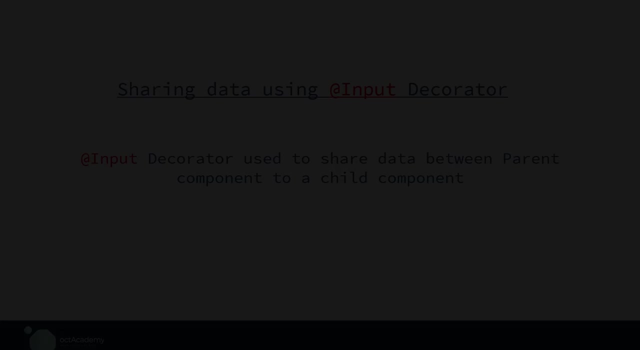 type of decorator input which is used to share data between parent component to a child component. Wait, what is this parent and child component and how do we identify a parent- child relationship in angular components? We have these two components in our angular app navbar and the post component. 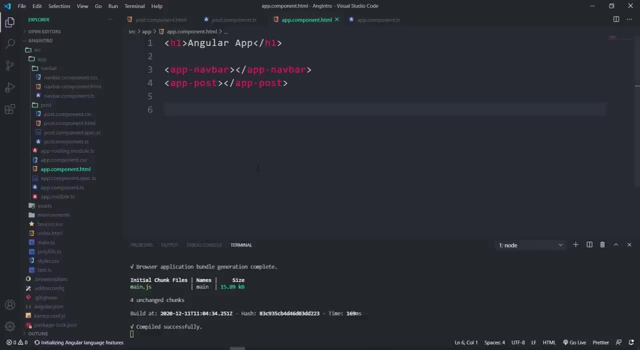 And we have our main app component. Inside the app component, we have linked the navbar and the post component using the components selectors. Because of this component, linking this main app component becomes the parent component And these two components become children components of this app parent component. Let me show you another example, As you should. 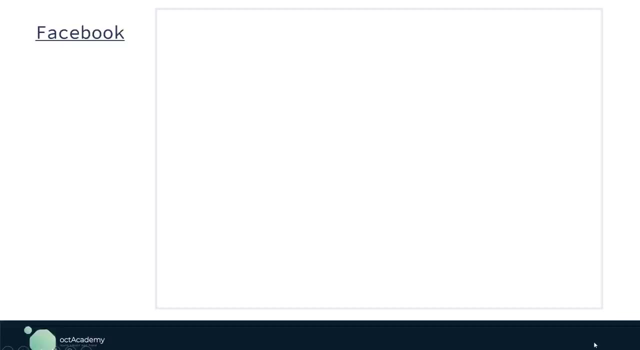 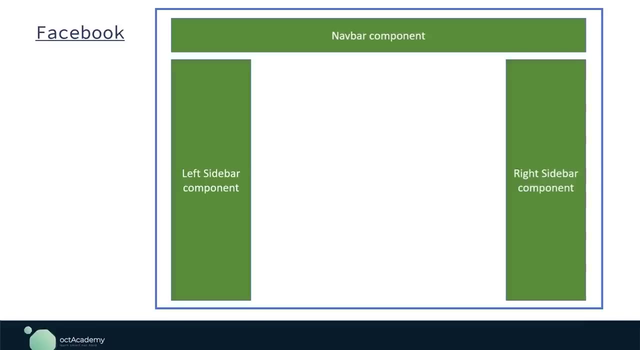 we will take the facebook. Inside the facebook app we have these components: Navbar, left side bar, right side bar and the post component, And all of these components inside one root component, which is this app component. So all of these components are children components. 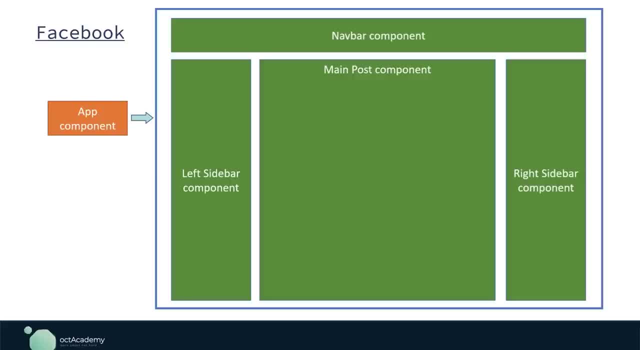 of this parent app component And also we have this single post component, which is inside this post component, not inside this app component. So in this scenario, this single component becomes the child component of this post component. Once again, now the single post component becomes the child component of this post. 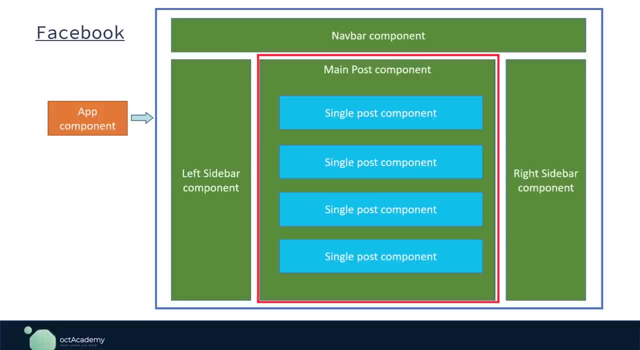 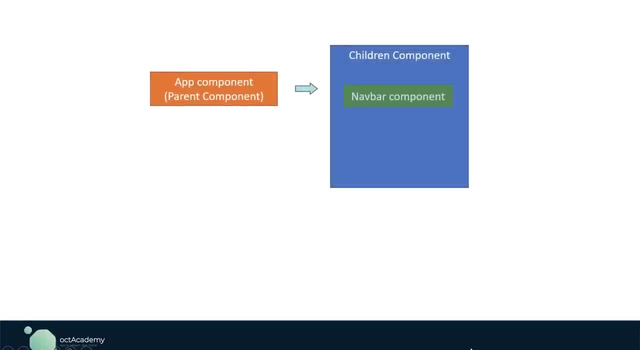 component, not to the app component. Okay, so in that case this post component becomes the parent component for this single post component. If you look at this in brief, the main app component has three children components, The snackbar sidebar and this post components. So if you look at further this post, 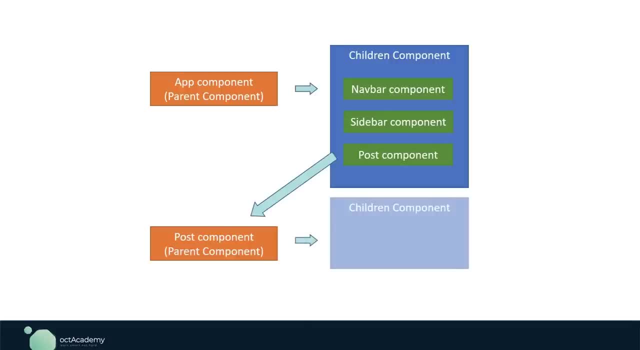 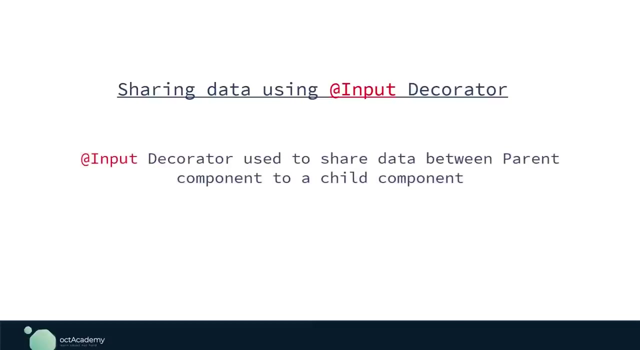 component is the parent for the single post component. So this is how we defined parent-child components in angular. Hope you guys got the idea Alright. so we learned we can pass data between parent component to child component using the input decorator. If we look at our previous example, we can share data from the app component to these. 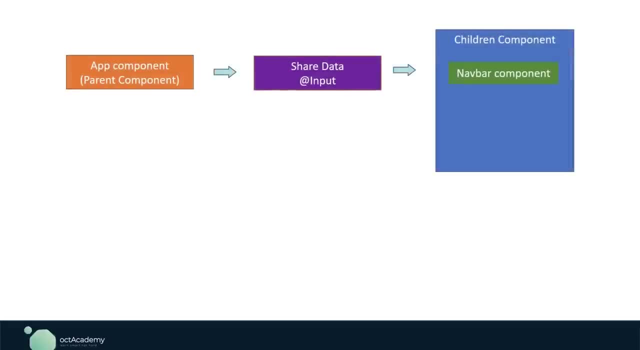 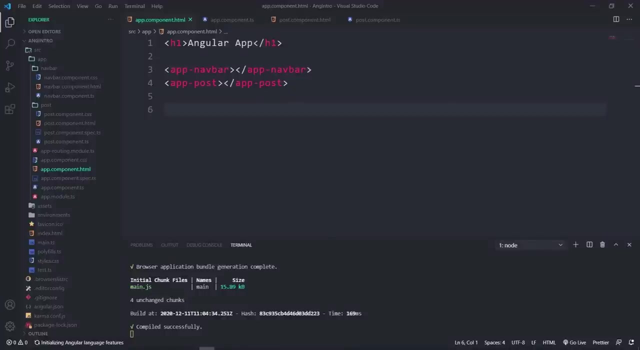 children components using the input decorator as well, as we can pass data from the post parent component to the single post child component using the input decorator. So in the next video we will see this in action. Alright, guys, in this video we will look at how to pass data from parent component to. 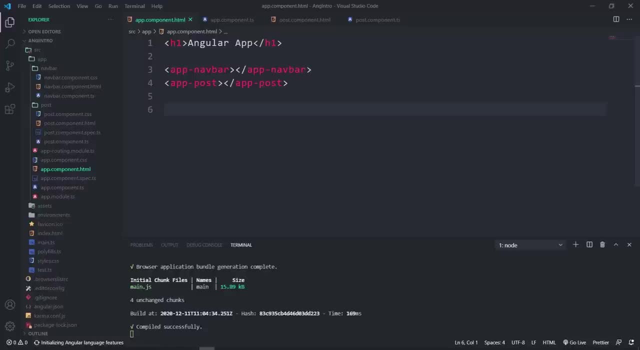 child component. So let's create a variable inside the app component, which is the parent component. Inside the app component is file. create a variable called parent message and this variable type will be a string. Now assign this inside quotes: message coming from the parent component. 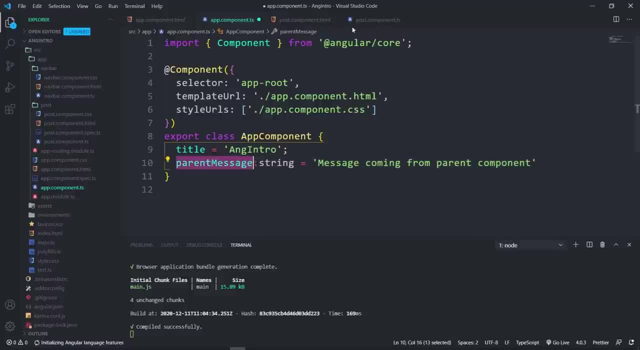 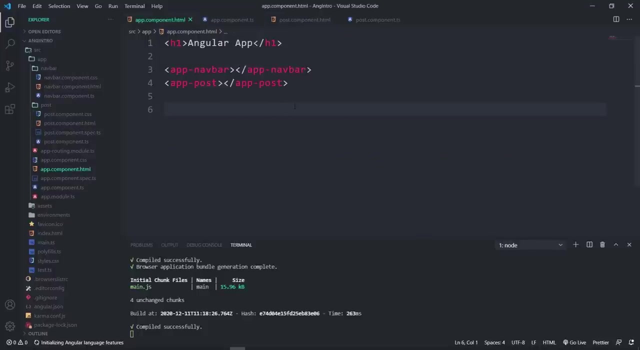 Now I want to access this variable from this post component, which is a child component of this app component. For that first we have to share this variable to this post component. So inside the app component html file we have this element for the post component. 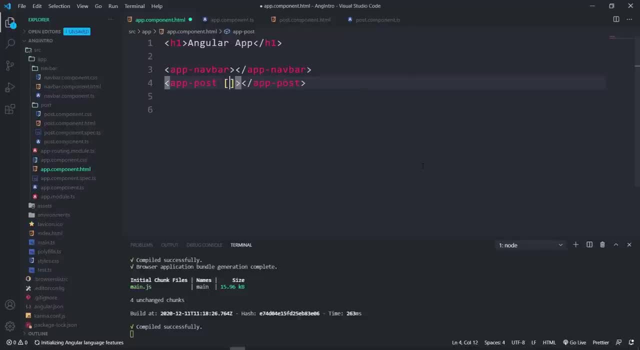 So inside this element: open and close square brackets. Inside this: give a name Something from parent equal sign. This name can be any name After this: inside quotes: give the variable name that we want to share with the post component. The variable name is parent message. 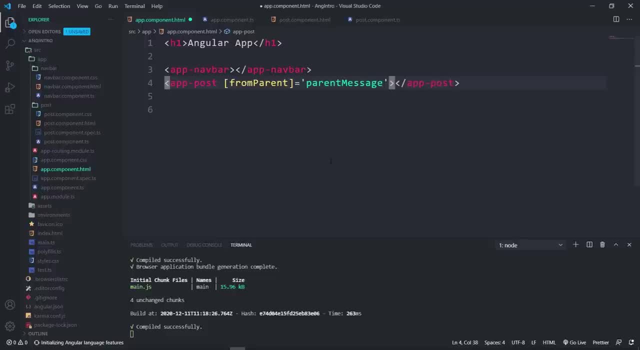 Ok, now, with this, we are sharing this parent message variable to the post child component. Now what do we have to do is We have to capture this variable into the parent component Inside the post component and show this parent message inside the browser. Alright, let's look at how to do that. 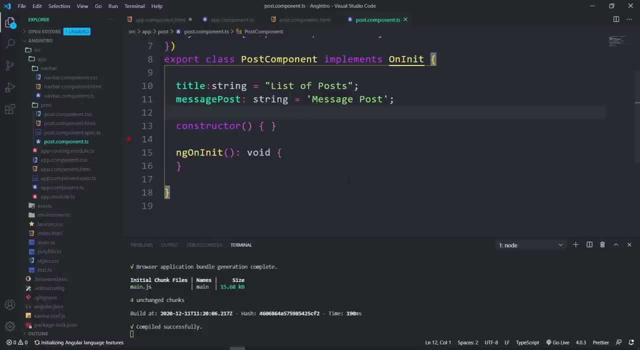 Open the post component ts file. Inside this we have to capture that variable. So we are passing the parent message variable to this component via binding to this variable called from parent. Now this from parent variable, which is coming from the parent component, is in front of this. 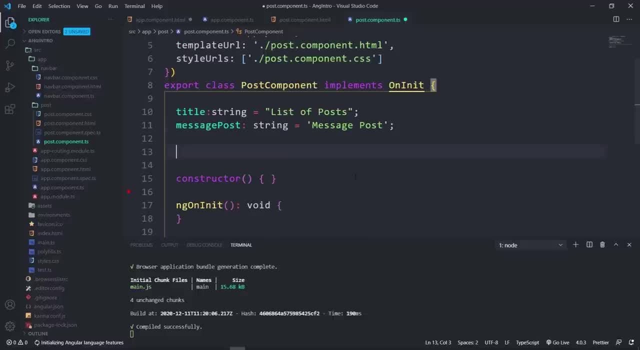 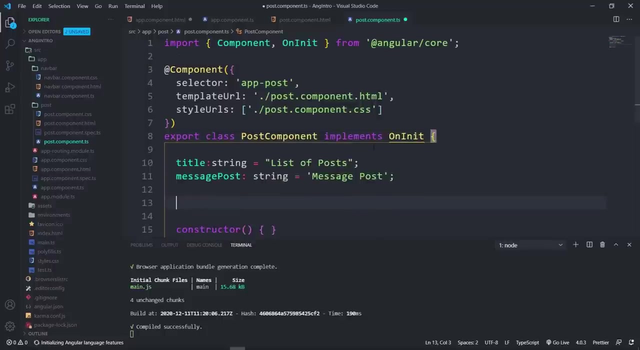 post component. But this variable cannot enter inside to this component, coz this child component's gate is closed. So first we have to open that gate. For that we use the angular input decorator. So first import the input decorator. Inside this input brackets put the input module. 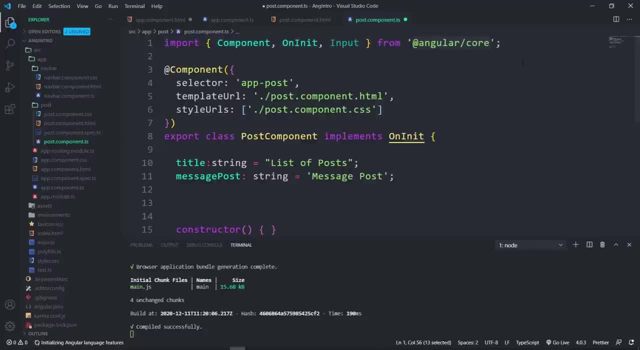 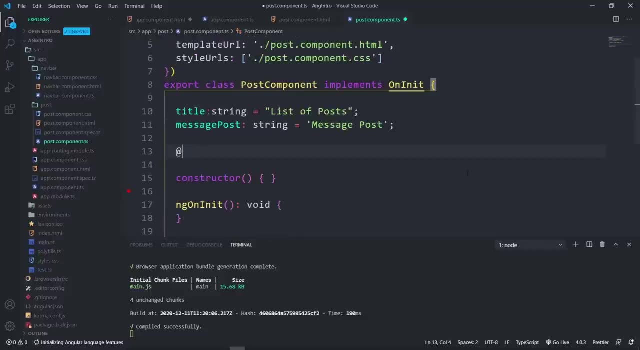 This also comes from the angular core, So we can put this inside this Same import. Next, we have to open the gate, So at decorator. start with at sign: Ok, We learned about this in the component section. Next, the decorator name input. 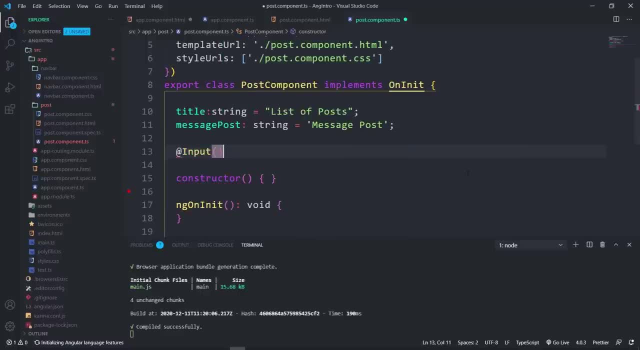 This first letter is capital. Now parenthesis: Alright, Now, with this input decorator we opened the gate, So now we can capture the from parent variable from here. So, after this decorator, from parent variable and the type is string: Alright, now we have the parent shared variable inside this child post component. 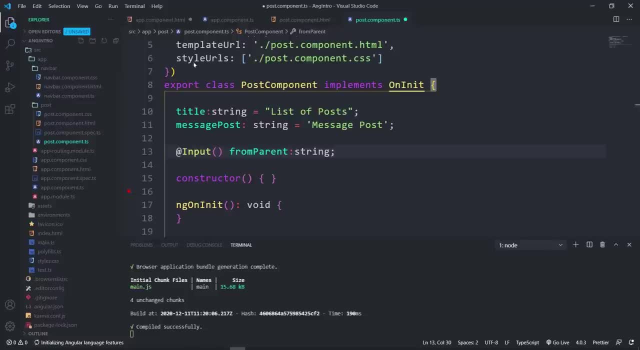 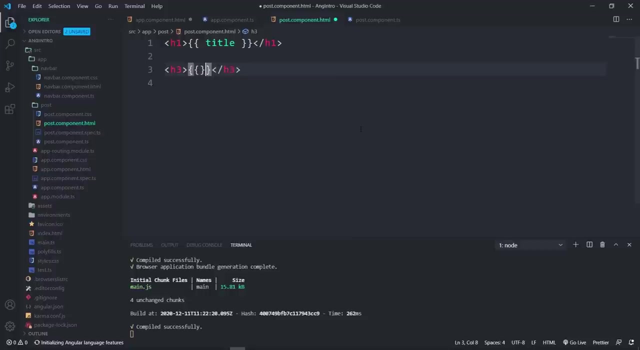 Lets show this component inside the browser. For this we can use the string interpolation, coz. now we have the variable inside this same post component, So create an h3 tag inside the post component html file. Ok, Inside this two curly braces, and between these braces give the variable name, which is from: 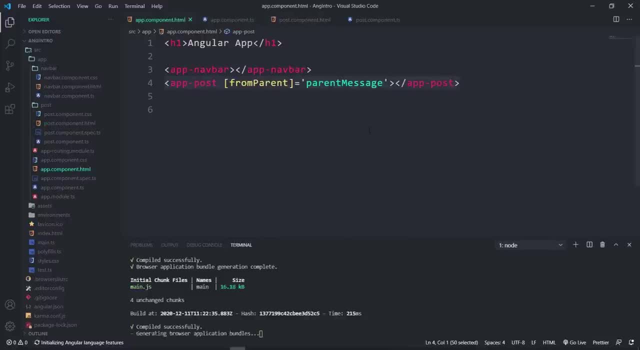 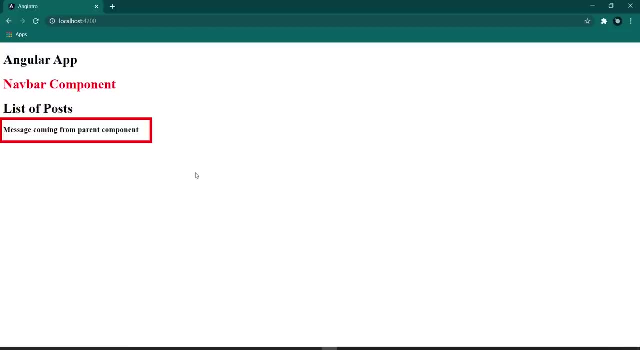 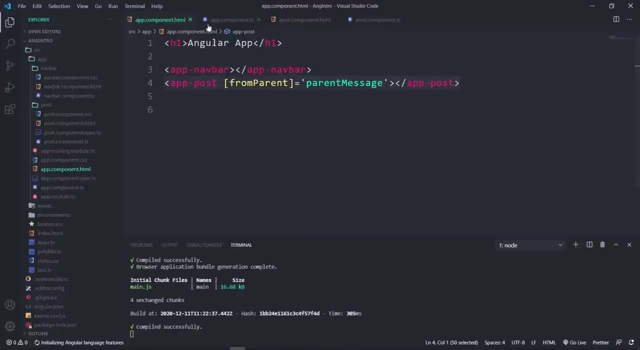 parent Now. save this all and back to the browser. Perfect Now we are not getting any errors and we can see this message Message coming from parent component. Perfect, right Now. lets change this variable message inside the app component. This time. change this message to message change. 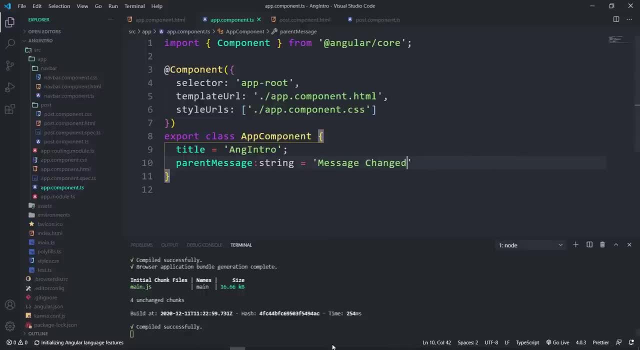 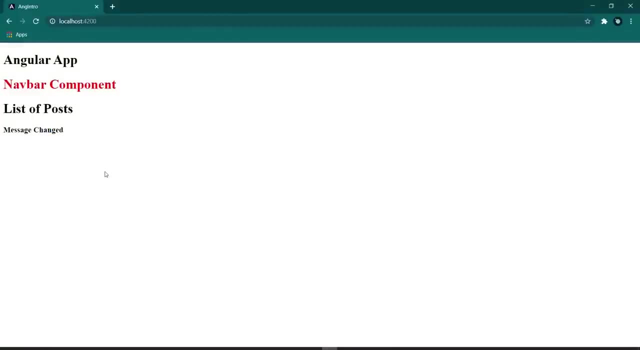 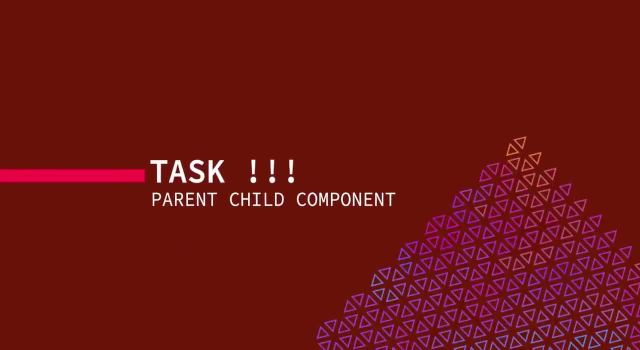 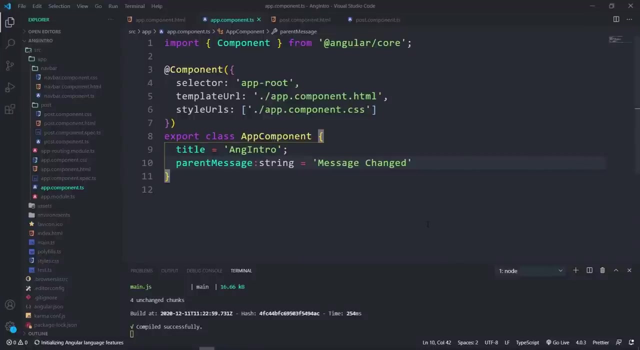 Save this and back to the browser. Awesome Right, This parent message also now changes to this message changed. So this is how we pass data from parent component to child component using the input decorator method. Lets do a small task. We learned how to pass data from parent component to a child component. 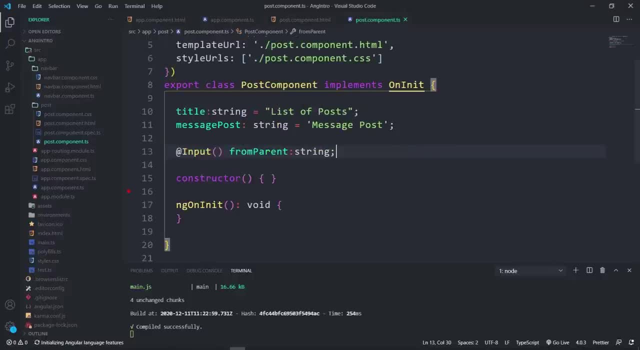 So do the exact same method and pass the data from post component to this post list component. This time, post component will be the parent component and the post list component will be the child component. If you noticed, still we don't have the post list component. 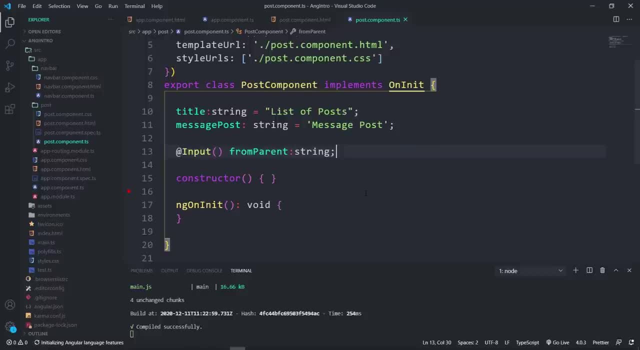 So first generate the post list component, Next create a variable inside the parent post component. Then pass the parent variable to the post list child component. At last, show that variable inside the browser using the string interpolation. Alright guys, if you don't remember, go back to the previous lectures and learn it again. 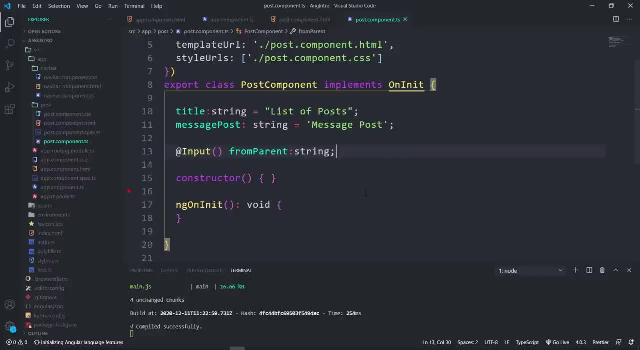 No need to hurry. Take your own time and try to do this task your own. Still, if you can't do this, Try it again and again. You can do this. Never give up. Alright, now pause the video and start the exercise. 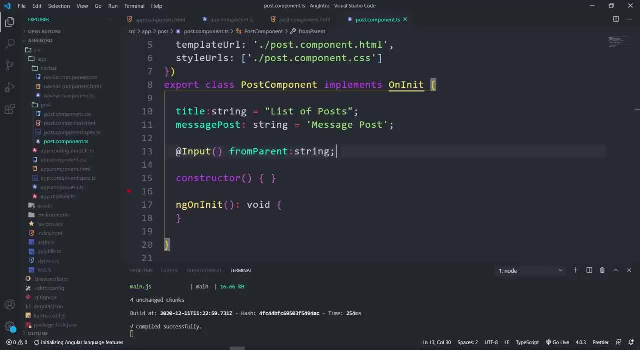 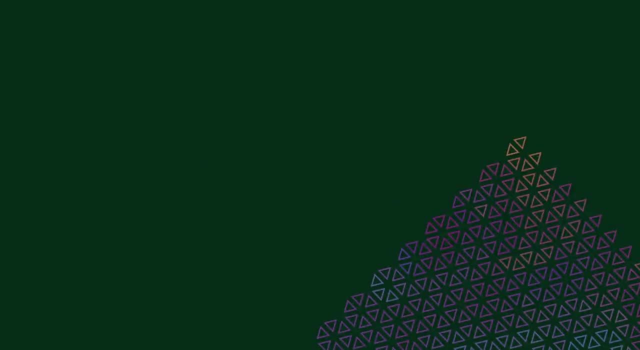 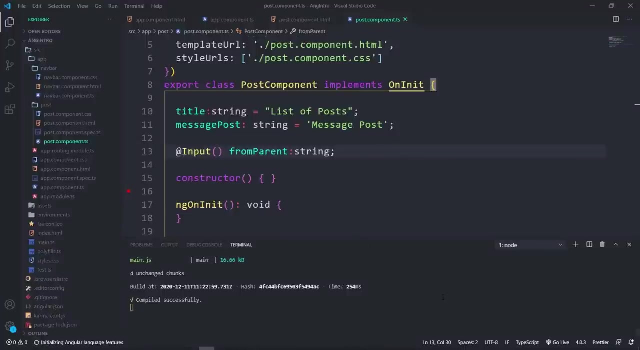 Once you have completed the task, continue with the next video. Alright, lets continue the task. Those who have successfully completed this task, good job guys. Those who are not completed this For them also very, very good job guys, Because you are trying to do this. 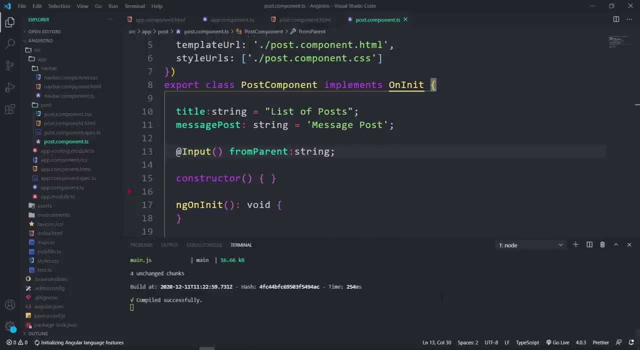 The final result is not important. You must try and try and keep trying to achieve your goals. That's what I wanted. Alright, lets see how to do this exercise. First, lets generate the post list component using the angular CLI inside the integrated terminal. 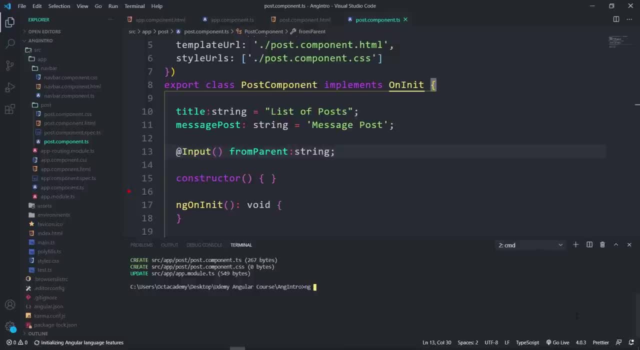 Run this command ng. This ng command is coming from the angular CLI g This stands for generate, c This is for component, And at last give the component name Post list. This post list is a two word name So as a best practice, if the component name is a two or more words name, just separate. 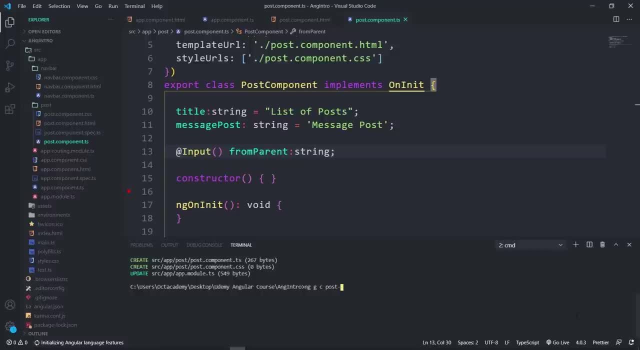 them with a dash, Something like this: Post dash list. This is not compulsory, but try to follow best practices. and one more thing: we cannot keep spaces in the component name, Like this: post space list. Hope you guys got the idea. So change the name to post dash list. 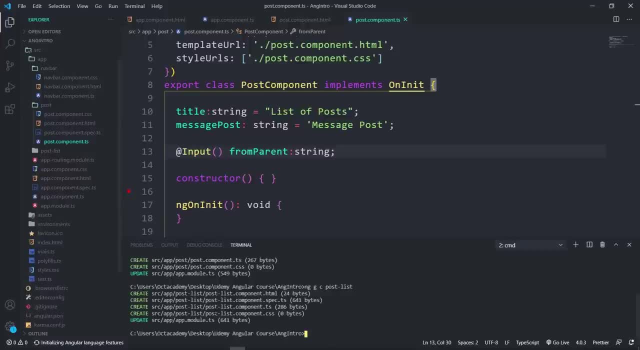 Now hit the enter. Alright. post list component is ready. Ok, first create the variable inside the parent component. This time parent component is this post component. So inside the post component is file. create the variable post parent message. This p and m will be capital. 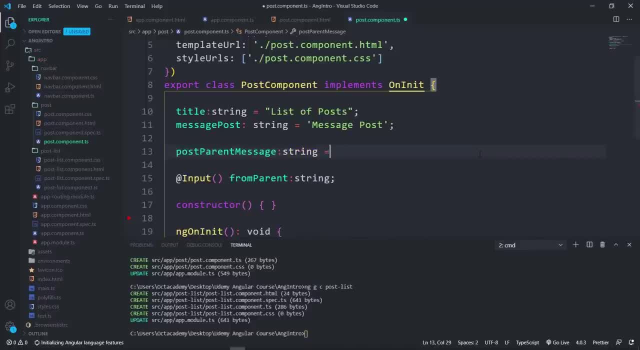 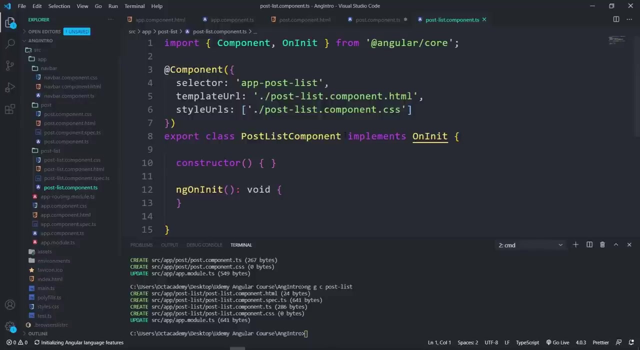 So this variable type will be string. After this assign, the message is message coming from the post parent. Next we have to send this message to the post list component. So for that, put the post list component inside the post component using the selector. The component selector is this app, dash post, dash list. 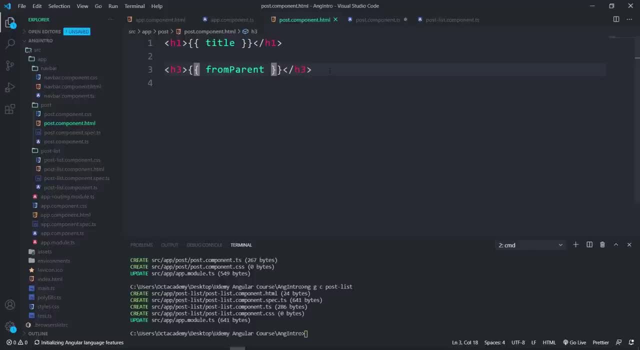 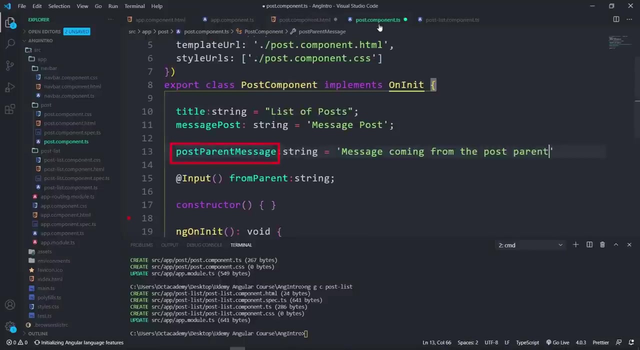 So inside the post component html file put this selector as html custom element: app dash, post, dash list And hit enter Alright. now let's pass the variable Inside this post list element. square brackets inside that something: variable name from post parent Equal sign. inside quotes pass the variable name which is post parent message. 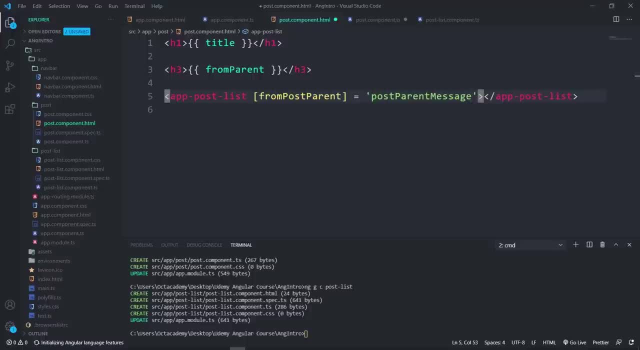 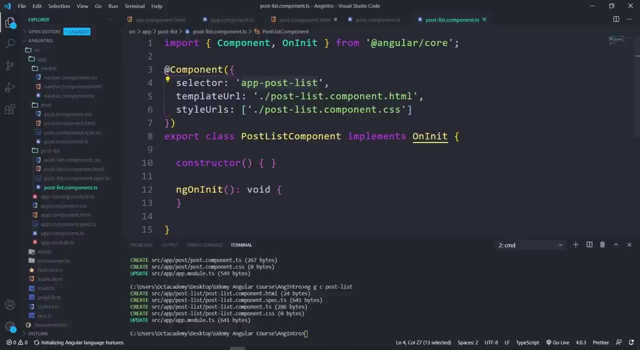 Next we have to capture this from the post list child component. For that we use the angular input decorator. So first insert this, First import the input decorator. Inside this import input, This input decorator also part of the angular co module. that's why we put this inside the 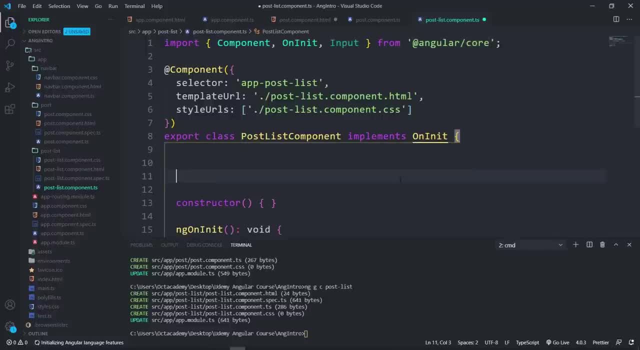 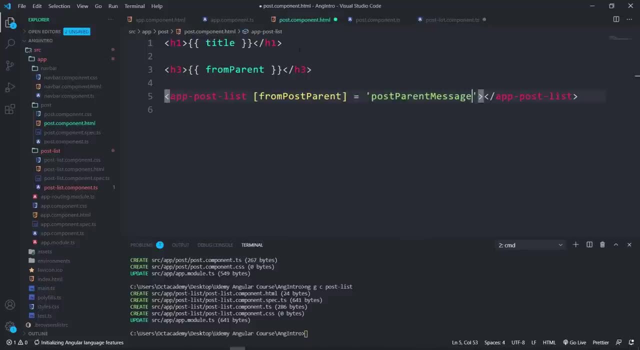 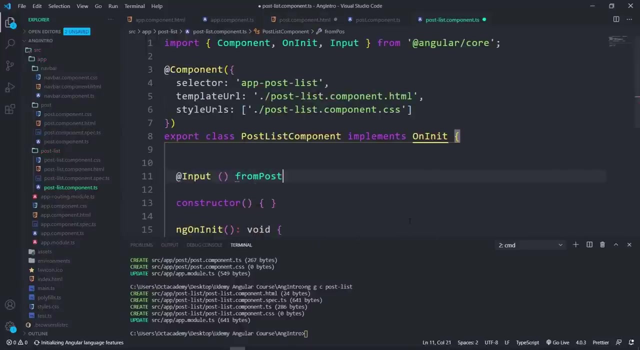 same input Next at input and parenthesis. So from the parent component we share the variable binding to this. from post parent variable. So put that variable name here. from post parent. So carefully follow this capital: simple letters. So this variable type will be string. 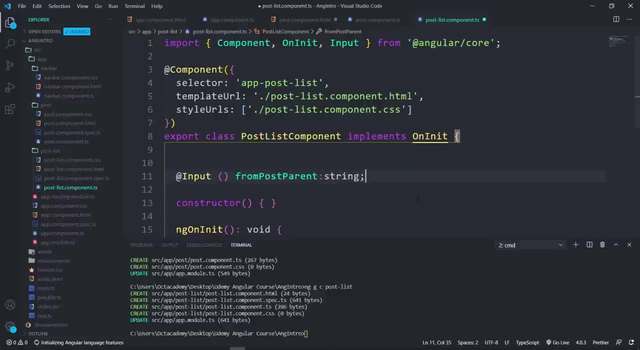 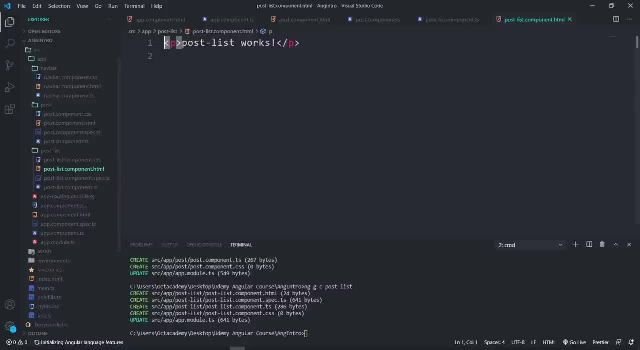 Now we have captured the post parent variable. Now we can show this inside the post list component using the string interpolation. Go to the post list html file. So remove this p tag and put h1 tag post list component. After this: Inside of a p tag, two curly brackets. 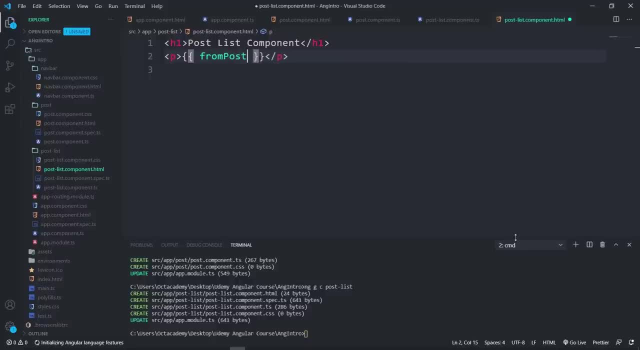 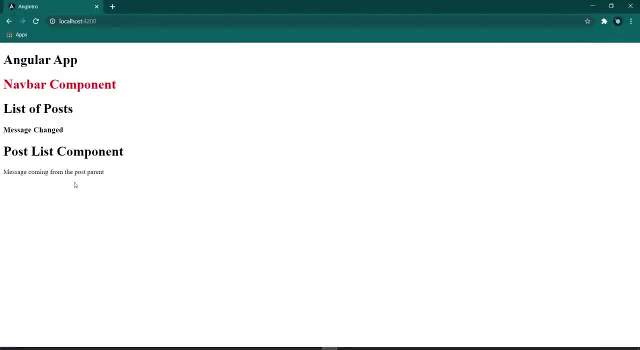 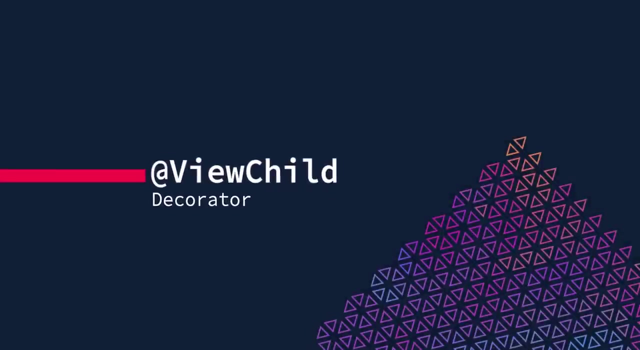 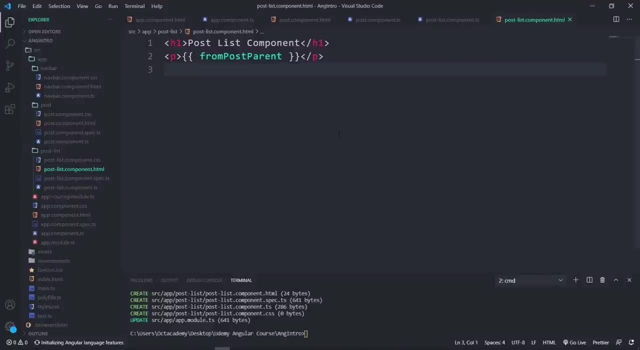 Inside that variable name is from post parent. That's it. Save this and back to the browser. Here it is. We can see this post parent message. Very simple, right? Alright, we learned how to pass data between parent component to a child component. 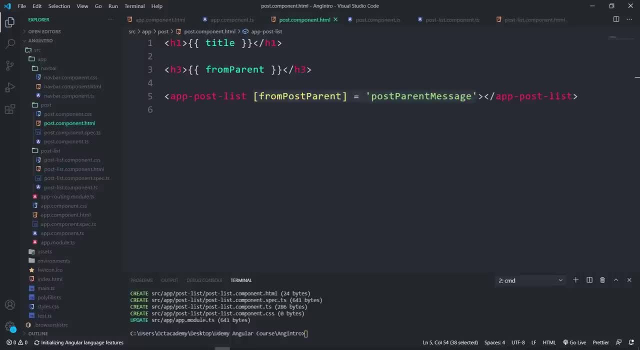 Now let's look at how to pass data from child component to parent component. We cannot do this using the input decorator, coz we don't have the parent component selector inside this child component. So then only we can pass the data to the relevant component using the input method. 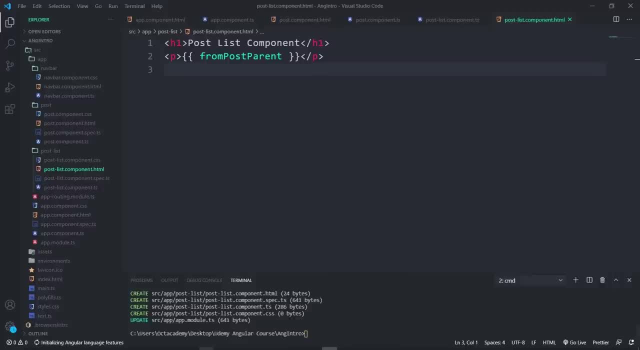 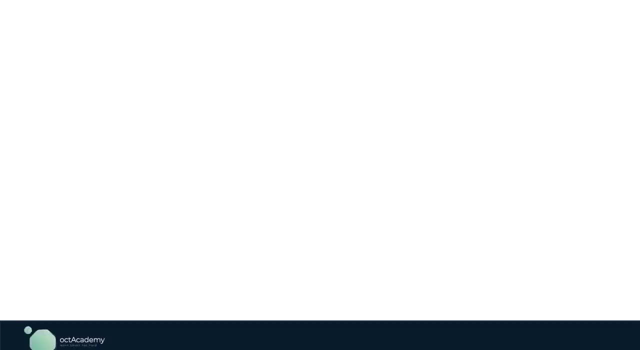 In previous, we pass the data to the child component via binding the data to the component selector. But think, If we want to pass data to a parent component from a child component, For that we have two methods. The first one is the share the data using the weave child method. 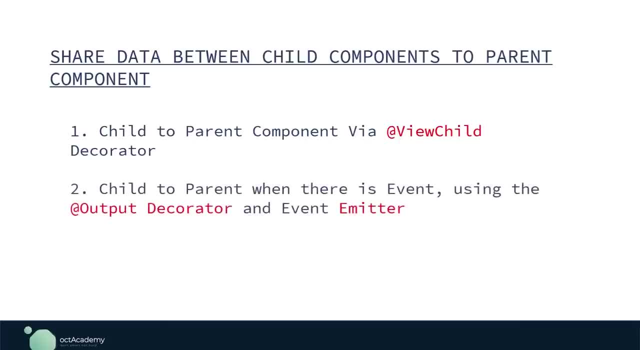 The second one is the output decorator and the event emitter method. In this video we will look at the first method: weave child method. We will look at the second method in the next video. Alright, Let's see this weave child method in action. 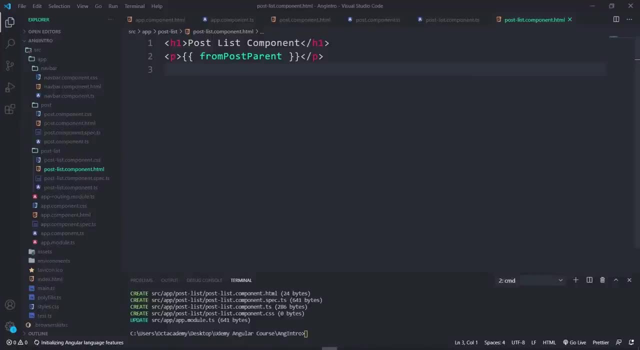 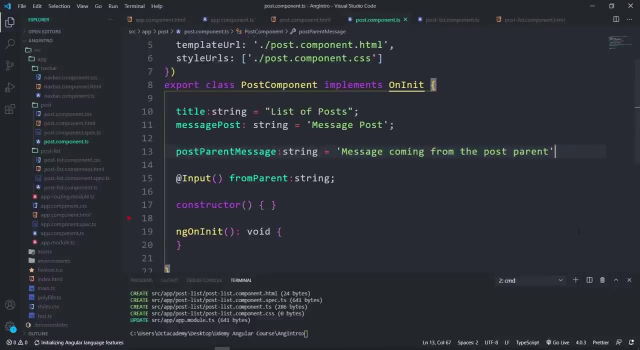 So this time we want to share data from child to parent component. So create the variable inside the child component, which is the post component. Inside the post component ts file, create a variable called child message, and this variable type will be string. Now assign this text as a value for this variable from child component. 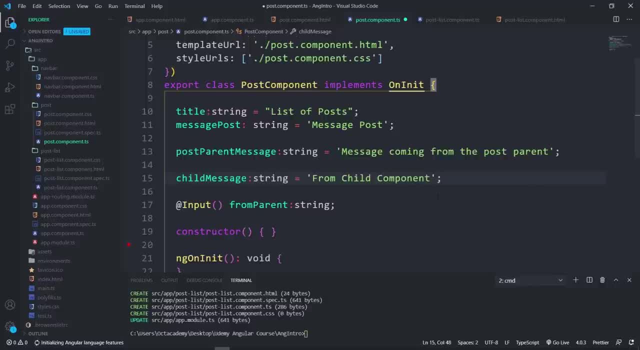 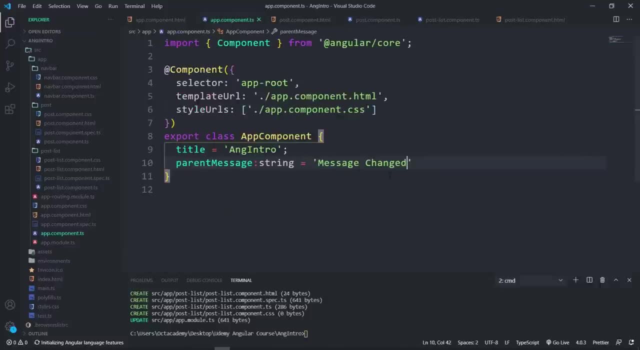 Alright, we have the variable. Now let's access this variable from this parent app component. For that we gonna be using the weave child decorator, So open the app component ts file and import the weave child. This is also coming from the angular core module. 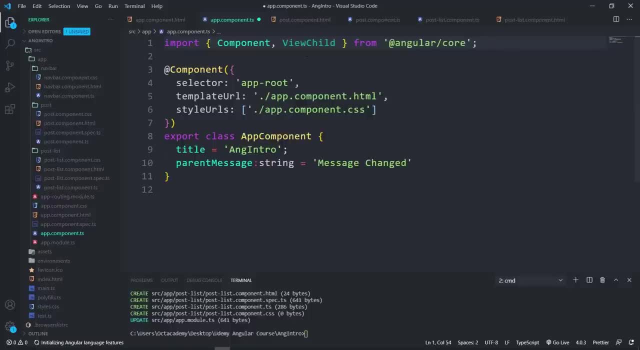 So put this inside this same import Weave child. Carefully follow this naming convention: capital and simple letters. This first v and this c is capital. So with this weave child we gonna look inside the child component. So inside the component class first add the weave child decorator at wave child and parenthesis. 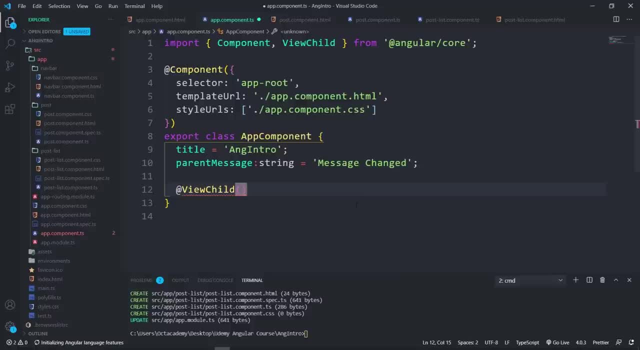 Inside this parenthesis we have to pass the child component that we want to get the data from. So now we want to get the data from this post child component, So pass the post component Inside this weave child parenthesis. For that first we have to import the post component. 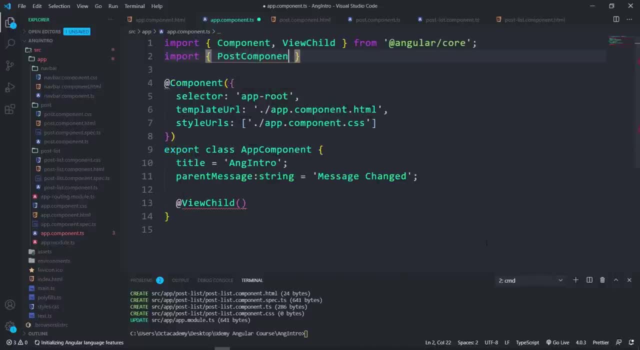 Import inside curly brackets, post component this p and c capital from inside quotes. this is inside the post folder. so dot slash, post slash and this post dot component. Now pass this post component inside this weave child parenthesis After this. give a name for this. This can be any name: child comp. 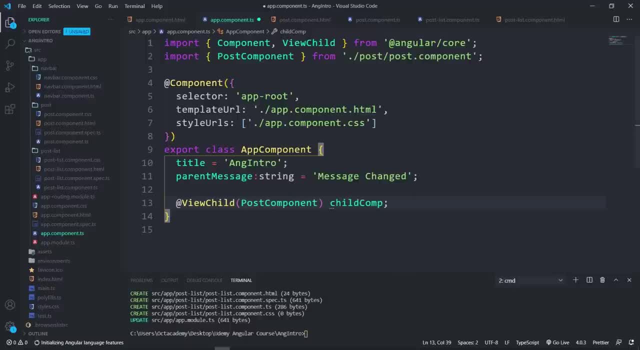 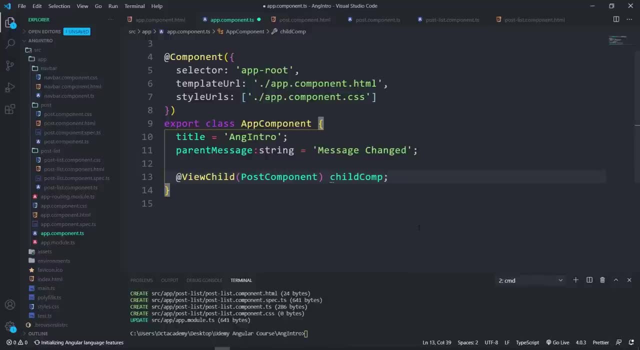 Alright, now we have the post component. Next we have to access this component and we have to get that variable child message. So first lets login, see what is coming with this component. So log this inside the constructor Now. so create a constructor, Constructor parenthesis and the constructor scope. 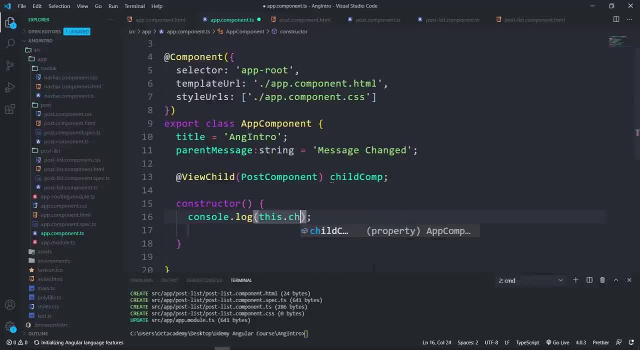 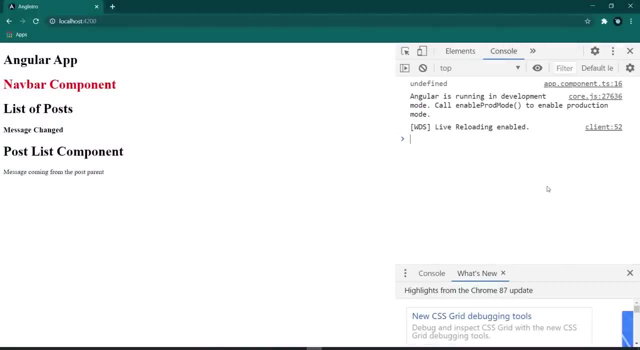 Inside this log, this component child comp. Save this and go to the browser. Now open the browser console. Inside that we can see this log. that's saying undefined. Why is that At the time this app component loads to the browser, this child component is undefined. 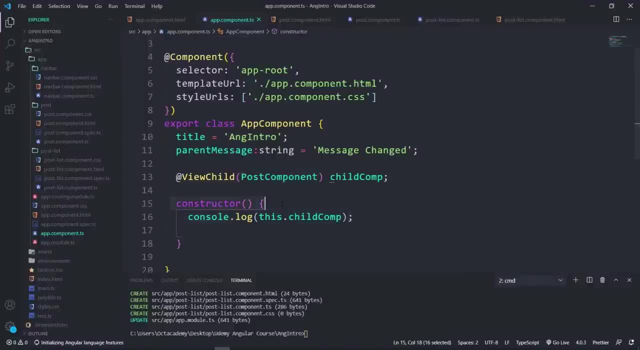 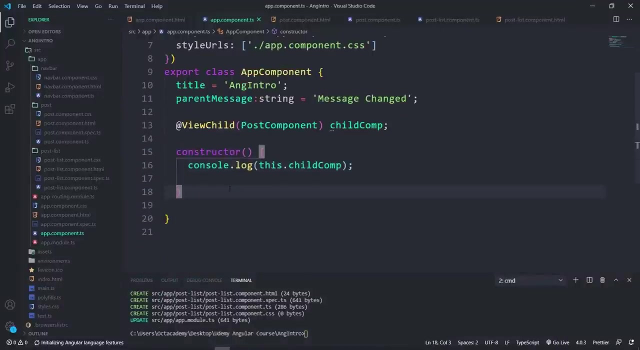 So you guys already know this constructor method Will load immediately the app class object created At that time. post component is undefined. That's why we are getting this undefined log. So to access this we have to use an angular component lifecycle method, which is the after. 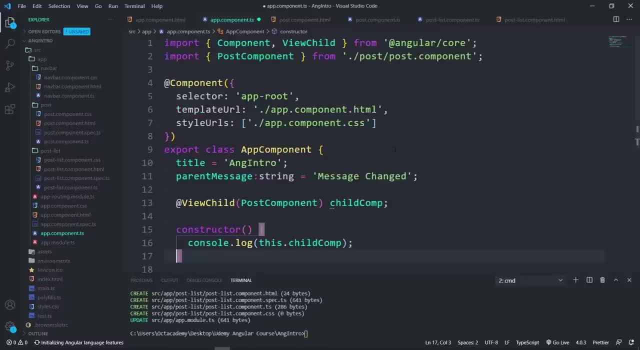 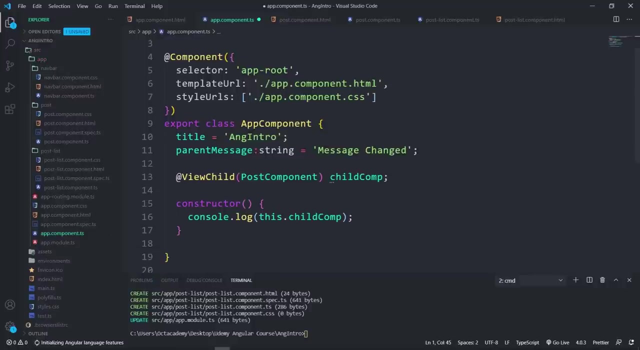 weave int lifecycle hook. First we have to import the lifecycle method to this component. This is also coming from the angular core, So put this inside this Same import after weave init- Alright. next we have to implement this after weave init lifecycle hook to this app component. 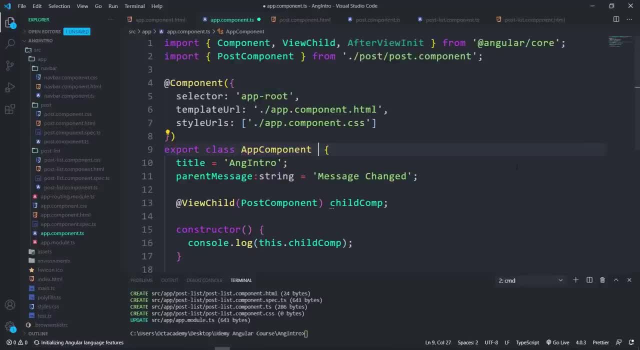 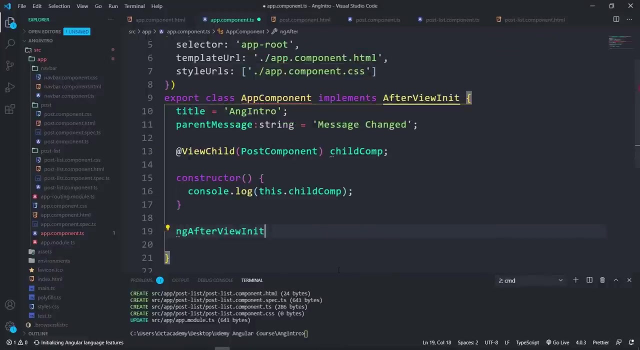 class. Then only we can use this lifecycle hook inside this app component After this class implements. after weave init. Once again, follow this capital simple letters carefully, otherwise this code will break. Next, create the lifecycle method: ngAfterweave init. This name must be the same as this: 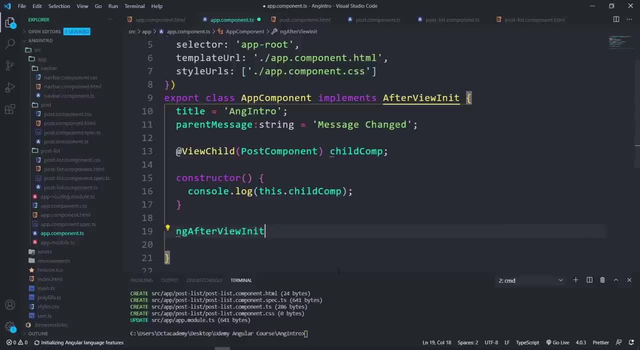 So carefully follow these capital, simple letters. So next, parenthesis and the scope. Now let's log this view child component inside this ngAfterweave method, Inside this method, consolelog. Now save this and back to the browser. Now inside the browser console. 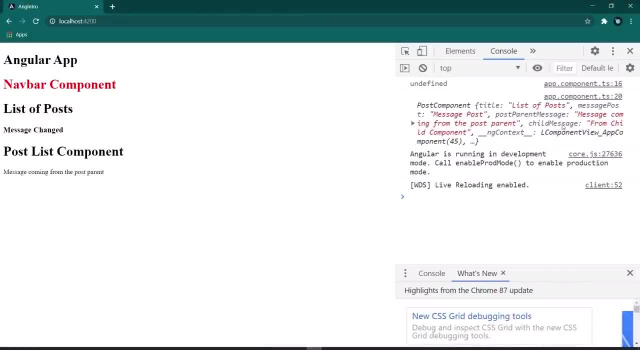 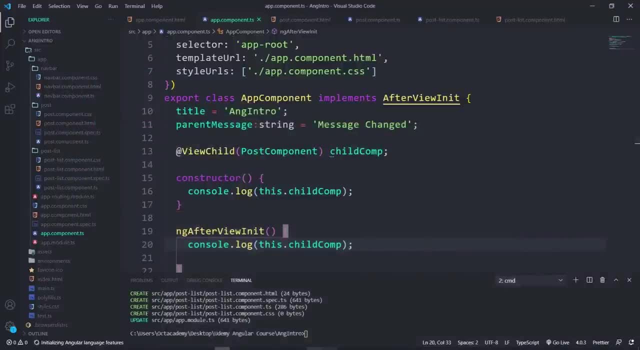 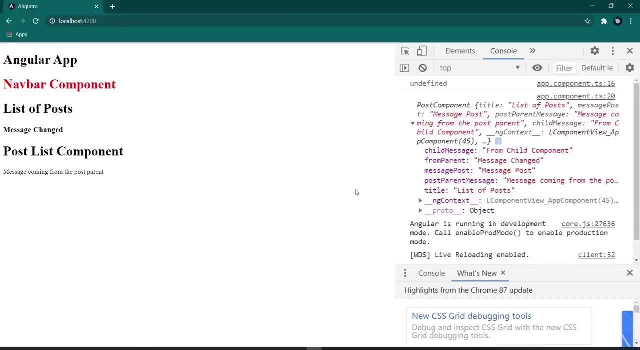 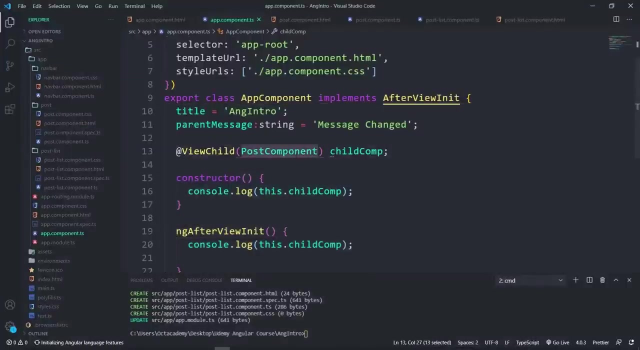 Now we can see this. We can see this undefined as well as this post component. This undefined printed from the constructor. This component printed from the ngAfterweave init method. So you guys may wonder what is happening here. As i mentioned before, when the time this constructor method works, this child post. 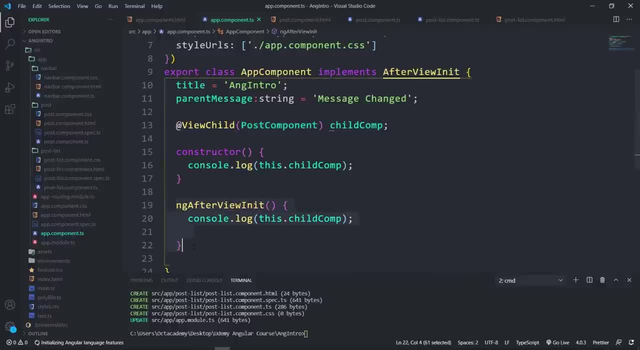 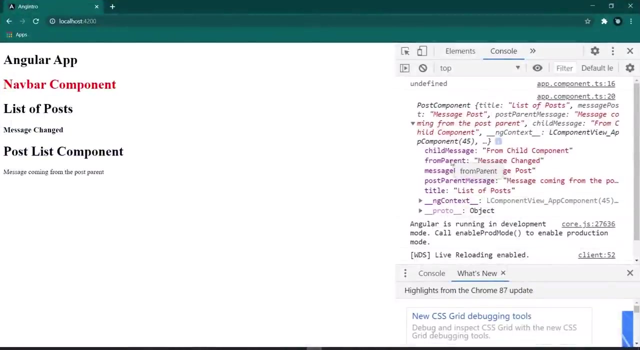 component is not initialized inside the browser component lifecycle hook after wave init. This method will call once after the total wave initialized on the browser. So that's why we are getting this log printed inside the browser. Hope you guys got the idea. Now look at this log. We are getting this how? 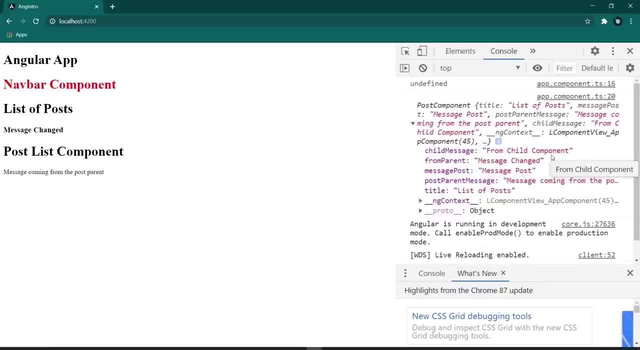 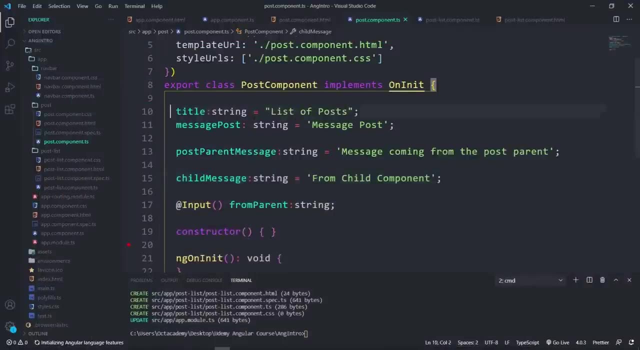 variable, child message and its value, which is created inside the post child component. If we look further, we can see other variables too. This is the beauty of this wave child decorator. With this wave child decorator, if we want, we can access all the child post. 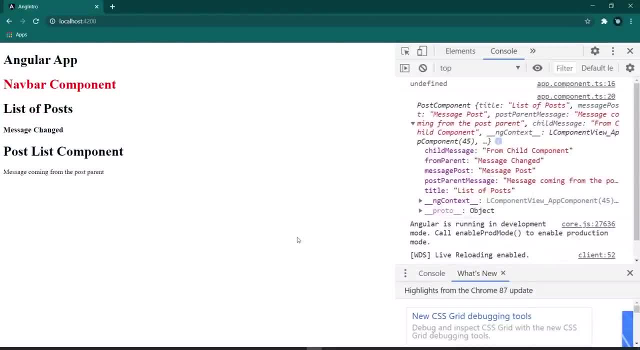 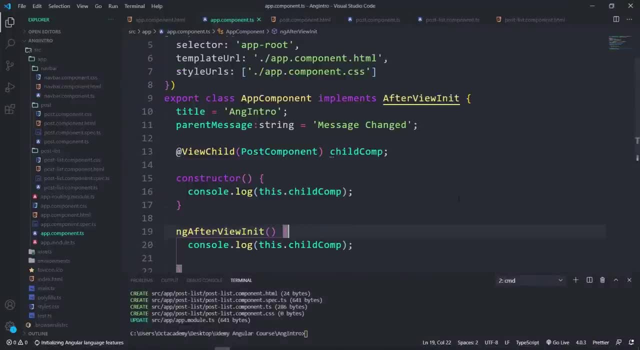 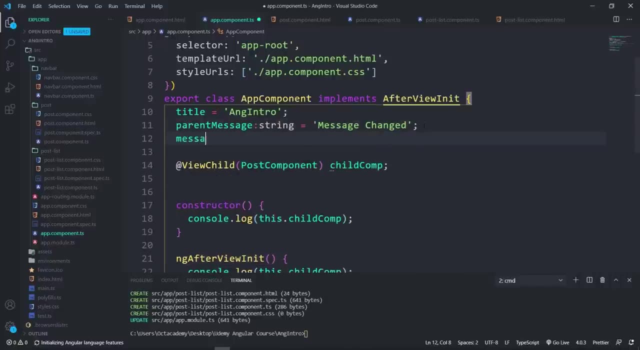 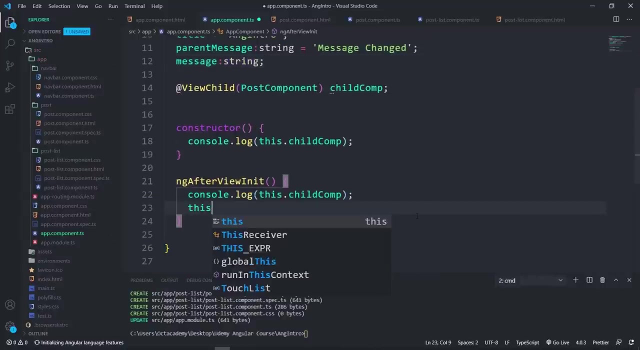 components variable from this parent app component. Ok, now we have the variable. Let's show this inside the browser using string interpolation. For that: first we have to assign the components to a variable. So create a variable message and the type will be string. Inside this lifecycle method, thismessage assign: 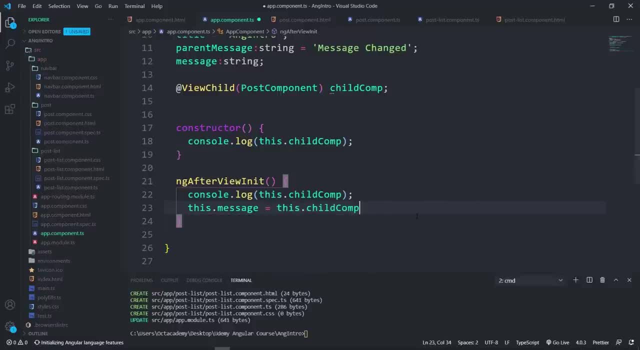 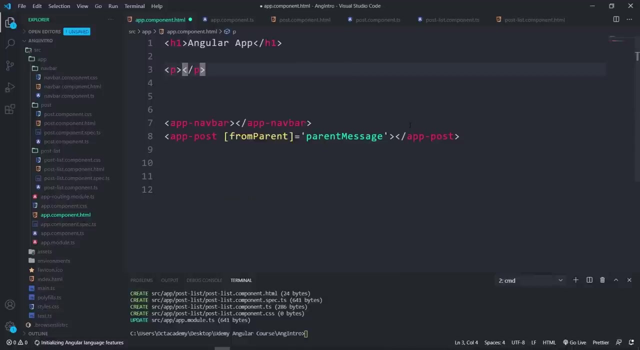 this dot. The component is child comp. Inside this child comp we have the variable that we want to access, which is child message. That's it Now. inside the app component html file, create a p tag Inside this, two curly brackets Inside that. 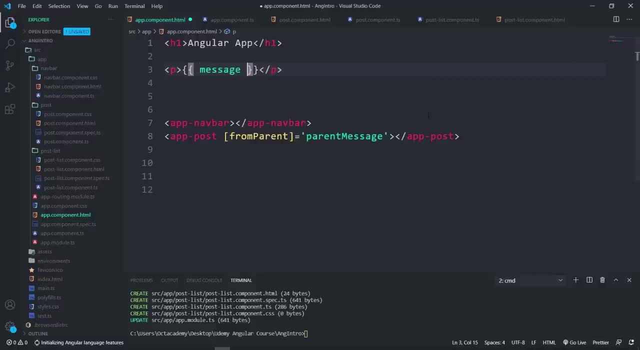 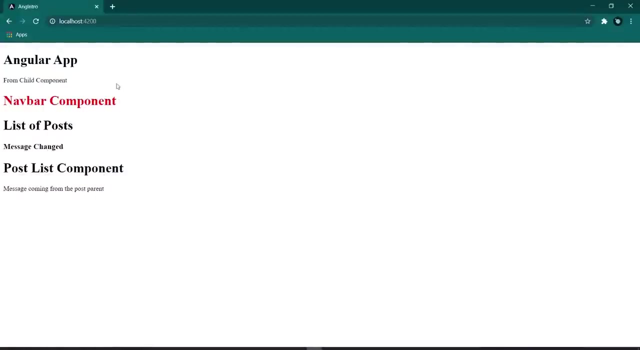 pass the variable message, Save this all and back to the browser. Beautiful right, We got this message from child component, which is coming from the post child component. This is how we passing data between child component to parent component using the wave child decorator. 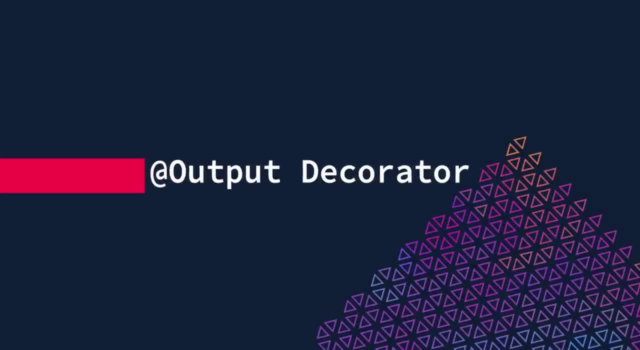 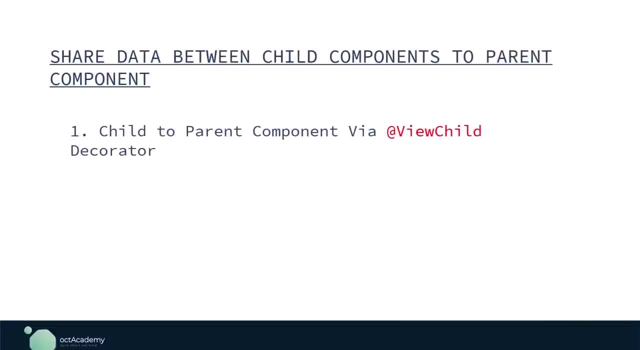 So in the last video we learned how to pass the child component to the parent component using the method1.ViewChildDecorator. So in this video let's look at how to pass data between child to parent component using the second method output decorator and the event emitter. 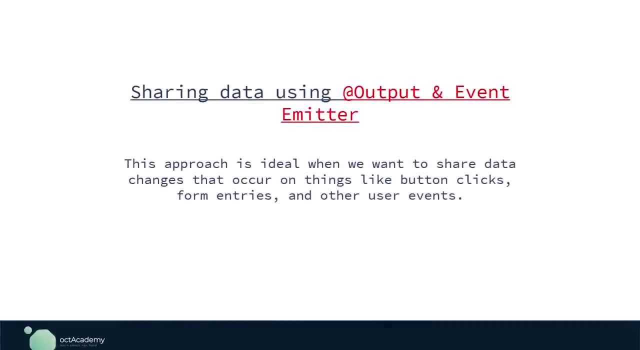 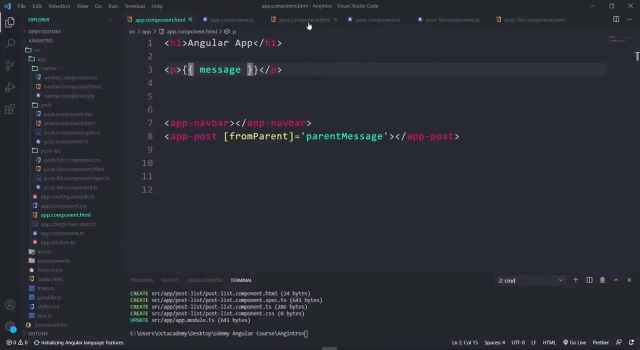 So this approach is ideal when we want to share data changes that occur on things like button clicks, form entries and other user events. Next, let's create the variable inside the child component, which is the post component. So go to the post component ts file and create a variable and create another variable. 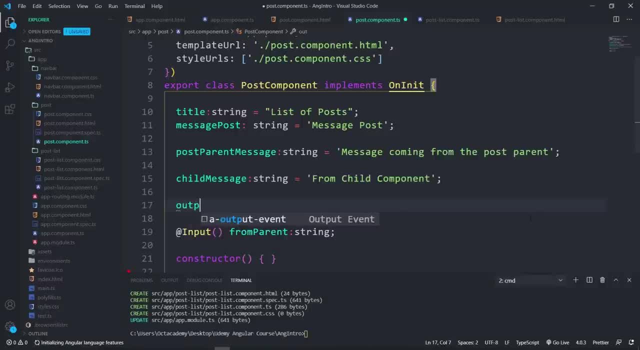 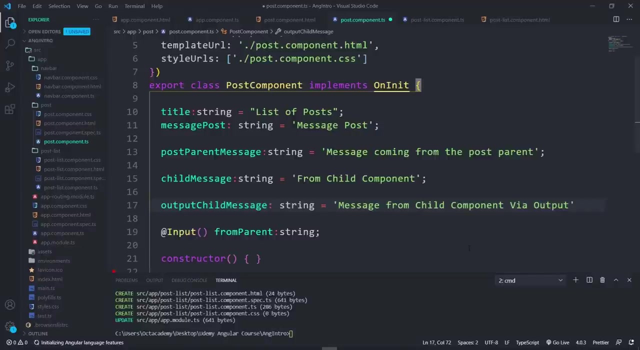 This time, variable name is something like output child message. So this variable type will be string. The value is something: message from the child component via output. Next we have to create a new event emitter. Let's create a new event emitter with the output decorator. 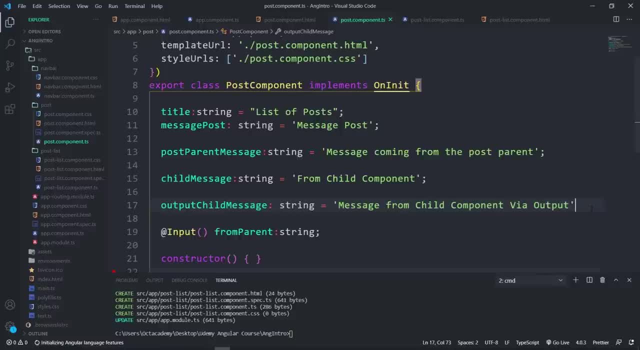 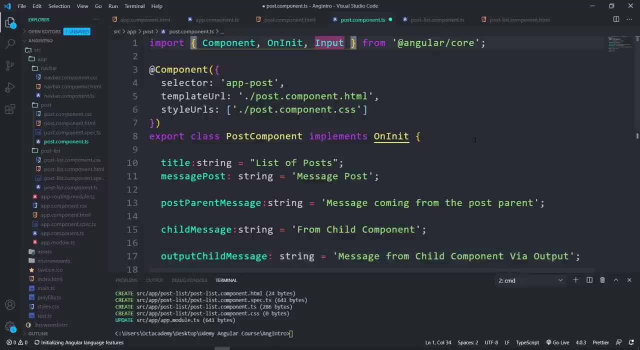 For that, first we have to import output and event emitter to this post component, which also comes from the angular core. So put these two imports inside the same import First one is output, So this O will be capital. Next event emitter. This two ens are capital. 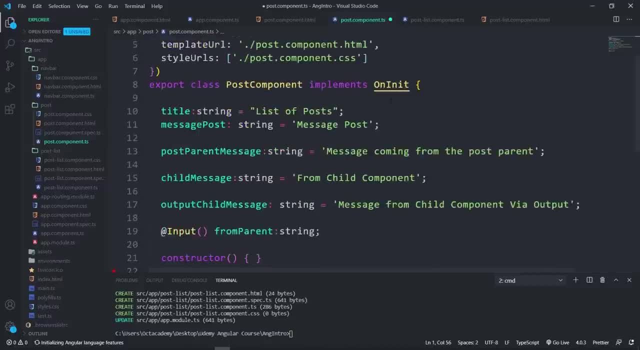 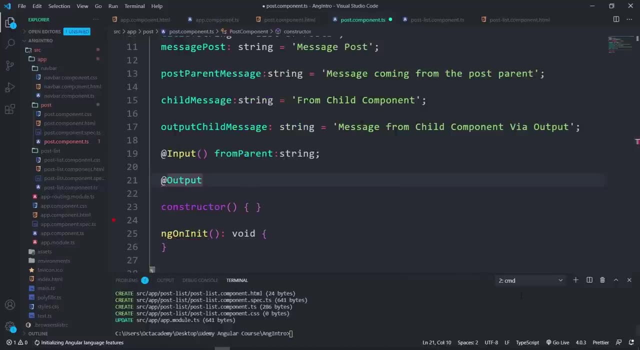 Alright, Let's create the event emitter with the output decorator. At output, follow all the capital simple letters carefully. The name for the event emitter: message: event. Then assign niv event emitter. This event emitter type is string and parenthesis. Alright, we have created this event emitter. 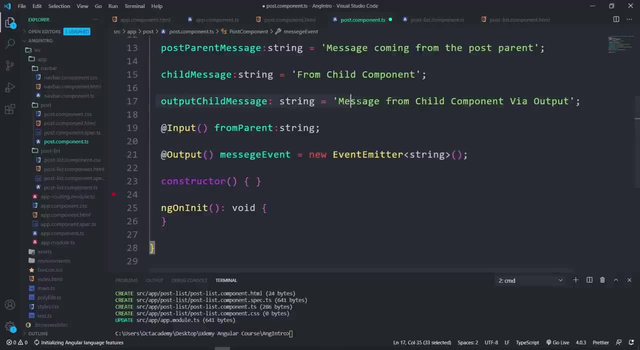 Now what I want to do is I want to emit this message to this event emitter. This event emitter type is string. I want to emit this message to this event emitter when clicking a button. As I said before, this approach is commonly used when there is a user action. 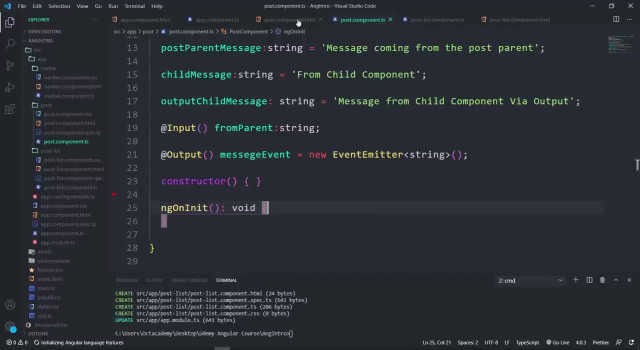 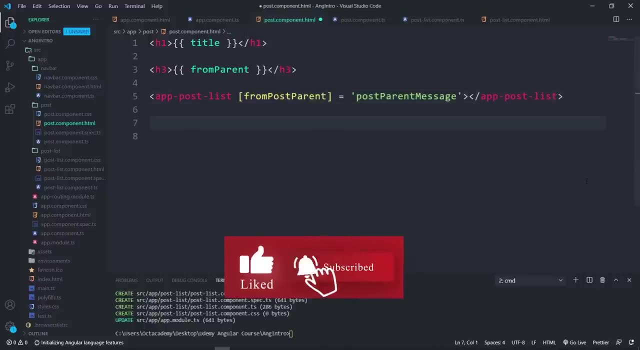 Alright, let's create a button inside this post component. Usually we put all html markups inside this html file, So go to the post component html file and create a button, Just a simple button Button tag Inside that Click. Now I want to call to a function. 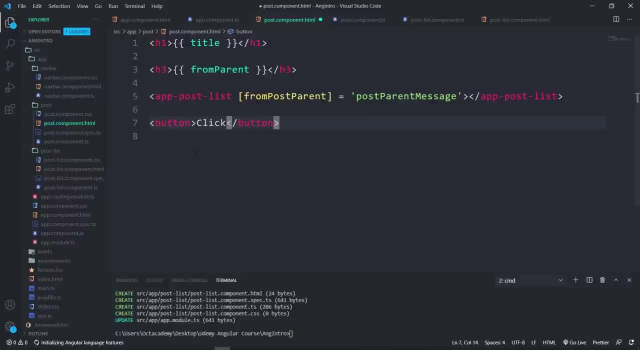 When clicking this button. For that in plain javascript we can use the onclick event. But in angular this is a bit different. Angular has its own click event. So inside the button tag create a pair of brackets. Inside the brackets click all simple letters. 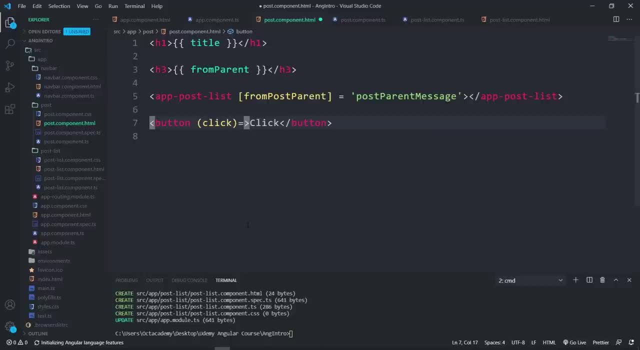 So this is the click event in angular. After this equal sign, Then inside codes: Click. Now I want to call to a function when clicking this button. So let's put that function name inside this codes. Still, we have not created the function yet. 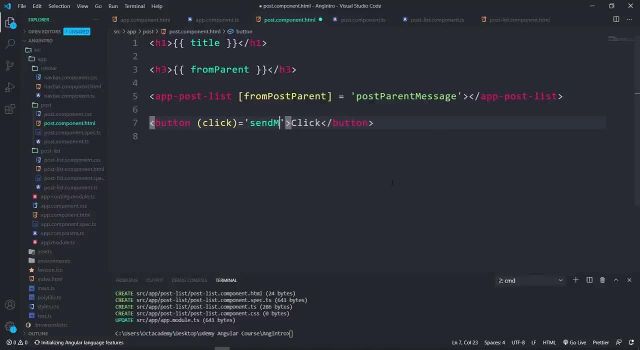 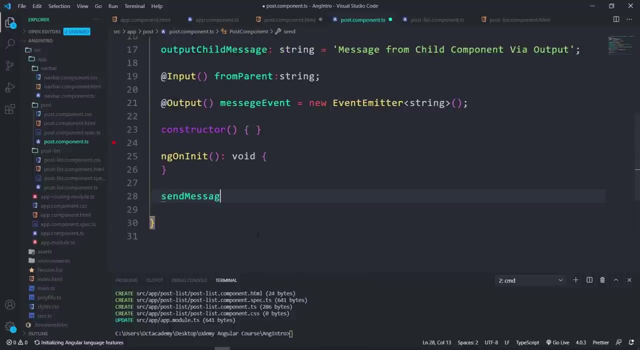 So give a name, just Send message and parenthesis. Alright, now we have the click event. Now let's create this method inside the component ts file. So inside this class scope Create a method. The method name is SendMessage, Parenthesis, and the method scope. 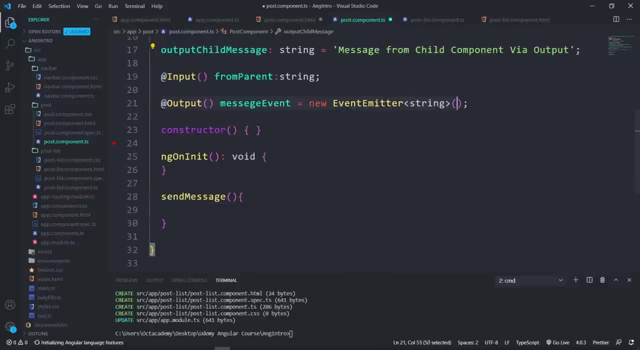 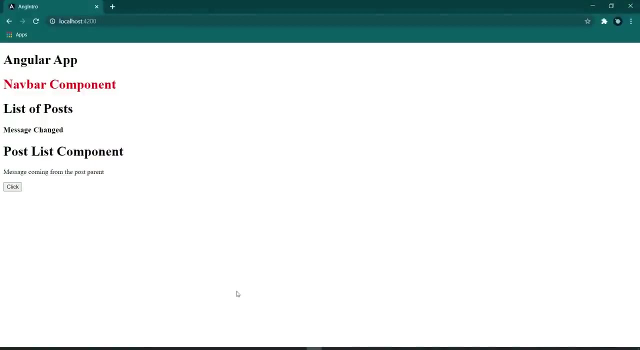 Inside this method. I wanna emit this message to this event emitter. Before that, let's check whether this button click event is working or not. So let's log clicked inside this method. So save this and back to the browser. Now we can see this button. 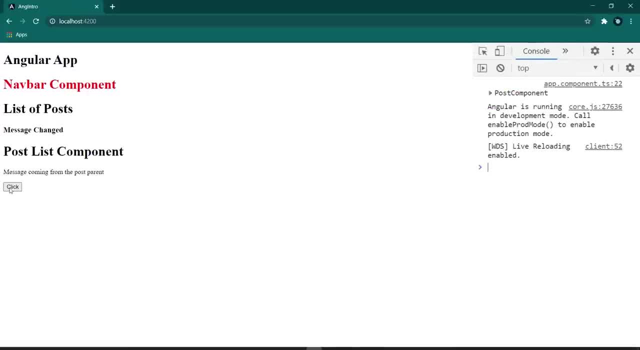 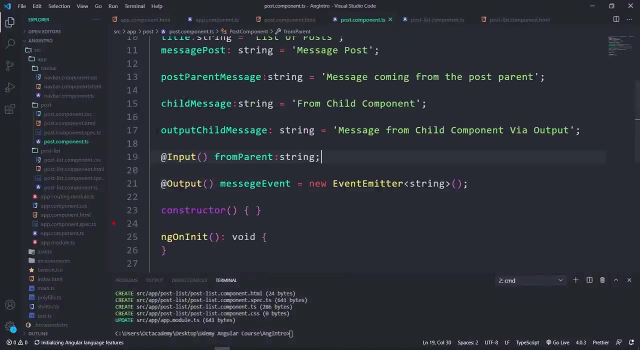 Click that button. Perfect Click event is working without any problem, So that's why we are getting this clicked. log inside the browser console. Alright, the clicked event is working. Next, let's emit this message to the event emitter. So, inside this method. 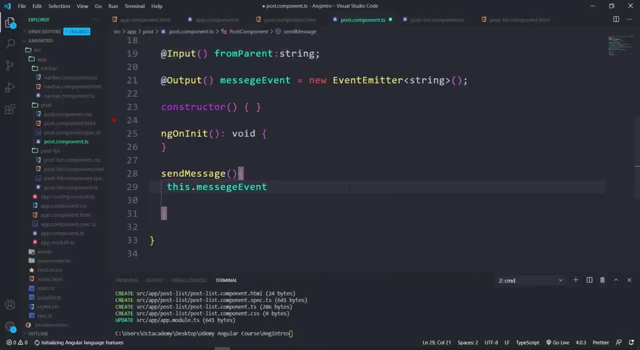 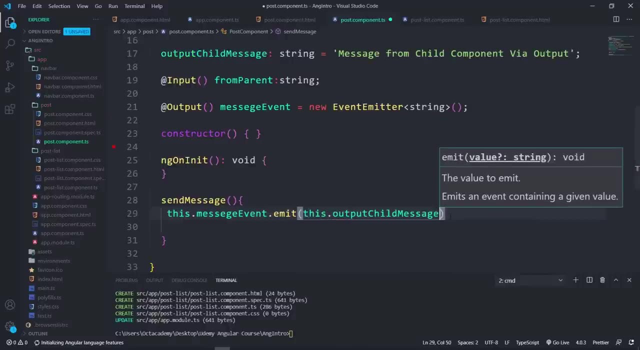 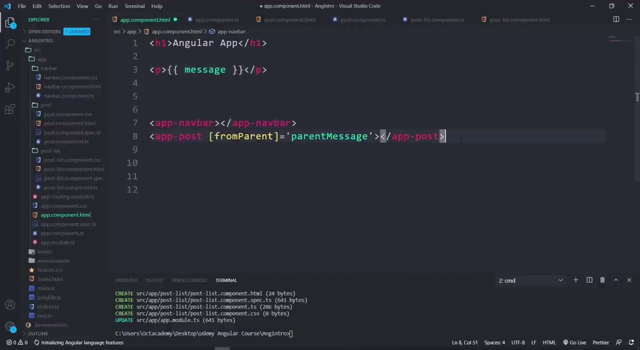 This dot message: event dot emit. parenthesis inside that this dot message. That's it. We have successfully emitted this message. This is the message variable to the event emitter. Ok, next we have to capture this event from the parent component. For that go to the parent app component: html file. 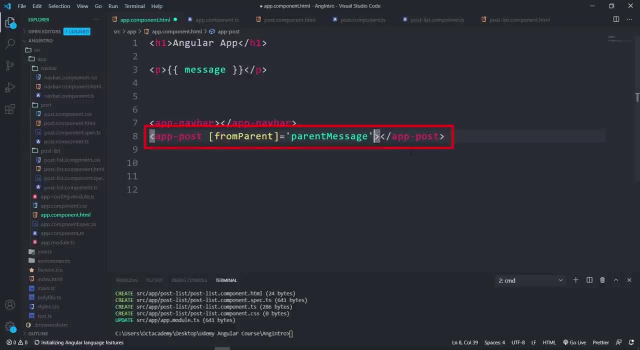 So this is the selector element for the post child component. So what I am going to do is I am gonna bind the event emitter to this post element. So inside this selector element, brackets, Inside brackets- Event emitter: Event emitter name is this message: event. 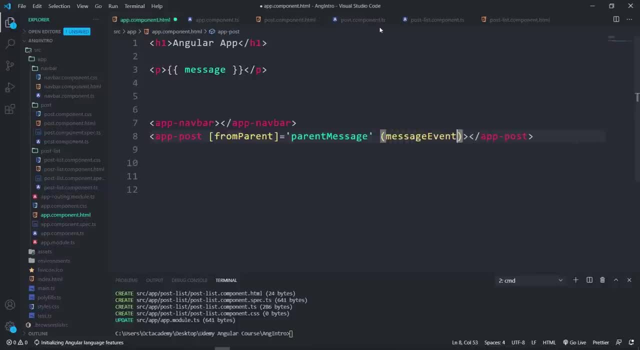 Put this inside these brackets. Next, I wanna call a method when this event emitter triggers, So equal sign inside quotes, pass the method, receive message, then parenthesis. So inside this parenthesis pass the event as the parameter. So still, we don't have this method inside our app component html file. 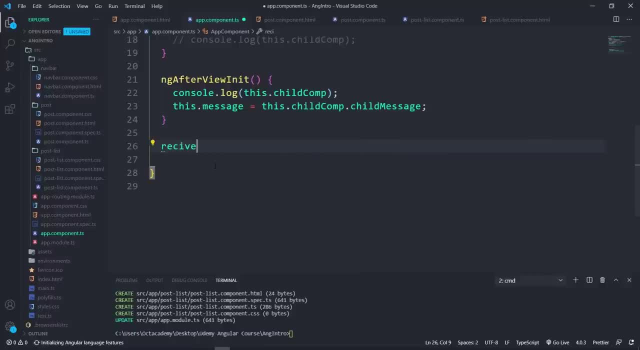 So create this method. receive message. this m is capital parenthesis and the method scope. We are getting an event parameter for this method, So passed event for this parenthesis. Alright, now let's see what we are getting with this parameter. So log this event inside this method. 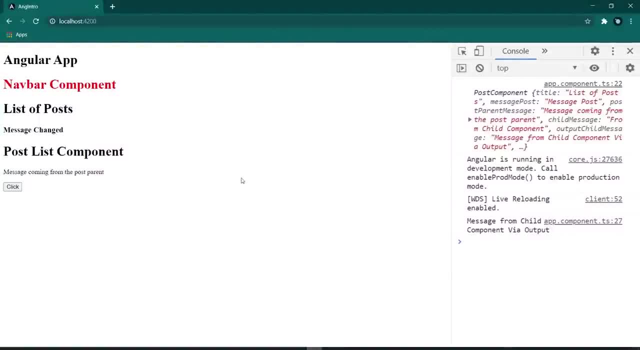 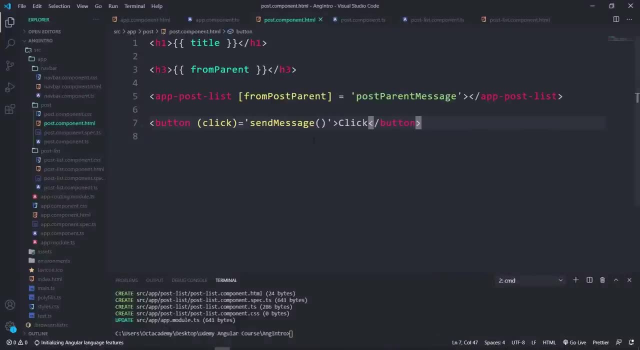 Save this file and back to the browser. Now click this button. Perfect, Now we are getting a message from the child via output, which is coming from post child component. Awesome, right. So what is happening here? We are getting this child component, variable data inside this parent component when clicking. 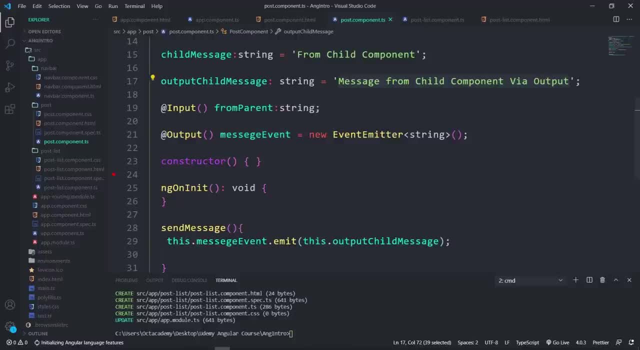 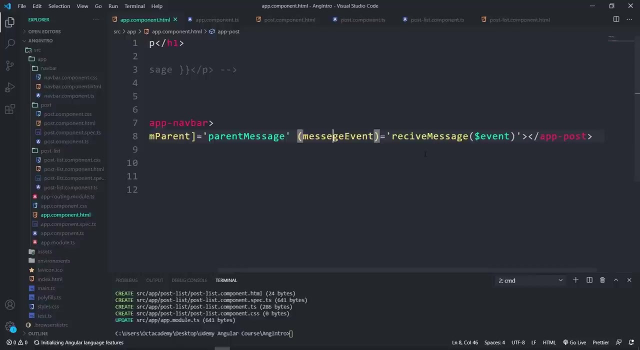 this button, This button also inside the child component. This all magic is happening with the output decorator. When we clicking this button, We are emitting this message to this parent component. We are getting a message to the event emitter cause of this output decorator we can access. 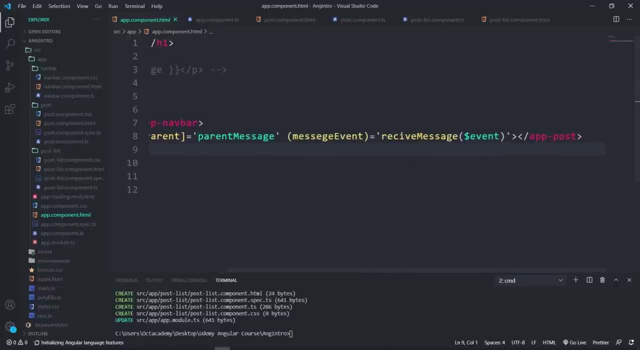 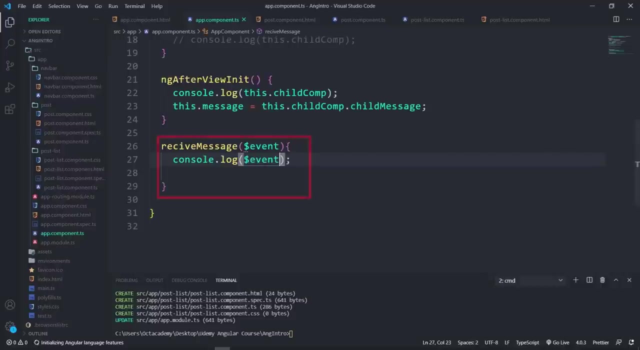 this from outside of this component. So next what we did is we bind this event emitter to this post component selector element, which is inside the parent app component. Then we call to a method when this event emitter triggers. this event emitter will trigger or get active. 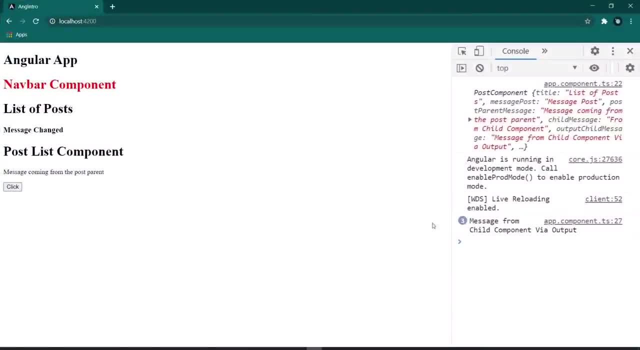 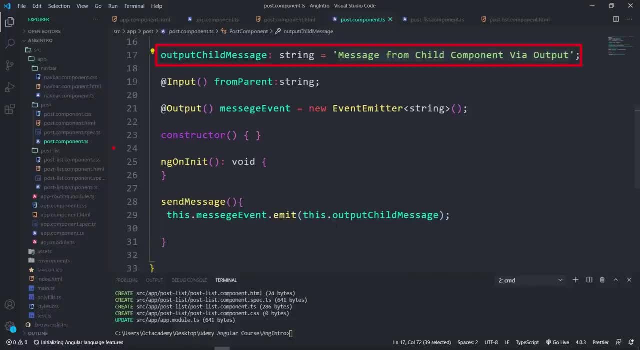 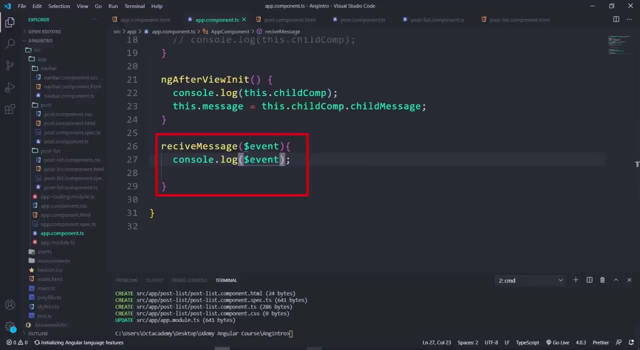 Every time we click This button. So inside this we logged the event which carries the child component's message. So every time we click this button this method will emit the variable to the event emitter. Every time this event emitter is getting active, this event inside the app component also get. 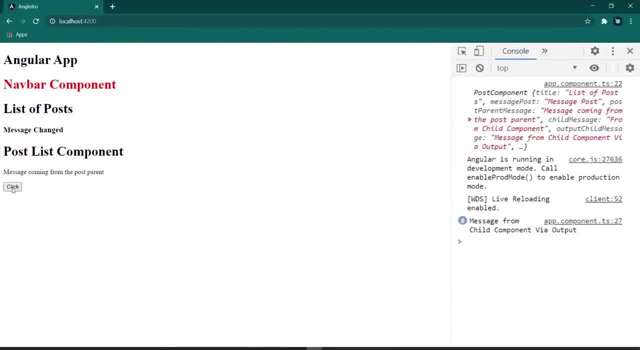 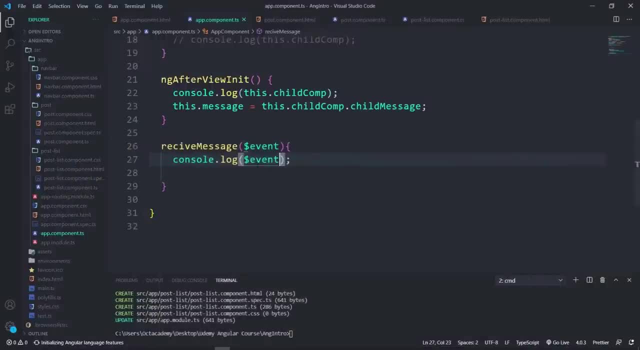 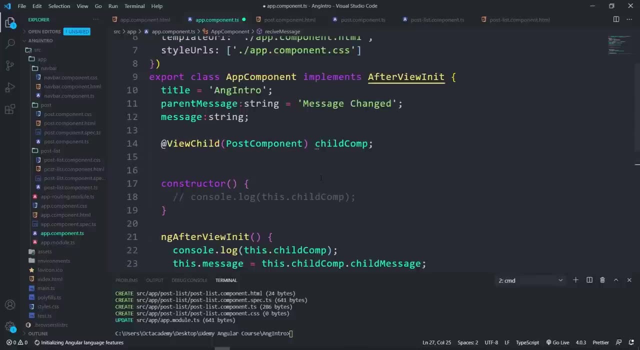 triggers. That's why we are getting this log inside the console every time I click this button. You got the idea right, Alright. next what I want to do is I want to show this child message inside the browser. For that, inside the app component ts file, create a variable from child output type is: 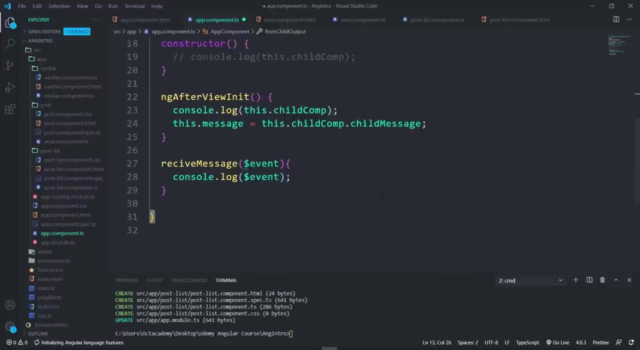 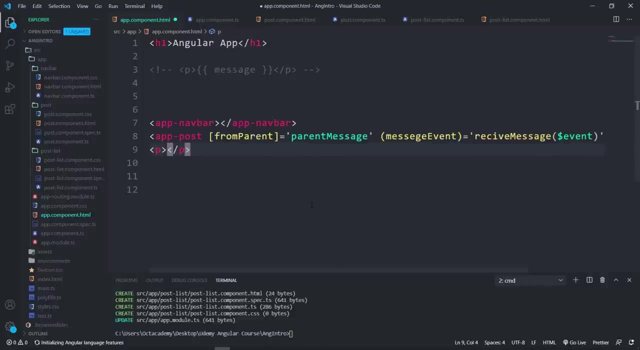 always string Now. assign this parameter event to this variable. inside this method: this dot from child output. assign this parameter event Now. I want to show this inside the browser using the string interpolation inside the app component html file. after this p tag: inside the paragraph tag: two curly brackets. inside this brackets: 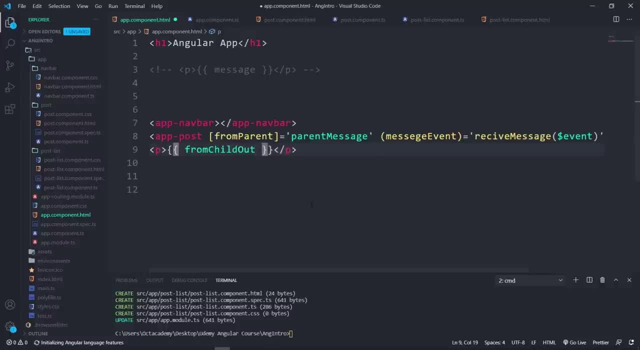 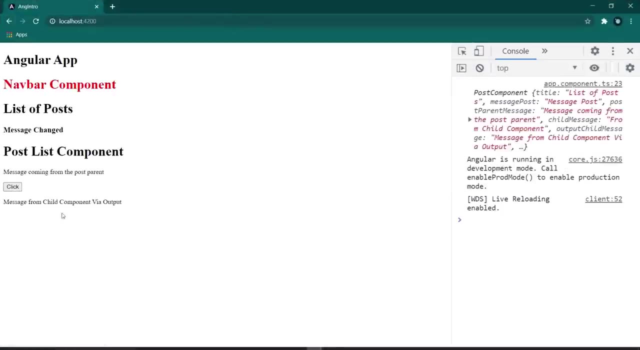 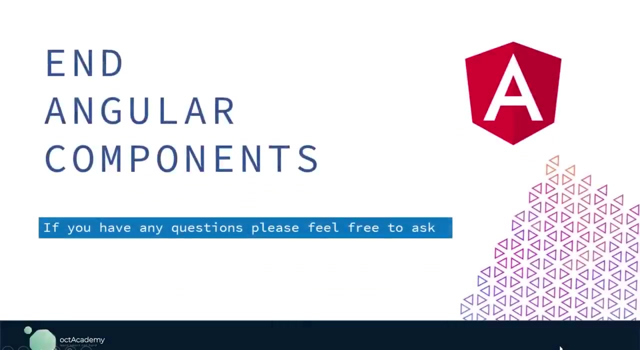 variable name is from child output. That's it. save this and back to the browser. perfect, right, we got this message inside the browser, beautiful. So this is how we share data from child component To parent component using the output decorator and the event emitter. right, this is the end. 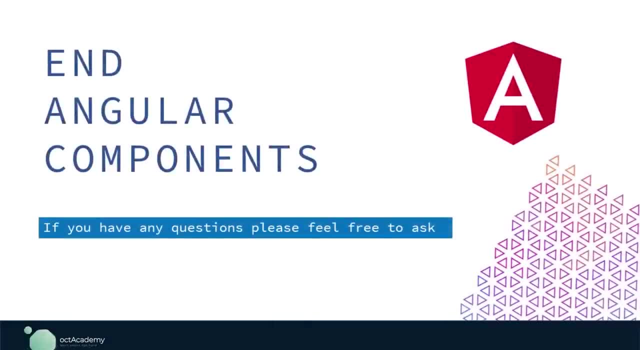 of this section. in this section, we learned all about angular component and the use cases. after this, we learned parent- child component relationship and, finally, we looked at how to share data between components for different situations, such as parent to child component using the input decorator. child to parent component using the view child decorator- child. 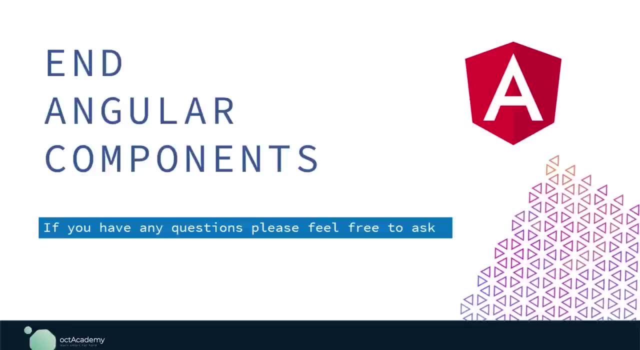 to parent component using output and event emitter when there is an event. hope you guys learned this section well. if you missed anything, go back and learn this again. if you have any questions, please feel free to ask in the q and a area. all right, this is it for this. 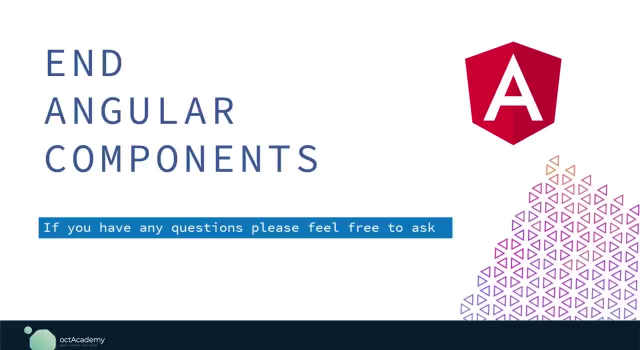 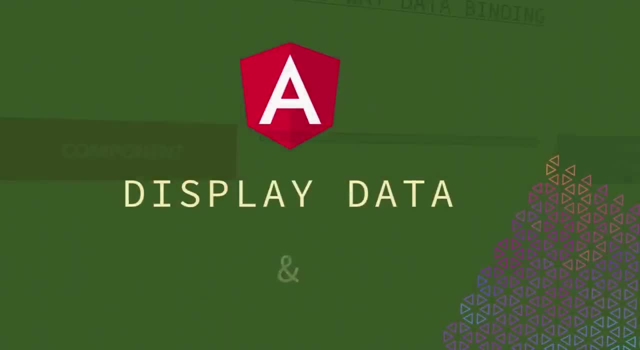 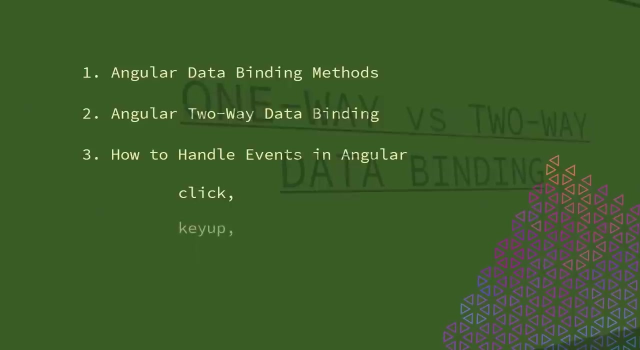 section. we'll meet you in the next section. So in this section we will look at how to display a data inside of a view and how to handle events in angular. at the end of this section you will know angular data binding methods, angular two-way data binding, how to handle events in angular, such as click key. 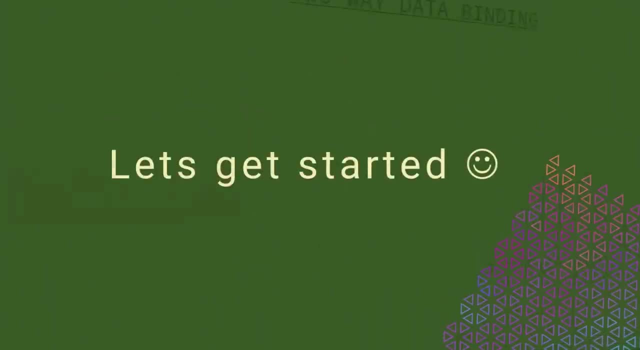 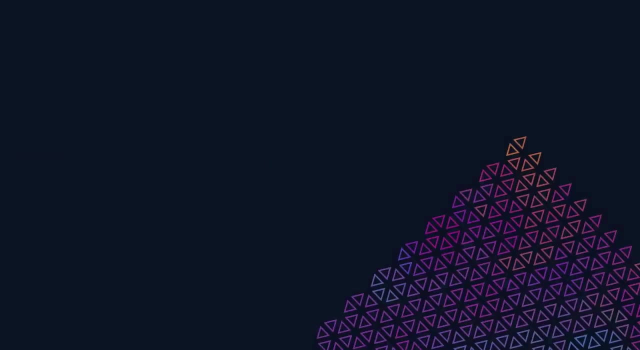 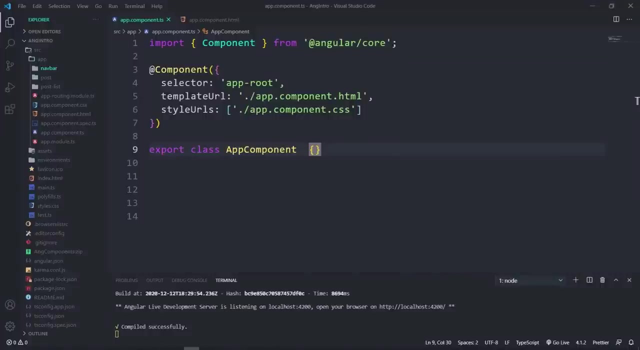 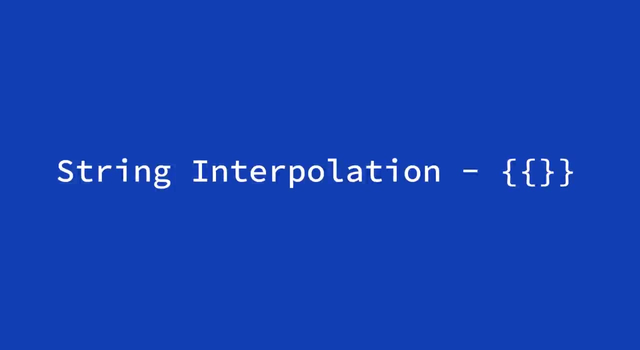 up events and event filtering. let's get started. All right, let's get started with display data. for this displaying data, we have several methods in angular, so let's look at the first method. so the first method is string interpolation. this may sound like a bit familiar to you, is it? yes, you are correct, we learned this. 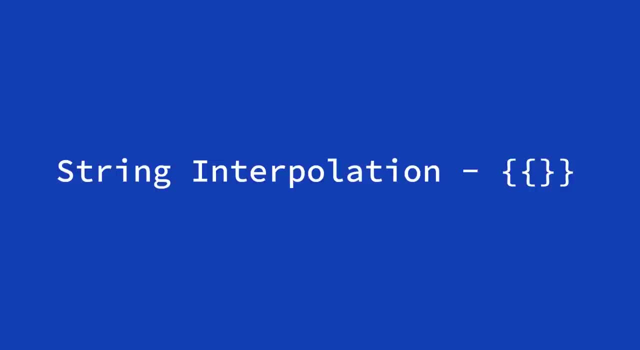 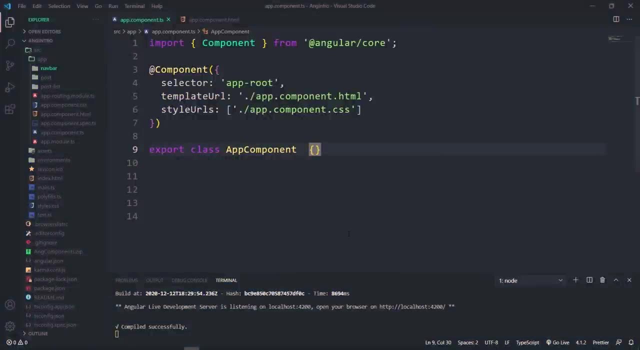 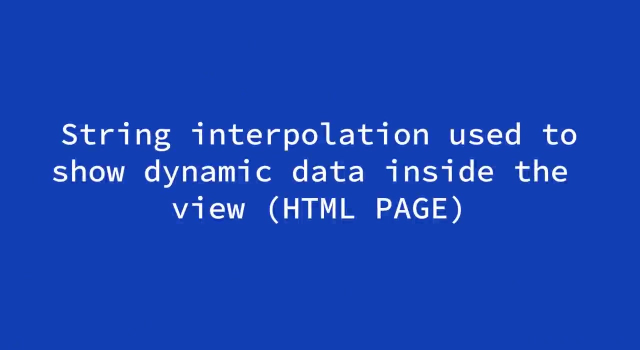 string interpolation when we learning components in the previous section. so in this section let's learn the string interpolation in detail. So what is this string interpolation? as you know, we used this string interpolation to show dynamic data on the html component page. so in the angular component we have three. 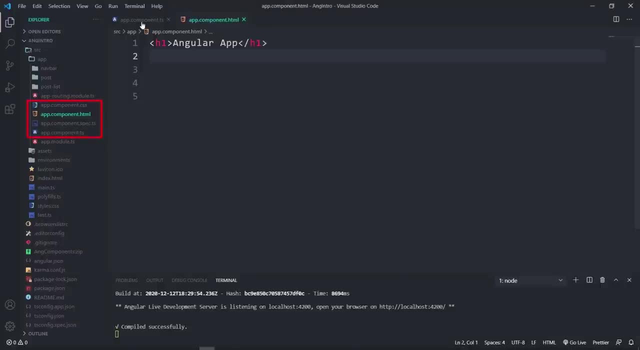 files: this html file, css file and the typescript file. so this typescript file is the main entry point of an angular component. so we do all the dynamic things inside this typescript file. So let's create a variable inside this app component file. something message, if you can. 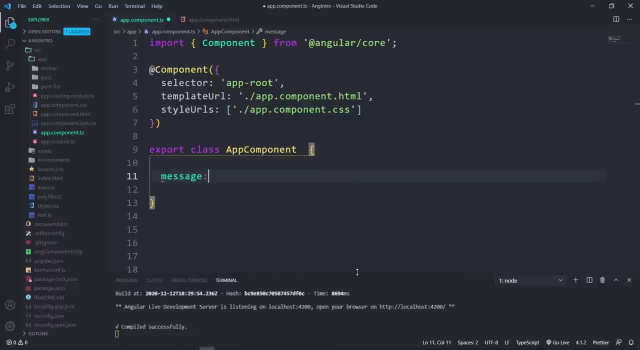 remember, in typescript we have to declare the variable type when we creating a new typescript variable. so this variables data type is string. now assign a value for this something. message from the typescript component file. Now I want to show this message to the app component. 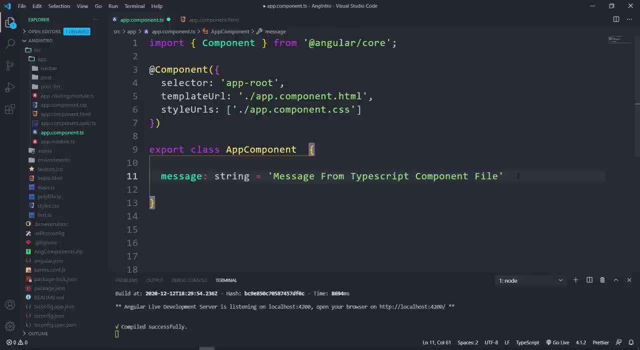 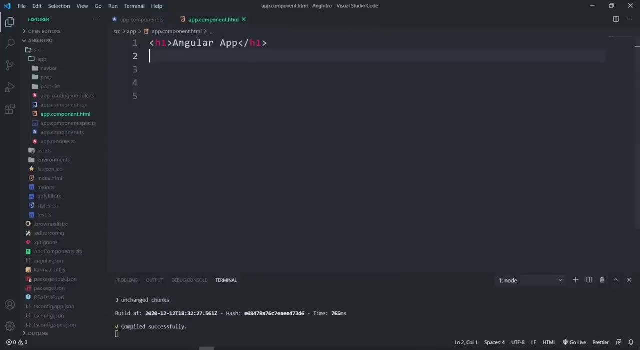 to the end user. The browser shows only the HTML page to the end user, not the CSS file or this TypeScript file. So in order to show this TypeScript variable inside this component HTML page, we use this string interpolation approach. So let's see this in action Go. 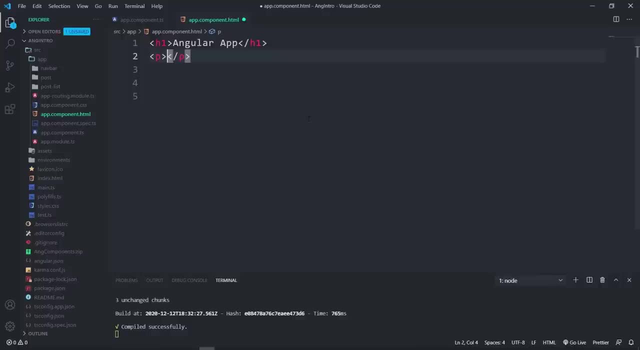 to the app component HTML file Down here. create a p tag Inside this. let's show this message variable. inside this p tag, The variable name is message. So what do you think, guys? Is this correct? Yes, this is wrong. Why is that? because this variable is a TypeScript. 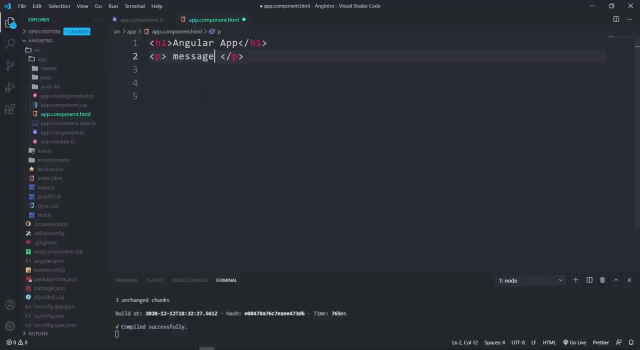 variable. So first we have to create a TypeScript scope inside this HTML page. you guys know, inside HTML page we can write inline CSS using the style tags. So between the type tag and the variable name inside the p tag we have to be able to copy. 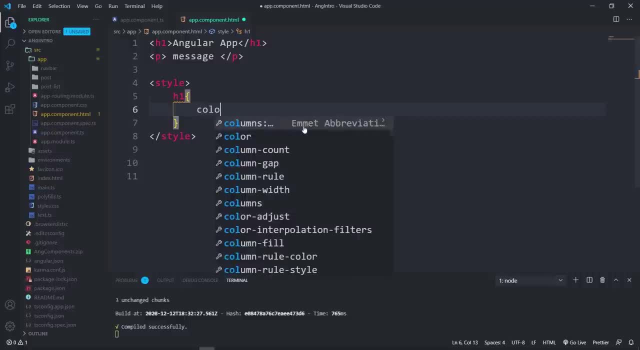 this tag. we can only write css coz. now this scope is a css scope, not an html scope. if i write html inside the scope of this style, this won't work. you got it right like this. if you want to write some logic in javascript, we have to create a javascript scope inside. 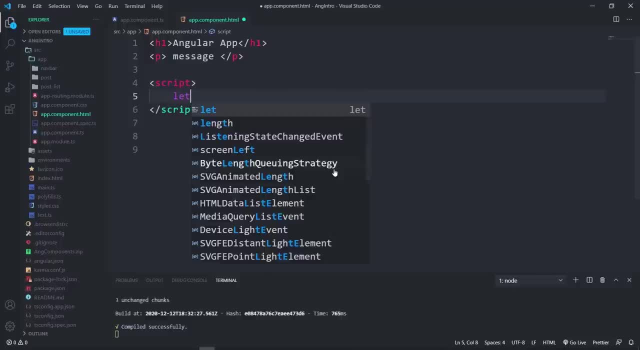 this html page. so we do that using the script html tags. so between this we can write any valid javascript logics, so like this: in order to show this typescript inside this html file, first we have to create the typescript scope inside this html file. for that we use these: 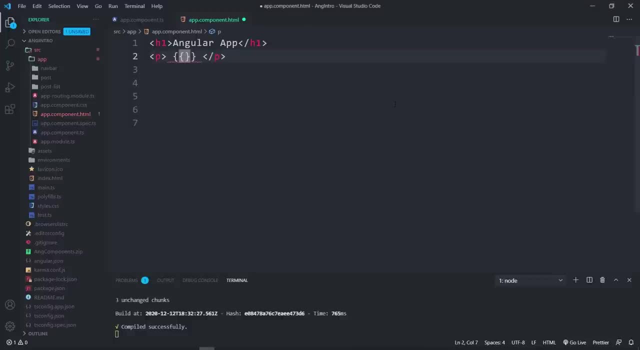 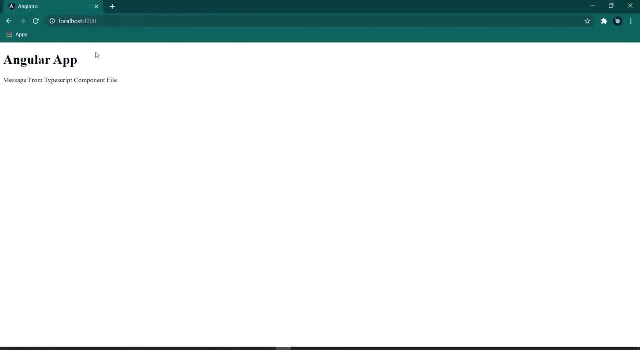 two curly brackets. so open and close two curly brackets. alright, now inside this place, this various typescript scope, inside this html file, we have to create a javascript scope table name message. now save this and go to the browser. perfect, as you can see here, we got this message printed here. so inside this scope we can add even simple calculation something. 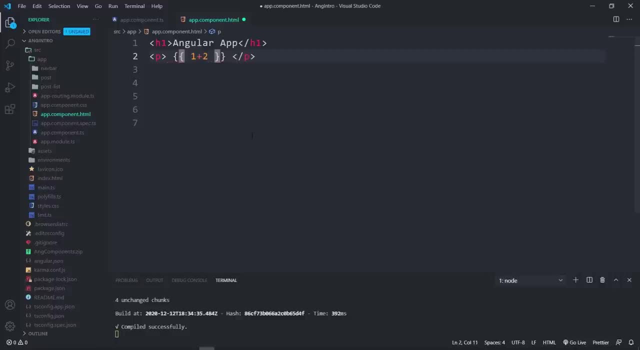 like this: 1 plus 2, save this and back to the browser. perfect, right, we got this 3 printed here. so with this curly brackets, we are creating a kind of a typescript scope inside the browser, so we call this string interpolation. using this, we can show data inside of an html file, which is declared. 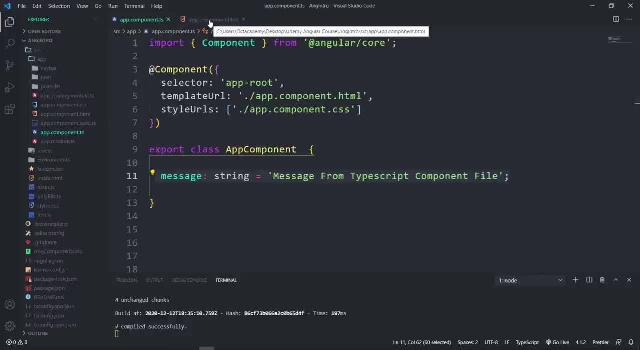 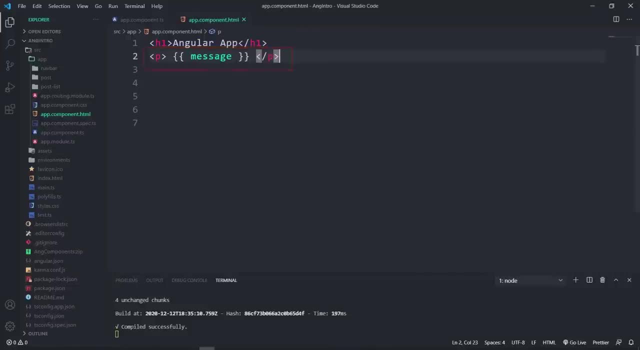 inside of the component file. when the angular compiler sees this string interpolation, this will automatically look inside the relevant component file and print this relevant variable data inside this html tag. so with this we can show any type of data to the user. and this name is string interpolation, but we can show numbers and boolean values inside. 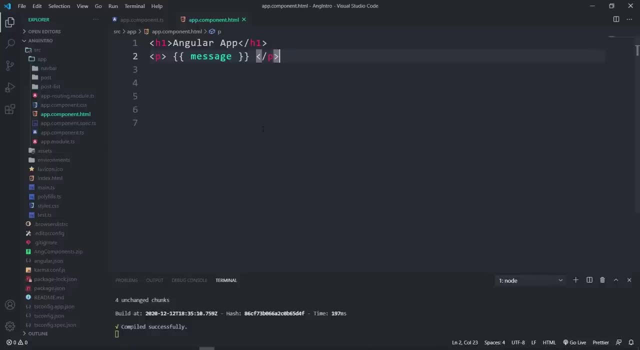 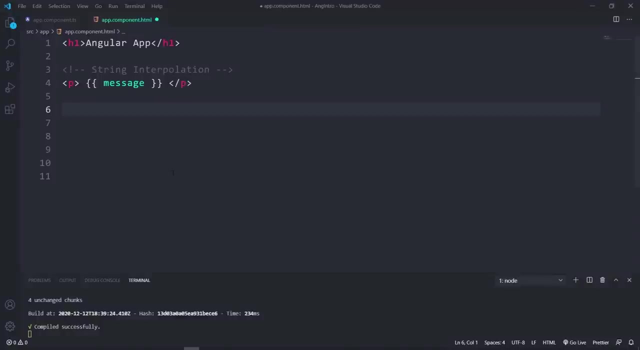 this string interpolation so don't get confused with this string name. okay, once again to show a variable data inside the browser. we use this special type of syntax string interpolation in angular. hope you guys got the idea. you in previous we learned about string interpolation in this video. let's look at the property binding. 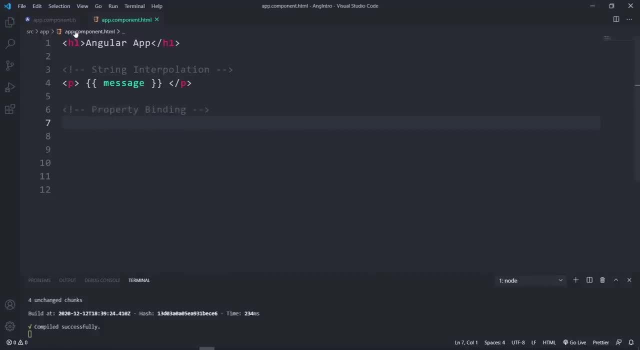 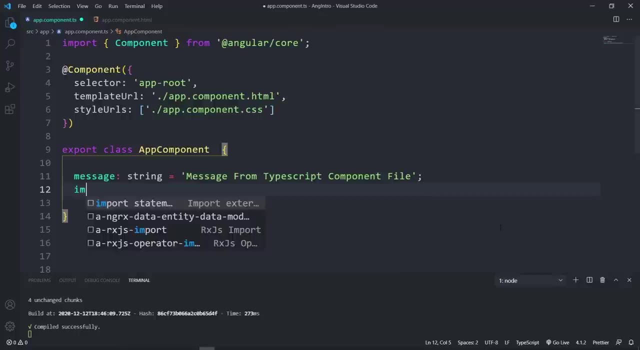 think there is an image in our data base and we got that image path to a variable inside this typescript file, something: image img url. this u is capital, the variable type is string and the value will be something. for now, let's add an image path from google, something like: 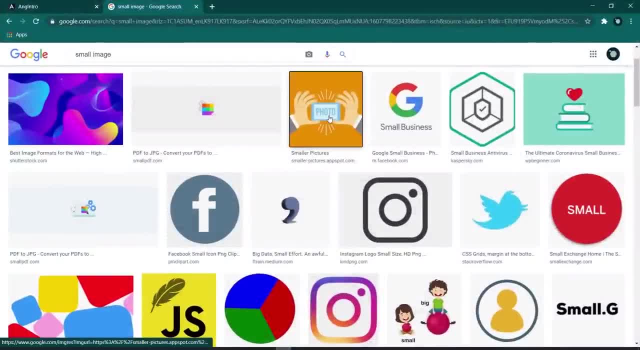 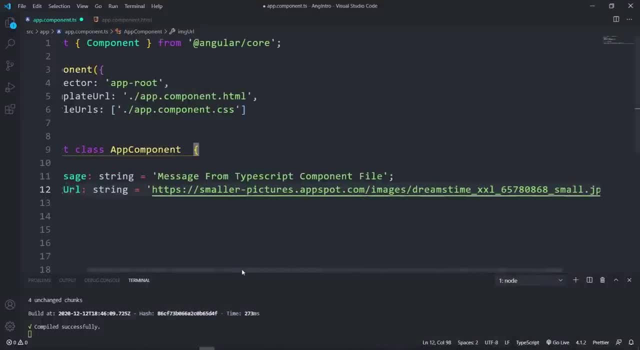 this. so let's add an image path from google, something like that. this will be an image search for an image. copy the url and paste it here. for now, we just think we are getting this from our database, alright. next, i want to show this inside the browser. so how we 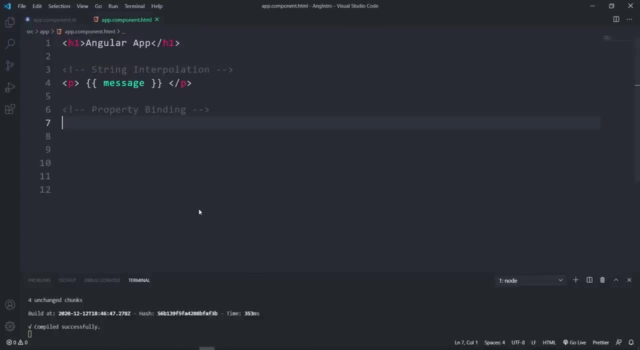 going to do that. if you want to show anything inside the browser, we have to add that inside the html page. so go to the app component html file. we want to show an image, so create an image tag: img, hit, enter, alright. next, for this src, we have to pass the image path. we. 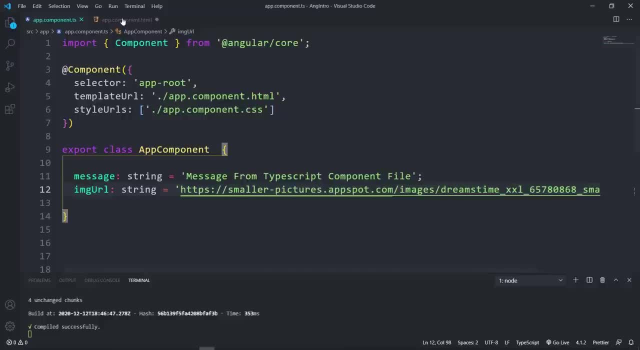 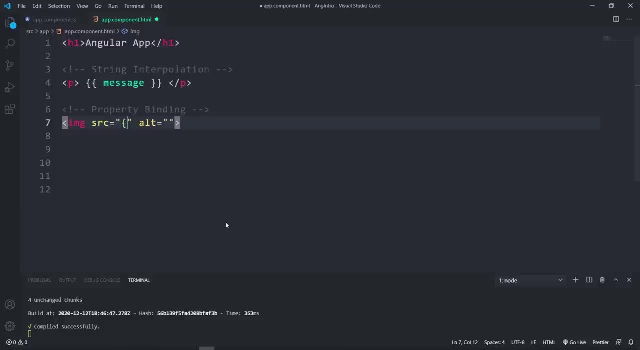 have this image path inside this typescript file so we can pass that variable to this src using the string interpolation. so inside this src codes double curly brackets. inside this brackets the image src variable is string interpolation. this img url now save this and go to the browser. beautiful, we got this image inside the browser. 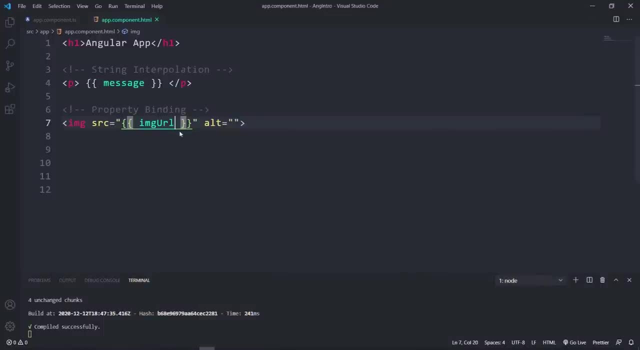 so like this: we can pass dynamic values for html properties using the string interpolation. but in angular we have a different and cleaner approach for this dynamic property values. we call that property binding. let's see this in action. this is very easy. you just copy and paste this img tag after this. now let's change this string interpolation. 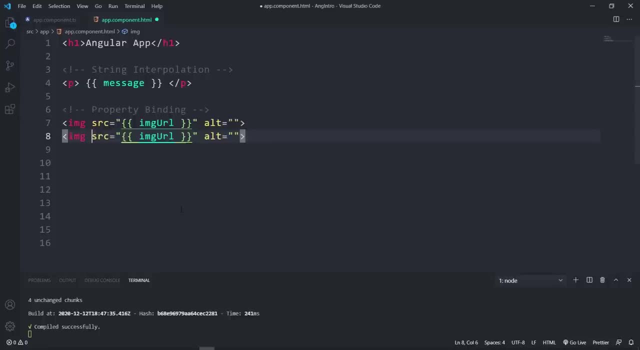 to property binding. wrap this src property with square brackets. now remove this string interpolation, curly brackets and keep this img url variable. that's it. this is the property binding in angular. so look at this syntax. this property binding is more cleaner than this string interpolation. give it a name to this, if ok. here let's change this src property. 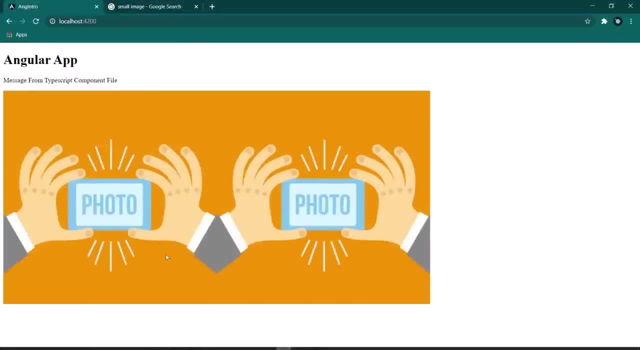 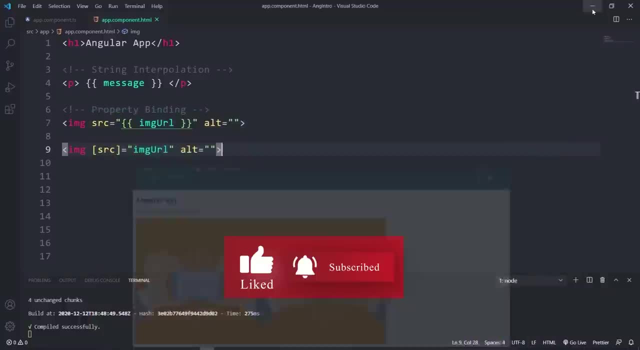 right, Save this and back to the browser. We got this image here, which means this property binding is working perfectly. This string interpolation is working for this, but we used this property binding coz this will give us some cleaner code. And another thing: when an angular compiler compiles this component, this string interpolation property is going. 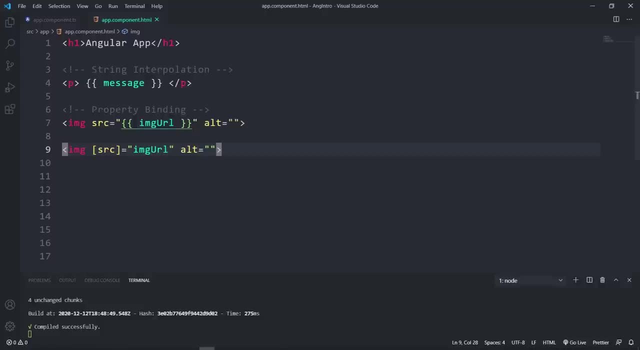 to be automatically compiled as this property binding. No matter what you are using, at the end of the day this will compile to this property binding method. So in my opinion, this property binding approach is better than using this string interpolation approach. So usually we use string interpolation to bind data inside of a tag, For example like: 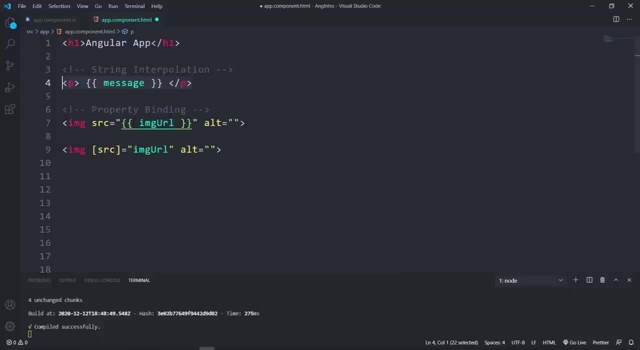 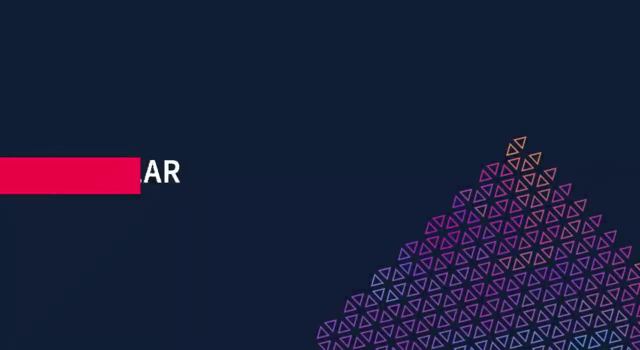 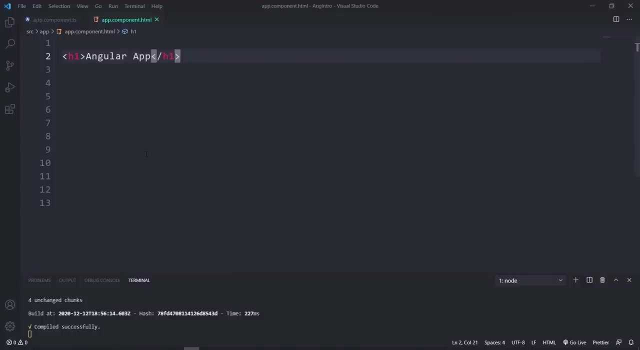 this heading tags, paragraph tags inside of div tags, And we use this property binding approach to bind a property of an HTML tag Like this image src tag. Hope you guys got the idea Alright. in the previous lecture we look at property binding, So in this video lets look. 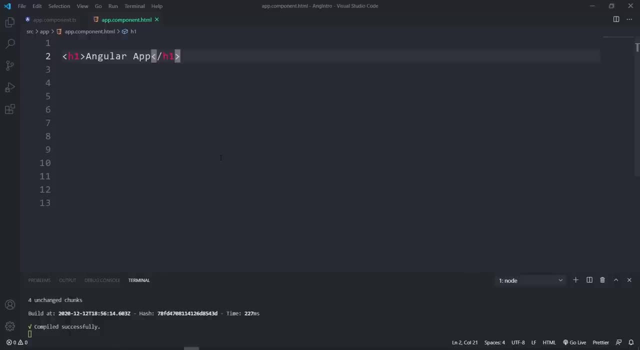 at how to bind a css class 1 HTML element. So we have this heading tag inside this app component HTML. Now I want to change this color to something red color, So I am going to change this color to something red. So normally we change this color using the css. 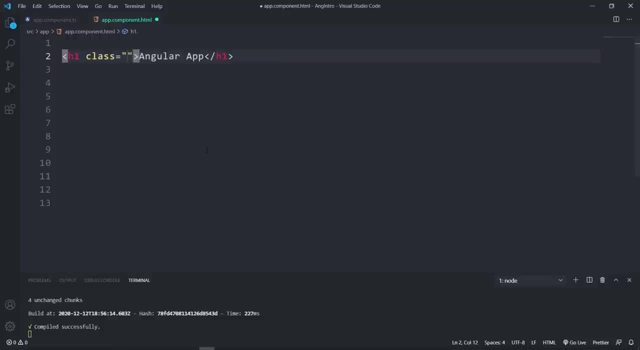 First we will add a class to this Class. Class name will be something text dash red. Save this file. Now open the appcomponentcss file Inside. this lets add this style. So first the css selector, The class name is text-red, Then css scope. Next we will change. 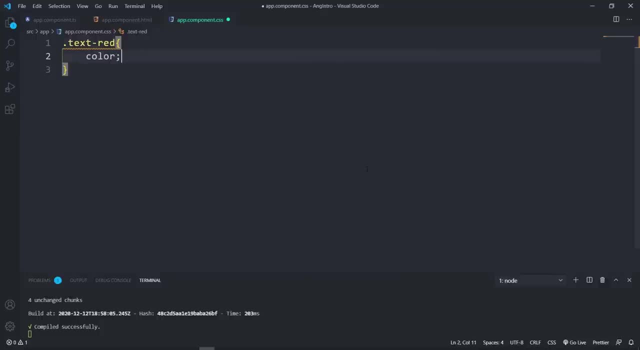 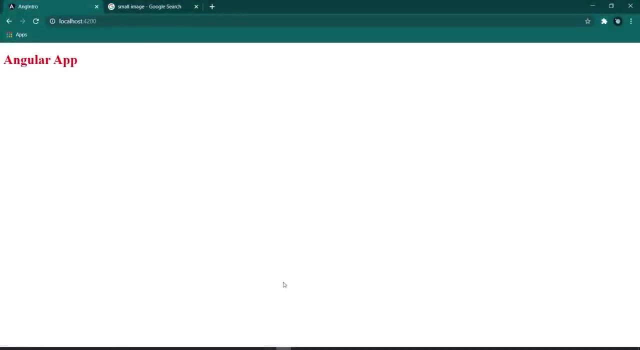 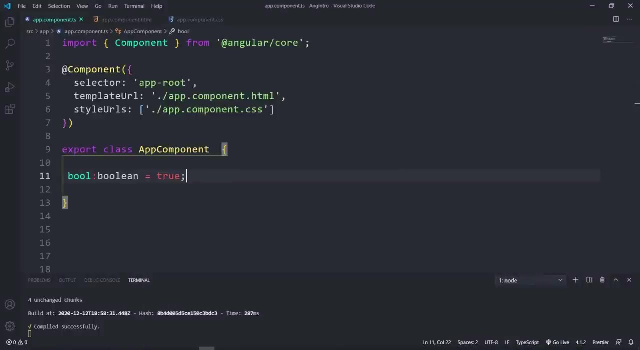 the style. Next, write the style inside this scope, Color, colon, and color will be red. Save this and back to the browser. As you can see here, this h1 tag is now red. Perfect, Alright. now what I want to do is I want to make this h1 tag red color when this boolean. 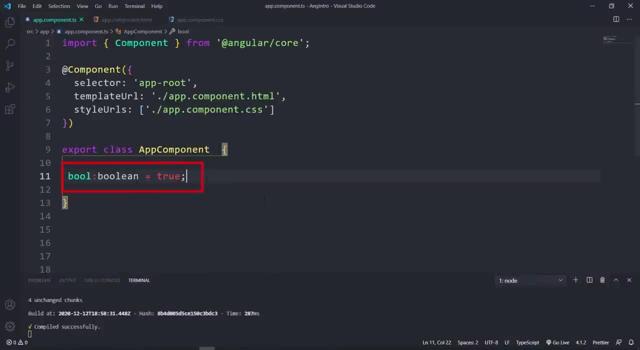 value is true. For that we are gonna use the angular class binding method. So I am going to use the angular class binding method. So lets do that. Remove this class attribute. This also same like property binding. So first square brackets. Inside this brackets we are: 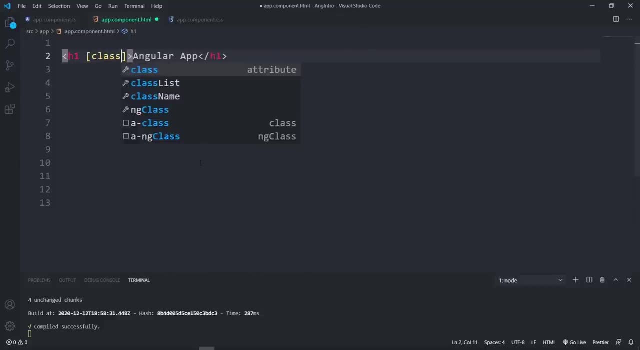 trying to bind the class property, So class. after this dot symbol. Then give the css class name: Test dash red. So now I want to apply this red color to this text. when this boolean value is true, Lets add the condition after this equal sign Inside quotes: give the boolean variable name. 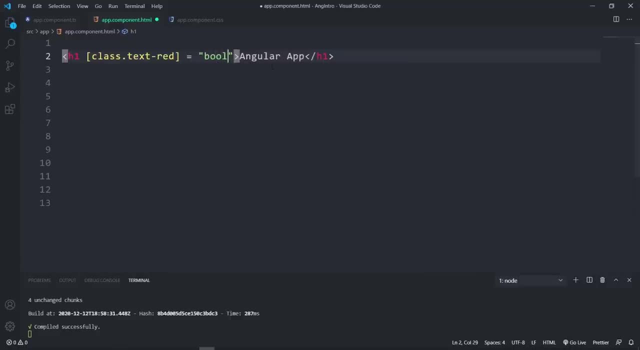 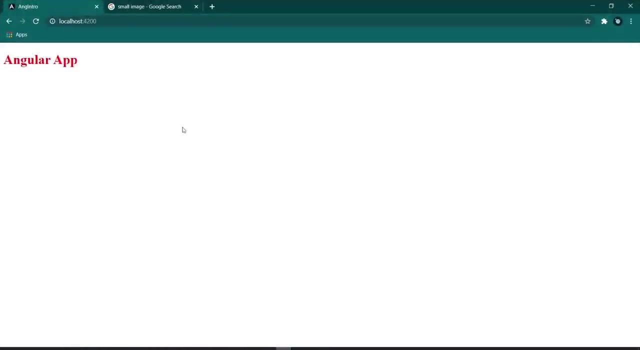 here B O O L bool. That's it Now. this red color will apply when this condition is true. So we already created this css inside this css file, So save this all and back to the browser. Perfect, As you can see here, this text color is now red If I make this boolean. 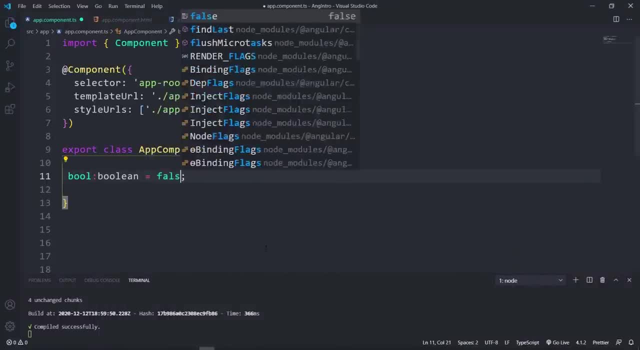 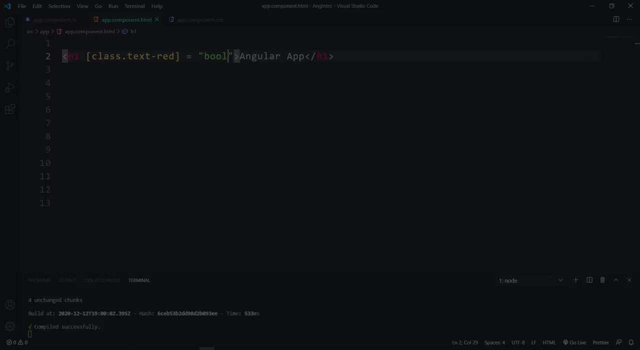 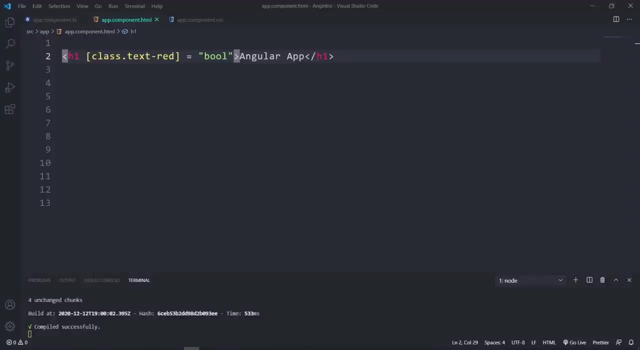 to false. Now look at this. This color is black Coz. this condition is now false. Hope you guys got the idea. So this is how we conditionally bind css classes to an html element using class binding in angular. Alright, Now we know how to bind a css class to an html element with the condition using: 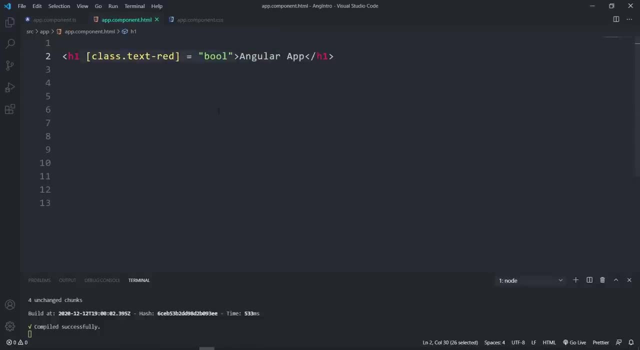 the class binding approach. In this video, lets see how to bind an inline css style with the condition to an html element using the style binding. This also a variation of property binding, but similar to previous class binding. Lets see this in action For this style binding. 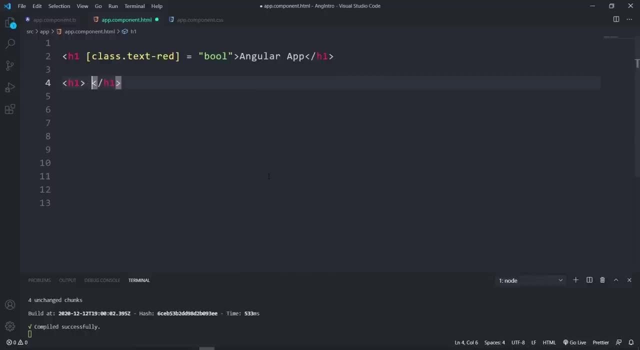 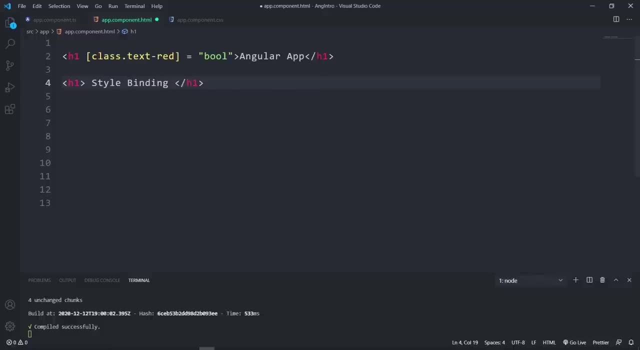 mentioned earlier. this also same as the class binding. So inside this h1 html tag, First square brackets Inside that. This time we are binding an inline style. So first style. After this we can pass any properties of the style object in DOM. So this is bit different. 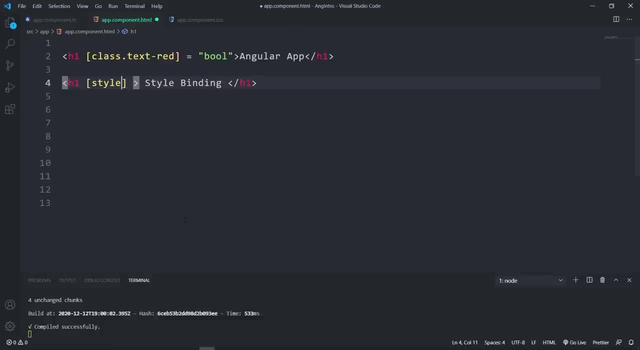 than regular css. For example, if we want to add the background color in CSS, we add that something like this CSS property is background-color, then the color value. But if we are passing this as a style binding, we have to use the HTMLDOMStyleObject property. 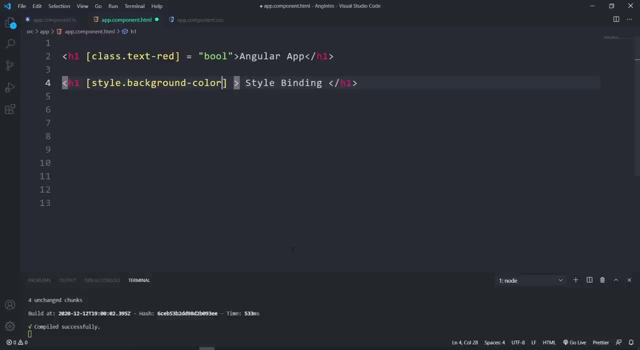 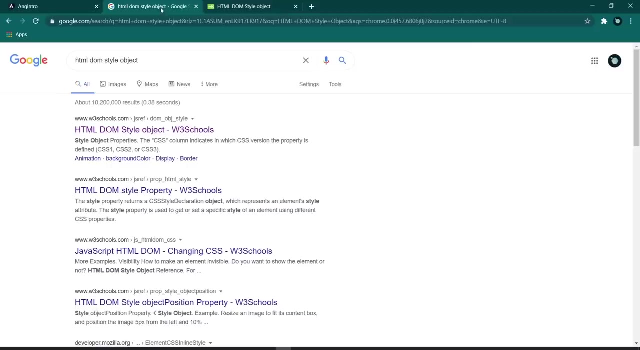 which is a bit different than the regular CSS property For this background color. we have to pass background this time. no dash, Just type color with the capital C. That's it. Go to the Google and search HTMLDOMStyleObject. Go to this first result: w3schoolscom. 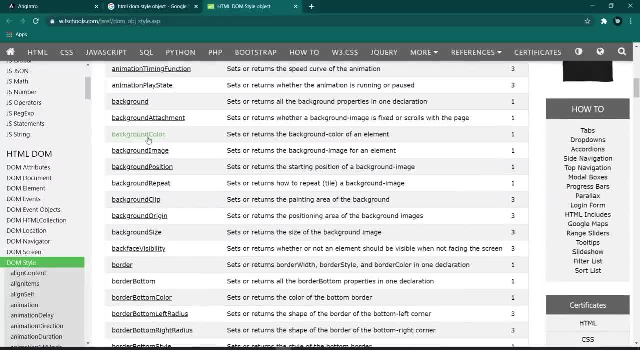 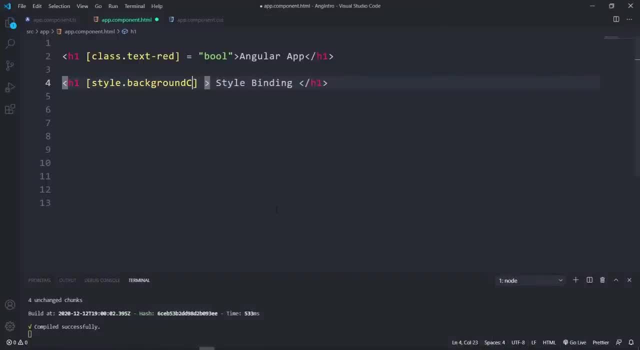 In here you can find all the DOM object properties of this style object. So alright, back to the work In here. I don't want to add a background color, I just want to change this text color to red. So the style object property is same as. 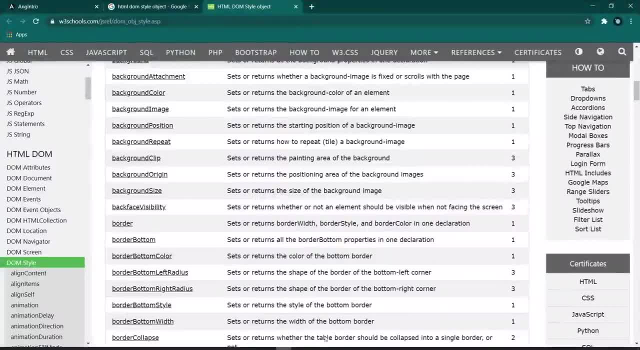 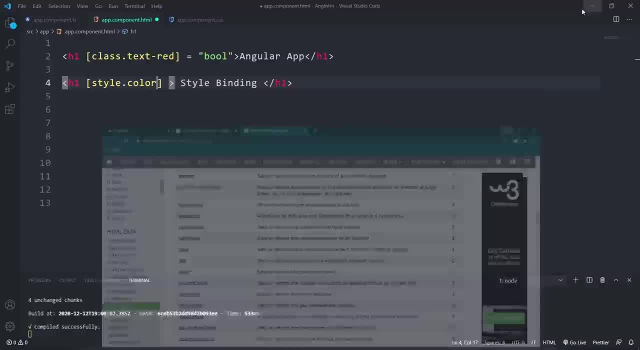 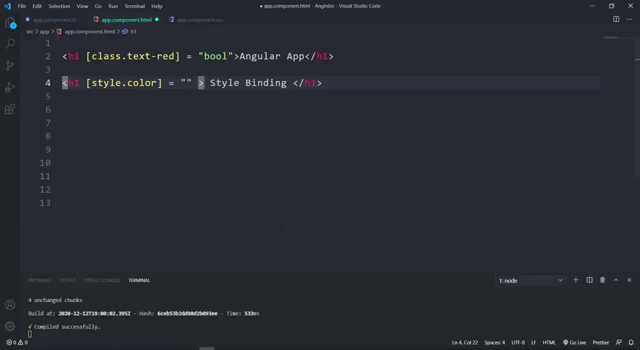 CSS property color. You can find this on this website. So after this, we gonna check this bool value is true or false. So after this equal sign double quotes inside this pass the argument bool. This is this boolean value. 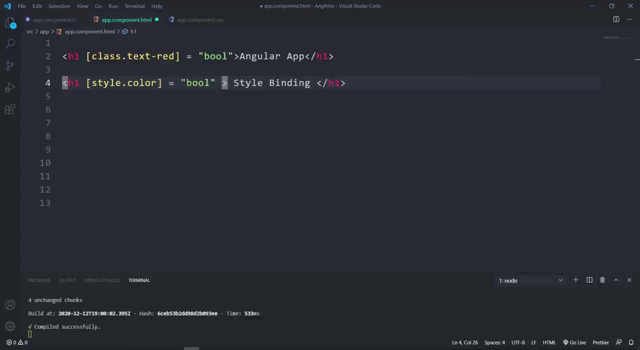 Okay, next we have to pass the CSS value. So if this argument is true, Set this color to red. If this is true, we define that using this question mark. So question mark after this single quotes and value is red. 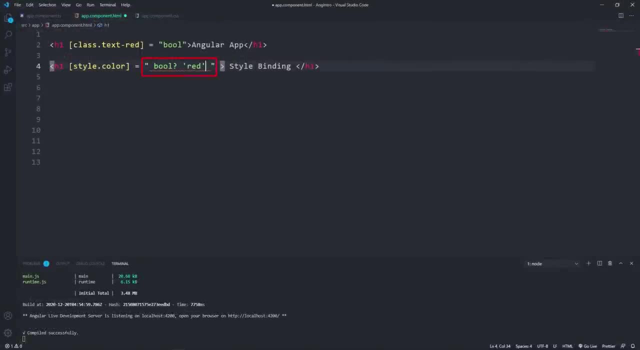 So this is not done yet. As you can see, here we are getting a compile error. Why is that? Because this argument required the else part as well. So after this colon sign, we use this question mark for the if statement. 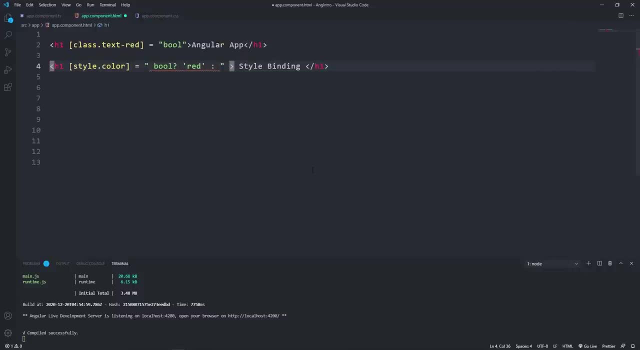 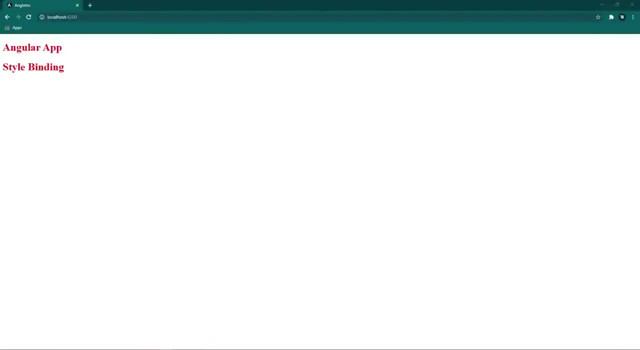 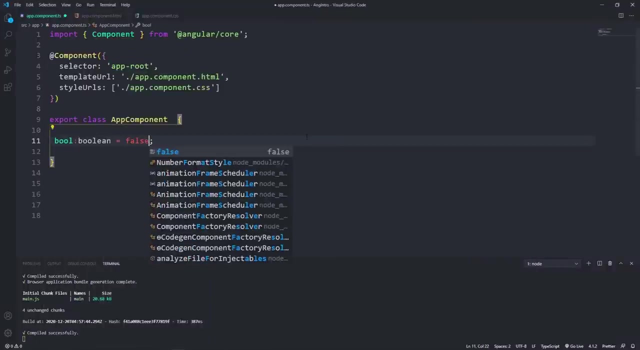 And for else we use this colon symbol. So after this, for now just pass an empty value. That's it. Save this and back to the browser. Perfect, Now this color is red. If I make this boolean value to false, this time, this h1 tags color is back to the default. 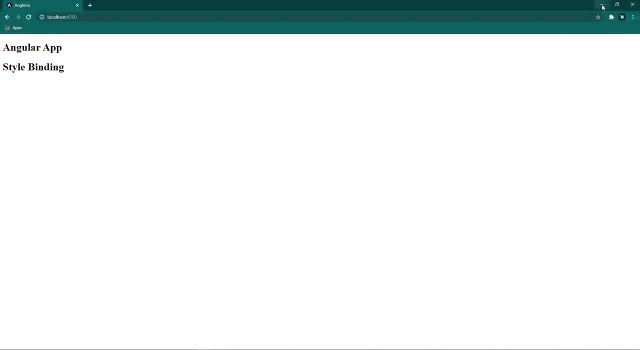 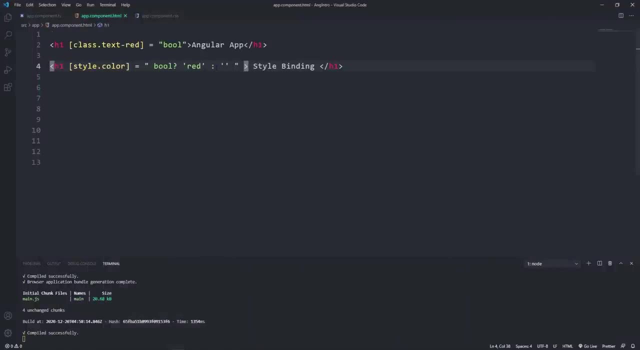 black color. Think: if you want to change this text color to something blue color when this boolean value is false, how do you going to do that? Very simple: We can define the else inline using the colon sign. We already added this. 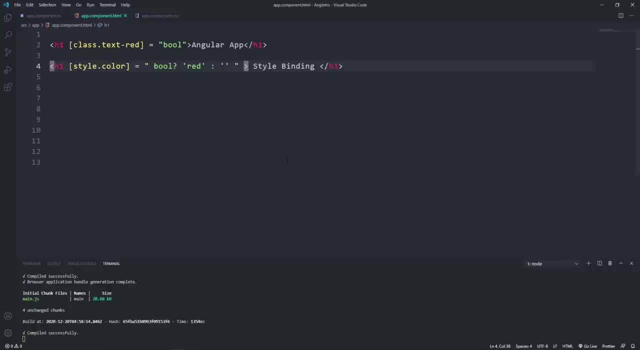 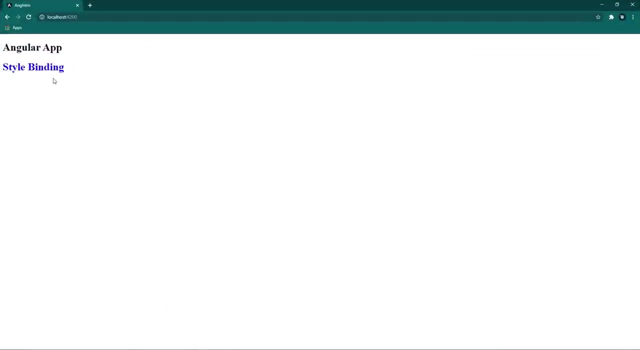 So, after this colon sign, inside single quotes, pass the color that we want to change. This time I want to change this color to blue, So pass the blue value inside this quotes, Save this and back to the browser. Perfect, right Now this h1 is blue. 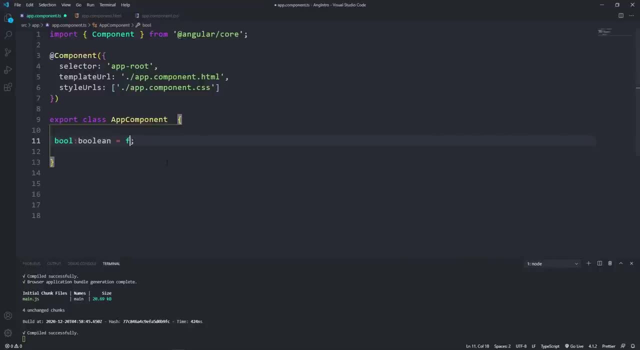 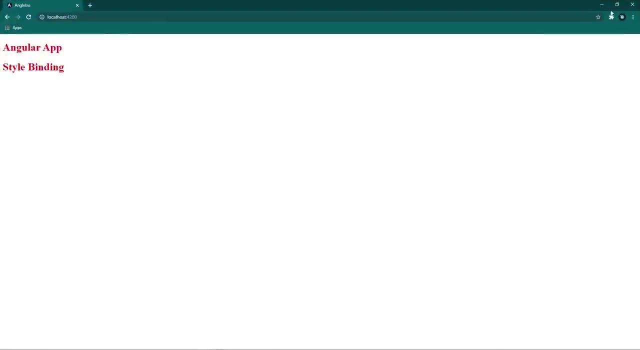 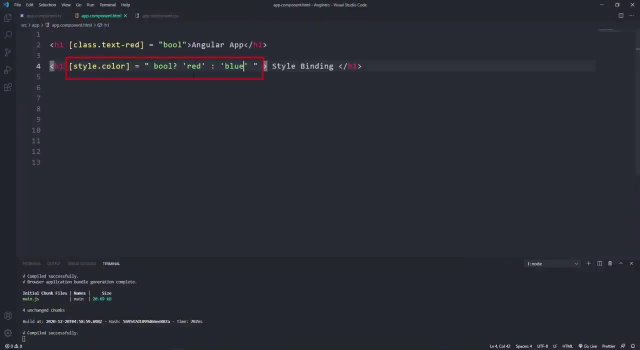 Because this boolean value is set to blue. Set to false Again. change this to true, Save this and back to the browser. As you can see, now this text is in red color. If we recap this quickly in angular, we can bind style to an HTML element using this style. 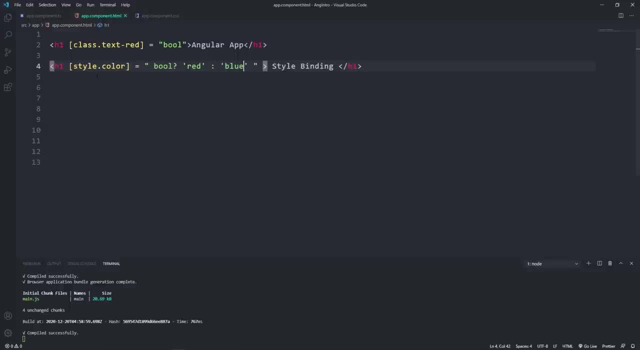 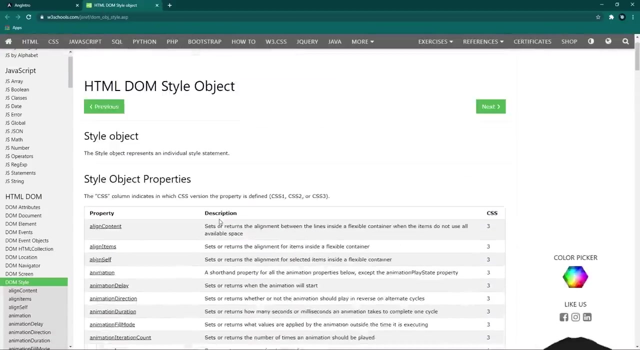 binding method. Inside square brackets we pass this. First style was: this is a style binding. Next, the DOM style object property. So, if you can remember This, CSS DOM object properties are bit different than regular CSS properties. You can find list of this style DOM object properties in this w3 school website. 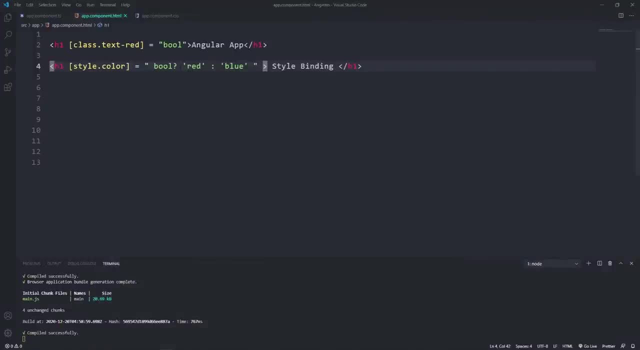 So I pass the color property Because I want to change this h1 color if this boolean value is true. So after this, assign inside double quotes the argument which is this bool: if this bool value is true, set red color. This is what we defined with this question mark. 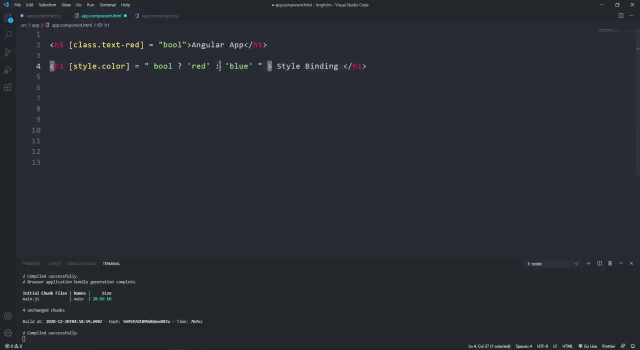 Okay, if this is not true, set the color to blue. We defined that using this colon symbol. This is something like inline if else. We defined if with this question mark and else with this colon mark. That's it, Very simple, right. 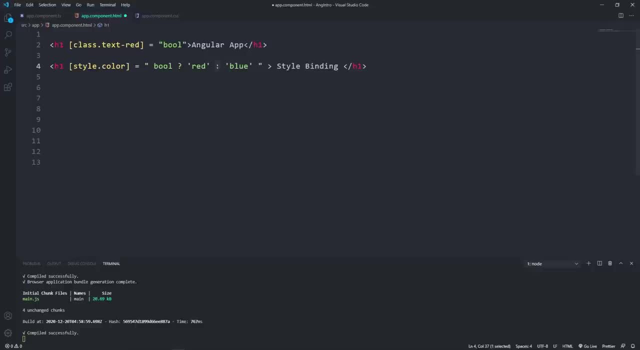 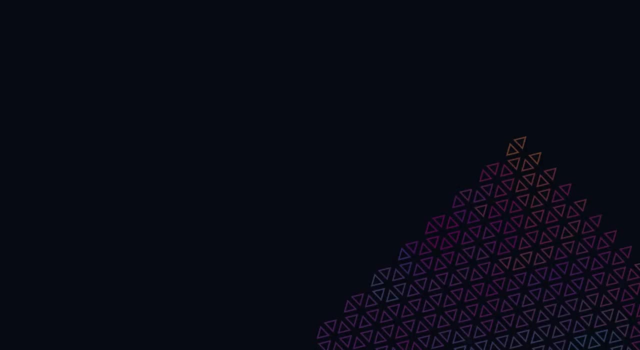 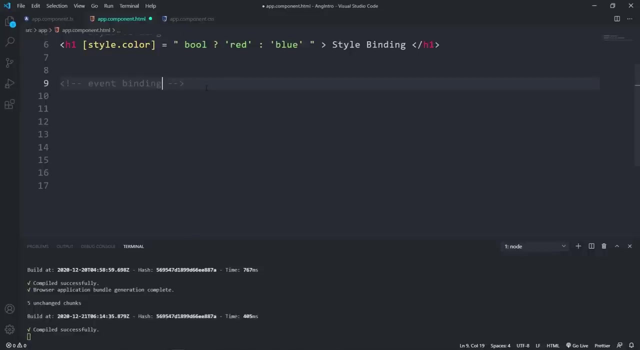 So this is how we do style binding in angular. Perfect, Alright. in this video, let's look at how to bind an event in angular using the angular event binding approach. When a user interacts with a web application, such as a keyboard keypress, a mouse click, 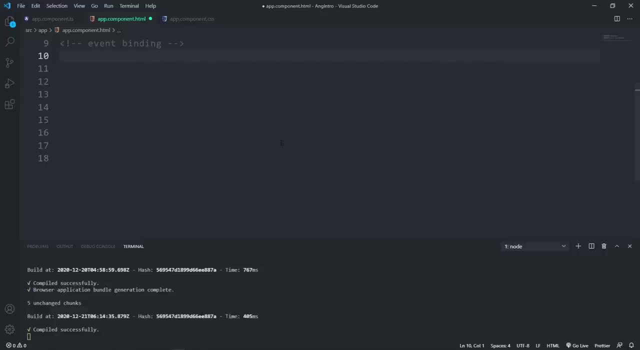 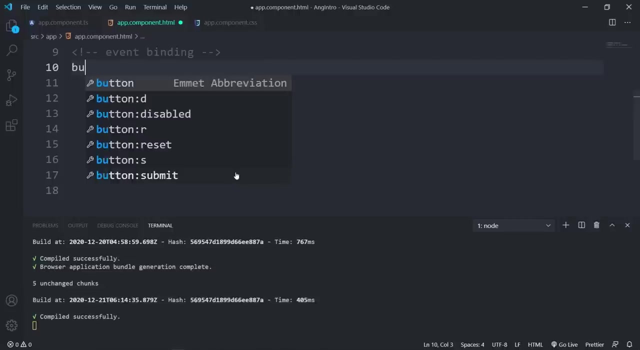 or a mouse hover, it generates an event. These events need to be handled to perform some kind of action. This is where this action happens. This is where this angular event binding comes to action. Alright, first let's create a button inside the app component html file. 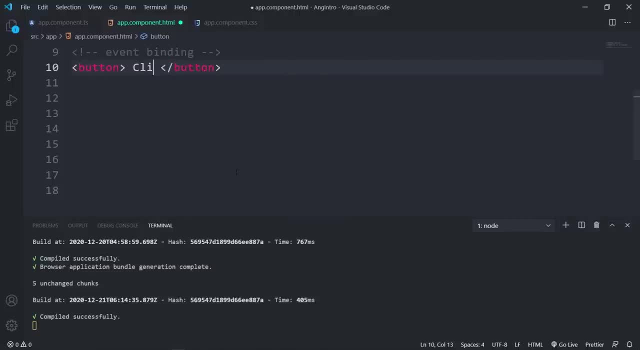 After this button text, hit enter and button text will be something: click me. Now let's bind the click event to this button. In plain javascript, we do something like this On click. Then we pass the javascript function that we want to execute when this button is enabled. 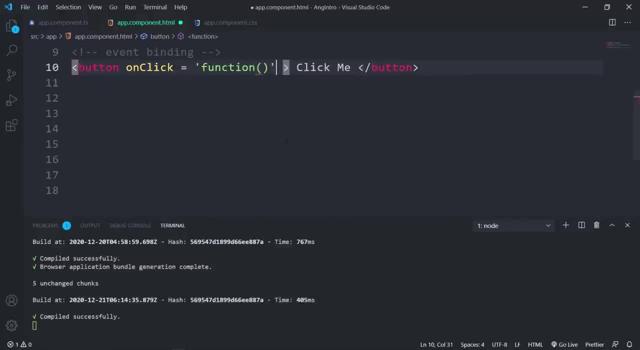 Then click. So this is the traditional way, but in angular we have a different and more cleaner approach, which is angular event binding. Let's do that. Remove this javascript on click. If you can remember, we used square brackets for data binding, But for event binding we use this normal brackets. 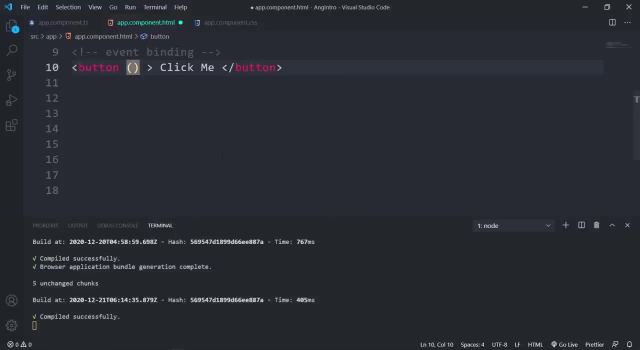 So don't get confused: For a data binding We use square brackets, and for an event binding we must use normal pair of brackets. So otherwise this click event will not work. Alright, brackets Inside of this bracket pass the event name. So, as I mentioned earlier, I want to bind the click event. 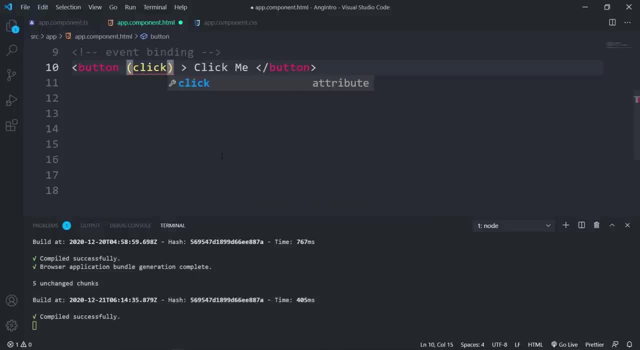 So the event will be click. All simple letters. In plain javascript We use on click event, But in angular we use just click. event name, Simple, Right After this, as usual, equal sign And pass the target method name inside of this quotes. 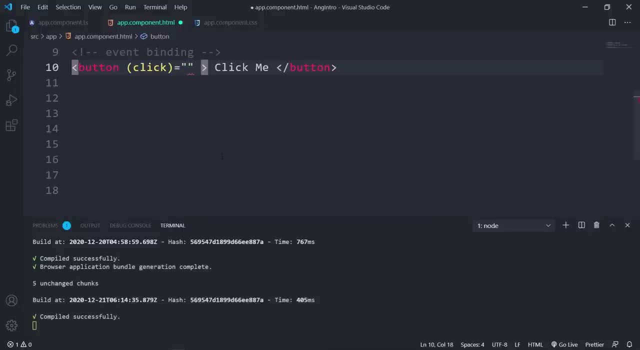 In plain javascript we pass the function name here. But in angular- you already know angular use typescript instead of javascript. So in typescript we can create methods. So we pass the method name here, Button click and the parenthesis This c will be capital. 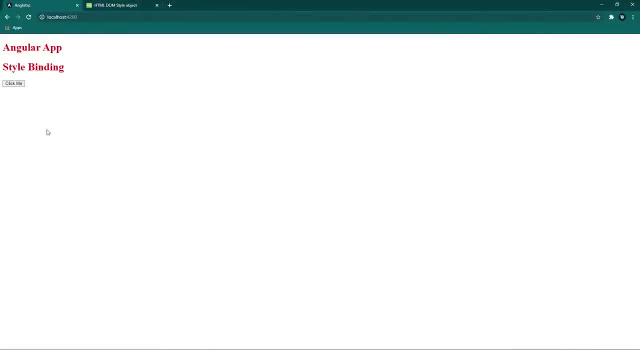 Now save this and back to the browser. Click this button. Look at the browser console. In case if you forget how to open the browser console, Right click and select this inspect element. After this, go to the console tab Or you can use the keyboard shortcut. 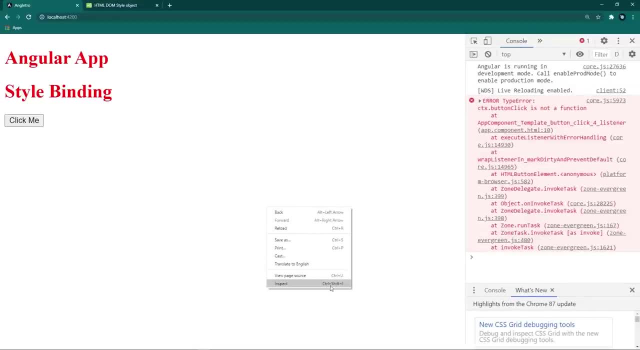 Shift Control I And go to the console tab. So in the console we are getting an error. What is this error? This error saying that this button click is not a function. Why is that? Can you guys guess? Yes, ofcourse. 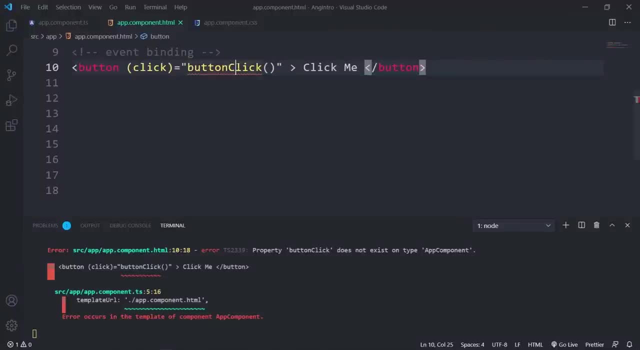 We just only link this method to this click event, But still, we don't have this method initialized or created inside this component class. That's why we are getting this error. To solve this error, Let's create this button click method inside the app component file. 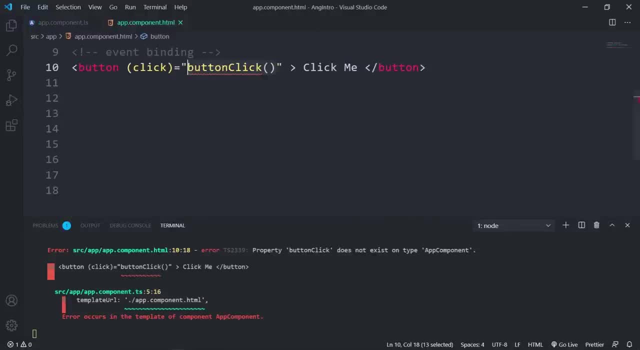 Right, Wait, before that I wanna show you something. You guys may be noticed this. So look at this. We got this compile error that saying this button click is not defined. Not only that, Look at this internal terminal window. We are getting the same error and also we are getting the line number as well. 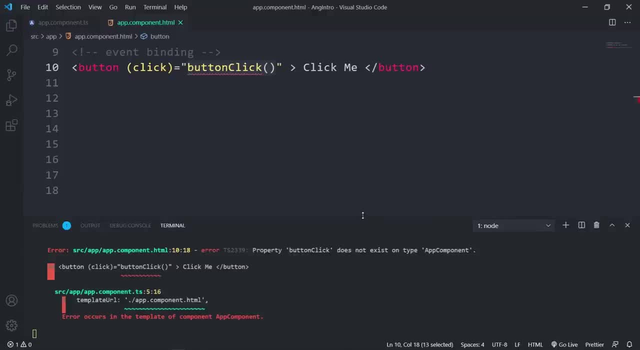 See how this is easy to debug the error. This is the beauty of typescript: We can get the error on the stage of compile. We don't have to wait until the runtime of this app to identify the errors. Alright, get back to the work. 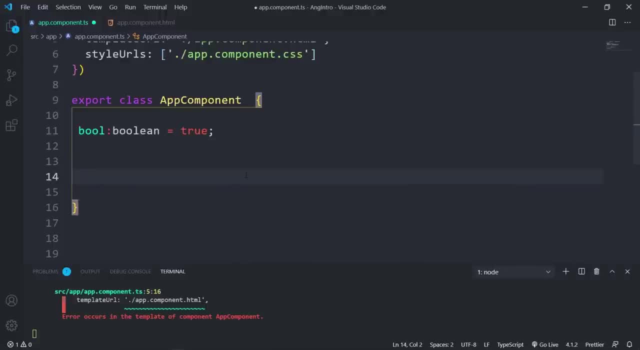 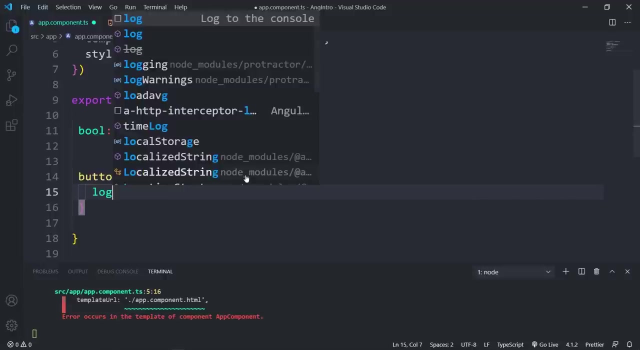 Go to the app component ts file and create the button click method Inside this class scope. the method name is button click. This c is capital. After this parenthesis and the method scope Inside this method, let's log a simple message. Button click event worked. 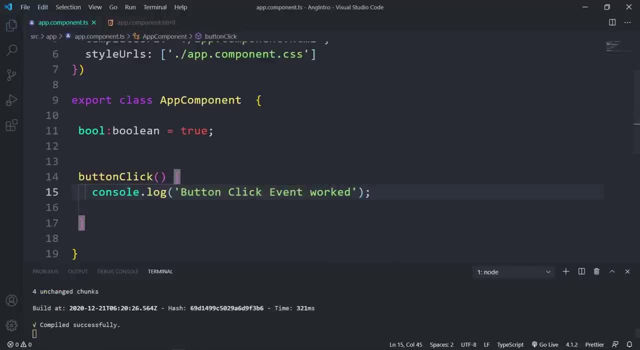 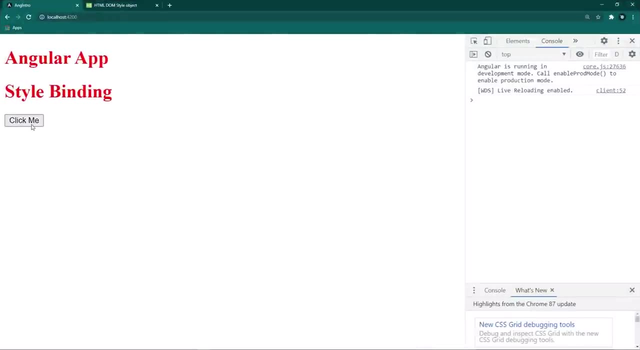 Done, Save this file. Now look at this This time. we are not getting any compile errors. Perfect. Go to the browser. Now click on this button. Look at the browser console. We are not getting any errors like previous. If we look further, we can find this button: click event worked log printed inside the 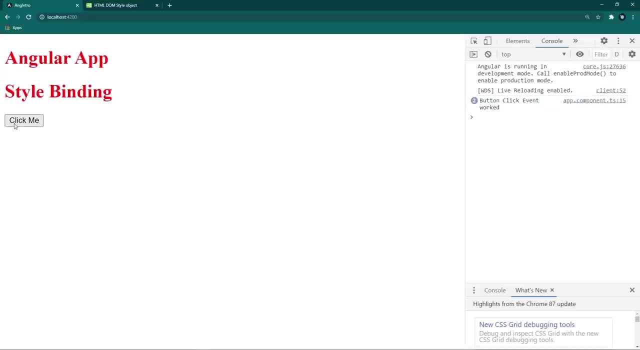 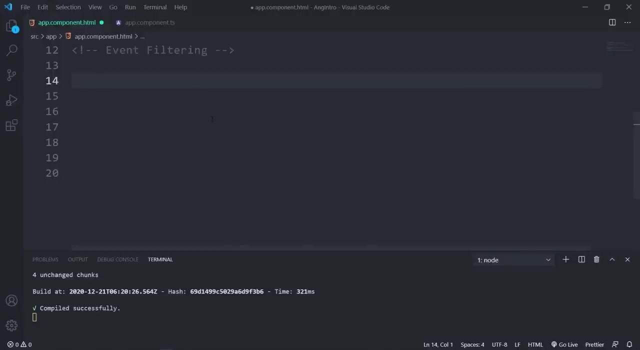 console, Which means the button click event is working perfectly. So this is how we use event binding in angular. In angular, we have a concept for event filtering. Let's see an example for this. Create an input field. For this input field, I am gonna bind keyup event. 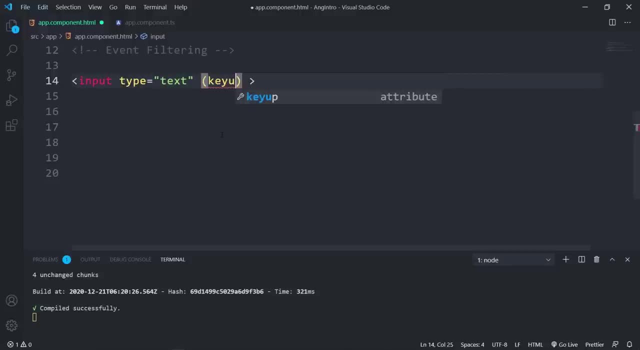 So inside brackets: keyup, event: You guys already know this. For data binding we used square brackets, For event binding we used this default brackets. After this it works. After this: equal sign. Let's call a method from here: onKeyUp, then parentheses. 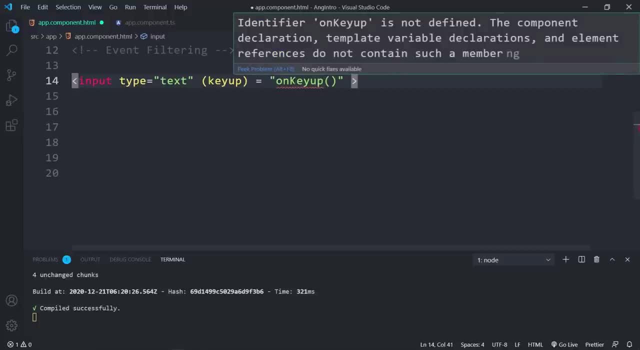 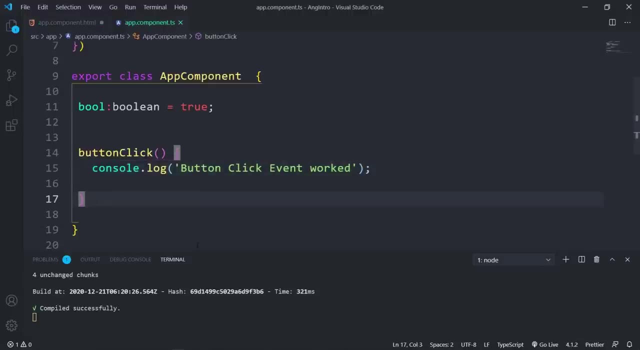 Now we are getting this compilation error saying that this onKeyUp is not exist. To solve this problem, let's create this method Inside the app component ts file. create onKeyUp method. After this onKeyUp. this k is capital parentheses and the method scope. 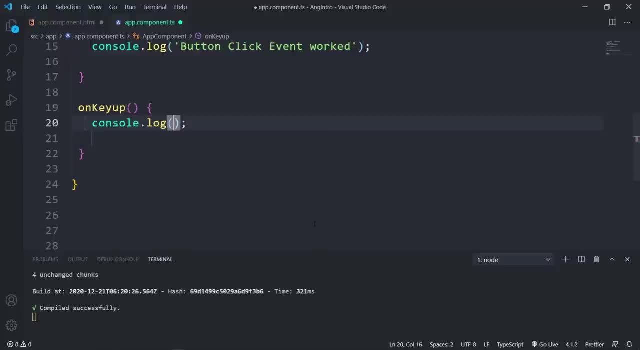 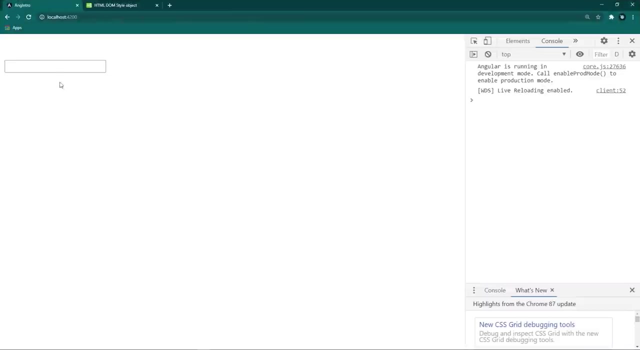 Inside this. for now, Let's log something. Let's see whether this method is working or not. So consolelog inside brackets. let's log keyup event working. Save this and back to the browser. Now we can see this input field, So type something inside this input field. 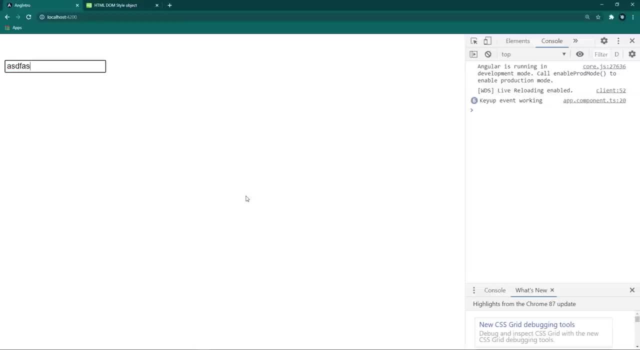 Now look inside the browser console. Perfect, We got this log. Every time we type something inside this text field. We got this logpng, Logpng, Logpng, Logpng And enter inside the browser console- Perfect. Now what I want to do is: I want to log this message only when I press the enter key. 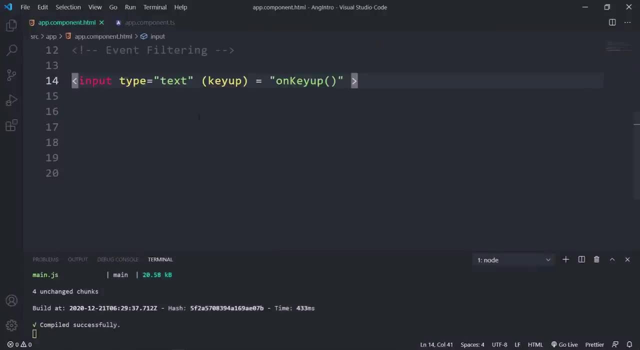 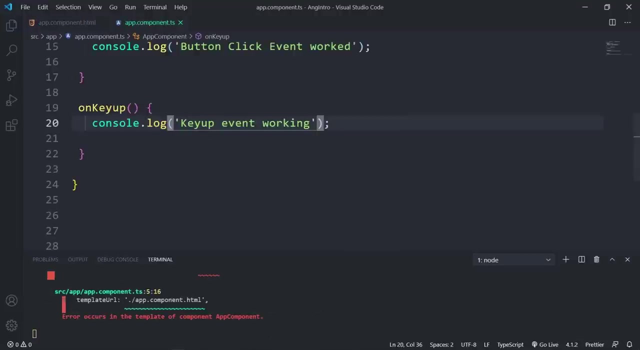 Not all the time like this, So let's do that. First we have to capture which key pressed on the keyboard For that. pass the event object with this method: $event. Now capture this event parameter from the onKeyUp method inside this parenthesis: $event. So this time log this event parameter instead of this text. 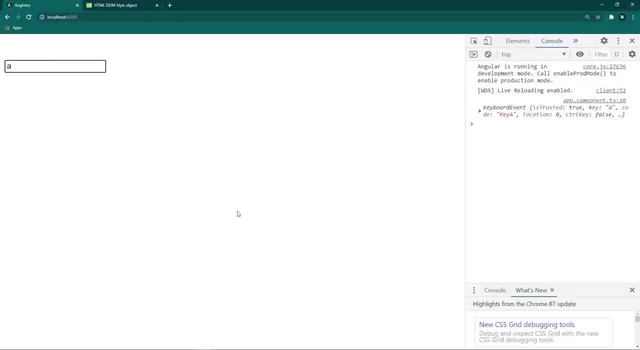 So save this all and back to the browser. Type something inside this input field. Now look at the console. In here we got this event object log. If I expand this, we can find a list of useful properties of this key event object. We can use this event object properties as per our 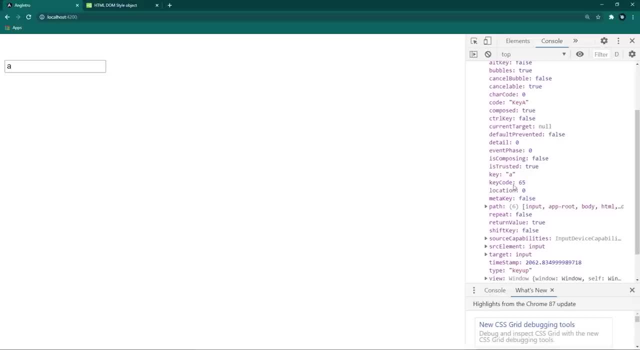 requirement. So in our case we gonna use only this key code. I typed a inside the text field. I can see that with this key property. After this we can see this key code for this. a key is 65. This time I type s: Look at this, we got another event object printed here. The key code is: 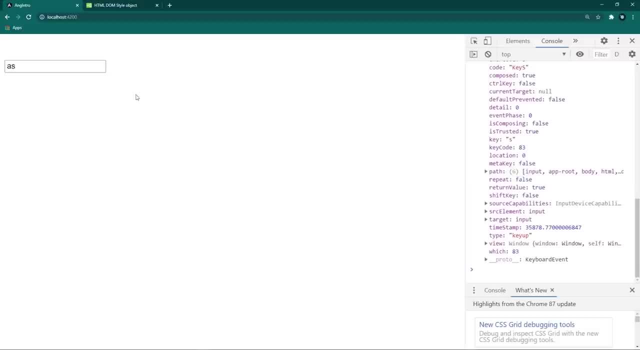 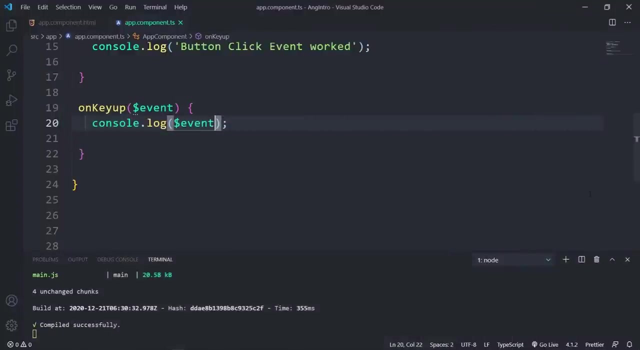 for the s letter $event. Again, if I type inside the input field Wait, rather getting this all object log, We log only this key code. Then we can see this clearly. So back to the app componentts file. Inside this we are logging the event parameter. Now I want to log only the key code. So after this: 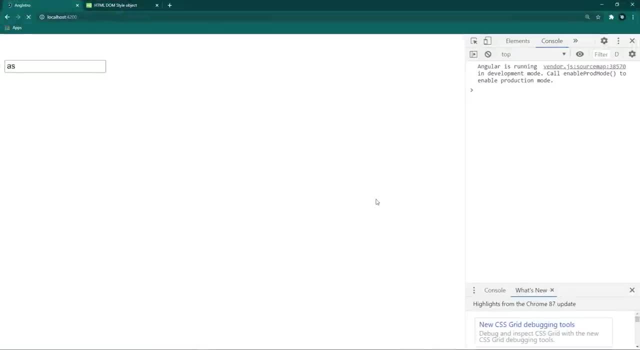 keycode. this c is capital. Save this and back to the browser. Now type a Inside the terminal. Perfect, we got this key code printed here. Like this: we will get a unique key code for each and every key that we typed inside this text field. Perfect, right, Alright. 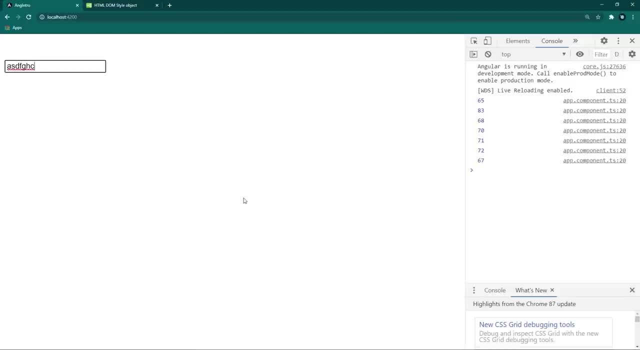 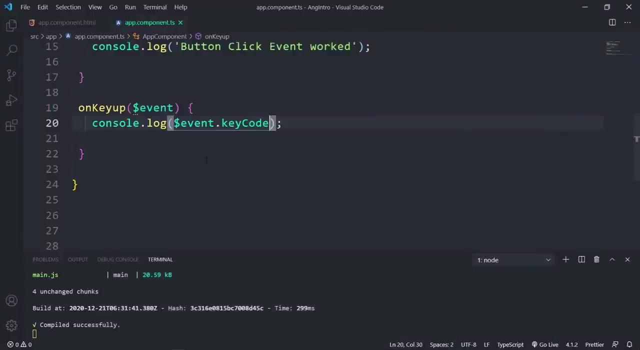 Now I want to log this when only press the enter key, Not all the time like this. For that, first let's look the traditional way, Then we'll look the angular event filtering way. In traditional we will add an if statement And check whether the key code is equal to the enter key's key code. Let's do that First inside. 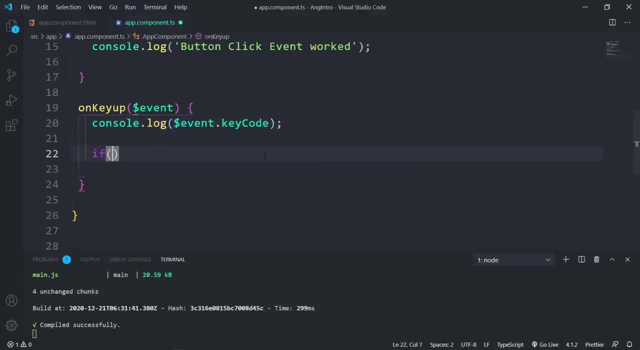 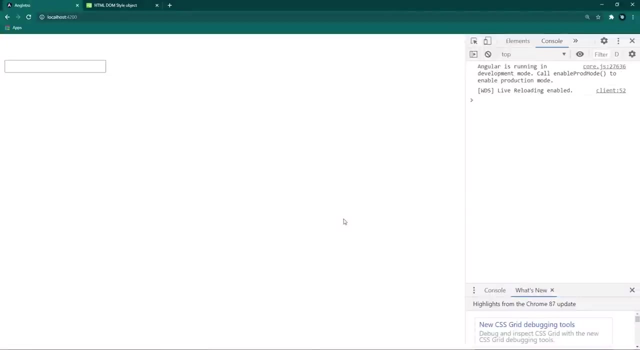 this method. If statement- Inside brackets- Pass the logic $eventkeycode equals, Now set this equal to the enter key's key code. Back to the browser and inside this text field, hit enter. This is the key code for the enter key. 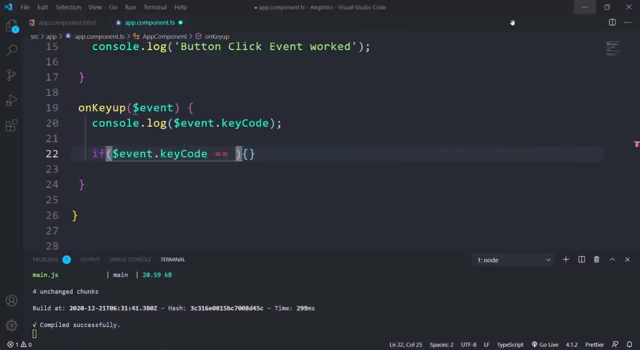 13.. Now add this key code 13 here After this: if statement scope: Inside the scope, put this log. Cut this from here and put it inside this: if statement Change the log to enter key pressed. Save this and back to the browser. Now type something inside the text field. 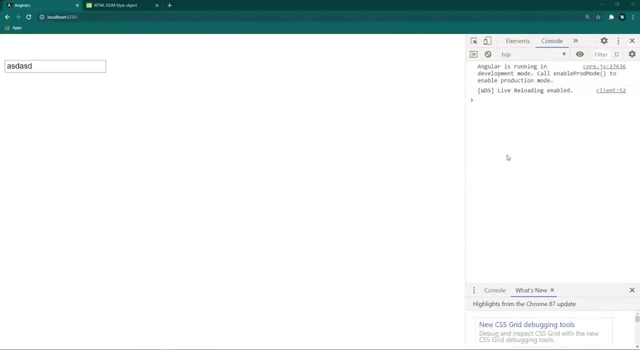 Look at the browser console. Nothing printed here. Now hit the enter key. Look at the console. Perfect, This time we got this log when enter key is pressed, So now we are getting this log only when we press the enter key, Not all the time. we typed inside this input field, like previous. 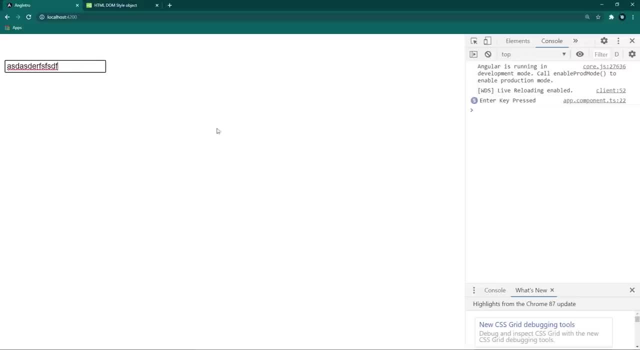 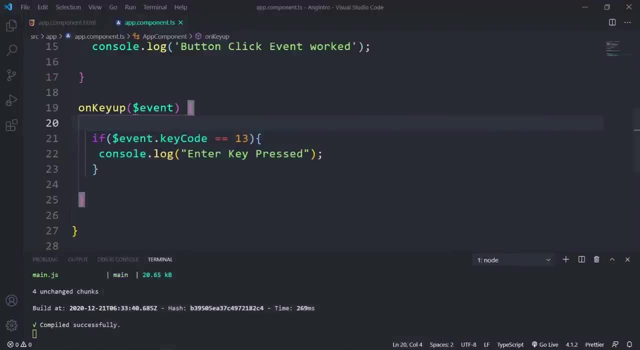 So this is how we doing this, using the traditional way, But in angular we have something cleaner and very easy method. Let's look at that. In angular we have event filtering. It is a simple method. We are filtering the keyup when only pressed the enter key using the event. 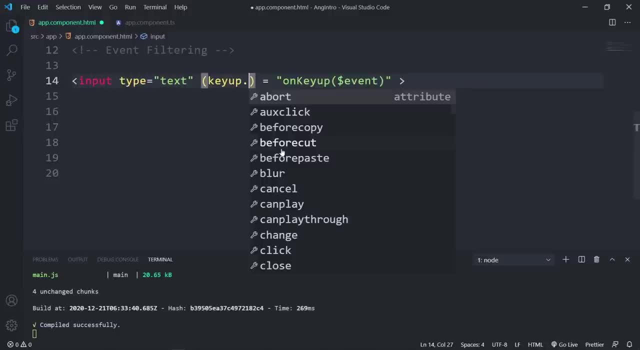 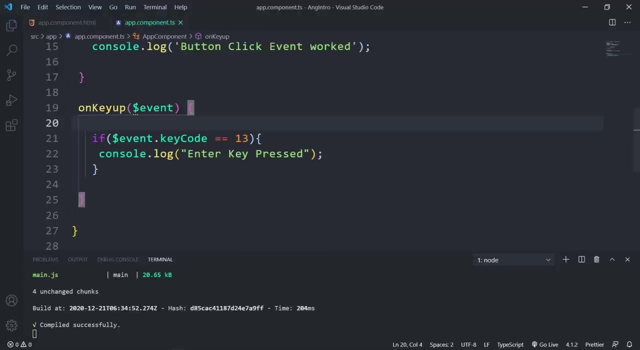 filtering. This is very easy. Just type after this event dot and enter. So with this we are filtering. the keyup event only work when pressed the enter key. Simple, right Now. we don't have to pass the event object here Inside the ts file. remove the event parameter, Of course we are not getting any. 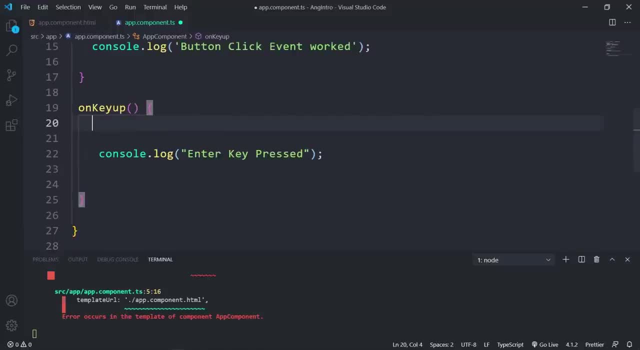 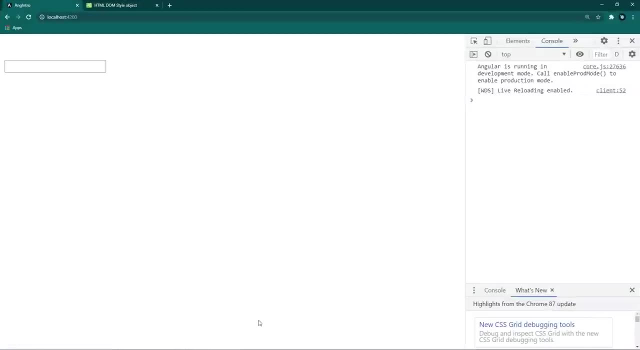 parameters. We don't need if statement and this key code logic. Remove them all and keep only this log. Now save this and back to the browser. Type some characters inside the text field. Look at the console. We are not getting anything. 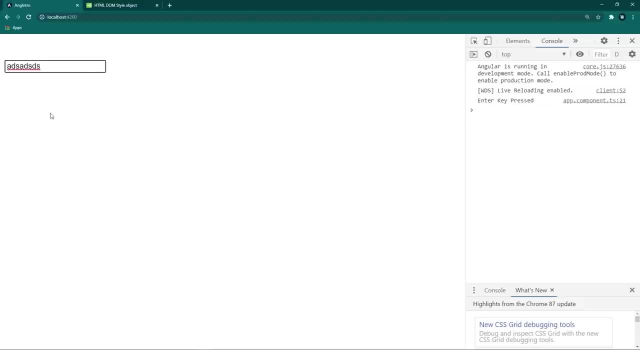 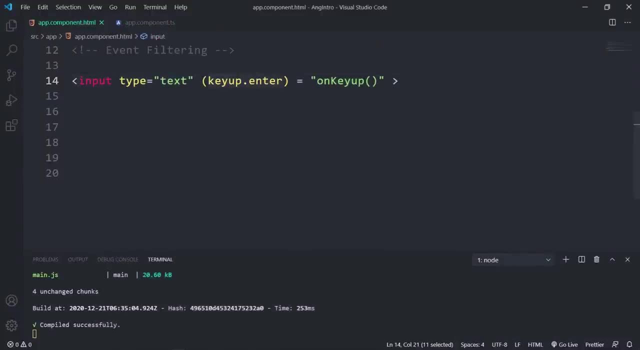 Now hit the enter key. Beautiful, We got this enter key pressed log. Perfect, right. With this simple line of event filtering, we got this log. This is very cleaner and understandable rather than the previous code. Hope you guys got the idea. Alright, this is how we use event filtering in angular. 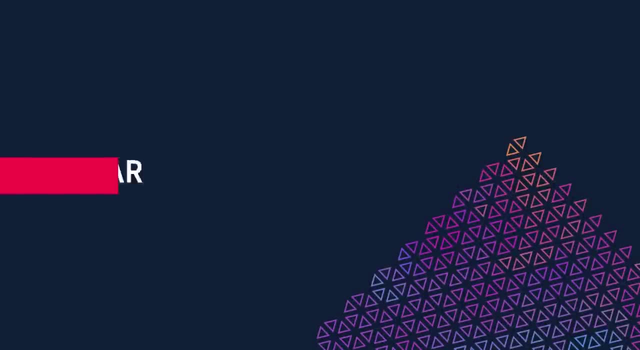 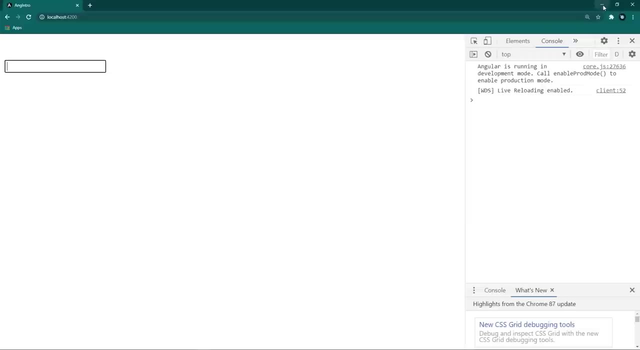 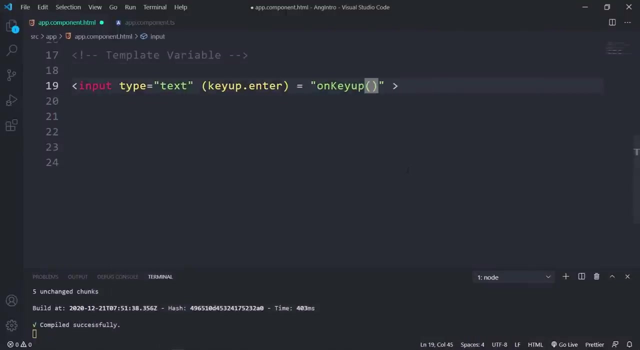 Awesome. So, in any case, if we want to get the typed value of this input field, how do we going to get that? We can do that by passing the event object like previous. Pass the event object as a parameter for this method: $event. 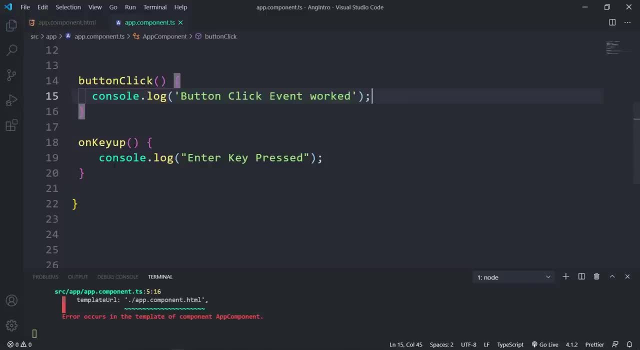 Go to the app component ts file. Inside this method on keyapp, pass the event parameter $event. Alright, let's log this value using the event parameter. So remove this previous log This time to get the typed values inside the input field, log this $eventtargetvalue. 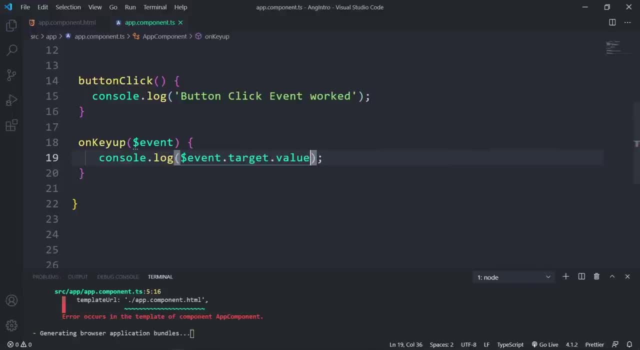 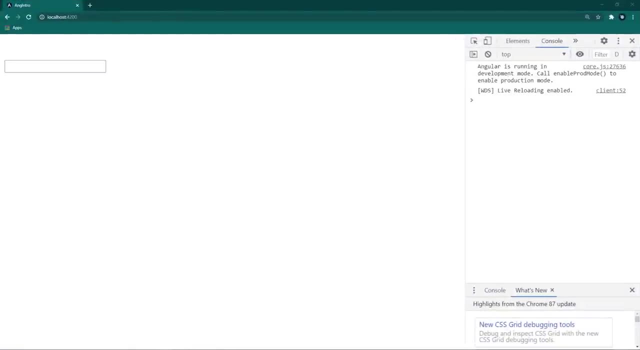 So this is how we get the values from this event object. Save this all and back to the browser. Type something inside the input field. Let's type angular, Hit enter. Look at the console. Perfect right, We got this value inside the console. 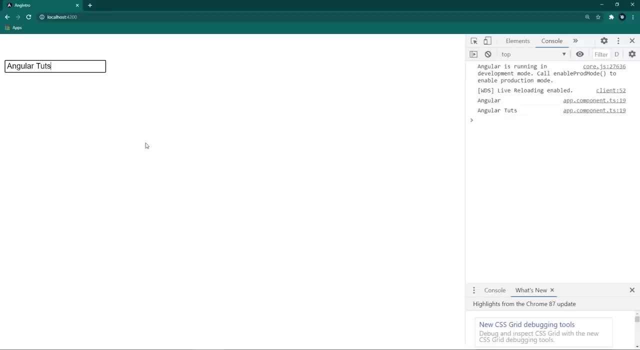 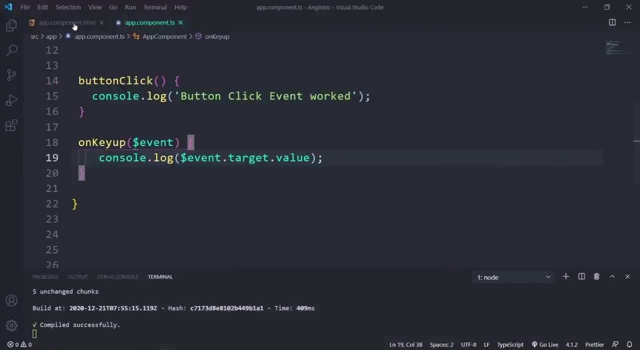 So this is how we get typed values inside of an input field, But in angular we have a cleaner approach for this. So let's see that in action. First we have to identify this input field. So we can do that using the template variable in angular. 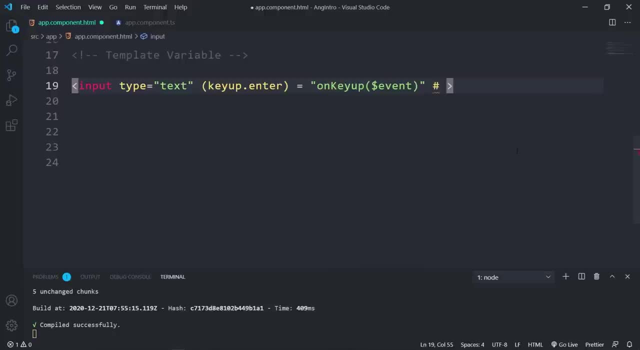 It's very simple: Just as sign. After this, just give any name for this field. Just assume this field is used to get usernames, So give this field name as username. Keep this in your mind. This as sign is important. Then only this becomes as a template variable in angular. 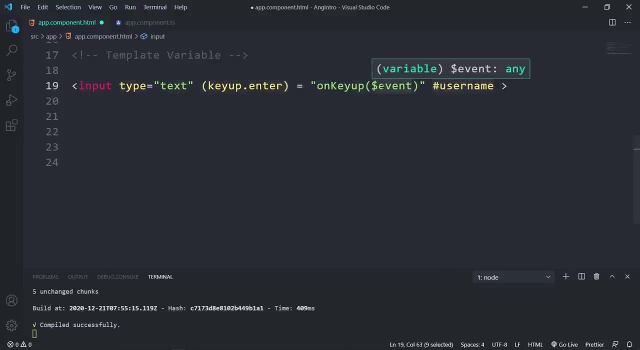 Next we have to pass the typed value to this method when pressing the enter key. This time we don't need the event object, So remove this. Now pass the values using this template variable. Template variable is username, So this is this template variable which represent this input field. 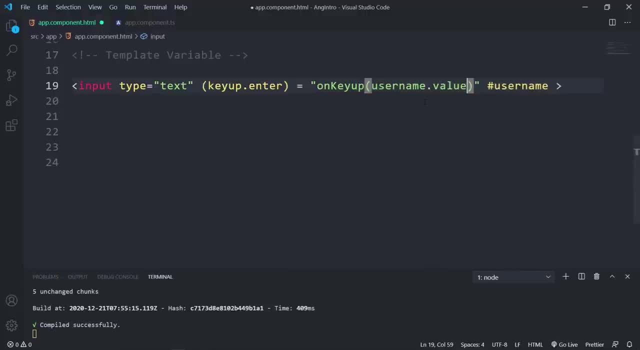 After this: dot and value. That's it. With this we are passing this input field's value to this method as a parameter. Save this and now go to the app component ts file Inside this keyapp method. This time we are not passing the event object. 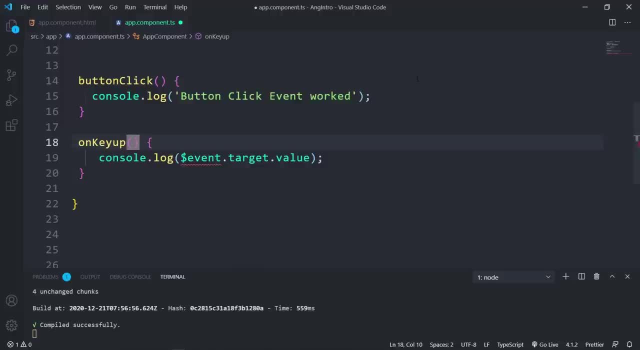 So remove it and simply add a variable to capture the parameter Username. After this, simply log this parameter in the console. Save this and back to the console. Save this and back to the console. Save this and back to the browser. Type something inside this input field. 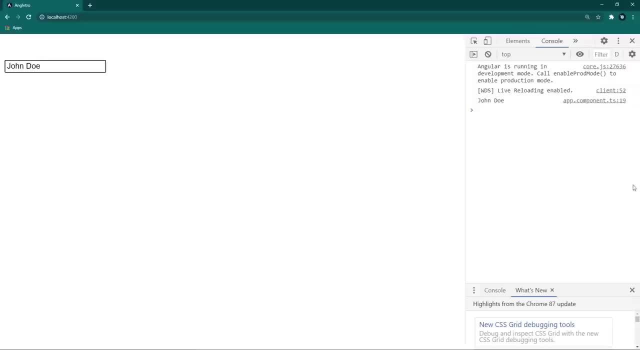 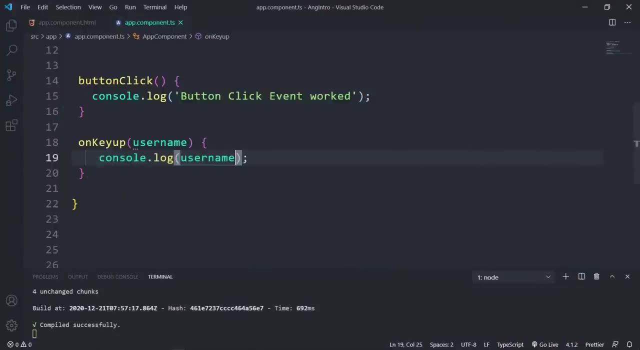 John Doe Hit enter. Look at the console. He got this value, John Doe, printed inside the browser console. Perfect right. So this is how we use template variables in angular. Hope you guys got the idea. So in previous We learned. 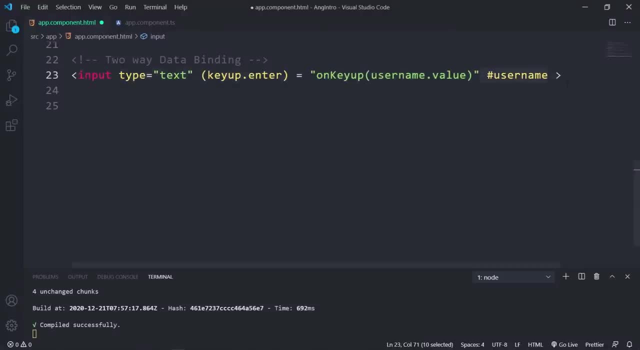 How to get the value from the input field using the angular template variable. So in this video let's look at another, cleaner way of getting data from this input field. In previous we declared a variable in HTML file and we passed that variable values to this method and we captured that parameter. 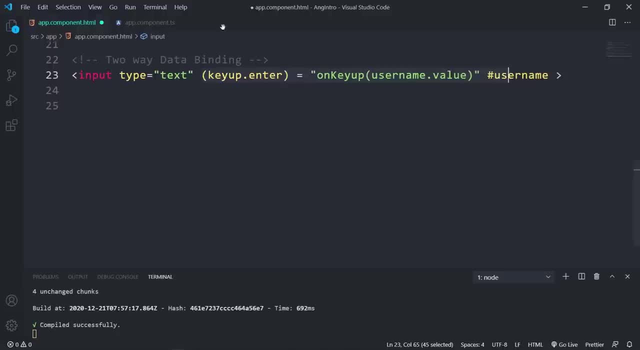 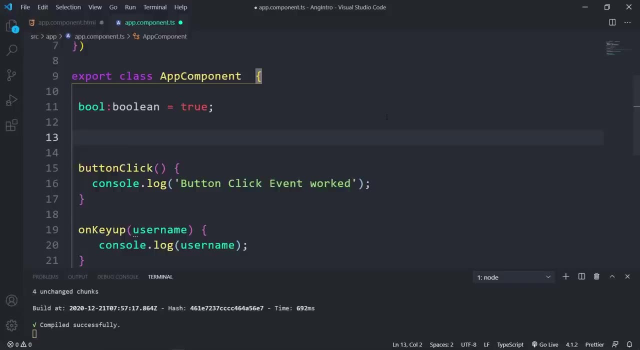 But now let's see how to assign this input field value to a variable created inside the component class. Alright, first create a variable inside of this component class. Variable name is username. This n is capital. The variable type will be string. Now what I want to do is: 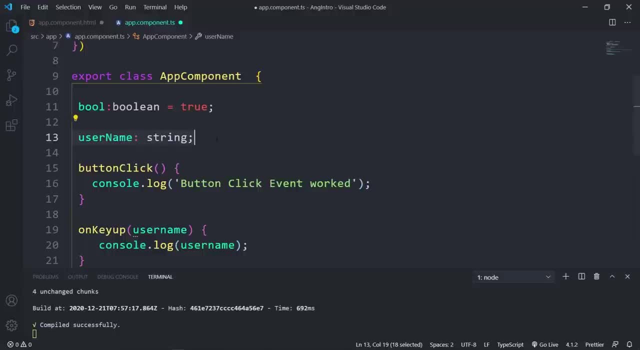 I want to assign this text field value to this variable. How do we going to do that? This is very easy. For this we have another data binding method in angular, like the string interpolation property binding. So for this we have angular two way data binding method. 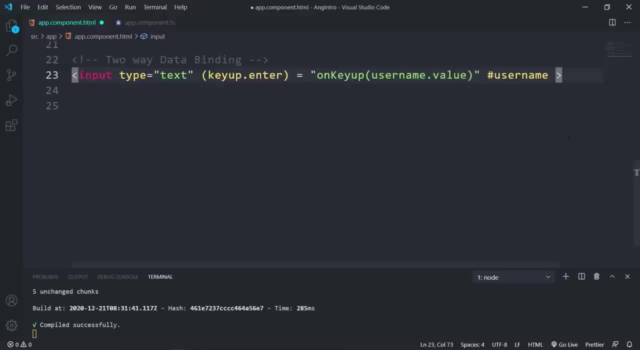 Let's see this in action. Keep this previous example. After this, create another input field. The type will be text. Now let's see how to bind this text to this component variable. Very simple: Inside this input, first create square brackets. Inside this square brackets, open and close, simple brackets. 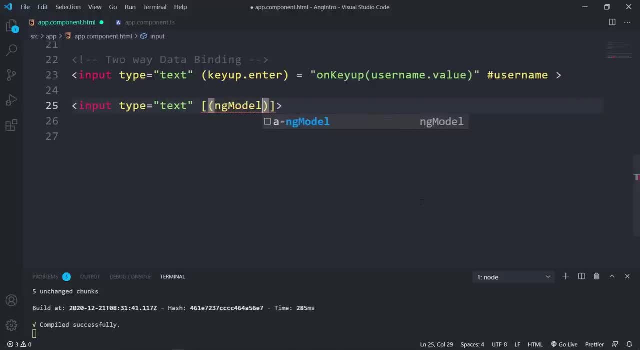 Inside this brackets: Type: ngmodel. This is ngmodel is a special angular syntax for this two way data binding. Keep this in your mind. This m must be capital. Next equal sign. Now, inside this codes, pass the variable name that we created inside the component typescript. 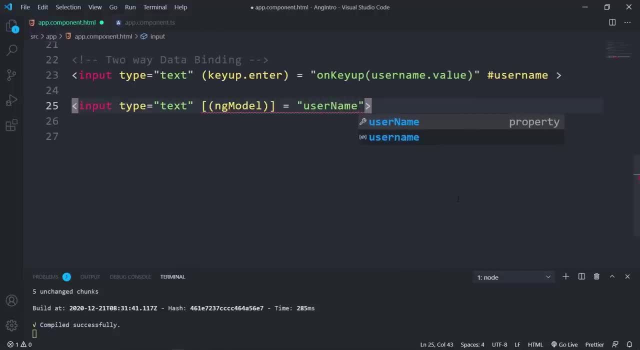 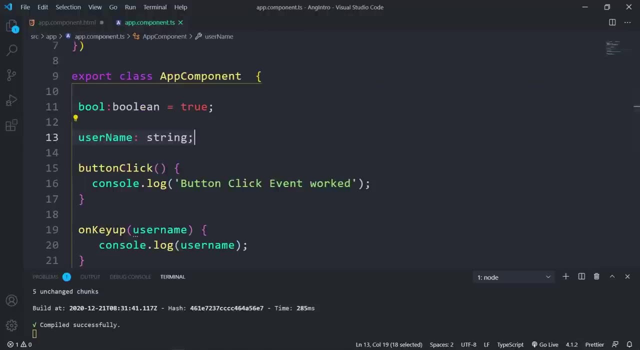 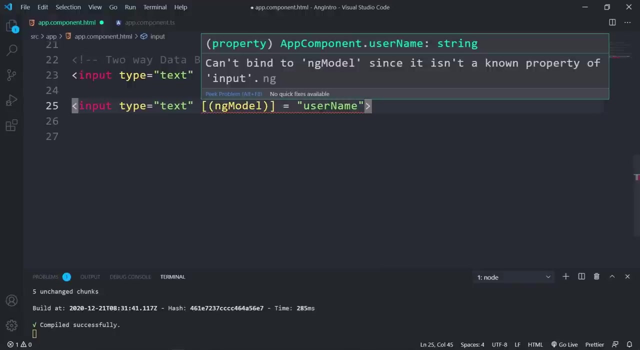 file Username. This n is capital. That's it. We have successfully assigned this text fields value to this component Username variable, which is created inside this ts file. If we look at this carefully, we are getting a compile error. ngmodel isn't a known property of this input field. 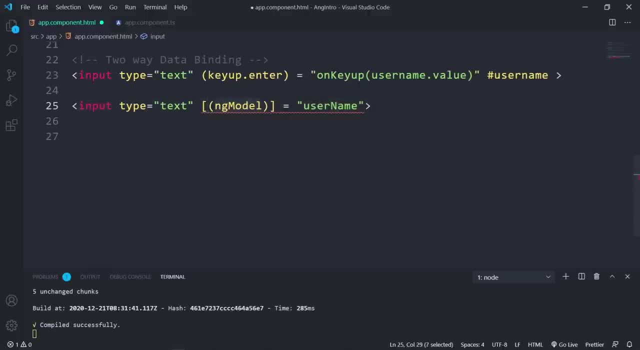 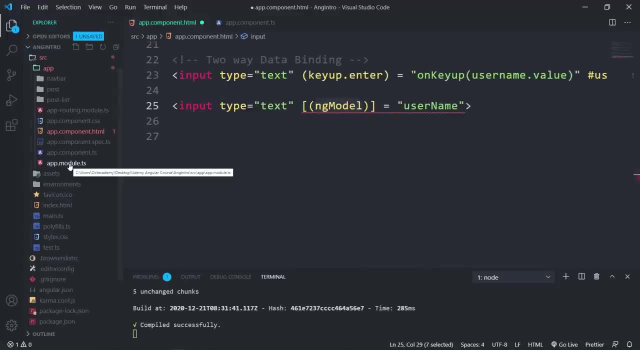 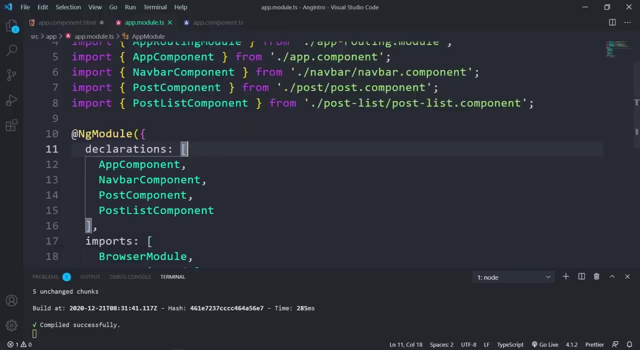 Why is that? Coz this ngmodel is inside of angular forms module. So in order to remove this error, we have to import the forms module to our angular project. So open the appmodulests file Inside this. let's import the forms module. 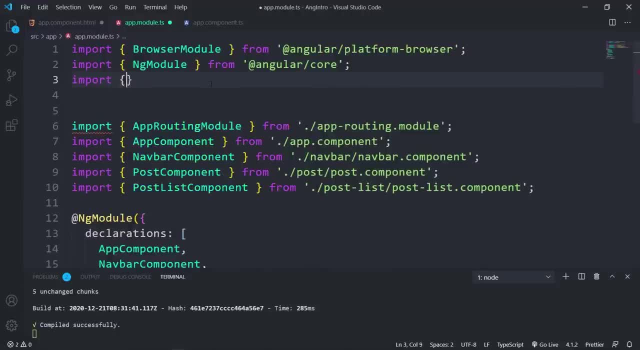 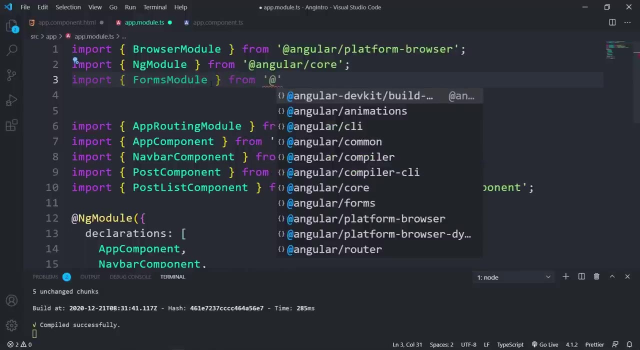 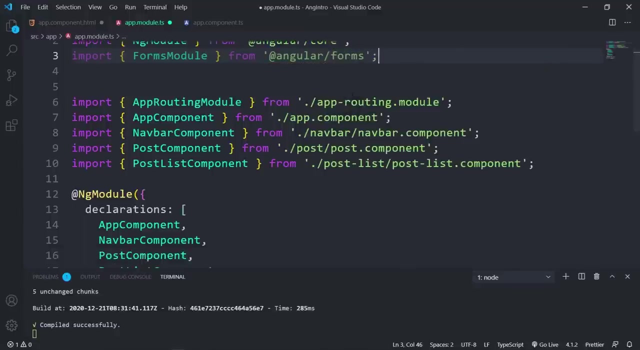 At the top of this import section add the import statement. Import- Inside curly brackets: Forms: module. This, f and m will be capital letters. Next from Then, module path will be at angular slash forms. Pass this inside quotes After this: 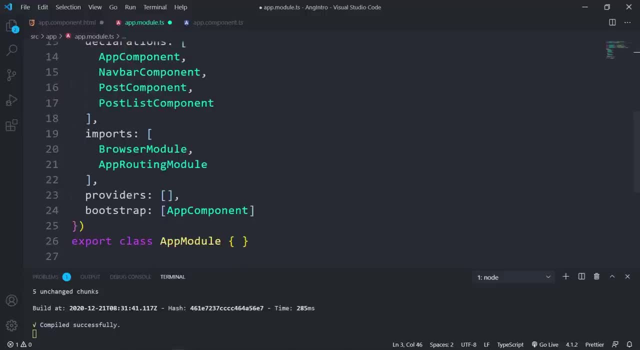 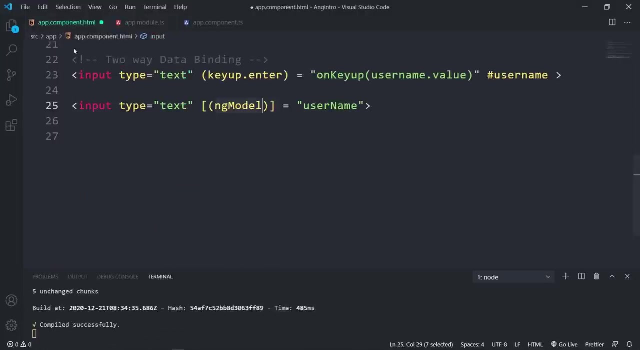 Add this imported forms module inside this import After this browser module: comma forms module. That's it. Now our angular app knows that we are using the forms modules features inside our angular app. Now go to the app component html file. Now look at this. 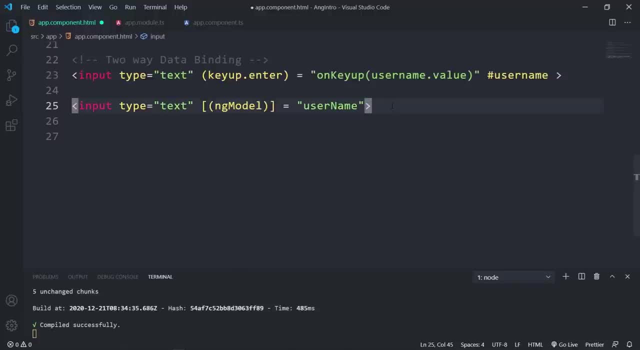 This time we are not getting any compile errors. Beautiful, Alright. Now let's simply add the keyup event with the event enter key filter Like this: Now let's simply add the keyup event with the event enter key filter Like this: 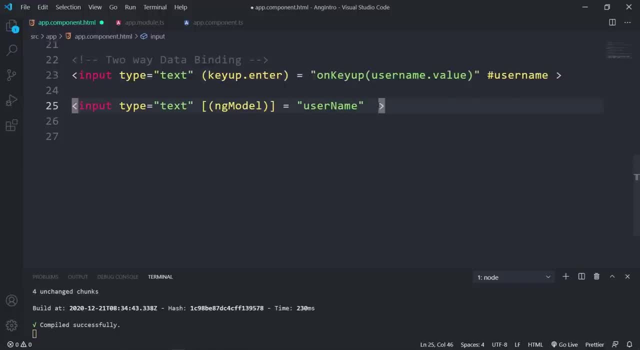 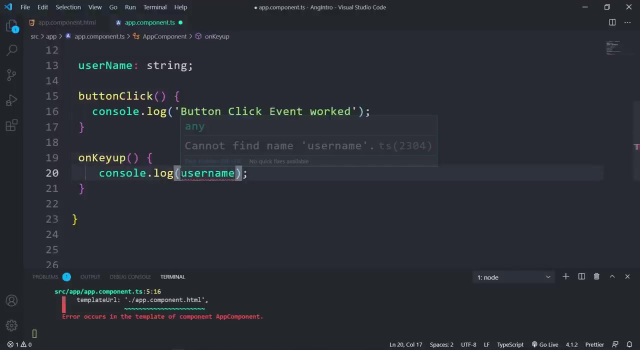 Just copy and paste it here. This time we don't need to pass this template variable. Remove it, That's it. Now go to the app component typescript file And remove this parameter. We don't need that anymore. This time. lock this username variable instead of this parameter variable. 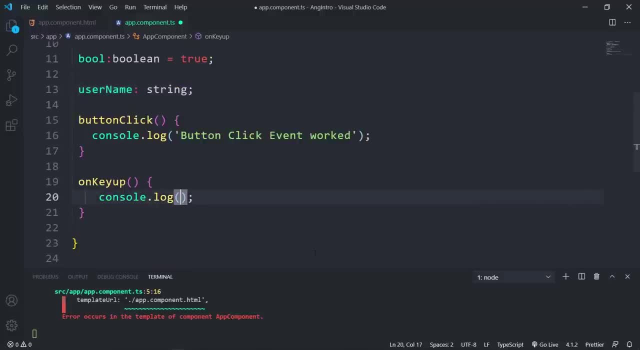 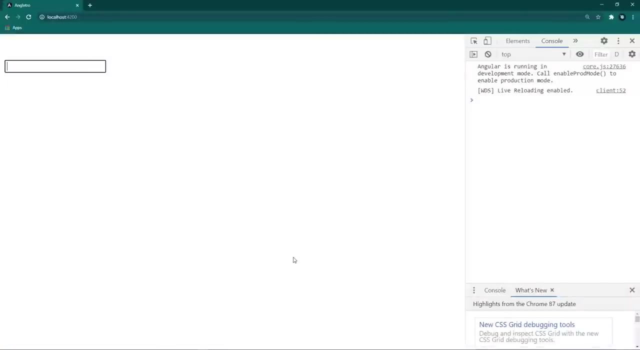 If you can remember, in order to access a typescript class variable inside of a method, we have to use this class, this keyword, So thisusername, this n is capital. Now save this all and back to the browser. Type something inside this text field and hit enter. 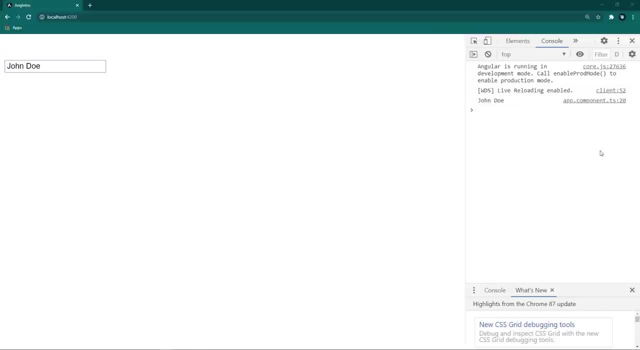 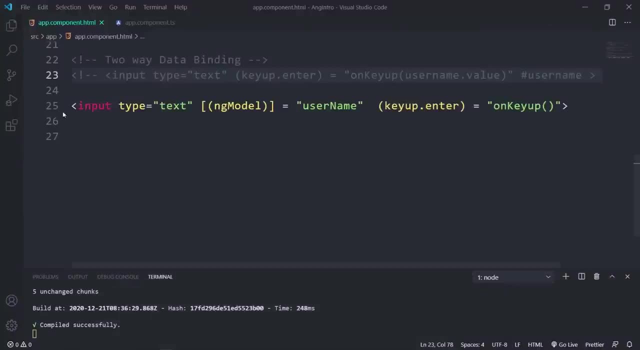 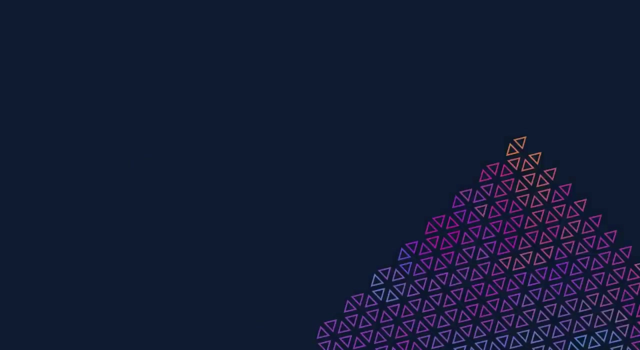 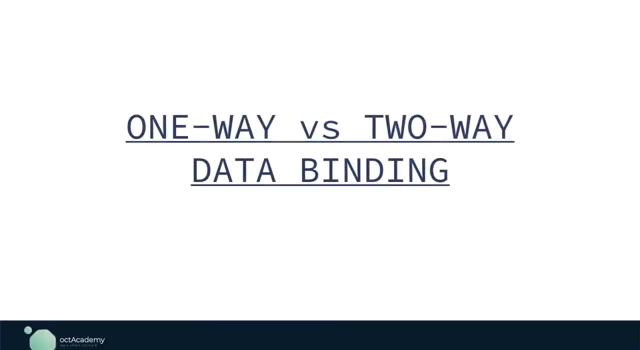 We got this John Doe inside the console. beautiful, isn't it? So this is how we use two way data binding approach to get the values of input field. In the previous video, we learned about the two way data binding. Some of you may wonder what is this two way data binding, how this is different from this. 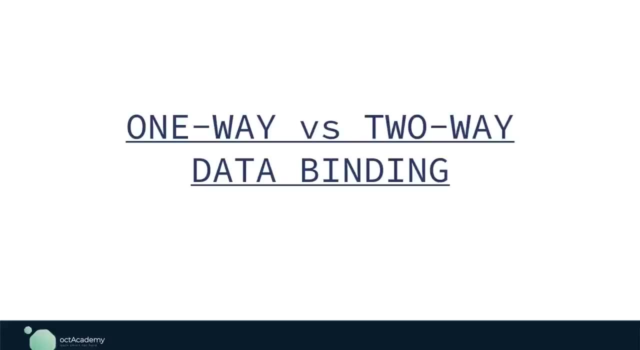 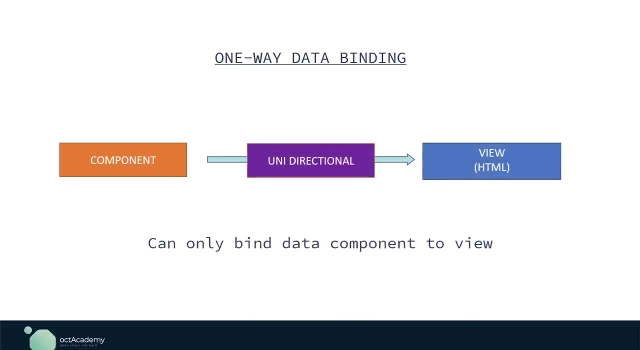 property binding. and actually what is this? two way data binding and one way data binding. So if you look at the one way data binding, so this one way data binding will bind the data from the component to the web. So this one way data binding is unidirectional. 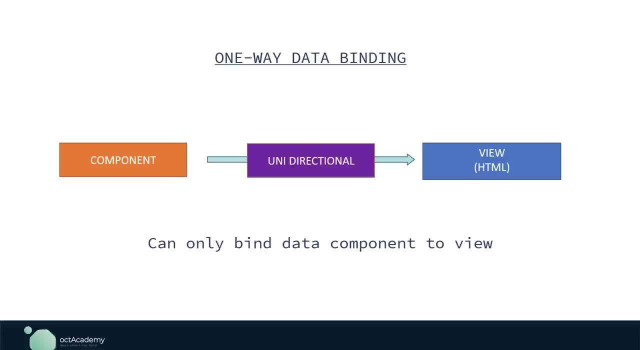 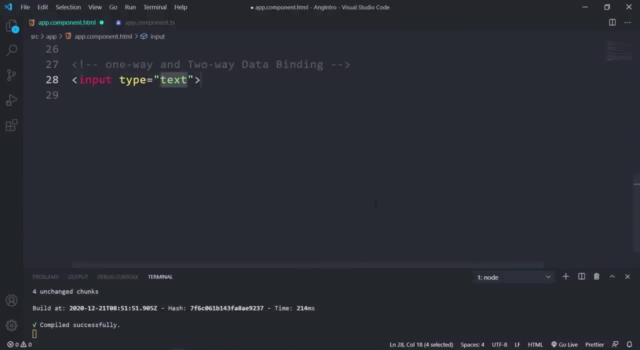 So you can only bind the data from the component to the web. Let me show you a quick example for this. Create another input tag after this input and hit enter. Input type will be text. Now I want to add value to this input. 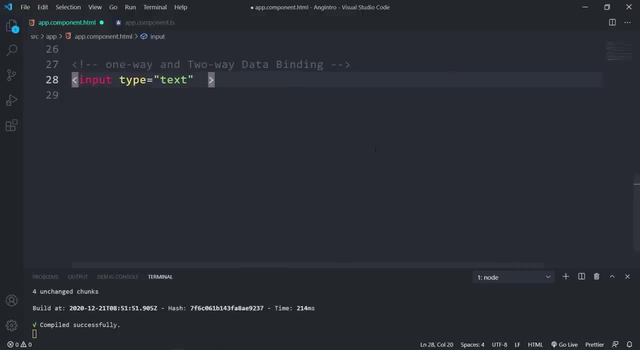 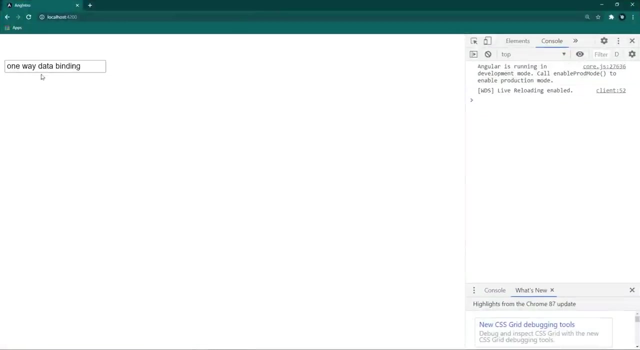 How do we do that? normally We set the value property to this input field and we'll add the value inside the quotes. Value will be something: one way data binding. So save this and back to the browser. Look at this. We got this two way data binding inside this text field. 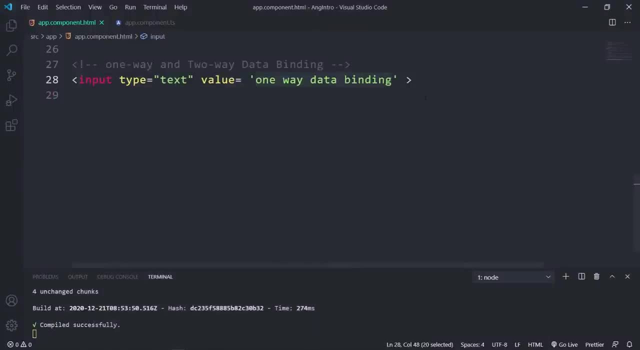 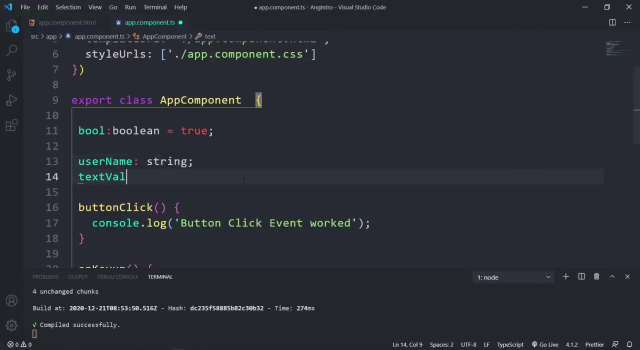 So this is how we doing this in normal HTML, But I want to make this dynamic, So I will create a variable inside the component ts file, Something text value. This v is capital. This variable's data type is string, So after this, assign a value for this. 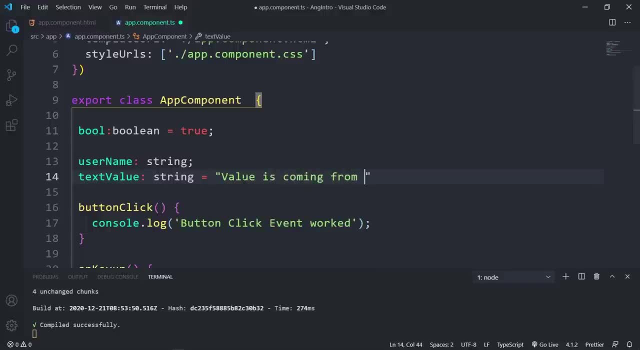 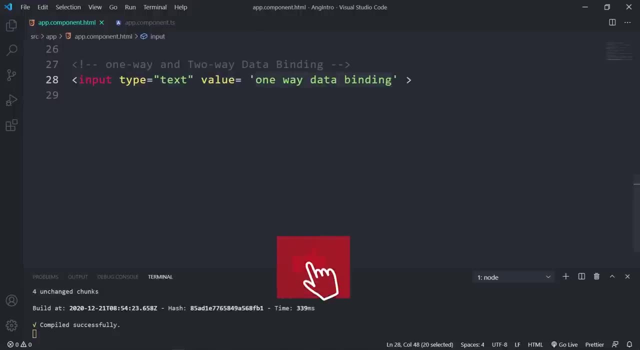 Inside quotes. Something value is coming from the component, So save this. now Go to the app component html file. Now I want to pass the text value variable to this input. How do we do that? If you can remember, we learned earlier how to show a variable inside of this HTML wave. 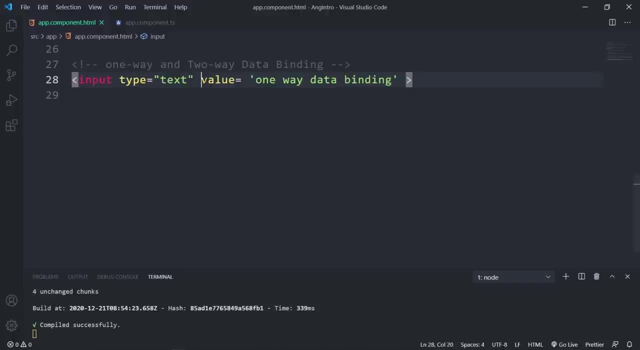 using string interpolation and property binding. Now we are dealing with this value property, So let's use the property binding now. So let's make this value property as a property binding By wrapping this inside of a square brackets. Now we are getting the value from the component. 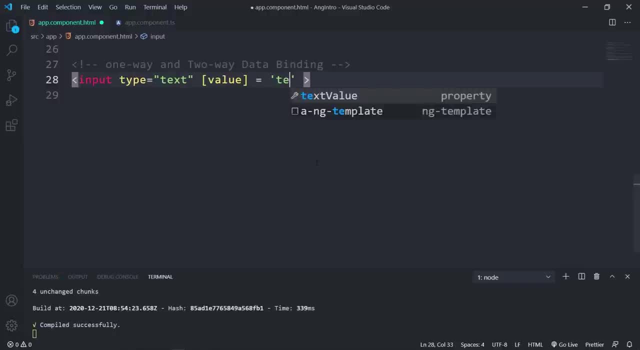 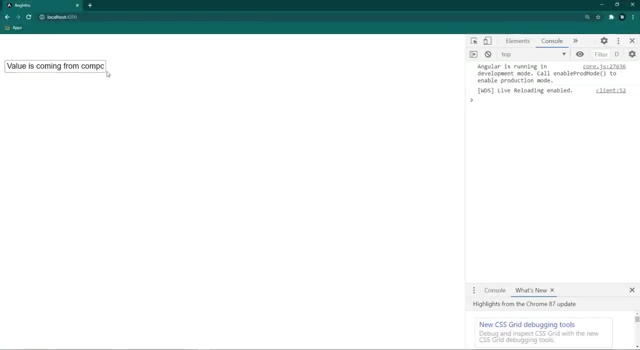 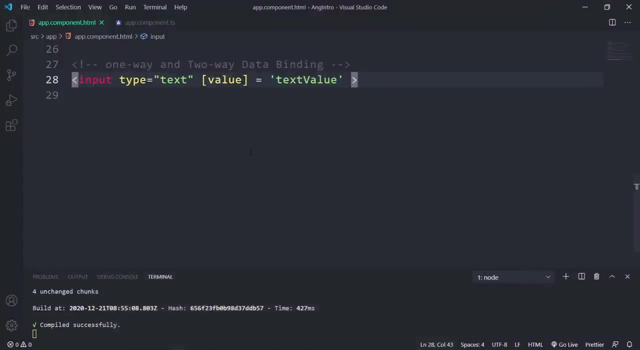 So remove this hand coded value and add the variable name Text value. Now save this and back to the browser. Perfect, Now we got this value inside this input field. Now think if we want to capture this value when we press the enter key. 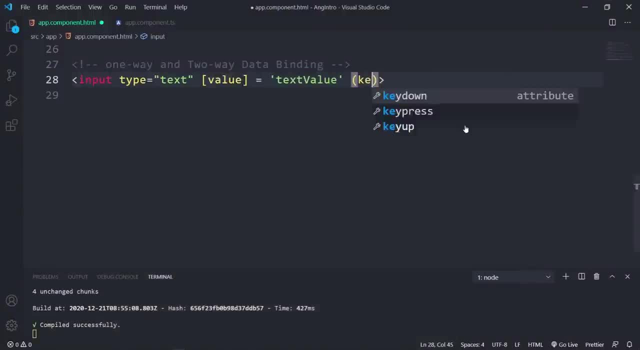 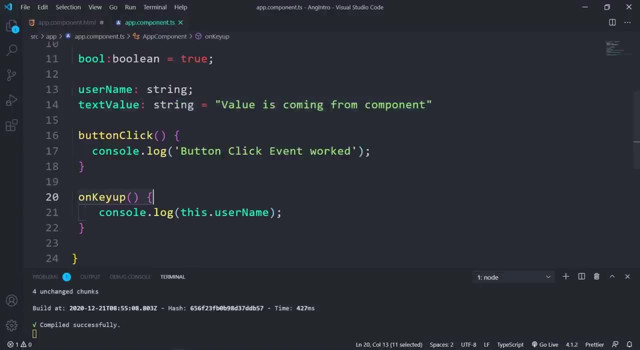 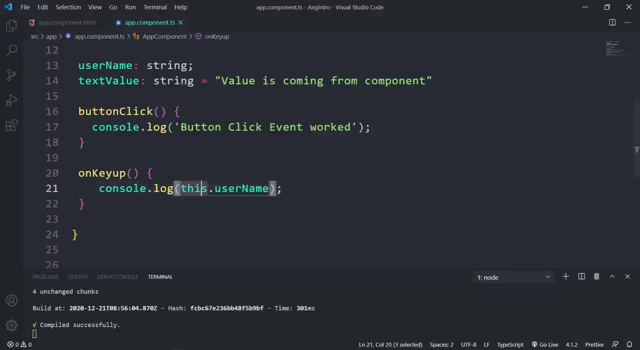 Like previous video example For that: first: bind the event with the event filtering for enter key. Assign it to this same onKeyApp method. Save this. Now go to the componentts file and remove this previous log and add this new log This time log this text value variable. 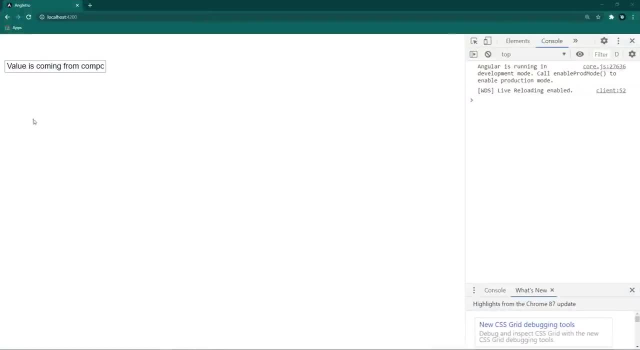 Save this all and back to the browser. Now we got this value inside this text field, So hit enter. Look at the browser console In here we got this log saying value coming from the component, which is same as this. Now let's change this value to value coming from wave. 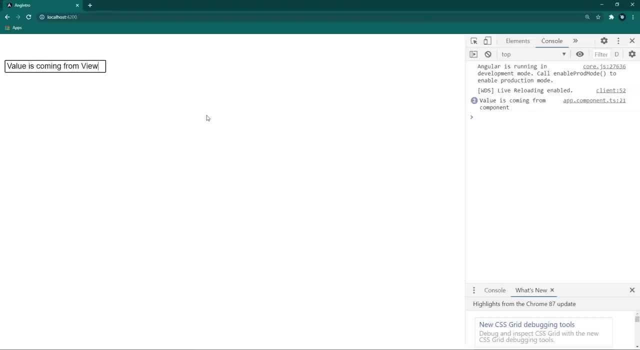 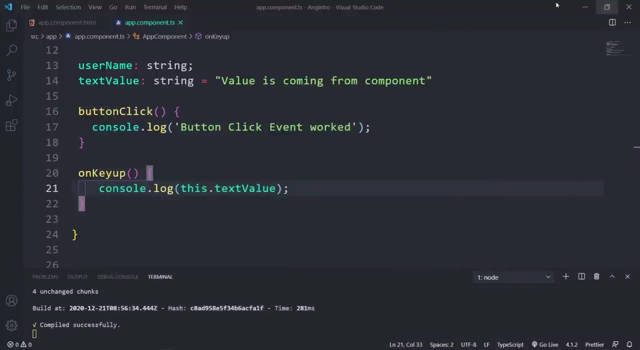 Now hit enter. Look at the console. This time also, we got this same previous message Again. change this to something else. Still, we are getting the same message. What is happening here? If we look at the code, this is passing this text value- variable's value- to this input. 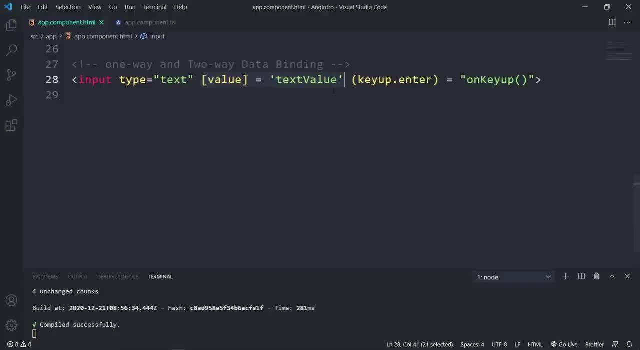 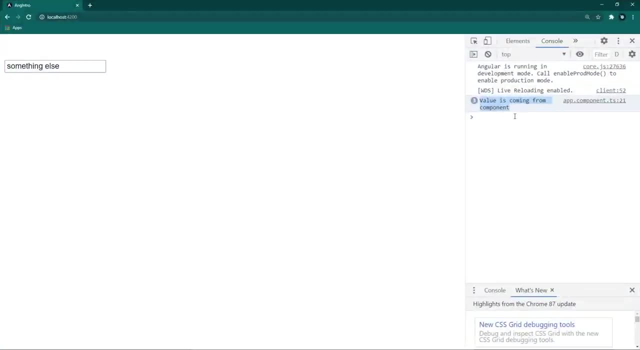 with property binding, But this cannot modify this changed value and assign it to this component text value variable. That's why we are getting this same value from this log. So Let's see what we called one way data binding. With this, we can only bind data from component to wave. 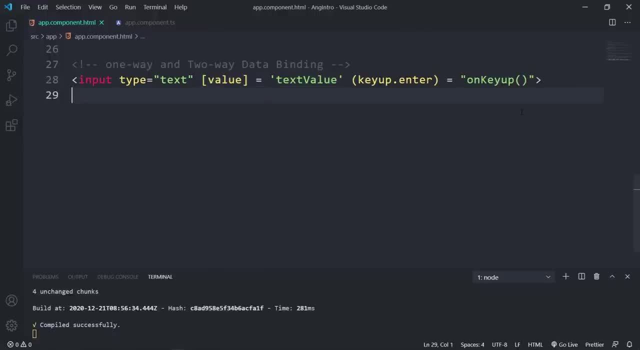 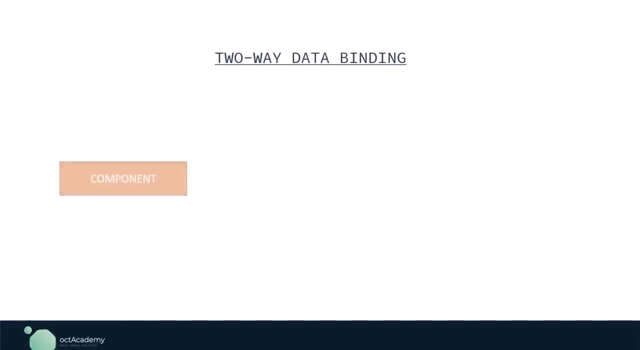 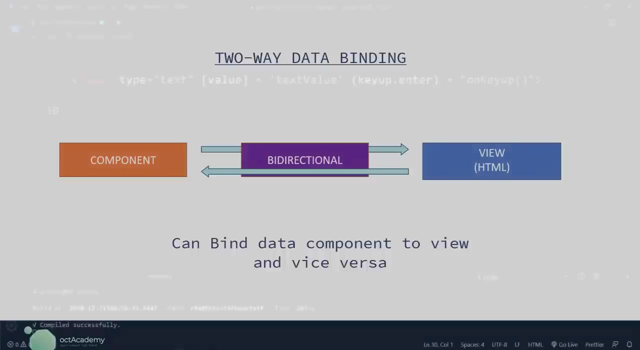 We cannot change this variable's value from inside of this wave or with this html page, But with the two way data binding we can pass data from component to wave and also we can send data from wave to component. Let's see this in action. 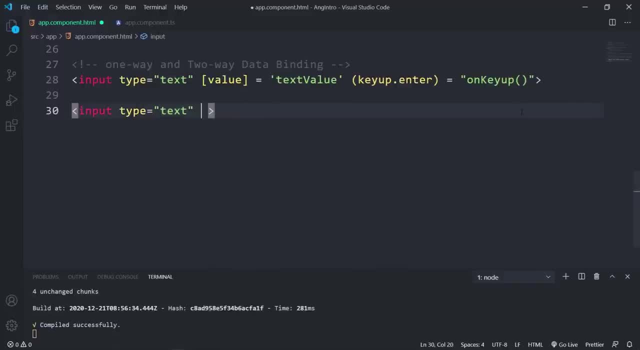 Again. create another input field. Input type is text. Now bind this text value variable to this. In previous example we did this using the property binding. This time let's do this with the two way data binding. We learned about this in the previous video. 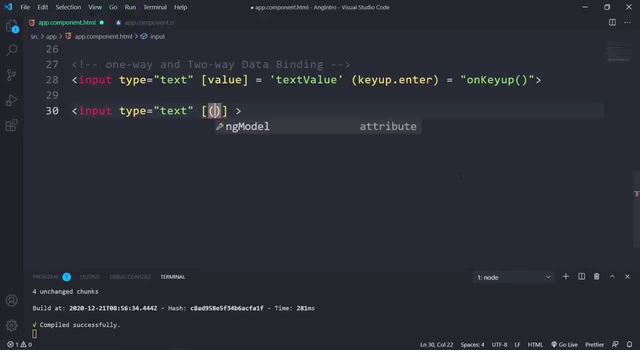 So open and close square brackets Inside this, again, simple brackets Inside this type ngmodel. So this is the special angular syntax for two way data binding. So after this equal sign, Now pass the variable name inside quotes, Text value. After this, add this same keyup function. 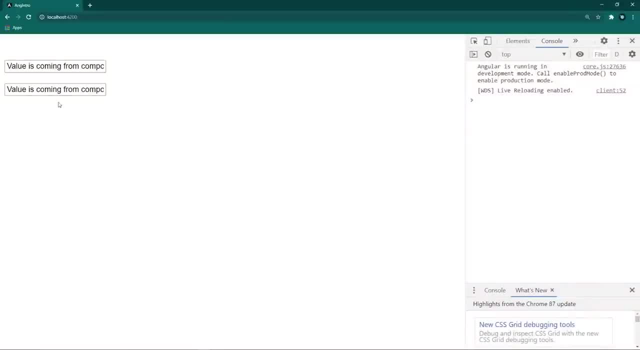 Copy and paste it here. Save this all and back to the browser. We got this value inside this second input as well. Now change this value to value coming from the wave and hit enter. Look at the console. This time this value. change to this value. 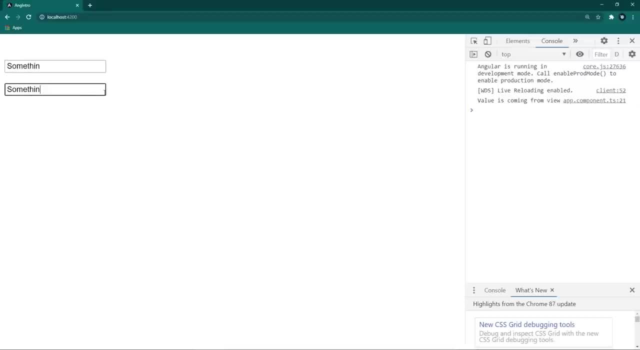 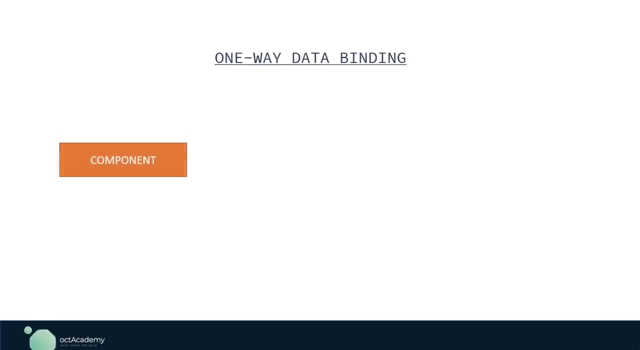 Again, type something else and hit enter. Perfect Right, we got this value log inside the browser console. So this is the usage of two way data binding. If we quickly recap this: With one way data binding, we can only set data from component to wave. 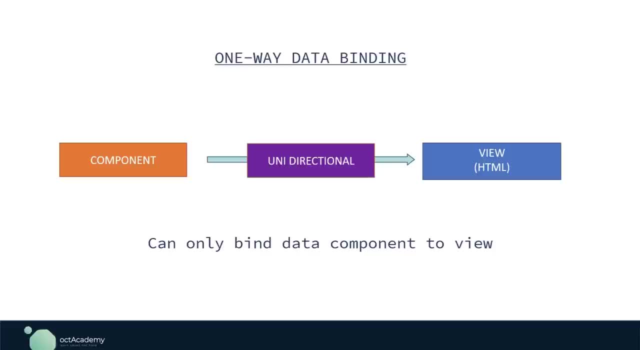 We can not modify or add changes to that data from wave and send it back to the component, But in two way- data binding. We can pass this value, We can pass data from component to wave and also we can modify that data and send it back. 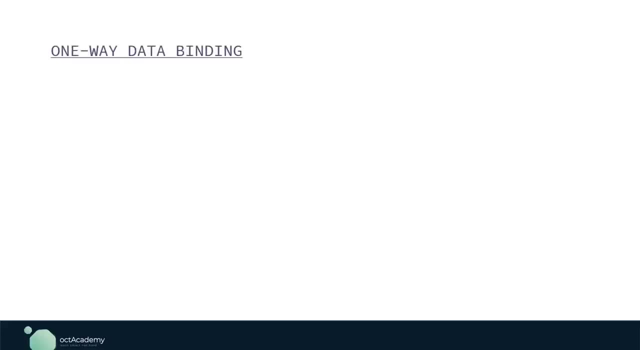 to the component from the wave. This string interpolation, property binding, class binding and the style binding- All this data bindings are included into the one way data binding category. We can only do two way data binding using only this ngModel syntax. Hope you guys got the idea. 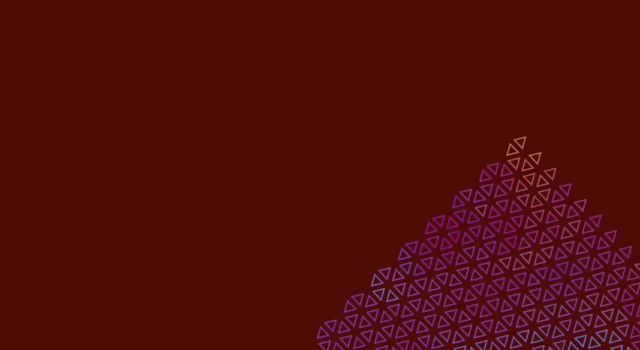 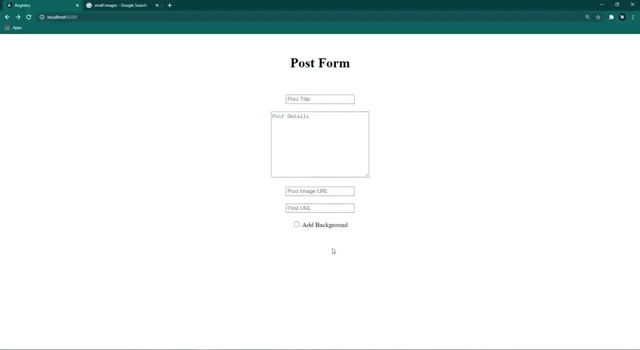 Alright, let's do a small task. This is going to be a very quick, small task. All you have to do is create this simple form and display the input fields typed value down. here We have this simple form which includes these fields: A text field for the post title. 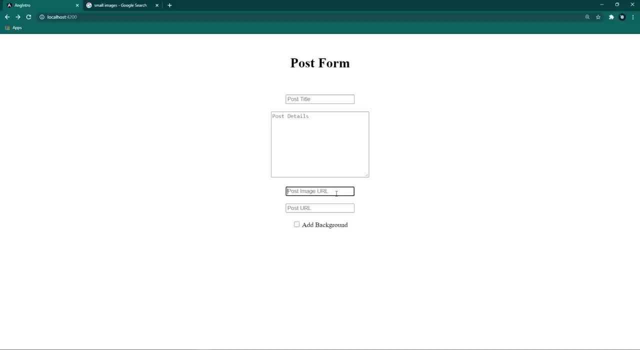 Next a text area for post details. After that another text field for post image url. After this, we have a text field for post title. Next a text area for post details. Then we have this text field for post url and at last we got this checkbox to highlight. 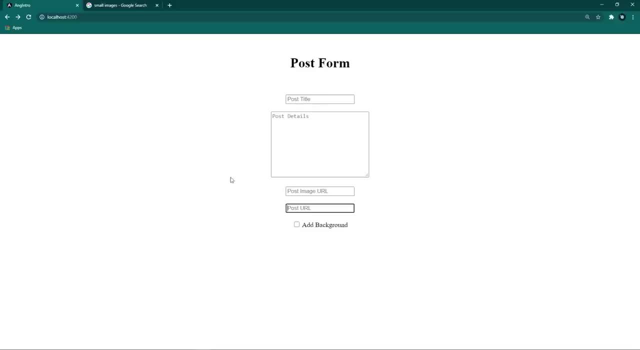 the background color of this post title. If I type a post title inside this, this will show the post title real time down here. Like that, If I add a post details, it is also rendered down here. Next, if I add an image url which I got from google, this image also rendered down here. 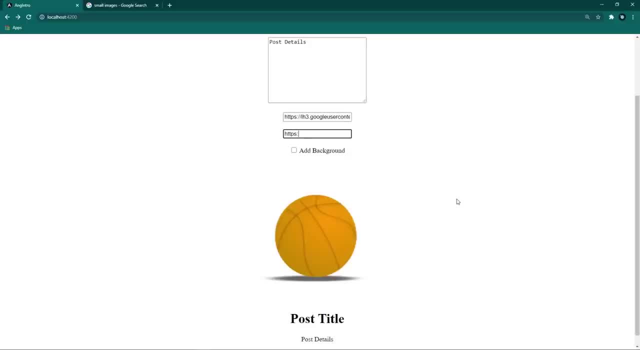 If I add a post url which is also a down here- Ok, Bye, Bye, dummy- URL which I got from Google, this will show us this more detail link, And if I click this link, which will open this added website link inside of another browser. 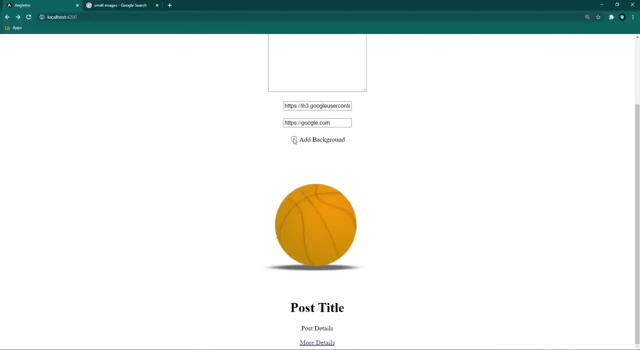 tab At last. if I check this checkbox, this will give us this nice yellow background color for this post title. If I uncheck this checkbox, this will remove the background color. That's it. nothing fancy, very simple task. All you have to do is first design the form, then use the two-way data binding approach. 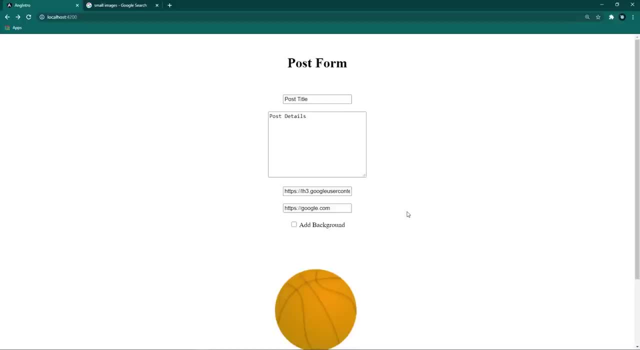 to capture this form values. After that, using the string interpolation, property binding, class binding and event binding, create this preview area. Don't worry, nothing fancy here. very simple task. All you have to do is just think and apply one of the data binding approaches to generate. 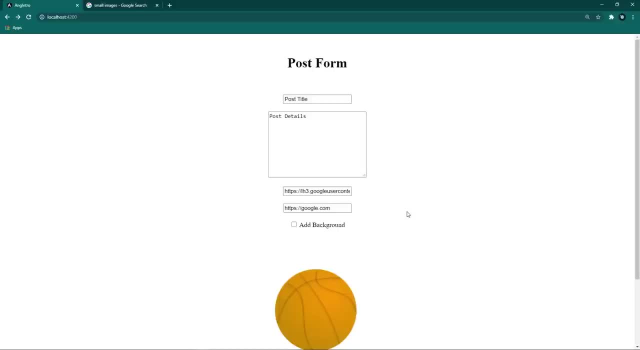 this preview area. As always, try to do this. Put this task on your own. If you forget anything, just go through on this section again and learn it again. Don't give up. take your own time and complete this task. Once you have completed the task, continue with the next lecture. 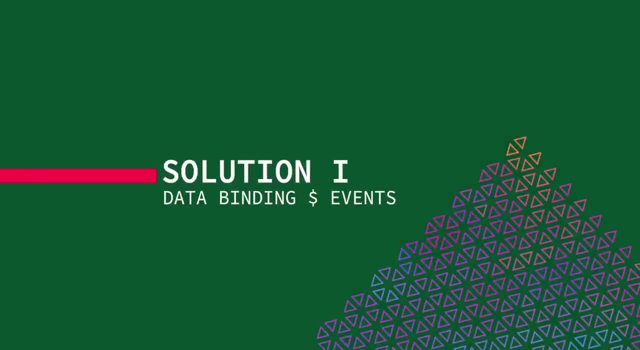 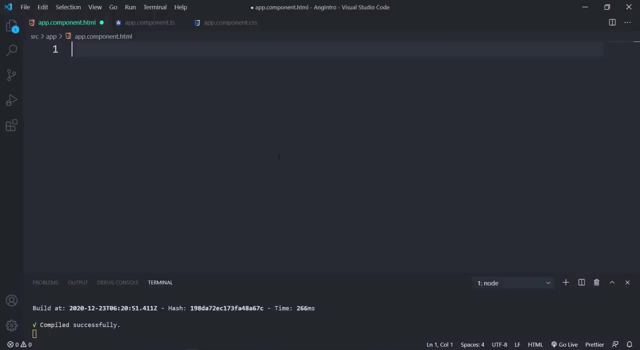 All the best. Hope you guys did the task well. If any of you missed to complete the task, don't worry, let's continue the task with me. Alright, inside the component html file, let's create the html form. So create a div with form-area CSS class. 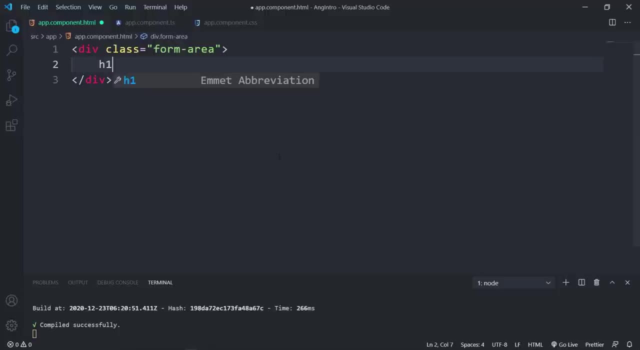 Inside this. first we have the heading, so h1 tag Inside this post form. After this, create an input field: input, hit enter. the type is text and placeholder: post title. Next the textarea. so type textarea and hit enter. 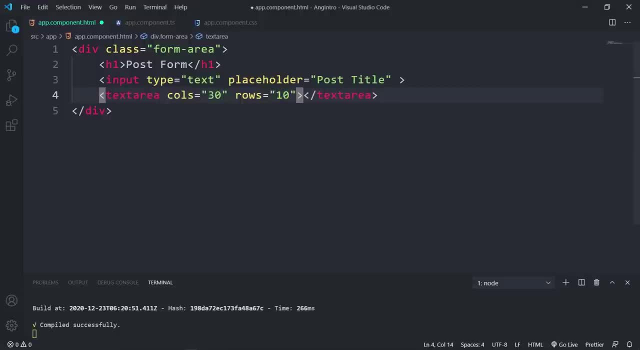 We don't need this name attribute, so remove it. And placeholder post details. Next, again two input fields: one for the post image URL and another one for the post URL. At last, create a checkbox Input textarea. Input type will be a checkbox. 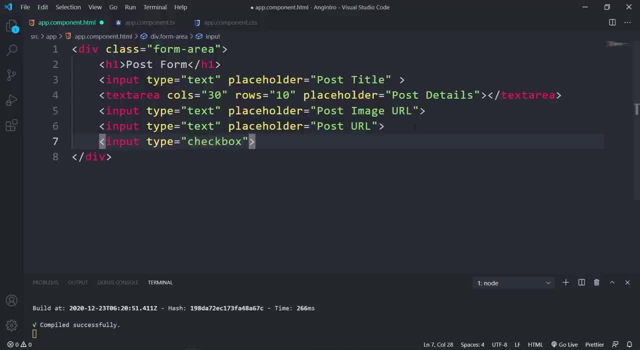 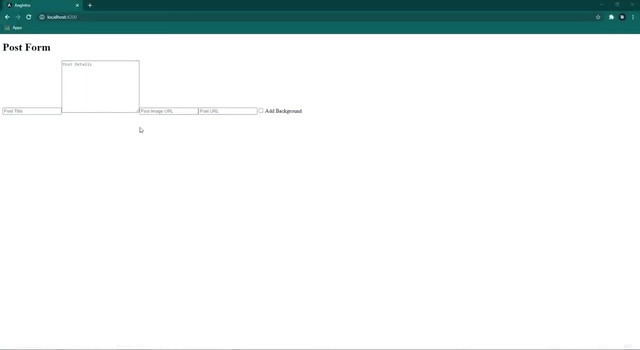 Add text after this input. add this text after this input. add background. So now save this. and back to the browser. As you can see, here, all these input fields are in one row. I don't want this. Make this form vertical. 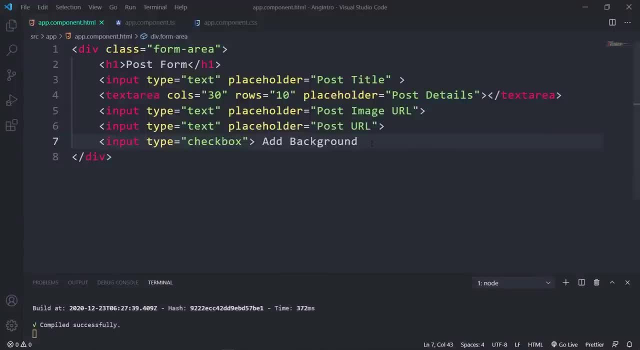 Back to the vs code. We can do this using CSS, but I am not going to do that. Just simply add br tags to achieve the vertical layout. After this h1 tag, add two br tags. copy these br tags and paste it. after these all input. 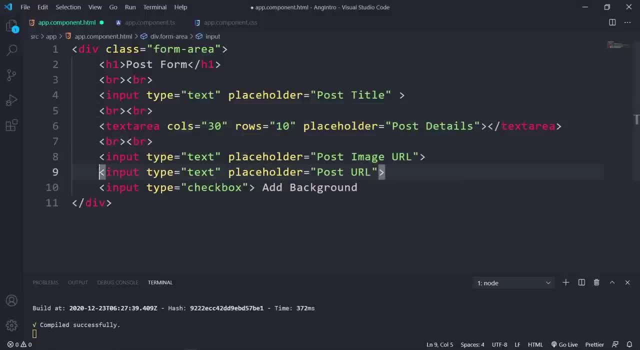 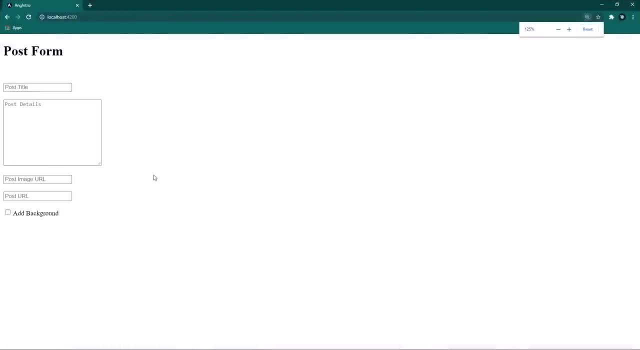 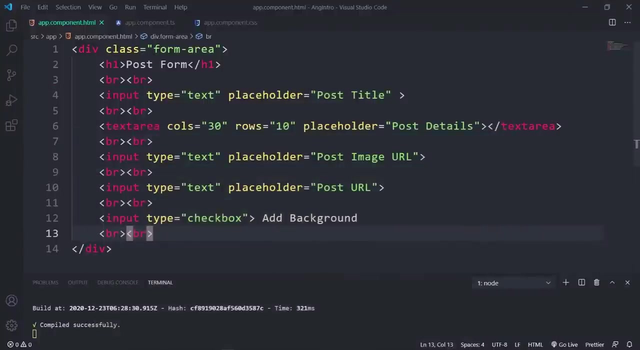 fields. Now again save this and back to the browser. As you can see, here we got this beautiful vertical form. Now let's make this form center. So again back to the VSCode. let's add the style to this Form-Area. 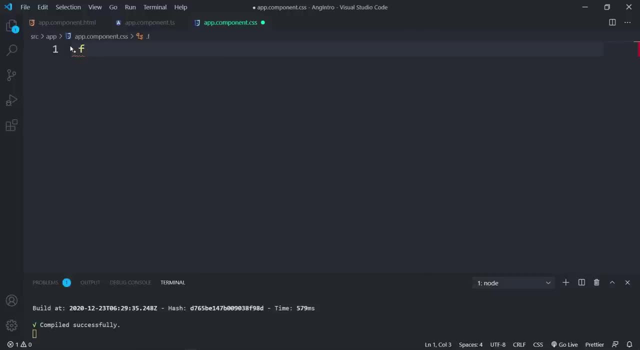 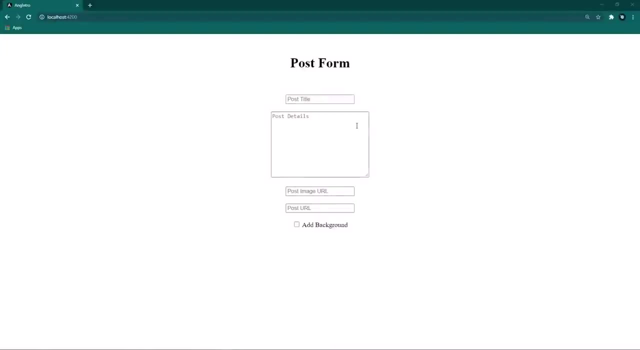 Inside AppComponent CSS file. CSS selector is this class, Form-Area and the CSS scope. Inside this add these CSS styles. So set margin-top to 50px and set text-align to center. Save this and back to the browser. Now this form looks perfect, right. 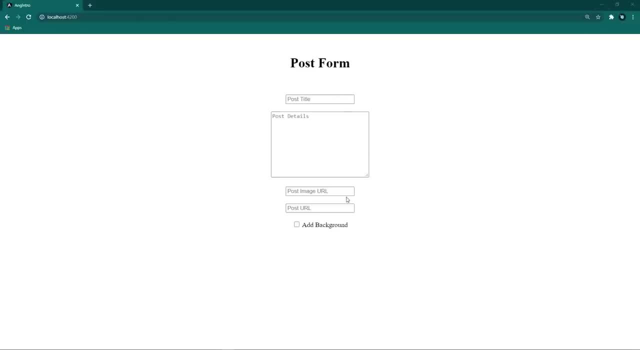 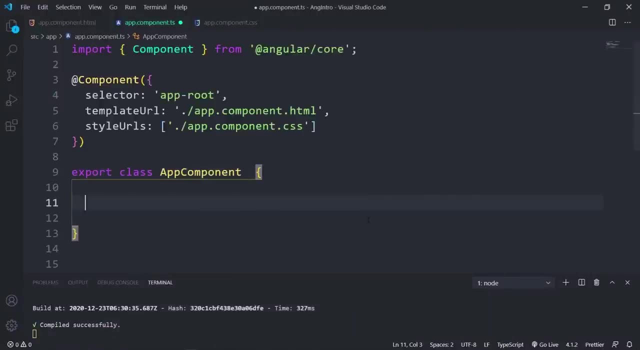 Alright, now let's create TypeScript variables for two-way data binding. So inside the PostComponentts file, the first variable is for the PostTitle, So the variable name is PostTitle. we use the CamelCasing naming convention. The data type is string. 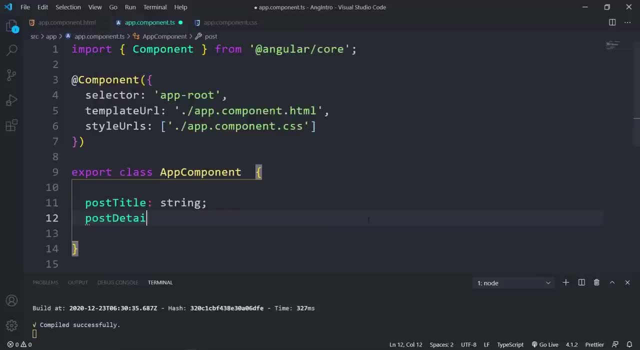 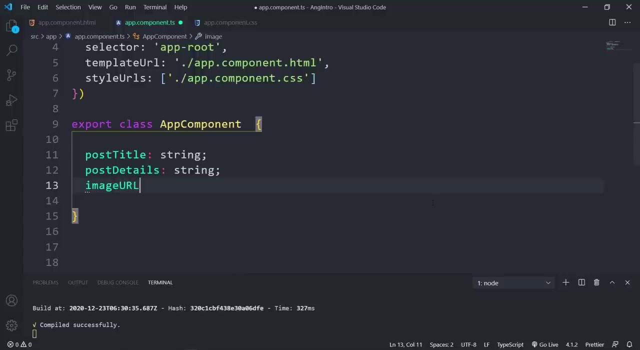 Next for the PostDetails, so variable name is PostDetails. this d is capital, This data type also string. Next, we need a variable for this ImageUrl, So variable name is ImageUrl. this URL old capital Data type will be, as always, string. 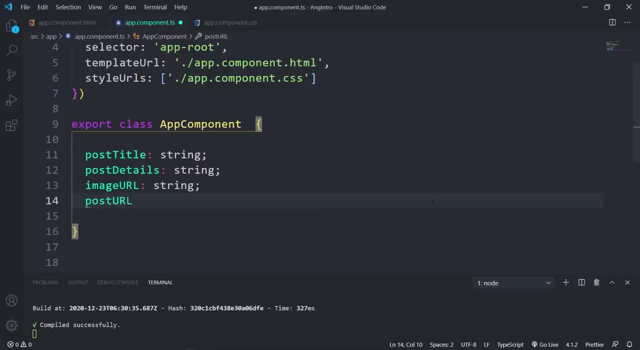 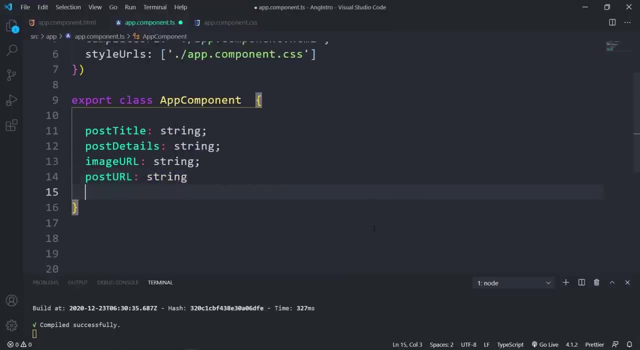 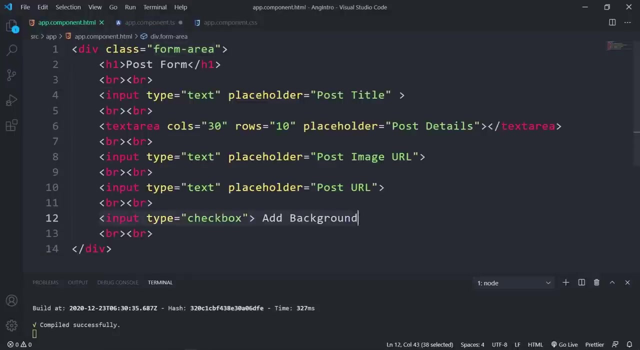 Next, for the PostUrl. this, also same as previous variable data type, is string. At last, we need a boolean value for this checkbox. As you know, checkbox will return boolean values. If this checkbox is selected, the value is true. If this checkbox is unselected, the value is false. 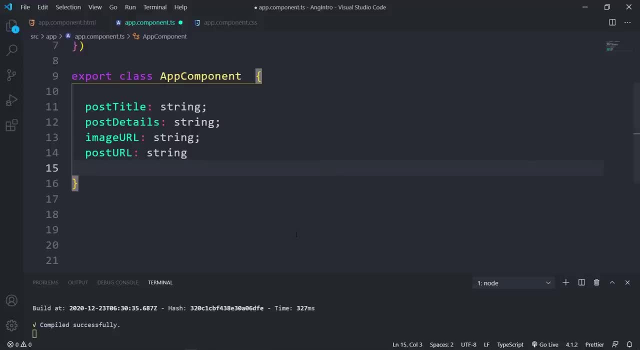 So to bind this checkbox value, we have to create a boolean variable. The variable name is AddBackground. make this be capital. This time, data type is boolean. Alright, we have successfully created variables for all these form values. Now let's do the two-way data binding. 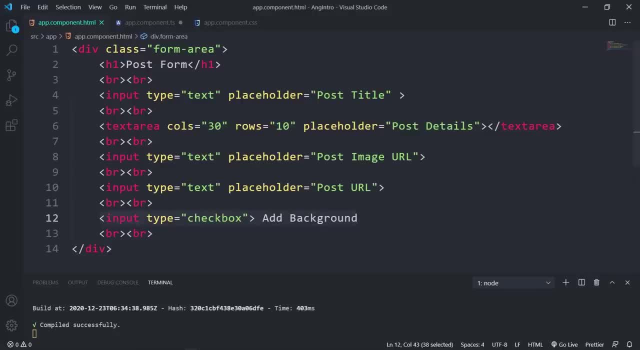 As you know, to create a two-way data binding inside this input tag, first, square brackets. Inside this square brackets add a pair of normal brackets. So inside this brackets: ngModel. After this equal sign: Inside codes pass the variable name that we want to bind to this input field. 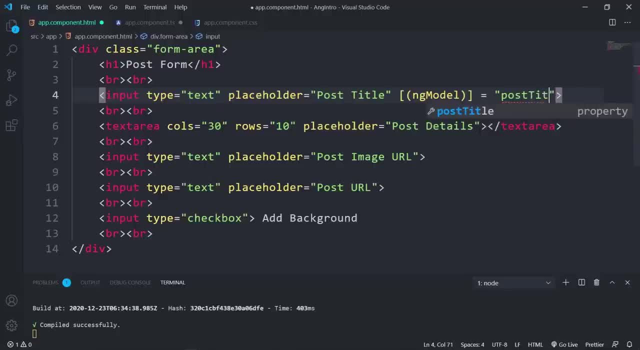 This input field is for the PostTitle, so the variable name is PostTitle. If you can remember, this is how we bind data to a TypeScript variable using the two-way data binding approach. Likewise, bind these all inputs to the relevant variable using the two-way data binding. 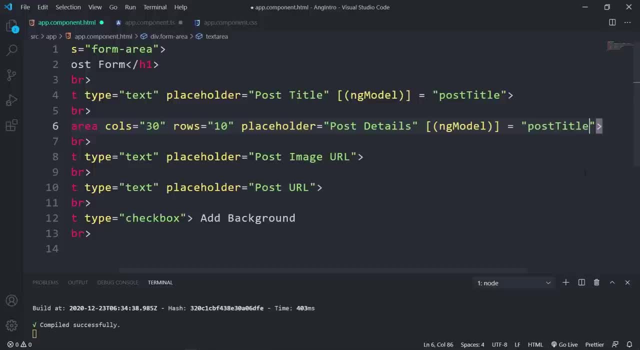 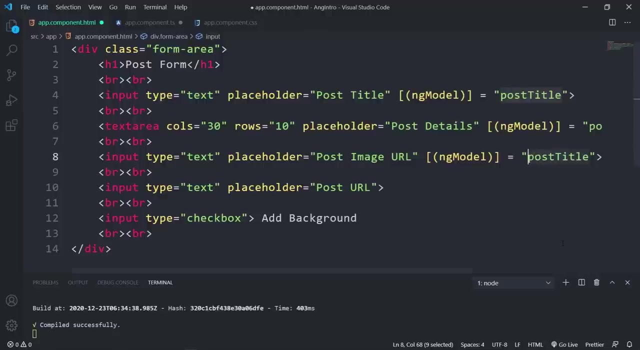 So next one is this text area. So copy this previous ngModel and paste it here This time. variable name is PostDetails. Again, paste the ngModel for this image URL field. Change the variable name to image. Let's paste it Again. paste this inside this PostURL input. 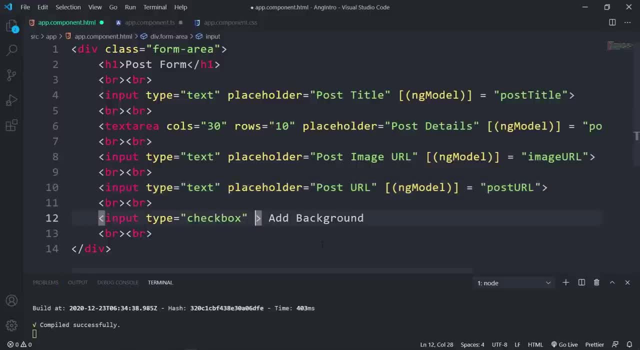 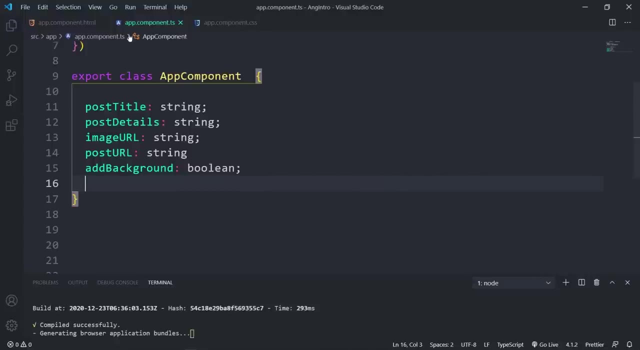 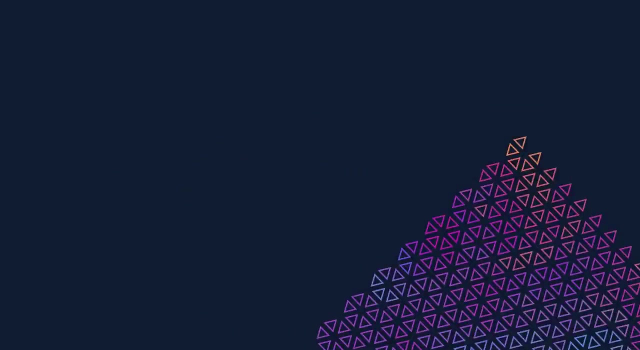 This time, variable name is PostURL. At last, paste the ngModel for this checkbox input and change the variable name to AddBackground. That's it. We successfully completed the two-way data binding. Simple, right, Alright. now let's show these input fields value inside the browser using the string. 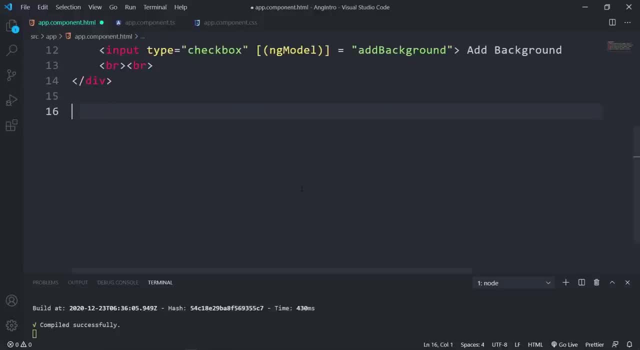 interpolation. So after this form area create another div, PreviewAreadiv, So divpreview-area, and hit enter. This also going to be the same as this form area style. So inside the CSS file add the preview-areadiv class after this form-area. 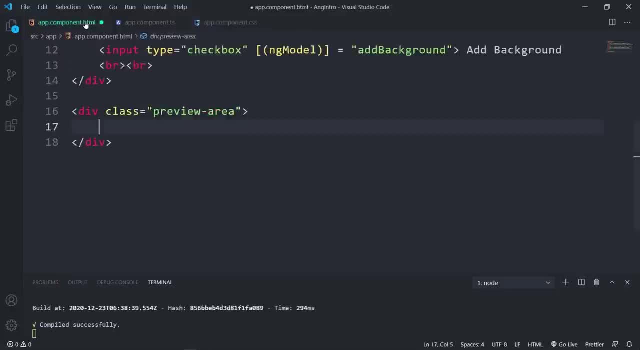 So now save this and back to the html file. Now, inside of an h1 tag, let's render the post title using the string interpolation. How do we do string interpolation? Open and close two curly braces Inside this add the post title variable. 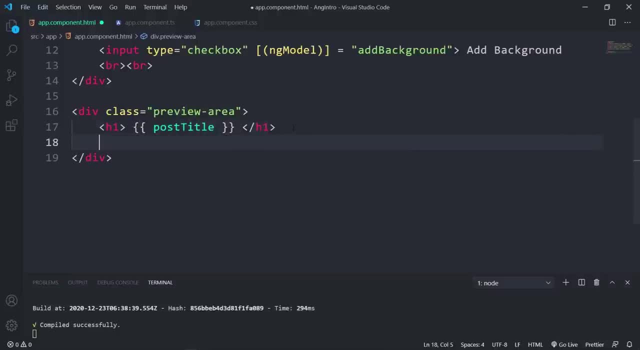 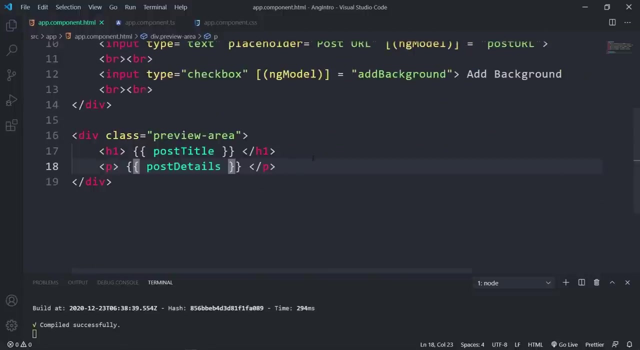 Next let's add the post details inside of a p tag. So p hit, enter Inside this, open and close two curly brackets. Inside these brackets, pass the post details variable. Let's see how this looks like. Save this and back to the browser. 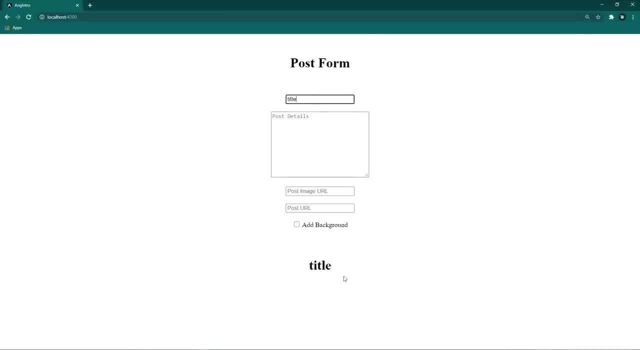 Type something inside the post title. Look at this: When I type inside this text field, this is automatically rendered here in real time. So this is the beauty of this two-way data binding. Again, type something inside this post details. Perfect, We got the post details. 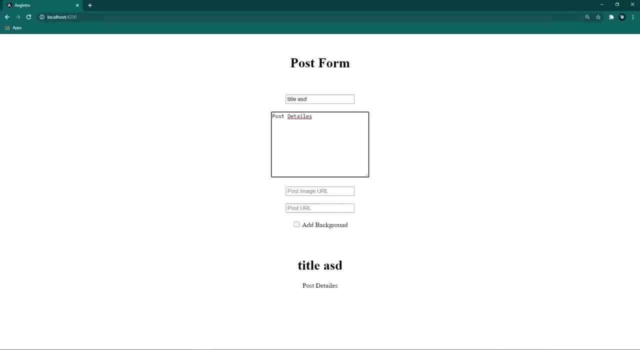 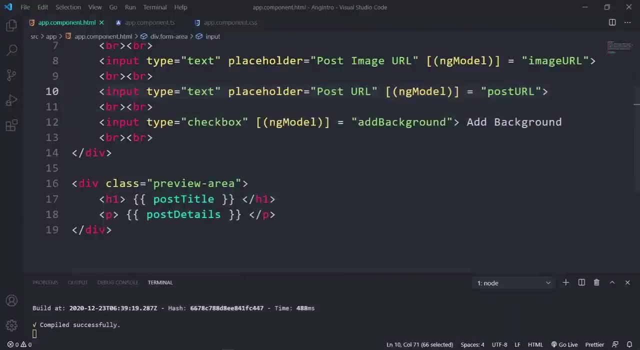 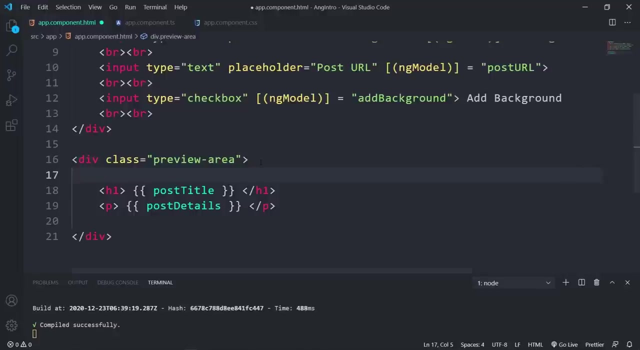 Beautiful. Alright, get back to the work. Next let's show the image when we type the image url inside this input field. So back to the vs code. Let's render the image at the top of this preview area. So img, hit, enter. 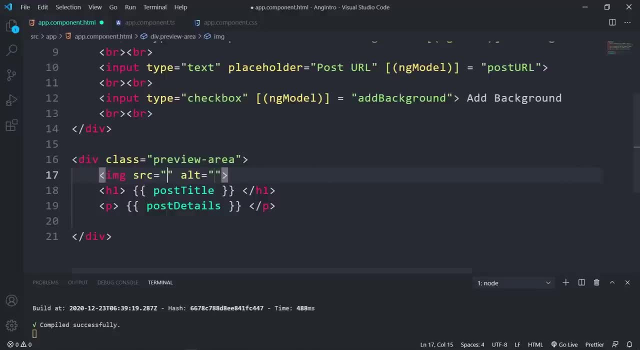 This time we are going to add this image tags src. This is a property of this image tag, So this time we gonna use the property binding approach. So wrap this src inside of square brackets. Now pass the image url variable to this property binding. 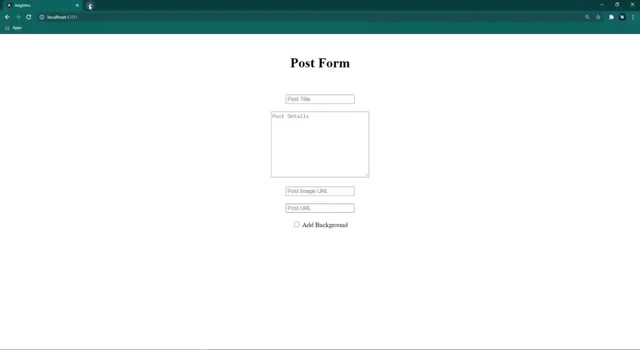 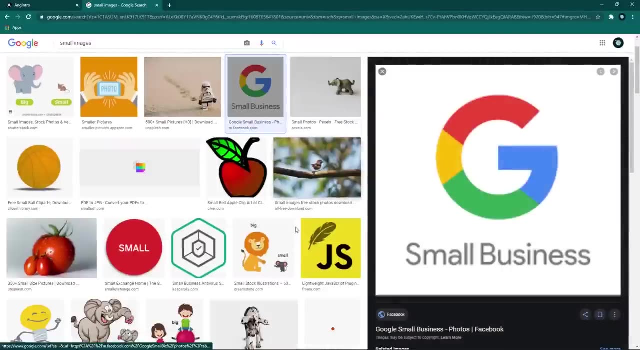 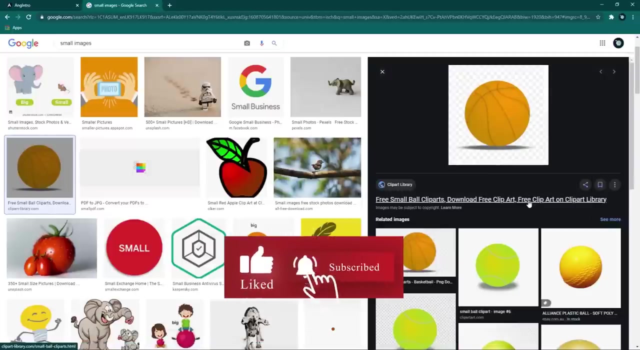 Save this and back to the browser. Add an image url inside this. Let's get an image url from google Search for small images. Go to the image tab and select any of this image and copy the image address. Now go to the avango lab. 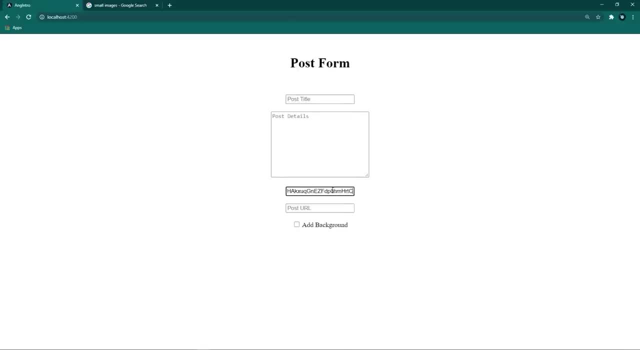 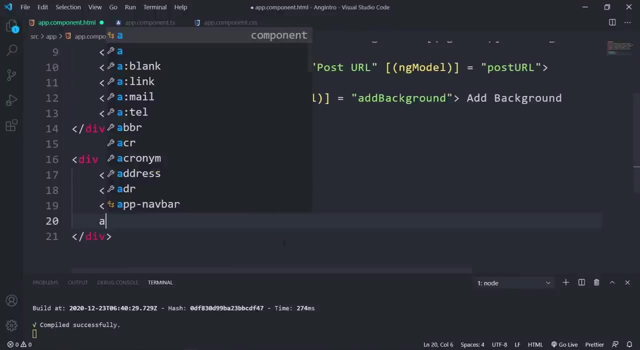 And paste the image url inside this Perfect right. As you can see here, we got this image rendered inside this preview: Beautiful, Alright. next, let's add link tag and bind this post url. So a and hit enter, Let's bind the post url to this href property. 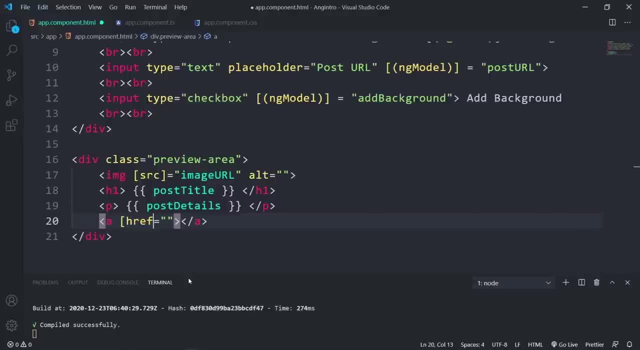 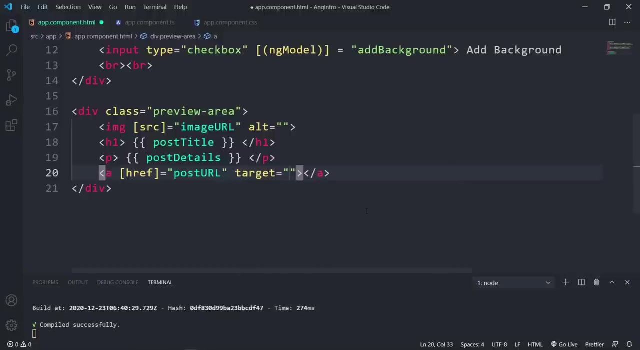 To make this property binding, put this href inside of a square brackets and bind this property to post url variable. Next, I want to load this url inside of another new browser tab when someone clicks this anchor tag, So add this target blank. After this, add this anchor tag text. more details: 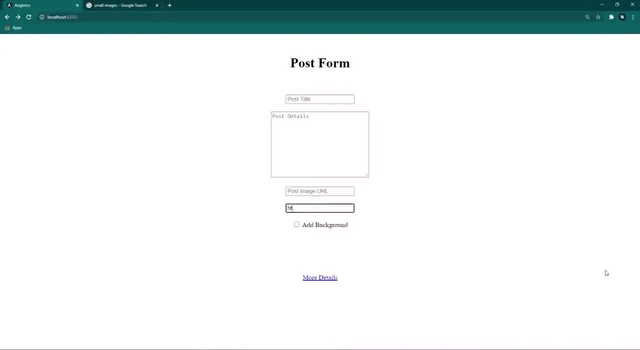 Save this and back to the browser. Just simply add a simple url. I add wwwgooglecom. Now click this. more details. As you can see here, This opened the googlecom inside of another browser tab. Perfect, right, If you noticed here. 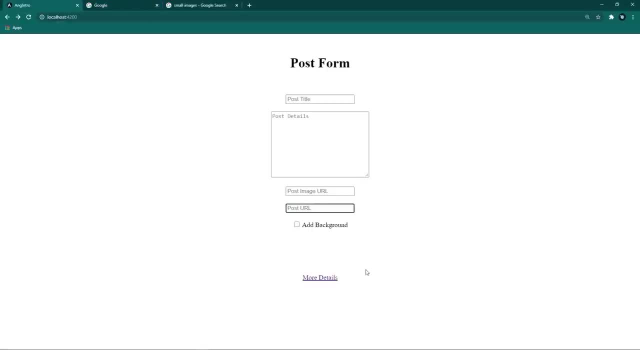 This more details anchor tag is showing here even when this post url field is empty. I don't want that. I want to show this more details anchor tag when this field has a value. Otherwise I want to hide this link. So let's do that. 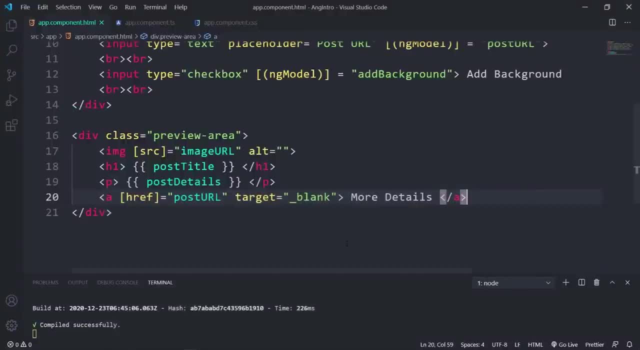 For this, I am gonna use this style binding approach. What I am going to do is, If this post url variable is empty, I am gonna set this anchor tag display none. If this is not empty, I will set this anchor tag display block. 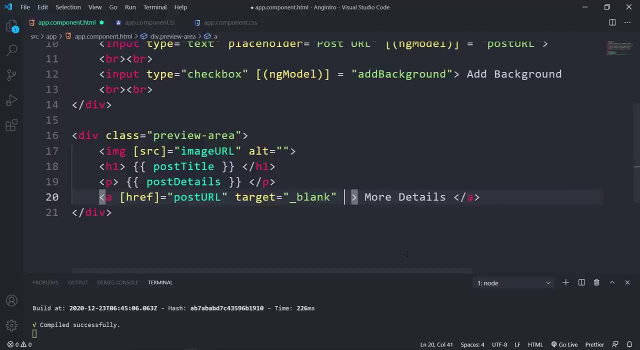 So we gonna use this style binding. So inside this anchor tag, square brackets, Inside this style dot, Then the style dom object property is display After this equal sign. Now let's pass the condition Set double quotes. The variable name is post url. 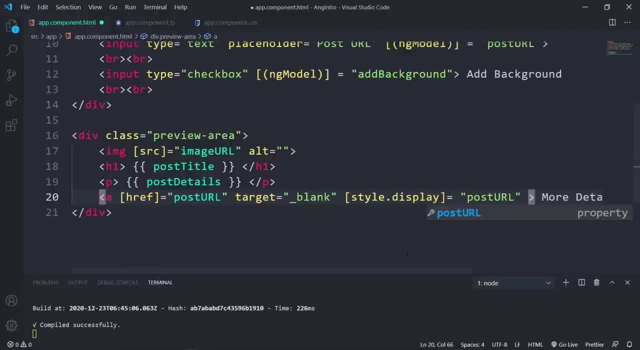 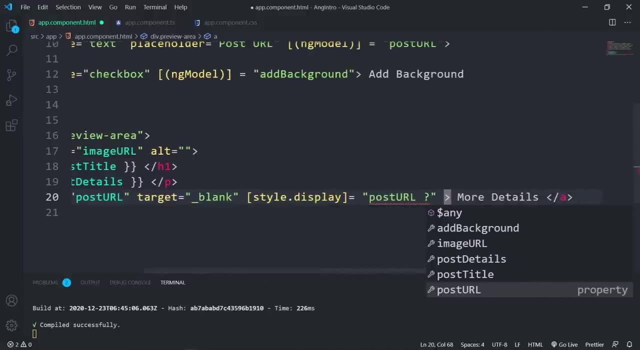 So please carefully follow this capital simple letters, Otherwise you will get errors. Post url After this question mark. Which means, if this is true, Set the display value to block. Insert single quotes. Pass the block Else semicolon So we define else part with this semicolon. 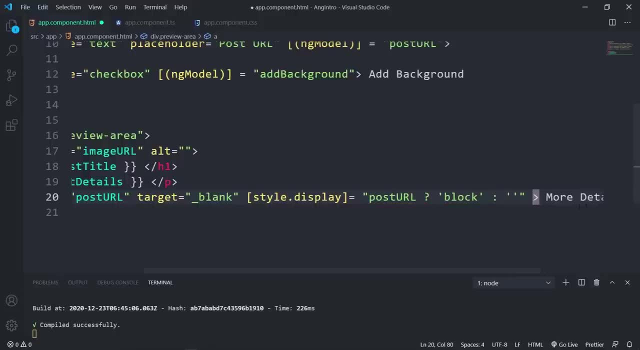 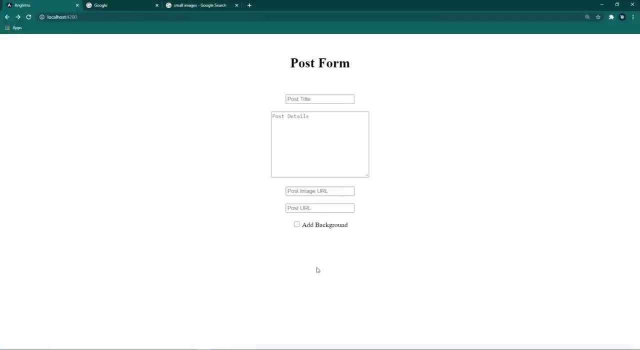 Set this to display none. So this is the display value. So inside single quotes: none. So now save this and back to the browser. As you can see here, Now we cannot see the more details link If I type a link inside this post: url. 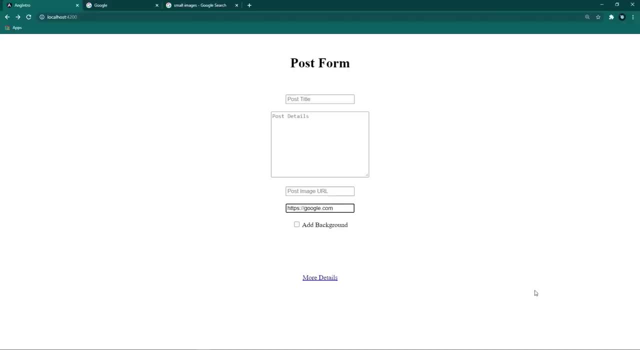 We got this more details link. If I again remove this url, Look at this. Now. we cannot see the more details link. Perfect, right, So alright. next let's do the background effect For this. I want to apply a background color to the post title. 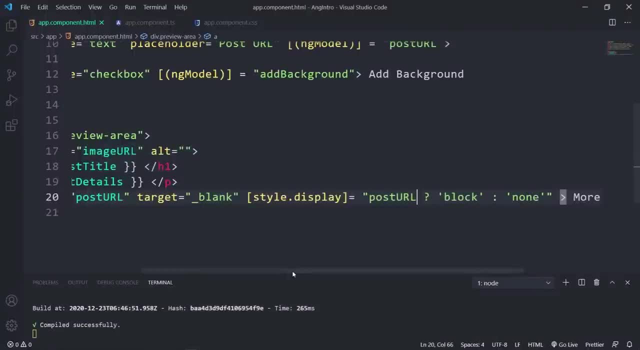 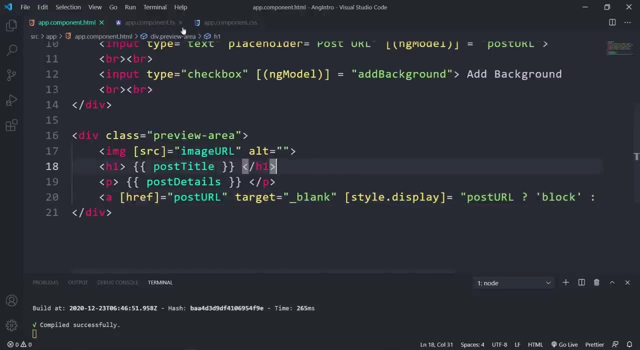 And this checkbox selected. Let's do that. This is also very simple. For this, let's use the class binding approach. Before that, let's add a style. Go to the app css file For the css selector. we gonna use a css class. 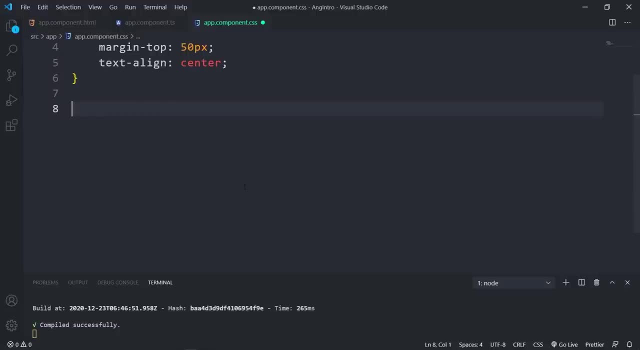 Coz. now we are going to deal with class binding. Let's name this css class something add-background After this css scope. Inside this, set the background color to yellow And set the padding to 10px. Perfect, Now our add-background css class is ready. 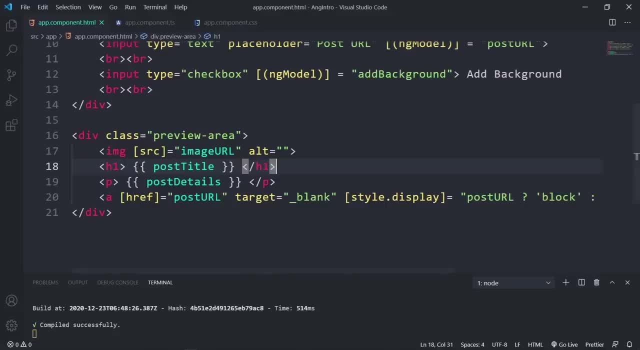 Alright, let's do the class binding Inside this h1 starting tag. Open and close a square bracket Inside this we are doing the class binding. So class after this: dot next The css class name that we want to add: Add dash background. 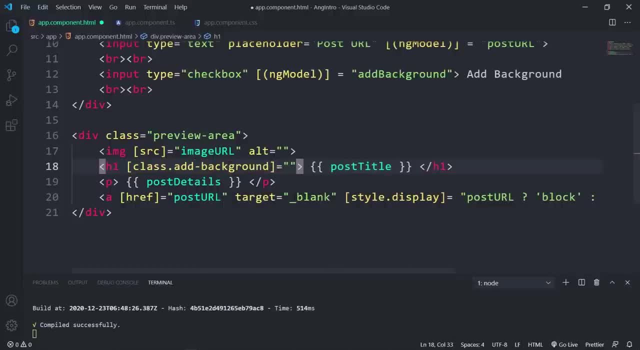 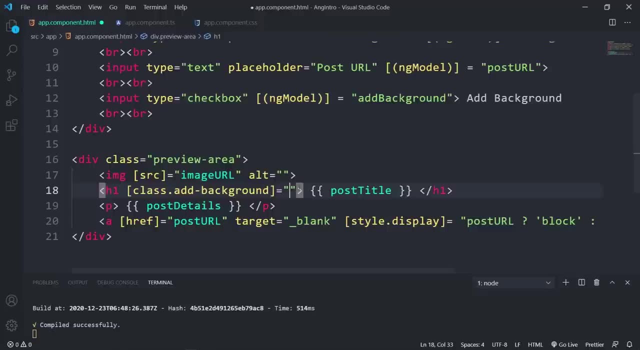 Next, equal sign And after this, inside codes: pass this variable add-background, which is bounded to this checkbox. That's it Very easy, right? When someone checks this checkbox, this add-background variable will set to true. If this is not checked, this will set to false. 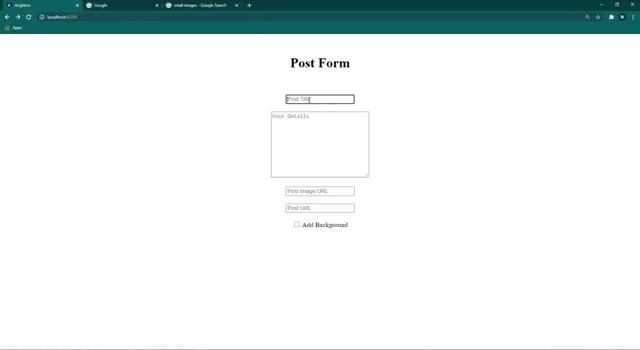 So save this all and back to the browser. Type something inside this post title. Now check this checkbox. We got this background yellow color, But this is applied to this full row. I don't want that. I just need to apply the background color only to this title, not to this whole row. 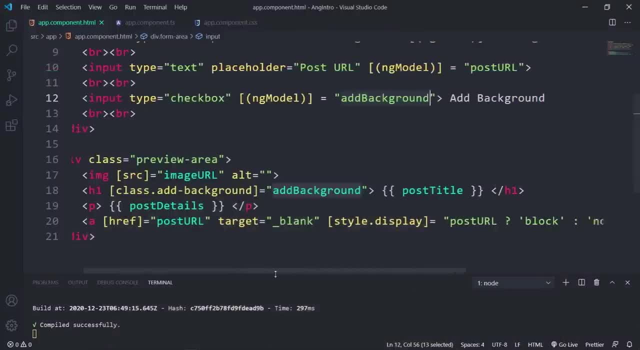 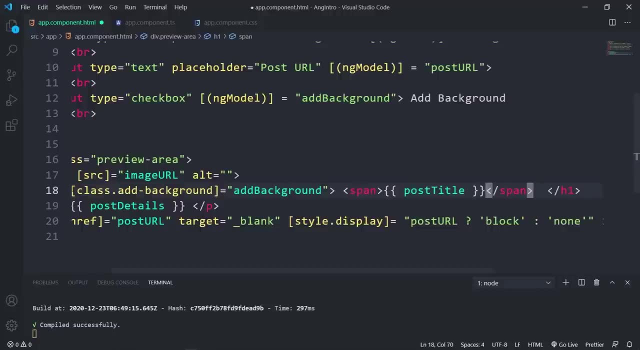 To solve this. back to the vs code Inside this post. title: h1 tag: create a span. Put this string interpolation inside the span tags. At last, remove this binding from h1 tag and put it inside this span tag. Now we are done. 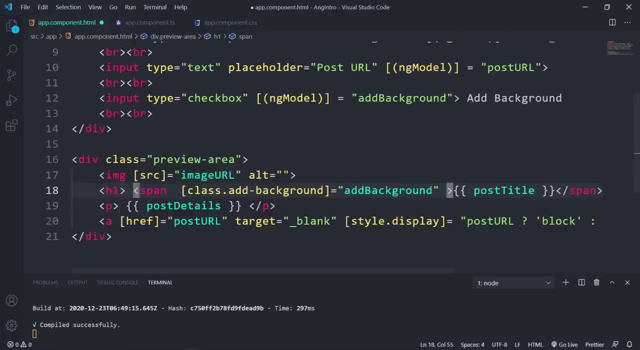 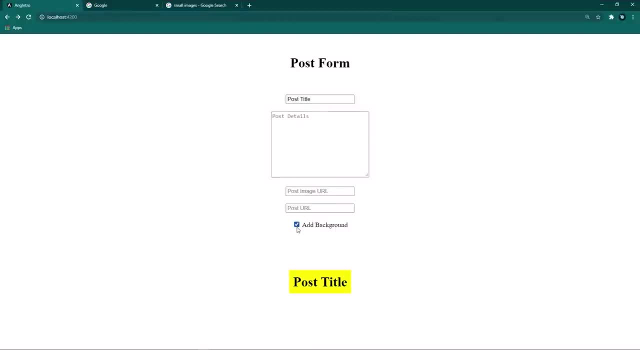 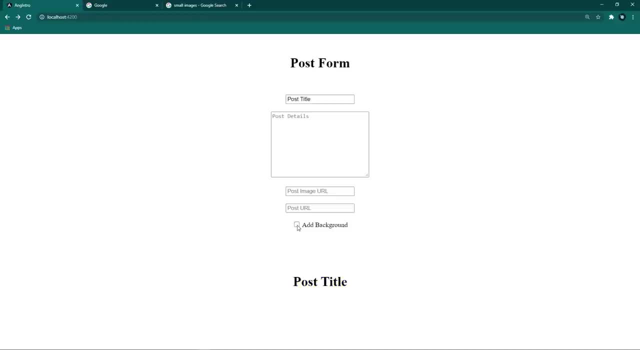 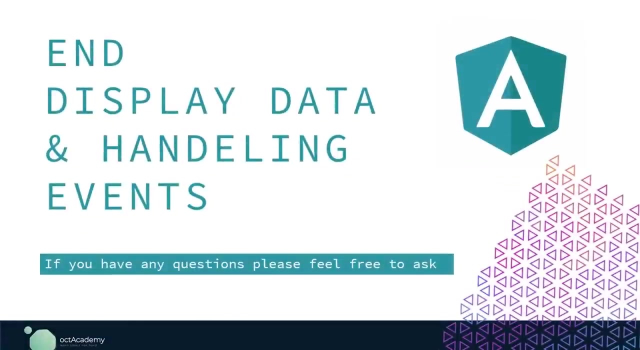 This time this remove the background color. Perfect, So this is the end of this task. Hope you guys got the idea. All right, This is the end of this section. So for this section, We learned about how to handle data and display data in angular. 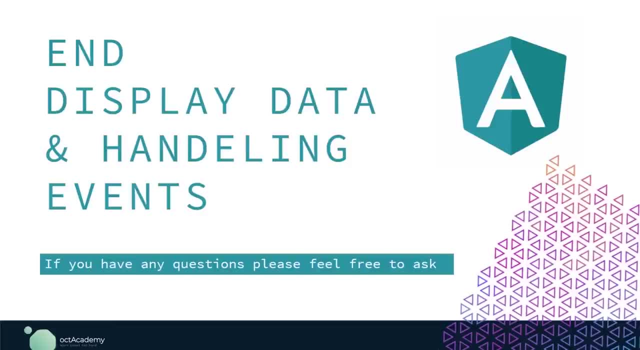 We learned about string interpolation, property binding, class binding, style binding and, at last, we learned about two-way data binding. and also we learn how to use this two-way data binding by doing a small task. If any of you did not get any of the parts of this section, go back and learn it again. 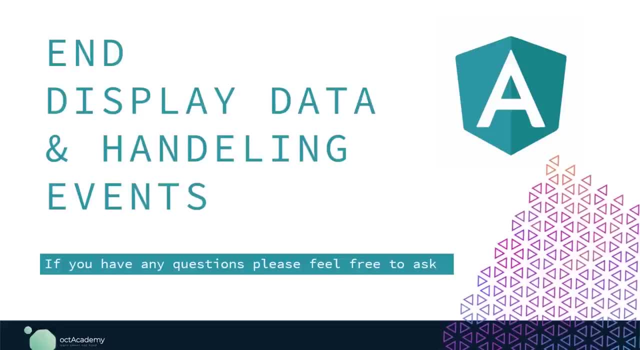 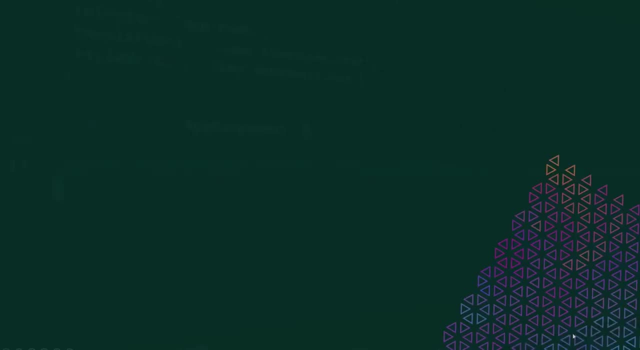 If you still don't get it, learn it again. Never give up. And also, as always, if you have any questions, please feel free to ask in the Q&A area. All right, We'll meet you in the next section. So in this section we're going to learn about angular directives in detail. 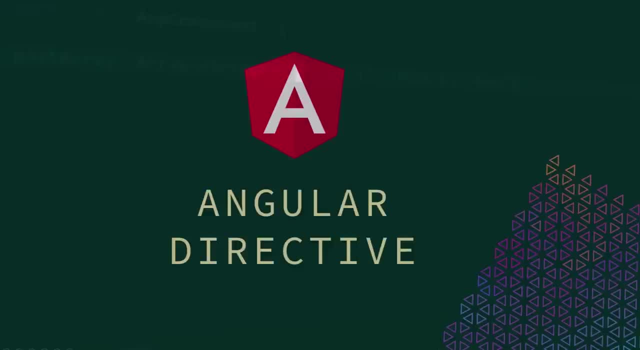 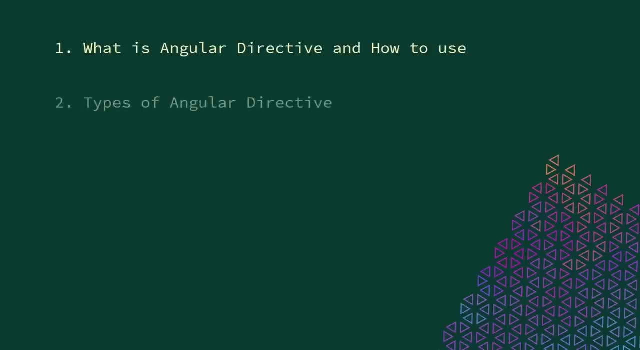 At the end of this section, you will know what is angular directive and how to use that. Types of angular directives. Type of angular directives. Type of angular directives. Type of angular directives About NG directive, NG template directive, NG switch cases directive. 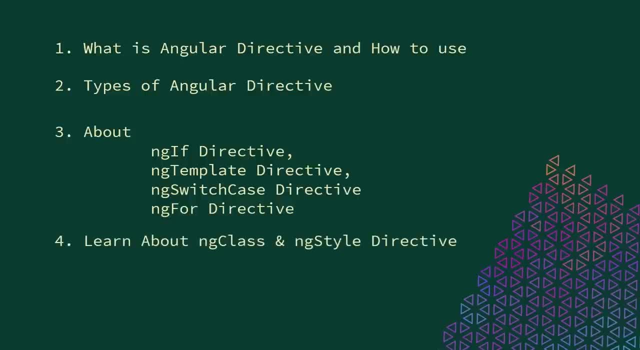 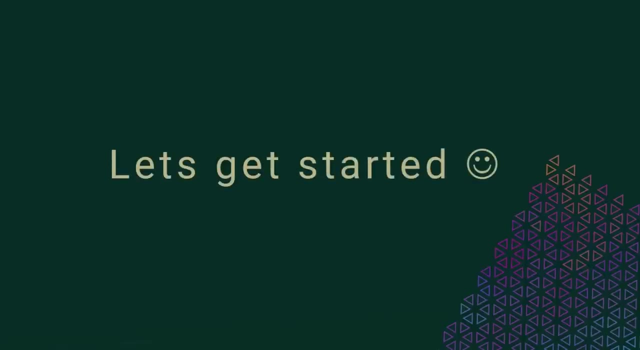 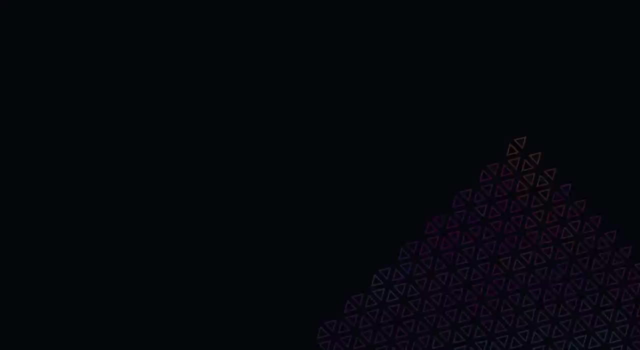 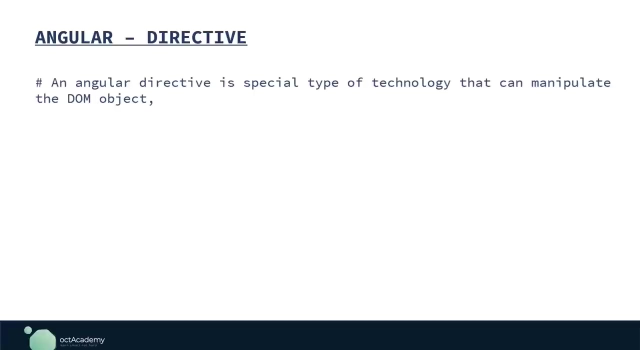 NG4 directive, And also we will learn about the NG class and NG style directive. At last, we will learn about the difference between structural and attribute directives. So this section is going to be awesome. Let's get started. An Angular directive is basically a special type of technology that can manipulate the 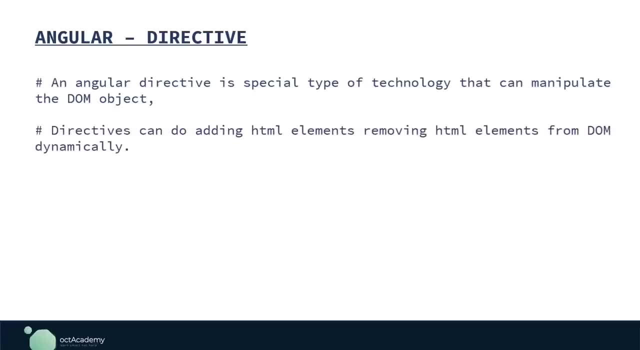 DOM object, like adding HTML elements, removing HTML elements from DOM dynamically. Directives are one of the very, very important feature in Angular. In the previous video we learned about Angular components right, So this Angular component also including to this Angular directive category. 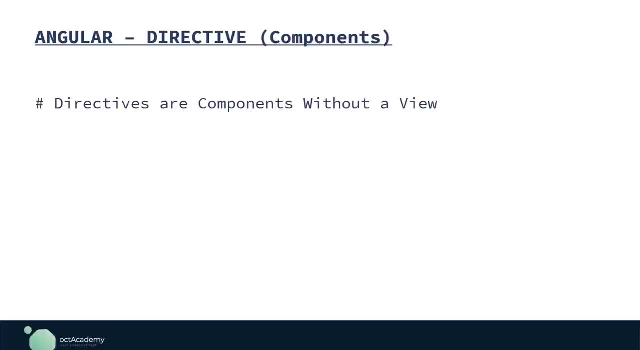 Directives are components without a VIV. They are components without a template. or to put it another way, components are directives with a VIV. Everything you can do with a directive, you can also do with a component, But not everything you can do with a component you can do with a directive. 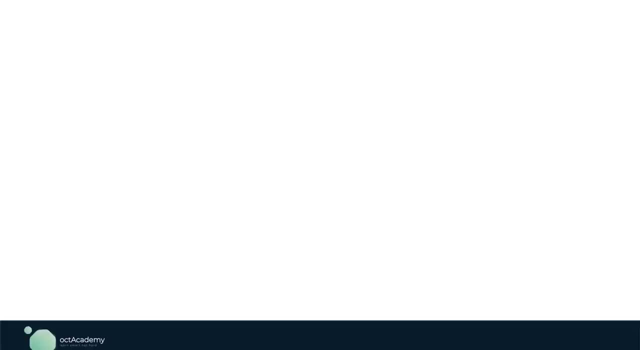 Alright, in Angular we have four types of directives: Component directive, structural directive, attribute directive and custom directives. So this first type of component directive, which is an Angular directive with a template VIV, So we already know about this Angular component as this template VIV HTML page. 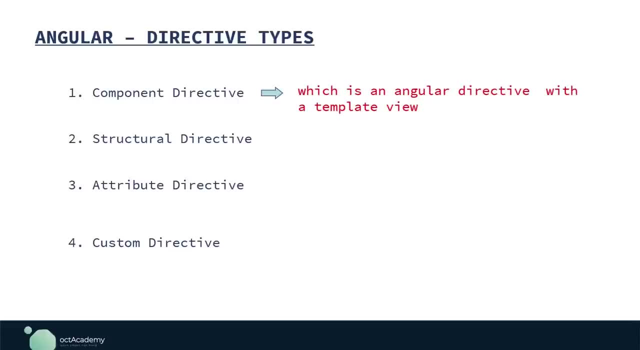 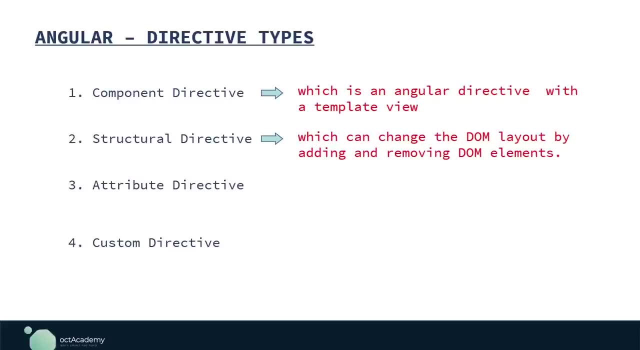 Using this type of angular directive, we can change the DOM layout by adding and removing DOM elements. With this, we can change the appearance or behavior of an element, component or another directive. At last, we got this custom directive. With this, we can create our own custom directive from scratch. 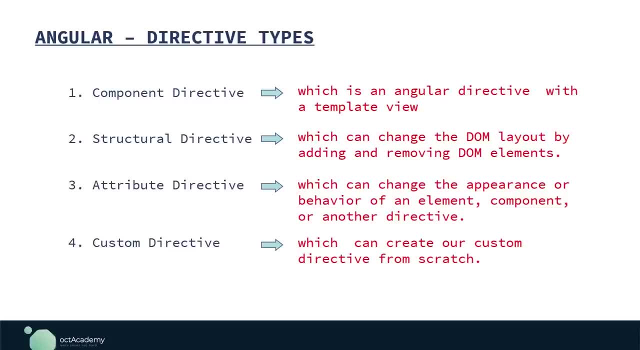 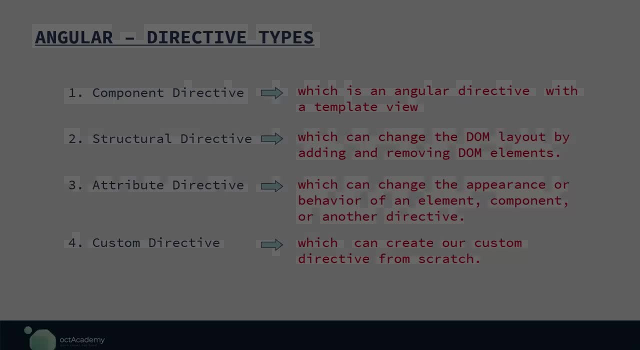 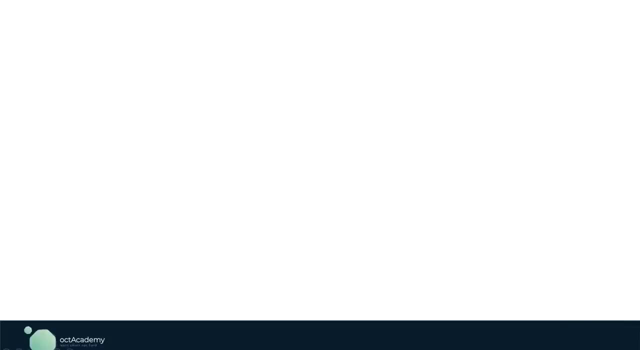 Yeah, I know these definitions may got confused you, but don't worry, we will learn about these all types of directives one by one. Alright, in this video let's look at the first directive, ng4.. We use this ng4 angular directive to render an array object inside of the array. 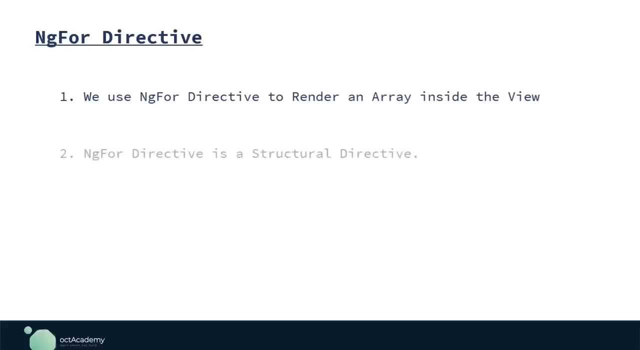 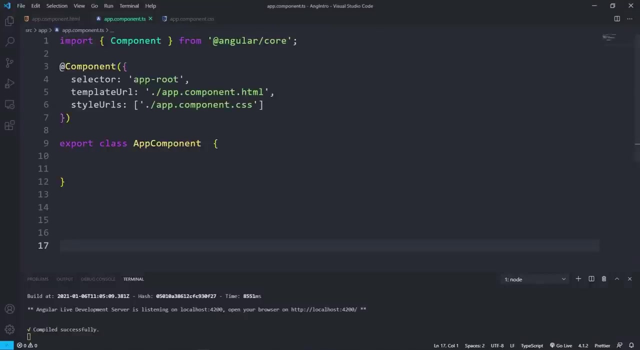 This ng4 is a structural directive coz. using this ng4 we do DOM manipulation, such as adding, removing HTML elements to the DOM. Let's see this in action. So, inside the AppComponentts file, create a simple array for a list of POST. The array name is POST array. 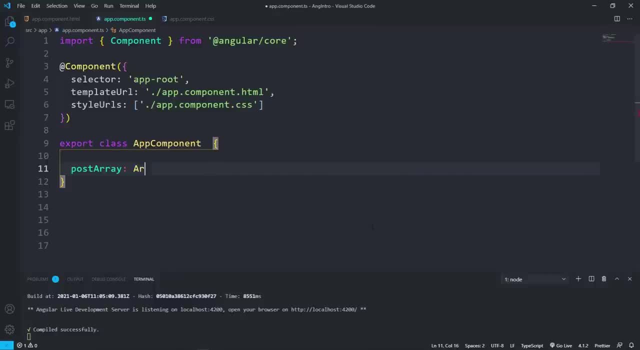 Make this A capital. The type is array And the array type is string. Now assign these two simple array values inside of square brackets. The first value is POST1.. Put this inside of the codes, coz we are creating a string. data type: array. 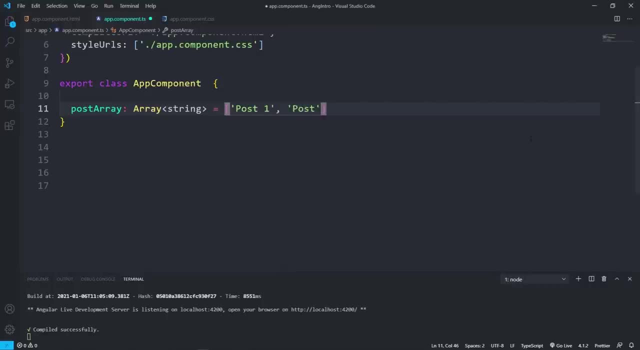 The second value is POST2.. Likewise POST3, POST4 and POST5.. Now I want to show this POST array inside the browser. As previous, we can use the string interpolation for this. Let's do that and see how it looks like. 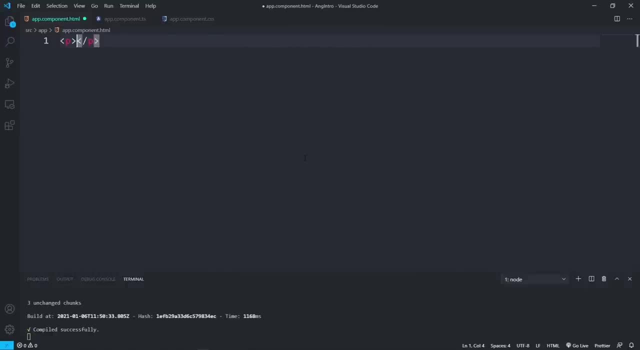 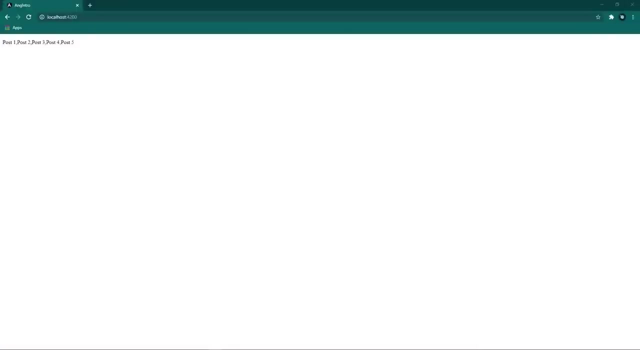 Inside this gmail view page, Inside of a P tag, let's add this string: interpolation, Double curly brackets Inside this array name is POST array. Save this and back to the browser. As you can see here, we got this array printed here. 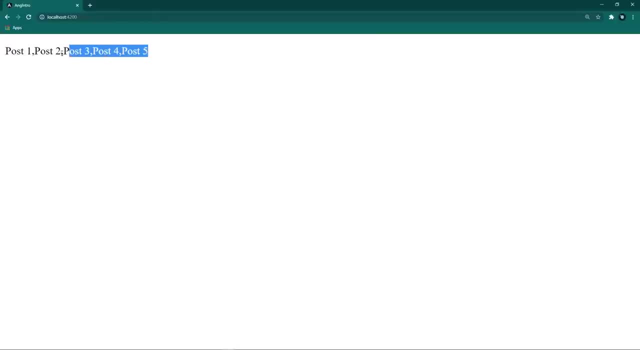 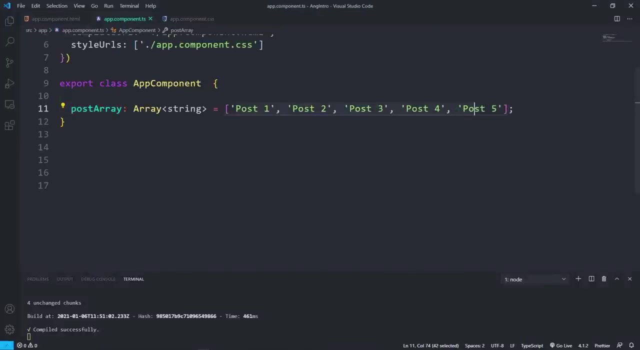 But this is actually not looking good. right, All array values stacked in one line. So now I want to render this array values one by one inside of an unordered list. How do we going to do that? Now we know inside this array we got these five values, coz we hand coded this array. 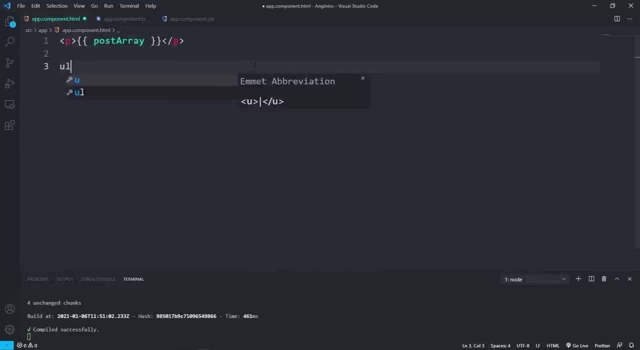 So we can render this one by one, something like this: Create a ul tag with five li tags. Inside this first li tag, We can use the same approach as previous string interpolation. This time I am gonna print the first value of this array, rather printing all values, like. 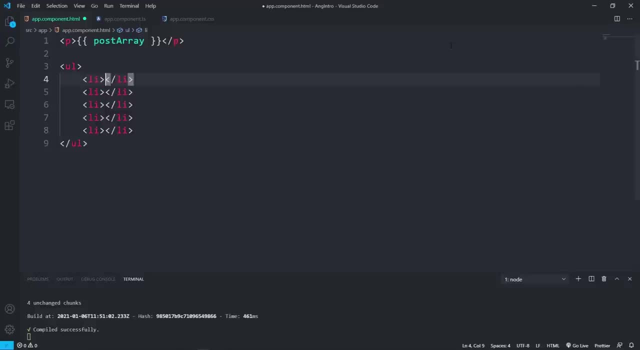 previous. So from an array we capture single data using the array index number. So first the array name, POST array, Inside square brackets. to print this first array value inside this li tag we have to pass the array index. This is the array index number, which is zero. 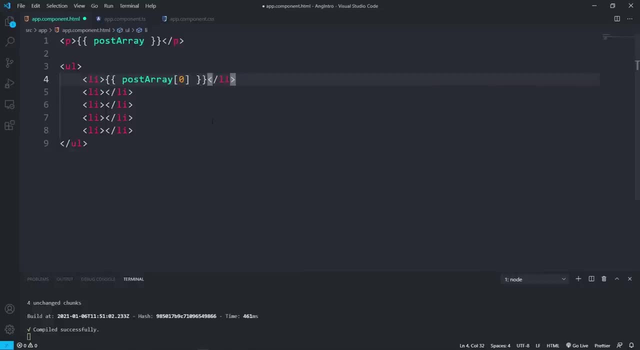 Hope you guys already know about the array. Array index start with zero, not with one. So the index of this first value is zero. After this, inside this second li tag, this time the index number is one, Next two, Likewise three And four. 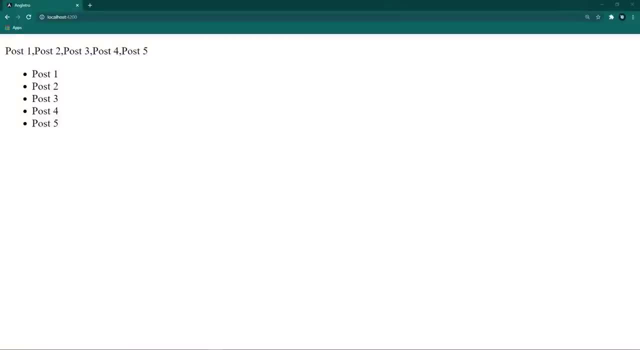 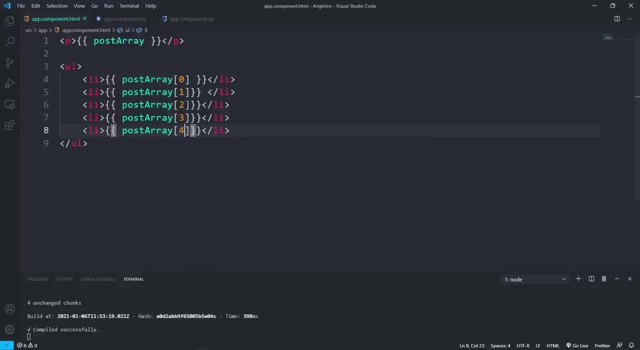 Now save this and back to the browser. This time we got this beautiful list instead of previous ugly stacked array values. Alright, Now this is ok, But this is not the best approach to fetch a list of array values. We did this string interpolation approach coz we know the array value. count coz we hand. 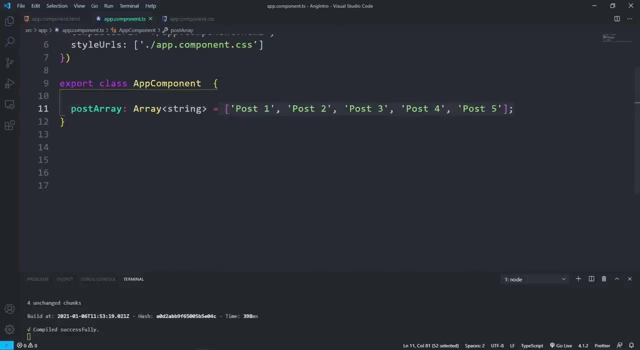 coded this array. Think if there is a situation We are getting this array from the database and we don't know the length of this array. In that case we cannot use this string interpolation approach directly. In that case we don't know exactly how many values are inside the array. 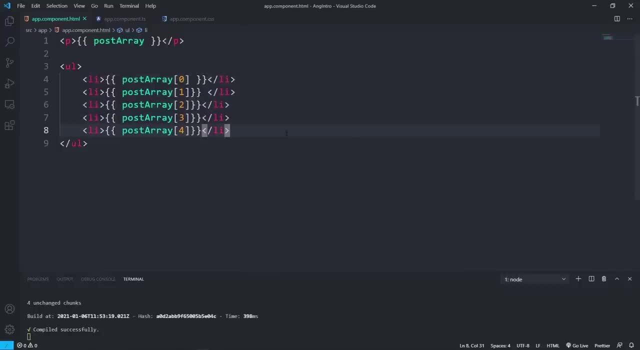 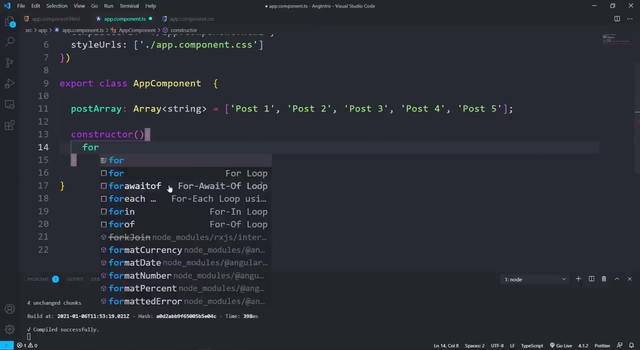 As solution for this situation, we can use the ng4 directive. Normally we use for loop to fetch an array in javascript, Something like this: So inside the constructor method, follow keyword, then the logic Inside the brackets: let i assign zero, coz array starts with zero. 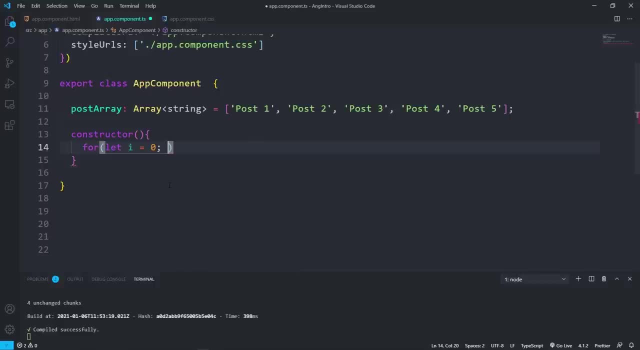 Semicolon. Next we will define the follow condition: i, this, i variable smaller than this: dot post array, dot length. With this condition we are telling to the array: So inside the constructor method, follow keyword, then the logic inside the brackets. So inside the constructor method follow keyword, then i this, i variable smaller than this: 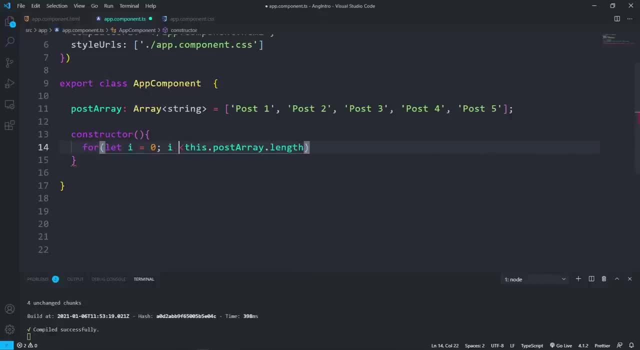 dot post array dot length. Another system we use is the loop. In this particular method we use the loop. So until this i variable is less than this array length. After this semicolon, and add an increment to this: i plus plus. Alright. 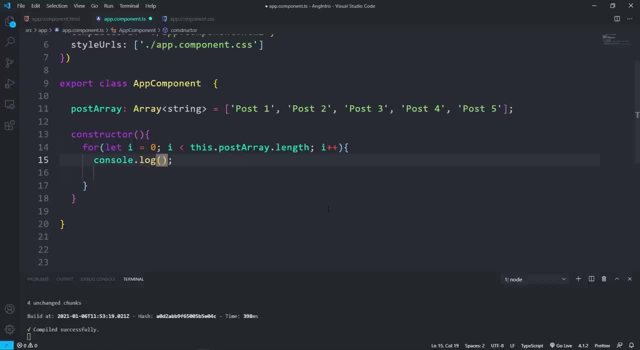 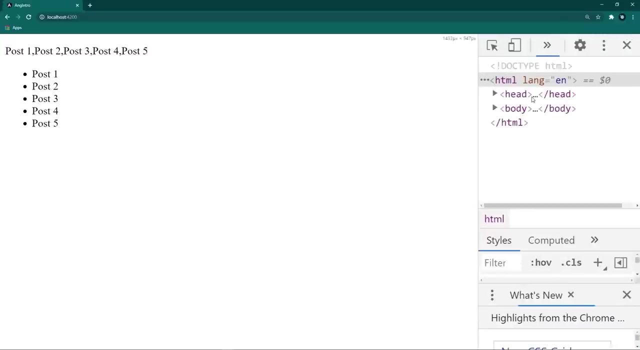 Inside this for loop: log the array values Log: Hit. enter. Inside brackets: post array. Inside square brackets the array index we represent with a combination. After this, we'll assign an increment to this array represent with this: i variable. Save this and back to the browser. Look at the browser. 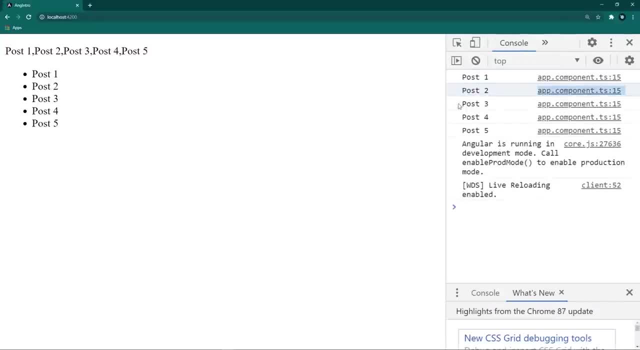 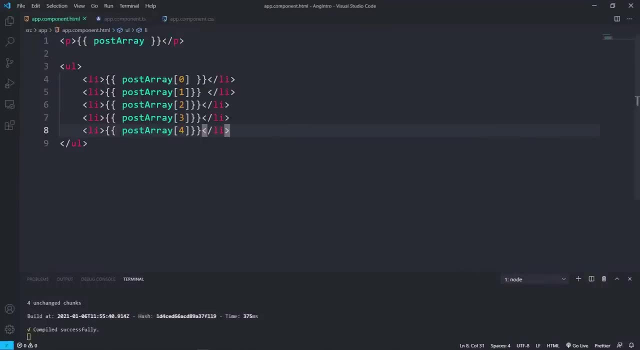 console. We got this array values printed one by one, So this is the javascript way. But in order to render this array values inside the weave template, we use angular ng4 directive. So let's see this in action Inside the html file. we gonna render this inside of an unnoded 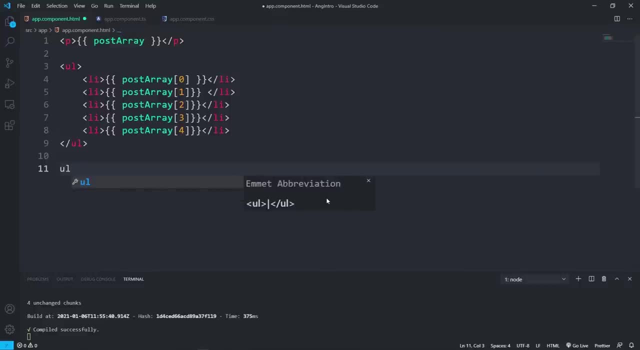 list like previous. So after this, create another ul tag. This time we need only one li tag. Now, inside this li tag, asterisk for the star symbol ng4.. This f is capital. After this, assign inside quotes: let post of post array. 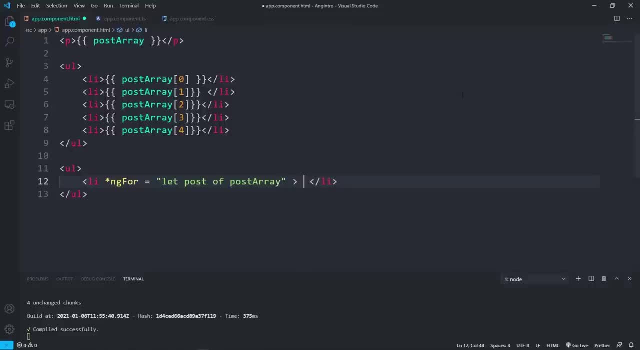 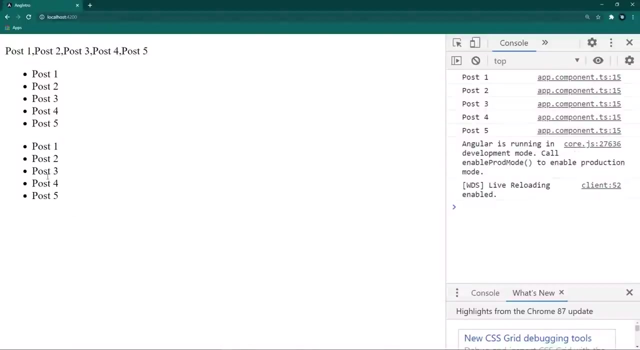 After this: inside this li tag: Now we can use the string interpolation to show this array values: Open, close. two curly braces Inside this post, which is this post variable. Save this and back to the browser. Look at this. we got this list of post which is fetched using the ng4 directive. 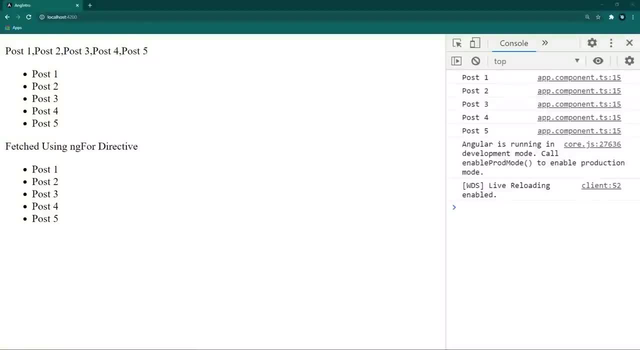 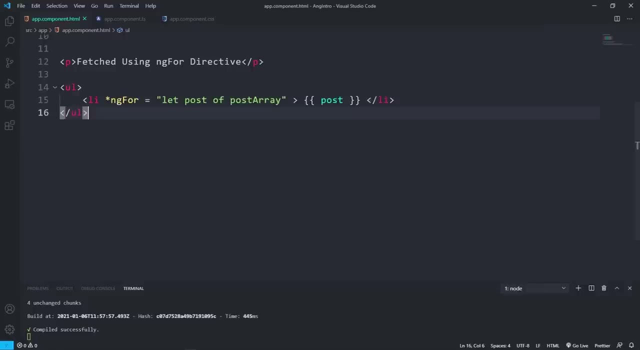 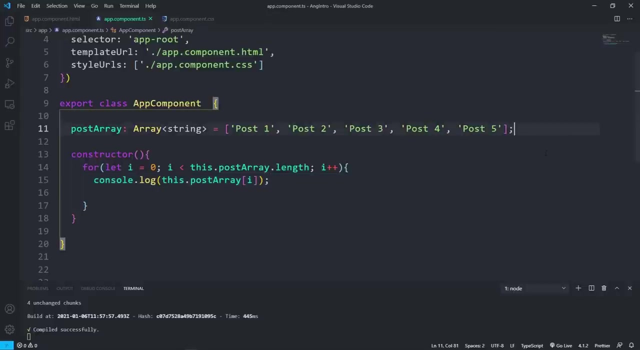 In previous we fetched this stringarray using the ng4 directive. Now let's look at how to fetch an object array using the ng4 directive. This also the same as the previous string array. First, let's create an object array inside the component ts file, The array variable. 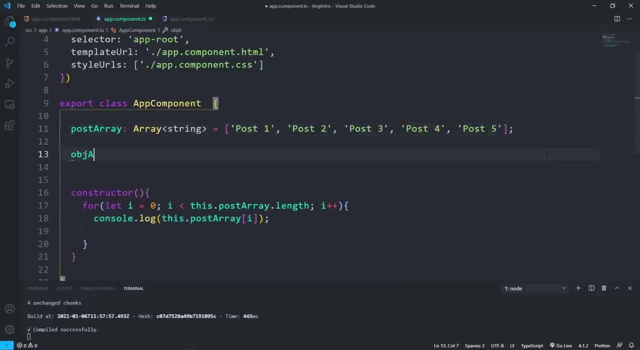 name is objArray. This a is root for std S ar deciding the fine std functions for this Class� to look at. compare with our previous string array. First let's create an object array inside the component ts file. The array name is objArray. This a is 하는. 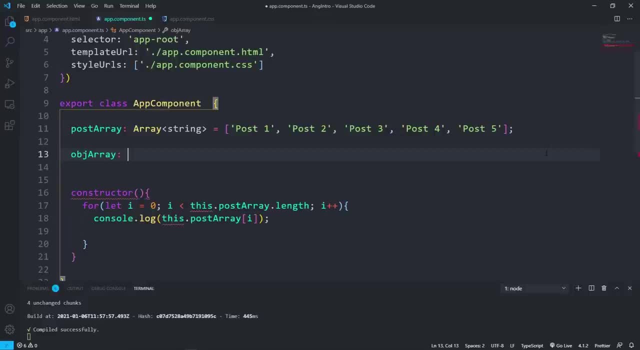 is capital, the data type is array and the array type is object. Now assign this to a list of array objects: square brackets for define array. inside this lets create an object. we create object using the curly brackets. so open and close curly. 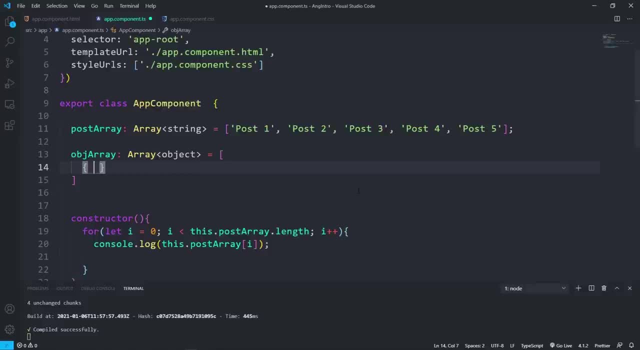 bracket inside. this lets pass the object key and value. So as a first object key value pair, add this: the key is id and value is 1,. after this comma, next object key value pair is post title and value is post 1,. put this inside quotes, coz. 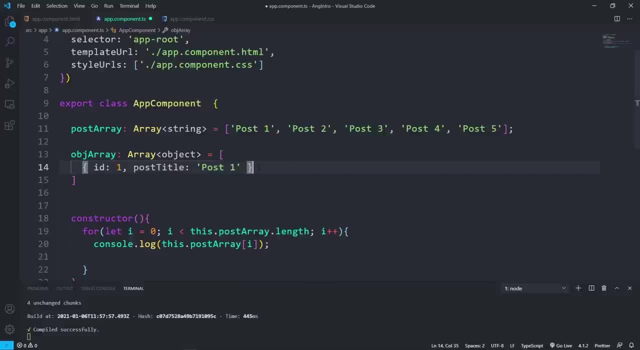 this value is a string like this: create 4 more objects. copy and paste this and add code. The id is 2 and the post title is post 2, id 3, post 3, id 4, post 4,, at last id 5 and. 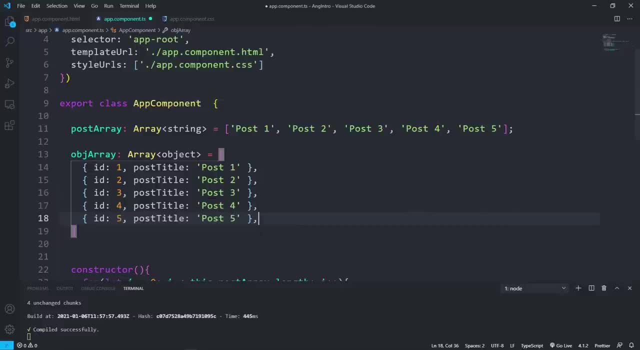 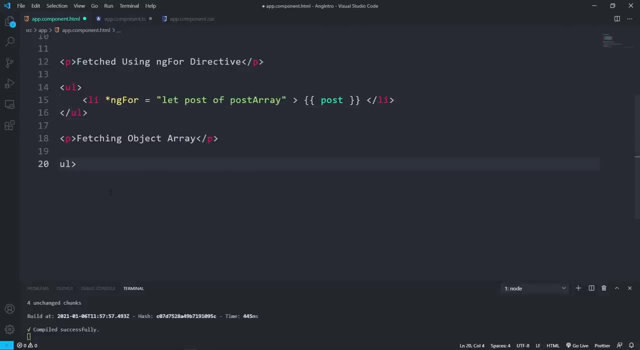 post 5.. Now lets fetch this inside the browser using the ng4 directive back to the html file and create a ul tag with one li Inside this li tag asterisk ng4,. assign inside quotes: let post of obj array so this: 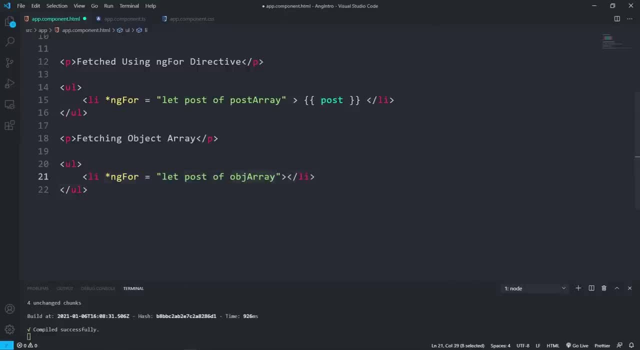 is the new variable and this is the object array variable that we created inside the component typescript file. So inside this li tag, lets print this using the string interpolation: open and close two curly brackets And the variable name is post. save this and back to the browser. 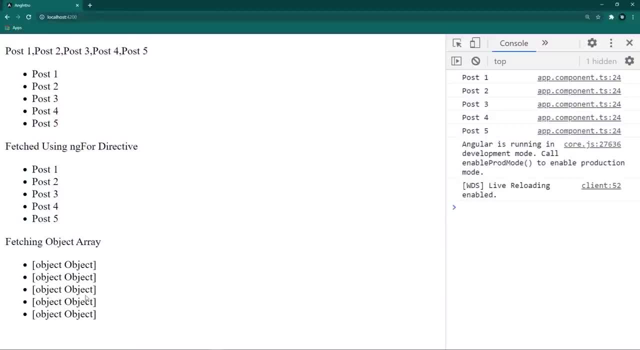 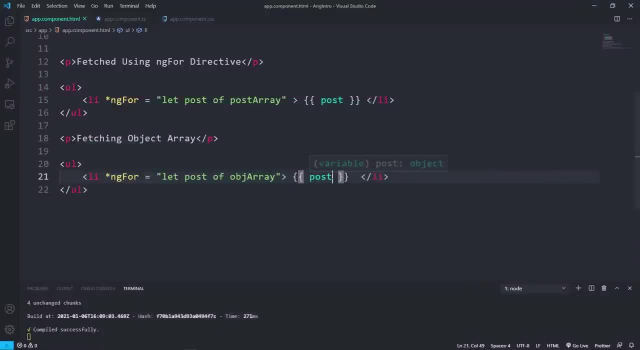 As you can see here, we got this object object printed here. What's going on here? In order to show an object inside of the html view, we have to convert this to a json value. We cannot directly show an object inside the browser view. that's why we are getting this. 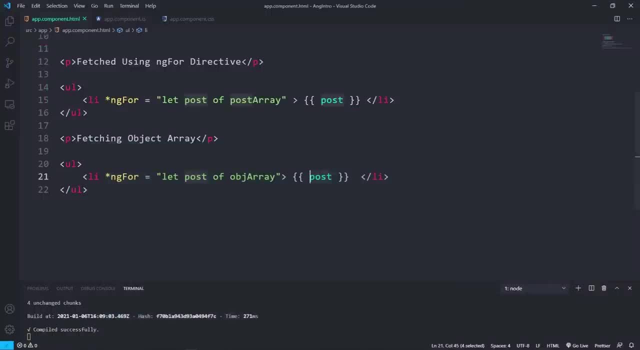 object: object printed here. To solve this, we have to convert this to a json format data So we can use the angular json pipe. Just add the pipe operator after this Inside this string interpolation, and the pipe name is json. That's it. 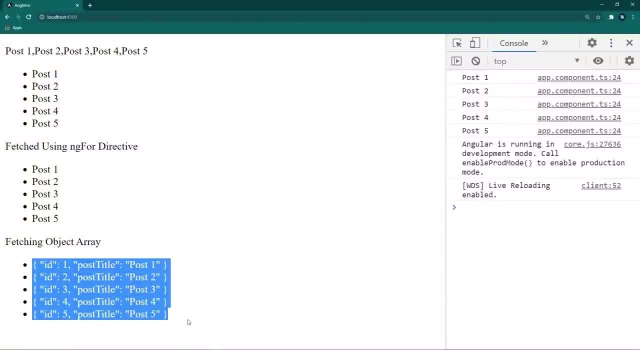 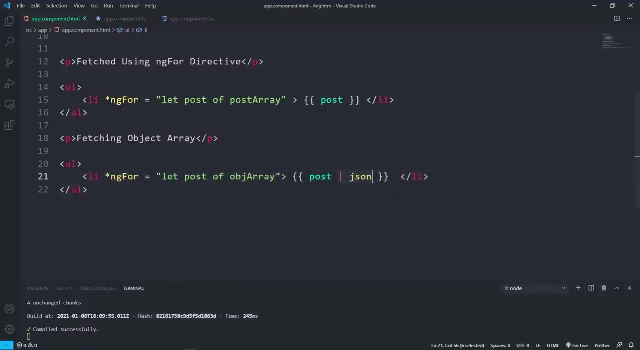 Save this and back to the browser. Perfect, We got this object values printed here with json data format, Got it? Ok, Guys, don't worry about this angular pipe thing. We have whole separate section for these angular pipes, So in that section you will learn about these pipes in detail. 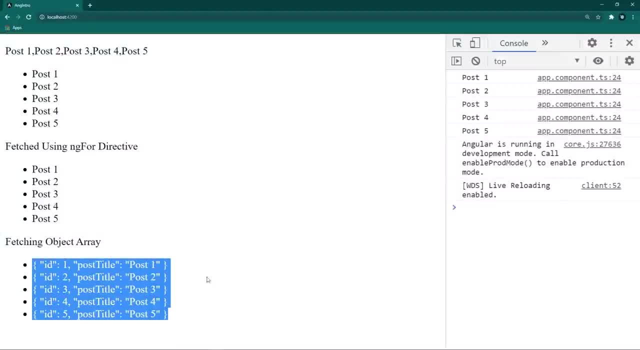 Alright, back to the work Now. we got this object array values printed here, But we don't show data inside the browser like this. right, Lets fetch only this post title value inside this li tag. For that back to the vs code. 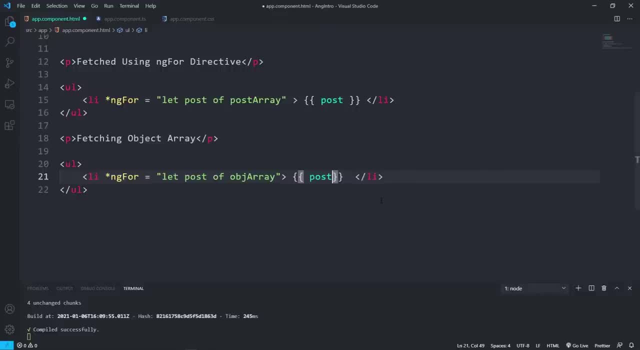 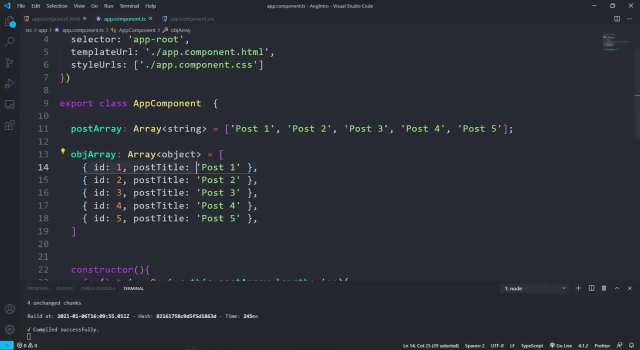 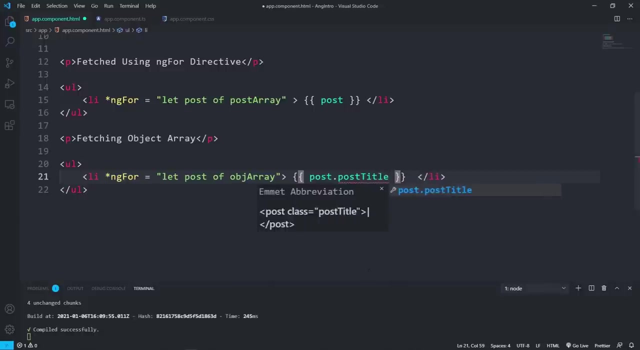 Remove this pipe. we don't need that anymore. We are going to print only the post title. With this post variable we got all the object key value pairs. So after this dot, post title, which is the object key for post title. 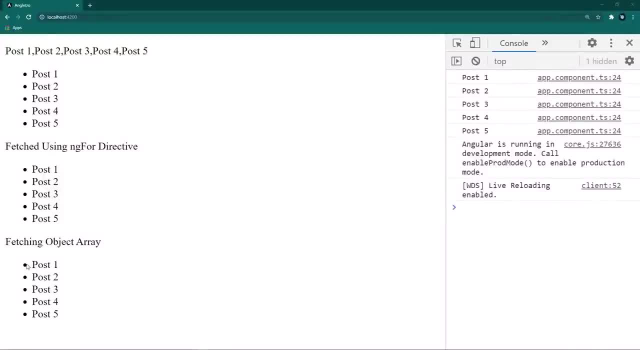 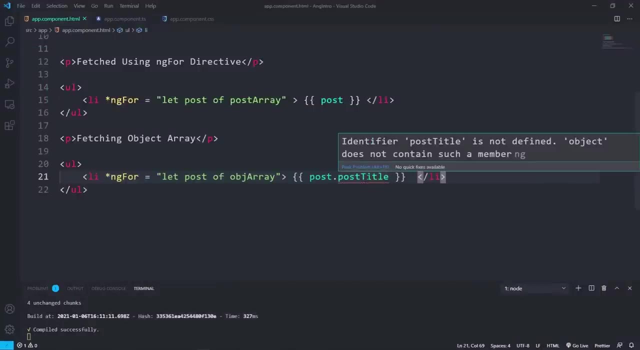 Save this and back to the browser. Perfect, right Now. we got this post title printed with this unordered list. Ok, Before the end of this video, one more thing. You guys may be noticed this already: We are getting an error here saying that this post title is not defined and there is no. 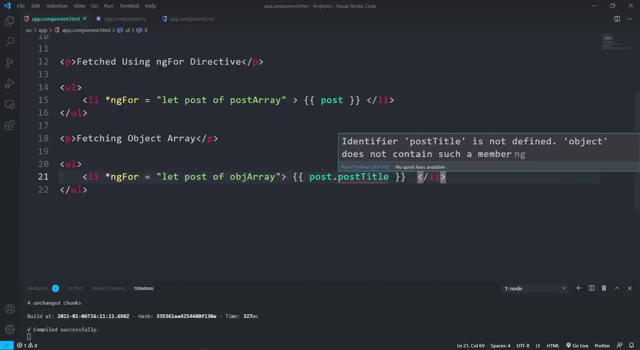 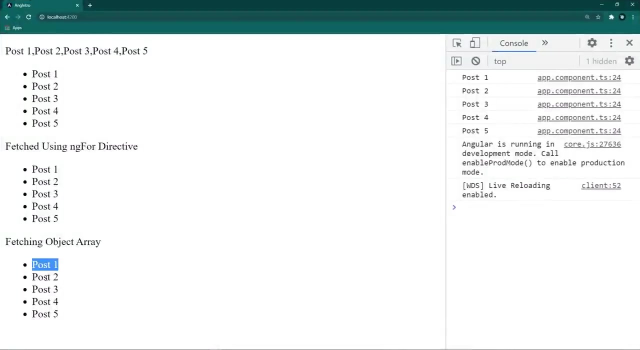 this value inside the object. Actually, this is not a compile error, Because if this is an compile error, we will get that error inside the terminal and also this code will not work. As you know, we successfully rendered this post title inside the browser without any 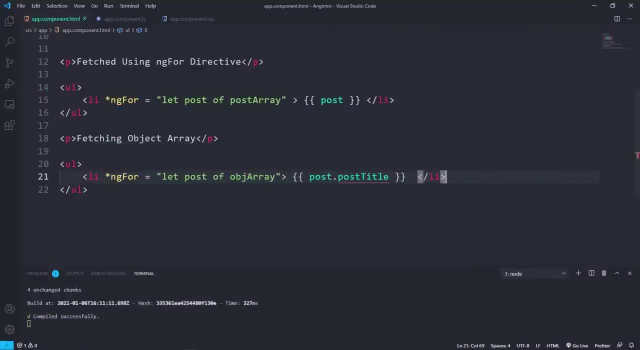 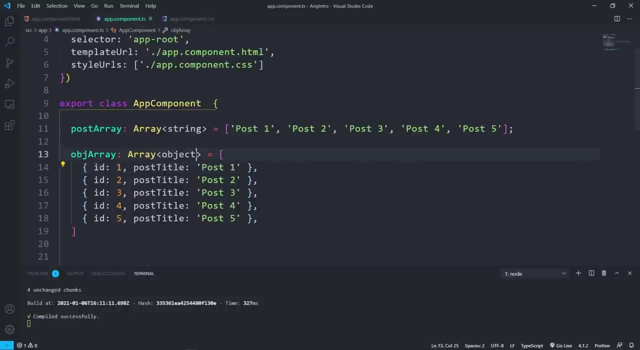 problem. So what is wrong with this? Actually, this is a kind of a bug in ESLint plugin. In order to solve this problem- we have few solutions, But I recommend you guys to do this- Just change this array type object to any. 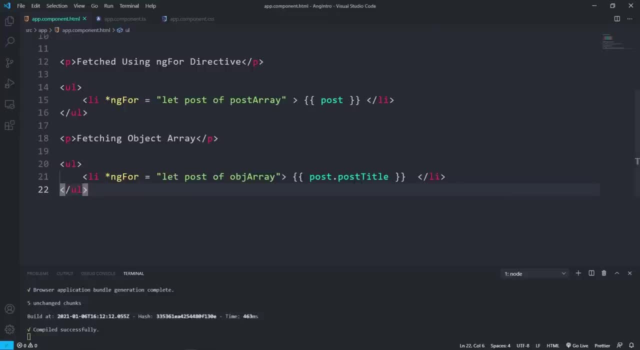 Now save this and back to the HTML file. Look at this. This time we are not getting this error, So this is just a small bug in my opinion. Hope the ESLint plugin works. Thanks for watching. ESLint team may fix this soon. 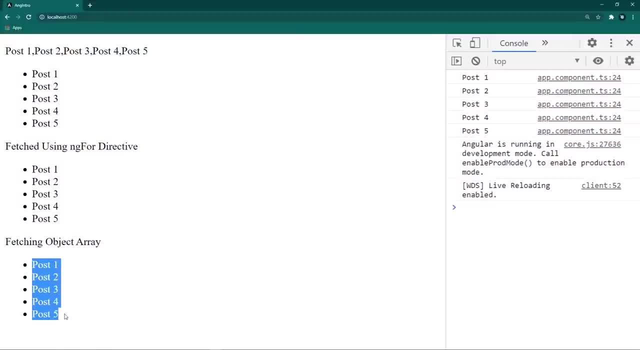 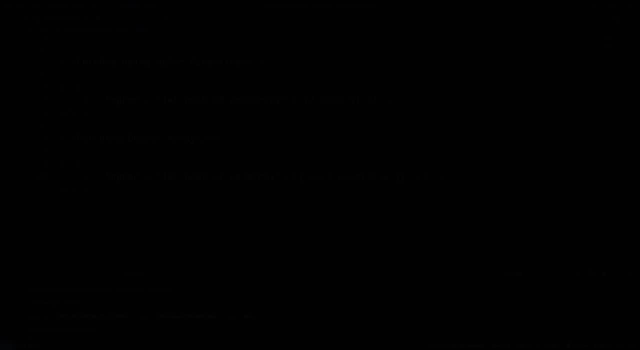 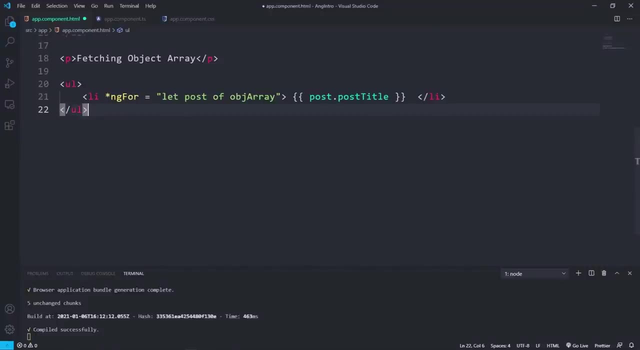 Alright, so this is how we fetch data of an array object using the ng4 directive. Hope you guys got the idea. Alright, let's add the new data object to this array when we click a button. So create a button before this ul tag button. 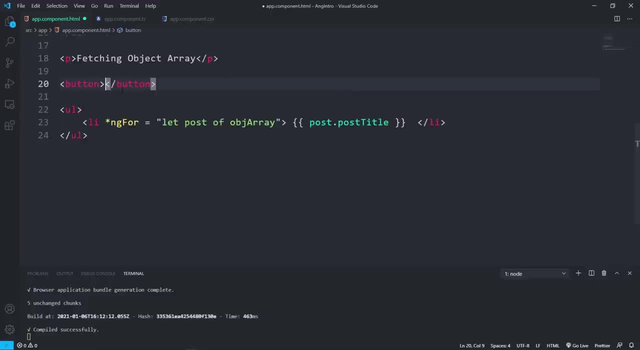 Hit enter. The button text will be: add new data. Now I am gonna bind a click event to this button. Inside this button: tag brackets. Inside brackets: click Now. assign this to a method, something, add new and parenthesis. We are getting this compile error coz this method is still not created. 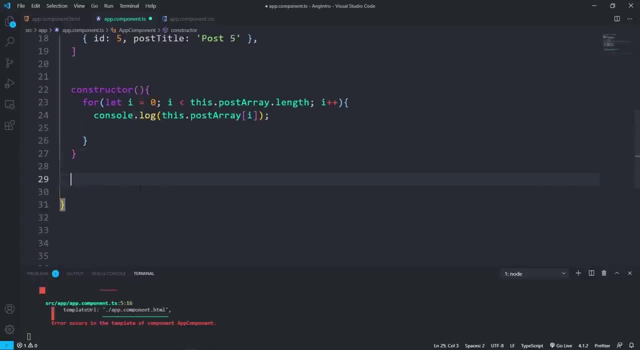 So go to the componentts file And create this method, Add new. This n is capital, Then parenthesis and the method scope. Inside this. let's add a new object to this array: ThisobjArraypush. We add new values to an array using the push method. 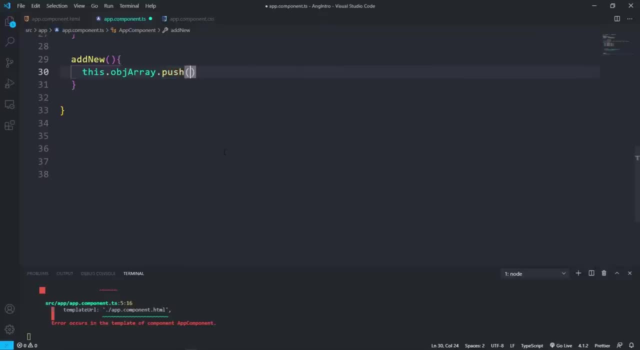 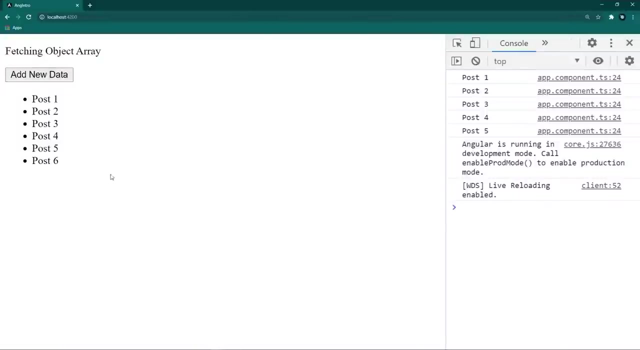 This is just javascripts, So inside parenthesis push the new object. Curl brackets Inside this id 6 and the post title is post6.. Now save this. and back to the browser. Click this button. As you can see here, we got this new post value rendered here without reloading the page, and 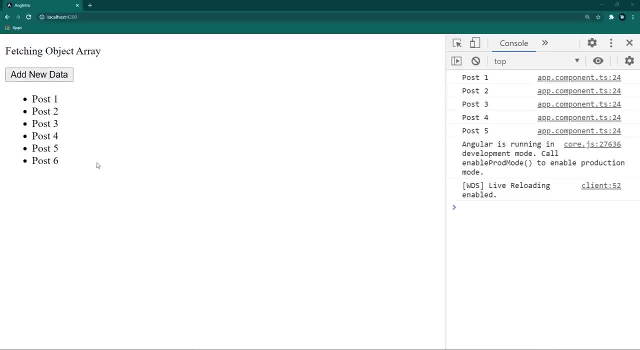 this happened in real time. How this happened In angular. we have this change detection mechanism. when we click a button or if we do any DOM events, ajax request or any timer function, angular will perform this change detection mechanism and apply all the changes to the DOM in real time. 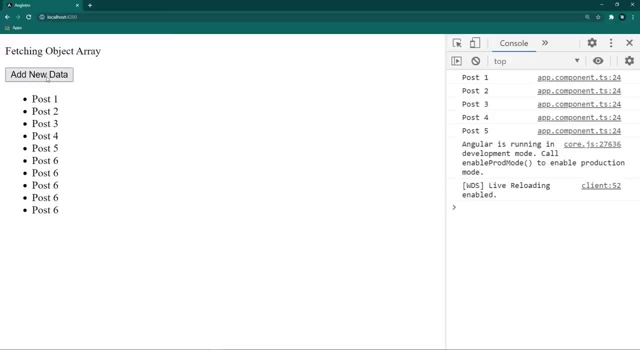 So in our case, when we click this button- add new data button, angular will perform this change detection and check whether there are any changes. So with this mouse click we added a new object to this array. So in this case, angular change detection will detect these changes and apply it to the DOM. 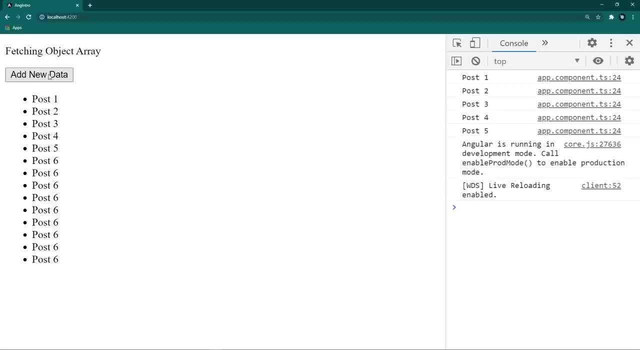 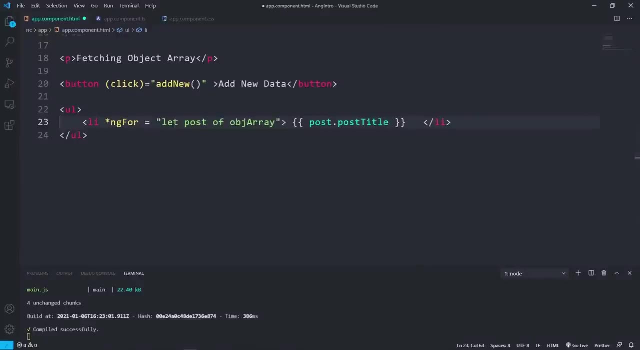 That's why we got this newly created post object rendered inside this list. Let's remove an object from the array and see what's happening here. To delete a value we need a delete button. Add a delete button inside this list button. hit enter button. value is delete. 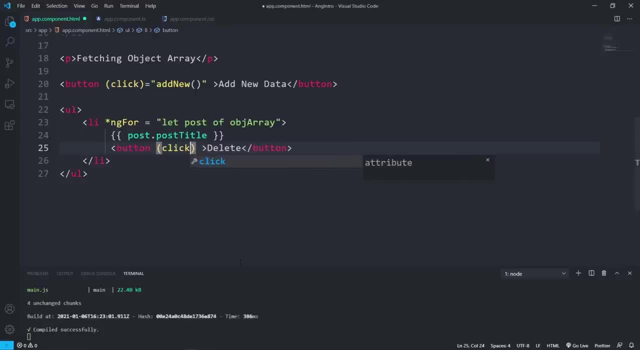 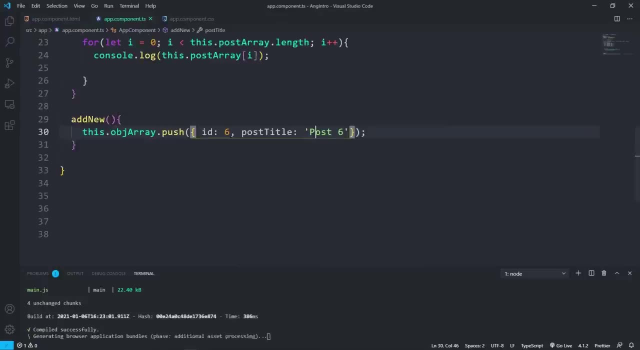 Now bind a click event for this button inside brackets. click and assign it to a method: something onDelete. Create this method inside the ts file. method name is onDelete, parenthesis, and the method scope. So, in order to remove an array object from an array. 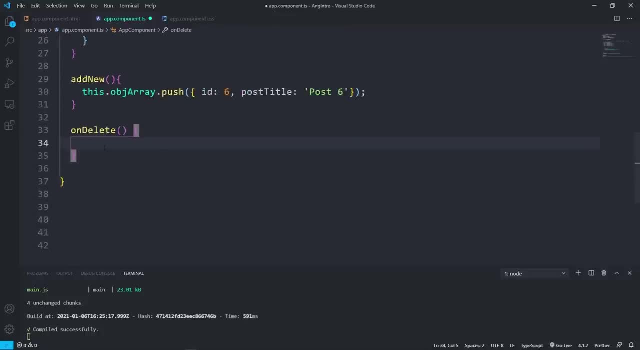 First we need the index of the array. Then only we can remove an object from an array using that index number. So in order to get the array index number, we have to pass that array value to this method. So back to the html file and so pass this post object to this onDelete method as a parameter. 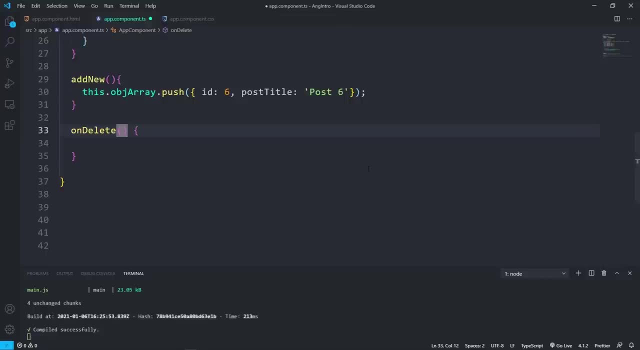 Say, we send back to the ts file From here. capture that parameter from this method, This method onDelete. Create a parameter variable post. Now let's get the index number. Let index assign this dot. the array name is objArray dot. index. of this O is capital and 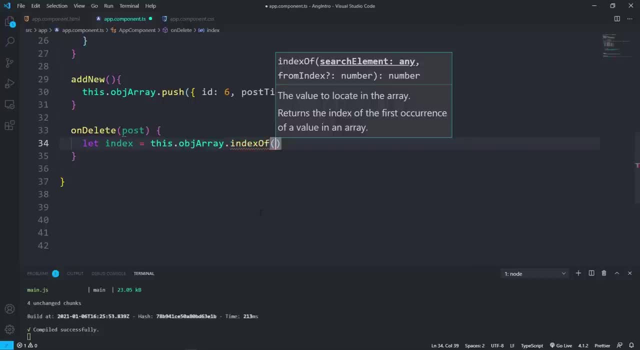 pass the parameter array value to this inside of the bracket. So with this we are getting the index number of this passed array value. Now let's go back to the html file and see what's happening here. So we need to remove an object from this list. 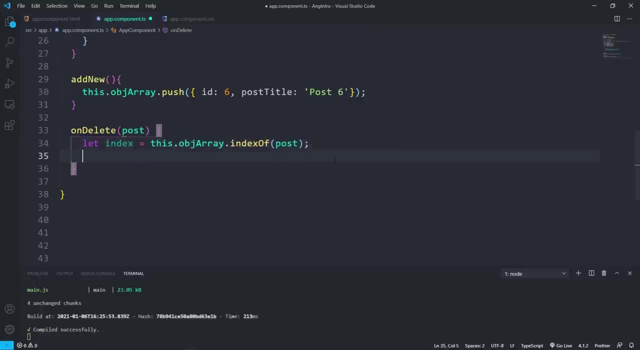 Now let's remove that array object from this array. This dot array name is objArray dot splice. We can use this splice method to remove an array value from an object. Alright. next, inside brackets, pass the index number that we want to remove and then pass. 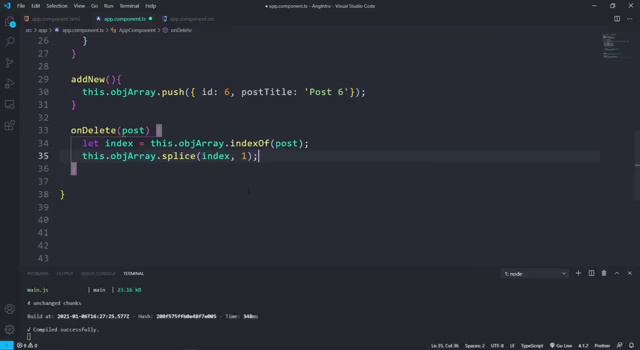 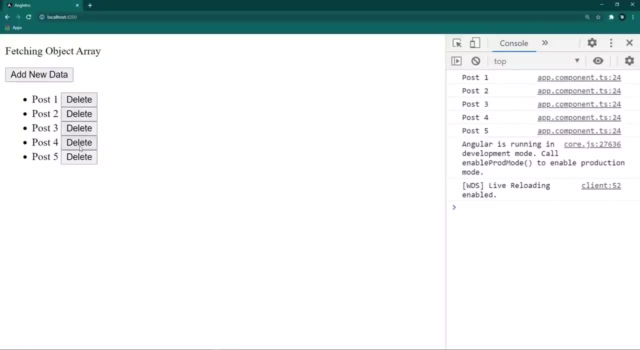 the number of object that we want to delete. In our case, this is 1.. Now let's go back to the html file. This is 1.. Save this and back to the browser. Click on this delete button, So this will remove this post 4.. 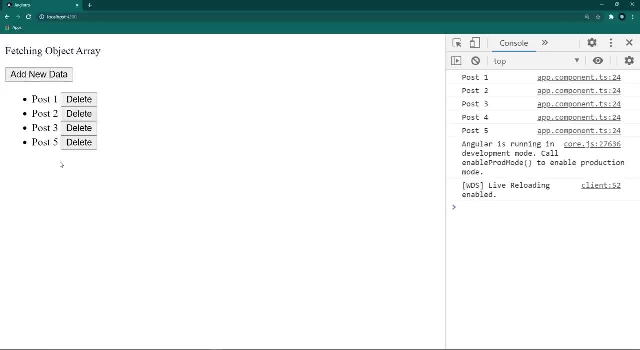 Click it. Perfect right. This post 4 is removed. If you noticed, this also happened in real time. So this is the beauty of angular: Every time we performed some changes on our app, the angular change detector will detect the changes and render it to the wave in real time. 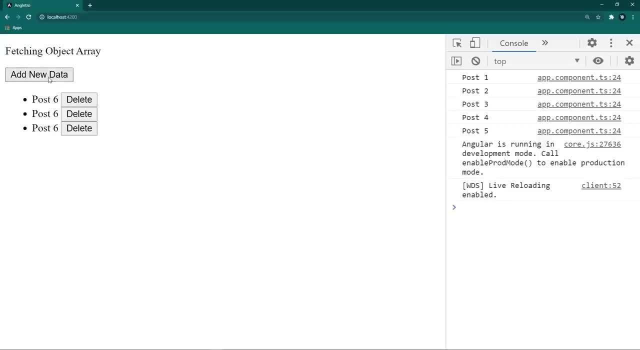 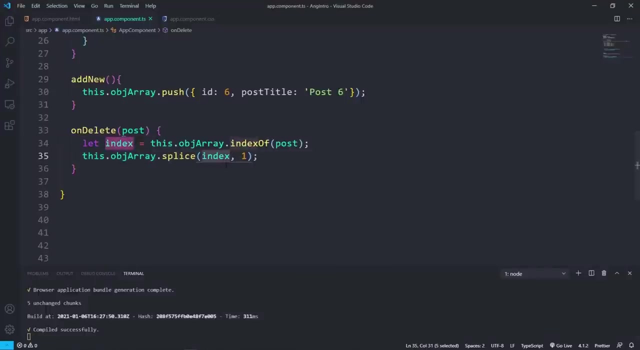 In previous we learned how to remove an array object value from an object array when we click this button, And also I said that in order to remove an object from an array we need the index number of that removing object value. Then only we can remove that object value from the array. 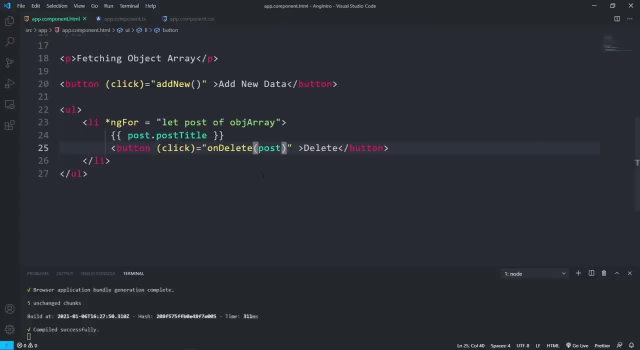 So let's go back to the html file. So for that we use the traditional javascript approach to get the array index. We pass the target array object to this onDelete method as a parameter And inside that method we captured that target object and we got that array object values. 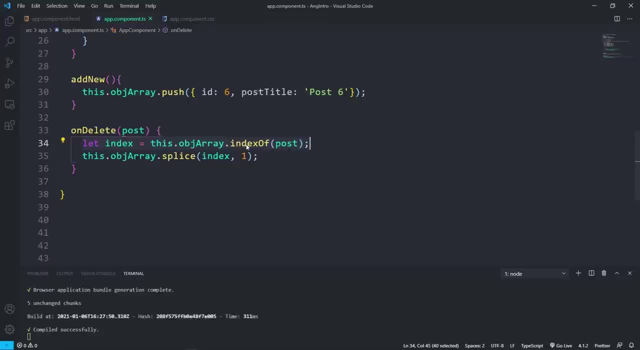 index using this index of method. After that we removed that object from the main array using the splice method To get the target array index. we have a very simple and cleaner way in angular: With this ng4 attribute we can fetch the index number as well. 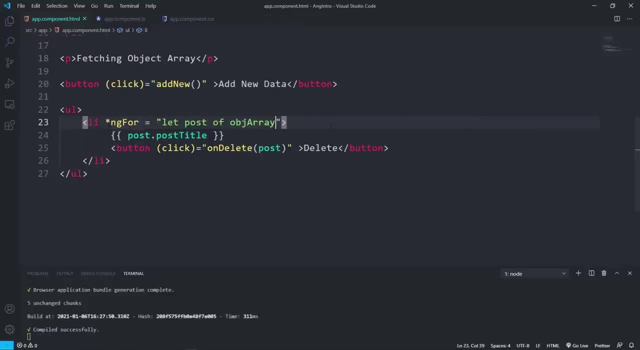 Let's see this in action. After this: ng4, add a semicolon and add this index as i. So what is happening here? I just assign this array index to this. i variable: This variable name can be any name. This variable name can be any name. 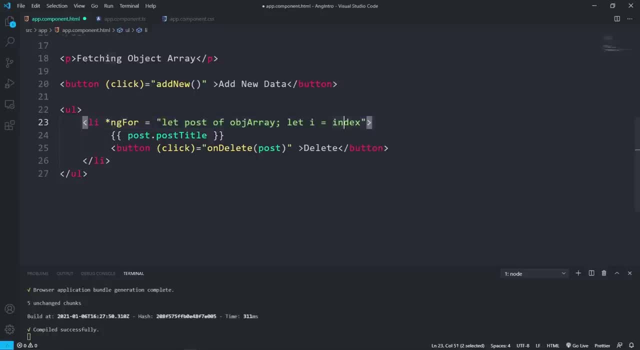 So what is happening here? I just assigned this array index to this i variable. This variable name can be any name. This variable name can be any name. Now we can use that index number on this view. Let's render this index number inside the view. 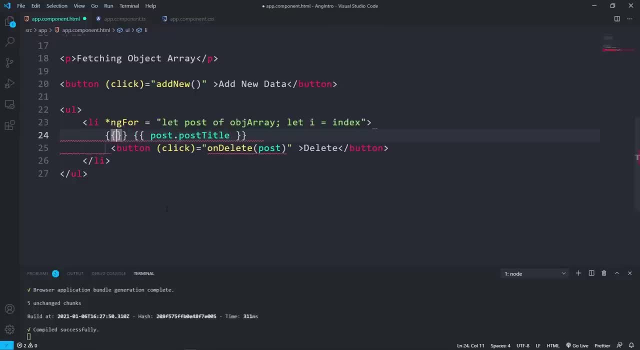 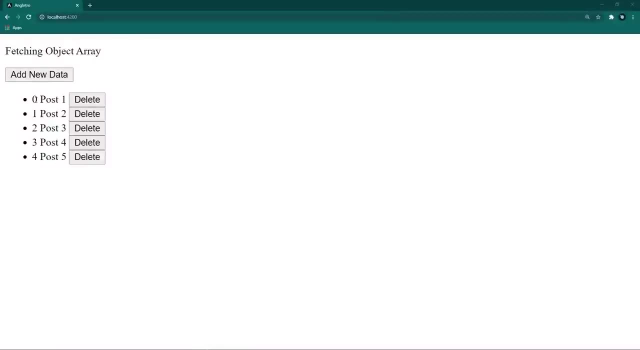 Before this, just add the i variable which is assigned to the index, Save this and back to the browser. Look at this. We got this array index in front of this post title, Starting from zero, Because you guys already know, array starts from zero. 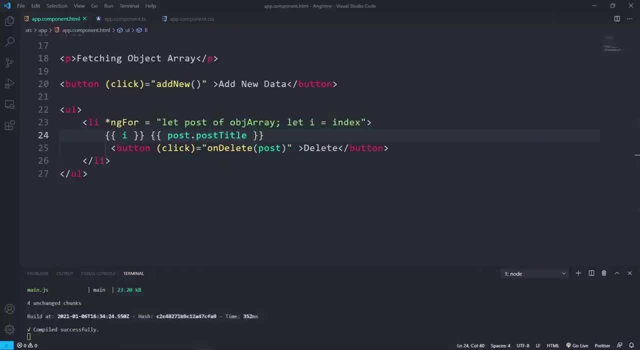 Alright, now all we have to do is just pass this index. Pass this i variable instead of this full post. object to this onDelete method. So remove this post parameter and pass the index variable. i Save this and go to the componentts file Inside onDelete parenthesis. 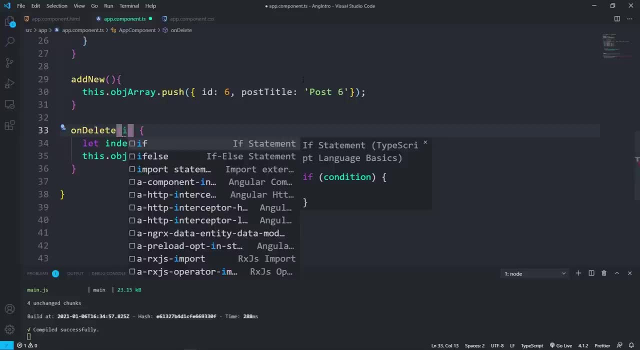 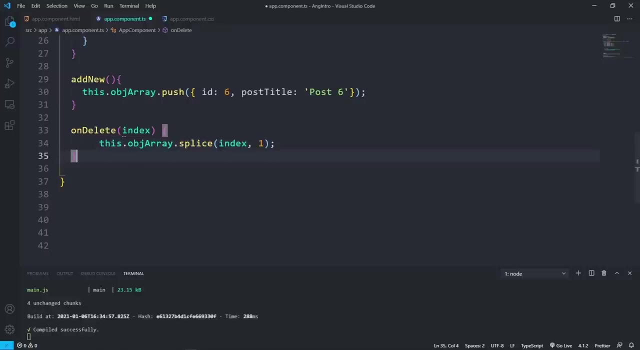 This time we are not getting the post object, So remove this and create a new parameter variable to capture the index number. So I will define this as index. Now we don't need this indexOf method. Remove it. That's it. This time, this index is this parameter, which is coming from the HTMLB. 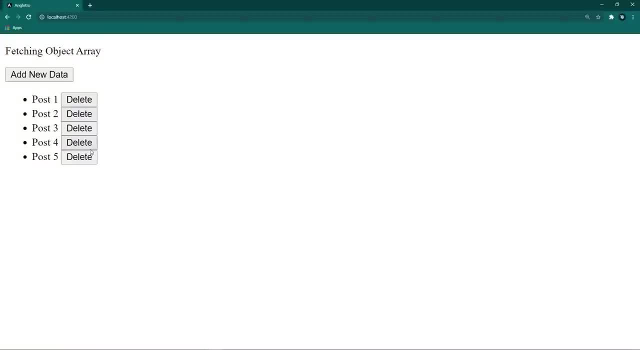 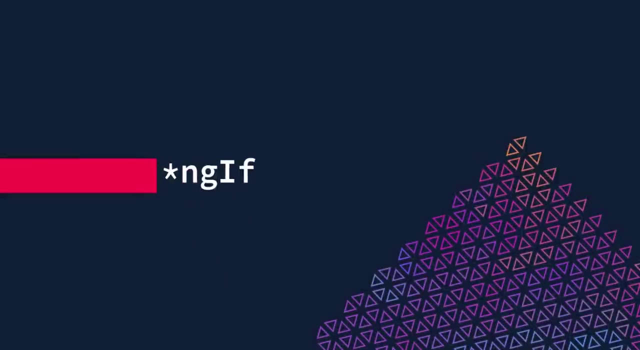 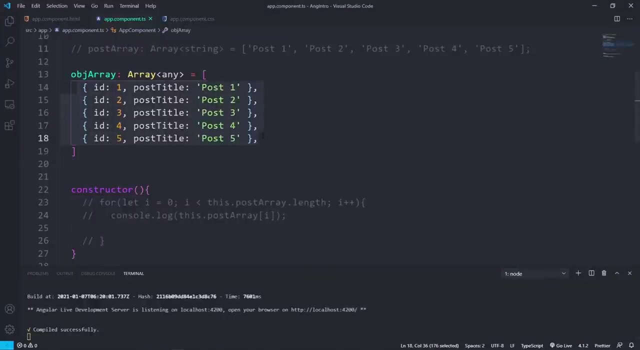 Save this all and look back to the browser. Click one of this delete button. As you can see here, this removed this array object. So this is how we use the index of an array using the ngFor directive. Think: if there is no data inside of this array, this is empty. 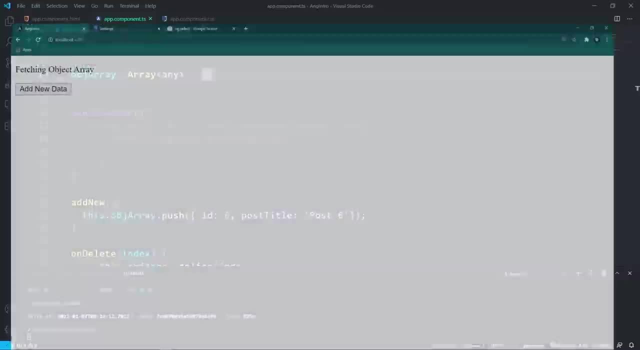 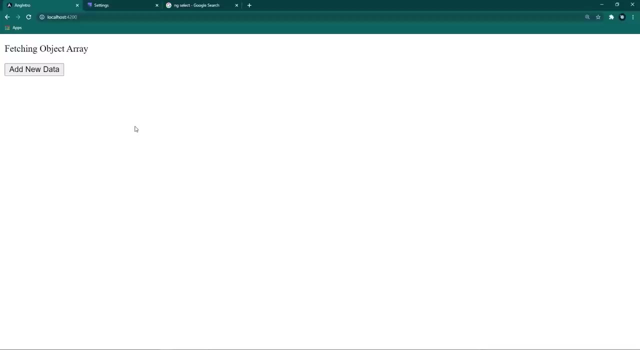 So in that case, if we render this inside the browser, we are not getting anything Because we don't have anything inside the array. Now what I want to do is, instead of this empty view, I want to show a message here, something there is no data to fetch. 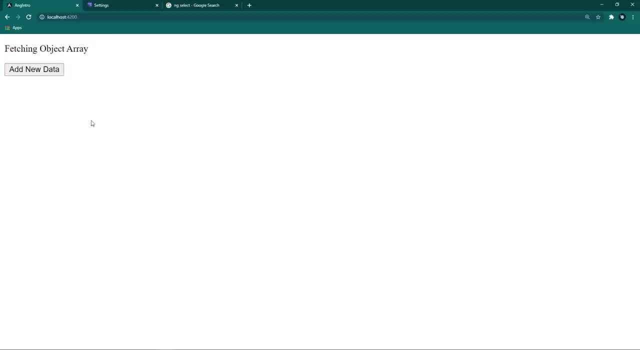 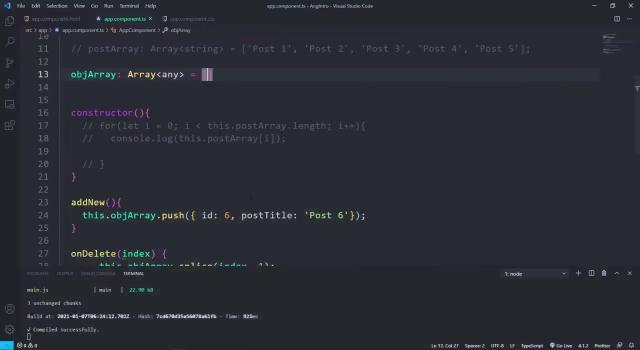 If there is any data inside the array, I want to fetch them here. If there is no data, I want to show the message: there is no data to fetch. Clear right To do this. we gonna use another directive in angular, which is ngIf. 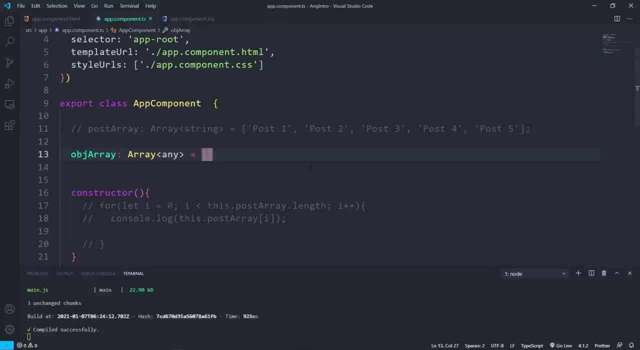 This is something like if else in javascript We use this ngIf directive to show something conditional. So if there is no data inside the array, I want to fetch them here. If there is no data, I want to show the message: there is no data to fetch. 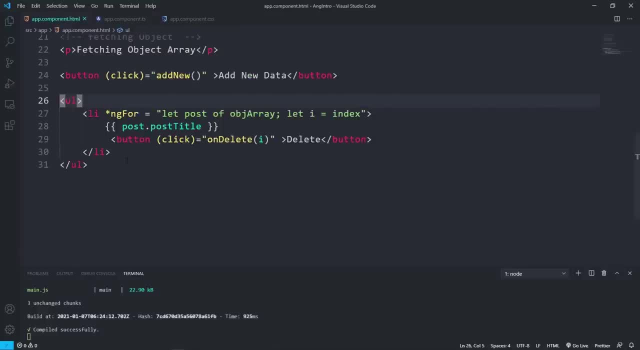 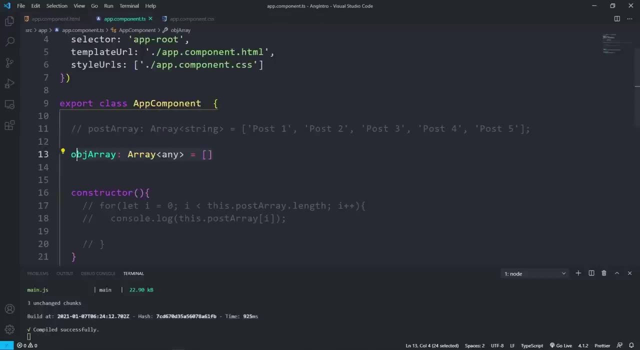 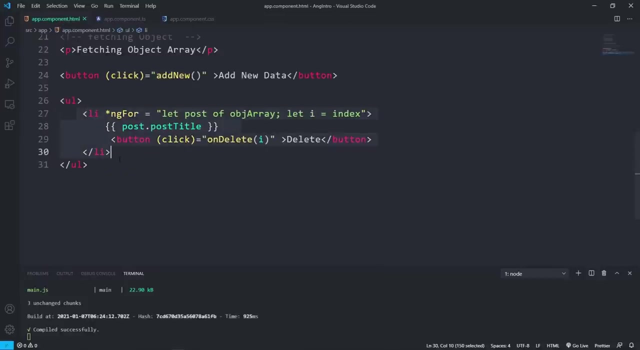 So let's see this in action. Once again. what I want to do is I want to fetch this list if there is data inside the array. If there is no data, I want to fetch a message instead of this empty list. So before this, let's create a div and put this unordered list inside this div. 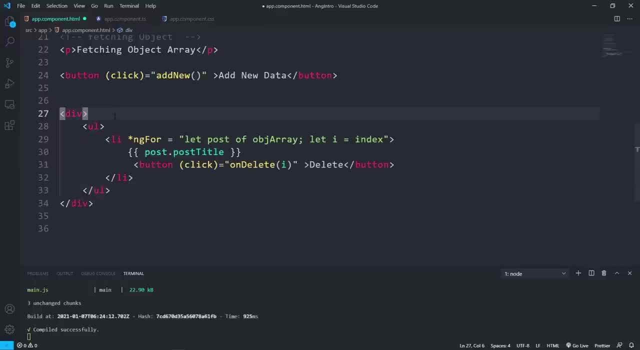 Now I want to fetch this unordered list. when there is no data inside this div. when there is data, So inside this div tag, let's add the ngIf directive. This is also structural directive, So asterisk ngIf, This i is capital. After this, equal sign Now. 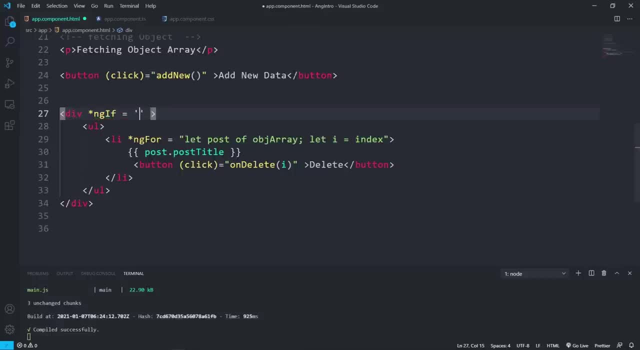 pass the condition inside quotes. Pass the array name, which is objArray, then dot length after this: greater than sign and zero. So some of you may wonder what is happening with this condition. With this condition I am checking, that is, this array's length is greater. 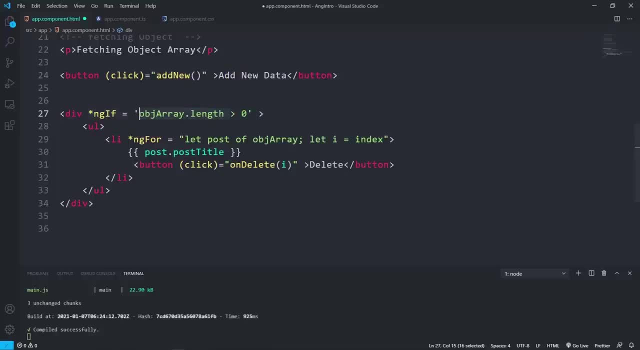 than zero. If there is data inside of this array, the length of this array will be greater than zero, So in that case, this statement becomes true. If this is true, this div will show inside the browser. Very simple, right. Next, I want to show message when there is no data. So down here. 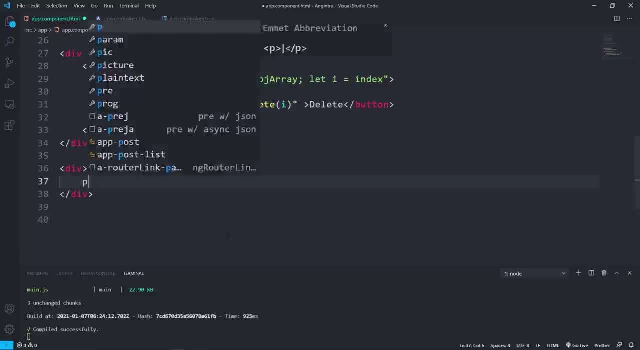 create another div Inside this div, create a p tag and add this message: There is no data to fetch. Now let's add the ngIf directive to this second div. Inside this div tag: asterisk icon: ngIf equal sign. Inside this, the condition. 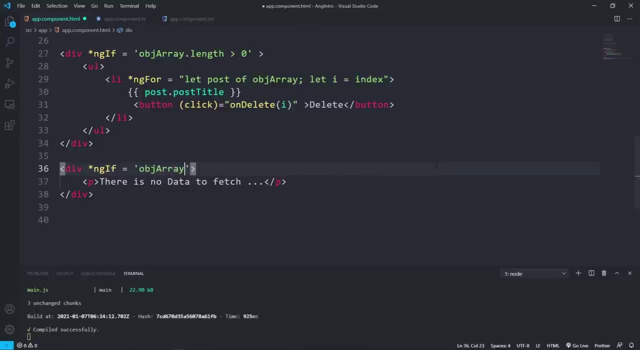 This time the condition is: objArray dot length equals zero. With this condition, we are checking the length of this array is equals to zero or not. If there is no data in the array, the length of this array becomes zero and this statement will be true. So in this case, 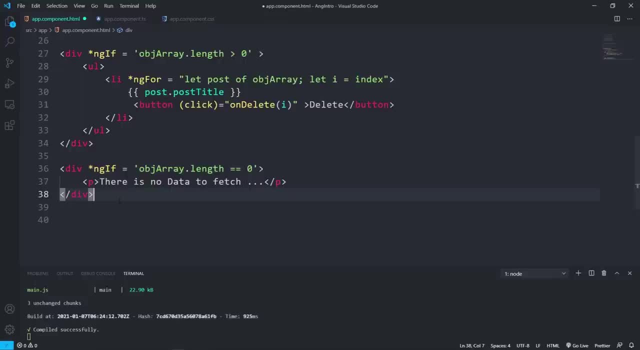 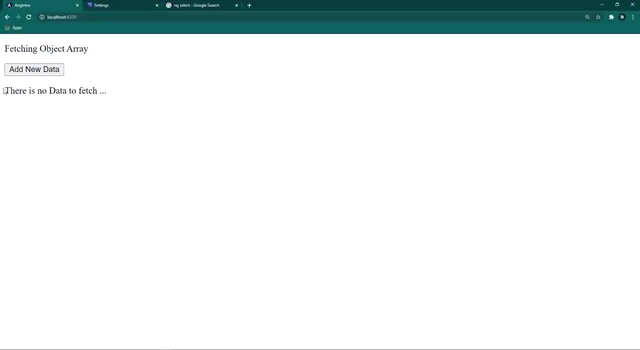 this div will show inside the browser: Very simple logic. Hope you guys got the idea. Save this and back to the browser. As you can see here, we got this message: There is no data to fetch Because there is no data inside the array. Now click this button, add new data. This added the new data to the 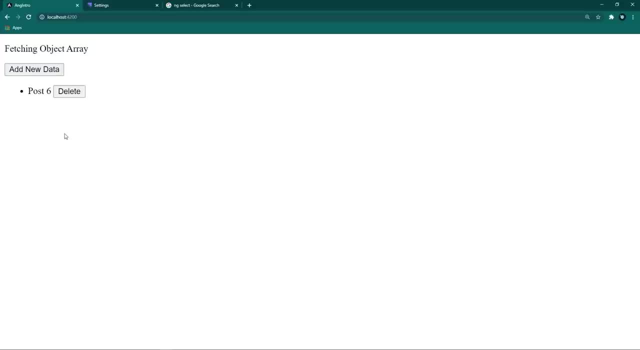 array. Now look at this. This time we got this unordered list, Because now inside our array we have this new data. If we click this again, we got this second value printed here. Now remove one of this value using the delete button. Now we have only one data. Also, if I removed this last, 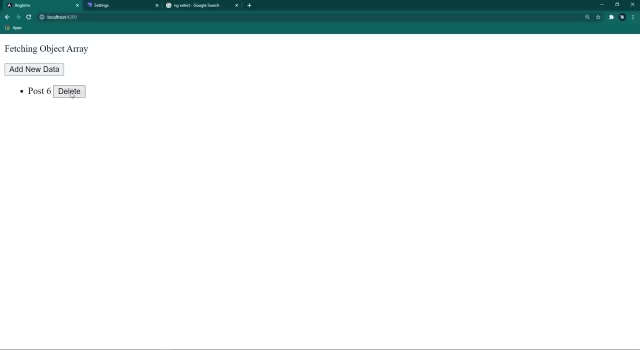 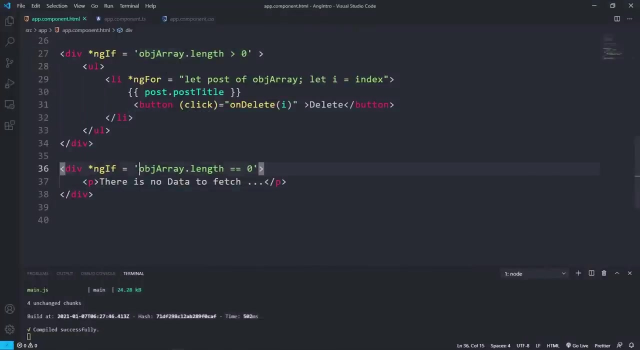 array value. can you guys guess what will happen here? Yes, you are correct. If I remove this last data from the array, the array becomes empty. This ngIf statement will return false Because there is no data, And this second statement becomes empty. 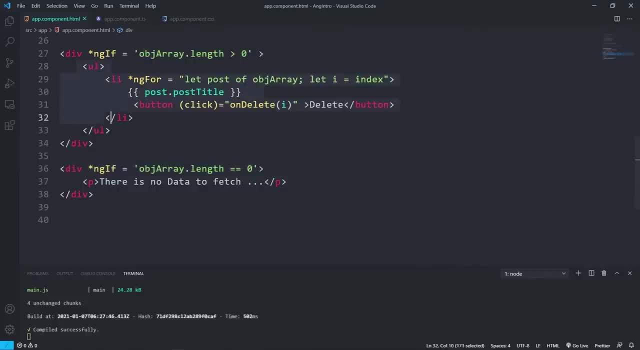 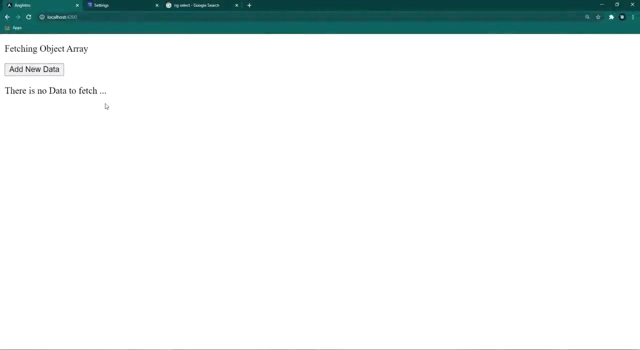 So this ngIf will remove this unordered list from the DOM and this will show this message: p tag inside the DOM. So let's see this in action. Click this delete. We got this message Beautiful right. So this is how we use ngIf directive in Angular. 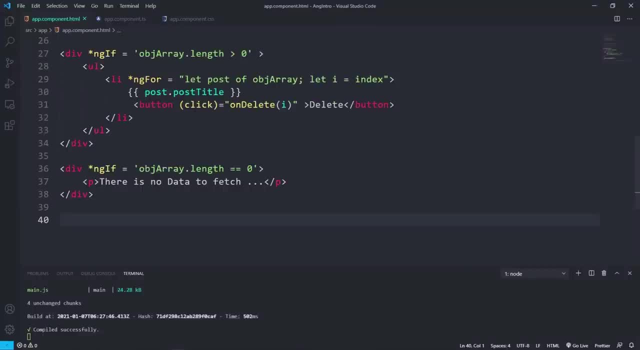 Alright. in the previous video we learned how to use ngIf directive. We used ngIf directive to show this array data conditionally. If you look at this, you can notice that we used two ngIf directives to do this. In JavaScript we have this, if else We add the condition. 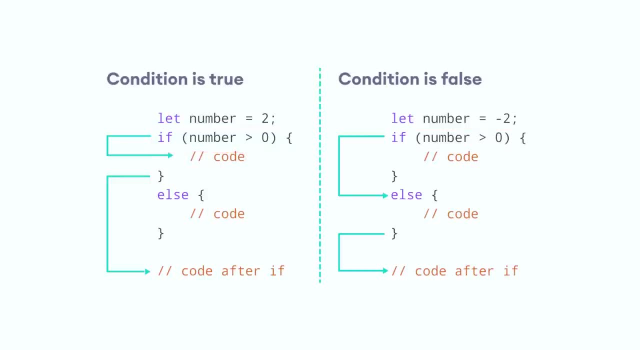 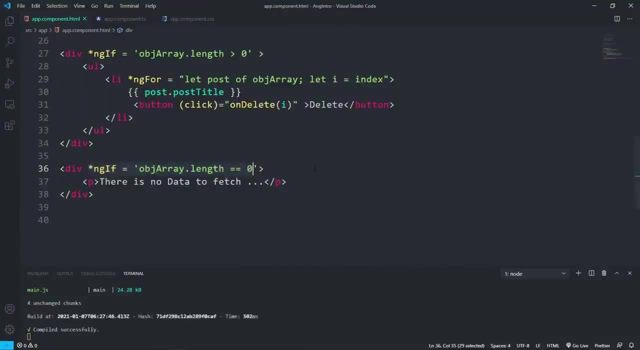 in if. If this condition is false, then else part will execute. We can implement the same thing. We can add else approach using this Angular ngIf directive rather than adding these two ngIf directives. Let's see this in action. We can add else after this condition. So 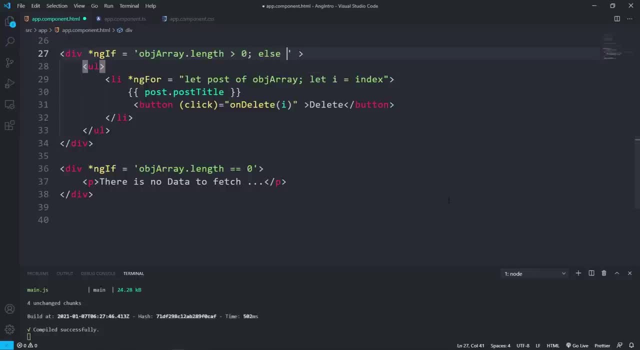 add a semicolon else. Now we have to tell this to show this: no data message. How do we going to do that? In Angular view, we can identify an HTML element using template variables. You can remember We learned about this in the previous section. So give an identifier to this div. Now we 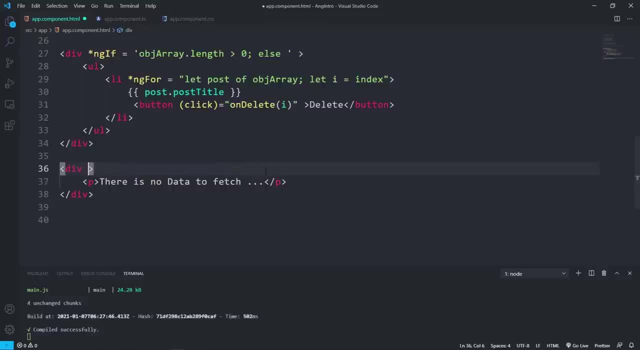 don't need this ngIf, So remove it and give an identifier to this Hashtag. template variable name: something: no data. This name can be any name. Now pass this template variable to this else After this else: template variable name is no data. Pass this here without the. 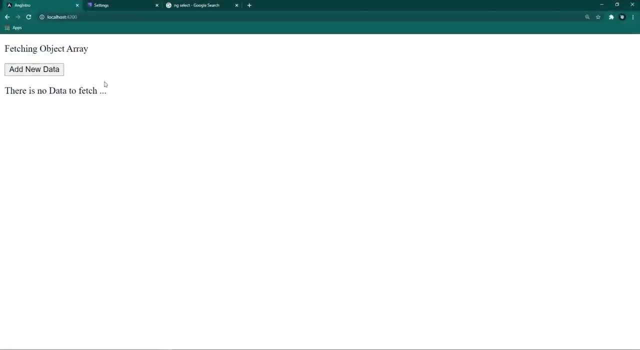 hash sign. Save this and back to the browser. We got this- no data message. Of course, we don't have any data inside the array, So let's add a new data using the button. As you can see here, we got this new data here, But we have a problem here Still. we can see this. 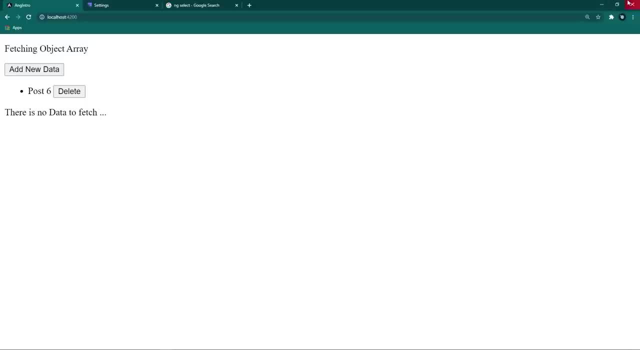 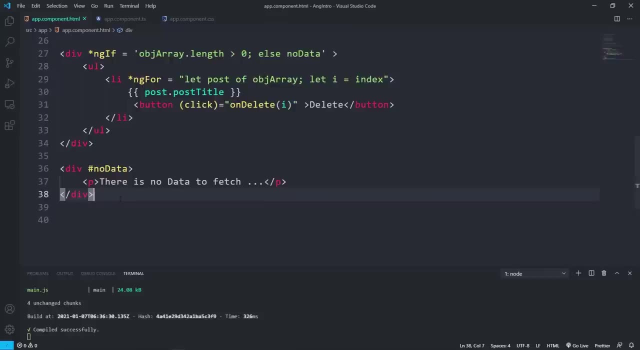 no data message. What's going on here When we are using a structural directive? if we use a div tag to show data conditionally using template variable, something like this, We can see that this is no data message. So let's add a div tag to show data conditionally using. 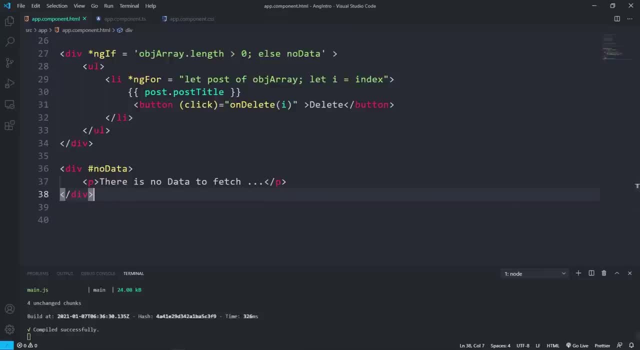 template variable something like this. Now we can see that this is no data message. What's going on here? When we are using a div tag to show data conditionally using template variable something like this, This condition won't work. That's why we are seeing this. 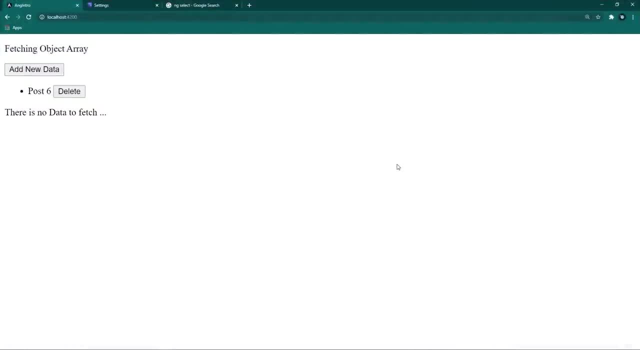 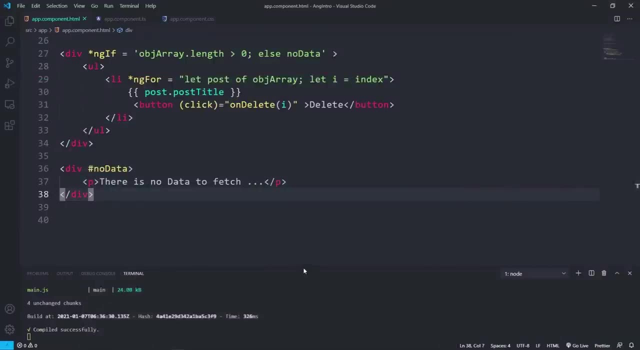 message even when there is data inside the array. To solve this problem, we have a special type of tag called ngTemplate. With this ngTemplate, we can load data to the browser conditionally, using the structural directives. So change this div tag to ng-template. 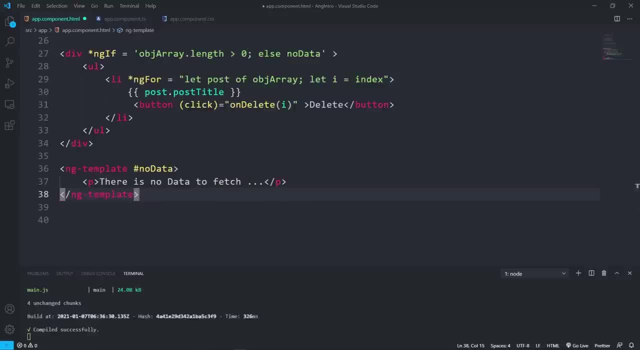 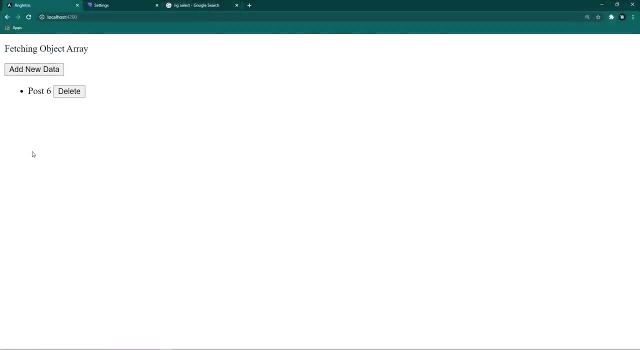 Now save this and back to the browser. Now we are seeing this no data message. Add a new data. As you can see here, this time we are not getting the no data message, So delete this data. Perfect, We got the no data message, which means now this else statement is working. 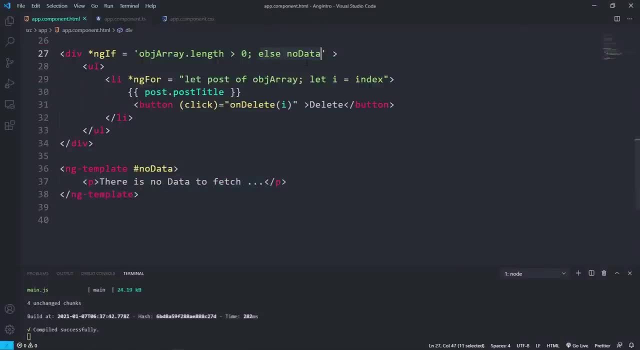 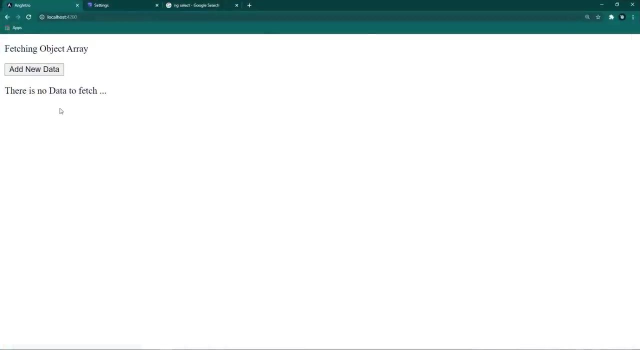 perfectly. And one more thing: we cannot use this ngTemplate tag as a normal HTML tag. If I create another ngTemplate tag, we can see that this ngTemplate tag is not working. Save this and back to the browser. We cannot see this ngTemplate tag here, Because we cannot. 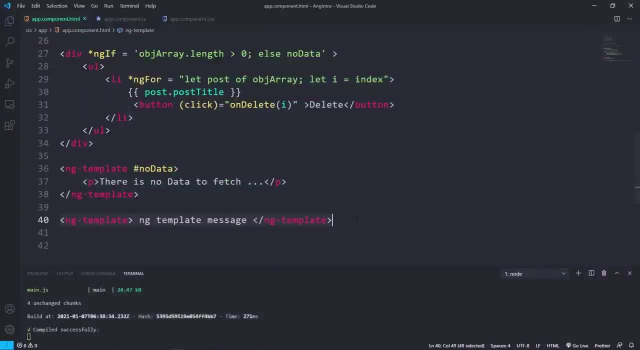 use this as a simple HTML tag. We can only use this ngTemplate with the structural directive, something like this: If not, this will not display inside the HTML view. Alright, we have another approach for this. We can use ngTemplate for both this and this. 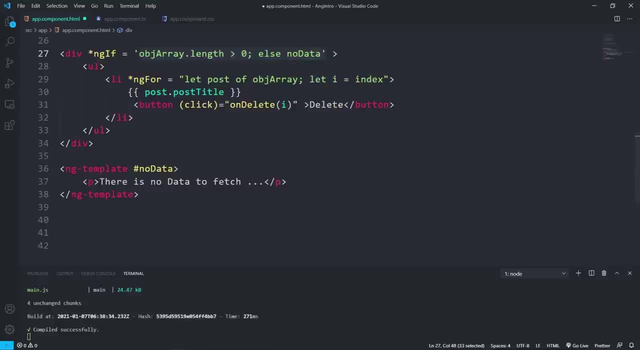 truthy and false conditions. Let's do that. Create another ngTemplate tag Inside this. cut this unordered list and paste it here inside this ngTemplate. Give a name for this ngTemplate to identify this Hashtag post list. Now I want to show this ngTemplate when: 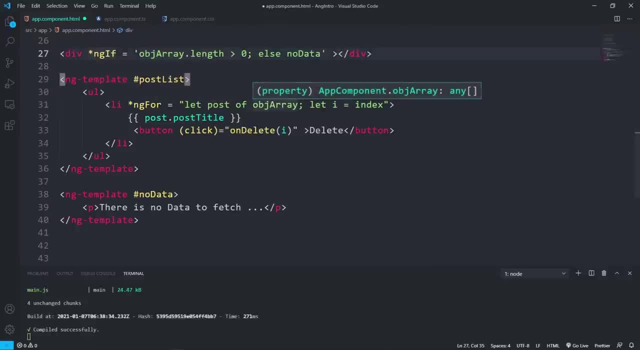 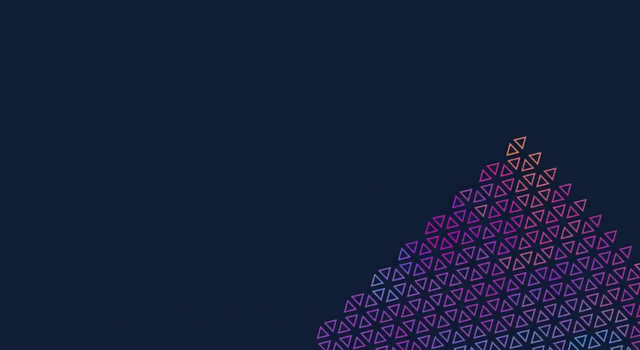 this condition is true and pass the template variable name: postList. That's it. Save this and back to the browser. This is working as we planned. So this is just an approach. If you don't like it, you can use the previous approach, no problem. So this is how we use ngTemplate in angular. 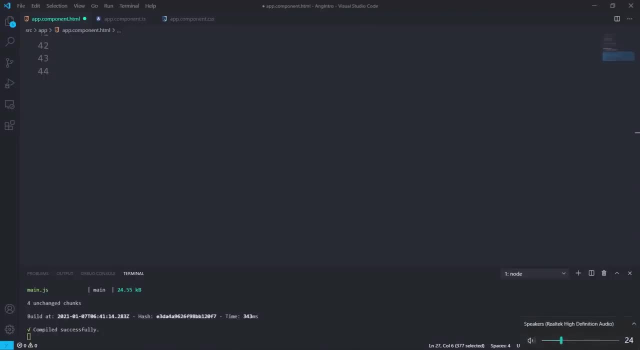 In this video. let's look at another angular directive: ngSwitchCases. This is also the same as javascript or any other programming languages- switch cases. Let's see an example for this. Let's create a simple step form. First, let's create 3 buttons for 3 steps. 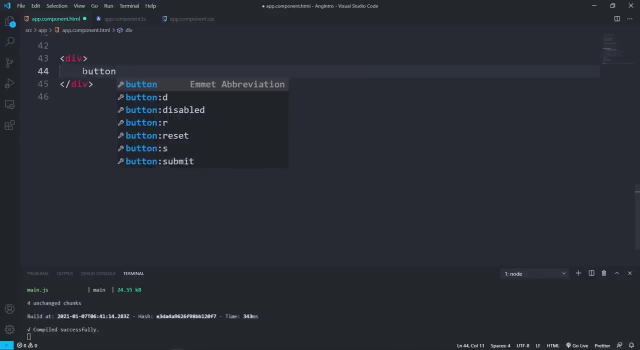 Create a div. Inside this div, create 3 button tags. Button values will be step1, step2 and step3.. After this, create another 3 div tags Inside the first div- step1 form. Second div: step2 form. Third div: step3 form. Now I want to show one of this div when I click the relevant. 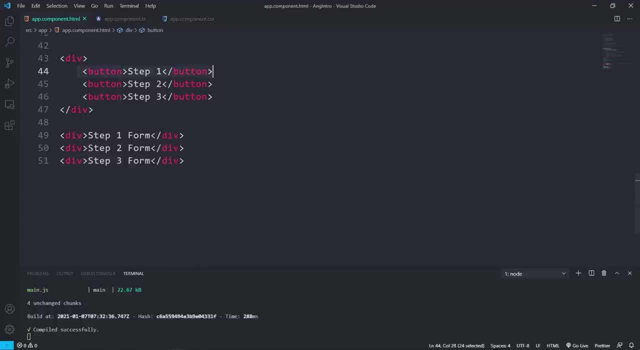 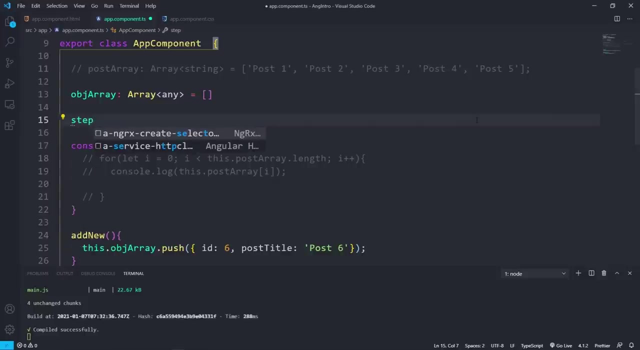 button. For example, if I click this first button, I want to show this step1 div. If I press this step2 button, I want to show this step2 button. Let's do that. Inside the typescript file, create a variable, something step form. The variable type will. 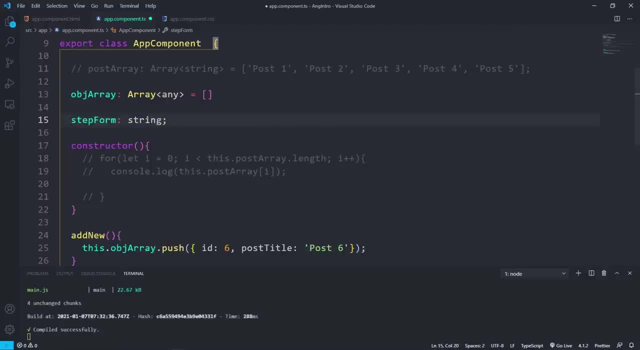 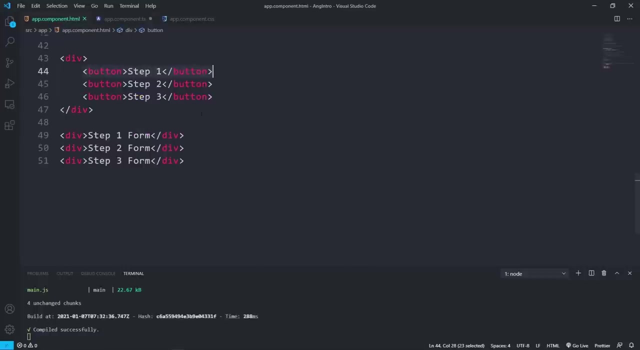 be string. Now what I want to do is I want to change this variable's value when clicking the button. For example, if I click this step1 button, I want to change this variable value to step1.. So let's do that. We can do that simply using the click event. So create a. 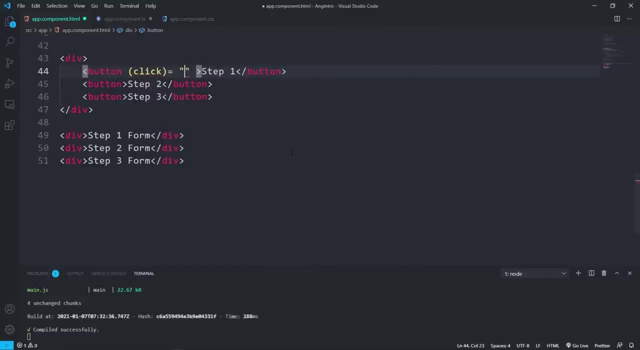 click event Inside this click event. So let's create a click event Inside this click event Inside this step button. brackets: click equals sign. the method name is OnClick Pass step1 as parameter, Coz I'm dealing with the step1 button. 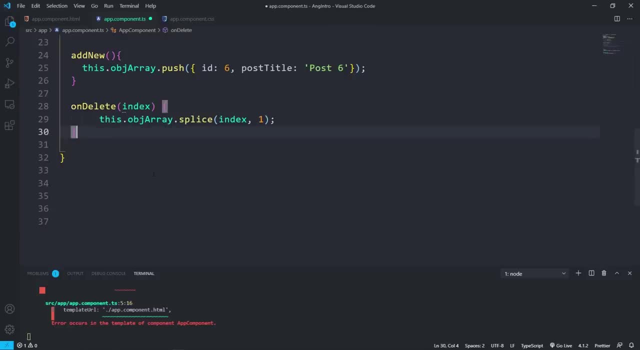 Now inside the typescript file, create the OnClick method Inside this class scope. onclick. This c is capital Parentheses And the method scope. We are getting a parameter with this, So capture that parameter. create a parameter variable inside this parenthesis status. 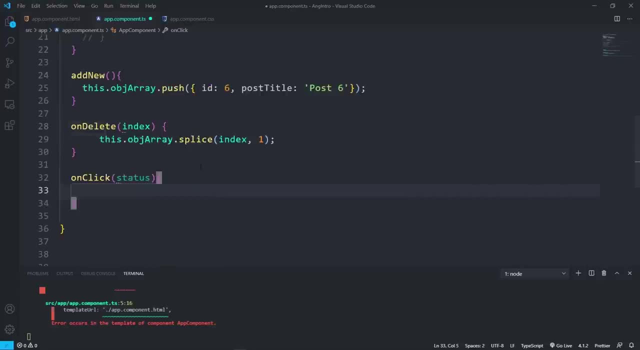 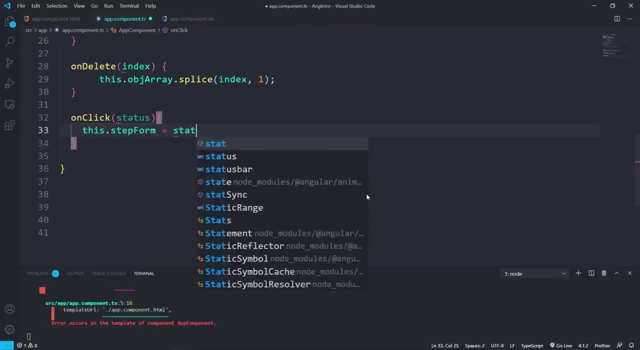 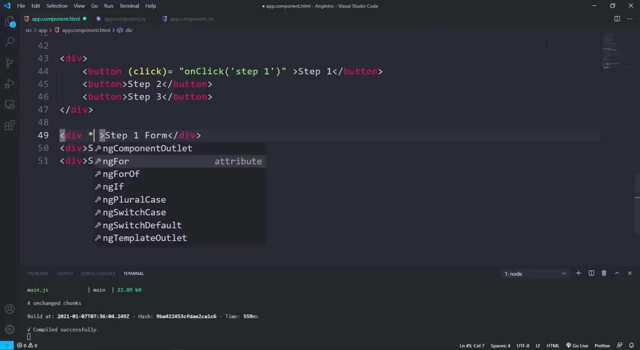 Inside this method: assign this status to this step form variable. This dot step form. assign this parameter variable is status. Alright, now we can show this step1 div using the ngIf directive. Inside this first div, let's add the ngIf directive asterisk- ngIf equal sign. inside: 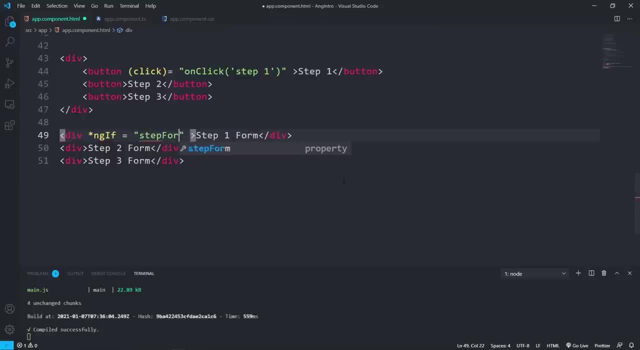 quotes This statement is: if this step form equals step1.. If you noticed, I passed this as a string inside single quotes. I used double quotes for this whole statement and for this I used the single quotes With this condition. I am checking that: is this step form variable value equal to step1. 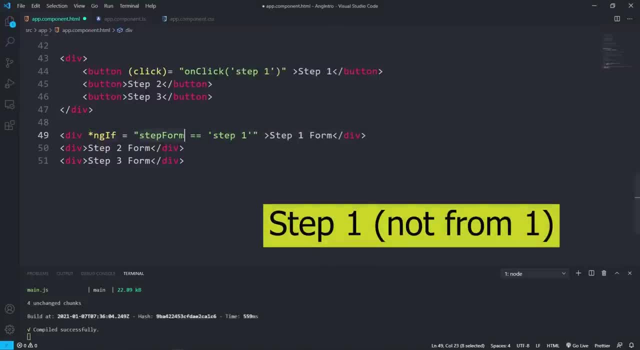 If this is form 1, the statement will become true and this div will appear on the browser. So let's do this to all of these divs. So first, add the click event for the button. change the parameter values to step2 and step3.. 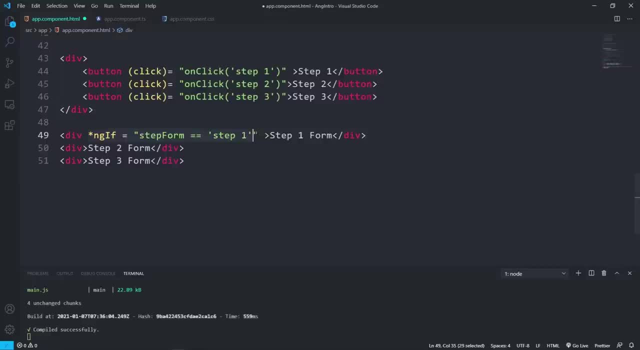 After this, copy and paste this ngIf to other divs and change the condition. this one is to step2.. Because I want to show this div when click this step2 button. Likewise, this last div statement is step3.. Alright, save this all and go to the browser. 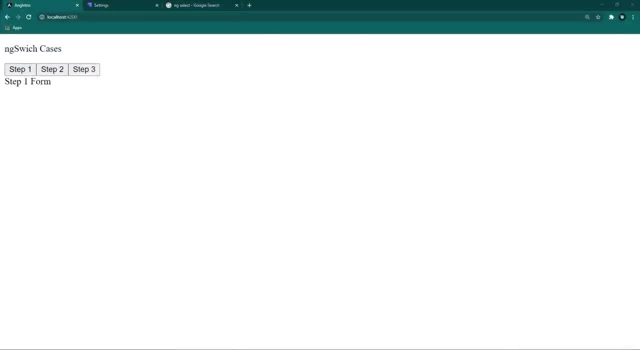 We can see these buttons. Click this step1 button. we got this message. step1 form. Click this button. step2,. we got this step2 form message. Again, click this last step3 button. we got this step3 message. So this is working as we planned. 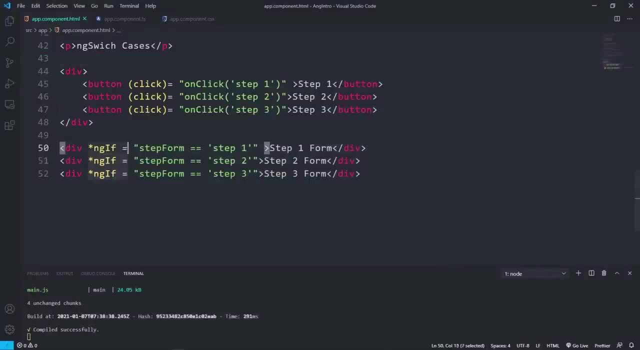 But if you look at this code, we are using the ngIf directive several times. So rather, using this ngIf directive, we can use a switch case. So let's see how to do that. Put these divs inside of another div. 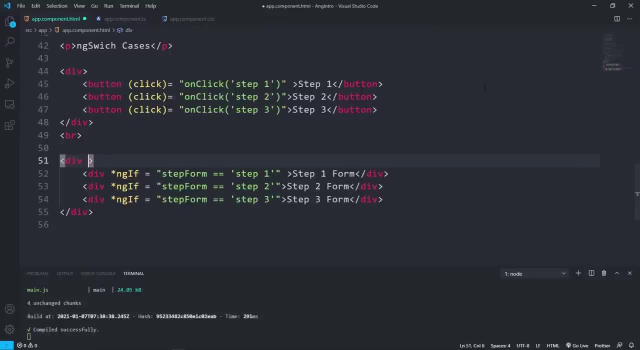 Now add the ngSwitch to this div. For this: we gonna use the property bind. Now add the ngSwitch to this div. For this: we gonna use the property bind. Now add the ngSwitch to this div. For this: we gonna use the property bind. 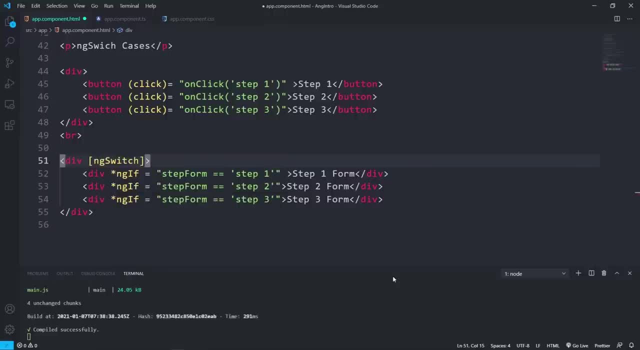 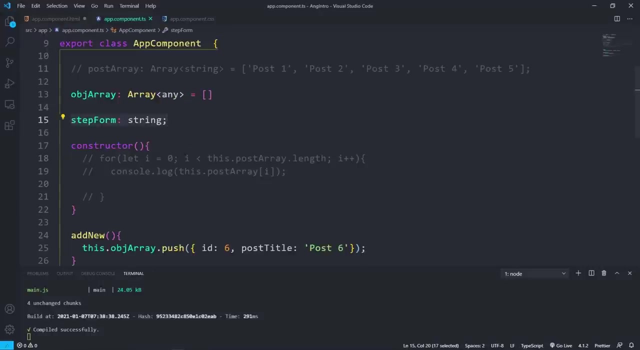 So inside square brackets: ngSwitch. Keep this in your mind: this is not an actual property in the DOM, This is just a property for this switch case directive. Now bind this to the variable step form which is declared in the component TypeScript file. 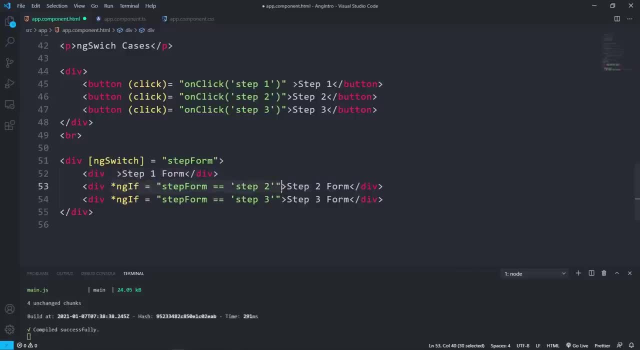 Now remove this all ngIf directives, Because this time we are going to use the ngSwitch case directive, So let's add the ngSwitch case, So let's add the ngSwitch case directive to these divs. This is a structural div. 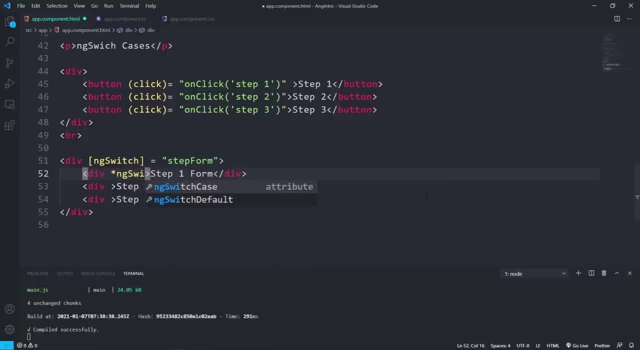 So asterisk, then ngSwitch. case This s and c uppercase. After this equal sign, Insert double quotes. Now pass the condition. I want to show this step1 form div if this variable value is equals to step1.. So pass this as a string. 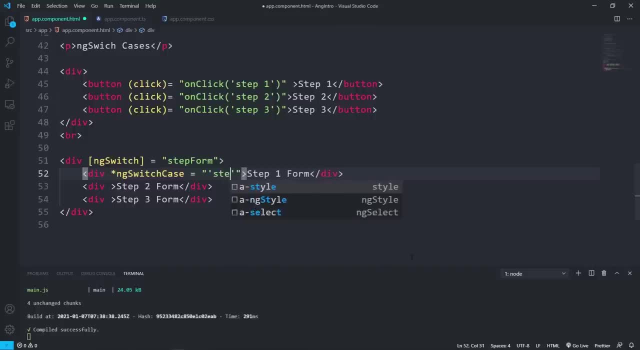 Insert this: double quotes: single quote. Now insert this: single quotes: step1.. Like this: add this ngSwitch case directive to these divs as well. Copy and paste it. This one is for step2.. This one is for step3.. 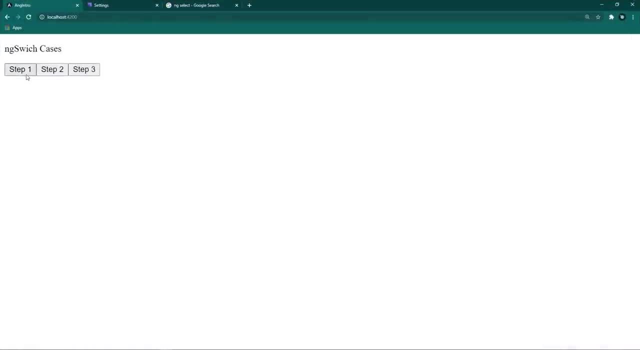 Save this and back to the browser. This is now empty, So click this: step1.. We got this message from step1.. Click this: step2.. We got this message Step3.. We got this step3 form message. So this is working as previous without any problem. 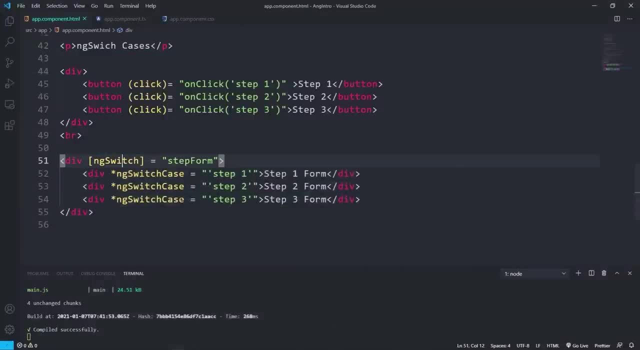 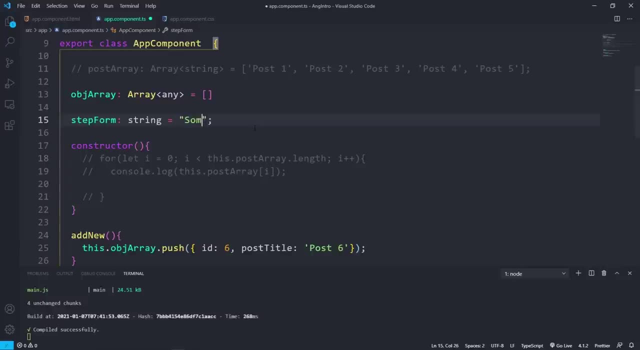 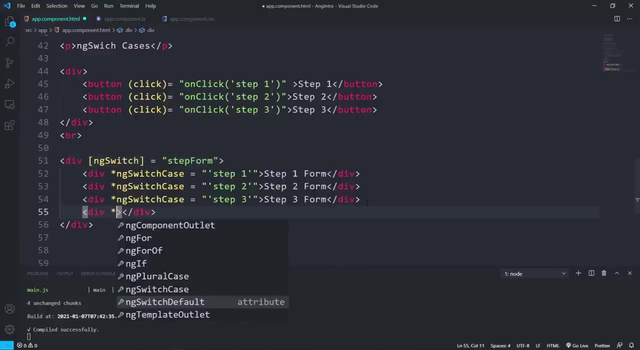 So in this switch case directive we have another option to show when this variable value is something different from these values. Let's assign a different value to this variable, Something else. Insert the html file, Create another div. after this, Insert this asterisk: ngSwitchDefault. 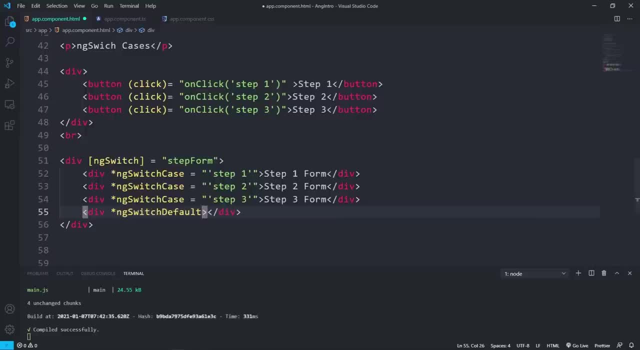 Save. So with this we are telling this switch case to show this div when there is this variable value is something different than these. So insert this div, Add this text, Something else, Save this and back to the browser. Look at this. 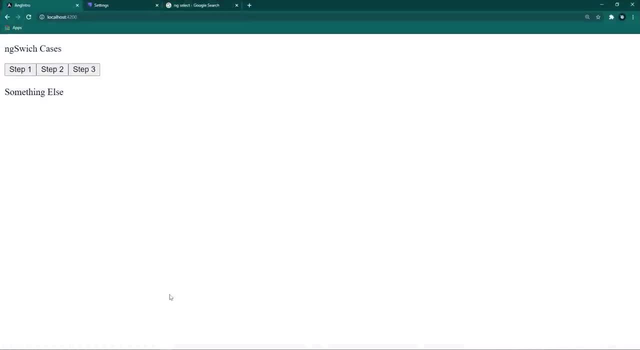 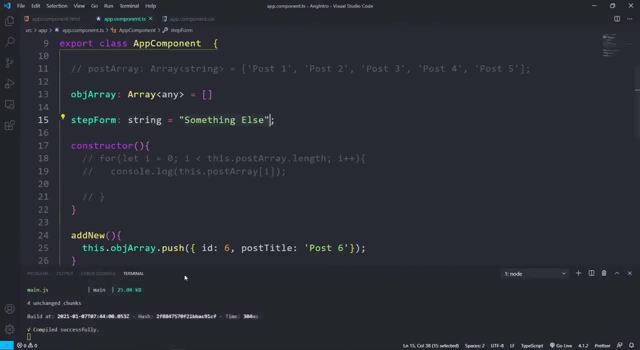 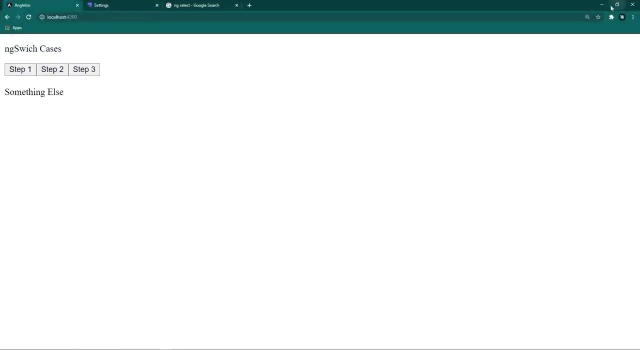 This time we got this something else message here. Why is that? At the first time this component loads inside the browser, the value of this variable is different than these switch cases, So in that case this will show this div something else. Hope you guys got the idea. 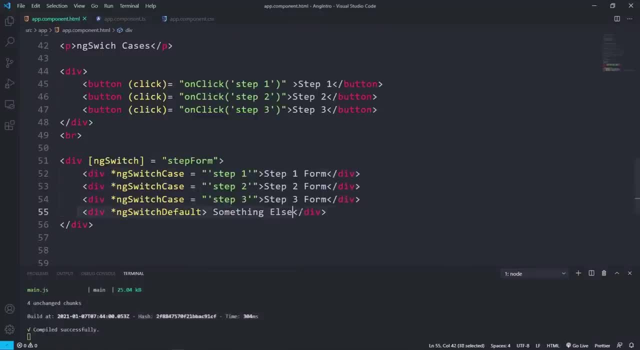 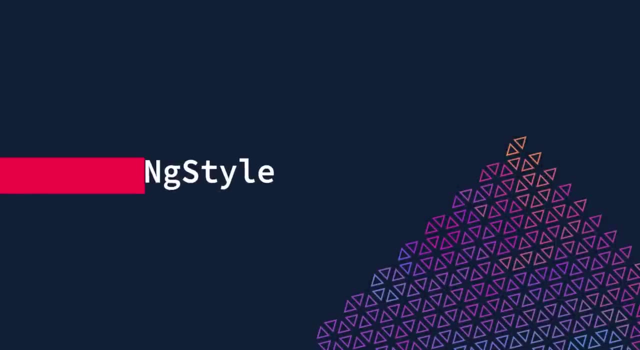 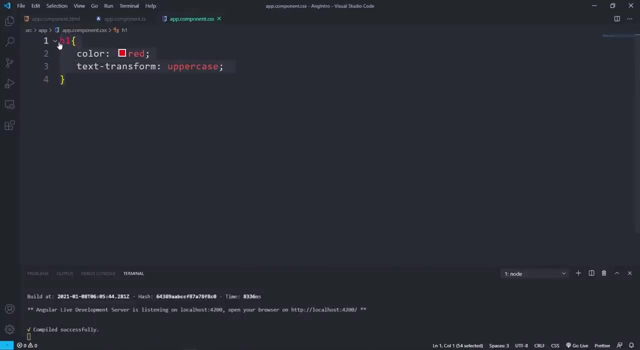 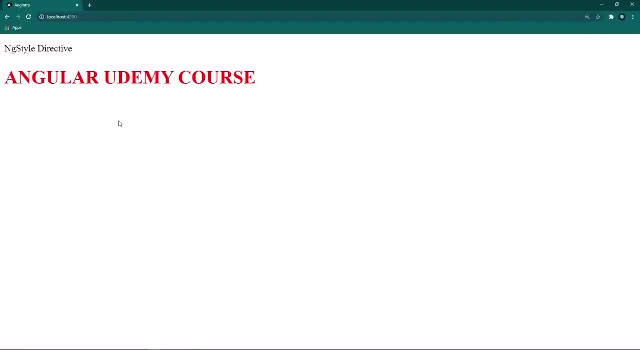 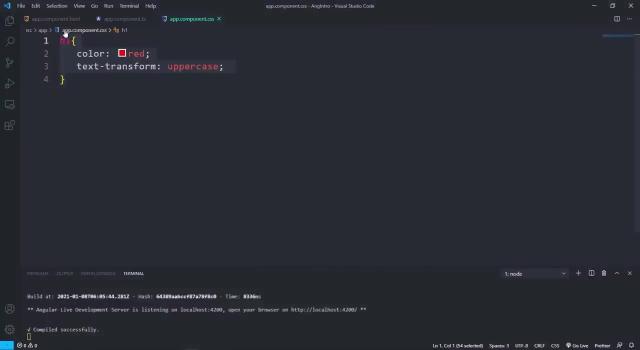 So this is how we deal with ngSwitchCase directive. in an angular app. I have this h1 tag and this has these inline styles for text color and this text transform style. This will look like something this in the browser: Think, if we want to show these styles with a condition, how we going to do that. 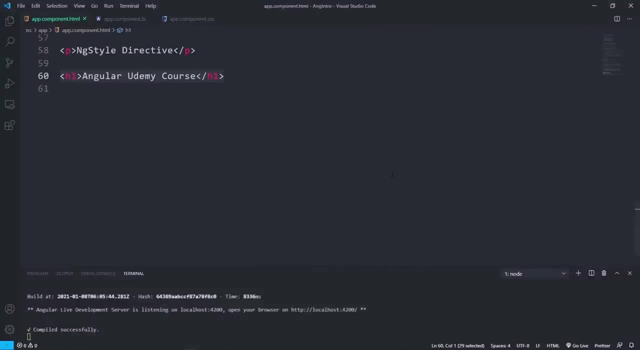 In previous, we used this style binding approach for this. Something like this: Inside this h1 div square brackets. So we are doing a style binding, So style dot and the CSS property color. Assign this to the condition variable that I already did. 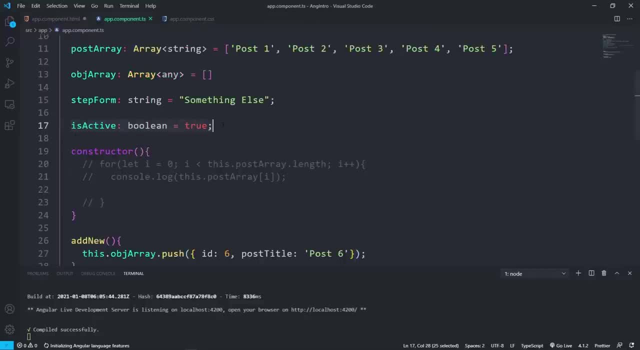 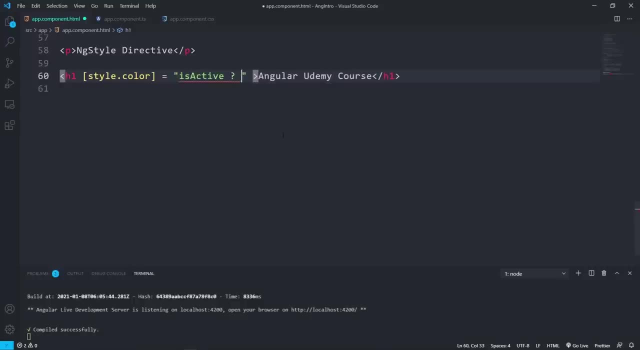 Defined in the TypeScript file is active variable, So pass that variable to: this Is active. If this is true, this will set this h1 tags color to red. otherwise set this to black. In here we have another style to make this uppercase. 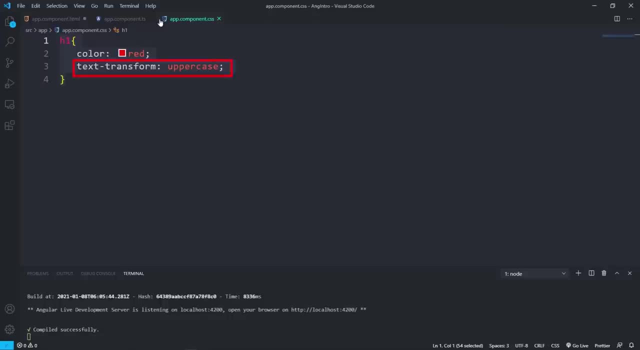 Let's add that also using this style binding, After this, another style binding. I'm going to break this to next line so we can see this clearly. Inside quotes: style dot text transform. So this is the DOM style object. So this T is capital. 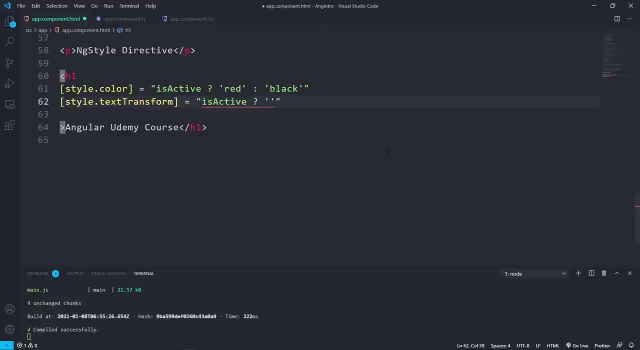 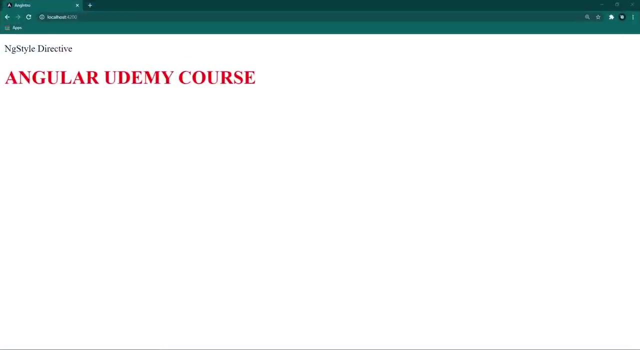 If this is active variable is true, set this to uppercase. If not, set this to lowercase. That's it. Now we don't need this inline style, So remove it, Save this and back to the browser. We got this uppercase red color h1 text. 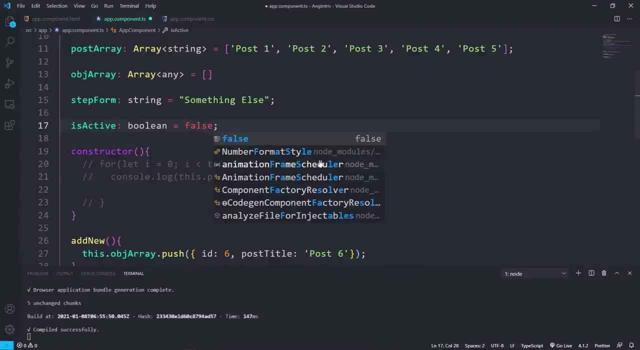 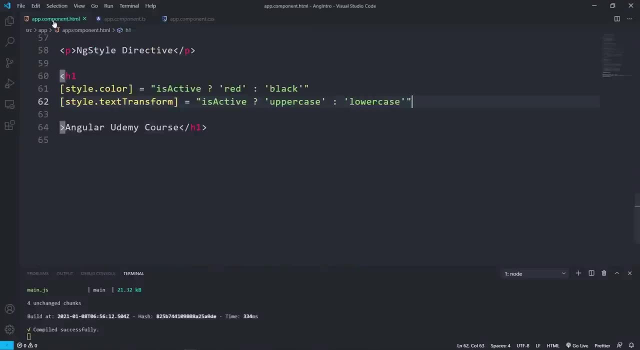 Let's remove this. If I change this to false, now this h1 is in lowercase and black color. If you look at this code, we are repeating the same style binding syntax several times. This is now looking nice right In angular. we have a better and cleaner solution for these kinds of multiple style binding. 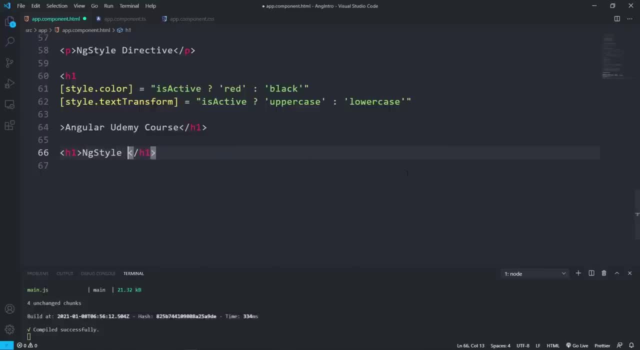 approaches, which is ng style directive. We can do this Same. We are going to add a style binding using this ng style binding. Let's see this in action. This is an attribute directive, So inside the square brackets ng style, this S must be capital. 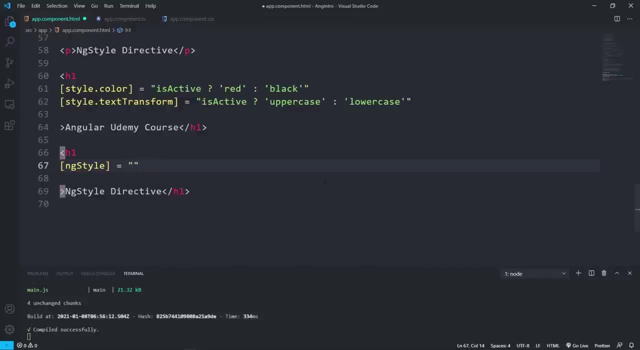 Equal sign. double quotes. Inside this quotes: we're going to pass the all style bindings as an object, So open and close square brackets. Now add the style binding using the key value pair. As a key, We pass this style property and as the value, we will pass the conditional CSS value. 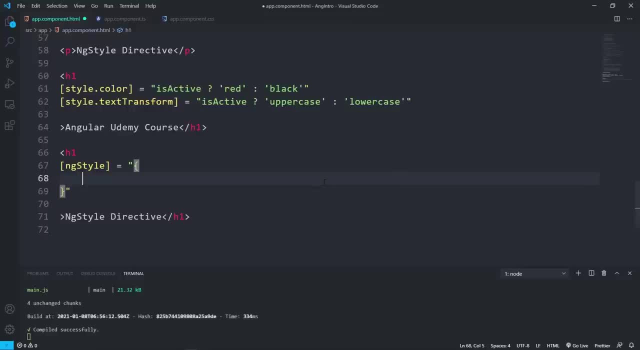 Pass the CSS property as the key. First I want to set this h1 text color, So CSS property is color colon. Now the condition is active. If this is true, we represent that using the question mark. Set that. Let's add this to red color inside single quotes. 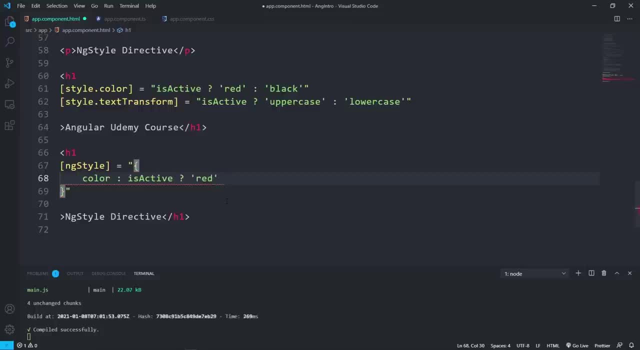 CSS value is red. That's it Like this. let's add the second style After this comma key is text transform. This T must be capital. Colon Condition is is active. If this is true, set text to upper case. 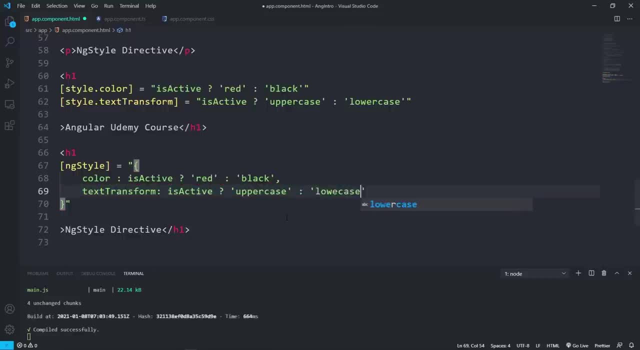 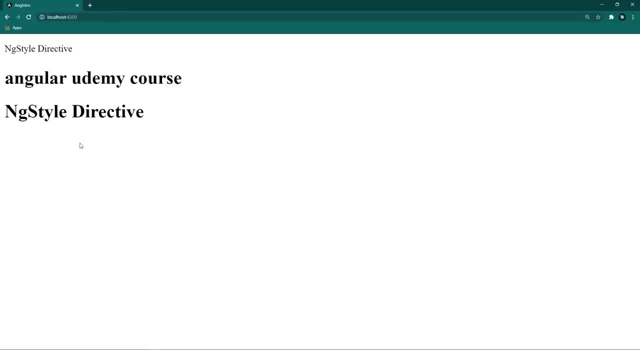 Otherwise, set this value to lower case. That's it. Look at this code Now. this is more clean and readable than the previous code. Now save this and back to the browser. As you can see here now this h1 text is in lower case and black color. 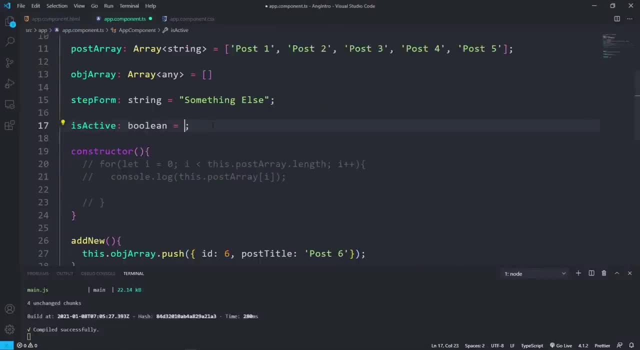 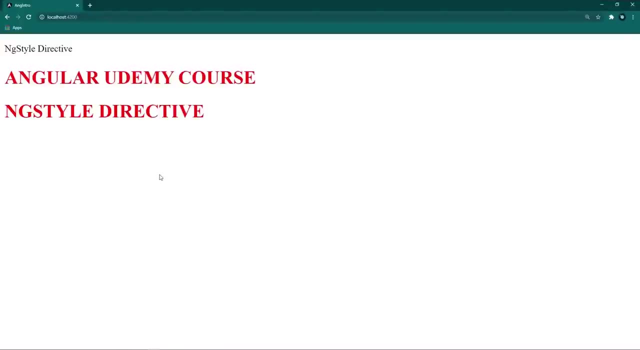 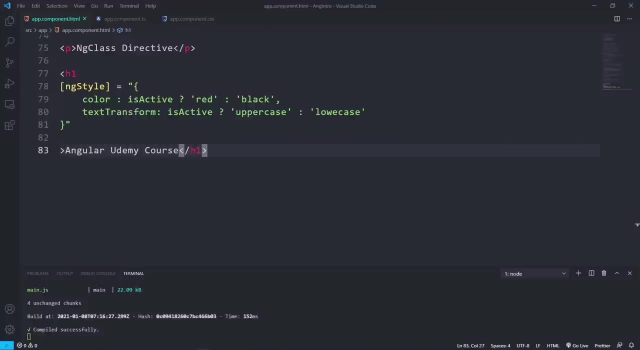 Now this condition is false. Set this to true, Save this and back to the browser. Perfect, Now we got this red upper case h1 text. Beautiful, isn't it? So this is how we use ng style directive in angular. Always doing this multiple inline style binding is not a good practice. 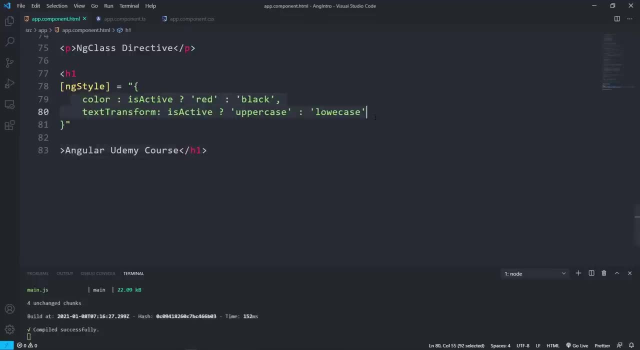 Usually in CSS, if we have something multiple CSS like this, we put this alt style inside of a CSS class and we'll add that class to this h1 tag, Right? So I'm removing this ng style directive In case, if we want to show this class conditionally, we can use the class binding. 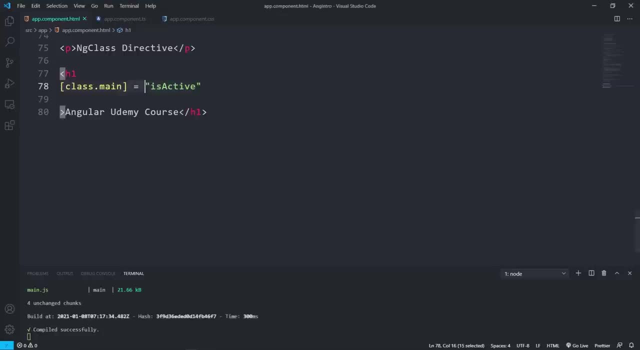 Something like this: Right Think, if we have another separate CSS class for font-weight and we want to add that class also using the class binding conditionally, How do we going to do that? Very simple, We have to nest another class binding here. 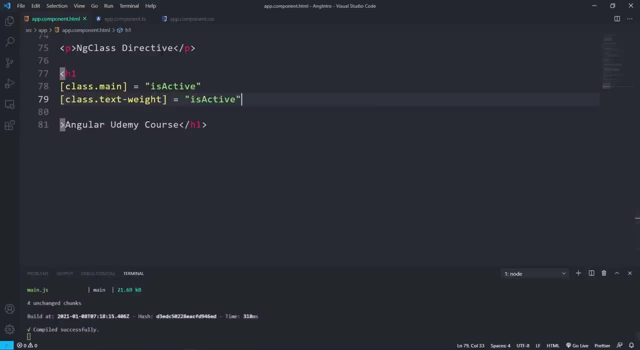 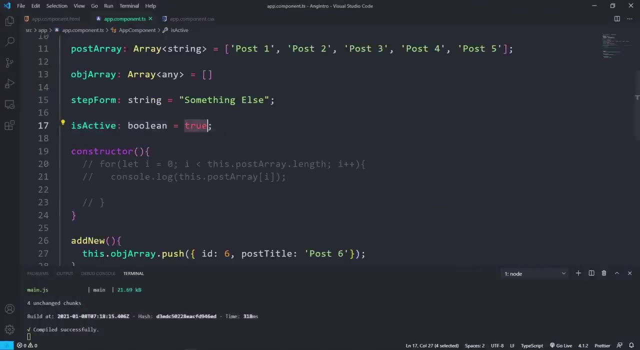 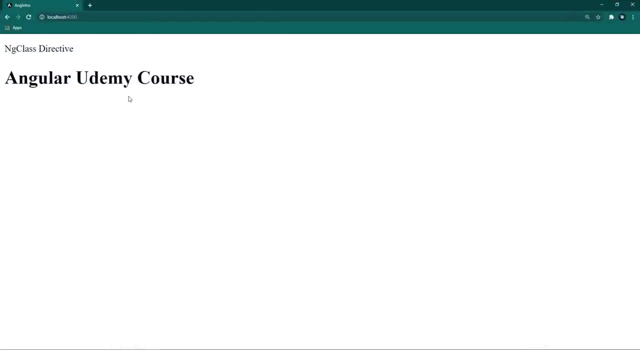 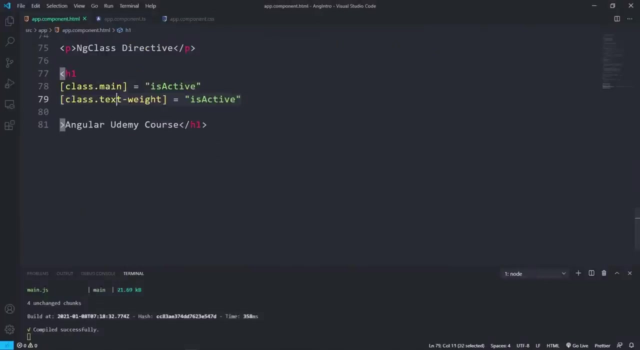 Like this. Save this and back to the browser When this variable is active is true? we got this. If I set this variable to false. save this and back to the browser. So this is what we got. All right, As I said earlier, we have a better approach. rather than nesting these class bindings. 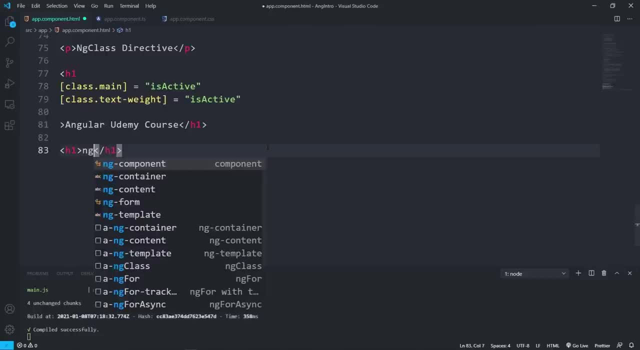 Like the previous ng style binding, we got another directive for bind CSS classes, called ng class directive. Very similar to the previous ng style directive. So let's see this in action. Inside this h1 tag: open and close square brackets. Inside this: 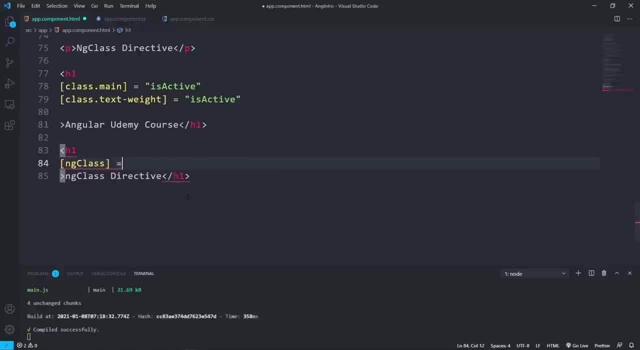 ng class. This C must be capital, after this equal. Now we have to pass the CSS classes that we want to bind to this h1 tag as an object. So inside double quotes, open and close a square bracket. Now, inside this object, pass the target CSS class as a key. 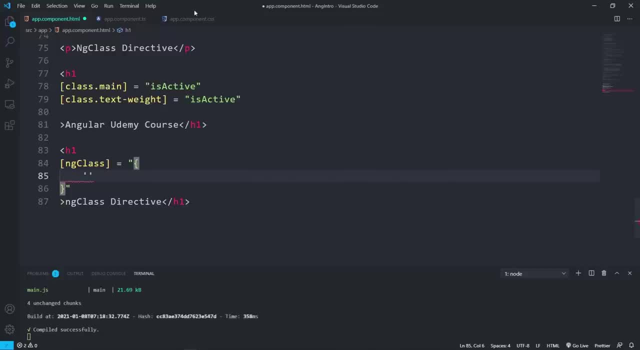 So inside single quotes, The first CSS class is This main CSS class, CSS class colon. now pass the condition as a value for this isActive, that's it. Do the same for the second text weight CSS class as well. The key is this CSS class: inside single quotes, text dash: weight and value is the condition. 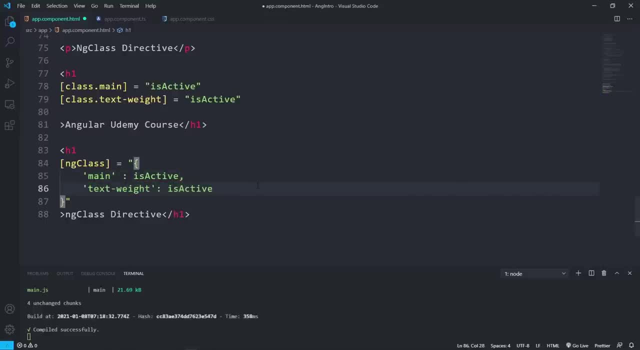 isActive, don't forget to add the comma after this first condition. So with this we are saying: if this condition is true, bind this CSS class to this h1 tag. Very simple, right? Look at this code. very clean, right. 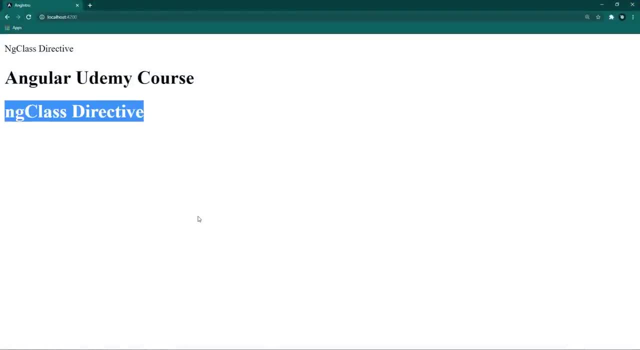 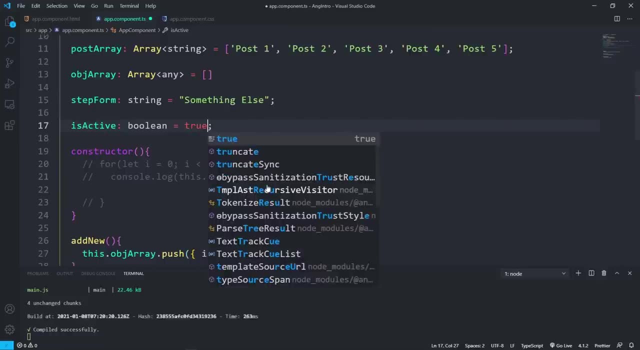 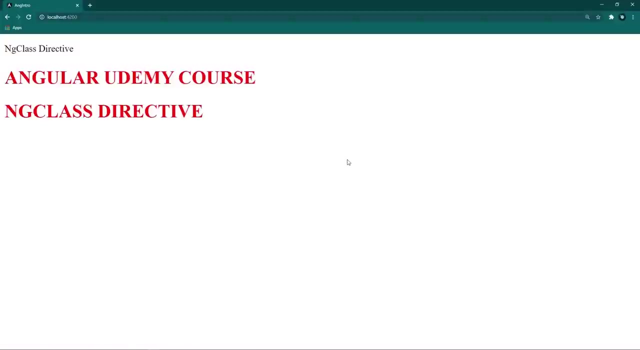 Save this and go to the browser. We got this black color lowercase: h1 text. cause: this condition is now false, So make this to true, save and back to the browser. Perfect, We got this red uppercase. This is boldy, look. h1 text. 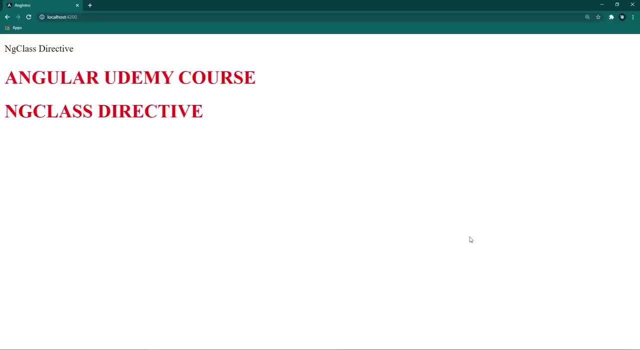 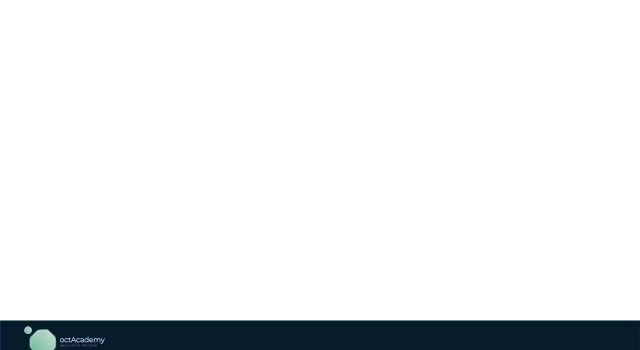 So this is how we deal with ng class directive in angular. Alright, now you guys have an idea about angular directive. In the first lecture of this section, if you can remember, I said that we have four main directive types in angular. The first one is component directive, which is the angular class. 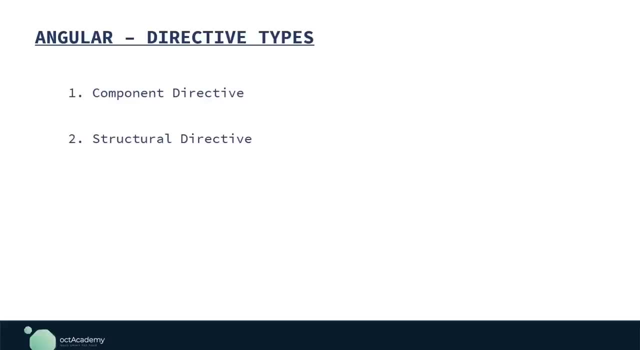 Angular component. the second one is structural directive. third one is attribute directive and the last one is custom directive. So in this section let's look at what is structural and attribute directive. The first: what are the structural directive? Structural directives are responsible for the HTML layout. this structural directive. 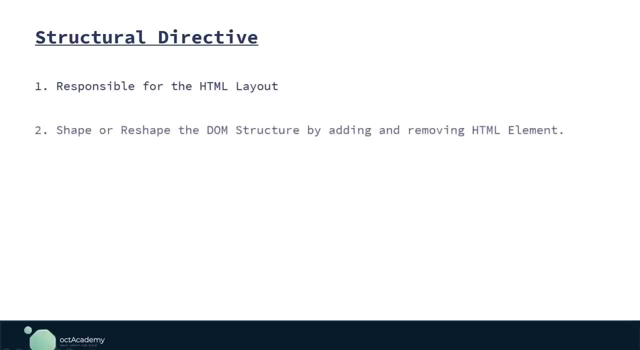 shape or reshape. It is the DOM's structure, typically by adding, removing or manipulating the DOM elements. Structural directives are easy to recognize with the leading asterisk symbol. So we learned several directives in this section. So we have few directives with the leading asterisk or the star symbol which are ng. 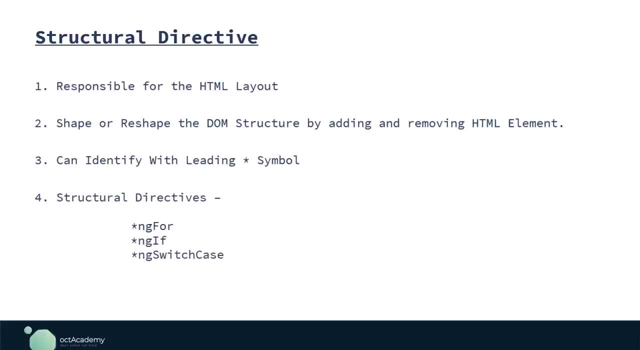 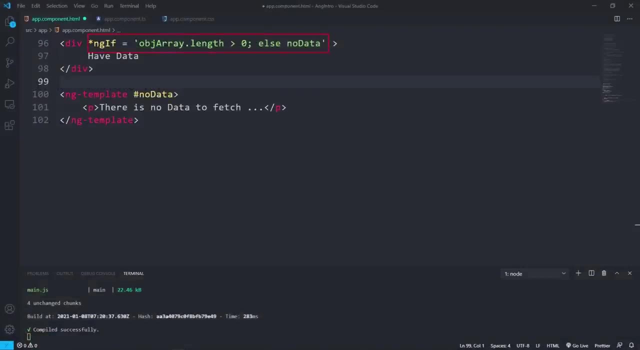 for ng if and the ng switch cases. So these are the structural directive. Let's look at some examples. I have created just a few examples for this. The first one: the ng if directive. So what is happening here With this ng if directive? we're showing this div when this statement is true. 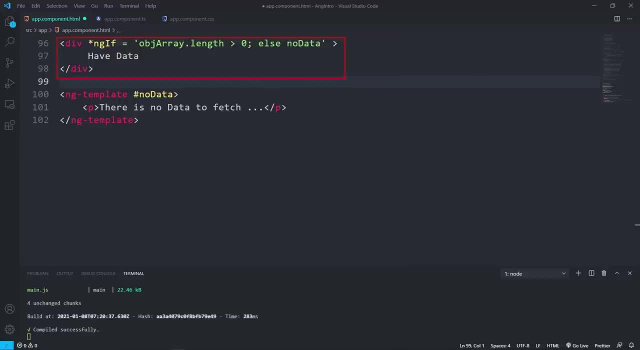 So this will add this div to the DOM when this is true. If this is not true, this will remove this div and this will add this ng template inside the DOM. So with this ng if directive, we are manipulating the DOM's structure by adding and removing. 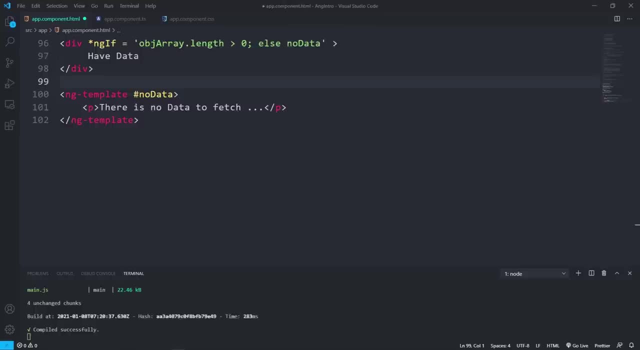 elements to the DOM. So this is why we called this ng if directive as structural directive. If you look at this second directive, ng for this- also add this list element to the DOM by fetching an array. If there is a data inside the array, this will add list elements to the DOM. 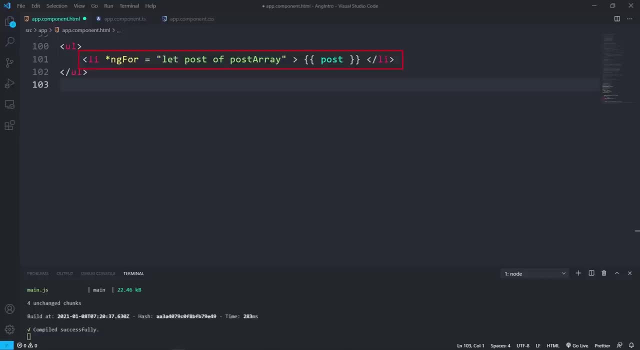 If there is no data will remove the list element from the DOM. The switch case also the same. If this is condition is true, this will add this to the DOM. If the statement is false, this will remove this from the DOM. So this is what we called structural directive. So here is the lesson With the 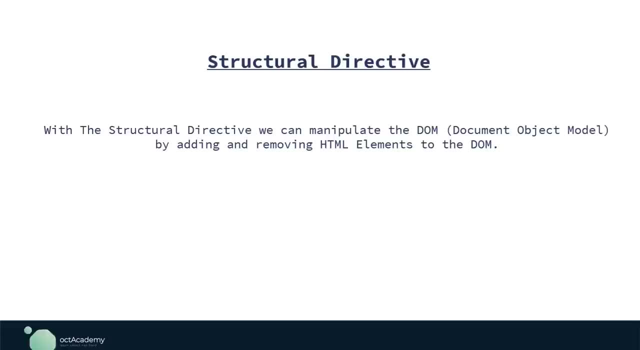 structural directive. we can manipulate the DOM by adding and removing DOM elements dynamically. So for a structural directive we use this leading asterisk symbol, So we can easily identify a structural directive with this leading asterisk. So let's look at the attribute directive. So what? 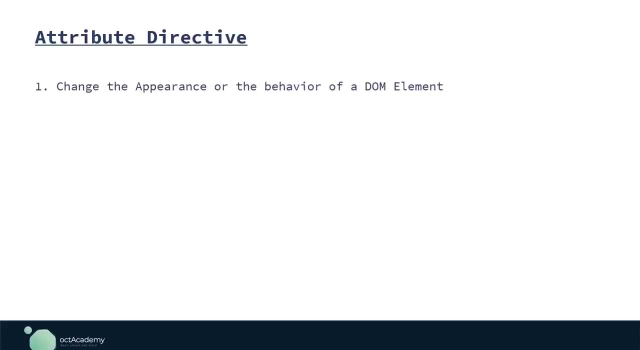 is attribute directive. An attribute directive changes the appearance or behavior of a DOM element. We can name ng-style and ng-class directives as attribute directives. You guys already have seen the attribute directive, So let's look at attribute directive in our example. knew with these attributes, we applied styles to an element conditionally If the statement is true. 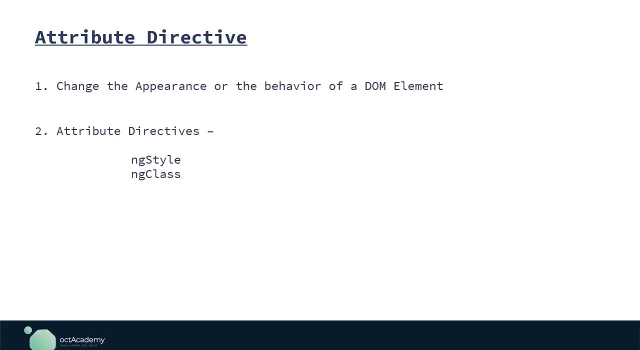 this will add this style to the DOM. If the statement is false, this will remove the styles from the DOM. So, simply, this is what we can do with attribute directive. We use these attribute directives as like property binding inside of a square brackets. We are not adding any leading. 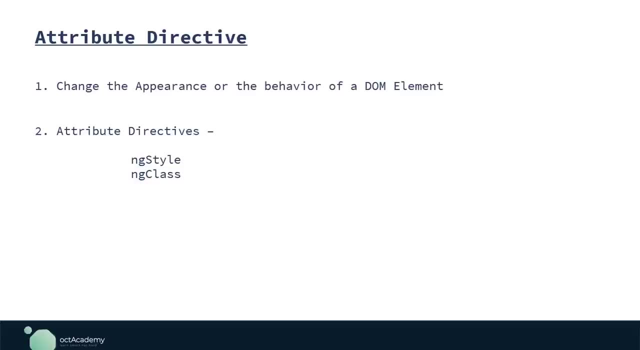 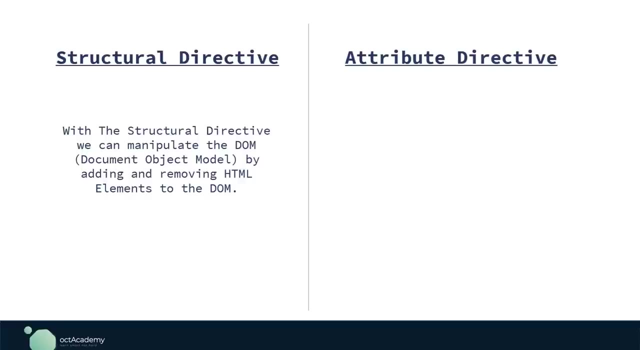 asterisks, because this is not a structural directive. So here is the lesson: With the structural directive we can manipulate the DOM by adding and removing elements to the DOM's structure, But with the attribute directive we can only change the appearance of a DOM element. 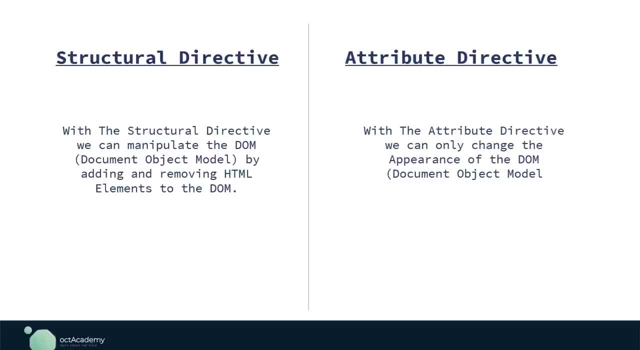 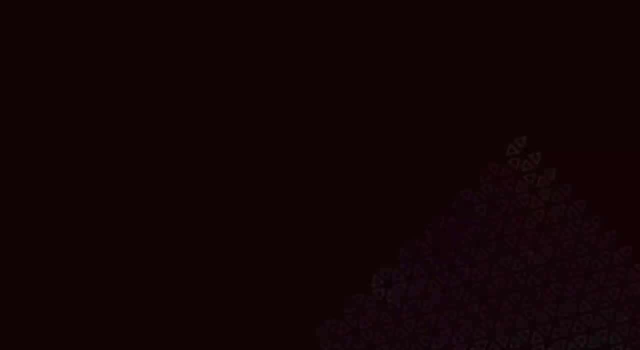 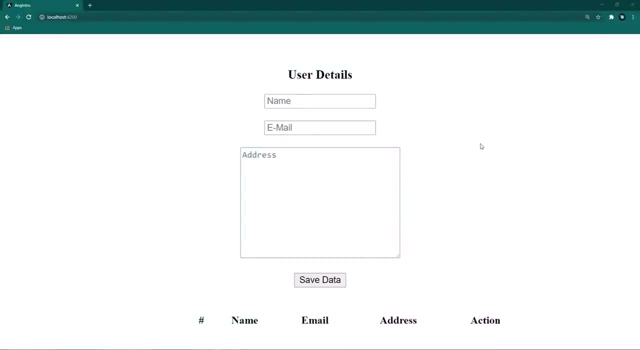 We cannot manipulate the DOM using these attribute directives. So hope you guys got the idea. All right, let's do a small task to recap what we learned in this section. So this is the task: Create a simple form like this. This form has three fields: Name, email and address. For the address: 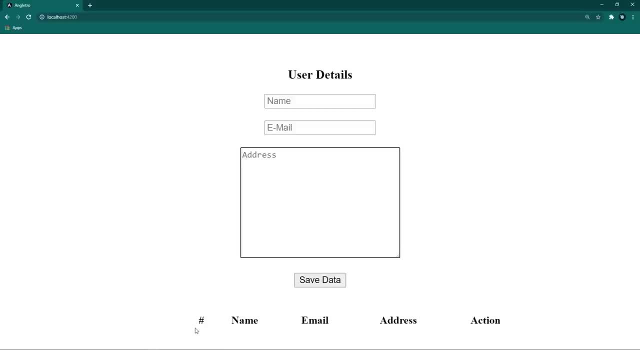 use a text area. Down here we have a button called save data. So after this form, we got a table with these TH heads. The first column is for the number, Second column is for name, email address and the last column is for action. So fill this form and click this button. Look at the table. This will load this. 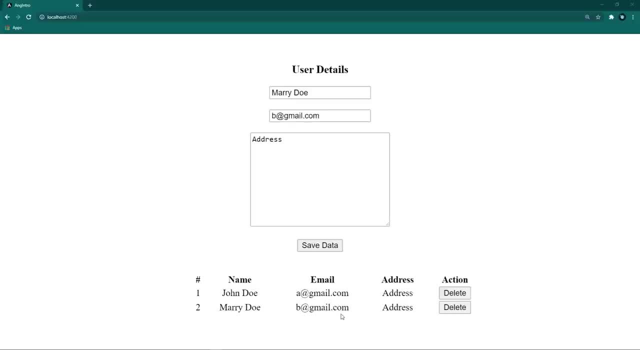 form's data Again, type something and hit the save button. This time also, data loaded inside the table. Inside the table, every row got this Delete button Inside the action column. If I click this delete button, this will delete this data from the array. 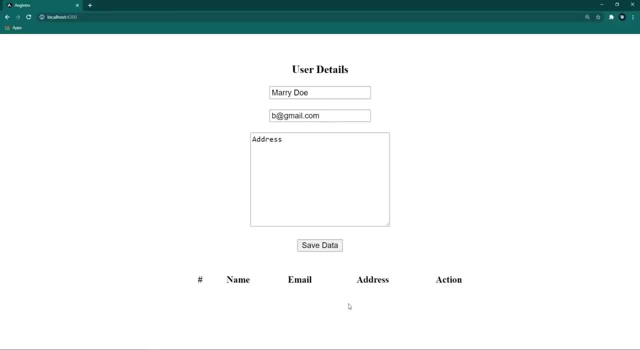 Again. click this delete button. This is removed from the table. So create this simple app using the help of angular directive methods and data binding. Very simple, As always. try to do this on your own. Once you completed the task, continue with the next lecture. See you soon. 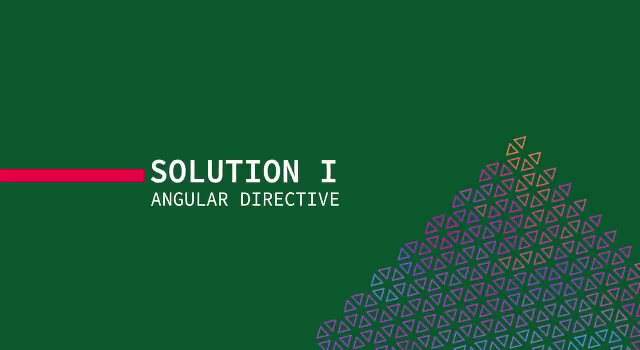 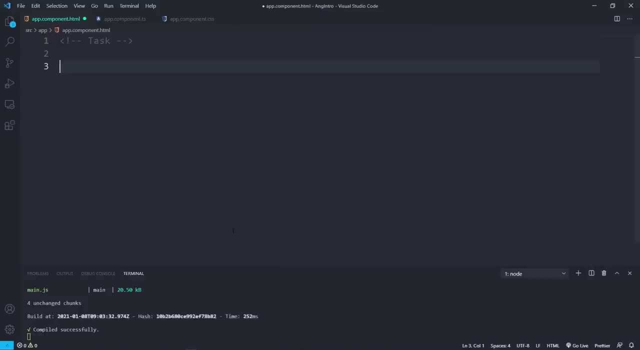 reinforcement. All right, I hope you guys did the task well, Imcast. if you missed any thing, continue the task with me. First, let's start with the form. So create a div with class form dash area. So inside this form, x3 tag with text user details. 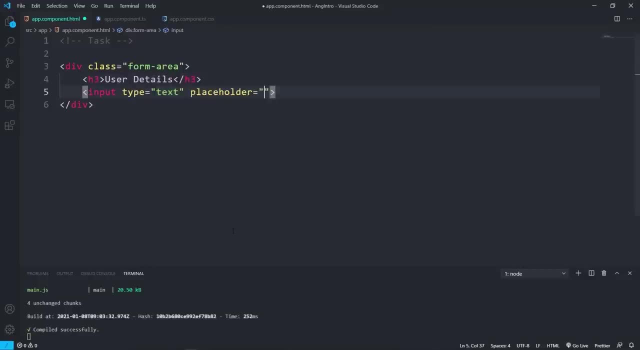 The first input field for the name. second field is for email. at last text area for address. after this, a simple button for save data and don't forget to add BR tags to get a nice vertical form layout. save this and back to the browser. let's make this form. 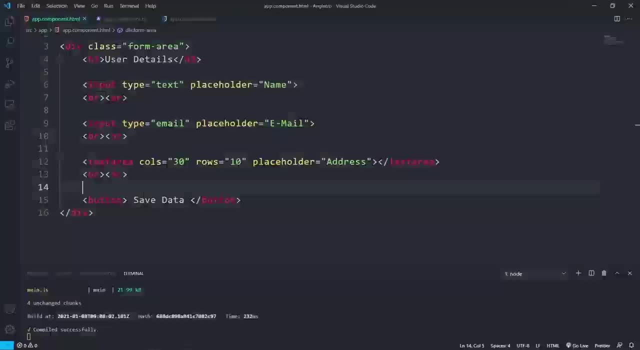 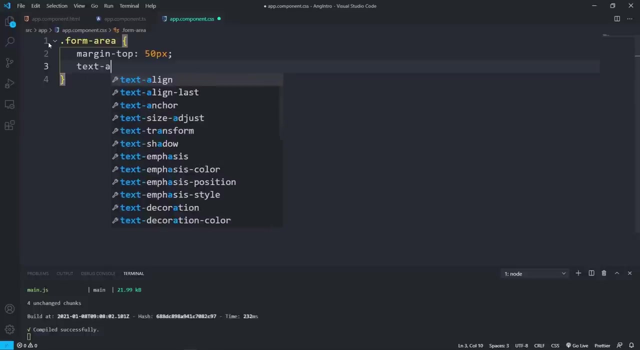 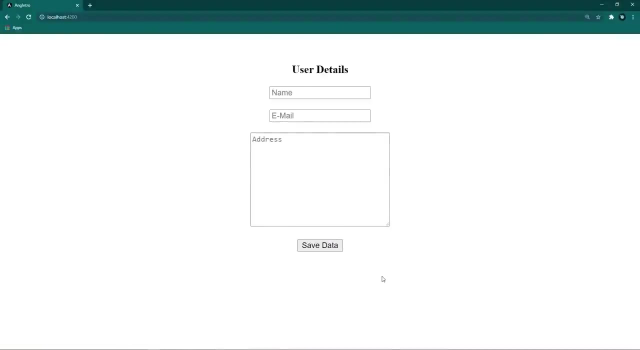 center to the page. add a CSS style to this class form dash area inside the CSS file dot form dash area and the CSS scope inside this. add these styles: margin dash, top 50 pixels, text dash, align center. now save this and back to the browser. perfect, we got this nice looking form. next we have to do the two-way data. 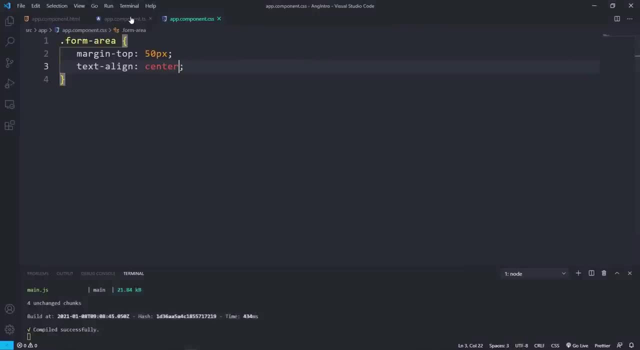 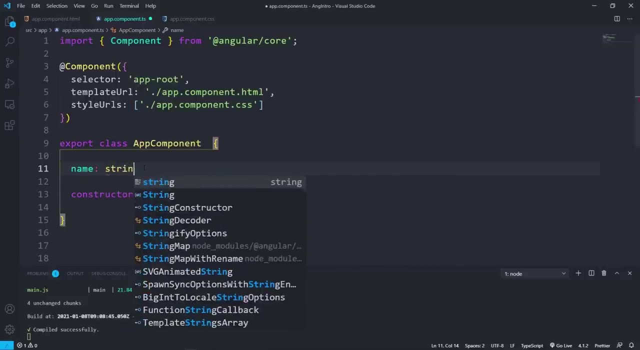 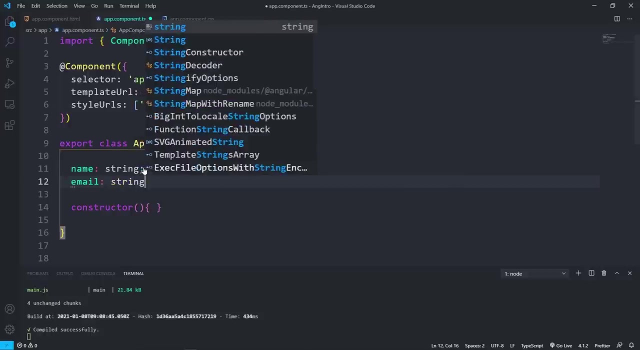 binding to get these inputs values. so create three variables inside the component TS file. first one is name and the data type is string. the second variable is email and the data type is string. the last one is for the address field, so this also a string. all right, now let's bind the data to these input fields. 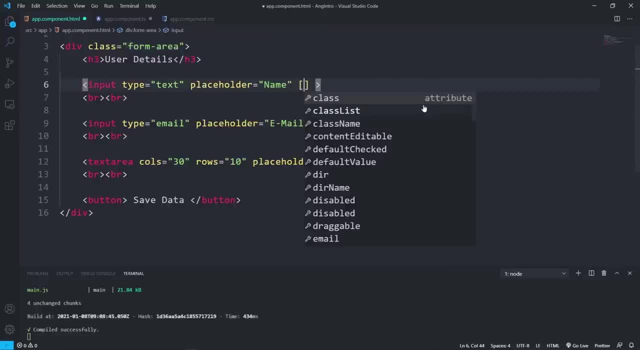 using two-way data binding. inside this first input: open and close square brackets inside this. open and close another simple bracket. so inside this ng model now bind this to this name variable simple. right after this, copy and paste this ng model to the second input and change the variable name to email again. 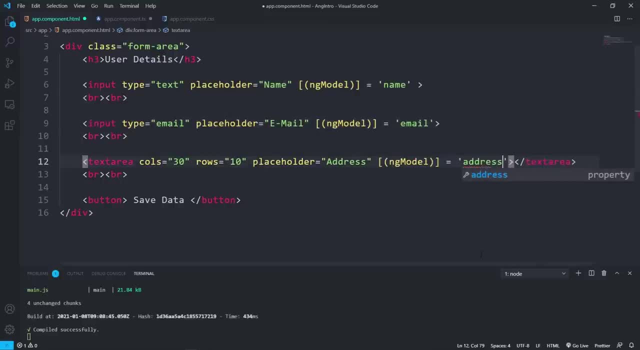 paste the ng model for this text area as well and change the variable to address. all right, now we have successfully bound all the input fields to these variables. next let's make this save data logic. so here's the logic: if someone clicks this button, I want to save this text: fields value to: 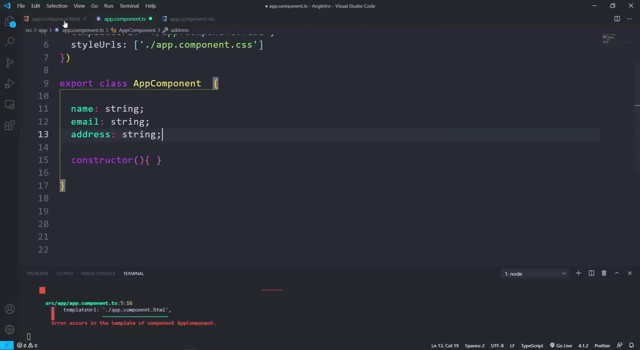 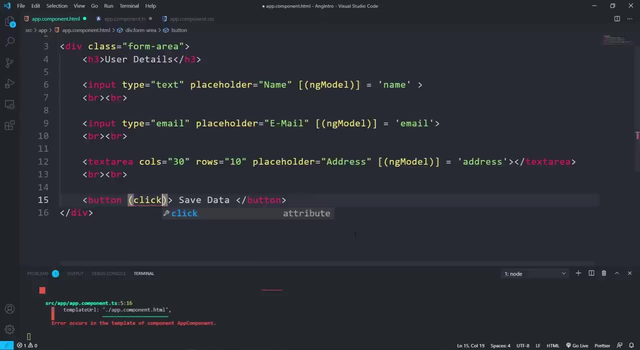 to an object array. So let's do that. First, let's add the click event to this button. Inside the button tag: open and close a bracket. Inside the brackets, the event is click Equal sign. Inside quotes: method name is onClick. after this parenthesis, Still we don't have 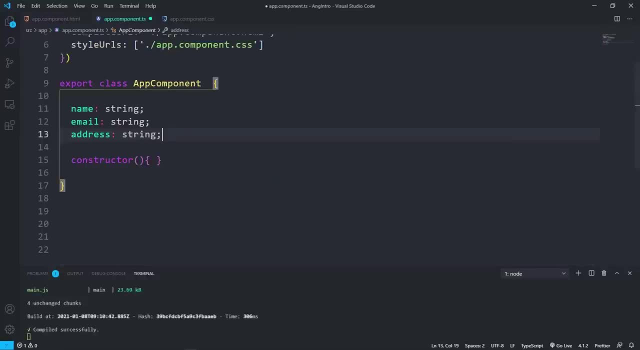 this onClick method. that's why we are getting this error. Let's create this method inside the TypeScript file. Method name is onClick parenthesis and the method scope: Let's declare an empty array variable: User array, the data type is array and array type is any. Now assign. 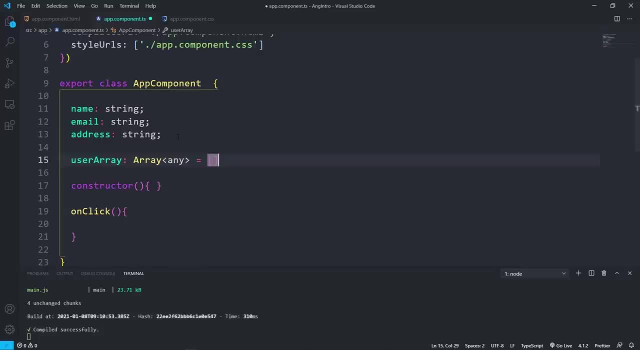 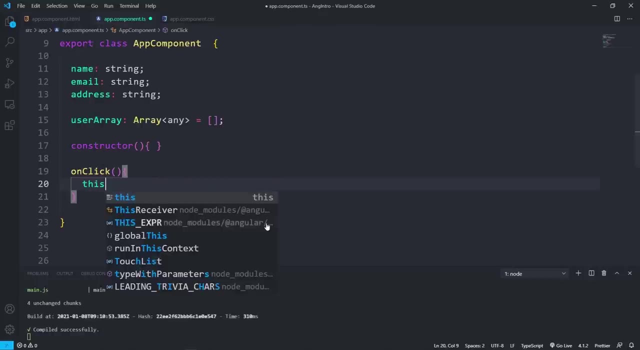 this to an empty array, then only we can push data to this array. Now let's push the data to this array using this onClick method. This dot array name is user array dot push. after this parenthesis, Now let's pass the object here, So open and close the curly brackets Inside this first key value pair. 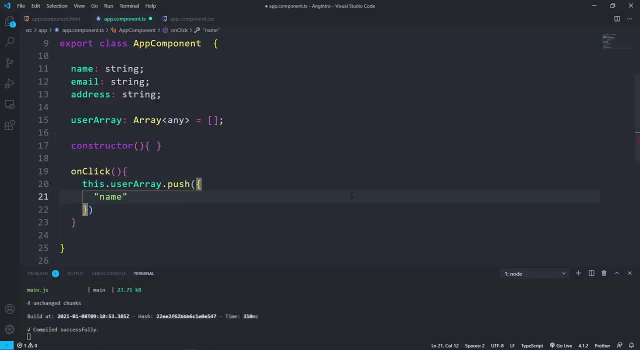 is for this input name, So the key is name and value is this variable name, So this dot name, This comma. The next one is for the email field. The key is email and the value is this dot email. After this again comma. The last one is for the address, So the key is address. 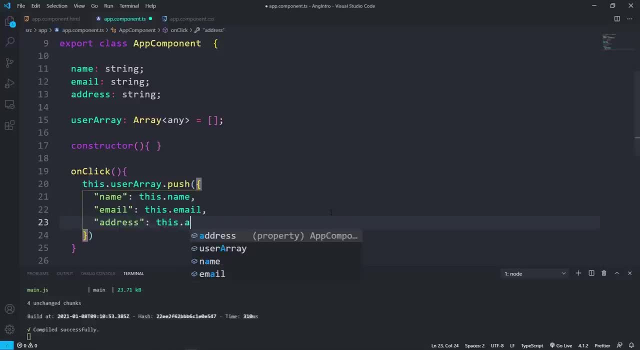 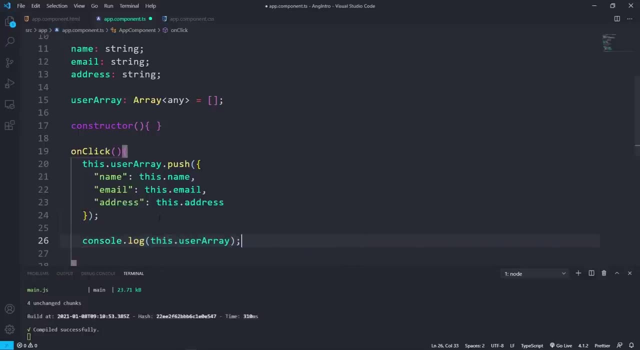 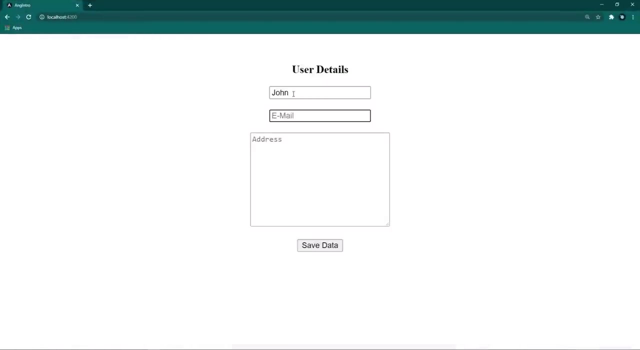 and value is this variable address, This dot address. That's it For now. let's log this array to see whether this is working or not. So save this all and back to the browser. Fill this form. Just fill it with random text. 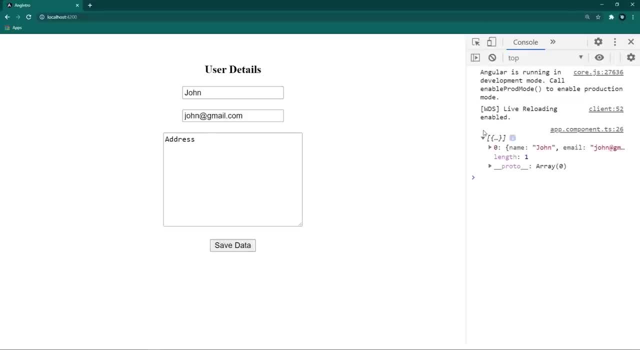 Click the save button. Look at the console. Awesome, We got this array log with this object, So click this button again, again, again. Perfect Right, We got all the data pushed inside the array. Okay, Great, I hope you find this today helpful. Next, we have to render this array inside: 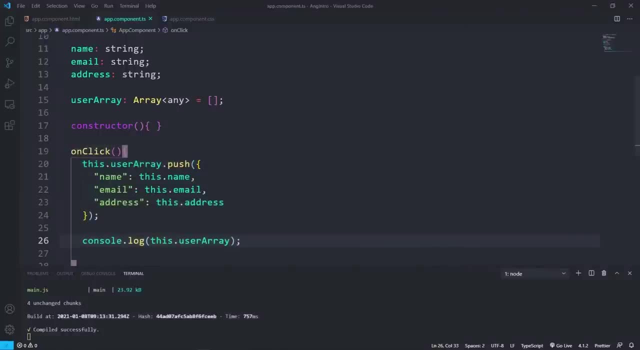 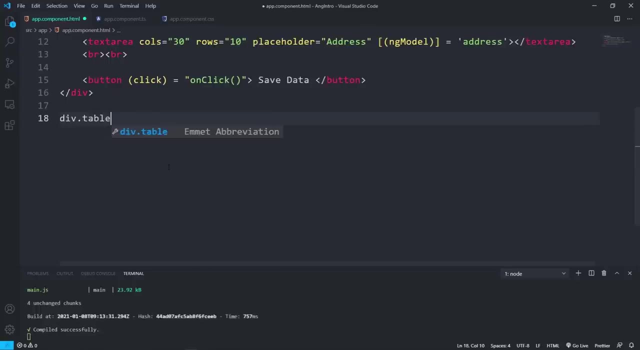 some HTML table. Let's create the HTML table down here. Oh yeah, I'm pretty good with my audio and I'll post the más inside the HTML file After this: create a div with class table dash area Inside this div. let's create the table table. Hit enter Inside this t head. Hit enter Insight: this: 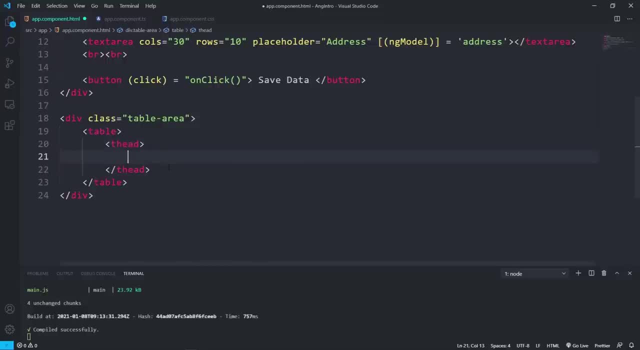 t head, Hit enter And we're done. wandering complicated Very fast, So before we start this field, Let's look into page 4.ğıç przyp Hash�ar y チ, Idahoی. Inside this THead 5 columns, so create 5 th tags. 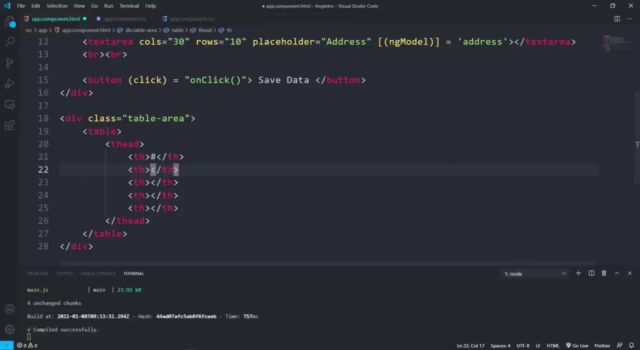 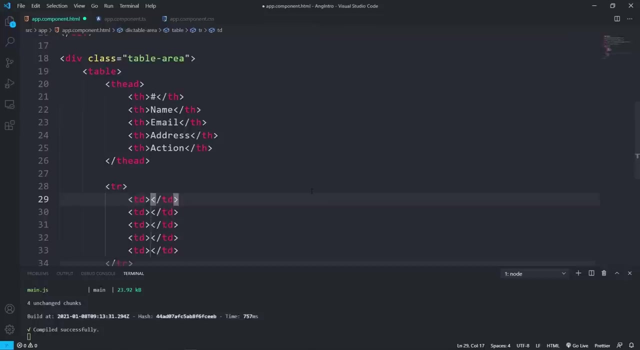 The first one is for the number, so add the ash symbol. The second column is for the name. next email, next address, at last action column for the delete button After this THead tr tag inside this. we need 5 td for these 5 column, alright. 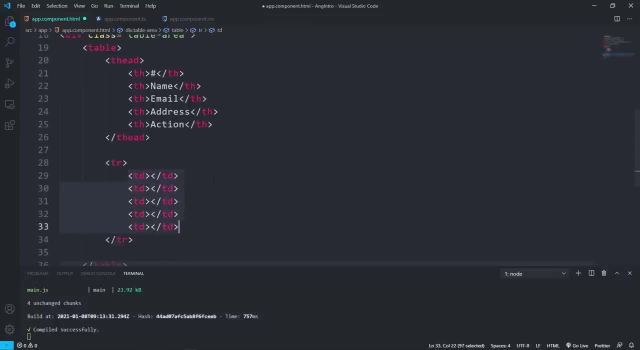 Now let's render the arrays data inside this tr tag. For this we gonna use the ng4 directive, So this is a structural directive. so asterisk symbol ng4, assign next inside the codes: let user of array name is user array. 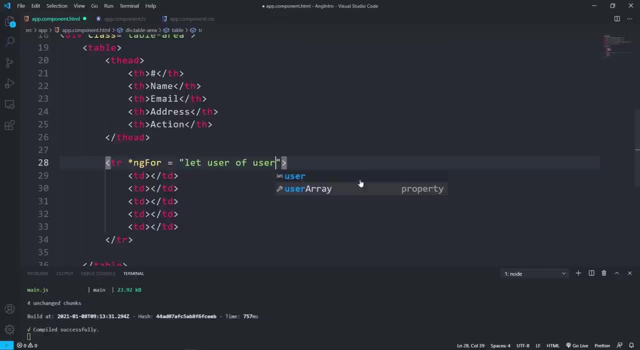 So this a must be capital. After this semicolon, we need the index as well. So let index assign index. So this index variable is created now. This name can be any name and this index is coming from the ng4 directive. 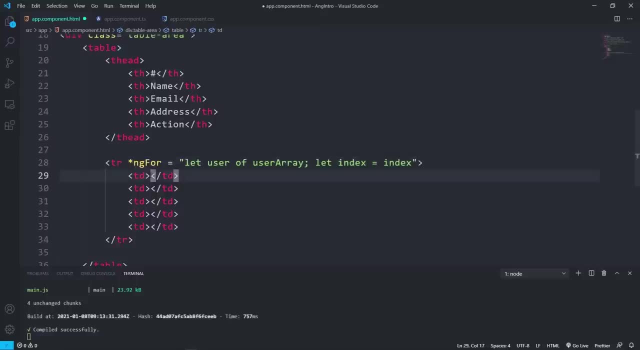 Okay, now let's show this ng4 data using the string interpolation. For the first tag: want to show the numbers, So for that let's use this index Inside string interpolation index. For the second td: show the name. next email after the email address: 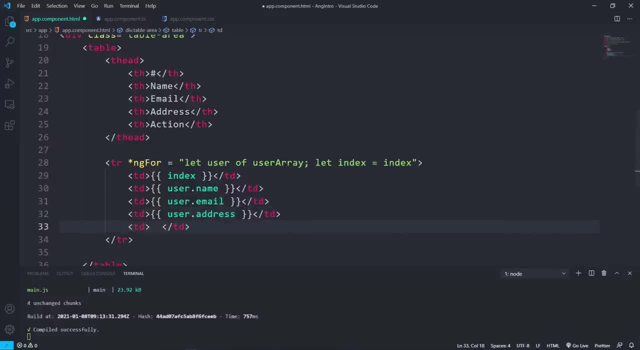 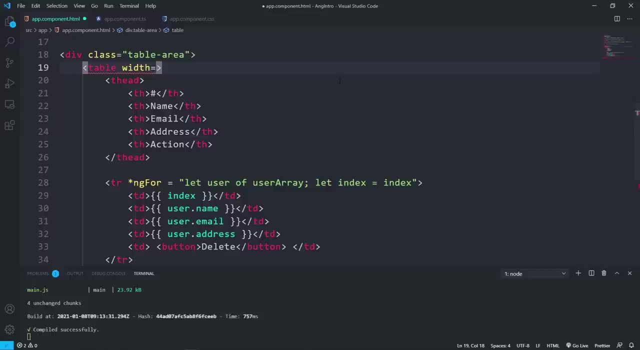 And for this last td, let's add a delete button Inside this tr. create the button tag. Button text will be delete. Now let's add the width attribute to this table to get a nice looking table. So set the table width to around 500.. 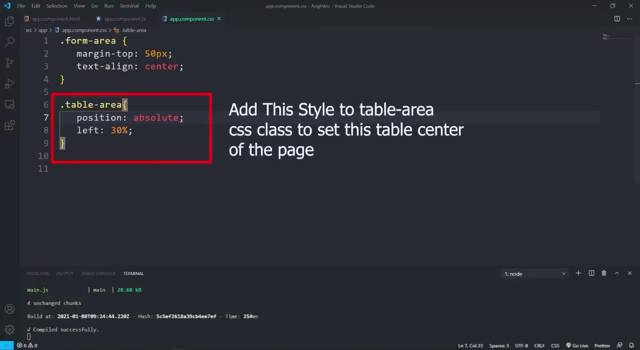 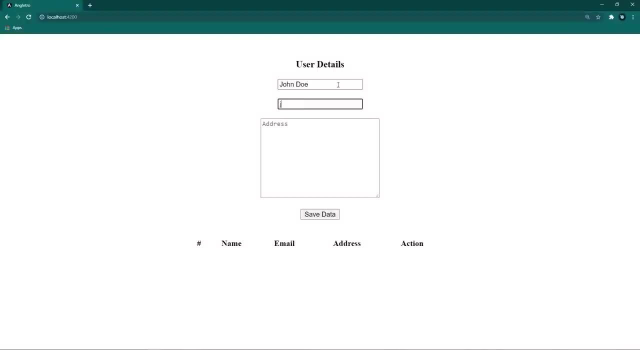 Save this all and back to the browser. Fill this form and click this save data button. Look at this. we got this data inside the table Again. click this button. we got this again. So this is happening real time, without refreshing the browser. 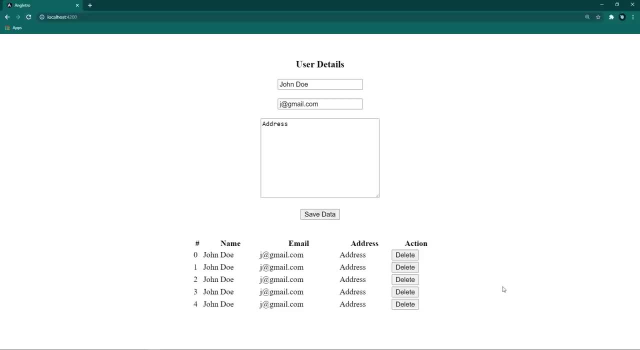 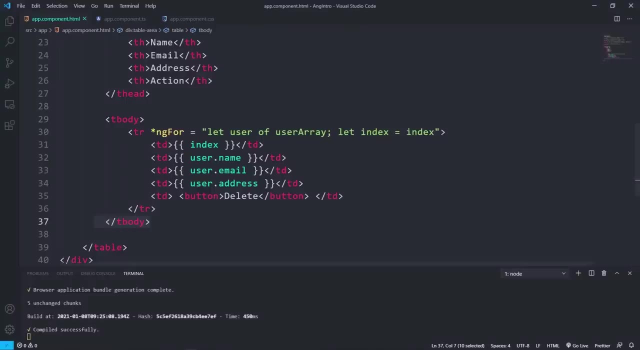 This is the beauty of angular change detection mechanism. So alright, Okay, Look at this number. this is started from zero. why is that? Cause array index is starting from zero, So I want to make this start from number one. So back to the vs code. 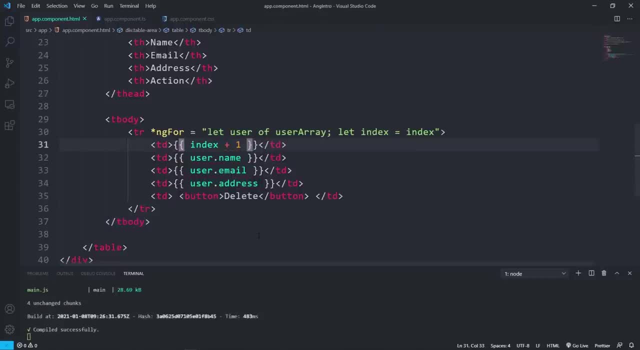 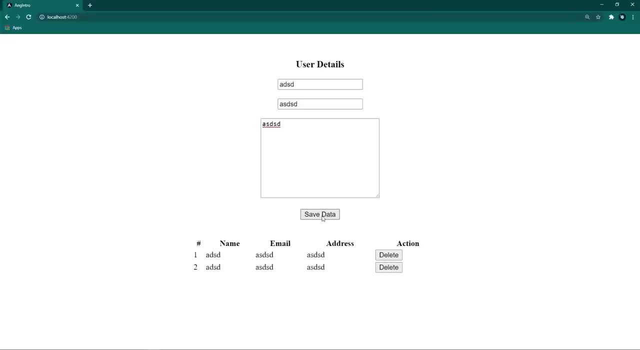 Increase this index value by one. Save this and back to the browser. Fill this form. Hit the save button. Perfect, Now we are getting these numbers starting from number one. Alright, Let's do the delete button logic. The logic is: when someone clicks one of these delete button, I want to delete that relevant. 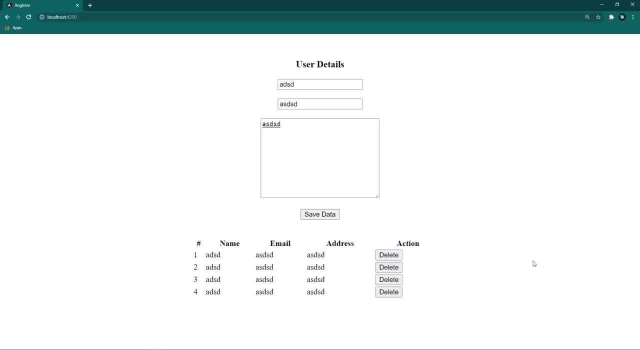 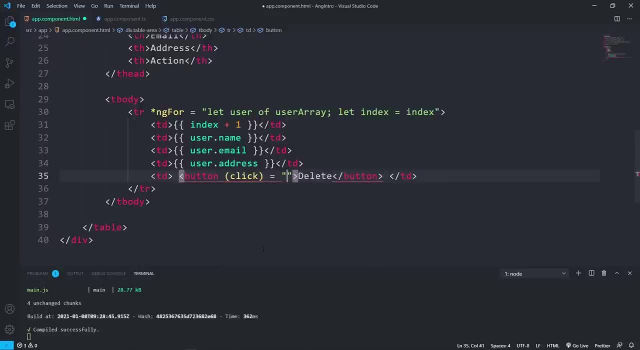 data from our user array. So let's do that. First, let's add the click event binding to this button. Inside brackets: click bind this to method name. called on: delete After this. don't forget to put the parentheses. cause: we are calling a method, not a variable. 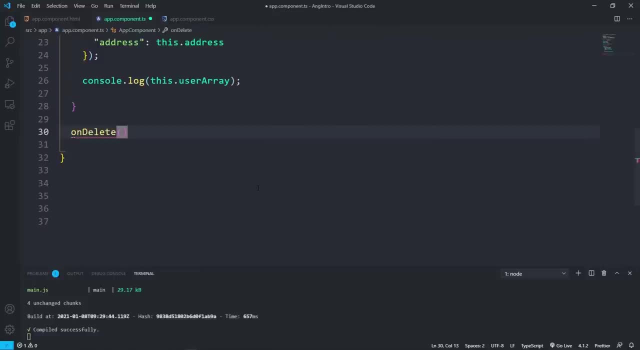 Now go to the componentts file and create this on delete method. Inside this, let's remove the data from the array. For that we use array slice method. So this dot user, array dot slice, After this parentheses. this required two parameters. 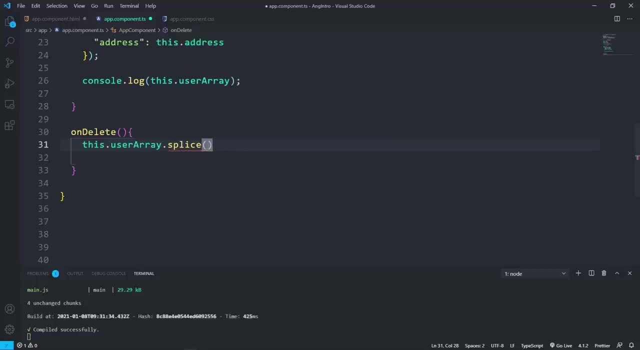 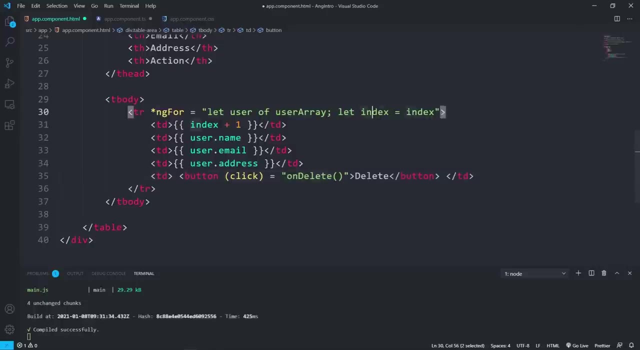 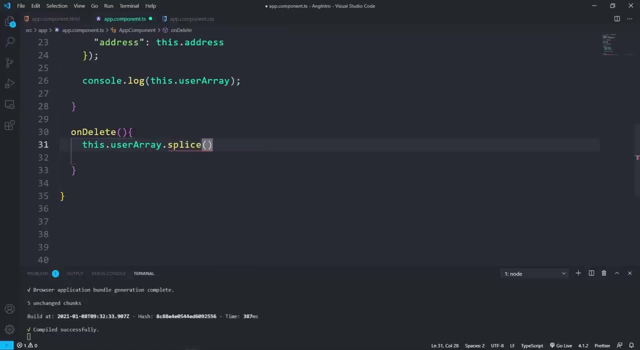 First one is the array index number. Let's pass the index number to this method from this click event binding. We are getting this. We are getting the index from this variable, So pass it here: Index, Alright. Next, let's capture that parameter from the method. 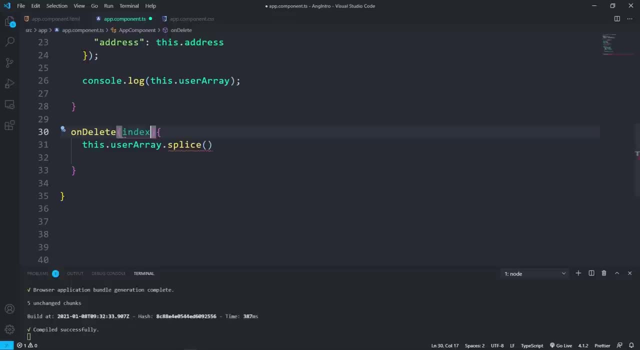 Create a parameter variable index. Now we have the index number with this parameter variable, So pass it to this slice method. After this, as a second parameter, pass number one. cause: we want to delete only one data from the array. That's it. 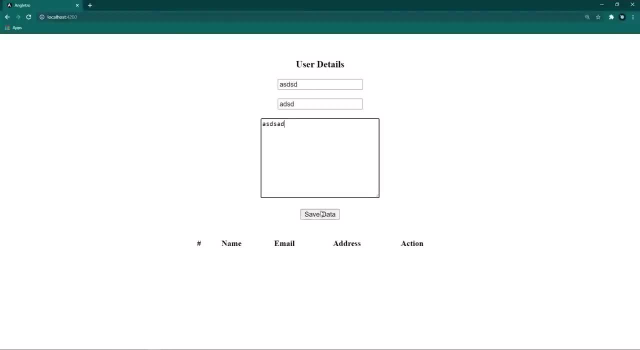 Alright, Back to the browser. Add new data. Now click this delete button. This will remove this data. Perfect, Everything working as we planned. At last, let's show a no data message when there is no data instead of showing this empty. 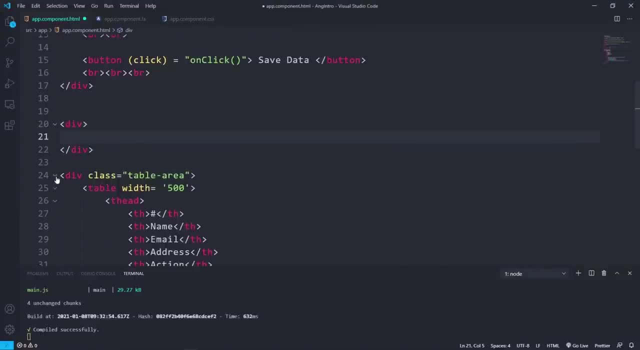 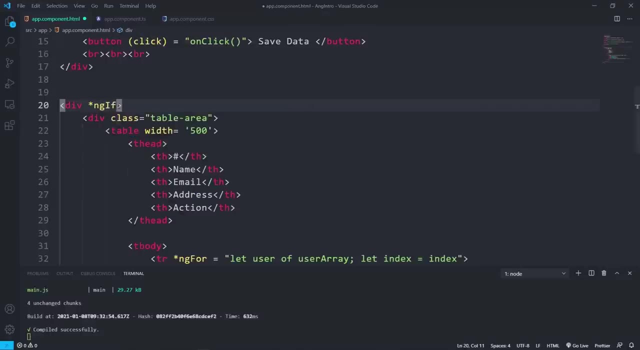 table. Back to the VS code. Let's create a div and put this table inside this div. Now let's add the ng if directive, Asterisk ng if div. So we have to create this. Well, we're using here an array to do this. 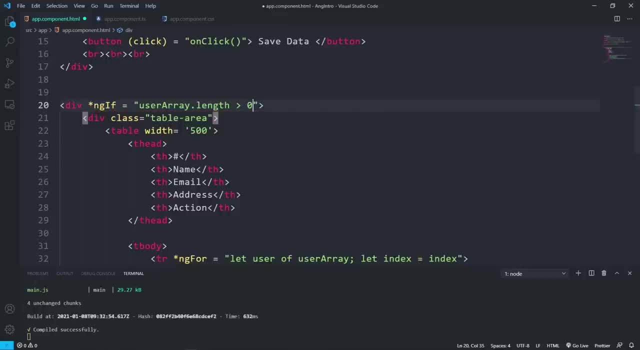 But the problem is- we learned about this earlier. UserArraylength greater than zero. If user array length is greater than zero, show this table. If not semicolon Else, show this ng template: no data. We are getting this error cause. still we don't have created this ng template. 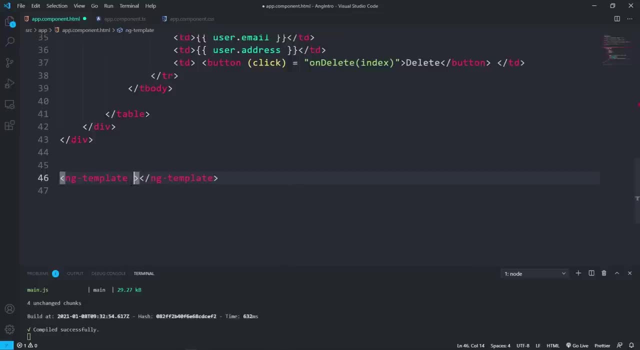 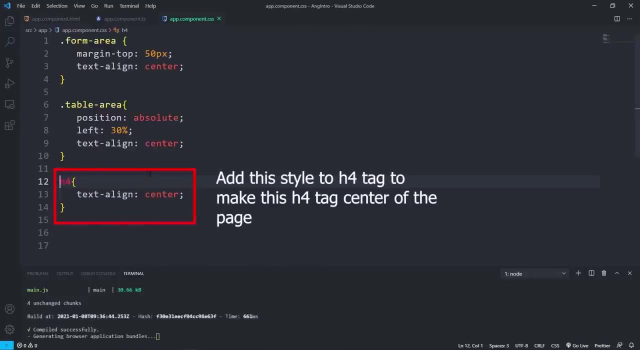 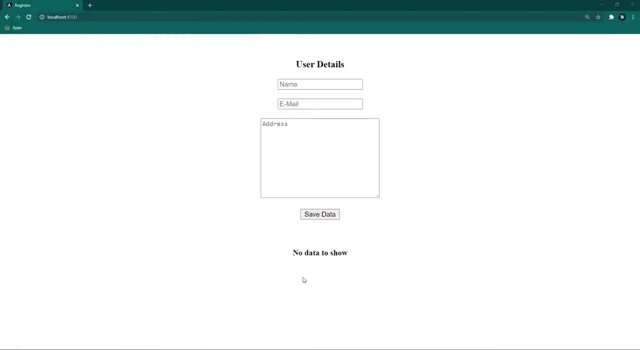 div. create the ng template. this template identification template variable. is this: no data hashtag. no data inside this. create h4 tag with this message: no data to show. save this and back to the browser. as you can see here, this time we got this message instead of the empty table: fill the form and click the save button. now the no data message is disappeared. 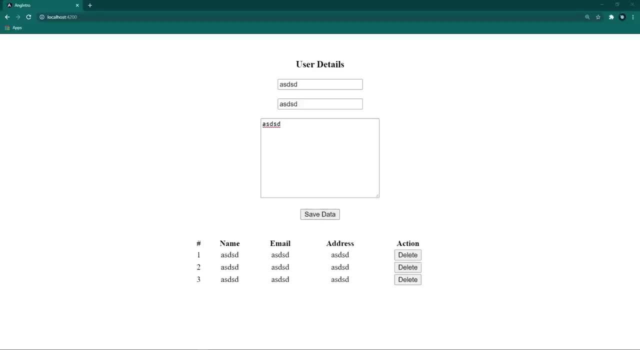 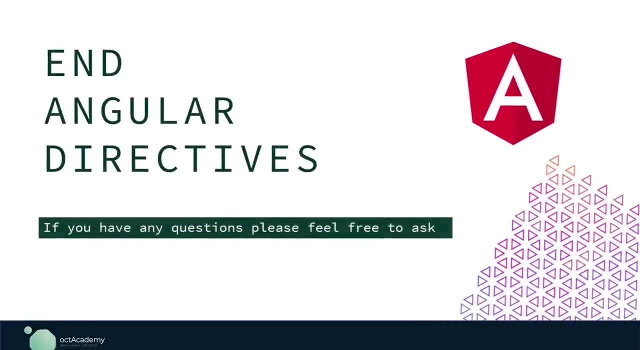 and now we can see this user table. beautiful, isn't it? so this is the end of this task. hope you guys understand this task well. all right, this is it for this section. in this section, we learned about angular inbuilt directives in detail. we learned about structural 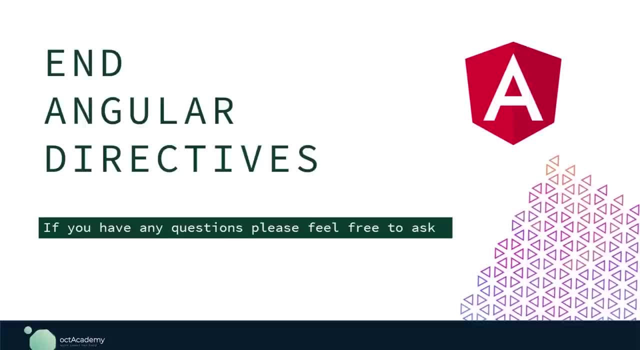 such as ng-for, ng-if, ng-switch cases. We learned about attribute directives, ng-class and ng-style. At last, we learned about what is difference between structural and attribute directives. So, guys, don't stop this from here If you guys have any problem with any. 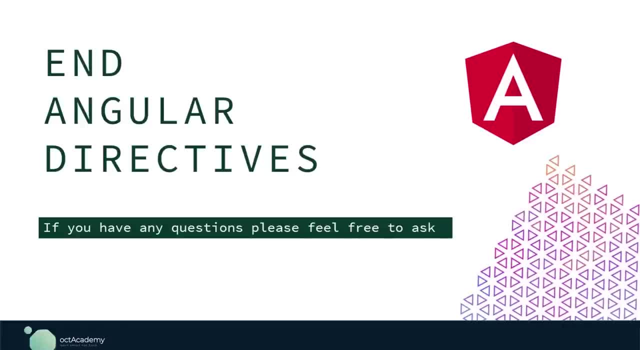 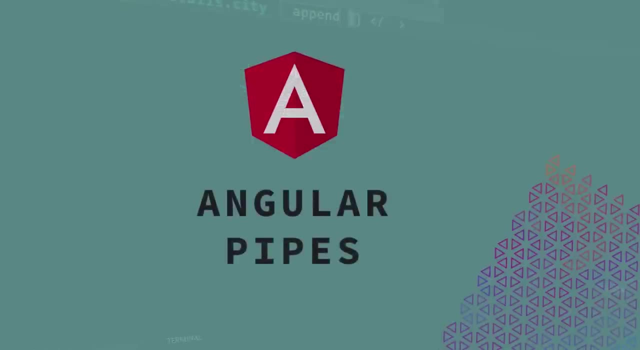 part of this section. try to learn it again. If you still don't get it, feel free to ask your question in the Q&A area. Alright, let's continue to the next section. In this section we gonna be looking at angular pipes and how to use them with our angular 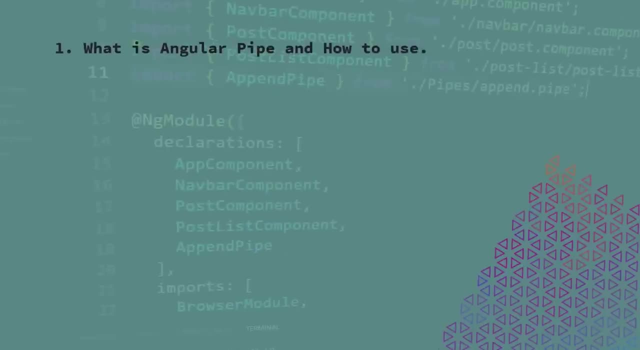 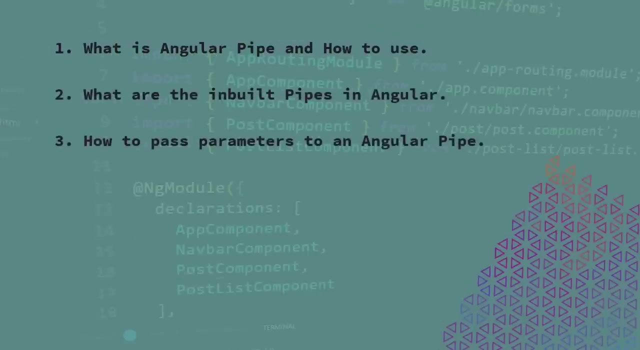 app. At the end of this section, you will know what is an angular pipe and how to use them. what are the inbuilt types of angular pipes, how to use parameters to an angular pipe. At last, you will learn how to create a custom pipe for 5 different requirements and how. 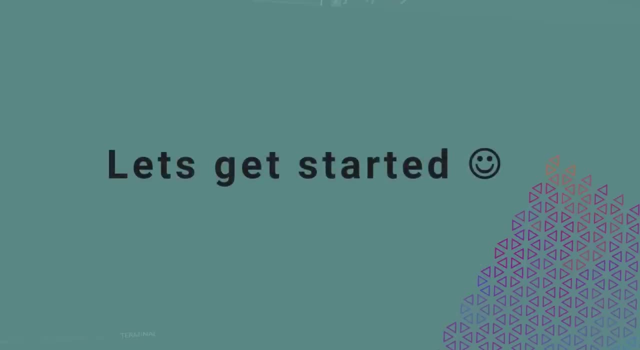 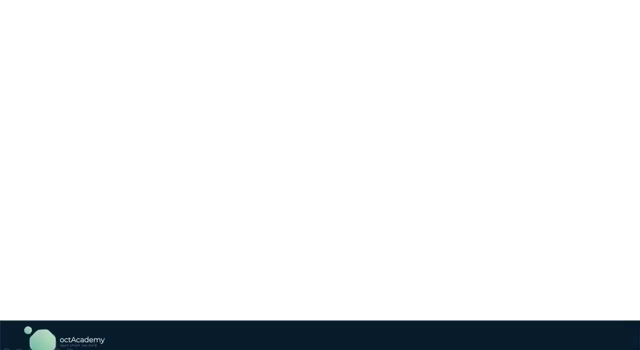 to use them from scratch. Let's get started. So what is angular pipe? Pipes are used to transforming data into a particular format when we only need that data transformed in a template or the HTML web, For example, think we have a something- total value of an invoice- 100,000- saved inside of a database When we 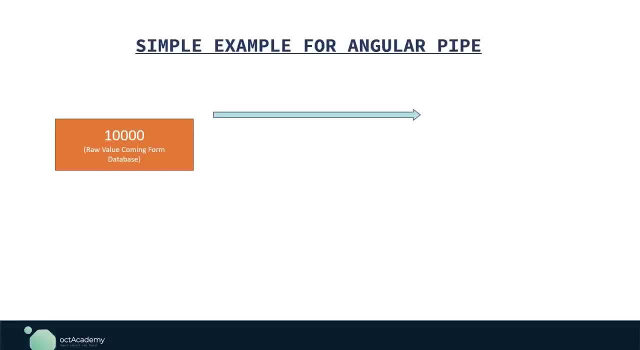 are showing this to the user. we can show this something like this with these comma separate using the angular number pipe And also we can display the currency symbol using the currency pipe. We will learn about this in detail with upcoming lectures. So in angular we have few inbuilt pipes which are uppercase and lowercase pipe, decimal. 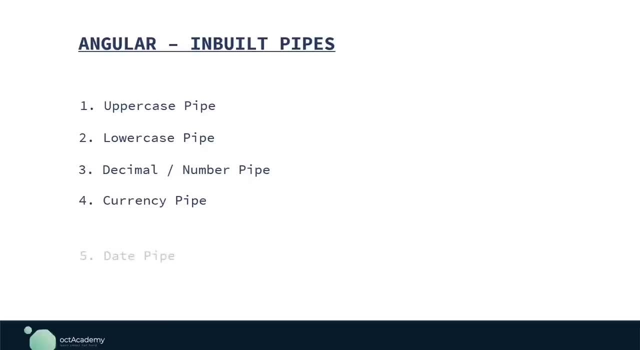 pipe or the number pipe, currency pipe, date pipe, decimal pipe or the currency number, JSON pipe, present pipe and slice pipe. So total we got 9 inbuilt pipes in angular. So from the next lectures we gonna learn these pipes one by one in detail. 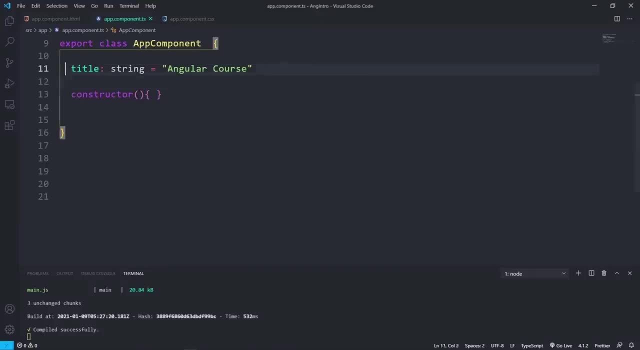 I have a variable inside the app component ts file title, which data type is string and value will be something angular course. Now I will render this variable inside the view using the string interpolation, So h1 tag inside these two curly brackets. inside these brackets, the variable name is: 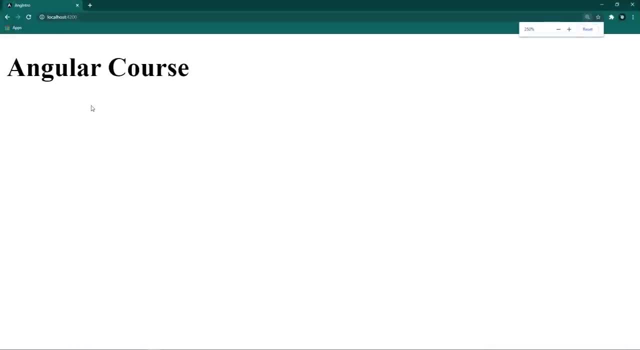 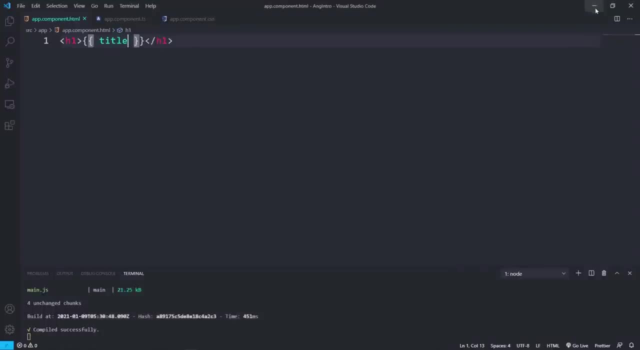 title: Save this and back to the browser. perfect, we got this title angular course. Now I want to make this all letters capital. how do we going to do that? We can simply do that using the css. Just go to the app component cs. 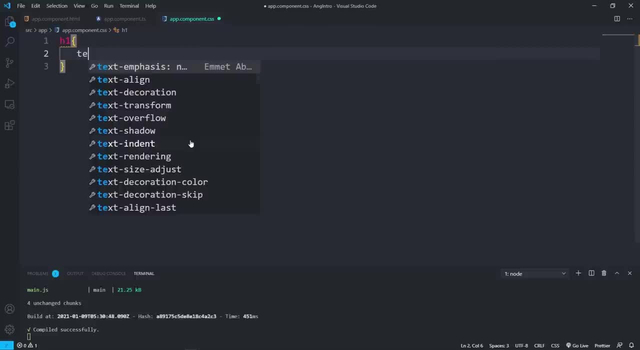 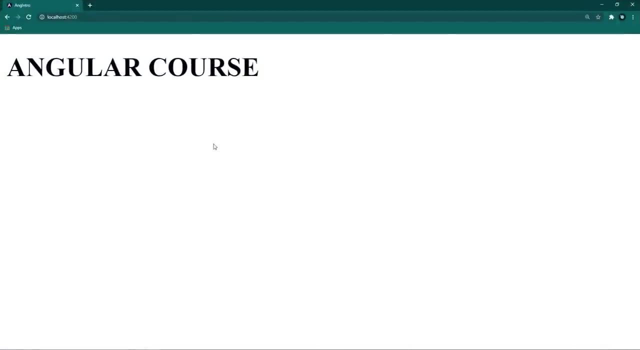 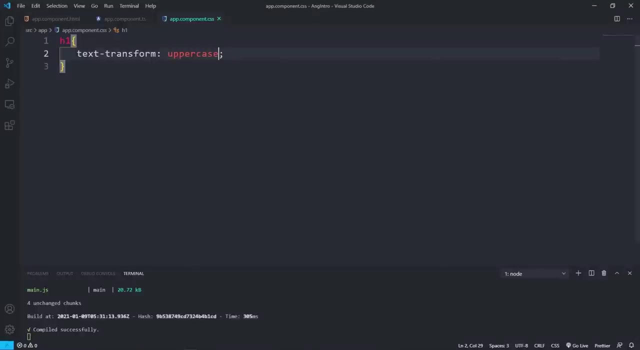 css file. css selector is h1, css property is text-transform, value is uppercase. Save this and back to the browser. as you can see here, Now this turned into uppercase letters, So we did this using the css. but now we have a better way for this in angular, which is: 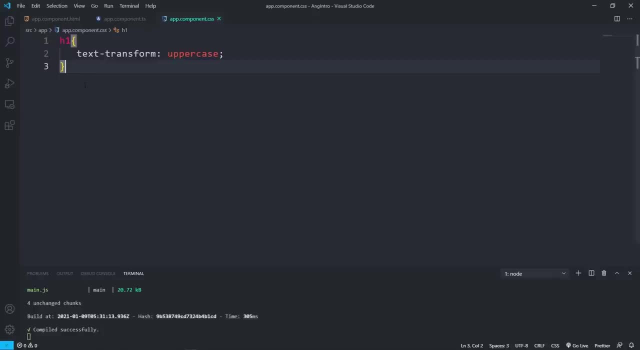 angular pipes, So we have different types of pipes for different types of data. The first one is the uppercase pipe, So this pipe will convert the letters to uppercase. Let's see how to do that Now. we don't need this css, so remove it back to the browser. 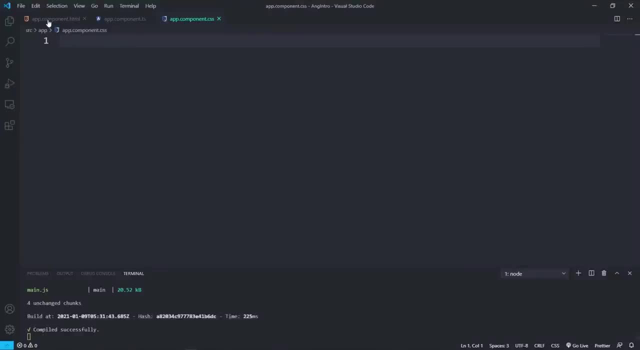 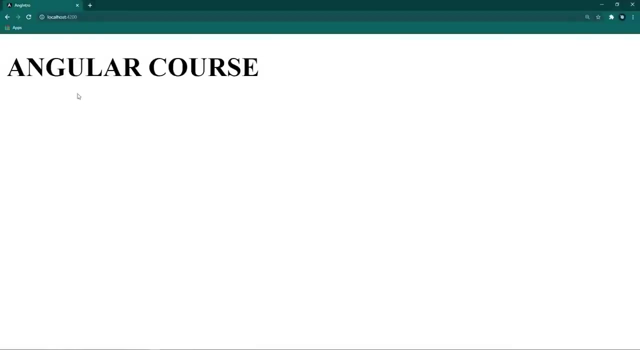 Now all set as previous. Let's add the uppercase pipe For this. first add this pipe operator. after this, inside this string interpolation Pipe operator, is this vertical line located before the keyboard enter key. Add the pipe name: uppercase, all simple letters. Save this and back to the browser. perfect. 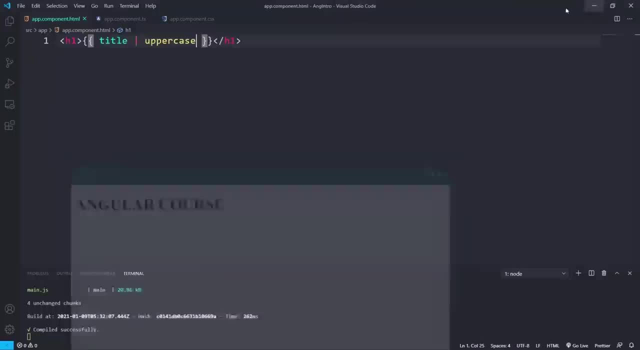 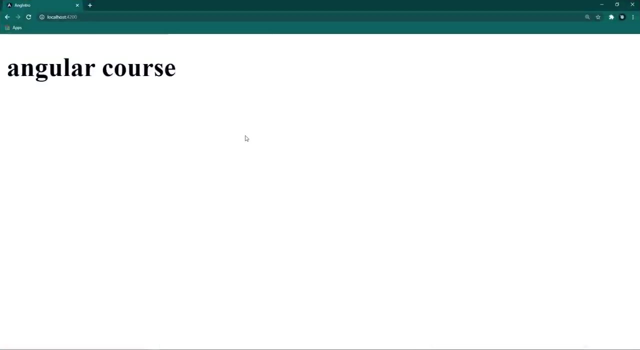 Now we got this all letters uppercase And also we can make this letters lowercase using the lowercase pipe. Remove this uppercase pipe and add lowercase. Save this and back to the browser. As you can see here, this time this is in lowercase letters. 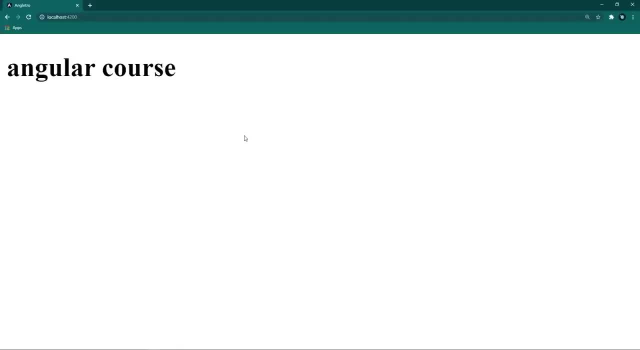 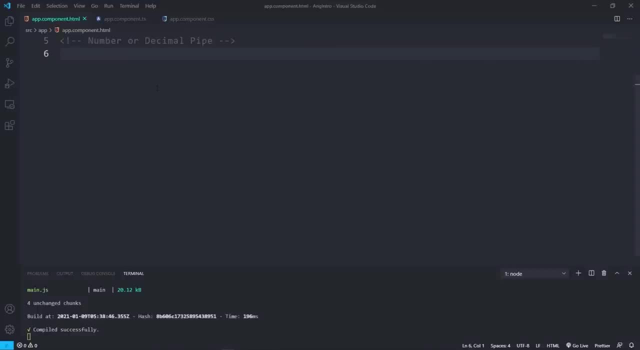 So this is the usage of angular uppercase and lowercase pipes. Alright, next we have the number of the decimal pipes. So let's see this in action. Let's declare a number value inside the component ts file. Something count and the type will be number. 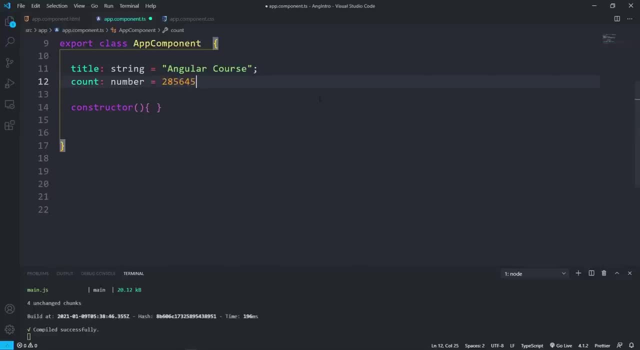 Assign this to a number value: 285645.. Save this. Now render this count value inside the weave using string interpolation. Another h1 tag Inside that two curly brackets Inside that variable name is count. Save this and back to the browser. 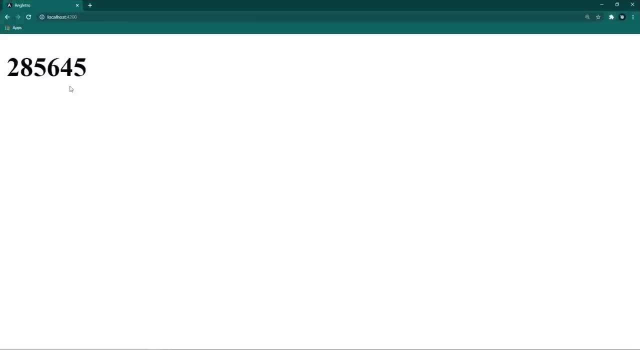 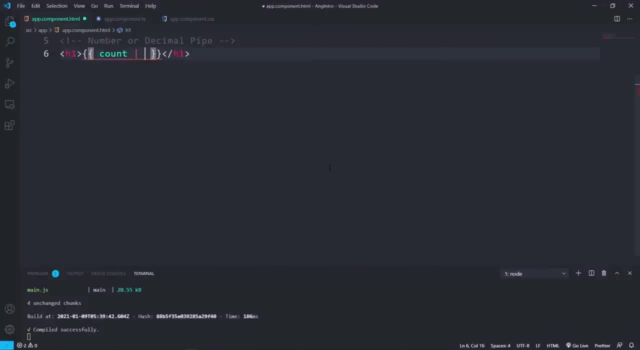 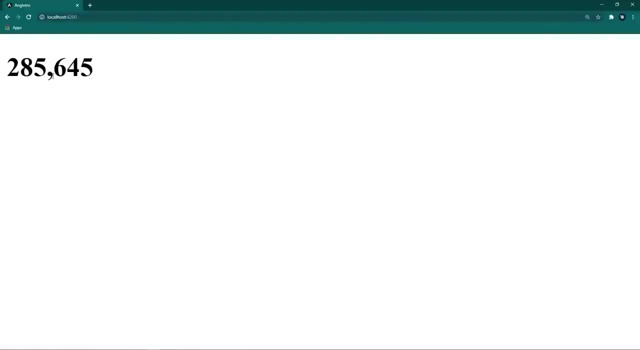 Perfect, we got this number. Now we can make this number value more readable using the number pipe. So back to the VS code and add the pipe symbol. Then the pipe name is number. Save this and back to the browser. Now this number is more readable with this comma symbol. 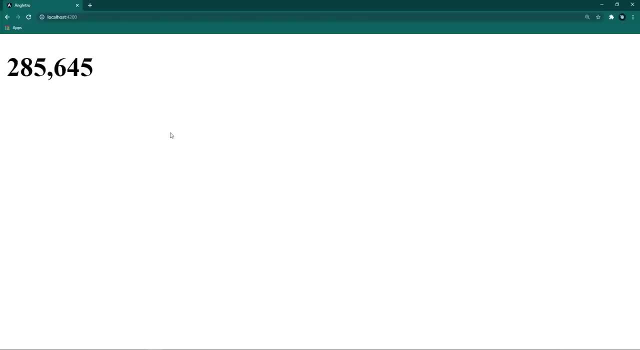 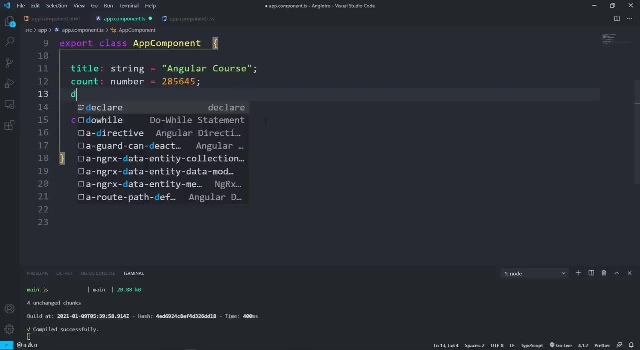 Which comes from the pipe number, So we can use this number pipe to decimal values as well. Let's declare a decimal value, Something dec, value Type will be number- And assign a decimal value- something- 3.85674.. Save this and back to the html file. 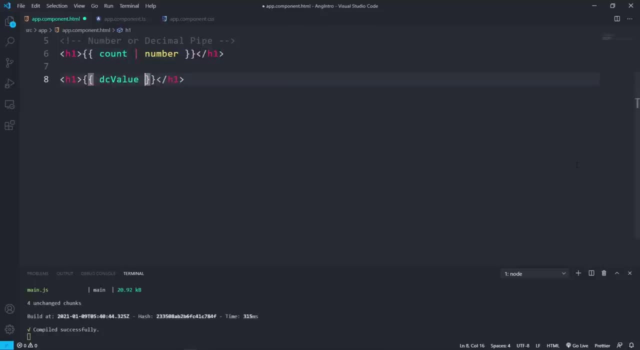 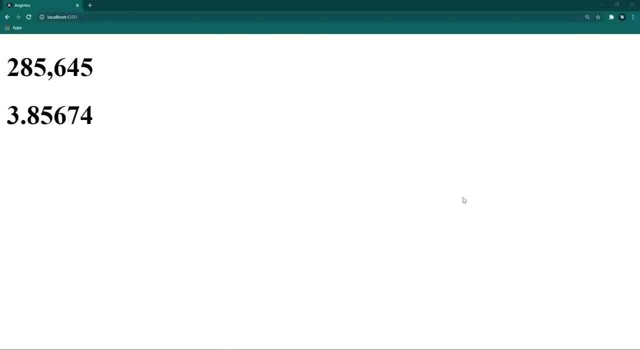 And load the decimal value here using the string interpolation. Save this and back to the browser. Perfect, we got this decimal value Alright in here. we have five digits of decimal values. Think if you want to reduce this to two decimal values. We have a solution for this. 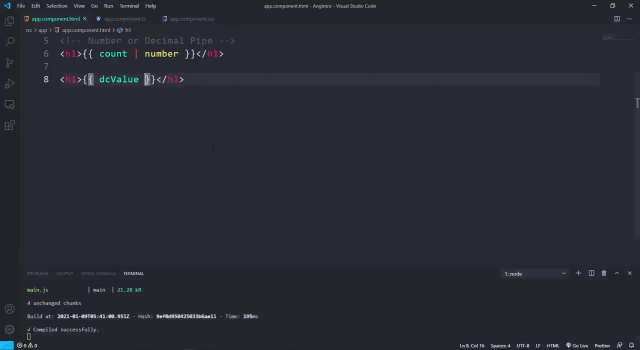 We can do that using the number pipe. So let's see how to do that. Back to the VS code. Inside this app component HTML file, Simply add the number pipe Pipe symbol and the number. Now we can pass an argument for this number pipe. 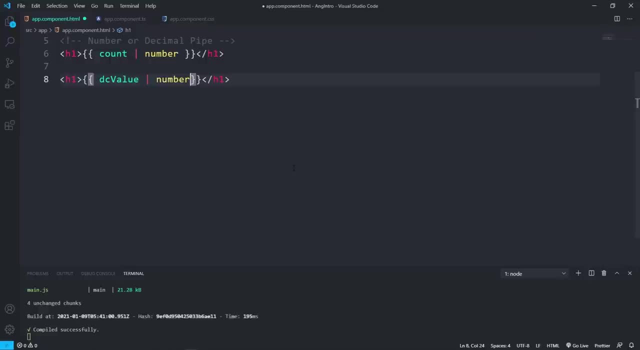 To control this integer value and for this decimal values. Let's see that Colon Now inside quotes. First we have to pass the integer value control. With this we can specify exactly how many integer number digits that we want. In our case we have one integer digit value here. 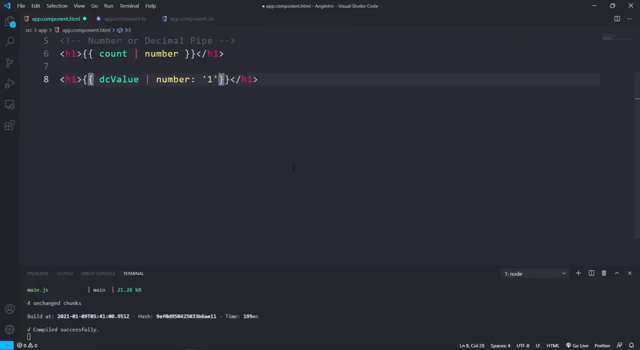 So put number 1.. After this we have the decimal digits control. With this We are separating the integer value and the decimal value, So now we have to pass the decimal digit control values. As I mentioned earlier, we want to reduce this five decimal digits to two digits. 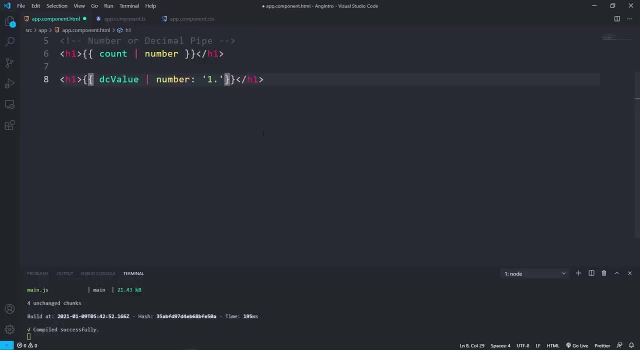 So now we have to mention minimum and maximum digits count after the decimal point. In our case, we needed only two digits, So pass, the minimum digit count is two. Then dash After this maximum decimal digits, it also two. Now save this and back to the browser. 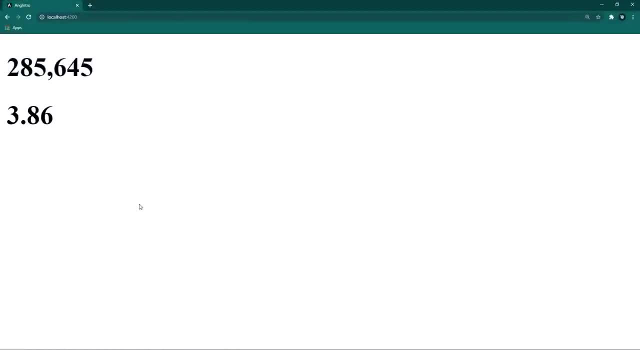 As you can see here, This decimal digits count reduce to two digits. Perfect right. So with the number pipe we can control digit numbers of this integer value as well as the decimal digits. If I add two for this integer digit count, Look at this: 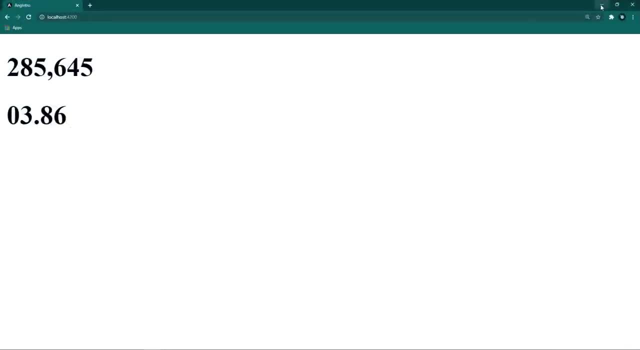 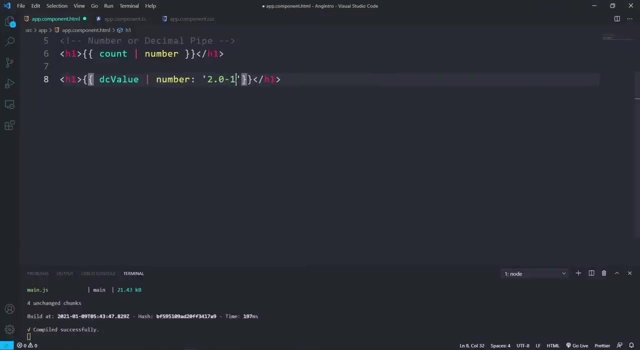 This added zero before this integer value To make this digits count two. And also, if I make this decimal digits count to one, Look at this: This is rounded this three point eight to three point nine, If I make this decimal digits count to zero. 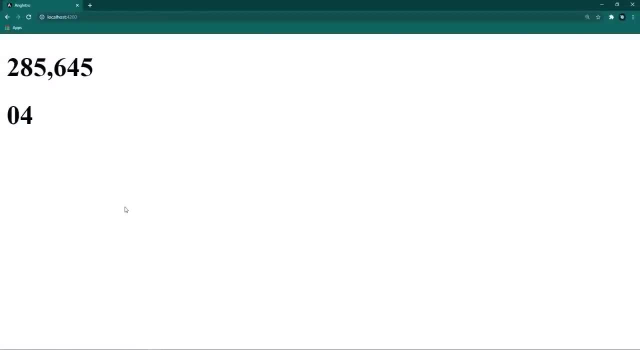 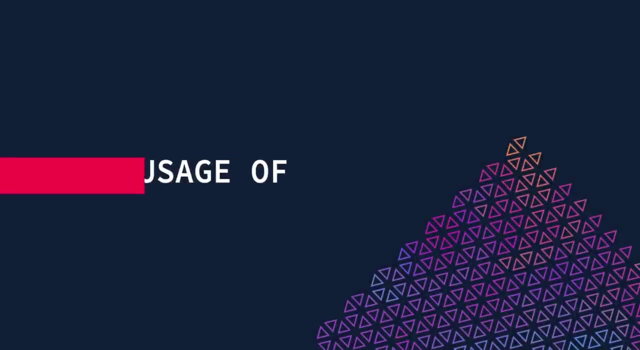 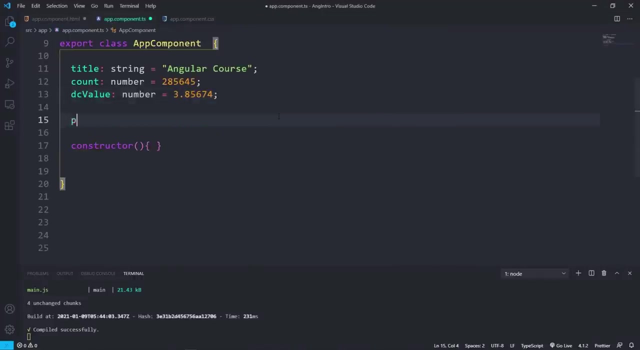 Look at this. This number is now rounded to the nearest integer value, number four. Beautiful right. So this is how we use the number or the decimal pipe in angular. Next, let's look at the currency pipe. All right, Just create a price variable and assign a value, something. ninety nine point nine nine. 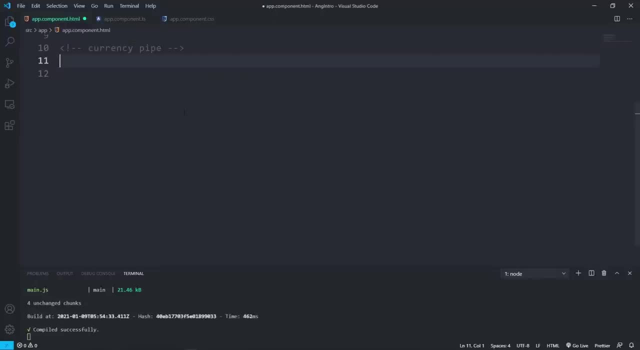 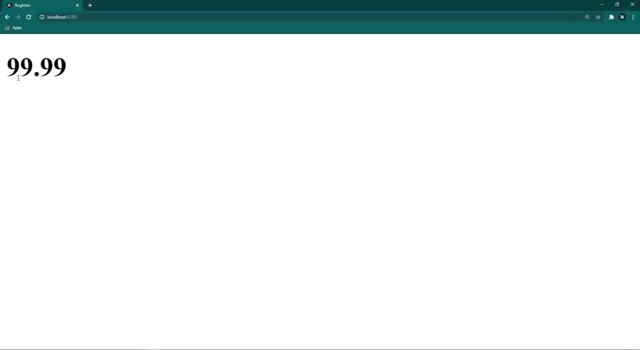 Save this and go to the html view and add this: another h1 tag Inside this. place this string interpolation to show this price value. Save this and back to the browser. We got this price. Now we can add the currency symbol for this using the currency pipe. 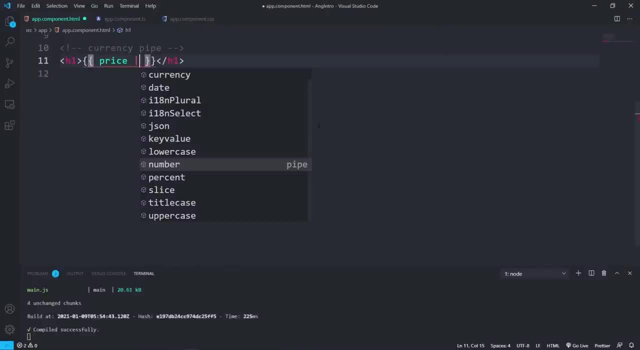 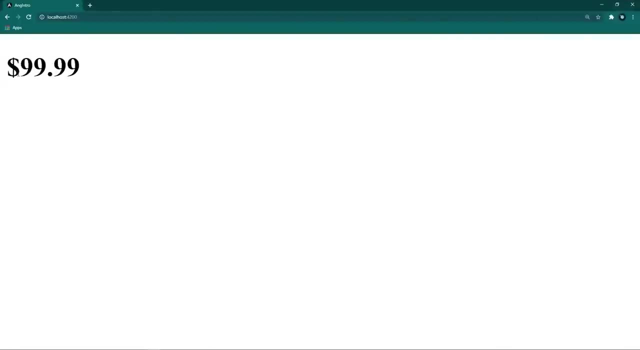 Back to the vs code. Add the currency pipe after this Pipe symbol and the pipe name is currency. Save this and back to the browser. Look at this. We got this US dollar symbol before this price. Perfect, right By default in angular. we got this US dollar symbol. 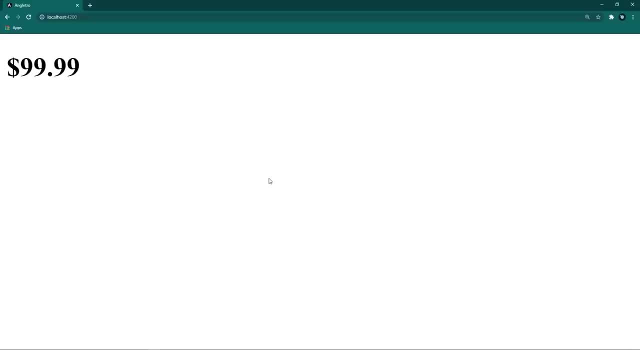 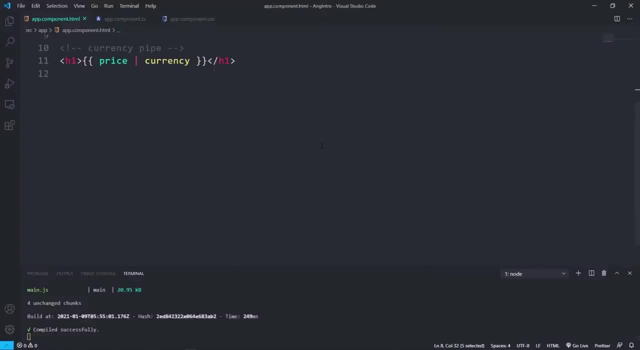 But if think, If we want something else, For example Canadian dollars, How do we going to do that? Very simple, Like this number pipe. we can pass an argument for this currency pipe to define the currency type. After this colon, Then inside quotes, define the currency type that we want. 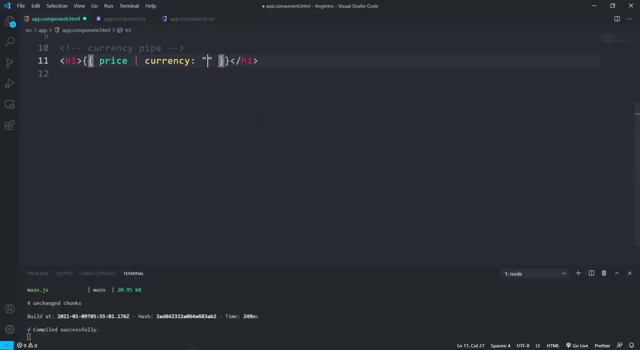 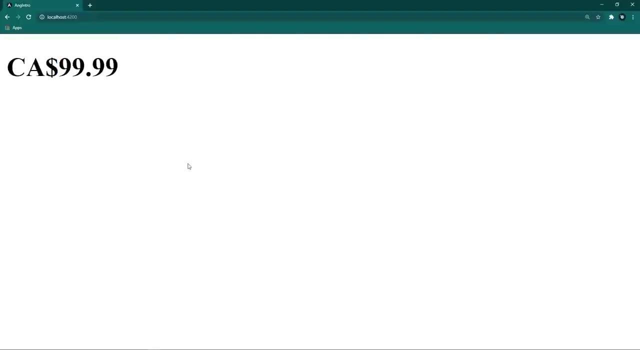 In our case, we want to show Canadian dollars In here. we have to pass the currency code, So the Canadian dollar currency code is CAD. All capital. Save this and back to the browser. As you can see here, Now we got this Canadian dollar symbol. 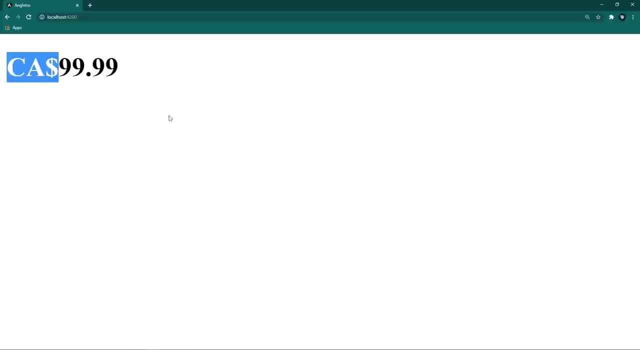 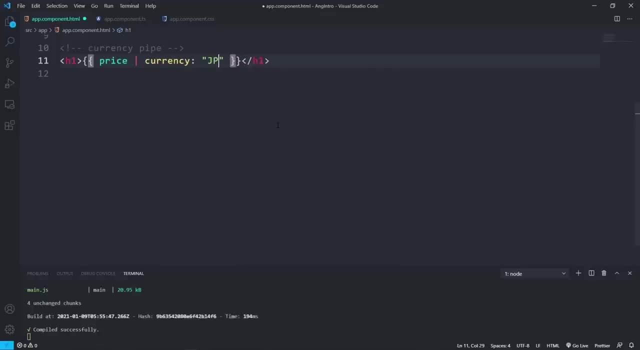 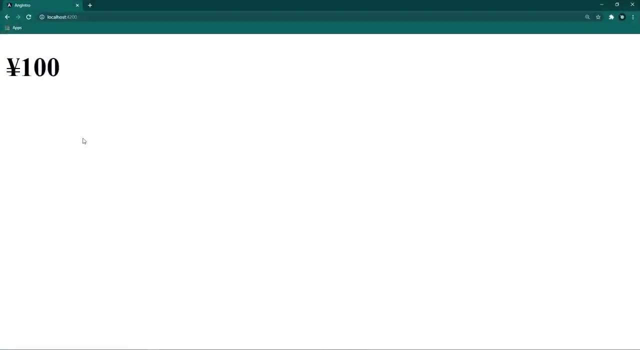 Let's look at another example. If we want to define Japanese yen currency, For that we have to pass here the Japanese currency code, JPY. Save this and back to the browser. Awesome right, We got this Japanese yen currency symbol In case, if you wondering how to get the currency code. 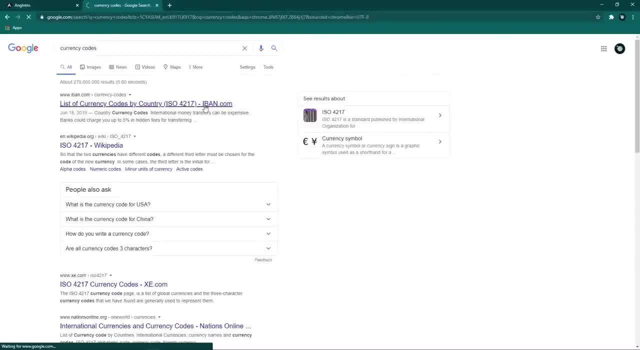 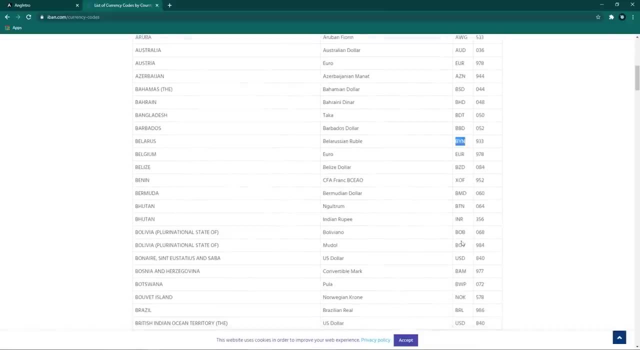 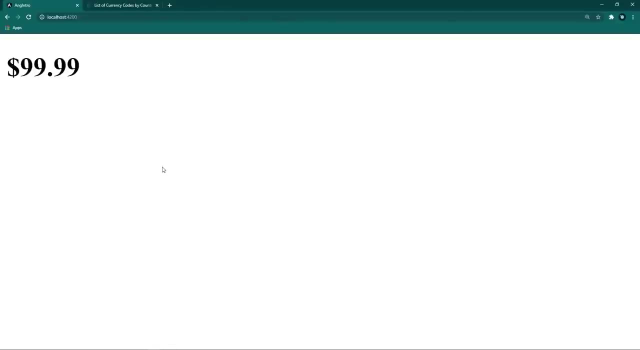 Just google it currency codes. In the first result, You guys will get all the currency codes in the world. All right, Back to the work. Reset this to USD, Save this and back to the browser. We got this dollar sign, Okay, in any case, if we want to show the currency code instead of this currency symbol, 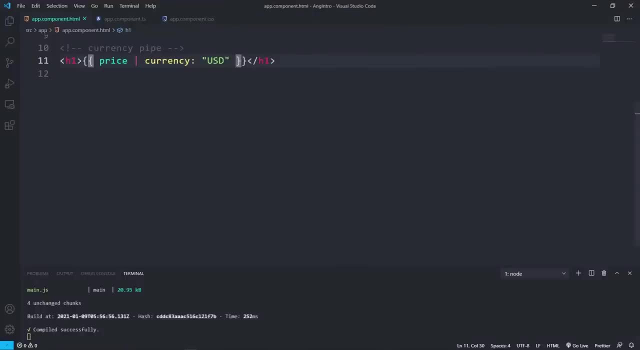 How to do that? Very simple. Pass another argument here. This is going to be a Boolean value, True or false. If we pass true, This will show the currency symbol. If we pass false, this will show the currency code. So in our case, 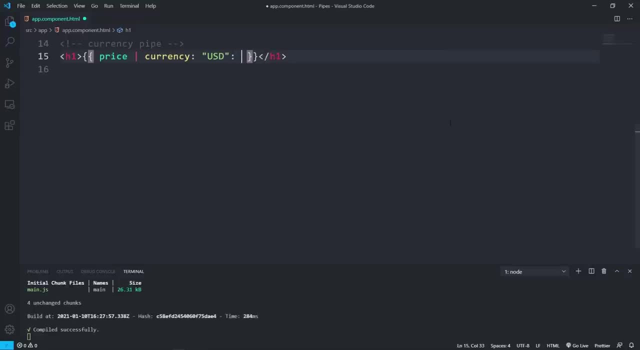 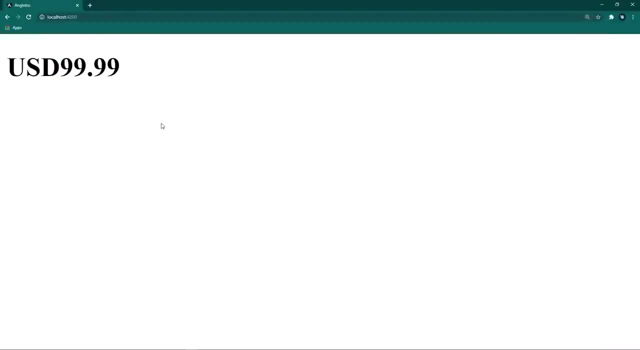 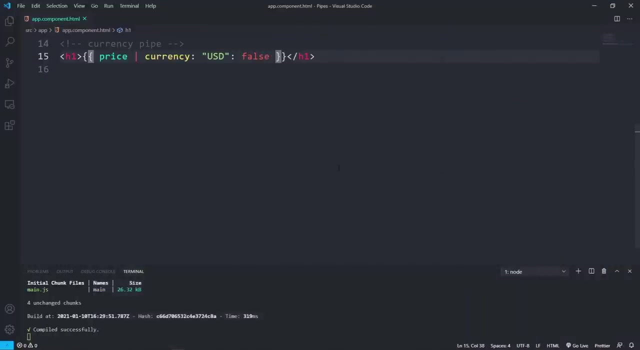 We are planning to show the currency code, So pass false here. Save this and back to the browser. Perfect, Now we got this USD currency code Instead of the previous currency symbol. Save this symbol and also, like number pipe, we can control the digits counts. just simply pass another. 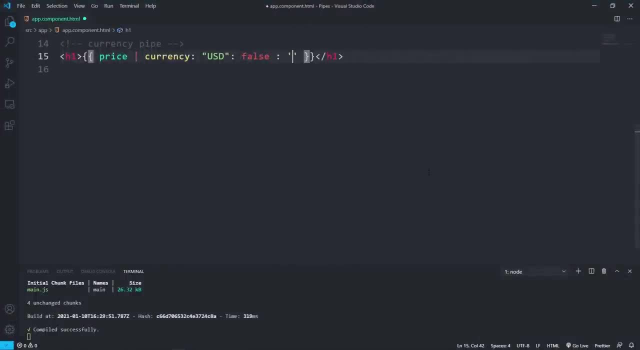 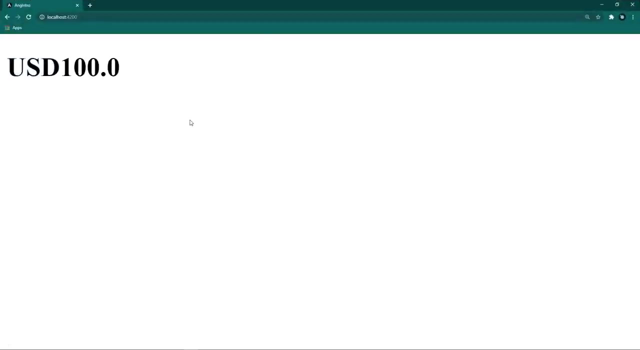 argument inside quotes. as a first value, we can pass the integer digits count. we have two digits, so i pass two digits for decimals. i will add the minimum and maximum digits count as one. save this and back to the browser. perfect now this price is rounded to the nearest value, 100, and this decimal. 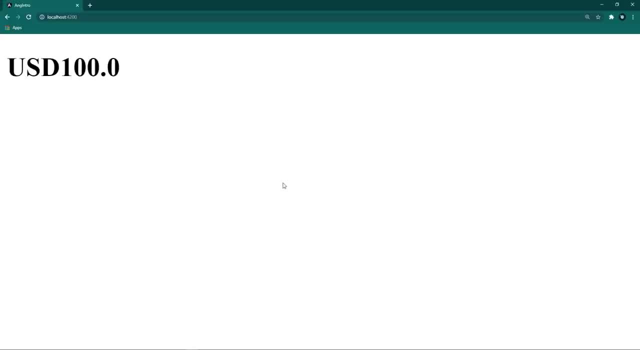 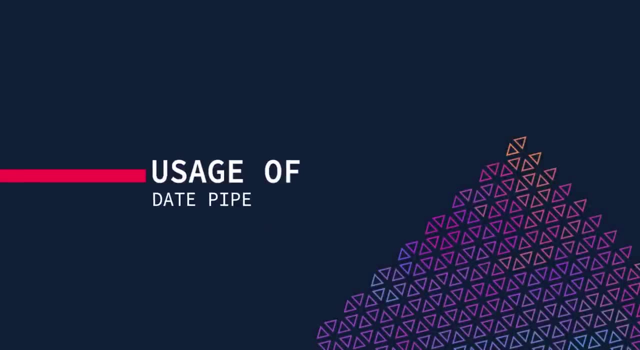 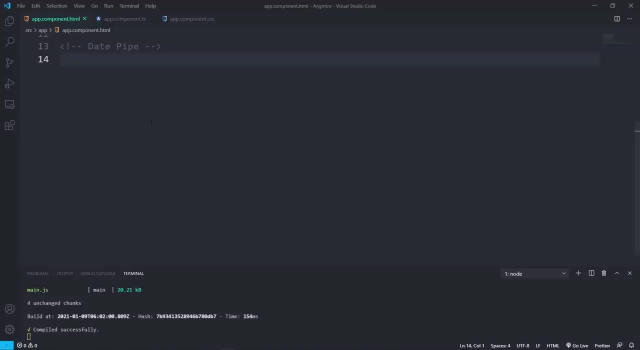 digit count is set to one digit. so this is how we deal with currency pipe in angular- all right. next we have the date pipe. let's see this in action. create a date variable and assign a date value. the variable name is today, data type is date. this d is capital. assign this to new date object. 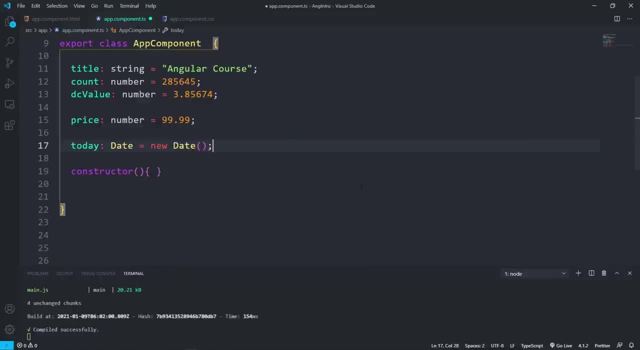 new date and the parentheses. this will give us the current time and date. this is not a typescript or angular thing. this is just a simple plain javascript date object. okay, back to the html file and load this inside of an h1 tag using the string interpolation method. save this and back to the browser. 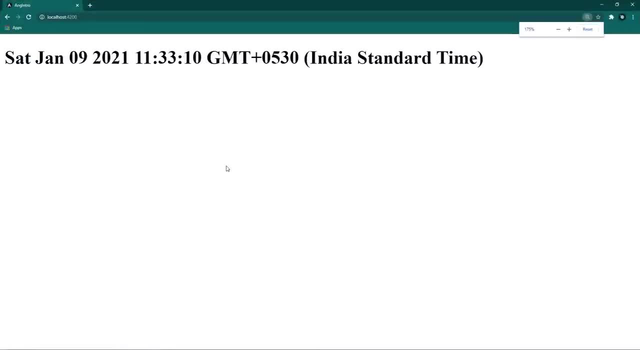 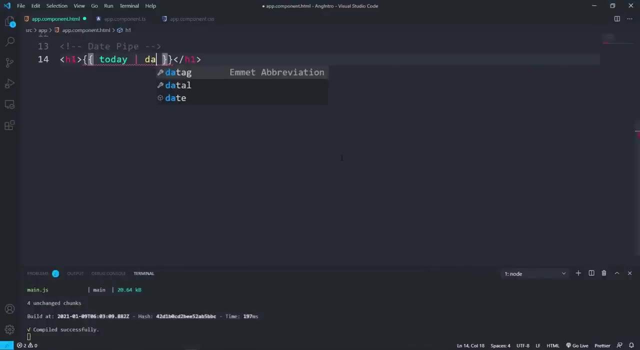 as you can see here we got this date and time value. this date value is not clearly human readable, so we can make this more readable using the date pipe. so back in the vs code: pipe symbol and the pipe name is date. after this we have to pass an argument inside quotes. 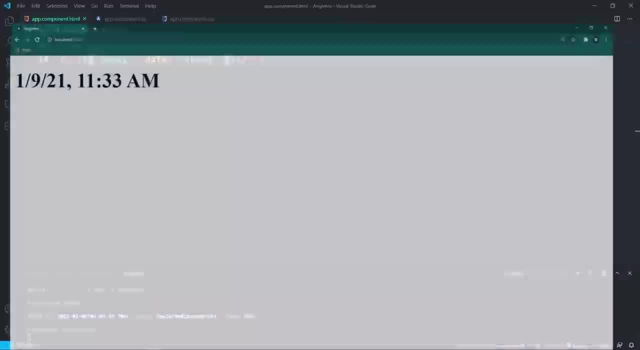 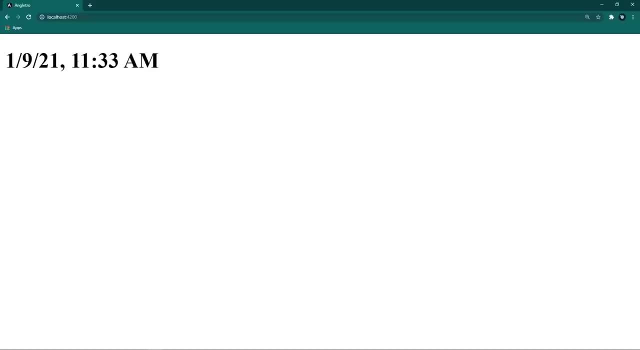 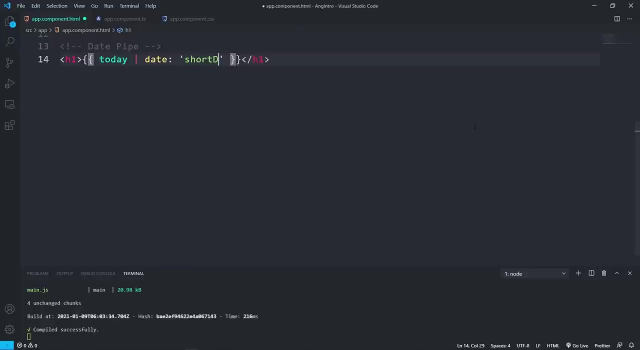 short, save this and back to the browser. awesome, right now we got this readable and date and time think. if you want only the date, not the time, we can do that simply by passing the short date argument for this. save this and again back to the browser. beautiful, right. 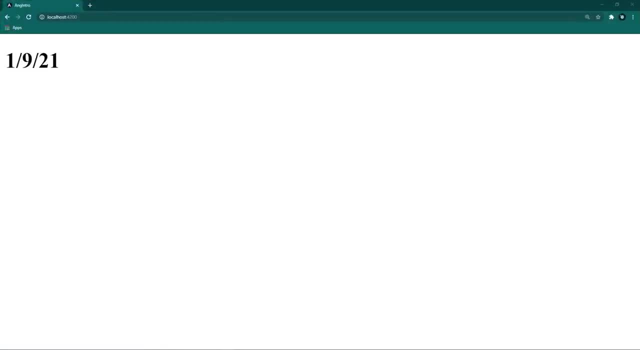 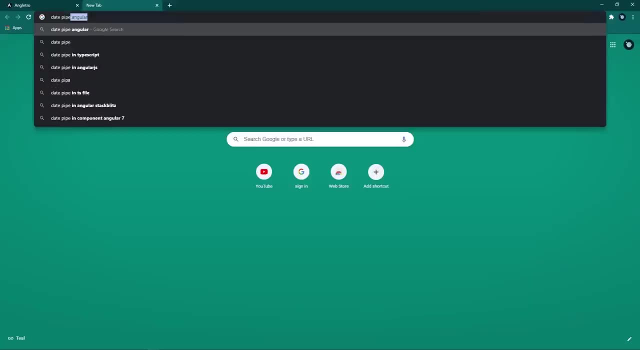 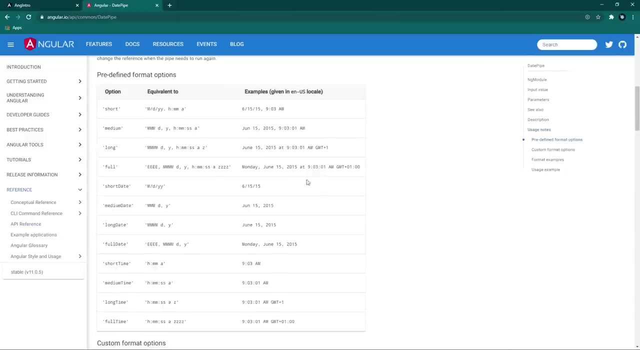 this time we got this date without the time, so If you may wonder where to get these arguments for this date pipe, So just simply search for date pipe- angular. With this first result, which is the angular official website, we can find all the arguments. 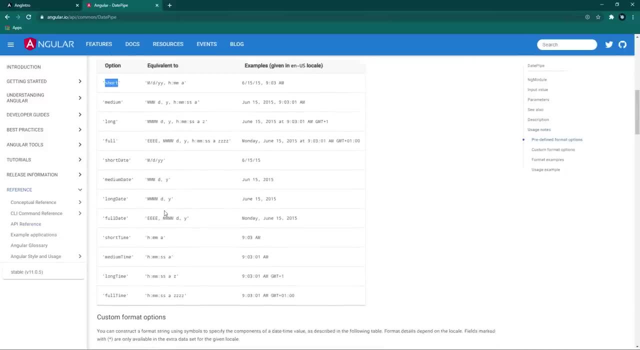 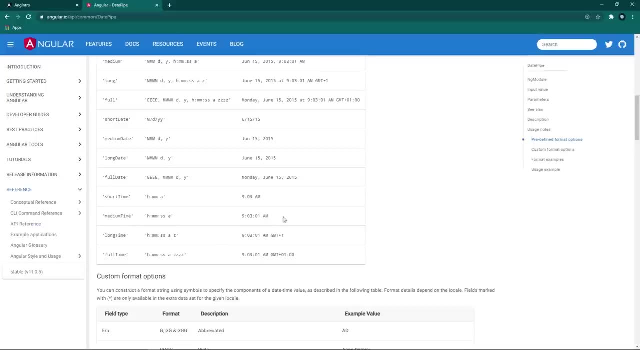 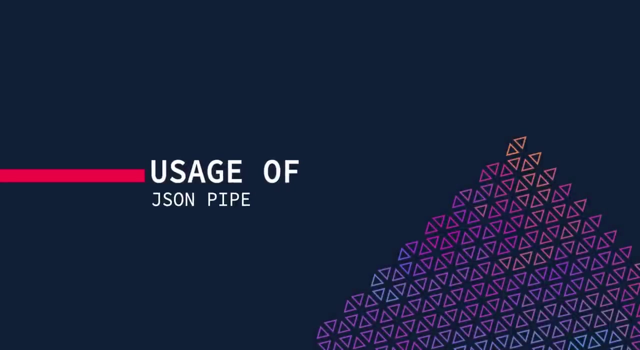 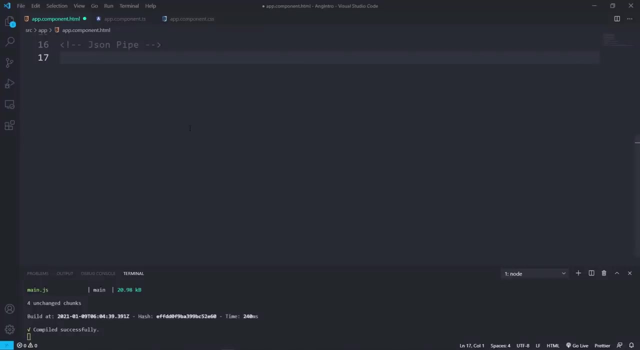 for this date pipe. If we need only the time without the date, we can use one of these time arguments. So this is how we use date pipe in angular. Hope you guys got the idea right Alright, in this lecture. let's look at another angular pipe, the JSON pipe. 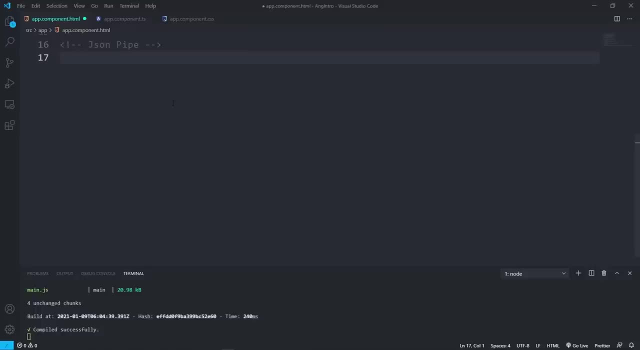 We use this JSON pipe to show an object inside of a V. Let's see this in action. First let's create a simple object inside the component TS file. Object variable is something post object and assign this to simple object inside curly brackets. First, key value pair is ID and the value is one. 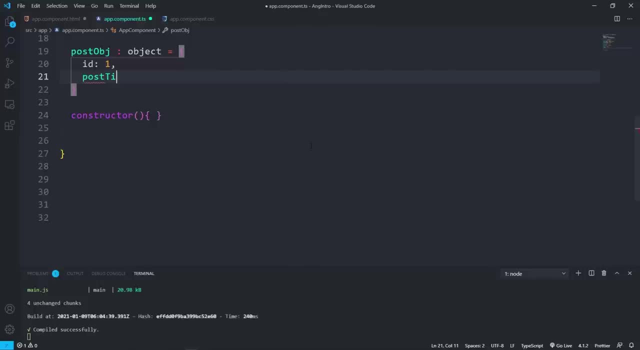 Next, the key is post title and value is post one. Save this Now back to the HTML file and let's show the object inside the browser using the string interpolation. So create a P tag inside this string interpolation. Object variable name is post object. 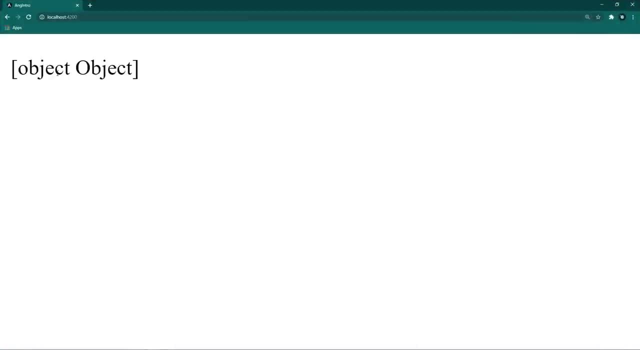 Save this and back to the browser. Look at this. We got this object object printed here instead of the object key value pairs. So inside of the browser view we cannot show an object directly. In order to show this inside the browser, we have to convert this object to a string. 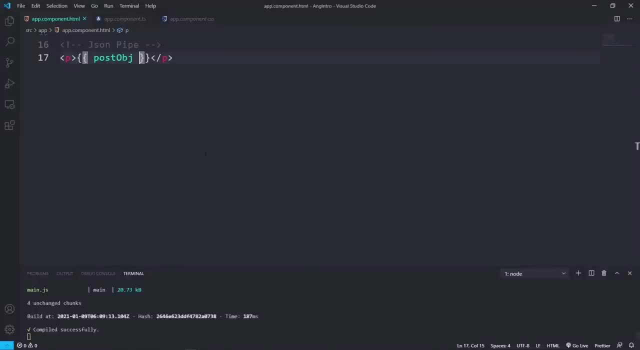 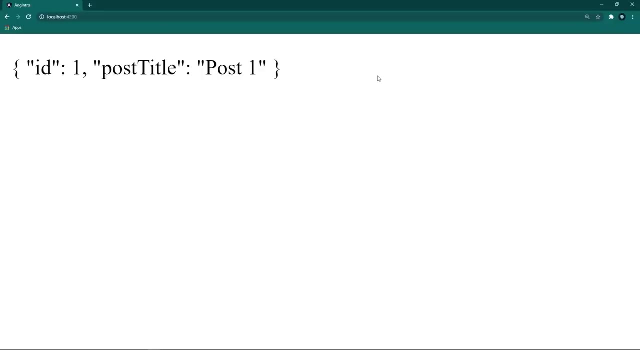 JSON format data. For that we can use JSON pipe. So let's do that Pipe operator And the pipe name is JSON. Save this and back to the browser. As you can see here, this time we got this object values printed here instead of the. 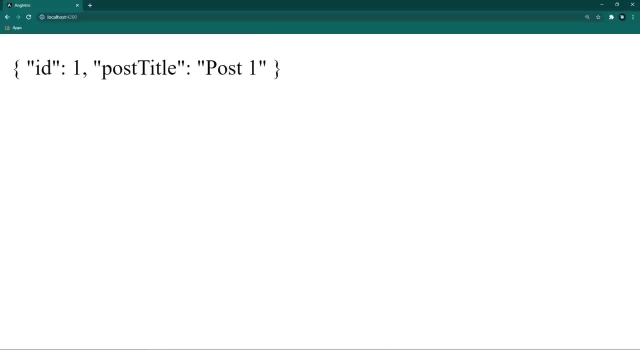 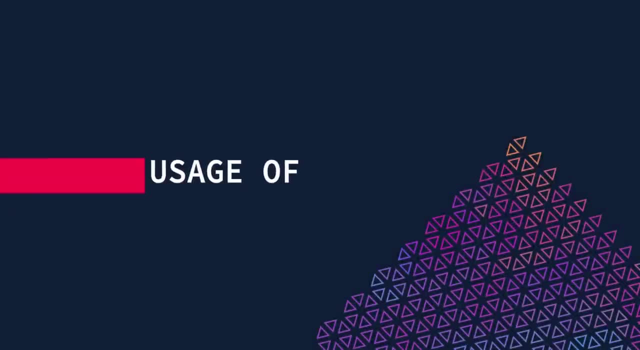 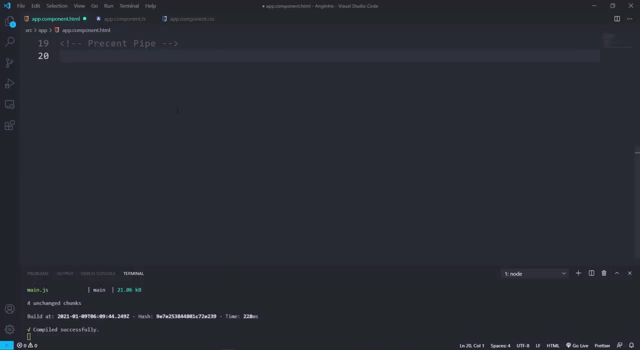 previous object object. So this is the usage of this JSON pipe. Next we have the percentage pipe. With this we can show a percentage string. Let's see this in action. Inside of an h3 tag, add a string, interpolation type, a decimal number, something 0.567, and add. 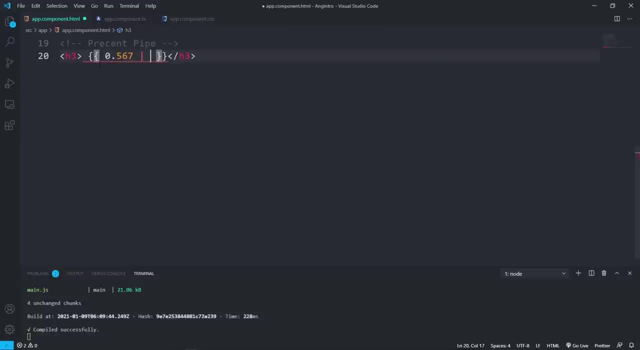 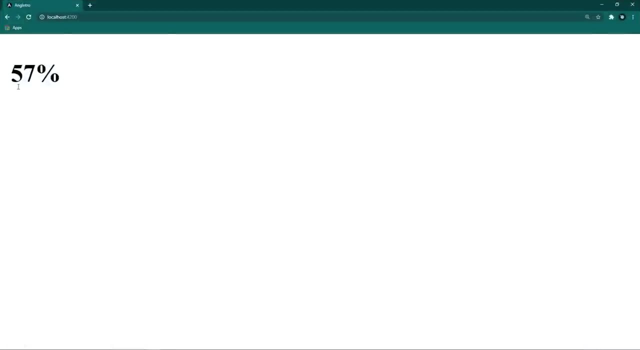 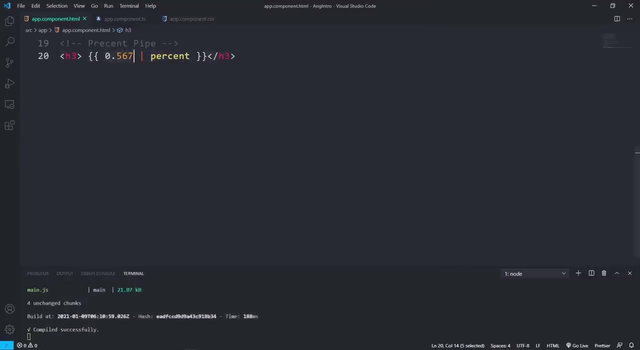 the present pipe. So pipe operator and the pipe name is present. Save this and back to the browser. As you can see, here we got this 57 percentage. So this present pipe will multiply this given value in 100. And give us the percentage value. 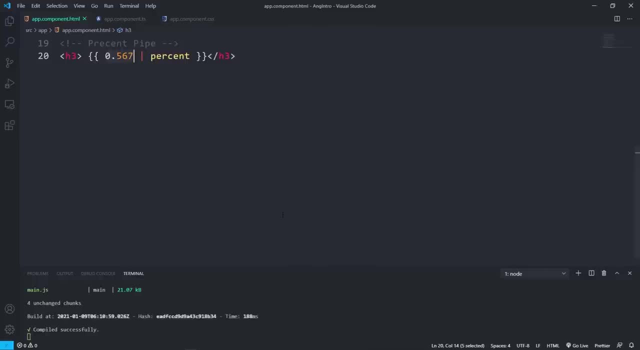 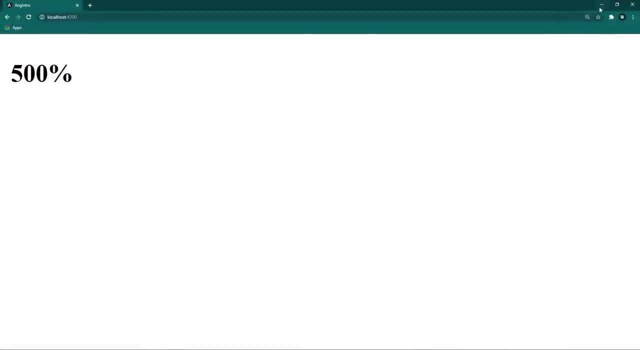 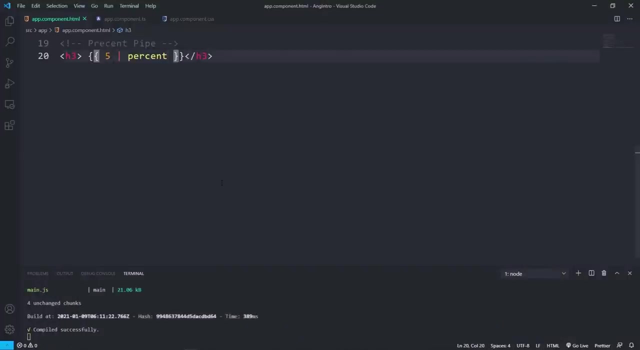 If I change this to the integer value 5,, as you can see here we got 500 percentage, Cause this present pipe is multiplied this given value in 100. That's why we are getting this value. This also has format string, like decimal pipes. 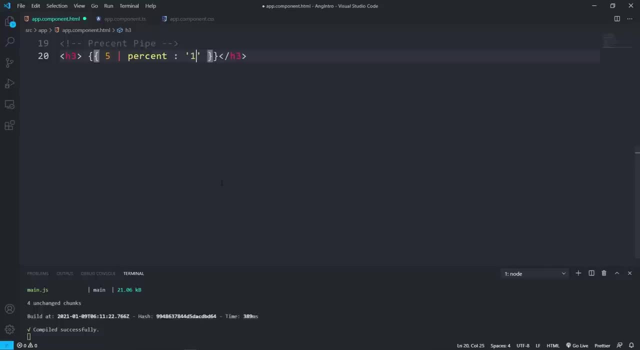 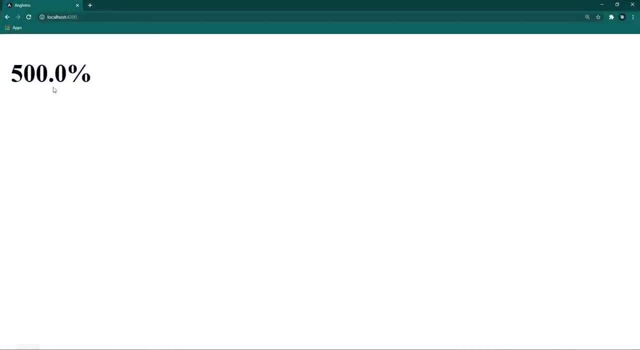 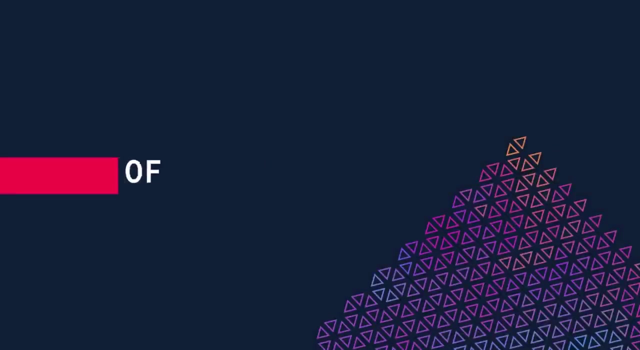 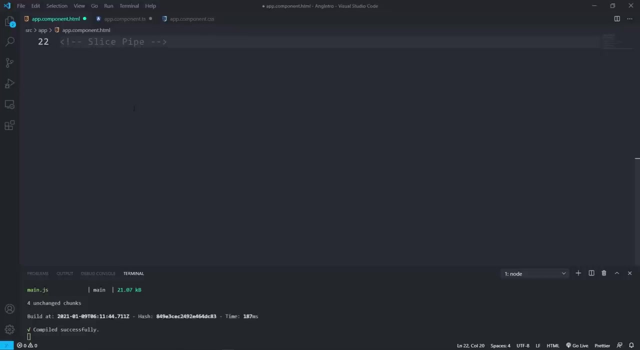 We can control the digit counts- decimal digits- and the integer digits- like this. So this is how we use the present pipe. Next we have the slice pipe, So with this we can slice an array. Let's see this in action. Create a simple array inside the componentts file. 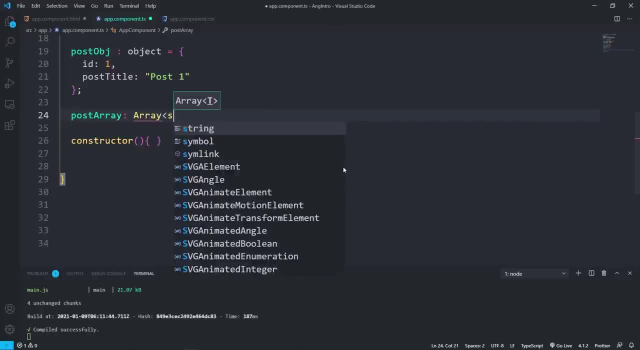 Post array. The array type is a string. Now assign a simple array to this Inside square bracket: Post 1.. Put this inside quotes cause: this array type is a string: Post 2. Post 3. Post 4. Post 5.. 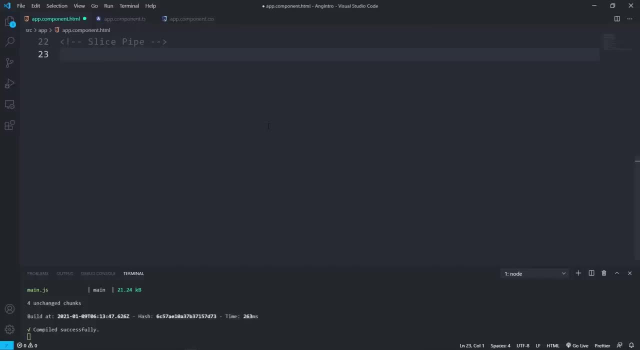 And so on. Save this and back to the componenthtml file. Now let's show this array inside the browser using the string interpolation Inside of an ht tag, String interpolation Array. variable name is post array. Now save this and back to the browser. 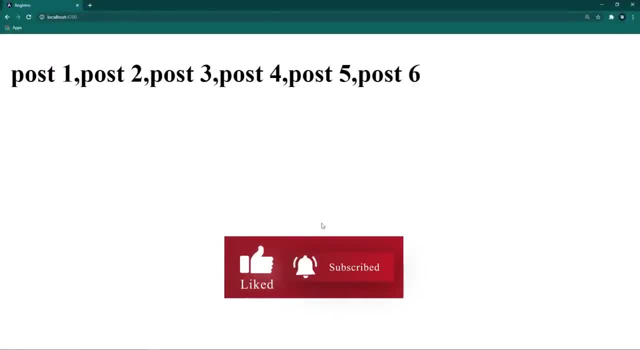 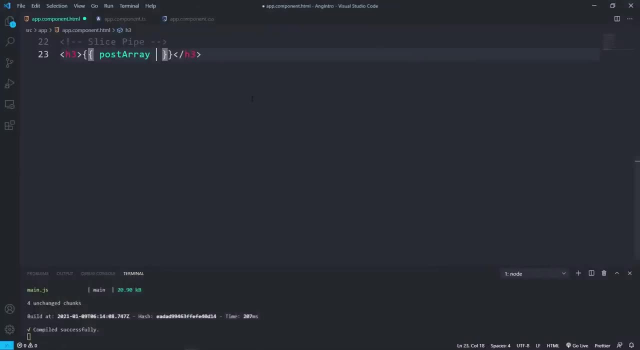 As you can see here, we got this array values printed here. Now think, if we want to show only this first three values of this array inside the browser, How do we going to do that? For this we can use the angular slice pipe Back to the evs code. 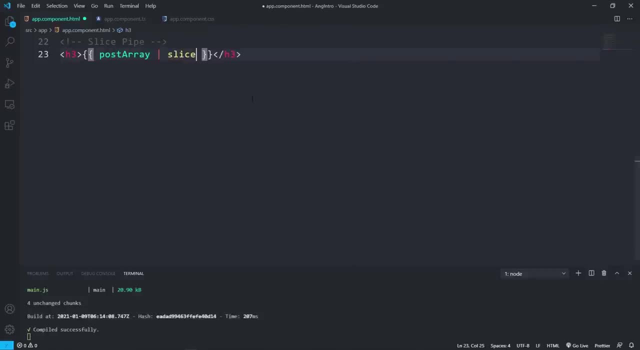 After this pipe operator and the pipe name is slice, Now we have to pass the start index and the end index That we want to slice. So now I want to show these first three values. So the start index is 0.. And this end index is 3.. 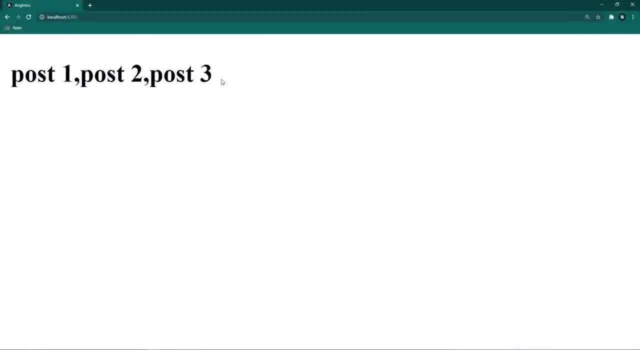 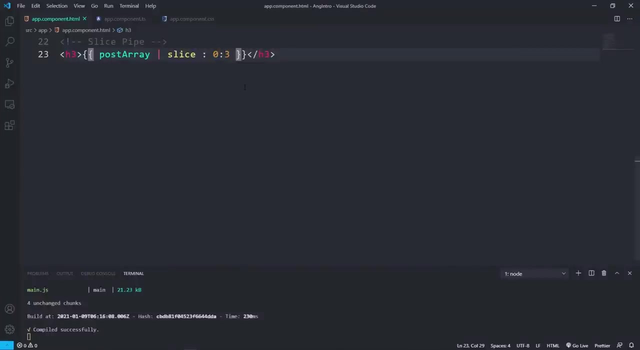 Save this and back to the browser. Beautiful. This time we only got this first three values from the array. Think if I want to show these middle two values, Post 3 and post 4.. For that change these index values. This time the start index is 2.. 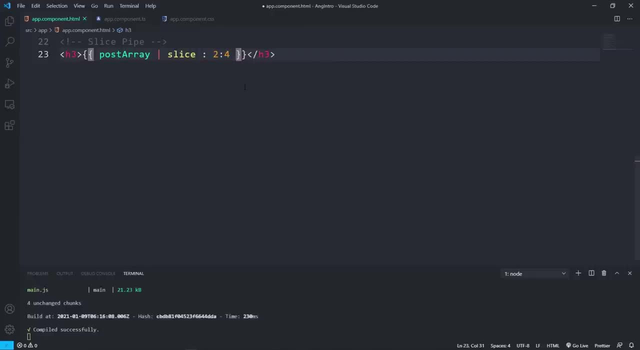 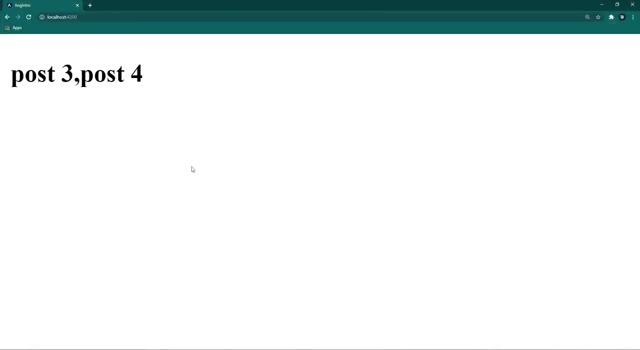 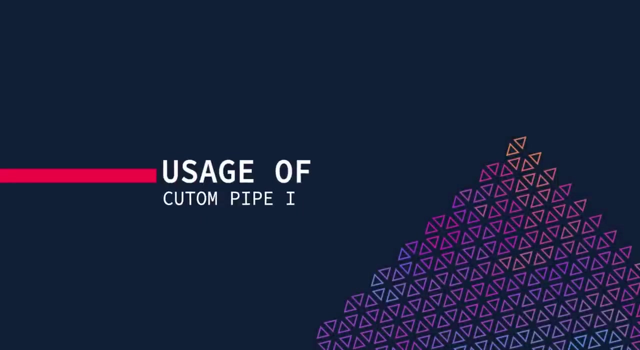 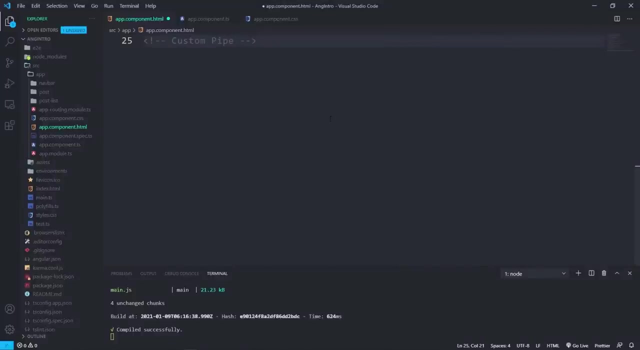 And this end index is 4.. Save this and back to the browser. Perfect. So this is the usage of the angular slice pipe. Hope you guys got the idea. So until now we learnt angular built in pipes Somehow. The built in pipes are limited to some particular situations. 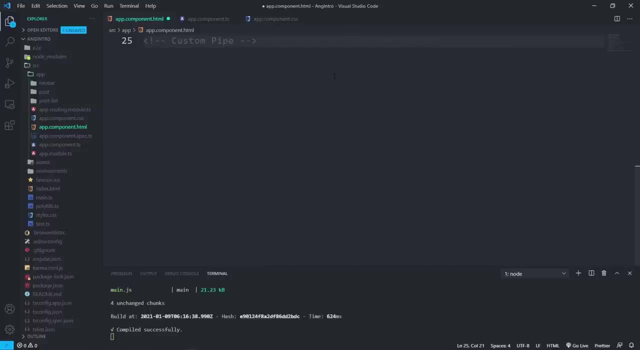 Think if we have a requirement to format the data inside the view, But for that particular situation we don't have any built in pipes, So in this situation we can create our own custom pipes. So in this video let's look at how to create a custom pipe that fits our requirement. 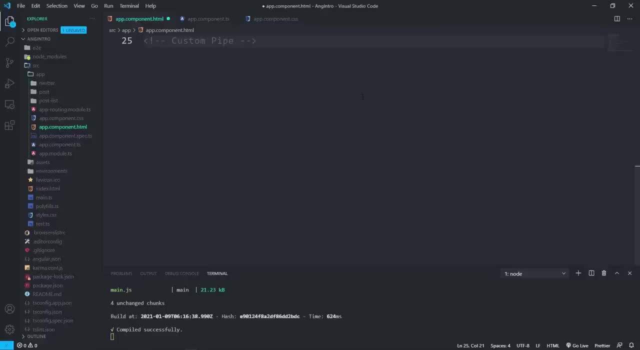 So to create a custom pipe, We can generate a custom pipe file Using the angular CLI, But first let's look at how to create a custom pipe from scratch. Then we'll see how to generate a custom pipe using the angular CLI. Alright, let's create custom pipe for a situation, something to prefix a string value. 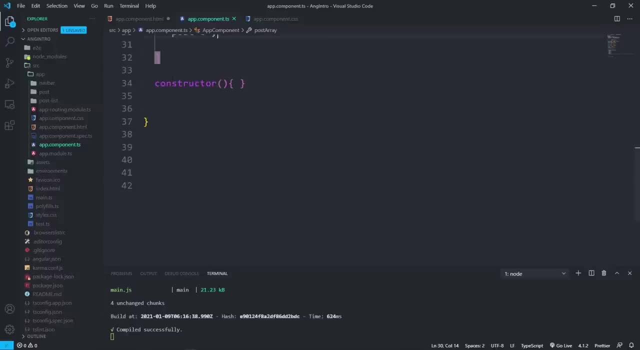 Let's create a simple object. inside the component is file. Object variable is user details. Now assign this to a simple object Name: user1.. And the city is New York And country code is US. Now let's show this inside the browser. 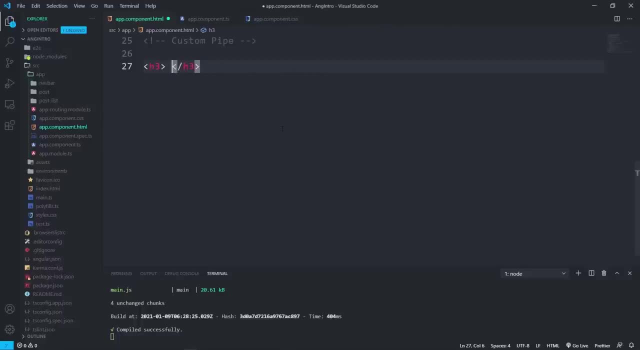 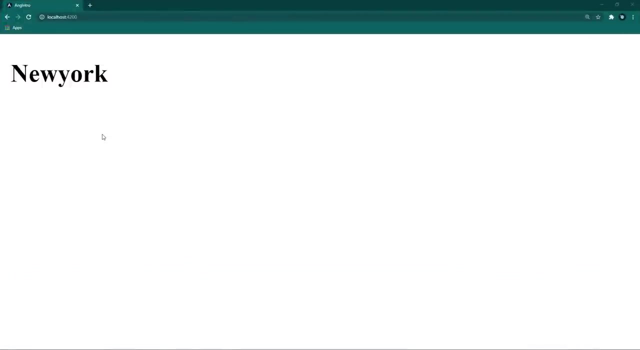 Save this and back to the HTML file And show this city using the string interpolation. Object name is user detailscity. Save this and back to the browser. We got this New York printed here. Now what I want to do is prefix this city with city name. 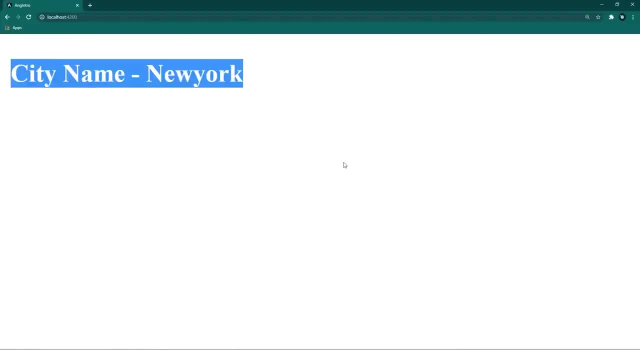 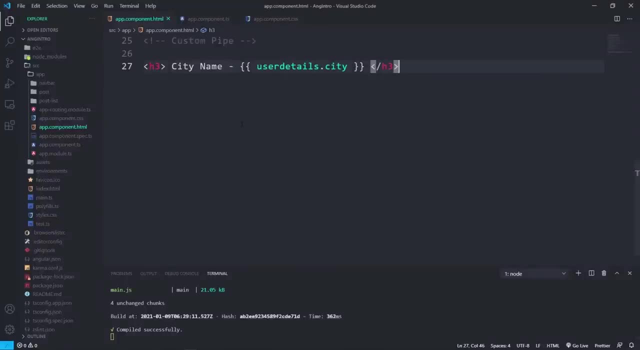 Something like this. This time I did this by hand coding, But I want to do this using an angular custom pipe, So let's do that. First we have to create a file. I'm gonna create this file inside of a folder called pipes. 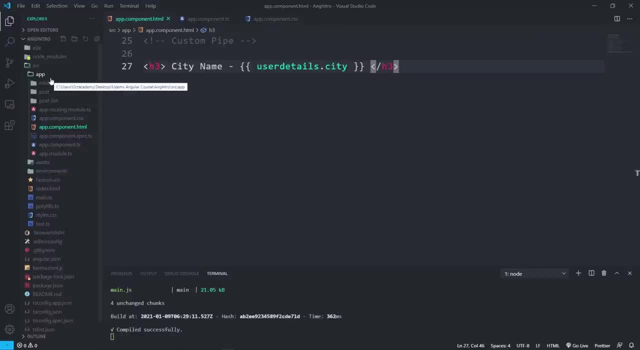 Inside this app folder. We do all the stuff inside this app folder, Right. Let's create the folder inside the app folder. The folder name is pipes. Now, inside this folder, create a file, File name, something append: dot, pipe, dot ts. Look at the naming convention. 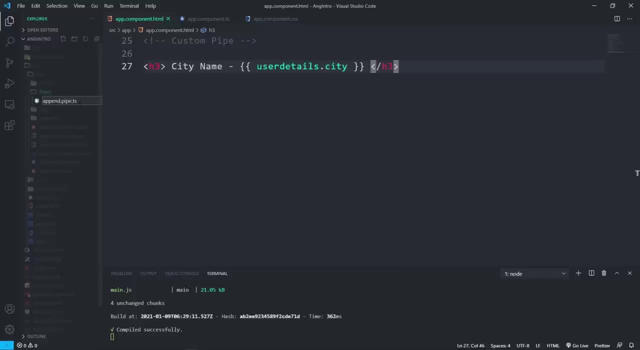 This is also same as components naming convention. First the pipe name, Then pipe keyword And the file extension. Follow this naming convention for best Practice. Now, inside this append pipe file, Let's create the our custom pipe. First thing. first, we need to import two modules. 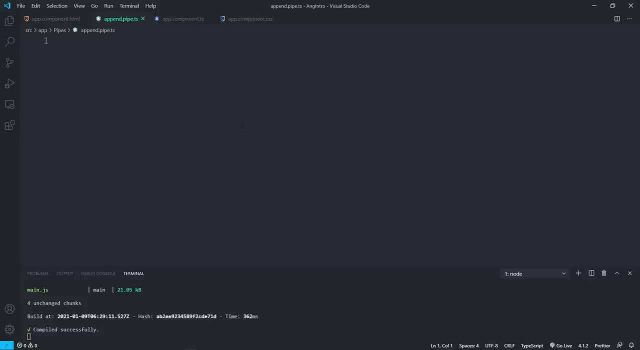 Pipe and the pipe transform Which is coming from the angular core. First let's import the pipe module- Import pipe- And the path is at angular slash core. Next we have to define the name for this pipe, For that we will use this imported pipe as a decorator class. 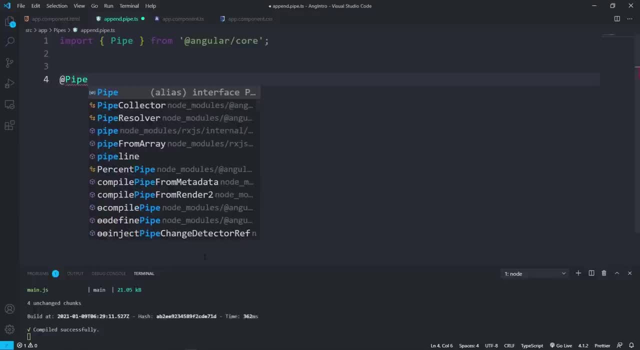 So at pipe brackets, inside this we have to pass the pipe name as an object. So inside curly brackets the key is name and the value is append. If you can remember, we do the same when we learning the components. This also same like angular components. 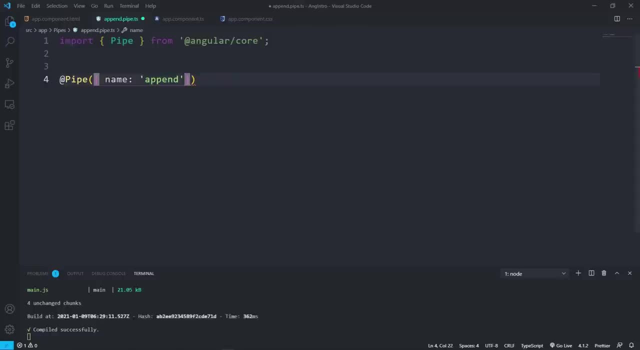 So this name is the identifier to this angular custom pipe. This can be any name, But we are doing the custom appending pipe. That's why I used the name as append. Now we have to create the typescript class, So first add the export keyword. 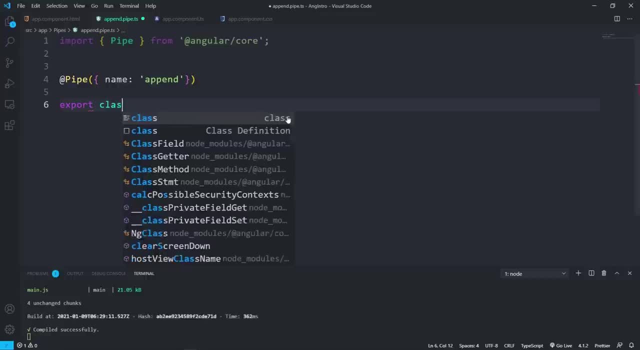 Of course, we will use this from other files. After this class And the class name is append pipe: This A and P capital After this class scope. Now, in order to make this class as a pipe, We need to implement this class to an interface called pipe transform. 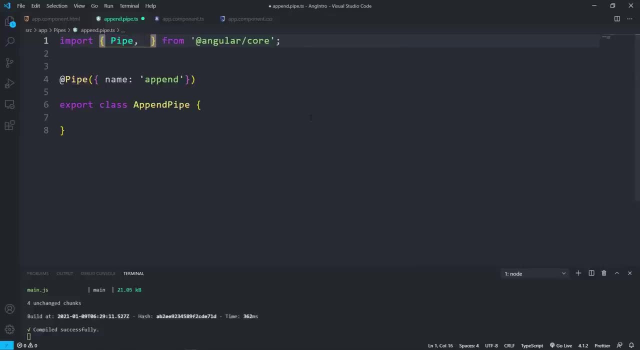 So first, import the pipe transform interface Inside this import statement Pipe transform, This also coming from this same core module. Next, implement this pipe transform to this class. With this implementation, We are telling the angular compiler that this append pipe class also getting exactly the 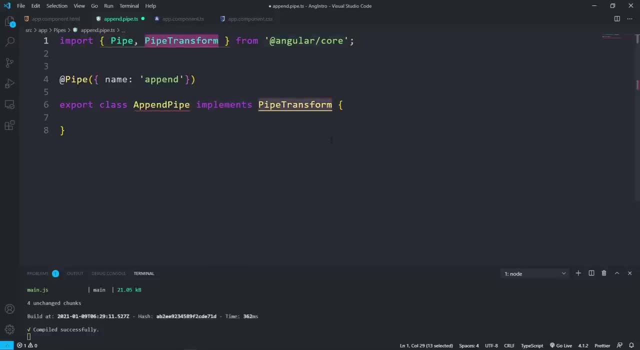 same shape of pipe transform interface. So this pipe transform has a method called transform. So we have to create the same method in this pipe class as well. So that's why we are getting this error. To get rid of this compile error, Create the transform method here. 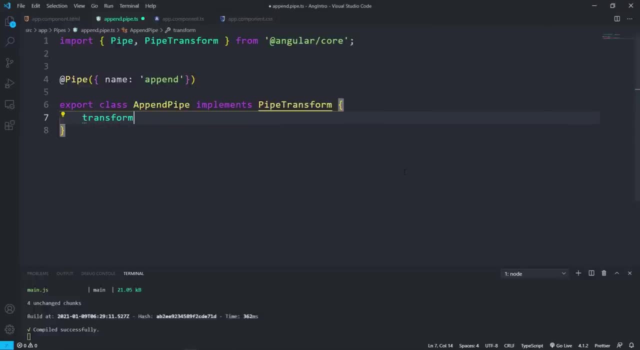 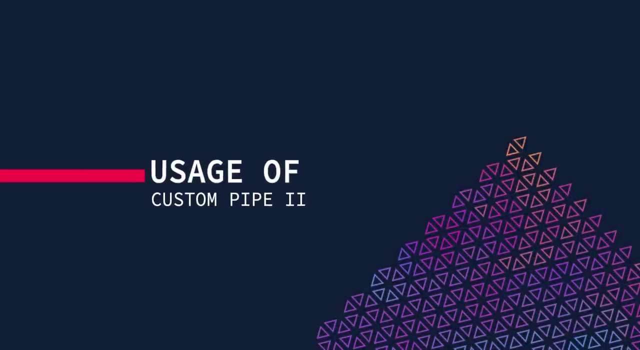 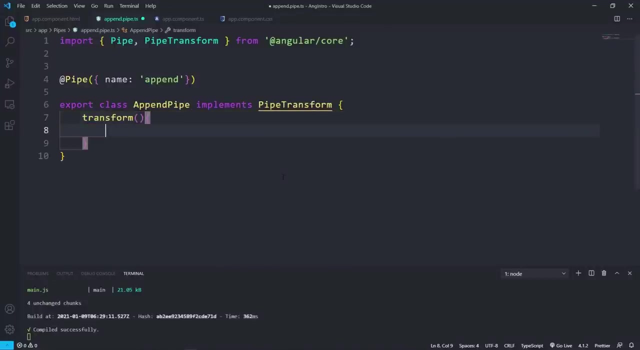 Method name is transform. This is the name of the method. This name must be exactly as this. Don't mistake the spelling mistake or capital simple letters mistake, Otherwise you guys will get compile errors. Next, parenthesis and the method scope. This transform required two parameters. 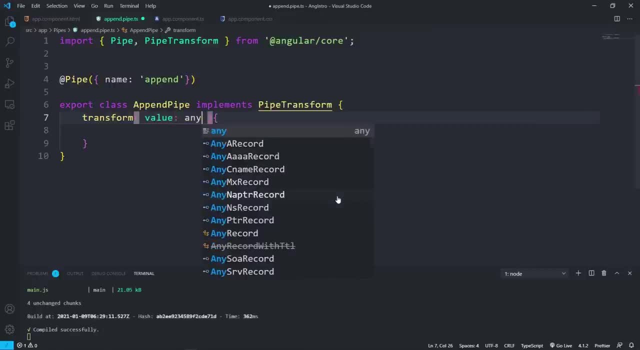 First one is the value parameter. This value can be any. Next, we have the args parameter, Which also can be any. This args parameter is optional, So we can define an optional parameter with this question mark. That's it. This is the process of creating a custom pipe. 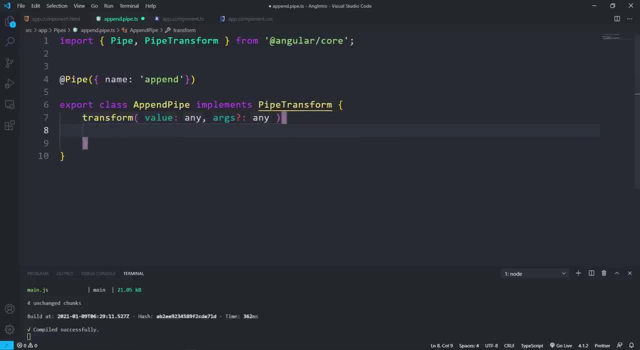 Now all we have to do is the logic inside this transform method. So I just want to append this city name before this value. Just return this value Inside quote City name colon And add a space After this This value parameter variable value. 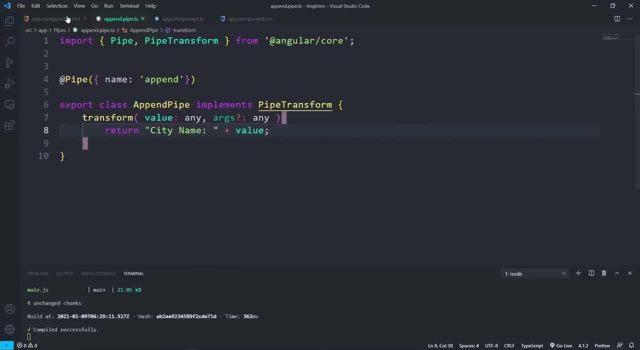 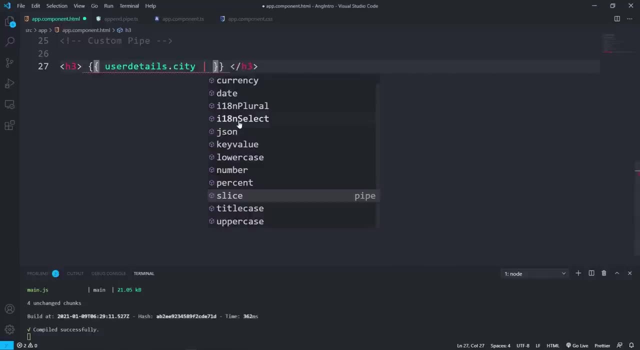 That's it. Now we have successfully created our custom pipe. Let's add this custom pipe to this string interpolation After this pipe operator. This time the pipe name is this: append. Wait, We are getting a compile error Saying that Append pipe is cannot be identified as a valid pipe. 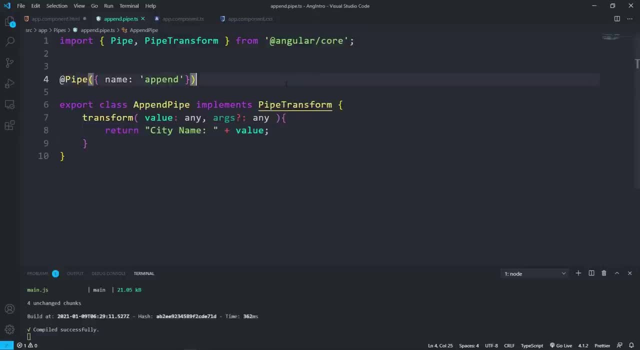 What's going on here? We just created this pipe, But in order to work with this custom pipe, We have to register this pipe in our angular app. Otherwise angular doesn't know about this pipe. This also the same as components: When we creating a new component. 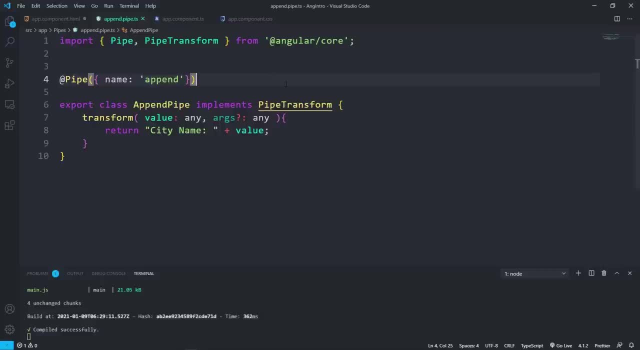 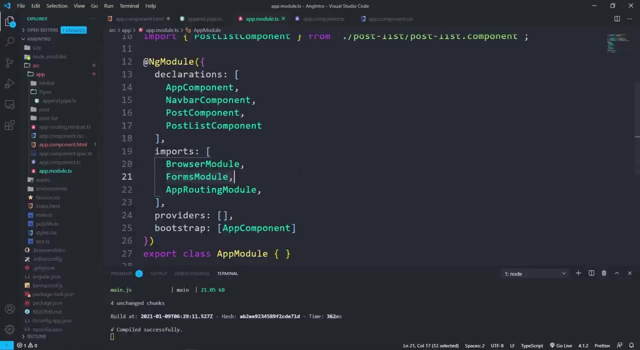 We have to register that component in angular modules, Otherwise that component will not work. The same thing applies here. To solve this compile error: Register this custom pipe. Go to the appmodulets file And register this under this declaration modules. We add all the components and pipes under this module. 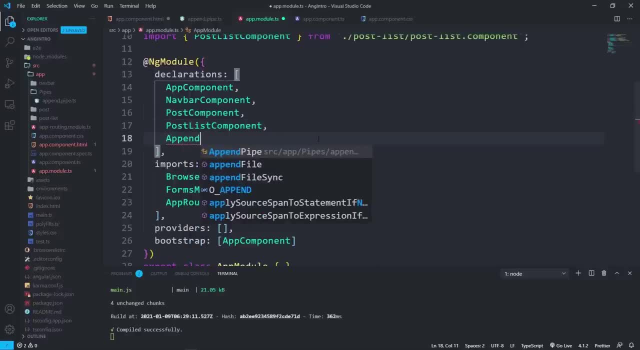 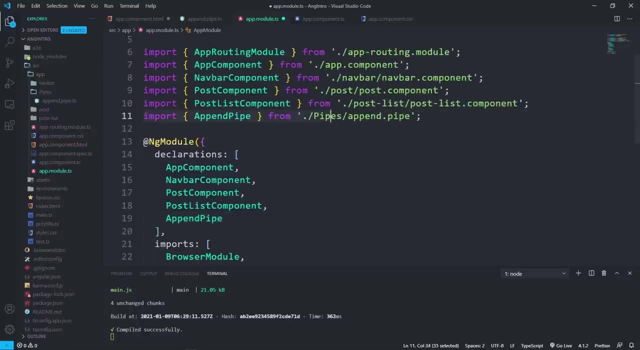 So the pipe class name is append pipe. Look at the vs code intelligence. We got this autocomplete Select that This will automatically import the path of this pipe to this appmodules file. This is the beauty Of vs code intelligence: We don't need to always encode the import statement. 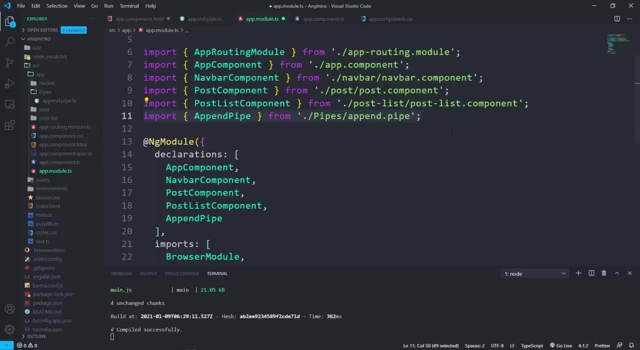 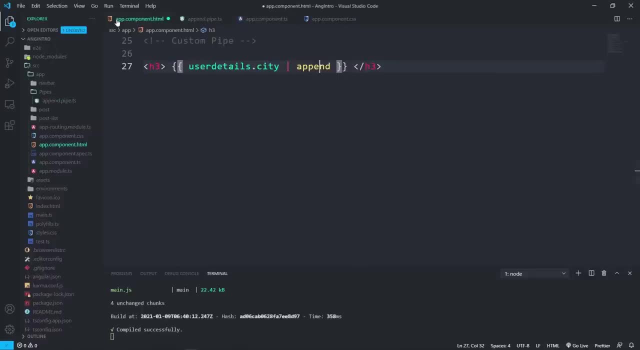 We can simply use the autocomplete vs code intelligence to import the relevant module. That's it. We have successfully registered our custom pipe. Look at this Now. we are not getting any compilation errors. Save this all and back to the browser. Perfect. 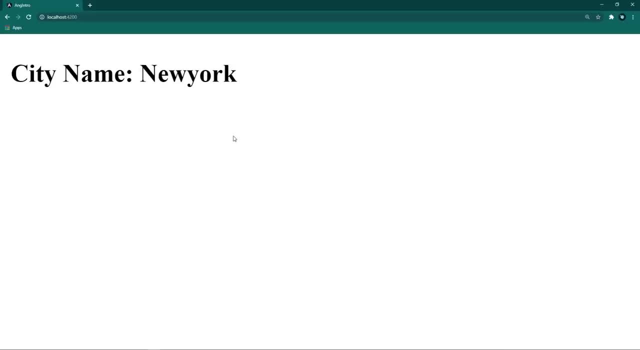 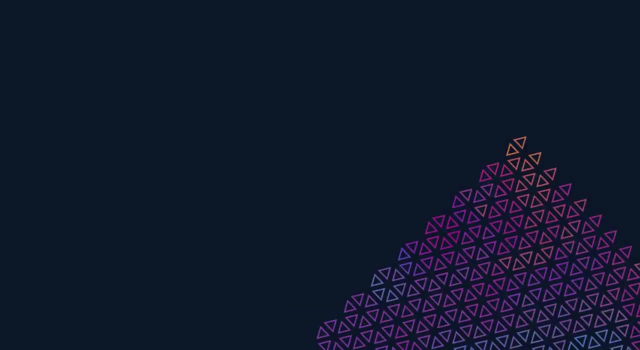 Now we got this city name prefix before the city Beautiful. So This is a very simple use case of angular custom pipe. So now we know how to create a custom pipe from scratch. In the next lecture we'll look at some custom pipes examples for different situations. 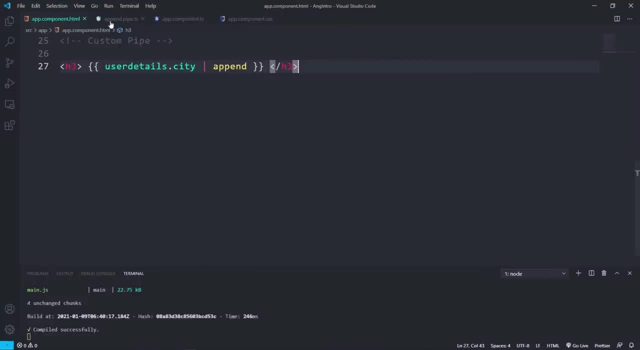 In previous, we learned how to create a custom pipe from scratch. In this video, let's look at how to generate a custom angular pipe using the angular CLI. This is very simple, So Let's start by comparing to the previous method. 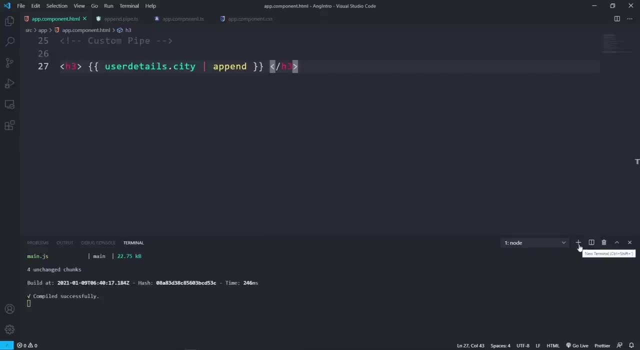 Let's do that Inside the integrated terminal type. this command ng generate. This time we are generating a pipe, So pipe and the pipe name something append CLI. I want to generate this also inside the pipes folder, So add the pipes folder before the custom pipe name. 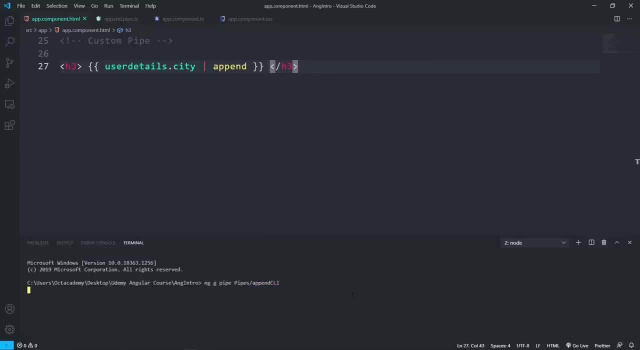 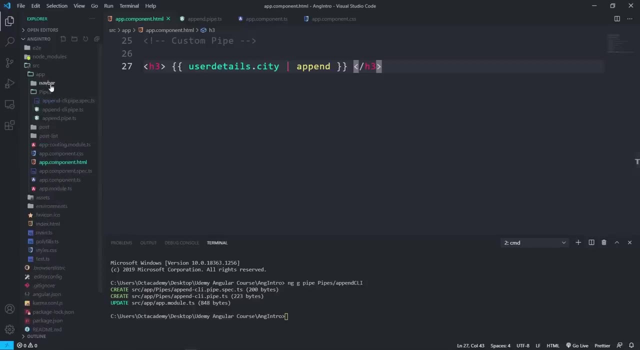 So add the pipes folder before the custom pipe name. So add the pipes folder before the custom pipe name. That's it. Hit the enter key. That's it. Hit the enter key. All right, As you can see here, this generated the custom pipe file inside the pipes folder. 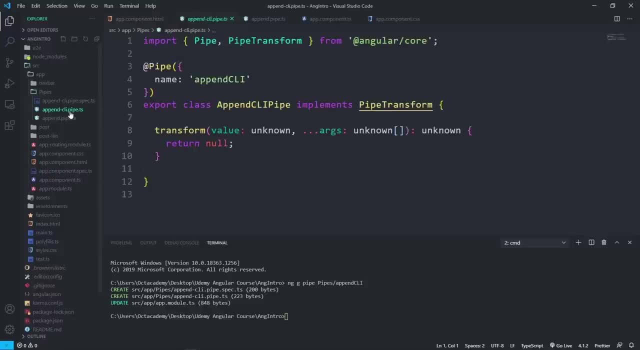 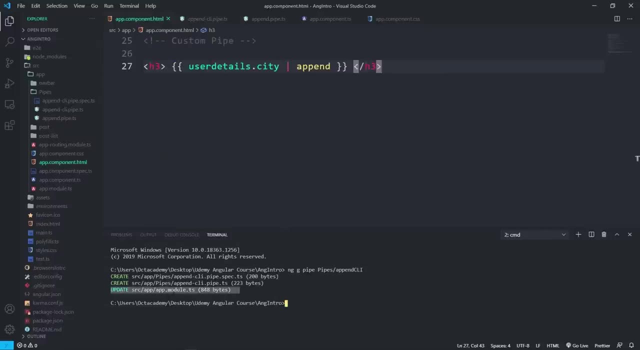 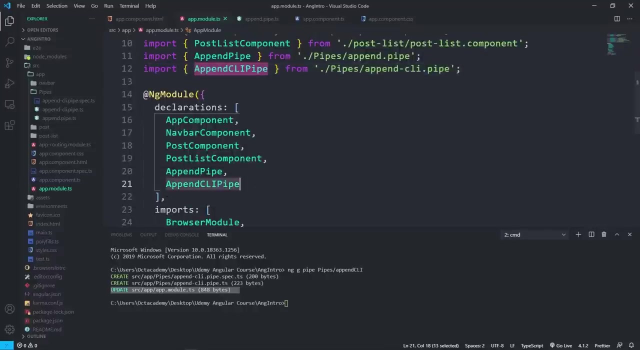 As well as this, created this another spec file for unit testing. Don't worry about that. We are not going to deal with unit testing After this. as you can see here, this automatically registered this custom pipe inside the angular module. This is the beauty of this angular CLI. 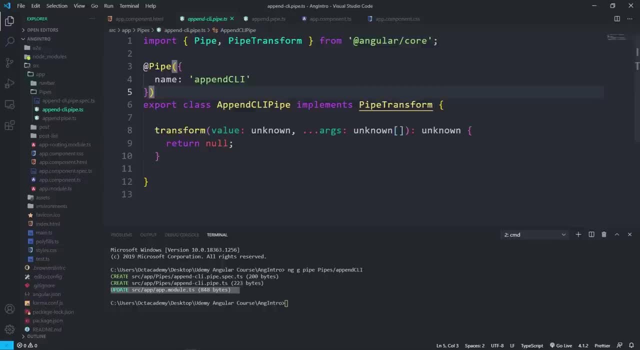 If you look at inside this append CLI custom pipe file, we got all the markups, So all we have to do is add the logic inside this transform method. Just copy this previous logic and paste it here. Change this append text: city name, CLI. save this and back to the HTML file and change. 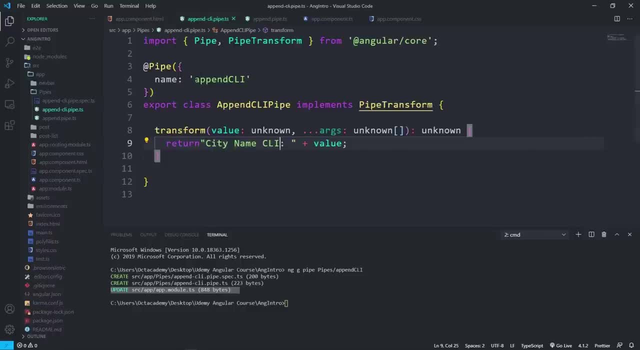 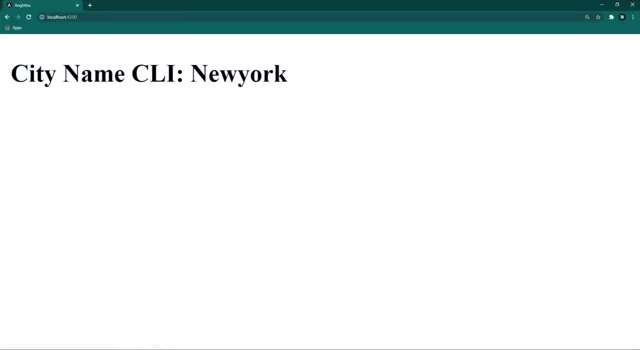 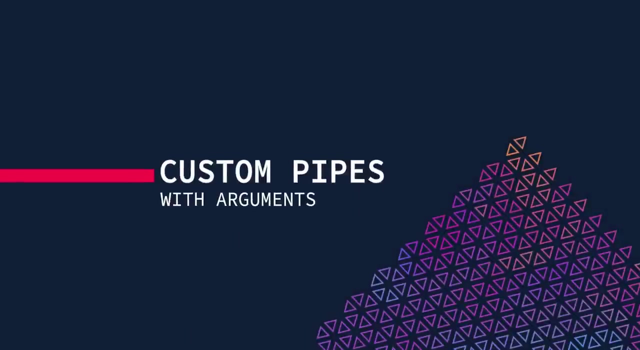 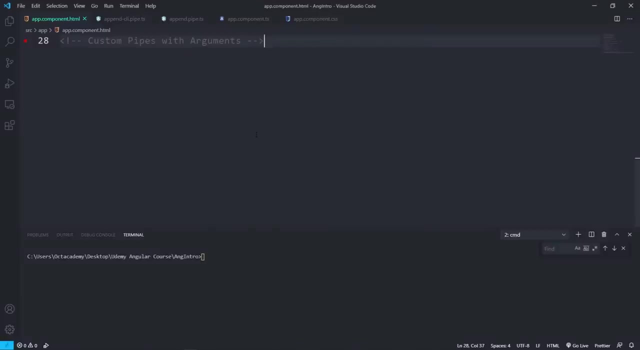 the pipe. This time pipe name is this: Save this all and back to the browser. Perfect, We got this city name CLI appended with this city Beautiful. So this is how we generate custom pipes using the angular CLI. So now we know how to create a custom pipes. 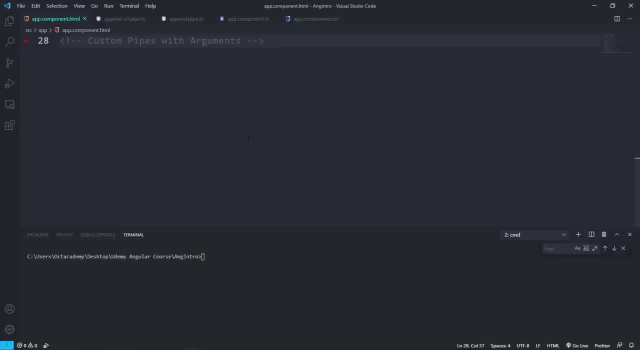 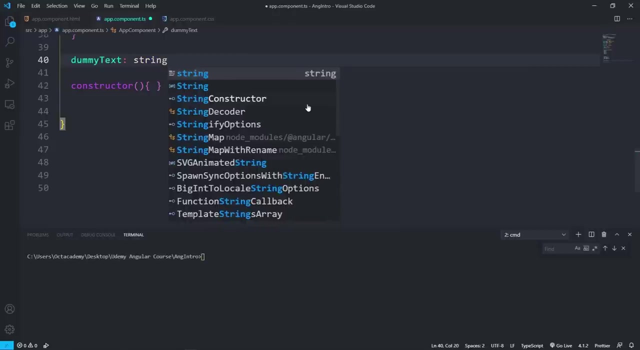 In this lecture, let's create a custom pipe that gets arguments Inside of the component TS file, create a variable for dummy text, something dummy text and assign it to a dummy text. Now I want to show this inside the browser, So do this using the string interpolation. 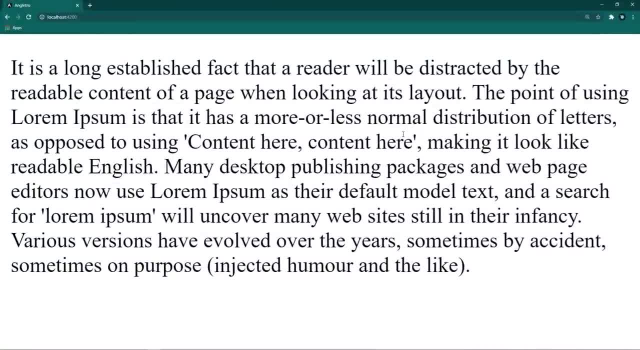 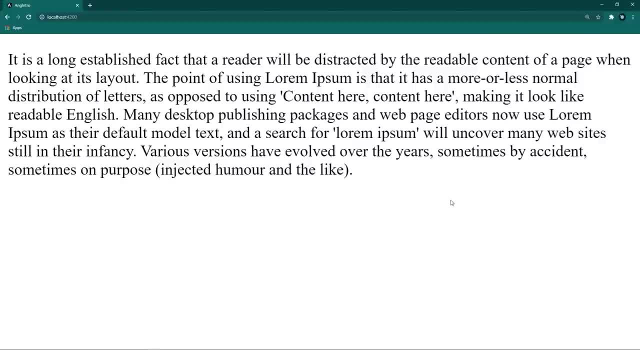 Save this all and back to the browser. We got this dummy text paragraph. Now what I want to do is I want to create a custom pipe. What I want to do is I want to reduce this paragraph's length to 20 characters. 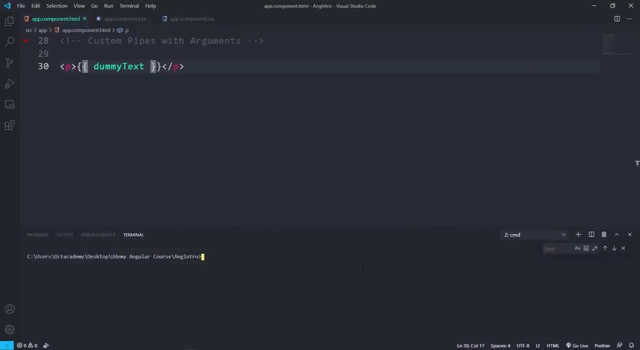 So let's see how to do this using a custom pipe. First, let's generate a custom pipe using the angular CLI. Inside the integrated terminal, run this command ng g. this g stands for generate. We are planning to generate a custom pipe, so pipe. after this, pass the custom pipes. 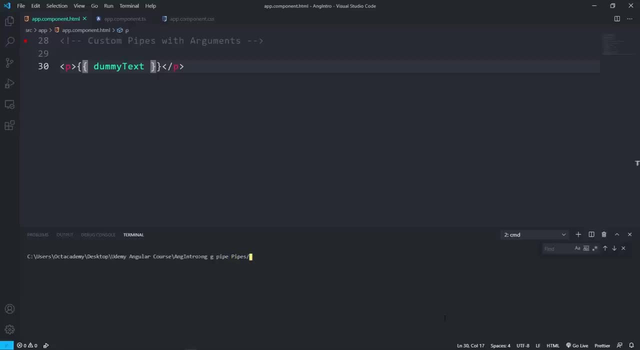 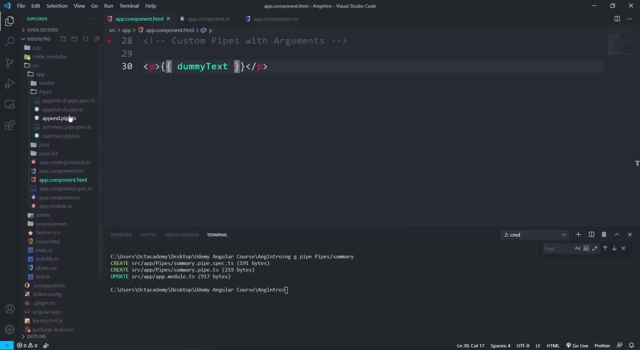 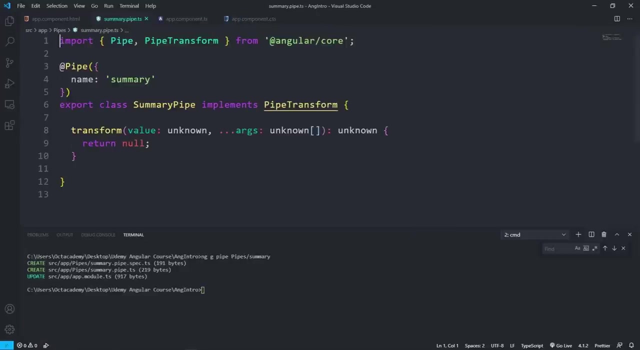 path and the pipe name. The path is pipes slash and the pipe name is summary. Hit enter Perfect. We got this summary pipe. Open it Inside this. let's do the summary logic inside this transform method. Change this type to string. 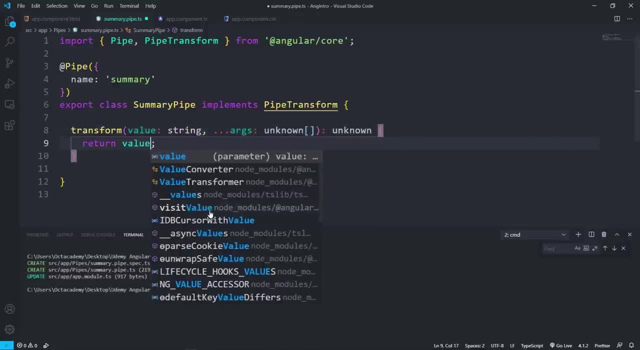 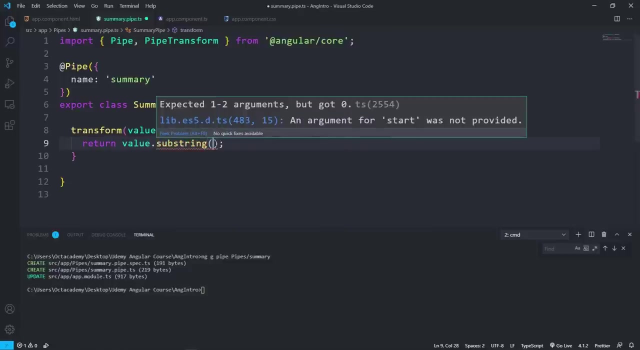 Now let's do the logic return value dot. we can reduce the length of a string value using the substring method. This is a string. This is not an angular thing. This is just a JavaScript string method. So after this substring, pass the minimum and the maximum value. 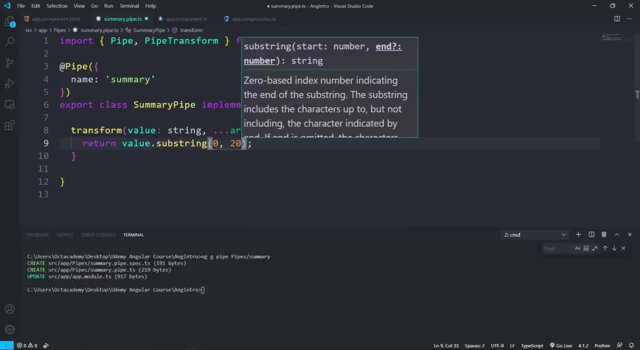 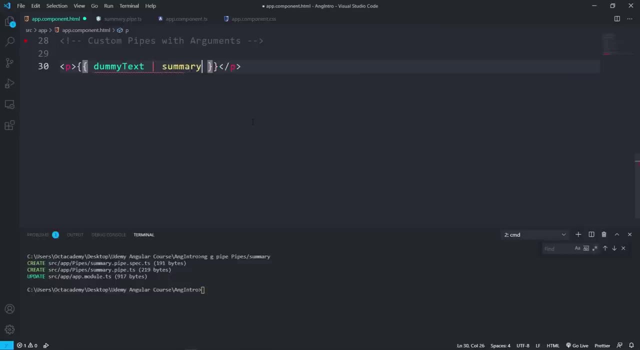 The minimum is 0 and the maximum length is 20.. That's it. Save this and back to the HTML file and add this summary pipe to this dummy text paragraph: Pipe operator and the custom pipe name is summary. Save this and back to the browser. 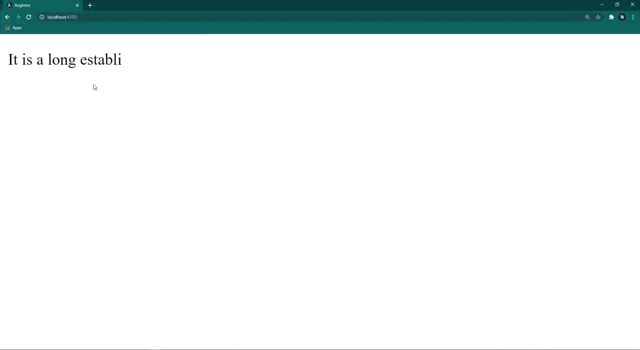 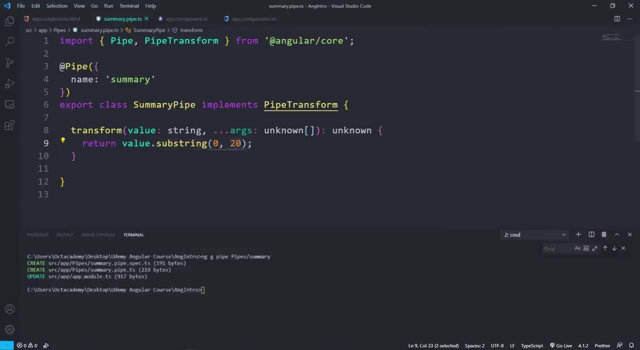 Perfect. This time we got this summarized text, Summarized dummy text with 20 characters. Now what I want to do is I want to make these letters length 20 dynamic. As you know, we can pass arguments with pipes, So I want to pass these letters count from this pipe dynamically. 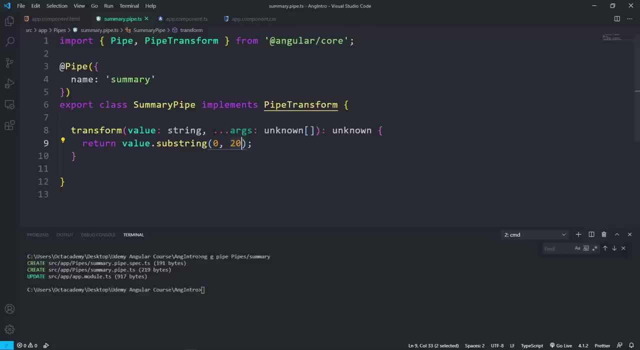 Let's see this in action. This is very simple. Just modify these args, Remove this and add the argument variable as length. This can be changed. This can be any name and this type will be number. Now pass this length value as the second maximum length value. 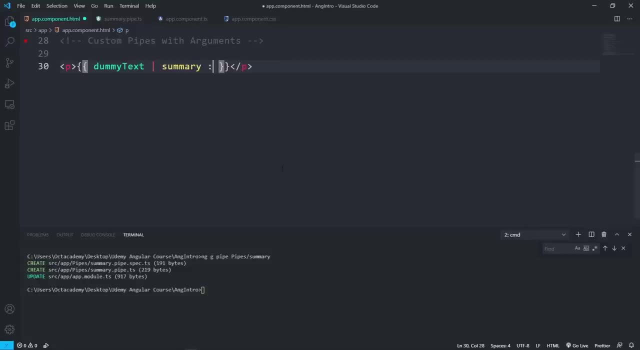 Save this and go to the HTML file. Now we can pass an argument to this colon and the pass a length value around 10.. Save this and back to the browser. Perfect, We got this short, dummy text. Change this length to 50.. 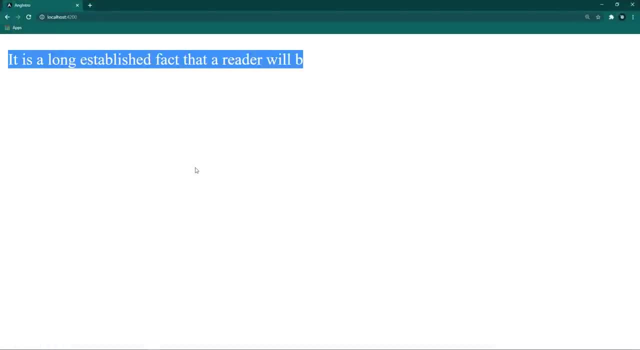 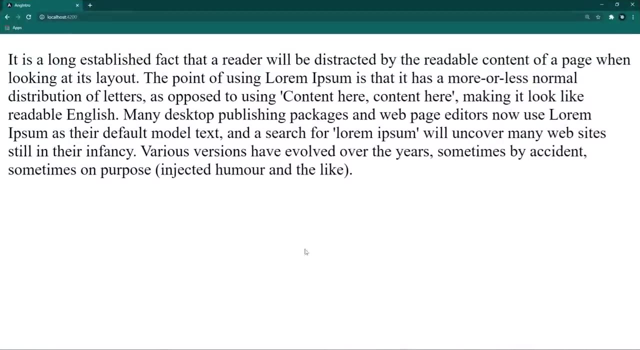 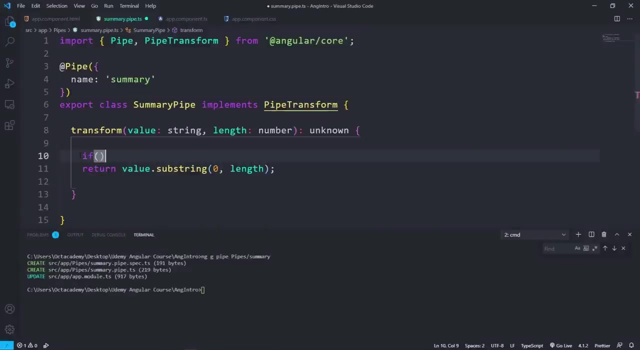 As you can see here, This is working as we planned. If I remove this argument, what will happen? Save this and back to the browser. Now we get the full width of dummy text Cause. now we don't have any argument, So let's set a default summary length to this. 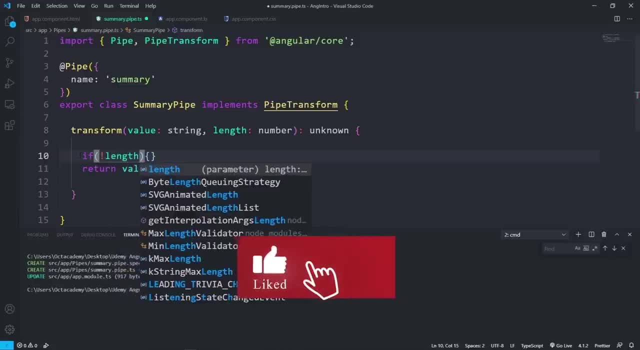 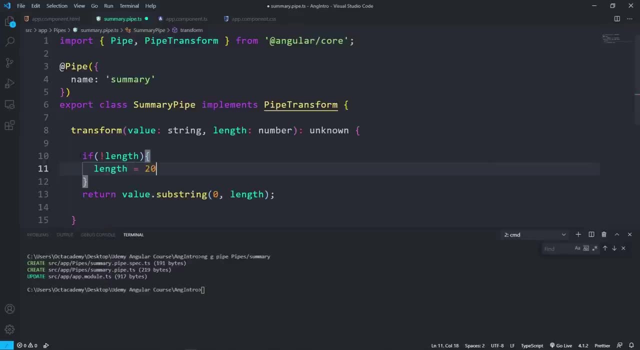 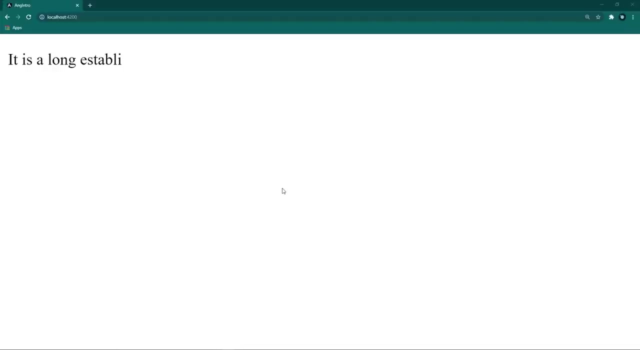 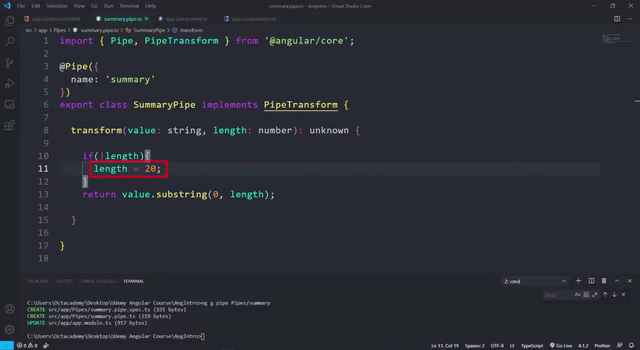 For this we can use a simple if and else, If this length is not set, set the length default value to 20.. That's it. Save this and back to the browser. This time we got this summarized dummy text: When there is no argument, this will automatically set this dummy text character limit to 20.. 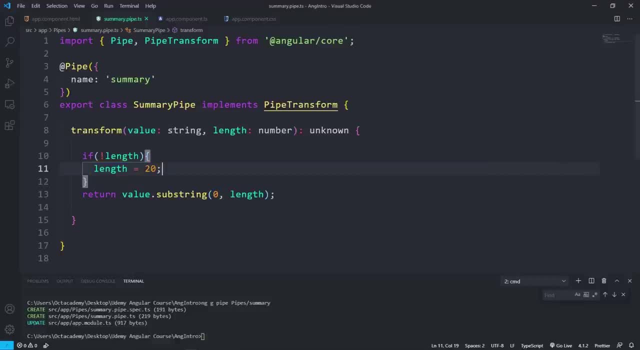 In case, if we want to pass more argument to this, we can simply pass them to this transform method as parameters. Perfect, So this is how to pass argument to a custom pipe. So in this section we gonna be learn about the custom pipe. 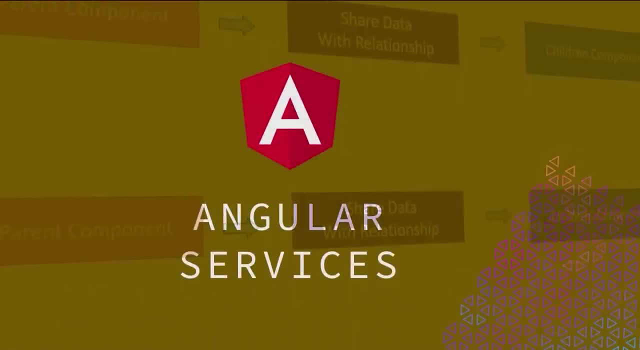 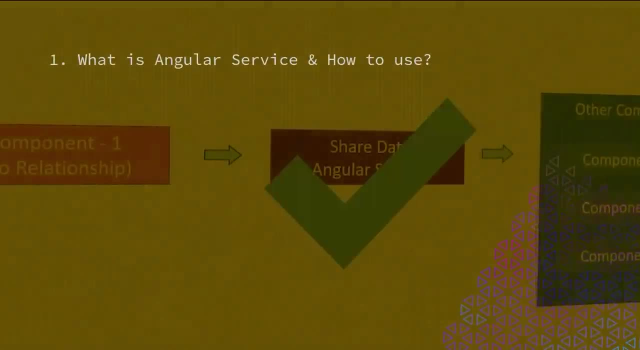 So in this section we gonna be learn about the custom pipe From our last tutorial. at last we gonna be learn about Angular Service and how to use an Angular Service. By the end of this section, you will know about Angular service and use them. 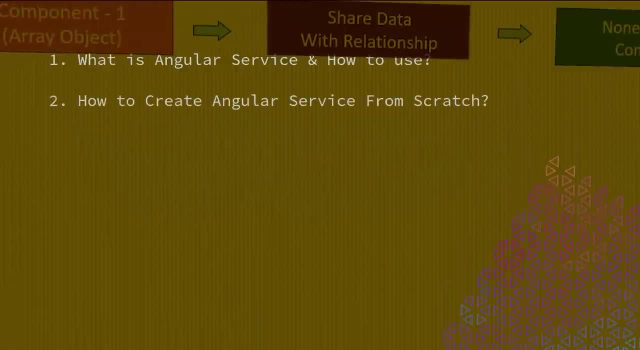 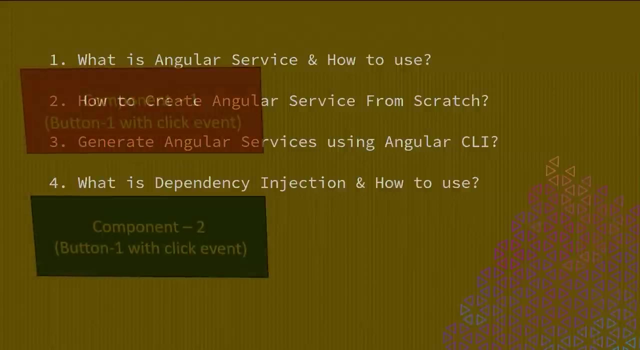 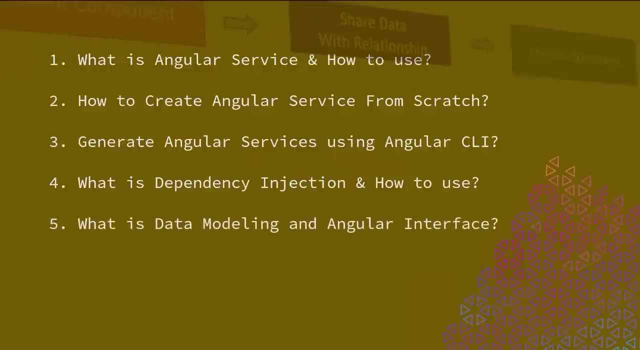 How to create an Angular Service from scratch, How to generate an Angular Service using Angular Clr, What is dependency injection and how to use dependency injection with angular services. At last, we will learn about Data modelling and interfaces in Depot. and let me tell you. 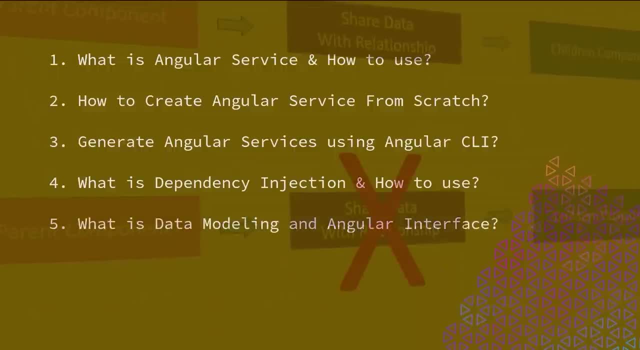 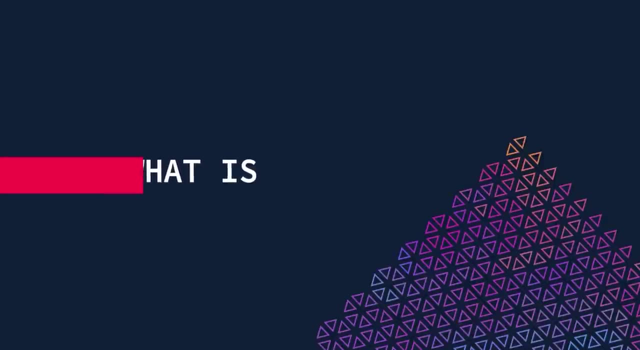 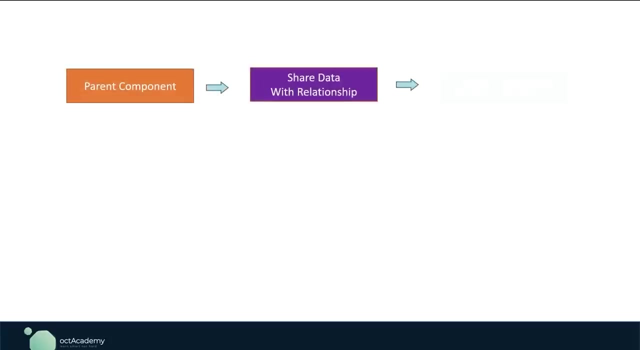 that now's what we'll be learning. Thanks for watching. Let's get started Alright. in previous we learned about sharing data between components when there is a parent child relationship. But think if there is a component that is not related to any other component, and I want 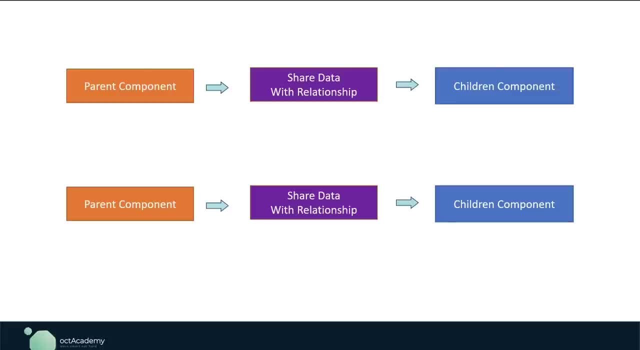 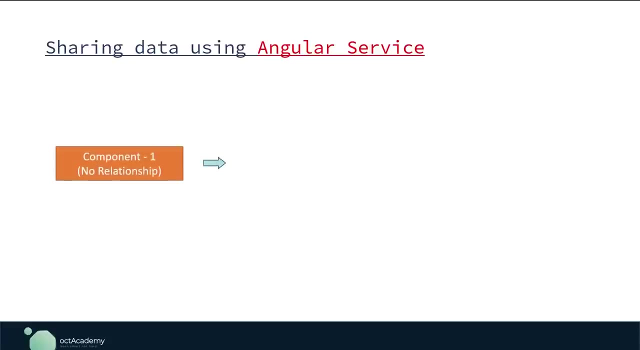 to share data to that component from another component. In that case we cannot actually share the data using any of previous relationship methods. For this we have a solution: We can share data or methods between all other components using the Angular service, Whether there is a relationship between components or not. 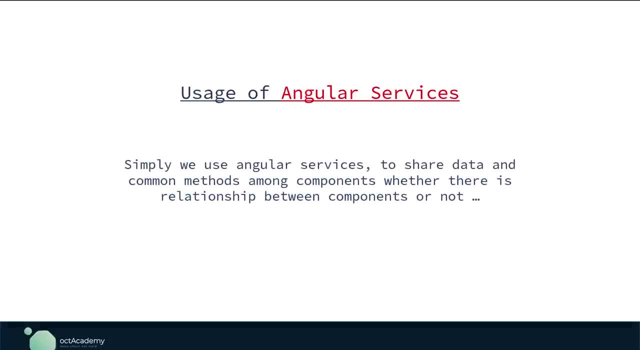 So, simply, we use Angular services to share data and common methods among components. For example, Think we have an array of components. We can create an Angular object for a list of post inside this post component And we have another component which is not related to this and I want to render this. 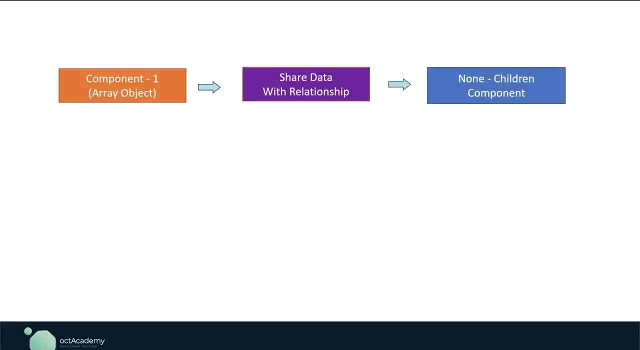 post array inside that component. In this situation, we cannot use any input or output decorators and share data between these two components. Of course, these two components don't have any relationship, So in this case we can create an Angular service And we can declare this post. 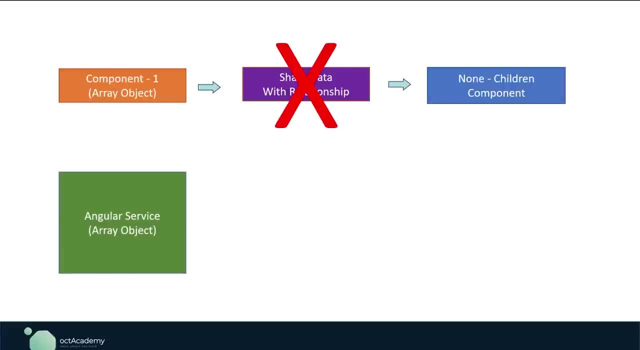 Array inside this Angular service and import this service to this both components, Then we can access this array from this both component. This is not only applicable for variables, We can share methods as well. Think there are two buttons located inside these two components. 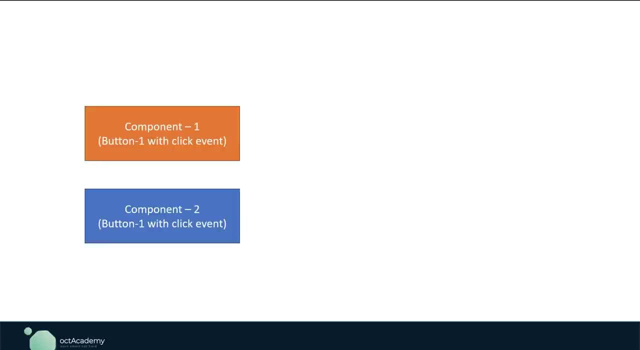 And both buttons, click event, is performing the same logic. So in that case We can create Here one onClick method inside the Angular service, Rather than creating two same methods with this same logic inside these two components. So with this Angular service we can access this onClick method from these two components. 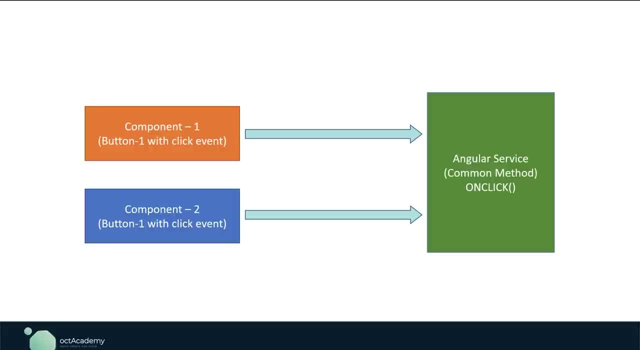 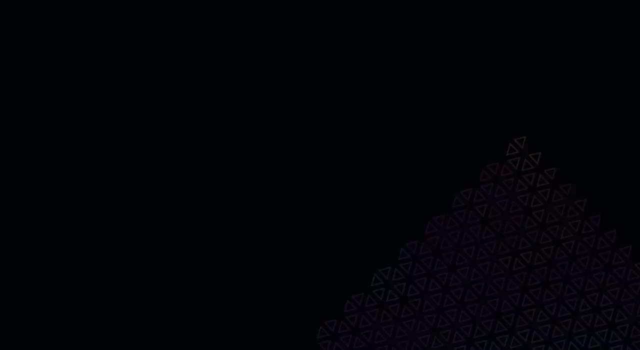 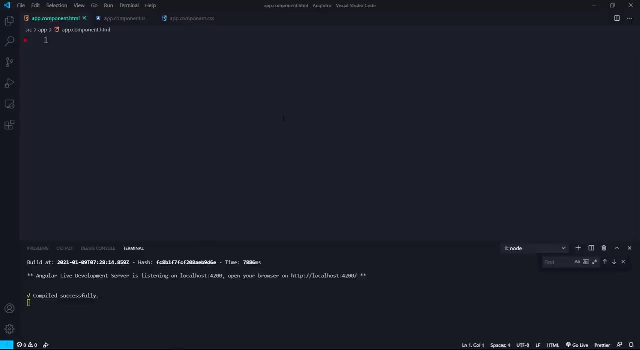 This will help us to reduce code repeating and this will save lots of time. So this is the simple idea about Angular service. With the next lectures, We will understand exactly how these Angular services work And when to use them. Let's create an Angular service manual. 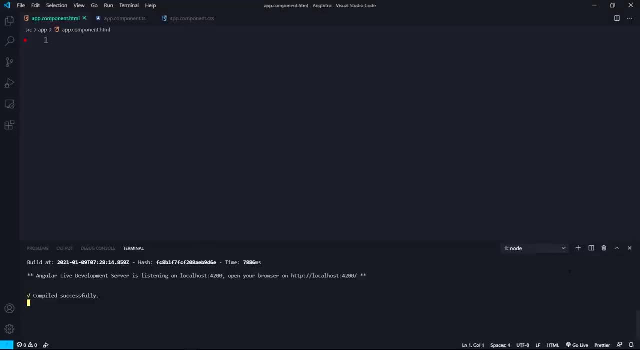 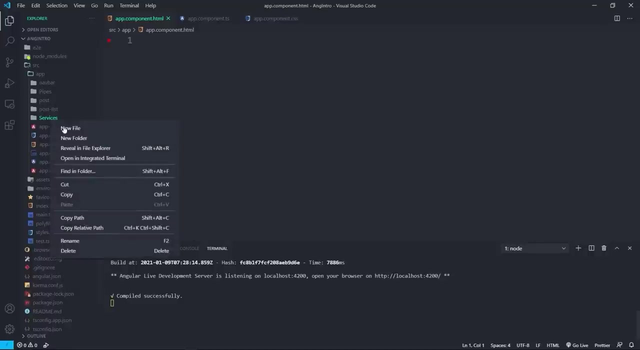 Which is very easy. Just create a file inside the app folder. Wait, let's put all the services inside of a folder called service. So create a folder inside the app folder. The folder name is services. Now, inside the services folder, Create a new file. 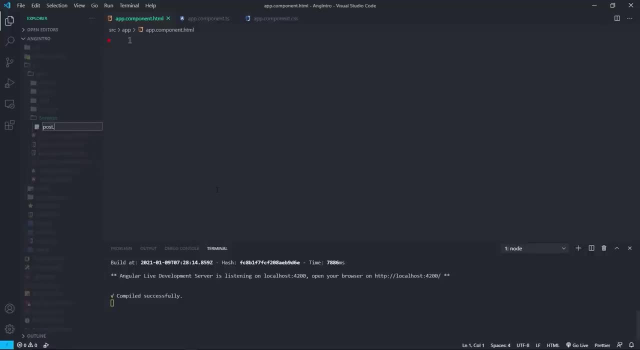 The file name is post dot And we are creating a service, So service dot And the file extension is dot ts. Nothing fancy, This is just a naming convention. If you can remember, we named components and custom pipes like this. All right now open the service file. 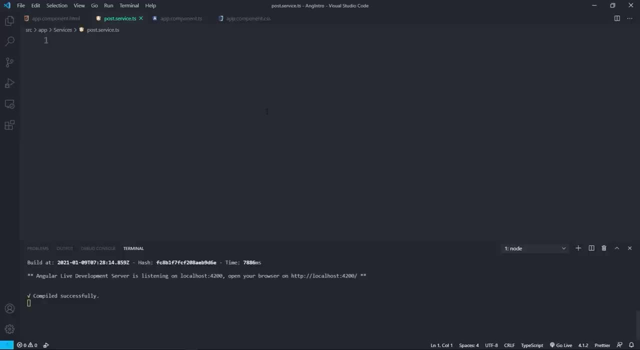 Inside this Let's create a TypeScript class Export. So We gonna access this class from outside of this service. So we have to export this class. So the export And class, The class name is PostService. This first letter, P, and this S, Capital letters. 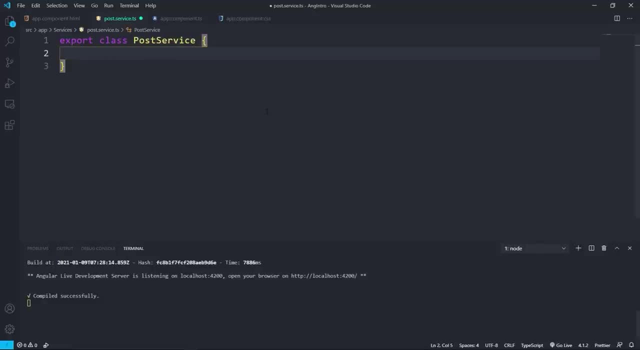 After this Class scope. This is it. We have successfully created the Angular service. So, like components and others, there is no fancy code for service. Angular service is just a simple TypeScript class. Now, inside this, we can create the method or data that we want to share with components. 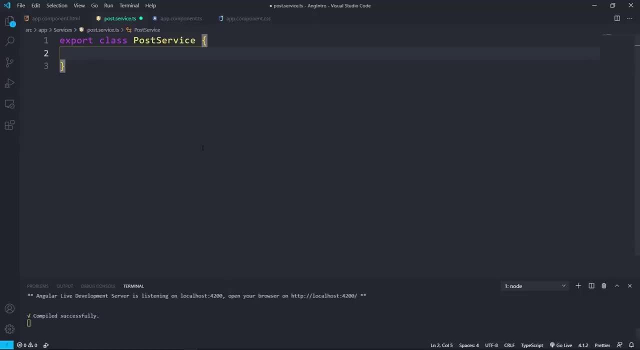 So let's create a simple array of objects for post, This time name, This post list And this type is array, And set the array type to any. Now let's assign some data to this. The first object key value pair is id. 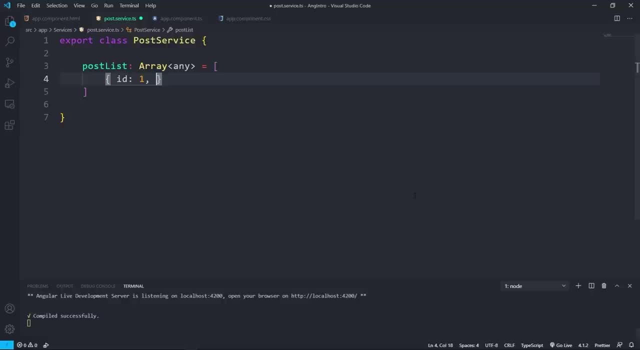 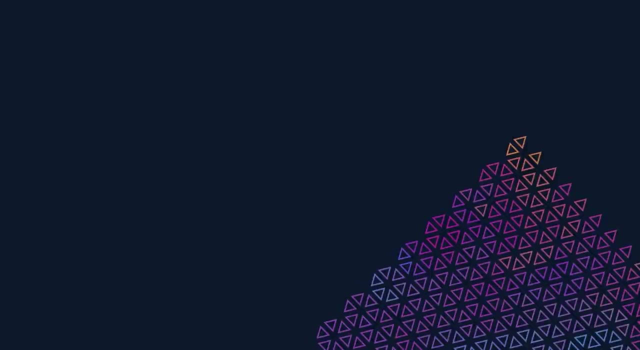 Value is 1.. Next The post title And the value is post1.. Open and paste this object. few times Change the id and the post title. So now we have created the data. Let's see how to access this data from another component. 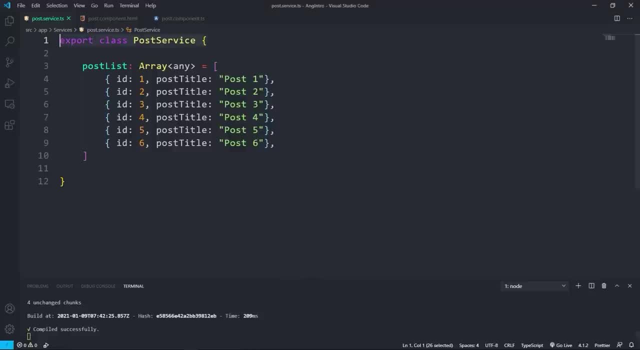 In previous we have created this postService and this postList array. Now let's see how to access this postList inside this component and show this inside the post component v. As you know, we have created a TypeScript class inside this postService, So in order to access this class from this component, we have to create a new instance. 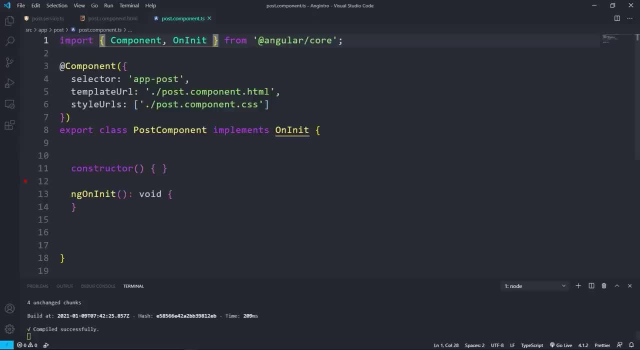 of this class. So inside the component constructor. let's create the instance of this service class. So first import the service class to this component. We already exported this service class. So inside the component, import inside curly brackets. service class is postService. Follow the capital, simple letters carefully. 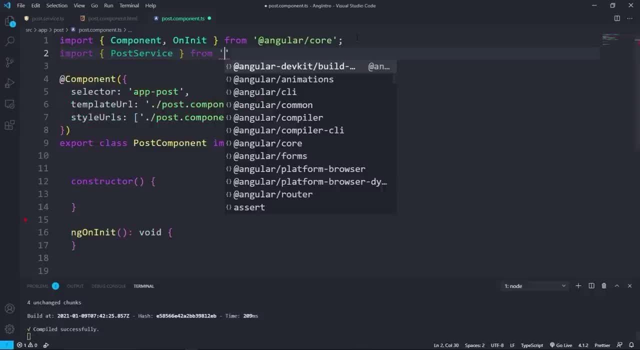 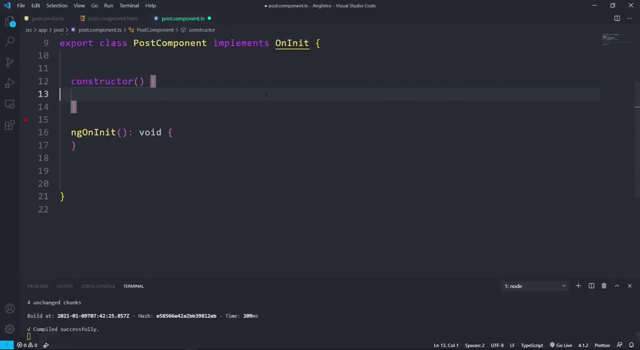 So after this from and give the path of this service class, Go on folder back. double dot slash Inside the services folder: post dot service. That's it. Now let's create the new instance inside this constructor New, and the service class is postService and parentheses. 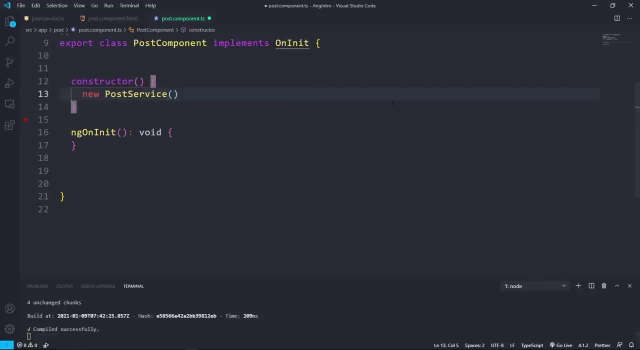 Assign this new instance to a variable. let postService Note this. we created this variable. first letter is simple and this l is capital. Note same, like this service class name. Now we can access this service class variable and methods. So postService, which is this new instance variable and dot. now look at this intelligence. 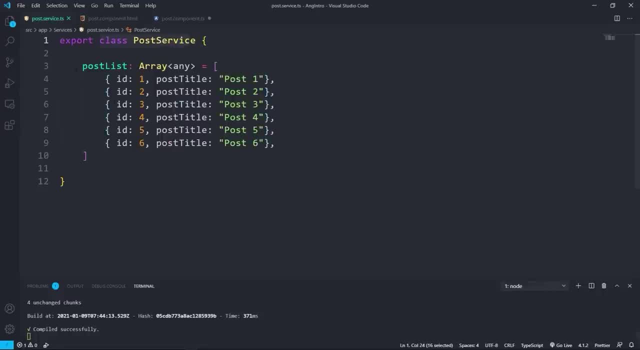 We got this post list array variable, which means now we can access that variable from this post component. So select this post list variable. Now assign this to a global variable so we can access this from the component html file and render this array to a beef. 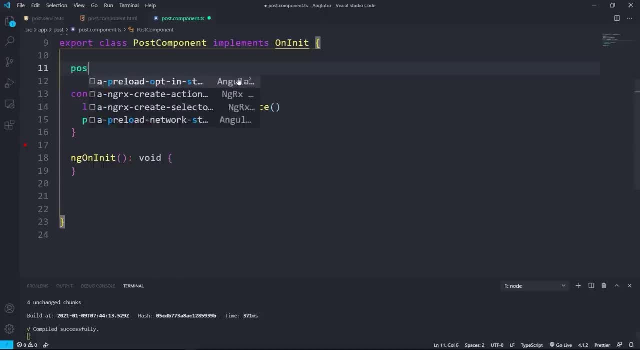 So inside the class code, the variable name is post and data type is array and array type is any. Now assign this to this post, this dot post. assign Now inside the html beef: create a ul tag with li tag Inside this li tag. this post is an array, so in order to show this array data inside the 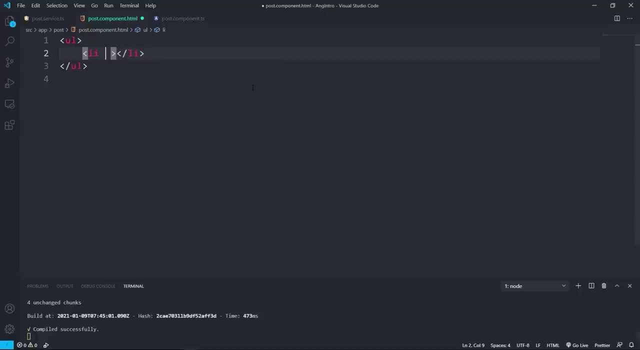 beef. We have to use ng4 directive, So asterisk and ng4 equal sign inside quotes. let post of posts Inside this li tag lets show the post title using the string interpolation. So open and close two curly braces inside this post, which is this variable dot post. 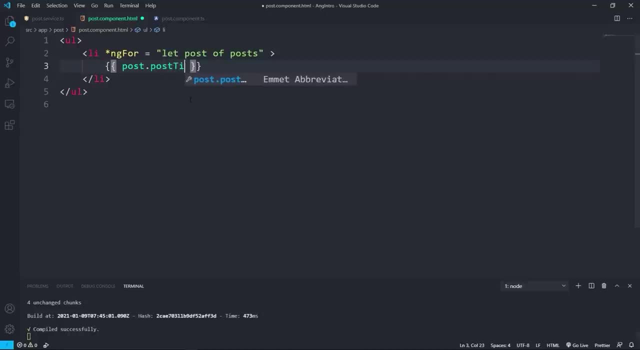 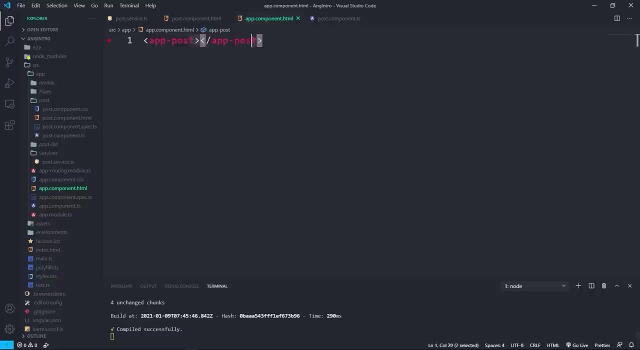 title, Which is the object key for the post title. So in order to see this inside the browser, we have to add this post component selector inside the app component. Inside the app component html file, add this component selector- app dash post and hit enter. 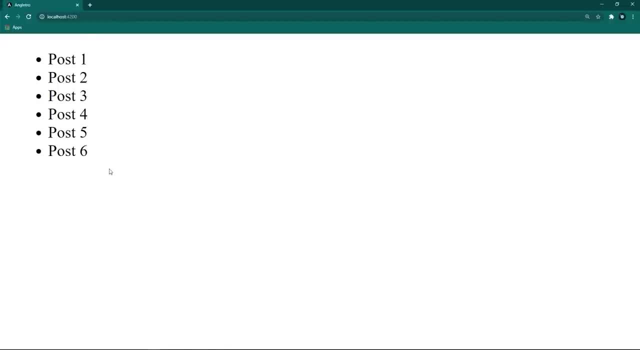 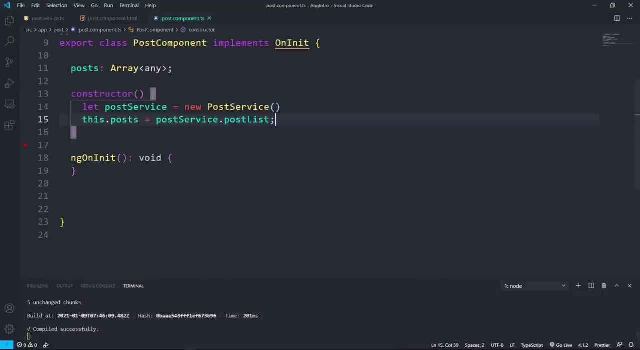 Now save this all and back to the browser. As you can see here, we got this list of posts here, So this is the normal, traditional way of using post. But we have another, cleaner way to implement this, which is angular dependency injection. When we creating this new class instance, this will become dependent on this component. 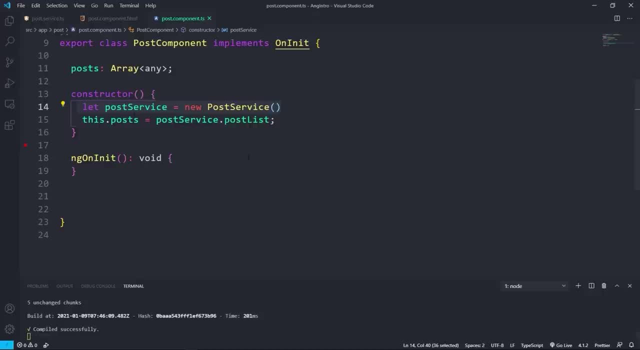 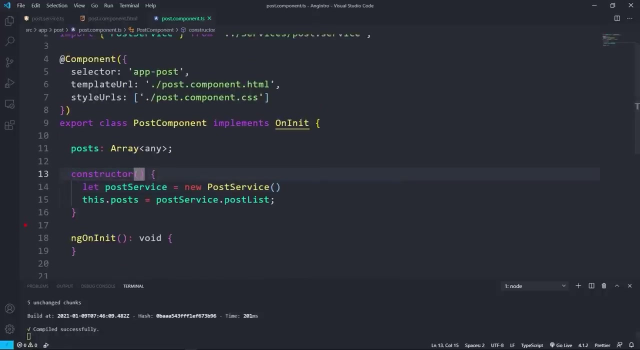 So angular giving us another design pattern framework called dependency injection for us to manage dependencies. This is a kind of framework inside of a framework. So this is very simple. all we have to do is inject the service class into this constructor. So lets do that. 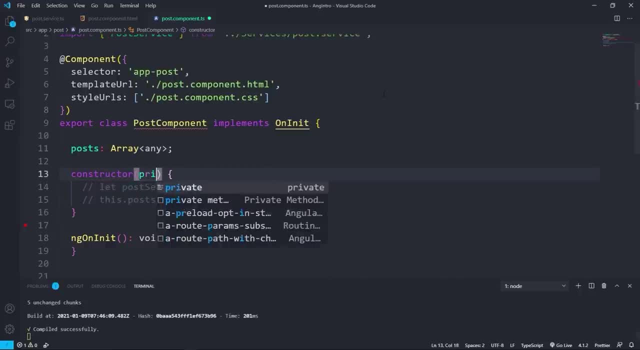 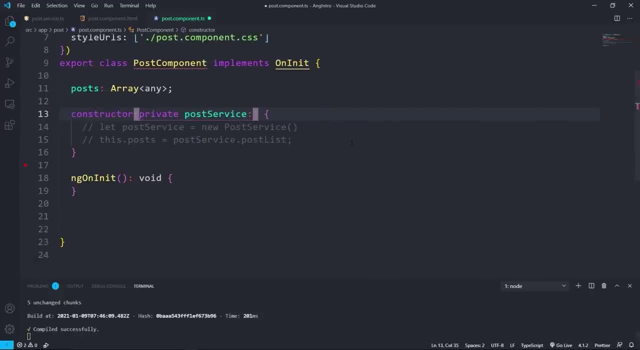 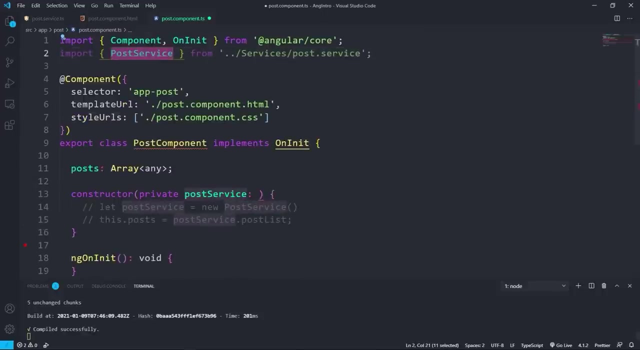 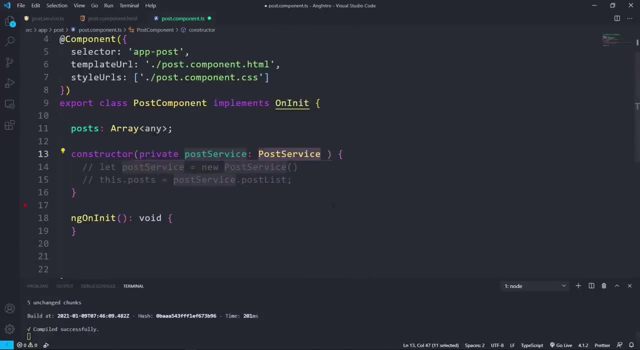 First remove this new class instance. we don't need that anymore. Inside the constructor: parenthesis: private post service. this is just a variable name. this can be any name After this. set this variable data type to this imported post service class. That's it. So this will inject all the post service class properties and methods to this constructor. 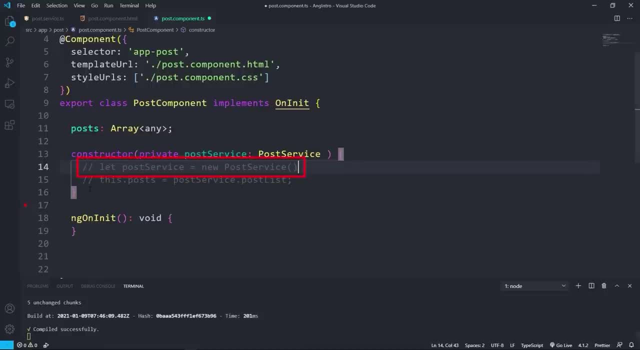 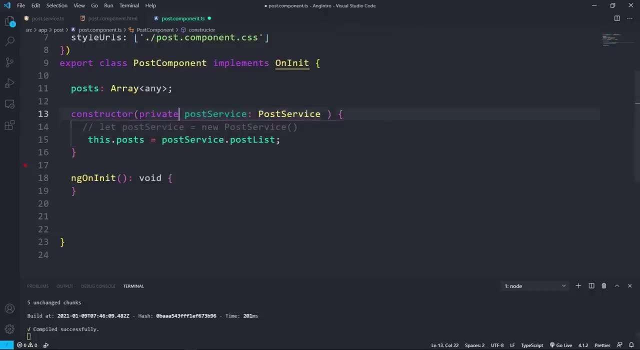 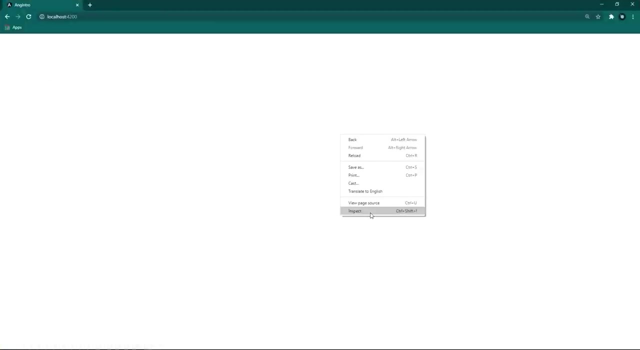 Which also like creating the new instance: Nothing fancy, but cleaner and more maintainable code style. This time, this post service is this injected post service, So save this and back to the browser. we got this empty view. Open the browser console. inside this, we got this null injector error. 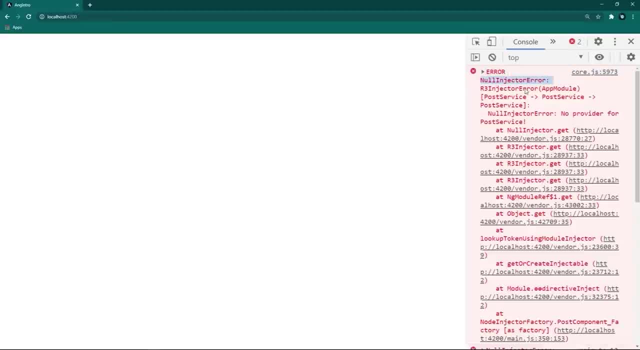 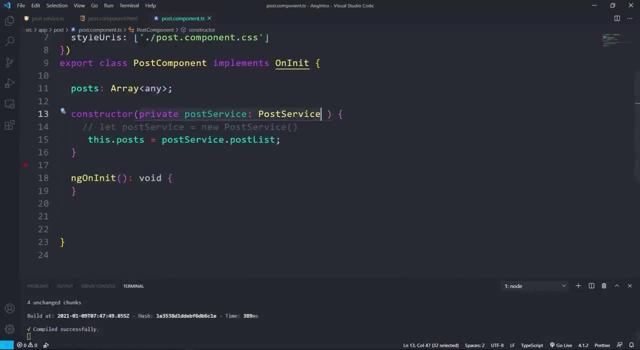 We injected this to this component, but angular doesn't know this data service class as an injectable class, So all we have to do is we have to provide this service class as a provider In the previous work, like component custom pipes register, we have to register this data. 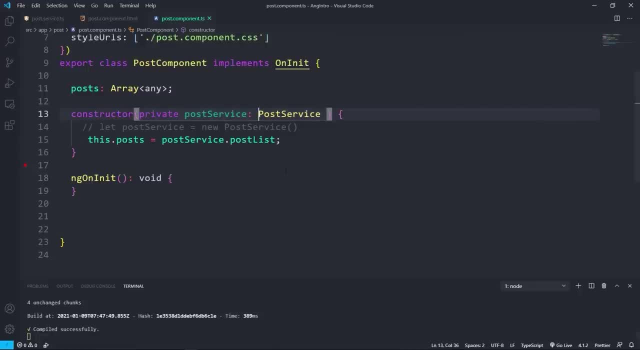 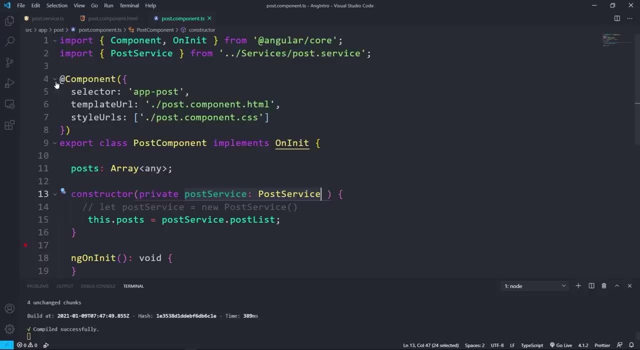 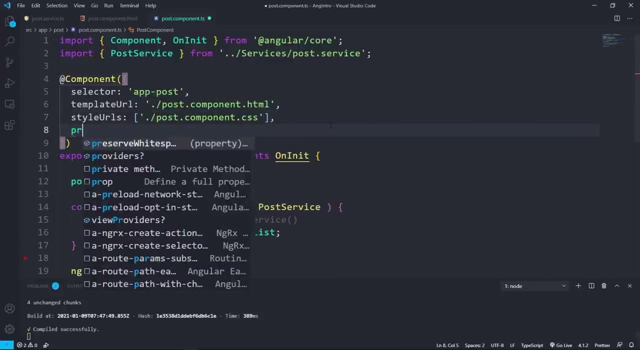 service class as a provider, Then only angular understand this data service class as an injectable service class service class. so we can do that by passing the provider parameter to this component decorator. so after this, just pass the provider, and this required an array, so square brackets. 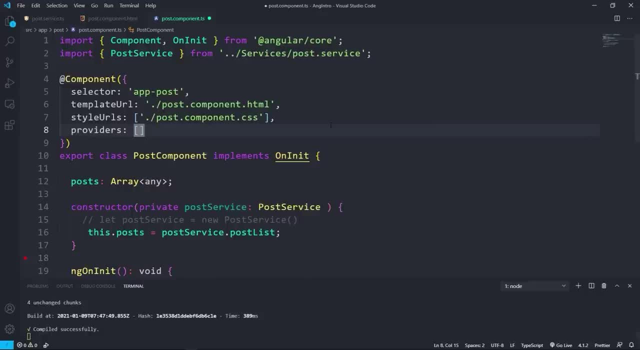 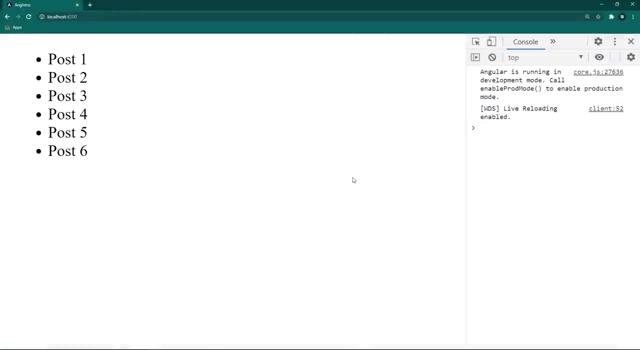 insert this pass, the service class that we want to inject to this component class: constructor: post service. so please don't forget to follow the capital simple letters correctly, otherwise this can lead to unnecessary bugs and errors. so that's it. save this and back to the browser. perfect, we got this list of posts, which means everything working as we expected. 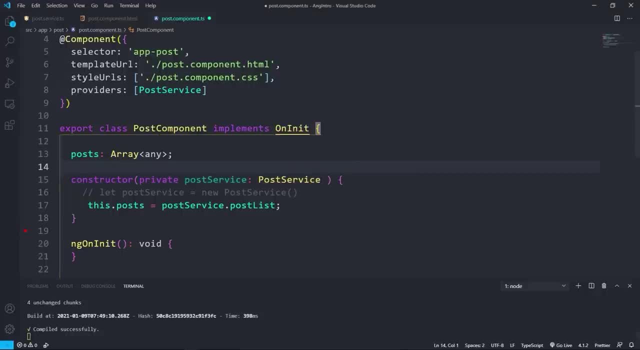 so in previous we did this dependency injection. in order to work this dependency injection we have to tell. so in previous we did this dependency injection. in order to work this dependency injection we have to tell: angular to this service class is an injectable class. so we did that using the provider's. 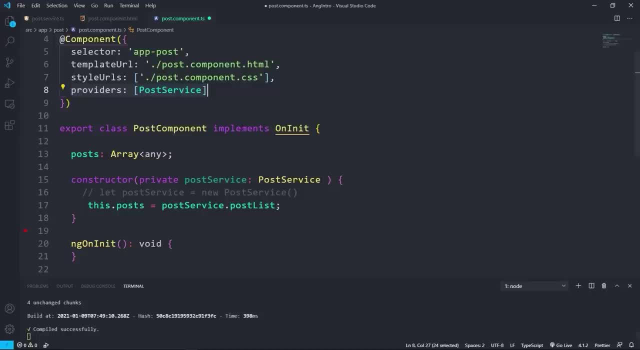 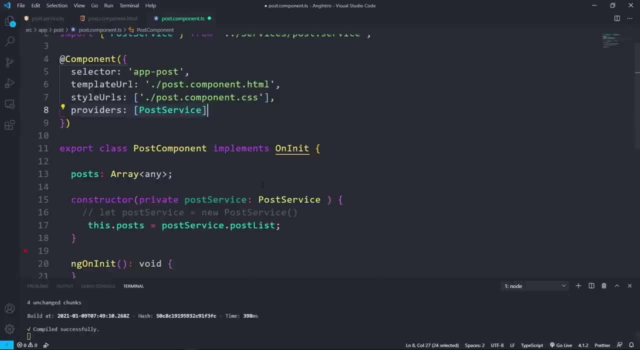 parameter for this component decorator. so with this we are creating a new instance of this data service class which can be accessed only from this component class. think if there is another component and i want to access the same post list array from that component also, or we can do that. 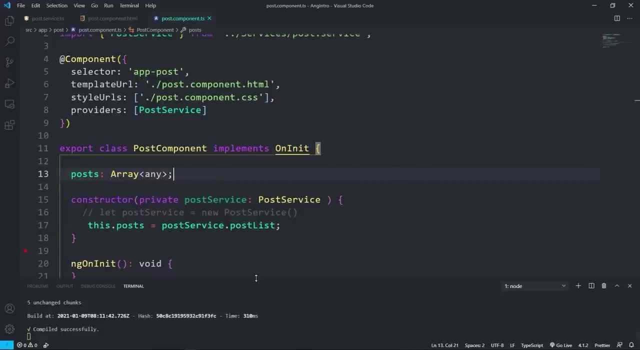 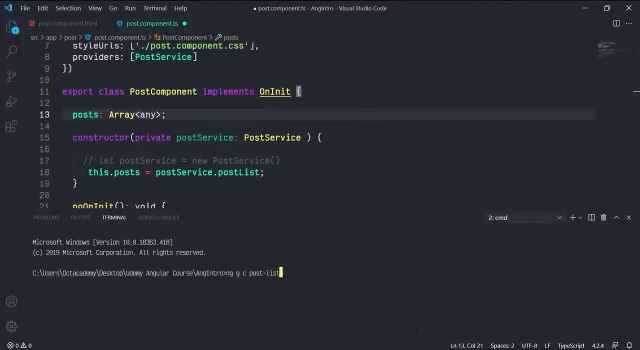 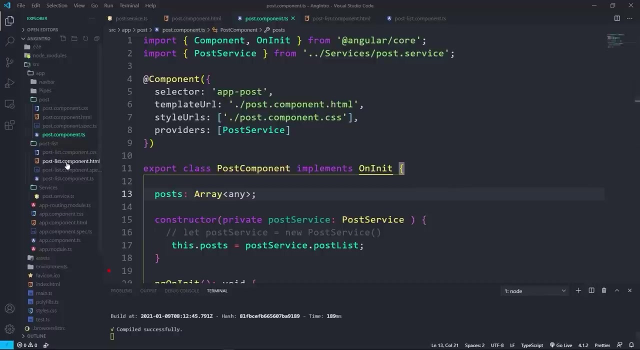 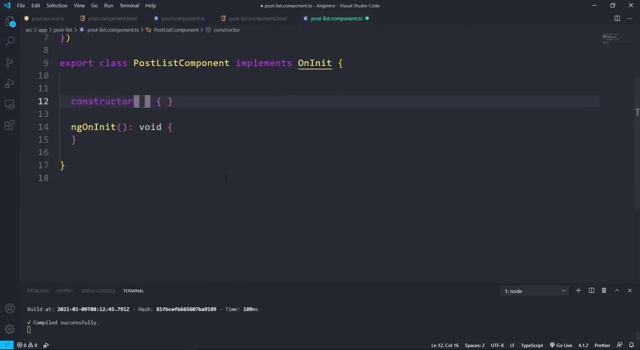 so first let's create a component inside the terminal ng g c post list and hit enter. now i want to access the service post list array from this component. so first we have to inject the service class to this component, so private post service, and this variable type is service class: post service. 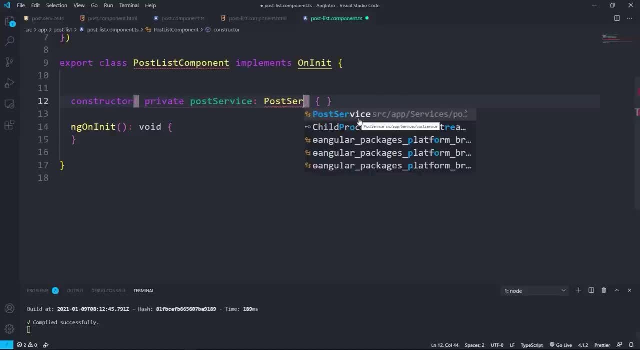 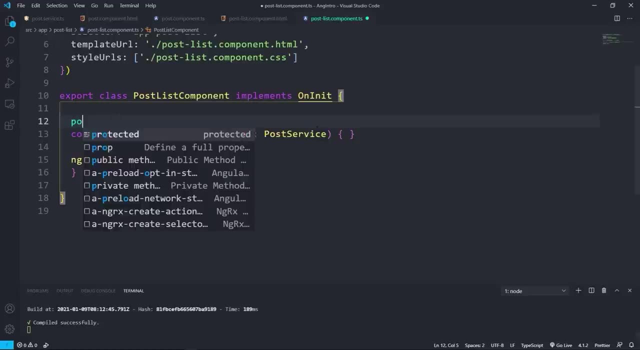 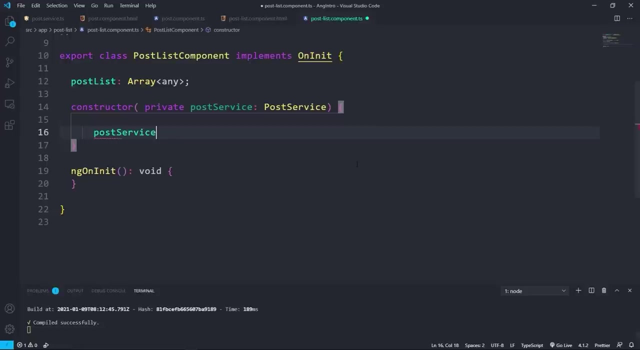 now select this from the autocomplete, which will automatically import the path of this service class. let's create a global variable post list and set this data type to an array and array type to any inside the constructor method. get the post list from this service post service dot post list. 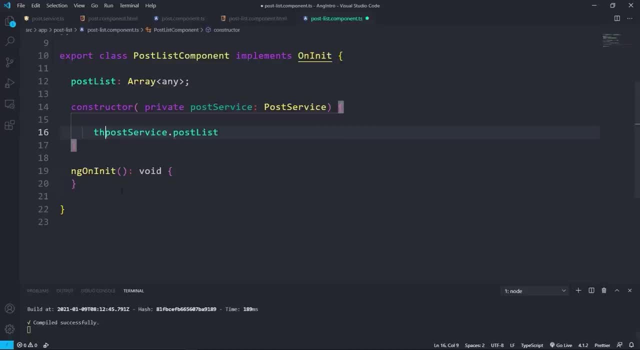 assign this to this global variable post list. now save this. now go to the post list html file. let's render this array to the view ul with li tag. inside the li tag ng for directive. the statement is: let post of post list inside the li tag show the post title. 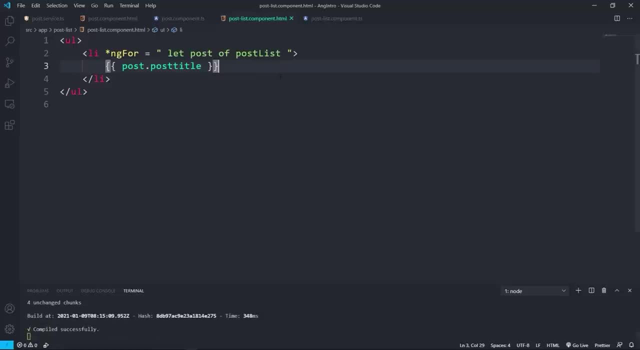 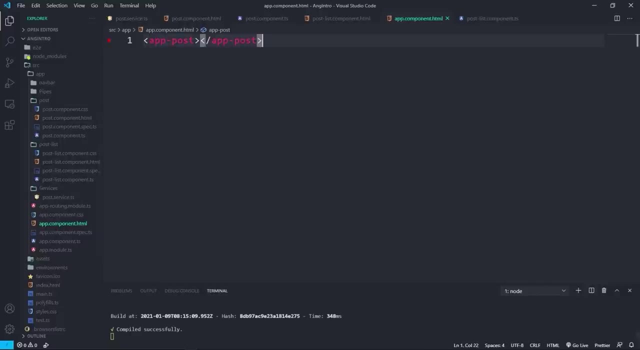 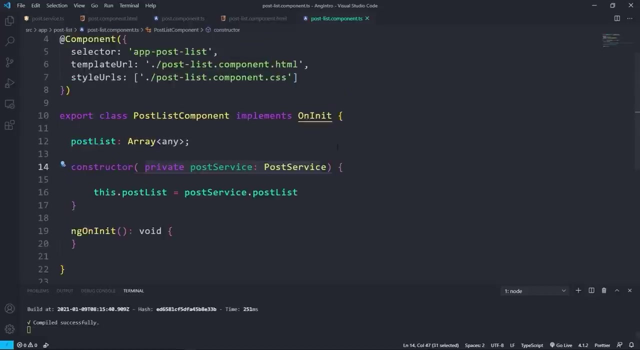 in order to show this inside the browser, add this to the app component. inside the app component html file, add this apppost list, save this and back to the browser. this time also, we got this null injector error. why is that? because we did only the injection. we didn't provide the injector class, so we have to. provide the injector class and we need to enter to the injector class and in the file list we also have to Text News: estado c- testimony to local browser or window. as the file list will be created, it will be in a later version, when the information that we collected here will be posted sooner or later. so don't forget, thanks for watching and I will see you in the next part of this video. See you in the beautiful future. Bye, BYE for future videos. Bye, bye. 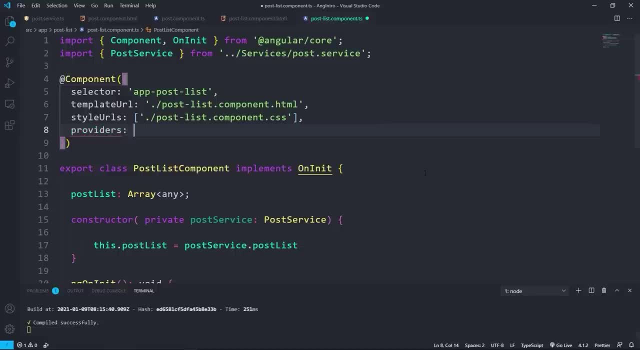 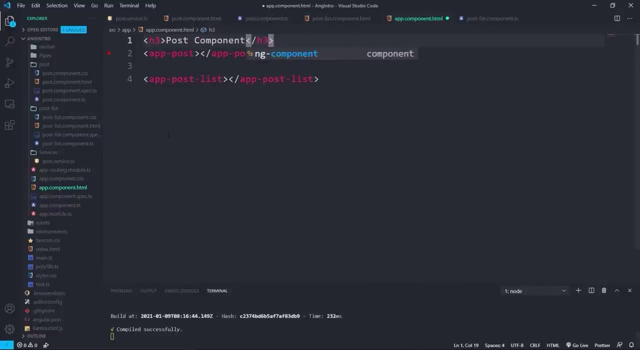 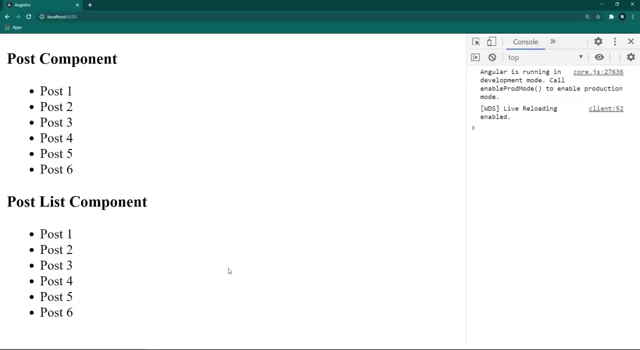 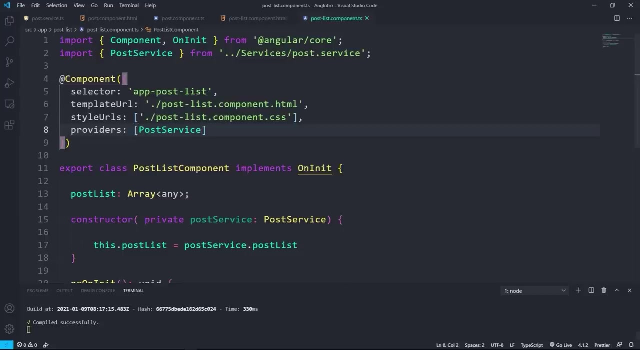 to this component as well. So insert the component decorator provider and this service class is postService. Save this and back to the browser. We got this postList. One is from the post component and another one is from the postList component. So let's see what is happening with this provider By passing this to this component decorator class. 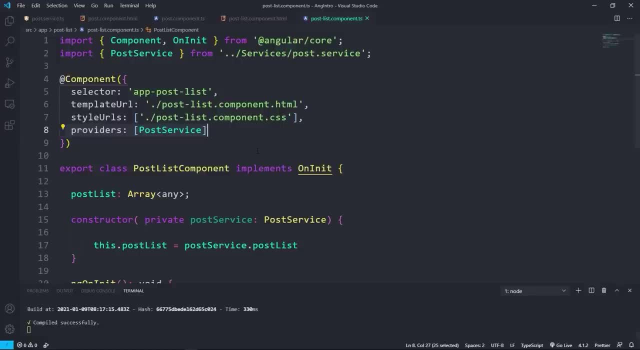 we are telling that to Angular to create this class new instance only for this component. So that's why we got an error when we accessing the service class from this second component postList. So we add another provider to this component decorator as well. So with this two 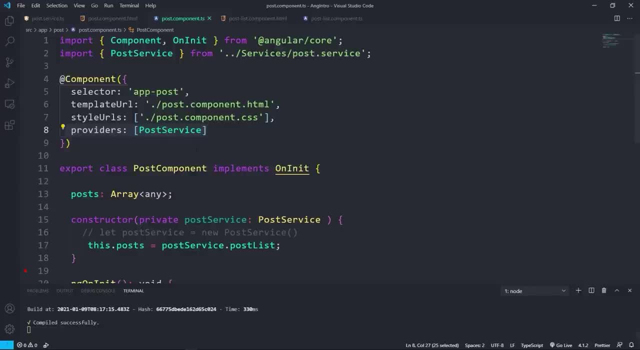 providers. we created one two new class instance of the same post service class and this time we got only two components that injecting the service class to components constructor. So for this situation this is okay, but think in real words we may have hundreds of components that injecting the same post service. 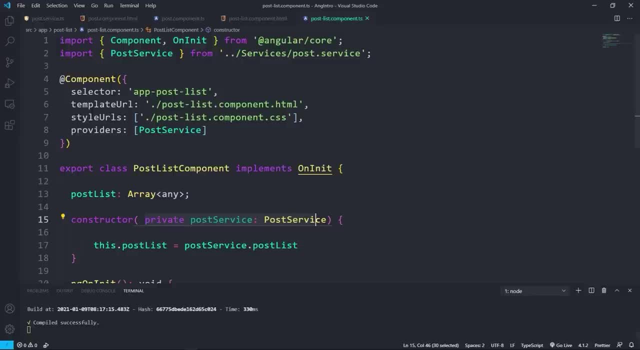 class. So in that case, if we use the provider in each and every components decorator, this will create hundreds of same new class instance for the data service class in the memory. So this will reduce our app speed and this may reduce the entire computer speed. 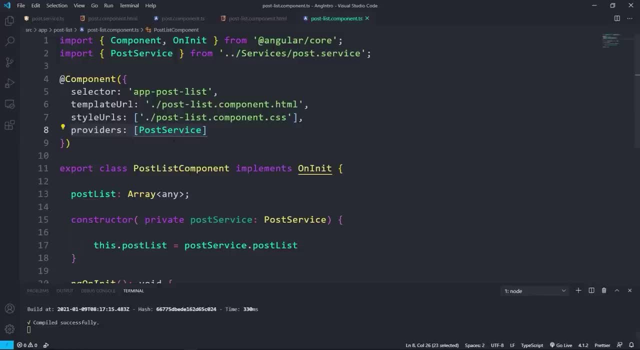 So this is not a good practice. If we're using this post service only for one or two components, this is okay, but in a real world app, we use angular service as the main data repository for all our components, No matter how many components are there. To solve this, we have two solutions. 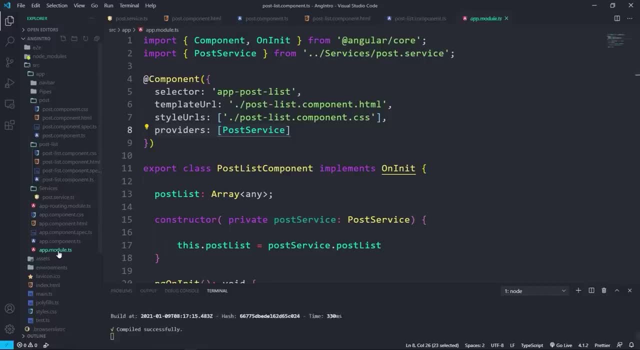 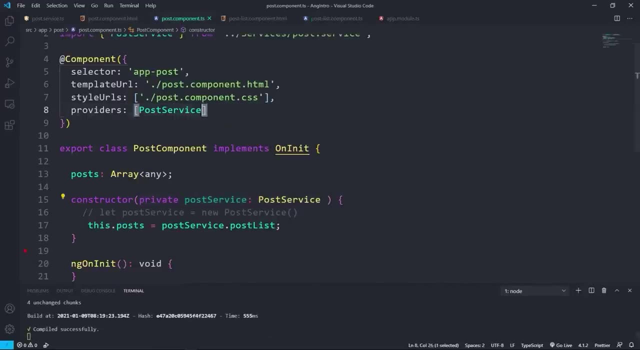 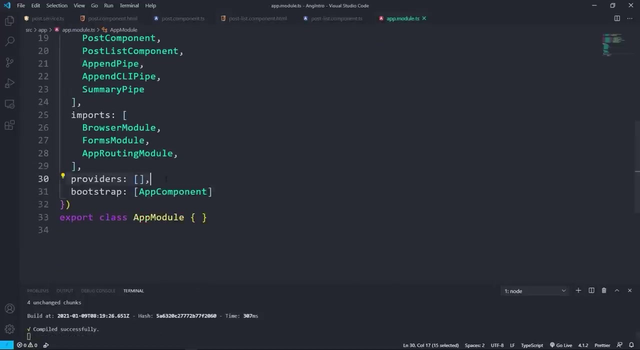 One is: we can provide this service class inside the app modules. So let's see this in action. Remove this- both providers- inside the component decorator. Inside the app modules file we can find this provider parameter inside this ng module decorator. So inside this provider array, pass the service class name that we want to inject to the 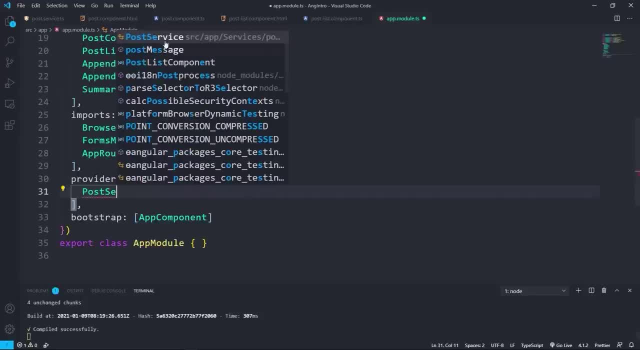 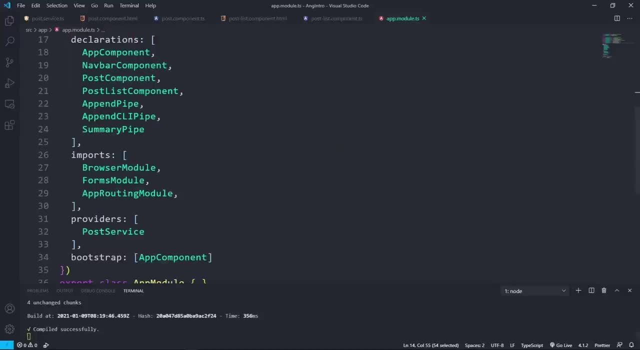 app module. After that we'll set the parameter by the corresponding class and after that we'll set the parameter to the set class name. To do this, if we want to import this service class, we'll do a quick test here. So let's do a quick test here to see what happens. 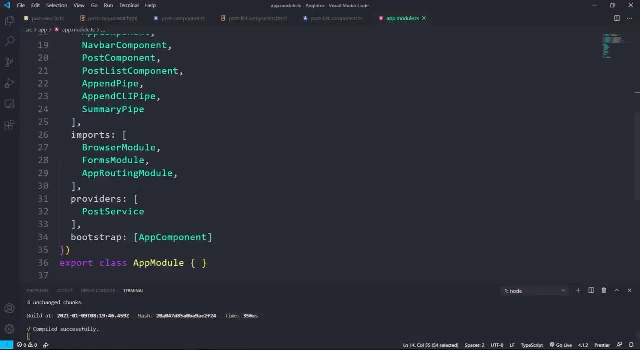 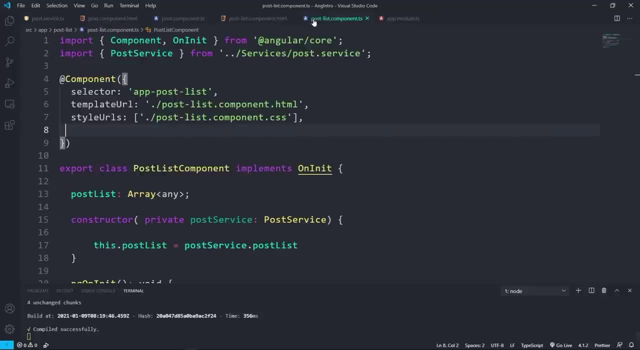 If we want to import this service class from the app module. Let's say we believe that this app module is the best service class available for the app module. So let's say we do a check and we will see what happens inside our app module. 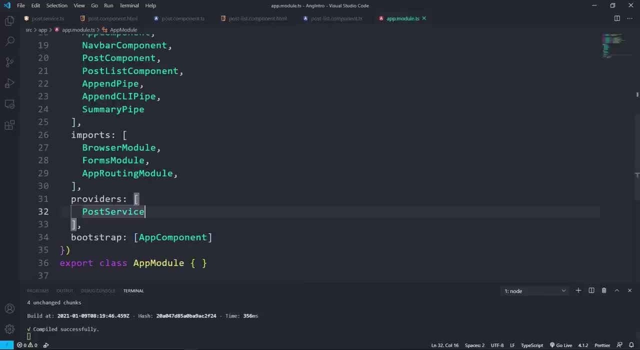 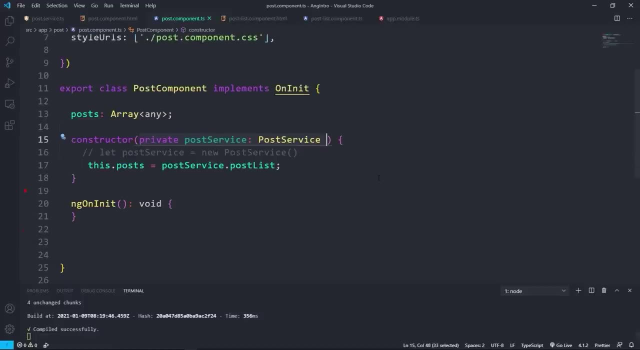 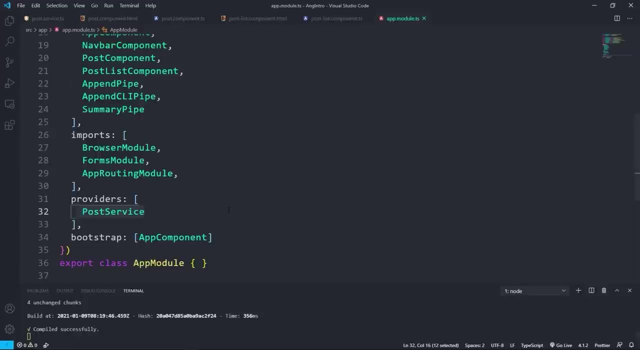 So after that, we're ready to export this service class to the app module, this service class to a component constructor. this will only access this already created new instance. no matter how many time you are injecting this service to many components, This will only create this service new class instance in the memory once. 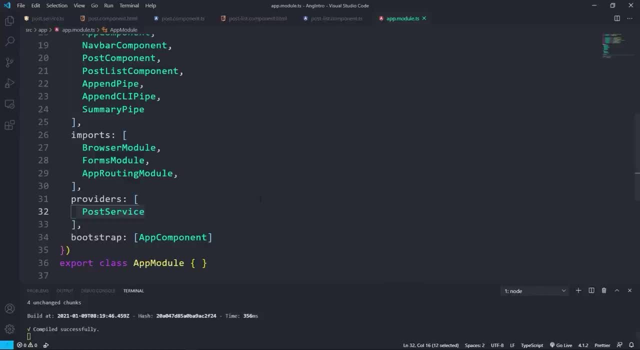 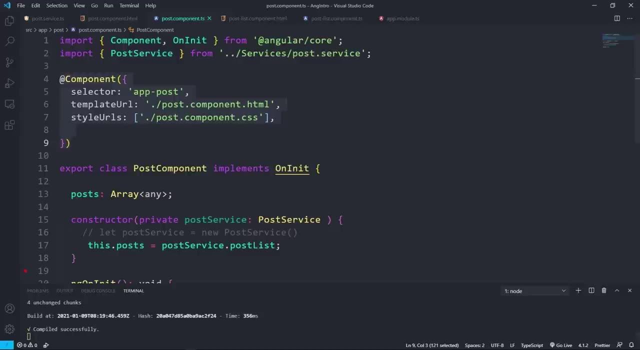 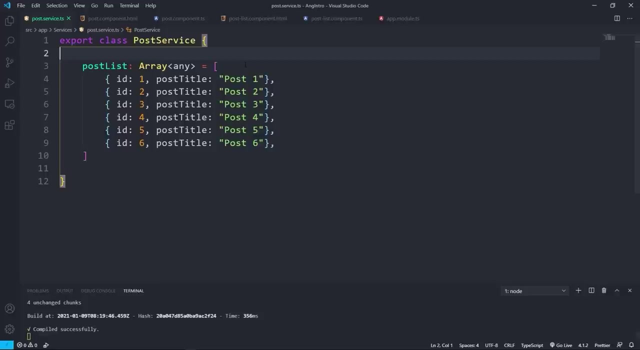 So this will make our angular more efficient. Alright, the second method is: in angular we have an injector decorator for service classes, like this component decorator. So with this injector decorator class, we can make this service class injectable for all components. So let's see this in action. 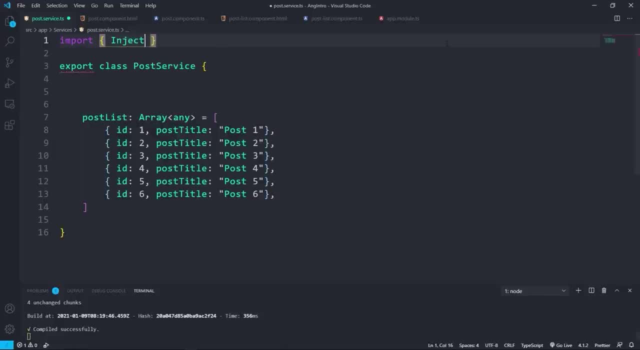 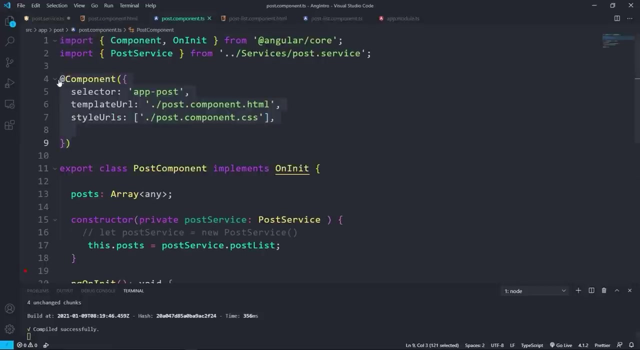 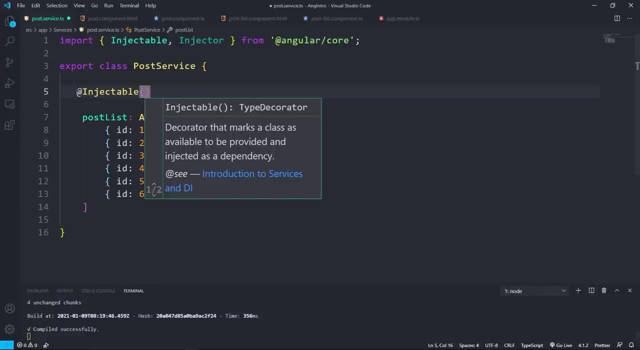 First import the injectable to this service class. this I is capital and this decorator is coming from the angular. go After this: Like this component decorator At injector parenthesis. inside this parenthesis, pass an object parameter. The key is provide in and value is root inside quotes. 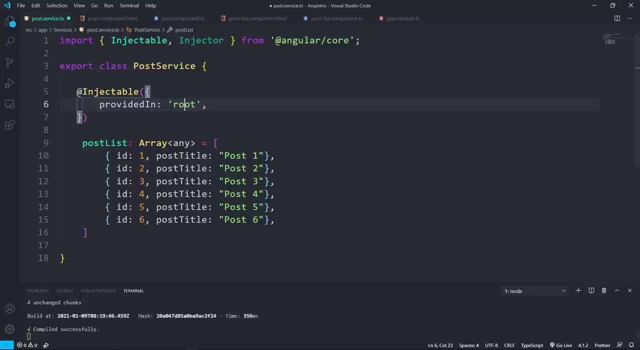 With this, we are providing the service class as an injectable for root app, Which means we can inject this service class to any components in our app without creating a new instance for each and every component. So this is what happens behind the scenes when we creating the provider. 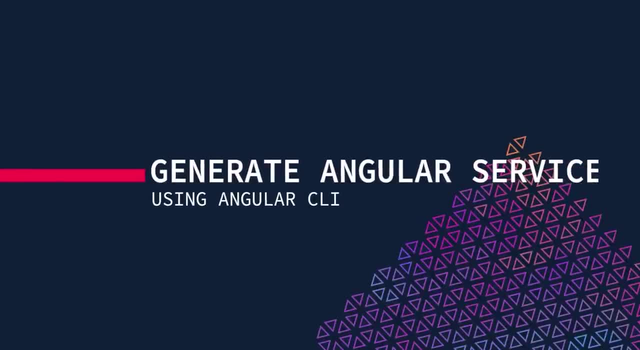 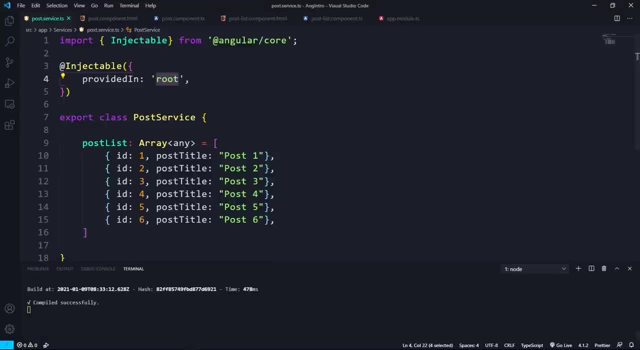 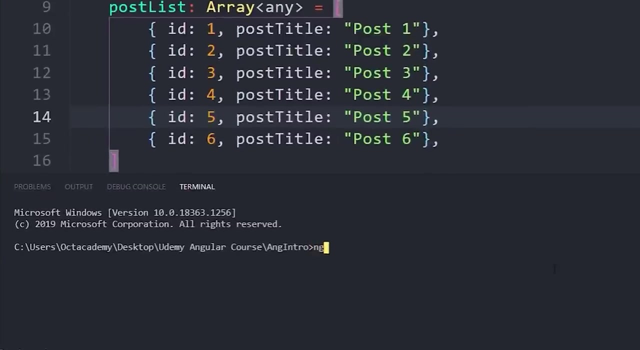 Hope you guys got the idea. Alright, we have successfully completed the hard part. now let's do the easy part, which is creating an angular service using the angular CLI. So let's see this in action. Inside the integrated terminal, run this command ng: this ng is for angular CLI g. this is 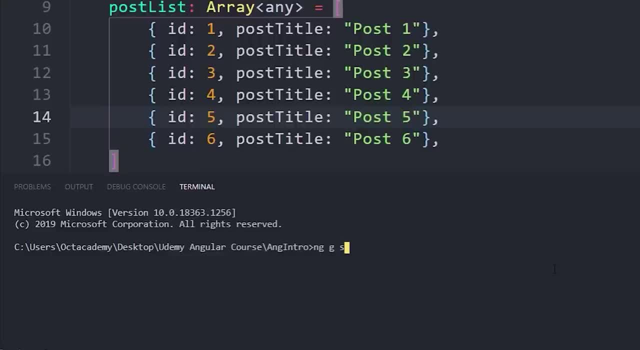 for the generate and s this is for the service, We will put all the angular services inside of one folder, So folder name is services slash and the service name is: this time let's create service for user service, So service name is user. 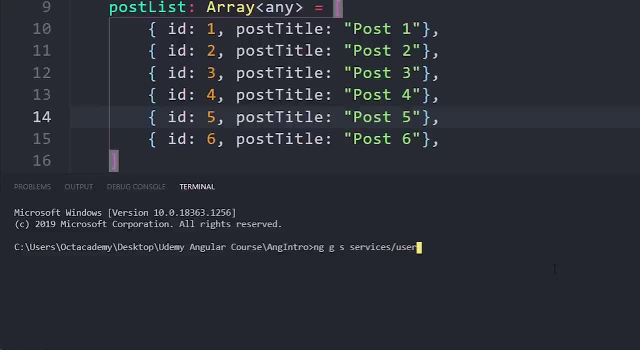 Note this. I just only add this service name. Note the naming convention. like this: userservice Angular CLI will automatically add the service. So that's it. Hit the enter to execute this code. Perfect angular CLI generated these two service files for us: this servicets file and this. 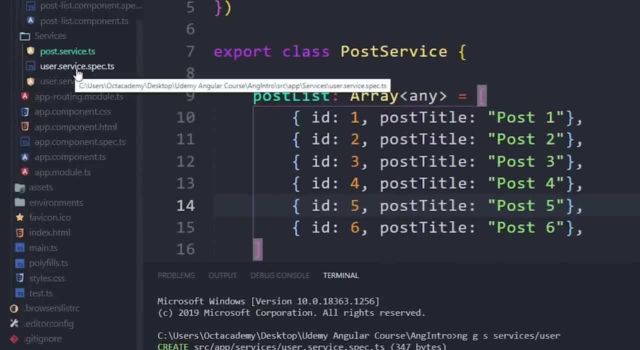 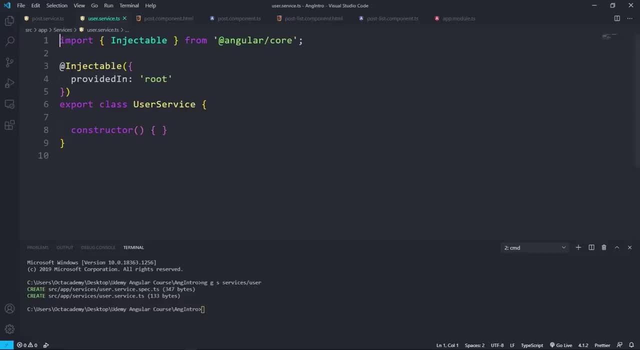 spec file, which is for the user Unit testing. Inside the service folder. we got this userservice file open it. look at this. In this service. this automatically added this injectable decorator, So we don't have to do this again. 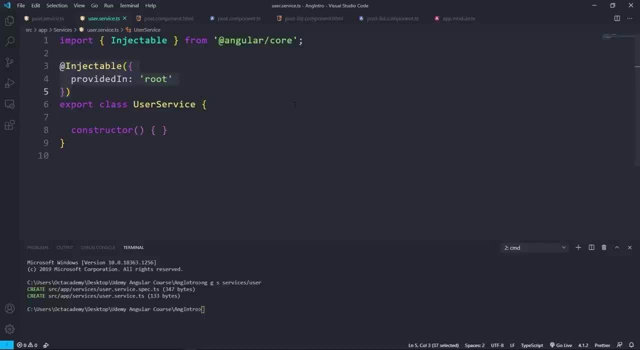 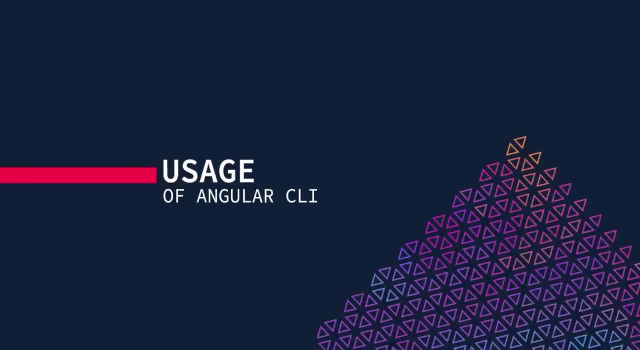 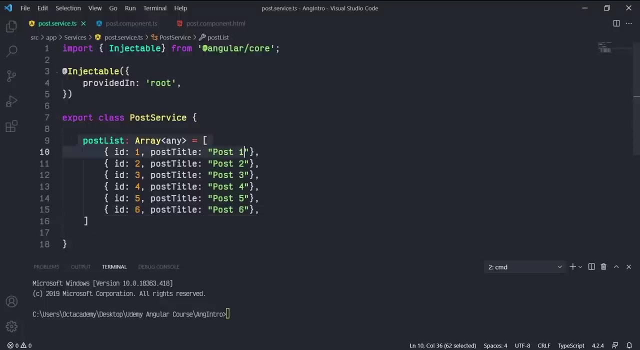 So this is the beauty of angular CLI. So this is how we generate angular service by using the angular CLI. So throughout this course we will use this angular CLI method to generate service. So let's see how we generate angular service. So in here we got this post array and inside this we got this object list for post. 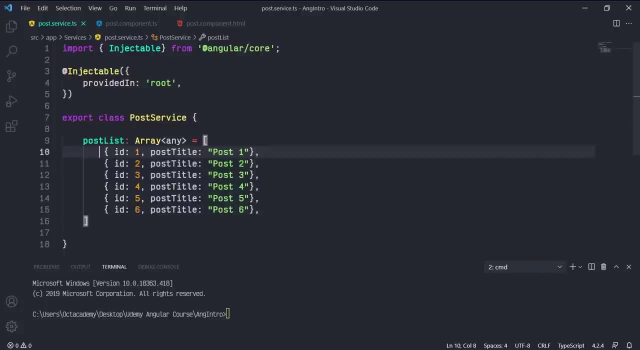 In this object we have these two key value pairs: id and this post title. So let's push a new data object to this array when clicking a button. If you can remember, we did this when we learning angular directives, right? Ok? 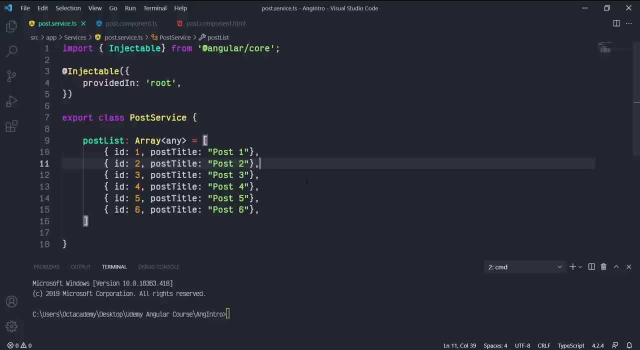 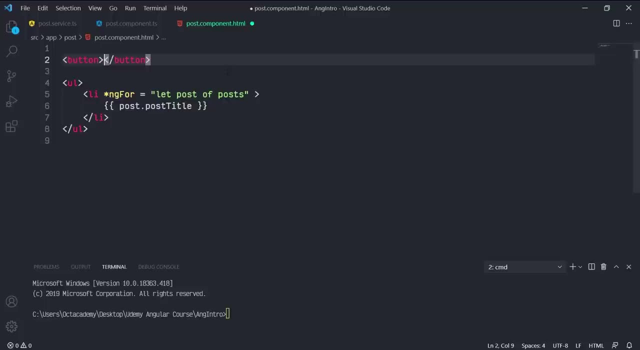 So let's do that again. So inside the post component file, create a button before this ul tag Button and hit enter. Button text will be addNiv. Now I want to call to a method: when clicking this button, something: addNivData. 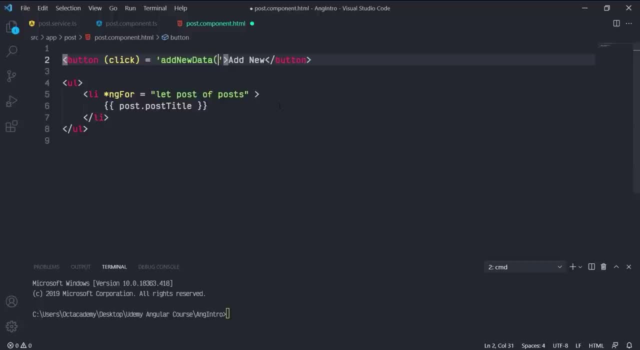 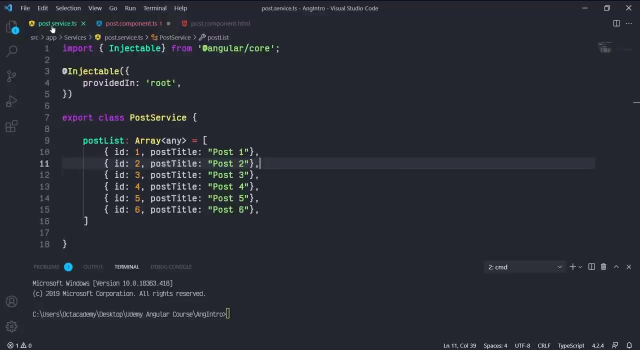 Don't forget to add the parentheses after this. So now create this method inside the post componentts file AddNivData. Inside this create the new object. So let new post assign and the object scope. So first key value pair is id and we already got 6 post inside the array. 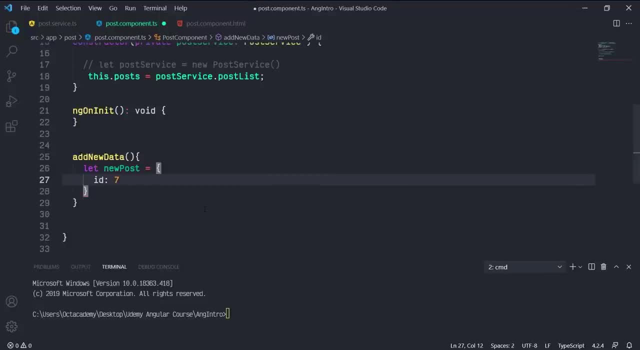 So set the id value to 7.. Next key value pair is post title and value is post 7.. Now I won't push this object to this point, So let's push this object to this post list array which is inside this service file. 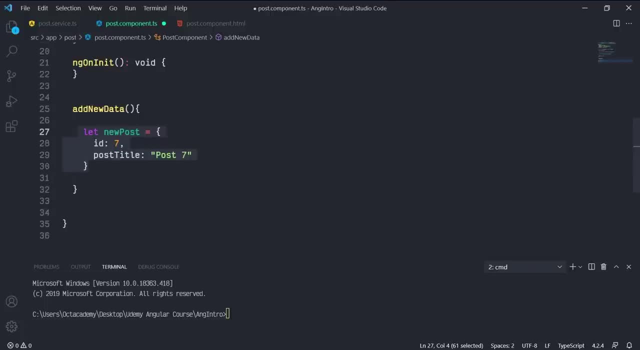 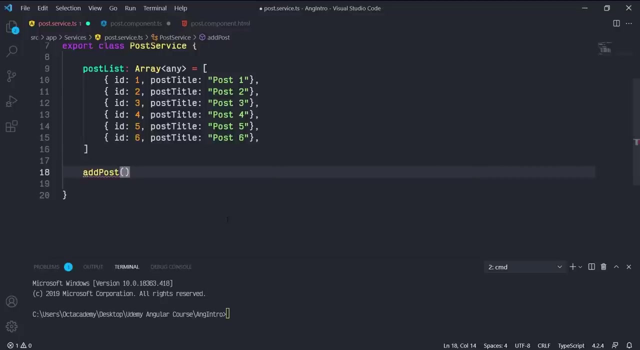 In order to push this data to this array, we have to pass this new post object to this service. So very simple. Create a simple method inside this service file, Add post and parentheses. With this parentheses capture the new post object as a parameter for this method. 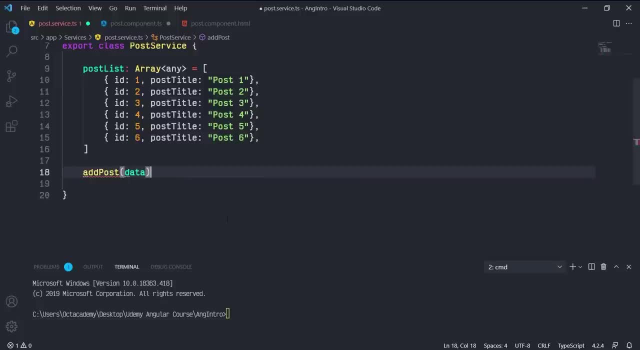 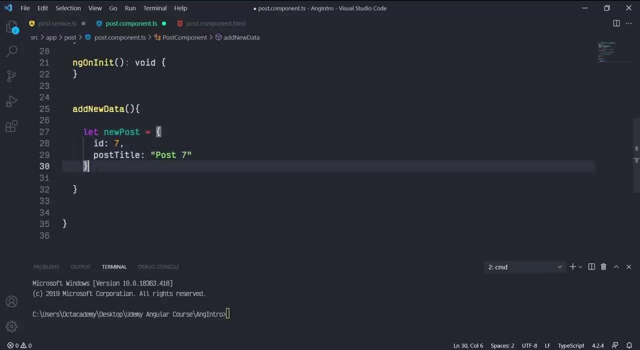 So I declared the parameter name as data Cause we gonna add data. We're gonna receive data from this At last. don't forget to add this method scope. Alright, now from the post component. pass this new post to this and post service method. 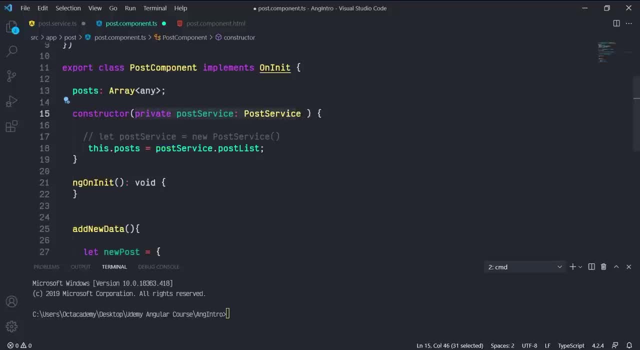 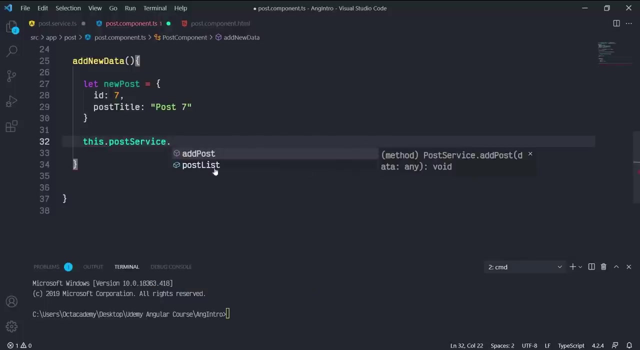 We already injected this service to this component, which means we can access all the methods and properties of this service from this component. So, post service Insight. we can find this addPost method, So select it. This required a parameter, So pass this. 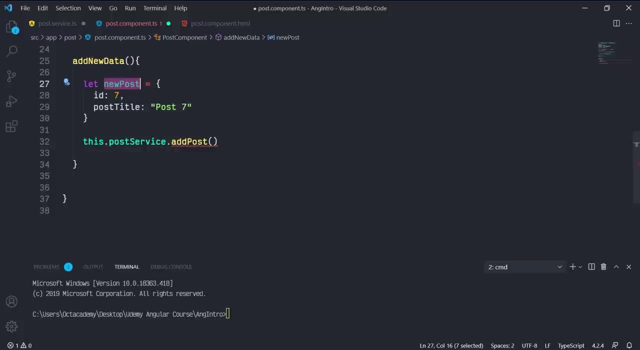 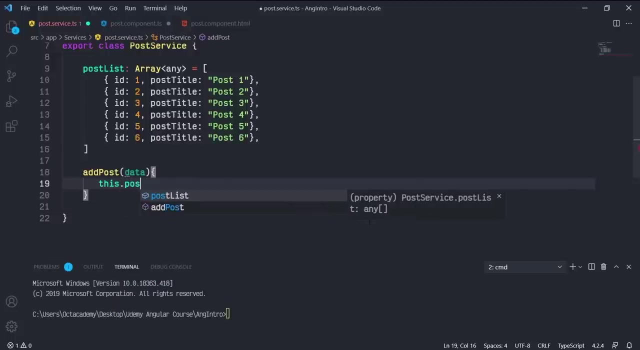 new post object as a parameter for this addPost method. So now we are passing the data to the service from this service method. So now let's push this data to this postList array, ThispostListpush, inside brackets. pass this data parameter variable, which is coming from the post component, That's. 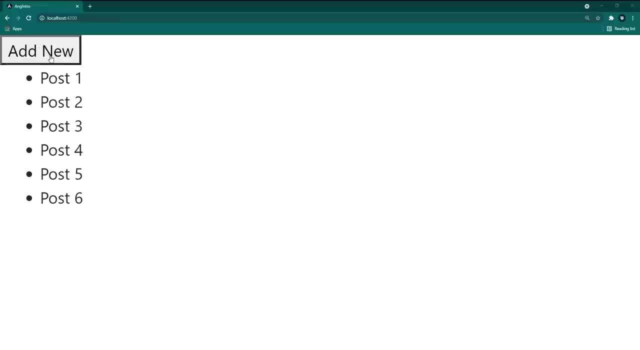 it. Save this all and back to the browser. Click this. add new button. Perfect, As you can see here, we got this new post inside this unordered list, Which means this data is successfully pushed into the postList array which declared inside the service file. So this is how we manipulate. 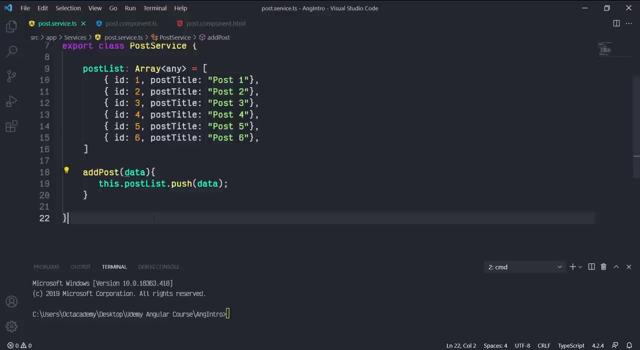 this data. So let's see how we can manipulate this data. So let's see how we can manipulate data using this service file. Usually, we do all the data manipulating, such as loading data, save data, delete data- inside one place, which is inside the angular service file. So this 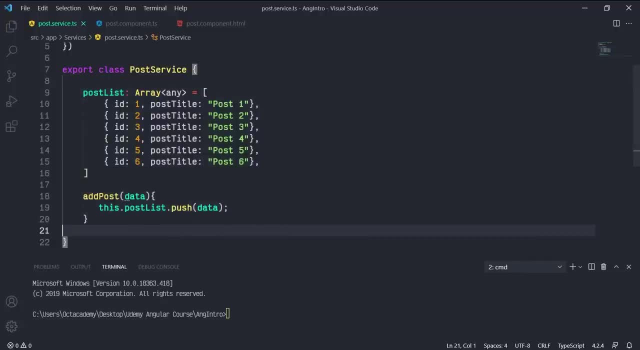 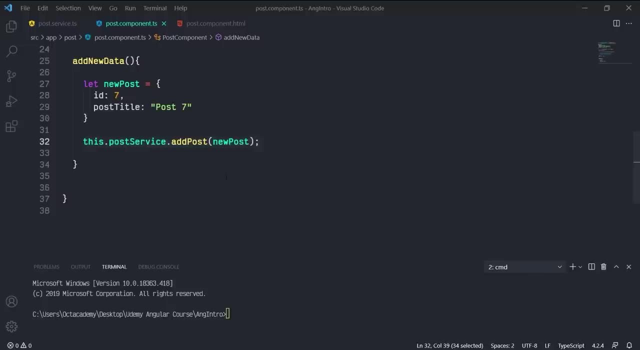 will give us the more cleaner and bug free coding experience. So we added this data to this service postList array. When we click this button, Think if somehow I missed spelled this post title key to something like this Post title with one T character. These kinds of human errors can happen more often, right, So save. 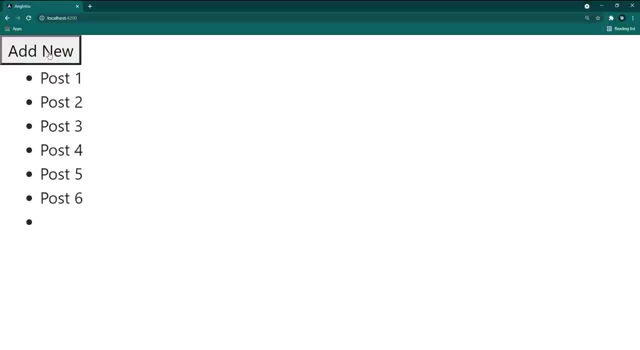 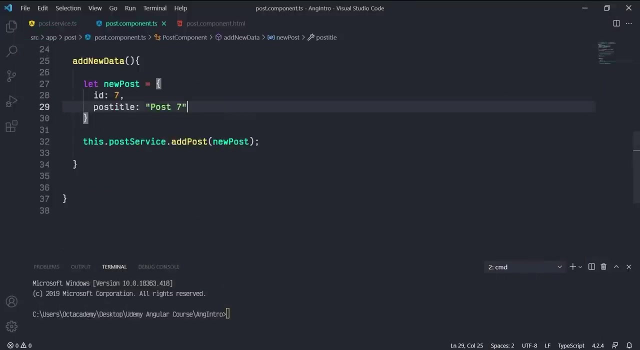 this and back to the browser, Click this add new button. Look at this. This time we got an empty list, So click this button again. We got this empty list again. Why is that? Because we know already we made a spelling mistake here, So with this add new, we pushing invalid data to this postList. 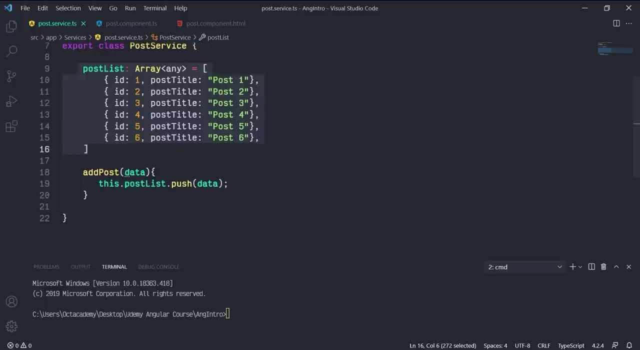 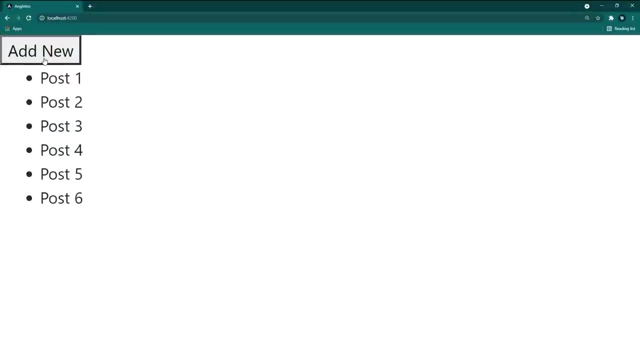 Wait, let's log this array. So inside this postService after this push method: consolelog thispostList. Save this and back to the browser. Click this add new button. As you can see here, we got this empty list. Now open the browser console. 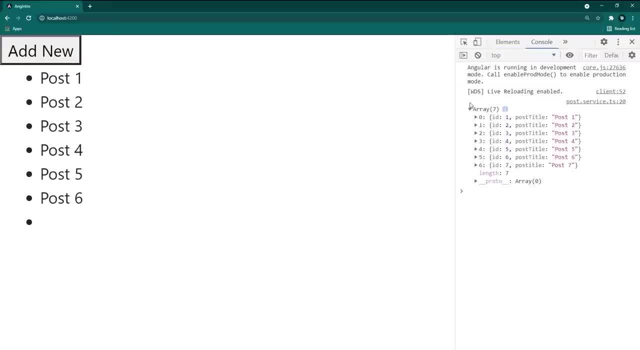 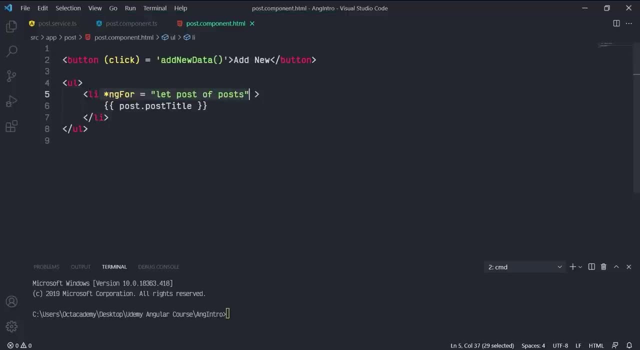 Look at this last object. This object post title key is not spelled correctly. So we rendered this list of post using the angular ng4 directive And we rendered this post using the string interpolation. So with this string interpolation we are showing this post title key's value, which has two T letters middle of the key, Not this spell mistake key. 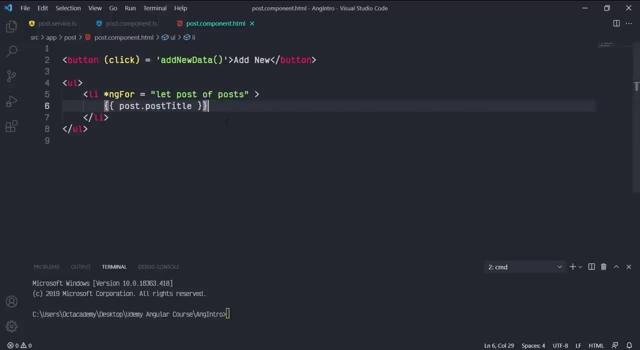 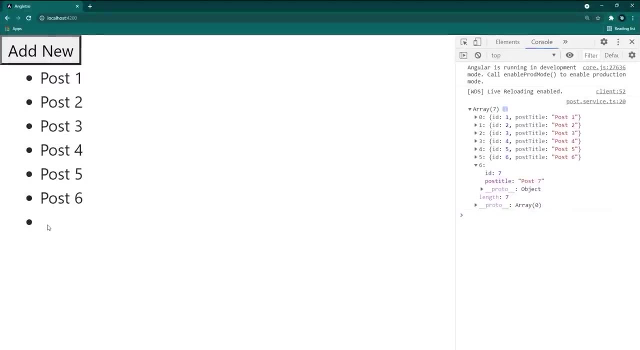 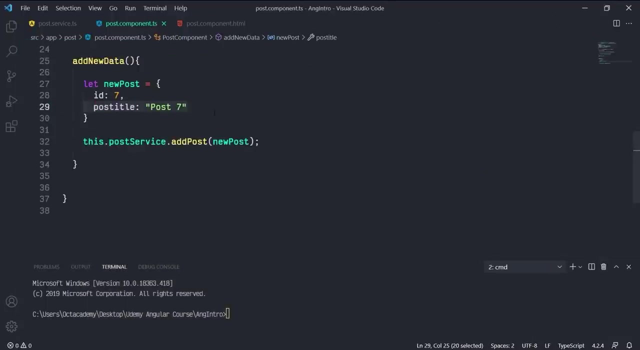 So in this case there is no valid key post title. Therefore, this string interpolation left this empty. That's why we are getting this empty list For this example. we know the error Because we intentionally did this spelling mistake. Think in a real world app. we don't push data to the arrays. 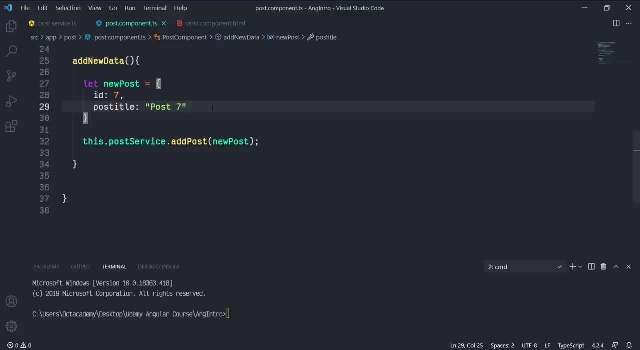 We save data inside the database Somehow if we missed anything at the beginning, can't even imagine right To solve these kinds of problems. we can create a blueprint of this array object by defining the shape type of the object And we can set that blueprint to this new post object's data type. 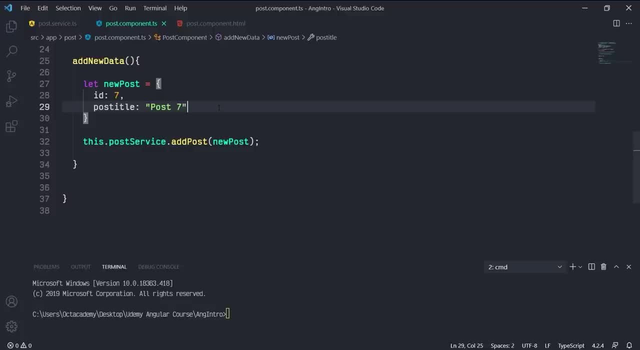 Then if I mistake anything, this will show me an error. From that I can identify the error before anything goes wrong. Alright, let's see this in action. To create the blueprint of this object, we will use a TypeScript interface. Generate an interface using the angular CLI, So inside the terminal, type this command. 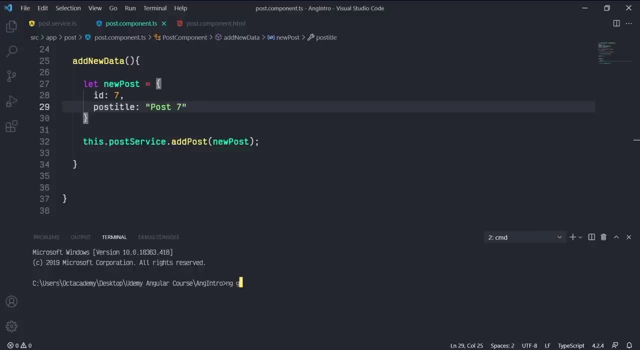 ng g, You guys already know, and this g stands for generate And i this stands for interface. I will put all interface inside of a folder called models. So the interface path will be models slash interface name: post. That's it. Click enter to run this command. 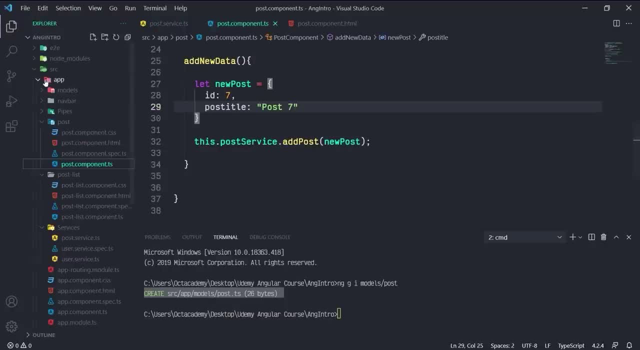 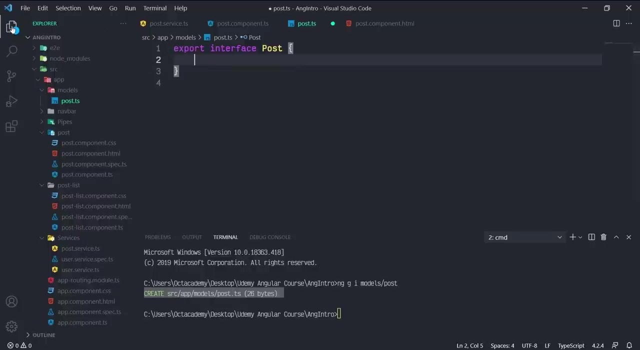 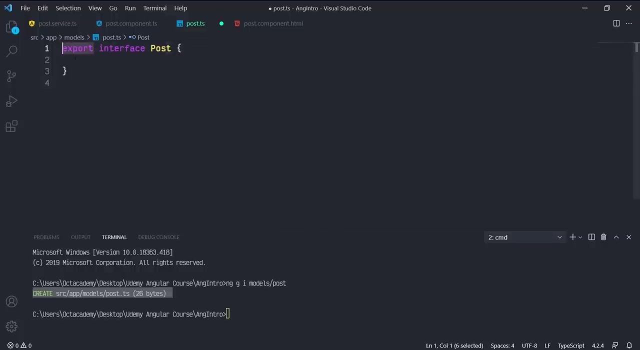 Perfect, We generated the interface successfully. So inside the app folder we can find this models folder Inside that we can see this newly created interface post. Now open it. So inside this we can find a simple markup for TypeScript interface Interface keyword and the interface name. So we're going to access this interface. 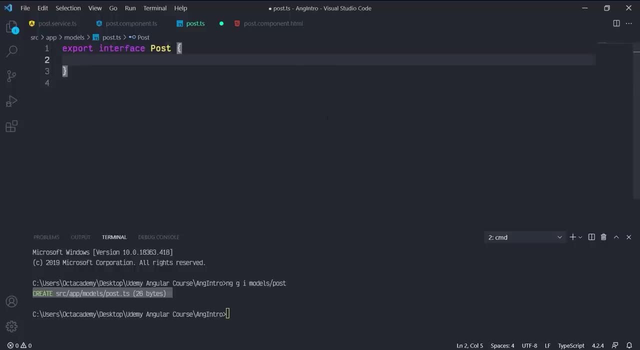 case name is not enter. Second, we will import a file- scripts file- and this type script interface. Next, we'll import a file coming from outside of this file. That's why we use this export keyword. This is just a simple TypeScript interface. Inside this we can create: 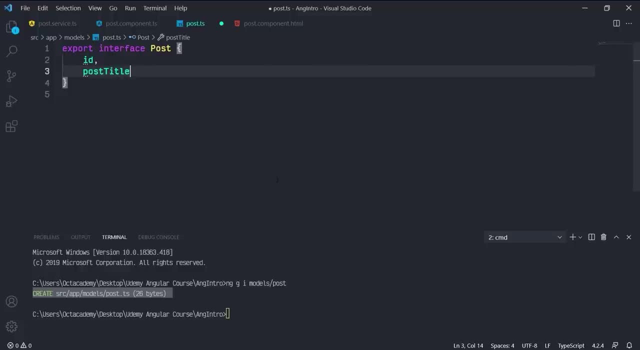 our post object's blueprint. So first we have the ID. After this we got the POST title. Save this. Now go to the post component es file and make this new post data type as this: First we have to import the post interface to this post component. 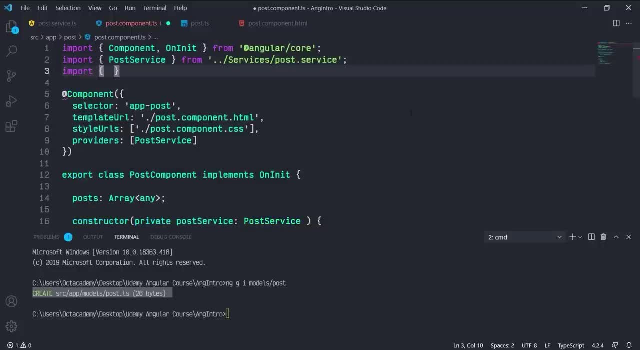 At the top of this page, import inside curry brackets. the interface name is post. After this from: and the path inside quotes: go back one folder. double dot slash models and this: select this interface post Now. add this post interface as this new post data type. 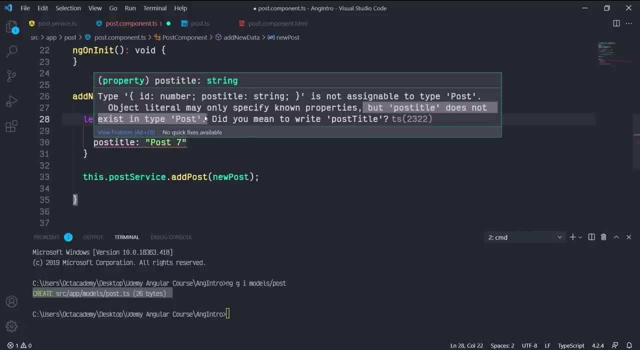 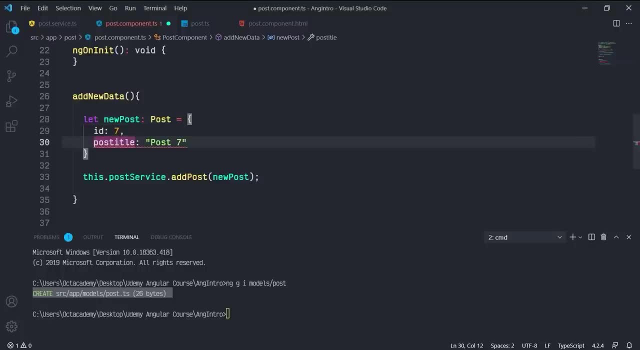 Perfect, If you see this carefully. now we are getting this compilation error saying that this spelled wrong Post title does not exist in the interface post. So this is the beauty of this interface blueprint: If you make any mistake on these objects, you can see. 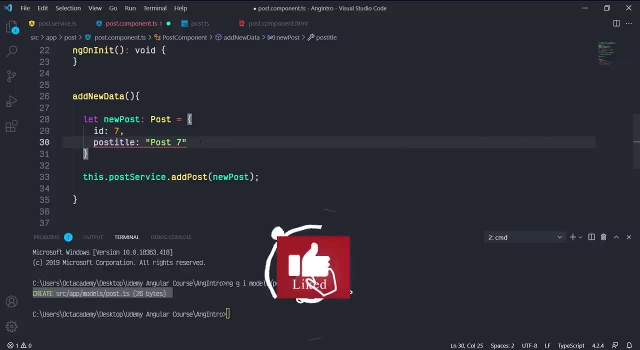 keys. This will give us the error on the compile time, So we can debug this mistake before the runtime. Like this object key name, we can define the types of all the values as well. Let's see this in action Inside the post interface, after this id colon and the 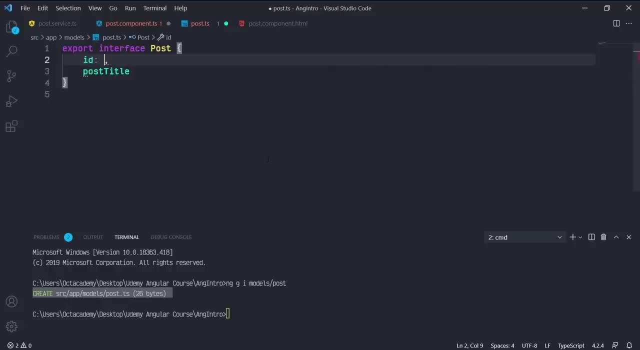 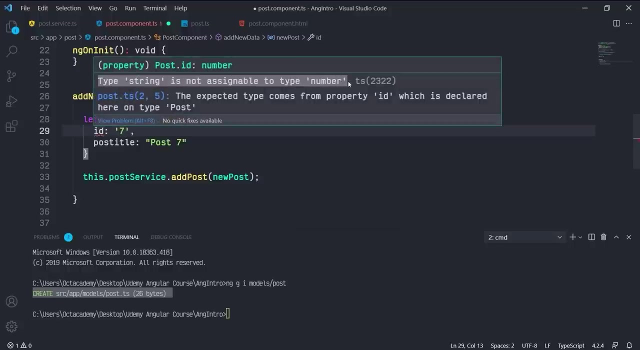 id type is number. Likewise, this post title type is: yes, you are correct, the type is string. Save this and go to the post componentts file. If any case, if I passed a string value to this id, as you can see here, we are getting a compile error saying that type string cannot. 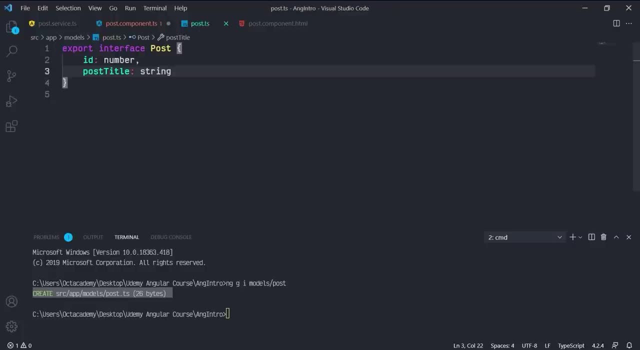 assign to type number. Cause in the blueprint we defined this id as string, So we must provide the correct data to this object value, otherwise we will get a compile error. Wait, not only that, if we forget to add the second value post title at this: 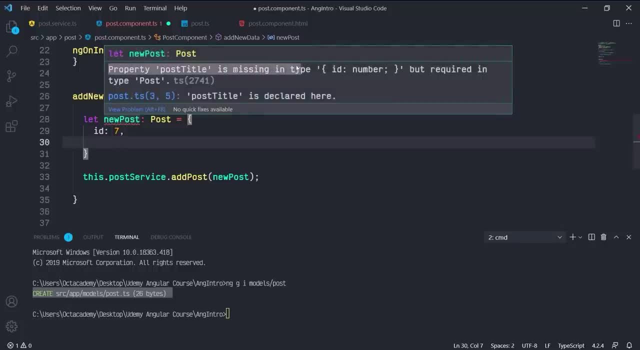 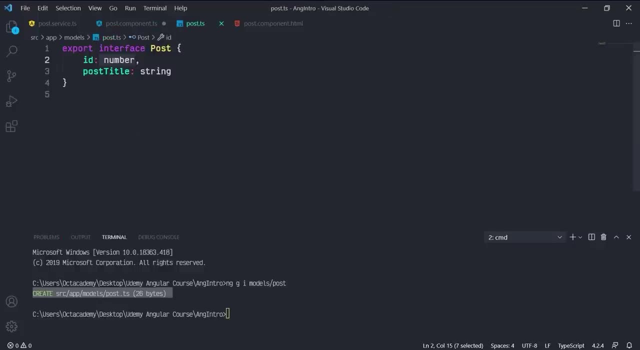 point. also, we are getting an error Property post title is missing And this post title is required. Perfect, right. With this simple interface technique, we can reduce almost every human errors when creating new object. And at last, one more thing: If we define the 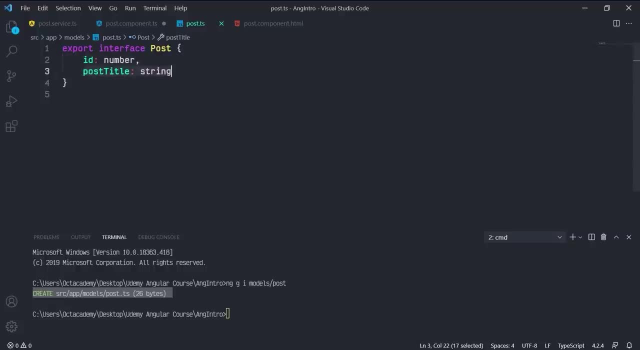 interface like this, these keys become required fields. Think there is a key for a date value and this is optional. How do we going to define that? Very simple, First define the key date and the date type is date. If I go to the component file, 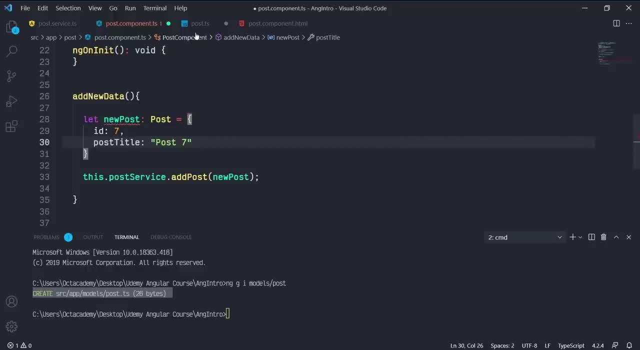 Now we are getting the error saying that date field is missing Cause this is required. now Let's make this date key optional Very simple. After this key name, before the colon symbol, add a question mark Which makes this key or the field optional. So save this and 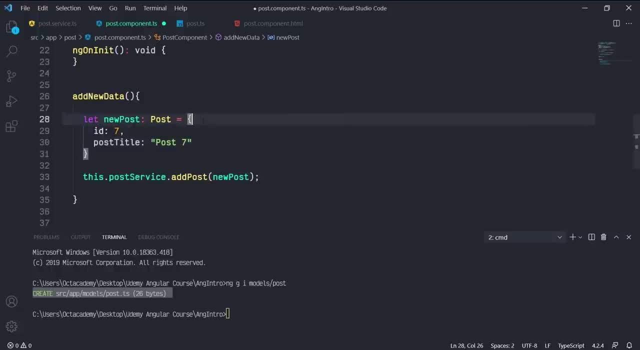 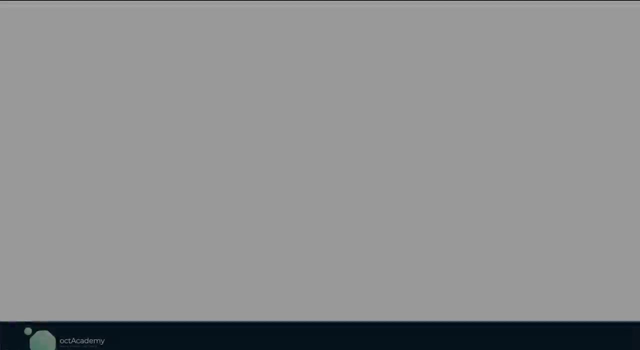 go to the post component Beautiful. Now we are not getting any compile errors, So this is the usage of typescript. So this is very, very useful when we dealing with a database. We can reduce lots of errors with this. Alright, this is it for this angular service section. In this section we learned all about. 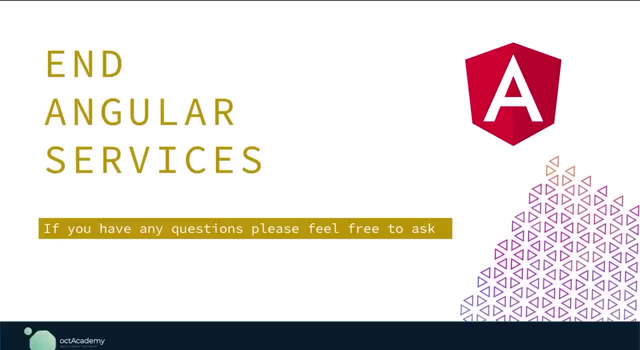 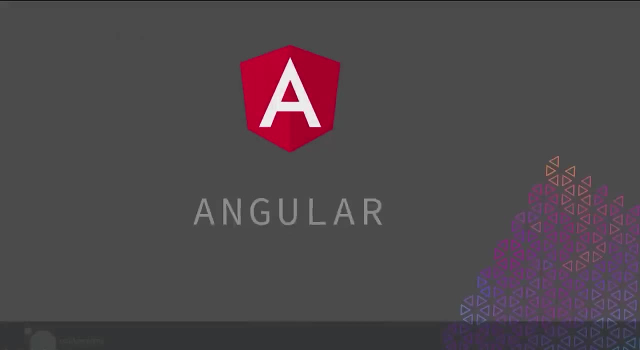 angular services and how to use angular service with our angular app. If you guys haven't any question, please feel free to ask your question in the Q&A area. Alright, let's continue. We'll meet you in the next section. In this section we gonna look at angular template driven form. By the end of this section, you 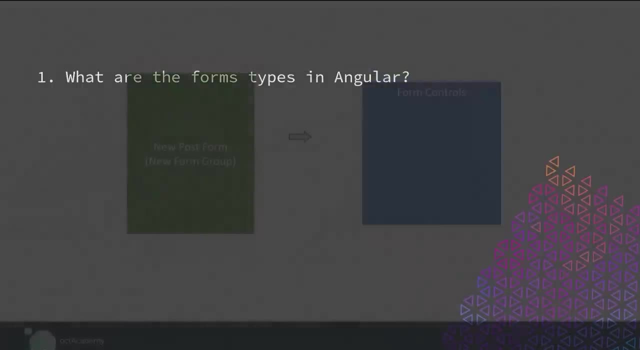 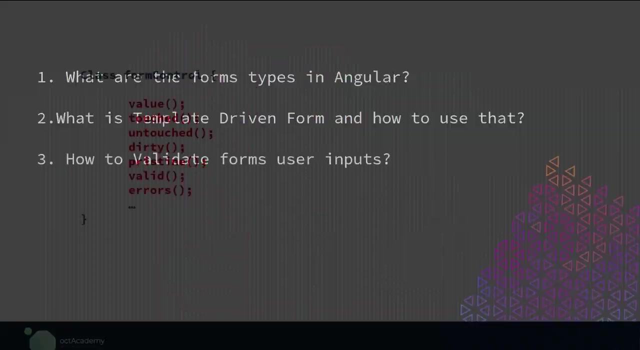 will get to know what are the types of forms available in angular, What is template driven form and how to use that, How to validate forms using the template driven method, And also we learn how to control the disable- enable- state of a button when the form state is valid. 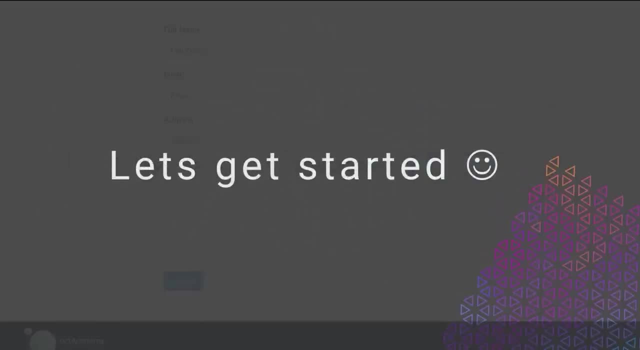 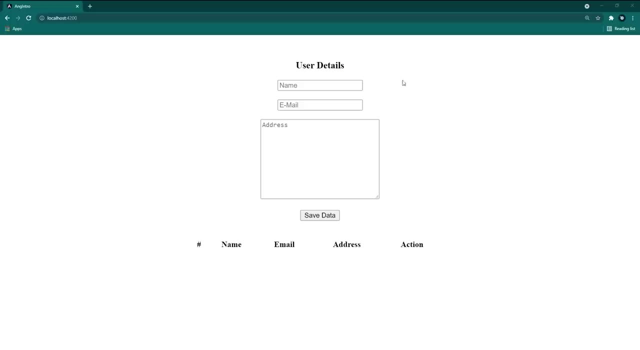 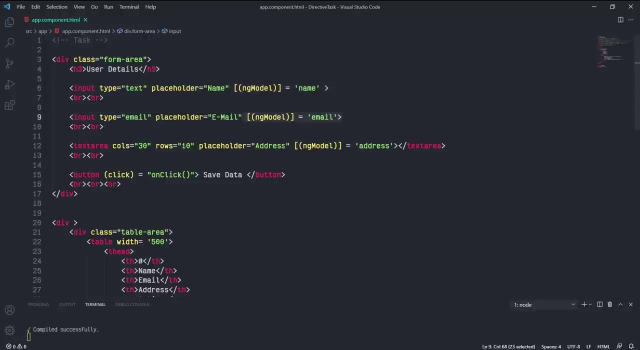 or invalid. Let's get started. In previous, we created this simple form and we did the simple data manipulation, Just adding and removing data to an array. For this we used the two way data binding approach. We not even used the HTML form tag. Actually, this is not a good practice and we don't have 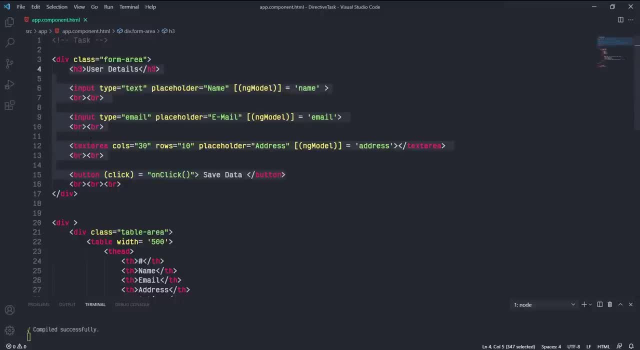 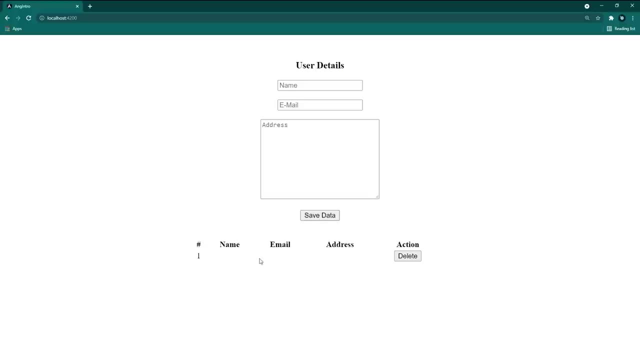 control to add validation for this input data. For example, if I click this add new button by keeping this form empty. Look at this: This is pushing this empty, invalid data to this array. That's why we are getting this empty data inside this table. For a simple example like this: 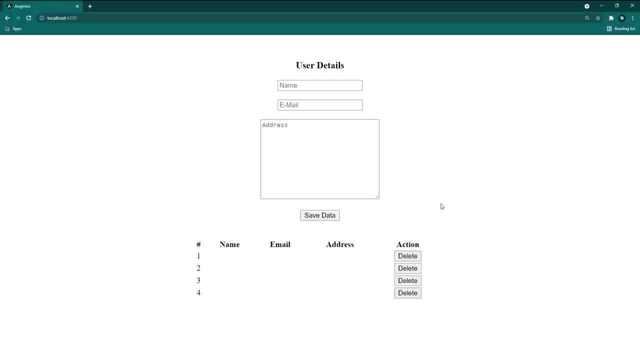 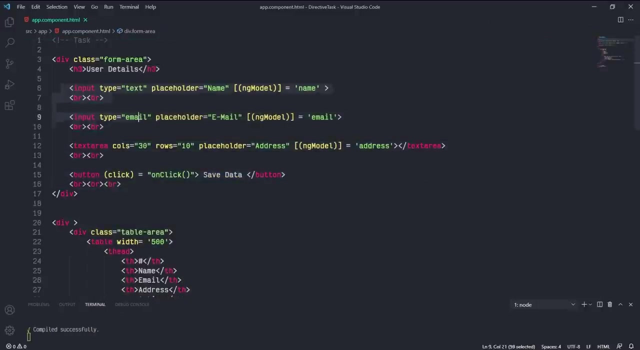 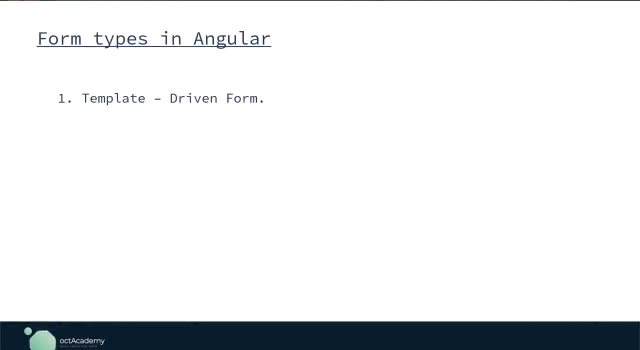 this is okay, but when it comes to a real world application, this is not a good practice And also this is not good for the security as well. So we can not do this form validation part by using only this two way data binding approach. So for this, angular has two approaches. The first one is template driven form approach. 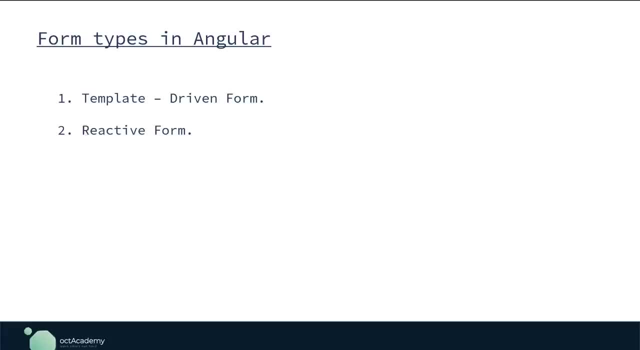 and the second one is the reactive form approach. So in this section we gonna learn the first approach: template driven forms: Haiti, jockey, jockey, jockey, jockey. This template can be- YEAH, I forgot the home. Crap Canada quickly somewhere. 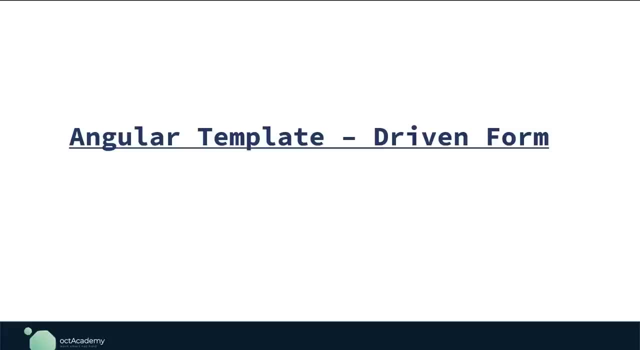 driven form, we can get the full control of the form and we can validate the input data as we want. In the next few lectures we will create a form and we're going to make that form as a template driven form and also we will learn how to do form validation using this template driven 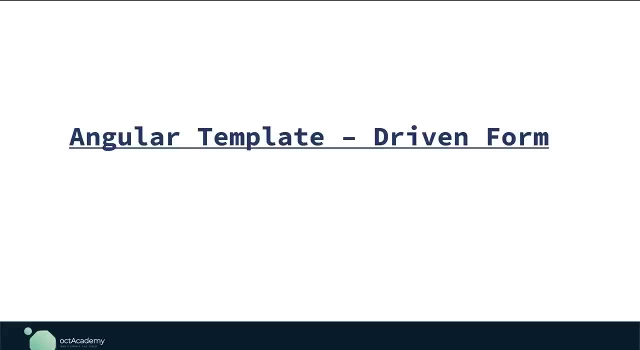 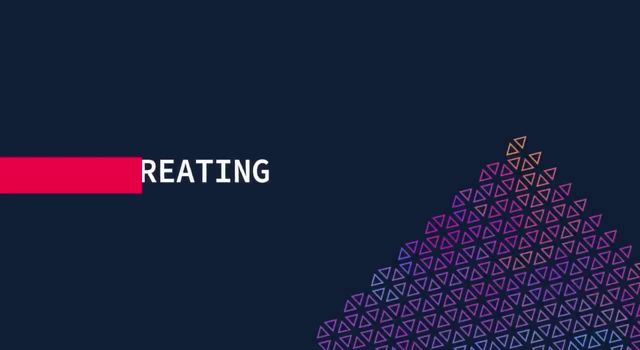 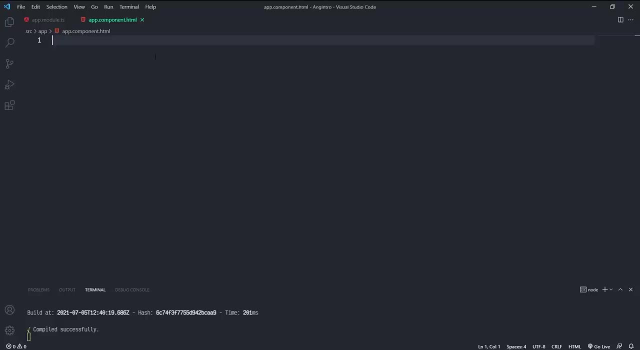 form architecture. This is very easy, so we'll meet you in the next lecture. First, let's create a simple HTML form inside the component HTML file. create a div with class name form dash area Inside this div. when creating a form, we must put all the input fields inside of. 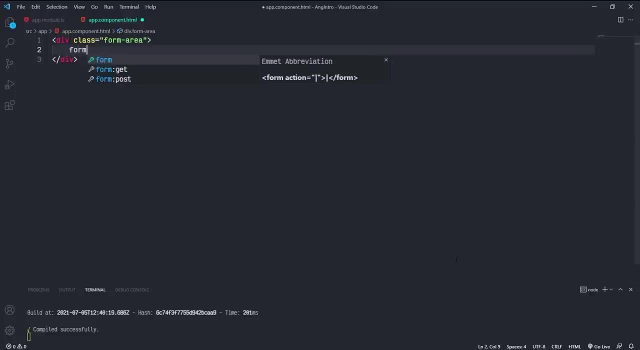 form tag, So form and hit enter. In angular we don't need this action, so remove it. Inside this form, let's add an input field- Input, and hit enter. The input type will be text. This input is for full name, so add a place. 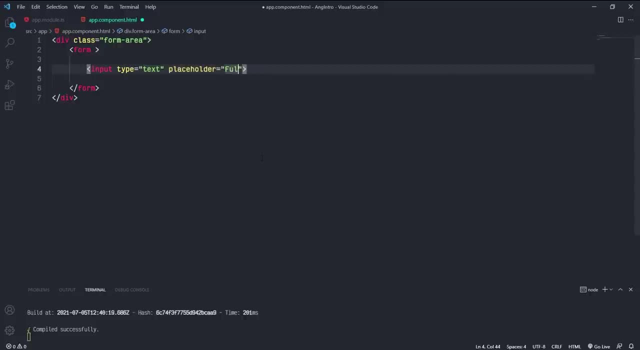 holder for this full name. After this, another input field, which is for email, so this input type will be email- and add the place holder email. After this, add a text area for address- Text area- and hit enter. and don't forget to add the place holder address. 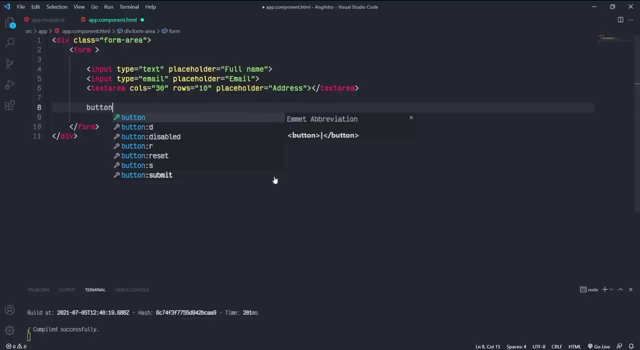 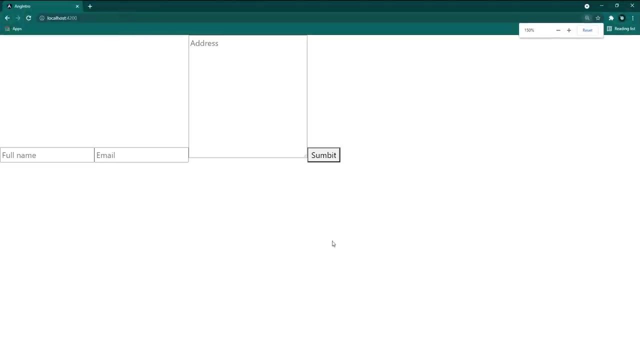 After this, the submit button, Type button and hit enter. The button type will be submit Alright. save this and go to the browser. This is not looking perfect, so let's add some style to this form. For this, let's use the bootstrap css frame. 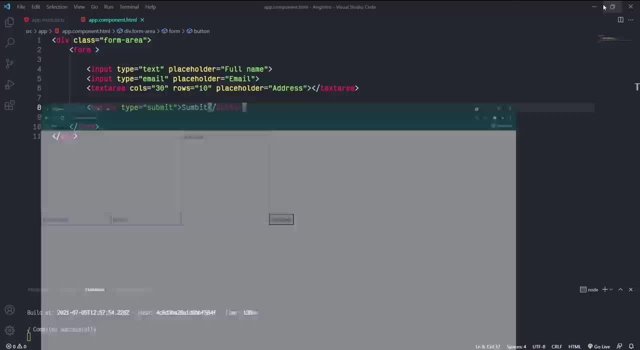 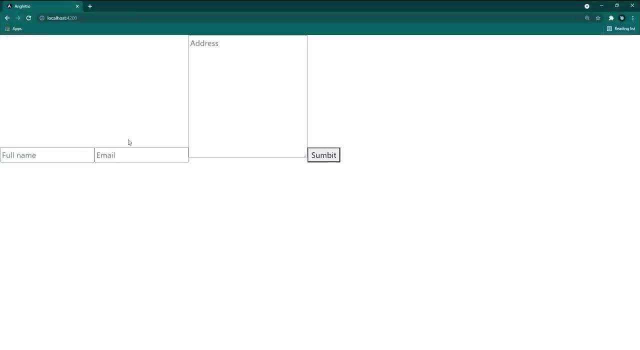 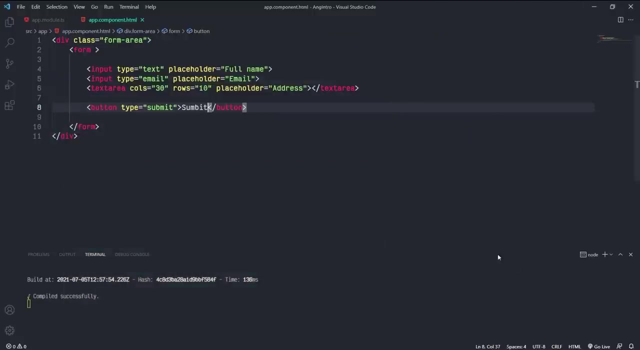 If you can remember, we learned about this in one of the previous section, So in this section let's make this ugly looking. HTML form looks better by bootstrapping this form First. in order to use bootstrap in this angular app first we have to import bootstrap into this angular app. For this we have few methods. 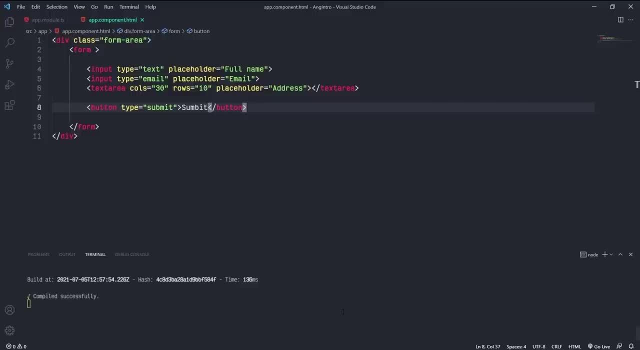 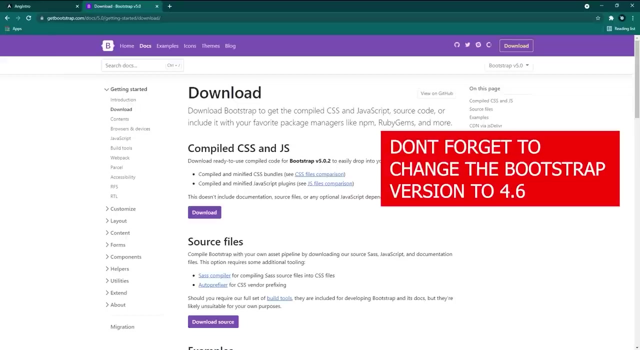 We'll learn about this. For now, let's simply import the bootstrap cdn linked to this angular app. As you know, we can get the bootstrap cdn link from the official bootstrap website, So go to the getbootstrapcom and click this download. 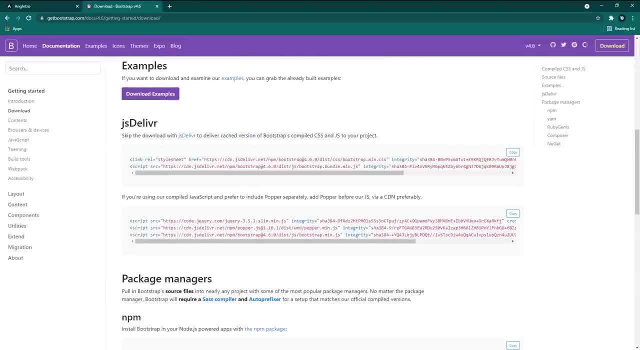 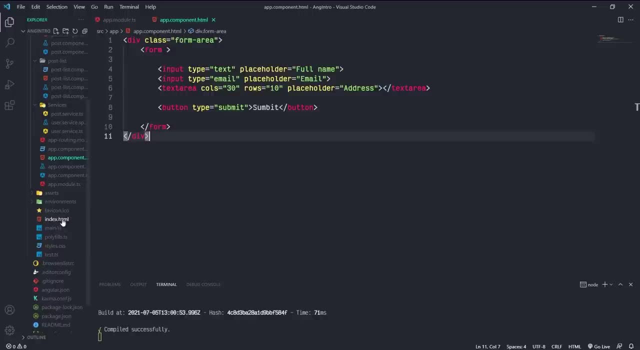 And go to this cdn area. In here we can find this cdn link for bootstrap css. Copy this cdn link Now go to the vs code and open the indexhtml file. This is the main entry point of our angular app. 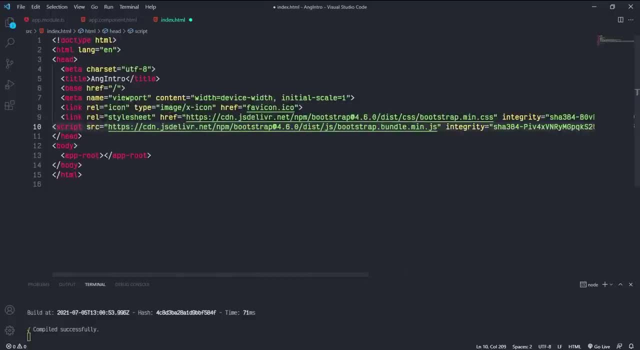 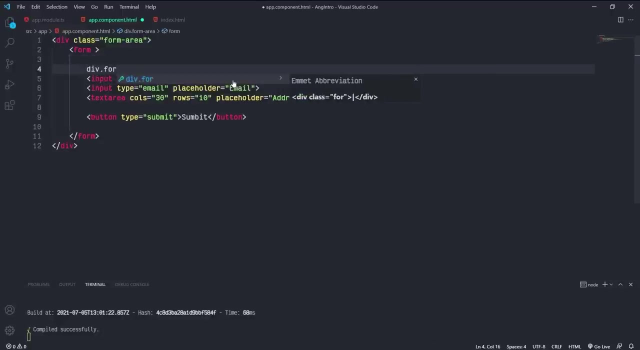 So inside this head tag paste this copied cdn link. So keep only this bootstrap css cdn by removing the script tag of the bootstrap javascript file. We're not going to use any bootstrap javascript functions with this, So remove it. Now go to the app component html file and let's bootstrap this form. First let's create a div with bootstrap class form-group. 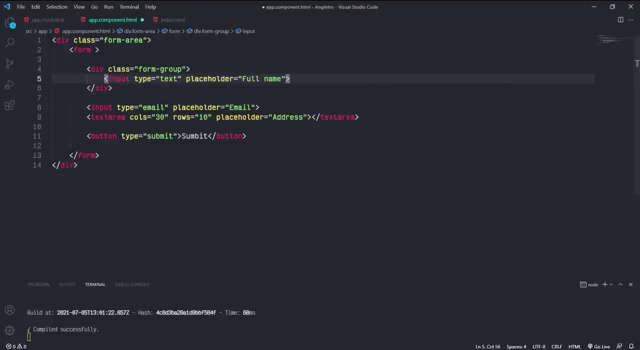 Inside this form-group dash group div. Put this first input field. After this: add this bootstrap class to this input field: Form dash control. This is not anything new. We learned about these bootstrap classes when we learning bootstrap, Right? So, all right, Let's add the label for this input field. 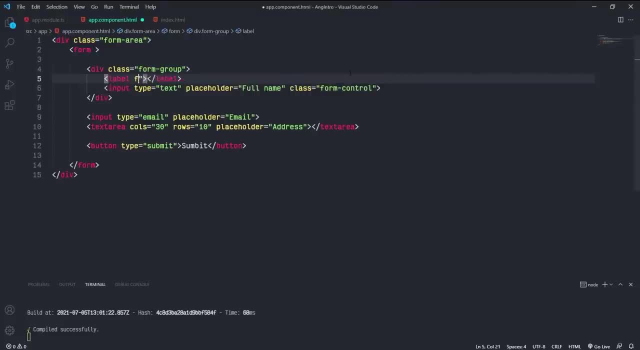 Label. Hit enter. So we don't need this for attribute. Remove it. This input labels text is the first name. Okay, Next, do the same for this, both input fields as well. Inside of a div with form group, create a label. Label text is email. Put this field inside this. 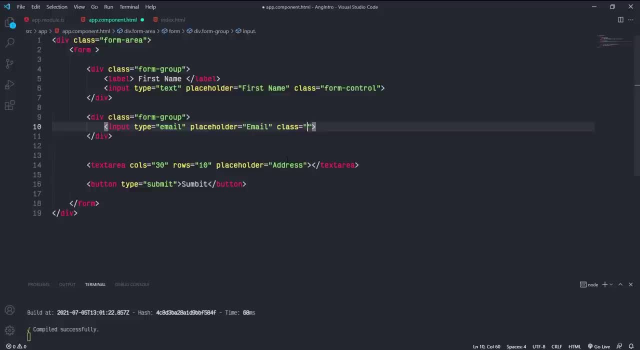 div and last, add the form control bootstrap class to this email input field. Next, do the same thing to this text area as well. All right, Now add the bootstrap btn class to this submit button. So class btn- btn-primary. That's it. 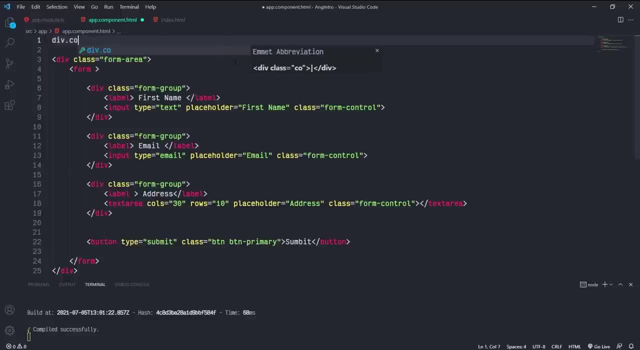 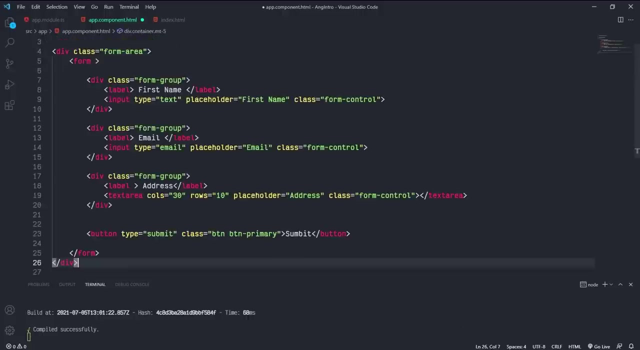 At last. Let's put this inside of a bootstrap container. So create a div with these classes: Container and empty dash 5.. This container class will make this form center of the page and this utility class will add a 5 rem margin top to this form. Hope you guys remember this, Save this and back. 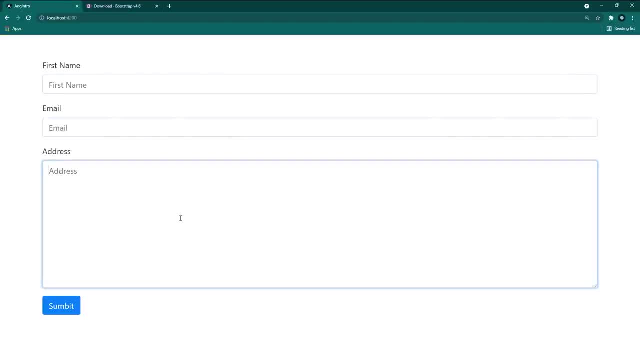 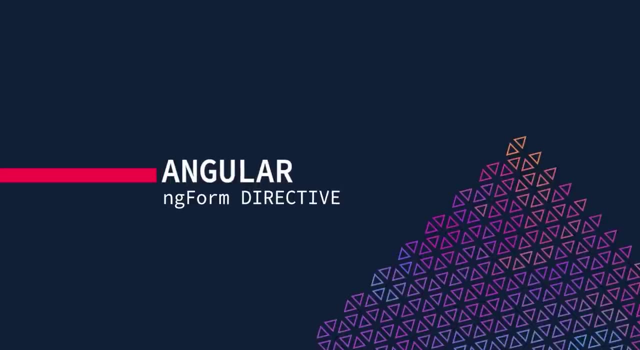 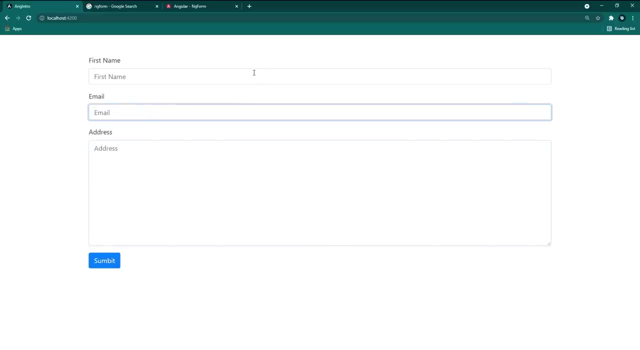 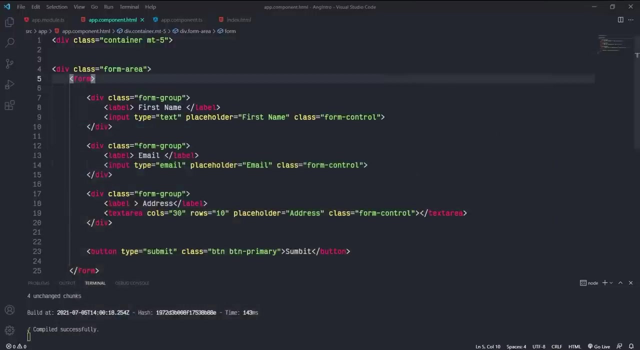 to the browser. Perfect, As you can see here, we got this beautiful bootstrap form inside the browser. Let's reboot And open convert Speed registrator. In the previous lecture we designed this bootstrap form, so in this lecture let's see how to make this simple HTML form into an angular template driven form. so first thing first. 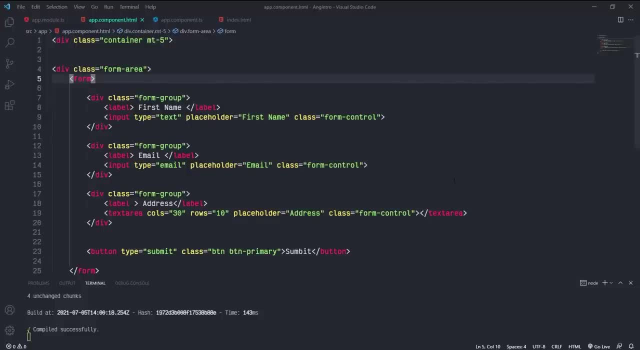 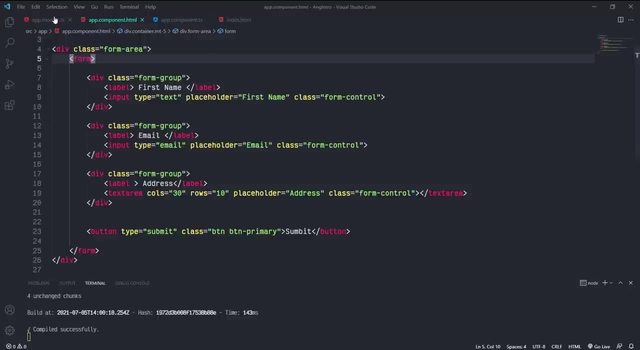 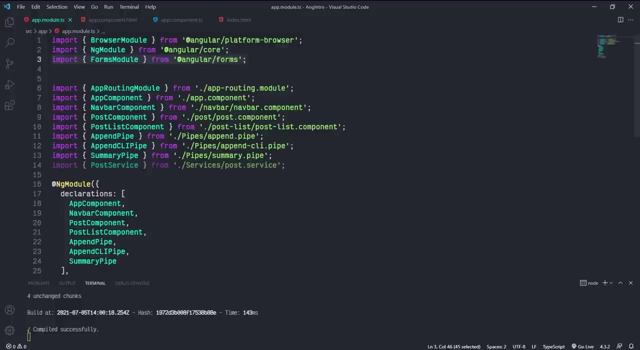 in order to work with template driven forms in angular, we have to import the forms module in app. template driven form architecture is built inside the angular forms module, so import this in app modules ts file. wait, if you can remember, we imported this forms module when we doing two. 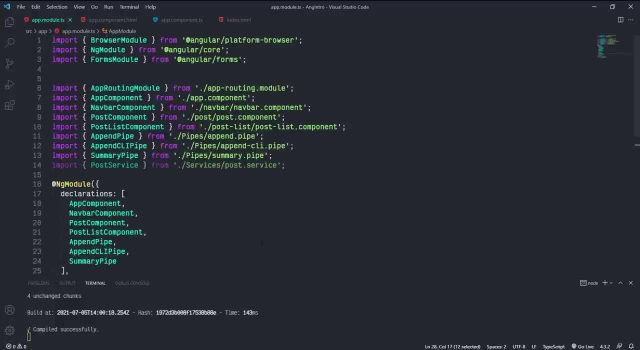 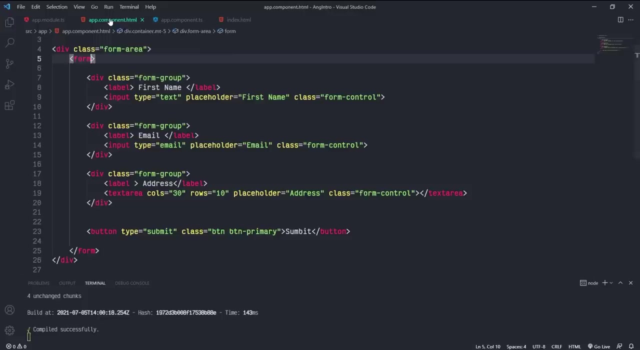 way data binding. that's why i got this form module import here. if any of you missing this forms module, import it now. this is must. in order to work with angular forms, we need this forms module. all right, after this import, go to the app component html file. now inside this form tag: 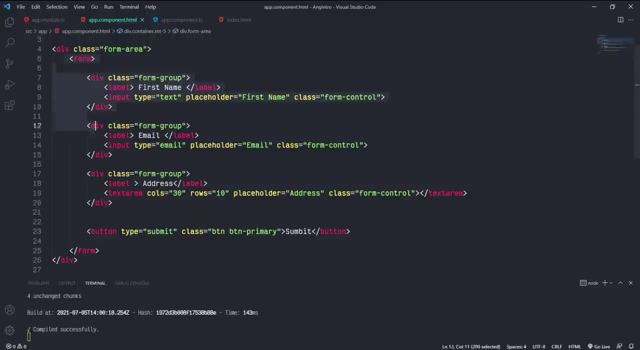 in order to make this form template driven, we have to add a special type of directive to this form tag, which is ng form. so let's do that. first, create a template variable. you know already about this template variables, so hashtag and a variable name will be- can be any name. I just add F as this template variable. once again, keep this. 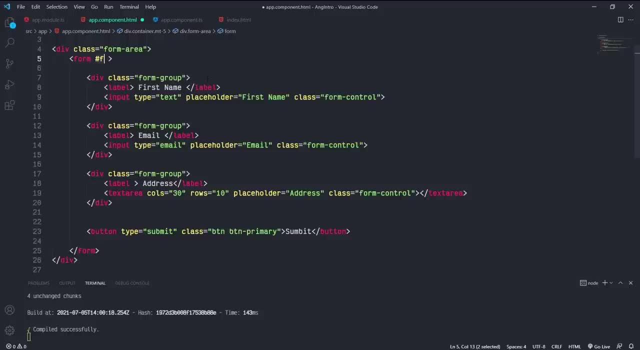 in your mind. this template variable can be any name. I just added the F letter cause. F represent the form right. all right, after this, bind this template variable to ng form directive inside quotes. all right now. we have successfully made this form as an angular template driven form by using this ng form. 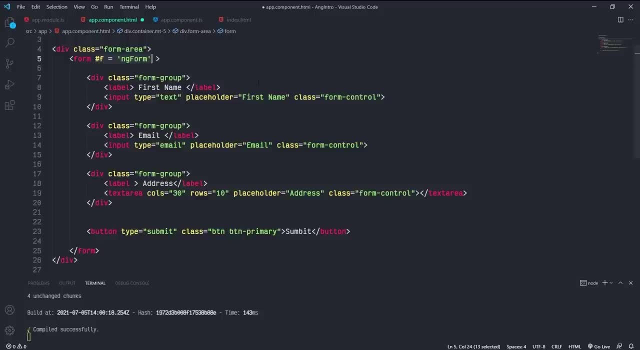 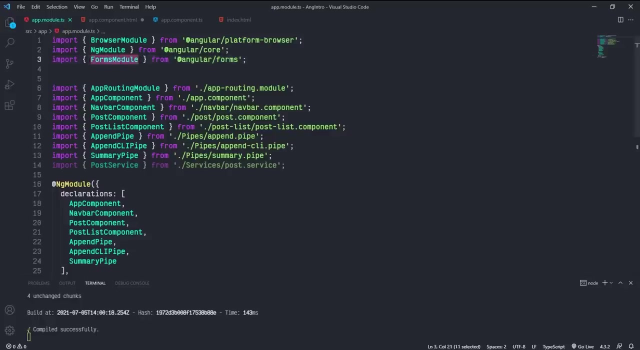 directive. some of you may wonder: when we learning directives, we didn't learn about this ng form. actually, this is a directive, but this is a special type of directive coming with the forms module, as soon as you import forms module, this directive becomes active by default on all form tags. 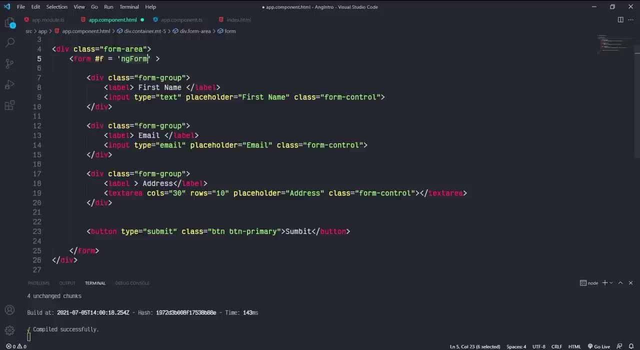 let's see how it works. let's see what is happening with this ng form directive. first let's lock this ng form, then we can discuss what is happening behind the scenes. first, bind submit event for this form inside brackets submit point the submit event to a method called onSubmit. so inside quotes onSubmit and the parentheses: 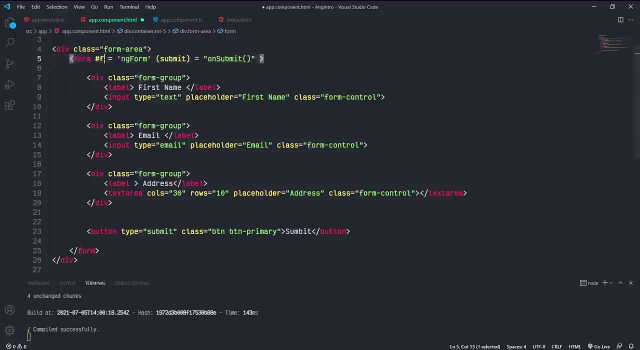 in order to lock this ng form, we have to pass this to this method. so this ng form is bound to this template variable F. so pass this F as a parameter to this onSubmit method. please note this: we use this hashtag sign only when declaring the template variable. when we use this template variable, we don't need to add the hashtag sign. so now, as. 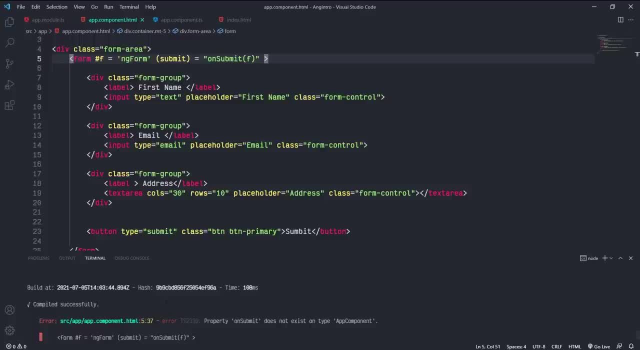 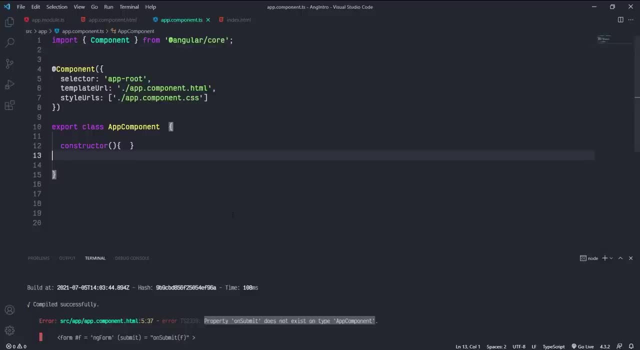 you can see here we are now getting a compilation error because this method is not exist, so let's enter inside the app component TS5 on submit. we are getting a parameter, so add the parameter variable inside this parentheses. I declare this variable also F and make this variable type ng. 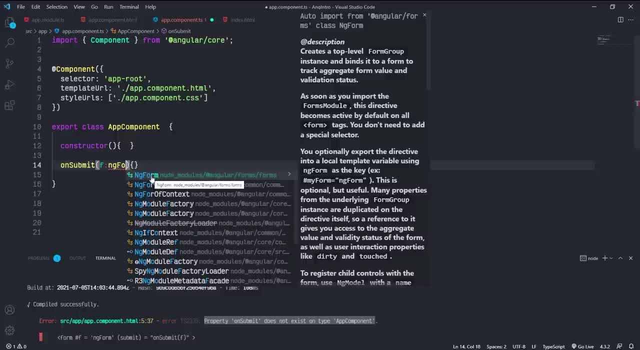 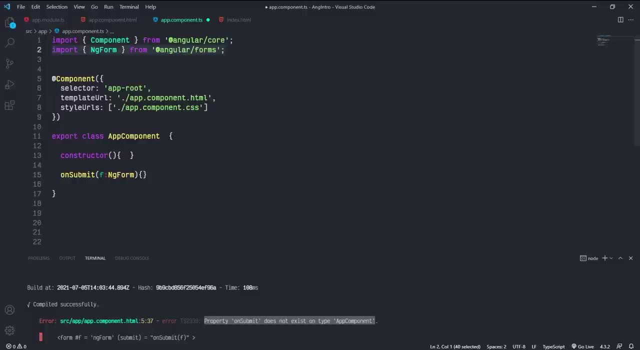 form. select this autocomplete. this will import this ng form to this app component TS5. with this we making this variable type is to ng form type. because of this we can send only the ng form data to this onSubmit method. if I send any string value as a parameter for: 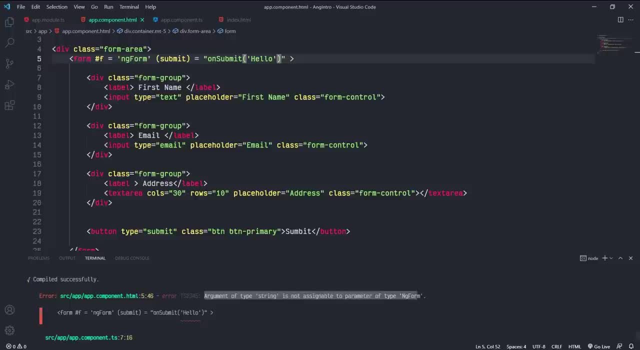 this onSubmit. as you can see here, we are getting a compilation error. if you can remember, when learning service, we learned how to make a blueprint for object using the interface. the same thing applied here as well. all right now let's lock this ng form F inside the browser console. 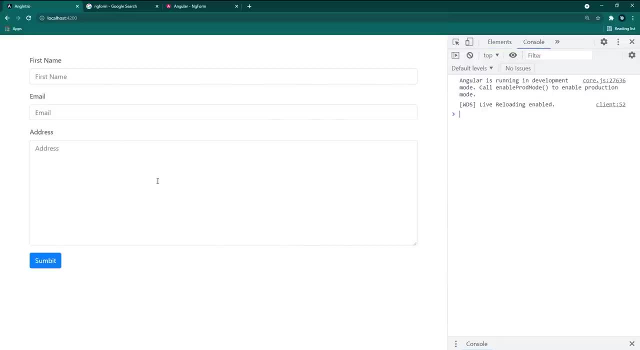 save this and back to the browser. now click this submit button. look inside browser console. we got this ng form object printed here. expand this. what's going on here? you got this list of data with this ng form. what are these and what is the use of this? let's learn this about in the next lecture. 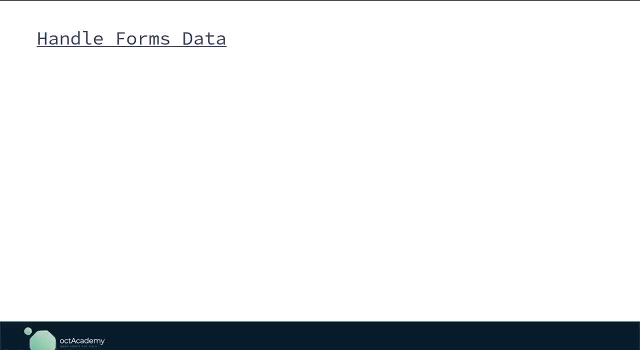 in angular to handle forms data, we have two classes: form group and form control. we use form group class with form tag and we apply form control class to the input field. for example, take this user details form. this total form is one form group and each of these input fields use the form control class. 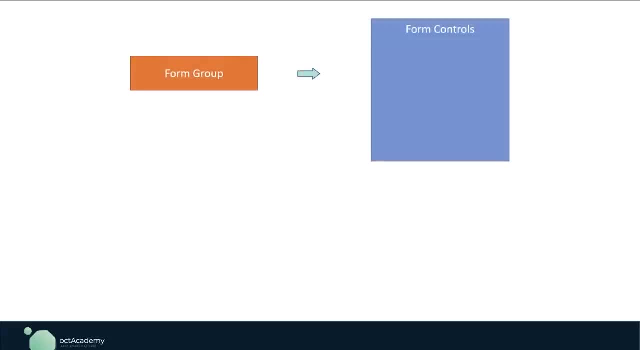 form group. we can have multiple instance of form control classes and inside of an angular app we can have multiple form groups, for example, the new post form. this is also another instance of the form group because this is a whole new, separate form. this form group also has a separate instance. 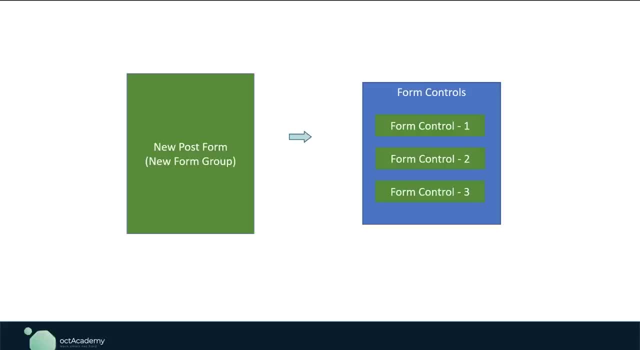 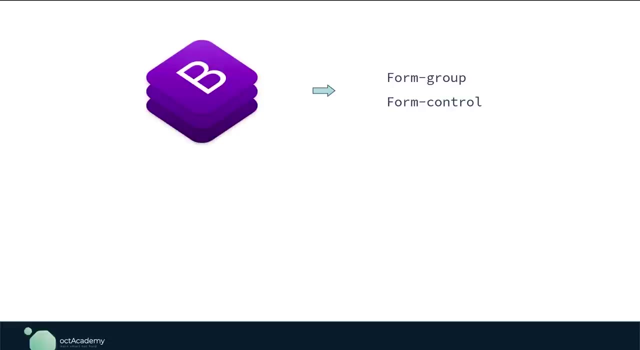 of form control class for each of these input fields. hope you guys got the idea. and one more thing: don't get confused with bootstrap CSS classes. in bootstrap also, we got these CSS classes form group and form control. please note this. I'm not talking about the bootstrap. 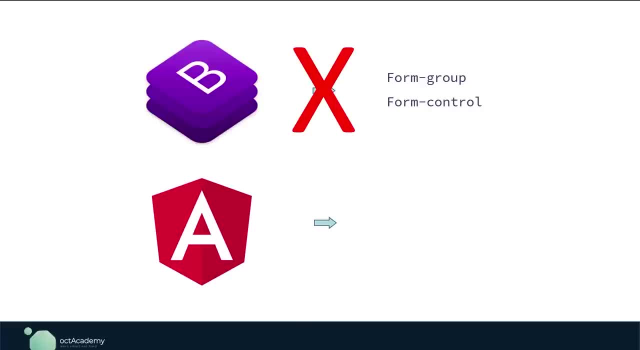 CSS class in this section. I'm talking about the TypeScript classes that are coming with angular framework. all right, as I mentioned before, this form control class is a TypeScript class, something like this. instead this form control class, we got few properties that useful for form validations: value touched, untouched, dirty, pristine, valid errors, so on, as you know, if you, 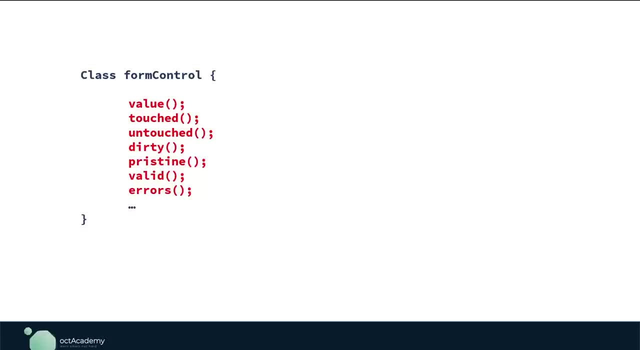 want to access these properties, which is inside of the form control class, we have to create a new instance of this form control class. to create this class instance angular as two approaches. one is the usual way, by creating the instance, by encoding. the other one is using an angular directive inside the template babe or the HTML file. 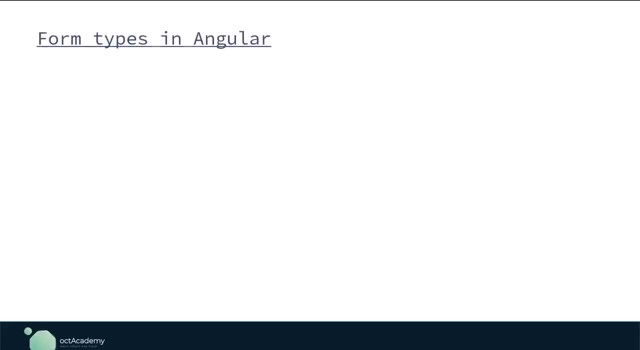 if you can remember, when starting this section, I told you in angular we have two types of forms: reactive forms and template driven forms. so these are the two methods creating this form group instance by hand coding approach is we called angular reactive form and this creating the form. 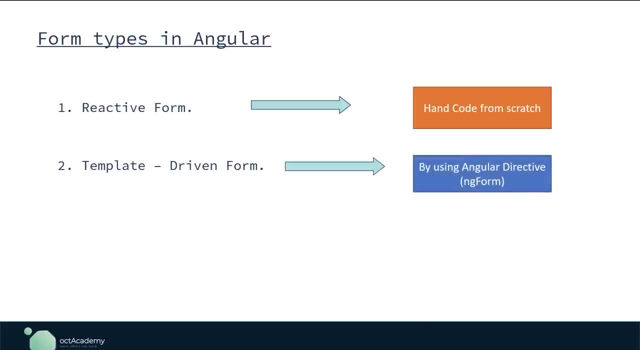 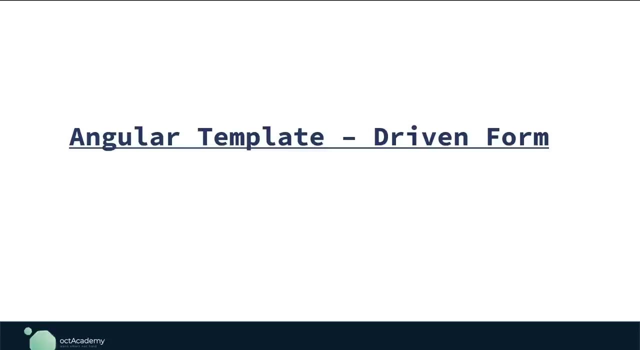 class new instance using a directive inside the template. we called this approach angular template driven form. as you know, in this section we are learning about the template driven form. so this is what template driven form we mostly do: all the stuff inside the HTML template view, all right, so 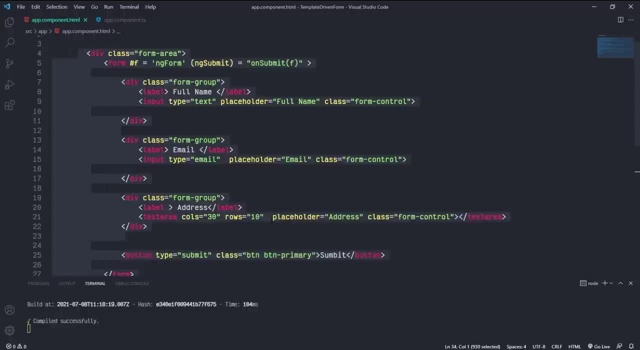 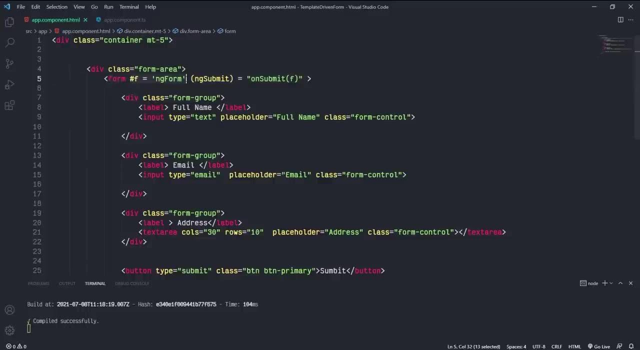 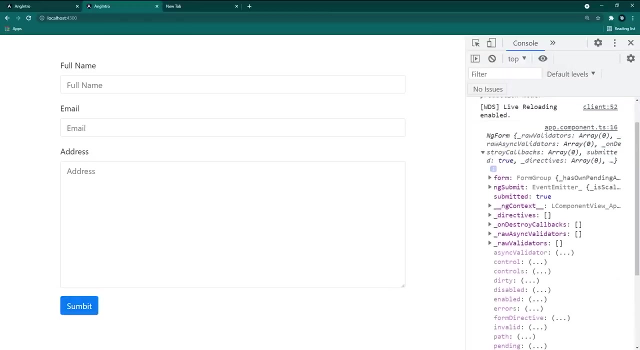 in the template driven approach, as I mentioned before, we use an angular directive to create a new instance of form group class. so that's what we did using the ng form directive. this is the directive which creates the new instance of the form control class. that's what we got with this control. expand this form control and. 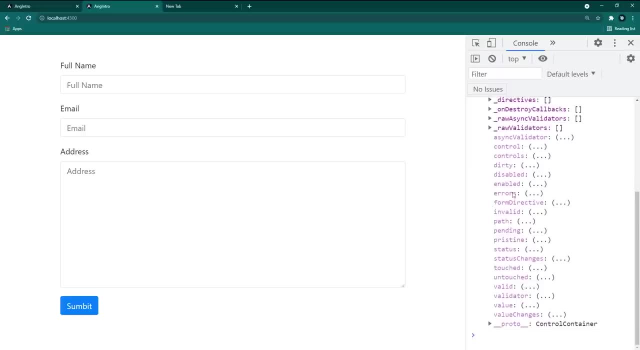 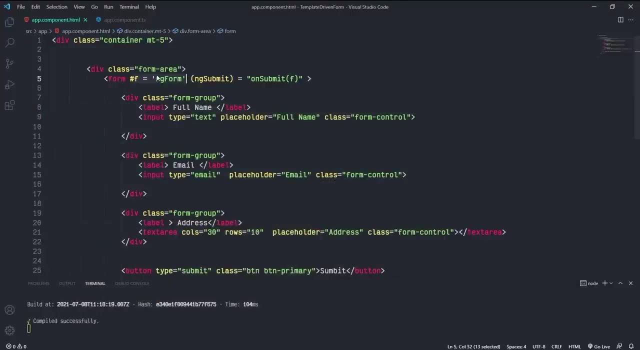 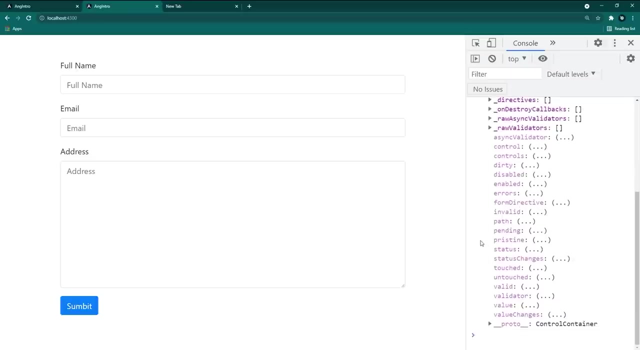 also. these are all properties of the form control class. we got these properties because we created the new instance of the form group using the ng form directive. now you guys may wonder: what are these properties? don't worry about that. we'll learn about this in a later section. 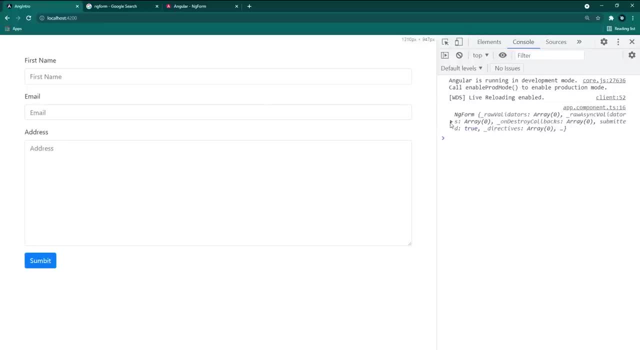 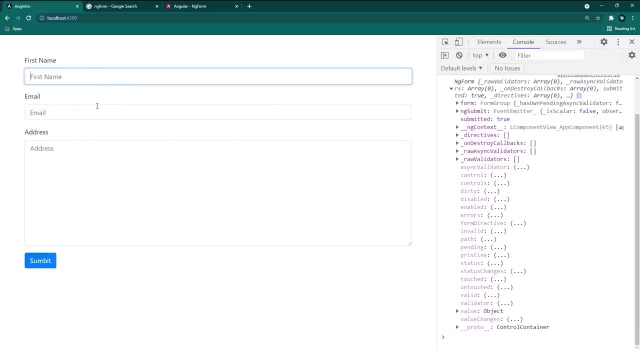 as you can see here inside the terminal, this form control instance carries this value property, which is the one get to all the values types inside this form input. now this is empty. this is inputs. so let's fill these inputs and try this now inside the browser console. still these values. 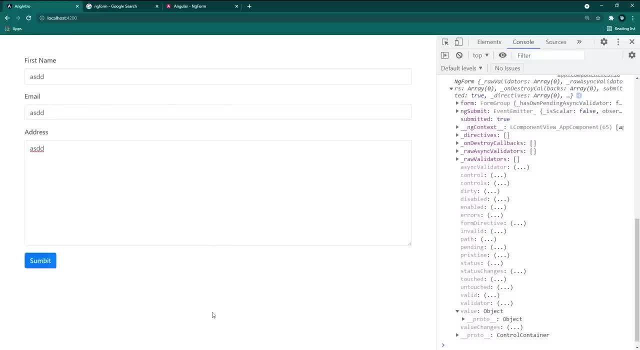 properties is empty. why is that? if you can remember, I told you that every form group can have multiple instances of the form control class. this form controller class also have the same properties as the form group class. in order to get the input fields value, we have to make a new instance of. 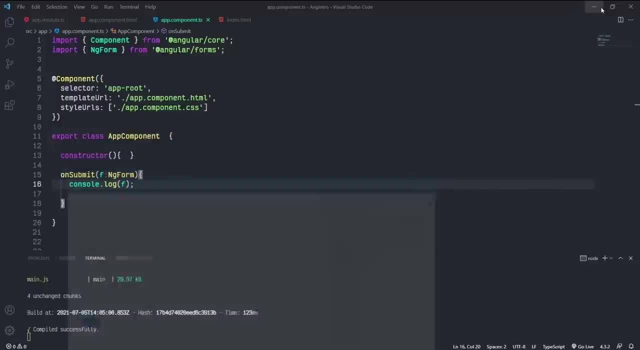 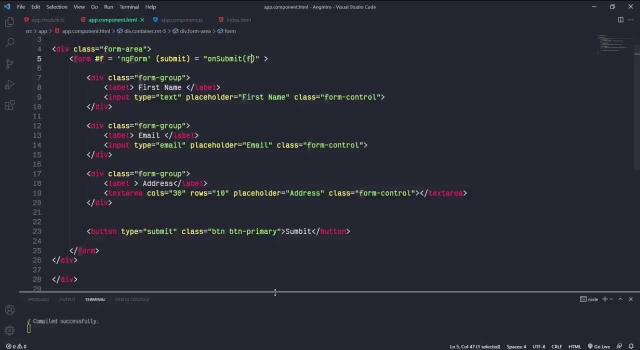 the form control class for this input field. to create this new instance of this form control class we got two approaches: by hand coding or using a directive. now we are dealing with the template driven forms, so for this we're going to use the directive method for form group we 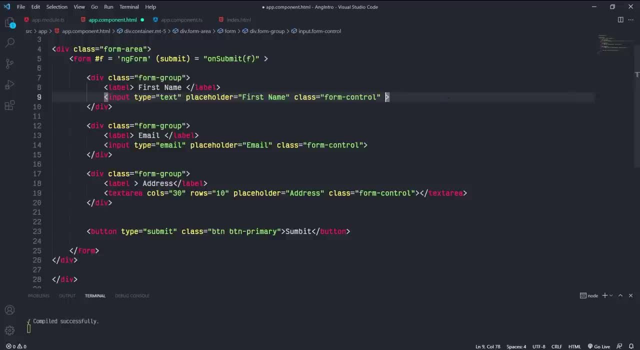 use the ng form directive for form control. we're going to use the ng model directive. what we have to do is just add this ng model directive inside this input tag, ng model. if you can remember, we use this ng model directive when we're dealing with the two-way data binding, the. 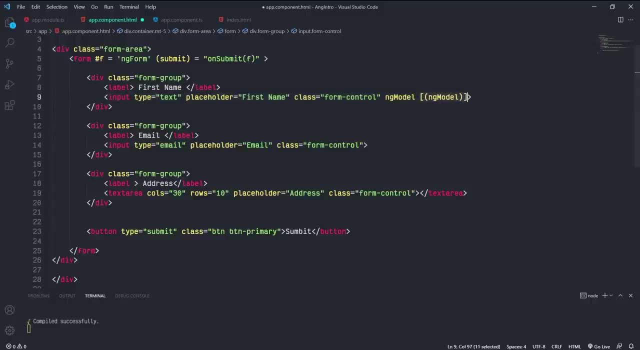 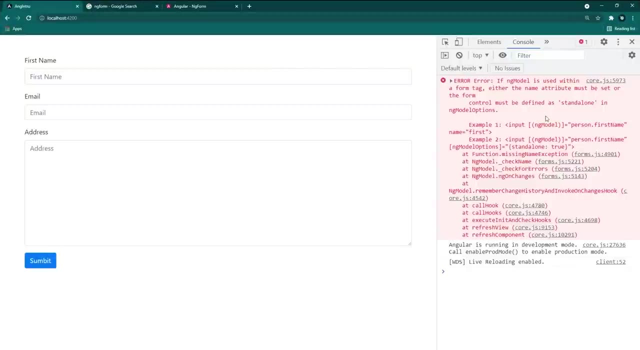 syntax was something like this, but this time we are using this ng model directive directly, so save this and back to the browser. inside the browser, look at this browser console. we got this error. if ng model is used within a form tag, the name attribute must be set. so when we're dealing with the ng model directive, this is a. 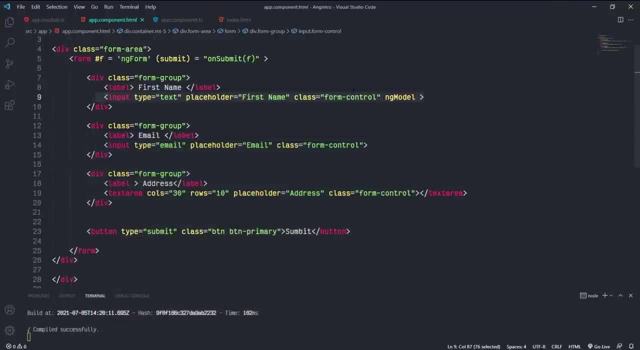 requirement. we must provide a name attribute for the input field, so inside the vs code name, and give a name for this input field. this input field is used for full name, so I will give full name as this input field name. I use the camel case naming convention, so this is optional. you. 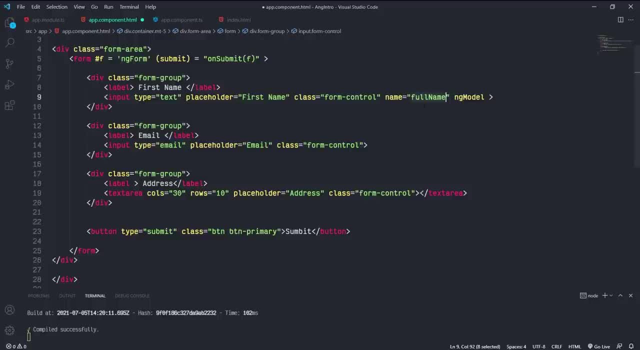 guys can name this name that you want. I use the full name because this field is for full name. So, as a good practice, always try to name something relevant which makes more sense. right, Once again, when you deal with ng model, the name attribute is must, Otherwise your application can be break at the runtime. 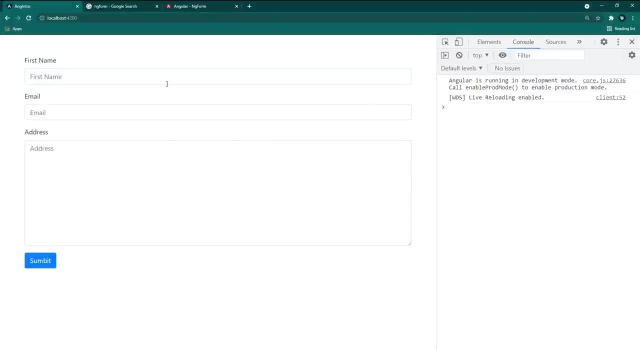 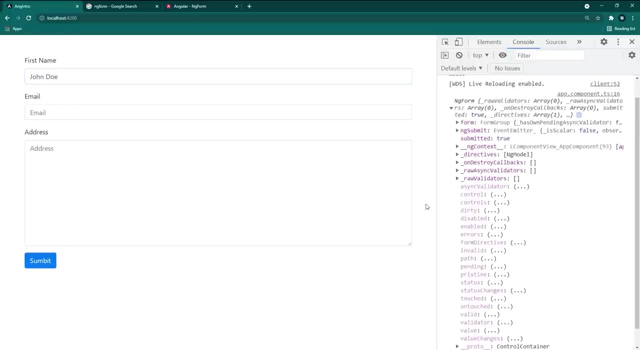 Alright, save this and back to the browser. Inside the browser console this time, no errors. So let's type something inside this full name input: John Doe. Now click the submit button. Look inside the console. We got this ng form object Inside this: expand, this value property. Awesome, right. So this. 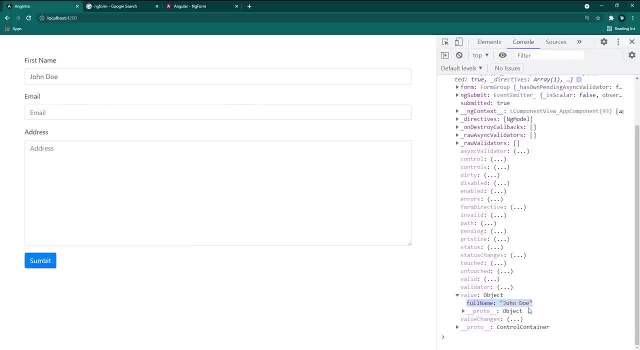 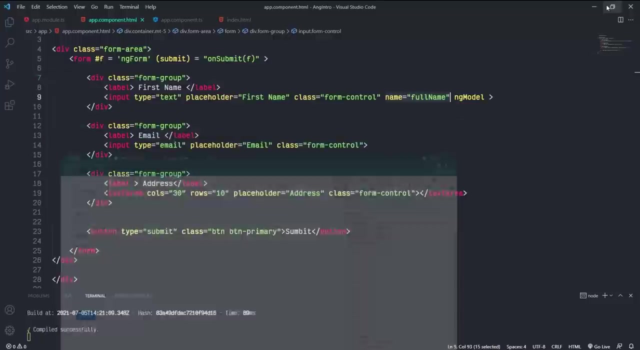 time we got this full names value John Doe. So this is how we create the new instance of the form control and access the value property of the form control instance. So like this, we have to add this ng model directive To this all input fields to get the values. So for the second input ng model and next, what is the? 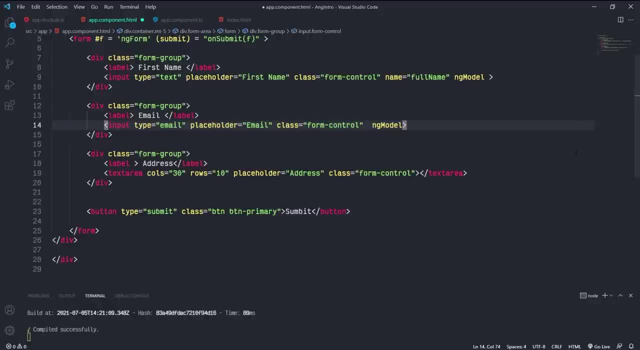 requirement. I am repeating this course. This is very important. So, in order to work with ng model, we must add the name attribute to this input Name and this field is for email, So pass email as for this field name. Next, we got this text area. This is also the same Inside this text area: open tag. 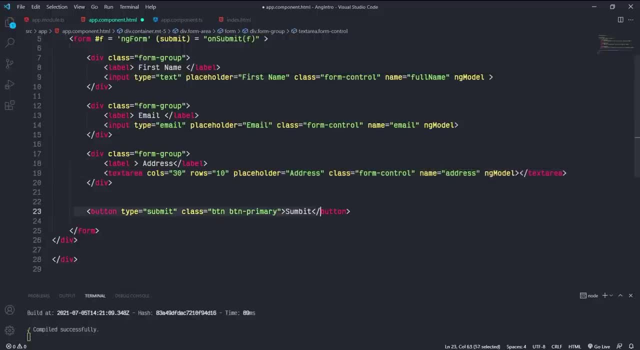 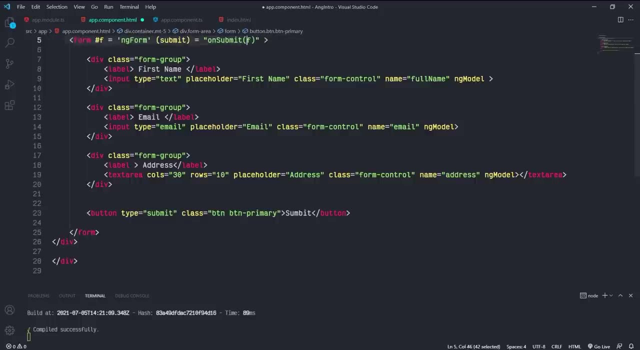 and we are going to add this text area. So we are going to add this text area, So we are going to add ng model and the name is address. That's it. We don't need to add ng model for the submit button, cause we are not getting any values from this button and this button is only used for submit. 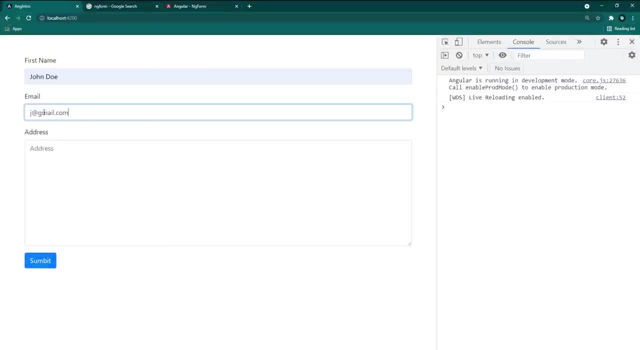 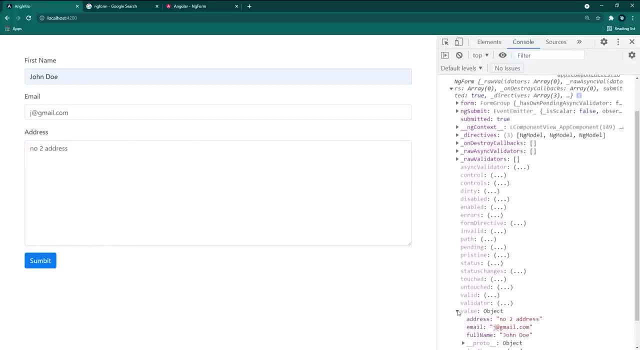 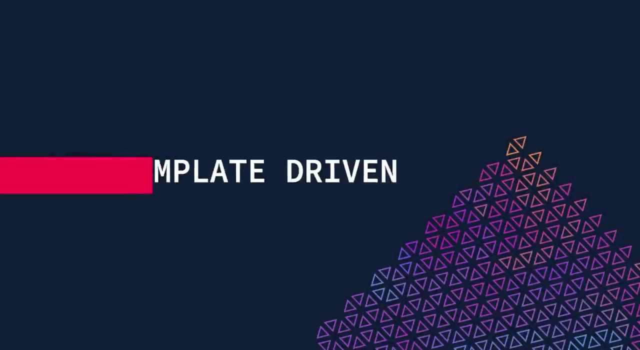 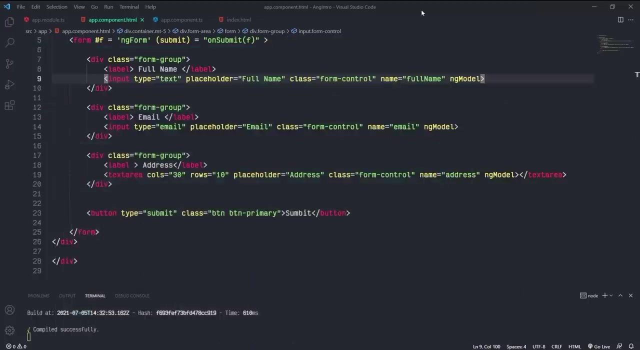 this form. Say this and back to the browser. Fill this form and hit enter or click this submit button Inside the console expand this value object. Inside this we got all three input fields, value, Perfect, Alright. in this section let's see how to do a simple required validation for these. 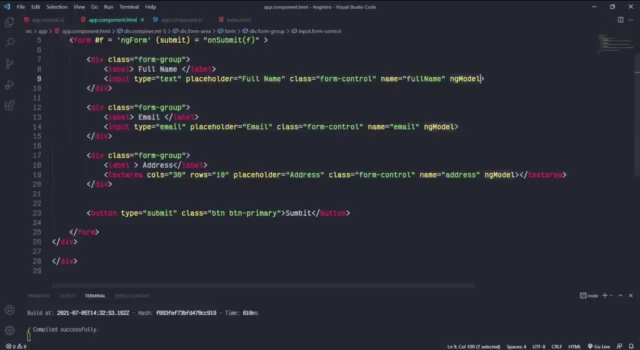 input fields. With this ng model, we are creating a new instance of form control class. Let's see what we are getting with this ng model For that, like this forms template variable. first we have to declare a template variable for this input field- hashtag, full name- and bind this template variable to this ng model. 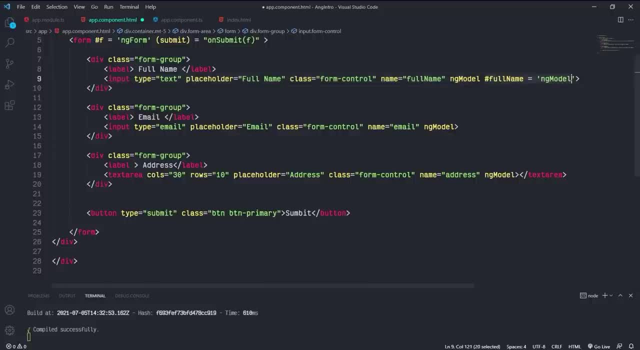 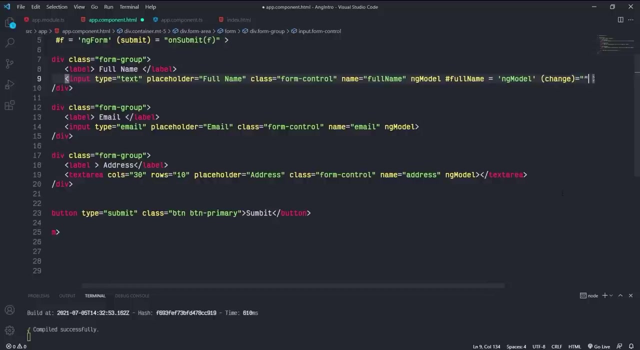 Put this inside of a quote. Alright, now let's look at this template variable inside the terminal. For this I'm going to use the change event binding, So inside brackets, change. bind this change event to a method called getValue. With this change event, pass this template variable of full name. 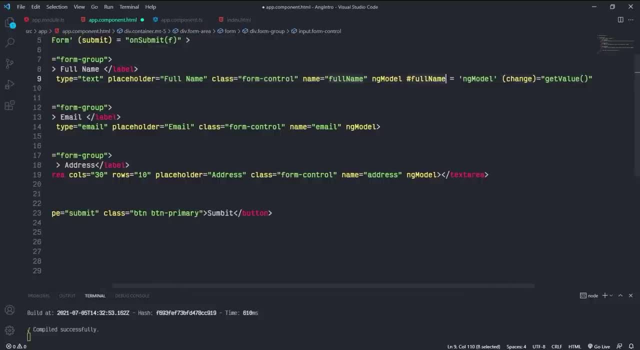 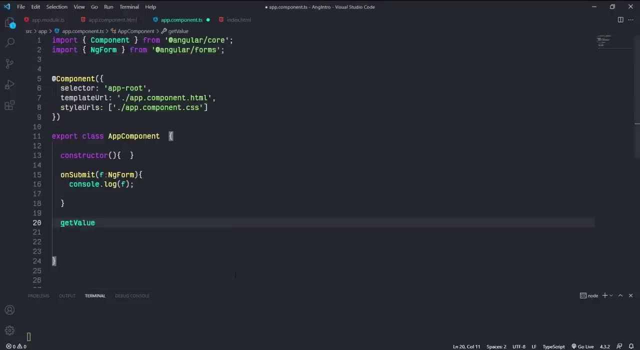 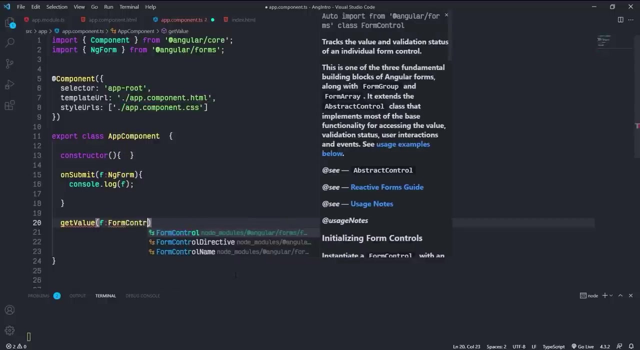 Which is bound to this ng model. Now, inside the app component ESPY, create this getValue method. We are getting a parameter, so capture it. I just add form control as this parameter variable Inside this log. this parameter. That's it. 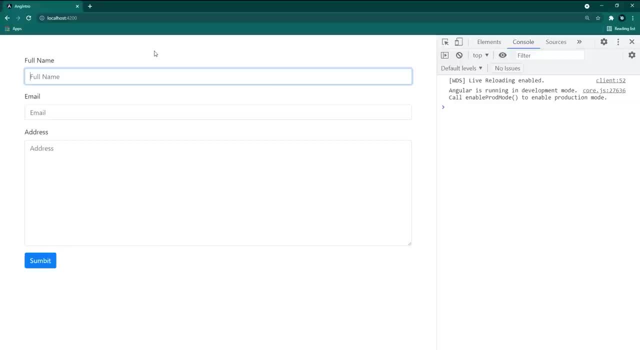 Save this all and back to the browser. Type something inside this full name input field And click outside of it. Look at this Inside the browser console we got this: ng model object. Expand it. This also got some properties like ng form. 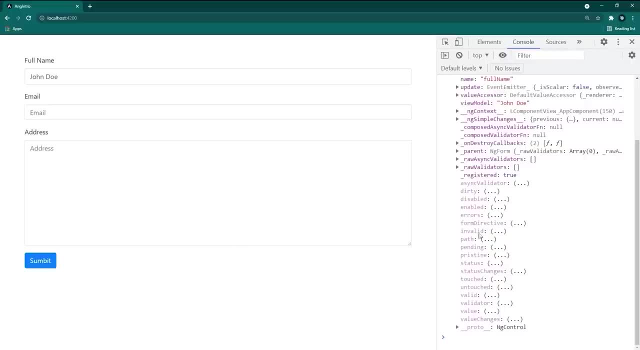 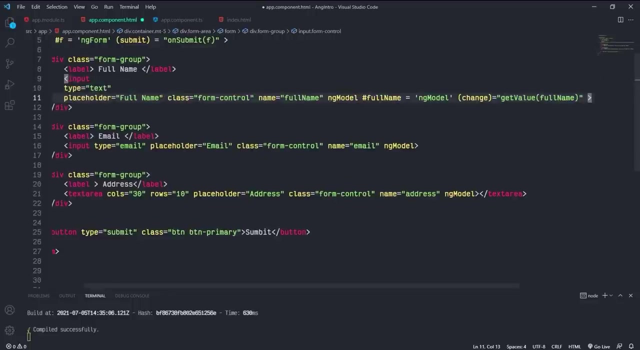 If you can remember, I said that this form control and this form group both have the same properties. This is what I was trying to tell you. As you can see here, we got this list of properties same as ng form output. Alright, let's do a simple form validation. 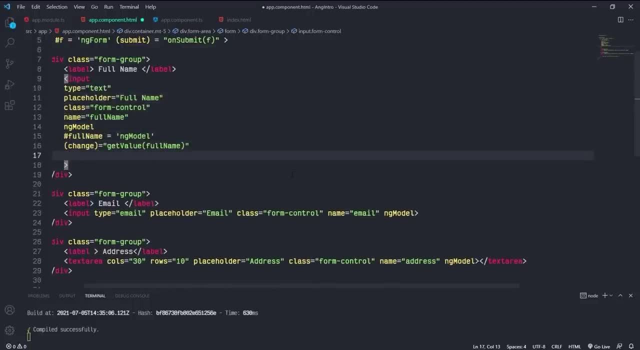 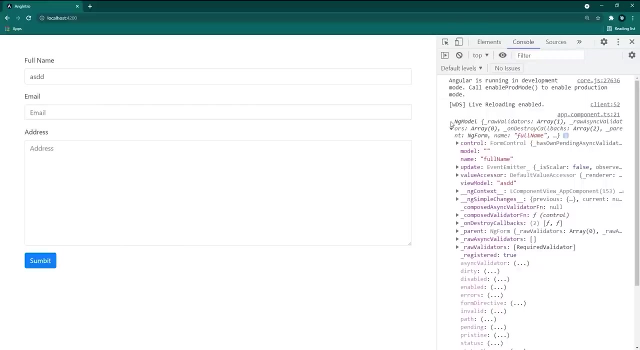 In HTML we have this required attribute. This will show us an error message when there is no data inside this text field. So save this and back to the browser, Type something and click outside of the text box. We got this object inside the browser console. 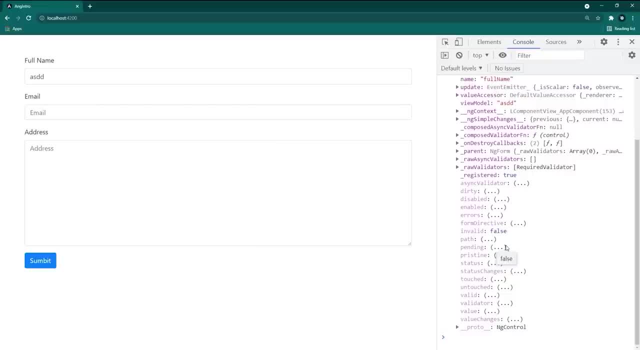 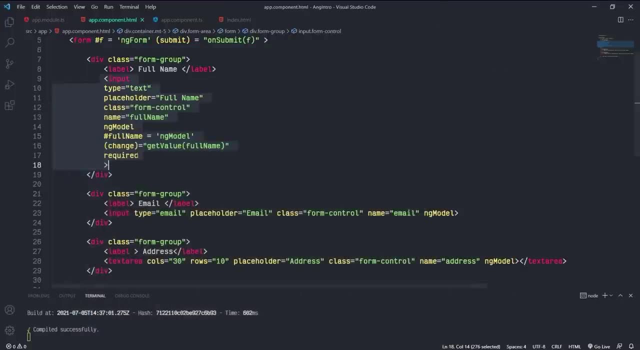 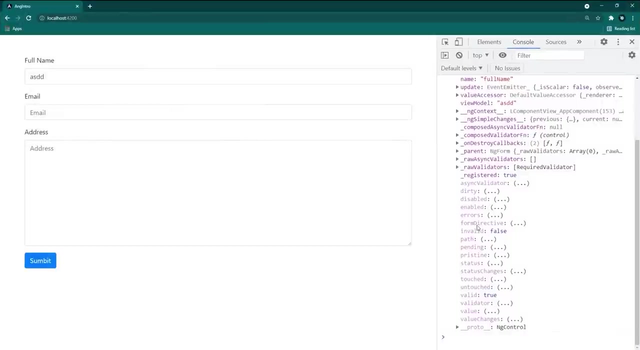 Inside this we got this invalid property Which is now set to false Down. here we got another property valid And this is set to true. We set this required validation to this input field. When there is any data typed inside this input field, then this input field becomes valid. 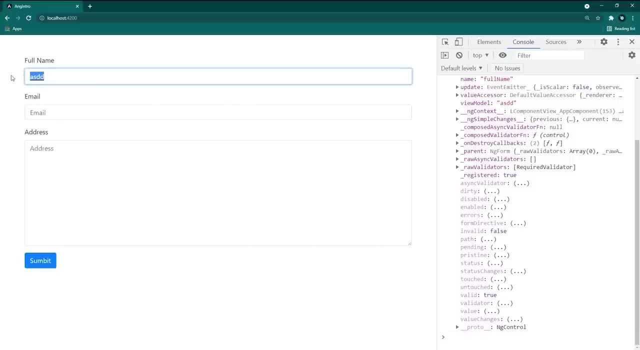 Cause this required validation is fulfilled. So now remove this all and click outside of it. Now we got another ng model log here. Look at this Now: this time this invalid becomes true and this valid becomes false. Why is that? This time we don't have any data inside this full name input field. 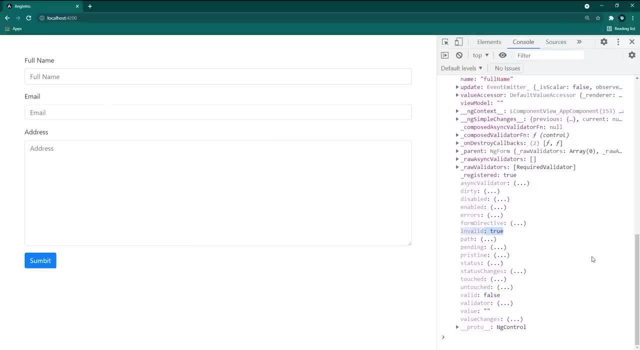 So this input field becomes invalid. So this set this invalid property to true And opposite of this: valid becomes false. So this is how this valid and invalid works. Now let's show an error message down here when this input field is invalid. 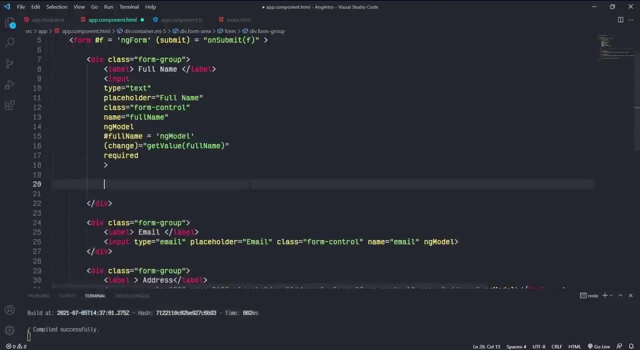 So get back to the VSCode. After this full name input field, Create a div with bootstrap class alert and alert-danger. So this will give us a beautiful red color alert. So inside this div add this error message: full name is required. 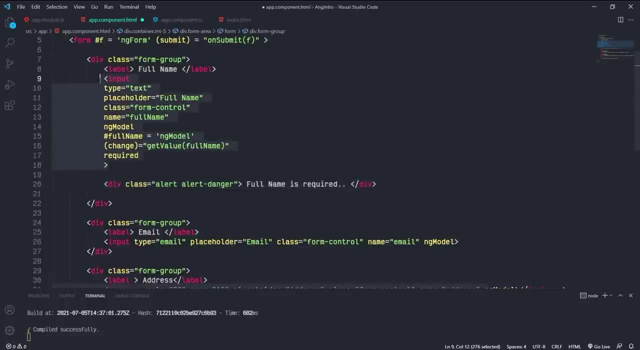 Now what I want to do is I want to show this alert when this input is invalid. For this we can use the ngif directive. So ngif, this statement is: When this field invalid. So this field representing with this template variable. 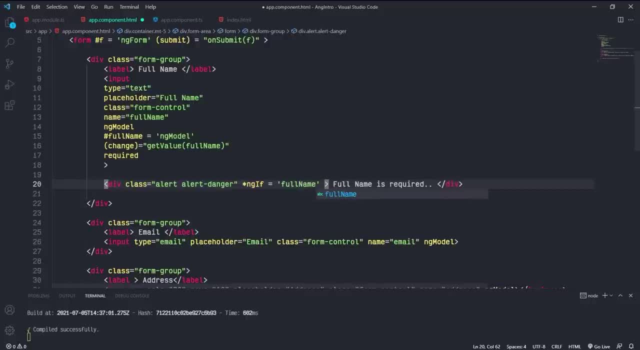 So template variable name is full name. When using the template variable we don't need to add the hash sign, So the template variable is full name. But I want to show this when this invalid is true. So in here the property is invalid. 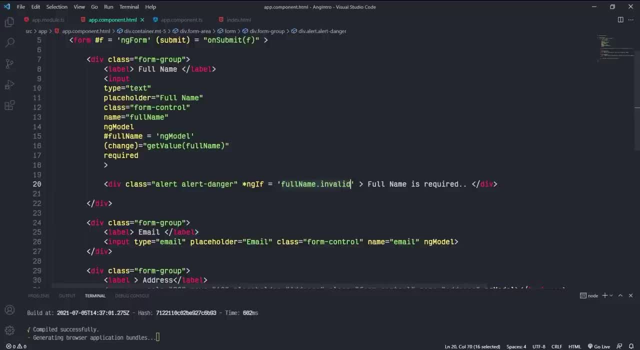 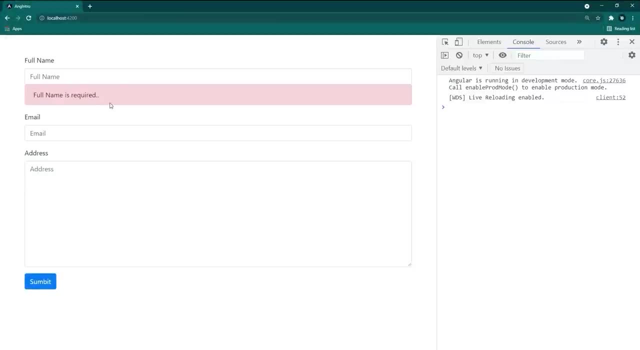 So, with this statement, This will show This error message when this field is invalid. So now save this and back to the browser. As you can see, here we can see this error message. Type something inside this input- full name. If you noticed, as soon as I start to type characters inside this input, this error message. 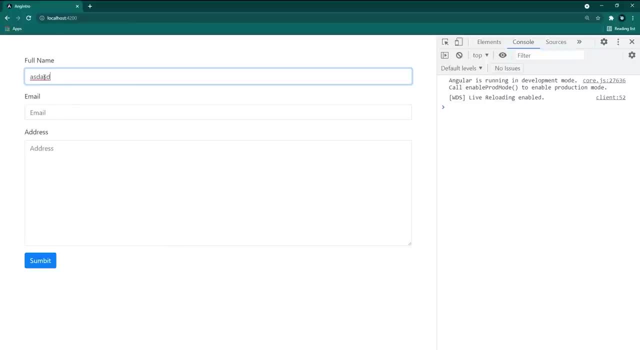 disappeared Because when we start to type inside this field, this field becomes valid Because this required validation is fulfilled. In that case, as you can see here, this invalid becomes false. If this is false, this error message will be removed from the DOM by this ngif directive. 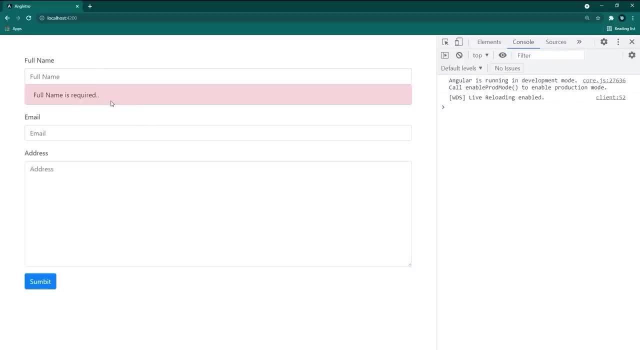 If you noticed, this error is displayed in the browser when this forms loads to the browser. This is not a good practice When a user comes to this forms page to enter user details for the first time, showing this error message to the user before doing anything wrong. 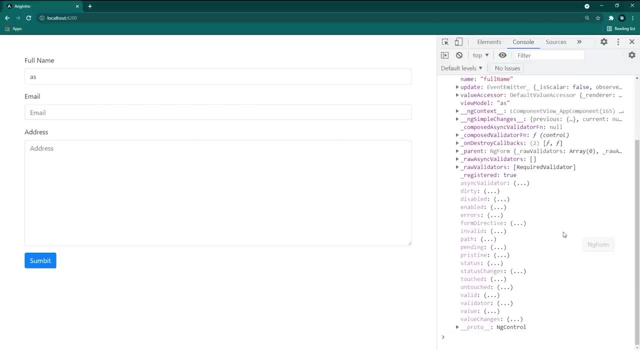 It's not good right To avoid this. we can use another form control property called touched. With this we can show this error message when the user clicks this input and move away without type anything inside the input. If this touched by the user, this touched property becomes true. 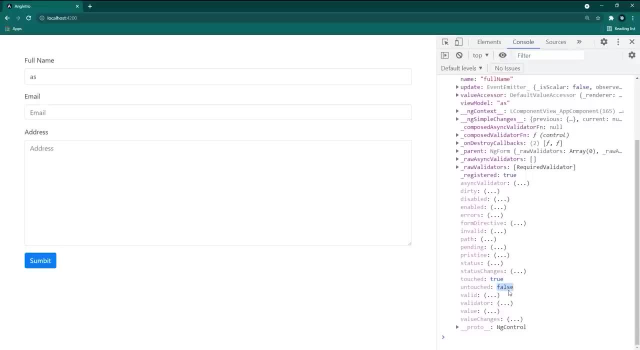 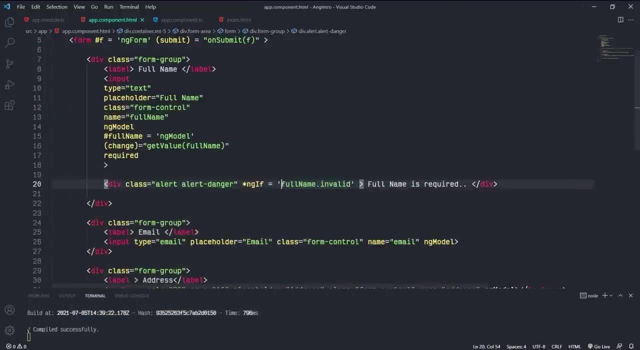 And this, untouched, becomes false. So back in the VSCode, Inside this ngif. first let's check the touched value. So before this template, variable name, first name and dot. This time we are checking the touched property, So pass touched here. 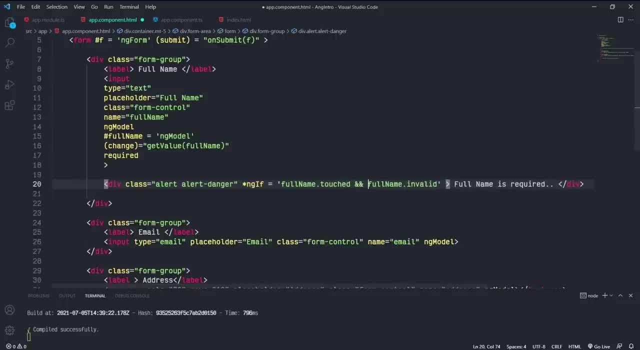 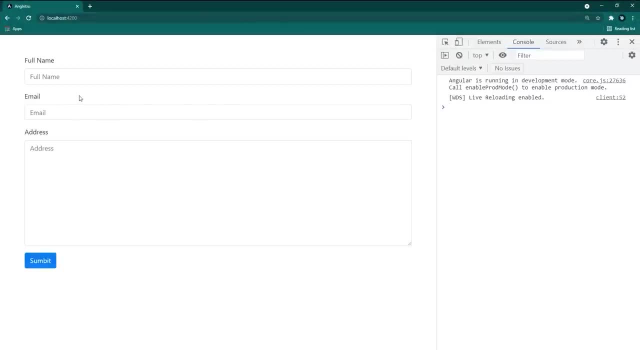 After this, add the AND operator. This time, this error message will show only when this true statement becomes true. Save this and back to the browser. Perfect, We are not getting any errors. Touch this and hit the tab or click this second input field. 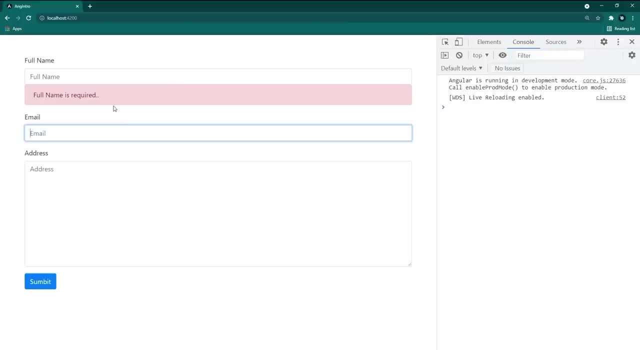 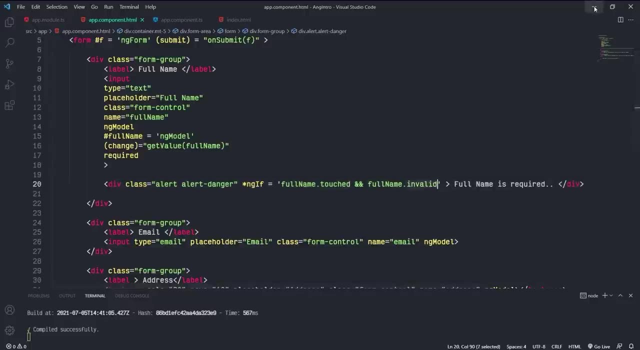 We got this error message. So when the first time this loads inside the browser, this touched becomes false And this invalid is true because this field is empty, But this is not showing the error, because when we using AND operator this, both statement must return true values. 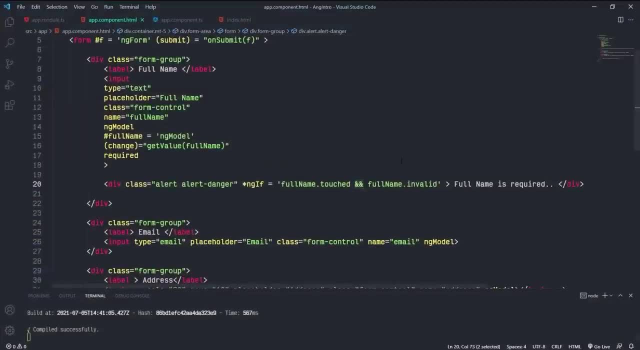 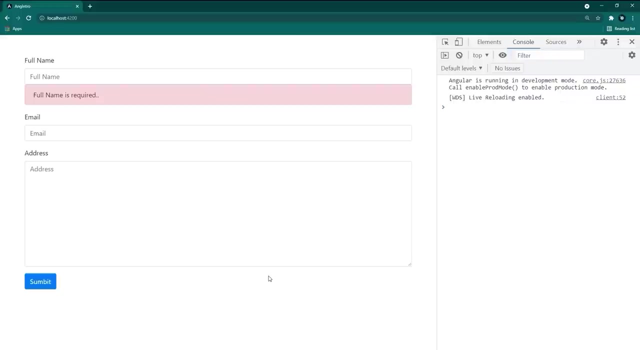 In the second situation, when we click this input field, this touch becomes true, And when we move out from the input field without typing, this invalid becomes true. So both statement are true. That's why we are seeing this message here. Hope you guys got the idea. 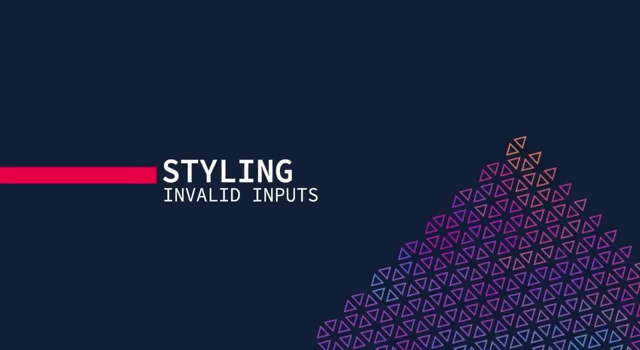 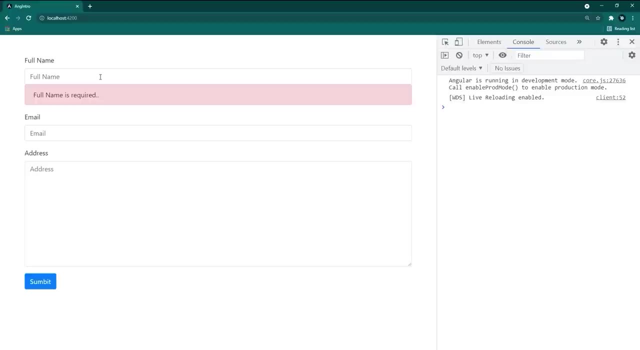 Right. Rather than showing only this error alert message, we can make these input fields border to red, Which will give a good experience to the user. To do this, we can use the bootstrap pre-built style, or we can use our own CSS style. 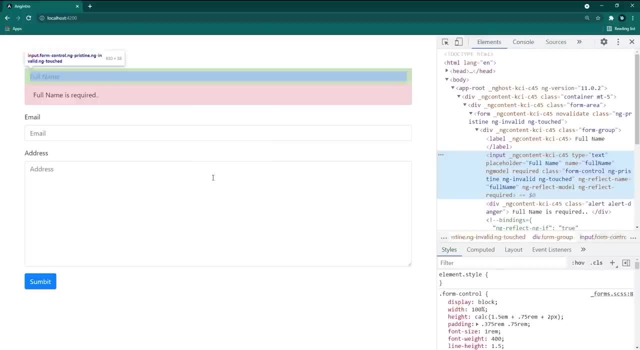 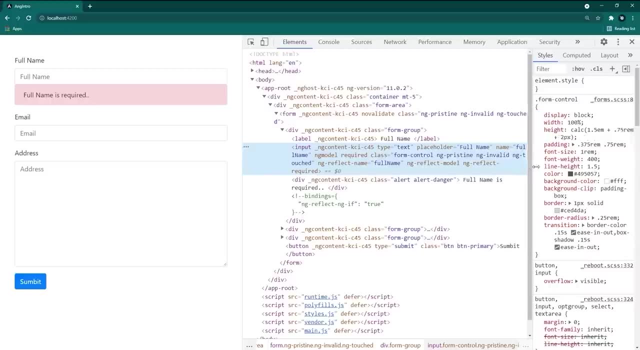 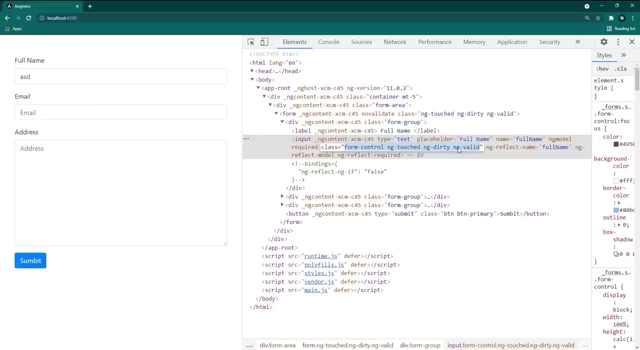 First let's encode the style. So inside the browser let's inspect this full name input. Inside this class attribute we can find this form-control bootstrap class. In addition to this, angular added few different classes for validation: This ng-touch, ng-dirty and ng-invalid. 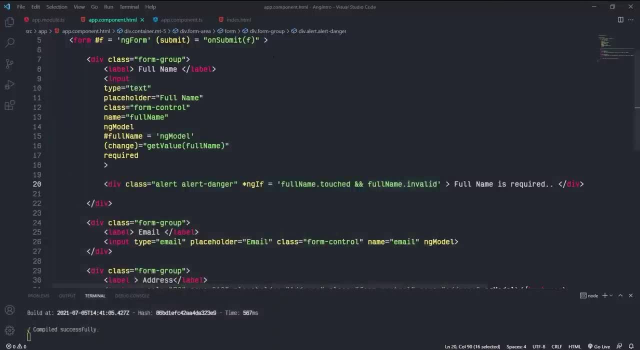 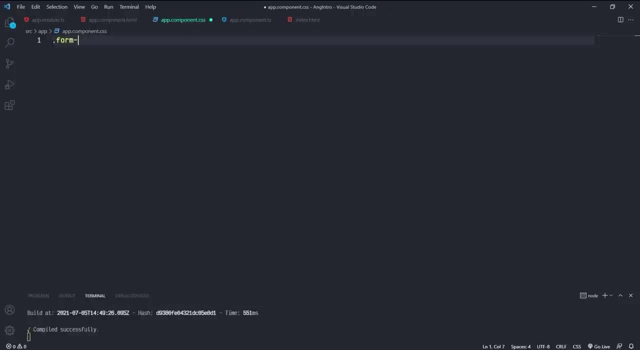 So we can use these classes to add CSS styles to this invalid input field. Let's see this in action. Inside the component CSS file form-control CSS class. In the same element we have ng-touched class and ng-invalid. So inside the CSS scope, define the CSS style. 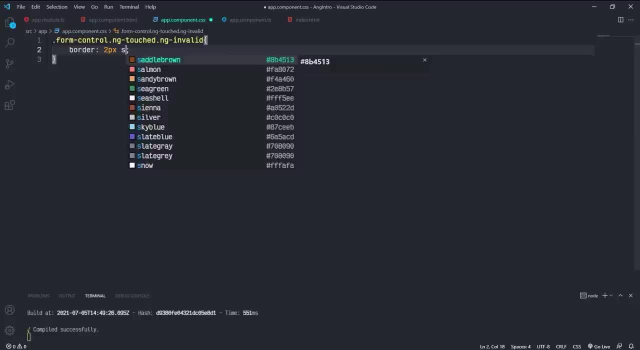 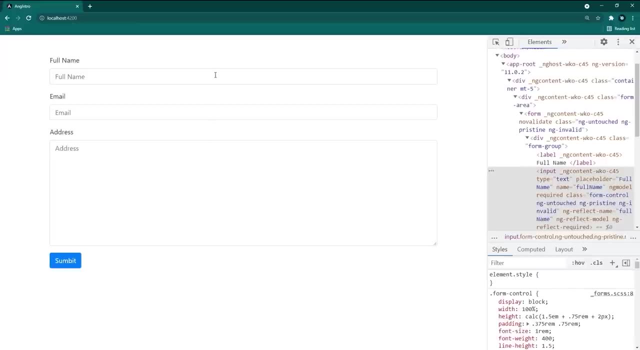 Set the border to 2px solid and the border color will be red. Save this and back to the browser. Everything looks okay. Click this and move without typing, Without typing anything inside this input field. As you can see here, we got this beautiful red border on this input field. 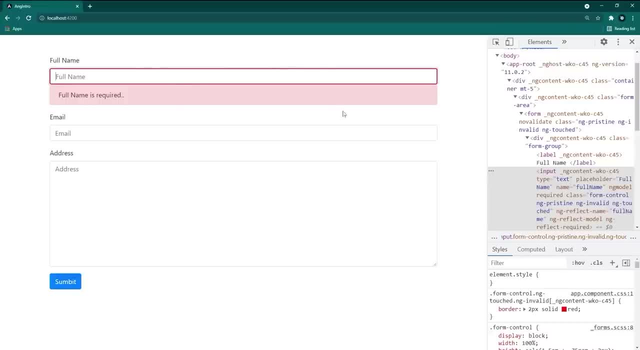 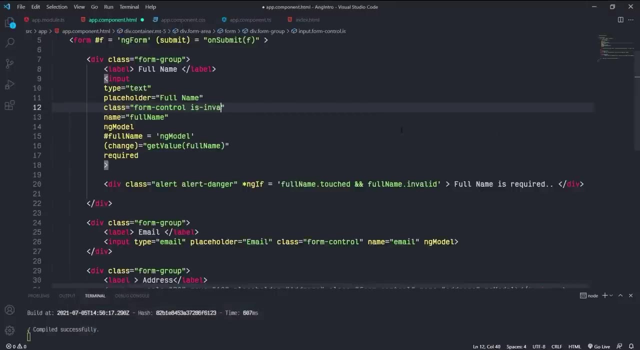 Awesome, right. Next, we can do this using a ng-class directive. In bootstrap we got a pre-built validation style class for input fields which is isInvalid, So let's try this: Add is-invalid bootstrap class to this input field. Command plus: 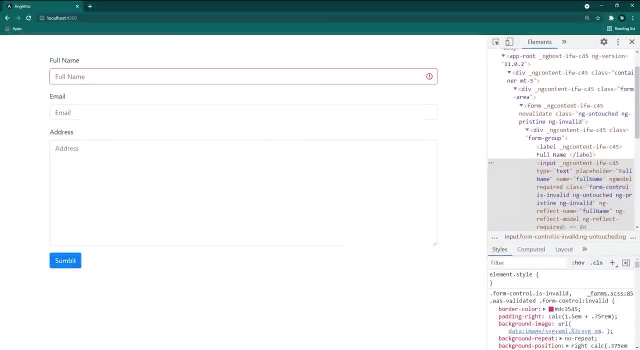 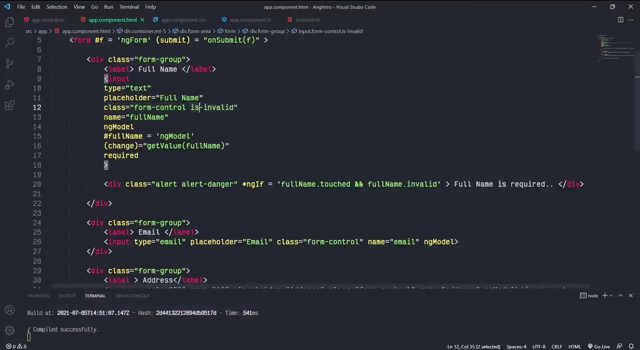 Command this CSS style. We don't need that. Save this all and back to the browser. As you can see here, we got this beautiful red border on this text field with this warning icon. We are seeing this always cause we didn't add any condition to show this CSS class. 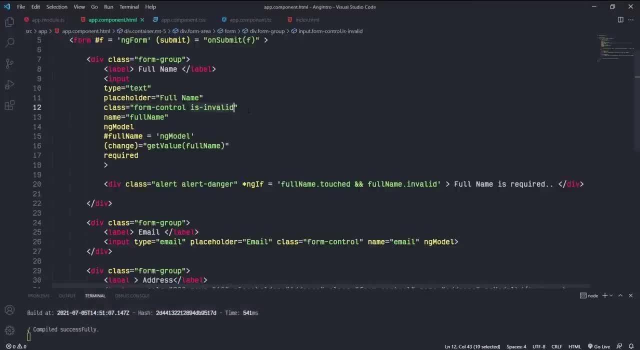 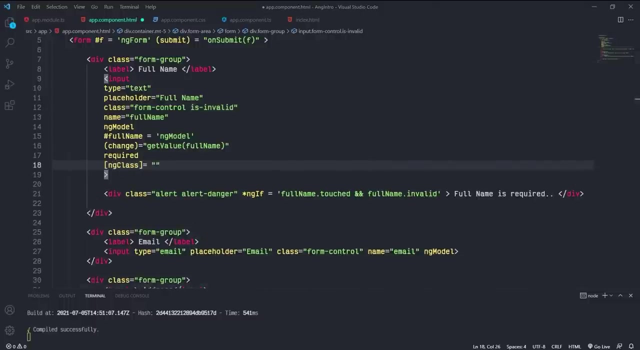 So let's do that. For this we can use class binding, But I'm gonna use the ng-class directive, which is more cleaner than class binding, Right? So inside square brackets: ng-class assign. Inside double quotes: curly brackets. 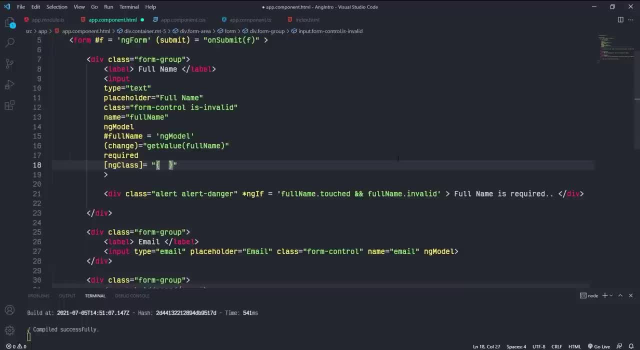 Inside this pass. this CSS class as key for this Inside single quotes is-invalid And the condition is same as this ng-if condition, So copy this and paste it here. That's it. Save this and back to the browser. Awesome. 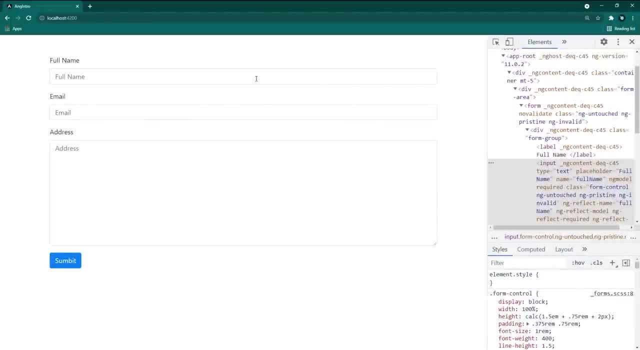 Save this and back to the browser. Look at this Now. we are not getting any errors. Touch this input and move to the next input. As you can see here, we got this error and this beautiful bootstrap validation border on this input field. 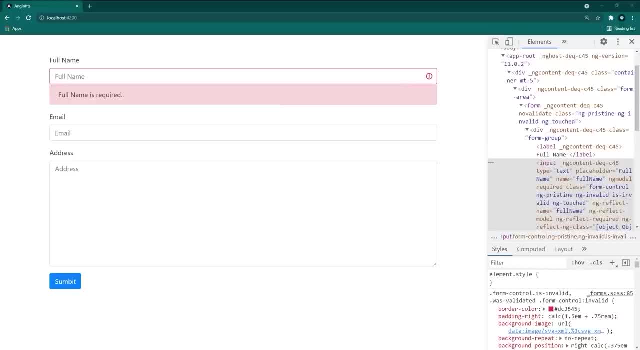 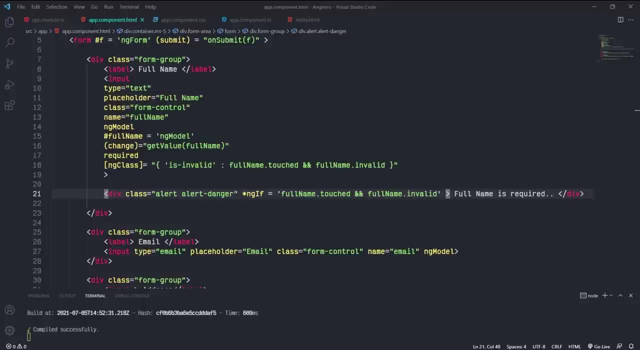 So this is how we apply validation styles to the input fields. In previous we learned about this required validator Like this in angular. we got few validators that are based on HTML validation attributes, So in this lecture let's look at them one by one. 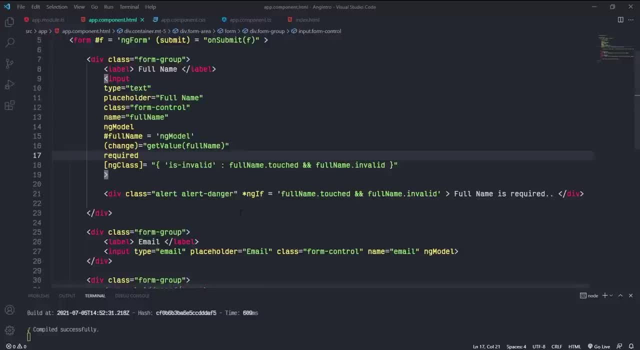 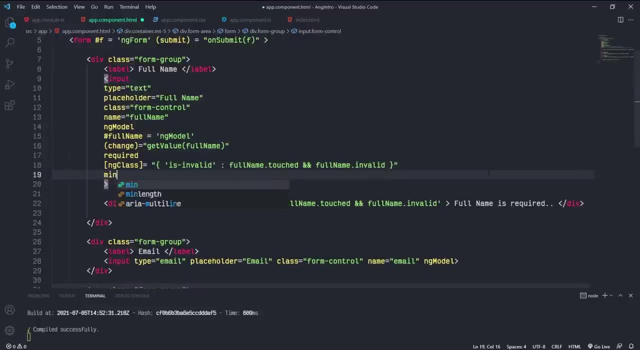 The first one is the maximum and minimum character count. So let's see this in action. First, we have to set the HTML attribute for this input: Min length and the max length, Set the min length to around 5 characters And set the max length to around 10 characters. 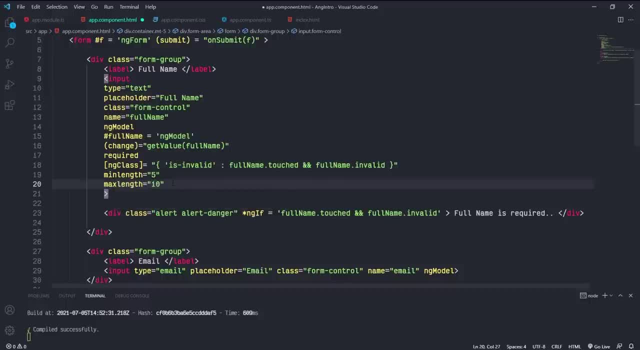 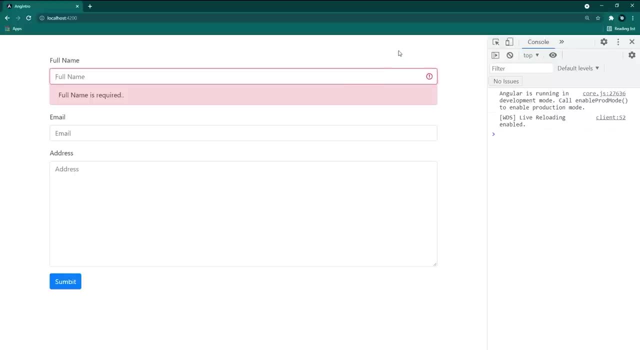 And set the max length to around 10 characters. And set the max length to around 10 characters. Alright, Save this and back to the browser. Click this input and go back. I want to show you something. We got this printed ng model inside the browser console. 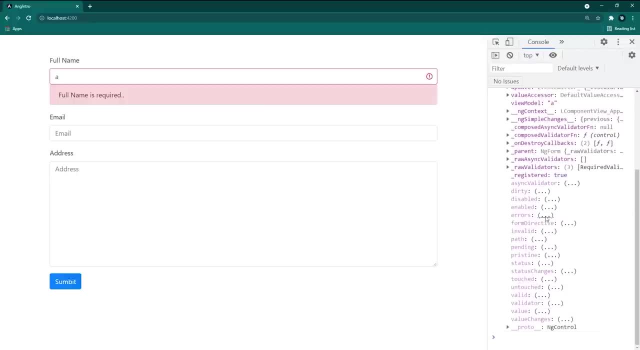 Inside this we are getting another property called errors. Inside this, as you can see, here we can find this min length error. So now let's add the error message for the min length validation. To show different validation, we have to change the length of the error. 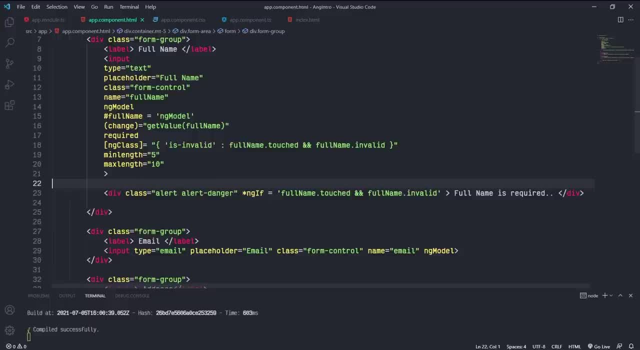 Let's go to the main menu. Set the min length to around 10 characters. errors: Let's add some changes to this error message div, Put this message text inside of another div and let's add a condition when to show this error Inside this div, ngif. 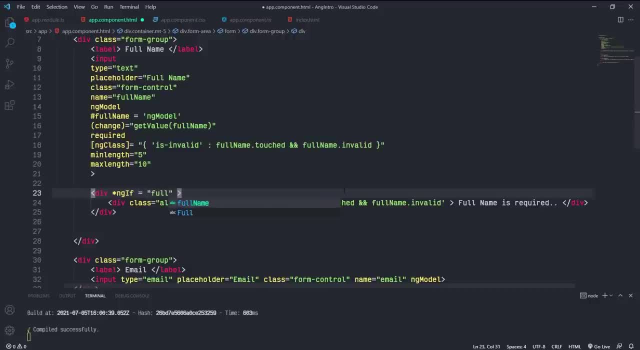 directive. the statement is full: name this template variable. This time let's use the errors property After this: errors required. So if this is true, this message will show up inside the browser Like this: add an error message for the min length: Duplicate this. 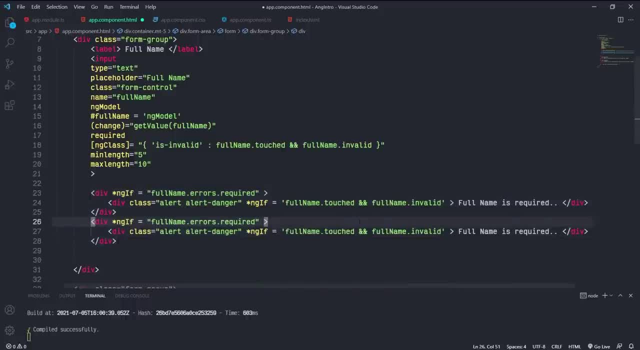 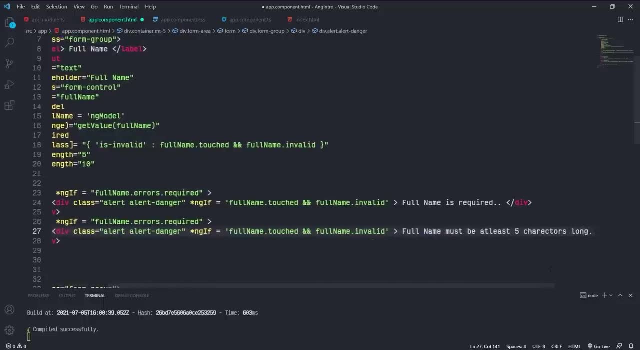 div and change the error message to full name Must be at least 5 characters long. Now change this statement. This message is for min length, So let's change this statement. This message is for min length, So let's change this statement. This message is for min length, So. 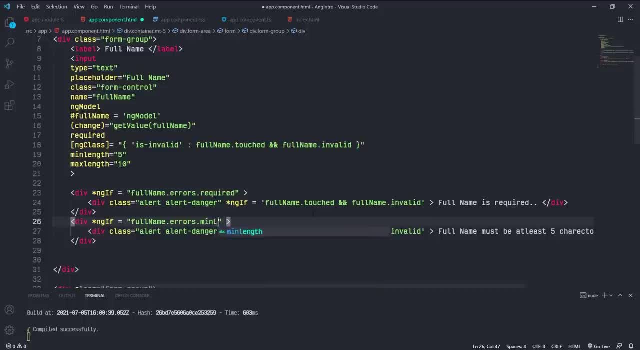 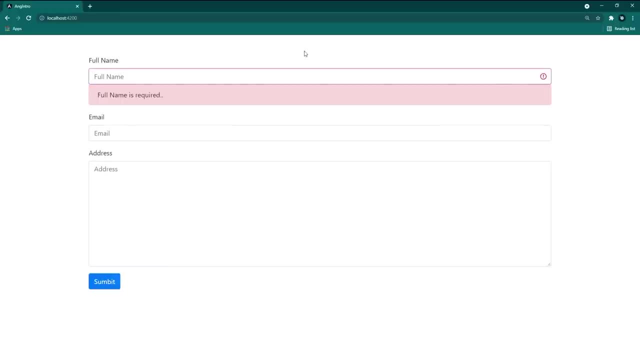 change this required to min length, all simple letters. Save this and back to the browser. Get the focus of this input. Move away. We got this required message. Now type a character here, As you can see here, now we got this min length error. Very simple, right? So this: 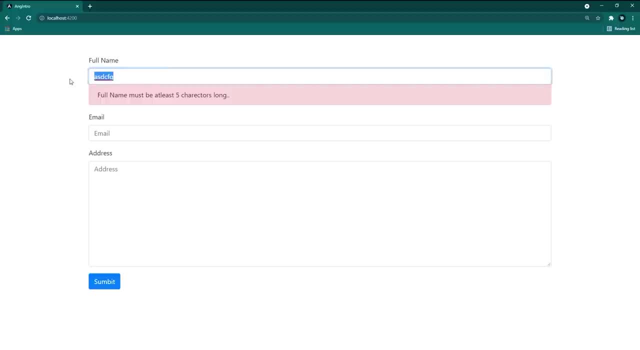 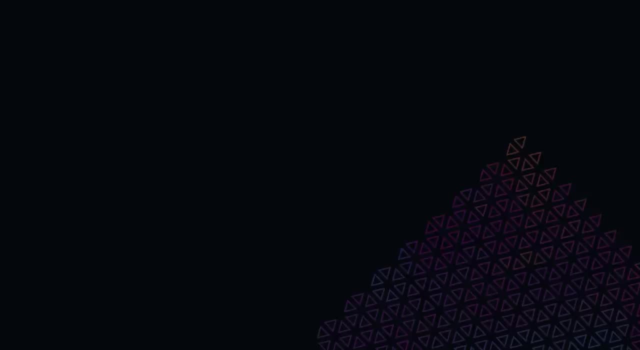 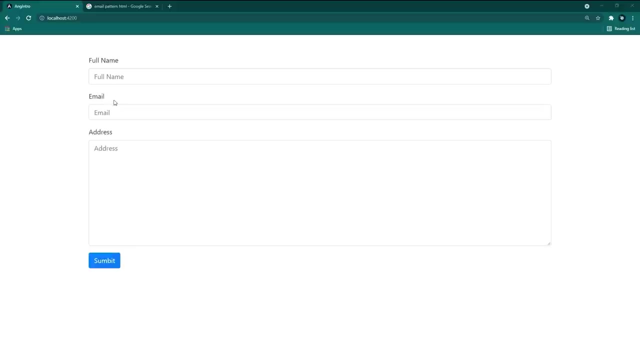 is how we handle different types of errors using the ng model. In previous lecture, we learned how to add validation to the first name field. Now let's see how to add the validation for this email field and for this text area. Let's add validation. 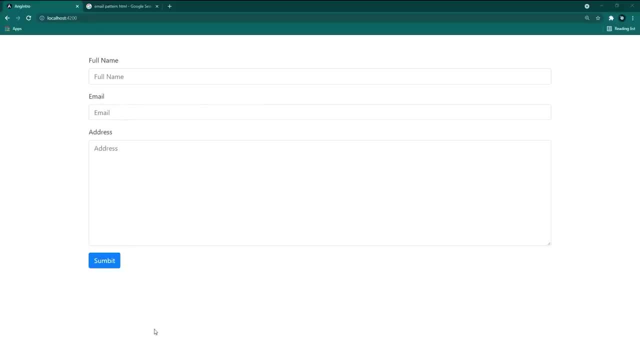 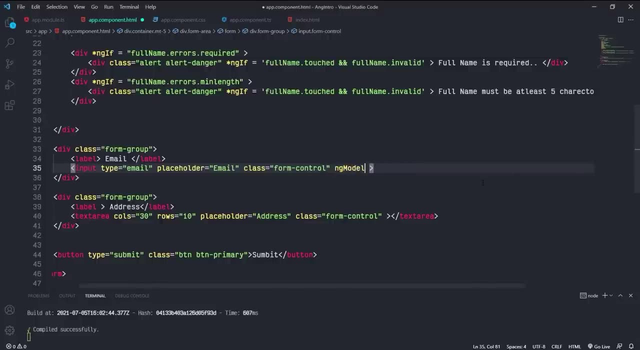 for the email input field. First add the ng model directive to make a new form control object class for this email field And always keep this in your mind when we using the ngmodel. we must declare the name attribute, So the name attribute and the value is email Create. 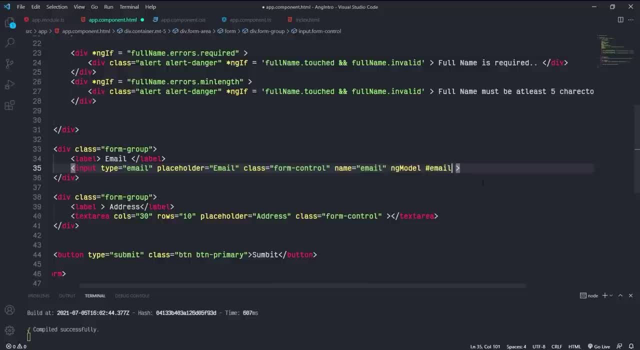 a template variable and bind that to this ngmodel Hashtag email and bind this to ngmodel. So this time to validate this email field we gonna use the pattern html attribute, So pattern Inside this. we have to pass the email pattern To get this pattern. 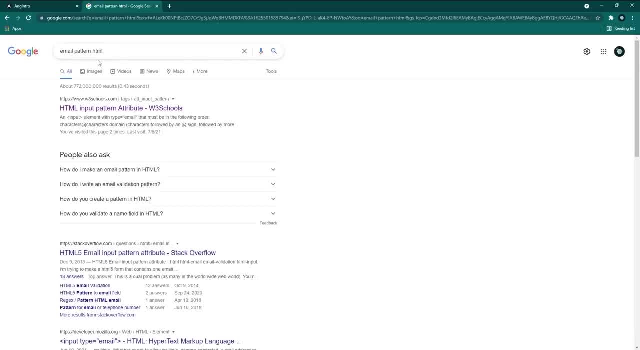 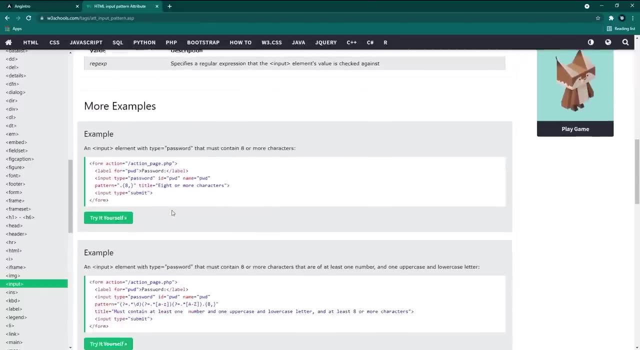 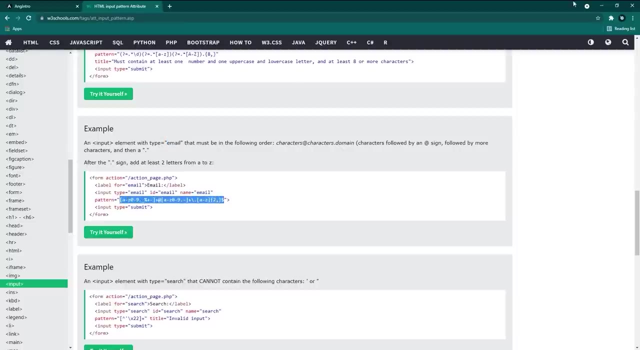 Search for email html patterns inside the google and go to this first result, w3 school website. In here we can find different patterns for different situation. Scroll down and find this email pattern, Copy this and paste it here. After this we need another validation. 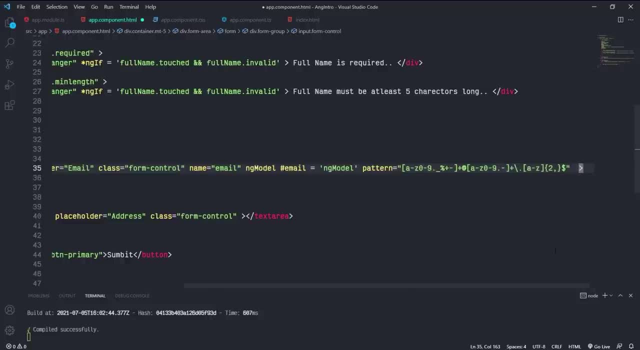 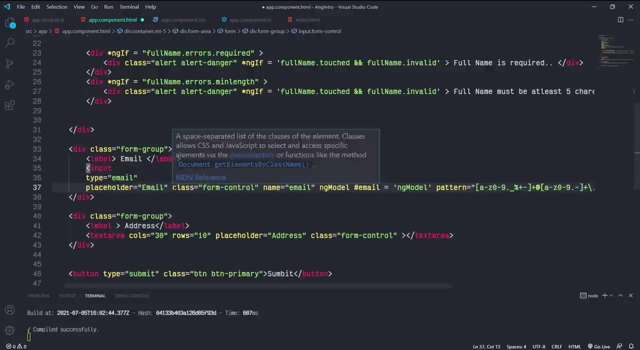 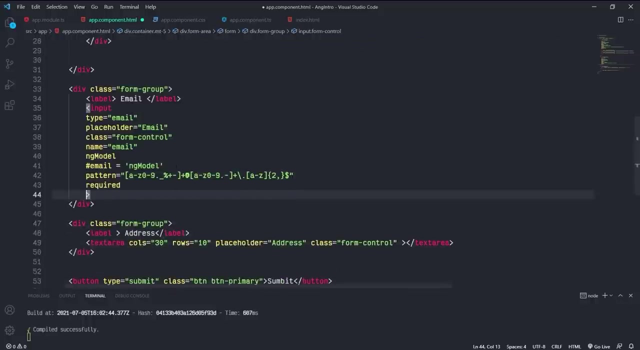 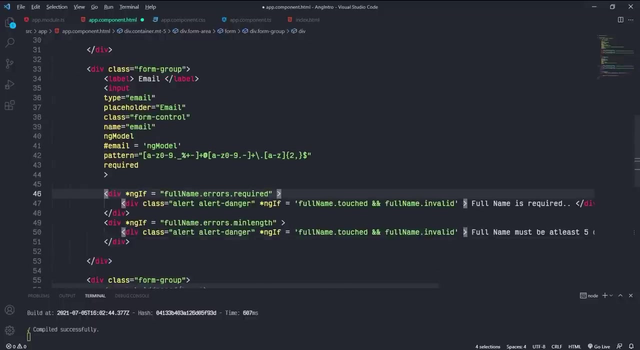 for this, which is required validation, So add that as well. Now let's define the error messages. Just copy the previous message div and paste it here. Change this conditions template variable to email. The main conditions are same, like this: Inside this: change this required template variable to email. 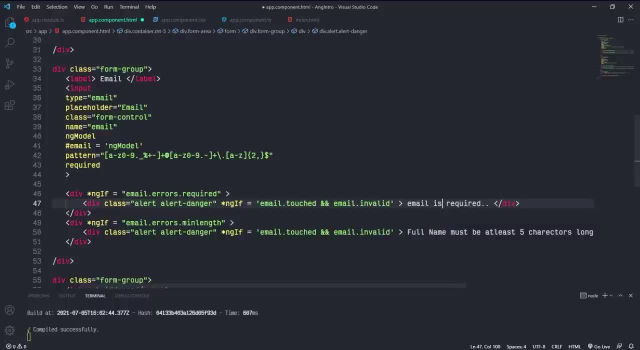 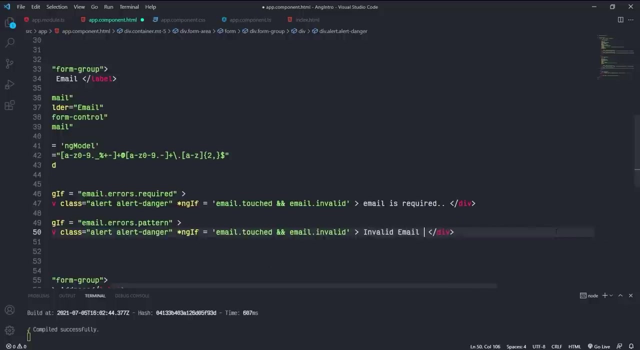 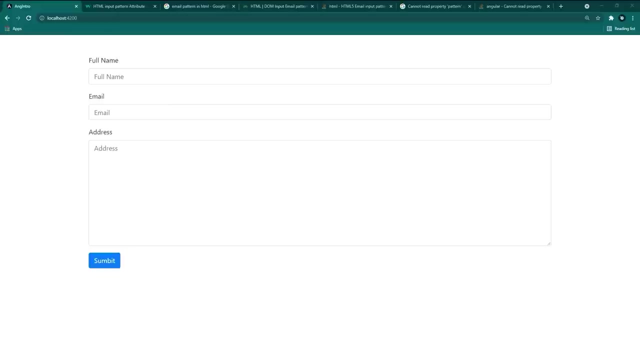 and change the message to email field is required. This time we are not using the min length, So first change the template variable name to email and change this validation property to pattern. Now change this message to invalid email address. That's it. Save this and back to the browser. Click this email field and click outside. We got. 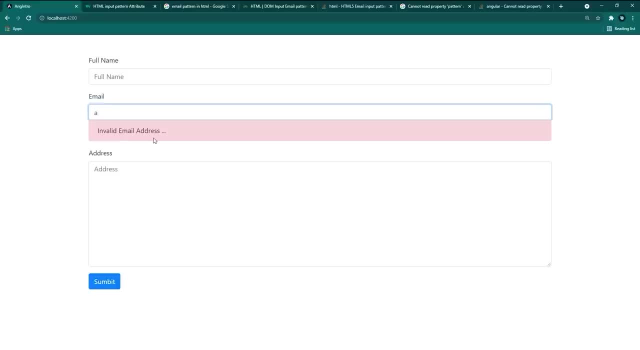 this required error. Type something: We are getting this invalid email error message. Type something: valid email address. Now we don't get any errors. Remove this at symbol. We are getting this error: invalid email address. Now we are getting this error: invalid email address. 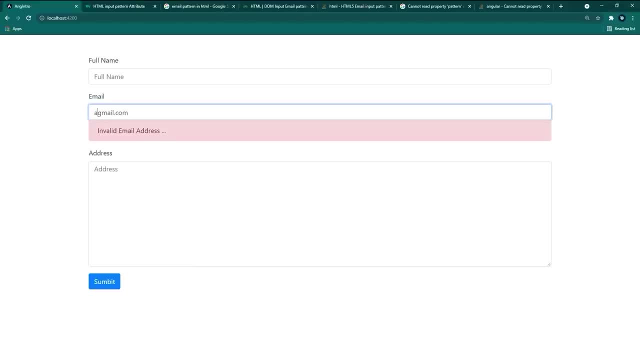 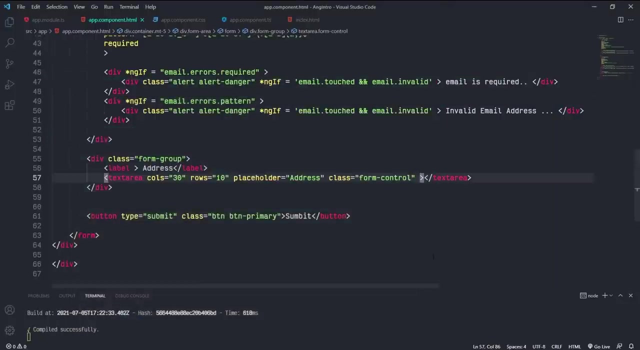 Cause this email is invalid. Looks perfect, right? So let's validate the text area. This is also the same as previous input, Nothing fancy. First enter the ng model directive and the name attribute. So this is for the address. So the name attribute will be address. After this, create a template variable and bind it to this. 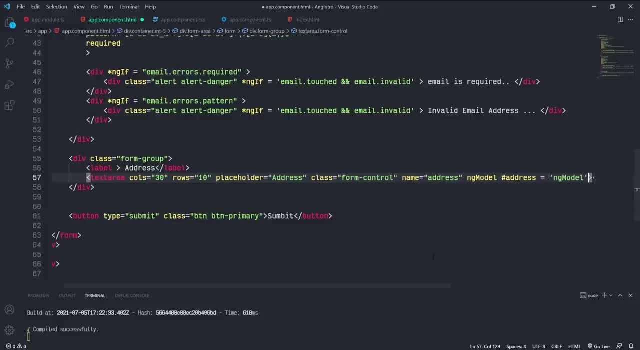 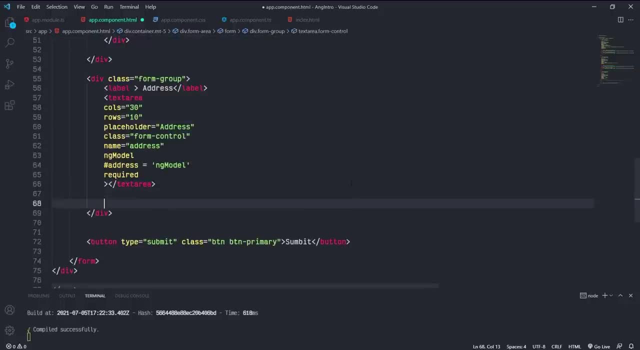 ng model. So this is for the address. So the name attribute will be address. After this, create a template variable and bind it to this ng model. The validating attribute is required. After this, add the required message here and change the template variable to the same as this address. 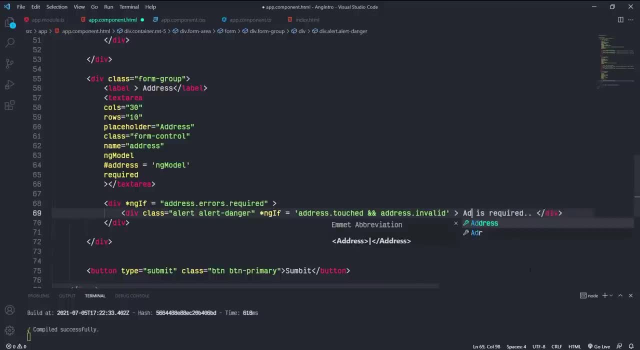 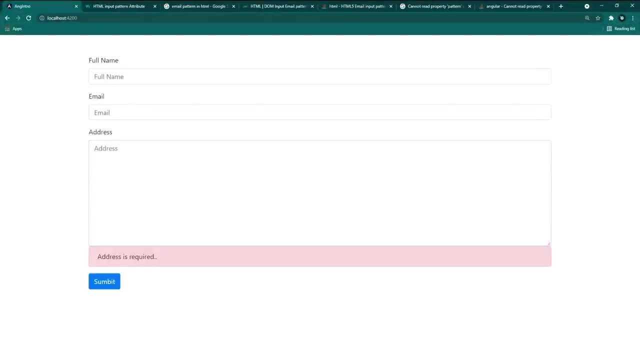 Change the message Address field is required. Save this and back to the browser. Get focus, Click outside, Perfect. We got this error message Like this: we can add validation for all the statements. Now we are getting this error message Like this: we can add validation for all the. 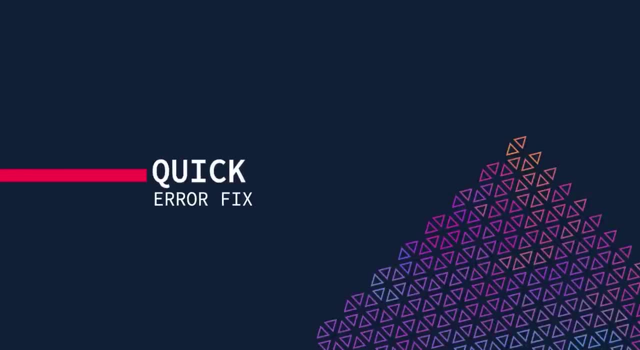 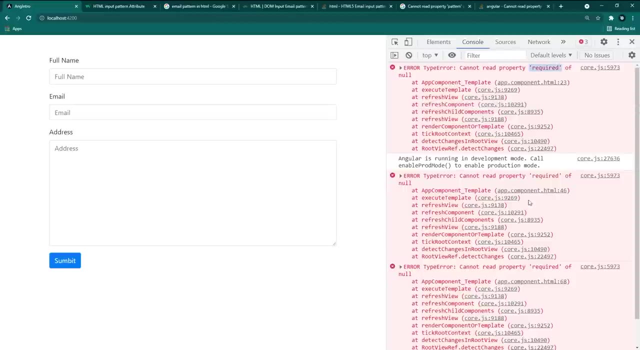 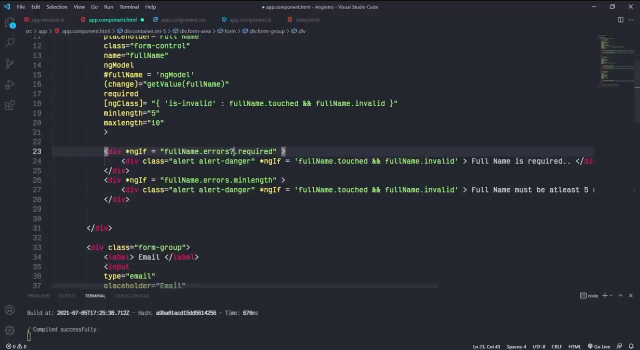 statements. Now we are getting this error message Like this: we can add validation for all the form elements. Some of you may found this error that saying cannot find required on your browser console. To fix this, just add a question mark. End of this. all error attributes. 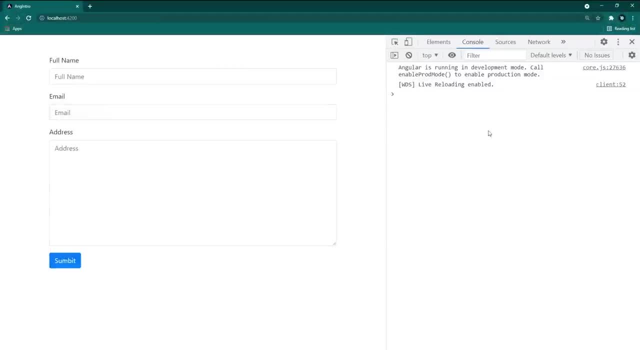 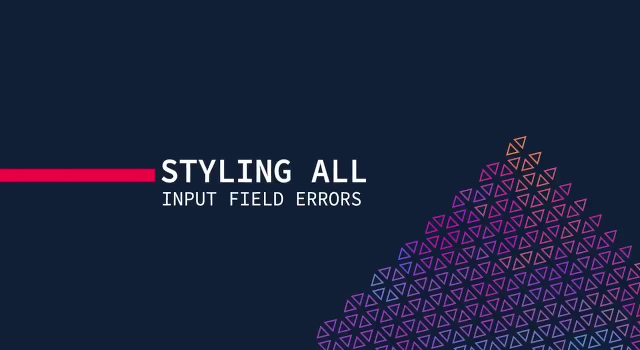 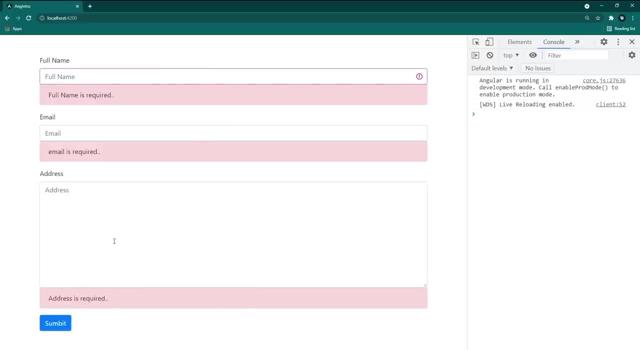 That's it. Save this all and back to the browser. Perfect. Now we are not getting that previous error. So we successfully added all the validation errors for all of these inputs. But, if you noticed, we just only added this alert message for this email and address fields, But not the input. 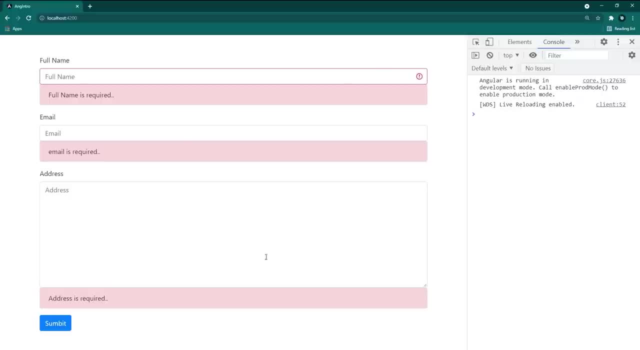 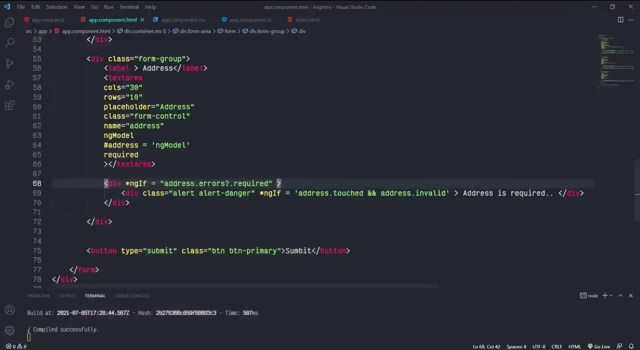 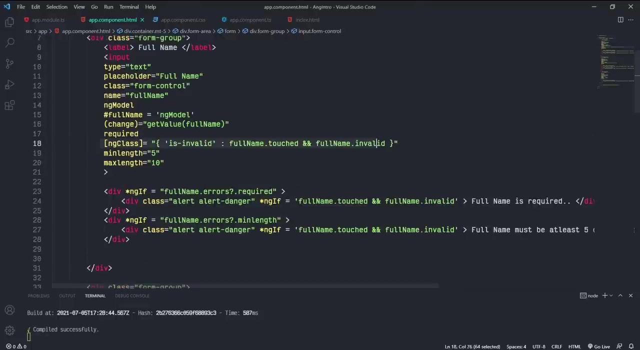 fields Error: red border, like this first input. So let's do that Very simple: Hold down the key. All we have to do is just add the is invalid bootstrap class to these inputs, conditionally using the ng class directive. Very simple, Just copy and paste ng class from this full name input. 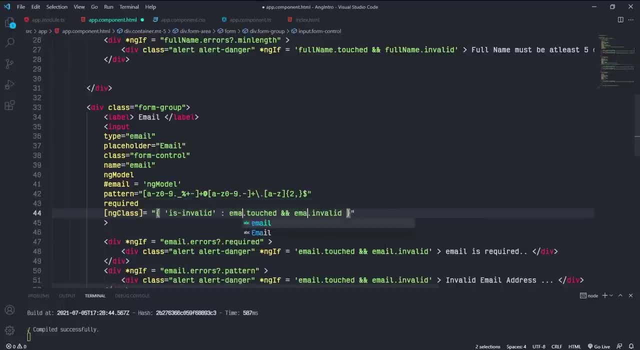 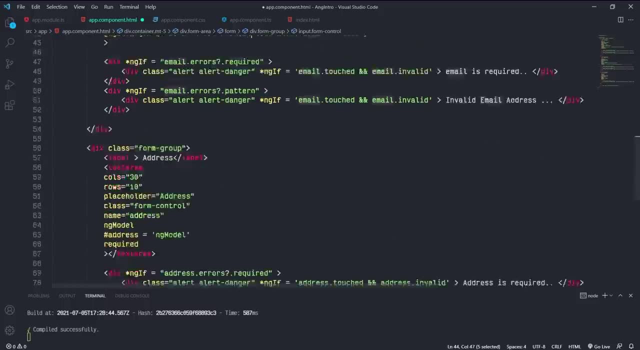 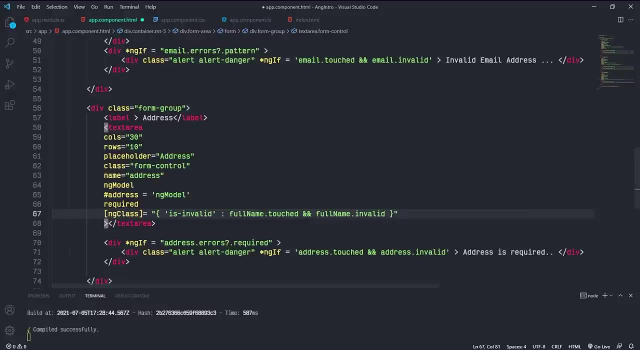 Change the template variable to email Cause. this email fields template variable is this email. That's it. Do the same for this text area. Copy and paste the ng class and change the template variable to address. Save this all and back to the browser. Perfect. 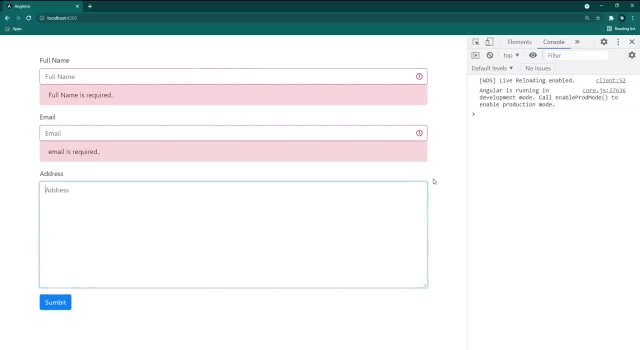 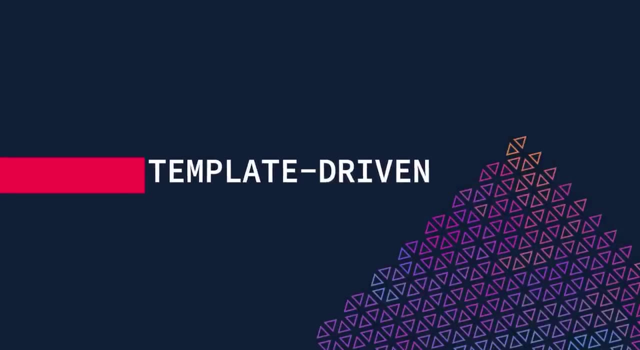 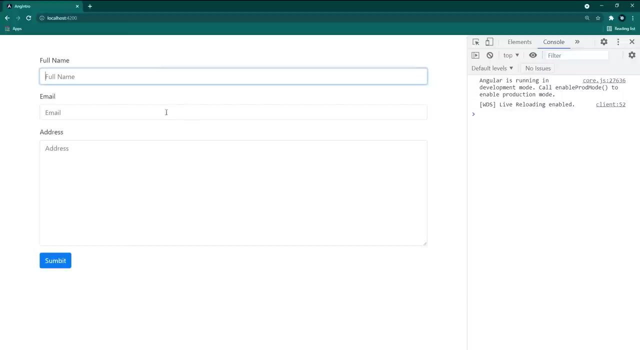 We got this red border on all these inputs Looking awesome right. So in this lecture, let's look at how to submit this form and get the values of these input fields. We kinda did this earlier when we learning in this course. We are learning in our tutorial, So let's. start. So if I click on save and go to the homepage, You can see that it's save and paste it and go to the browser. And once you click on save to the browser It will save the red border inside the node. We'll understand how we are adding the input fields And then click on save. 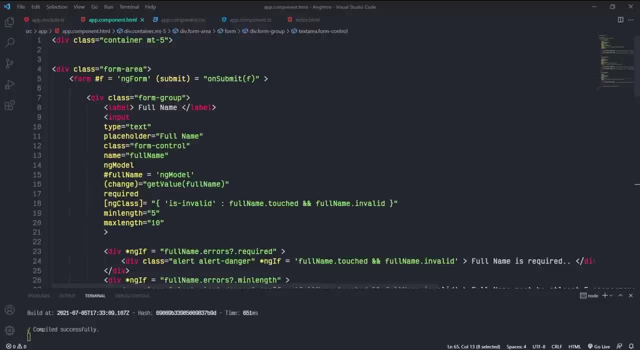 learning ng-form and form group classes To make this form submit. previously we use this submit event binding. This is the default HTML form submit event. This is okay. but in angular we got another separate directive for form submission, which is ng-submit. From now on we will use this ng-form directive to form submissions. Alright, so first change. 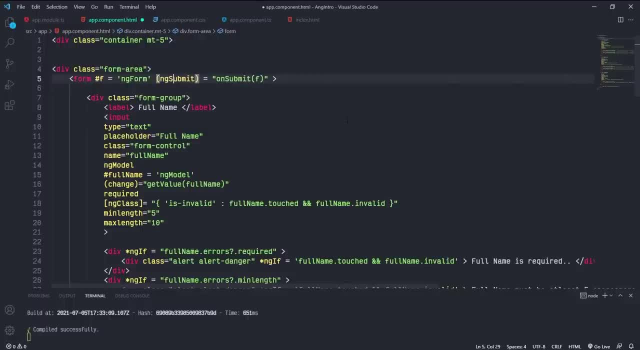 the submit event to ng-submit. This also like the same submit event- nothing fancy. So in order to access this forms values and validation status, we use this ng-form directive, which is creates the new class object of angular-form-group-class Right. we learned about this earlier With 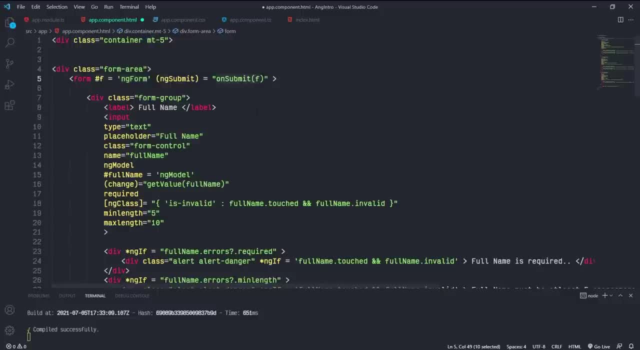 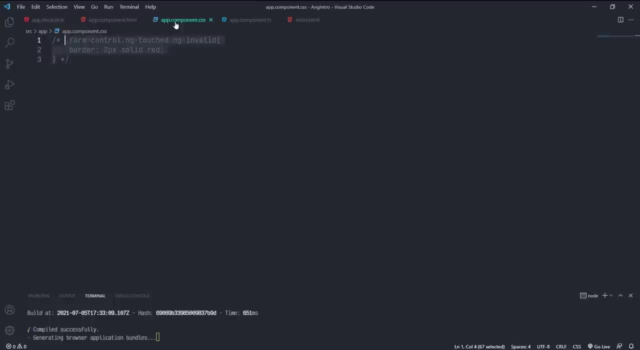 this ng-submit, we call a method called onSubmit. With this onSubmit we pass this ng-forms template variable From inside- the component is five- While we have this onSubmit method and with this we are logging this ng-form parameter variable inside the browser console. So now save this all and back to the browser Fill. 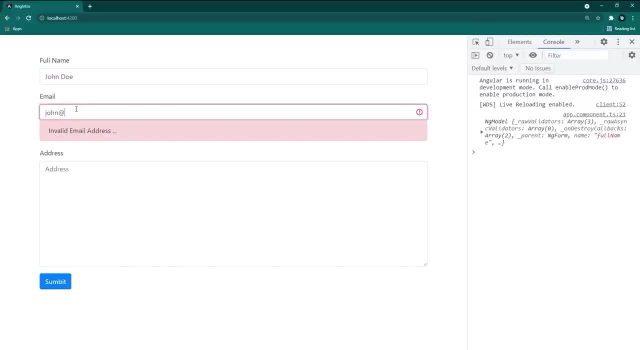 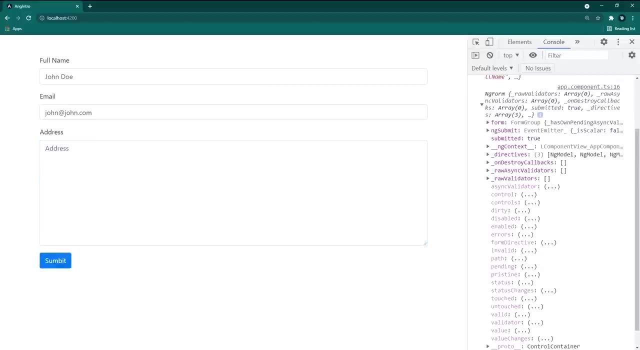 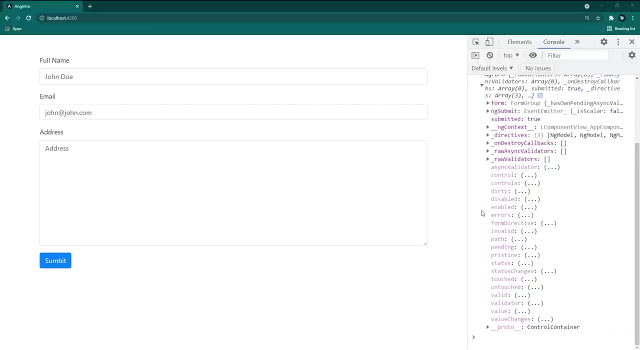 this form and click this submit button. Now look inside the browser console. we got this ng-form. This also same like the ng-model. We got all the properties inside the ng-model here. With this we can check whether the ng-model is working or not. 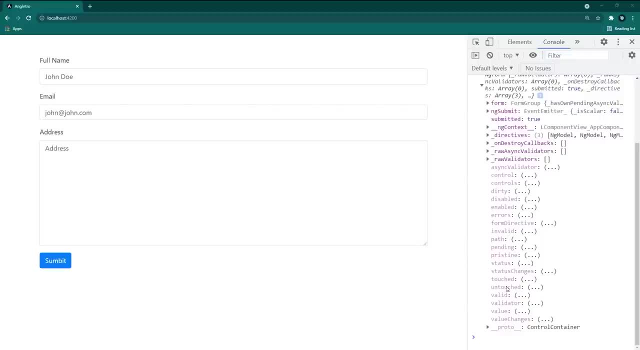 With this we can check whether the ng-model is working or not. With this, we can check whether this form is valid or invalid, dirty or pristine, etc. If we look this further, as you can see, here we got this value property. Expand it, which. 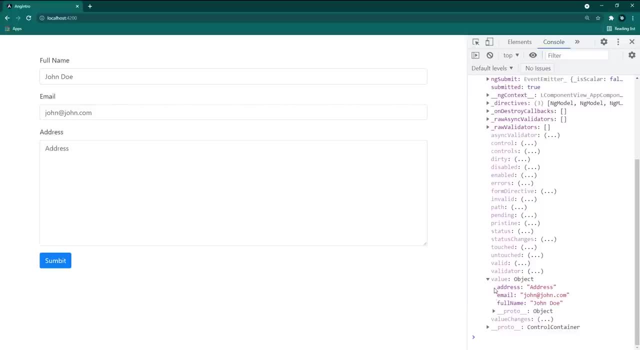 giving us the object type data. Now expand this. we got this full name, email and address data, key value pairs Which we type inside the input fields. By using this, we can access this forms type data values. By using this, we can access this forms type data values. 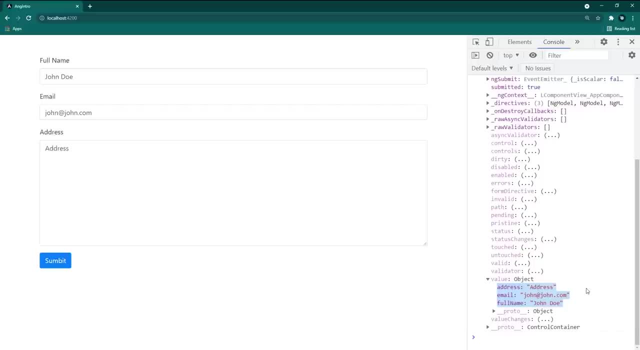 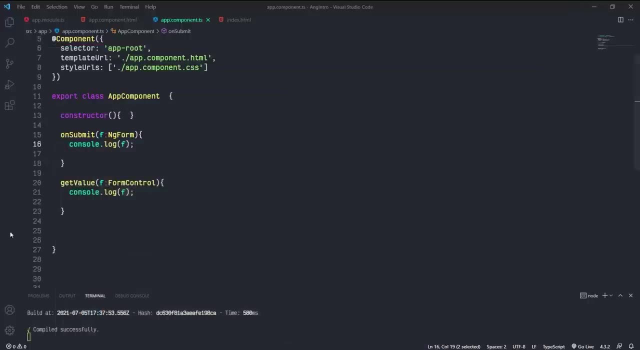 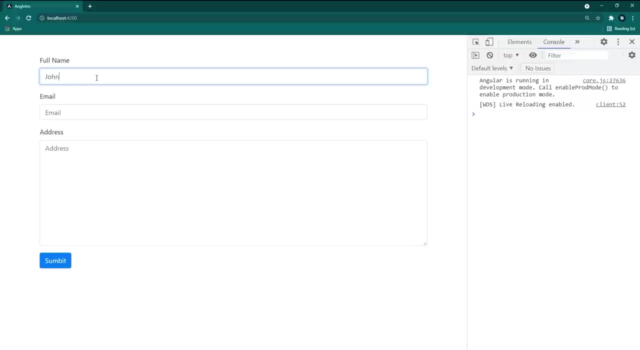 And set it to the database API endpoint and save this data inside the database. So now let's log this value inside the log Values property is inside this ng-form value. So after this dot value, this is this value. Save this and back to the browser. Fill this. 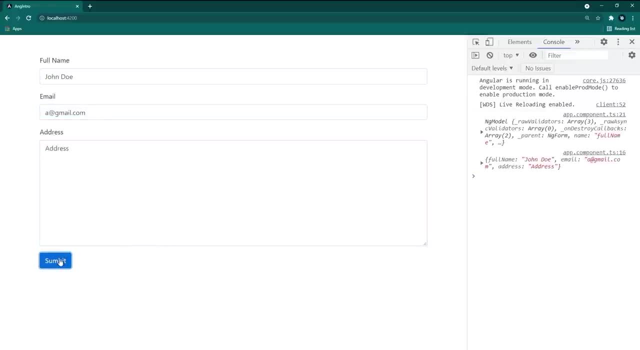 form and submit this form Inside this. we got this value object. Now we can, using this value object, we can save this data inside of a database. In the previous section we learned how to submit a form and how to get the form values, But we have a small problem here If I submit this form without filling this form Still, 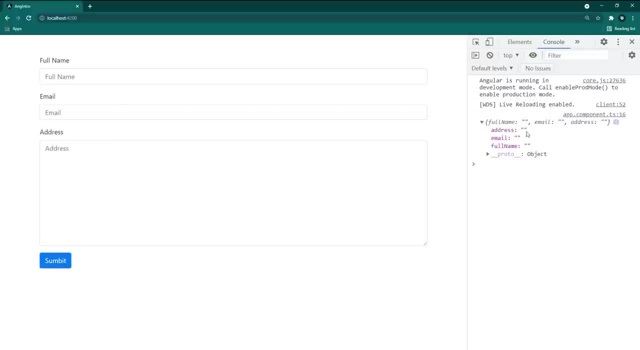 we are submitting this form, but inside the terminal Look at this value objects. All the values for these fields are not filled, So we have to submit this form without filling this form. All these fields are empty, So passing this form with empty data is not. 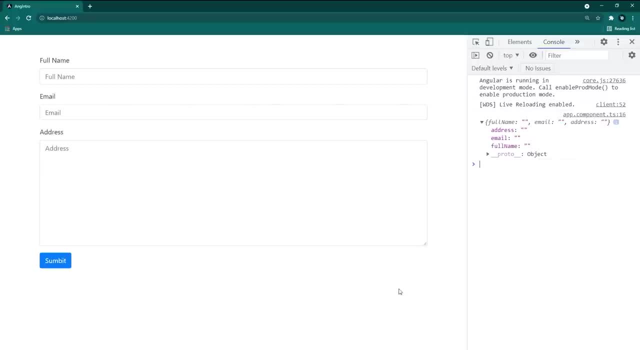 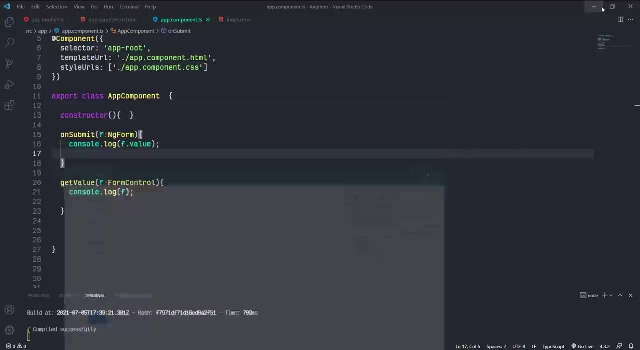 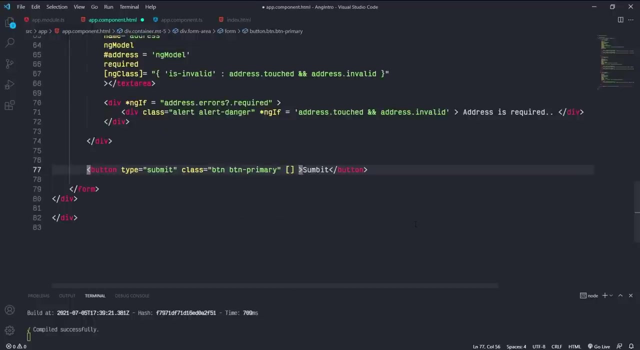 a good practice. So, as a solution for this, we can disable this submit button if this form is empty or invalid. This is very simple. For this we gonna use the property binding method Inside this button: tag: property binding- square brackets Inside this: the property that we want to bind disable. 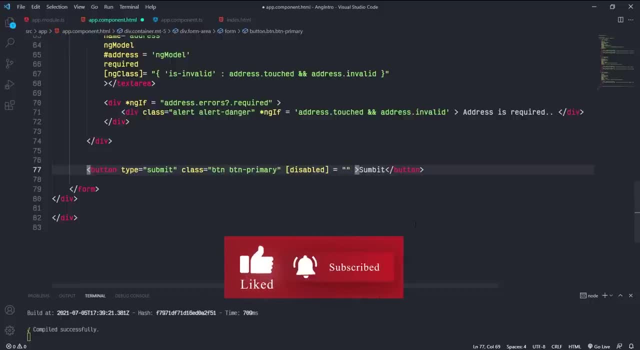 Now the statement: So we want to bind this disabled property To this button when this form is invalid. So the forms template variable is this f. So f dot invalid. When this form is invalid, this property becomes true. Therefore, this disabled property will bound to this button If this form is valid. this invalid property. 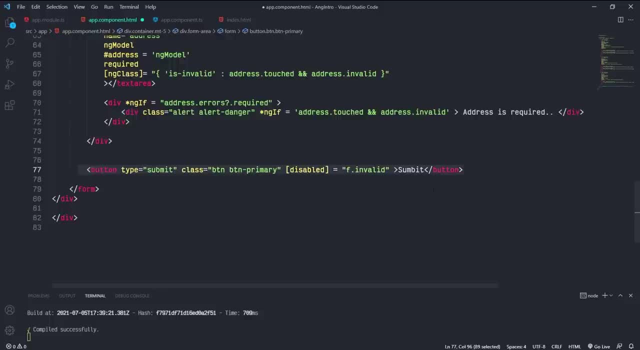 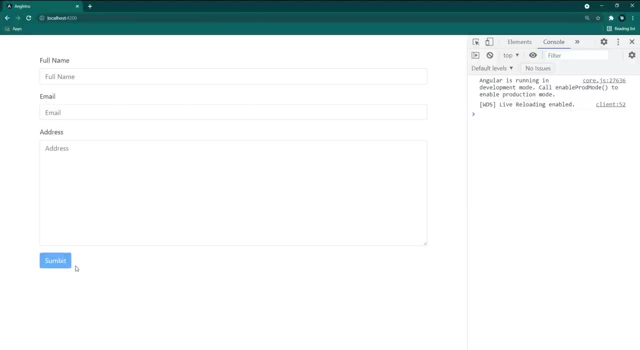 becomes false and this will remove the disabled property from this button. So let's see this in action. Save this all And back to the browser. Look at this button now. It's disabled. Cause this form is invalid. Fill this form correctly. Look at this button Now. this button is active. Cause now this: 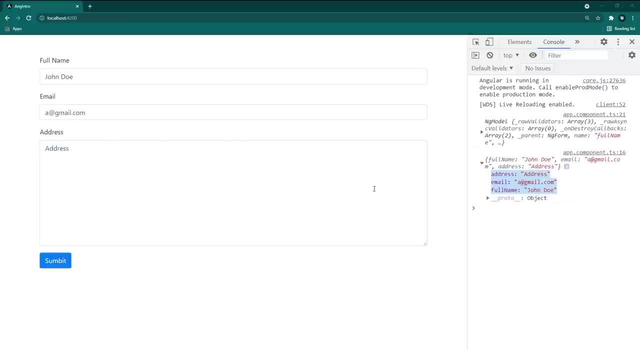 form is valid. Think if I made a mistake with this email. Soon after I make this mistake in this email field, this form becomes invalid. This button got disabled, So this is the end of this video. Thank you for watching. This is the beauty of form validations. Now we cannot pass invalid data to the database. 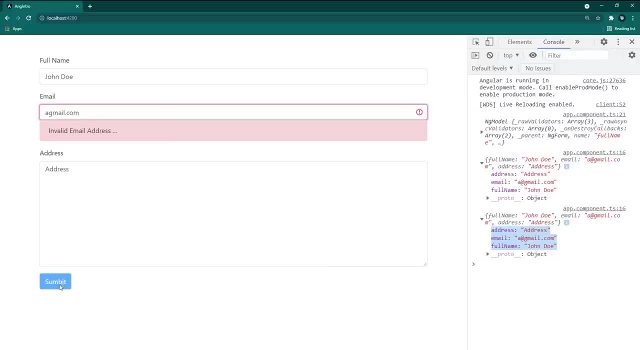 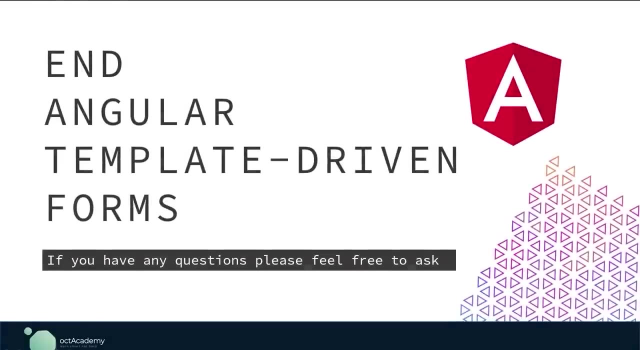 which make our app more robust. So this is how we enable and disable submit buttons according to the forms validity. So this is it for the angular template driven forms section. In this section, we learned all about angular template driven form and how to use them. How to validate the input. 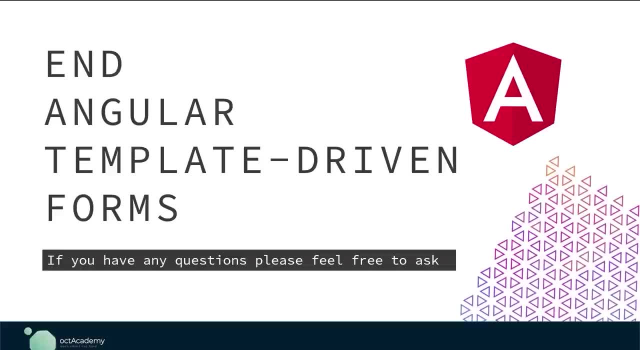 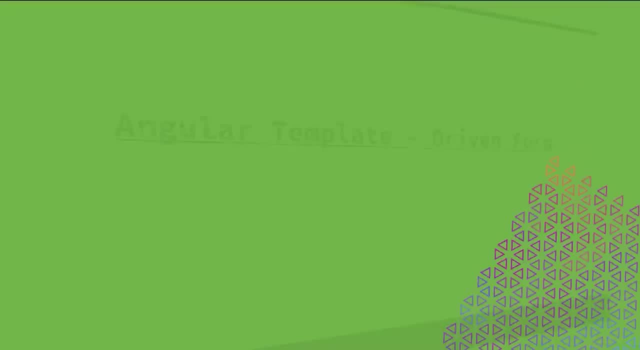 fields, How to get values from input fields and how to enable- disable Submit buttons. Hope you guys learned this well. If you have any question, please feel free to ask. So this is it. Let's meet you in the next lecture. In this section we gonna learn about angular reactive forms and how to use an angular reactive. 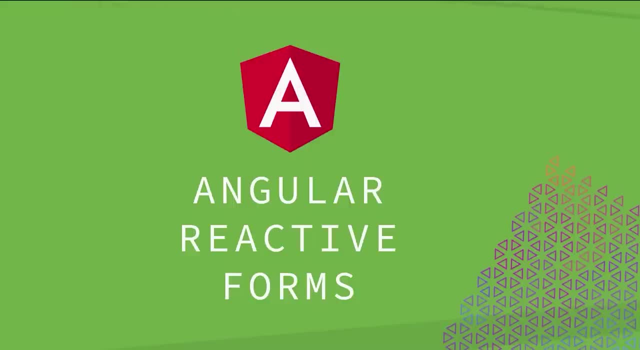 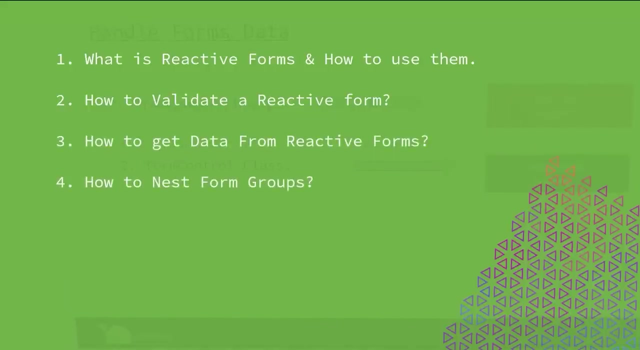 form in our angular form, step by step. By the end of this video, you will learn what is angular reactive form and how to use them: How to validate a reactive form, How to use a reactive form, How to get data from reactive forms, How to nest form groups And also. 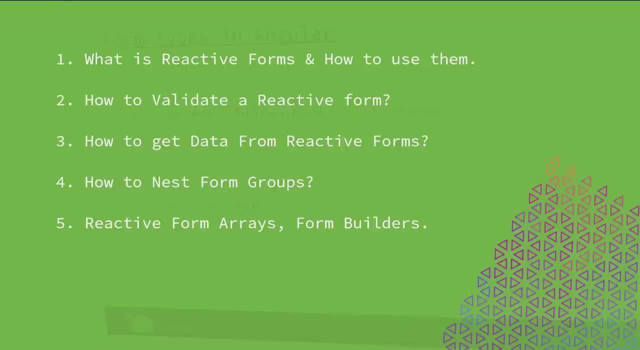 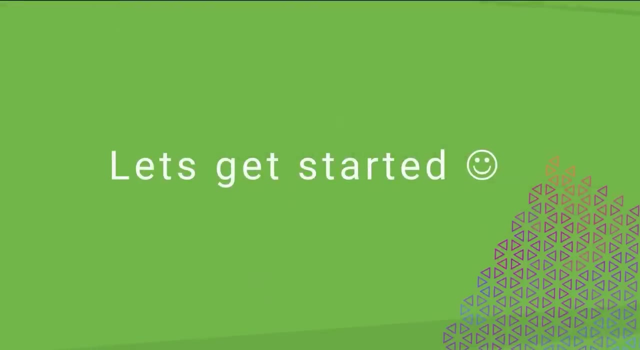 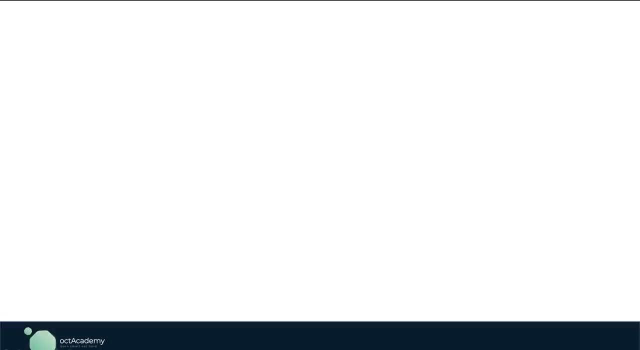 we gonna learn about form arrays, form builders and custom form validators. What are you waiting for? let's get started. In the previous section, we learned about angular template driven forms, So in that section I gave you small idea about what are the form types. in angular, We have two form types. 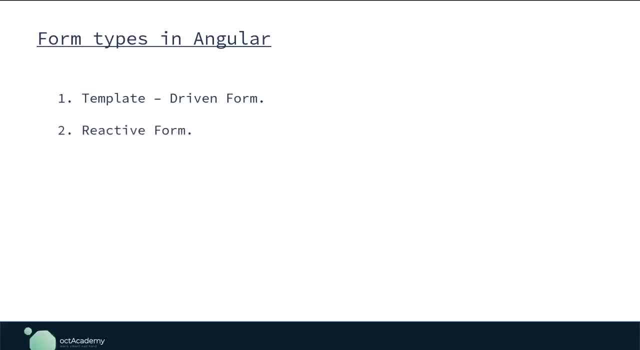 which are angular, template driven form and reactive form. So in angular we have form group class and form controller class. So in order to make an HTML form to an angular form, We have to make a new instance of these form group and form controller class. We make form group class new instance for form tag and we make 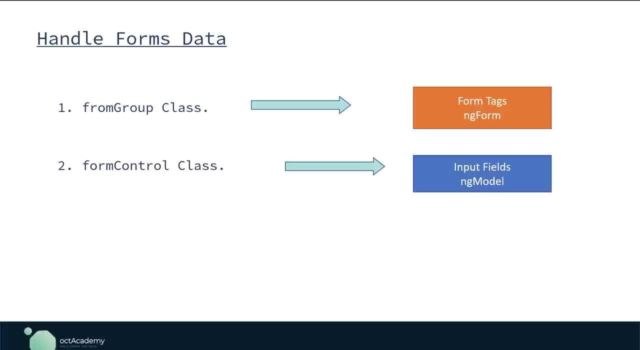 form control: new instance for each and every input inside the form In template driven forms. we created this using two directives called ngForm and ngModel. So in the template driven form we did all the declaration validation almost inside the HTML view page. But in reactive forms we will do all the declaration and validation and almost everything from. 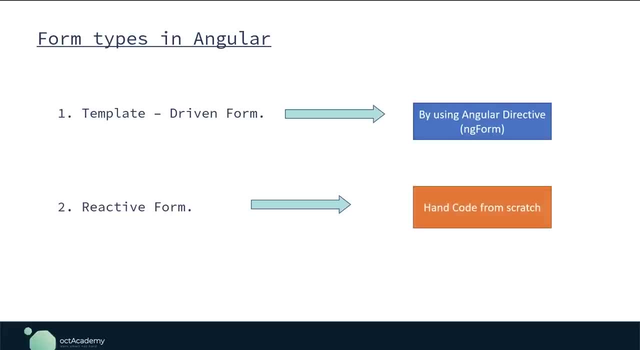 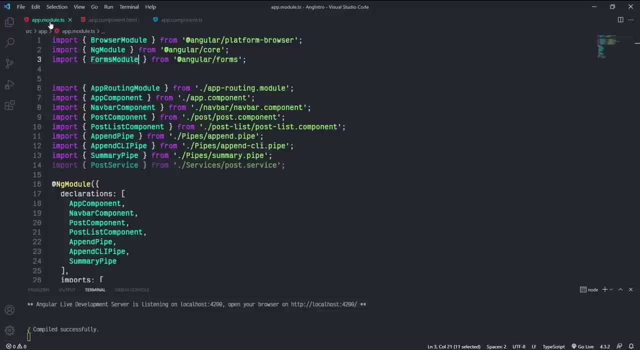 scratch inside the component file. So let's see this in action. So first thing: first we have to import and register the reactive forms module. So go to the app module ts file In here let's import the reactive forms module. Import reactive forms module from at angular slash forms. 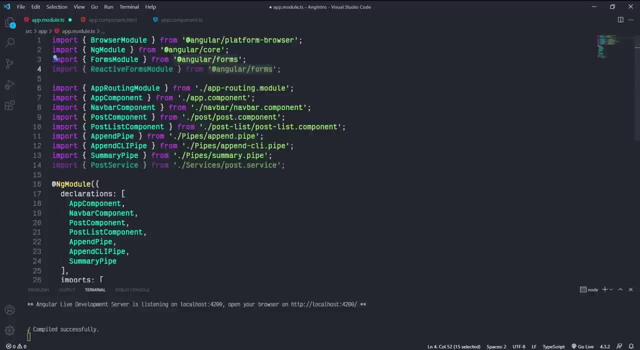 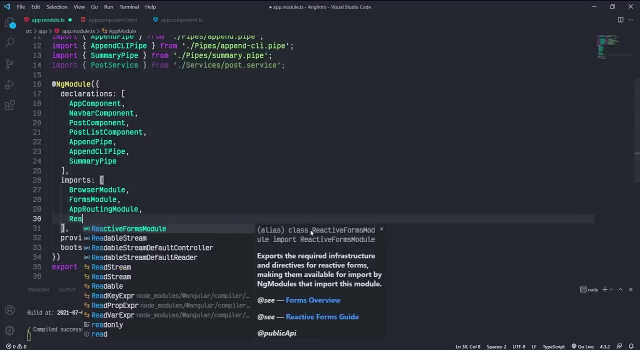 This also coming from the angular forms, like this forms module, So we don't need the These two import statement here. Just put this reactive forms module after this forms module import and don't forget to add a comma to separate these two modules. All right, now let's register this under imports- reactive forms module. 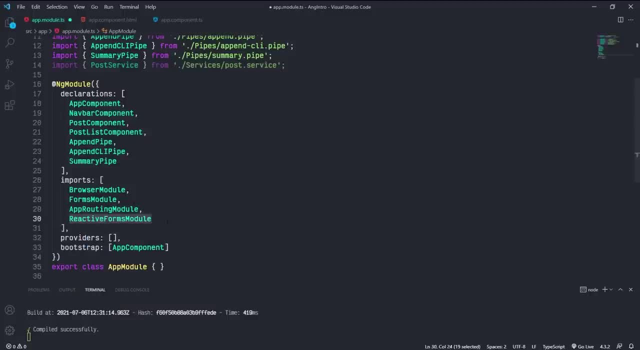 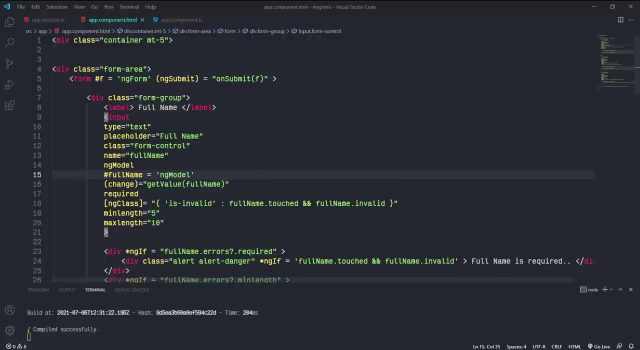 That's it. We have successfully registered the reactive forms module. Next, let's create a simple form For this. I'm going to use the same bootstrap form as the previous. Then we can understand The difference between template driven form and the reactive forms. 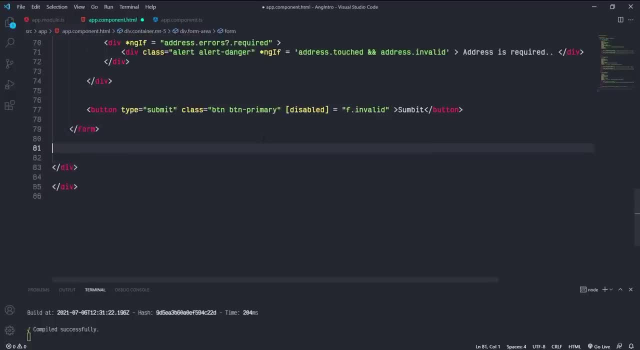 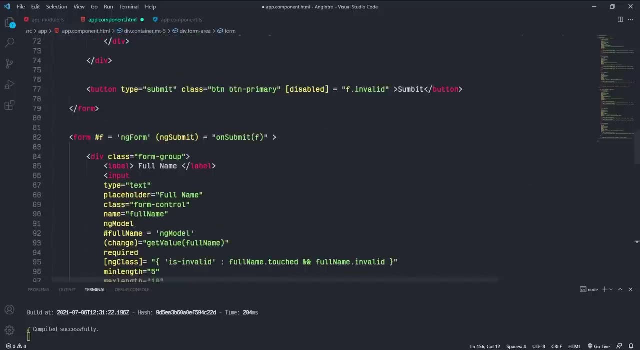 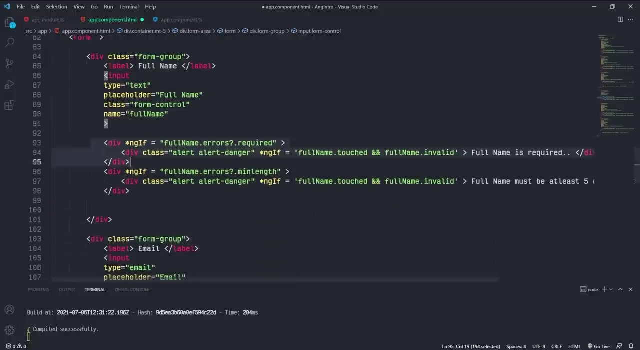 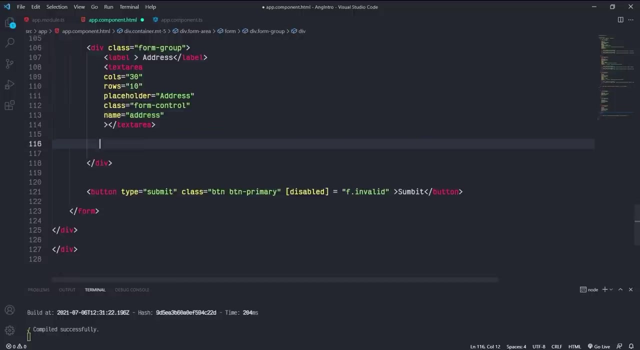 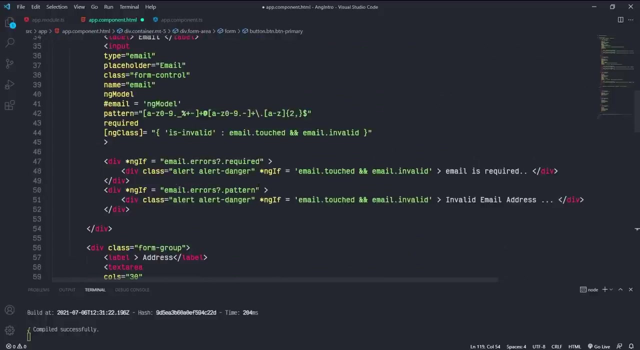 So let's copy and paste the previous bootstrap from here. Remove this all, ng-form, ng-model and validations, ng-if and all. Just keep this as a default bootstrap form. All right, the bootstrap form is ready. Save this and go to the browser. 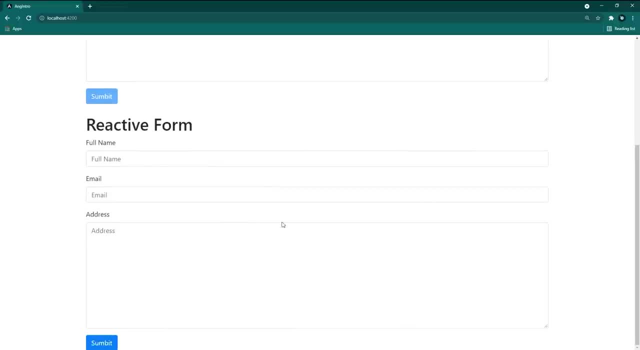 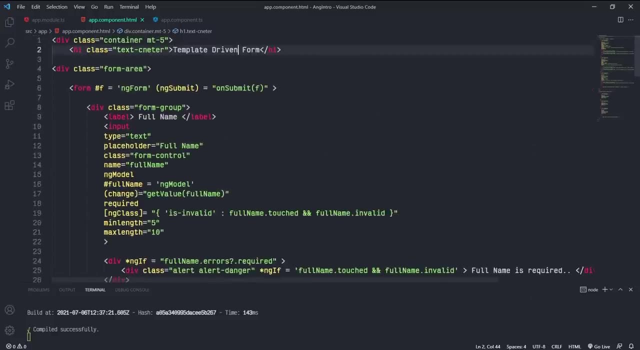 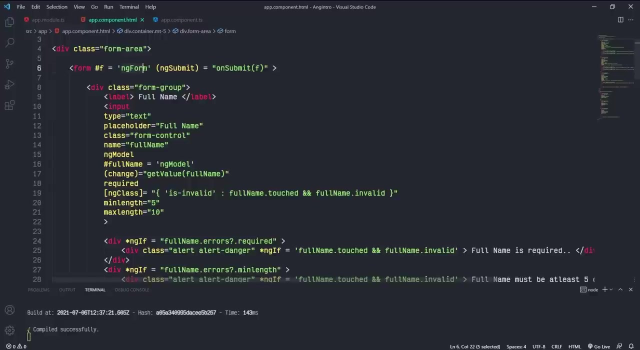 Everything looks perfect. Let's get to the real business. In order to handle angular forms, we have to use the form group and form control classes. In the previous, we used the ng-model and ng-form directly. In the previous, we used the ng-model and ng-form directly. 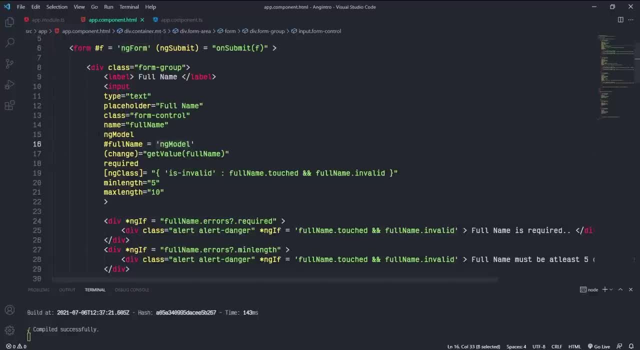 In the previous we used the ng-model and ng-form directly, But in reactive form we will not be going to use any of the directives. We will use this from scratch by writing codes, But in reactive form we will not be going to use any of the directives. 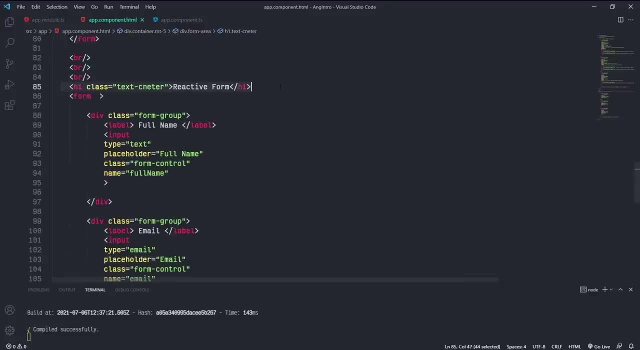 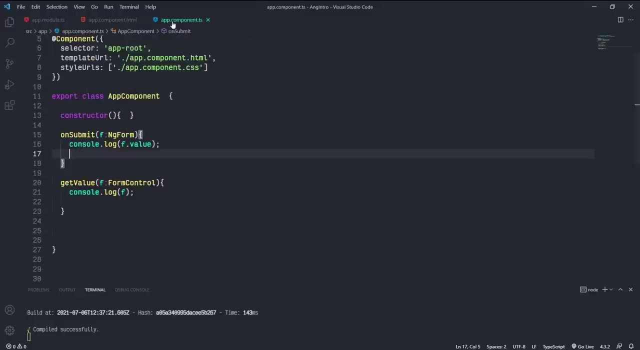 We will do this from scratch, all by writing codes. So let's see this in action. First we have to import two modules, So go to the app componentes file Inside this. First let's add the import. After this import, The first module that we want to import is form group. 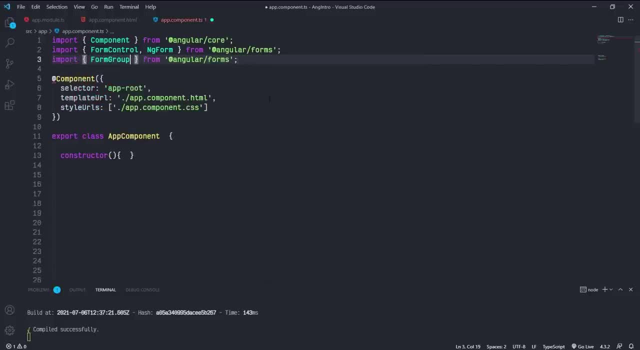 So this F and G is capital After this form group. this is coming from the forms module, So import this at angular slash forms, The next module also coming from this same angular forms. So add this second import also inside this same import. 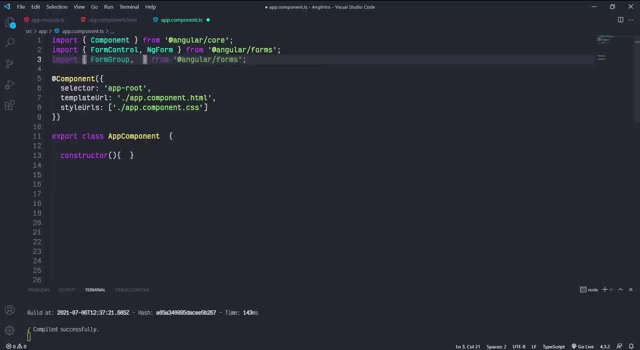 After this form group module, add a comma, and the second module is form control. That's it. So first we have to create a new instance of form group class, So let's create this inside the component class. First, the variable: something form. this can be any name. 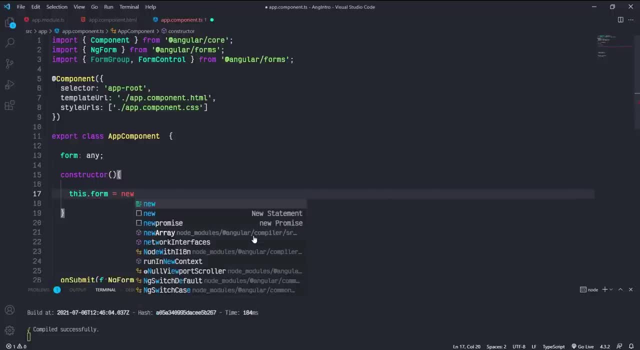 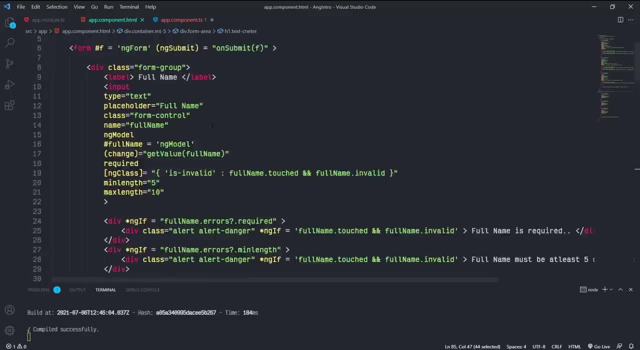 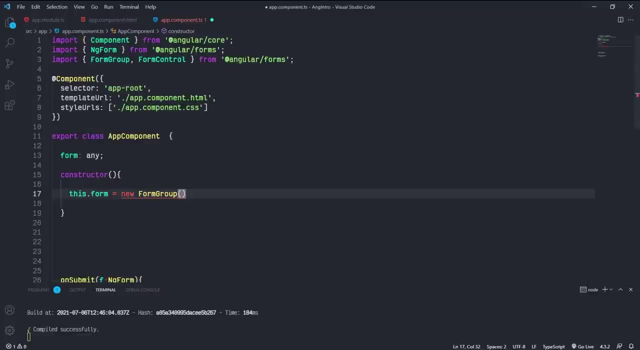 So, after this, assign new keyword, then form group and the parenthesis. In previous we did this using the ng form. If you can remember, We assign this ng form directive to a template variable- The something we did here, same as the previous. So this is the variable and we created the form group's new instance programmatically. 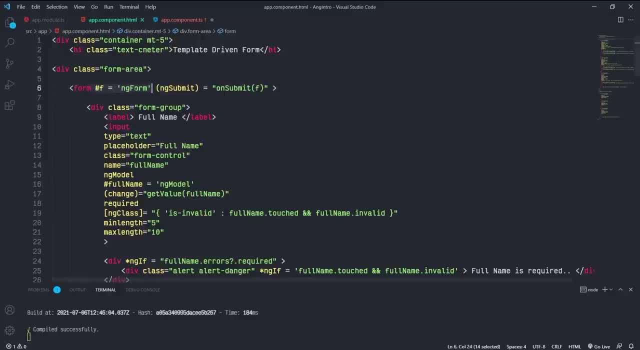 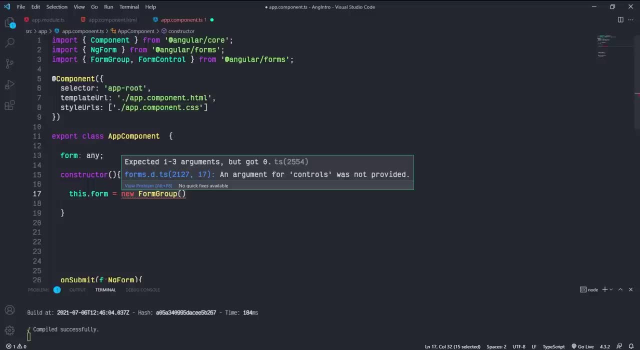 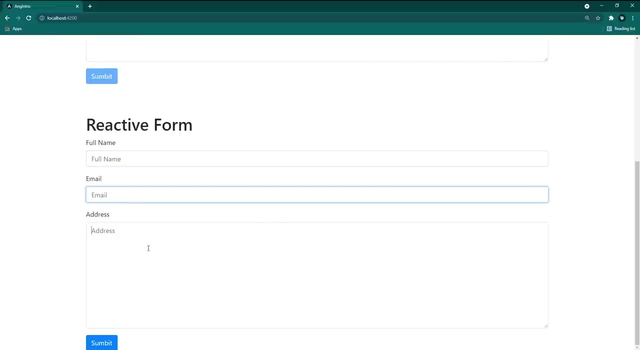 In template driven. this is automatically generated by this ng form directive, Alright. next, this form group instance required a parameter object of form controls, So let's do that. Add this parenthesis. Create an object. Open and close the curly brackets As a key value pair. create new form control. new instance for each of these input fields. 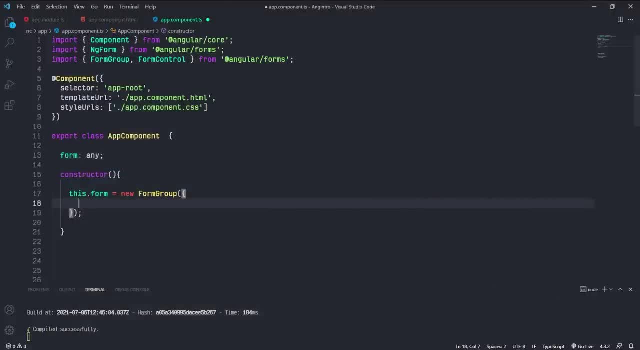 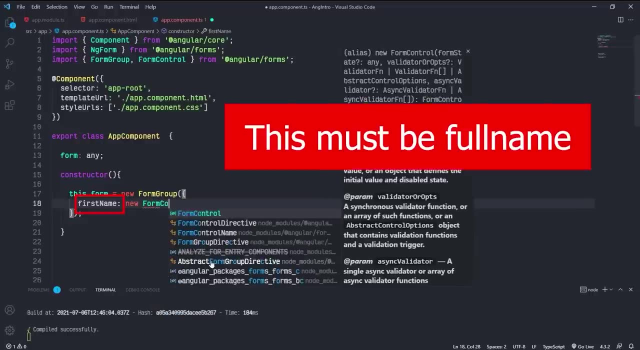 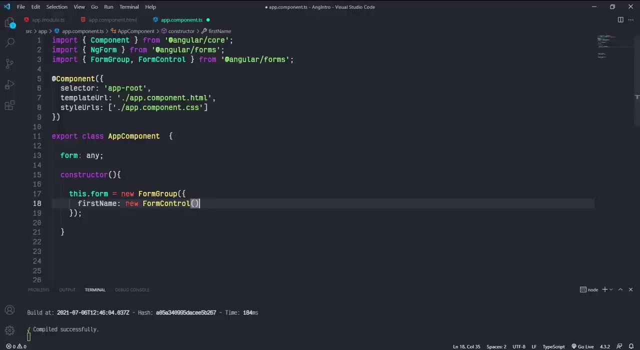 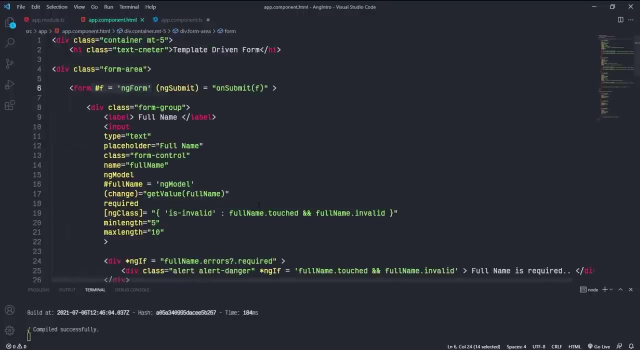 So first we have the full name field, So the first key is full name colon and value is new form control, which is this imported form control. So after this, don't forget to add the parenthesis. So with this we are creating a new form control instance for this first name input field. 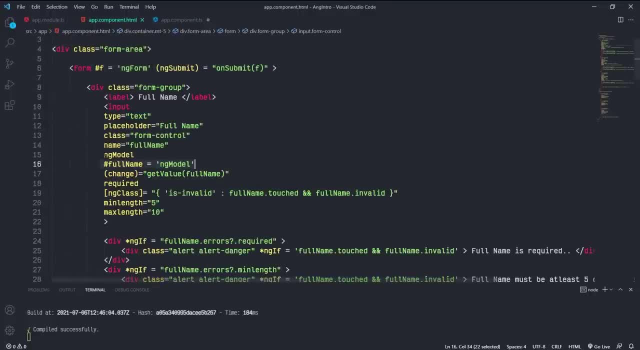 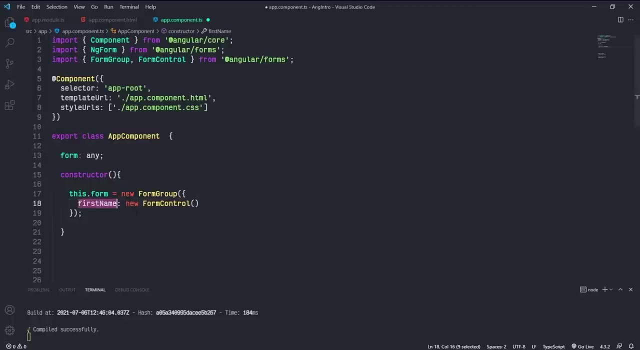 In previous, if you can remember, we created this using the ng model directive. When using the ng model directive, we required the name attribute of this input. The same thing happening here. This is the name. Now we pass this as the key of this object. 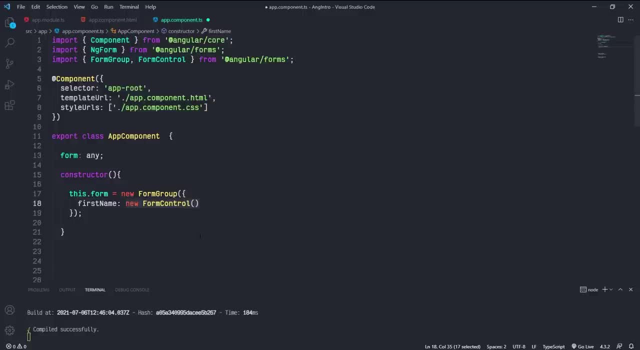 And this is the ng model. Now we do this. We did this by hand coding. That's the difference between reactive and template driven form. Hope you guys got the idea Alright. next, again create another key value pair for the email. The key is email. 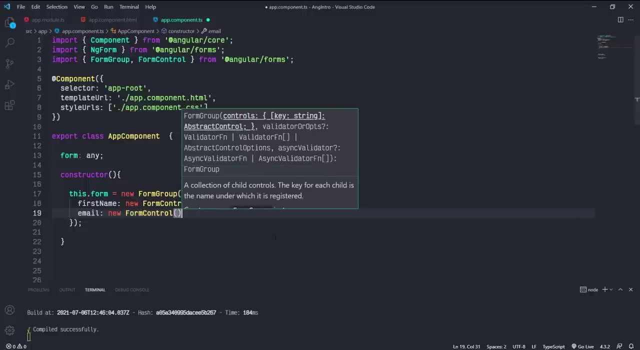 And value is new form control. Inside of a form group we can have multiple form controls. Next, at last we got this address. So the key is address And the value is the same as the previous: New form control. That's it. 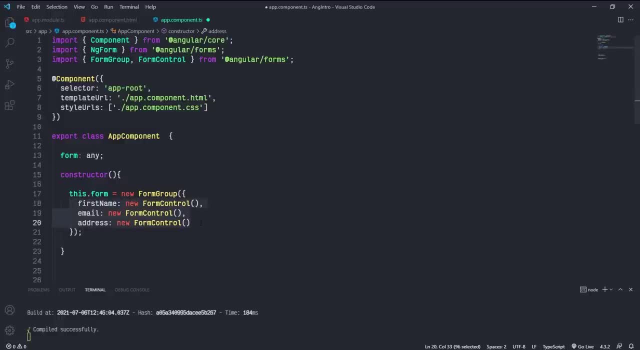 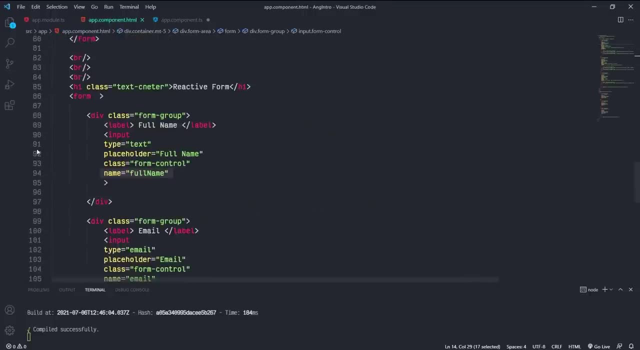 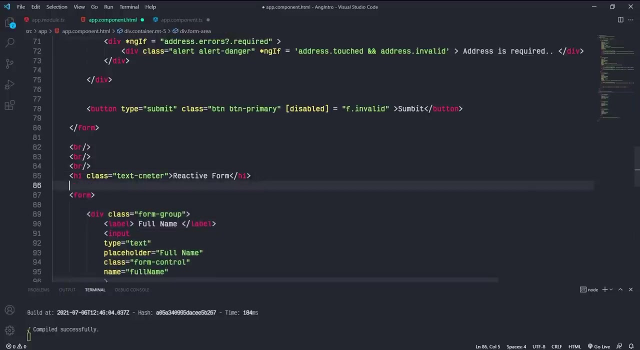 So we successfully created these new instances for the angular form. Now we have to connect this new instance to this form. So we connect this form to this form group's new instance. So for this we have a kind of a property binding. So inside the form tag, open and close, a square bracket. 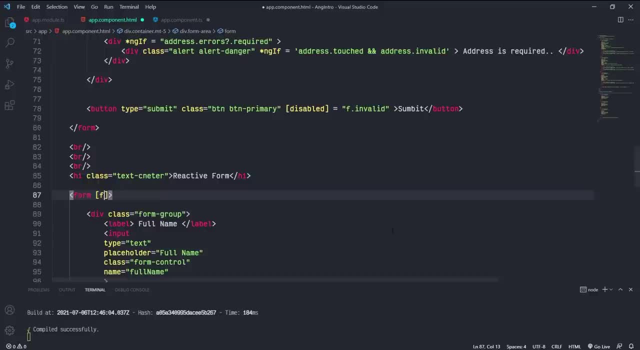 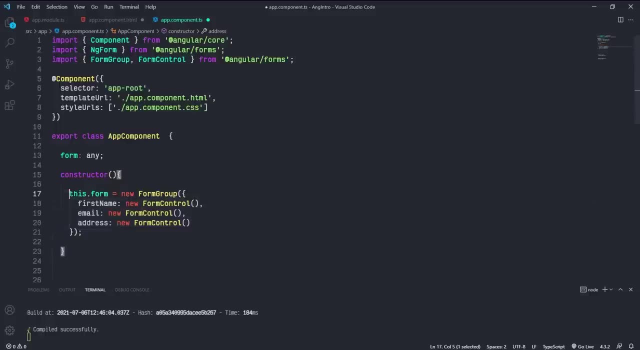 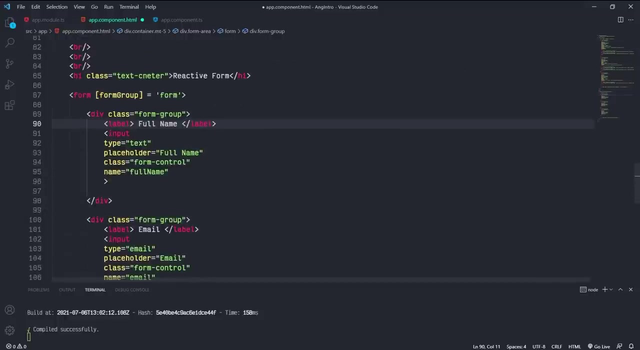 Inside this, the property name is form group. This first letter is simple and this g is capital. Now bind this to this form group. This variable name is form, So put this inside quotes. That's it. Now let's bind this input to these form controls. 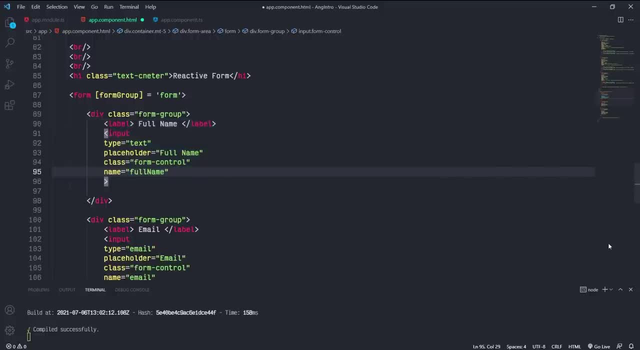 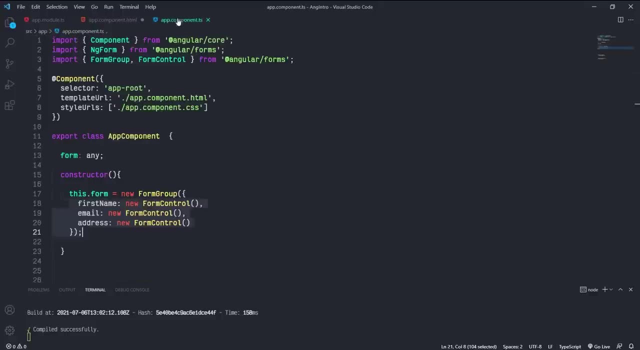 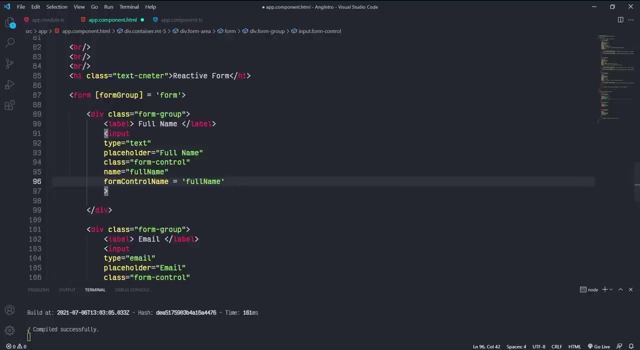 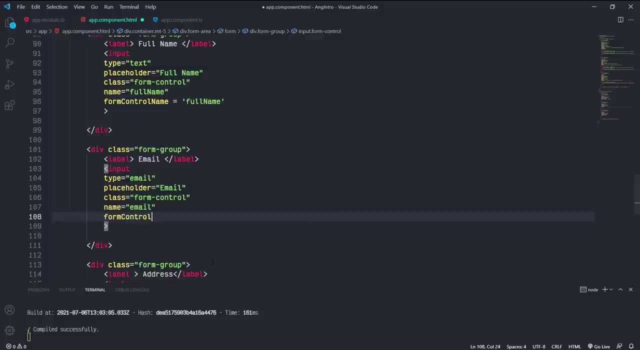 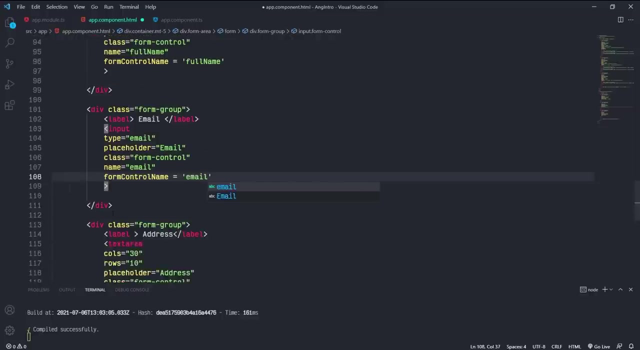 So for this we use a property form control name. Follow these capital simple letters carefully: Assign. Now bind this to this full name. Assign Form name Form control. Don't forget to put this inside quotes. So likewise for this second input form control name email. 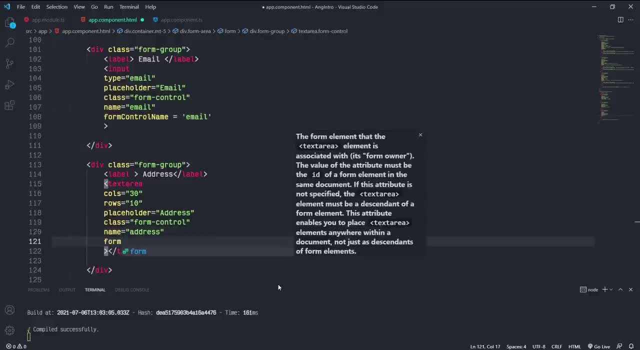 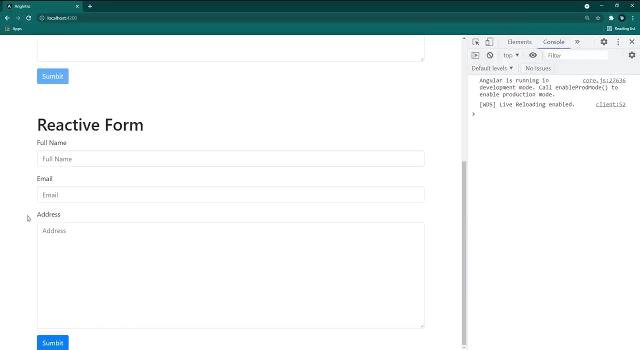 For this address: text-area form-control-name. assign it to this address. That's it. Save this all and go to the browser. Perfect, we are not getting any compile errors or runtime errors, Which means we have successfully converted this bootstrap class to an angular reactive form. 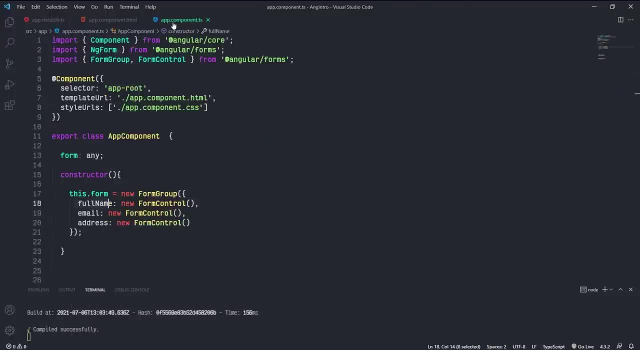 Beautiful. Wait before the end of this video. let me show you a small thing For this form-control-name. if you want to use any characters, for example for this first name, if you want to use the hyphen between first and name, put this inside of quotes. 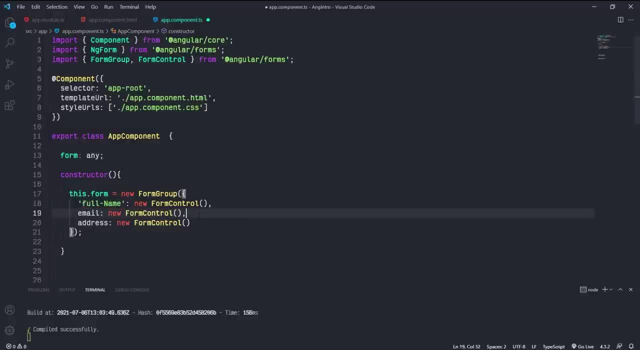 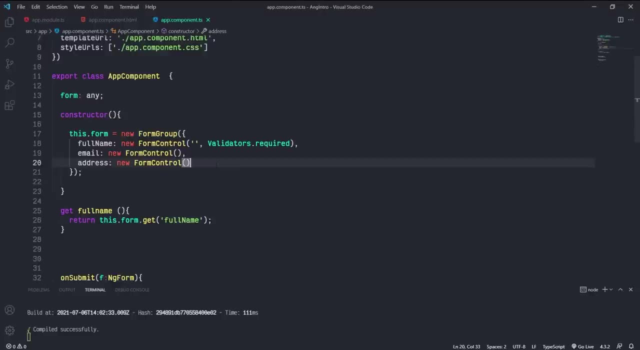 Otherwise this will throw a compile error. So in previous we did these required validations. Now let's see how to add multiple validation for this form. Very simple: We can pass this validator parameter as an array. So wrap this first validator with a square bracket to make this as an array value. 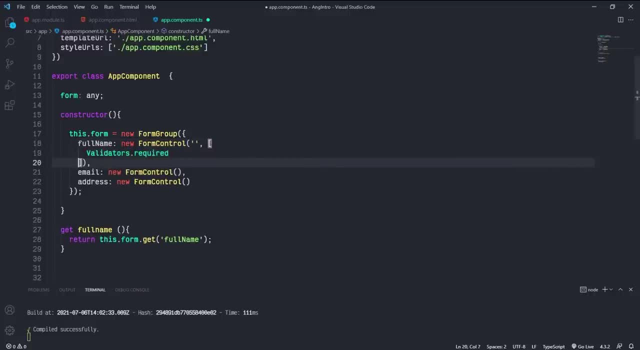 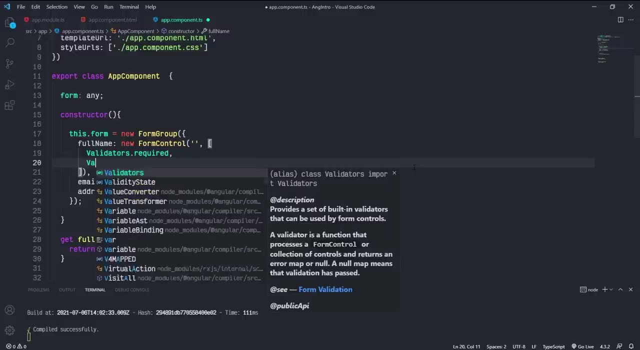 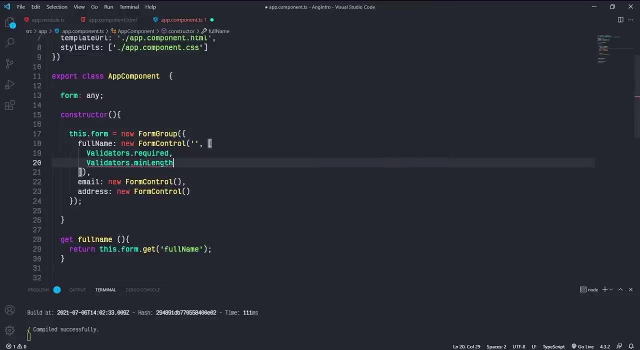 So break this into next line to see this clearly. After this comma, and again, we can define our second validation, minLength, So validatorsminLength. This is not like this required. We have to pass the minLength value, So parentheses, and the set the length to around 5.. 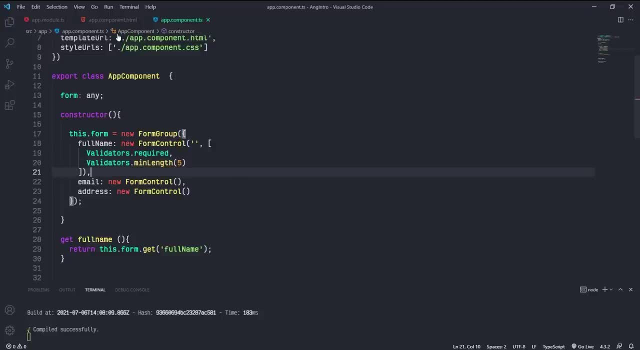 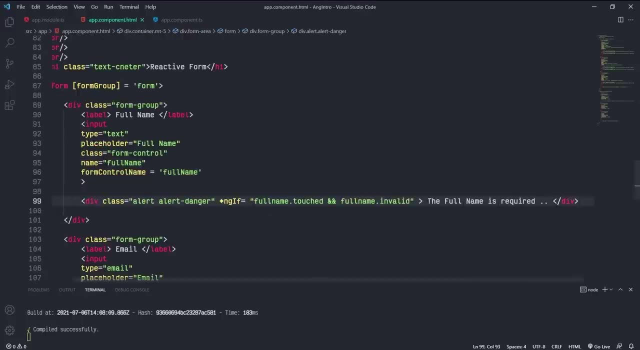 Save this. Now, inside the HTML view, add the error message for the minLength validation. Let's add a small change to this to show multiple error messages, So remove this required message inside this alert div. Create another div and paste the required error message inside this div. 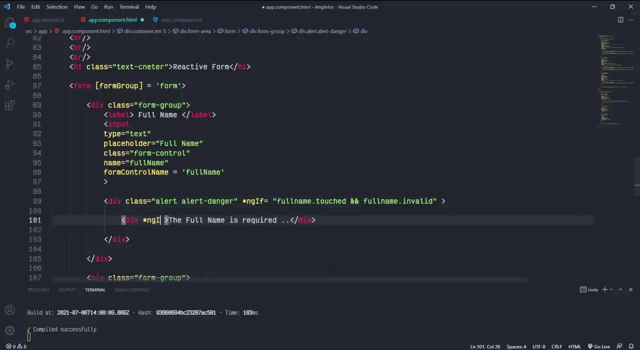 Add the condition for required. This form controls getter method. is this So: firstNameerrorsrequired. Next, duplicate this required error div and change the condition required to minLength. And also don't forget to change the error message as well. Now save this all and back to the browser. 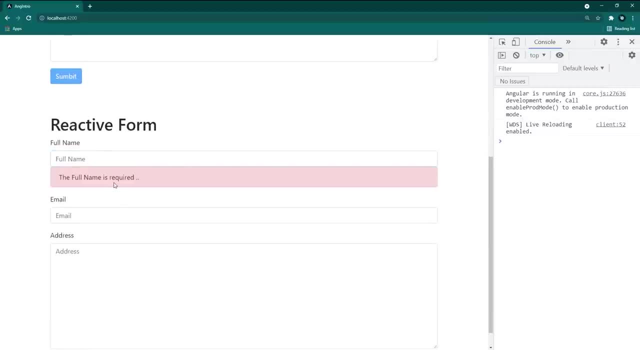 Click on this firstName and click outside: Perfect, we got this required error message. Type just one character inside this, As you can see here now we got this minLength error saying that firstName should be minimum 10 characters long- Perfect. so this is how we handle multiple validations in reactive form. 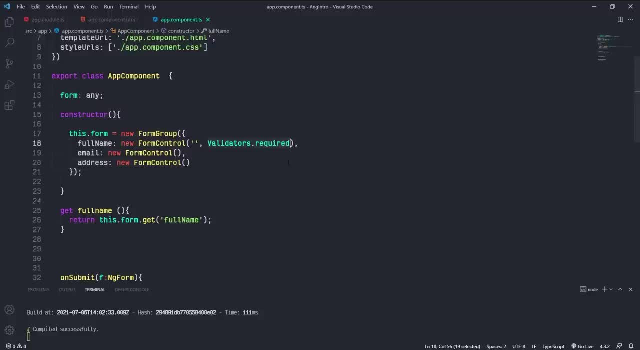 So in previous we did this required validations. Now let's see how to add multiple validation for this form control. Very simple: we can pass this validator parameter as an array. So wrap this first validator with the square bracket to make this as an array value. 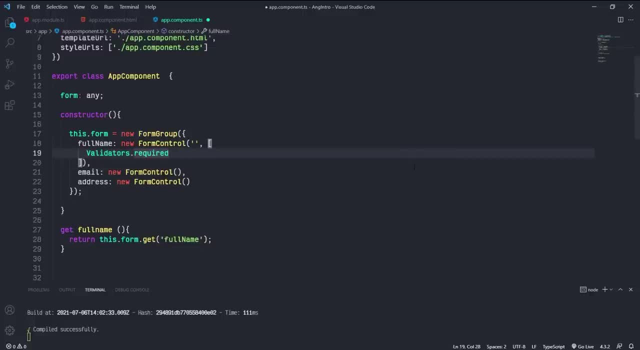 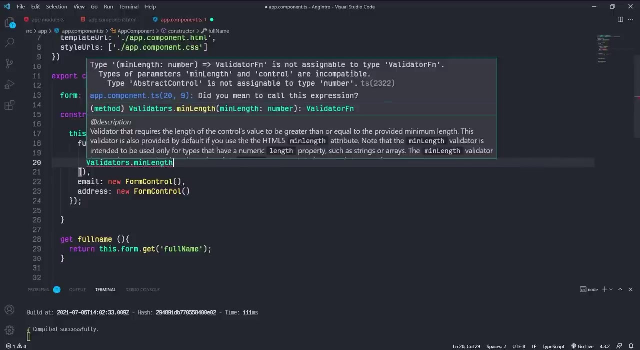 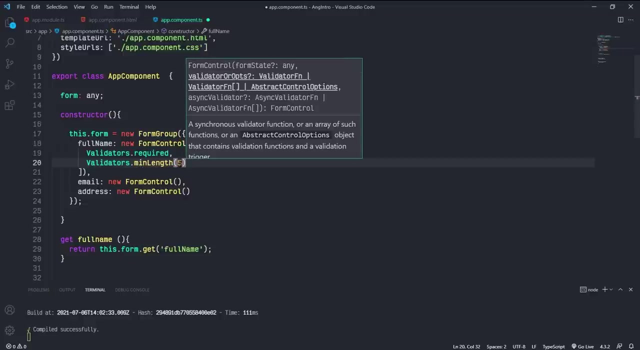 So break this into next line to see this clearly. After this comma, And again, we can define our second validation, minLength, So validatorsminLength. This is not like this required. We have to pass the minLength value, So parentheses, and the set the length to around 5.. 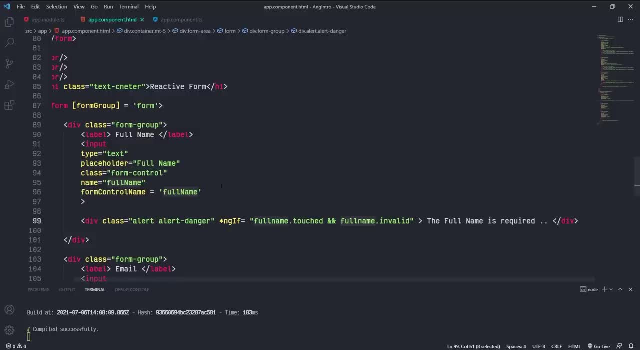 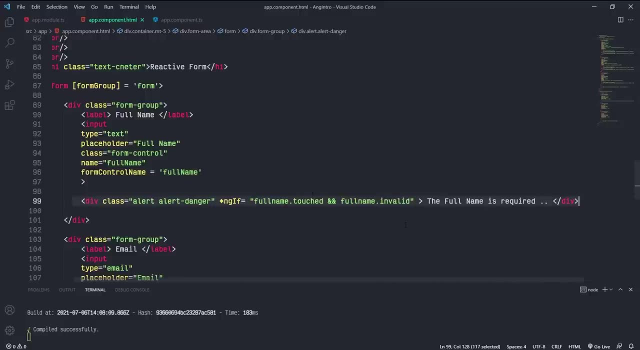 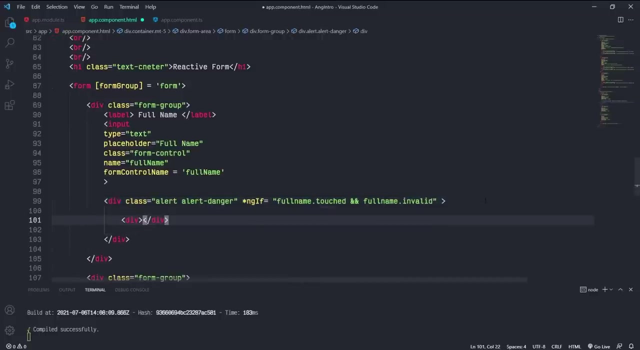 Save this. Now, inside the HTML view, add the error message for the minLength validation. Let's add a small change to this to show multiple error messages, So remove this required message Inside this alert div. Create another div and paste the required error message inside this div. 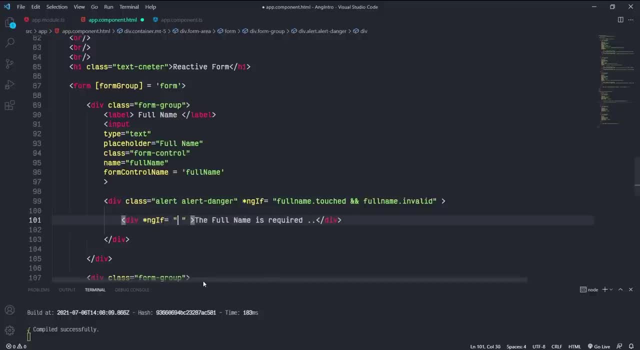 Add the condition for: required. This form controls getter method. is this So: firstNameerrorsrequired. Next, duplicate this required error div And change the condition required to minLength. And also don't forget to change the error message As well. Now save this all and back to the browser. 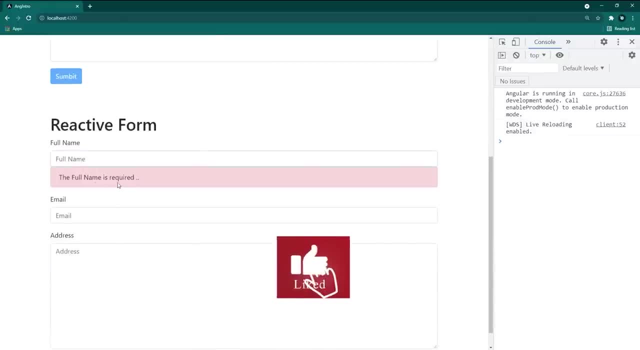 Click on this first name and click outside: Perfect, we got this required error message. Type just one character inside this, As you can see here Now we got this minLength error saying that first name should be minimum 10 characters long- Perfect, So this is how we handle multiple validations in reactive form. 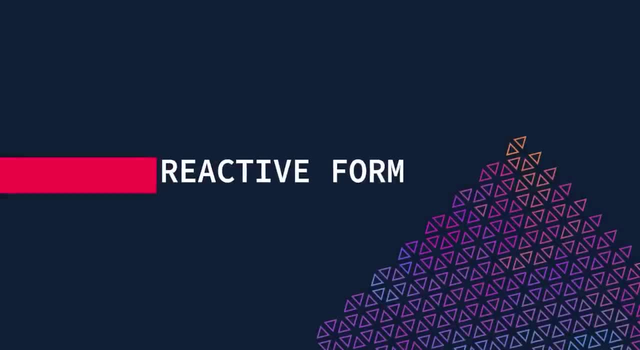 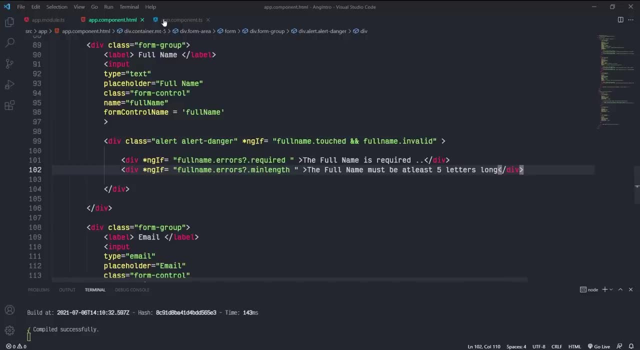 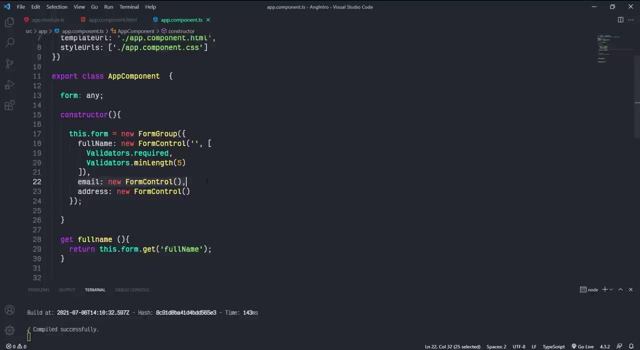 Alright, Let's add validation for all these inputs As a second field. we got this email field. For this also we need the required validator, And in addition to this we have the pattern validator for email validation. So, as a default value for this email field, set this for an empty value. 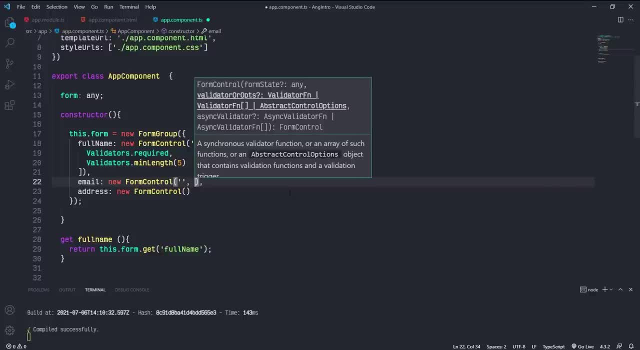 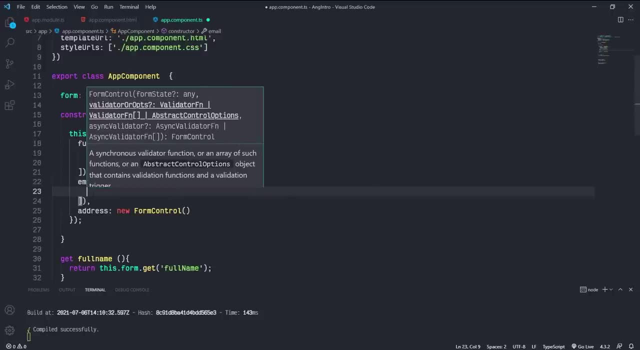 And as a second parameter For this, we gonna use the multiple validators. So define an array. Break this to the second line for more readability. Alright, First validation is required, So validatorrequired. No need to add the parenthesis cause. this is a static type method. 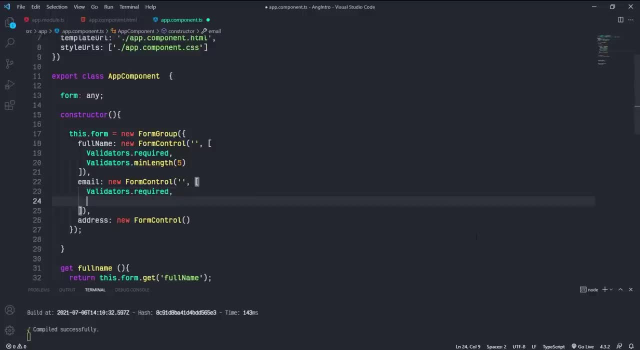 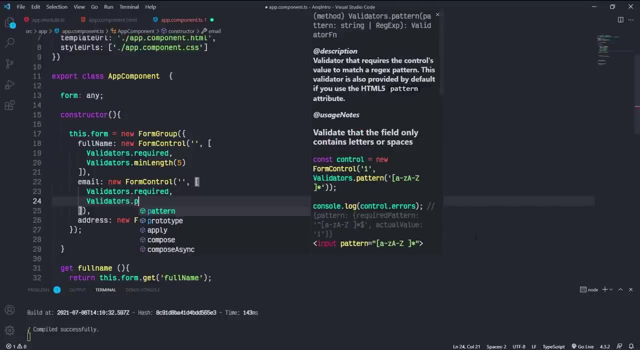 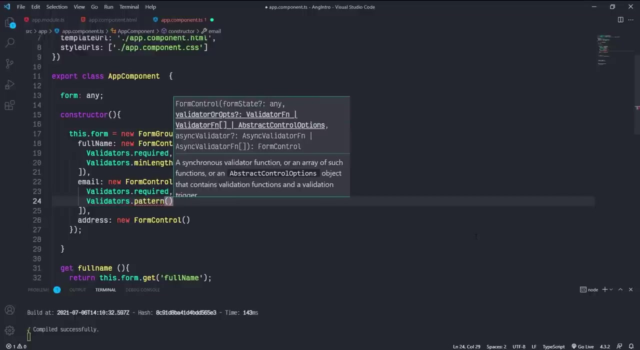 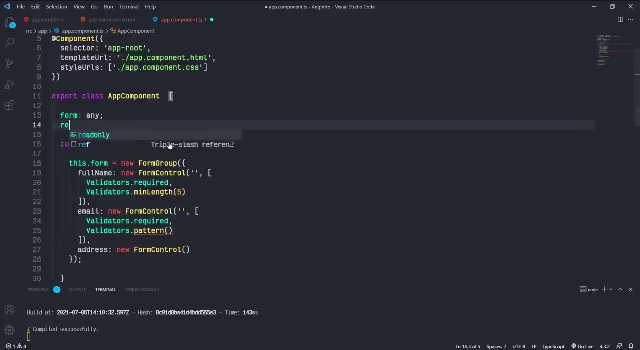 As a second validator, pass the pattern parameter. So after this, don't forget to add the comma Validatorspattern. This required the pattern rejects parameter Like this minLength. So first we need the pattern. So create a variable inside the class scope. The variable name is email rejects. 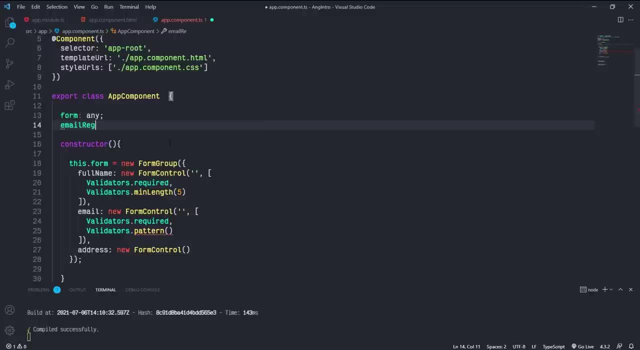 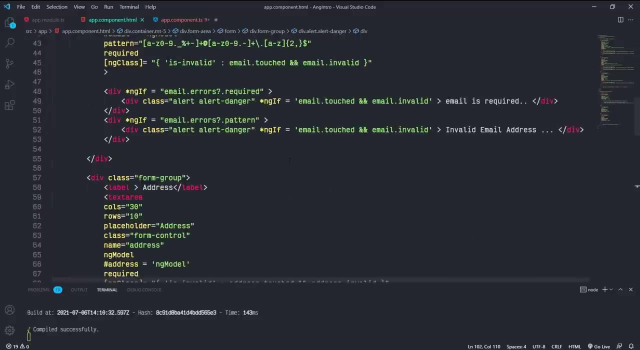 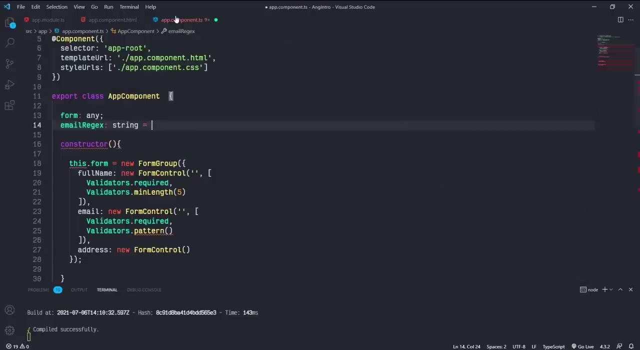 And type will be string. Now get the email pattern from the previous template driven form. Copy this pattern and assign it to this variable. Now pass this rejects to this pattern validator. Inside this parenthesis, This dot email rejects. That's it, Alright. now back to the template view and add the error messages. 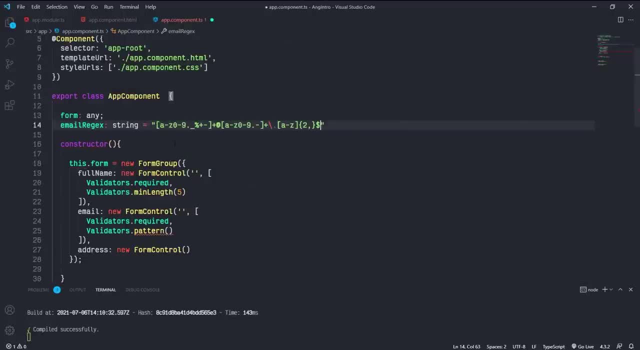 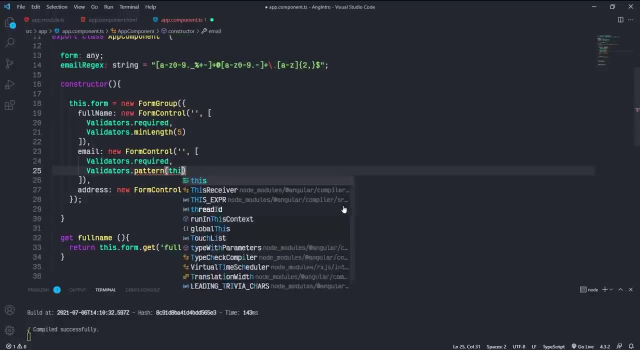 Wait before that Create the getter method for this email field as well. So get keyword and the method name, just email Parenthesis And the method scope. So insert this getter method at this return statement. This dot Form, Dot Get. 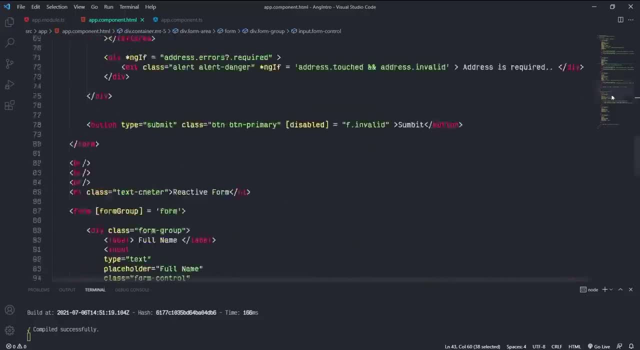 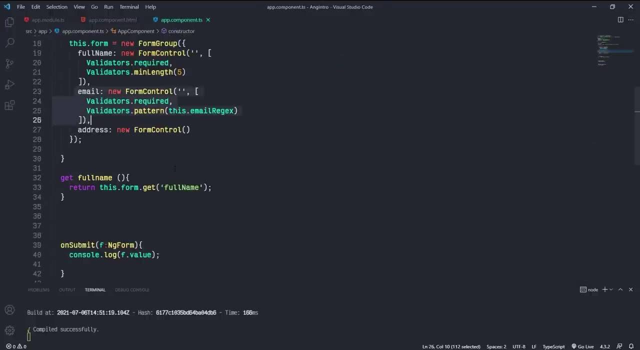 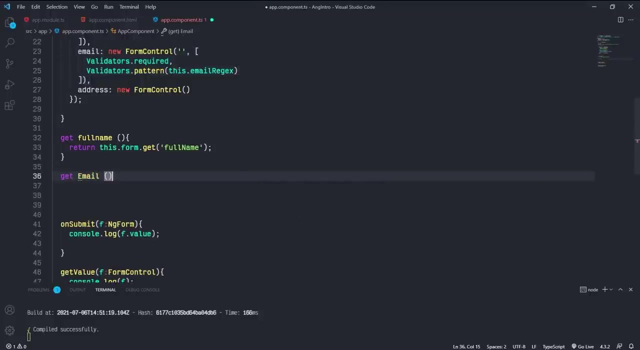 Inside parenthesis, Pass Email As a string. So this email is this form control key. Alright, let's add the error messages. Save this and go to the component HTML file. Copy this error message div from this first name. Paste it inside this email form control div after this email input. 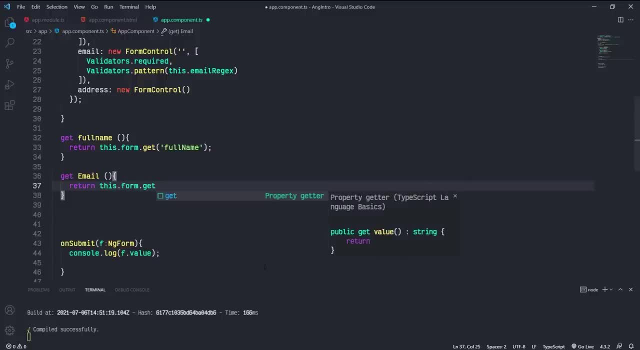 Change this getter method first name to email Once again. this is this getter method's name, Not this form control's name. Alright, these all are the same. No need to change. expect this min length, Remove this min length and add pattern. This time we are checking the email pattern, not the min length. 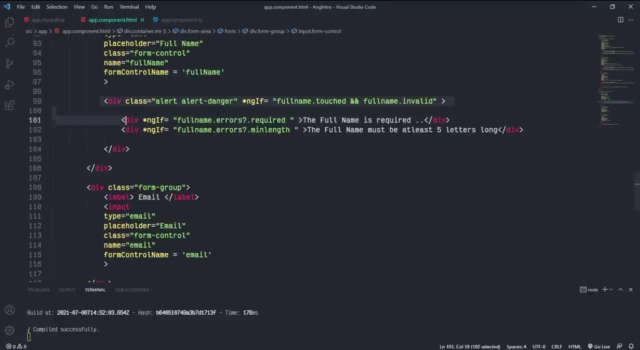 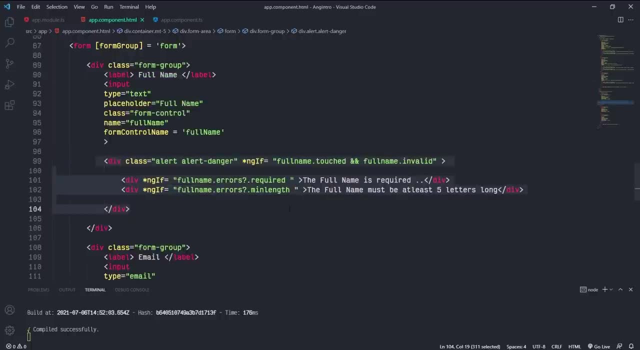 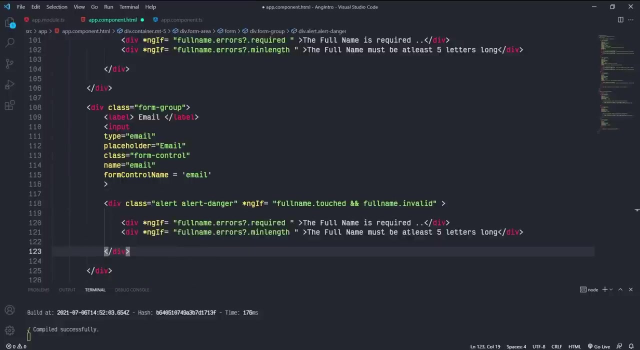 So change this message to invalid email. That's it. Save this and back to the browser. Click this email field and click outside. Perfectly, got the required message. Now type a character inside this email field. As you can see here, this time we got this invalid email. 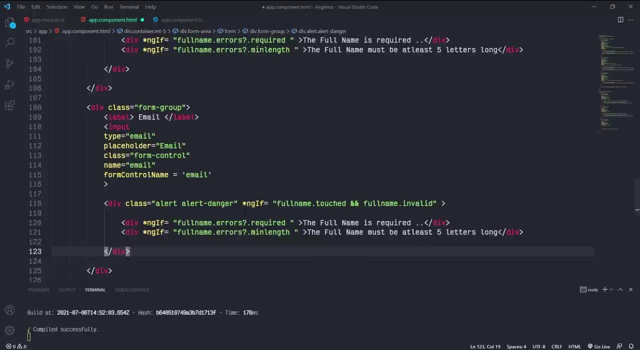 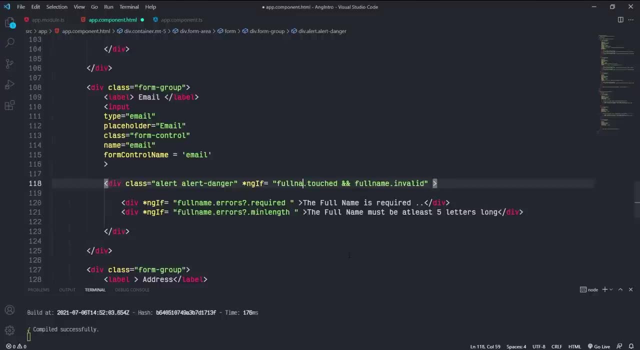 Now type a simple email address, Something a, at gmail dot com. Now we don't have any errors. cause: this email is in the correct format, So in the reactive form we have a simple way for this email validation, rather using this regex pattern method. 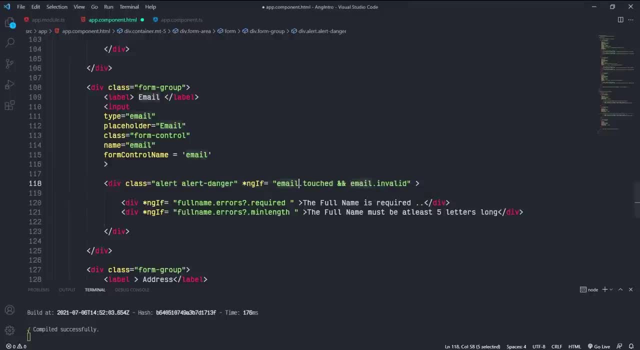 So let's see that in action. So very simple, Command this. Now we don't need this pattern validator. Instead of this, we can use the email validator. So after this validator, dot email, That's it. This also static method, like the required validator, static method. 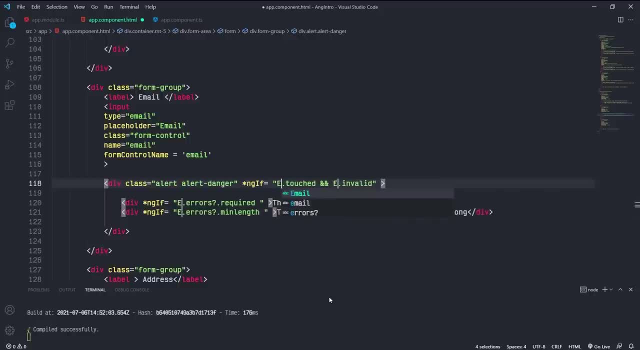 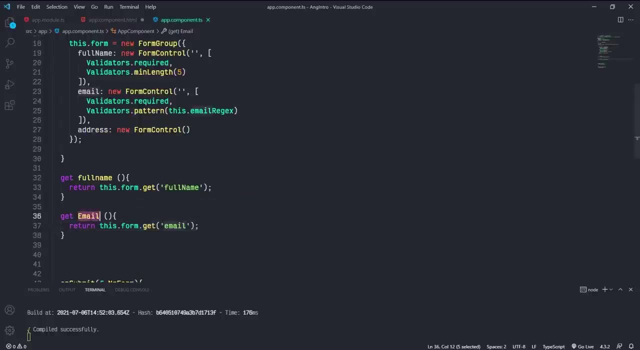 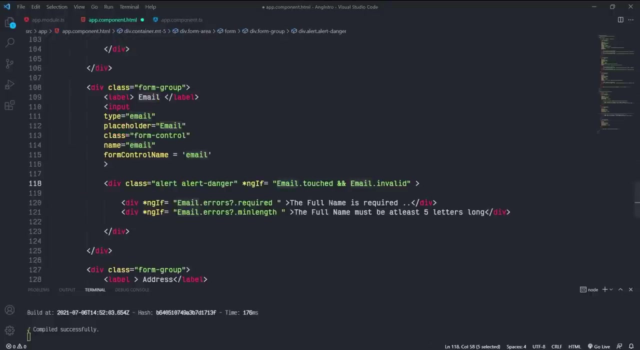 So very simple, right? So this is very clean and easy to understand, Right? Alright, save this and back to the component HTML file And remove this pattern Cause this time we are not checking any pattern, So remove this and add email. That's it. 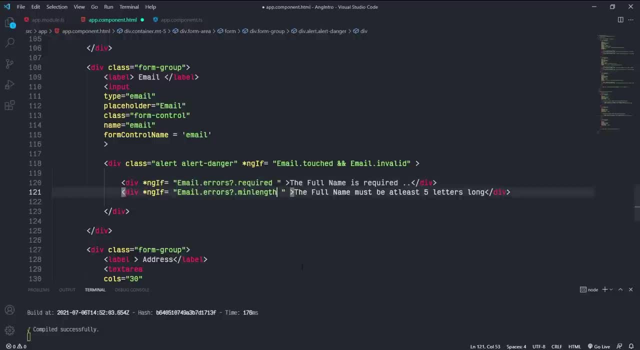 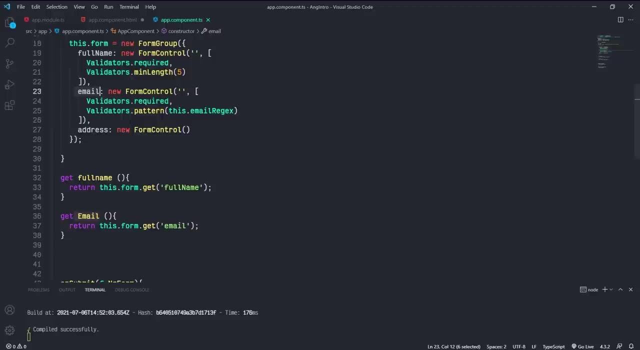 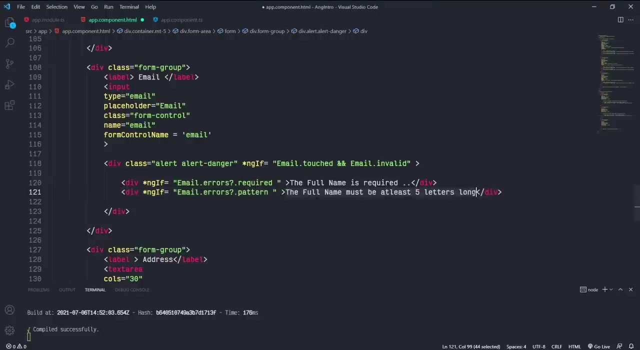 Save this all and back to the browser. Check this email field validation. Everything working as we expected, Perfect, Alright, let's move on. Next, add the validation for this address text area. So nothing fancy. This text area just need only the required validation. 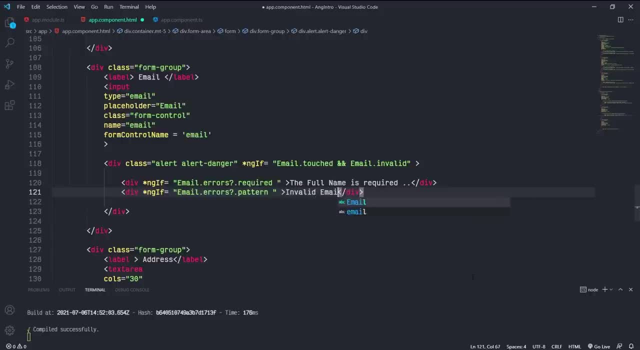 So inside the component is file, Inside this address: form control parenthesis. As a first parameter. set the default value, which is an empty string, As a second value validator. This time we got only one validator, So we don't need to pass this as an epic. 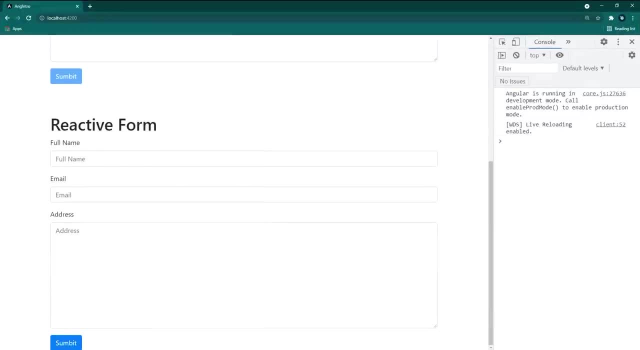 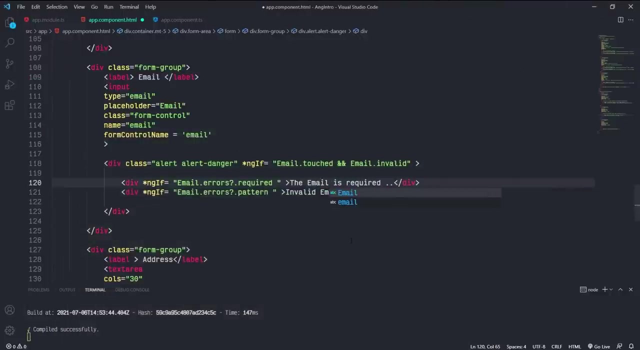 Just add it after this Validator dot required. That's it. Save this and back to the component HTML file And add the required error message. So just copy this previous error message. This time we only need this required message. So remove this second error message. 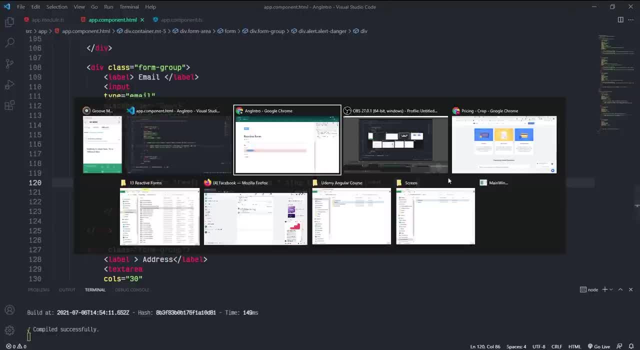 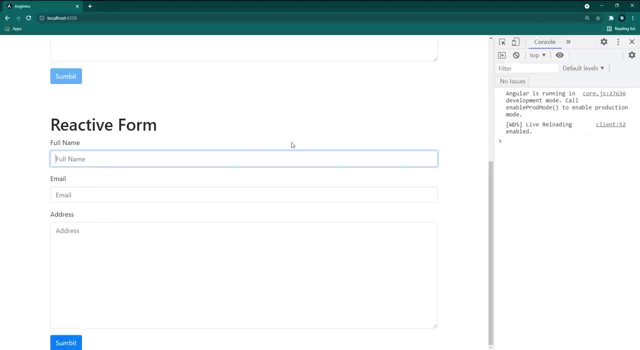 And change this required error message. So save this all and back to the browser. Get focus this text area. Lost the focus. Perfect, We got this error message. Type a character. as you can see here As soon as I typed a character inside this text area. 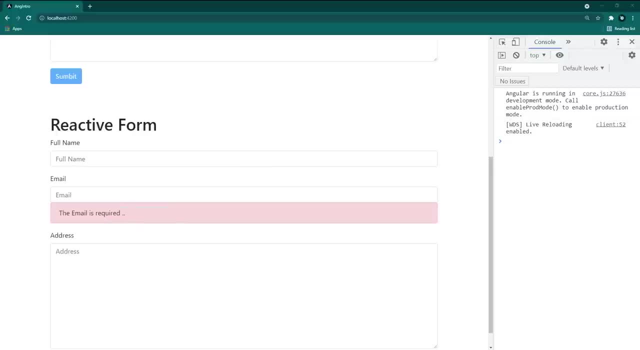 This required error message disappeared. Perfect, Everything working as we expected. Before the end of this lecture We want, I wanna tell you one more thing. Some of you may wonder From where we get this red border On this input, If you can remember. 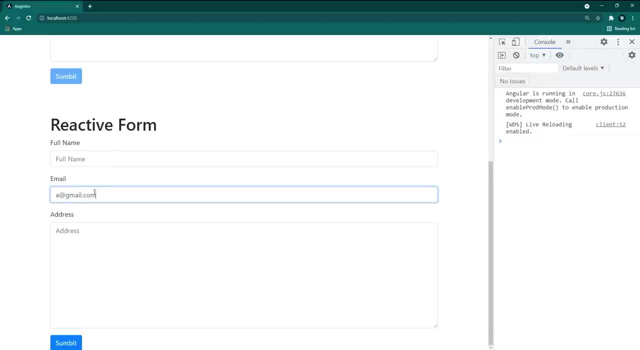 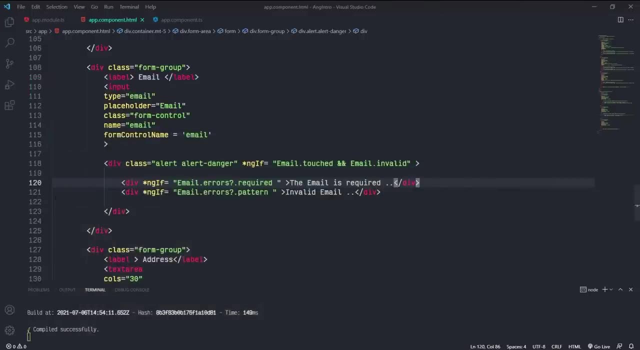 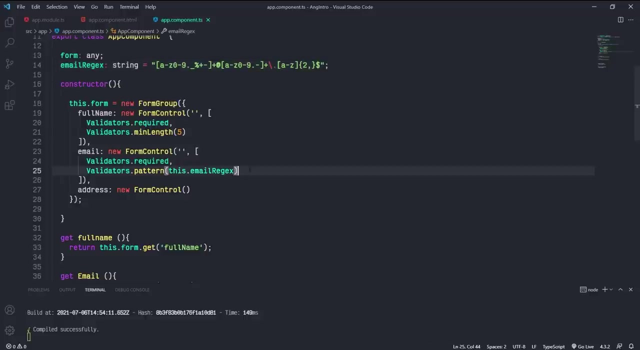 We define this CSS style For this ng-touch and for this ng-invalid. So this is how we getting this red border On the input fields: If this field is invalid, This angular classes will be added to these input fields. So we learned about this when we dealing with. 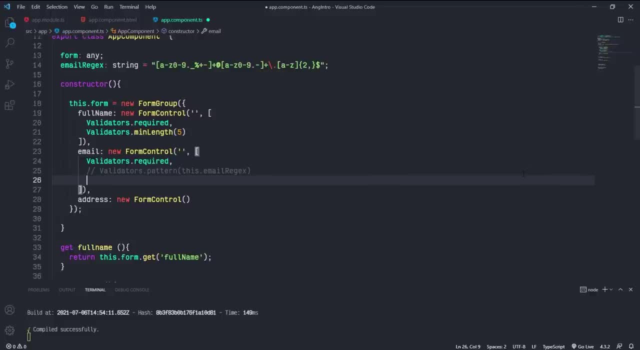 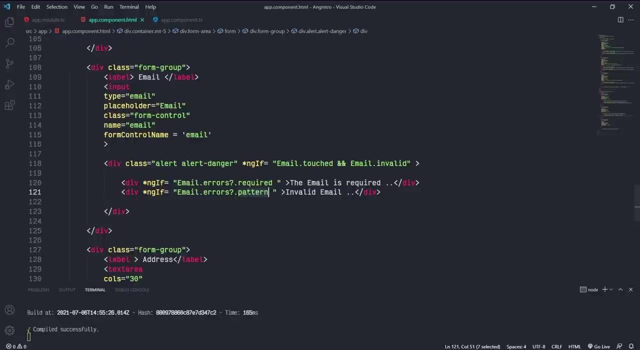 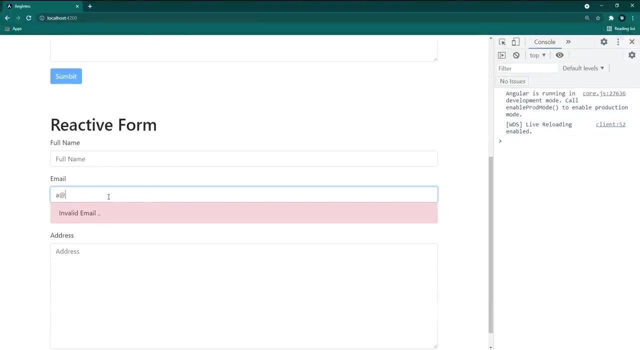 The template driven forms. Hope you guys remember this. So if you have any questions about this, Please feel free to ask. We'll get back to you in the next lecture. Thank you, Bye, Bye, Bye, Bye, Bye, Bye. 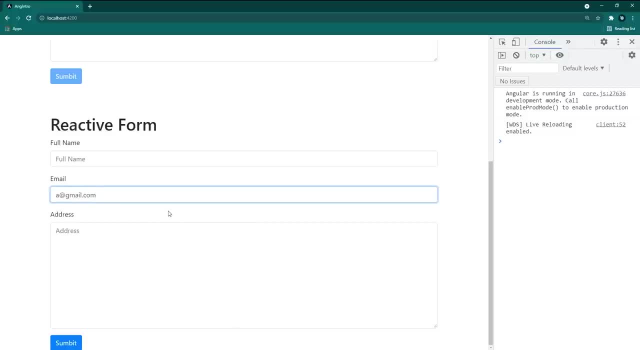 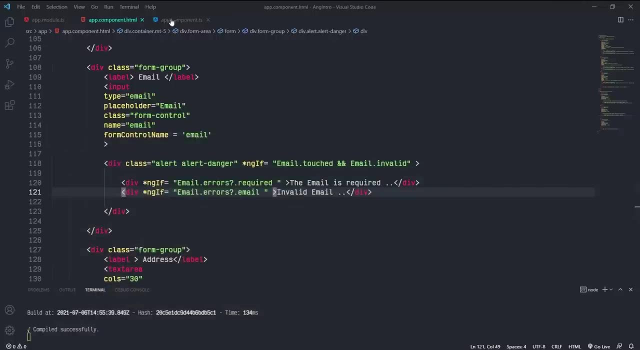 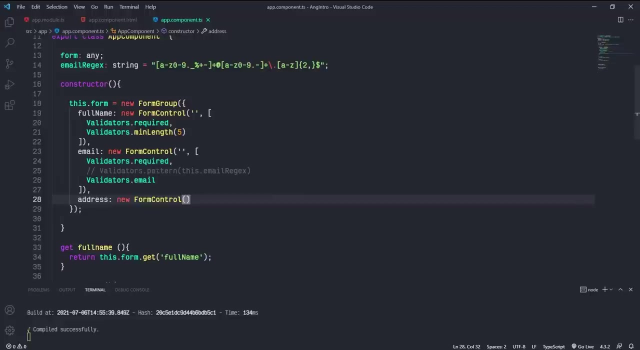 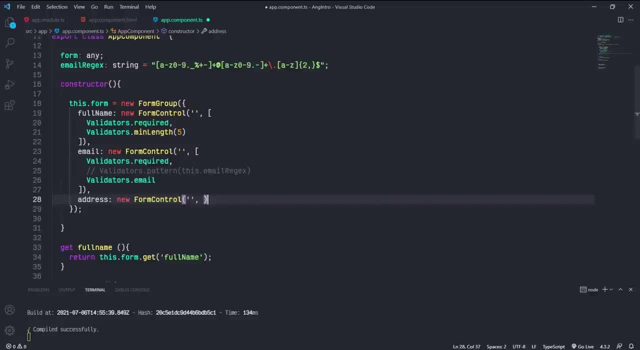 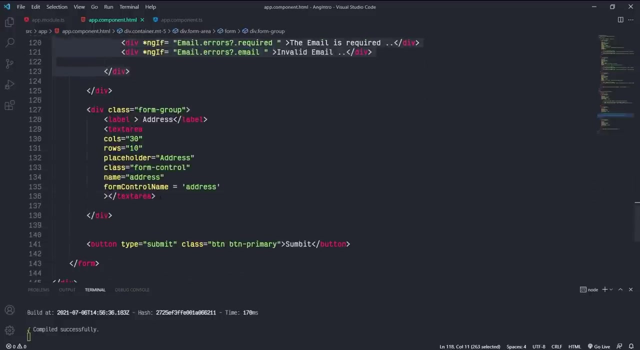 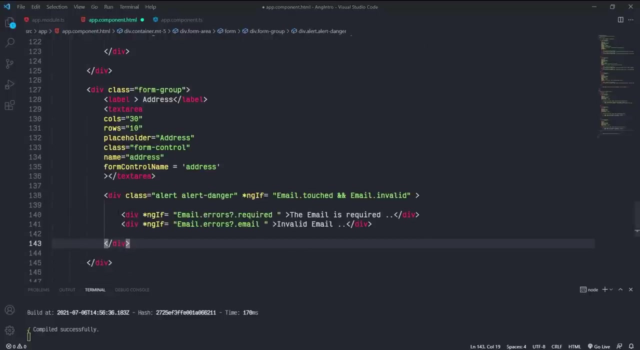 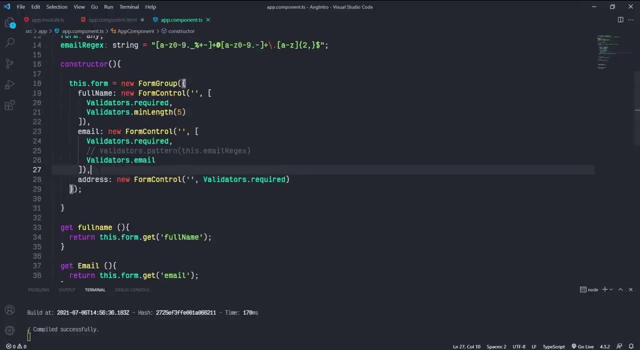 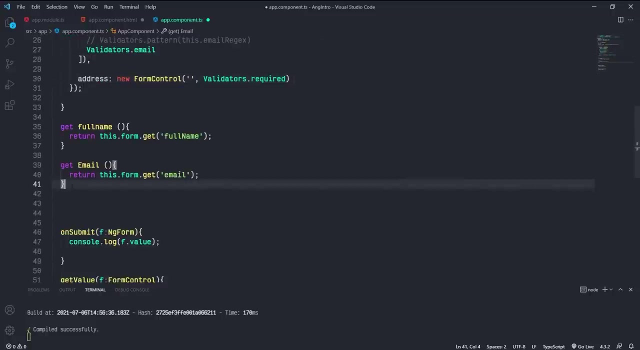 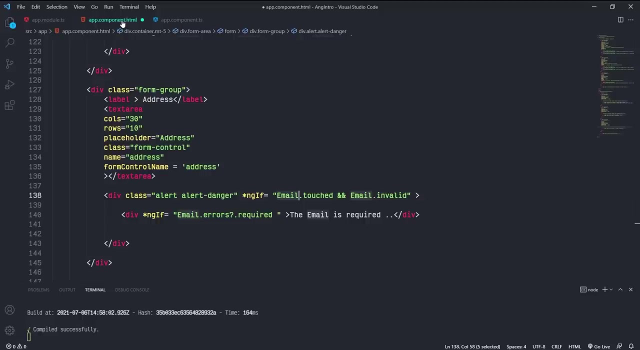 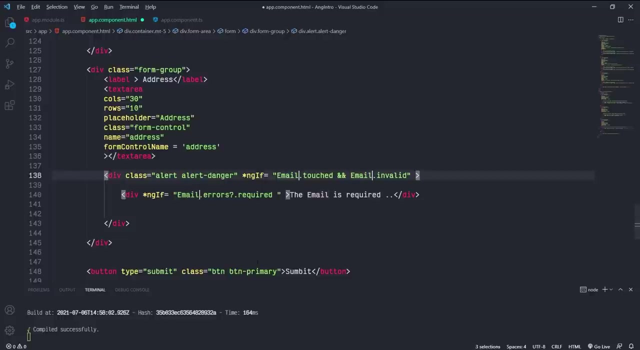 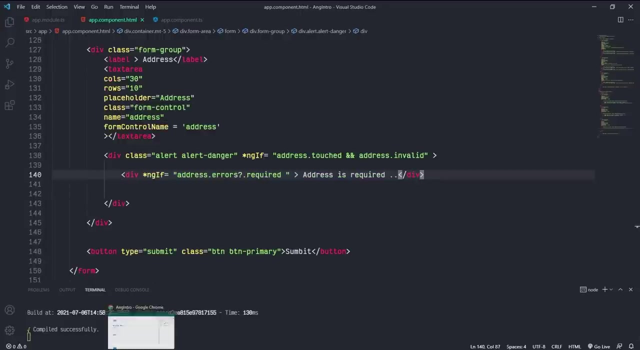 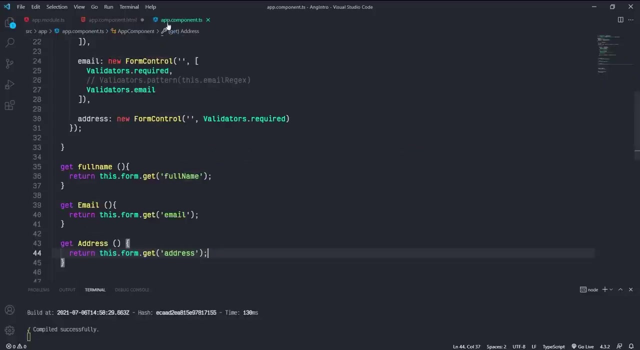 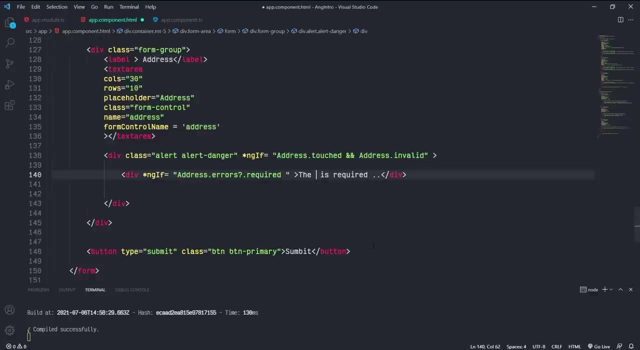 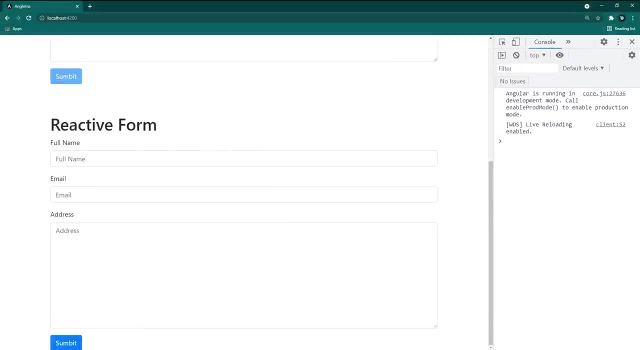 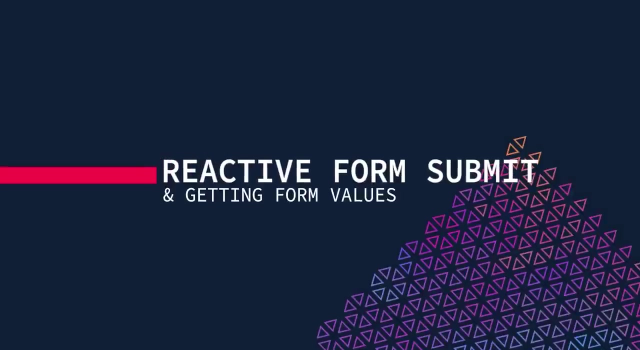 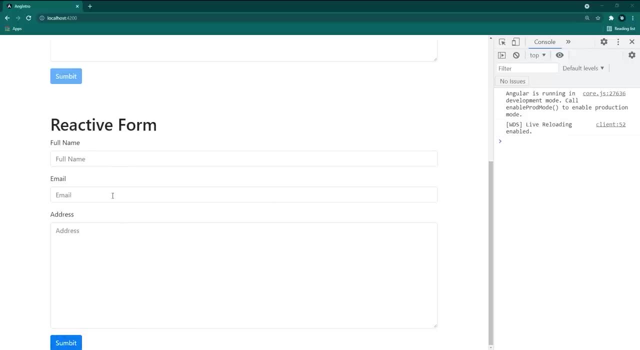 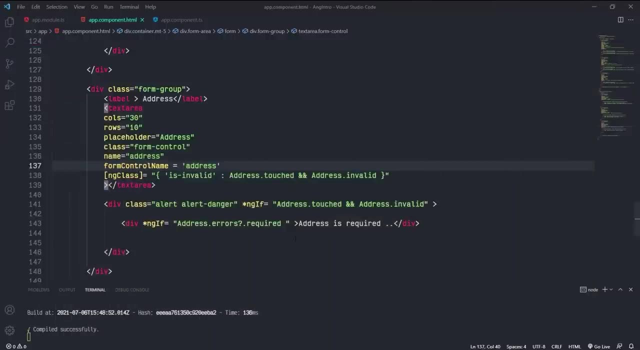 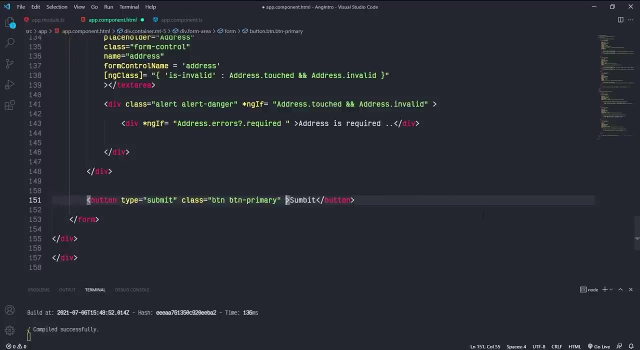 disable- enable the submit button when the form is valid or invalid. and also let's look at how to get the forms values all right. let's see this in action. first, let's do the button enable- disable. this is also same as the previous template driven form. for this we're going to use the property. 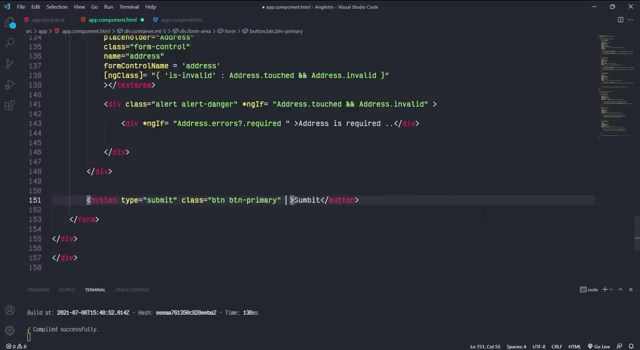 binding. inside the app component html file, add the property binding for the submit button inside this: open and close square brackets. inside this: the property is disabled. equal sign: the statement is form: this is this form group dot. form dot- invalid. if this form is invalid, this becomes true and this: 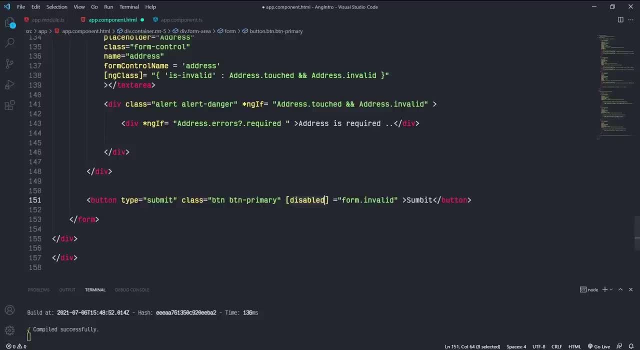 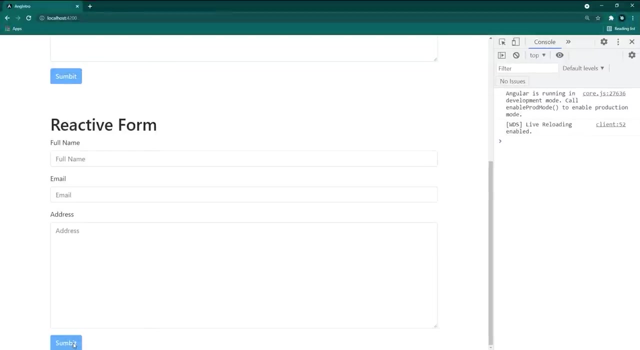 disabled property will be applied to this button. if this is valid, this becomes false and this disabled property will remove from this button. that's it. save this and back to the browser. as you can see here, this button is now disabled. fill this form correctly, without errors. look at this now. this form has no errors. 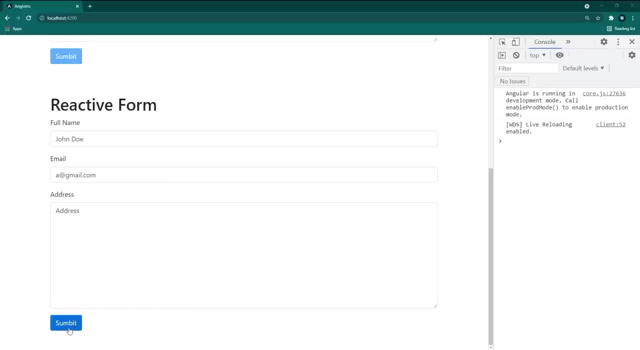 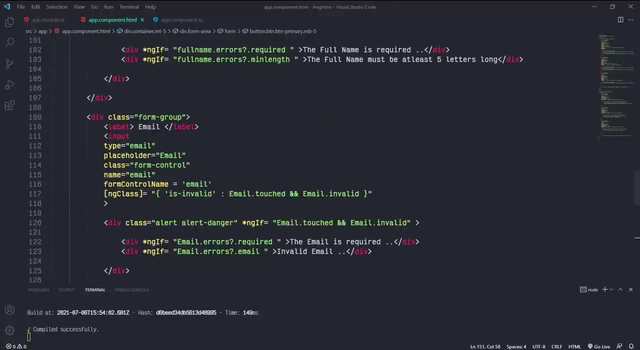 which means this form becomes valid, which means now we can submit this form by using the submit button. perfect right, all right. next let's see how to get these values when we submit this form. as usual, we gonna use the ng submit event for this form, same as the. 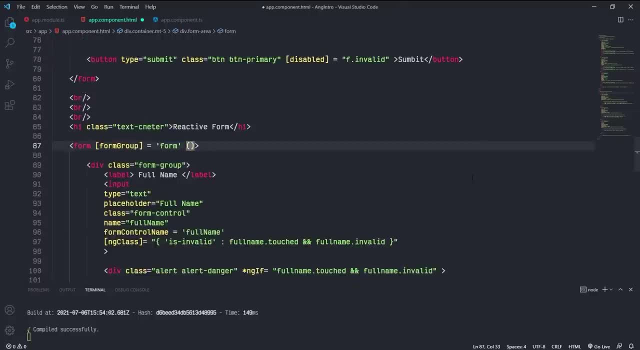 previous template driven form, inside brackets ng submit and bind this to a typescript method, something on submit and the parentheses. in the previous template driven form we send the ng form parameter with this ng submit event, but in reactive form we don't need to send any parameters. 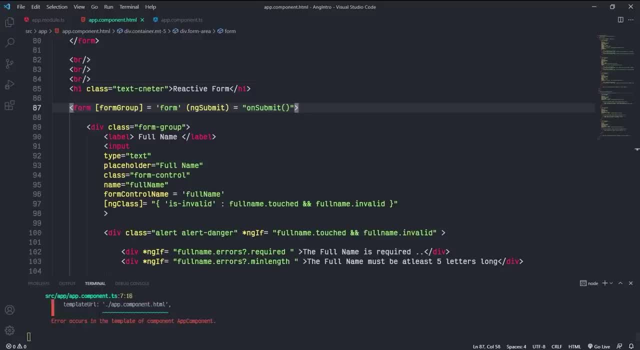 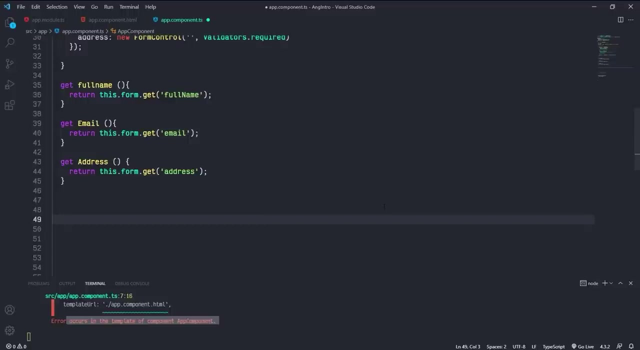 just call the method. as you can see, we, as you can see, here we are getting a compilation error because still we don't have declared this method inside the component is file. so go to the component is file and create this on submit method. so inside this class scope, the method name is on. 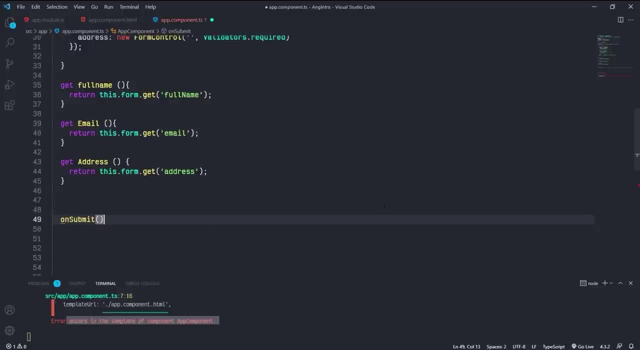 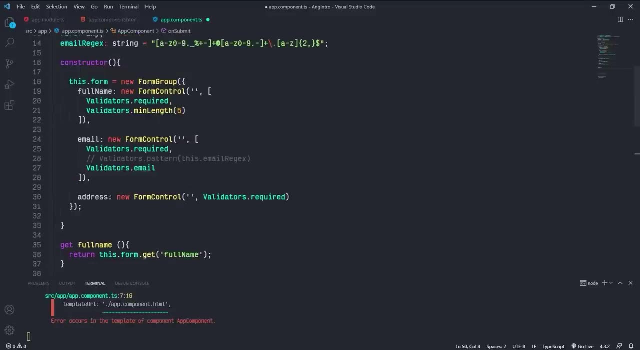 submit and the parenthesis after this. don't forget to add the method scope. all right, inside this we can get the form data very simple. this is the form group. we can access the form group data by values property. so inside this method we can get this form group data like this: this dot. 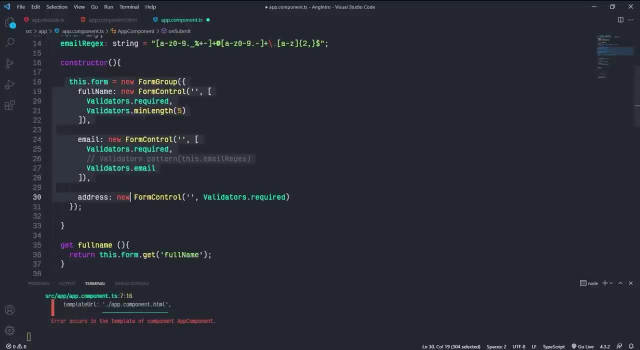 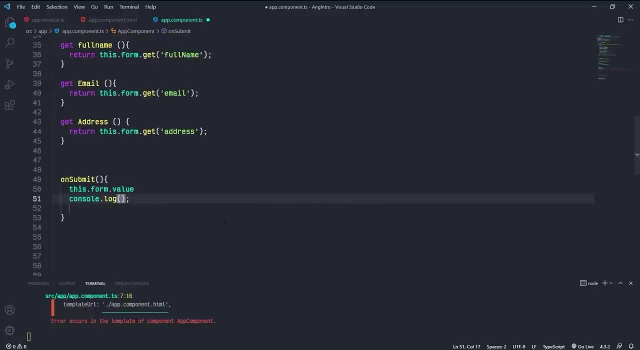 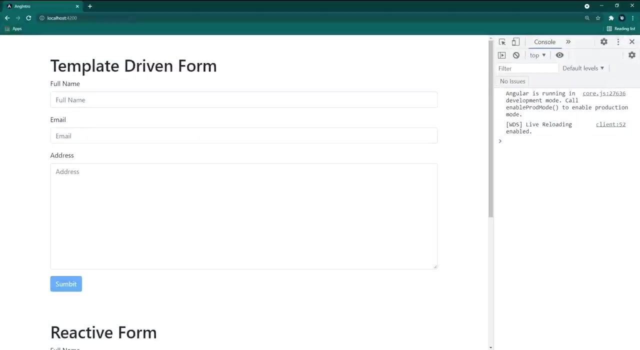 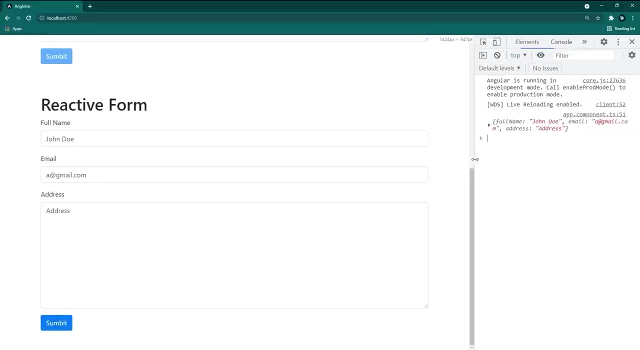 form. this form is this form group value. with this property we can get this form groups value, so let's log this to the console consolelog. put this inside this log, save this and back to the browser. fill this form and submit the form. this form. look inside the browser console as you. 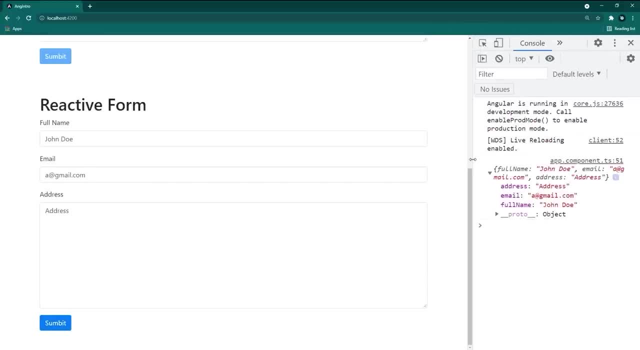 can see here. we got the value of this form as an object. now we can send this values object to the database and store this data inside of a database. don't worry about saving data inside the database. we will learn about this in the next lectures. so this is how we 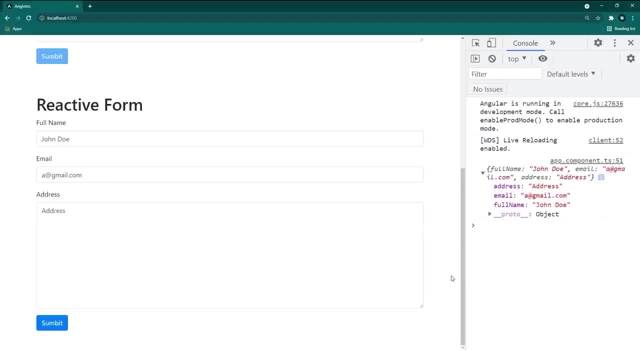 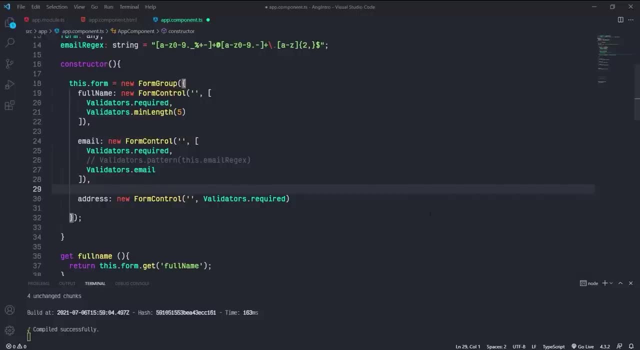 handle data in reactive forms in real world apps. when we saving data to the database, sometimes we nest object inside objects. for example, with this form, group value object, we are getting this data. think if we have another field for something- billing address and for contact numbers, likewise contact details input. and if i 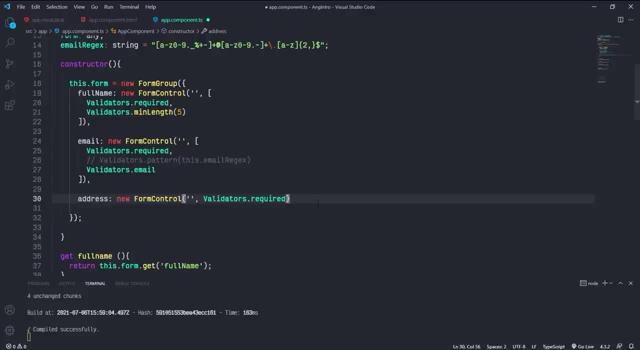 want to get that contact data as a separate nested object inside this main value object. how do we gonna do that? in reactive forms we can list form groups inside the main form group. so let's see this in action. inside this main form group, the key is contact details. 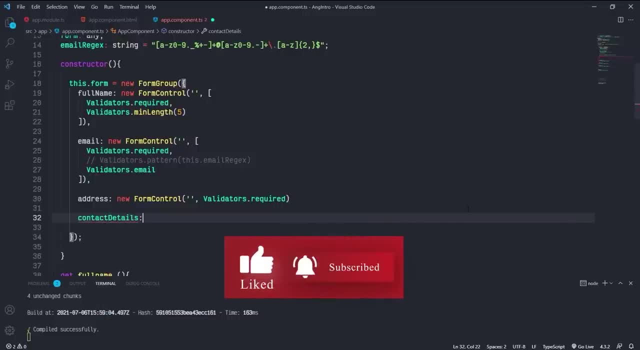 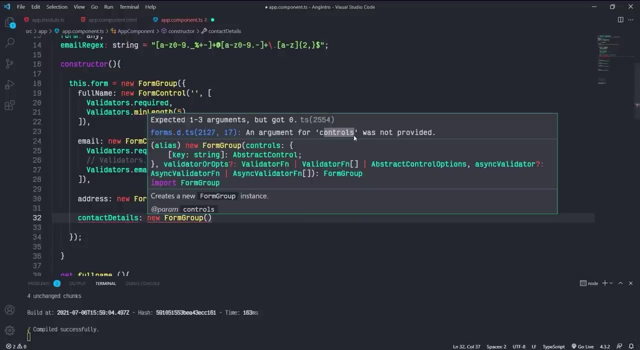 and this time, instead of this new form control, create a new form group instance like this main form group. new form group and the parentheses: this nested form group also required object of form controls. nothing fancy. same like this main form group. the only difference is this is the main form group and this is. 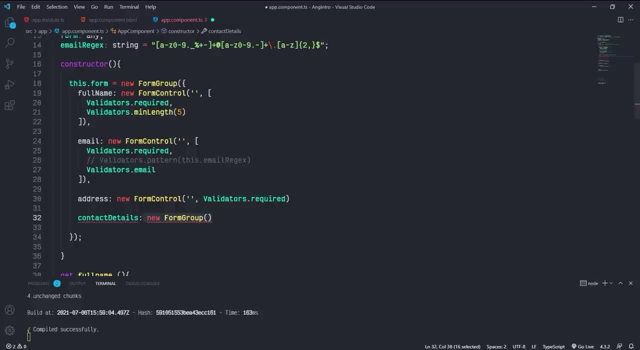 the sub or nested form group. all right now, inside this we can create the form controls. so put this address form control inside this contact details form group and after this let's create two sub form controls. first one is for something: shipping address. so key is shipping address. 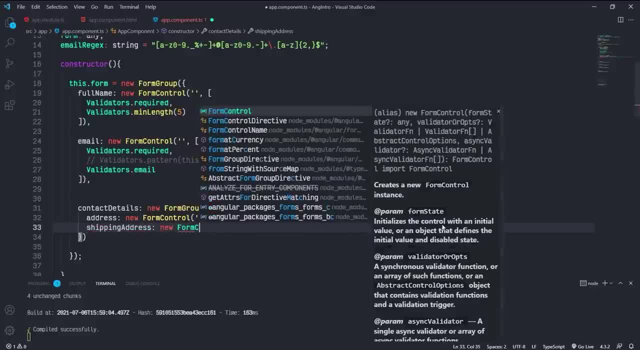 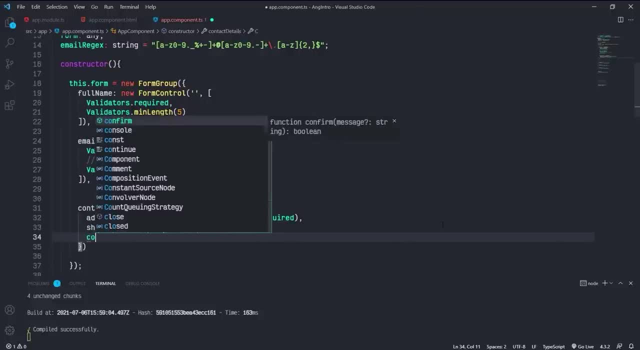 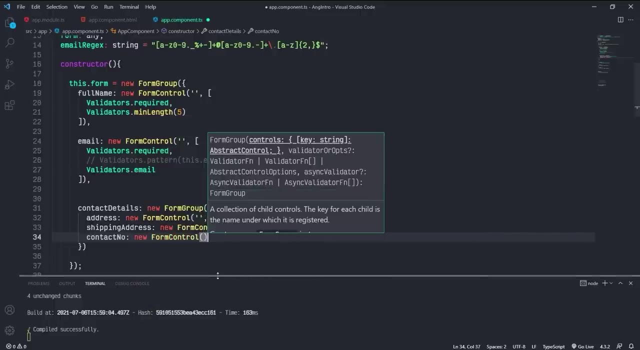 and the value is new form control and the parentheses. again, another field for a contact number. the key is contact number and the value is new form control. and don't forget to add the parentheses. that's it now. let's create new input fields for these. shipping address. 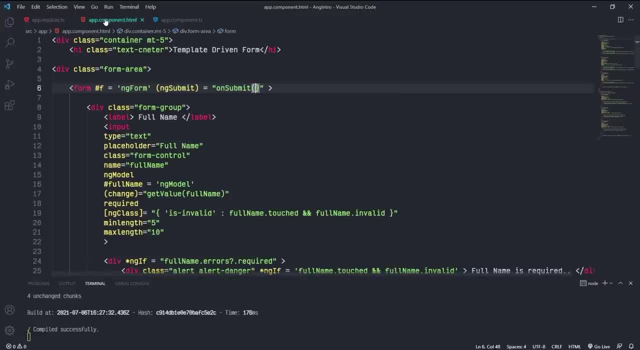 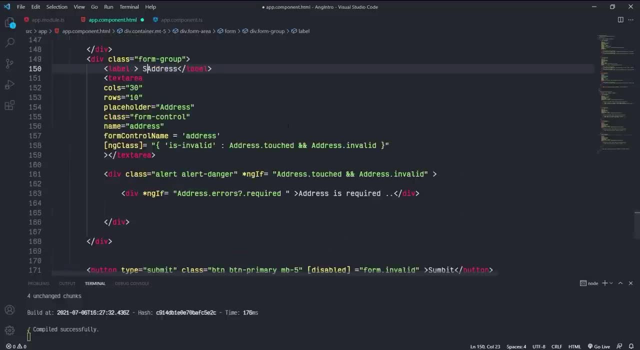 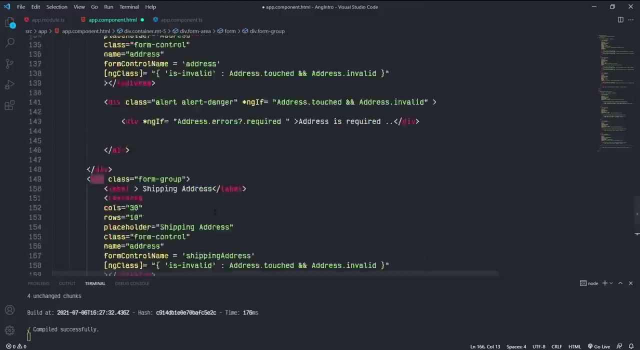 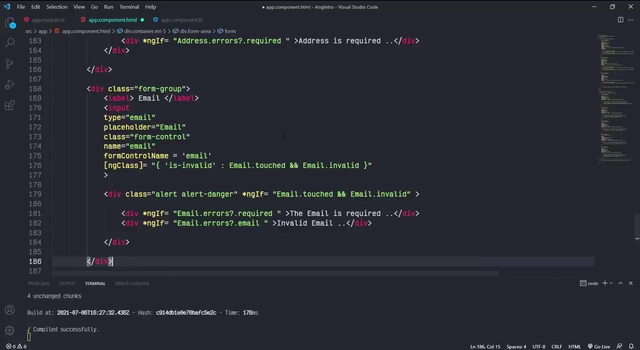 and for this contact number input field. so inside the template html we duplicate this address text area, change the label as the shipping address and change the form control name to shipping address. again we need another field for contact number. so copy this input field and paste it here. change the label to. 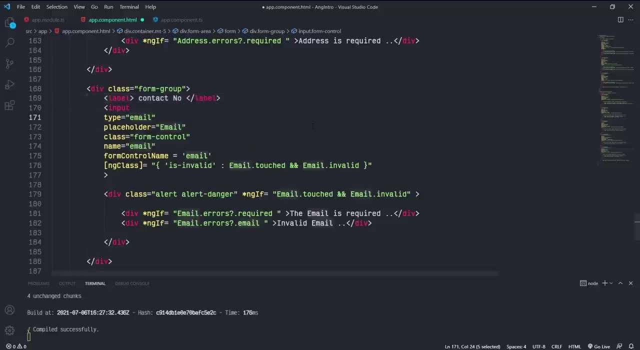 contact number. and also don't forget to change this form control name to contact number. that's it all right. let's add this contact input inside the contact details form group. this is still inside this main form group to create the contact number. now let's create nested groups inside. 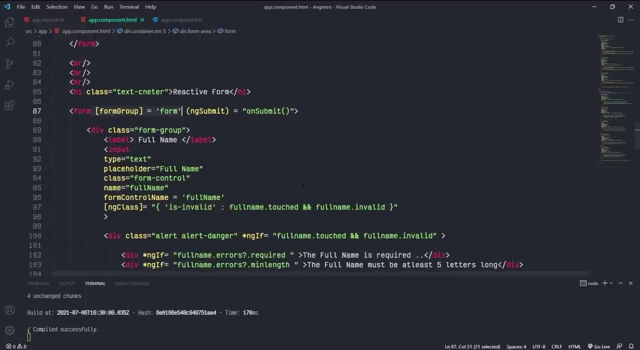 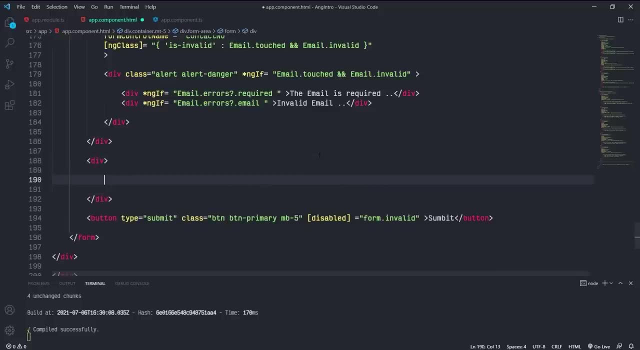 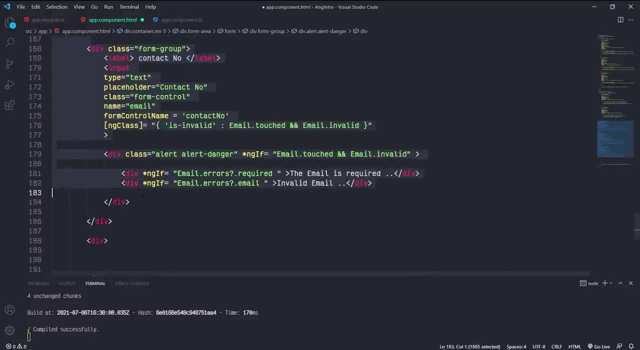 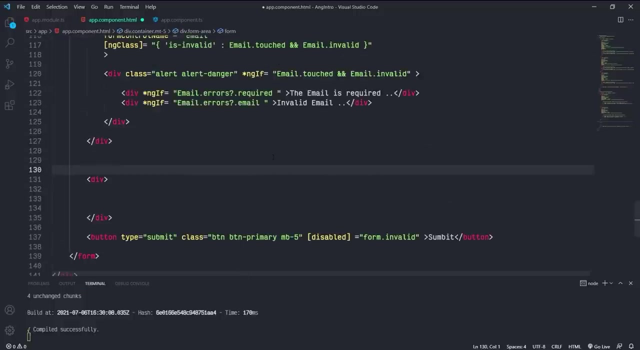 the view. we have a property called form group name, like this form control name, so let's do that: create a div and put these all in. put these all contact inputs inside this div. address, shipping address and this contact number inputs. now add the form group name property to. 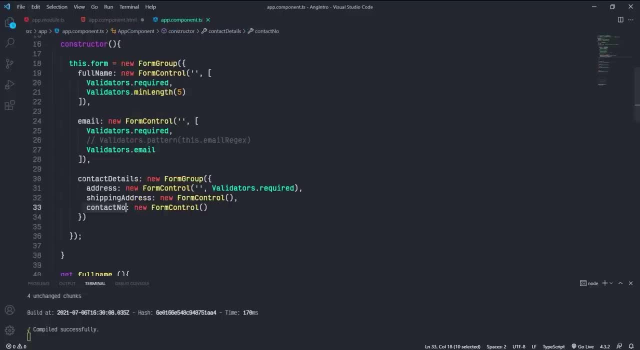 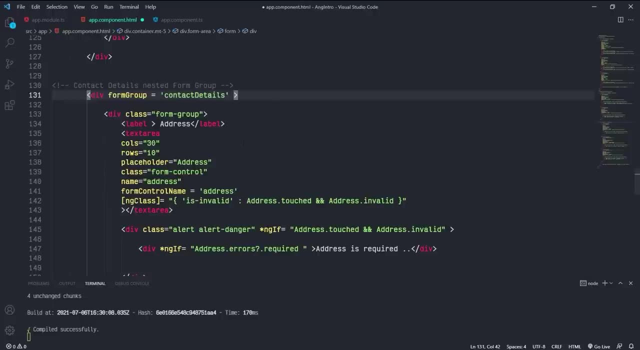 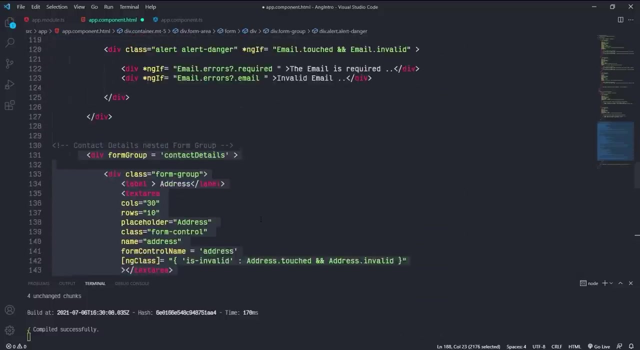 this div and bind this to this nested form group, which is contact details. pass this exactly same as this capital: simple letters. perfect, that's it. we have successfully created this contact details subgroup inside the main main form group: simple right, all right, now let's add the validation for these. 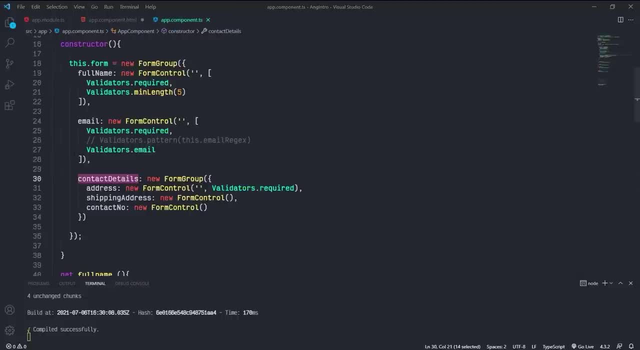 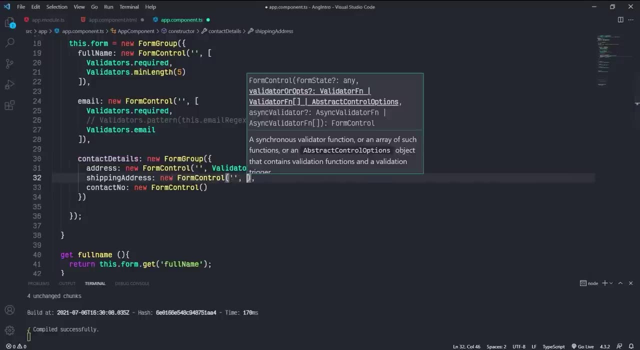 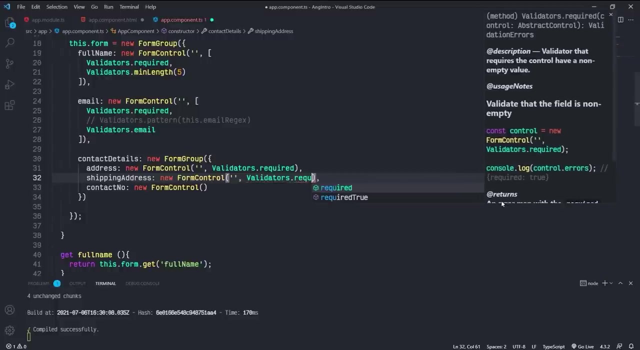 new inputs in the component file, pass the validation parameter for these inputs. first set the initial value, which is empty string. the second parameter for this shipping address, we're going to add only the required validator. so validator dot required for the contact number. let's add the validations for this. we're. 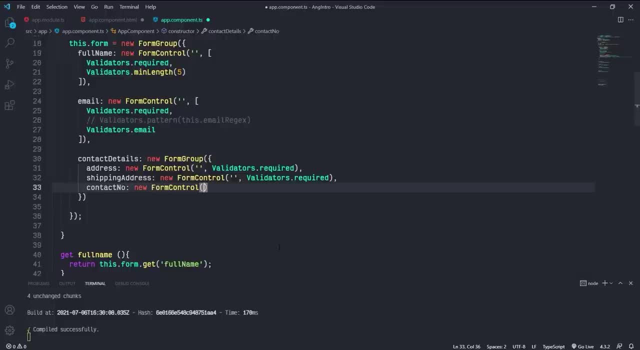 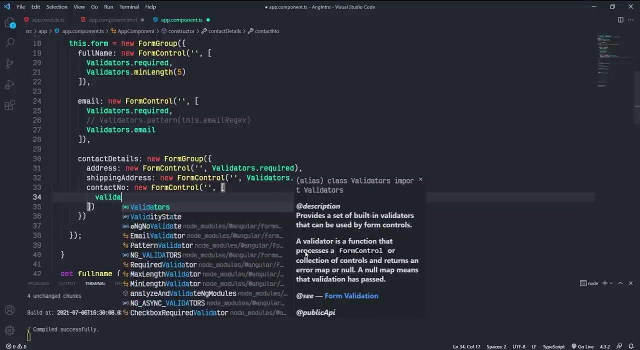 going to use two validations. first one is the required validation. first pass the default value as a second parameter. this time we're going to add the multiple validations for this, so pass this parameter as an array. so the first validator is required. validators dot required. the second validator is the. 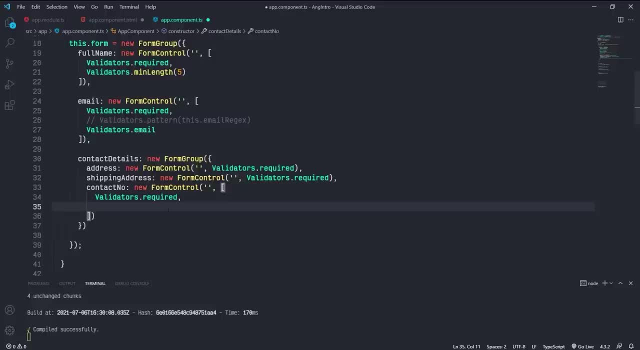 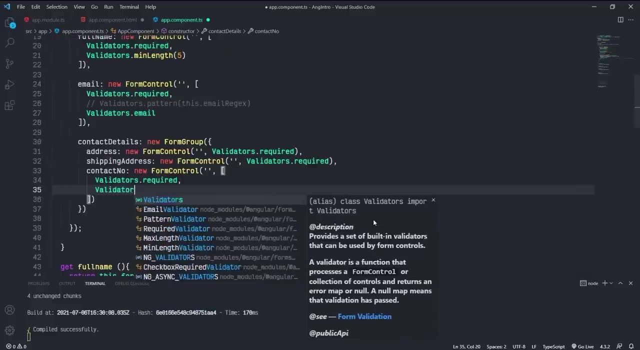 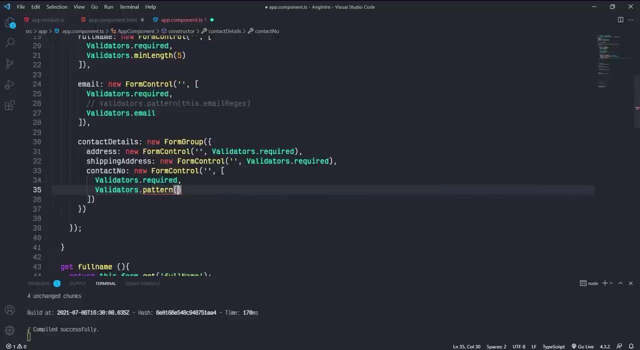 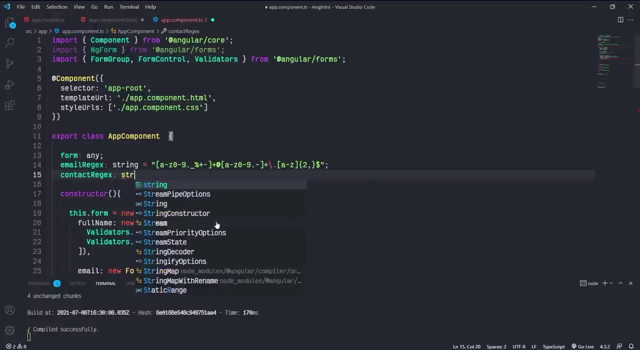 pattern. we will set the pattern validation rejects for this contact number like this email pattern validation. so validators, dot, pattern and the parentheses. now we have to pass the pattern so create a variable contact rejects. type will be string and the pattern will be this. so just pause this video and 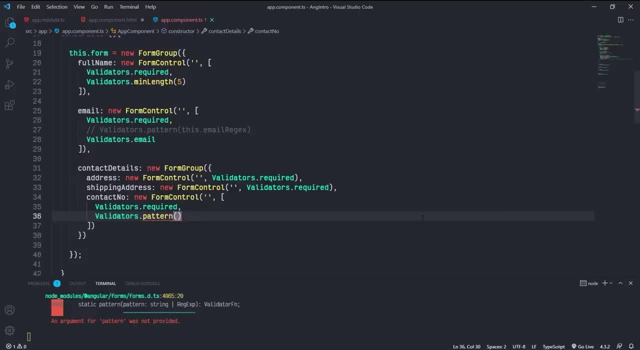 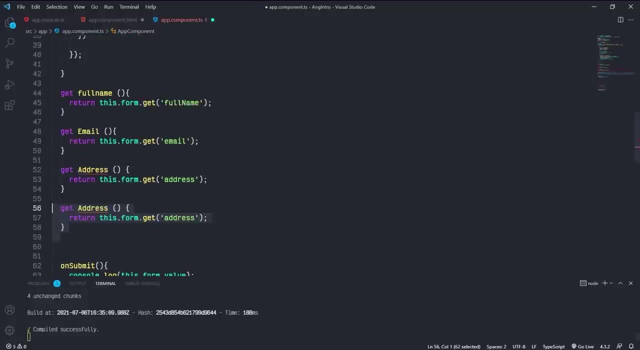 write it down now: pass this: contact rejects variable to this pattern validator. that's it now set the getters for these two fields, copy and paste. and this getters method. change the getter method name to shipping and also change this form control name. so this time this is not inside the main. 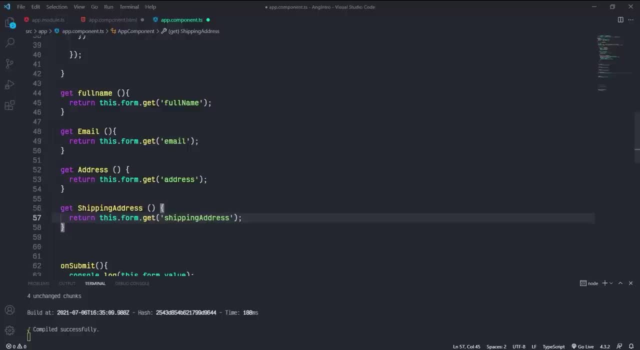 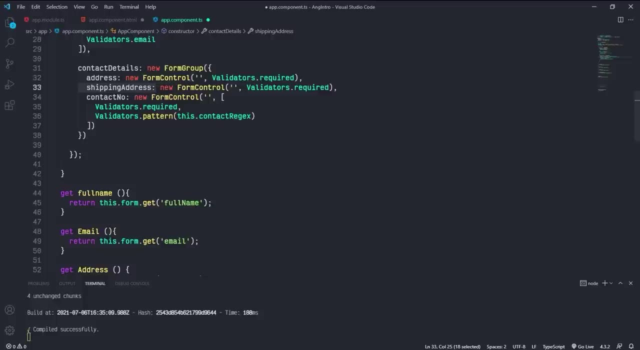 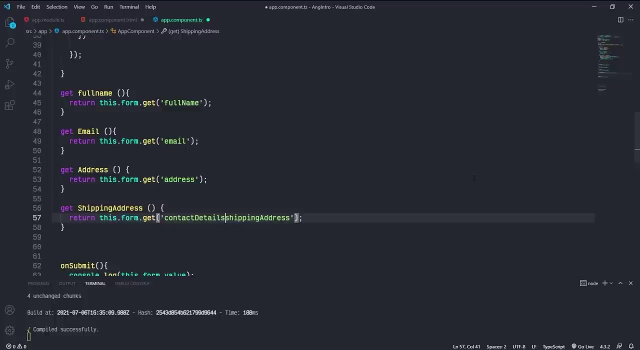 root form group. so in order to access this shipping address form control first we have to access this sub form group, which is this: contact details. so contact details, dot and the form control name is shipping address. again, duplicate this get method and change the method name to contact and. 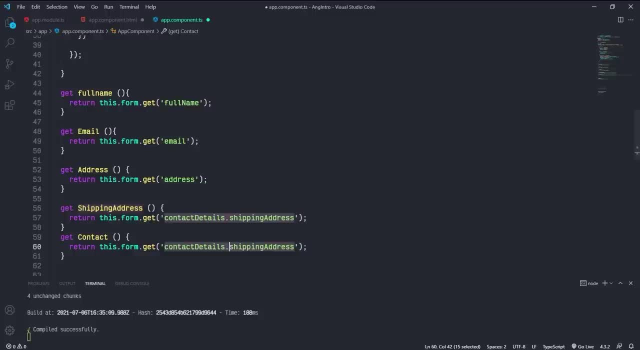 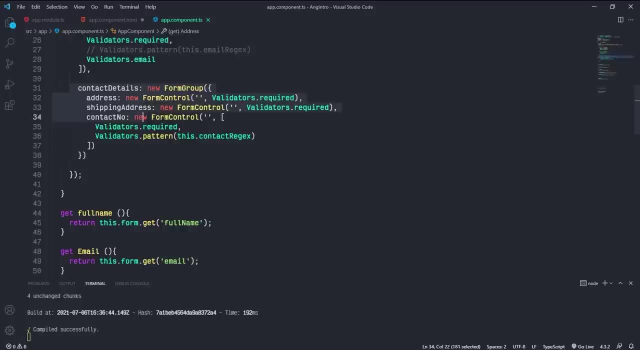 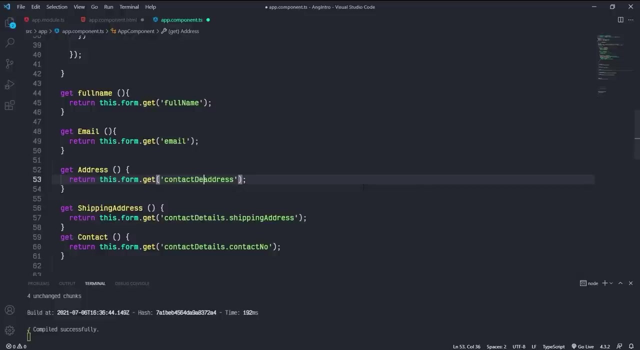 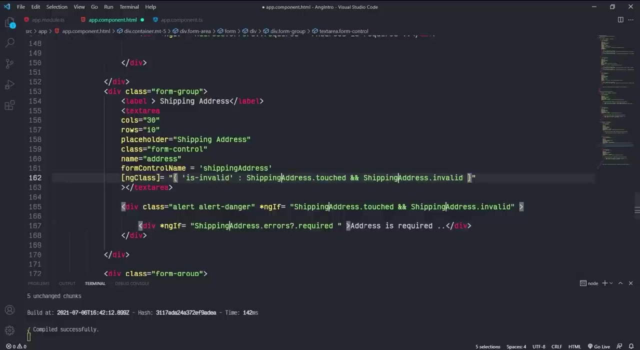 change the form control name to contact number. that's it. wait, we have another. change This address form control also now inside this form group contact details. So change this. Alright, save this file and back to the htmlb And let's add error messages. Now change this error directive names- This is shipping- and change the error. 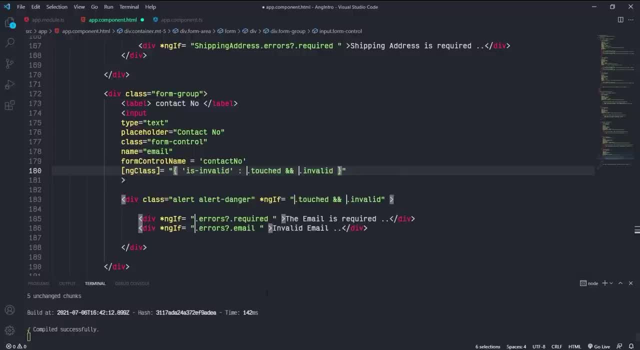 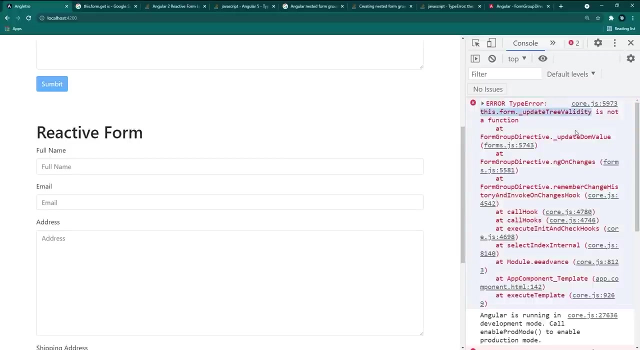 message. Next, change this to contact. and this is this time we are checking the pattern, So change this email to the pattern And don't forget to change the error messages. Save this all and back in the browser. Oops, we are getting an error here, Coz I made a mistake. 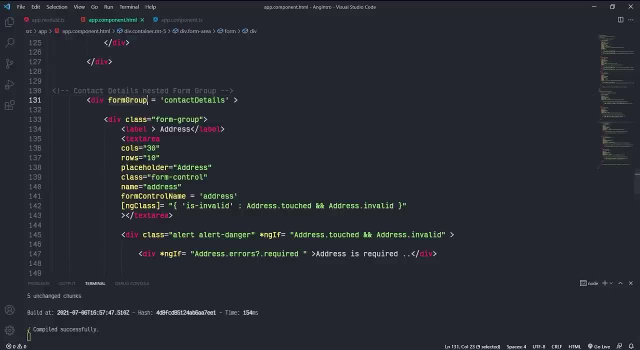 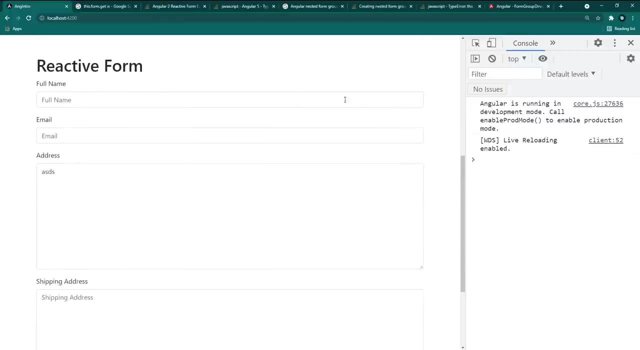 here, when we connecting this div to the instructor, Select form group. This directive must be form group name, Not just form group, So change this to form group name, Save this and back to the browser. Now we don't have any errors. 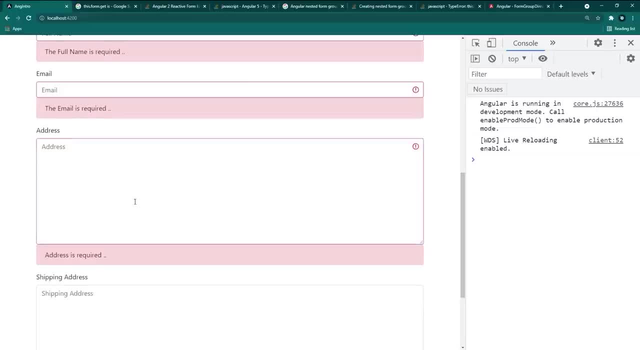 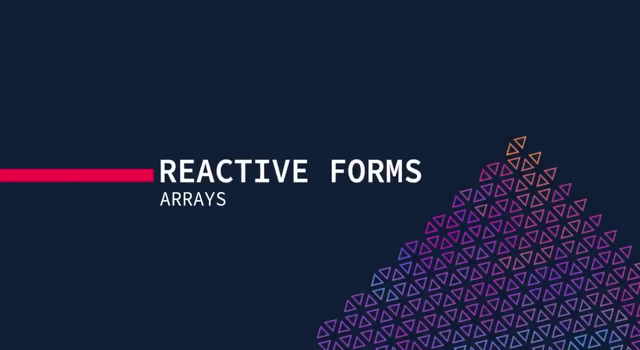 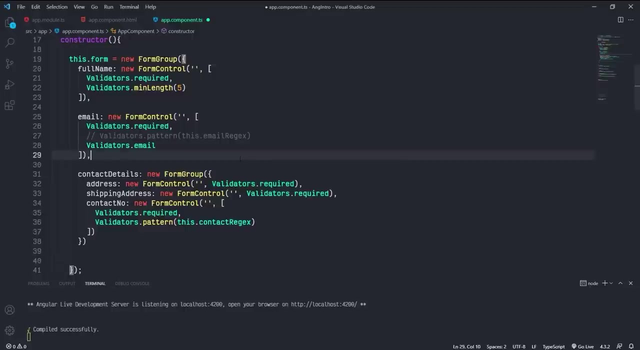 Perfect, Everything working as we expected- Beautiful. In the previous lecture, we have seen how to change the name of the file. Now let's see how to change the name of the file. In the previous lecture, we have seen how to change the name of the file. In the previous lecture, we looked at how to nest form groups inside. 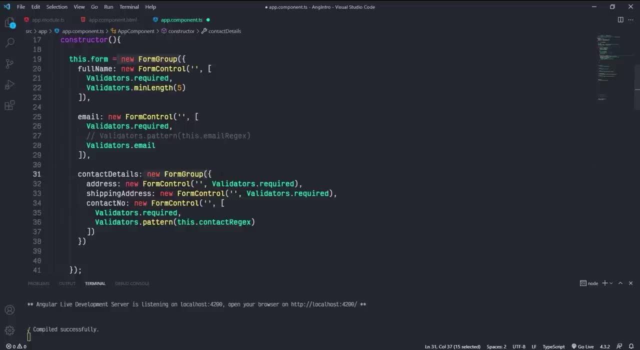 form groups. So in this section let's learn how to deal with form array class. Think, if we have an input field for add skills, A person can have multiple skills, right? So in that case we have to store those multiple skills inside of a form array. So let's see. 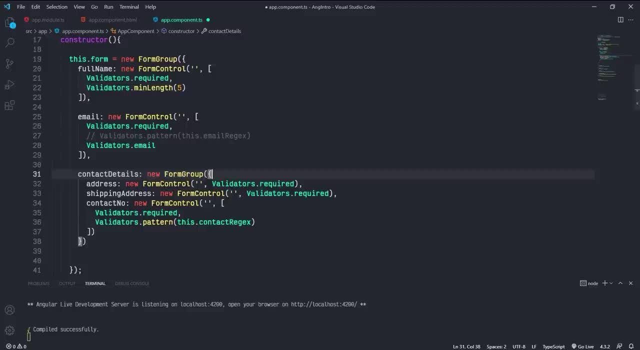 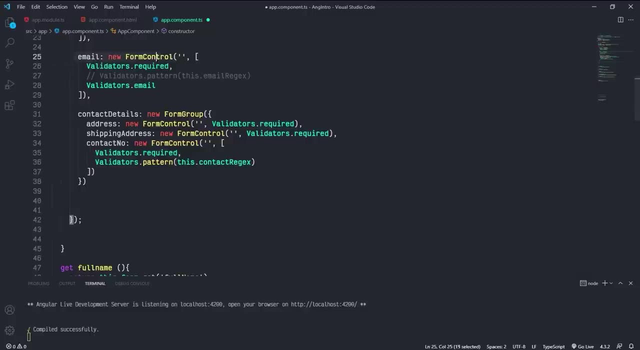 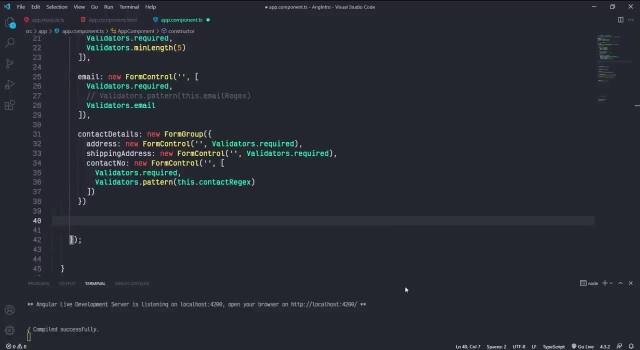 this in action. Let's create a form array inside this form group. This is also the same as creating these form groups and form controls. So, first, the key: I am creating this form array to store skills. So key is skills and value will be a new instance. 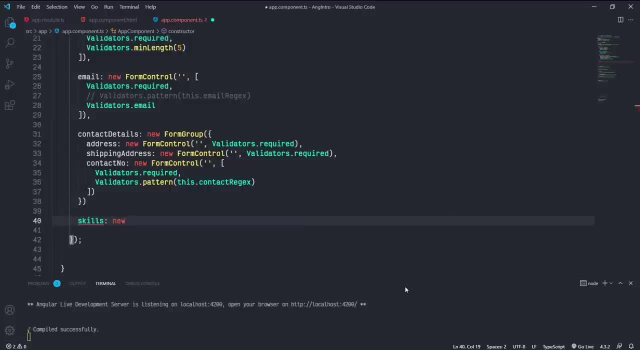 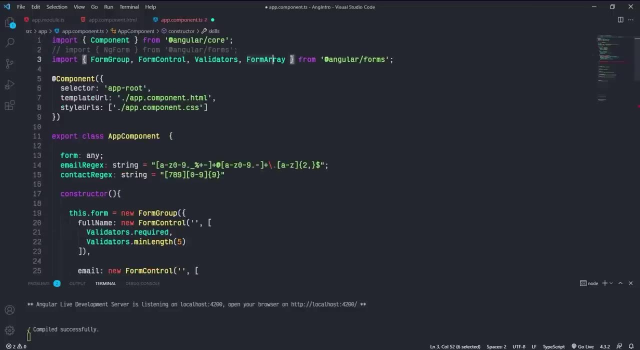 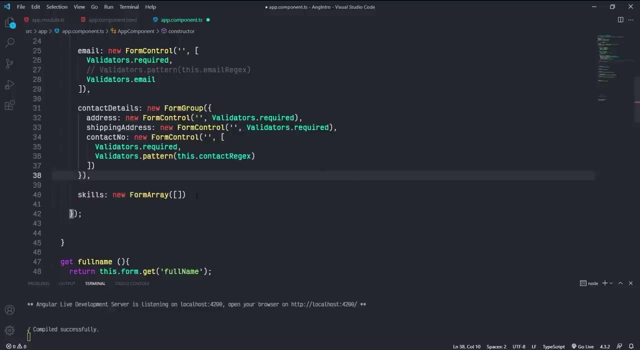 of form array. So new form array. Select this to complete. This will automatically import this form array module to this component. Alright, Pass an mtl Empty array as an argument for this form array. Now let's see how to push data dynamically. 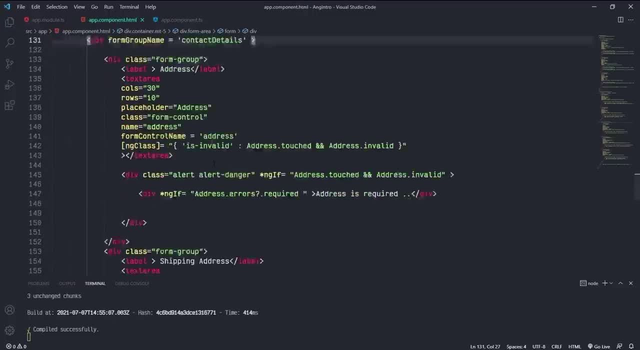 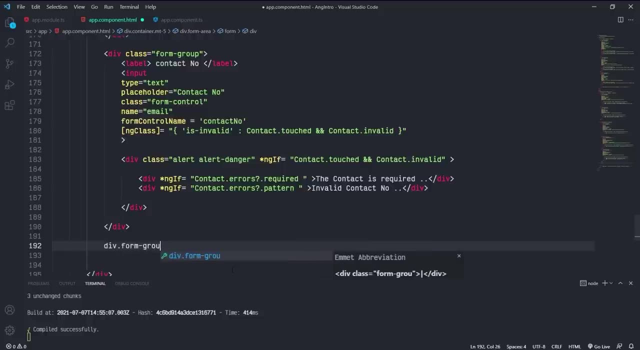 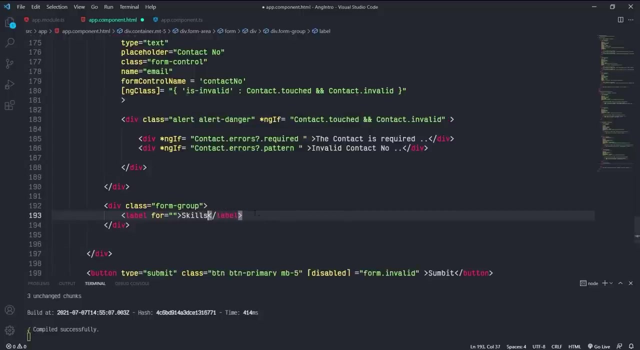 to this form array, Save this and create an input field for skills After this div with a bootstrap class form: dash group. Inside this label and label text will be skills After this input field with bootstrap class form: dash control. Now let's add a keyup event for this input field Inside brackets: keyup and I want to. 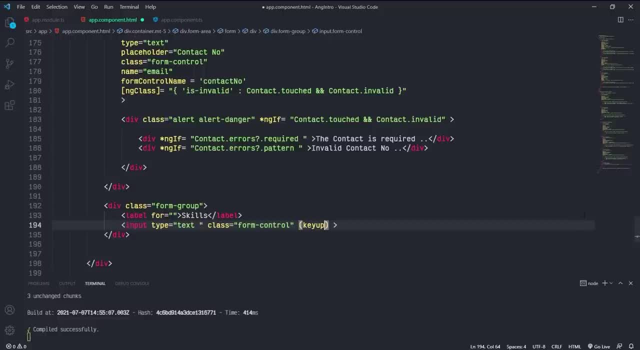 trigger this keyup only when the user press the enter key. So add an event filtering for this. So keyup After this dot and the enter. We already learned about this right, So now bind this to a method called something. add skills, And don't forget to add the parentheses. 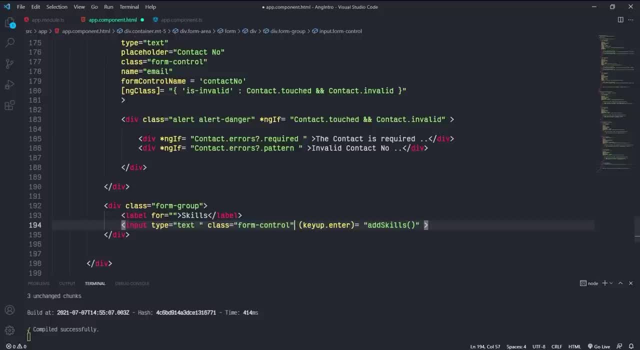 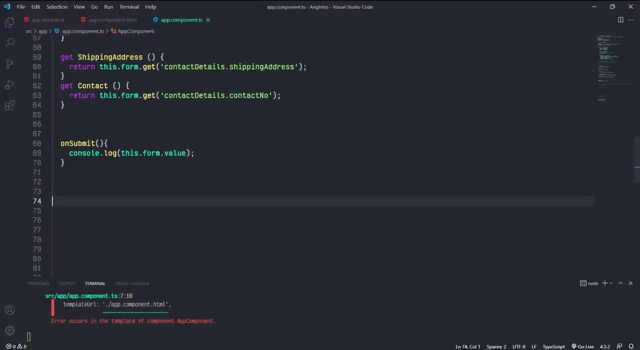 In order to get this input values, Create a template variable for this input Hashtag skill And pass the template variable to this method. That's it Now. save this and back to the component file and create this add skills method. So this sending a parameter. 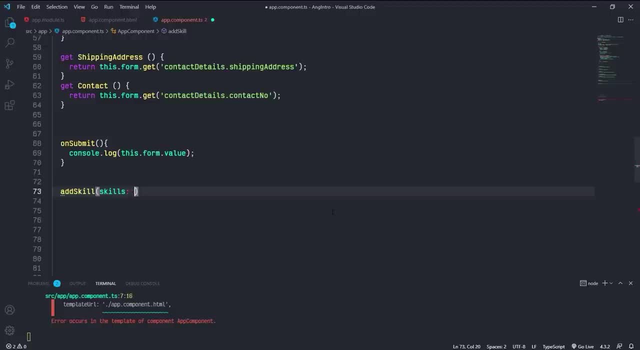 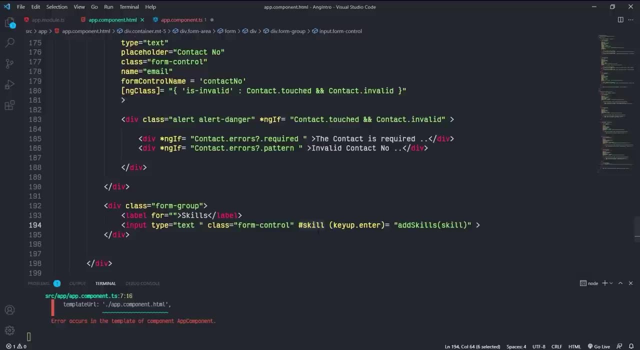 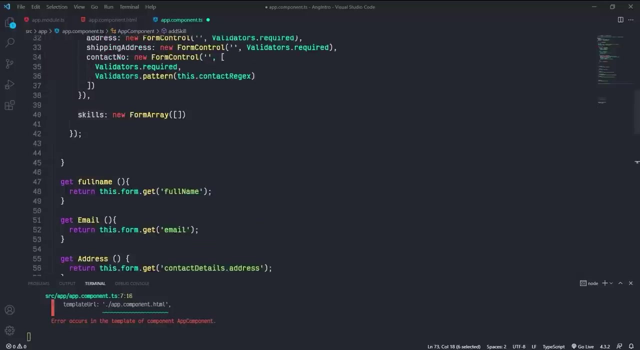 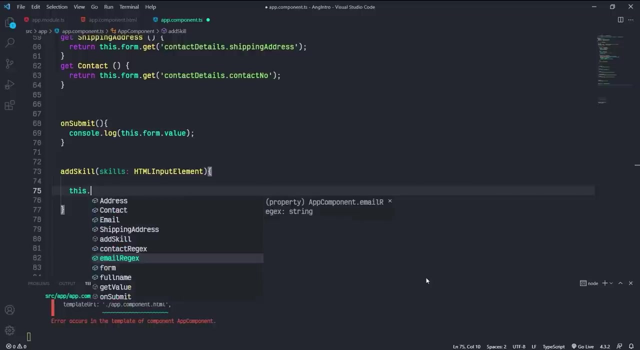 So capture it Skills Now set this variable type to html input element, Cause this is this template variable, which is an html input element. So now, inside this method, let's push this input value to this form array, So this dot form, Which is this main form, Dot get. 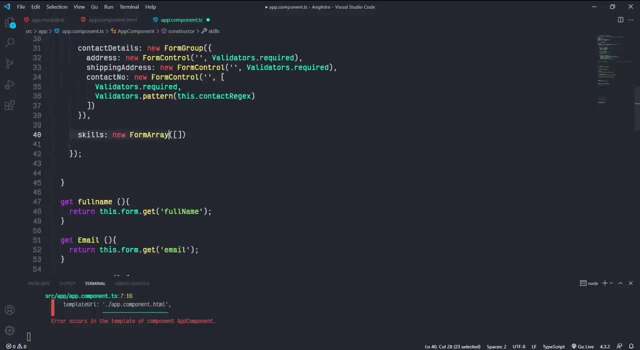 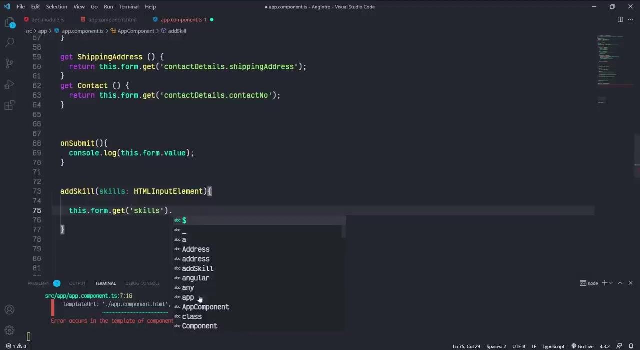 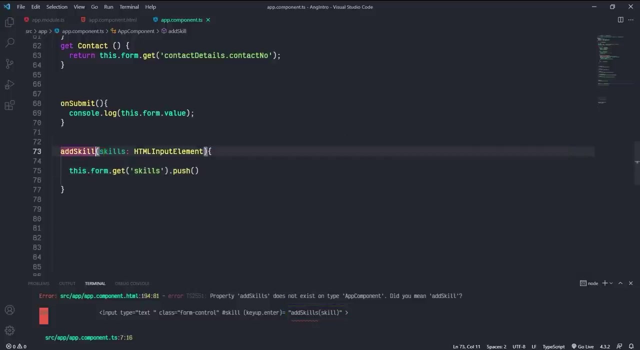 And we want to access this. skills So, skills. So pass this inside this parameter. In our order to push value to this array, We have to convert this to a form array. Look at this: We don't have any push method for this form group, So convert this to a form array. Very, 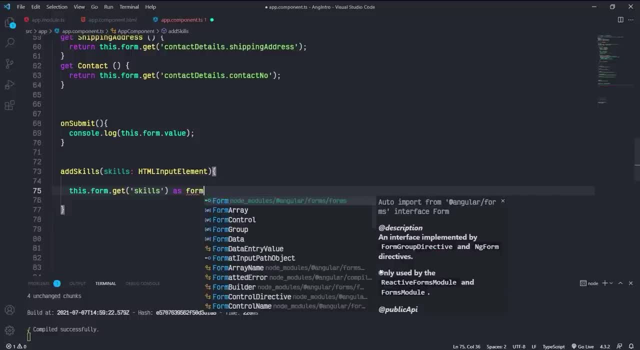 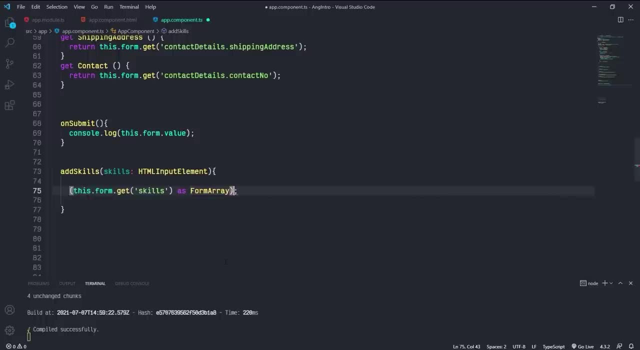 simple. After this, add this statement as form array. Alright, Now put this all inside of brackets. And now we can use the push method with this Dot Push. This time we are not getting any compile errors. Now push this inputs value to this form array. So first, 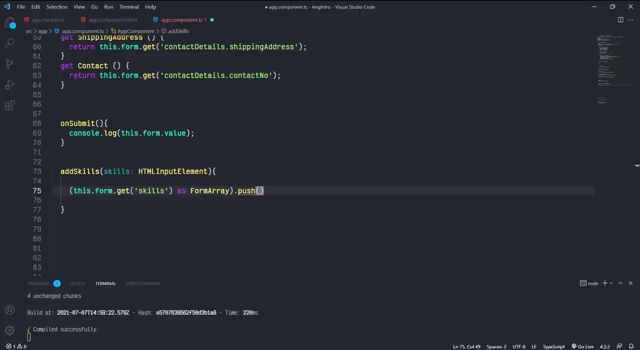 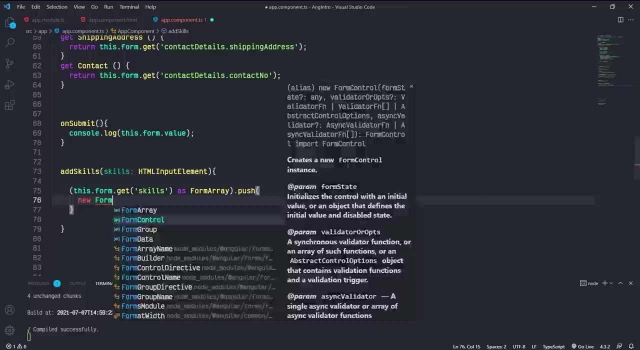 we have to create a new instance of form control or form group Like this. This is simple input data, So I am gonna create a new form control instance. So inside this Push method And add new form control and, parenthesis, Now push the value to this new instance Inside. 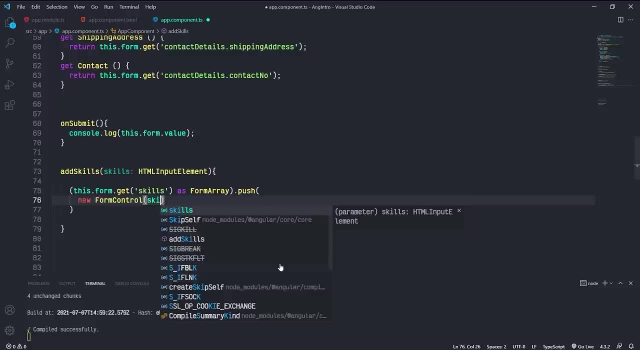 this parenthesis Skill, Which is this parameter, variable And value. That's it. Now let's log this form group's value to see whether this pushing is working or not. So after this log this form dot value, Save this all and back to the browser. Type something inside this skills field And hit. 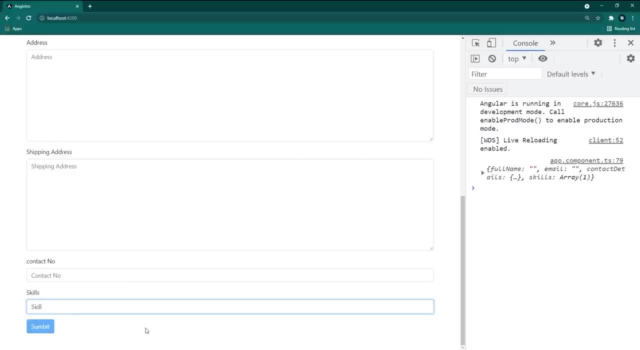 enter Inside the console. we got this form: group values. Inside this, we got this skills array. Expand it. Inside this array we got this type data Again. type something and hit enter. As you can see here, we got this second value also inside the skills array. 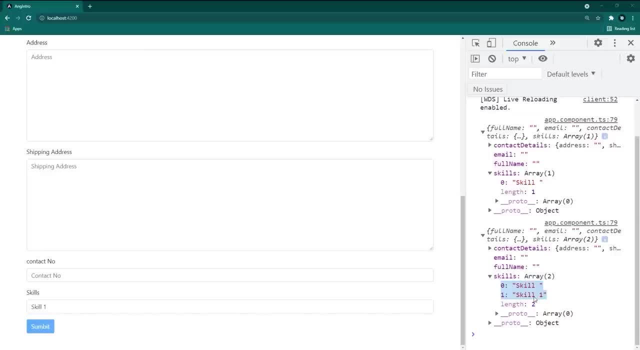 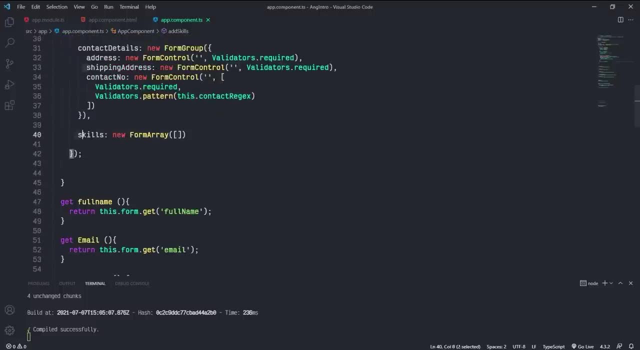 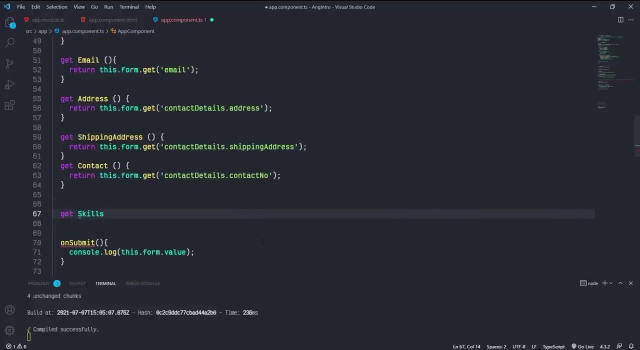 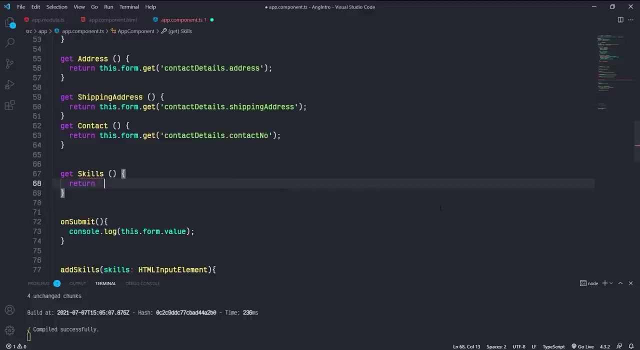 Alright, Now render this skill form array values inside the view Back in the vs code. First, let's make a getter class for this as well. After this get, The method name is skills. After this parenthesis And the scope Inside this return This dot form dot get Inside. 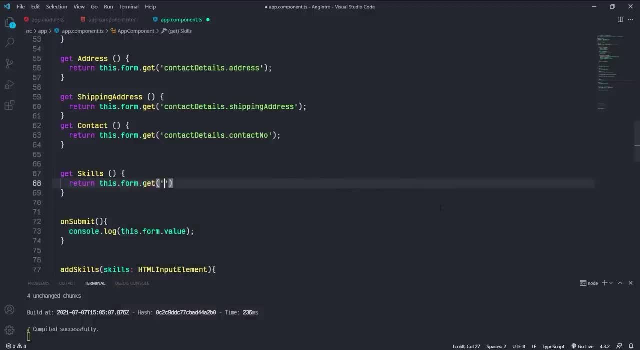 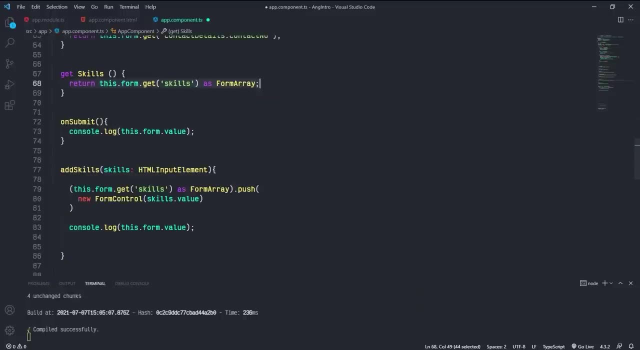 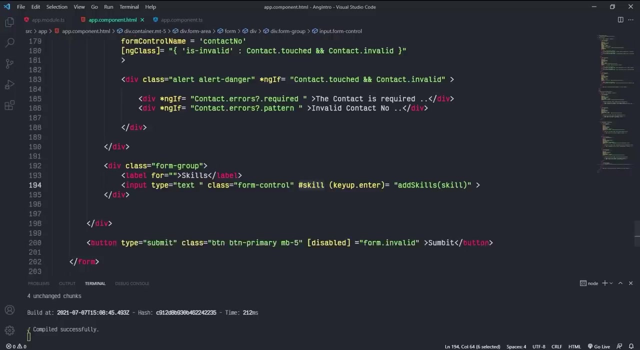 records: Skills dot. get Inside quotes. Don't forget to put this inside quotes After this- as form array. Now we can remove this entire line and add simply this getter method name: skills. That's it, Alright, now back in the html template. Now let's render this skills form array data using: 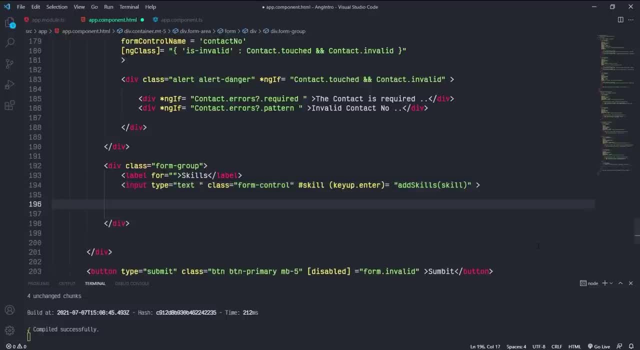 the ng4 directive Inside quotes. Don't forget to put this inside quotes After this as form array. Now we can remove this entire line and add simply this: getter method: name skills Again. return this to topElector Saygano. pivot to original aN. zumindest use your. 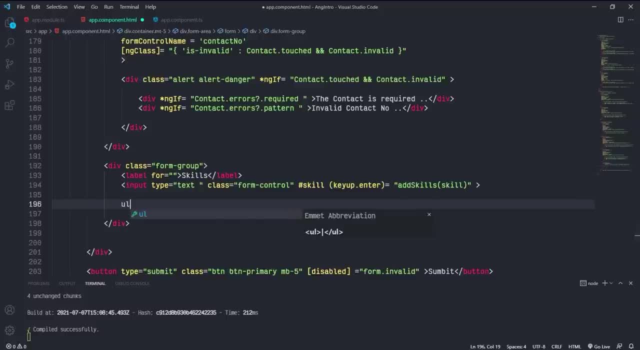 recursive form. So after this, skills input: Undoed list with booster class: list dash group. Inside this ul Li tag with list dash group, dash item: booster class. These booster classes will give a nice unolded list. Now lets render the array Here: write getter. array on it with. use a helper. Insert the list tag- ng4 directive. Insert the node with button. Oftentimes if you want it to actually run or kind of have aaku with empty word crt, then you can write in the Word lib lines. No need to change the code name for the other side. Not saying a knife, but 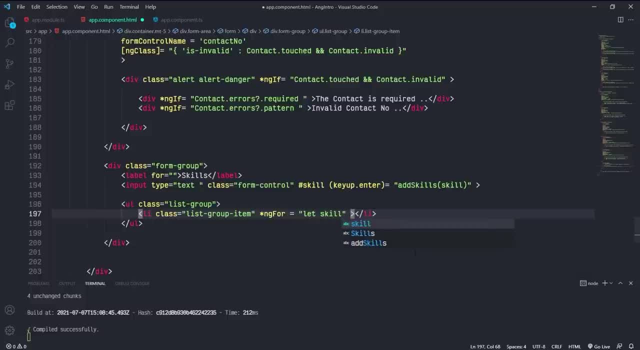 it's cool to the end of the argument. If you might want to keep things on a so called algorithm, it's very all. once you get a short of it, write a paragraph in the這 auna without in a inside codes. let skill of the getter method name is skills and if you can remember, we 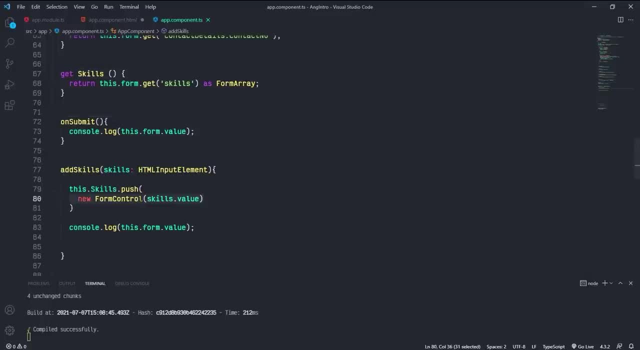 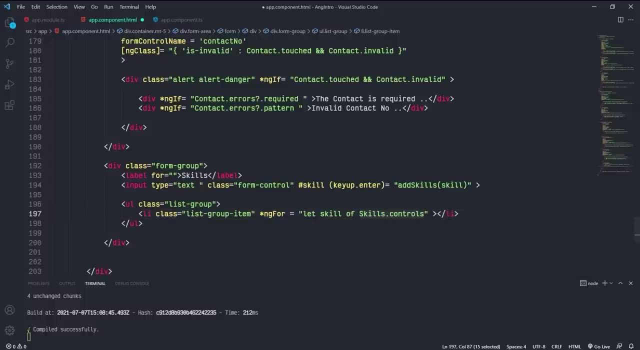 are pushing form controls to this form array. So after this controls, this will render all the form control values inside this form array. Now, inside this list, let's show the data using the string interpolation Add string interpolation skill, which is this variable and dot value. 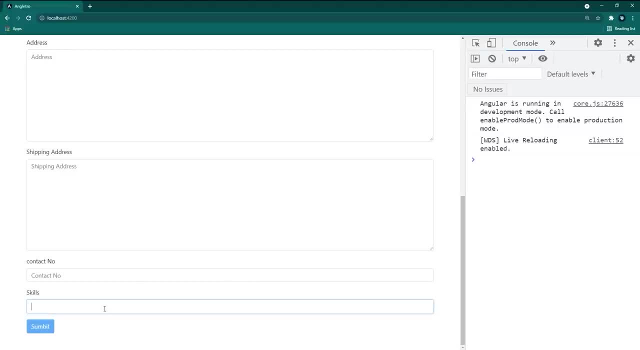 Perfect. now save this and back to the browser. Type a skill, something angular, Hit enter. As you can see here, this rendered inside this bootstrap list. Again, type something, react and hit enter. Perfect, right, Everything working as we planned. Now let's add a method to clear this input fields. 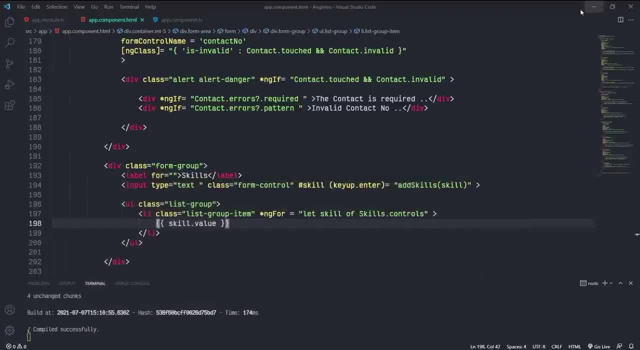 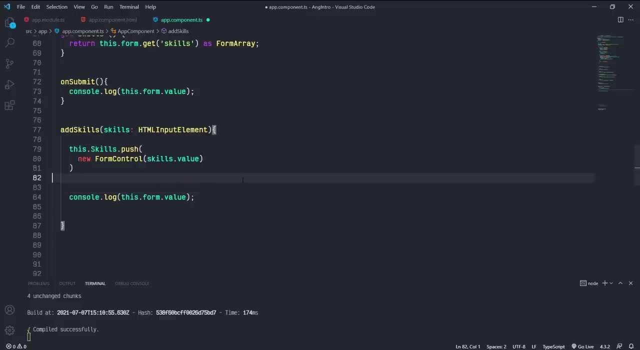 After adding a string, New skill. Very simple, Back in the VSCode, Go to this add skill method and reset this skillHTMLELEMENT value, Skill dot, which is this parameter Value. assign it to an empty value, Save this and back to the browser. 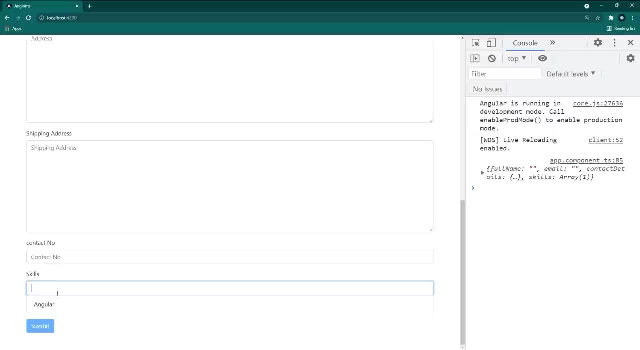 Type a simple skill and hit enter. As you can see here, soon after we click the enter button, this input fields Value set to empty. Beautiful, Alright, at last let's see how to remove a form array value programmatically. First, add a delete anchor tag for this list. 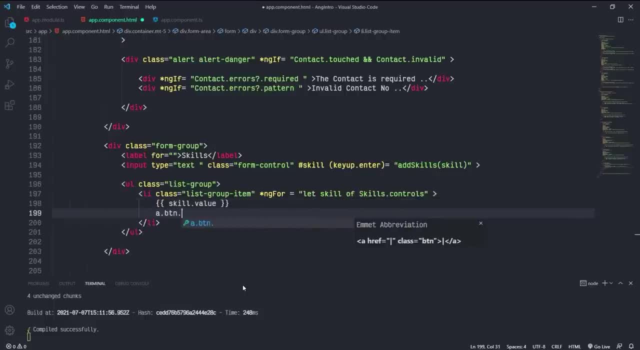 Now, inside this, create an anchor tag with these bootstrap classes: btn, btn-sm- this is for small buttons- and btn-tanger. The anchor text will be this: x as the cross icon for right Cross icon for removing data. Now add a click event for this button. 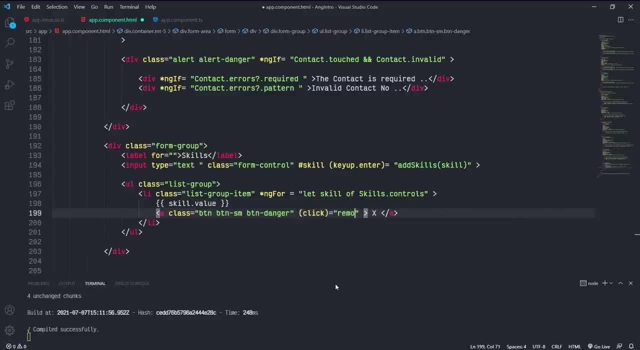 Inside brackets, Click Assign this to a method called removeSkills and the don't forget to add the parenthesis. In order to remove a value from an array, we need the index of that removing data. So let's get the index of this array. 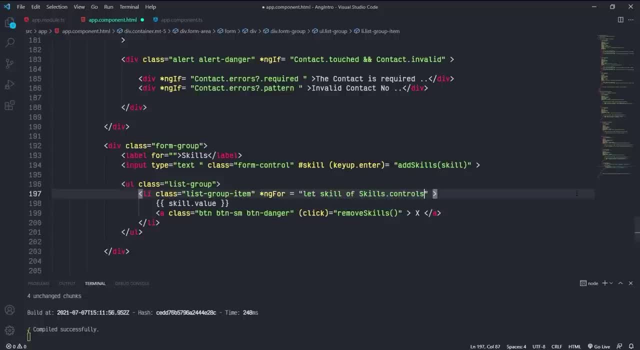 If you can remember, we learned about this when we learning ng4 directive. So after this, Add a statement semicolon. let i assign index. With this, we are assigning this array's index to this variable i. This can be any variable name. Now pass this index to this removeSkills method. 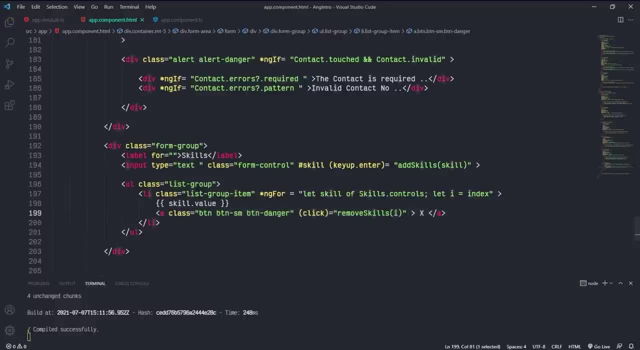 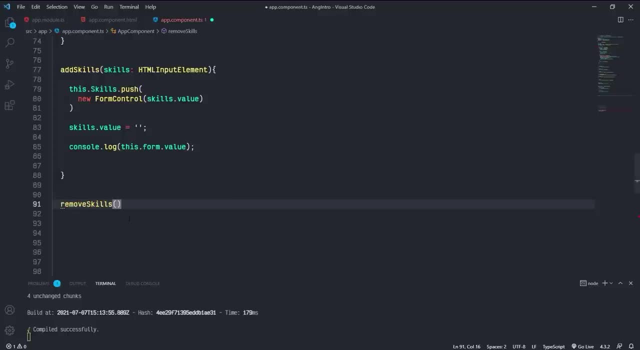 So we can remove that value from the array using the array index number. Alright, now go to the component is file. Create the removeSkills method. With this method We required the index number, So set a parameter variable index. Now, inside this, let's add the remove statement. 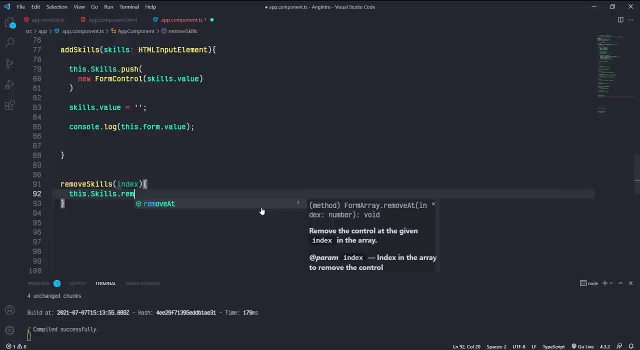 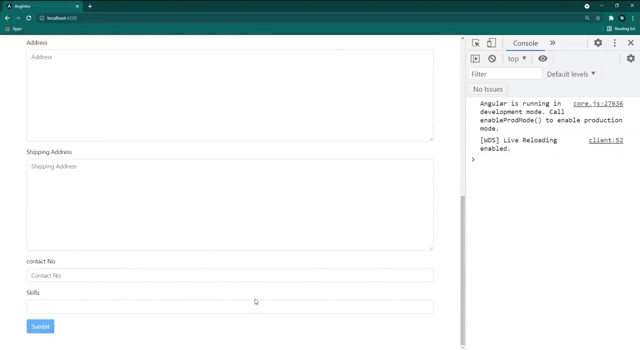 Very simple, This getter method, which is this: skillsremove- inside brackets. Pass the index number that we are getting from this parameter. That's it. Save this all and back to the browser. Add some skills Angular Javascript React. Now remove this angular from the list. 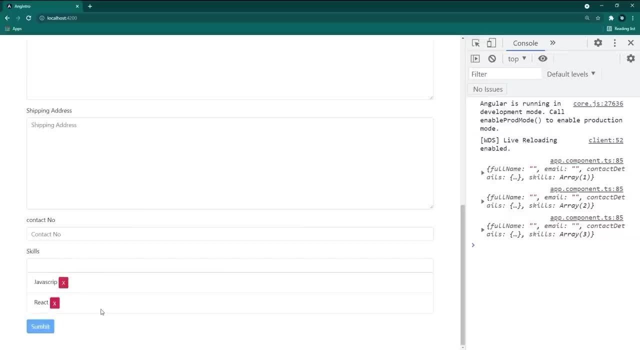 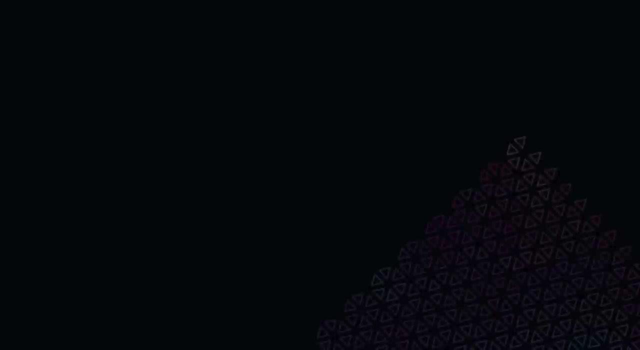 As you can see here, This removed from the list. Again, remove this react. This also removed from the list. Beautiful, Isn't it? So this is how we deal with angular reactive form arrays. So until now, we have created the Angular Reactive Form Arrays. 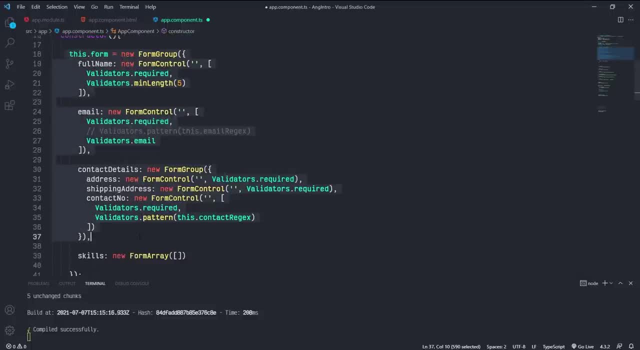 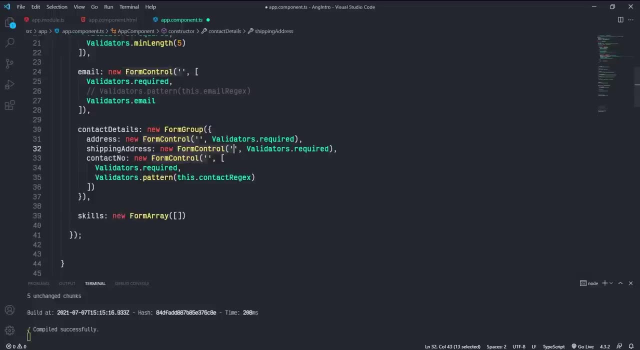 Let's see how we can use it. Let's see how we can use it. Until now, we have created these form groups and form controls. If you look at this, as you can see, we are repeating this same new form control instance again and again, which is making our code a little bit noisy. 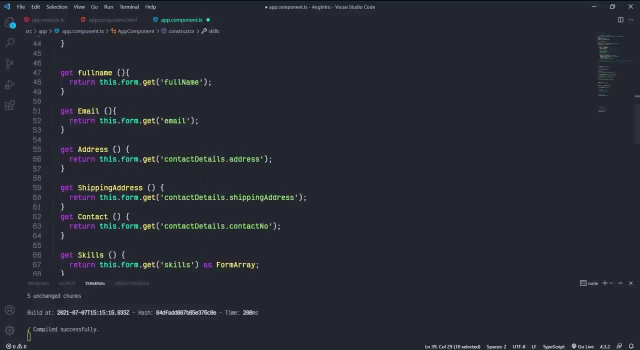 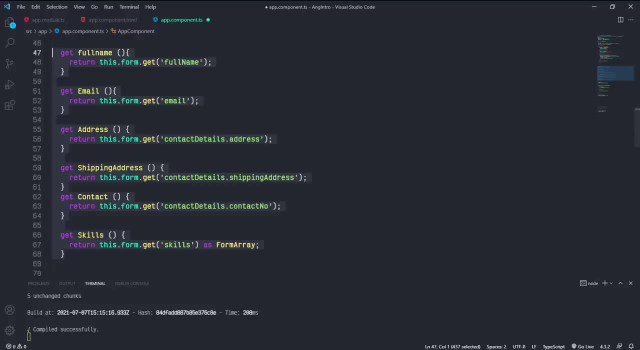 Right. And also we have another problem. We have almost created five getter methods for these form control to simplify this inside the HTML wave template. For a small form like this, This is okay, But think If we are dealing with more than 20-30 getter methods. 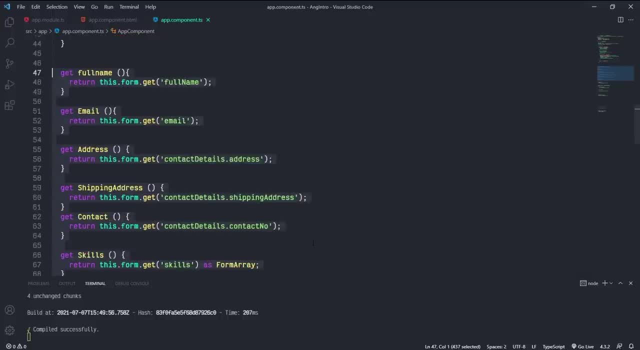 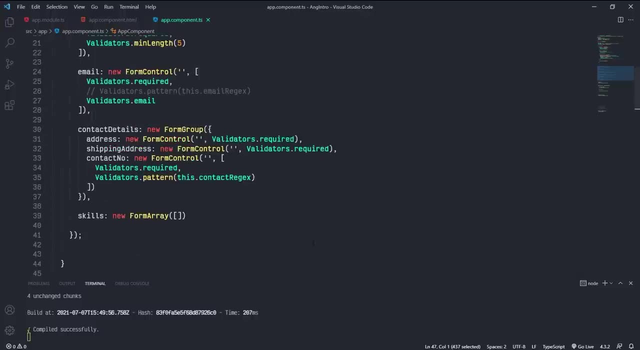 This is not enough If we are dealing with more than 20-30 form controls, creating these getter methods for all those form controls. it's a big pain, right. As a solution for this, we have a better approach, which is angular form builder. 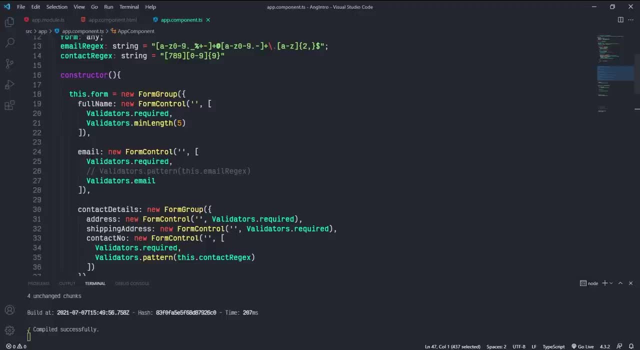 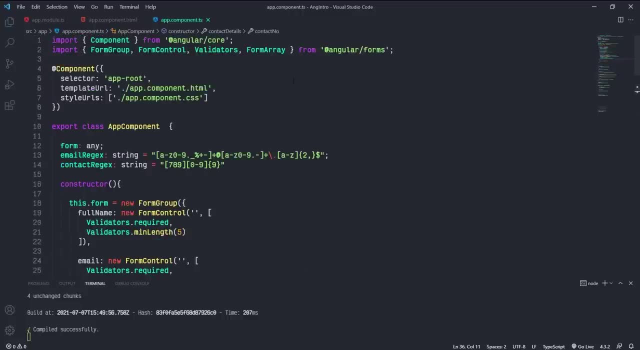 In this lecture let's look how to make this noise code to clean code using this angular form builder. First, import the form builder module to this component file form builder, this also coming with this angular forms module, So put this inside this same import form builder. 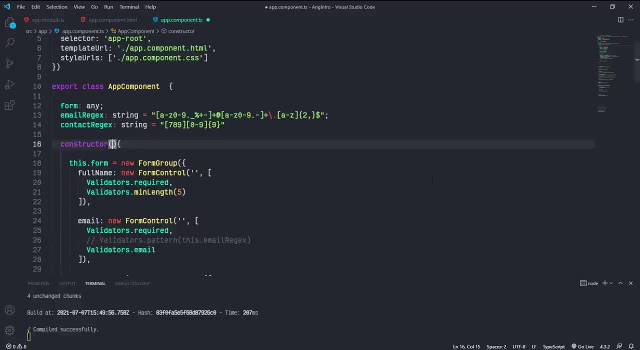 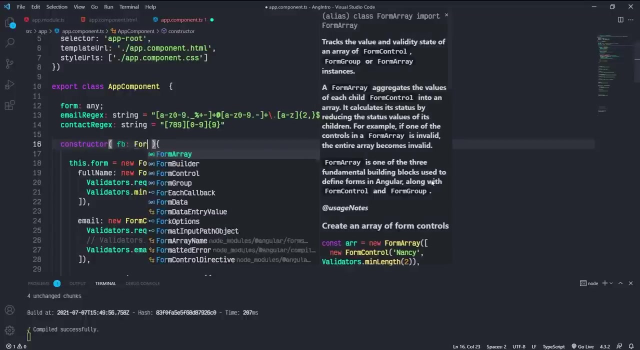 Alright, now we have to inject this into the constructor. We learned about this dependency injection when we learning angular services. Hope you guys remember this Alright. inside the constructor FB, this can be any name And this type is form builder. which is this imported form builder? 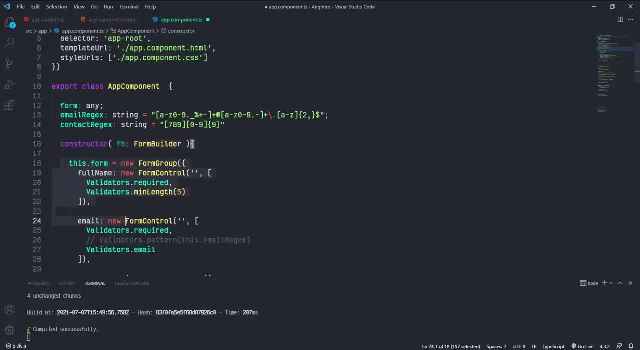 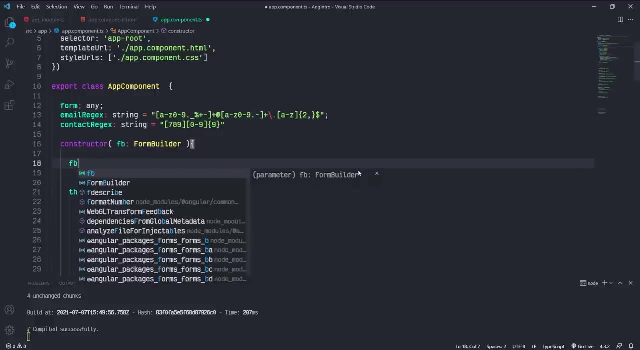 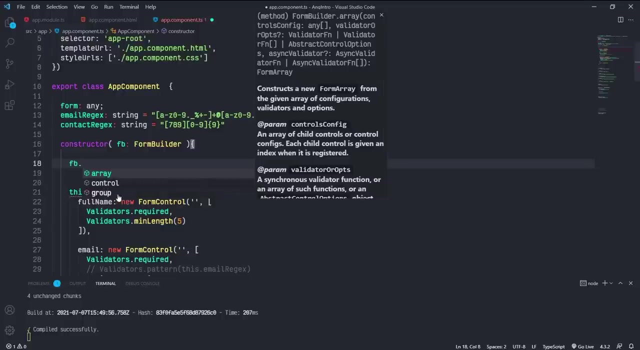 Now let's recap. Now let's recreate this form group using this form builder. Inside this constructor, let's create the form group FB dot. with this form builder, we can build these three types of new class instances: very simple group control and 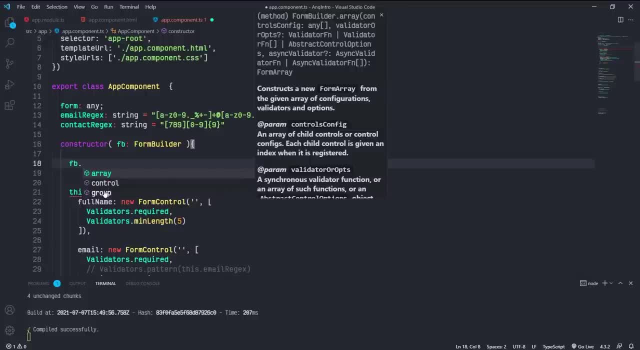 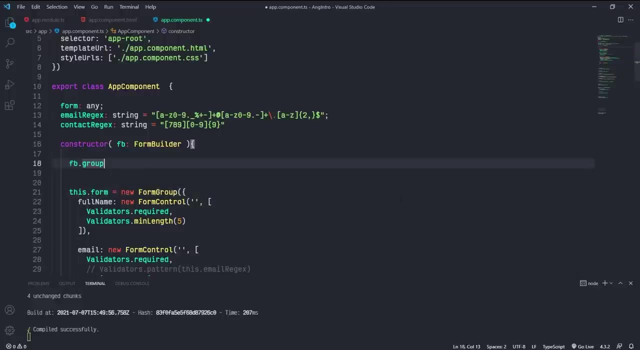 array. We use the group to create form group. we use the control to form control and the array for form arrays. Alright, So first we have to create the form group, So select the group For this, also same as this previous required an object. inside this we have to pass key. 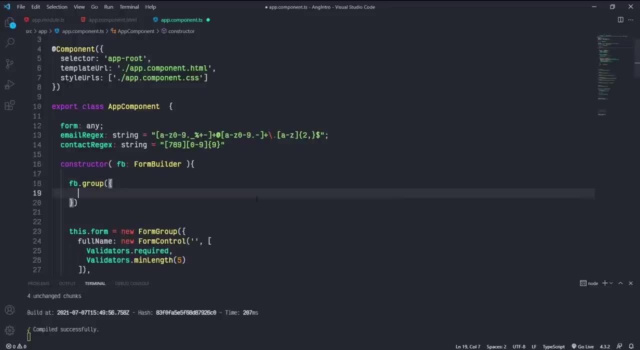 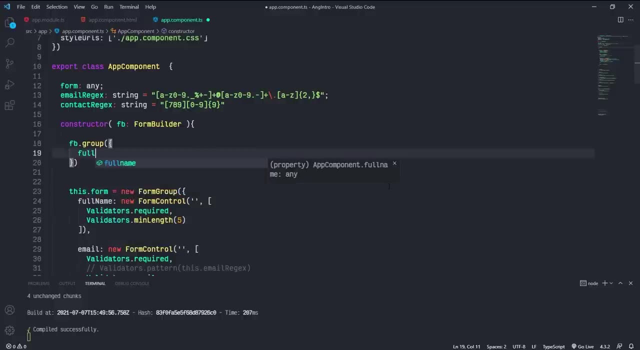 value pairs which can be form group or form control or a form array. So first we have the first name, So the key is first name and the value is FB, dot control and the parentheses. In form builder we have another, cleaner approach for this form control. 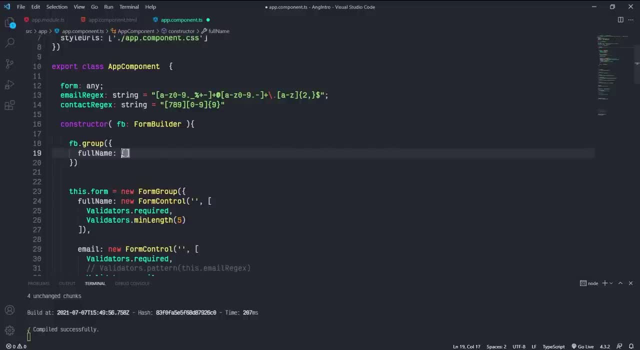 So remove this and just simply add a square bracket. This represents the new instance of the form control class. Less syntax and very clean approach, right. Next, we can pass the validation same as this. So inside this square bracket, first the default value and as a second parameter, we have to. 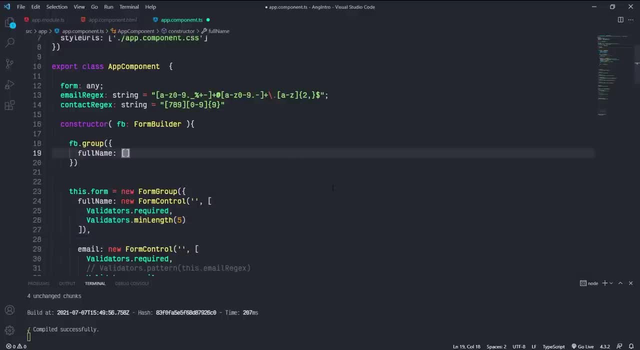 pass the validation. So nothing special here, same like the previous method. So we got two validations for this first name field required and the min length, So we can pass multiple validations as an array. So create an array inside this first validation. validator dot required. 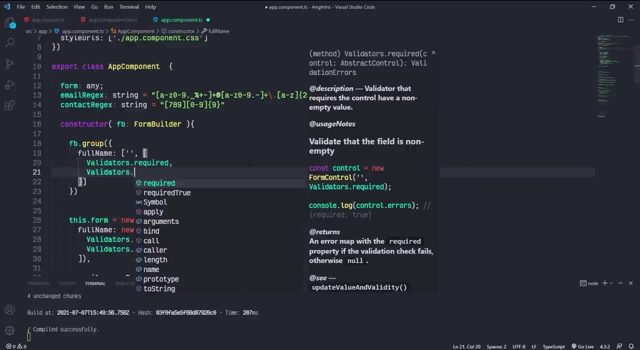 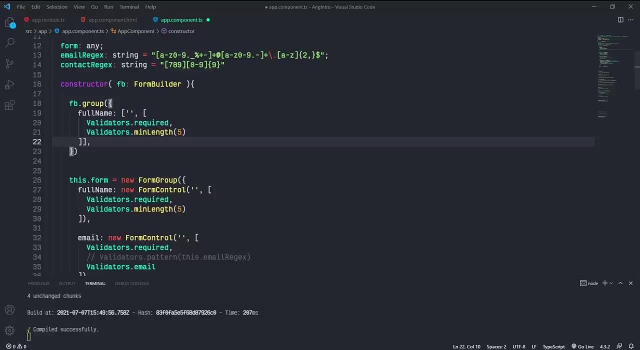 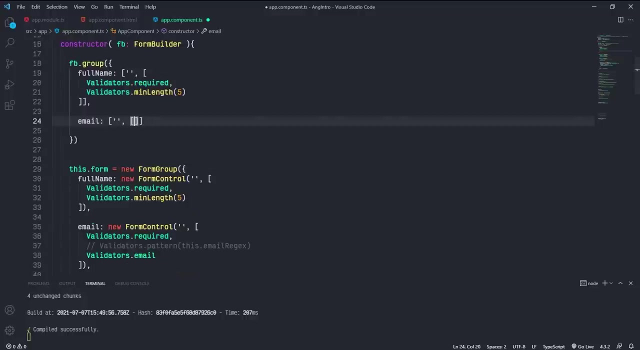 The second validation validator, dot min length. Inside parentheses set the min length count, 5.. That's it. So next we got the email field. same as this key is email and pass square bracket for new form control instance. Inside this, pass the default value and pass the validations required and email. 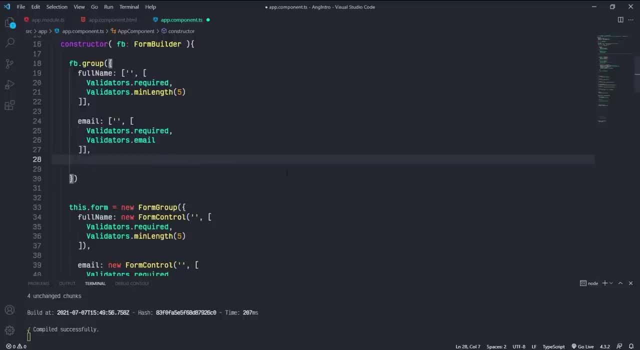 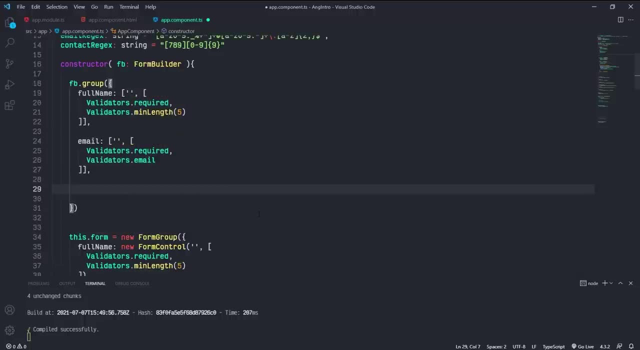 Next, we got this contact detail form group. The key is the form group name, which is this: form details. This time we gonna create a nested form group, So we have to type that This square bracket thing is only available to create form controls- new instance. 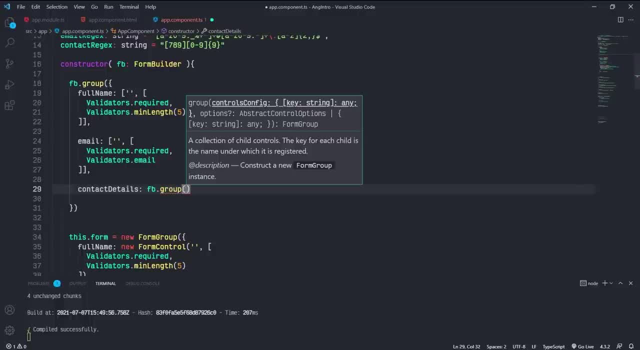 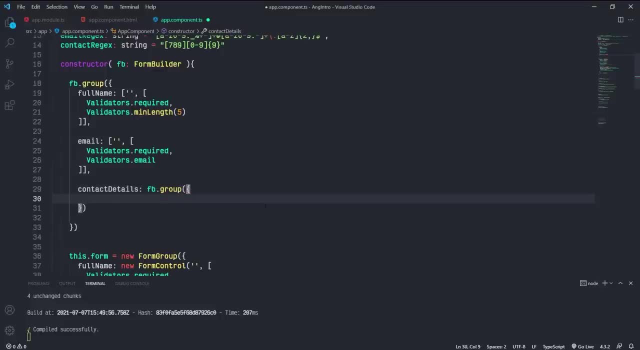 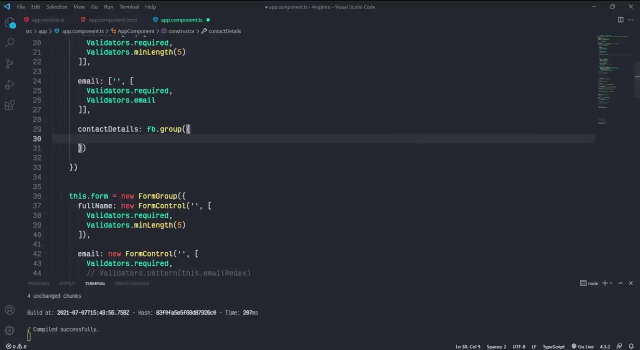 Okay, After this fb dot, which is this injected form builder Address group and the parentheses. So inside this parentheses we can pass the form controls as object key value pair same as this. So inside this create an object. 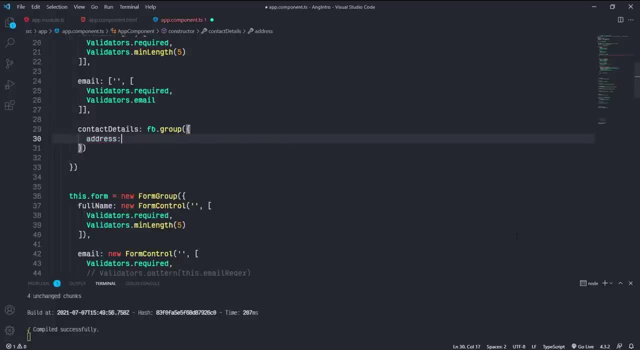 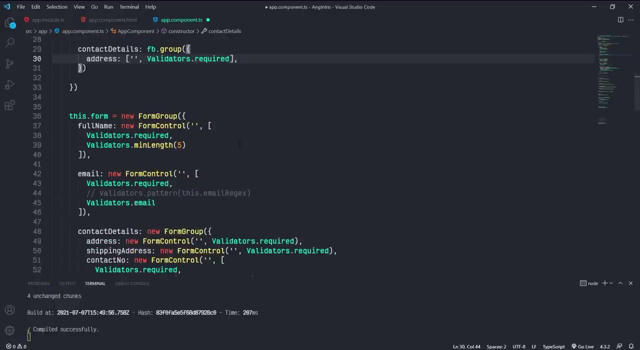 This first form control is address and pass square bracket as a value. So inside this pass the initial value and the validators For this address form control. we only have this required validator, So add the required validator. So second contact form form control is this shipping address. 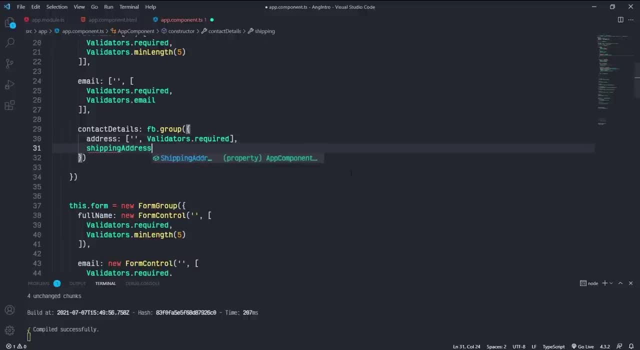 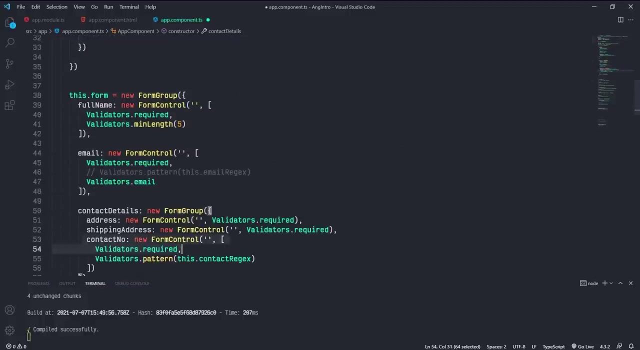 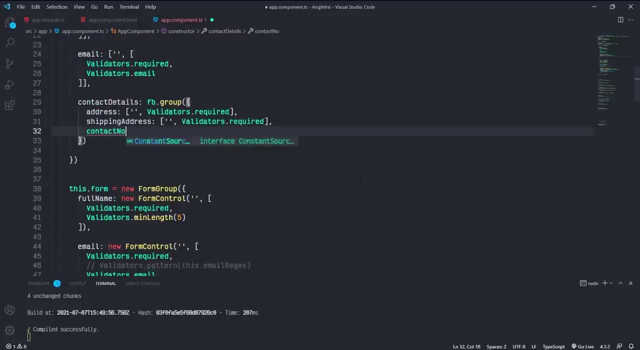 The key is shipping address and the form control. This also same as this pass, the initial value and the validations. So after this we got the contact number. So the key is contact number and the form control. inside this, This time we got two validators. 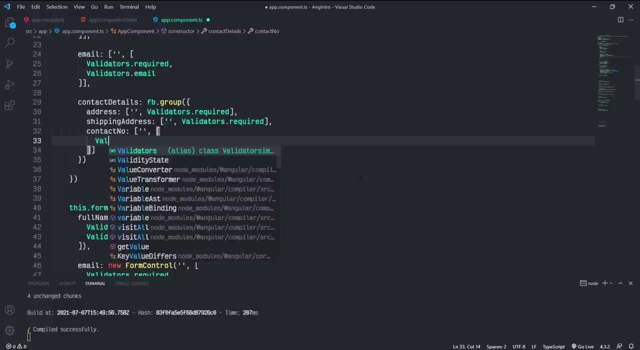 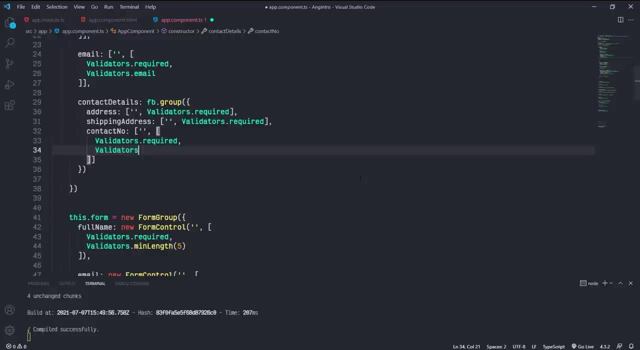 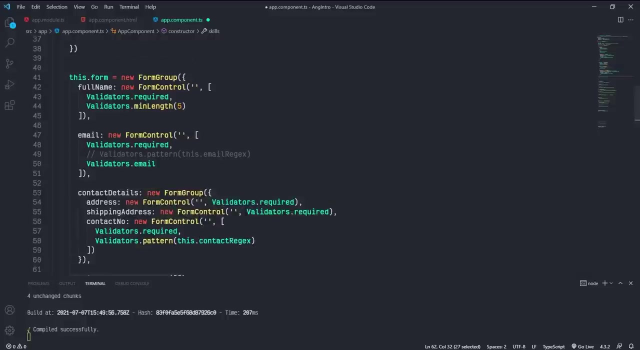 So pass two validators as an array: Validators- dot required and validators- dot pattern. Inside this pattern, parentheses pass. this contact number rejects. Okay, That's it for this. contact details form group. At last we got this skills array. Let's see how to define an array using the form builder. 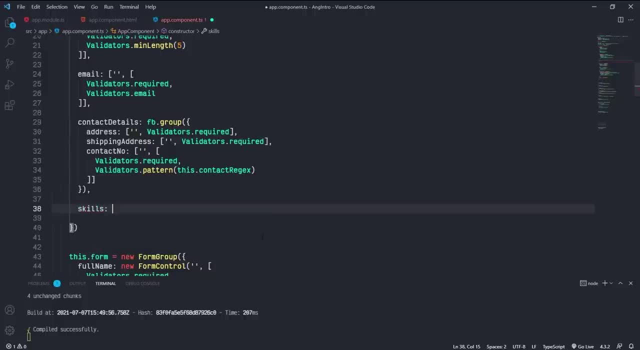 As a key pass the array name skills. Now let's define the array fb. this form builder dot. and this time we are planning to create an array, So select array and parentheses Inside this. create an empty array. Alright, so we have successfully created this form using the form builder. 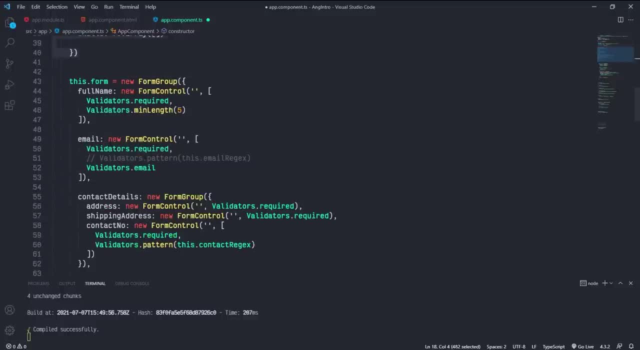 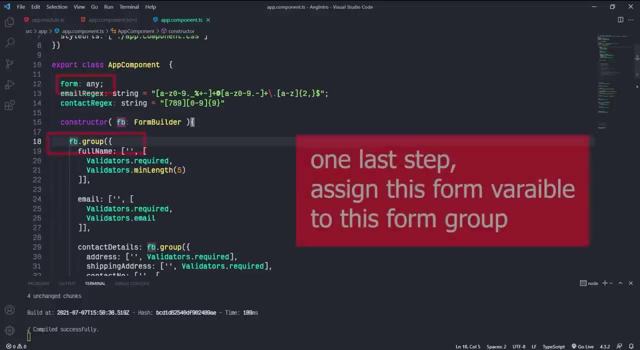 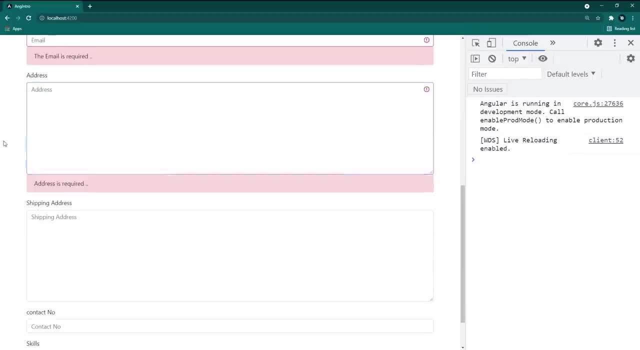 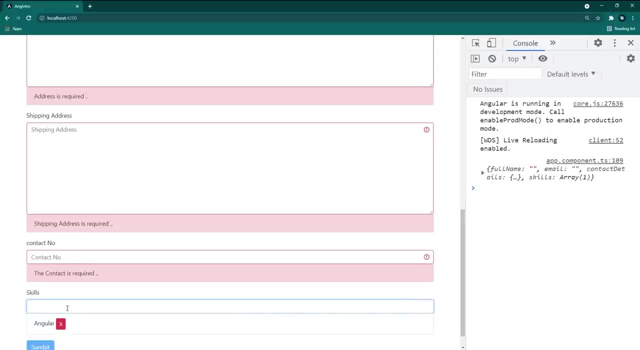 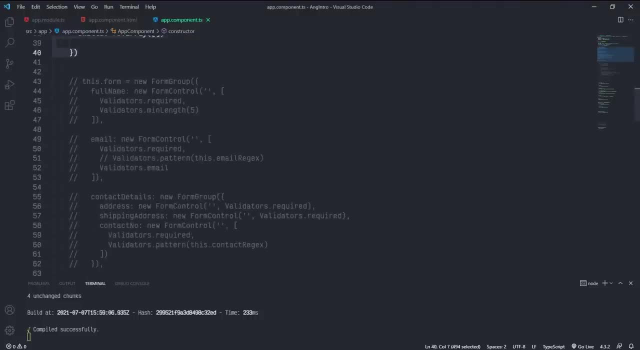 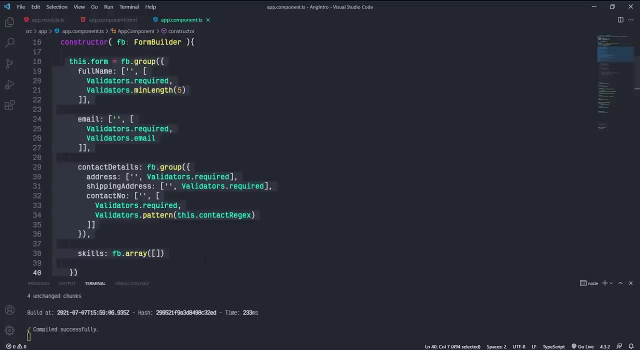 this form, every validation and everything working as previous Perfect right. Comparing to the previous form group, this form builder is slightly cleaner than the previous form group Right. So this is not mandatory to use a mobler. It is up your personal preferences. 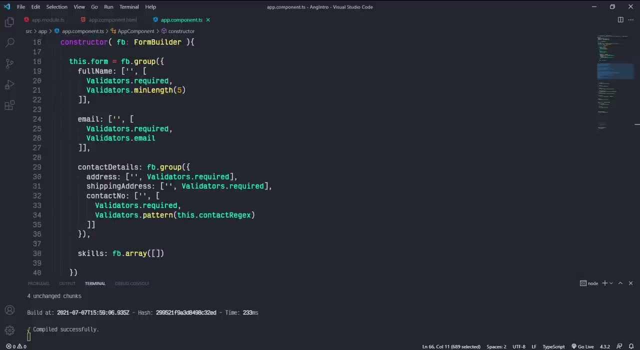 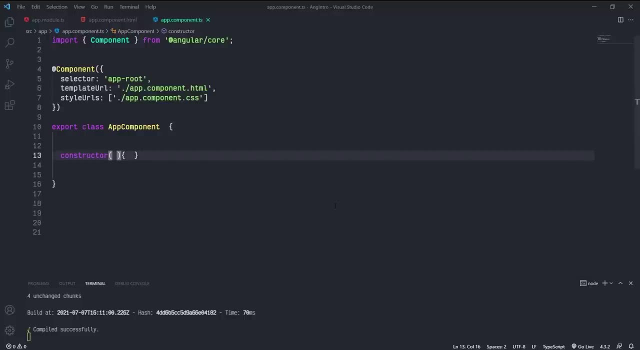 In case, if you like this previous syntax, you can use that, No problem in angular reactive forms. In reactive forms we can write a custom validator method for our own custom validations. As you know, we have few inbuilt form validation methods required: min and max length pattern. 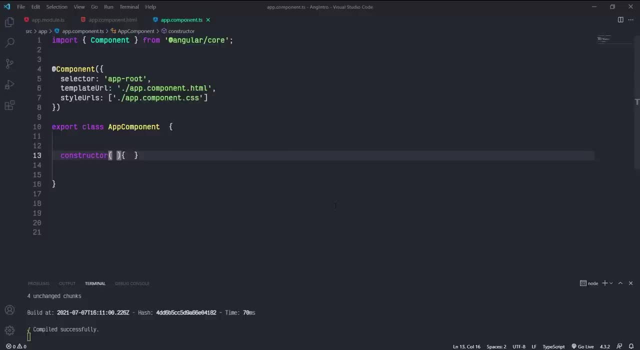 and the email html validations. Think, if we have an input for username and we want to validate the username without spaces, if someone types a username with space we have to show an error. So in this case we don't have any inbuilt validators, So we have to create that validator by ourselves. 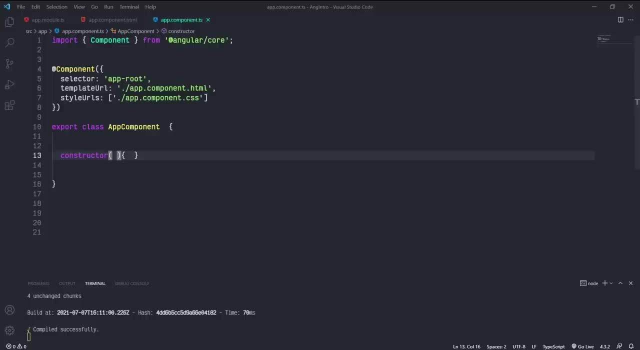 So let's do that. So, guys, now I have an empty app component. I removed all previous codes. Don't worry, if you need the previous codes, I have attached the file with the previous lecture. Alright, let's begin. First, let's create a simple signup form using 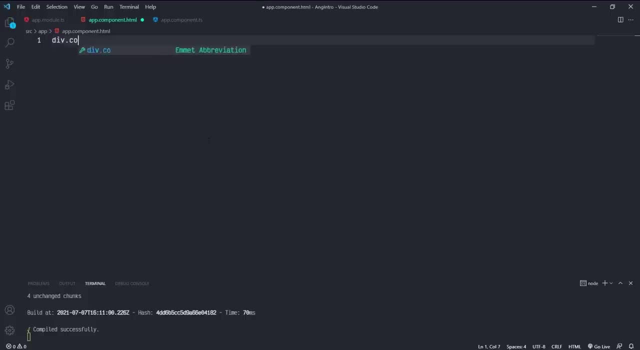 bootstrap. First, create a container div. Insert this div Form tag. Insert this form. Create a form group div. Insert this label username After this input field with form: dash: control bootstrap class. Next, again another form group div. Add this a label with password. 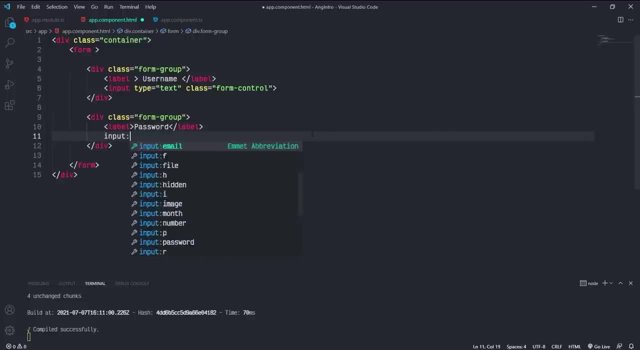 After this: a password input tag with bootstrap form, dash control class. At last, create a submit button for this form with bootstrap classes btn, btn, dash, primary. The button text will be submit. Now convert this simple bootstrap form to an angular reactive form. So go to the componentts file. 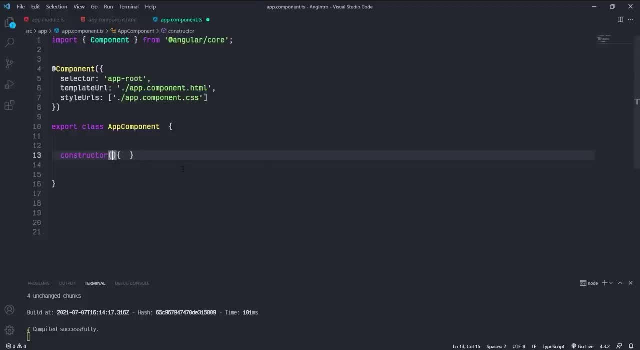 To create angular reactive form controls. I'm gonna use the form builder. So first inject the form builder to this constructor, fb, and the inject type will be form builder. Select this to complete. This will import the form module to this component. Create a form variable inside the class corp. 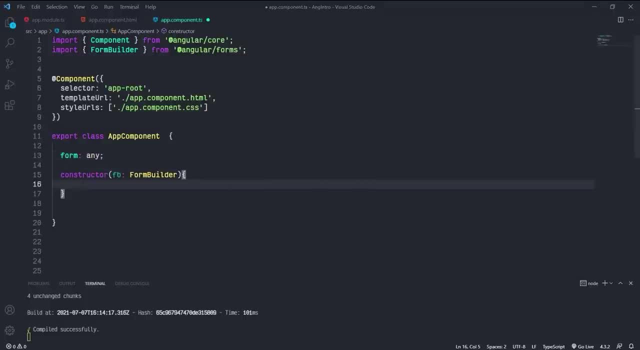 Alright, now inside the constructor, let's create the reactive form controls. This dot form. assign fb, which is this form builder, dot group and parenthesis. Inside this parenthesis, pass a form control object. So create the object as a first key value: pair, username, and this is a form control. 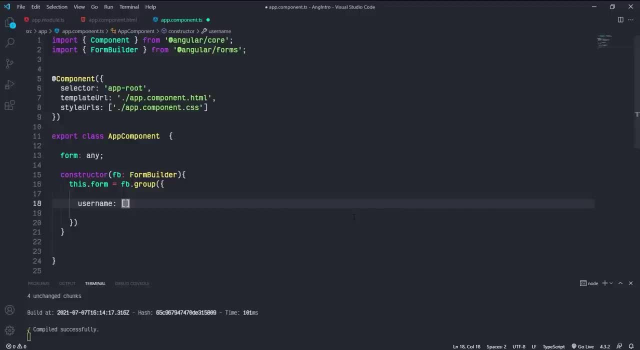 So use the short syntax: just open and close a square bracket. Inside this square bracket, Set the initial value, which is the first key value. Set the initial value, which is the first key value. This is an empty string. So, after this, validators. 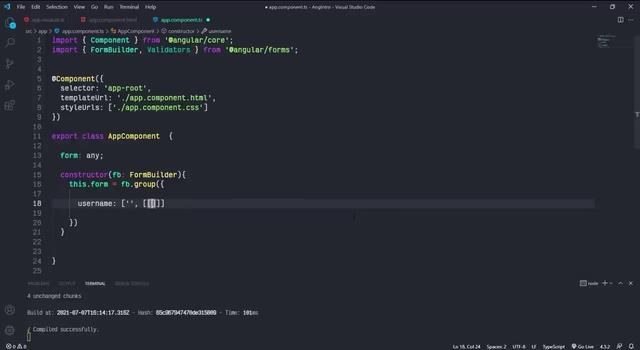 This username as more than one validators, So pass this as an array. The first validator is validators dot required. The second validator is min length And set the length count to around minimum 5.. Alright, next we got the password form control. So the key is password and the form control. 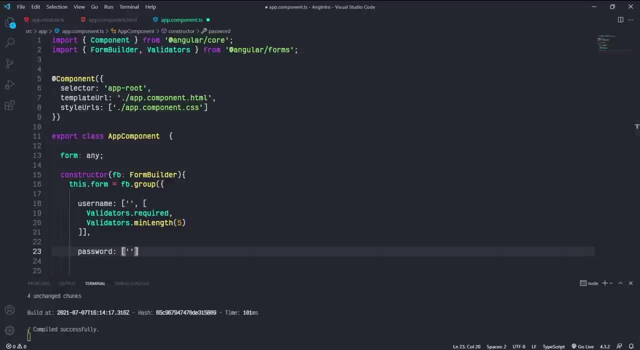 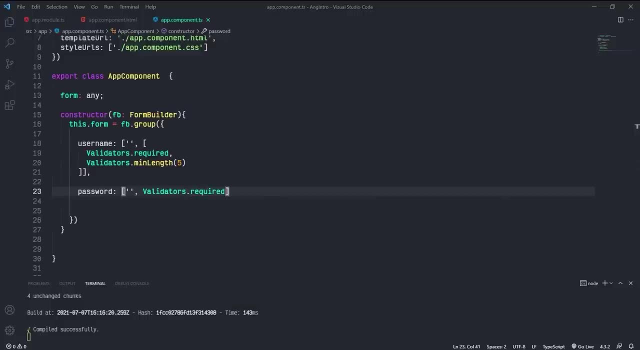 Set the length count to around minimum 5.. Alright, next we got the password form control. Set the default value For this. we gonna add only one validator, which is required. That's it. we have successfully set the form builder. Next let's set the getter method. 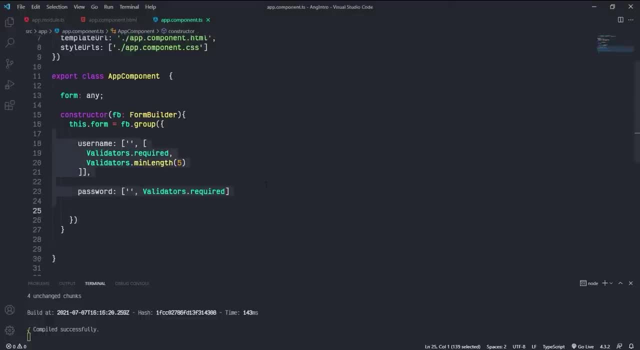 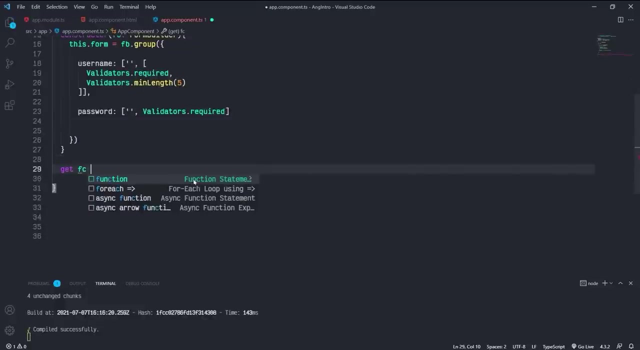 In the form builder we can set only one get method for all these form controls. In previous, we created getter methods one by one for each and every form control, But using the form builder we can simplify this. Get method name is something fc: Set the default value. 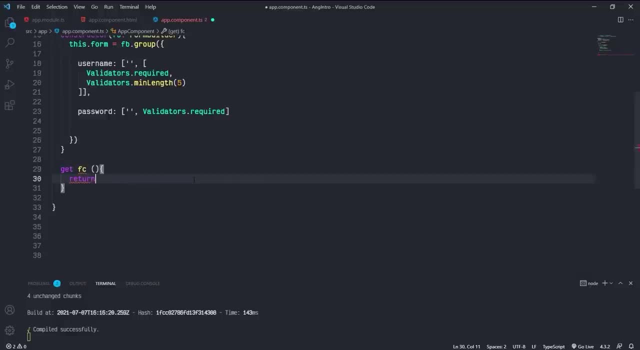 Parenthesis and the method scope Inside this simply return this statement. Return this dot form dot controls. With this we are returning all the form control instances, So we can simply access the form control instance like this: fc dot form control name, username or password. 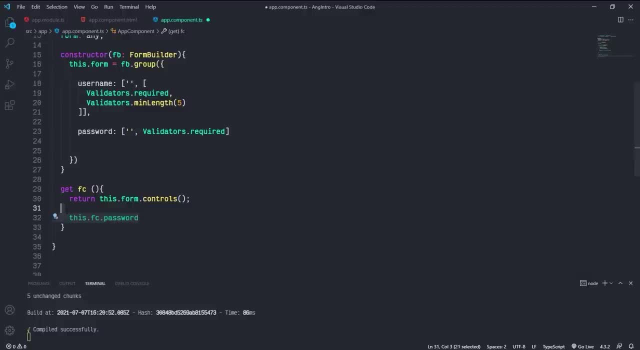 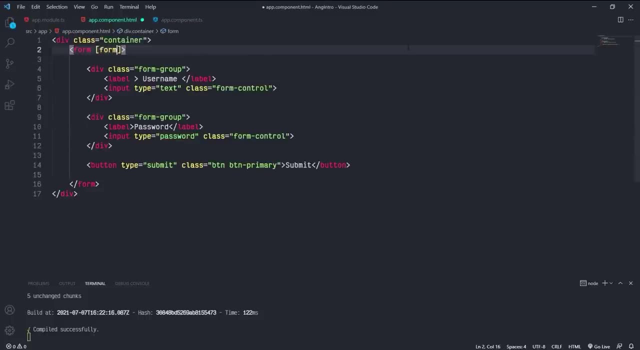 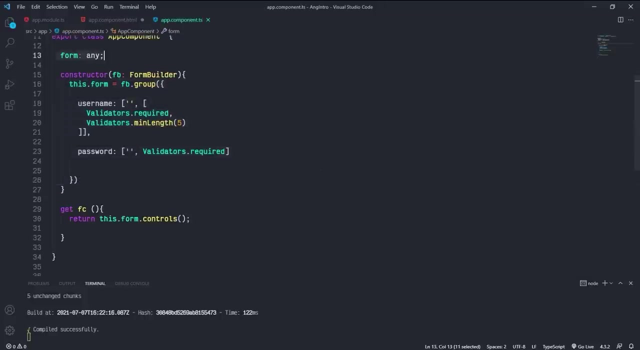 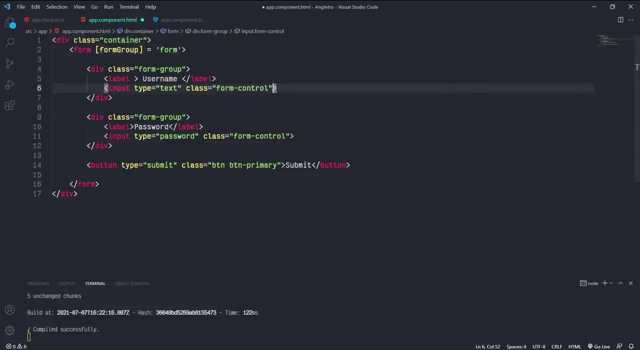 Alright, save this and open the components V file. Connect this form to this form Form group using the form group property binding Inside square brackets: form group and the form group is this form variable, So bind this to this form variable. After this, bind the input field to the form controls. 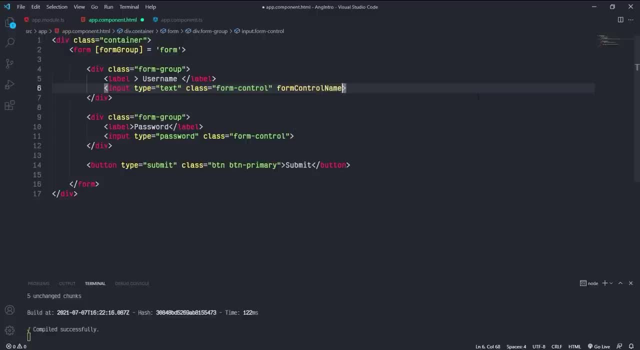 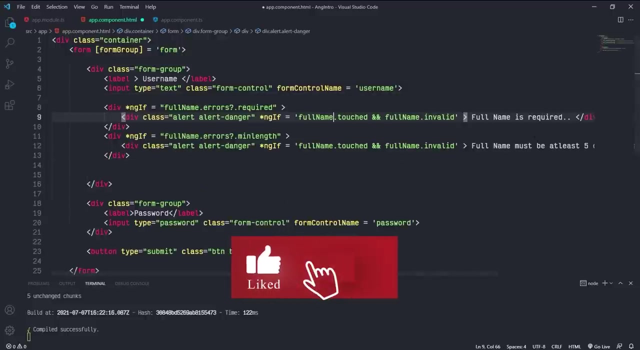 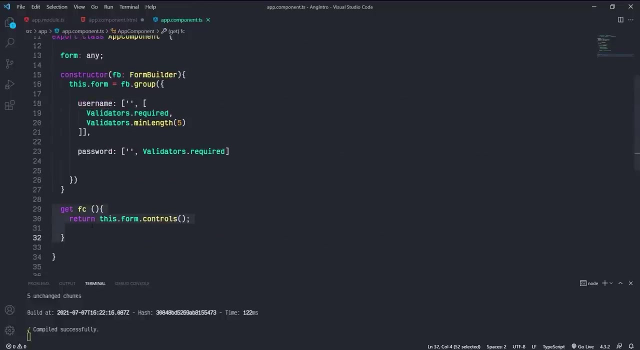 Inside this first input form control name: assign Form control name is username. Set the password field as same that this one and this one, And do the same for this password field as well. Next, add the validation error messages. I just copy and paste this form. the previous form. 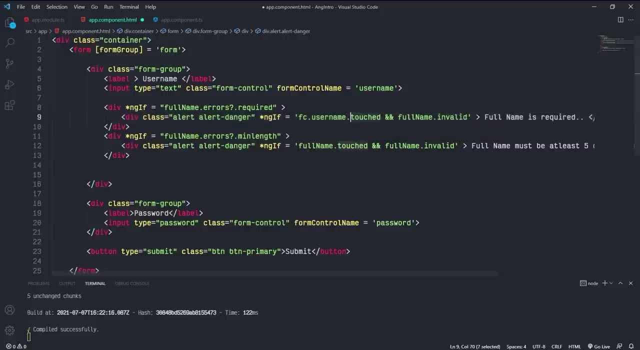 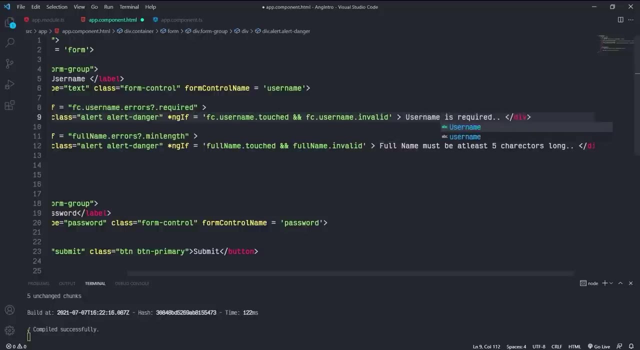 So this time form control is coming from this get method. So fc dot username, usernameinvalid. So same as this fcusernameerrorsrequired. At last, don't forget to change the error message to username required. Do the same for this min length error as well. 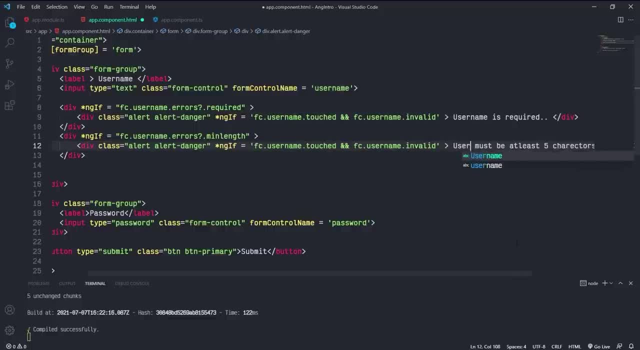 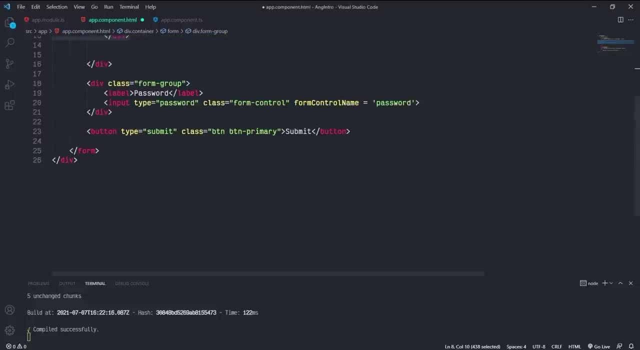 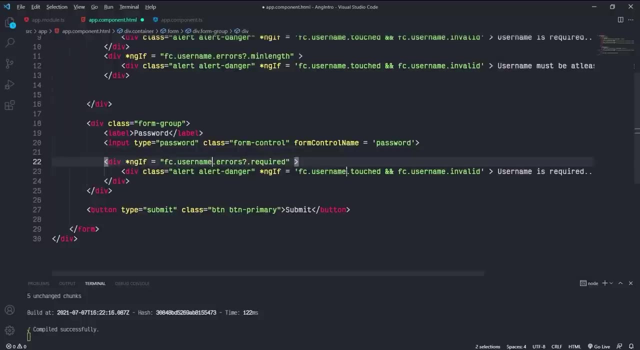 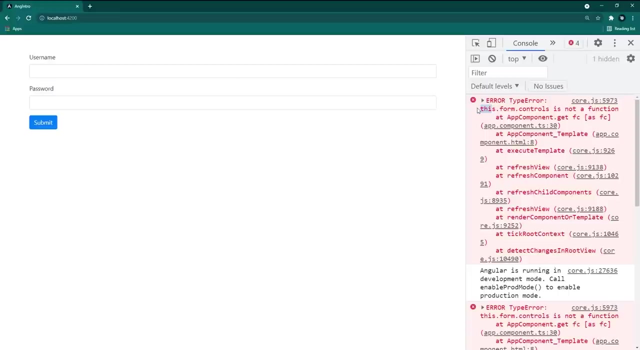 Now again, copy and paste this error to this password field. This password has only one validator which is required, So change all the details. So that's it. Save this and back to the browser. Wait, we are getting an error here saying thisformcontrol is not a function. Oh, I did a mistake here. 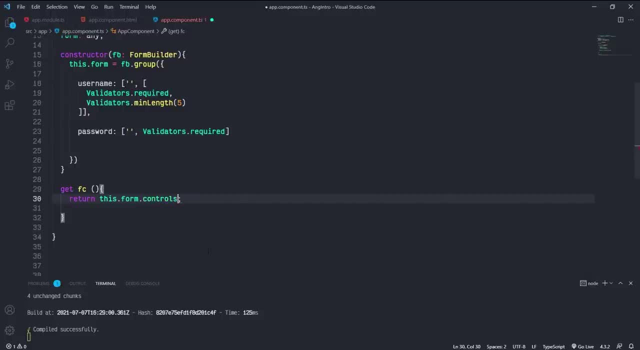 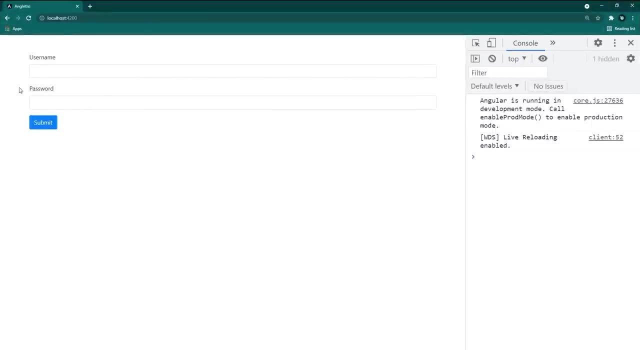 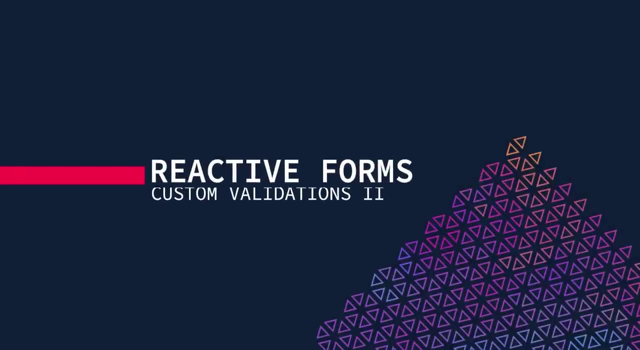 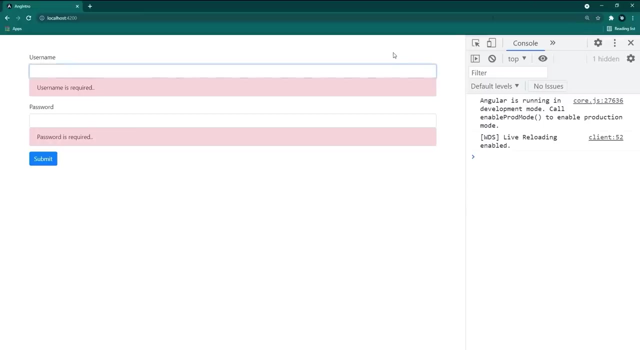 This control is not a function, So remove the parenthesis. That's it. Save this and back to the browser. Now we don't have any errors. Check the validations. Perfect, Everything seems to be working as we expected. Alright, now let's do the custom validator for this username field, Which is username. 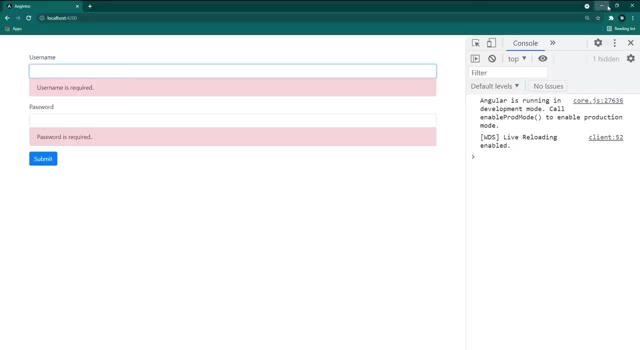 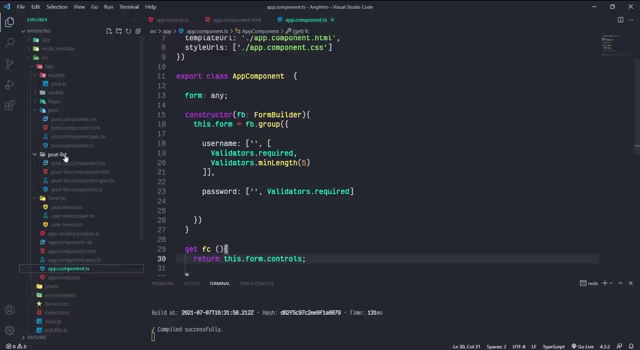 must not contain spaces. First we have to create a file for this custom validator. As a good practice, I will put all my custom validators inside of a folder called validators. So inside the app folder, Create a folder. The folder name will be validators. Inside this folder let's create our custom. 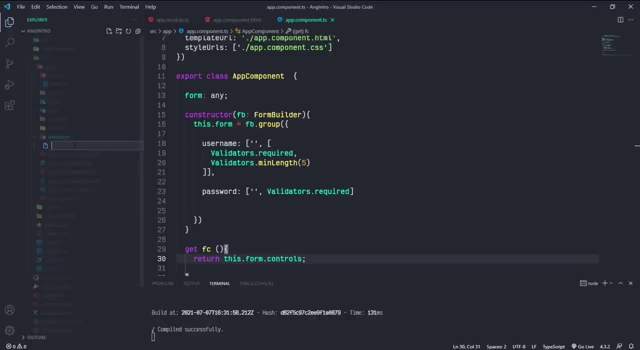 validator. So create a file File name. First pass the validator name, something, No space Dot After this. like this component, file naming convention, Validators. So we are creating a validators file. So validators Dot, Validators. Validators- Validators- Calculate the file. 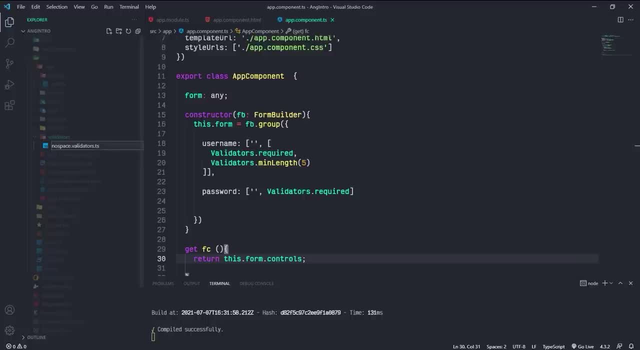 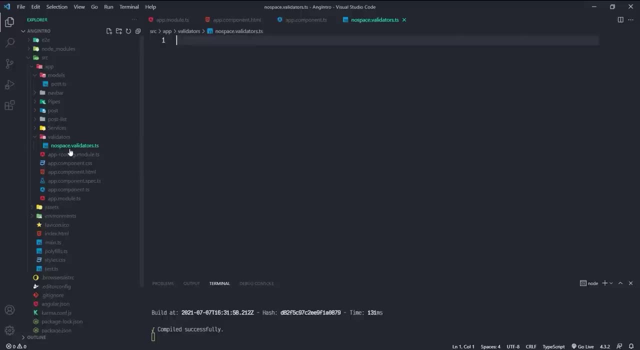 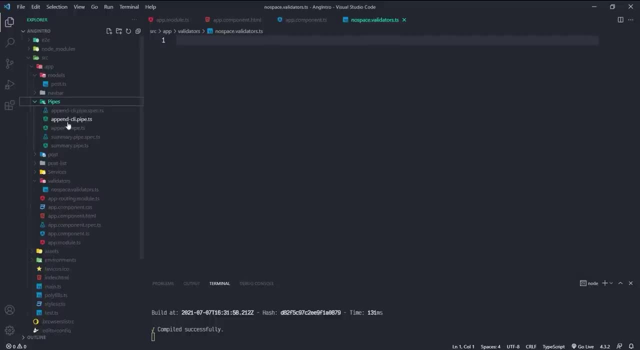 file, we will put the component. If it is a custom pipe file, we will put the pipe. between this. If it is a service file, we will put service here. So nothing fancy, just simple naming convention. Next, open this validator file. Inside this, let's create the custom. 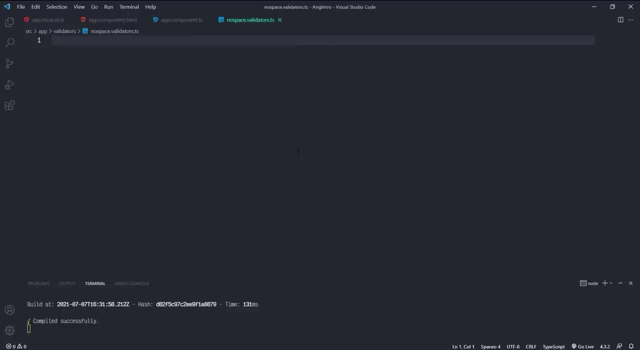 validator. First we need to import two modules. One is abstract control module and another one is validation errors module. Let's import these modules. Import inside curly brackets: abstract control from this is coming from at angular slash forms And this validation errors module also coming with this angular form. So pass this inside. 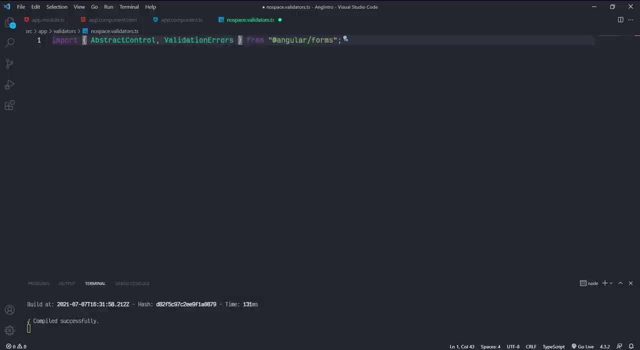 this same import. After this, create the typescript class, class keyword and the class name: no space validators Carefully follow this naming convention. Okay, now we have to define the validators method, So this method name can be any name. So I declared this method name as something: no space validation and parenthesis In order. 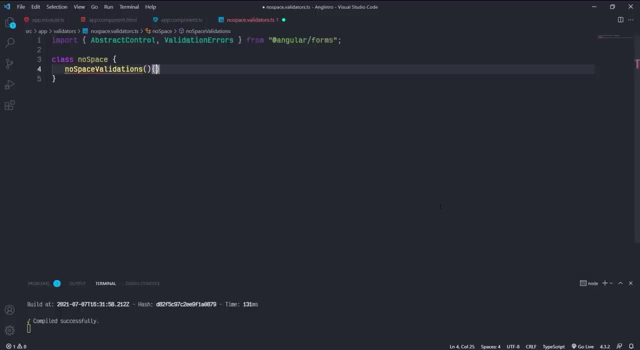 to make this a validator method, we have to do two things. First, set a parameter for this control, and this control must be an abstract control. After this, if there is an error, this must be returned. validation errors Or if there is no error, this must be returned. 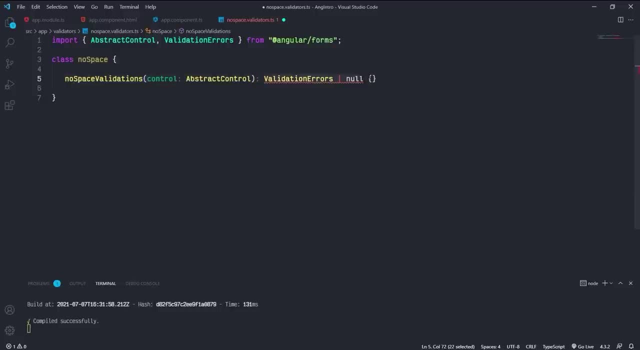 null. So add that after this method: scope. Okay, let's set the logic inside this method, Alright, first I am gonna capture the value. with this parameter, We are getting the form control. As you know, this form control object contains all the form validation status, such: 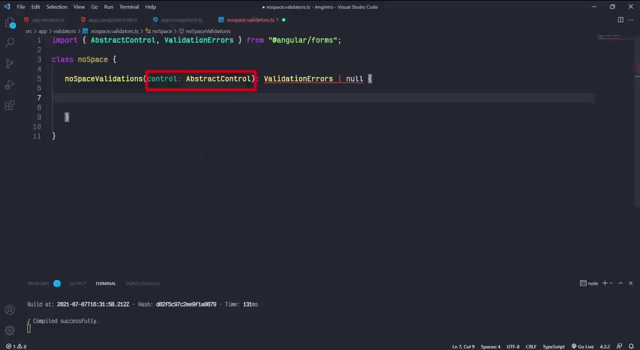 as touched, invalid, valid- You got the idea right. And also, this form control object carries the form inputs value. So now what I want to do is I want to get the form inputs value and assign it to a variable called control value. So let's do that, Let control. 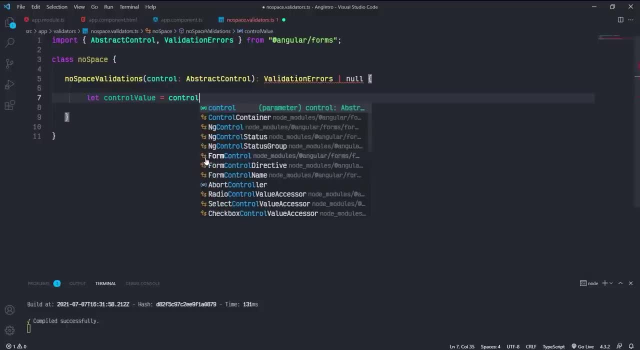 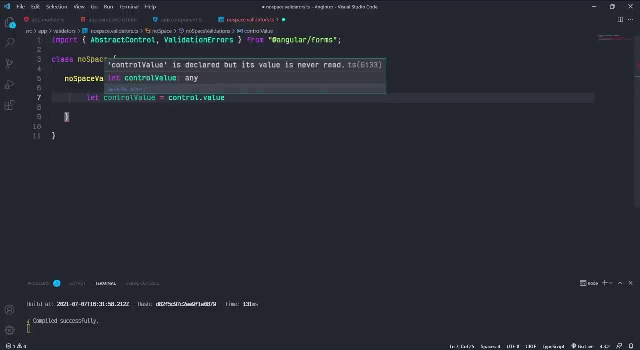 value, assign this control, this parameter control, dot value. So this control value type is any. I want to make this as a string, Then only we can check whether there are any spaces or not. So as string. So add this after this as string. Very simple, right? Alright, now we have the value, Let's do the logic. If 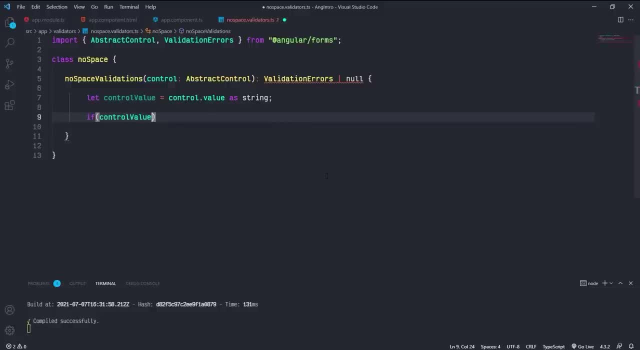 the statement is control value, which is this form control value, and then index of white spaces greater than or equals to zero. So with this index of method we can get any characters count If you want to check whether there is any special characters, something semicolon type or not. So we can pass that. 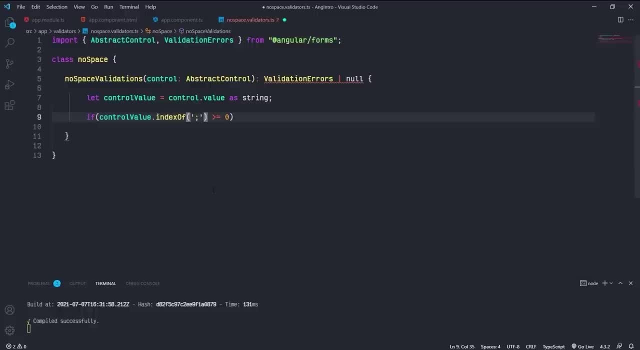 inside this index of parameter. In our case, we are checking whether there are empty white spaces or not. That's why I passed the empty white space as a parameter for this index of method. Alright, if there is space in the user name, we can return this as an object. So return no space validator as the key, As a value. 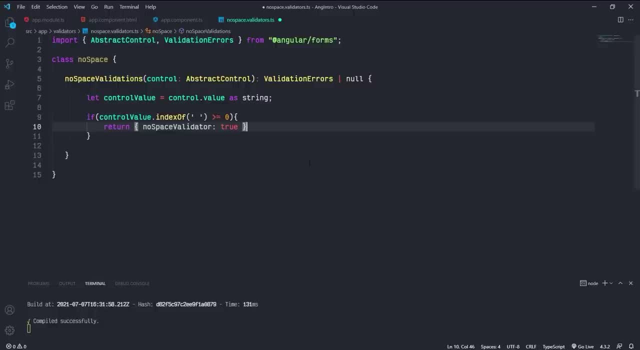 if you want, you can send an object with additional pieces of information. In our case, we don't need that, So just simply return true. Coz there is only one error: If this is not true, return null. So when we dealing with validators, we are not creating a new instance. So in order to 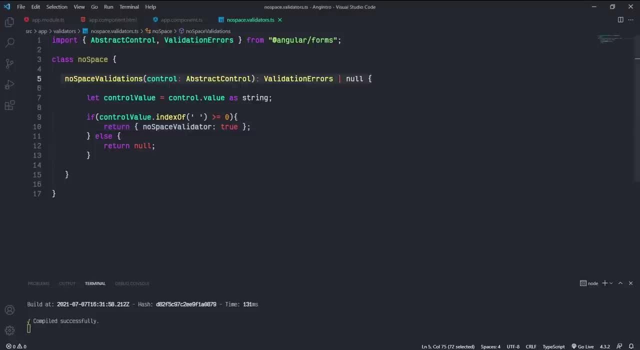 make this method accessible without making the new class instance. Just set this method as a static method, So we can access this validator method without making a new instance of this validator class. At last, don't forget to add the export keyword to this class Then. 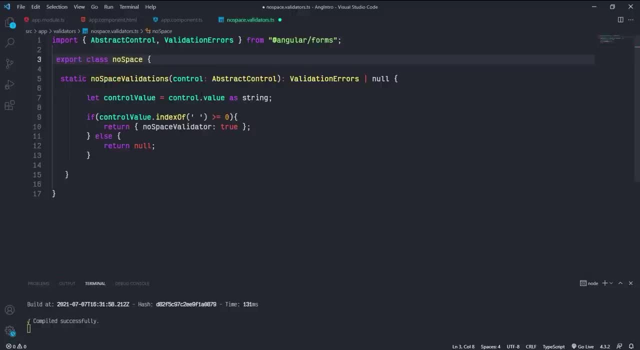 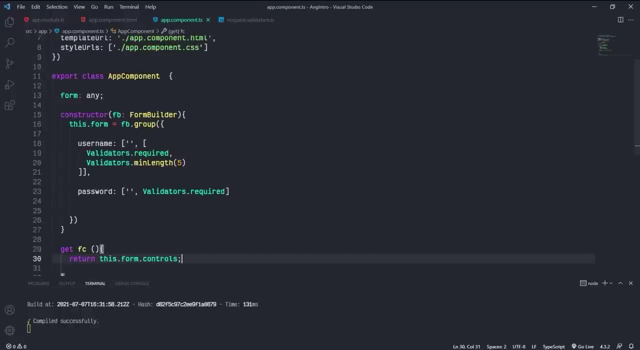 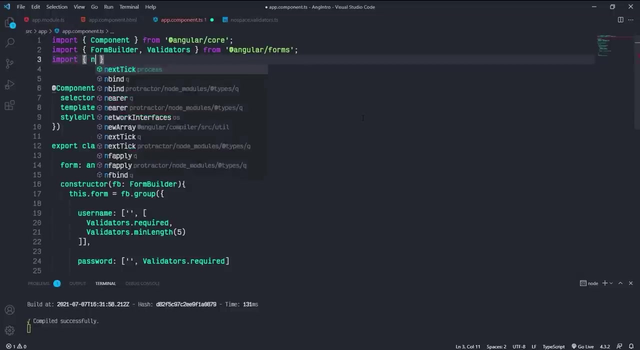 only we can access this class from outside. Alright, now we have successfully created our custom validator. Now let's see how to use this validator. In order to use this inside the component file, Import this custom validator. So import inside brackets the class name is no space validators. After this path from: 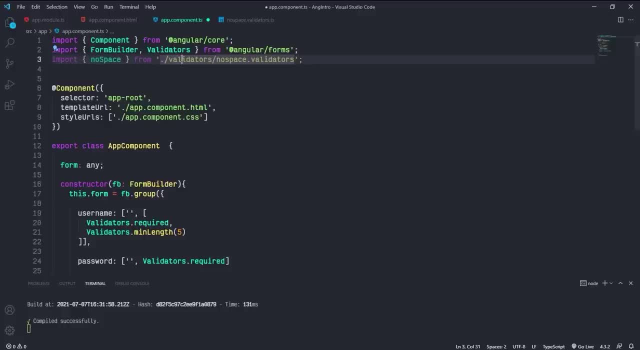 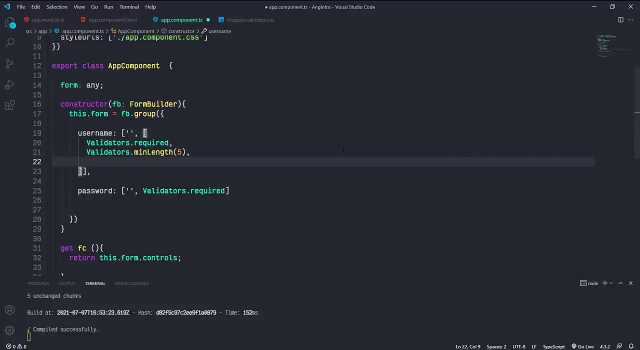 path is to this validators file. Go back one step Inside this. select the validators folder. Now, inside this, select this no space validators file. That's it Now. add this validation to this user name input. After this: This time, the custom validator module is this: no space. 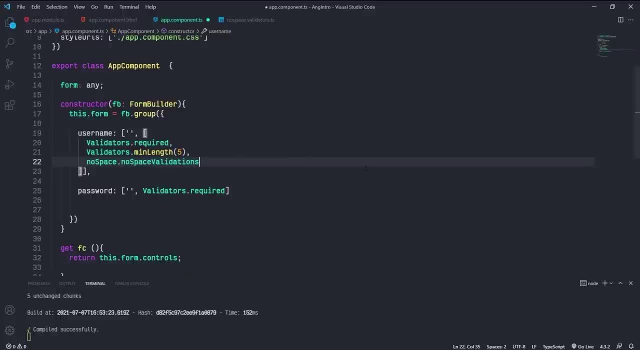 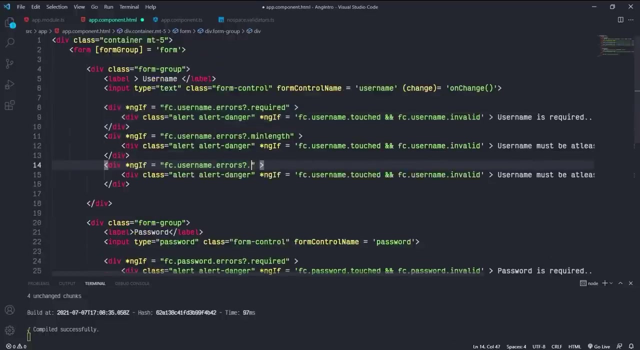 validators And the validator method is this: no space. So select it. That's it. Now go to the HTML file and add the error message for this custom validator. Duplicate this previous error message. Change the error to no space. Change the error message to user name cannot. 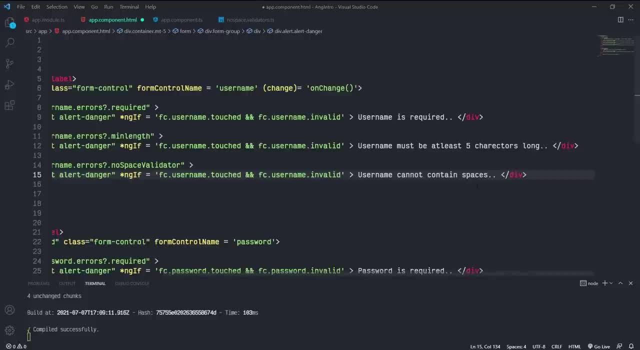 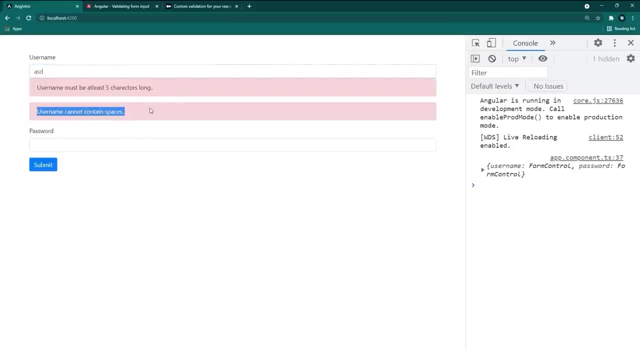 contain spaces. Save this all and go to the browser. Inside the user name, type a something and hit the space bar. Beautiful, right, We got this. no space error. Now remove this space space. Perfect, Now we are not getting any errors. Perfect. So, guys, this is how we create. 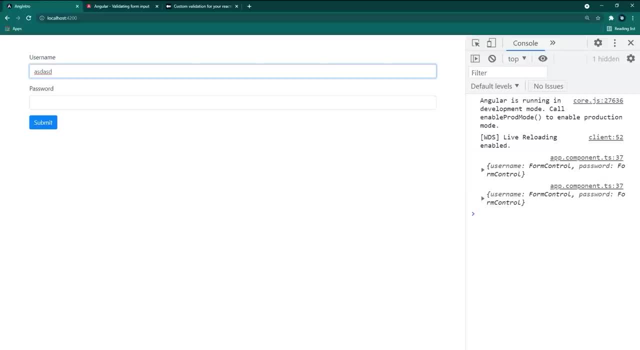 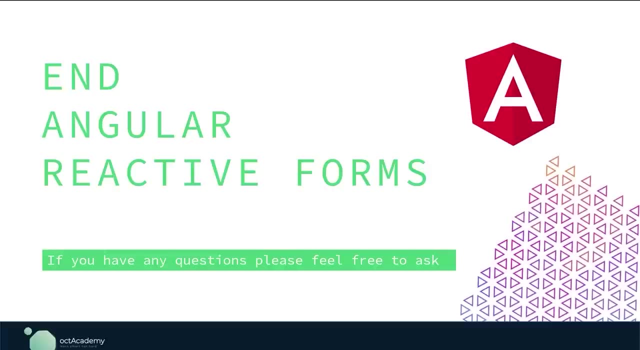 custom input validations in angular. So, guys, this is it for this section. This section is filled with lots of logics, right? Hope you guys learn it well and enjoyed it. In this section we learned what is reactive forms and how to set up a reactive form from scratch. 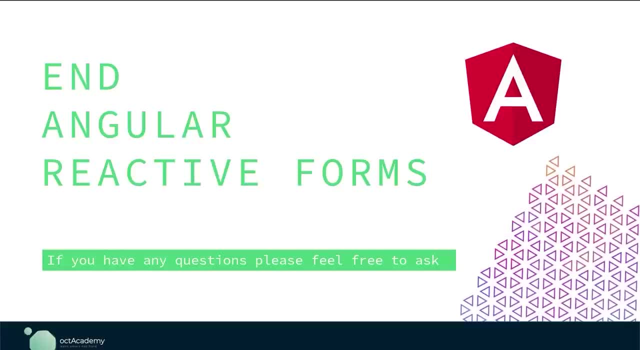 We learned about how to set up a reactive form from scratch. We learned about how to set up a reactive form from scratch. We learned about reactive form validations, and also we learned how to create our own custom reactive form validators from scratch. So after that, 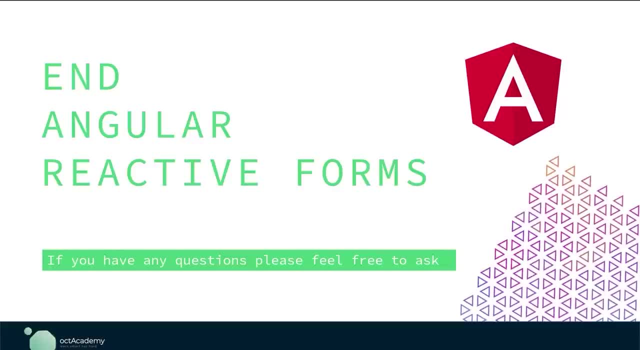 we learned about reactive form builders, form arrays, nested form groups and so on. Perfect. So, guys, we successfully completed this reactive form section. Hope you guys learned it well. If you have any questions, feel free to ask in the Q&A area. 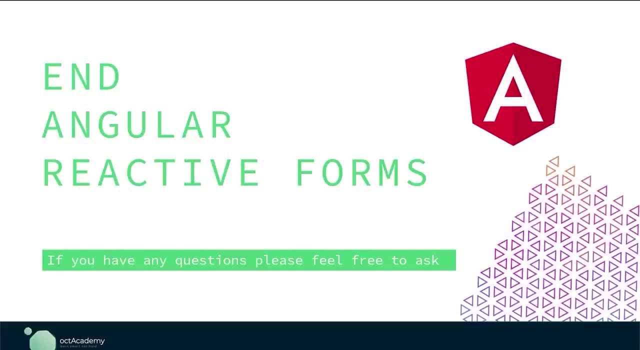 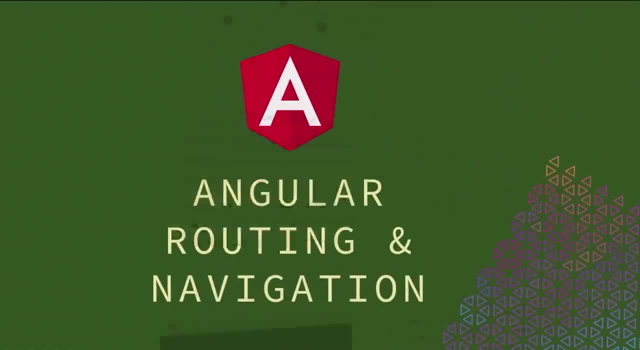 This is the end of this section. Let's move on to the next section, Alright? in this section, we are gonna be learn about angular routing and navigation. By the end of this section, you will know what are routing and navigation, How to implement an angular. 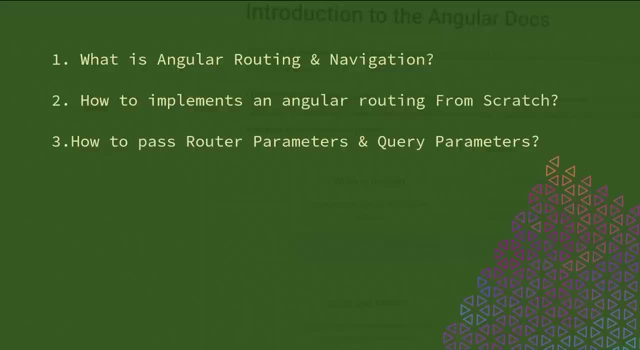 routing from scratch, How to pass router parameters and query parameters, What is observable and how to use that, How to get router parameters and query parameters And, at last you will learn a lot from this section- how to navigate routers programmatically. so this section gonna be a little big and 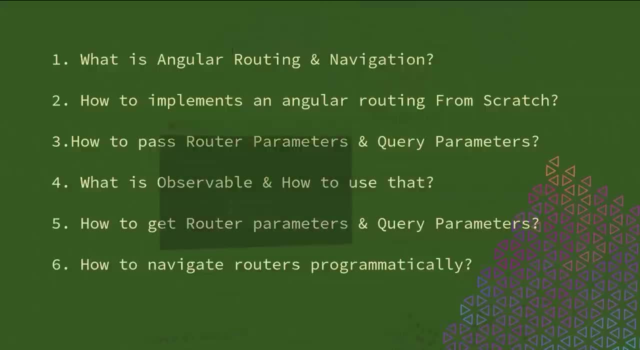 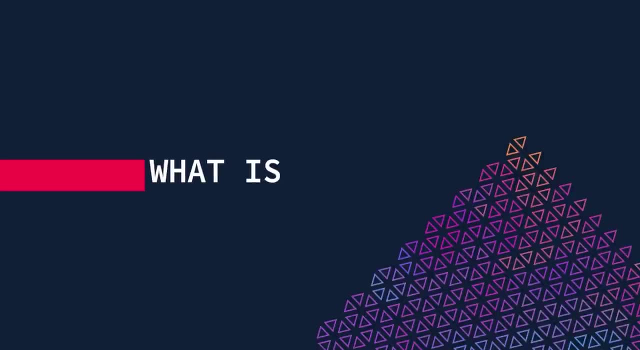 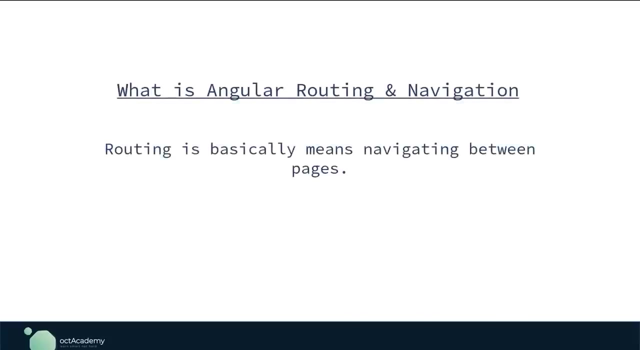 tricky, so please make sure to learn everything. so what are we waiting for? let's get started. so actually, what is this routing? routing is basically means navigating between pages. you have seen many sites with links that direct you to a new page. let's get an example just. 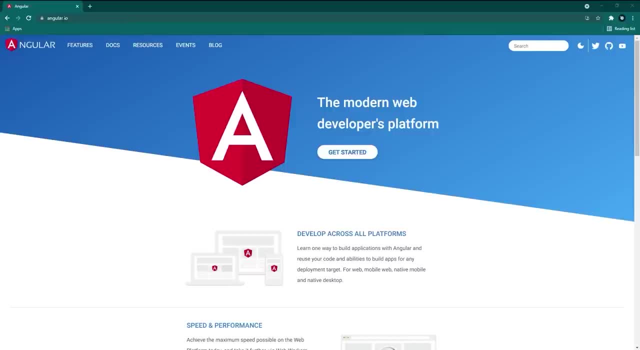 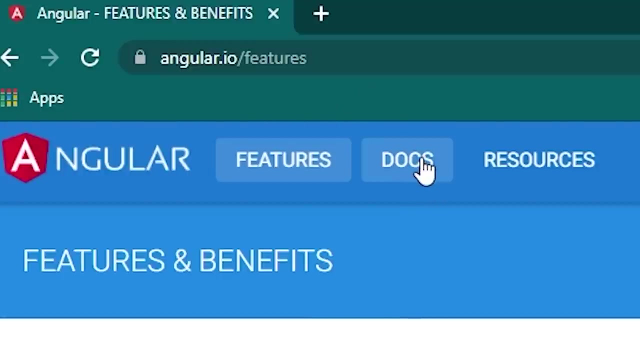 go to the angular official website, angulario. so this is the home page of this website. if you go to this features tab, this URL is changed to this. after this domain, we can see this slash features. if I go to the docs, this change the URL to Docs. so this is what routing this is. 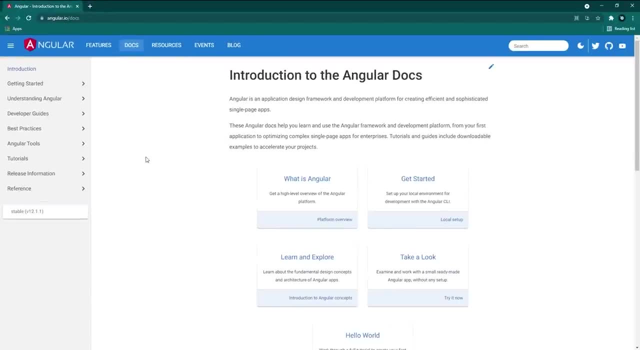 This routing is commonly used in all websites and web apps to navigate through the website pages. You guys already know angular is a component based frontend framework, So in angular we use the routing mechanism to navigate around components. So think this angular's official website is a build using the angular framework. 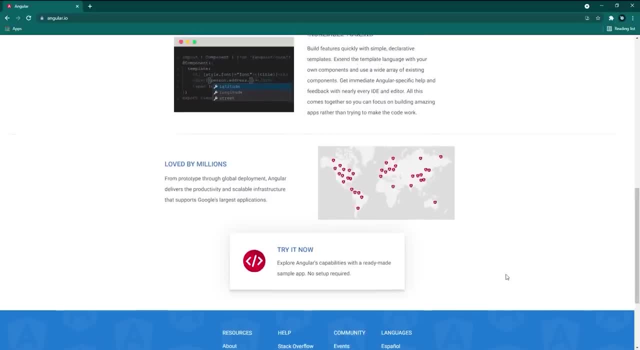 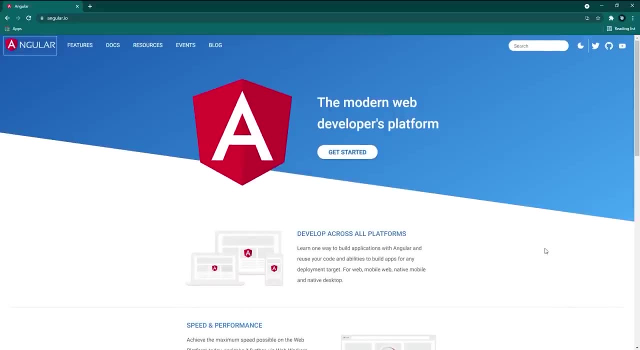 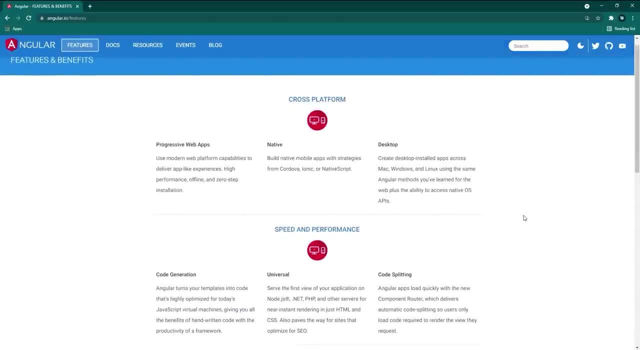 So, when we go to this angulario website, this is the main default router, which is this first page of this website, This showing us this homepage component. So, likewise, if I go to the features tab, this removes the homepage component from the DOM and show this features component inside the browser view. 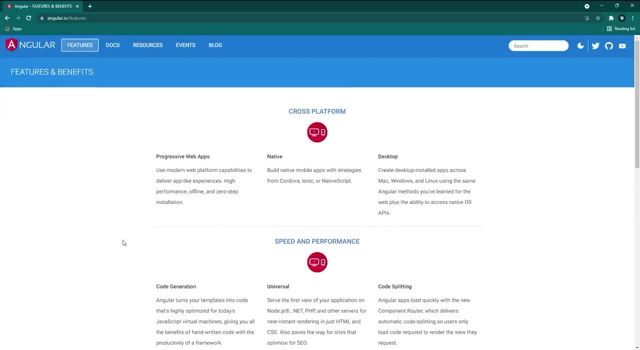 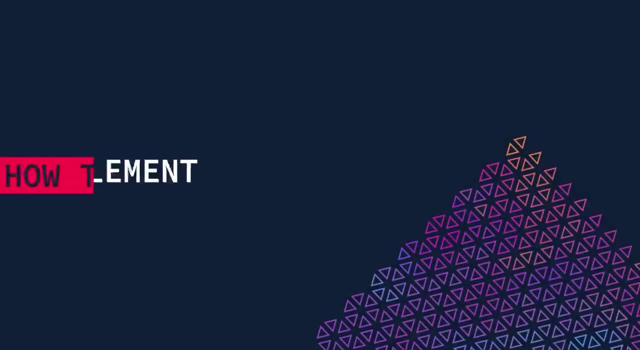 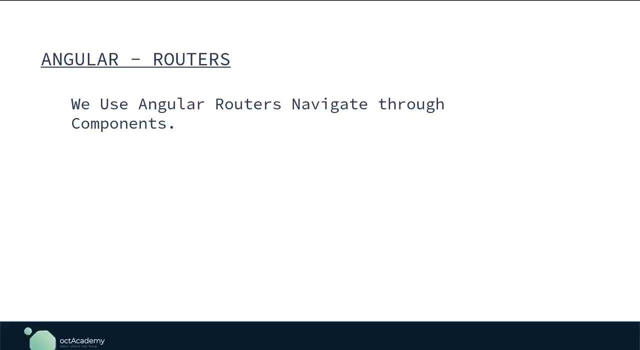 So this is the simple idea that I can give for angular routing. So, once again, using the angular router mechanism, we can navigate through different angular components or different views. We use an angular router to navigate through components, So router is a main built-in core module of an angular which includes a bunch of directives. 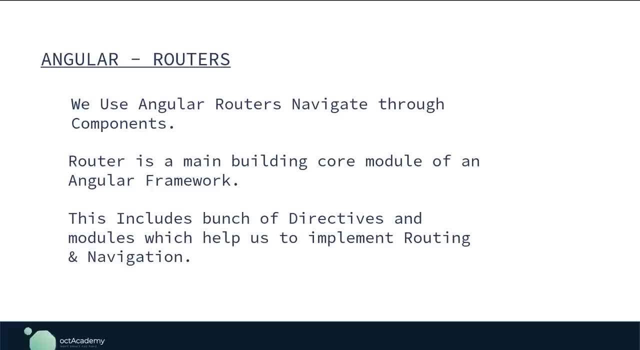 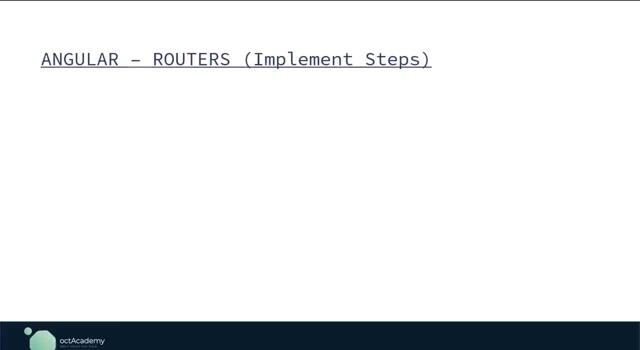 and services that used to implement navigation in our angular app. So throughout this section we will learn about this router module in detail. So there are three steps to implement navigation. First, we have to configure the routes With this. we have to configure the routes. 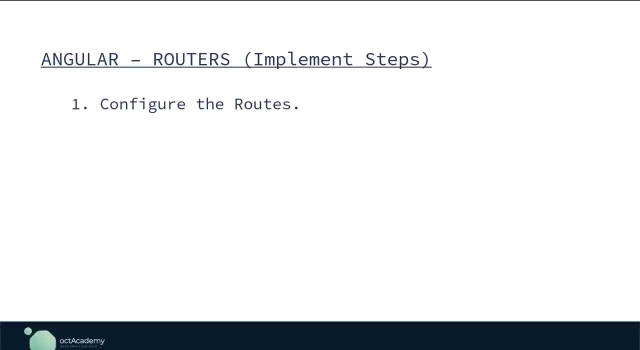 Next we configure which component should visible when user navigate to a certain URL. Next we have to add the router outlet. This will be responsible for showing the correct component view to the user on a certain URL. At last we need to add links to navigate through the website. 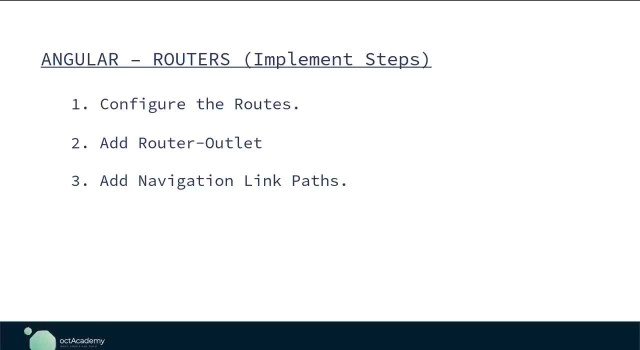 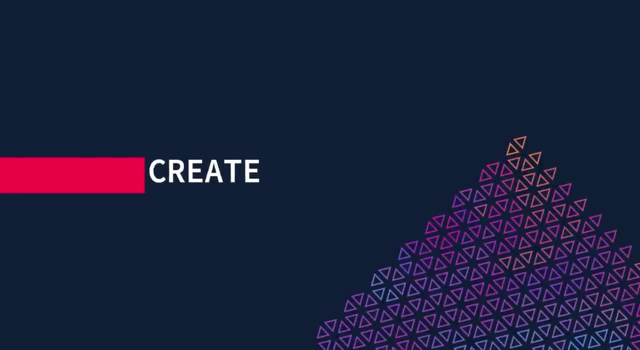 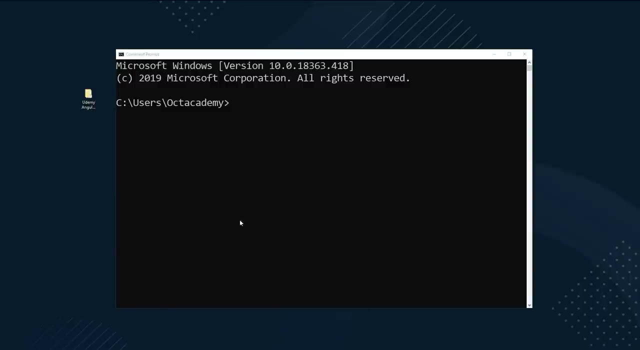 So in the next lecture we gonna learn these three steps one by one in detail. Alright, in this lecture let's setup a new angular project for this routing and navigation. So open the command prompt of the terminal, Navigate to the project folder. As usual, my project folder is inside the desktop. 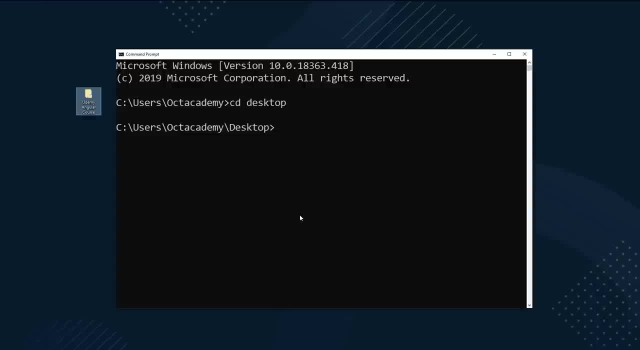 So cd desktop. Inside the desktop, my project folder is the udemy angular course folder, So I'm gonna navigate my command prompt to this folder, cd folder- cd folder- udemy angular course. Perfect, Now I'm inside my project, So let's create the new angular app inside this project folder. 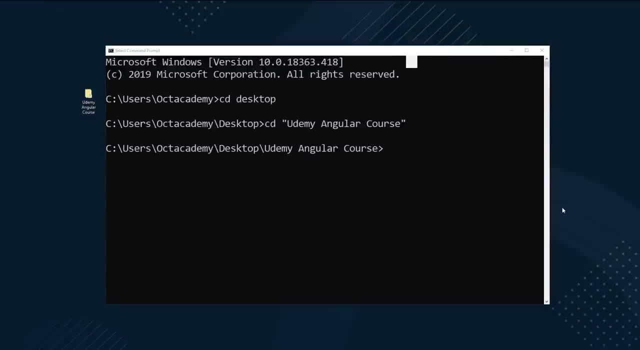 So we learned about this. So, in order to access the angular CLI, we use this ng command To create a new angular app, Niv. Then the project name Something ang-routing. This can be any name, No need to follow exactly as mine. 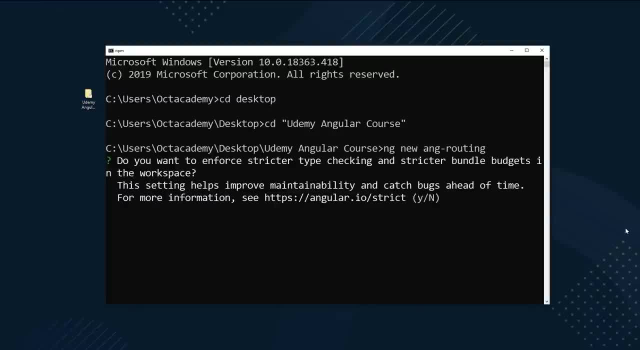 So now hit the enter to run this command. Give no to this strict typing mode And hit enter. Yes, of course we gonna use the angular router, But if we give yes to this, This will automatically setup all the necessary configuration for us. 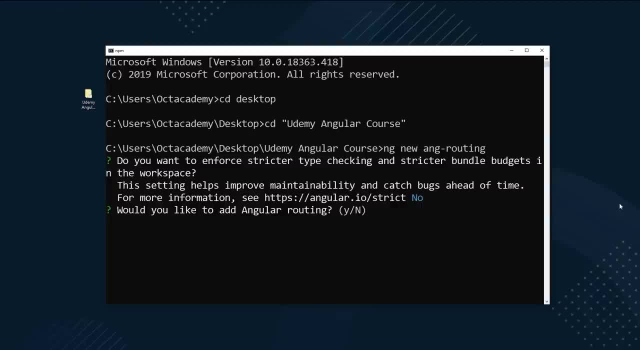 But we'll first see how to do this from scratch. Then only we can get the exact idea about this angular routing. Once we learn about this from scratch, Then we know the idea. So after that we can use this easiest way. So give no to this and hit enter. 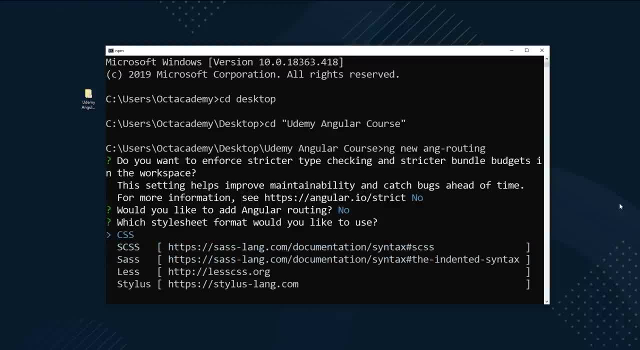 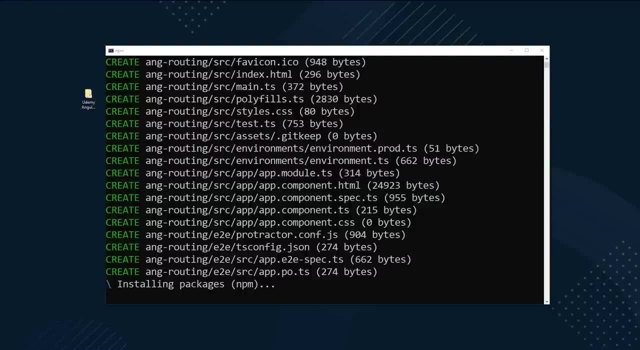 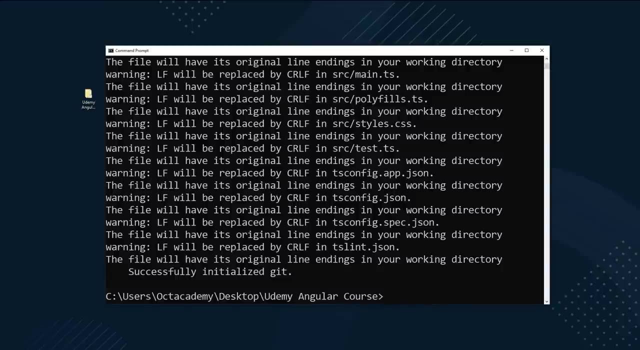 Now select the preferred styling method, Select the css method And hit enter. That's it Alright. The new angular app is ready. Now open this inside the vs code. So cd into the new angular app. Cd project folder name is this: ang-routing. 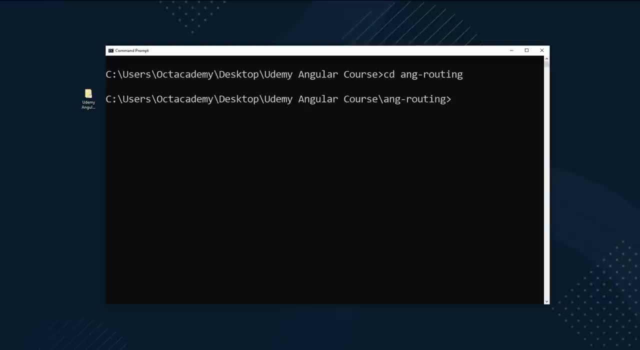 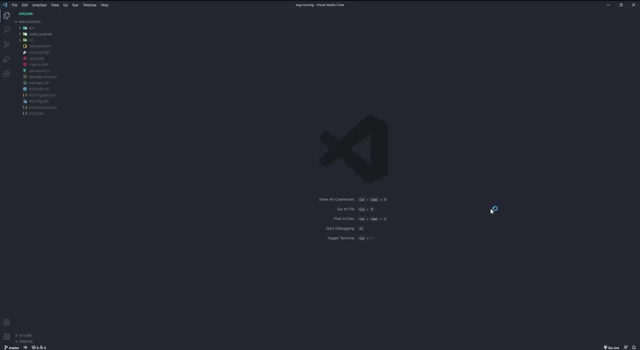 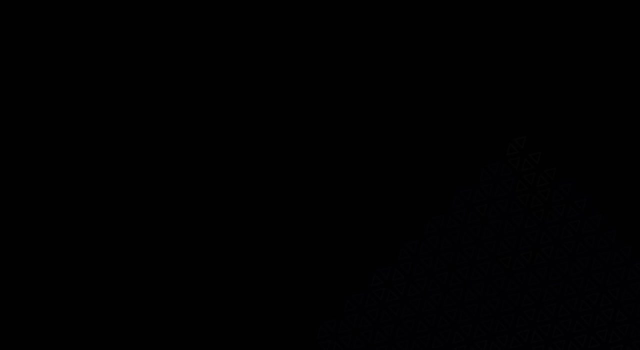 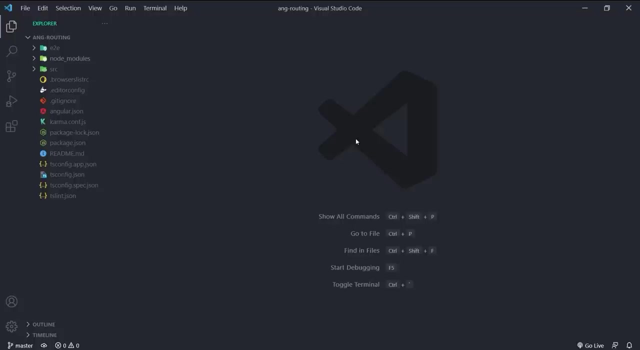 Now run this command to open this inside the vs code. Now run this command to open this inside the vs code: Code Base And dot Hit enter. In angular we got inbuilt a separate module for routing and navigation. We don't need to additionally install anything. 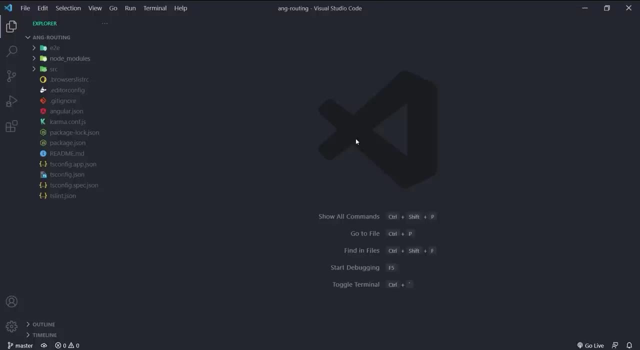 In this lecture let's see how to implement on this router and navigation to this angular, angular project. so first thing. first, let's create a simple app to manage post that has routing and navigations. for now, let's create a component for post list inside the integrated terminal. 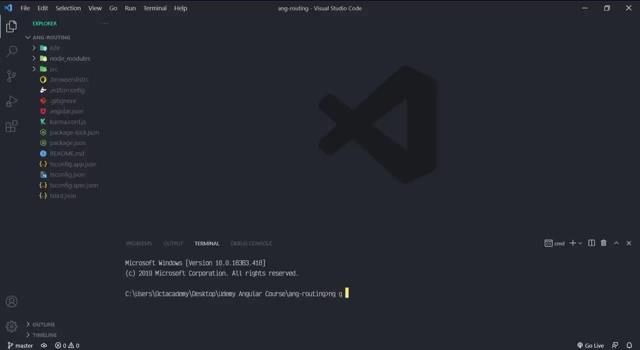 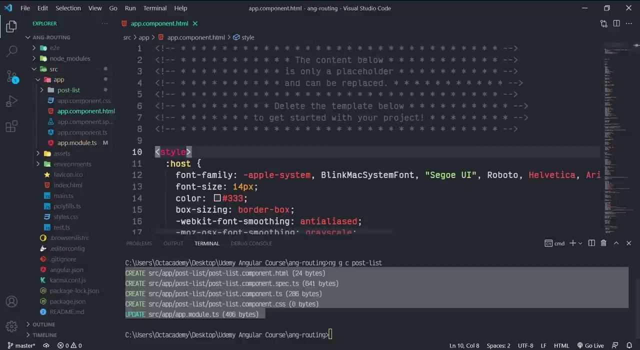 run this command: ng, g, c and the component name is post dash list. hit enter to execute this command. perfect, we got the component. in order to show this post list component inside the browser, we have to add this component selector inside the app component html file. we learned about this. 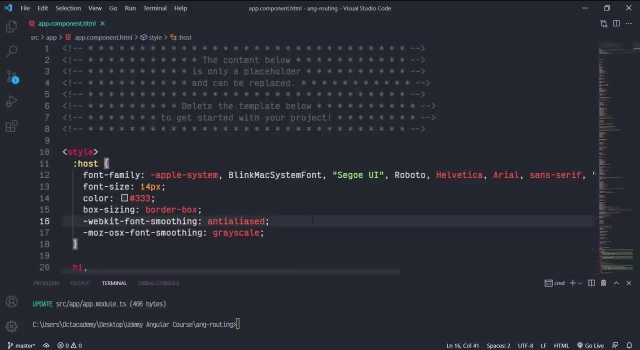 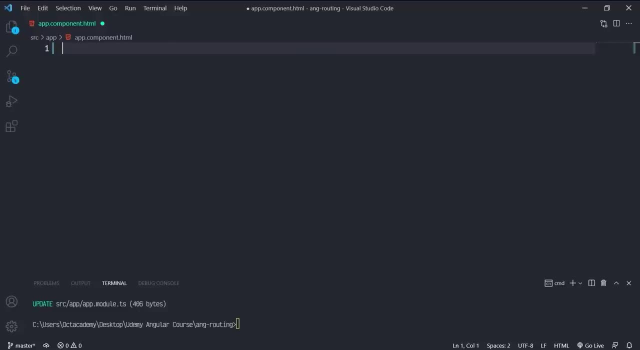 right, so let's add this inside the app component html file. remove this default html boilerplate. we don't need that now. add an h1 tag, something angular: blog site. after this h1 tag, Let's add the post list component selector, which is this app-post-list. So select the 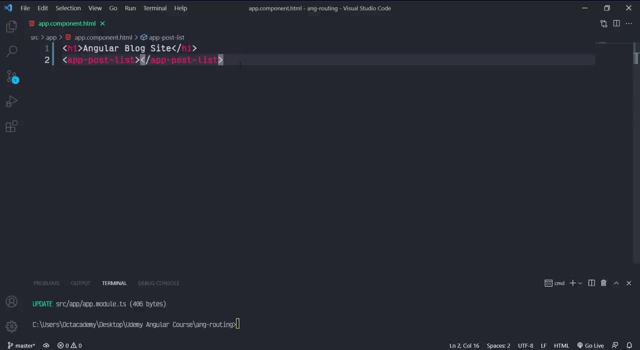 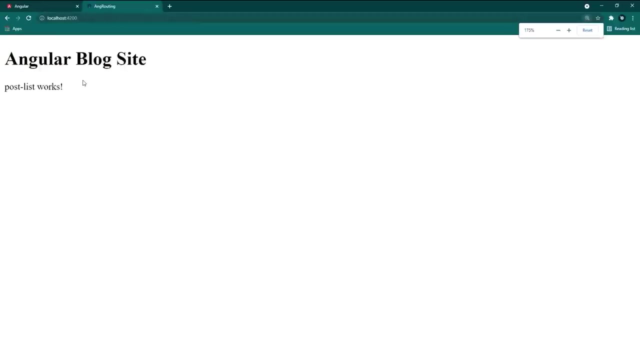 auto complete. This will complete this as an HTML custom tag. Perfect, Now let's run this app Inside the integrated terminal ng serve and hit enter. After the development server started, go to this url: localhost, colon 4200.. Perfect, We got this heading and this: 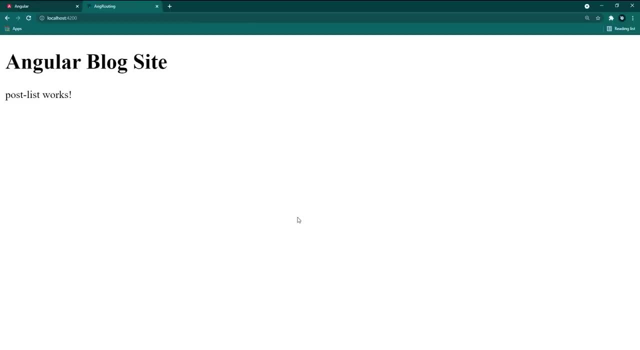 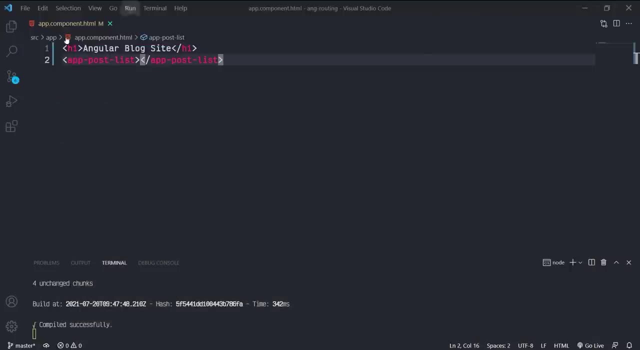 post list work text, which means our post list component is successfully rendered inside the browser. So, if you notice, we rendered this post list component directly inside the app-component HTML file. Now what I want to do is I want to show this component inside the browser. when a button 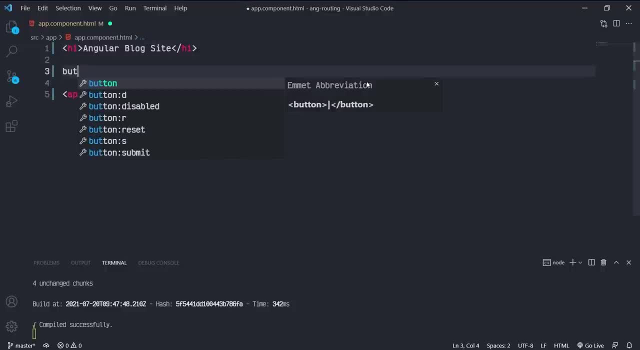 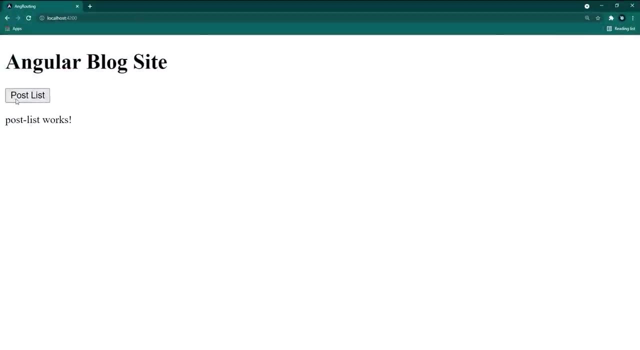 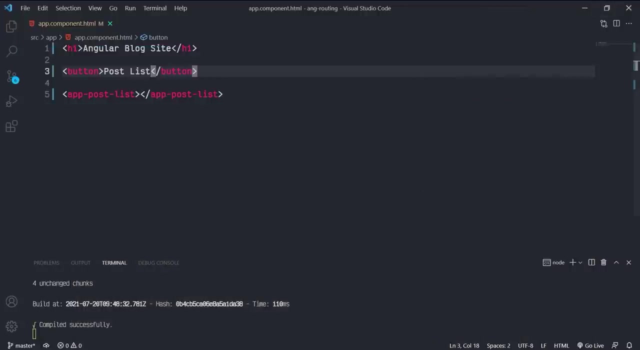 clicks. So create a button before this post list selector. The button text will be post list. Save this and back to the browser. Perfect. So, as I mentioned earlier, I want to show this post component when this button clicks. So let's see this in action. For this we're going to use the 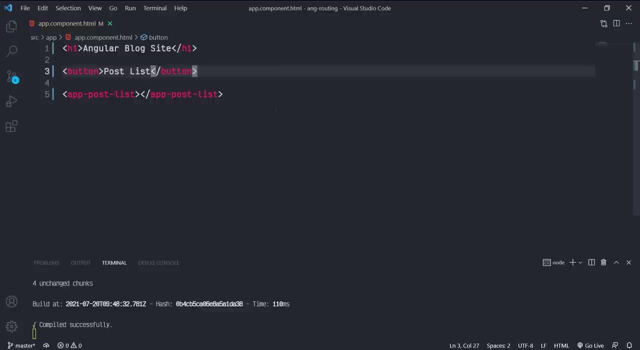 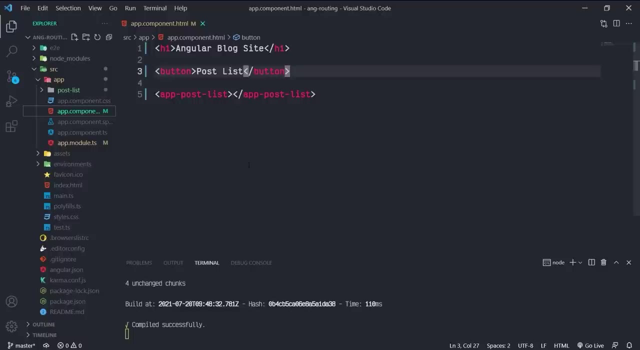 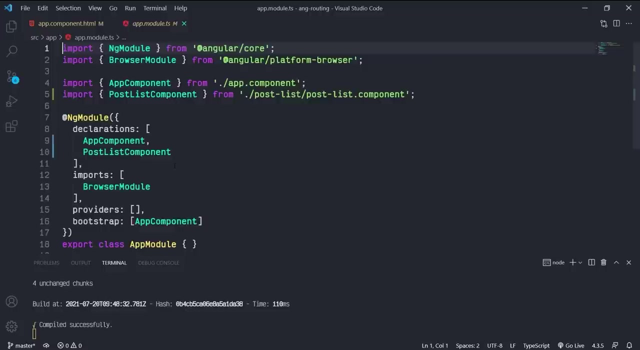 angular routing method. So in order to work with angular router, we have to tell angular to register angular router module inside the angular app modules- Very simple. This is also like previous components- pipes, service and module register. So open the app modulets. 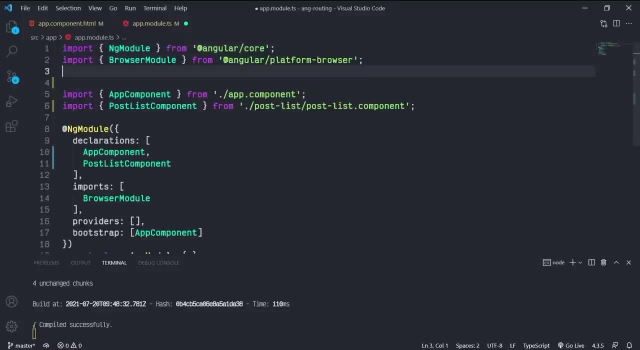 file Inside this. first import the router module. So at the top of the page. after this imports, import, the module name is router module. Carefully follow these capital simple letters After this from this module is coming from the router, So at angular slash router. That's it Now. 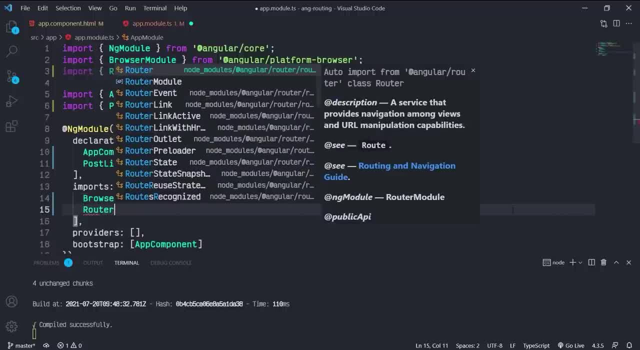 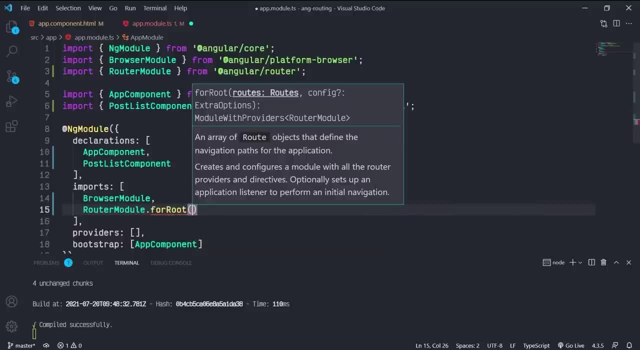 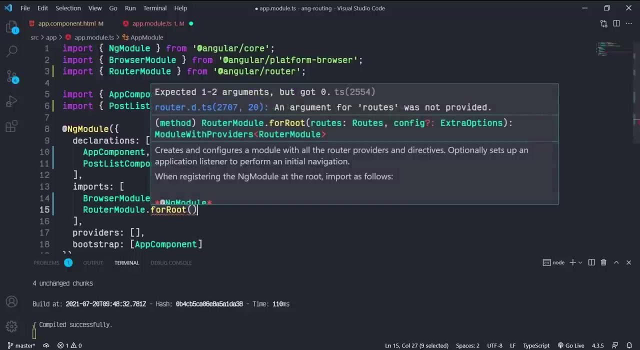 as usual, we register the modules inside the imports array. So after this comma, router module, dot for root and parenthesis: This for root is a static method that defines the router module class. So we use this method to define root or main routes for our angular application. So now we can pass the array of. 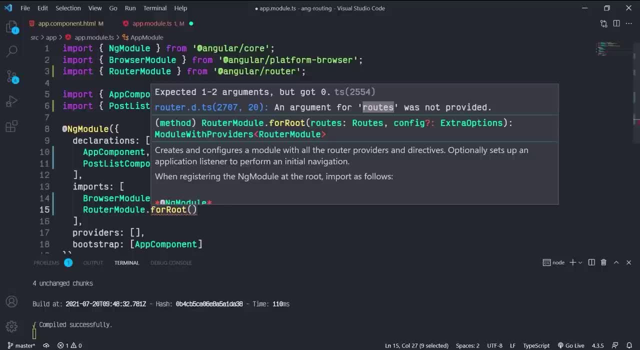 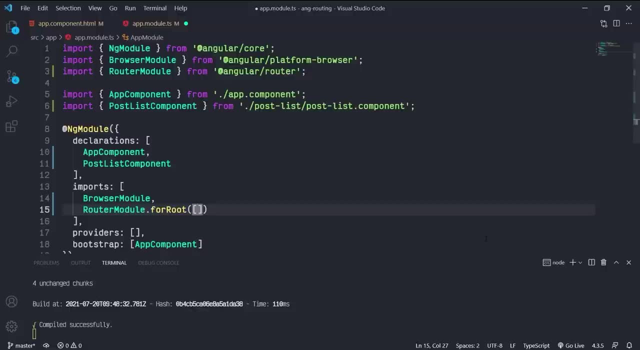 routes. object to this for root static method as a parameter, So array. Inside this we can define the router objects which must have the path and the component key value pairs. So let's see this in action. So inside this array object, as you know, we define objects using the curly brackets, So open. 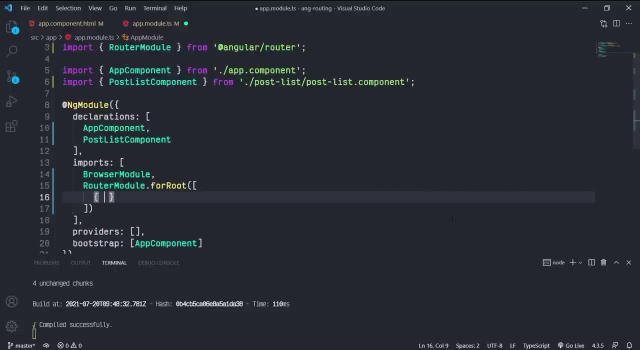 curly brackets Inside. this first key value pair is path and the value is, for now, just pass, an empty string. The next key value pair is component colon. So this value also set to an empty string. So with this key value pairs that we are telling angular to load this component when the browser 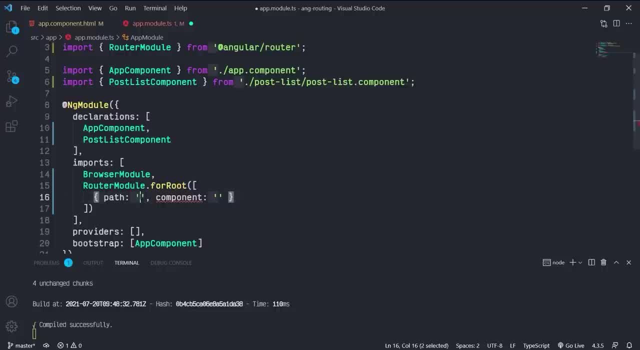 URL changed to this path. As I mentioned, we want to load the post list inside the browser when clicking the button, So let's define a path for the post list Inside this path value: pass the router path: post a plural word. Now pass the. 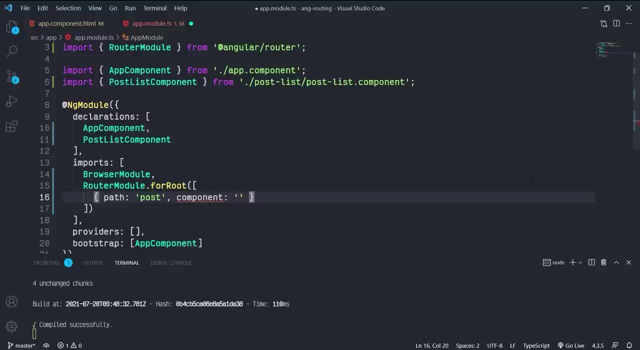 component that we want to show the post list component. So pass the component name. I made a mistake For the component. we don't have to pass this as a string, So remove these codes without codes. Just pass the component name: post list component. That's it. We have successfully created our first router. 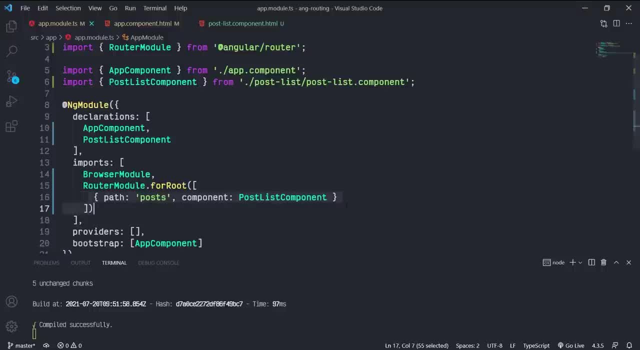 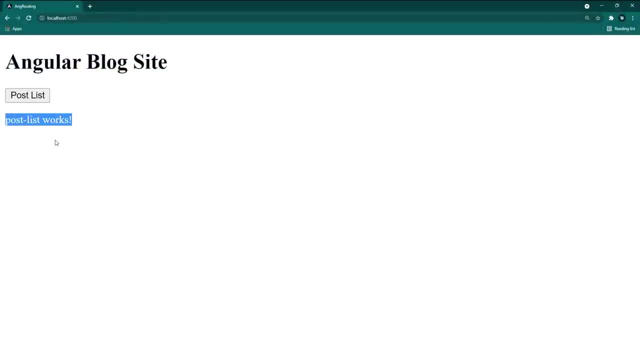 Now we have successfully created our first route. Save this and back to the browser. As you can see here still, we can see this post component cause: in the previous lecture we added this directly to the app component, which is why we are getting this post list works. 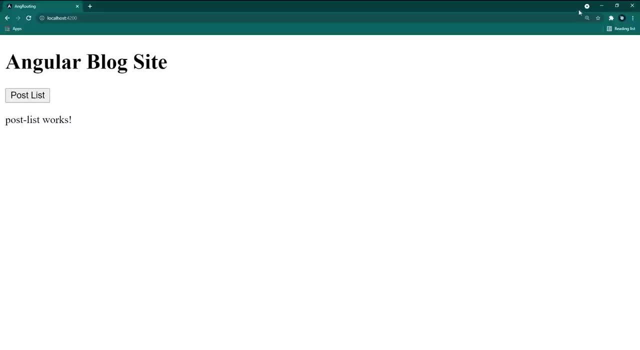 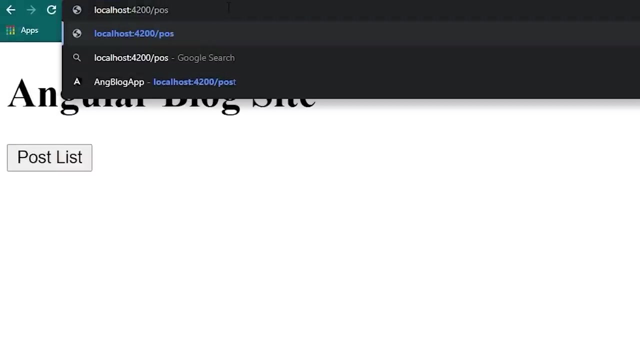 So now we don't need this. So remove it from the app component html file. Now save this and again back to the browser. Now, we got nothing here. Navigate to this post router. after this base URL slash and the router path is post: Hit enter. Still, we got nothing. If you can, 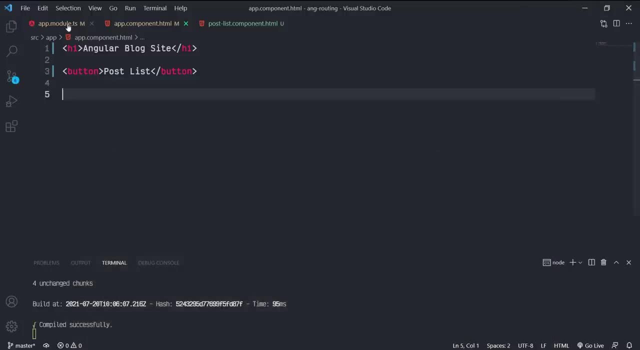 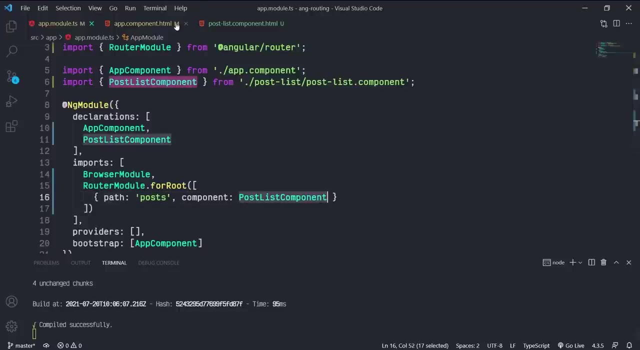 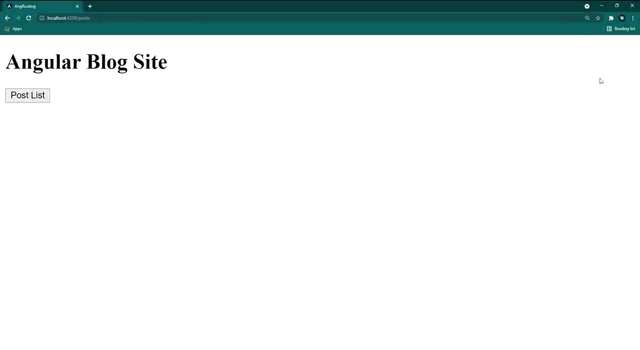 remember we defined the router. when the user navigates to this path, show this post list component. If this worked correctly, we will see this post list works p tag inside the browser, But we got nothing here. What's going on here In order to show the relevant component? we inside. 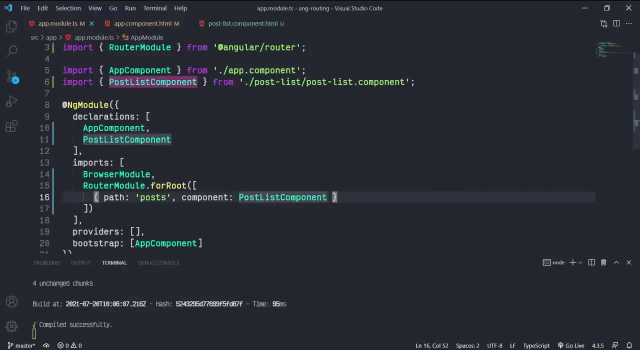 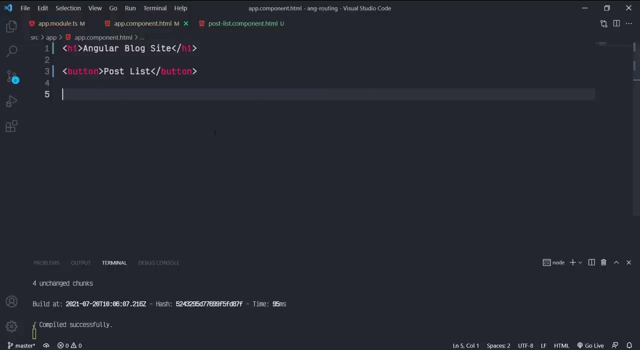 the browser. we have to use a special type of angular html element, which is router outlet, Without routing. we rendered the component weave inside the browser using the component selector as an html tag. So the same thing we gonna do here. This time we are showing the components inside the browser with the routers. 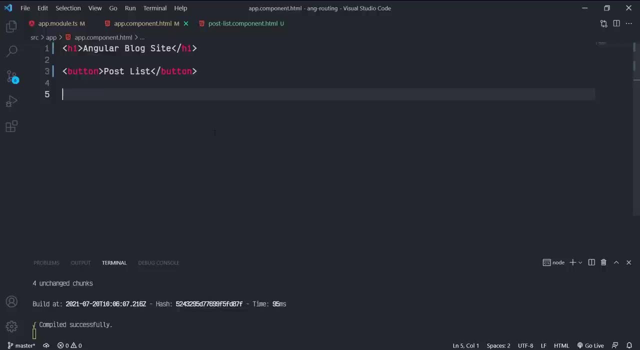 So for that we have to add the router outlet here, This router outlet also coming under angular directive category, But this is different. We use this as a custom html tag, Like the component selector, So let's add this Inside the component html file: router dash outlet. Select the auto, complete This. 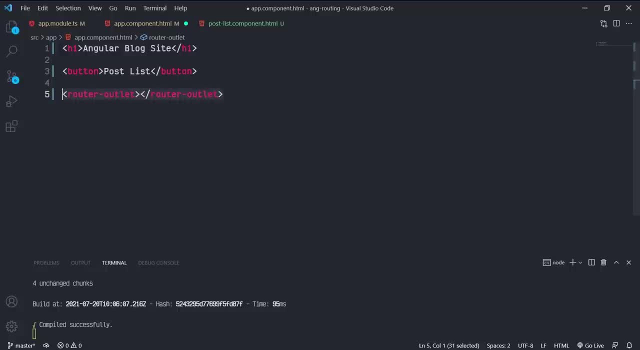 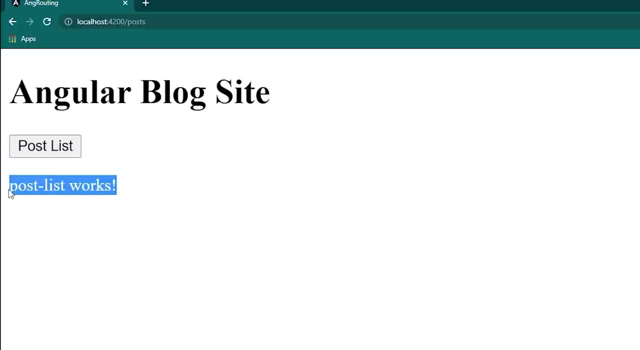 will automatically complete this as an html tag. Now save this and back to the browser. Navigate to the post path. As you can see here, this time we got this post list works, Which means now the router is working fine. Some of you may wonder what is happening here. It's very simple. In order to 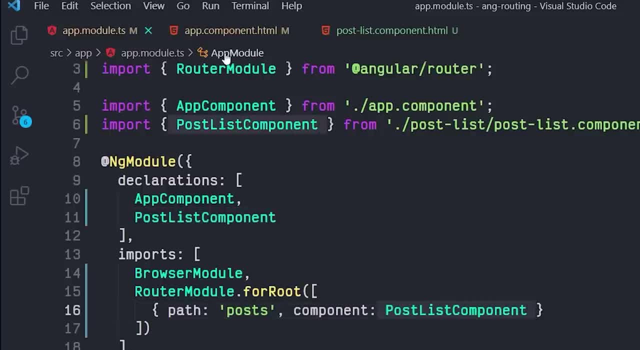 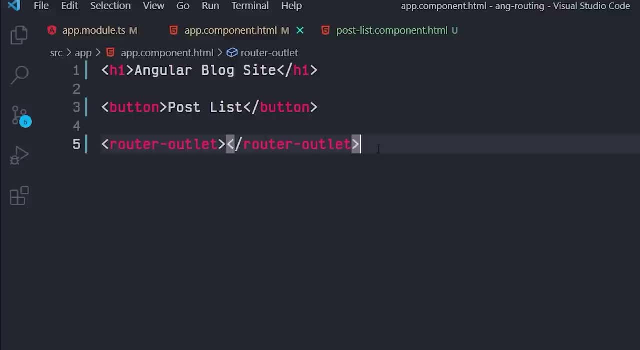 add a root. that is inside the weave. we added the component selector as an html tag inside the app component HTML file Like this: now we added this router outlet directive as an html tag to show relevant component when there is a router. So very simple. Hope you guys got the idea. 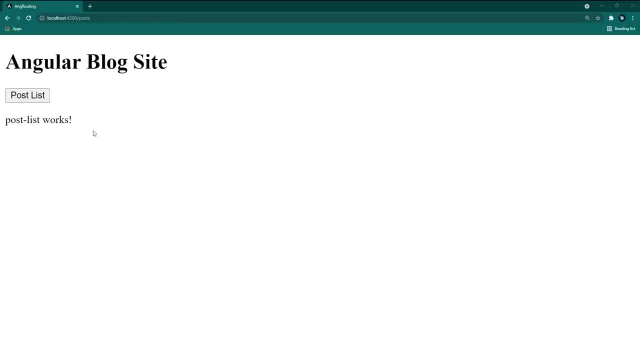 Okay, Now we can load the post list component inside the browser when we navigate to this post router path. We did this manually by typing the path inside the browser address bar. Now what I want to do is I want to load this component when clicking this button. 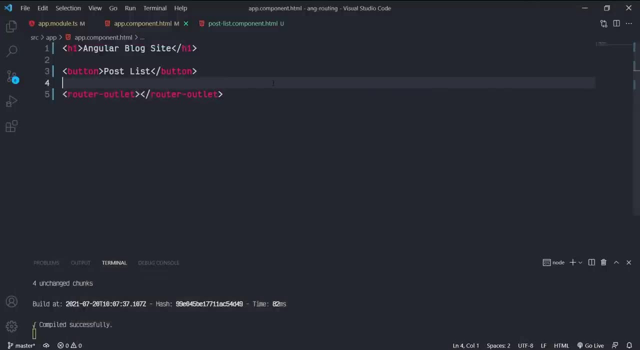 So let's see how to do this. Very simple. for this in angular we have another directive, which is router link. By using this, we can navigate to a specific router when clicking this button. So this is a directive, So add this inside the button starting tag. 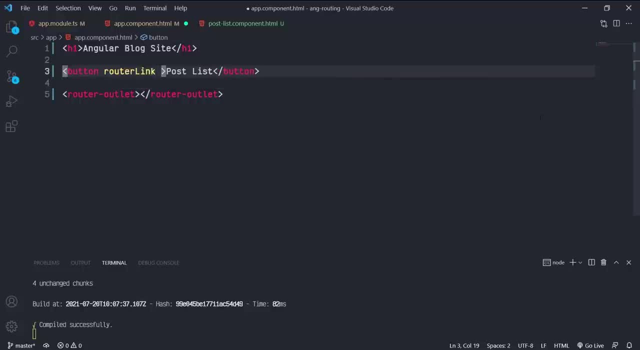 Router link. This L must be capital, As always, follow the capital simple letters correctly. After this: equal sign. inside quotes: pass the path that we want to navigate. Slash. the path is POST. Note this carefully When we define the route. We didn't use this slash. 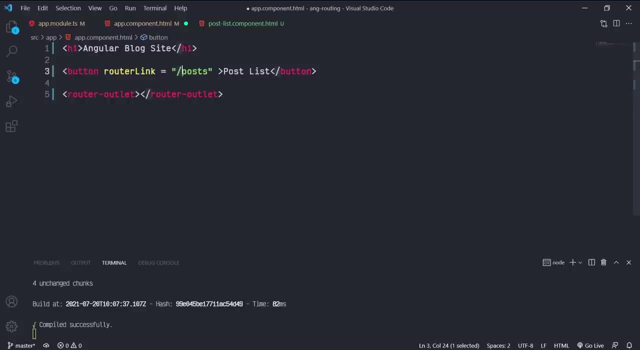 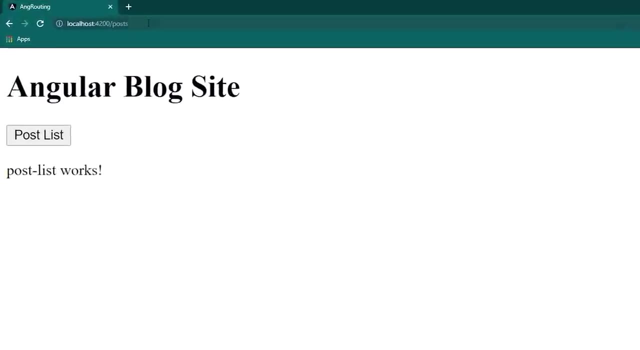 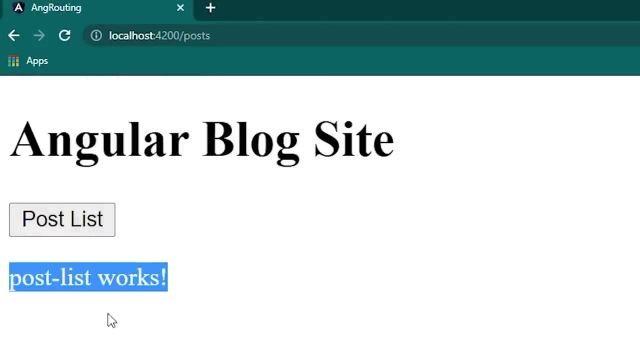 But when we, using that, define router path, we must add this slash before the router path. OK, that's it. Save this and back to the browser. Go to the main URL Now. click on this button. As you can see here, this loaded. this post list works here. 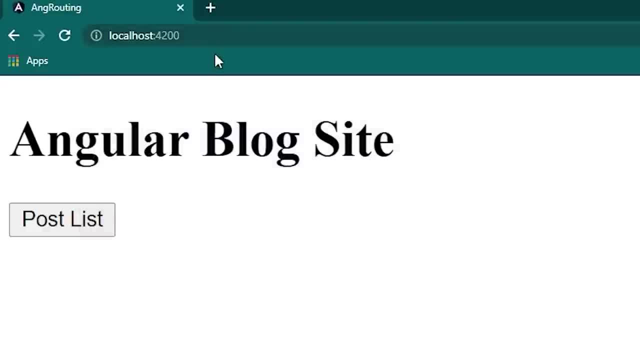 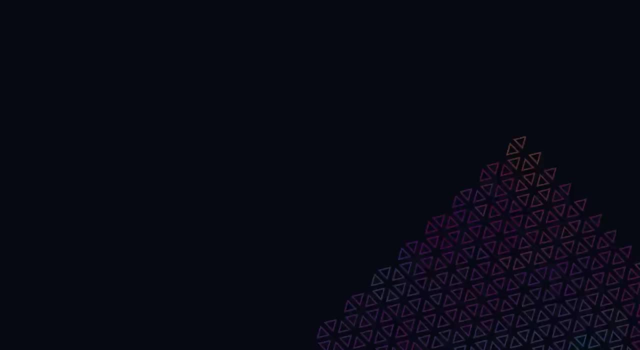 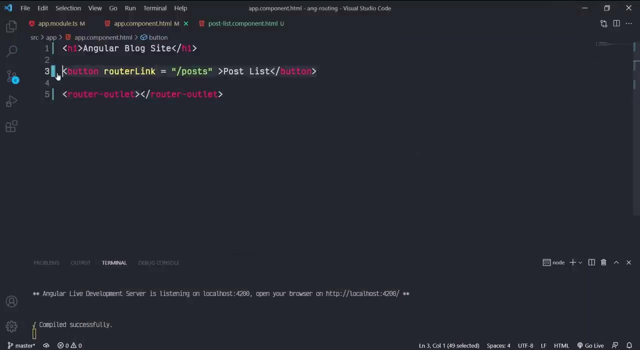 Look at the address bar. Perfect right. When we click this button, This URL change to this, This router path. That's why we got this. Now let's add a button to navigate to the main URL. So back to the VS Code. 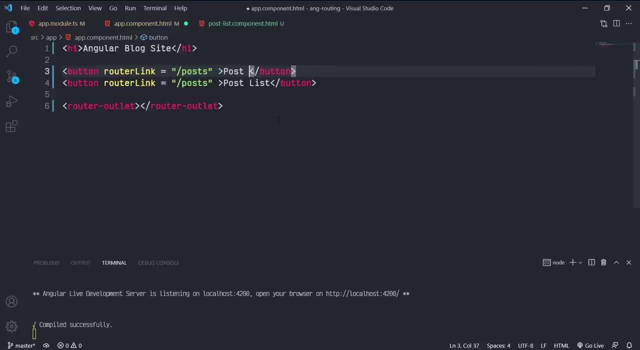 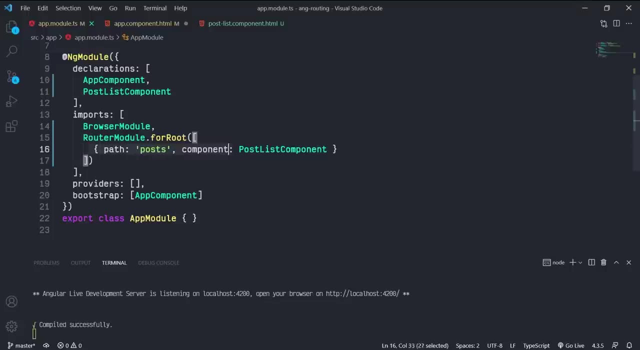 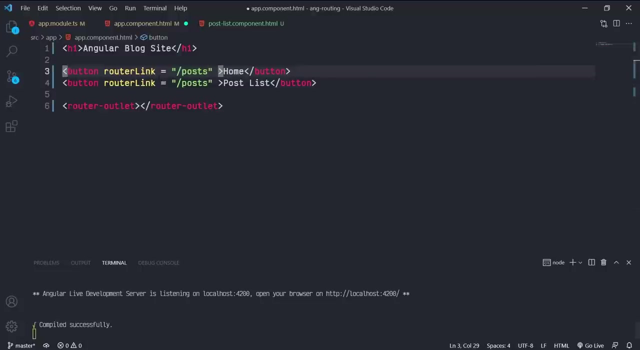 Before this button, create another button. The button text will be home. Set the router link to the main home page or the component. If you noticed, We don't have any relevant router for the main root component, But if we navigate to the project main URL. 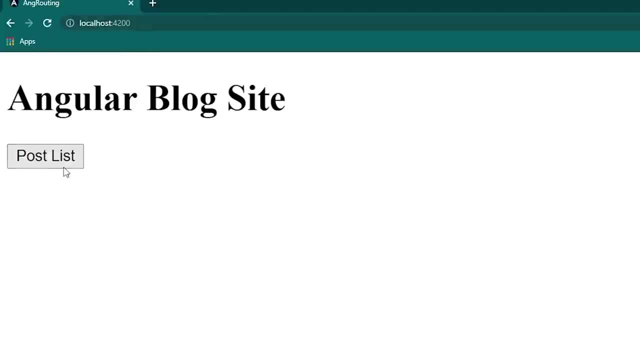 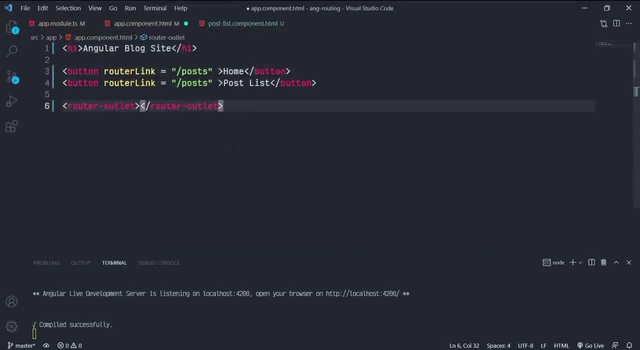 Which is this localhost, colon 4200.. We got this web, Which is this app component. How we getting this? As you know, the main root component is this app component. This generated automatically by angular CLI when we creating a new angular project. 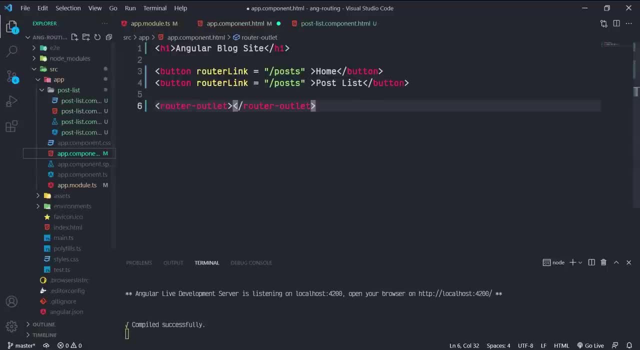 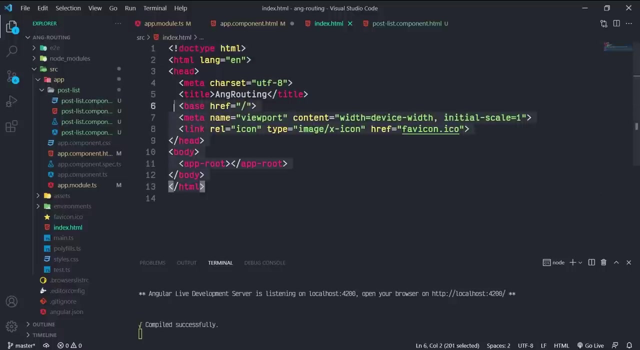 So let's add this: How this component load inside the browser. If you can remember, We learned about this When we navigate to the root URL of this app. This will first load this indexhtml page. So this is the main page that loads inside the browser. 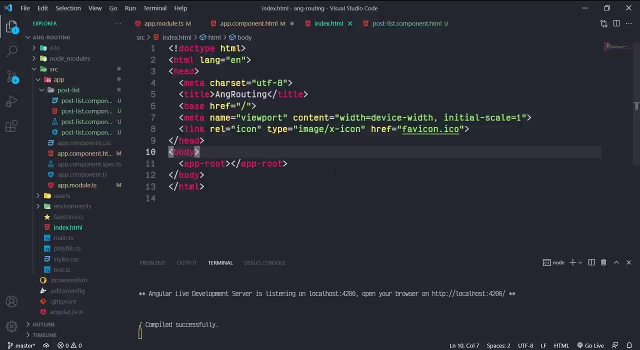 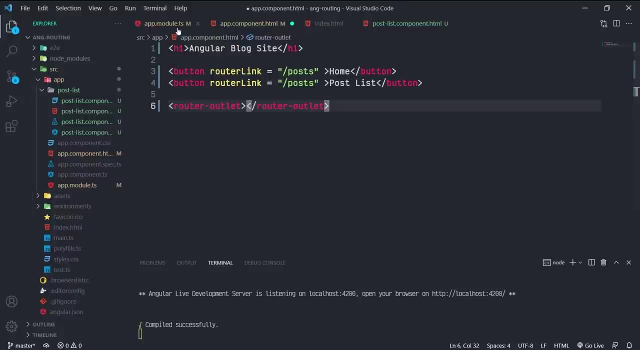 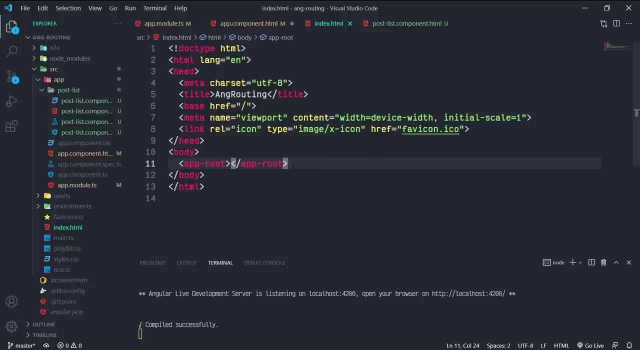 If you look at inside the indexhtml page, We got this component selector, app dash root, Which is this app components selector, So this component selector. So this is how we getting this main root components weave inside the browser. If you look at this further, 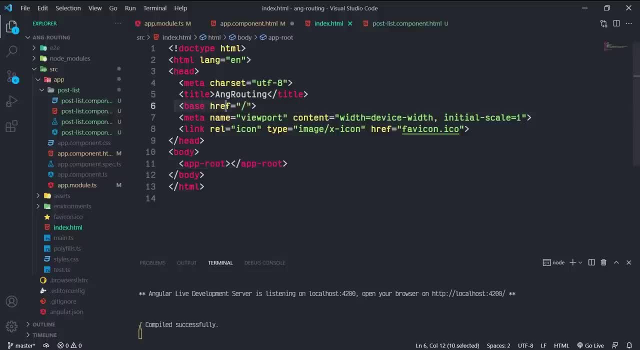 We got another new html tag, Which is the base tag. This is pointed to this slash URL. What's happening with this, With this angular nose? This is the main root file to load inside the browser When someone navigate to the root URL. 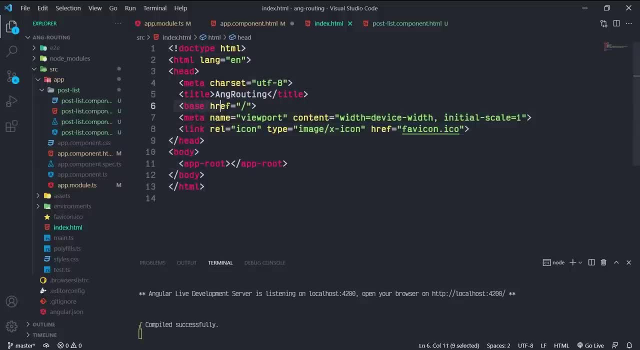 So this is what base URL. So without this, angular doesn't know how to open and navigate through the website. Let me show you a quick example: Remove this base URL, Save this and back to the browser. Look at this. This time we got nothing. 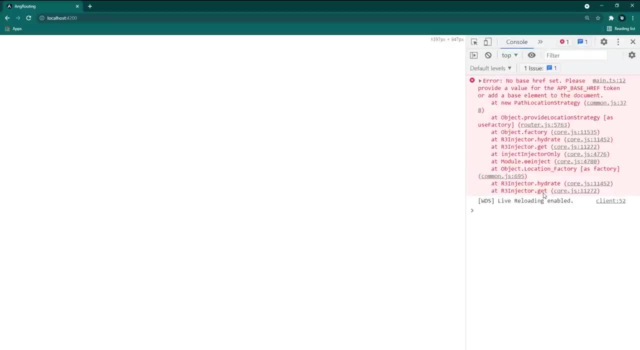 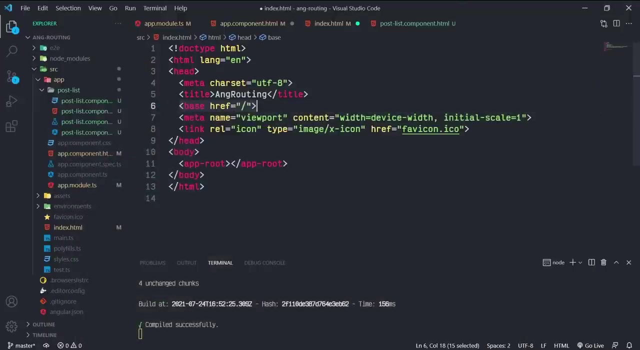 Look inside the browser console. As you can see here, We got this error saying that no base href set. So this is what I try to tell you guys. Without this, Angular cannot understand The navigation of this angular app. Hope you guys got the idea. 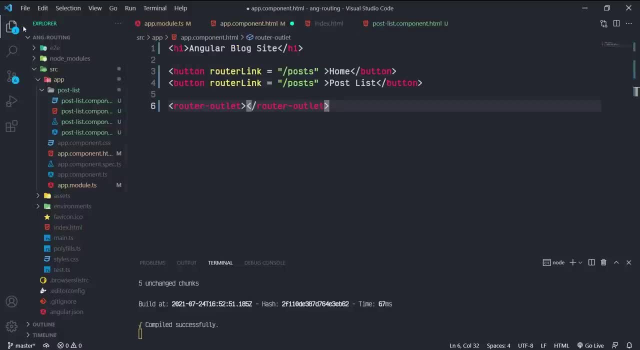 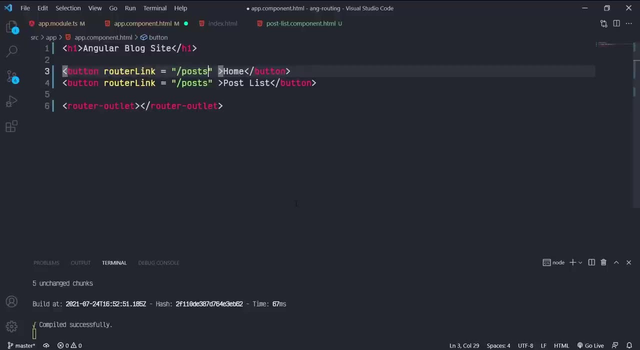 So now add the base URL, Save this and go to the app component. So now we want to add navigate to the main weave when clicking this home button. So, as previous, add the router link directive to this button. This time the URL path is this base URL, which just slash symbol. 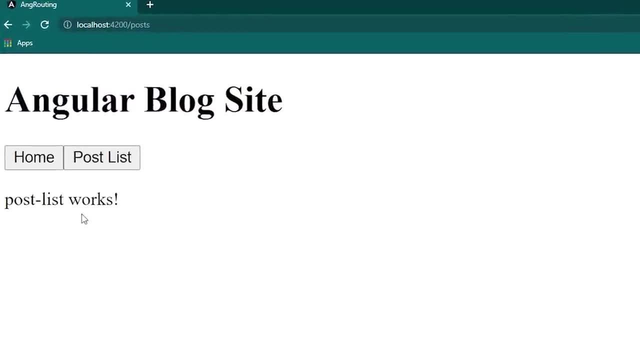 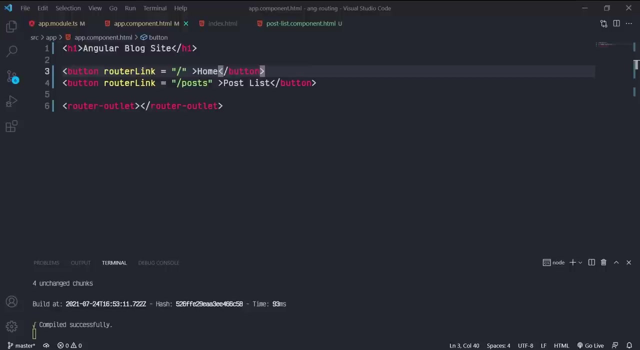 Save this. Click on this post list button. We got the post list component weave. Now click on the home button. Look at the URL. We again navigate back to the base URL. So this is how we deal with base URL. Hope you guys got the idea. 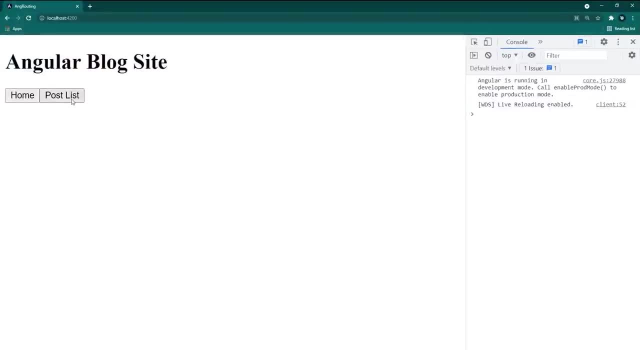 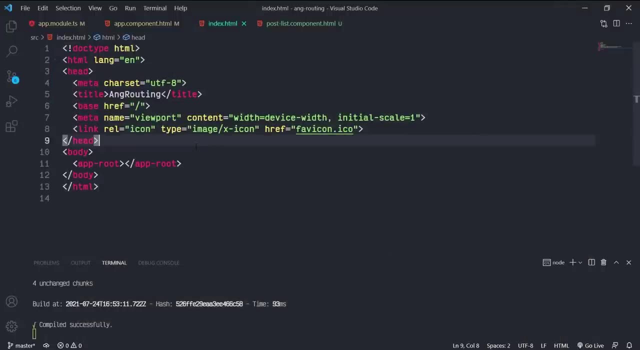 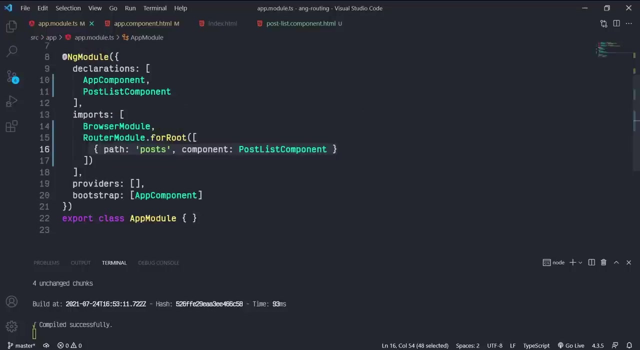 In the previous lecture we learned about the base URL. When we loading The base URL, This will open the indexhtml file inside the browser. Inside this indexhtml file we rendering this app component In routers we have, So in routers we have not defined any page to the base URL. 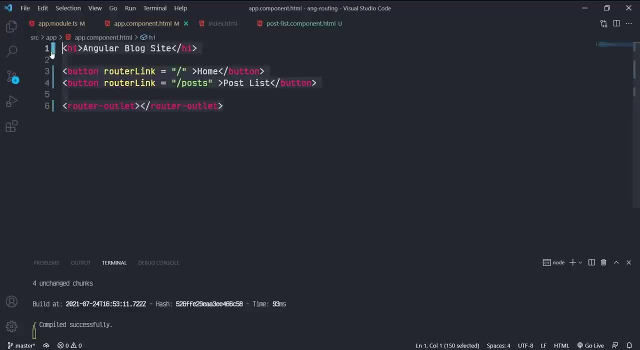 In real world app we don't put many codes inside the app component. We use separate components for this. So in this lecture let's see how to define a base router And point that to a another component. For this let's generate a component. 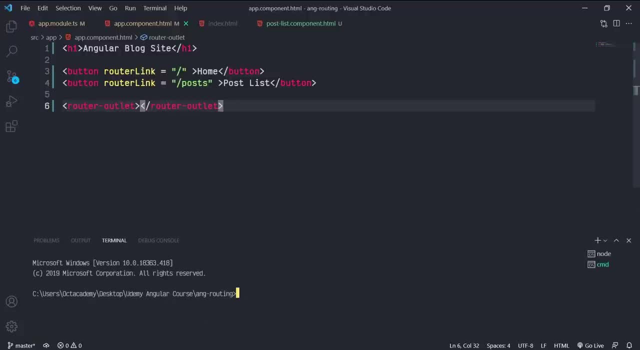 Inside the integrated terminal, run this command to generate a component: ng, g, c. The component name is home. Hit enter to execute this command. Now let's define a new router for the base URL Inside the appmodule ts file. Create another router object. 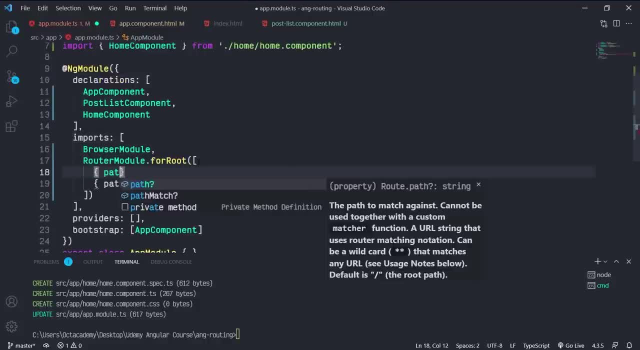 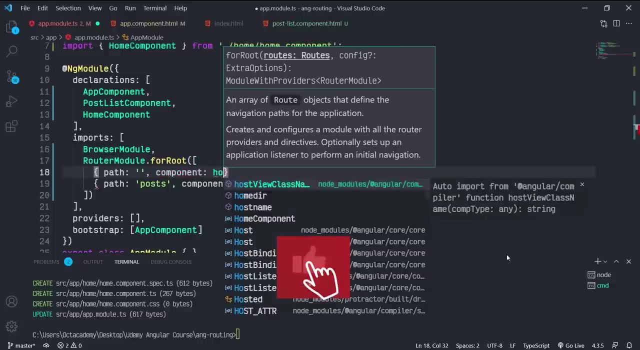 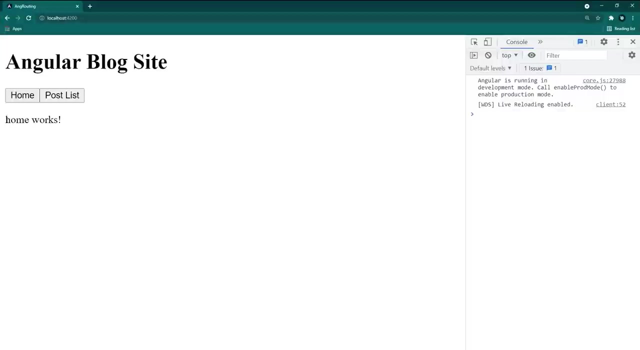 This time path is the base URL slash, But so in the router object we don't add this slash, So just keep an empty string. So this will represent the base URL. The component is the newly created home component. That's it. Save this and back to the browser. 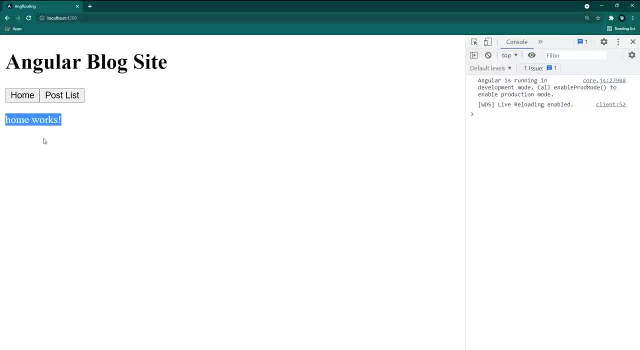 In the base URL. as you can see here, This time We got the home works- Which means home component loaded successfully inside the browser on this base URL. Now navigate to the post list. This time we got the post list component Again back to the home. 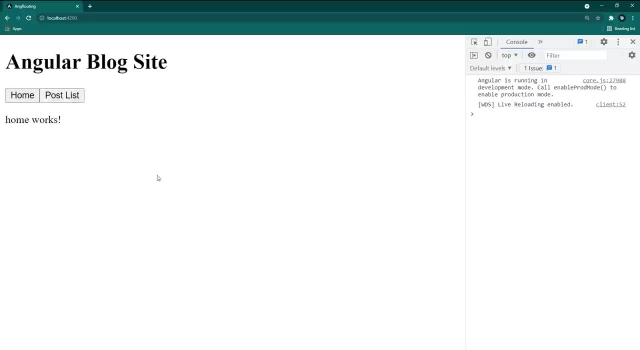 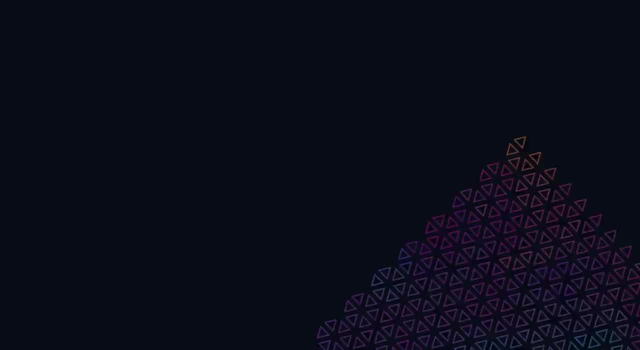 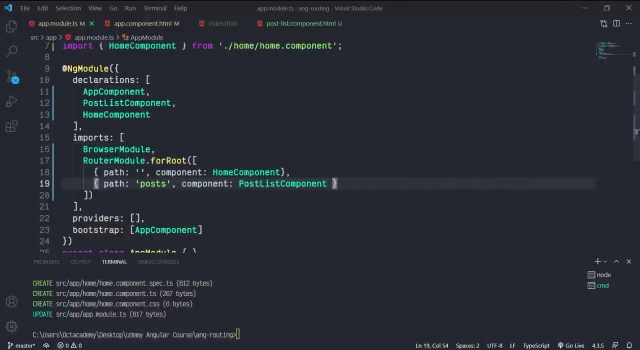 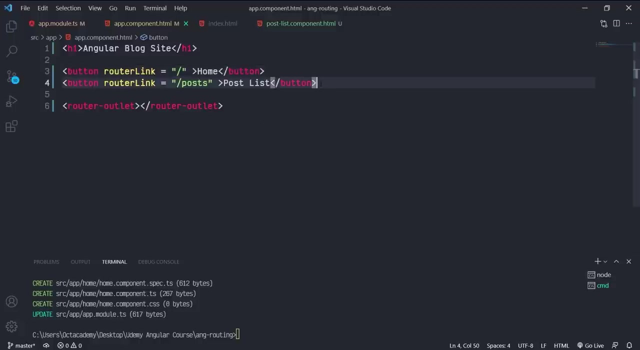 We got the home component. So this is how we define the base router When in traditional HTML pages We use anchor tags to navigate Through the website. But in our previous example we used a button tag, But in angular we can add this router link directive pretty much in every tag. 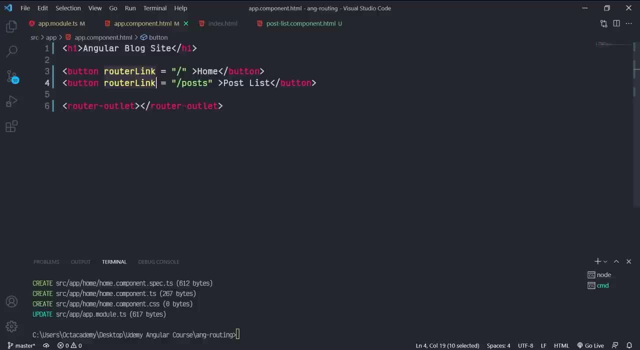 But in traditional HTML we can add links only in anchor tags, Cause. in traditional HTML website we don't have this router link. In order to navigate to a link, we must use an anchor tag, Cause. Anchor tag Is the href attribute. In some cases we use the anchor tags in angular as well. 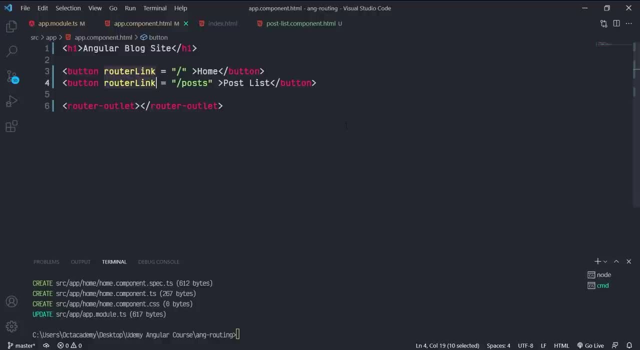 But in angular we will not use the href attribute. Instead of the href attribute, we will use the router link directive in angular. So let's see this in action. So simply create an anchor tag And remove the href and add the router link. 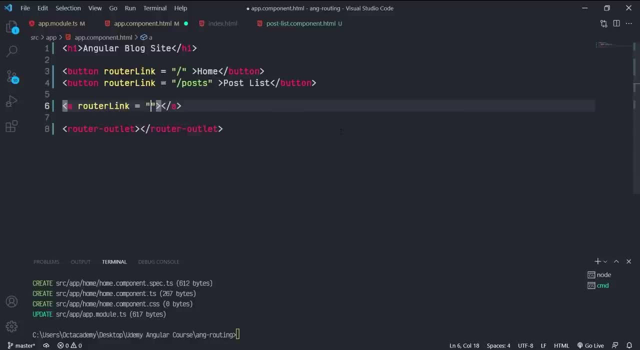 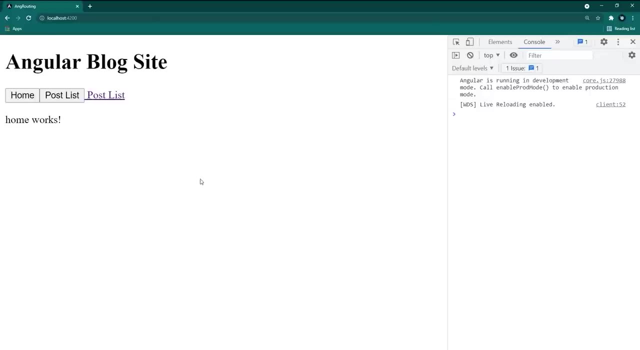 This router link is for post list, So add the post router path to this Link. text will be something: Post list. Save this and back to the browser. Click on this link. This is working as we expected. As you can see here, this is navigate to the post router. 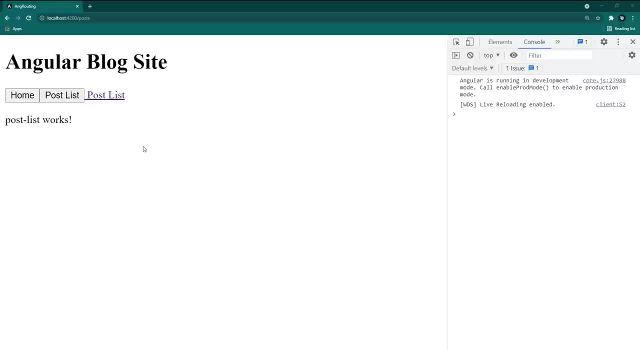 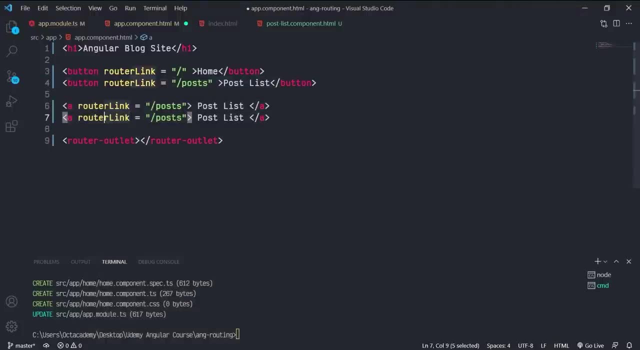 Some of you may wonder why we cannot use the href attribute with the anchor tag. So let's find the answer for this. Create another anchor tag after this. This time, remove this router link And add the href attribute. Check. change the text to post list href. Now save this all and back to the browser. Click on. 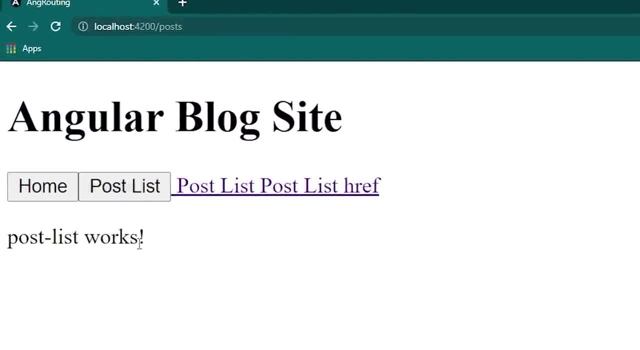 this href post list tag. This also successfully navigate to this post URL. But if we look at this carefully, when we clicking this href link, browser is loading the entire page. We can clearly see this with this loading indicator on the browser If we click on this. 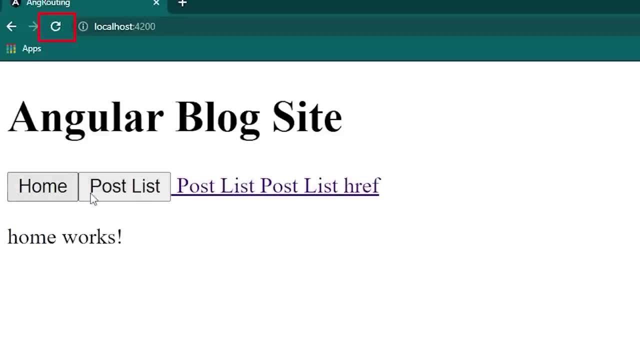 router link href. as you can see here, this will load this component without refreshing the page. So this is the problem with the href tag. When an angular application loads inside the browser at the first time, this will load all the necessary files like JavaScript. 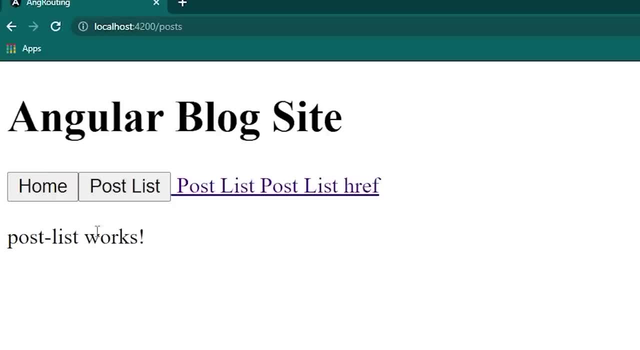 files and CSS files to the browser. After that, when we navigate through the website to other pages- components- the angular app will only download necessary files that need for that relevant component, not all the files like initial load. Wait, I'll show you this. Open the browser tools and go to the network tab. 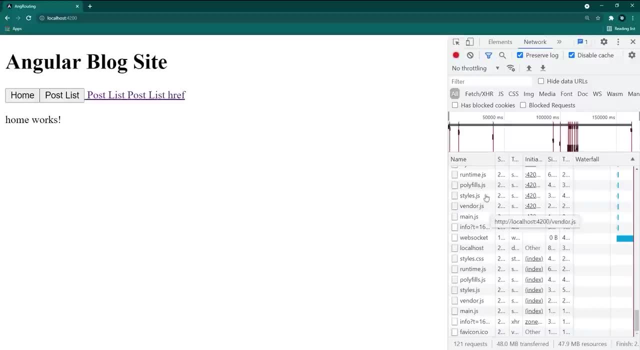 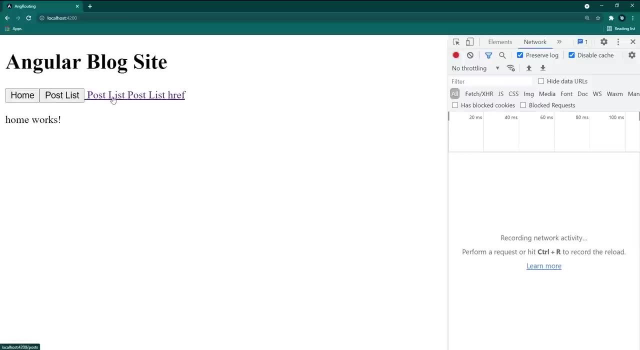 Reload the base URL. Look at this. This loads all the CSS and JavaScript files. Now I remove this all. Now navigate to the post list by clicking this anchor tag which, using the router link. Look at this network tab. Nothing loaded, Pause. As I mentioned earlier, this loads all the necessary files at the 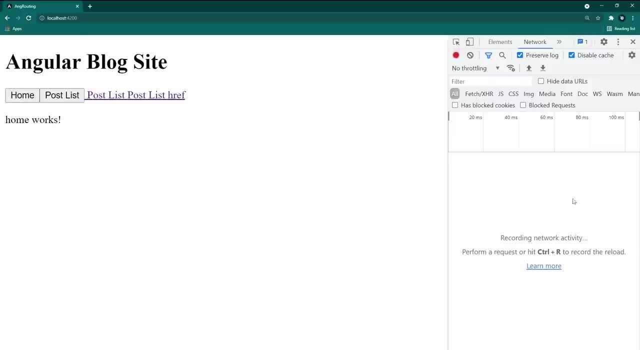 initial page loads Again back to the home Again. this not loaded anything, nif. But look at this carefully. If I click this href anchor tag- look at this- this loads again all the files. This is not a good practice for an angular app. So this is the problem with the 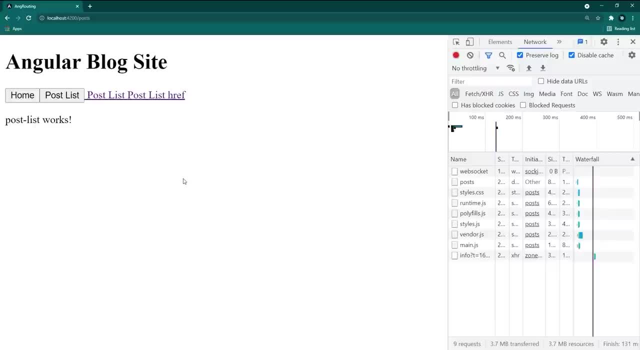 href tag- href anchor tag- html- website. we load websites pages like this. sometimes this will cost lots of time to load a page. so if we using the href with the angular, there is no use of using the angular framework. we can use the traditional way, right? hope you guys got the idea. 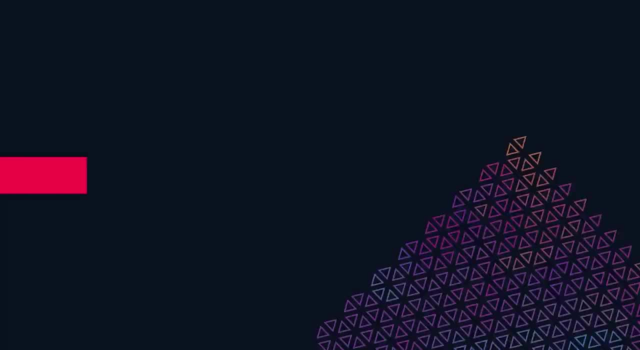 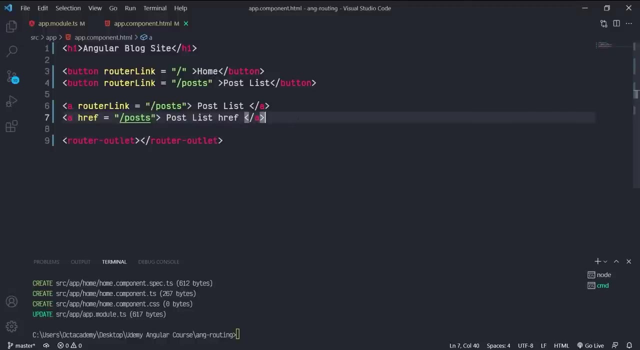 we learned about the angular outer link directive and href attribute in the previous lecture. now in this lecture, let's see how to show an active status on these router links. so we don't need these anchor tags, so remove them now. what i want to do is i want to change. 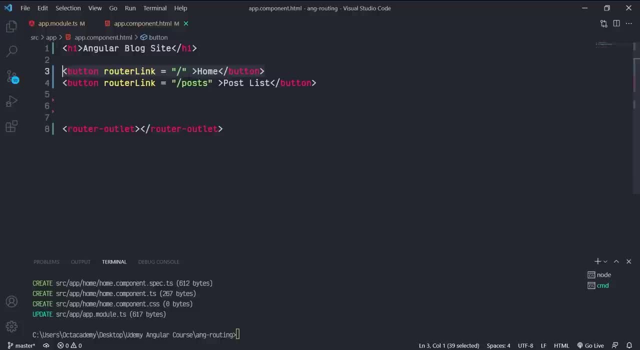 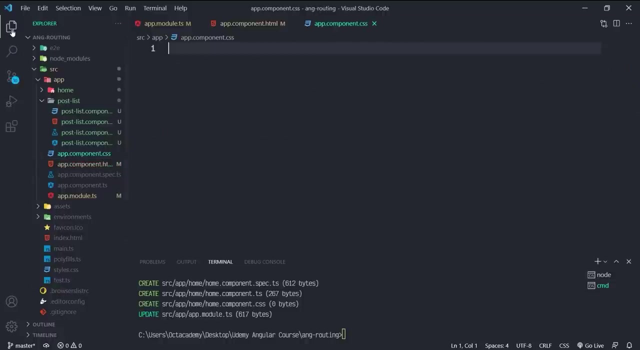 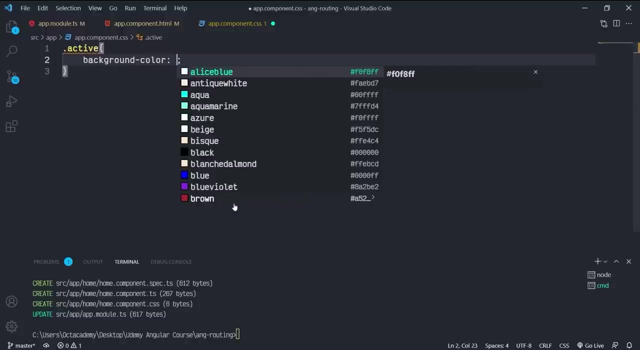 this button color to something red when we navigate to that router link. so let's see this in action. um, let's add a css class to this button, something active inside component css file. add the css style to this active class: dot active and the css scope inside this. set the background color to red and also. 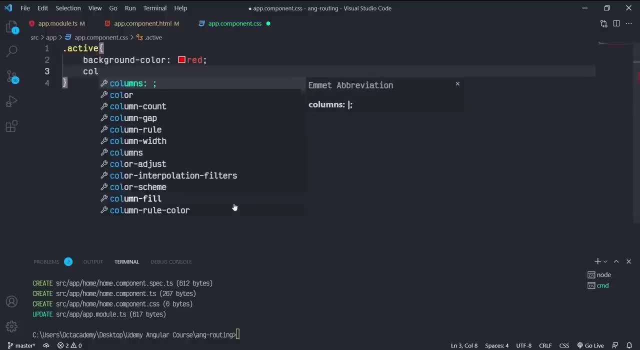 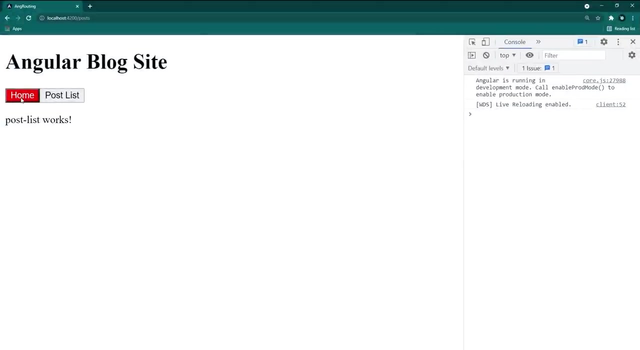 the font color to white. that's it. save this and back to the browser. we got this red color button. now what i want to do is i want to apply this active css class to this button when we navigate to that particular path, for example, if we navigate to the post path. i want to apply this active class to this. 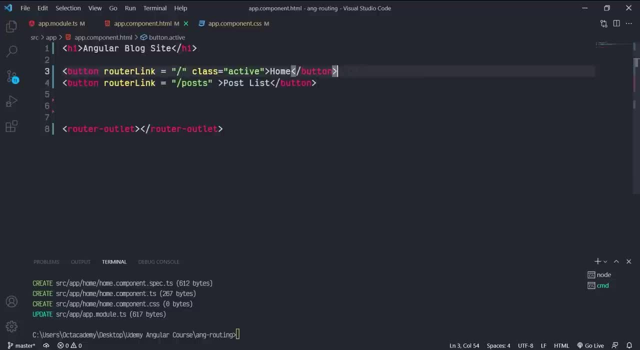 post list button. if i navigate to the home path, i want to remove that style from this post list button and apply that to the home button. so let's do this. if you can remember, we did conditionally css classes binding using the class binding and the ng class directive. 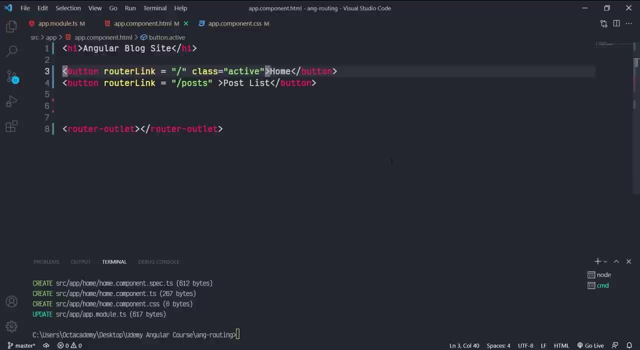 but for the angular routers we have a separate directive, which is router link active. so let's see this in action. first, remove this class. very simple, just add the directive router link active. follow these capital simple letters carefully. so after this, as usual, equal sign and the quotes: 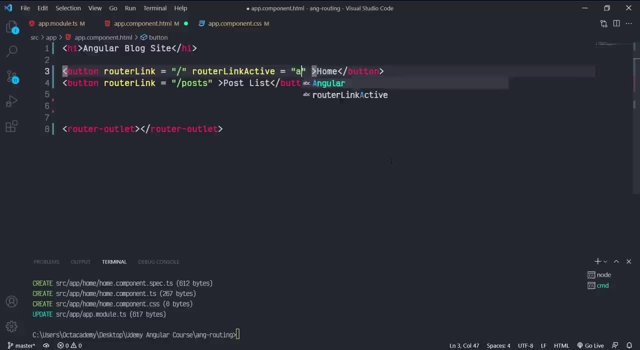 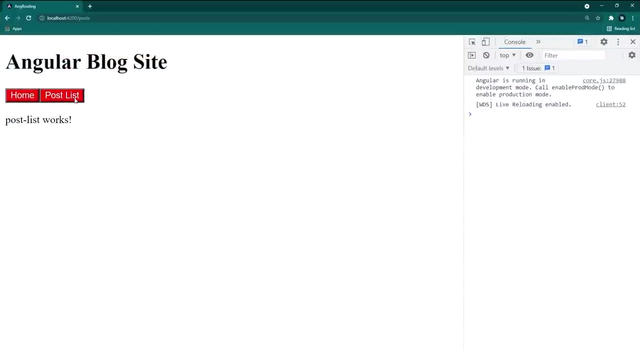 inside quotes: pass the css class that we want to apply active. very simple, right. add the same directive to this button as well. save this and back to the browser at the base url. we got this home button in red. navigate to the post url. perfect, now this post list button in red. 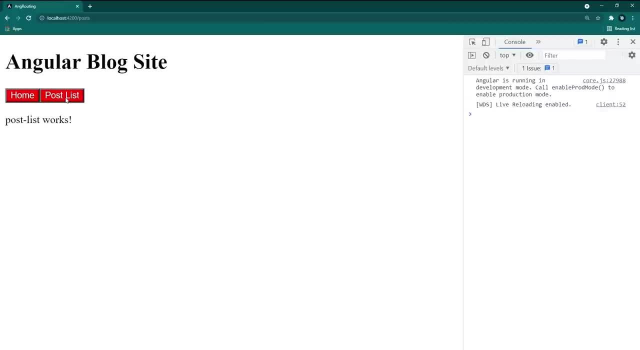 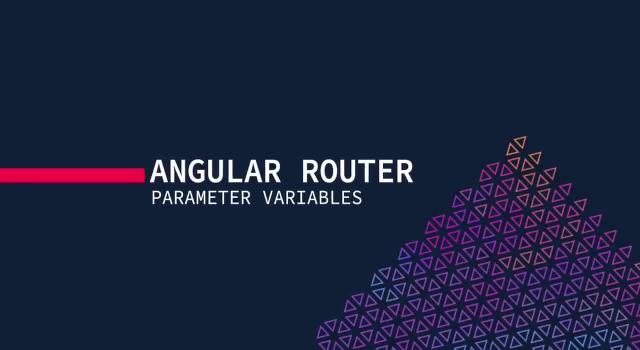 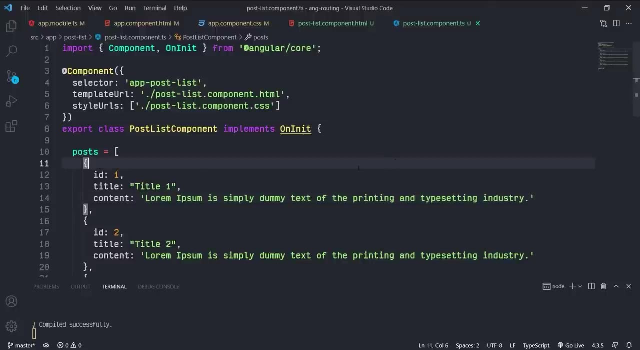 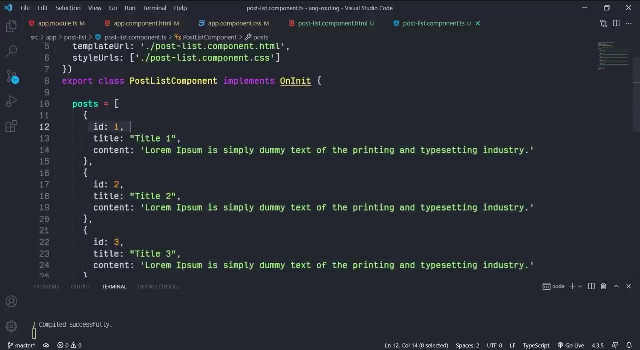 so this is how we deal with router link active directive. i added some modification to the post list component, so inside the post list component ts file, i created this post object array with these key value pairs, id, title and the content. you don't need to follow this as mine. 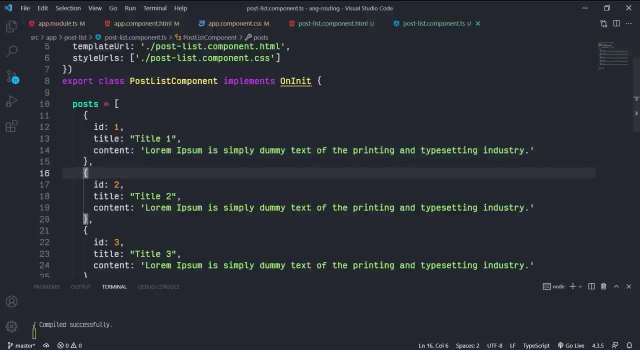 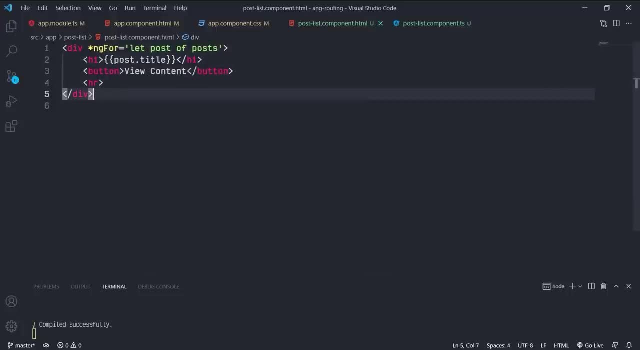 is now the same, but if you need this, you can get this code from the attached files. inside the gmail file, just added these markups to render the post array. with this ng4, as you know, we can loop an array. so with this h1 tag showing the title using the string interpolation. 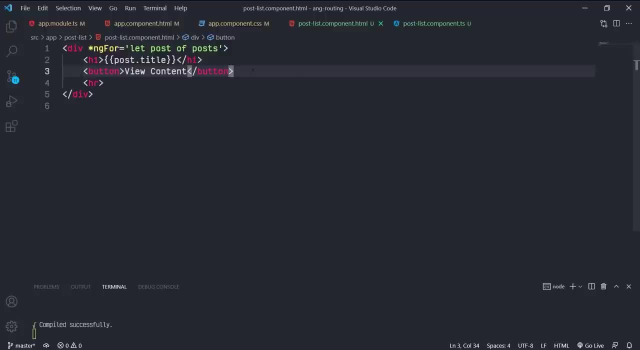 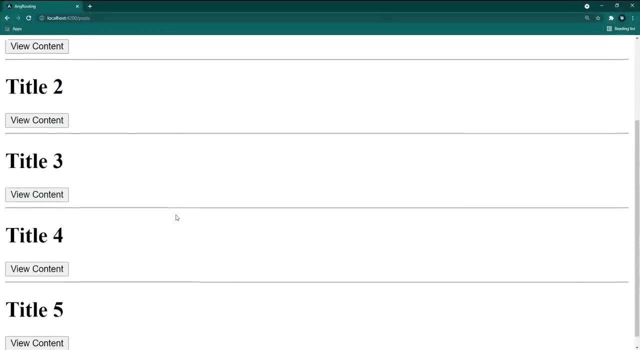 after this i added a button to be this post: just a simple markup for render post list inside the post list component. all about this in the previous sections. Alright, so inside the browser this will look like this: Now I want to make this wave button live. Still, we are not doing. 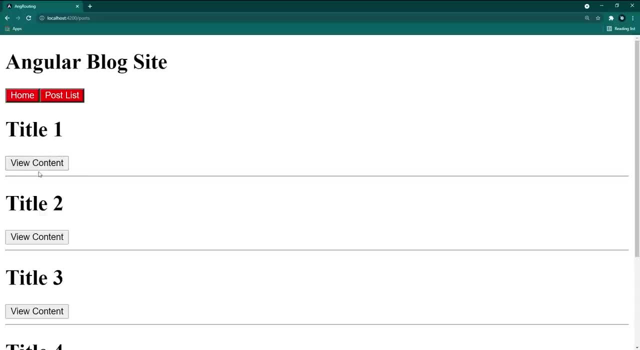 anything with this right. So what I want to do is I want to open a new component or navigate to a URL that shows only this post details. As you know, inside our post object array we have the post content. Inside the post list, we only 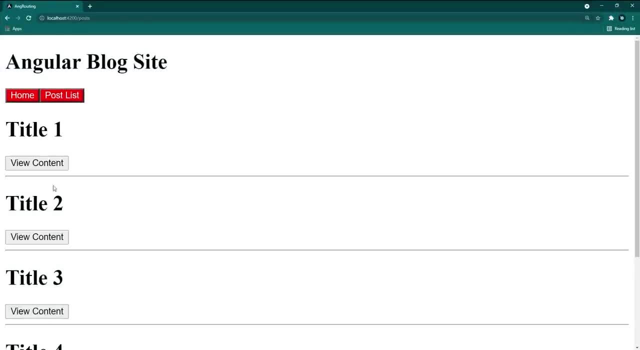 showing the post title. If someone wants to read this post content, they can click on this wave content and read the full blog post content. So let's see this in action. So first we need a component. So let's generate a component Inside the 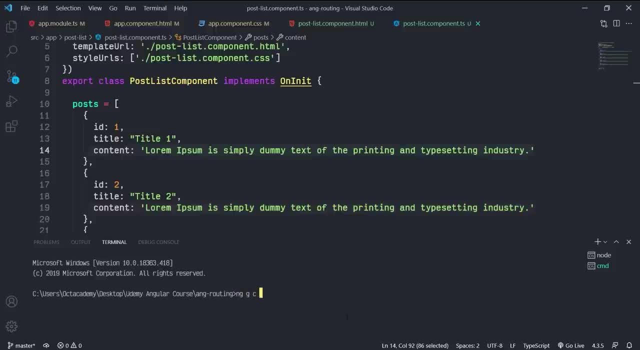 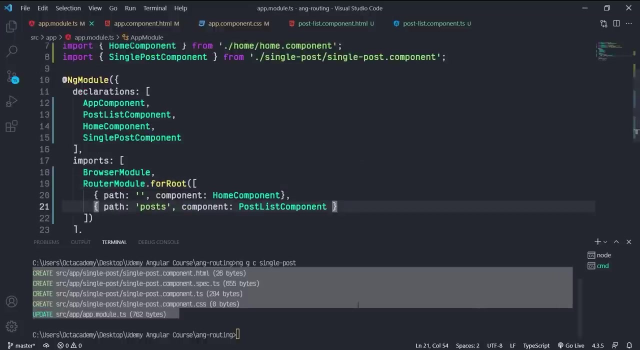 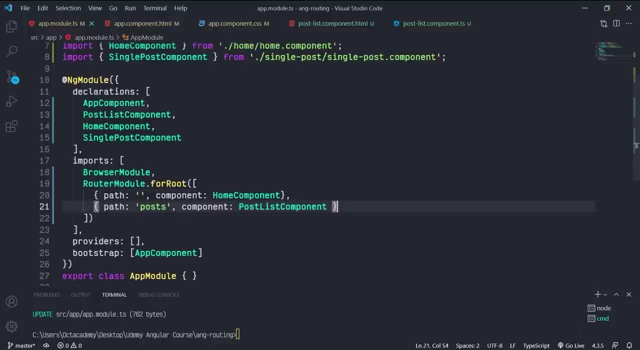 integrated terminal ng-g-c. the component name is single post. Alright, now let's define a route to this single post component. Go to the app model TS file Inside this router array. let's define the router. After this, create the router object. The path is post, Same as this. Keep this for now. We'll come. 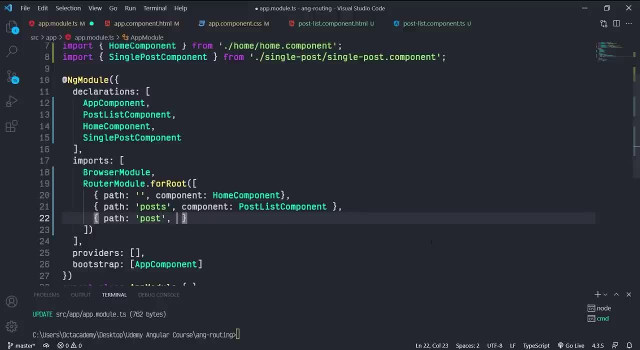 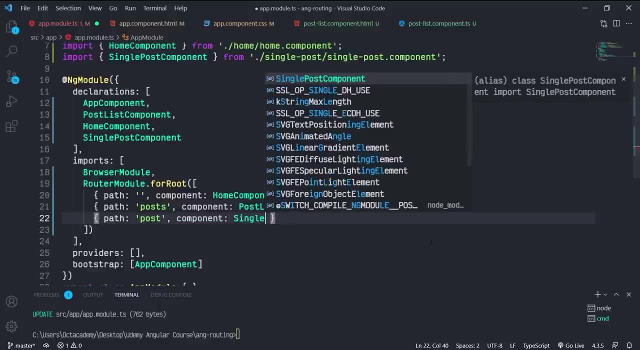 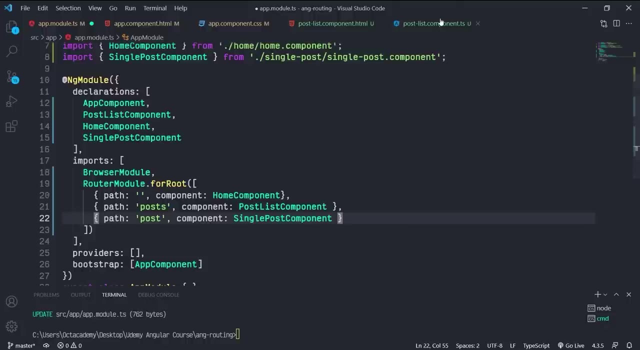 back to in a minute. Next, point this to the single post component. After this comma, key is component And the value is single post component. So now, in order to show the post details inside the single post component, we have to pass the index of that array. Then 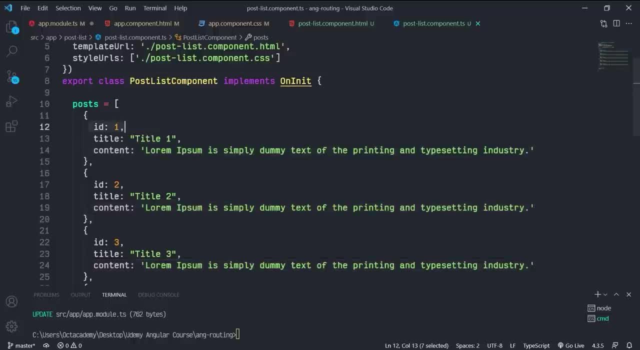 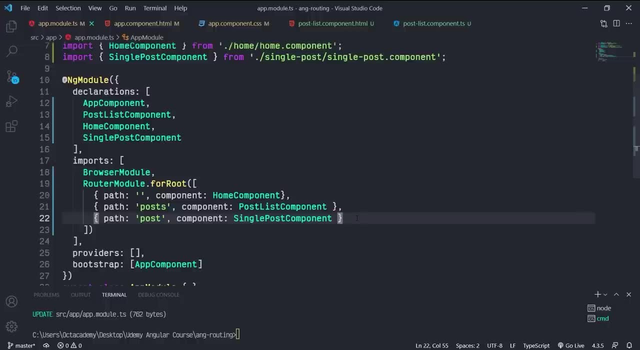 only we can fetch that array object details inside the single post component. So how do we pass that array index from the post list component to single post component? We have a simple solution for this: We can pass data between components via binding that data. 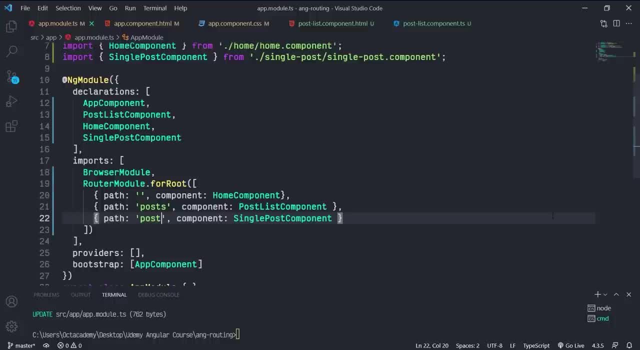 So let's see this in action. For that first we have to define that in the router. We define router parameters like this: After this slash colon sign and the router parameter variable name: something: id. This can be any name. So we define the router with the parameter. Now 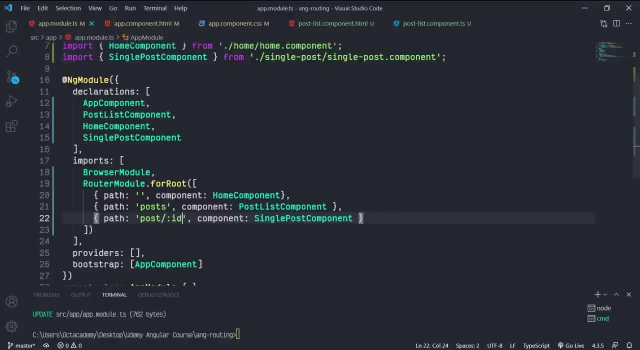 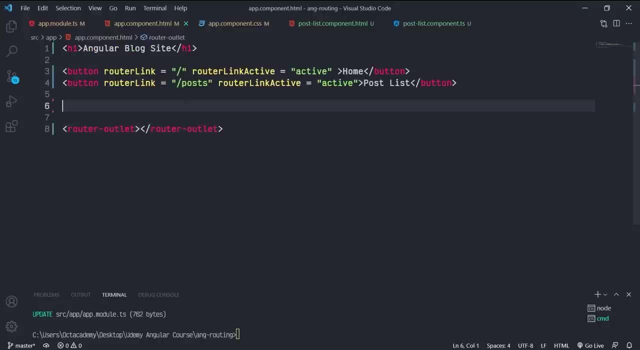 what I want to do is I want to go to that URL when clicking this weave button, So we can do that using the router link directive, as these om and post list buttons. So add the router link to this weave button And the router path is this post. Now we have to pass the router id parameter with this: 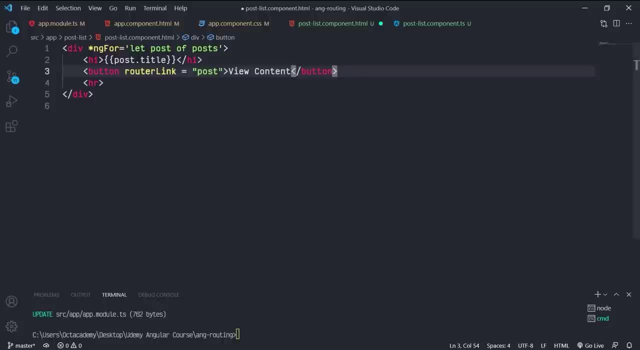 router as well. So how do we do that? For this, first we need the index of this array. We can get that with this ng4.. We learned about this right. So inside the ng4, let index assign index. This index is coming from. 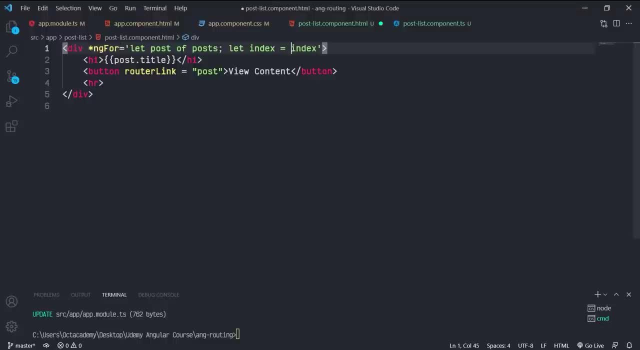 this ng4. And this is. we created new variable, So this can be any name. All right, Now we are getting the index number with this. Now what I want to do is I want to pass this index number with this router. as a parameter For this, we have to do a small modification to this router link. 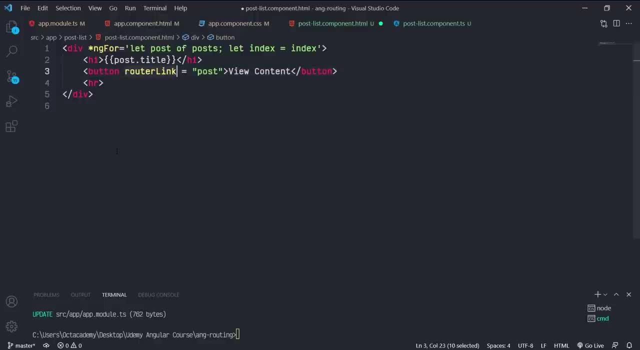 So first, make this router link directive as a property binding. We can make this with the square brackets. Wrap this router link with square brackets. Now, for this we have to pass two parameters. So remove this Inside double quotes. create another square bracket Inside this Router. 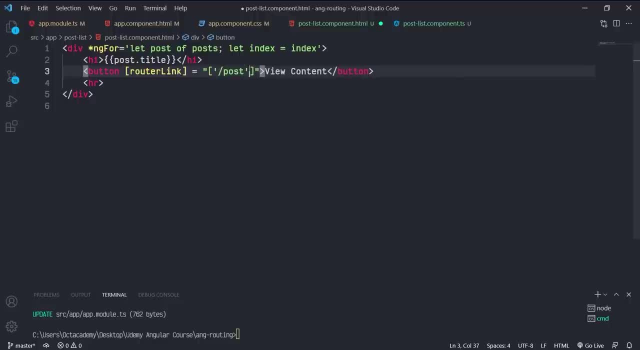 path. as the first parameter, Which is this Post, Pass this inside of a single quotes After this parameter value. as a second parameter, which is this index variable, just type the index variable name after this comma. that's it. we have successfully created the router with parameter. 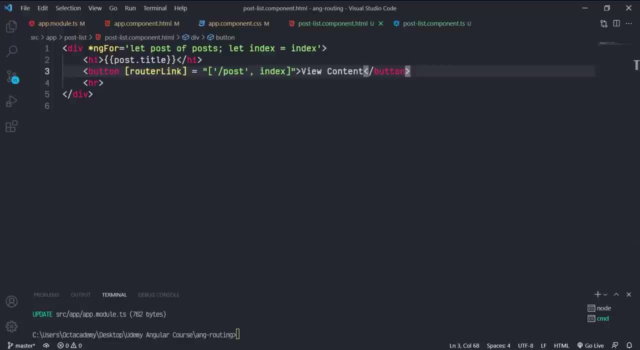 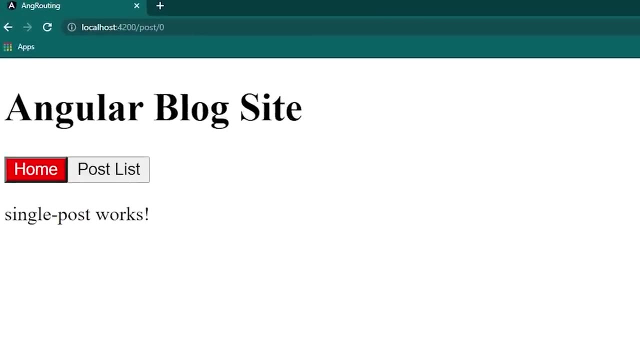 and also we learned how to pass the parameter variable with the router link directive. now save this all and back to the browser. now click on this weave button. this open the single post component. that's why we got this single post works. look at this url inside the browser address bar. 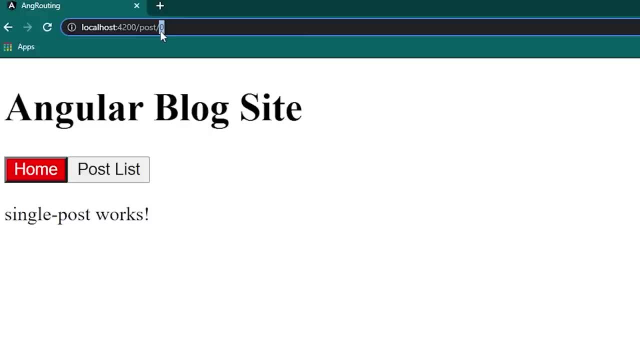 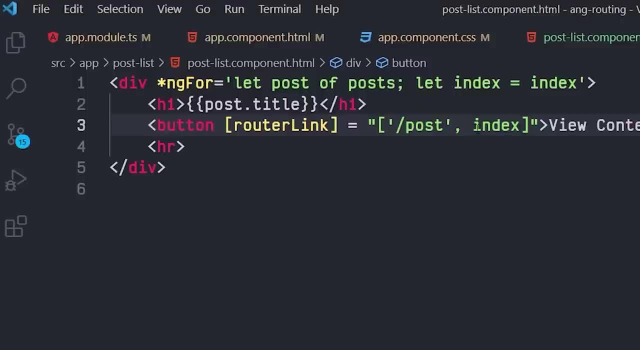 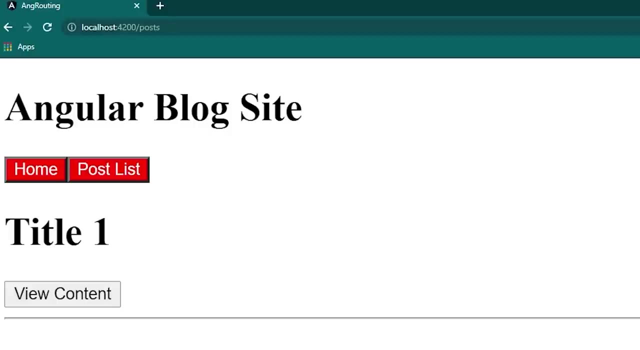 we got the url path and after this, we got this number 0. what is this can you guys use? yes, this is the parameter that we passed with this: this post array index number. go to the post list and click on the second post. we got the number one as the parameter. 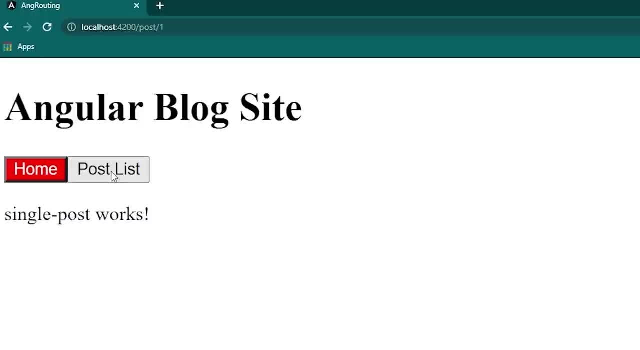 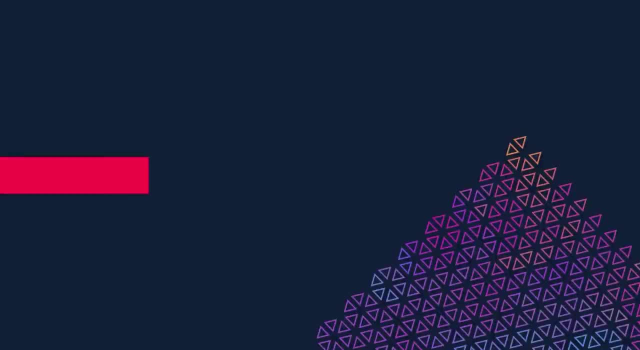 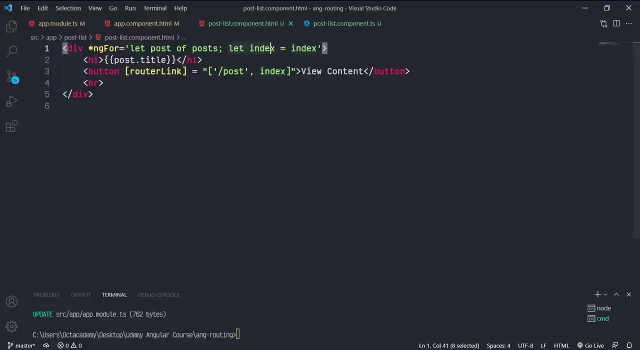 cause. as you know, array index started starts with 0.. So this is how we pass parameter variables from one router to another router. So in the previous we sent the index number of this array via binding to the router parameter. So in this lecture let's see how to get that parameter from the router and how to show the. 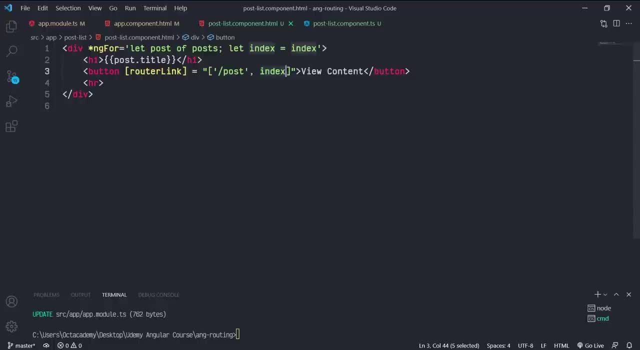 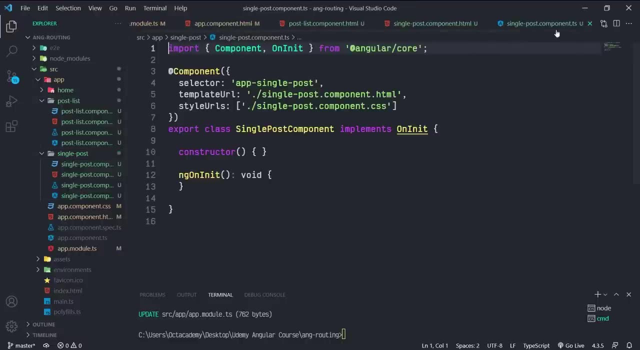 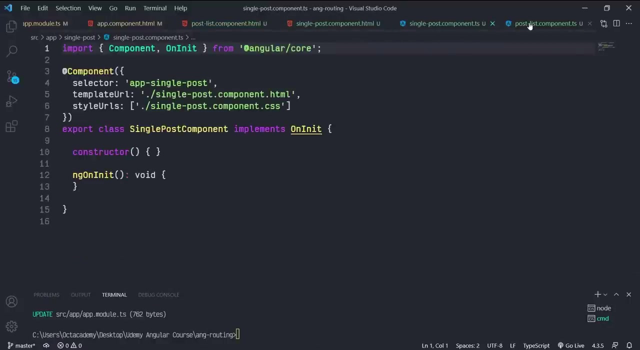 relevant array data to that array index. So we are sending that router parameter from post list component to single post component. So let's capture that router parameter from this single post component. Open. the single post component is file Inside this in order to capture the router. 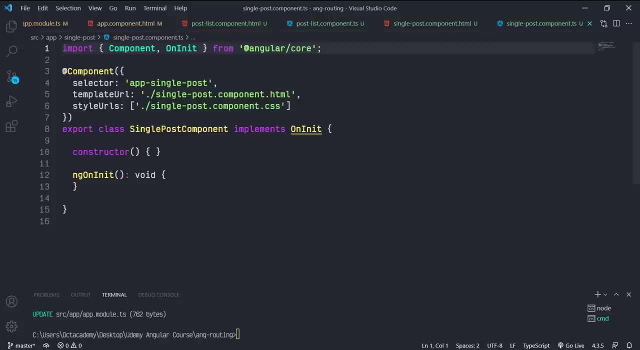 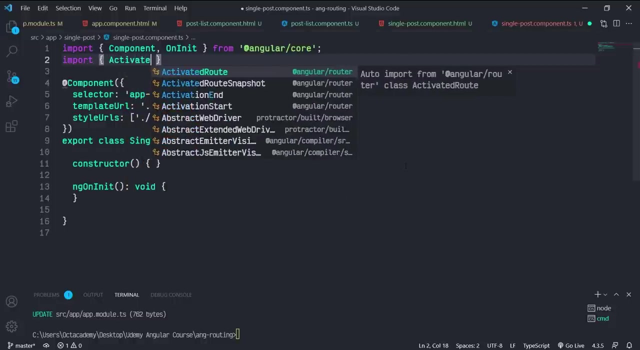 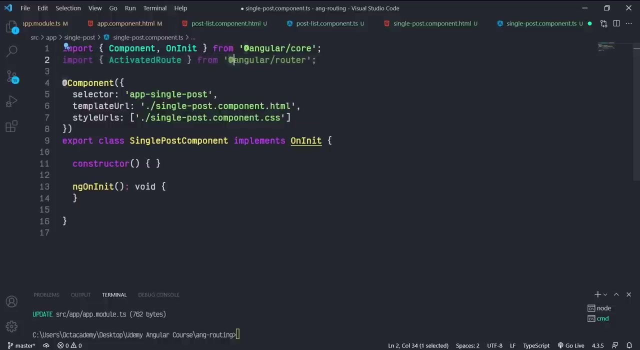 parameter. we have to use the activated route module, which also comes from the angular router. First thing: first import the activated router module to this component. So import inside curly brackets activated route, as always. carefully follow the capital simple letters After this FROM This also coming from the angular router. 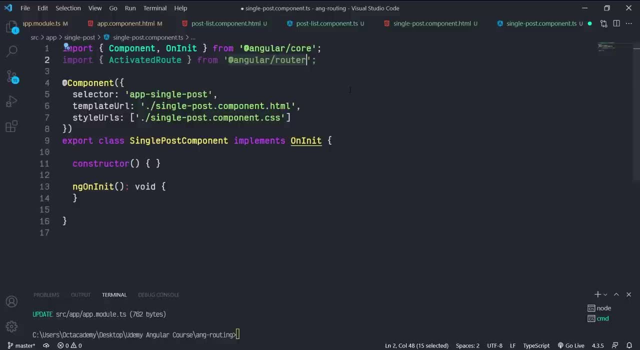 module, So at angular slash router. Now we have to use this activated route to get the parameters, But we cannot use this directly. In order to use this, we have to inject this activated route class into the constructor, like the angular services. So inside the constructor private route. this can be. 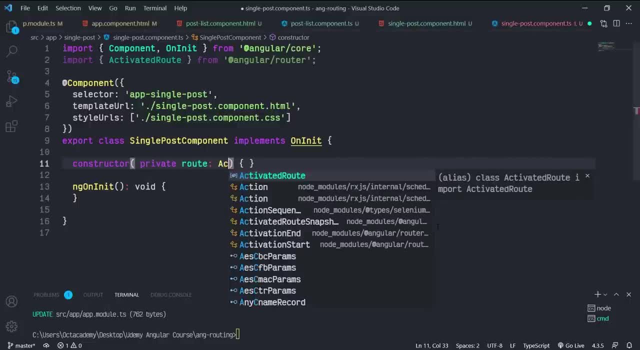 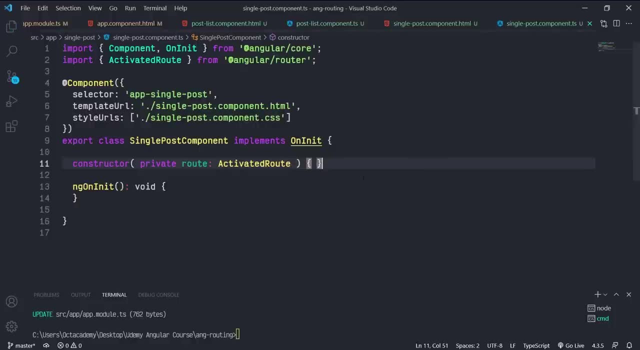 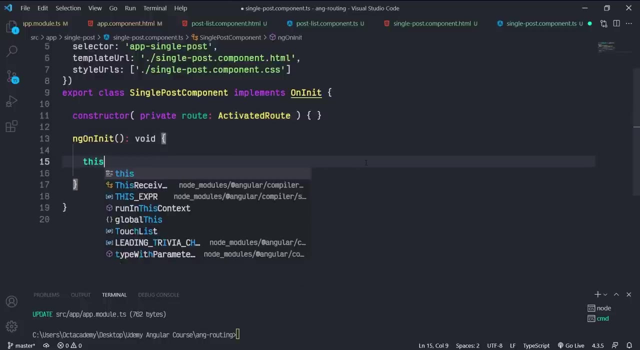 any name. so, after this colon and the class name, which is this activated route, That's it. Now let's see how to get the route parameter using this activated route. Now, inside the engine, init this dot route, which is this injected activated route. after this paramap, this m is capital. 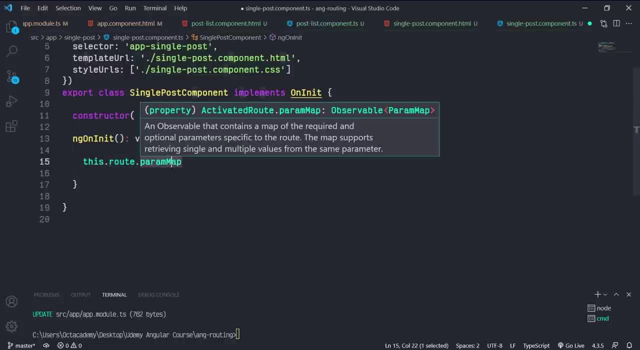 So this paramap is the property that gives all the router parameter values. If you look at this paramap type, as you can see here, this is an observable. Observable is something coming from rxjs, So leave that for now. In the next lecture we'll learn about this in detail. Okay, so in order. 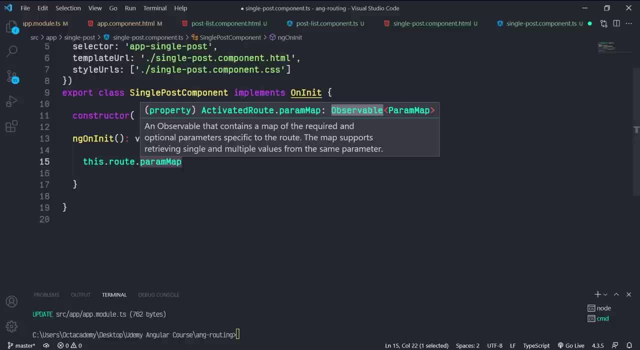 to get the route parameter, we need to get the parameter. So let's say we want to get the route values from an observable, we must subscribe to that observable. So after this: subscribe, this is a method. So after this, parentheses: this required a function with value parameter. 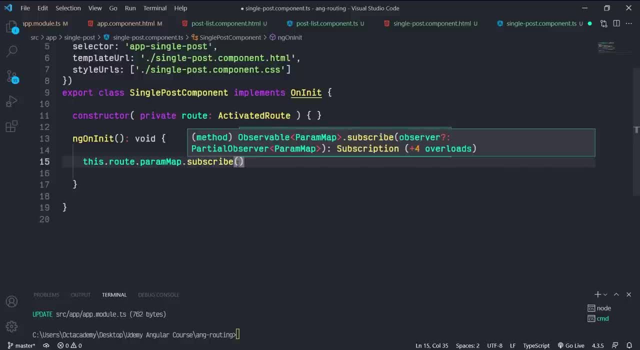 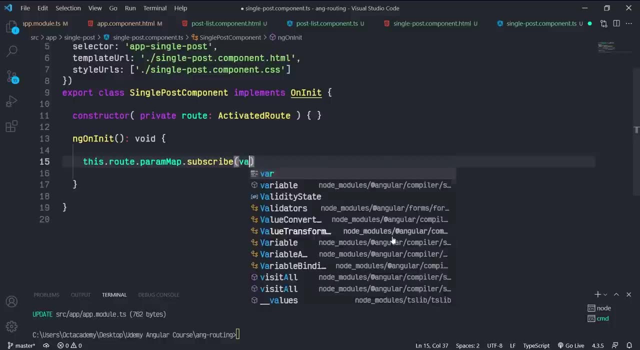 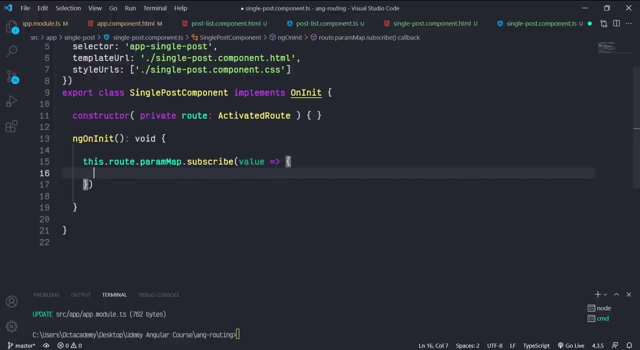 So this method required a function with value parameter, So I'm gonna define an arrow function. inside this, parentheses, The parameter name is the value arrow and the function scope. Now, inside this, let's log this value parameter and see what we got from this Consolelog and parentheses. 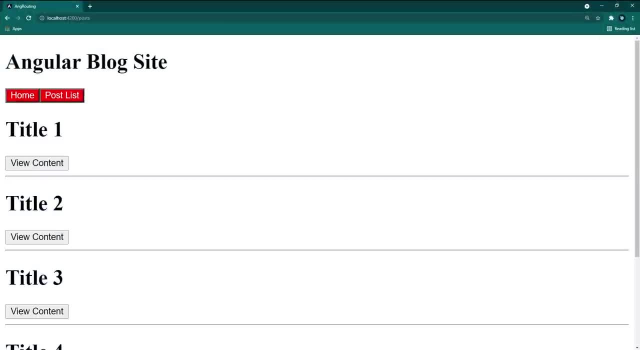 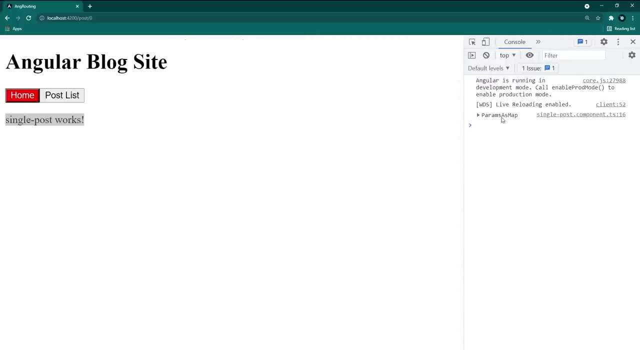 inside this parentheses: print this value: Perfect. save this and go to the browser. Click one of these view buttons. Please navigate to this url with the router parameter. Now open the browser console. Inside this, as you can see, we got this params map object. Inside that, we got these two. 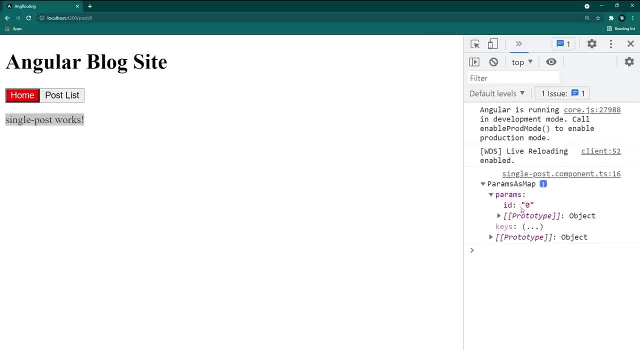 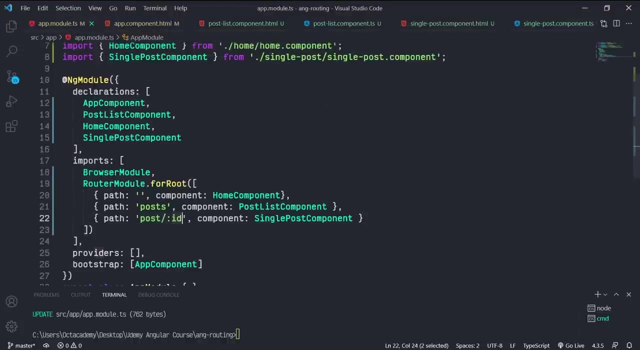 keys, Params and keys: Expand the params. Look at this, guys. Inside this param, we got the object of router parameter key and the value. This value is this router parameter. If you wonder what is this key id, which is this router parameter key? we define this when we creating this router. Perfect. 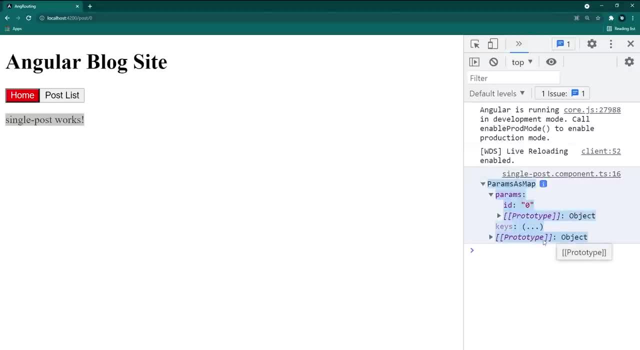 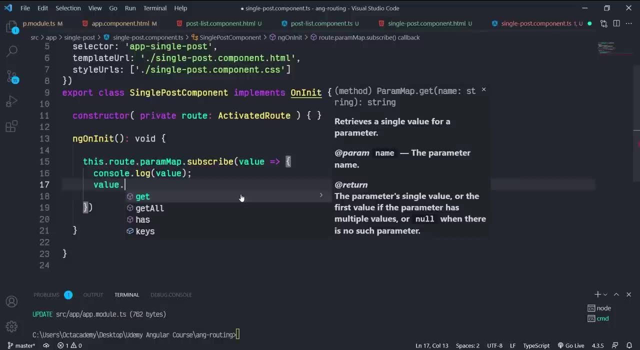 right Now we can use this params map to get the router parameter. So now, back in the video is code Value dot. look at this. We got these four methods. We can get a parameter value from this get method. We can get all the parameter values from this get all method We can check. 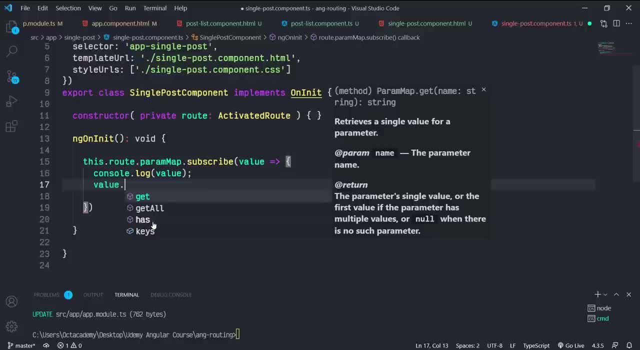 whether there is a router parameter or not with this as method. And finally, we can get a list of parameter keys with this keys method. So now we are dealing with one router parameter. So in that case we can use the get method to get the router parameter. So value dot get. 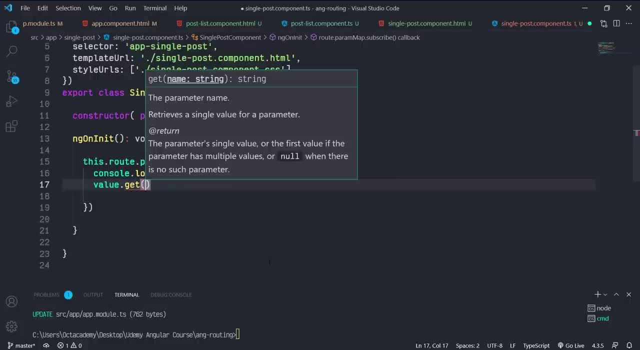 Value dot get. This is a method, So parenthesis, and this required the router parameter key. So our router parameter key is id. Pass this as a string inside quotes. Now I'm going to assign this to a variable, something let id Perfect. Now log this variable. 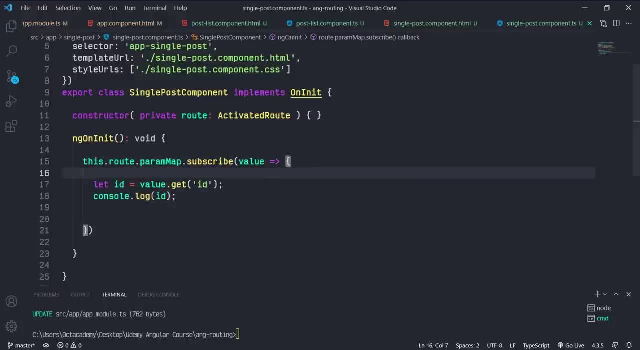 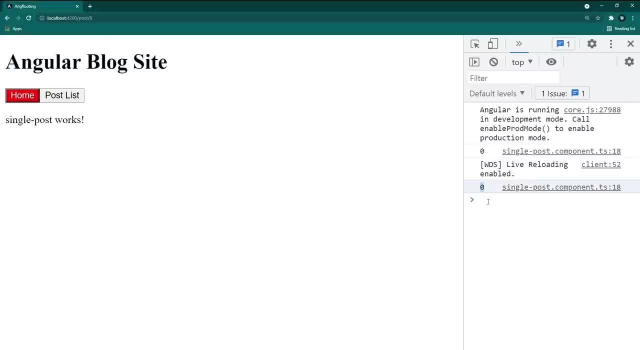 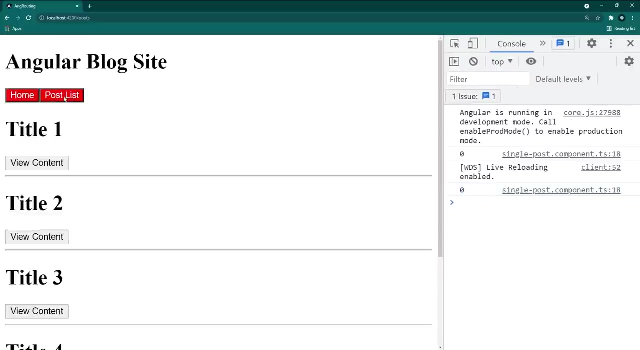 And remove this previous log. Save this all and back to the browser. Now click on this weave. Perfect, we got the index of this post printed inside the browser console. Again back to the post list component. We can navigate through the components using these. 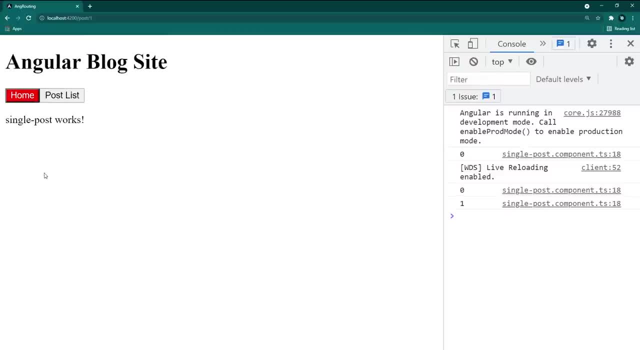 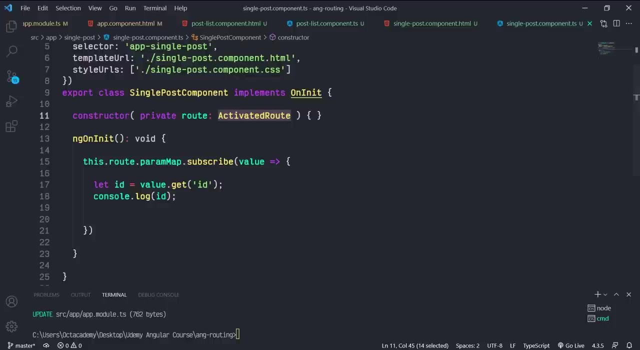 buttons Right, So again, click on this weave button. Perfect, we got the router parameter. Beautiful, isn't it? So, guys, this is how we access the router parameter parameter using the activated route module. In the previous lecture, I told you that this params map isn't observable. 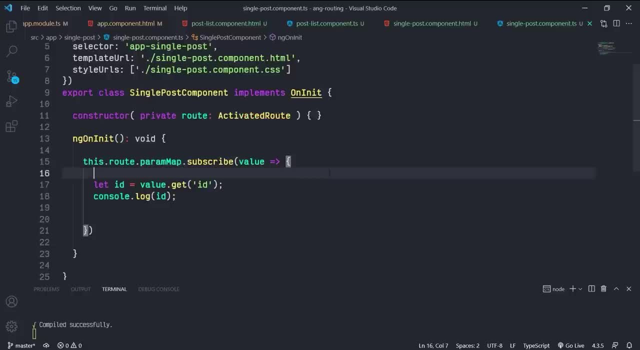 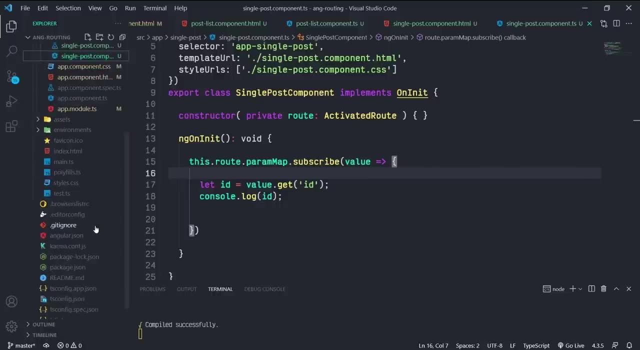 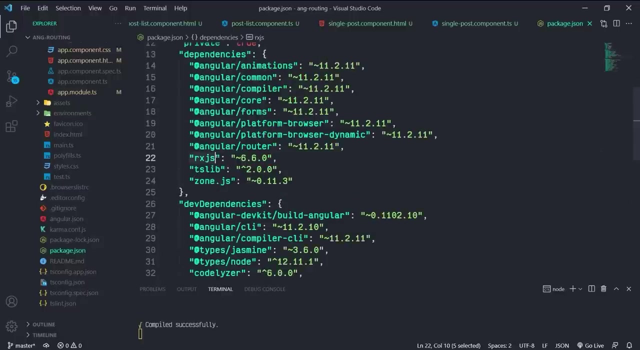 So you may wonder what is this observable? This is not an angular thing. this is coming under javascript reactive programming. In other words, this is coming from javascript rxjs. If you look at the packagejson file in here, we can find angular is using rxjs. 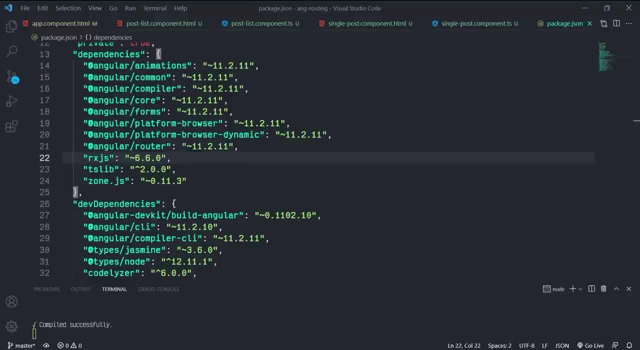 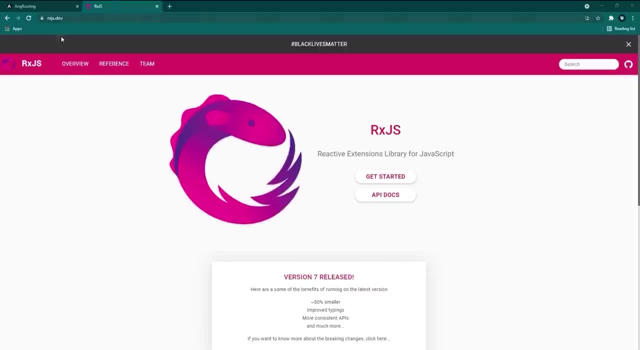 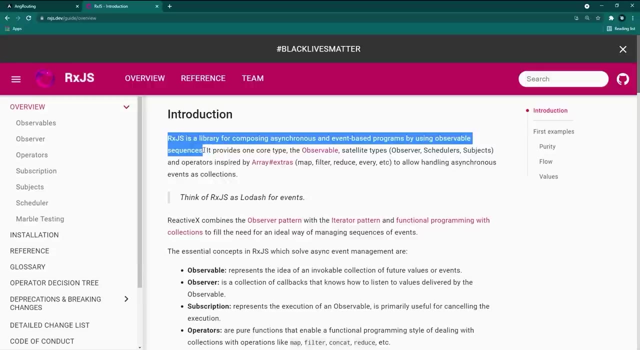 So what is this rxjs and observable? First let's go to the rxjs official website, rxjsdev. Go to this overview tab. So this is a library for composing asynchronous and event based programs By using observable sequences. So what is this observable? 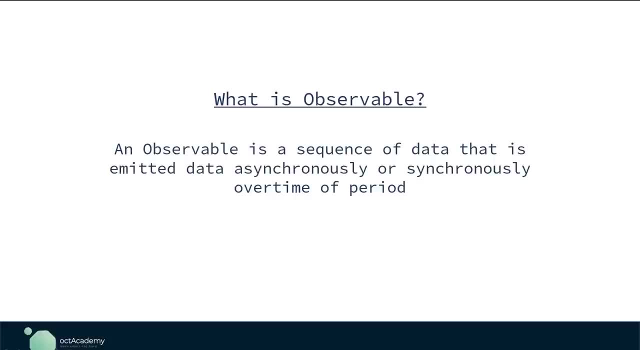 An observable is a sequence of data that is emitted asynchronously or synchronously over a period of time. In other words, observable will continuously observe a set of stream data and automatically update or track that sequence of data whenever there is something changed. So let's see an example. 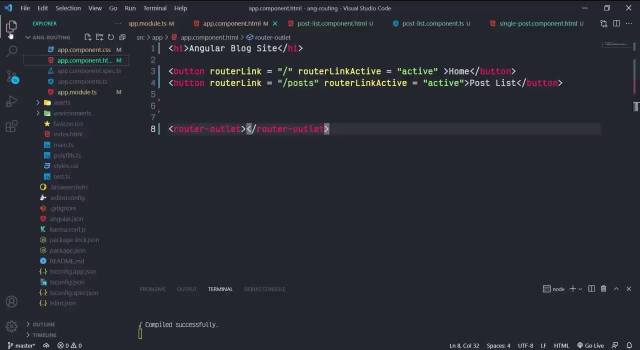 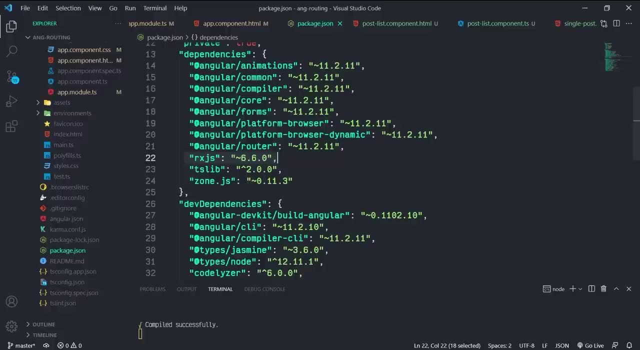 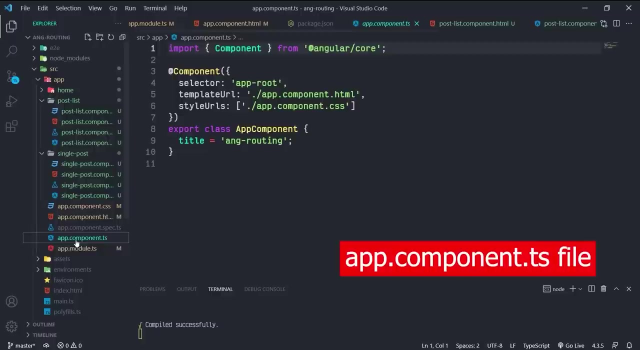 Then we can understand this correctly. As I mentioned earlier, angular is using the rxjs library out of the box. So we can use the rxjs observable with an angular project. So let's see a simple example. So let's do this inside the home componentts file. 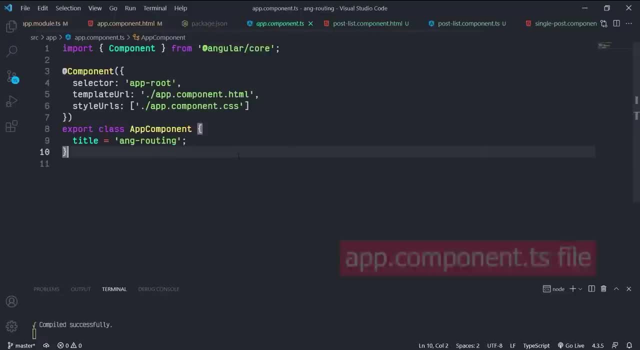 This is just an example, so that's why I am doing this inside the home component. There is no mandatory requirement to do this. You can do this any of the component files, as you wish. So in order to work with observables, We have to import the observable to this component file. 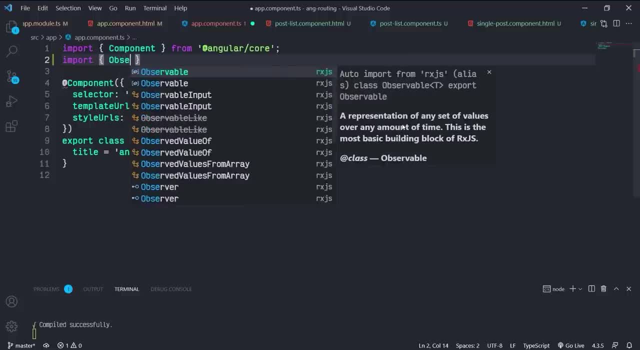 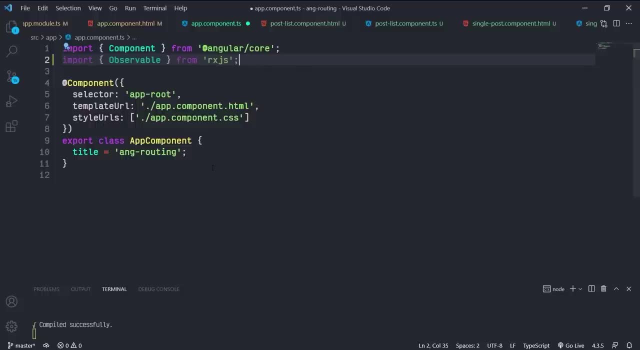 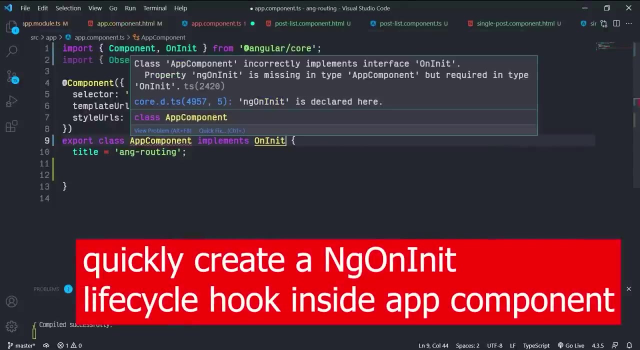 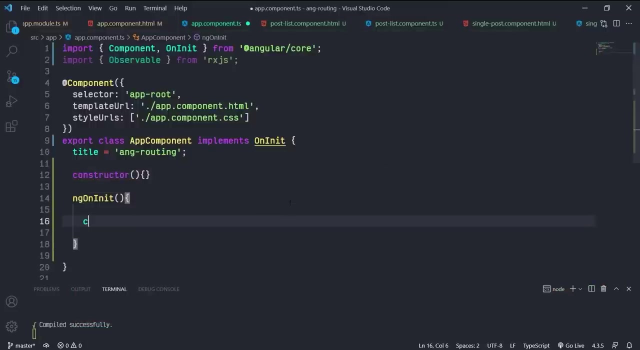 So import inside curly brackets: observable: this o must be capital from. this is coming from the rxjs library. that's it. So now let's create a new observable. So insert the ngOnIt method, Create a variable, Something const OBS, test, And at the end of this variable name just add an dollar symbol. 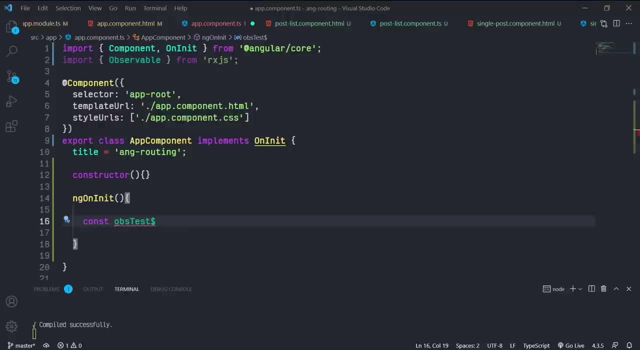 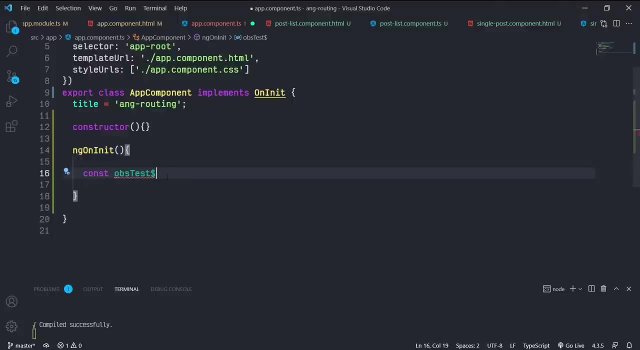 So usually we create observable variable something like this: This is just a naming convention. With this we can easily identify the observable variables. So this is not a mandatory requirement. This is just a naming convention. All right, after this: equal sign: new observable. 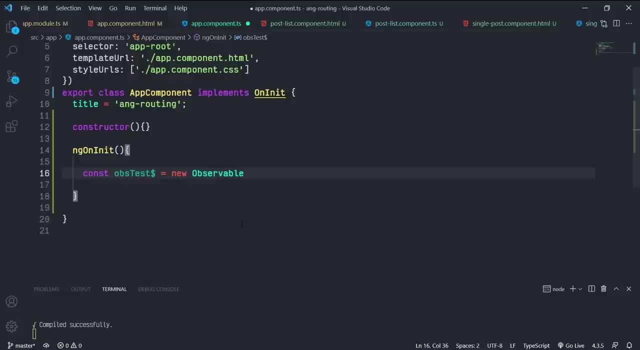 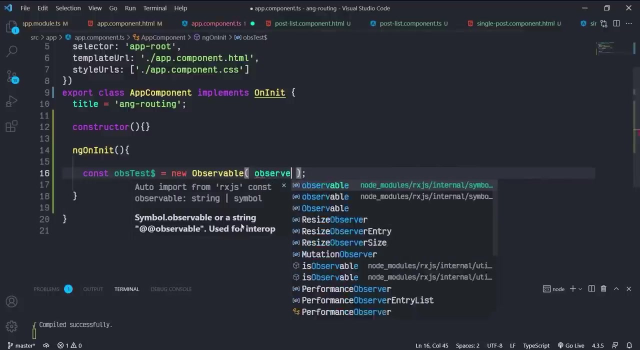 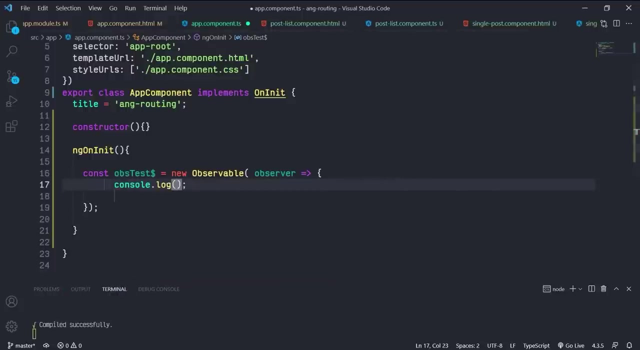 With this we are creating a new instance Of the observable class. So after this, add the parenthesis. Now this observable required an observer function as a parameter. So inside this parenthesis, let's create an arrow function: observer and arrow function. Now, inside this function, simply log this console dot log inside brackets, printed from observable: 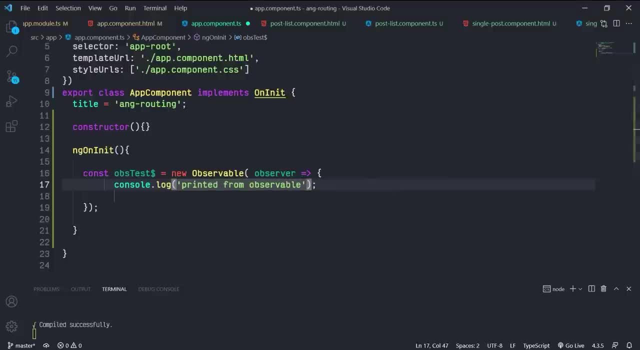 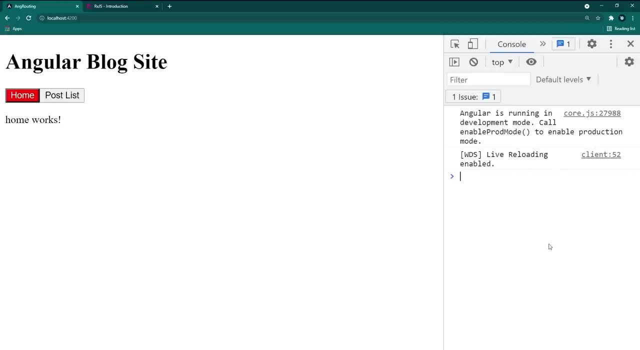 Perfect, Now save this And back to the browser. We are now inside the home component, So now look inside the browser console. We got nothing. We supposed to get this log printed inside the log, But we got nothing. In order to use an observable, we must subscribe to that observable. 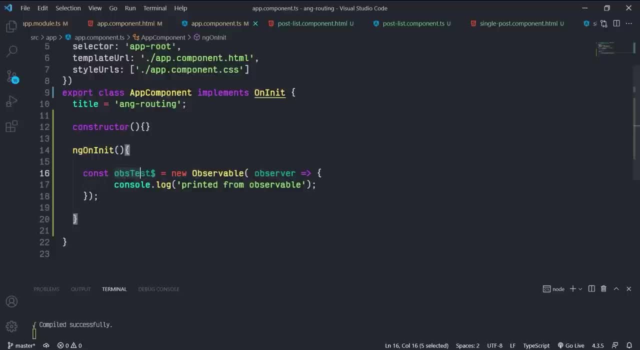 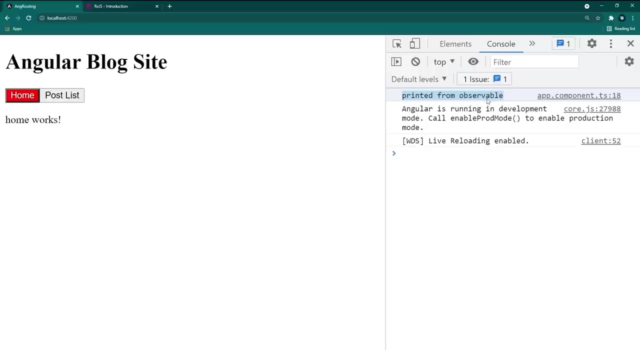 So let's do this. After this, we assign this observable to this obs test with the dollar sign. So dot, subscribe and parenthesis Ok, Now save this and back to the browser. Look inside the browser console, As you can see here. We got this log printed here. 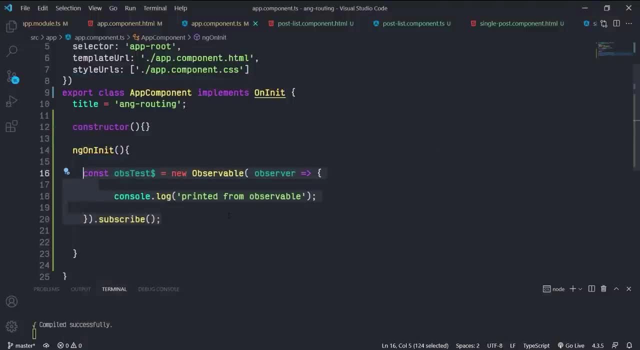 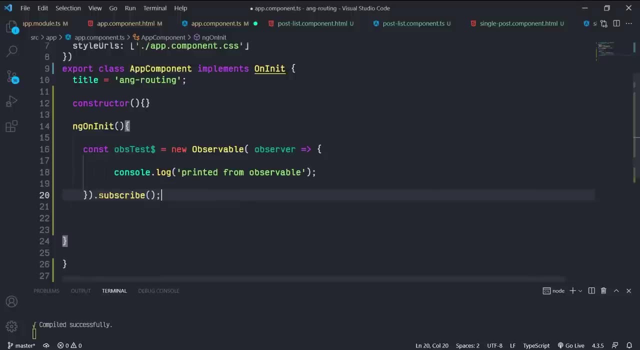 So this is how we create and access an observable. So you guys may wonder what is this subscribe and how this works. This is nothing fancy. I'll explain this with a simple example. This observable also like a jigsaw. It's a simple example. 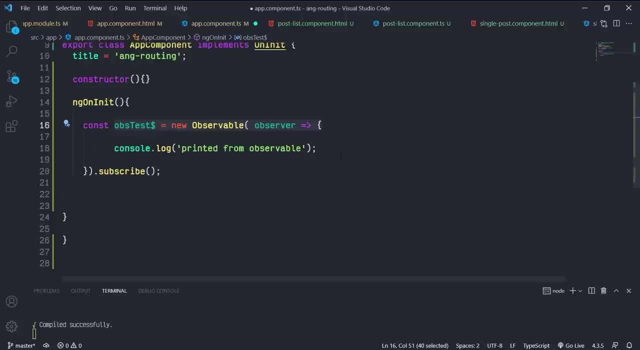 This observable also like a jigsaw, It's basically a javascript function that has some more additional features than the traditional javascript functions. Simply, let's create a simple function, const obs test, This time without the dollar symbol, coz. this is not an observable. 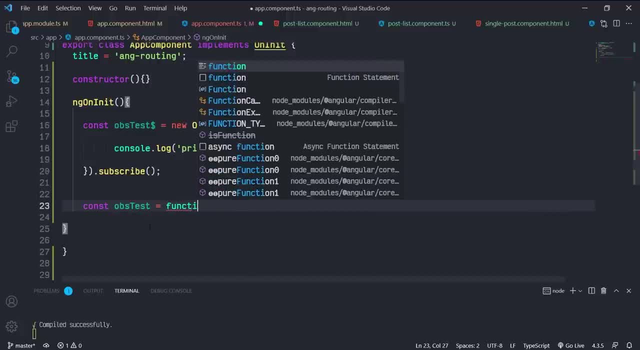 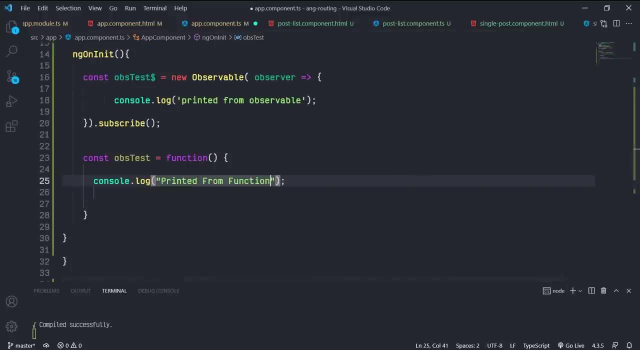 After this, assign this to a simple function: Function: scope. Inside this let's log something Uhm Printed from function. So in order to access this function, as you guys already know, we have to call this function. So after this, let's call this: the function name is this: OBS test, and parentheses. 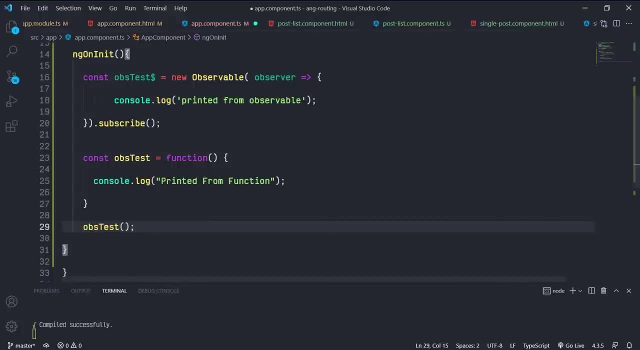 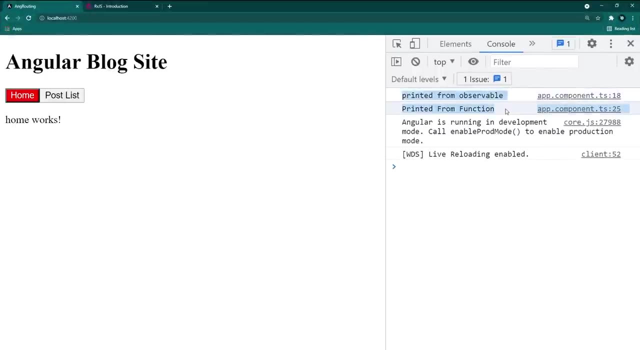 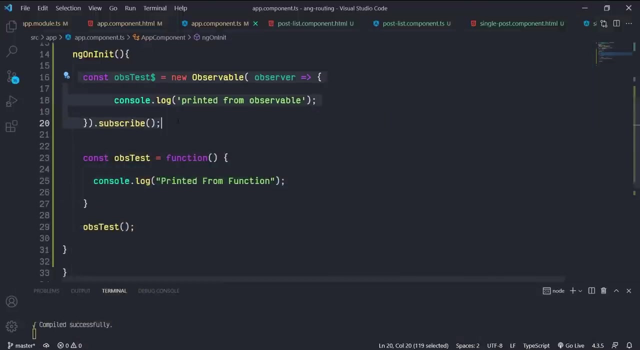 So this is how we call a JavaScript function, right? So save this and back to the browser. Look at this. we got these two logs: one is from the observable and the other one is from the function. So, guys, as I said earlier, observable, also kind of a JavaScript function. 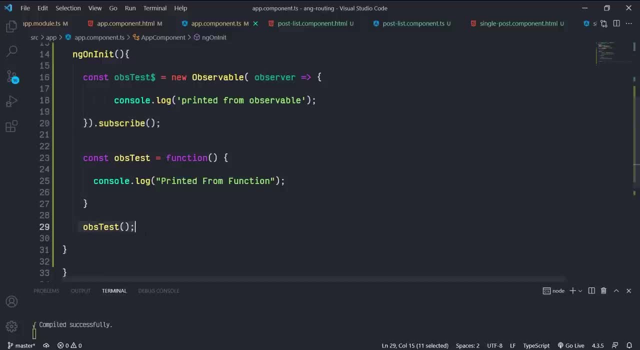 In order to execute a JavaScript function, we must call that function. The same thing applies for the observable as well. So we call a function like this, but we call an observable with the subscribe method. So this is what we're doing with this subscribe method. 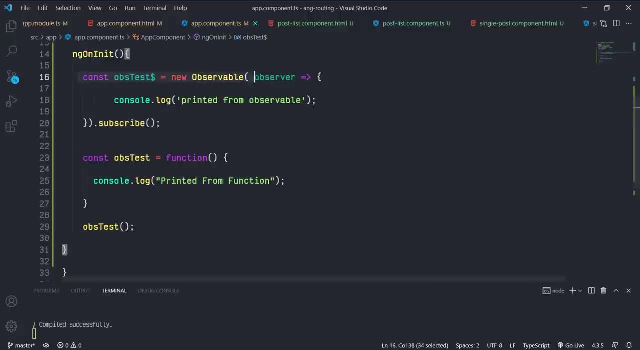 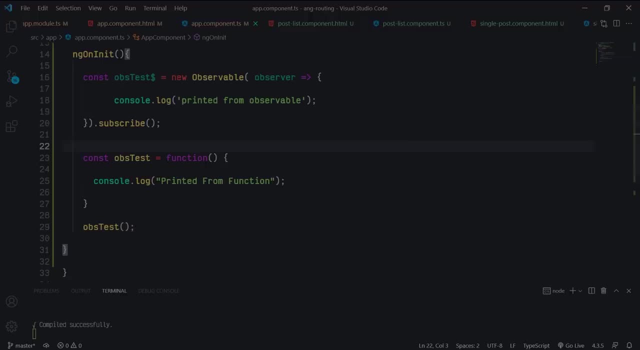 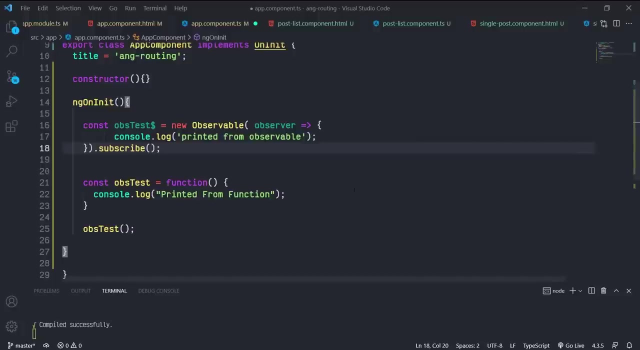 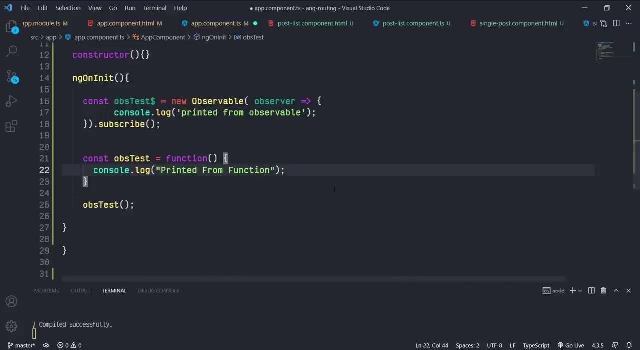 Nothing fancy, very simple. So with the subscriber, We are calling this observable, like this function calling Hope. you guys got the idea In a traditional JavaScript function. if you want to return something, we will return that using the return statement, something like this: return keyword and let's return a string. 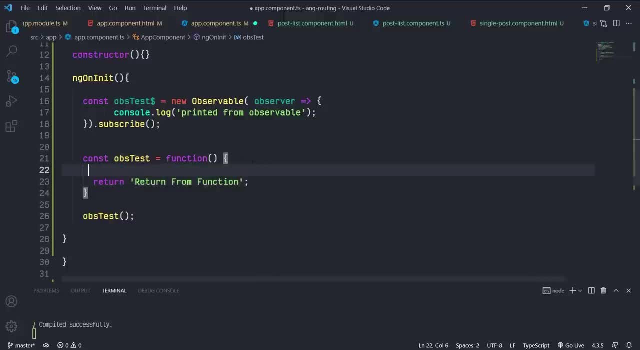 something returned from the function. Remove this log. We don't need that anymore. We can capture functions returns, something like this: Assign a variable to this function, call const return data. Now let's log this after this function call. Save this and back to the browser. 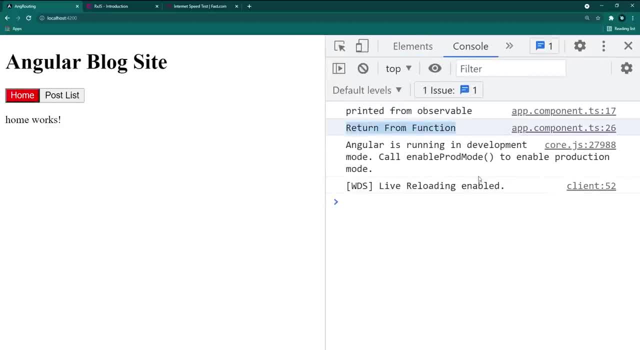 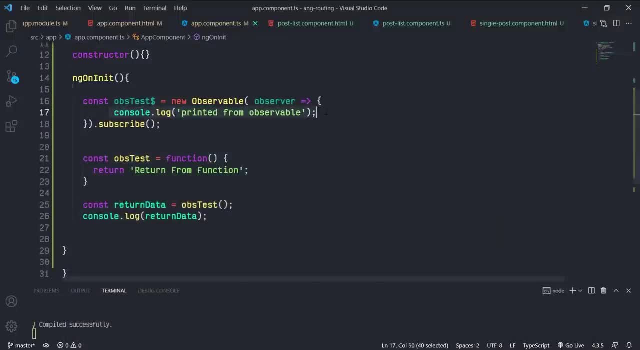 As you can see here, we got this return value printed here In observable. We have a different approach to return values, So let's see that in action. So remove this log. We don't need that. Like this return statement, we have next statement in observable. 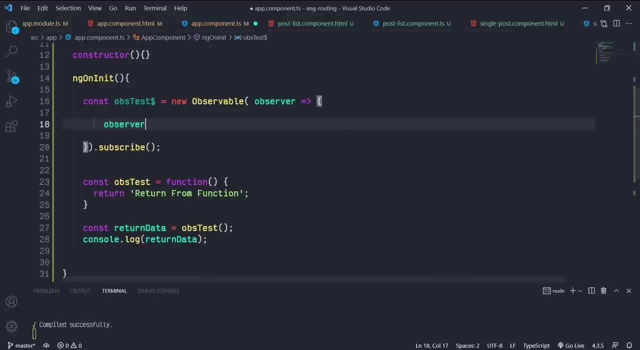 So this callback function, which is this observer dot- next inside parenthesis- we can pass the value that we want to return. So let's pass a string value returned from observable. So this is how we return something, Something from observable. Now we have to capture that returning value from this subscribe method. 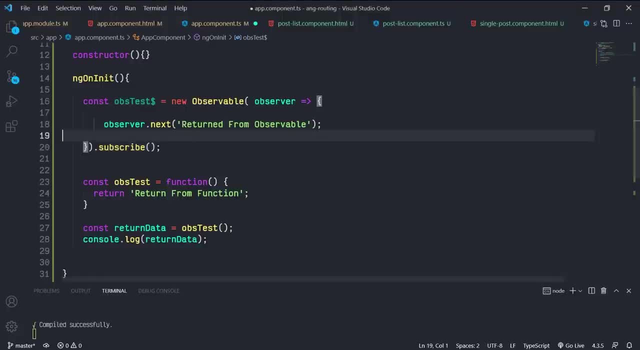 So we captured the returning value, something like this for JavaScript functions, But for observables we have a different approach, So let's do that with the subscriber. We can capture the returning value something like this inside the subscribe parenthesis: Create an arrow function. 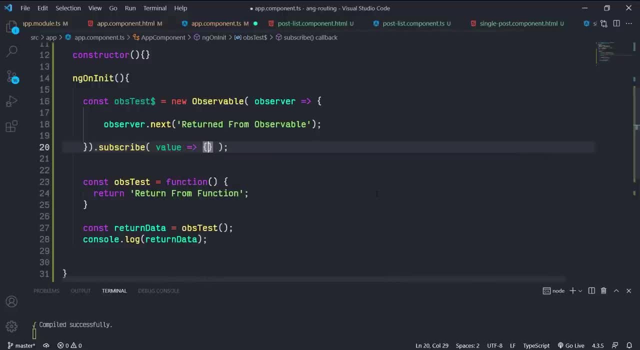 Value arrow and the function scope. with this value parameter we will get all the returning values from the observable. So insert this function, log this value parameter. That's it. Save this and back to the browser. Look at this. We got this log. 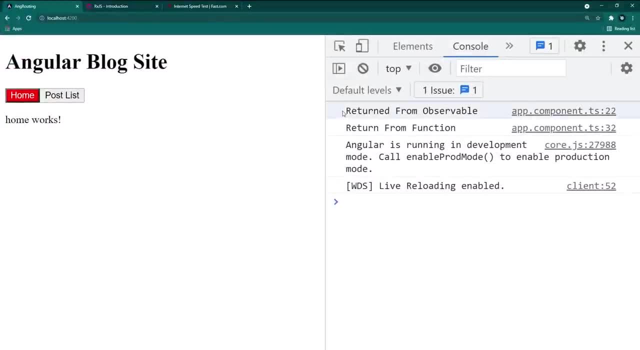 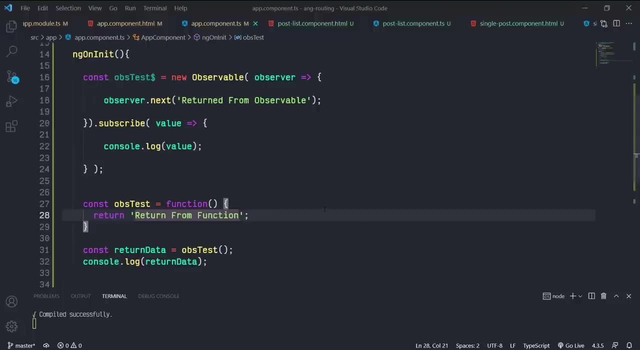 Perfect right. So, guys, this is how we return a value from an observable using the next observer method. Some of you may wonder that we are doing the same thing with the observable and this function. What is the difference And what is the use of this observable? 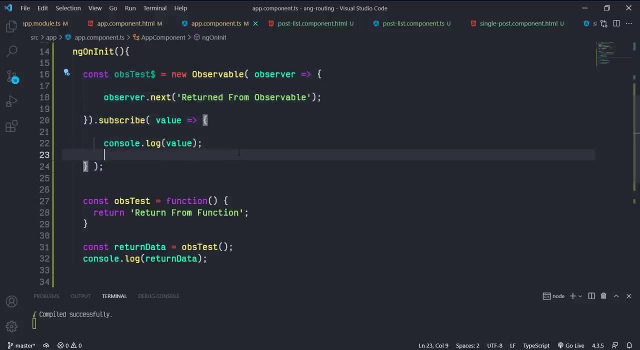 So we'll see this in detail about this in this lecture With this function. we returned this statement. In case, if you want to return another statement, you can return this statement. So we can return this statement. So we can return this statement. 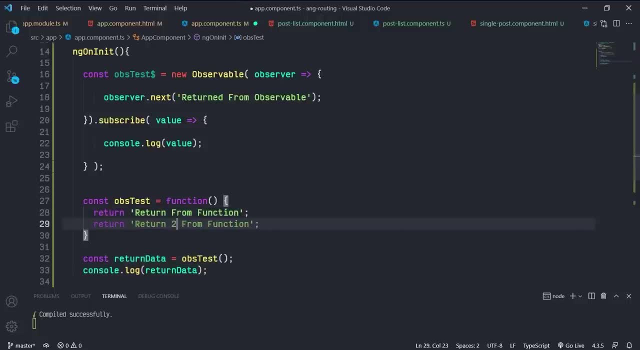 How do we do that? In traditional JavaScript functions, we cannot return another statement like this. This won't work. When we call this function, this method will execute until this first return. After this, this function will stop executing and move forward. 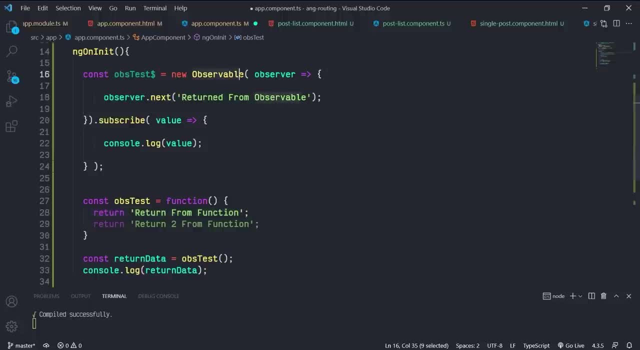 But in observable we can return as many data as we want. So let's see this in action. As you know, we return something from an observable Using this next method. So again, after this, this observernext, inside the parentheses- let's pass something. 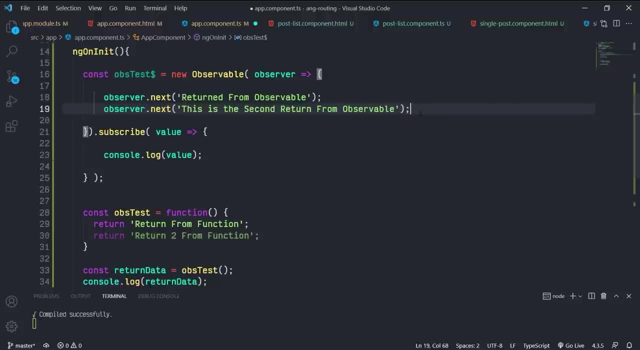 This is the second statement. If we need another data to return, we can again call the next method. This is third statement. Like this, we can return data as much as we needed from this observable. So now save this and back to the browser. 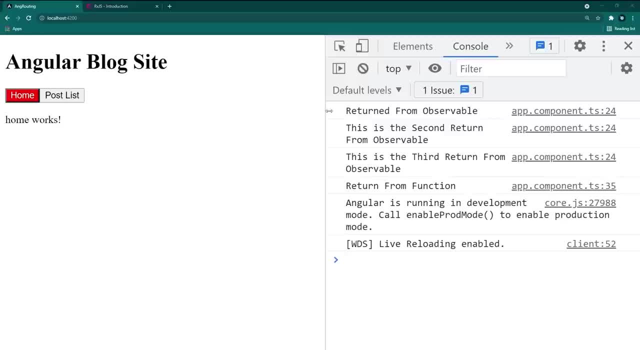 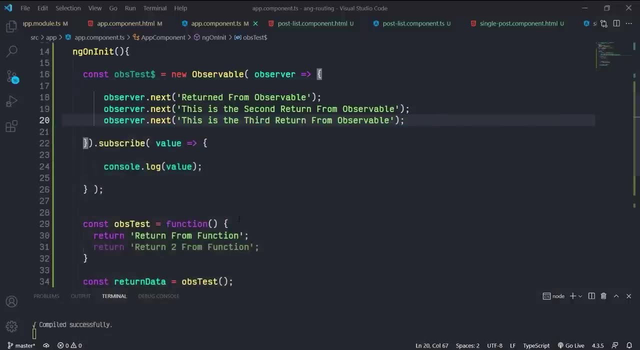 Look at the console. We got all the data. We got all these three statements printed here, But, as you can see, we got all three statements printed from the observable, But in the console we got only this first return statement from the JavaScript function. 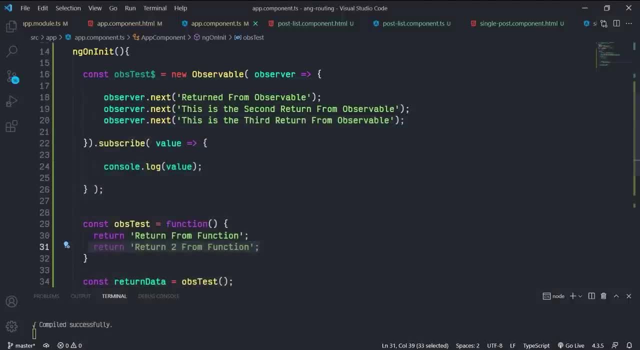 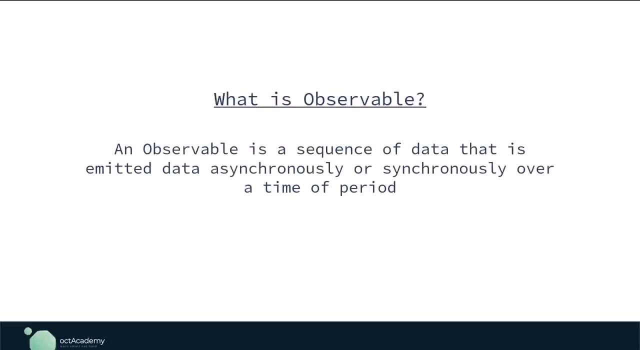 So we didn't get the second return statement. So this is the main difference between observable and the JavaScript functions. So with this observable next method, we can return data as much as we needed. So this is what I tried to say with this observable definition. 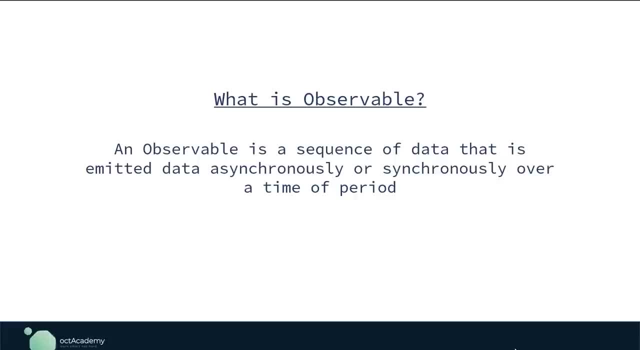 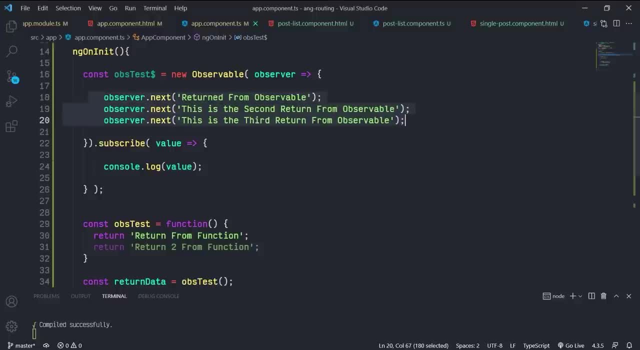 An observable is a sequence of data that is emitted asynchronously or synchronously over a period of time. This is the sequence of data that is emitted or returned over a period of time. So with this observable, we are returning multiple data with this next method, over a 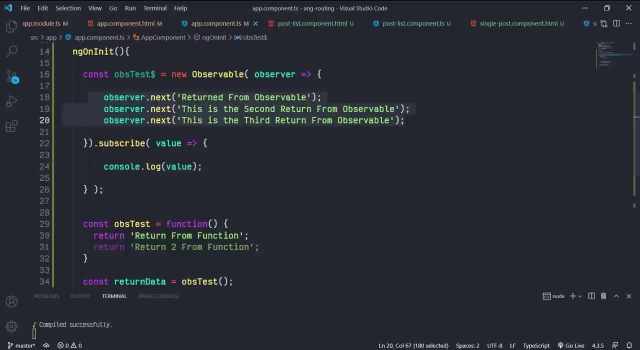 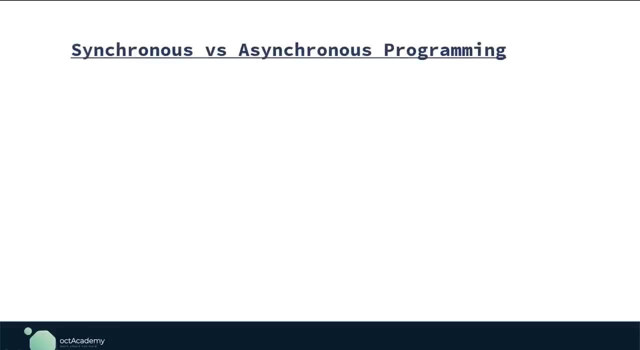 period of time. So hope you guys got the idea. What is this? asynchronous and synchronous programming. Synchronous code is executed in sequence. Each statement waits for the previous statement to finish. before executing Asynchronous code doesn't have to wait to execute the previous code completely. 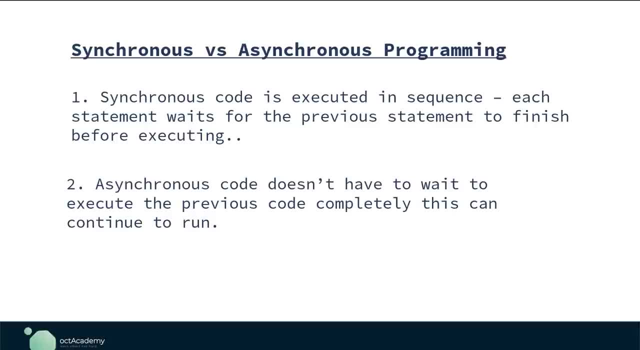 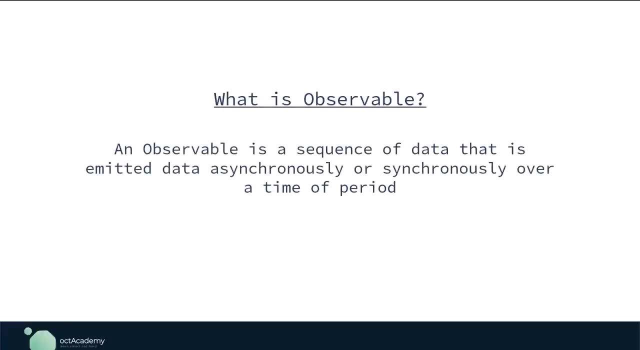 This can continue to run. So we do this to keep our site or the app responsive, Reducing waiting time for the user. So mostly JavaScript works as a synchronously when we're learning observable that I said observable is a sequence of data that is emitted asynchronously or synchronously over a period. 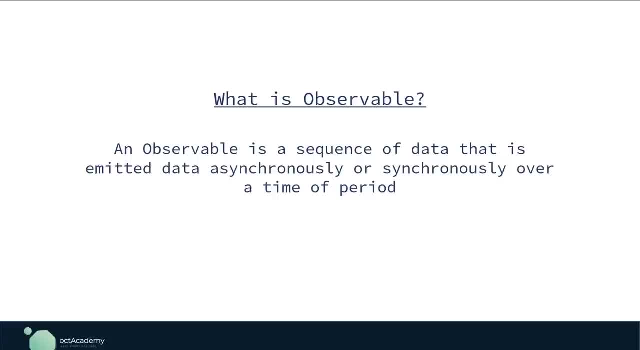 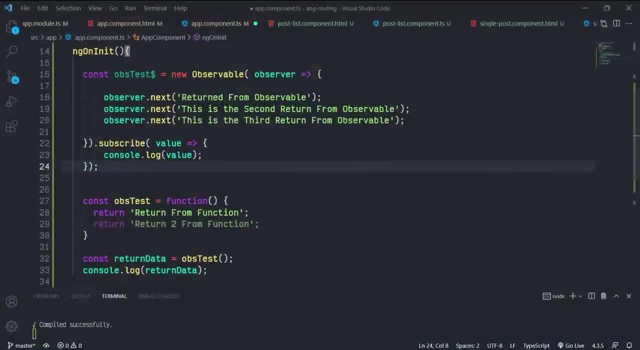 of time, So we can use the observable asynchronously or synchronously. So let's see this in action, So we can take this previous example for synchronous programming When this observable executes. So let's see this in action, So this will execute. 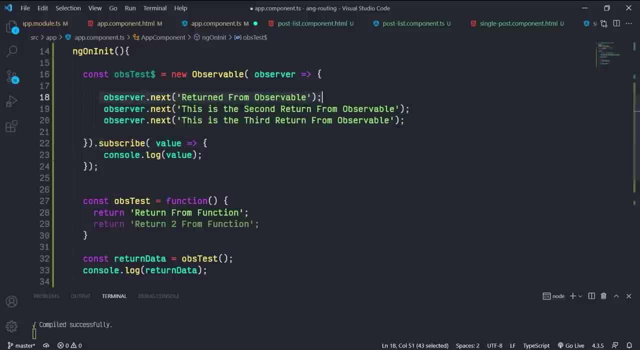 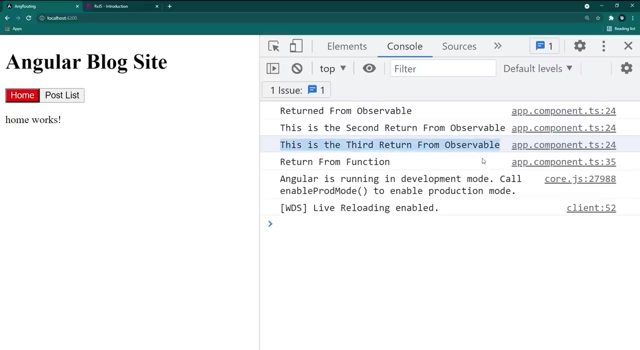 First, this will execute this next. After that, this will print this second next. After that, this will print this third next. So let's look at this in the browser. As you can see here, this printed one by one in correct order. So this is what synchronous programming. 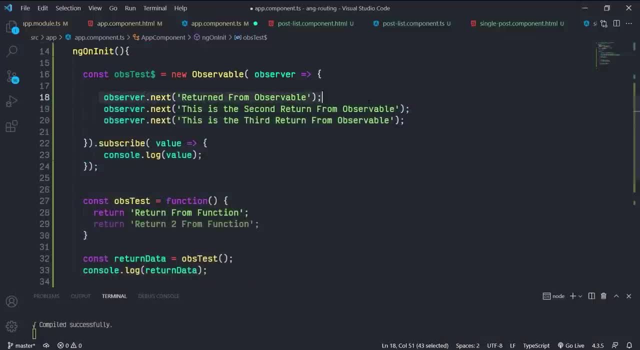 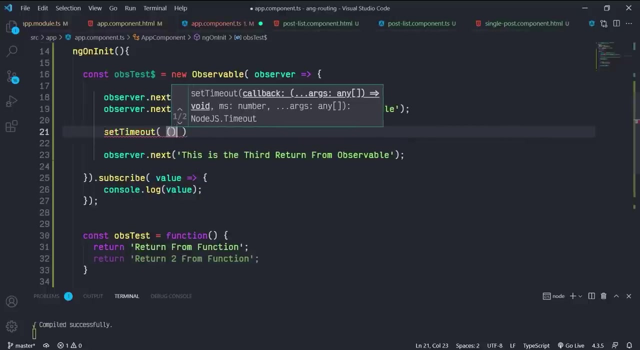 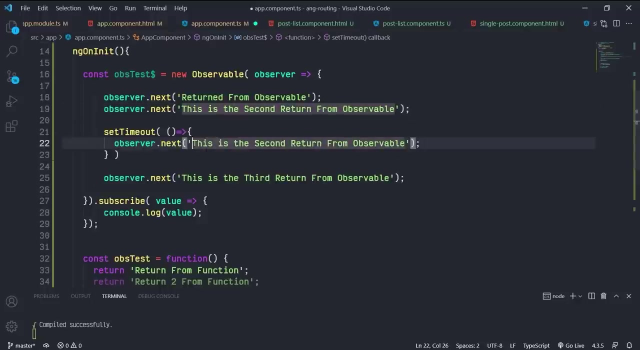 This code is executed in sequence. Each statement waits to finish. the previous statement Got it. Now let's add a timeout function between these. So set timeout Inside parenthesis arrow function and inside this function let's add another. next something: timeout, At last. set this time to 2000 milliseconds. 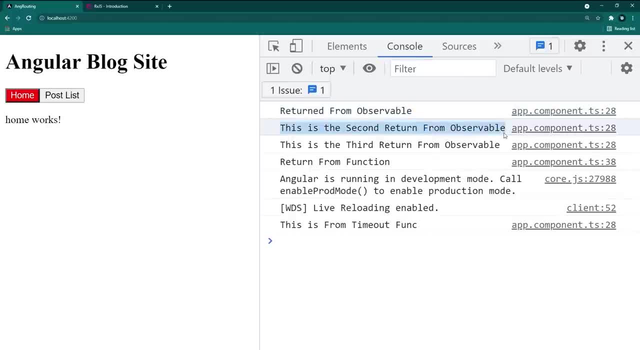 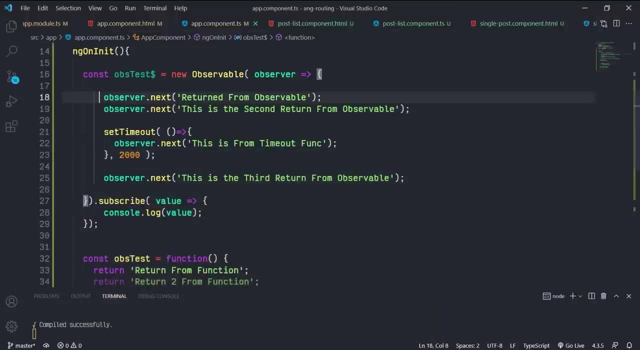 So, if you look at this inside the browser, This printer Printed first, second and third observable outputs. After two seconds, this printed this timeout Which, coming from this timeout, function. What's going on here Back in the VSCode When we run this inside the browser? 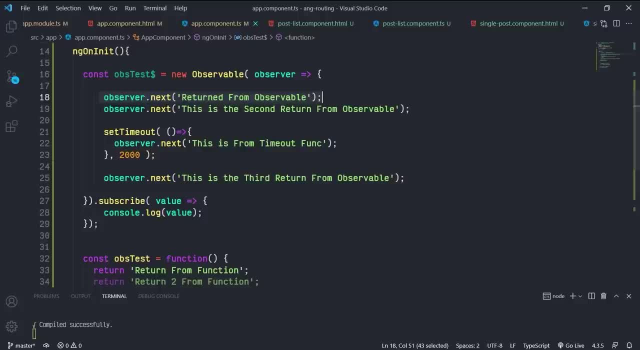 The browser will first execute this And return this value. Next, this, move on to the second line and return this. After this, This will execute this timeout function And this will move on to the next line. This not wait until this code fully executed. 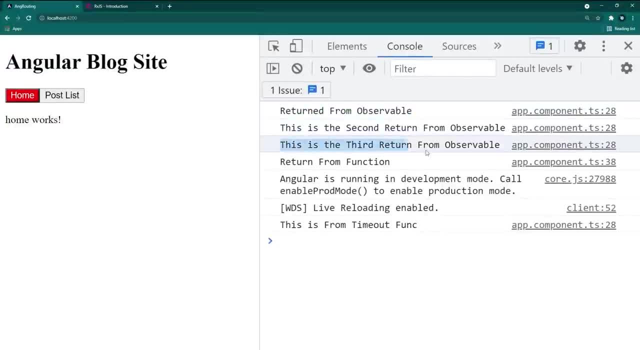 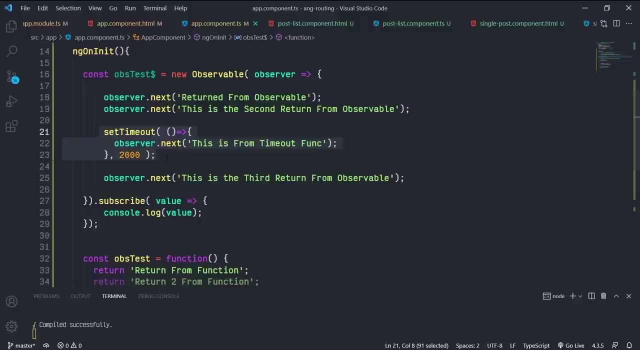 So that's why we got this first, second and third outputs printed here And at last, we got this timeout printed here. So this is what we call asynchronous programming. With this, user doesn't have to wait until this complete. Once this completed, User will get this. 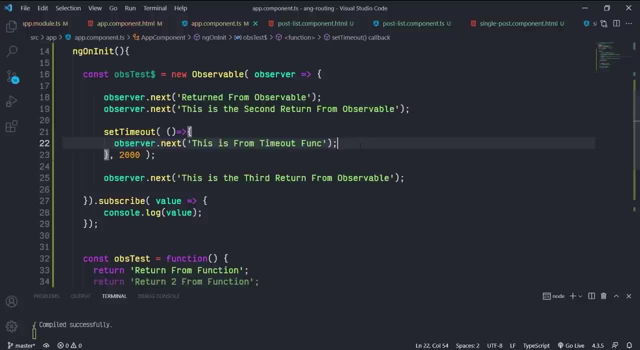 This is the timeout. This is data. This is one of the beauties of javascript: asynchronous programming, So we can use this observable for synchronous and asynchronous situations. But mostly we use this observable for asynchronous situations When we pulling data from the database. 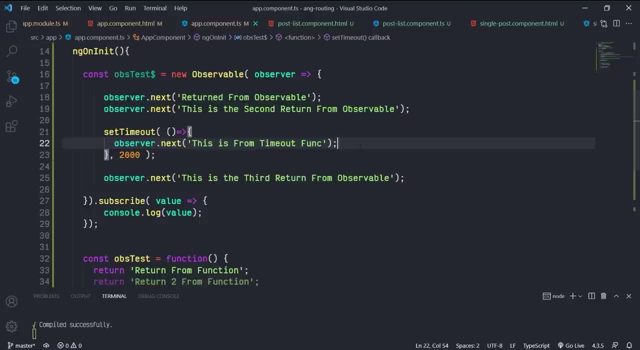 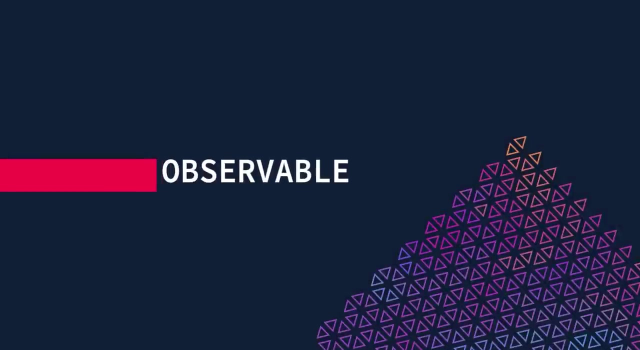 Sometimes this will take several seconds To communicate to the database server. In that case, with this asynchronous approach, we don't need to wait until the server responds With the data. Once we got the data, we can show that immediately on our app With the observables. 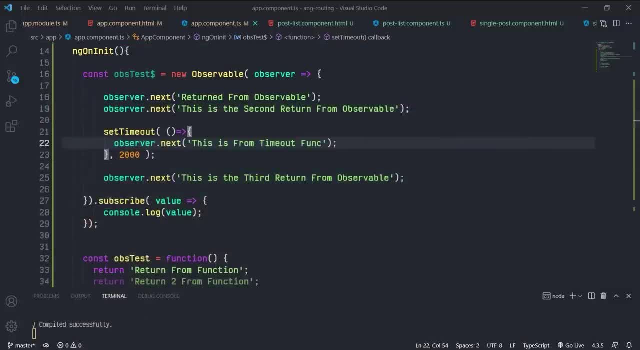 So i hope you guys now have a clear idea about the observable. So in this lecture lets look at some observable methods and how to use them. So first lets look at the method of using observable. First lets learn about this method, the subscribe method. If you can remember, I told you earlier this also something. 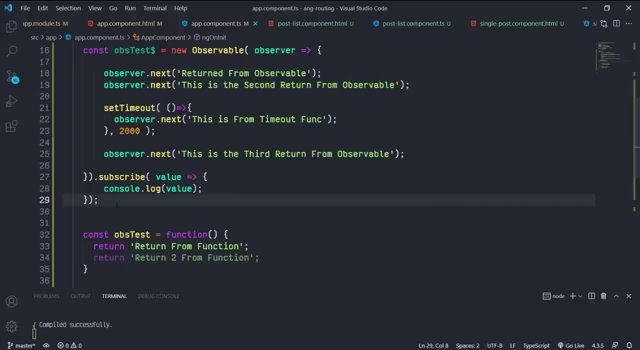 like method of functions calling. Yes, it's correct, but this is a bit different than the traditional method calling. When we subscribe to an observable, this will create something like connection bridge between this call and this observable Whenever there is any change happen inside the observable. 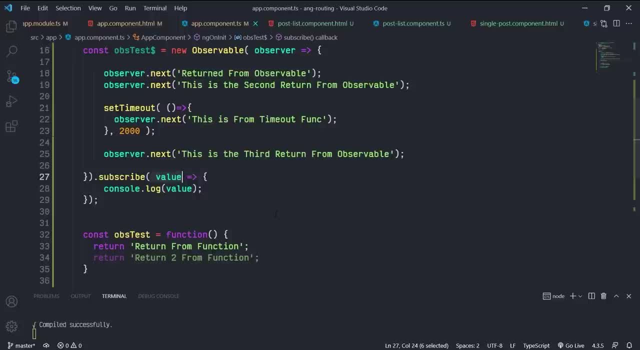 this subscribe method will trigger again and emit that new data to this value. So, as I mentioned earlier, this will always listen to the observable and whenever there is anything happens, this will automatically get that from the observable. We can get the same example as the previous When we subscribe to. 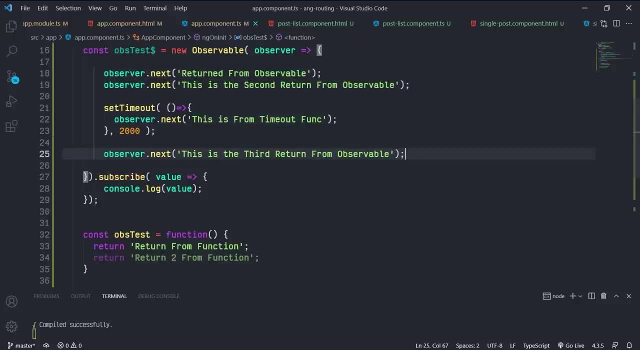 this observable. we get these values After two seconds again. we got this time out inside the observable With this timeout. we return another value again with this next method. So on that time a change is taking place inside this observable, right. So therefore this subscriber method will trigger again and printed. 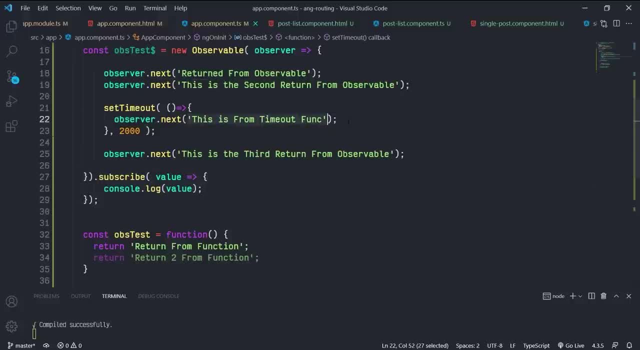 this value inside the console after this timeout. So this is how this subscriber method works. Another thing, if you can remember that I said, the subscriber will continuously watch the data of this observable. Now we have subscribed to this, So keeping this subscribe open all the time is not a good practice In a real-world. 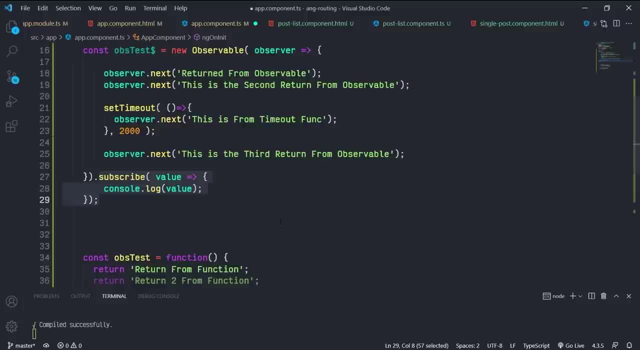 applications. we connect to the database from an API and almost every that connection returns the data as an observable. So always keeping this observable subscription can cost memory a lot and can be slow the application. So this is not a good practice. So we can close this subscription using the unsubscribe method. Very simple, Same like this: 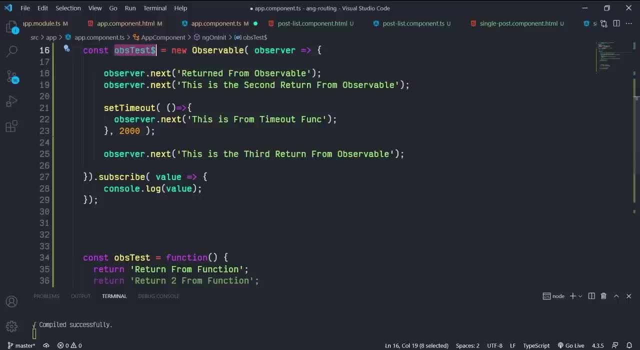 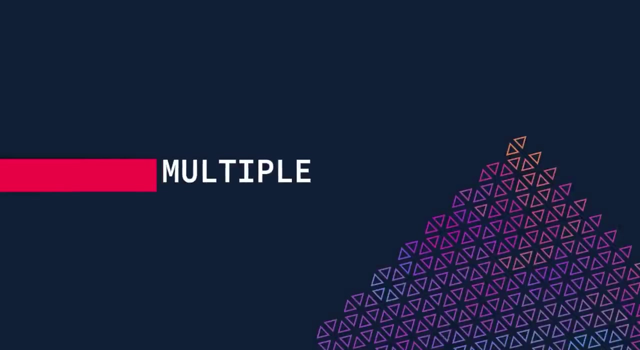 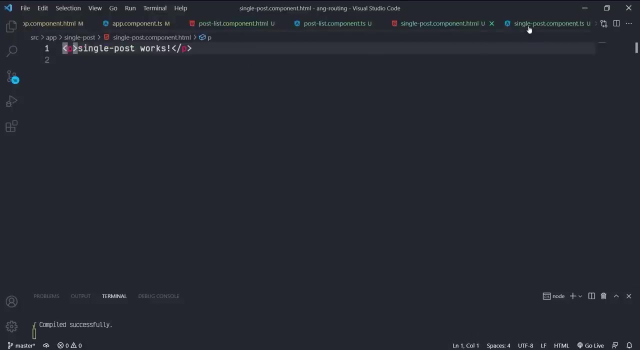 subscribe. oh so the observable is this OBS test with the dollar sign symbol, After this dot and unsubscribe and the parentheses. And's it very simple: Rt …. lecture. we learned how to pass a router parameter and how to capture that parameter, and also we 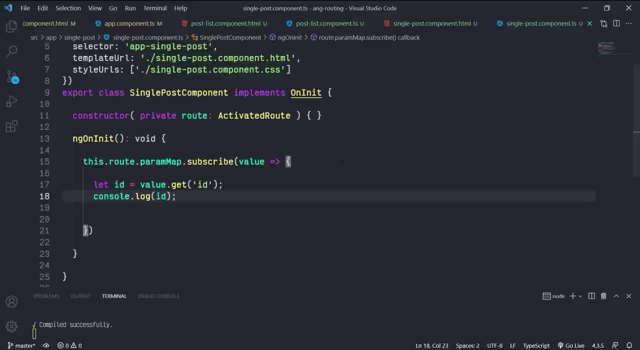 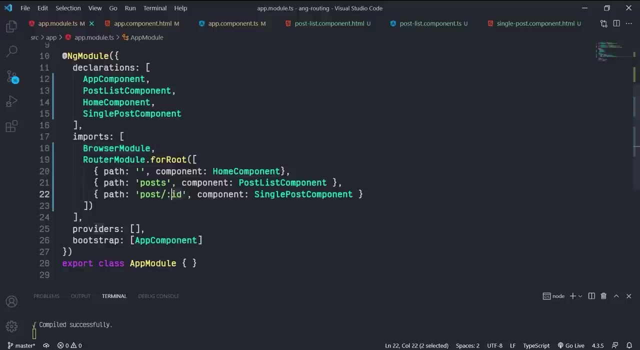 learned about rxjs observables. Hope you guys now have an idea about this observable. Alright, let's move on. So in this lecture let's see how to pass multiple router parameters. In some cases we may have to pass multiple router parameters to create SEO friendly URLs. In previous, we sent only the 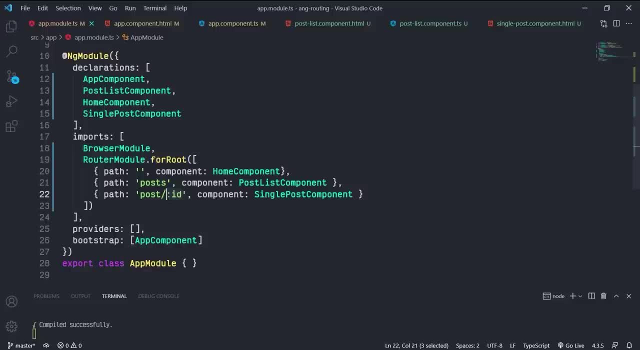 id of the array. Now let's see how to send another parameter Inside the app module ts file. inside this. this also same as this: just after this id parameter, define another parameter: Slash. we defined router parameter variables with this colon sign, So colon With this, let's. 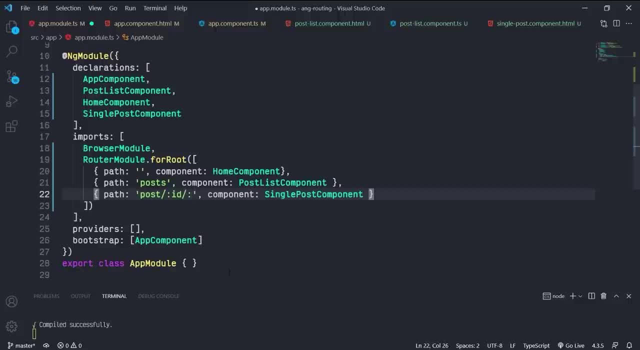 pass the post title right. So the parameter variable is something title Perfect. We have successfully defined the router parameter variable. Next let's see how to pass the router parameter value to this URL. So inside this post list component ts file, we sending the id router. 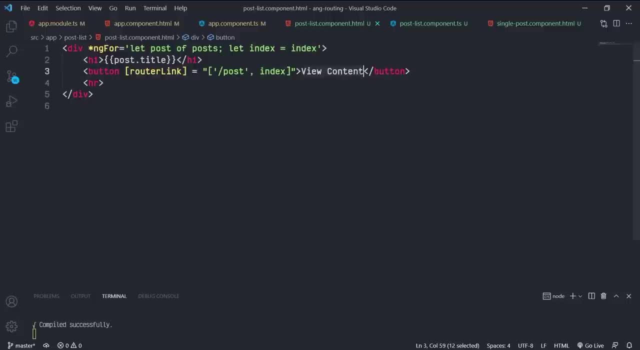 parameter with this weave button. So like this, we can send another parameter. So after this comma, and this time we are sending the post title, So post dot title. Perfect, Now save this and back to the browser. Go to the post list and click one of these weave. 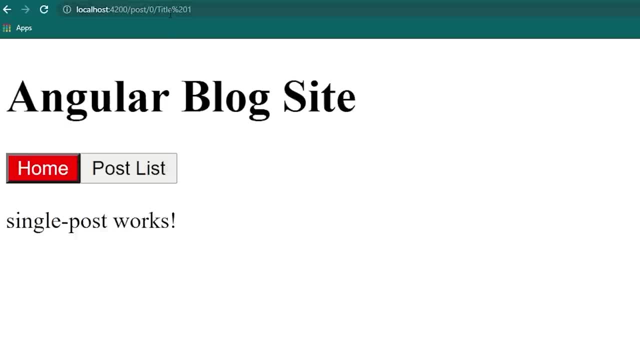 buttons. As you can see here, we got this id and the post title inside the browser URL. Some of you may wonder: what is this percentage sign and this? this number two and zero? A URL cannot include spaces, So when there are spaces, the browser will automatically prefix these spaces with this. 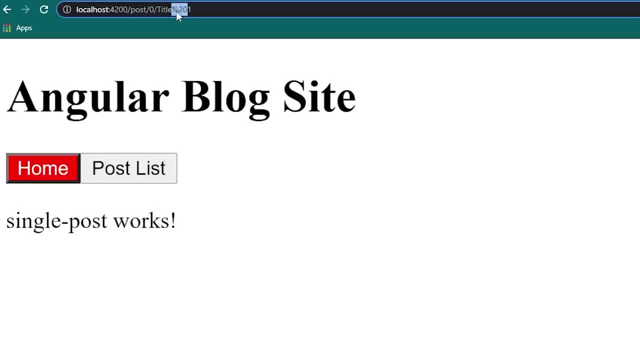 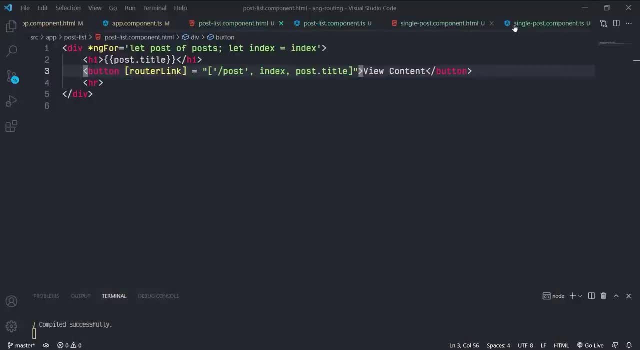 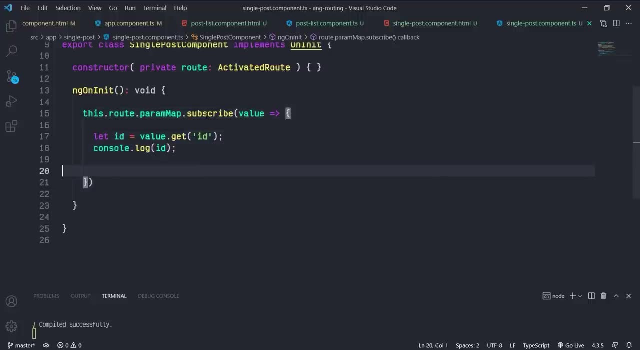 integer and two and zero. So this is what we got here. Now let's see how to get this router parameter from this single post component For the single post component ts file. Very simple. This also same as previous. We already subscribed to the params map, So inside this same subscribe. 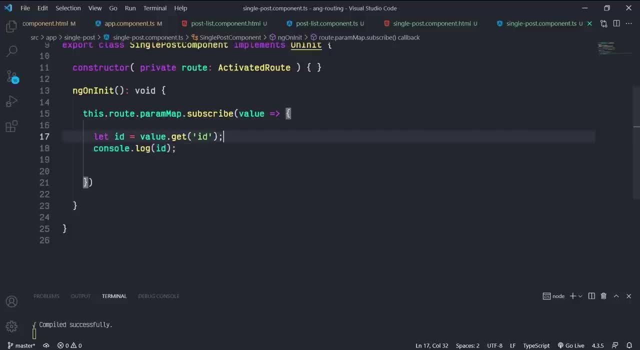 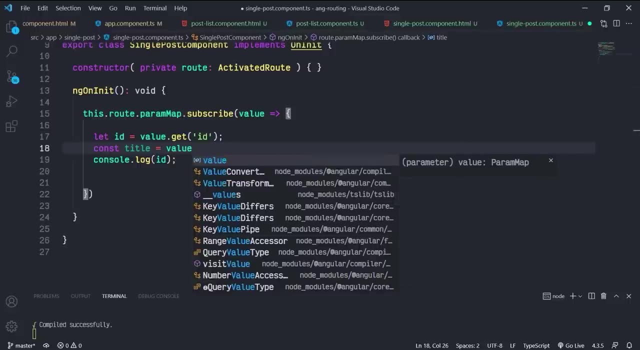 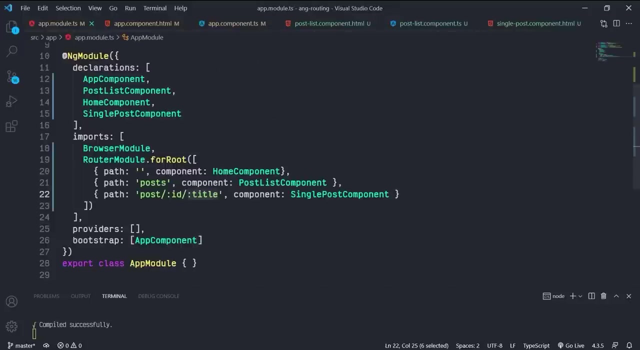 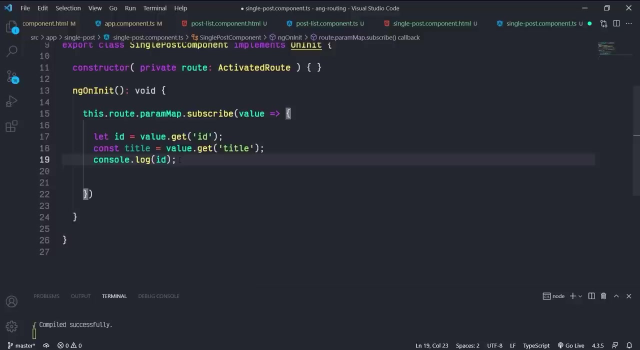 method we can get the parameter like this: id parameter, Const title assign Well, which is this: subscribe variable dot. get inside brackets. pass the router parameter variable name, which is the title. That's it Now. simply log this title, Save this and back to the browser. 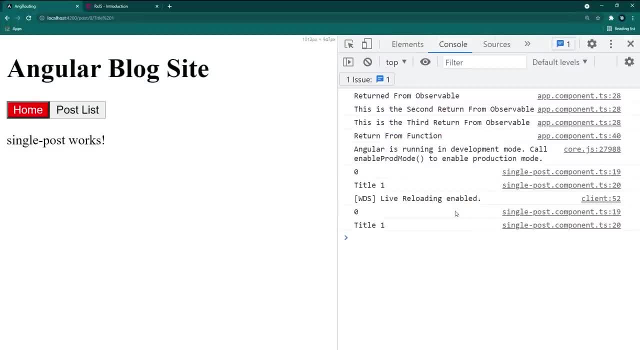 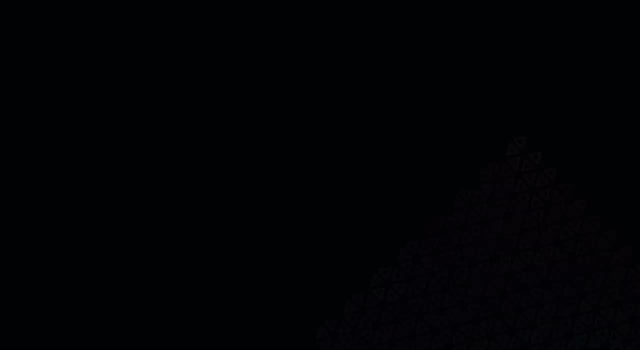 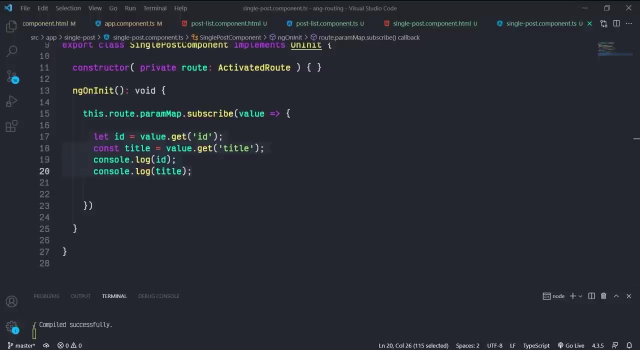 Now look at the console. Perfect, As you can see here, we got this title router parameter printed here. Awesome, right? So, guys, this is how we deal with multiple router parameters in angular. So until now we learned about router parameters. Now in this lecture, let's look at how. 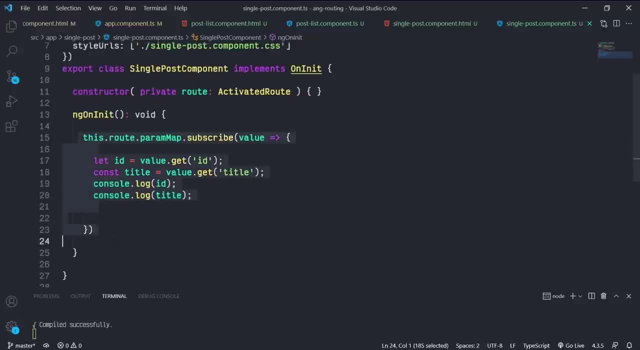 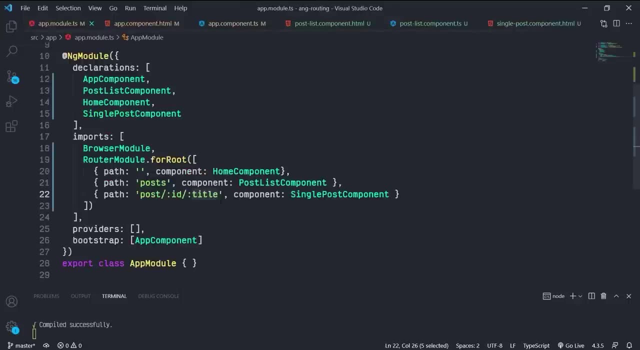 to pass query parameters with angular routers When we're dealing with router parameters. we defined that inside the app module file And also we defined that inside the app module file And also, if we defined a router parameter, we must pass that router parameter when we navigate to. 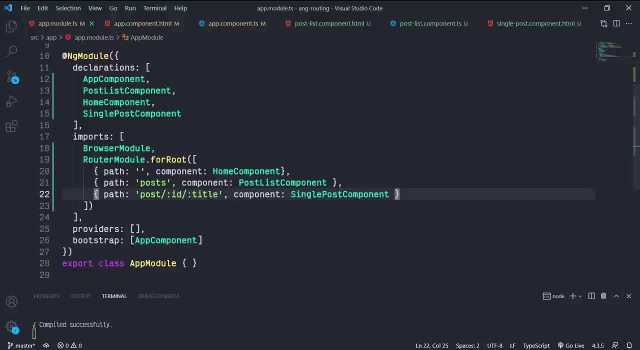 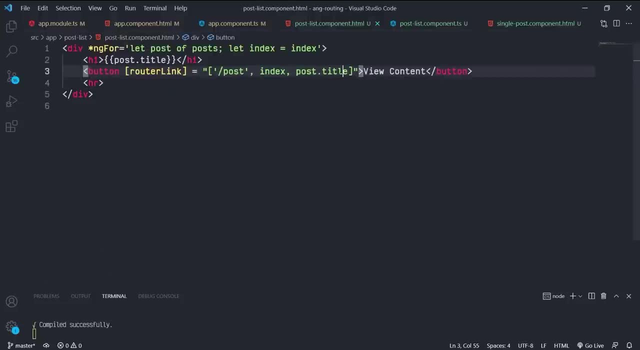 that route. So this is what we did with this, if you can remember. In any case, if we missed passing the router parameter, this router will not work. So wait, I'll show you an example. Remove this title value from this and keep only this id parameter. Save this and back to the browser. Now click on. 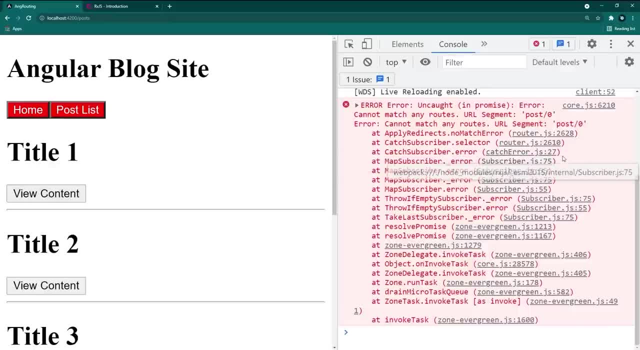 this website. Now click on this web. You can see that we have a route parameter here. Now click on this. we have a route parameter. So this is what we did with this, if you can remember. So this is what router doesn't change. Look at the browser console. As you can see here, we got this error. 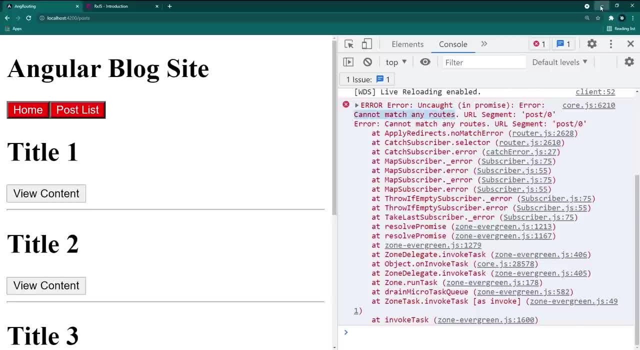 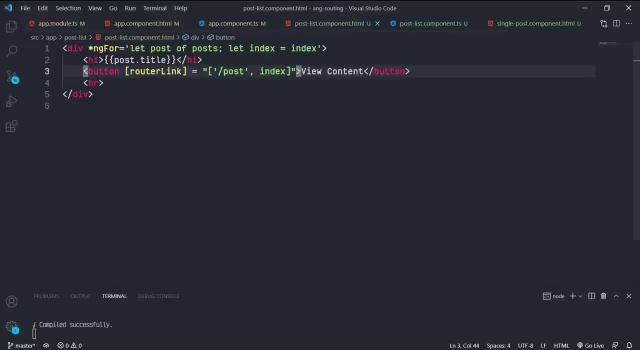 saying that cannot match any routes. So when we dealing with the router parameters, if we defined any router parameter, we must pass that parameter when we navigate to that router. But this query parameter is different. This is kinda like optional router parameters. If we want, we can pass the value to the router. If we don't, we can navigate to that router. 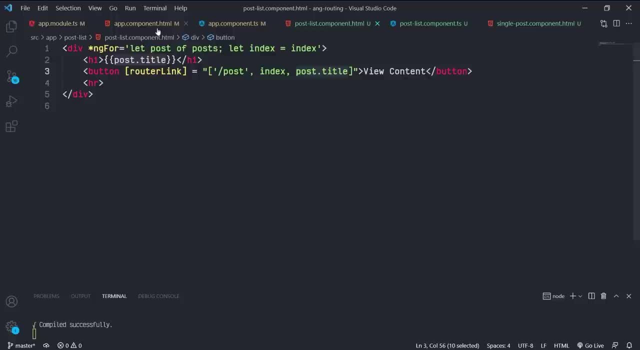 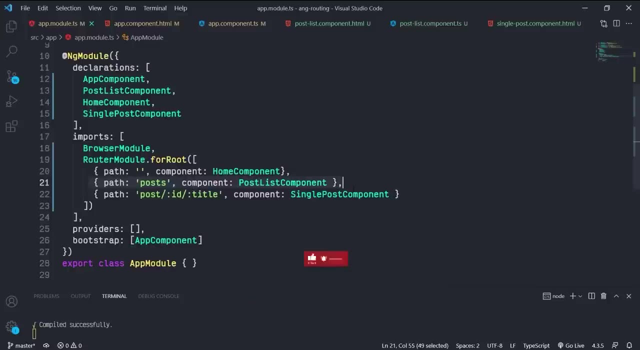 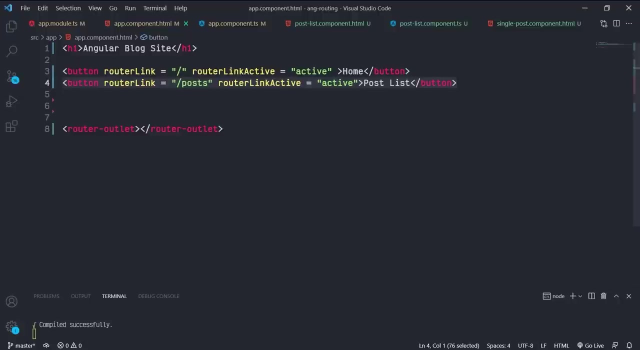 without any errors. So let's see this in action. We'll do this to post disk component router. We don't need to modify anything in the router module, Just go to the app component. So we are navigating to the post disk component with this post list button. 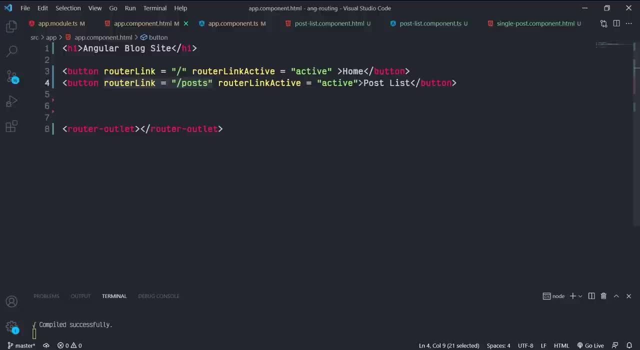 Very simple. For this we have another property: binding queryParams. So inside square brackets, queryParams carefully follow the capital simple letters. So this required an object. So assign inside double quotes the object with the query parameter list. So open and close a curly bracket inside this. First let's pass something, page number. 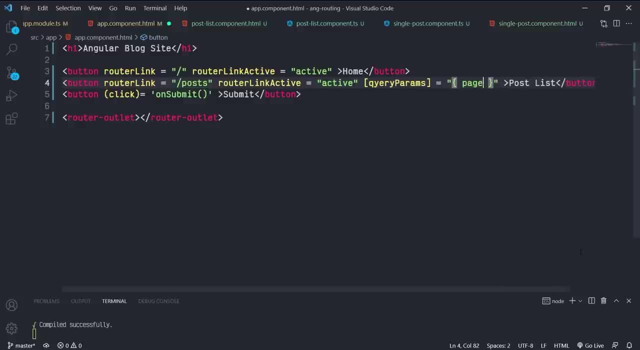 So the key is page and the value is something one. And let's pass another value, Something orderby, And value is newest. Pass this as a string, So inside quotes: Newest. Mostly we use these query parameters for sorting, filtering and for searching, And also guys. 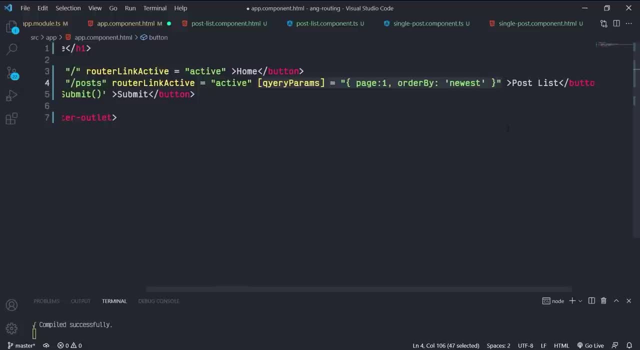 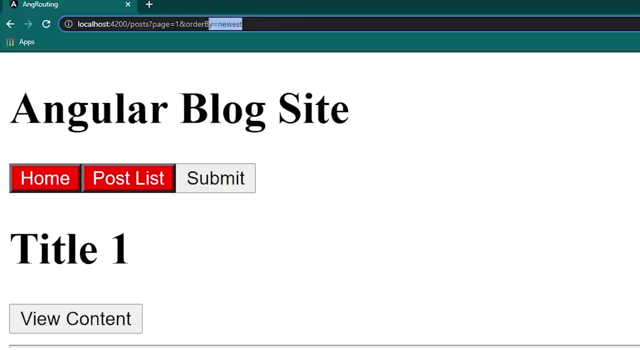 we can pass as many as query parameters with this. this. I just passed two values just for this example. Alright, save this and back to the browser. Now go to the post list. Perfect, look at the browser address bar In here we. 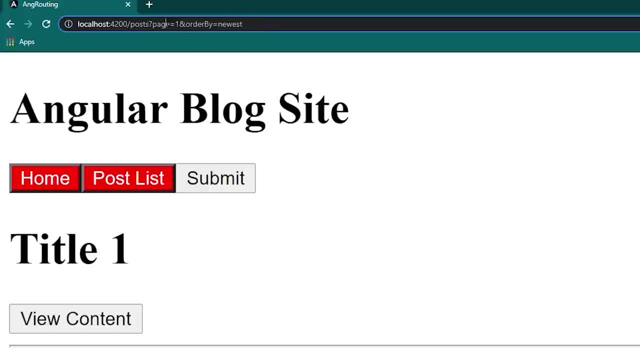 got these query parameters. We can identify the query parameters with this question mark and with this and symbol we can separate each and every query parameters. So we passed the page and order parameters. We got that in here. Awesome, right. So now let's see how. 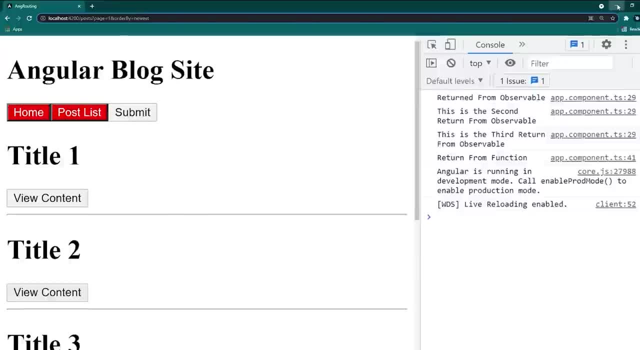 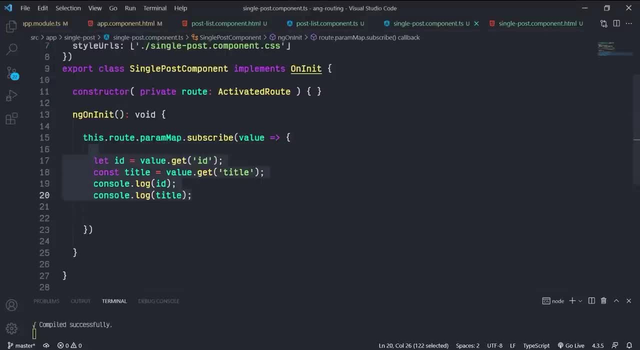 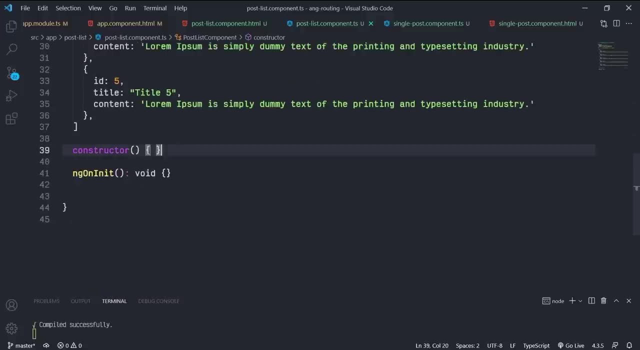 to capture these query parameters from the post list component. So back in the VSCode. this is also same as the previous router parameters, So go to the post list component, ES file. I think first we need to inject the activated router module to this component. So inside the constructor, parenthesis, private route. This can be any. 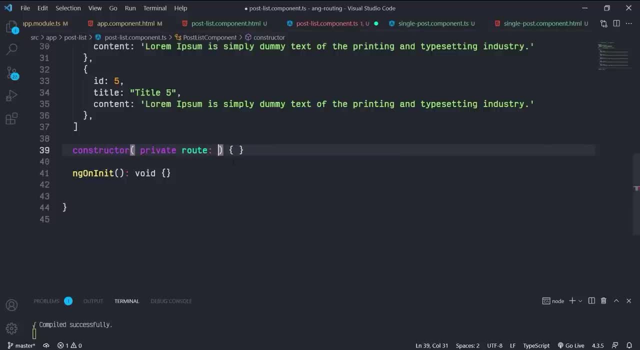 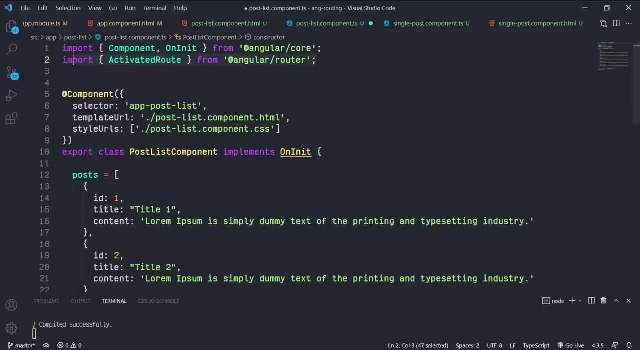 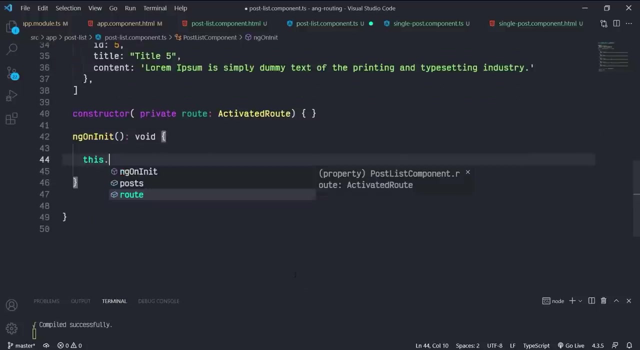 name and colon- This type is activated route- and select this autocomplete. This will auto import the path to this module. Perfect. next, let's get the values Inside the engine unit thisroute, which is this injected activated route. After this query parameter map. If you can remember, when we getting the parameters, we use the param map. 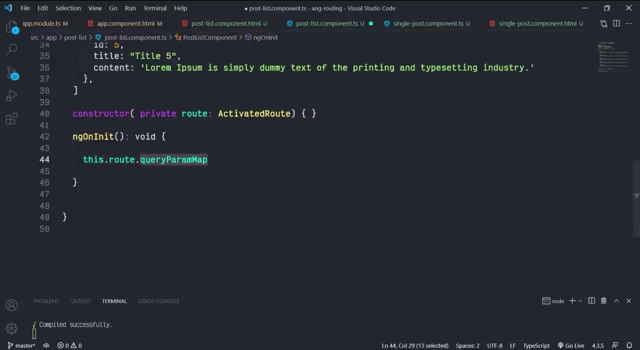 But to get query parameters we use this query param map Right. Ok, back to work. This also an observable. So in order to access this observable, we must subscribe to this query param map observable. So after this, dot subscribe and, inside the parenthesis, pass the arrow function. 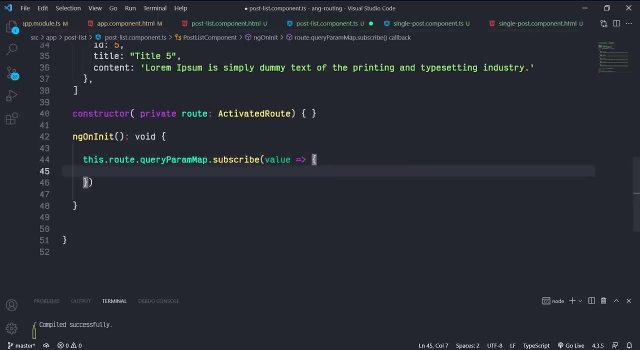 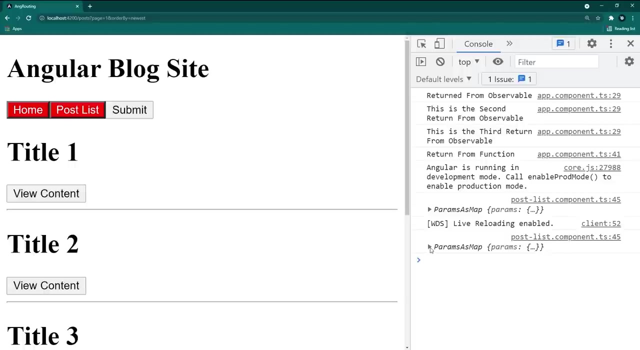 Value and the arrow function. Now, with this value parameter, we will get these observable values, So let's log this, Save this all and back to the browser. Go to the post list Inside the browser console. look at this. We got this query params- map object Inside this. we can. 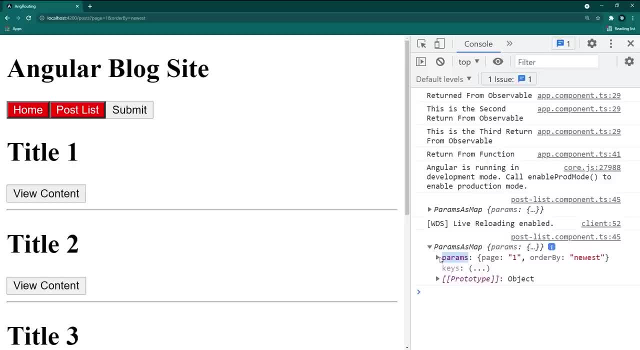 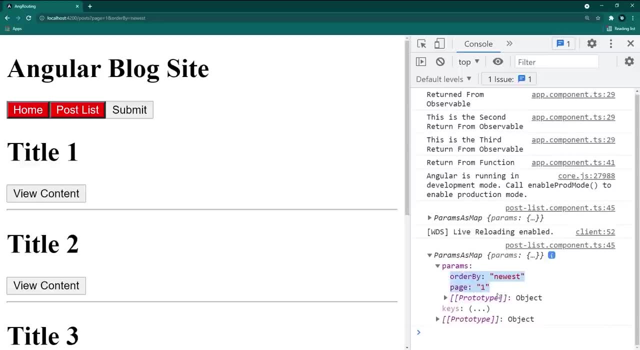 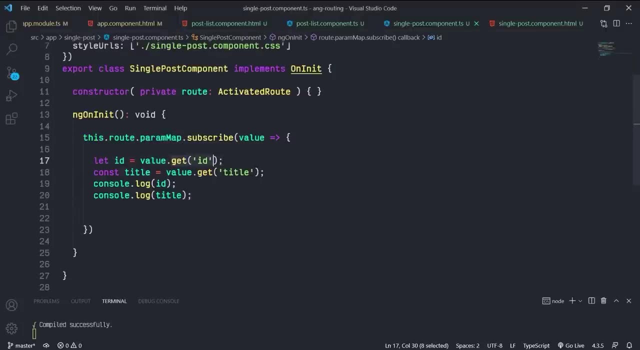 see this param object Inside that we got this order and the page query parameters. Perfect, right, Ok, back to the VSCode. Like this router parameter, we can access the query parameters also using the get method. So this value dot get inside brackets- Pass the query. 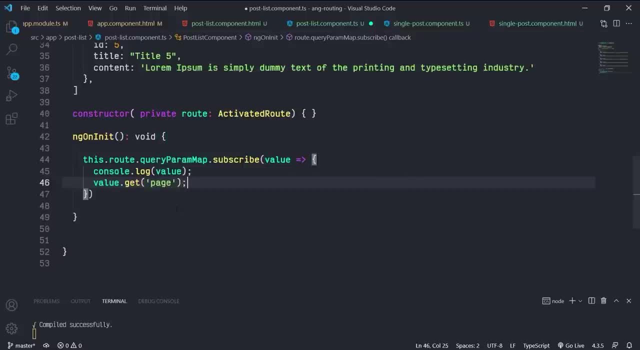 parameter key name page. Pass this as a string. Store it inside of a variable, something: const page- Perfect. We got another parameter, So const order assign val dot get and the parameter key is order, Perfect. Remove this previous log and log these two variables. 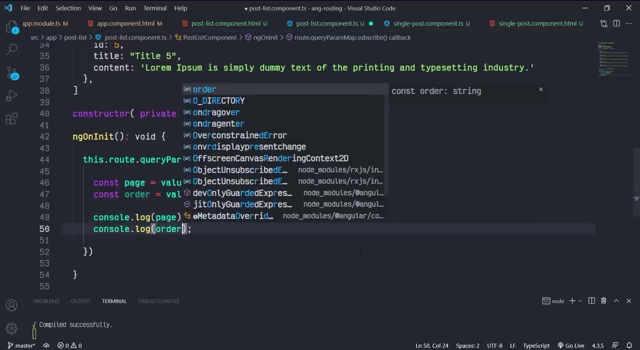 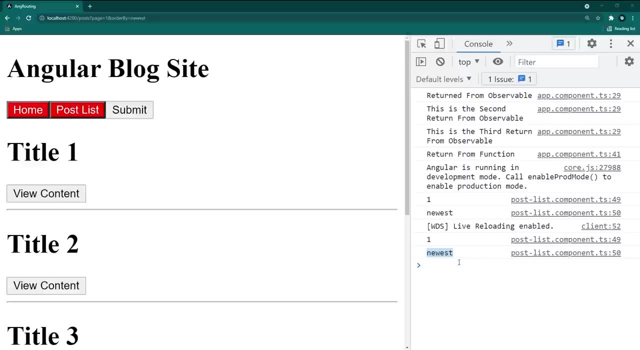 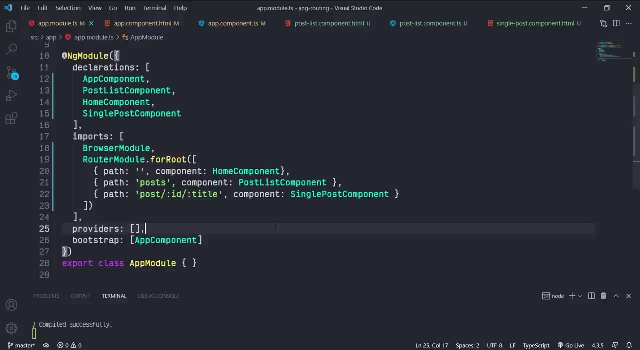 Page and the order. Now save this and back to the browser. Look at this. This time we got these query parameter values printed inside the browser console. So, guys, this is how we deal with query parameters. Alright, now we know how to use angular routing, As you know, 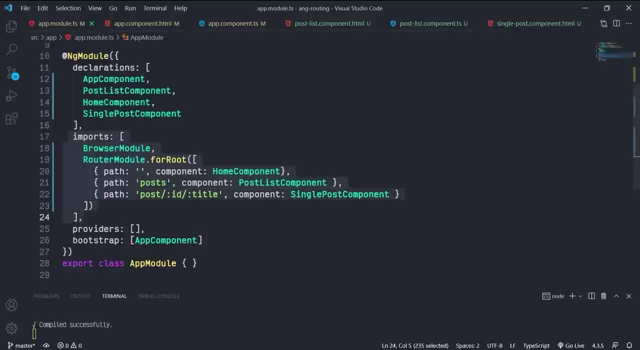 we defined all the routers in the browser. Now we will see how to use angular routing. This is not a good practice. Now. we got only a few routers So this looks ok, But think in the real world app we may need more than 10 routes, So adding them all inside this. 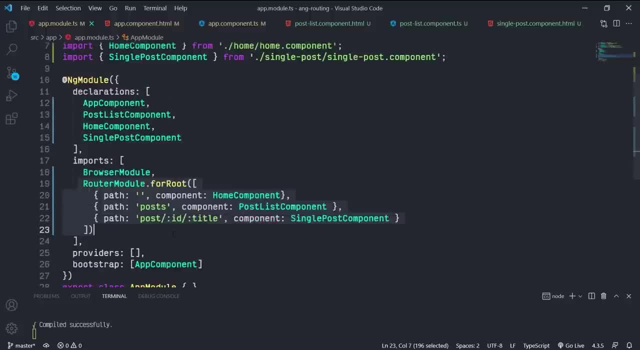 app module file. This will make our app code more busy and sometimes it may lead to unnecessary bugs and errors. As a solution for this, we can make a separate module file for this and angular routing. So in this lecture, let's see how to create a separate file for this. 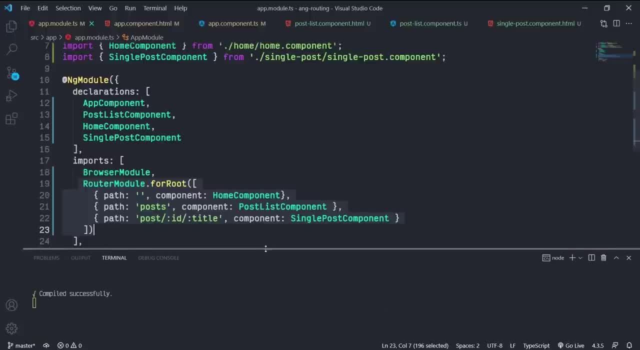 angular router. So let's begin. We can simply generate a module file using the angular CLI, So inside the uscode integrated terminal. Open another new terminal and run this command ng g. This g stands for generate. Now we are generating a module, So module After this. 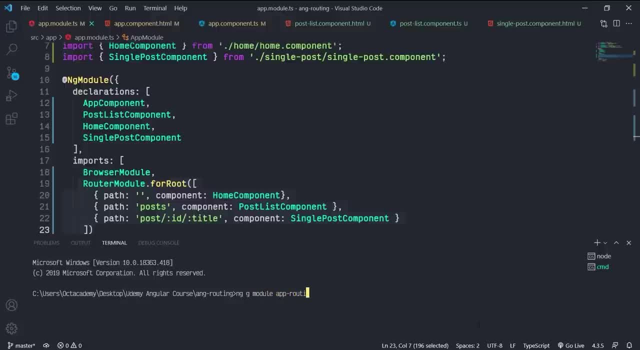 pass the module name app dash routing. This is just a name. You can use any name, but we are creating a router module, So normally we use this name- app dash routing- for this as a good practice. Alright, after this we have to register this module inside our default. 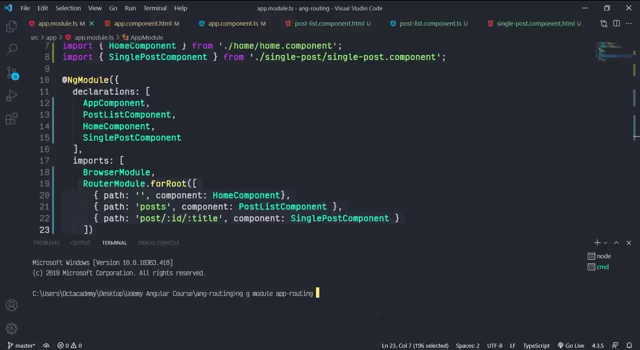 module. We can add that using the module flag. So double dash, module and the module name is this: app-routing. No need to pass the world name, Something like this: app, dot, module, dot, ts. Just pass the app. So, after this, add a flat flag, Double dash, flat. This will create this module inside. 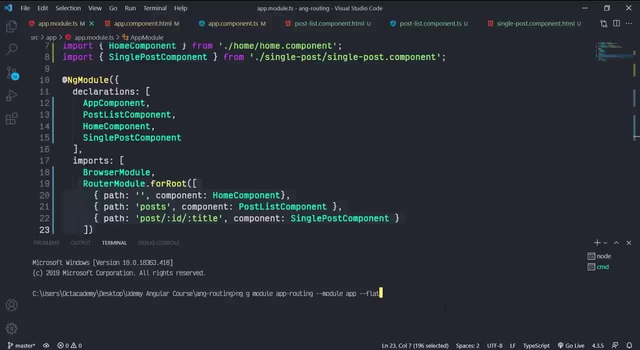 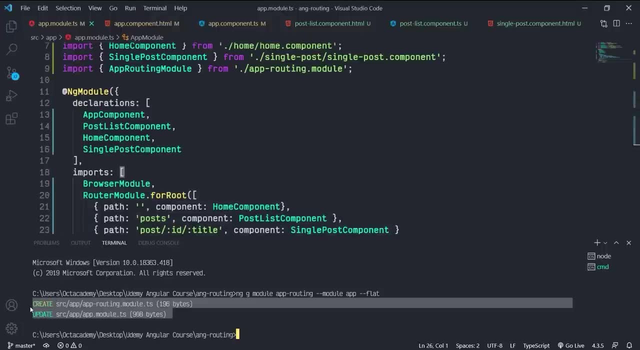 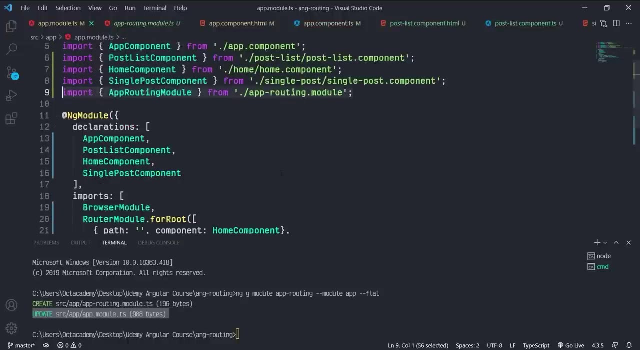 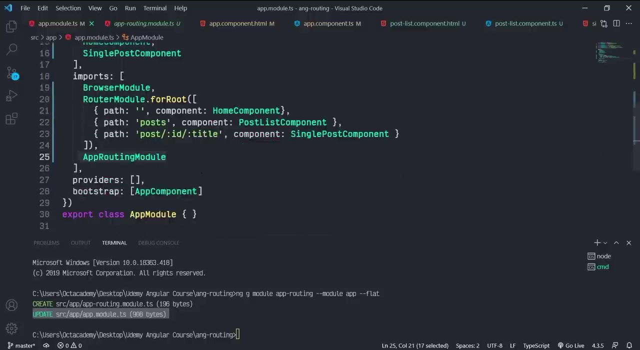 the root app folder without any sub folder. That's it. Now hit the enter to execute this command. Perfect. As you can see here, this generated the app-routing module And also this registered this inside the app module file. Perfect- Now open this newly created module file. Inside this we can see the basic code structure of 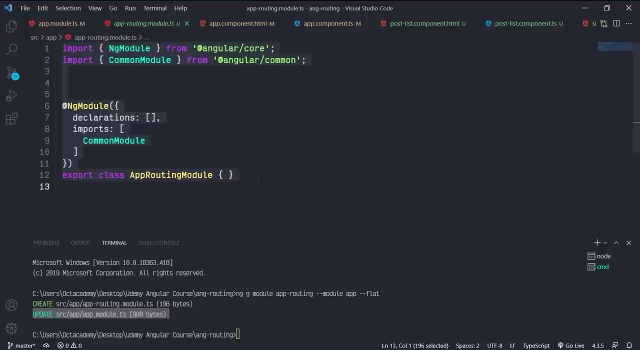 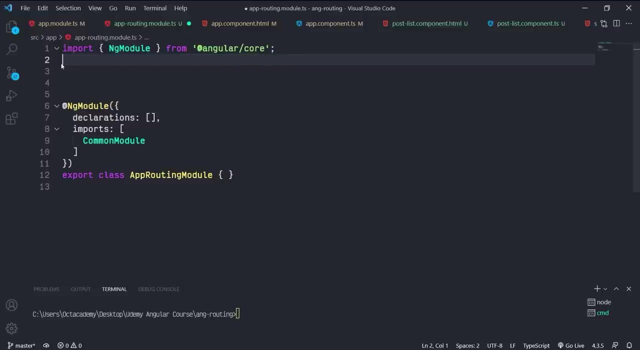 an angular module. Still, this is just an angular module, Not a routing module. So now let's see how to make this as a router module file. We need the command module, So remove it from the imports array and also this import statement. Now. we don't need the declaration module as well, So remove it Now inside this. 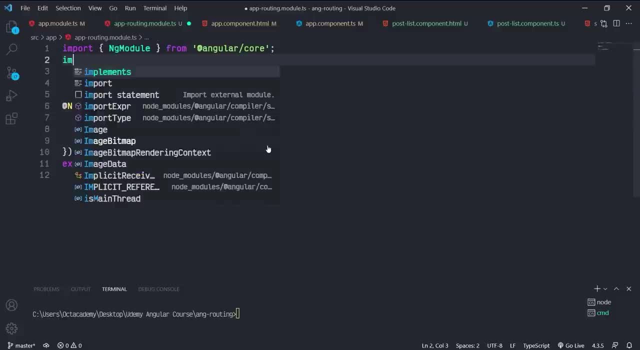 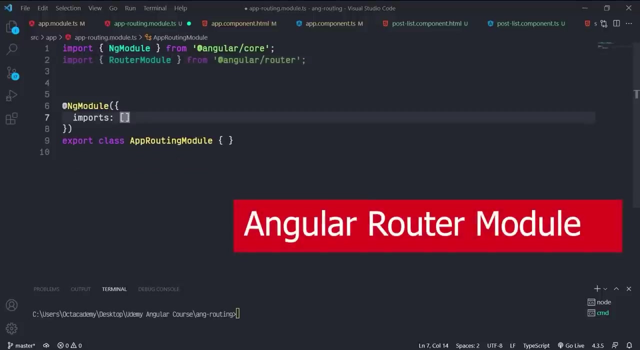 module. import the router module. So, as you know, in order to work with angular routers, we need to import the router module. Import Inside curly brackets: router module. This is coming from the angular core module. So now, inside this ngmodule decoration class, add this router module as exports. 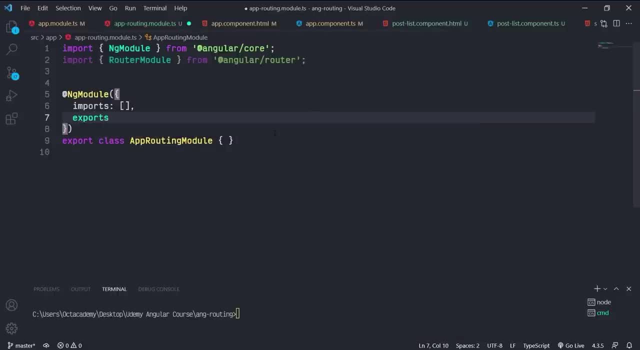 So after this exports, This also takes an array, So array, square brackets. Next, inside this import array, We will define the routes, Same as this app module imports. Inside this import module, We can use the pointsczenieurs loop, Simply type in 자� and then one plus to get one fourths, This 2 times the units. we get the weights here. Once you get the last hair path, it can be, however, come under. 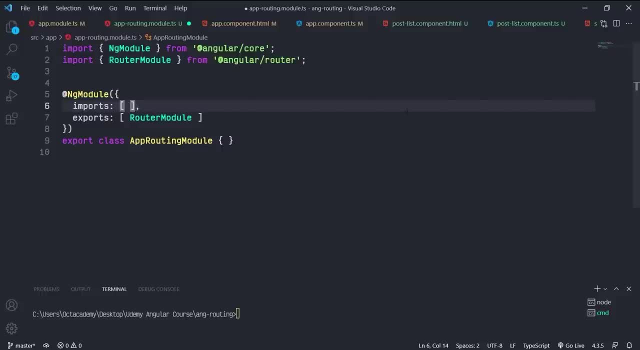 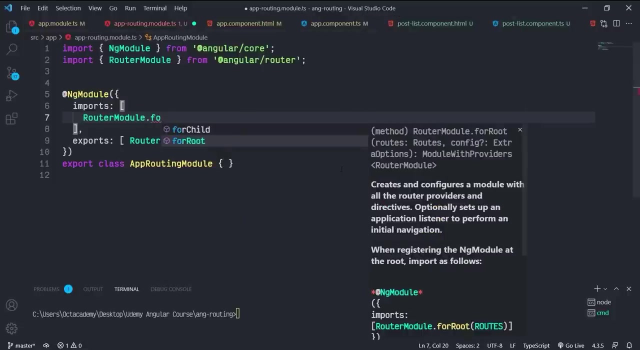 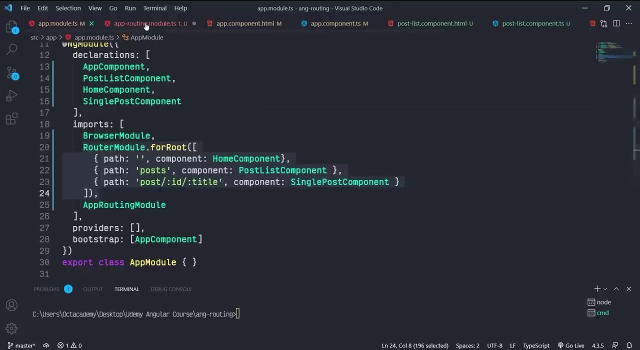 Next, inside this import array we will define the routes. same as this app modules imports. inside this import array, at this router module, which is this Imported module for root and brackets. inside this we can pass the routers. Nothing new here. same as this previous app module import. 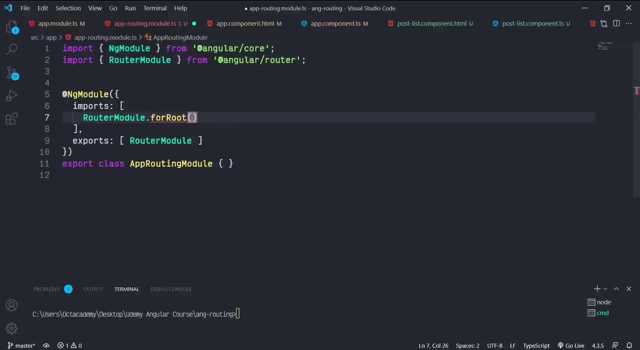 So this time I'm gonna create the routes array outside of this and store it inside of a variable. Then we can pass that variable inside this. for root parenthesis, Let's see this in action: Create a variable const routes and set this type to angular routes. 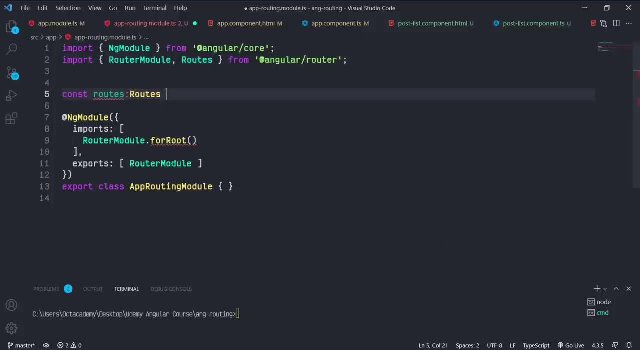 Select this autocomplete and this will automatically import this. Now assign this to routes array. For now, just simply declare an empty array. Now we can pass this routes variable to this For root. Very simple and very clean code, Right, Perfect. Now we can add our routes inside this array. 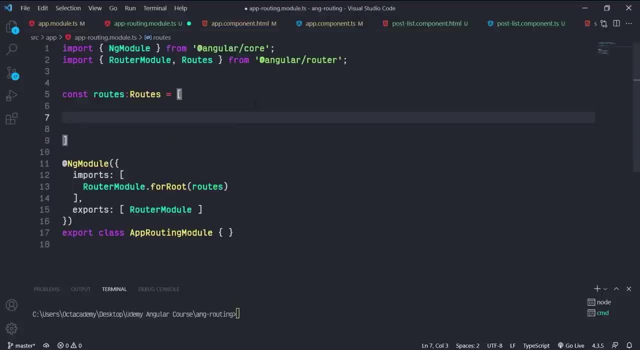 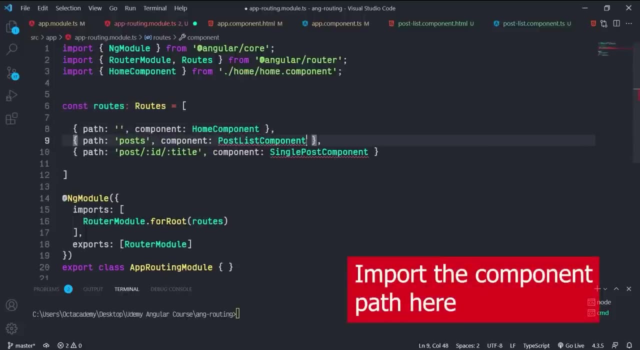 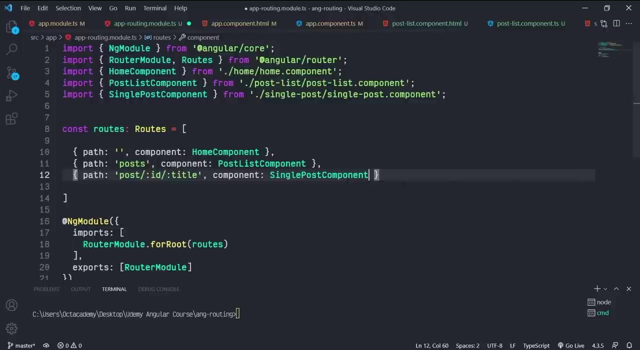 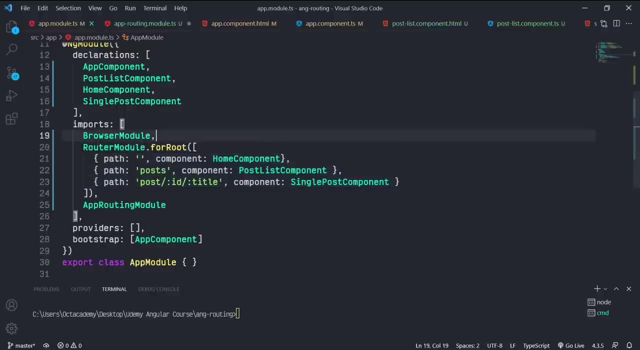 Copy this from the app module file and paste it inside this array. All right, now we have successfully created the app routing modules file for angular routing. Go to the app module ts file. Now we don't need this router module import and these routes. 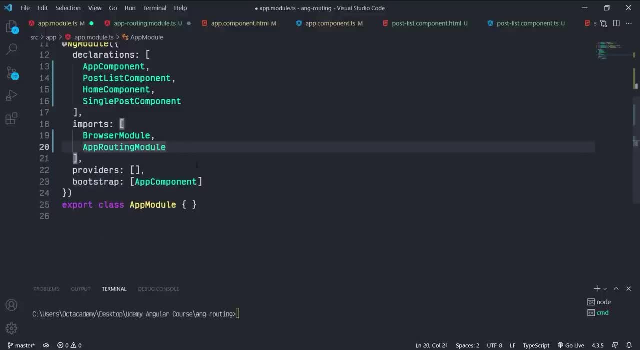 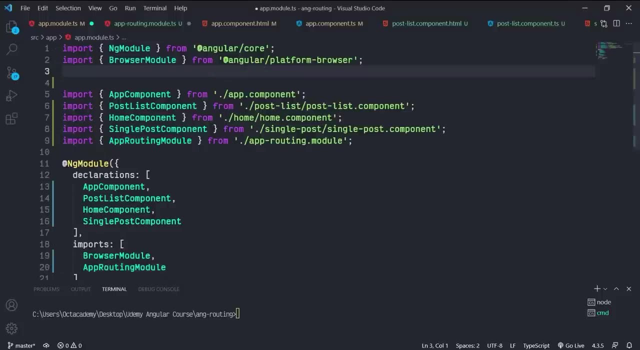 We declared them all inside the routing module file, So remove it from this imports array and remove the import statement as well. That's it. We have successfully created separate router module file for routes. Perfect. Save this all and back to the browser. 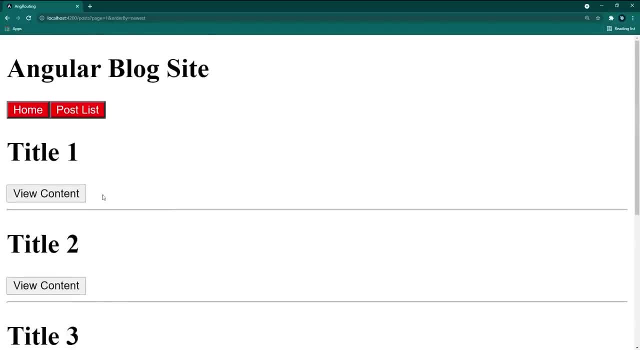 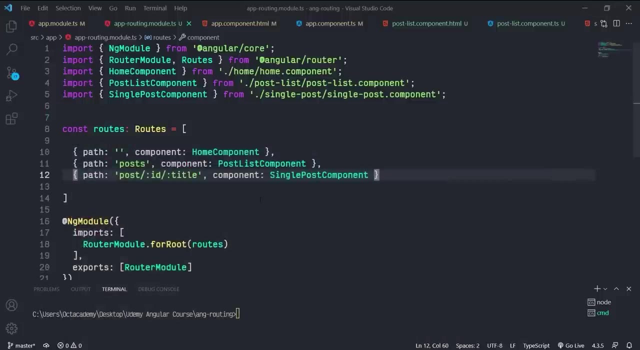 Navigate to the post list: Perfect, It's working. Navigate to the single post: This also working Again. navigate to the home: Perfect, Everything working as previous. So this is how we create a separate router module for our angular app. Before the end of this lecture, I wanna tell you one more thing. 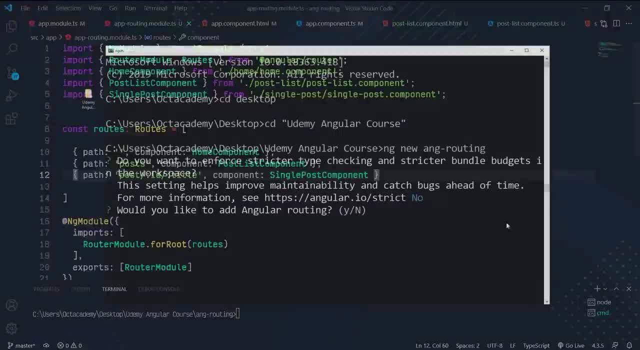 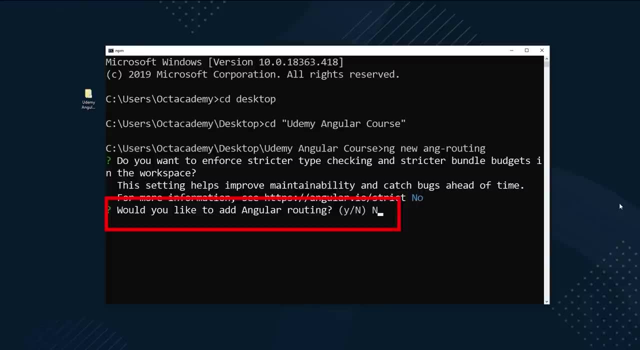 If you can remember, when we creating the new angular app, angular CLI was asked that we using the angular router or not. When creating this app, I gave no cause. I wanted to do this from scratch. So if we give yes to this, angular CLI will generate this routing module for us. 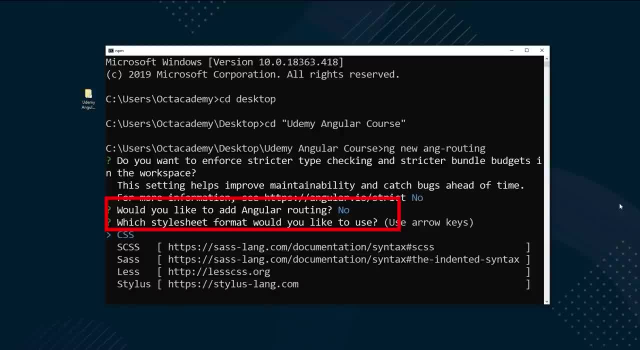 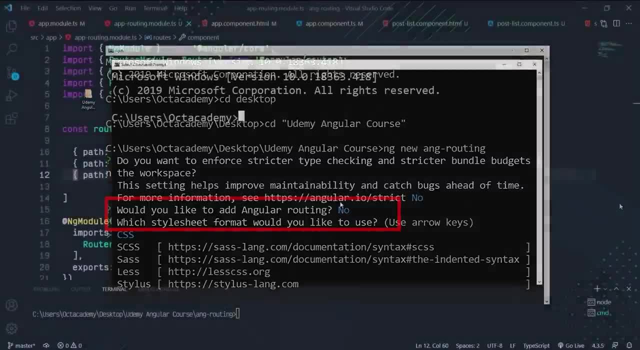 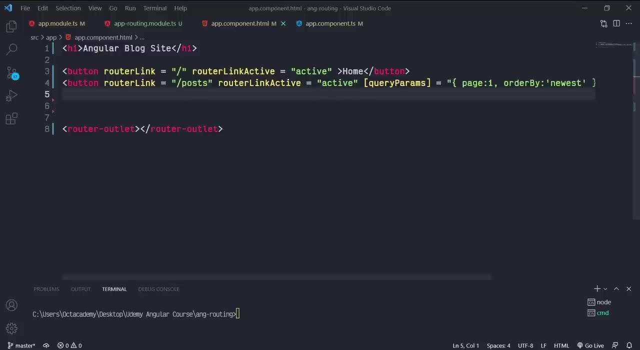 We don't need to hand code everything from scratch. From now on, we will use the angular CLI method to generate the routing module file. Perfect, Alright, now we know how to navigate to a router inside the html element Using the router link directive. 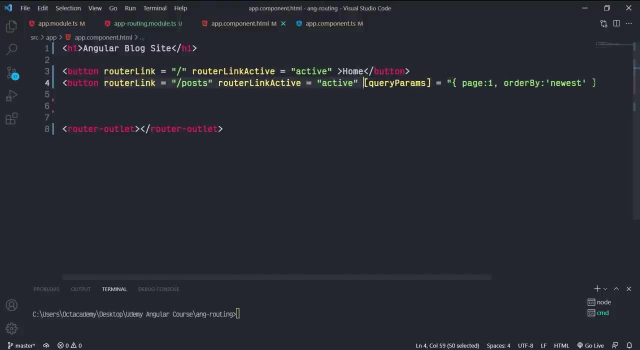 Think, if we want to navigate to a route inside of typescript method, how do we going to do that? Very simple, So first create a button. The button text will be submit. Now I want to call to a method when clicking this button. 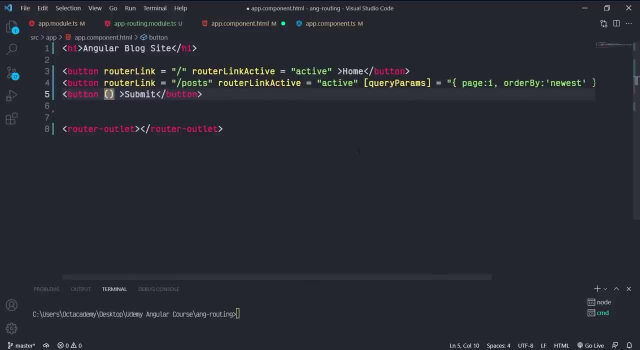 For this we can use the click event binding. So inside brackets, event is click Assign. Assign this to a method called something, onsubmit, And don't forget to add the parenthesis. Now go to the component ts file and create the onsubmit method. 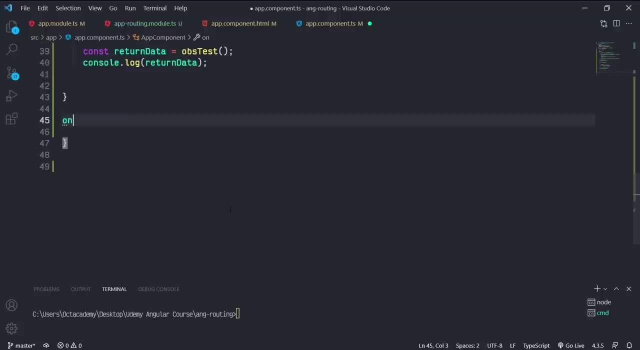 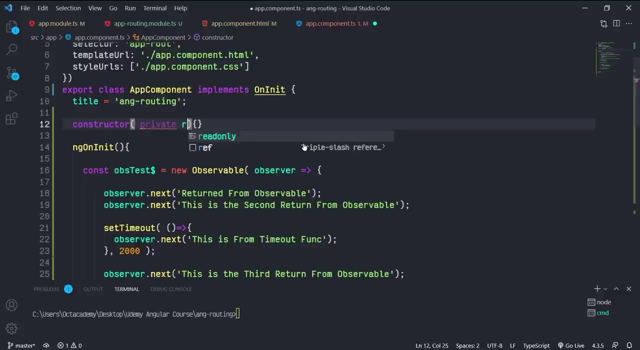 Onsubmit- parenthesis- and the method scope. In order to navigate to a route inside the ts file, first we have to inject the router service to this constructor. So inside the constructor Private router, This is just a variable colon and the this type is router. 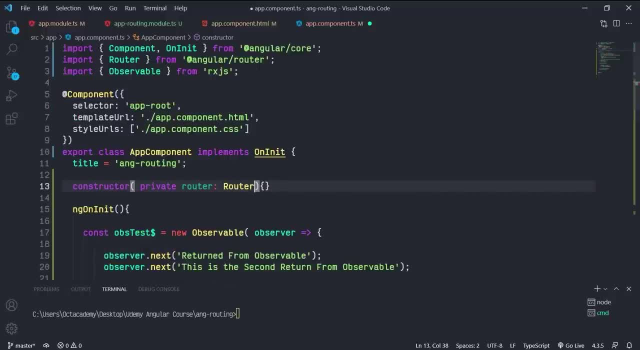 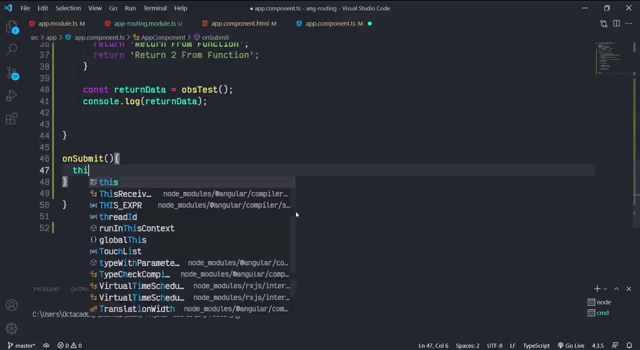 Select do to complete. This will import the router service to this component. Perfect. Now, inside the submit method, This dot router, which is this injected router. After this dot navigate and parenthesis. Inside this pass, an array with the router link, The square brackets. 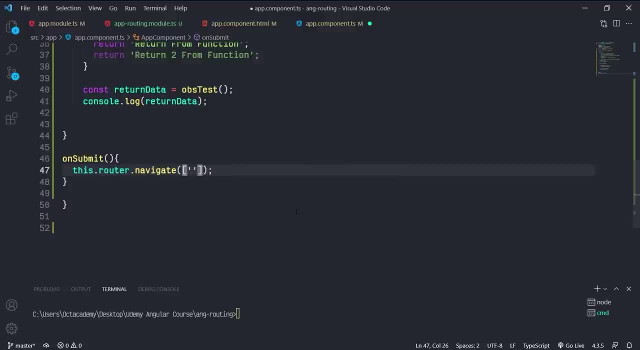 The square brackets Inside this quotes and the router is slash post. Put this inside quotes. That's it Now. save this and back to the browser. Click on this submit button. Look at this. We successfully navigate to the post list component. 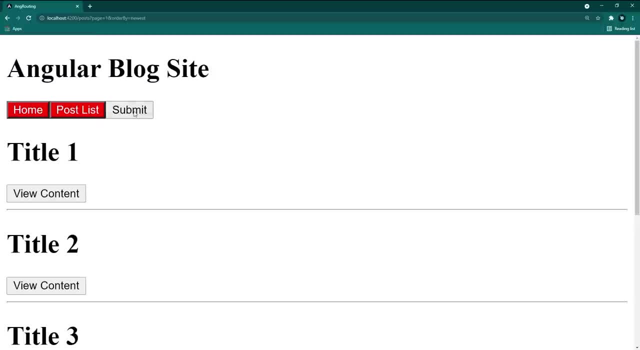 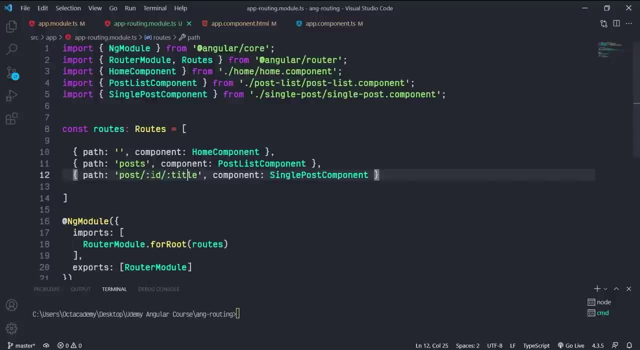 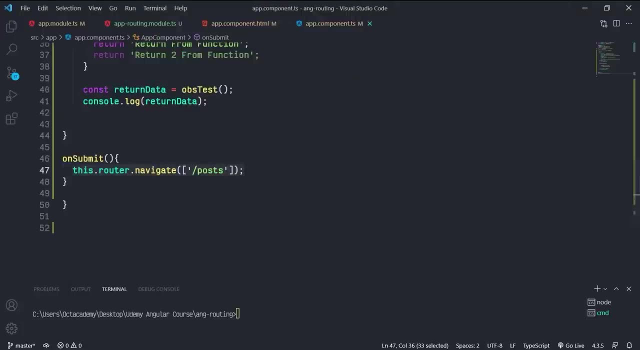 Perfect, Think. now we want to navigate to the single post components router, which required this id and the title router parameters. How do we define that With this router? navigate? Very simple. This markup also same as this router link property binding. So inside this navigate parenthesis. 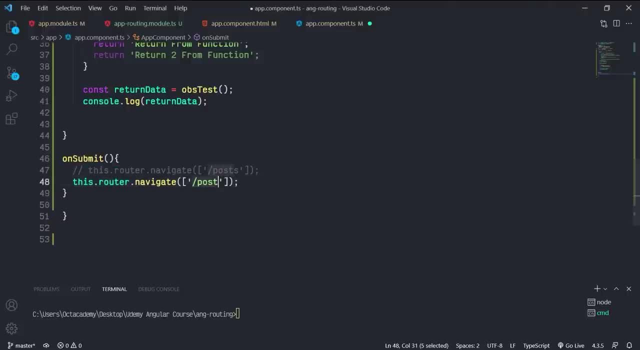 This array and the first array value is this router path After this comma, and we can pass the router parameter values like this: The id is something 1 and after this comma And the title is 1.. And the title is 1.. 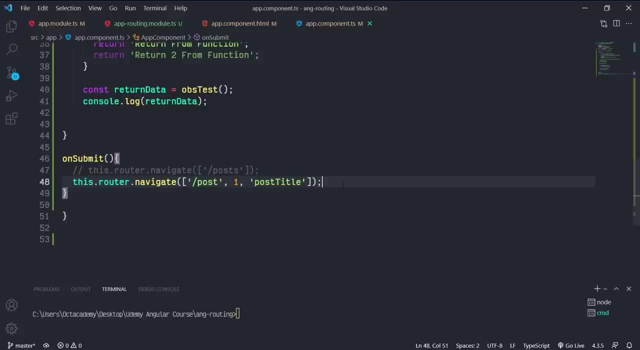 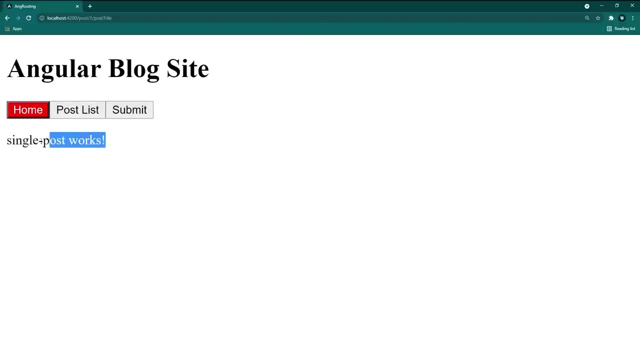 And the title is something post title. Don't forget to put this inside quotes. Save this and back to the browser. Click on this Perfect right. We successfully navigate to this single post component with these router parameters. Next lets see how to pass the query parameters. 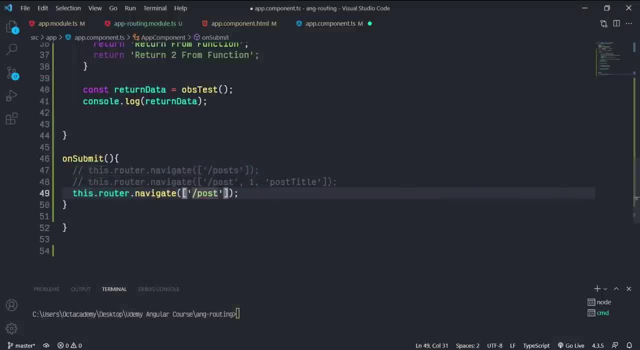 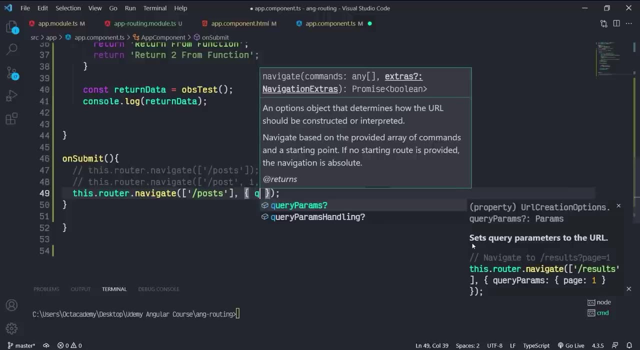 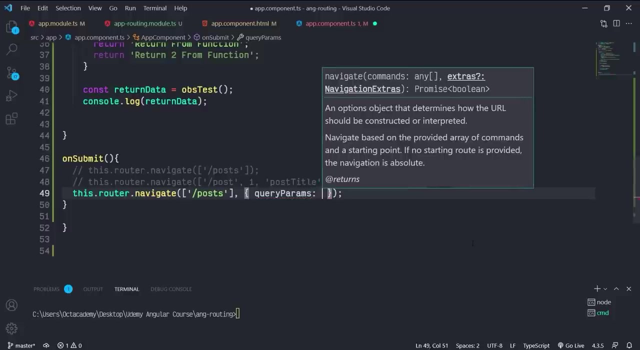 This also very easy Packet vs code. After this, create an object scope, Open and close the curly brackets. Inside this Put the query parameters Like this: Key is query params. This p must be capital. This value also required an object. 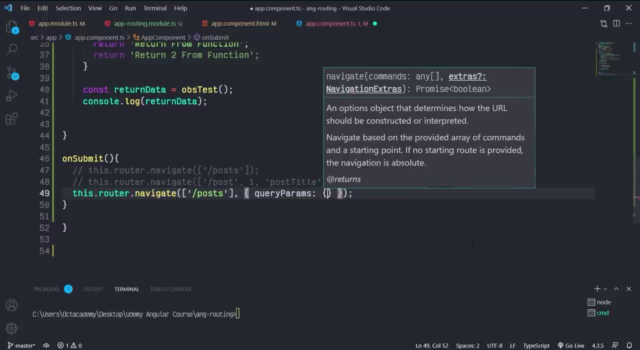 So open and close curly bracket Inside this first query parameter is page And the value is 1.. And another parameter, order And value, is newest. Put this inside quotes. That's it Save. Save this and back to the browser. 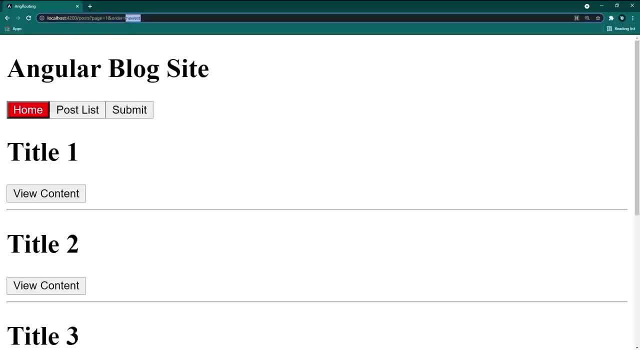 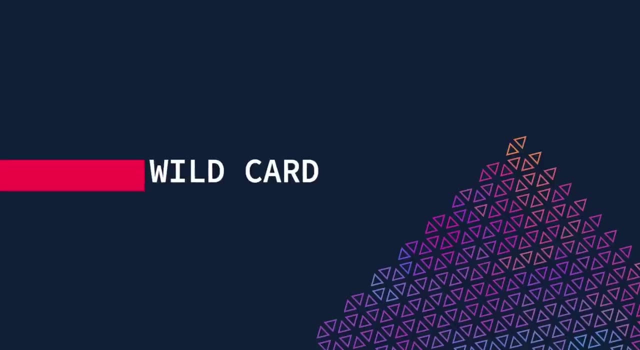 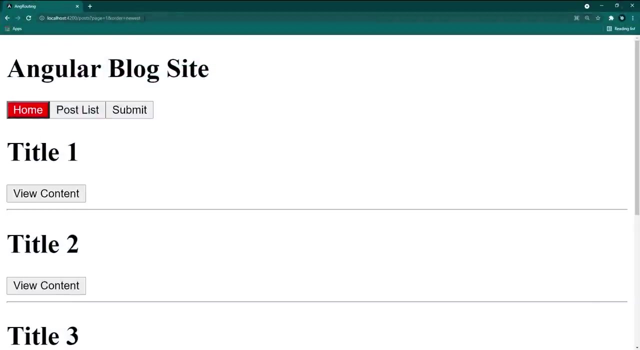 Once again click this submit button. Perfect, right, We navigate to this with these query parameters. So this is how we navigate to a router programmatically. Hope you guys got the idea. In angular router we can define the 404 routers. If you wonder, what is this 404.? 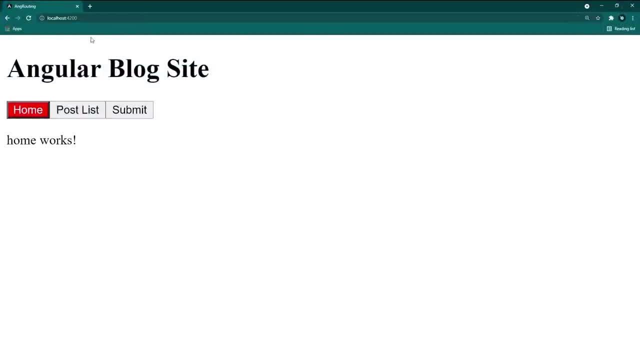 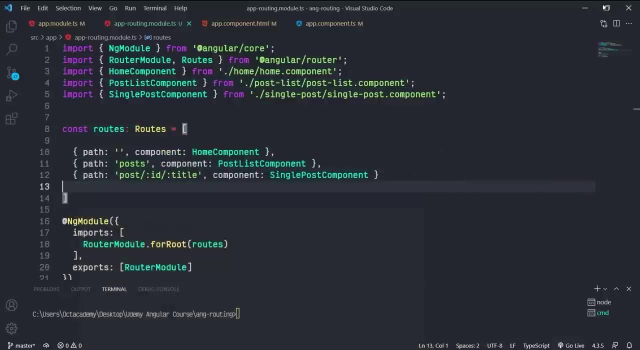 This is the 404.. This is the error code for page not found. If someone visit the router which is not declared in the angular app, it will redirect to the main router. That's why we are getting this form component. Now let's see how to add a page not found wildcard router in angular. 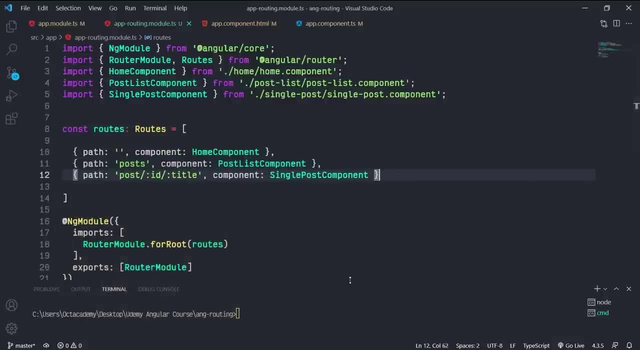 We call these 404 routers as wildcard routers. So let's see this in action. First, let's create a 404 component Inside the integrated terminal ng, g, c. The component name is something 404.. This is just a name. You can use. whatever the name that you want. 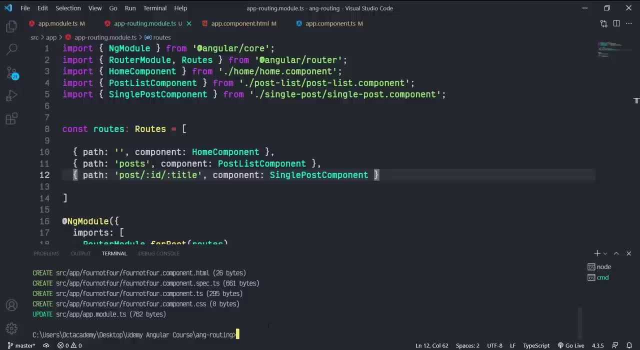 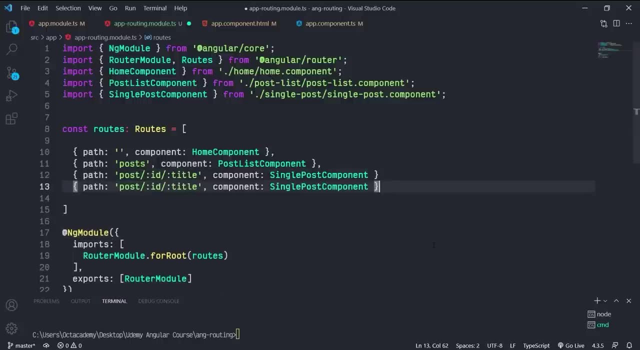 Hit the enter to execute the command. Perfect, We got the 404 component. Now let's define the wildcard router. Very simple: Duplicate this router object, The path will be two asterisks And the component is 404.. We define the wildcard router path like this: 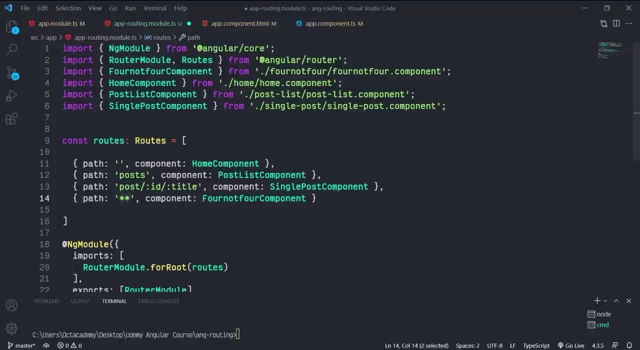 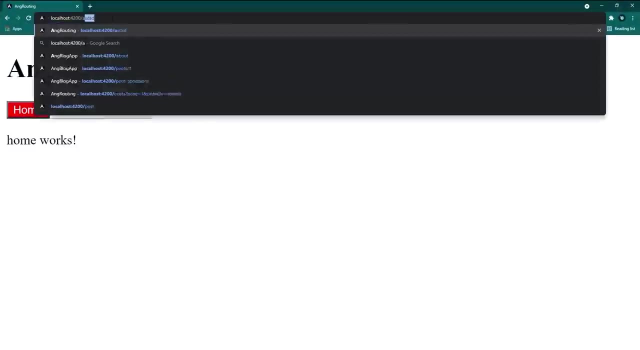 With this we are saying: if the browser URL is not matched with any of these defined router, show this 404 component inside the browser. That's it, Very simple, right? So now save this and back to the browser. Go to something different URL. 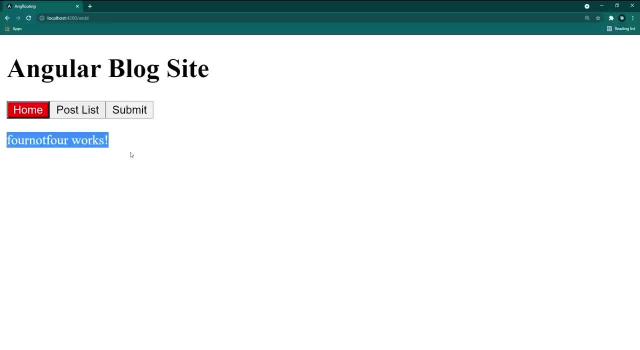 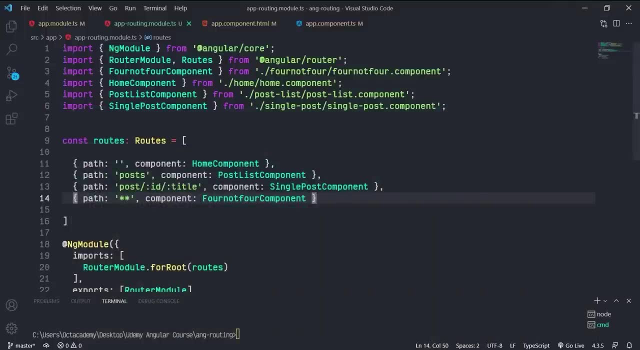 As you can see here, we got this 404 component. Perfect, right, Wait, At the end of this lecture I wanna tell you something. Always add this wildcard router end of your router list. If you add this top of this, this will show the 404 component for all of this router. 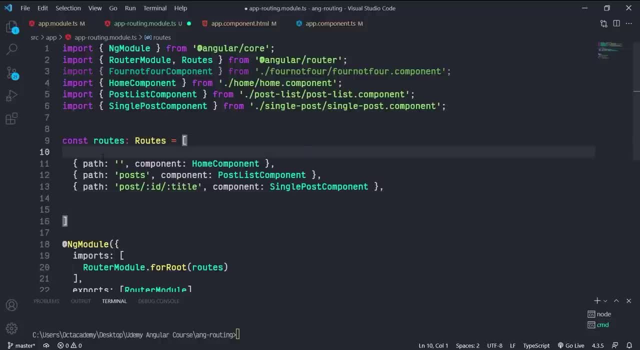 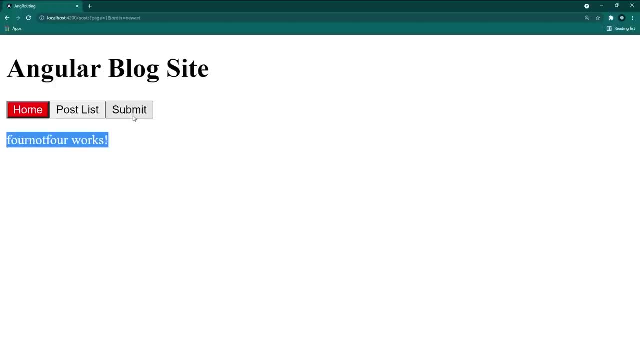 Wait, I'll show you this. Remove this from here and place it top of this router list. Save this and go to the browser. Look at this. Every route we visit, we got this 404 component, So always make sure to add this bottom. 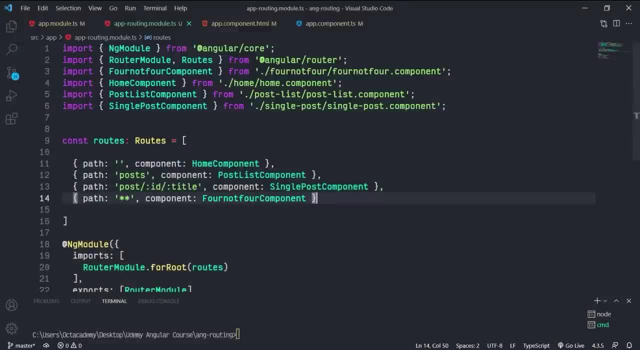 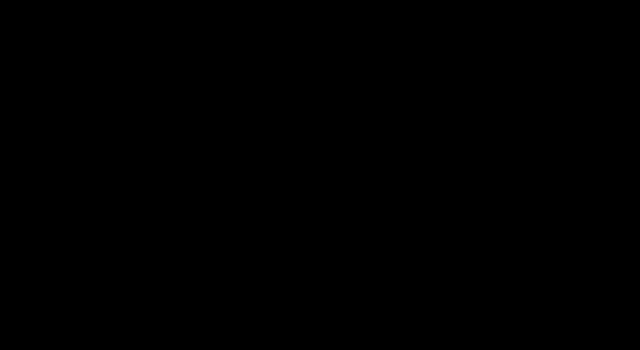 So this is how we deal with a wildcard or 404 or page not found routers in angular. So if you have any questions or have any questions, just ask me. I'll see you in the next video. Bye, Bye, Bye, Bye. 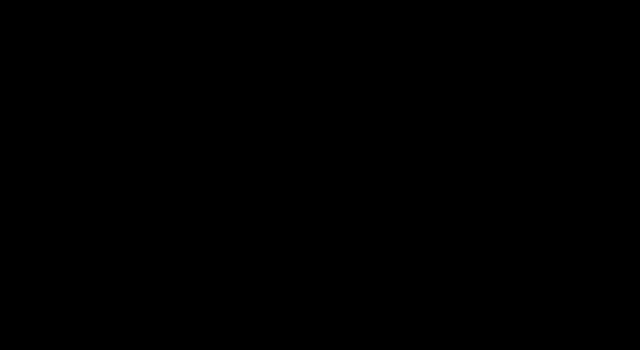 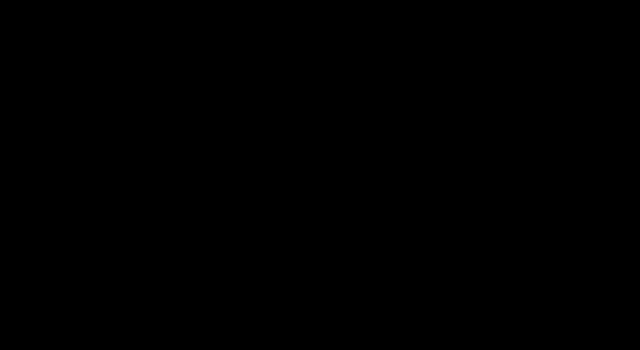 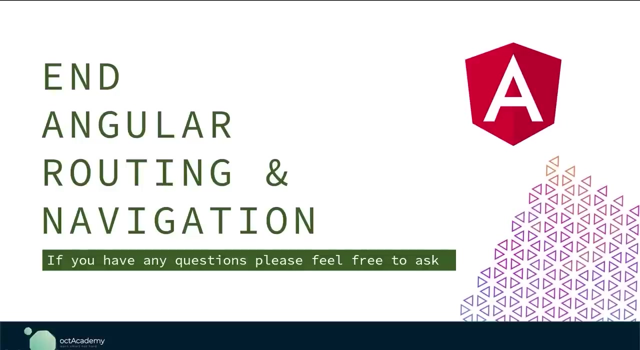